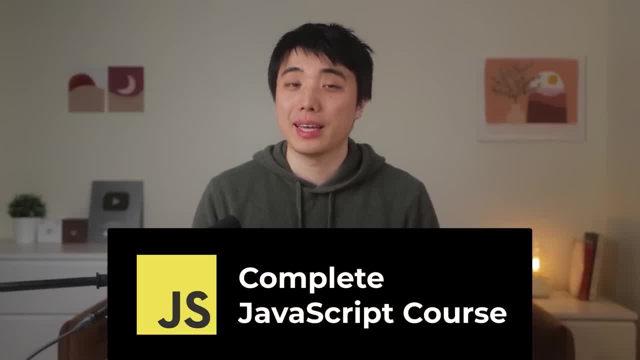 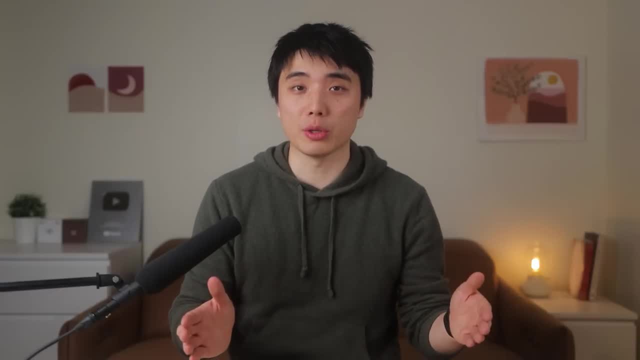 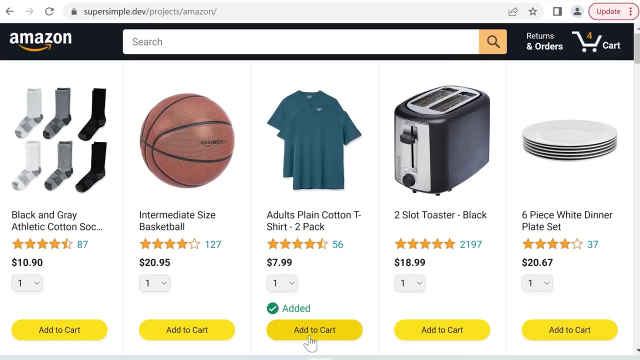 Welcome to the complete JavaScript course. In this course, we're going to learn how to build complex websites using JavaScript, from a beginner to a professional level, And by the end of this course we're going to build amazoncom. So this is an interactive, multi-page website. 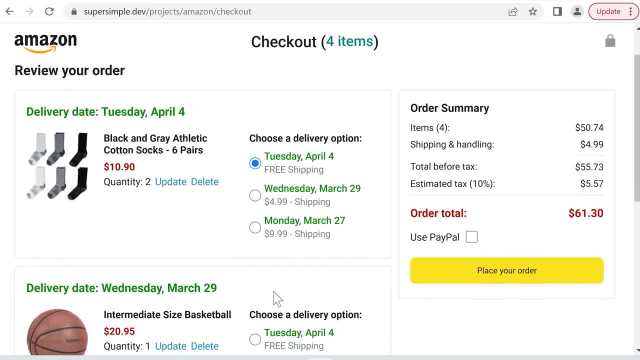 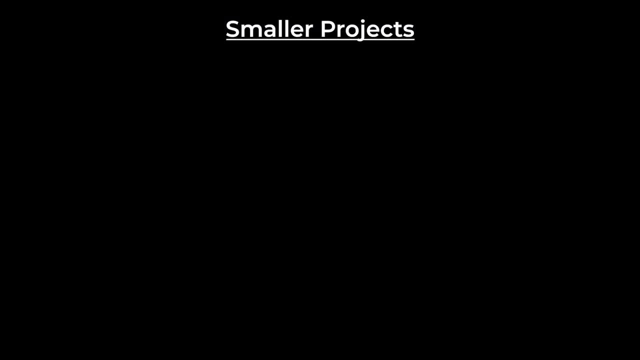 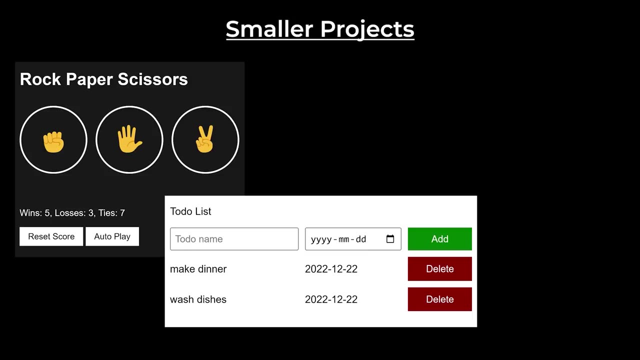 where we can add products to our cart, create an order and even track our order Along the way. we're also going to build some smaller projects like a rock-paper-scissors game, a to-do list and a calculator. Now you don't need any previous coding or technical experience. 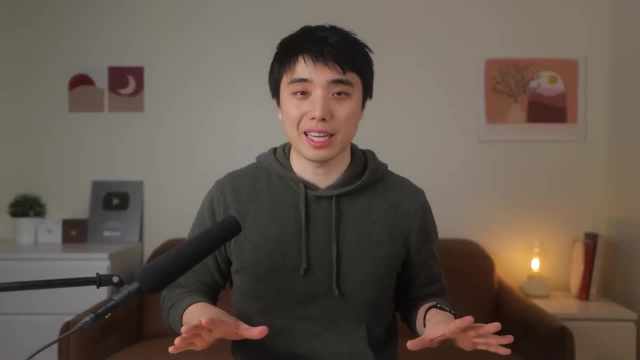 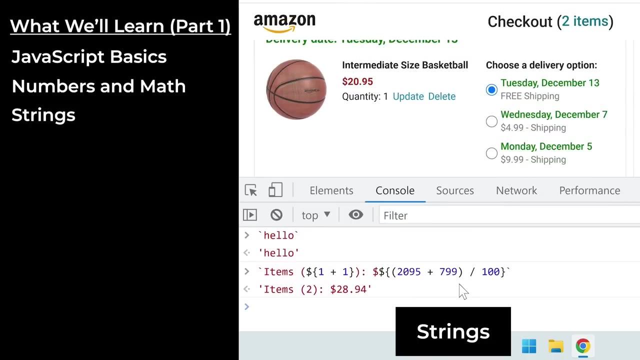 to follow along. This course will cover everything that you need to learn JavaScript. We're going to start from the very basics of JavaScript and we're going to build our way up step by step. We're going to learn the major features of JavaScript and we're going to learn. 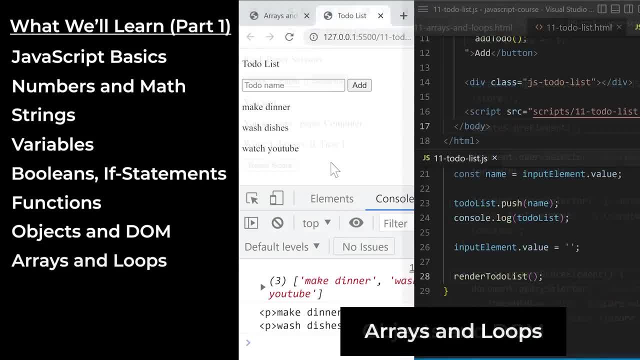 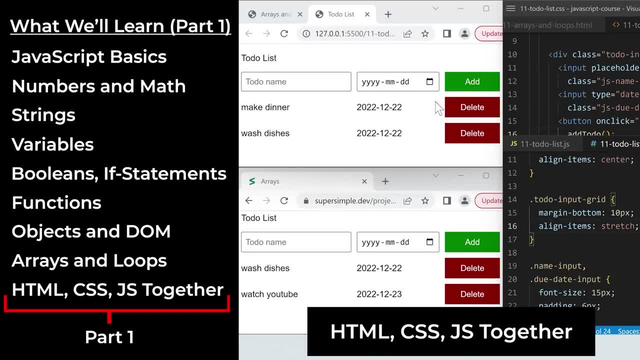 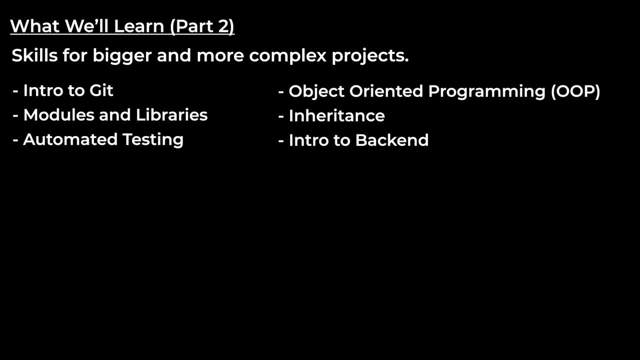 how to use JavaScript together with other technologies like HTML and CSS. These are the topics we'll learn in part one of this course. In part two, we'll learn skills that are useful for bigger and more complex projects, And we're going to start and finish the final. 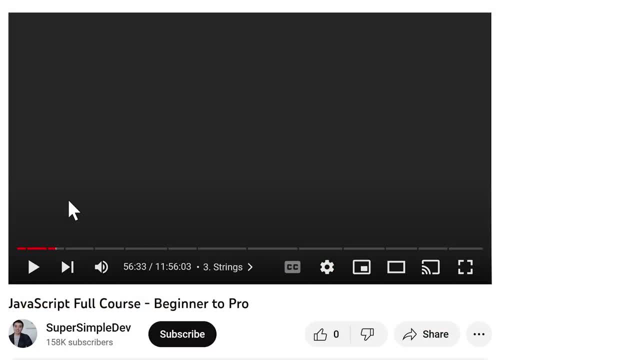 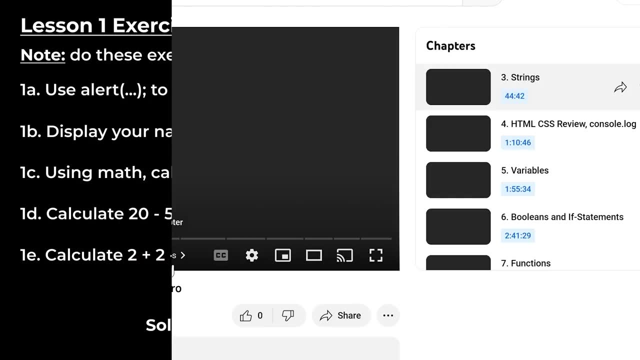 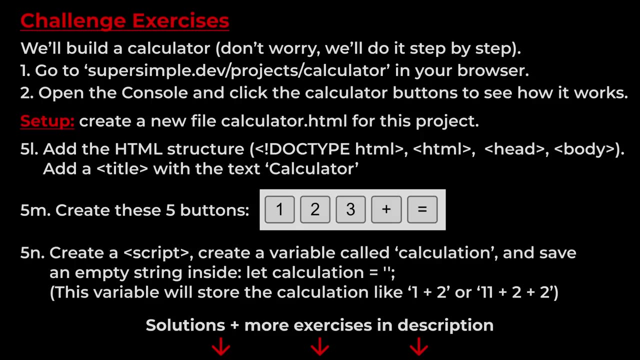 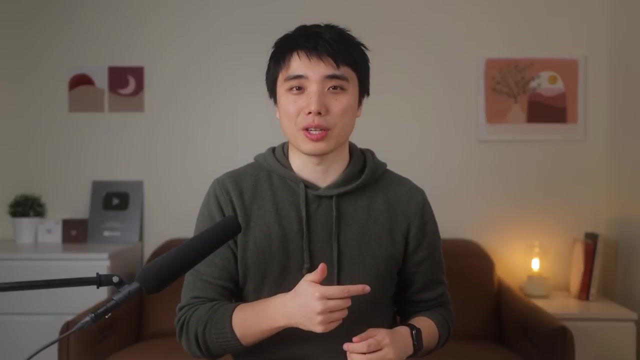 Amazon project. You can find the different lessons of this course below the video, here and here, And after each lesson, I'm going to give you a bunch of exercises that you can do on your own to practice the skills that we learned. In total, this course will have over 200 exercises. So, with that said, let's get started. 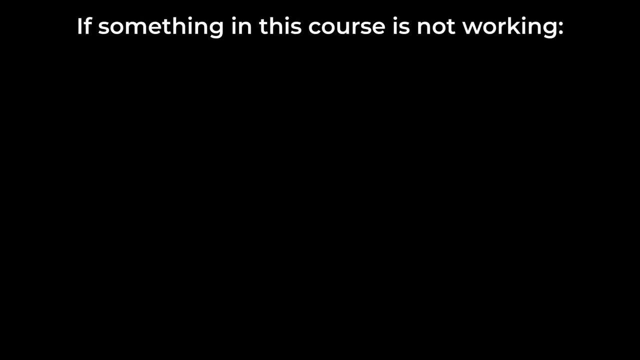 Before we begin, if something in this course is not working properly, make sure to check the first comment below. If you have any questions, feel free to ask them in the comment section below. If you like our video, hit like and subscribe, and if you would like to see more of our content, 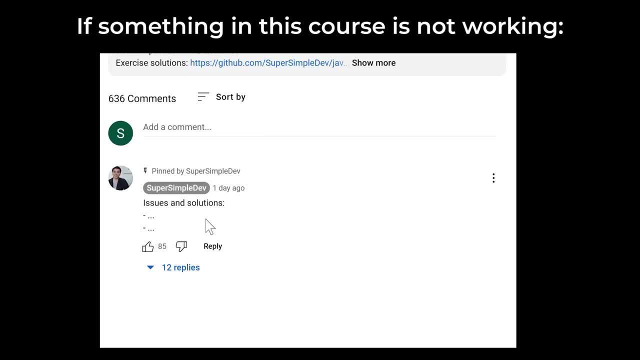 follow us on Facebook and Twitter And we'll see you in the next video. If you want to see more of our content, click below the video for a list of solutions. If you can't find a solution in this list, you can reply to this comment. 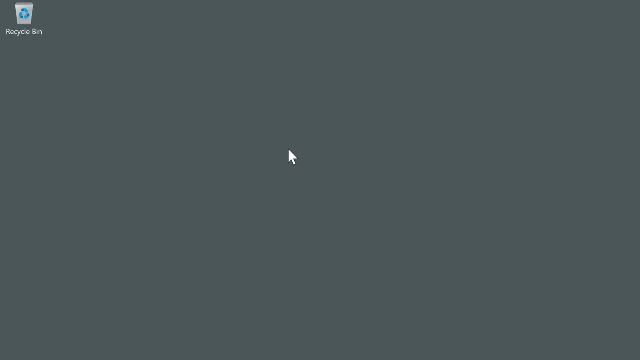 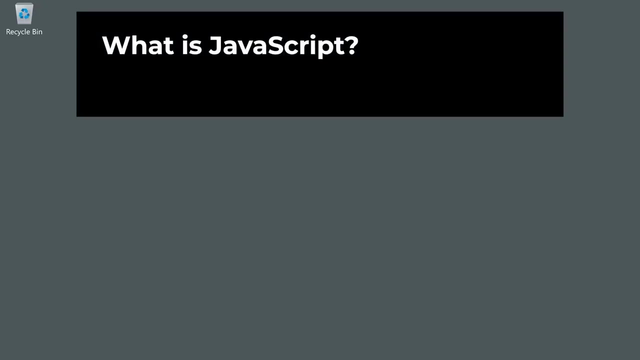 I'm going to be doing this course on Windows, But the steps are the same if you're using a Mac. We're going to start from the very basics of JavaScript and build our way up step by step. First of all, what is JavaScript? JavaScript is a technology that we 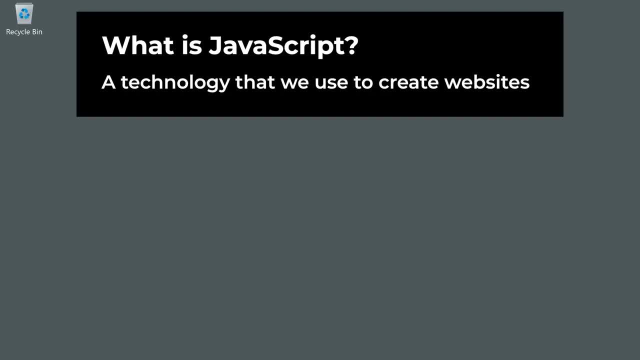 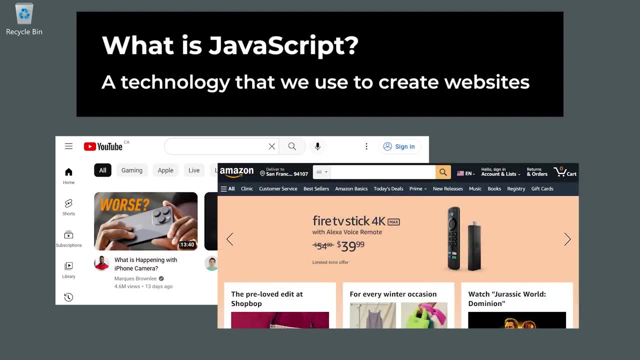 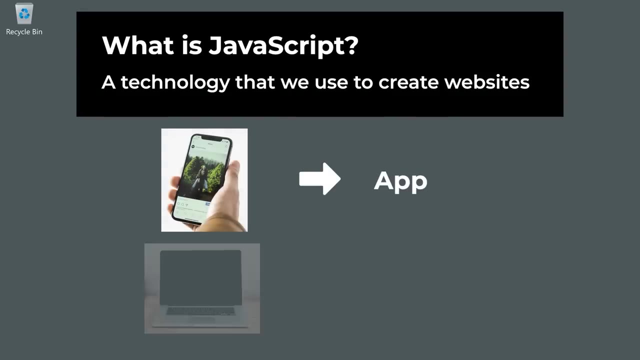 use to create websites. A website is like youtubecom or amazoncom. It's how we access YouTube and Amazon on our computer. If we were using a phone, we usually use an app, But on our computer we use a website. So there's actually three technologies that we 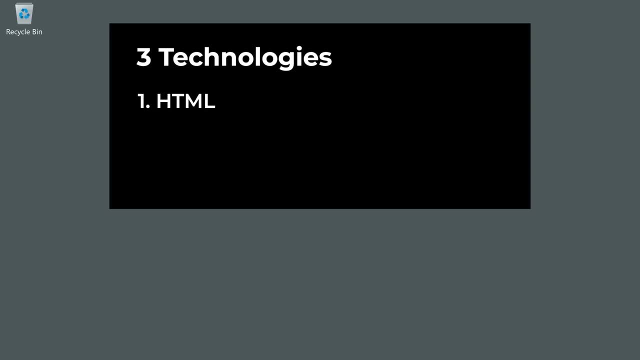 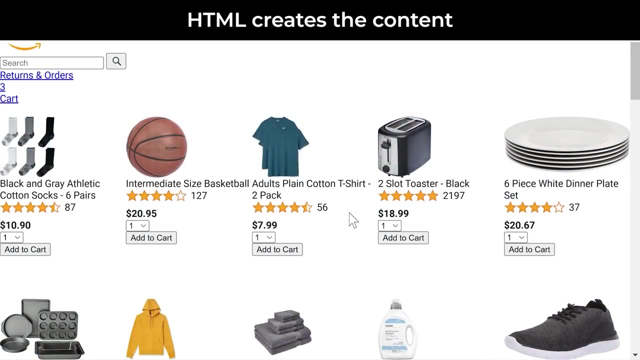 use to create websites: HTML, CSS and JavaScript. Each of these technologies has a specific purpose when creating a website. HTML creates the content of a website. It creates all the buttons, the text and the images. CSS changes the appearance of the website By adding CSS. 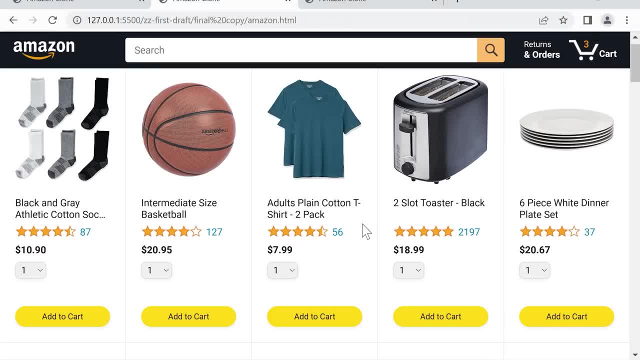 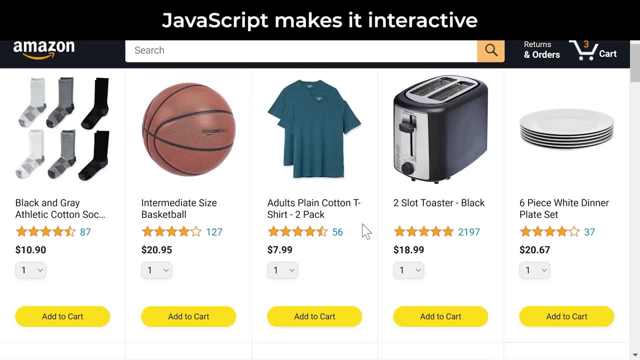 we can make our website look nice. And finally, JavaScript makes our website interactive. So if we only have HTML and CSS and we click one of these buttons, our website doesn't do anything. But once we add JavaScript, we can make our website do something when we click a button. 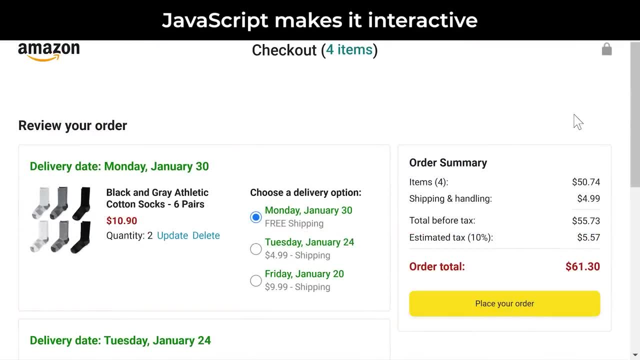 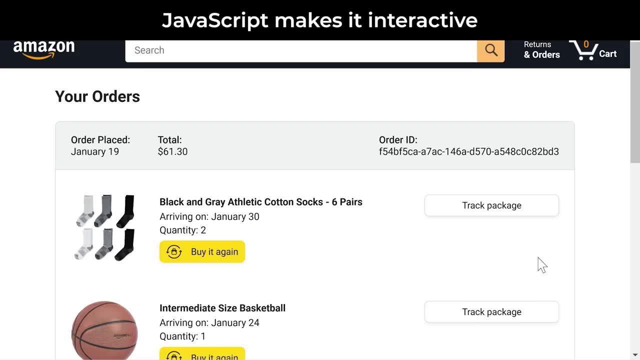 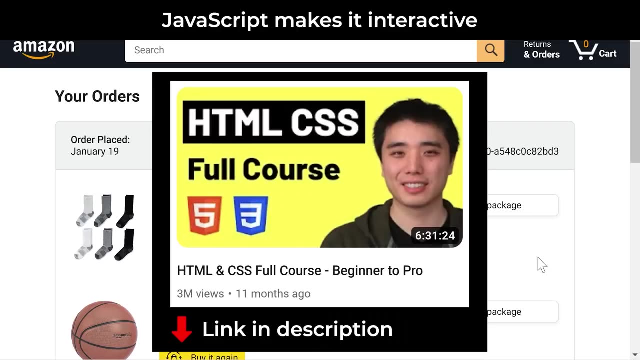 such as add a product to our cart or create an order, So this course is focused on JavaScript. If you want to learn HTML and CSS in more detail, I have a full course just like this one that you can find in the video description. 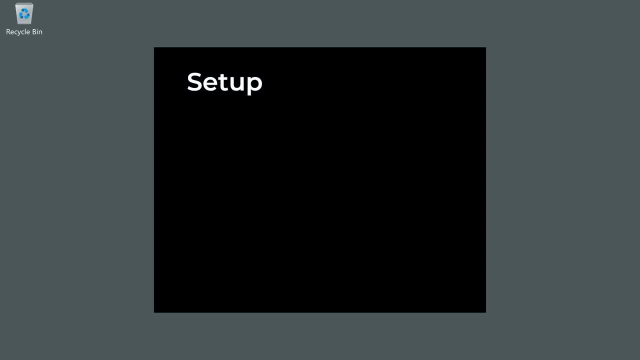 Let's get started with JavaScript. The first thing we need to do is to install a piece of software called a web browser. A web browser lets us view websites that we create in this course. The most popular web browser for web browsing is Google. 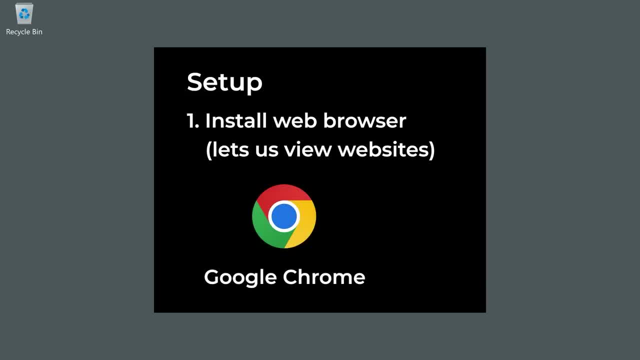 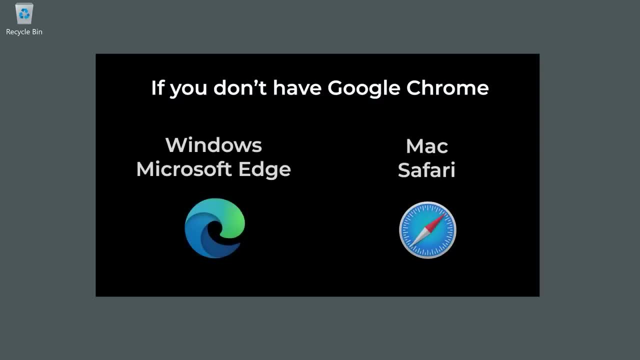 The most popular web browser for web development is Google Chrome, so I recommend using that. If you don't have Google Chrome, you can open the default web browser on your computer. For Windows it's Microsoft Edge and for Mac it's Safari. 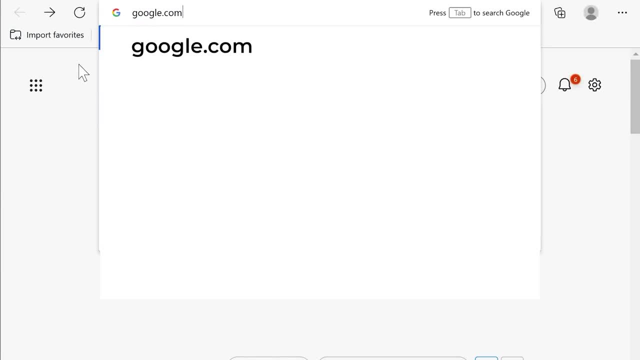 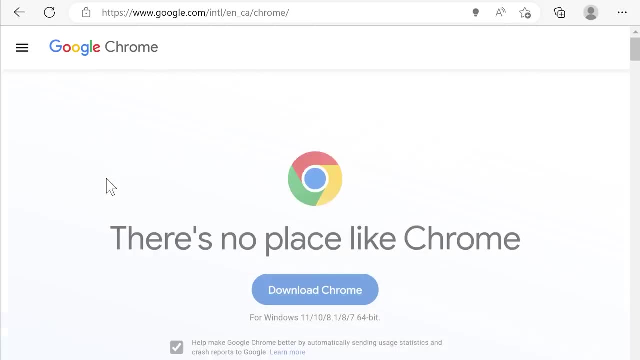 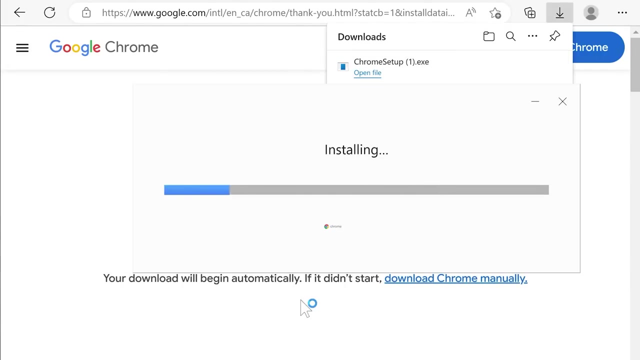 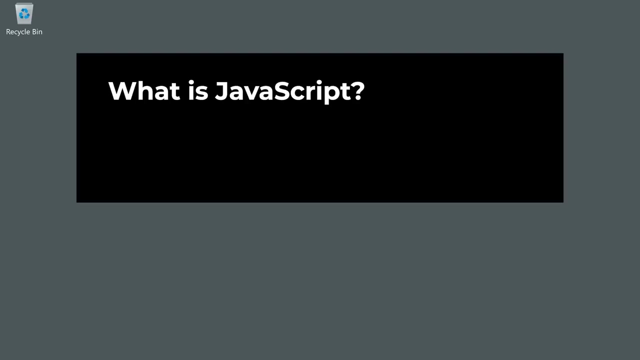 Type in googlecom at the top and press enter Search for Google Chrome, click the result and follow the instructions to download and install. Once we've installed Chrome, we're ready to begin. We're going to start by learning what exactly is JavaScript and how does it work. 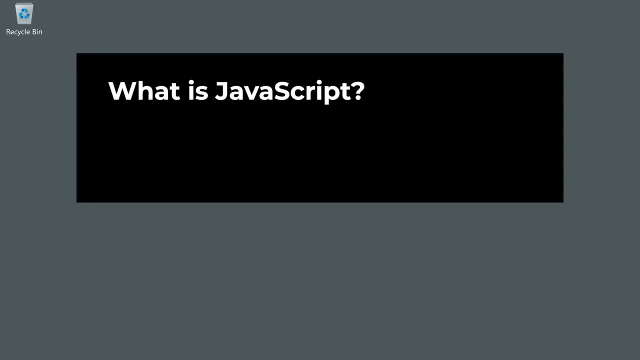 The easiest way to understand JavaScript is we're basically giving instructions to a computer and then the computer follows our instructions. I find the best way to learn this is to jump in and give it a try. So first let's open Google Chrome. 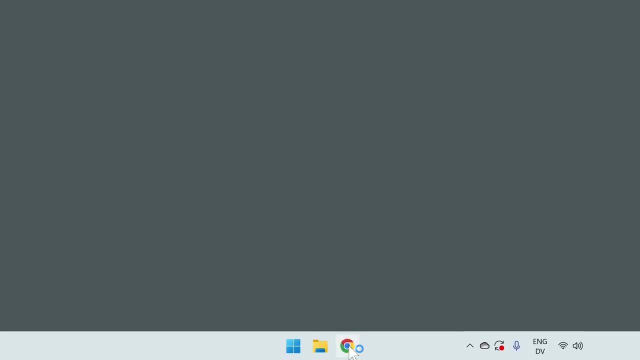 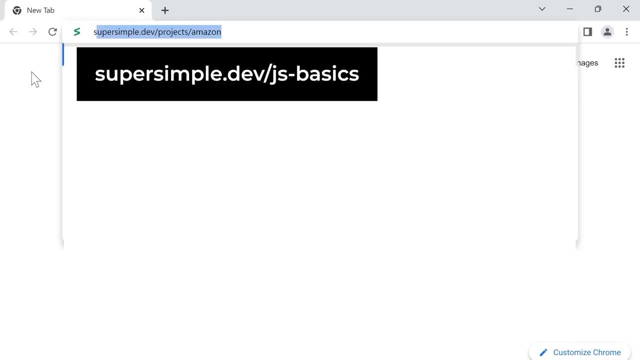 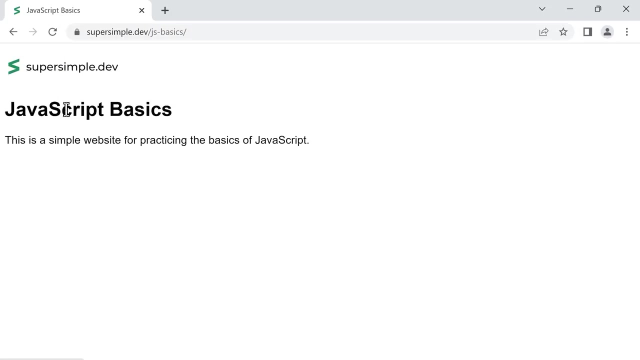 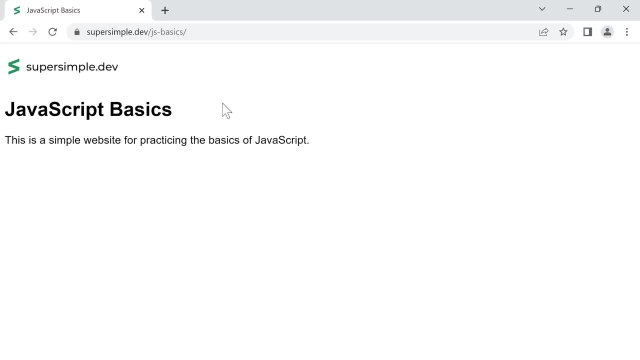 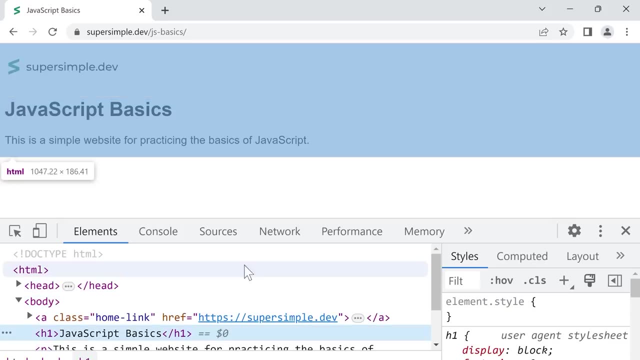 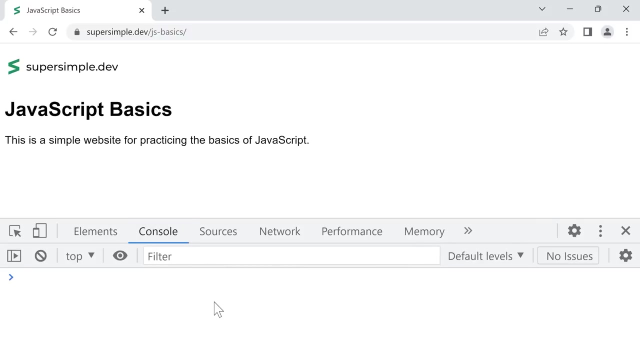 To do that? we're going to go to Google Chrome, We're going to go to a blank area of the webpage. We're going to right click, click, inspect and then click the console tab. Now, if your console doesn't show up at the bottom like this, you can click these three. 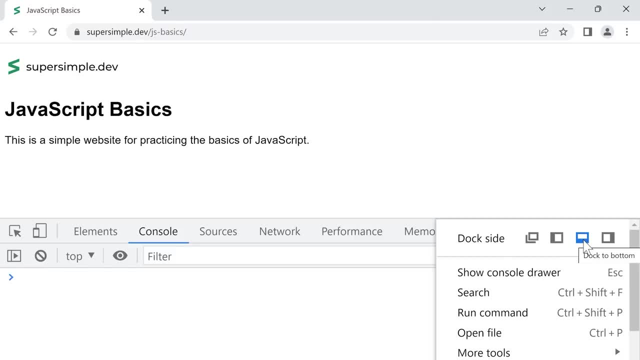 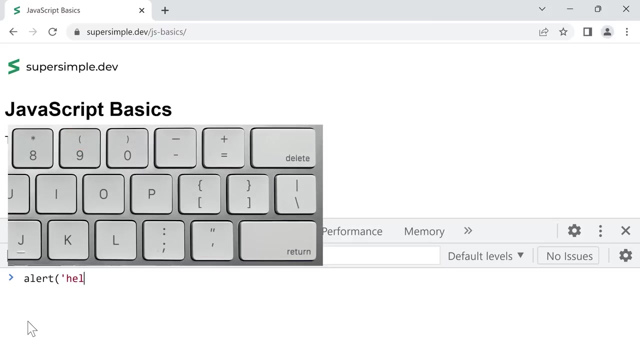 dots here and then select this icon. Okay, so inside the console we can give some instructions for our computer. Let's learn our first instruction. We're going to type here And we're going to type alert- open bracket. single quote. hello- single quote. close bracket. 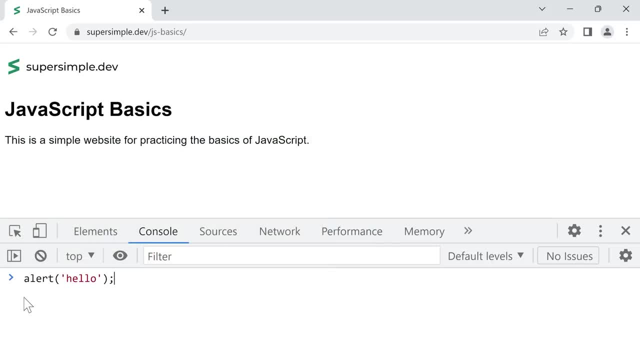 and semicolon. Make sure to type this out exactly as I have it here In JavaScript. if you don't type things out correctly, it won't work. So this is an instruction to create a plugin pop-up with the text hello inside to get the computer to follow our instruction. 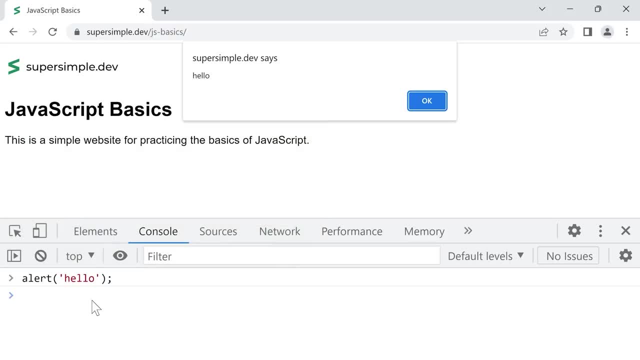 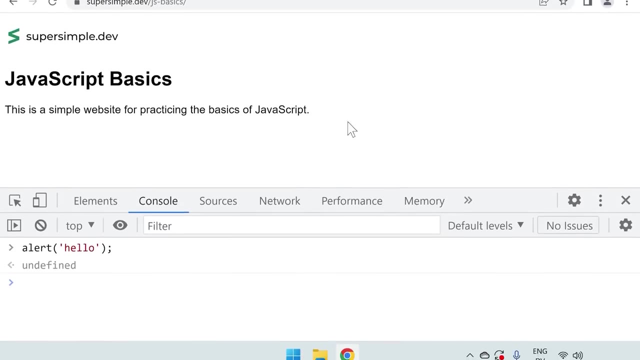 we can just press enter and, as you can see, the computer does exactly what we tell it to do. it creates a pop-up with the text hello inside. now let's press OK and let's give another instruction to the computer. so we're going to type here: 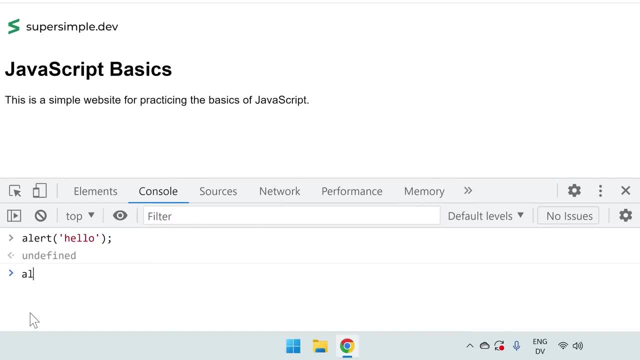 again and we're going to type alert again: open bracket, single quote. but this time we're going to type a different message in the pop-up: good job and single quote, close bracket and semicolon. so this is an instruction to create a pop-up again, but this time with the text good job inside the pop-up. 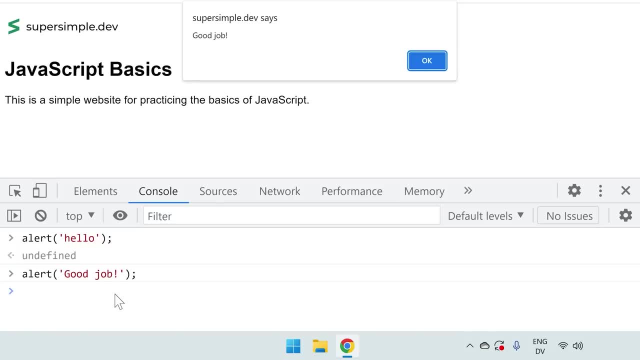 if we press enter, the computer does exactly what we tell it to do and it creates a pop-up with the text good job inside, and that's basically the main idea behind JavaScript. we're giving instructions to a computer and then the computer follows our instructions. so note that we can open and use this. 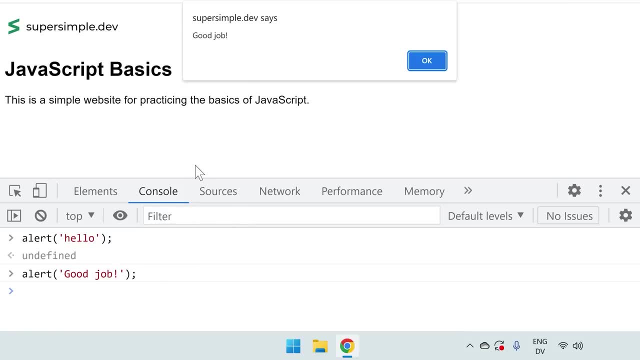 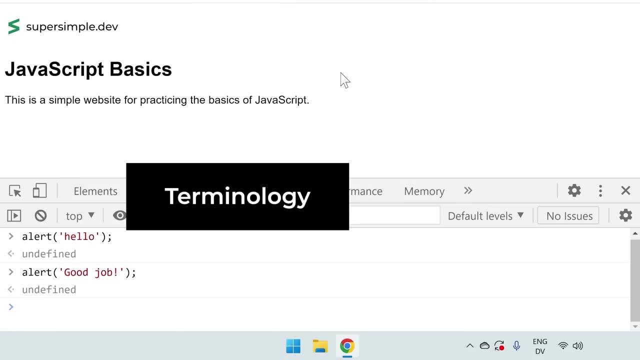 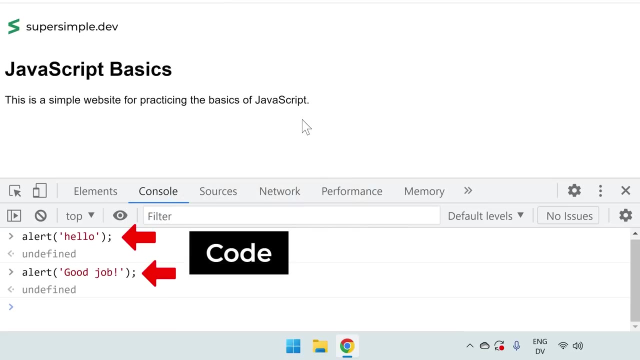 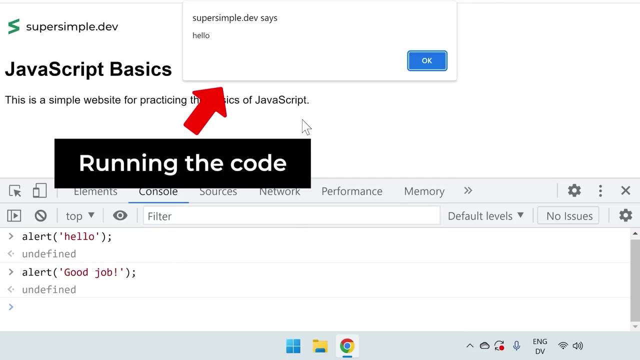 console on any website. we're just using supersimpledev as an example. let's press ok and we're going to learn some terminology: the instructions we give to our computer. these instructions are called code. when we press enter and the computer follows our instructions, this is called running the code. now 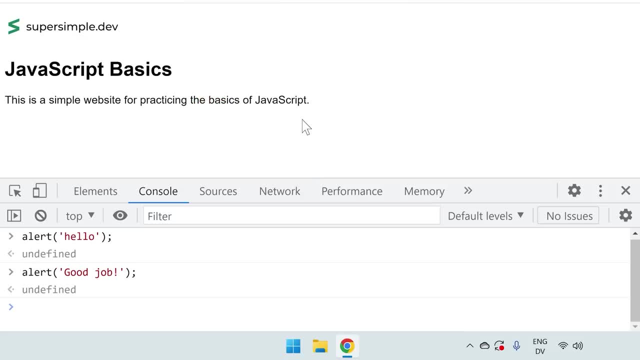 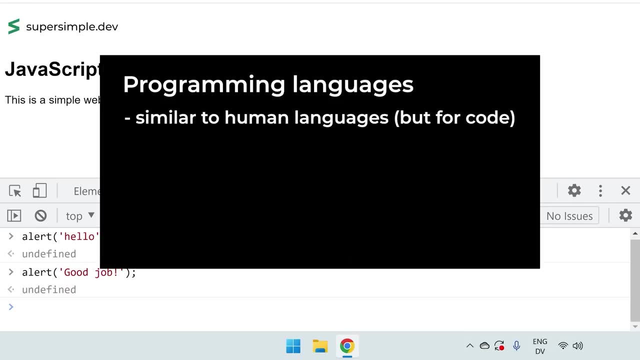 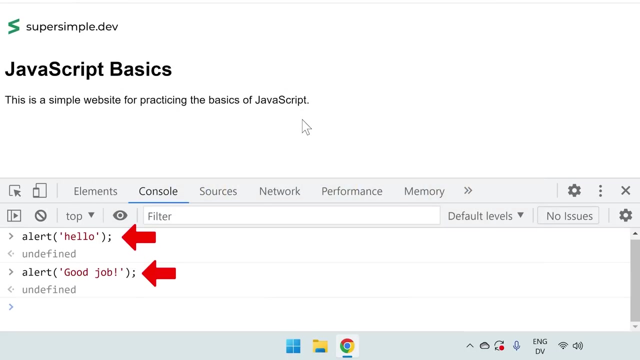 there are many different languages we can use to write code, called programming languages. it's similar to how we have many human languages that we can use to communicate. some examples of programming languages are JavaScript, Python and Java. so here we're writing our code using the JavaScript programming language, so we call this JavaScript code. now that we understand. 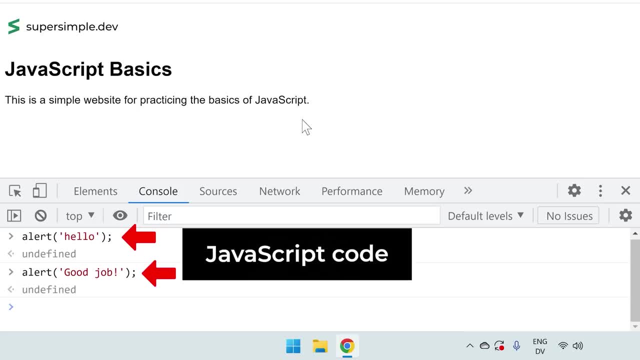 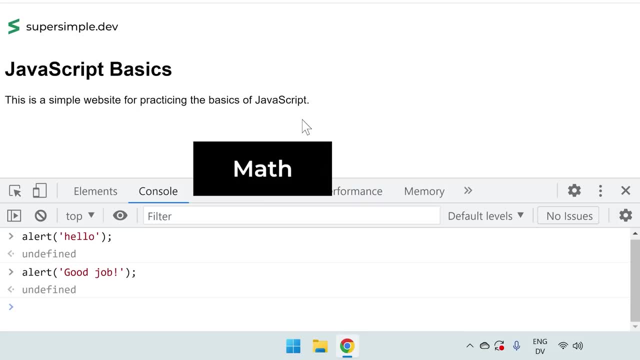 the basic terminology. let's look at some more examples of what we can do with JavaScript code. another thing we can do is math. let's go back to the console and type here, and we're going to type 2 plus 2. so this is an instruction or code that tells the computer to do some math, to. 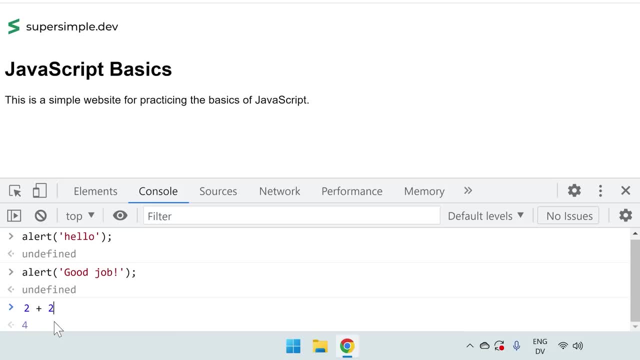 calculate 2 plus 2. when we press enter, the computer follows our instruction or runs this code, calculates two plus two and gives us the result, which is is 4.. Let's do another example. We're going to type 10 minus 3 and press enter to run this code. 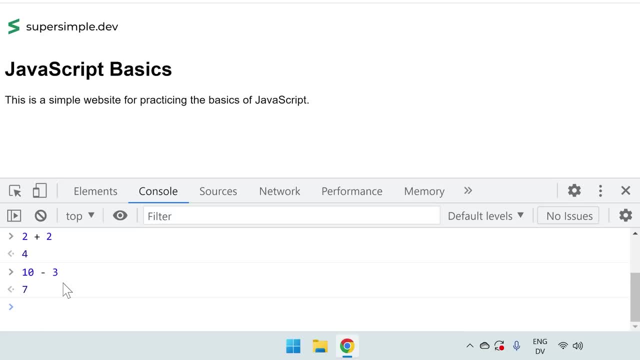 Again, the computer does this math, calculates the result and gives us 7.. So, as you can see, JavaScript can do many different things, like create pop-ups and do math. Let's look at one more example of what JavaScript can do. We're going to go to the bottom and type out this code: 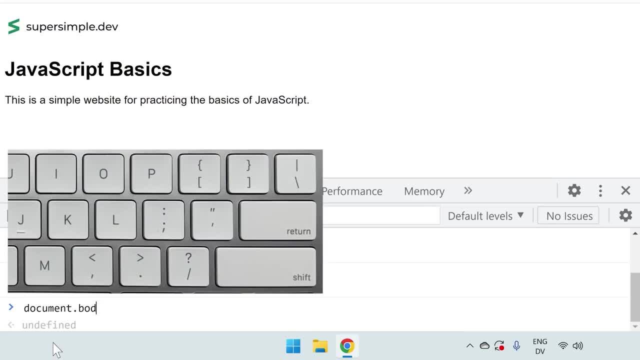 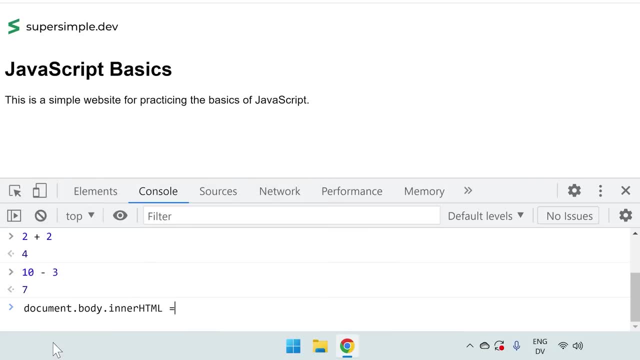 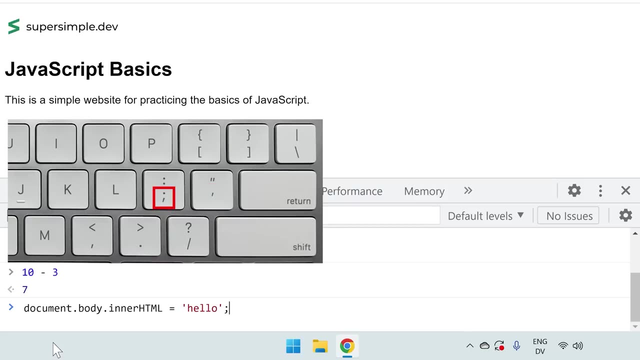 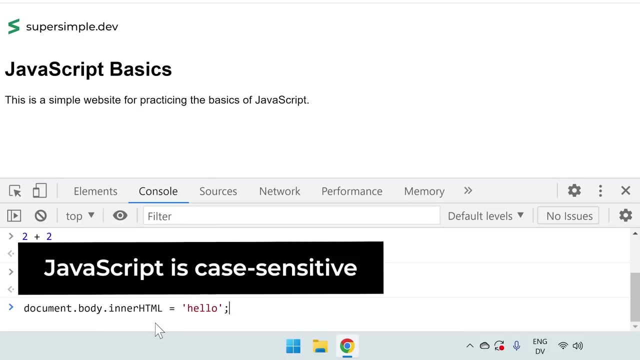 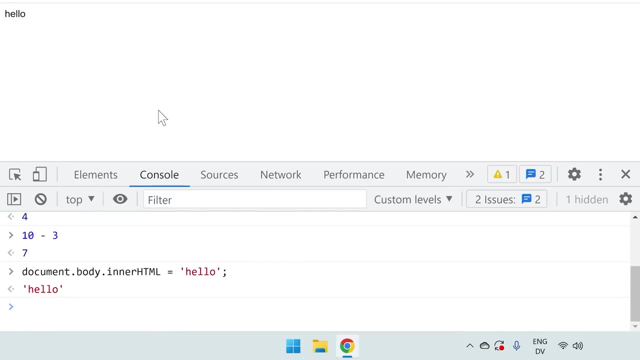 document: dot. body dot. inner capital html equals single quote, hello, single quote and semicolon. Make sure to write this out exactly as I have it here, With the dots and the capital letters, because JavaScript is case sensitive. Let's press enter to run this code. What this code does is that it removes everything on the page. 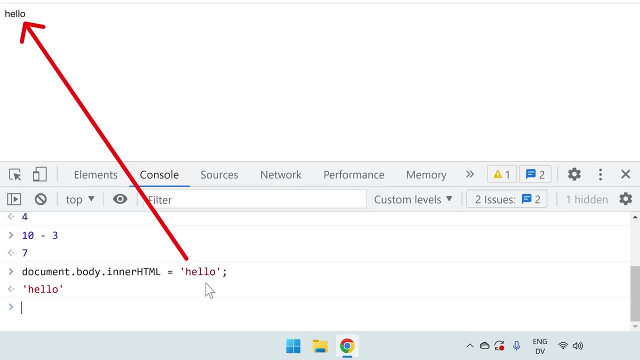 and replaces it with the text hello. In this example, we use JavaScript to modify the webpage. Modifying the webpage is one of the most important features of JavaScript and we're going to be feature throughout this course. And that's the basics of JavaScript. 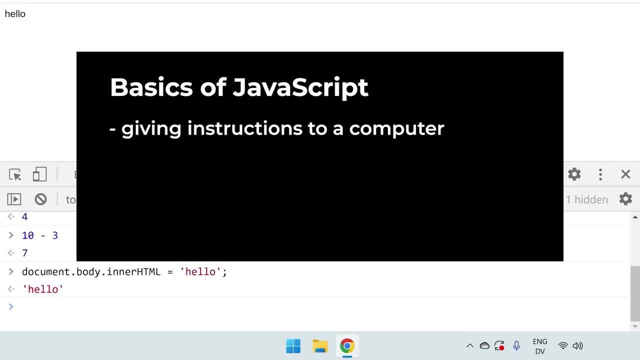 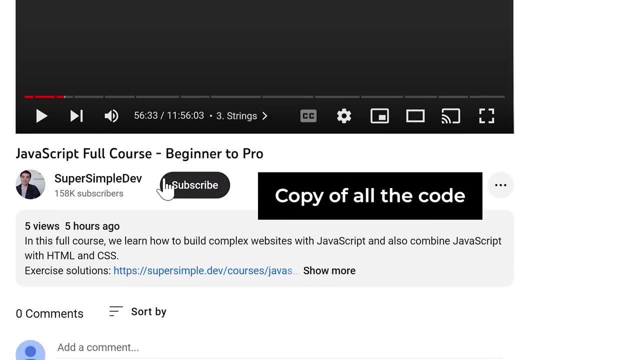 We're giving instructions to a computer. these instructions are called code, and then the computer follows our instructions. This is called running the code. And also, don't worry about memorizing all this code. you can find a copy of all the code that we write in this course in the video description. 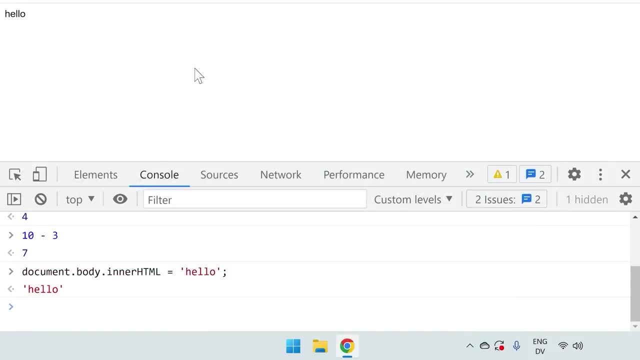 Now that we understand the basics of JavaScript, let's learn more about the JavaScript language itself. If we take a look at this code- alert and hello- you might be wondering what the brackets and the quote mean. All of these characters have a special meaning in the language. 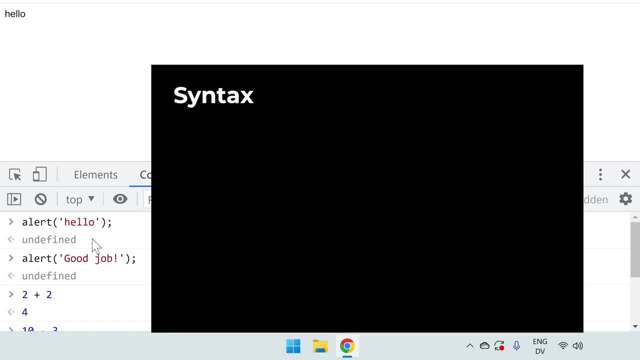 This is something called syntax. Syntax are the rules that we have to follow when using a programming language. This is sort of like in English. we also have rules that we follow, called grammar. The difference is that in English we don't have to follow the rules of grammar perfectly. 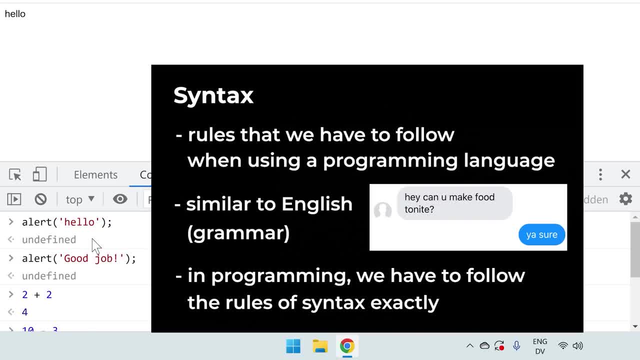 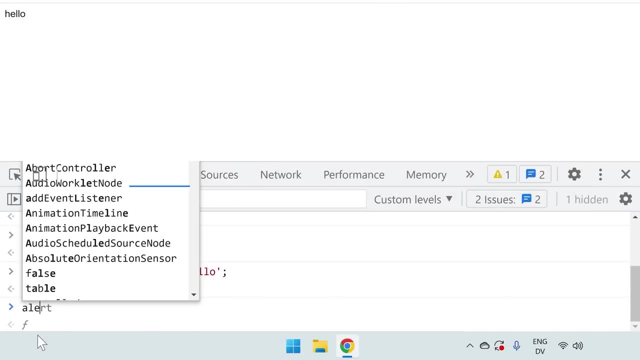 People can still understand us, But in programming we have to follow the rules of syntax exactly, otherwise the computer won't understand our code. For example, if we scroll down, If we scroll down, If we scroll down And we type this code: alert- open bracket, quote. hello quote. close bracket and semicolon. 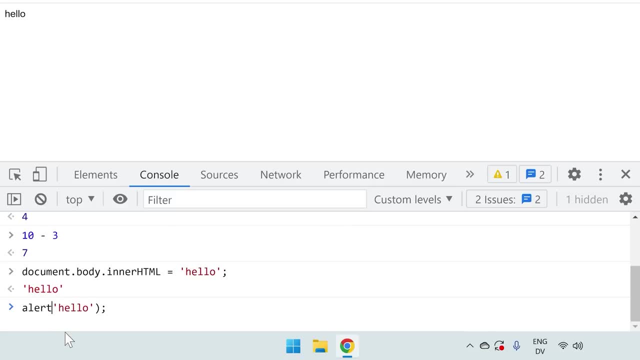 But this time we remove the first bracket and press enter, It will give us a syntax error. We're not following the rules of syntax, so the computer doesn't understand this code. Now, JavaScript has a lot of syntax, has a lot of syntax rules, and we can't learn them all at once right now. Instead, we're going to: 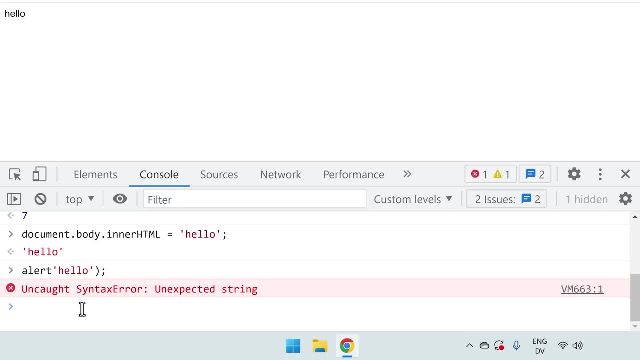 learn the syntax rules one by one as we go through the course. For now we'll just learn enough syntax to do the exercises at the end of this lesson. What we need to know is that if we scroll up, this part of the code tells the computer to create a pop-up. The text between these quotes. 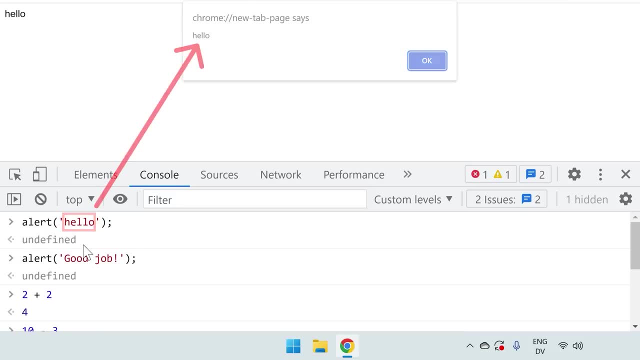 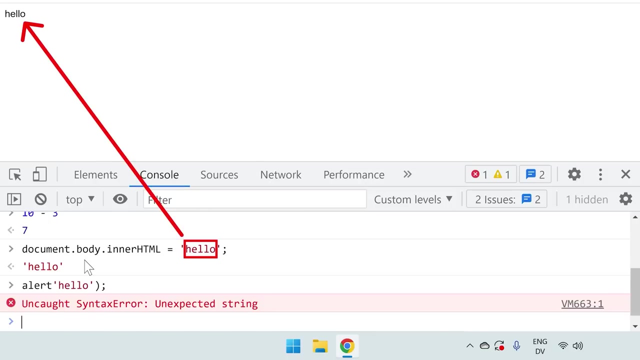 is the text inside the pop-up. If we change this text, we can change the text inside the pop-up. Same thing for this code down here: If we change the text between the quotes, it will change the text that appears on the page, And that's all we need to know about JavaScript. 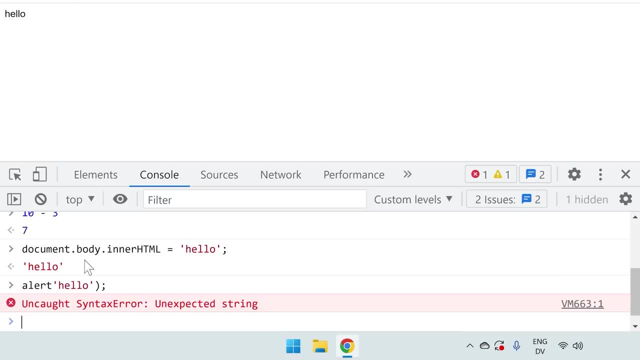 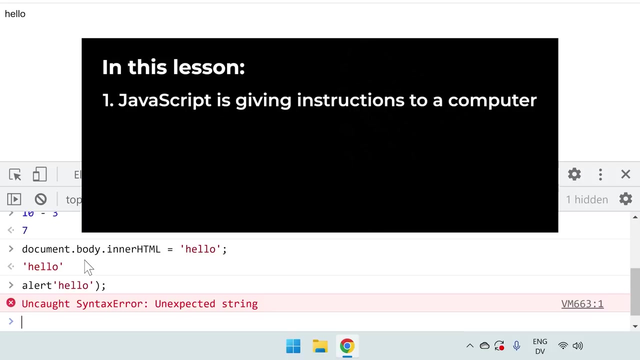 We'll learn exactly what the other characters, like the brackets, quotes and semicolon, mean later on in this course. So in this lesson we learned that JavaScript is basically giving instructions to a computer. We wrote our first few lines of JavaScript code. We learned how to. 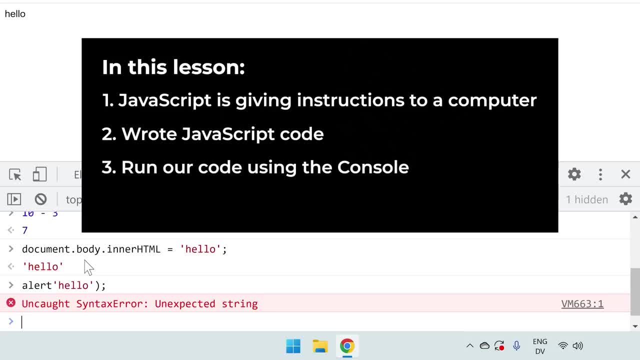 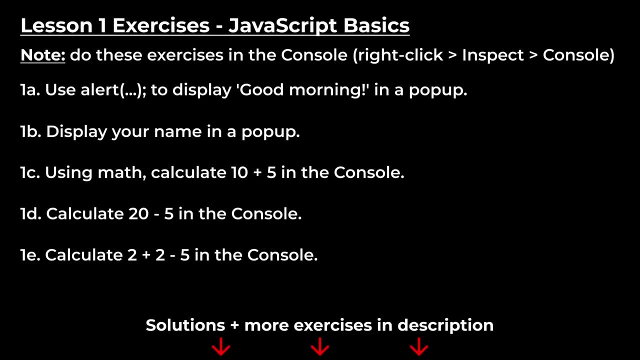 run our code using the console in our web browser And we learned about syntax, which are the rules that we have to follow when writing our code. Here are some exercises you can try on your own to practice what we learned in this lesson. You can find the solutions. 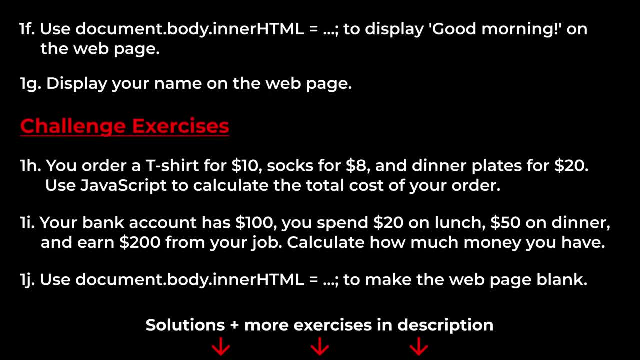 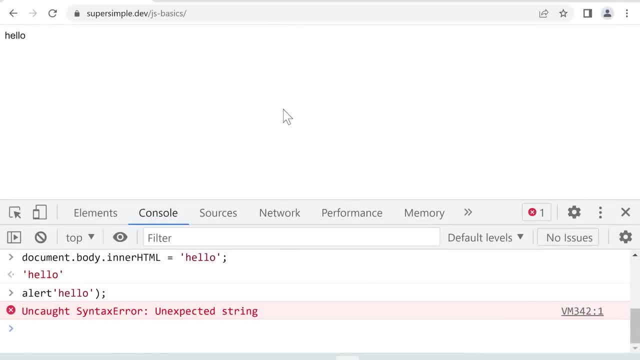 to these exercises in the video description. Now that we understand the basics of JavaScript, we're going to learn about each feature of the language. In this lesson, we're going to focus on numbers and math First. we can close the console for now. 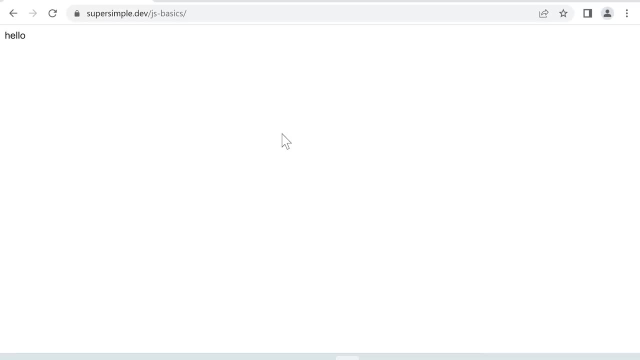 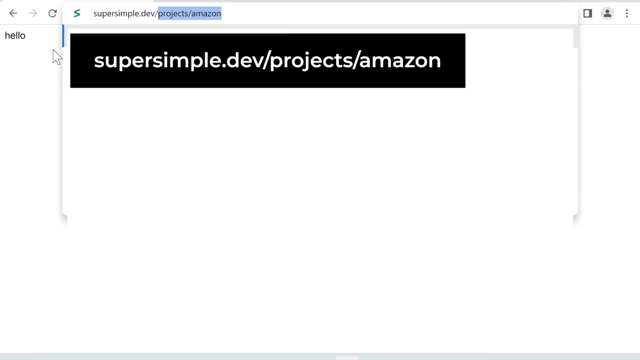 So I've actually prepared a project that we can use for this lesson. To open this project, we're going to go to our browser, click up here and type super simple: dot dev, slash projects, slash Amazon and press Enter. So this is actually the final project we're going to create in this. 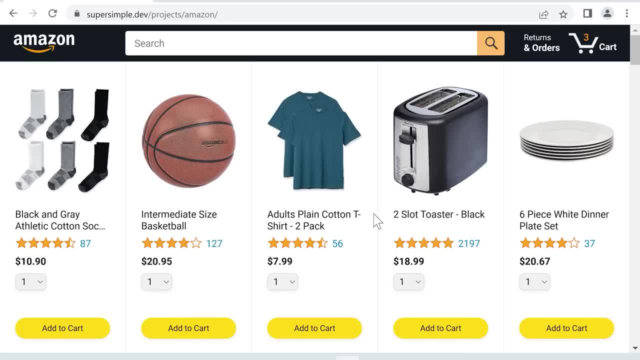 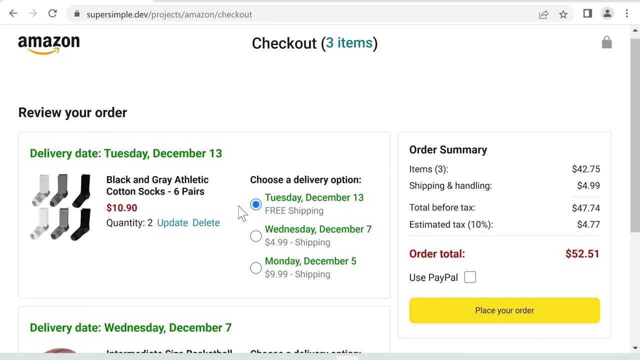 course, This is an ecommerce website similar to Amazon, where we can add products to our cart and then view our cart by clicking the top right, And on this page we can see the products in our cart cart, modify our cart and create an. 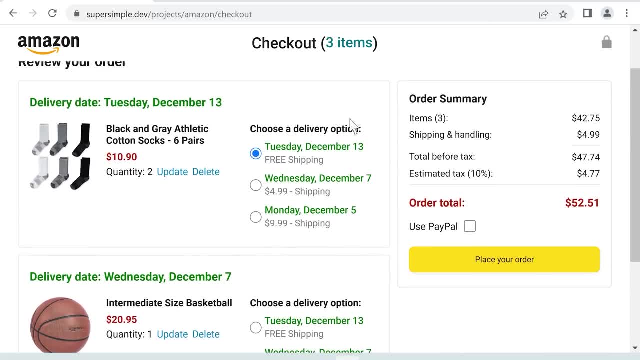 order For this lesson. we're going to focus on this write section, which calculates the cost of our cart, including the cost of the products, shipping and taxes. This section is a great way to learn numbers and math in JavaScript. First, let's open the. 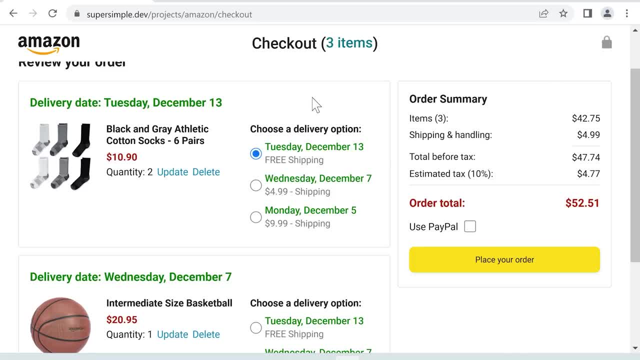 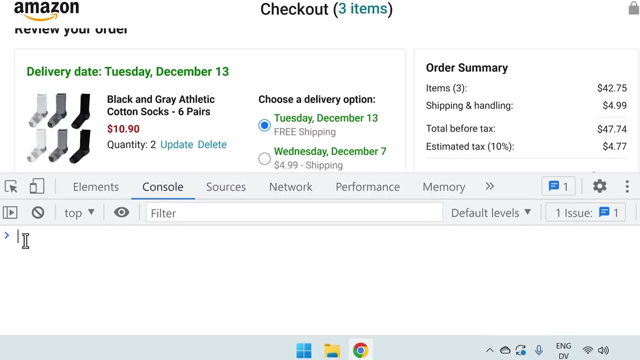 console again so we can write JavaScript code. We're going to find a blank area of the webpage, right-click, click Inspect and then click the console. So we already saw some examples of math in the previous lesson. For example, we wrote the code: 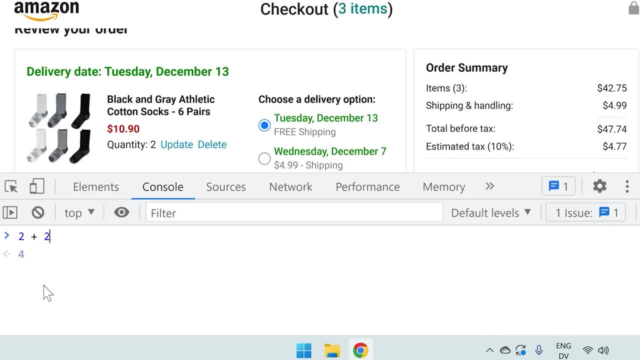 2 plus 2. If we press Enter, the computer adds these two numbers and results in 4.. We also did 10 minus 3. If we press Enter, the computer subtracts these two numbers and gives us 7.. In addition, 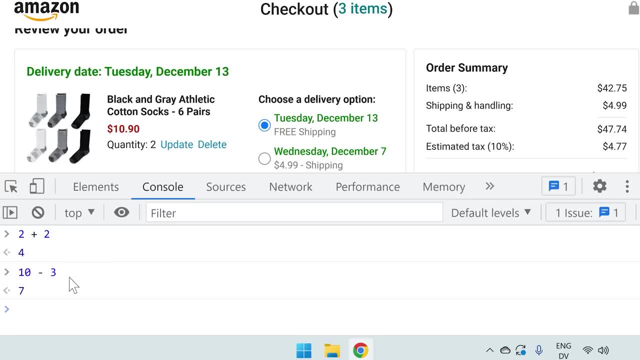 to adding and subtracting, we can also multiply and divide. To multiply, we're going to type 10 and press Enter, So star is the character for multiplying. To divide, we're going to type 10 and press Enter, So forward. slash is the character for dividing. 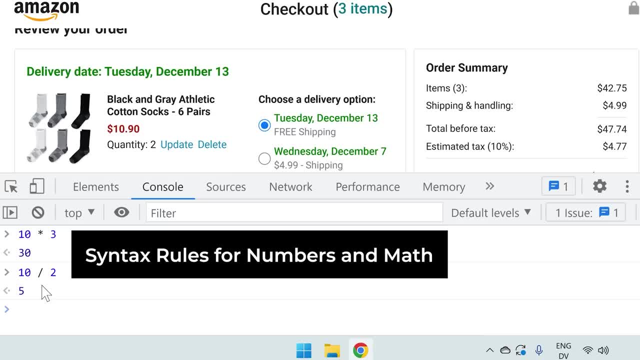 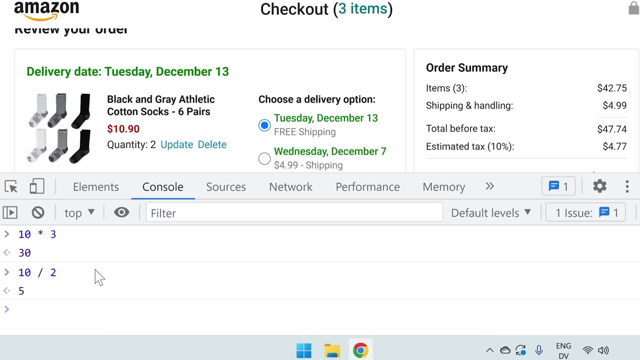 Now let's learn the syntax rules for numbers and math. The syntax for math is going to be very simple. syntax for math is pretty straightforward in JavaScript. We just write it out like normal math. We can also do math with more than two numbers. For example, we can add 2 plus 2 and. 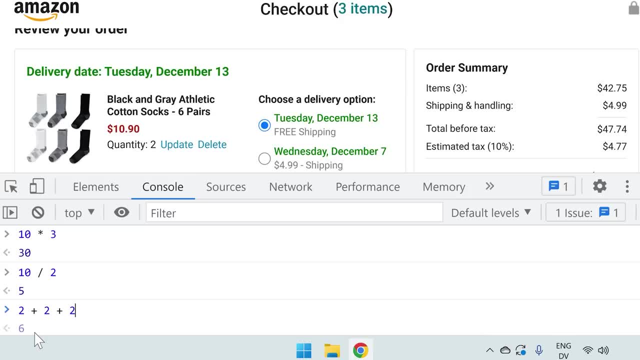 then plus another 2. If we press enter, the computer will add these three numbers together and result in 6.. And finally, JavaScript can handle decimal numbers like 2.2 plus 2.2. If we press enter, it will calculate these decimal numbers and result in 4.4.. 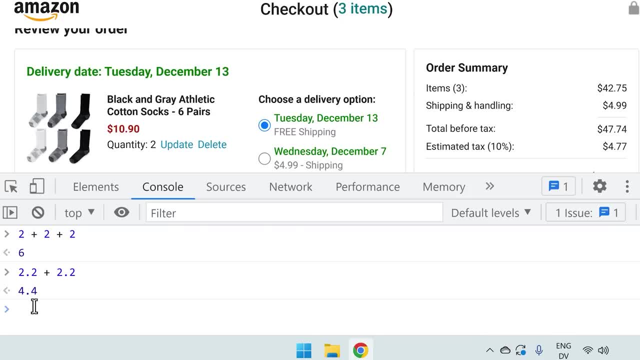 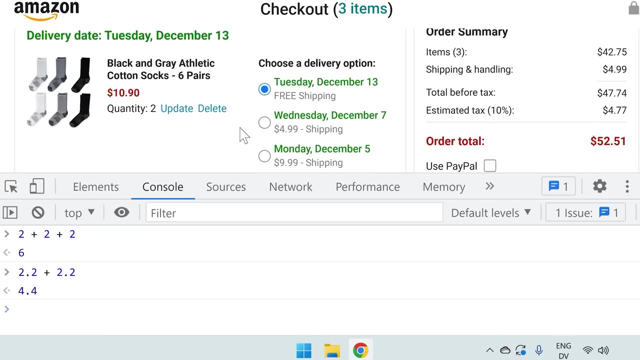 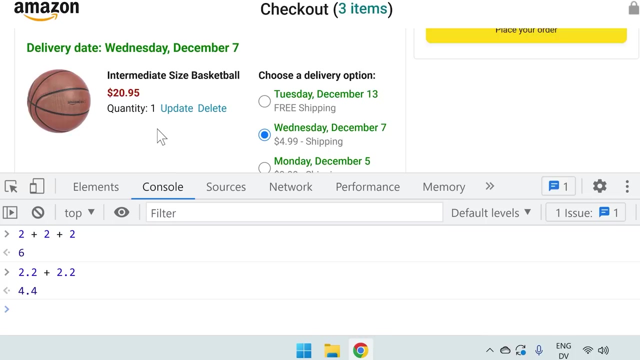 Now let's do some practical examples. We're going to calculate the numbers here in our final project, But first let's set up our cart so we have the same products in our cart. So make sure in your cart you have two socks with free shipping and you have one basketball with $4.99 of shipping. 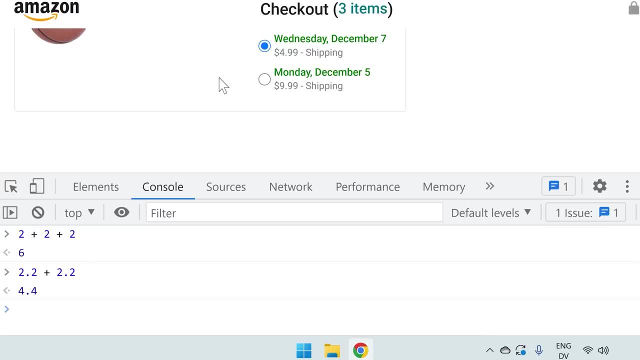 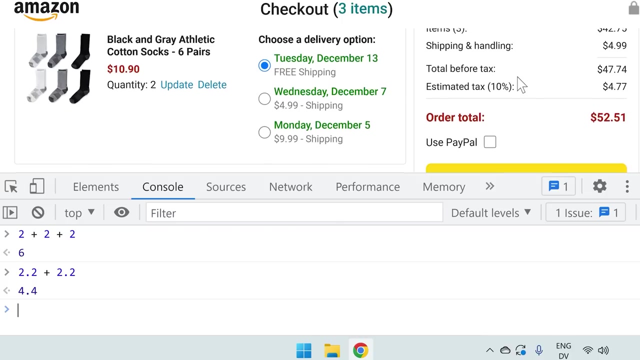 and nothing else in your cart. If you need to, you can modify your cart by clicking update or delete your cart, Or by going to the homepage by clicking in the top left and adding any products that you're missing. Once you have the same products as me in your cart and you have the same numbers on the 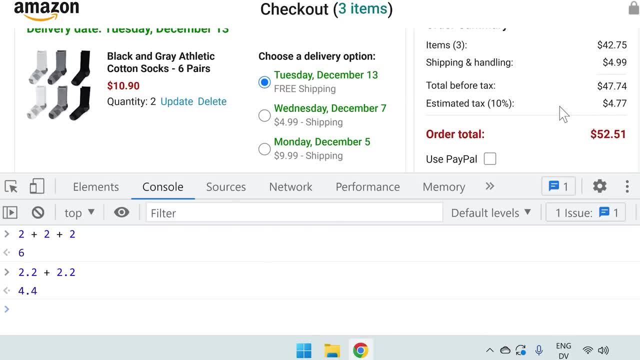 right, we're ready to begin. Let's start by calculating this number up here. This is the cost of the products before shipping and taxes. To calculate this number, you need to add a number. Using JavaScript, we're just going to add the cost of the products. So in our console we're going to add the 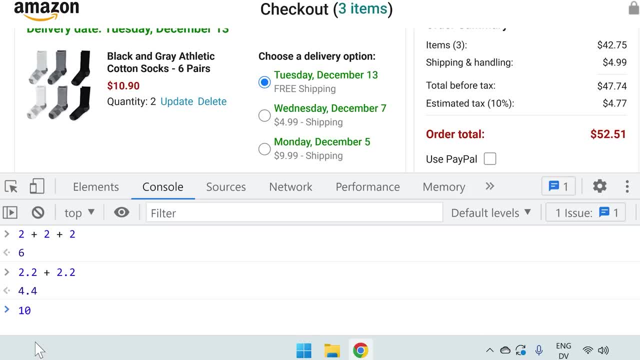 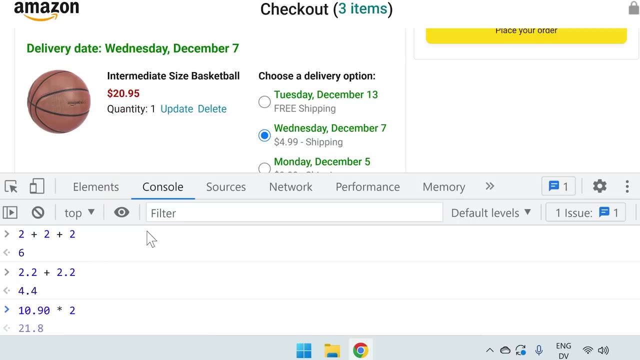 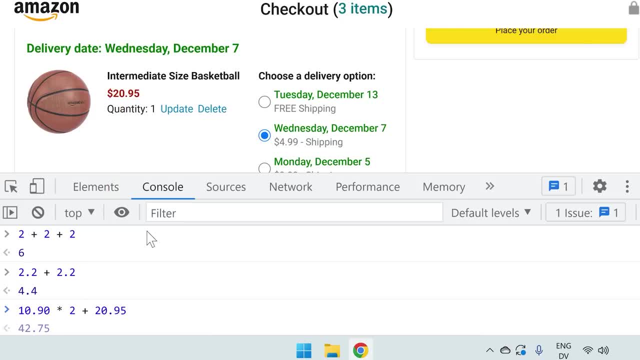 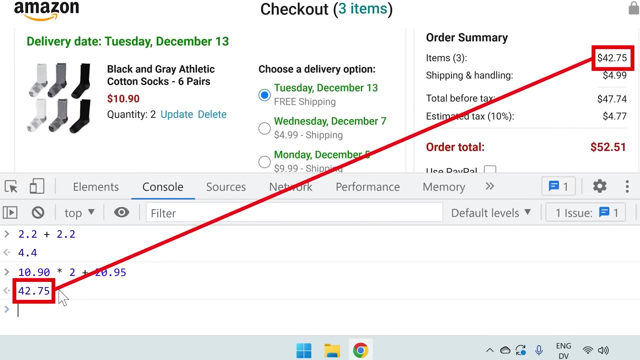 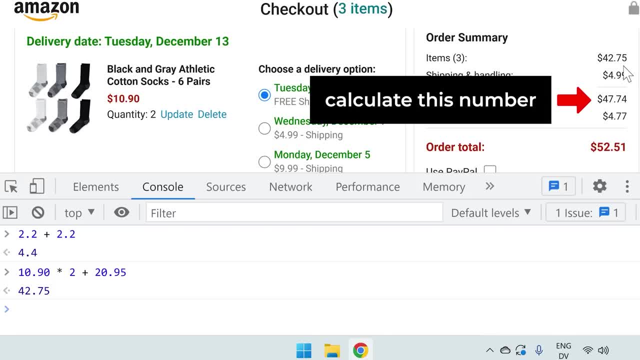 add this third number, which is the cost of the products plus shipping. Feel free to pause the video if you want to try it yourself first, Otherwise we'll do it together. Let's go back to our console And we're going to add the cost of the products again, which is $10.90 times two plus $20.95.. So we're going to add the cost of the. 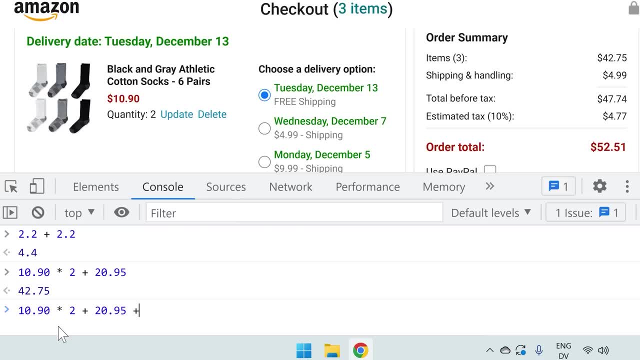 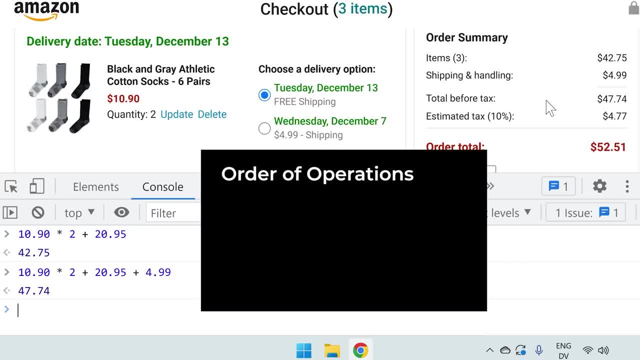 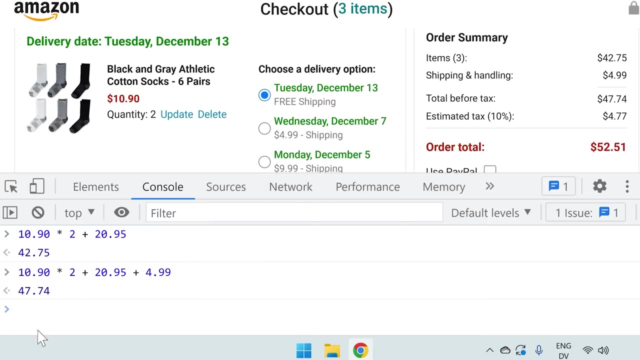 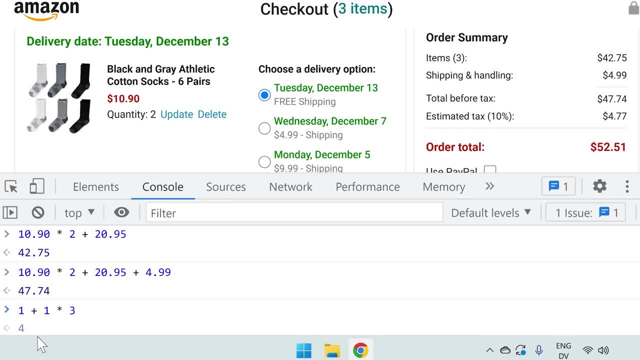 times 3, and press enter. Notice that it multiplies 1 times 3 first, which equals 3,, and then adds 1,, which equals 4.. Notice that it does not add 1 plus 1 first, which equals 2,. 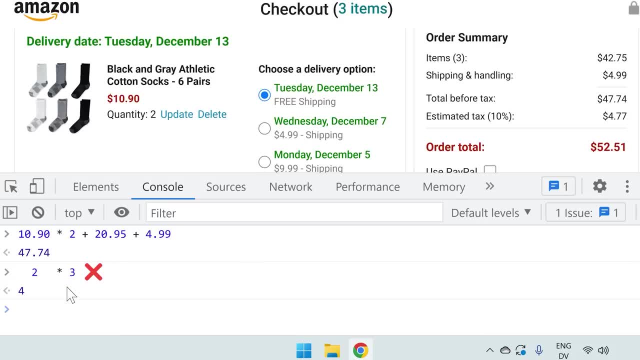 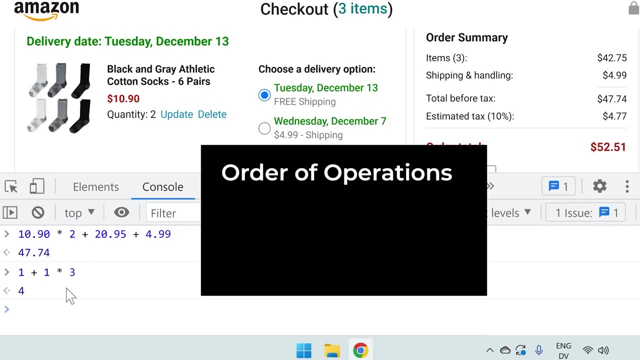 and then 2 times 3 equals 6.. The way math normally works is that multiply and divide are done first, add and subtract are done after. This is called the order of operations, and JavaScript follows the same rules. Multiply and divide are done first, add and subtract are done after. 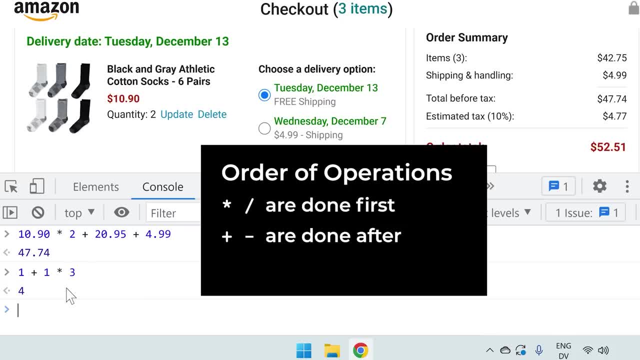 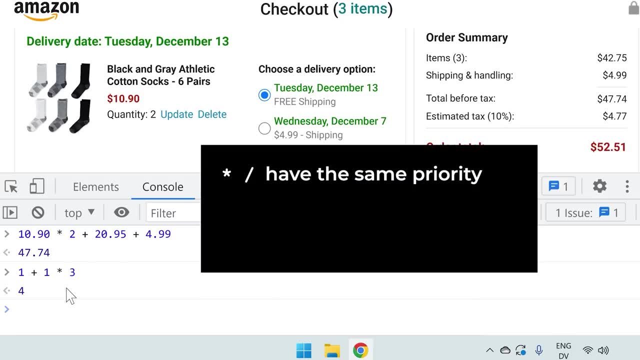 The order of operations is called the order of operations. The order of operations is also called operator precedence in JavaScript. One thing to note is that multiply and divide have the same priority. So if we have both in a calculation, it will calculate from left to right. Add and subtract also have the same 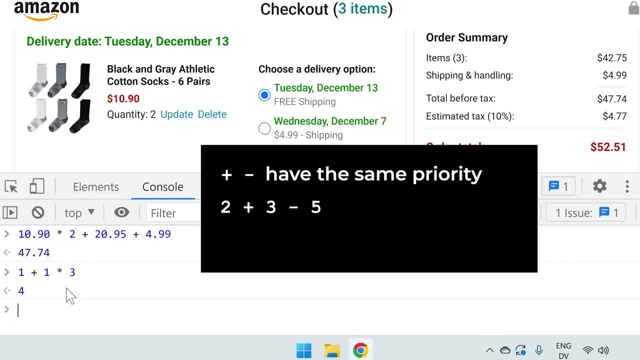 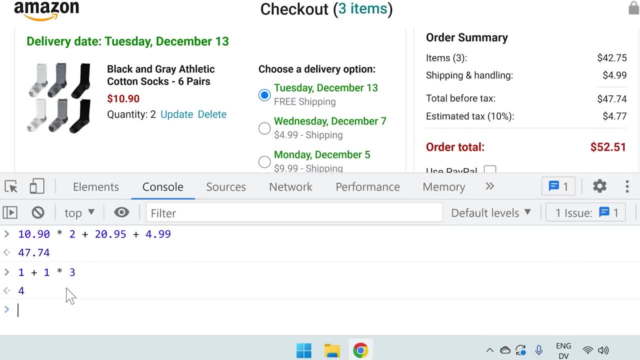 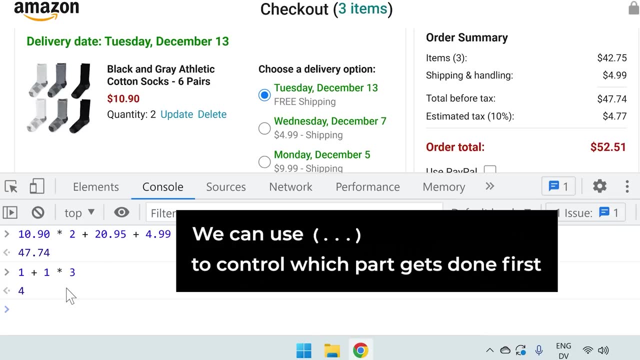 priority. If we have both in a calculation, it will also calculate from left to right. Another feature of the order of operations is that we can use brackets to control which part of the calculation gets done first. For example, let's type out this calculation again. 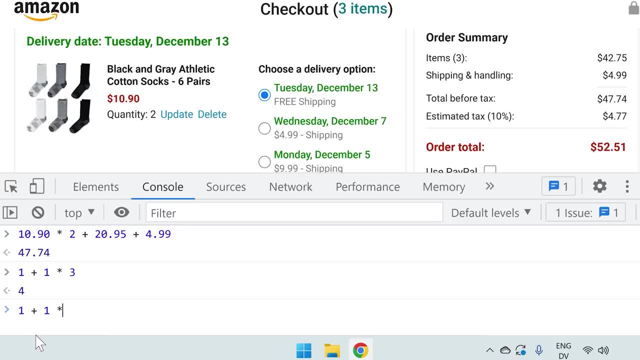 1 plus 1 times 3.. But this time we're going to add an open bracket and a closed bracket Around 1 plus 1.. If we press enter now, the calculation inside the brackets will be done first, So it will add: 1 plus 1 equals 2, and then 2 times 3 equals 6.. So when we use brackets, 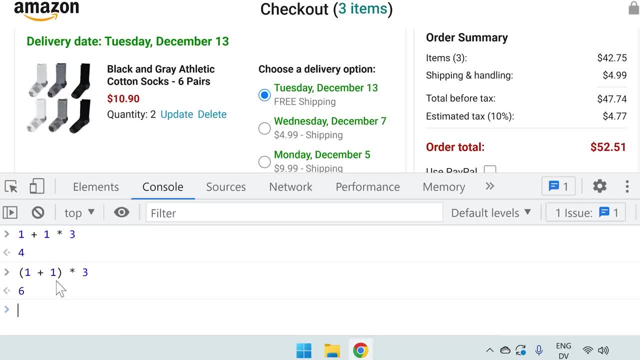 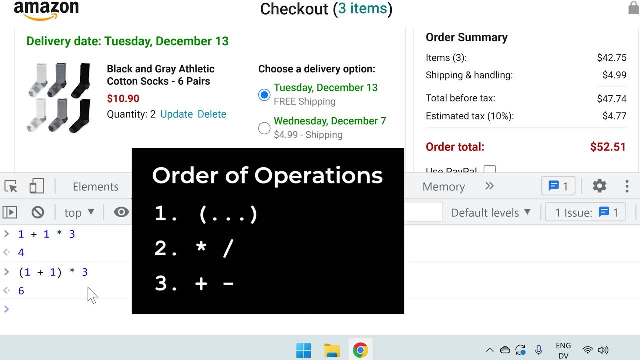 JavaScript will always do the calculation inside the brackets first and then do the rest of the calculation inside the brackets. So we're going to add 1 plus 1 equals 2, and then 2 times 3 equals 6.. Brackets have the highest priority in the order of operations. 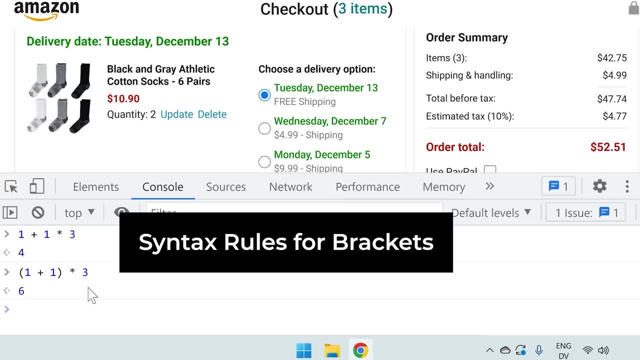 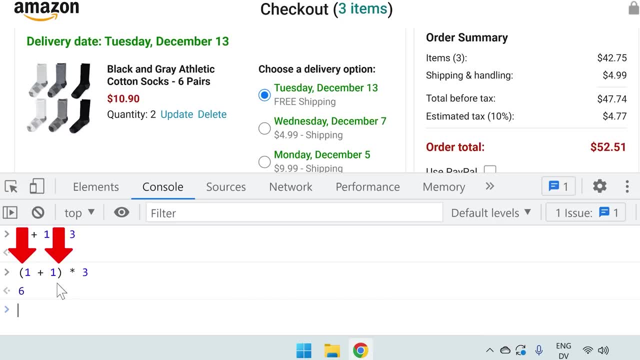 Now let's learn the syntax rules for brackets. So we just have to have a matching open bracket and closed bracket. So something like this doesn't work because we have two open brackets and no closed bracket. We also need to have a complete calculation in the brackets. 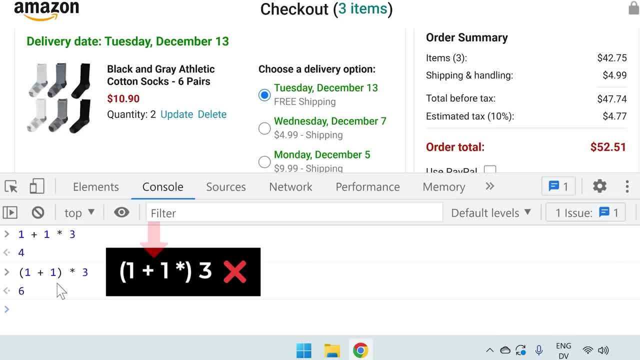 So this also doesn't work, because 1 plus 1 multiply is not a complete calculation. Now let's do some practical examples using the order of operations. First, we're going to do some more setup in the final project, So we're actually going to remove all the products in our 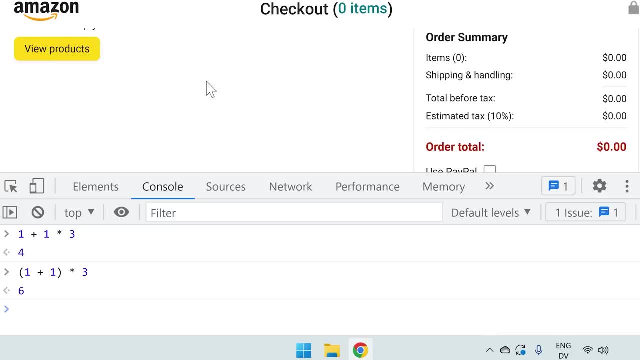 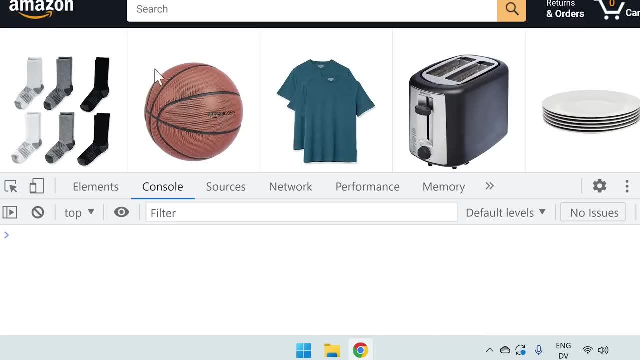 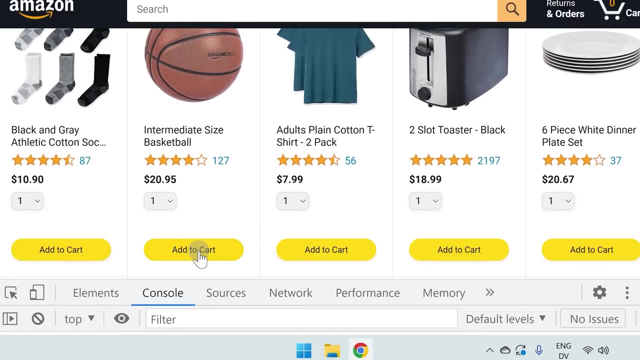 cart And then, once our cart is empty, we're going to do some more setup. in the final project. We'll go to the homepage by clicking the top left, And this time we're going to add some new products. So we'll add one basketball and two t-shirts. Now let's go back to our cart by clicking 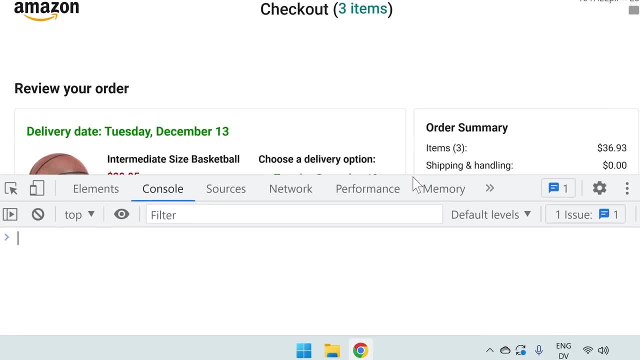 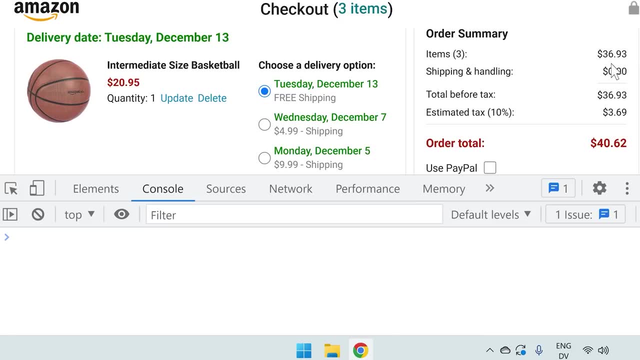 the top right. We'll scroll down and we're going to calculate the numbers in this section. again, Let's calculate this number at the top, which is the cost of the products. We'll go back to our console and add the cost of the basketball, which is $20.95, plus the cost of the t-shirts, which is 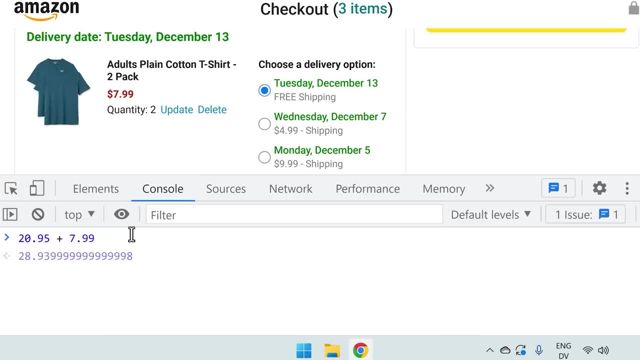 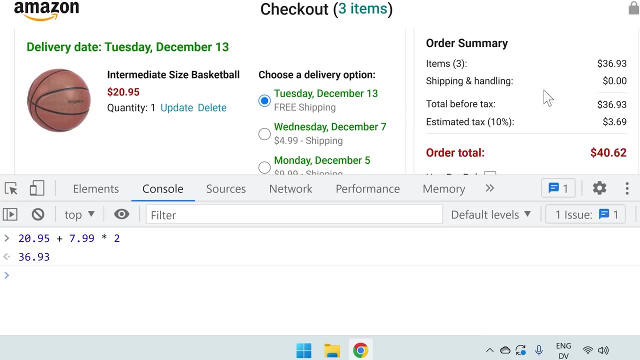 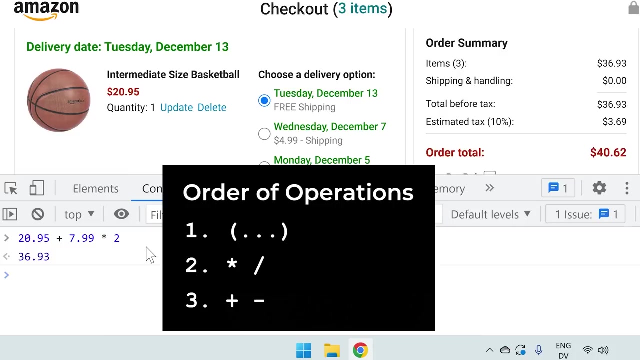 $7.99.. And we have two of them, So we'll multiply by two. If we press enter, this will give us the number that we see in the final project here. Notice that in this calculation we're taking advantage of the order of operations, Even though 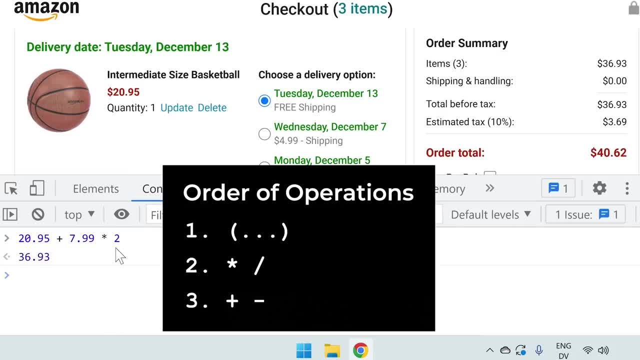 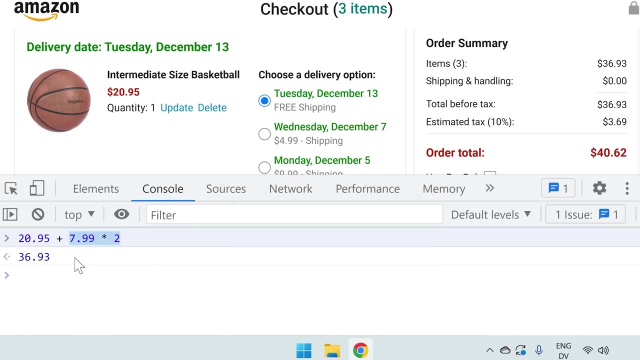 multiply is written last. we still multiply these two numbers first, So we calculate the cost of two t-shirts first, And then we add the cost of the basketball after. Okay, now let's try something a little more difficult. We're going to learn how to calculate. 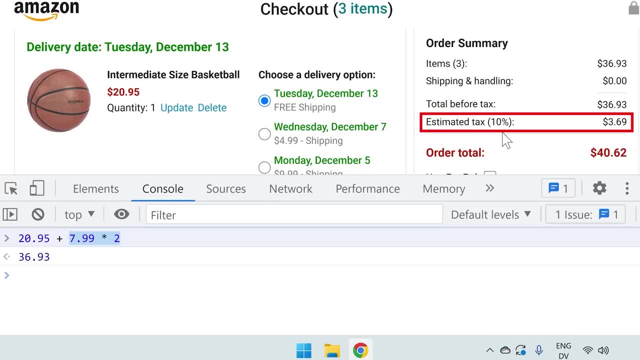 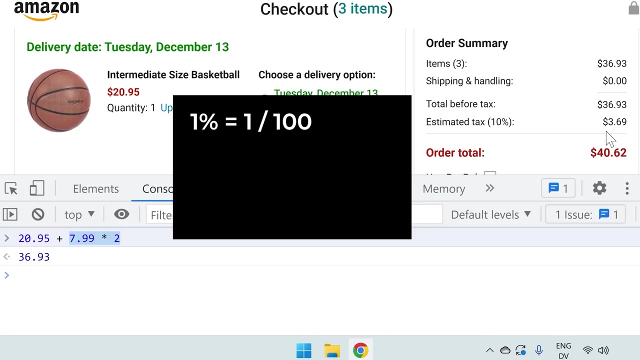 this 10% tax here. So how do we calculate 10% of something? Unfortunately, we can't just multiply by 10% in JavaScript. Instead, we have to calculate the percent manually. So how do we do that? 1% is actually equal to 1 divided by 100.. That's what per cent means. 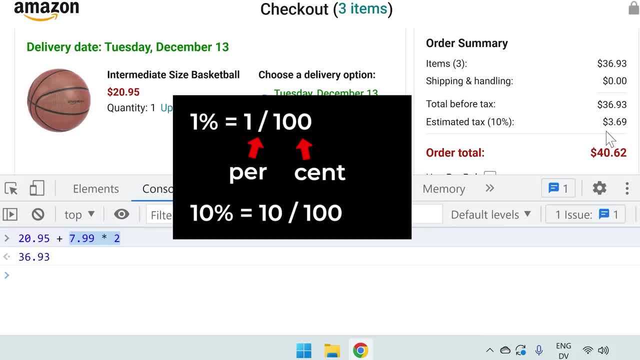 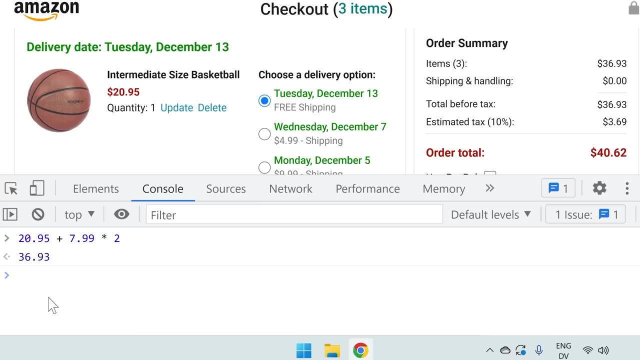 So 10% is equal to 10 divided by 100, which equals 0.1.. So to calculate 10% manually, we just multiply this number by 0.1.. So we'll type 36.93 multiplied by 10% or 0.1.. 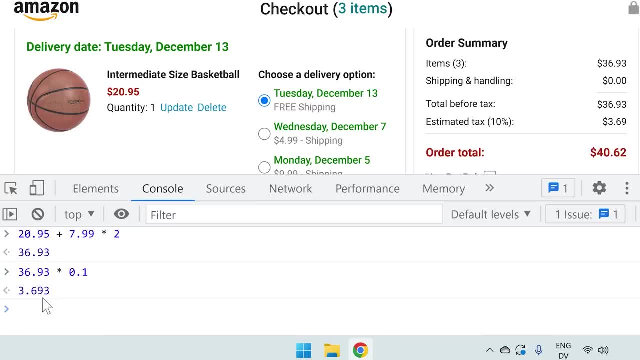 If we press enter, it will give us a number that is close to what we have in the final project. It's the same amount of money, but our number is more accurate than we need. So later in this lesson we'll learn how to round this number down to 10%. 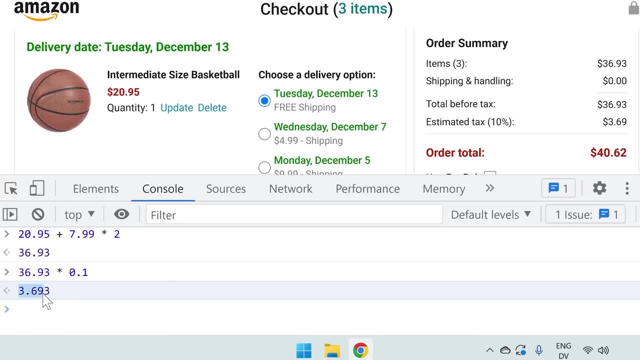 And we'll also learn how to calculate the cost of the basketball. For now, let's do some more practice with the order of operations. Let's calculate the tax again, except instead of using the final number, 36.93, let's calculate this number individually, like here. 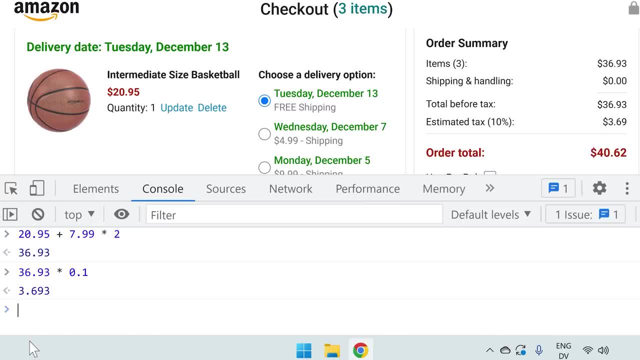 So at the bottom we're going to add the cost of the basketball- 20.95, plus the cost of the t-shirts- 7.99, times 2, and then multiply this by the tax percent times 0.1.. 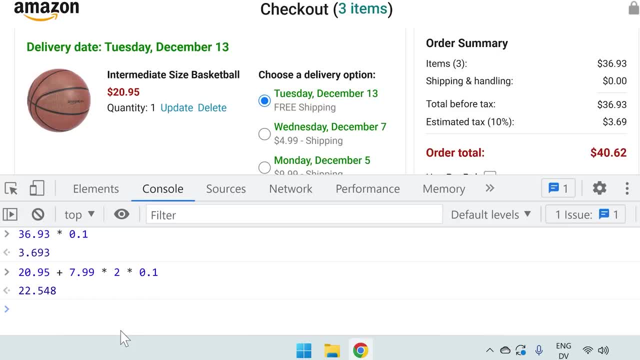 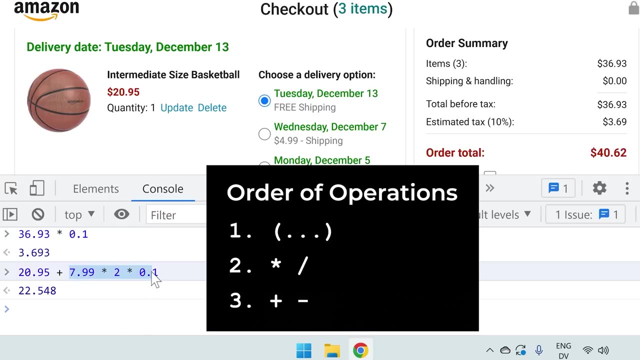 And press enter. Unfortunately, this number doesn't match what we got up here, And that's because, if we look at this calculation according to the order of operations, multiply is done first, So it will multiply these three numbers first and then add 20.95 after. 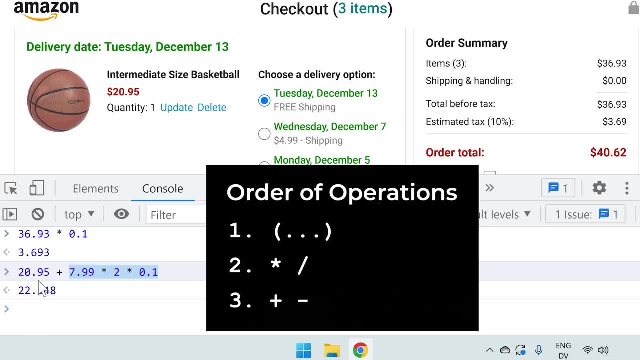 However, this is not what we want. We actually want to calculate this number first. This is the cost of the products. So how do we get the computer to calculate this first and then multiply by the tax percent 0.1?? 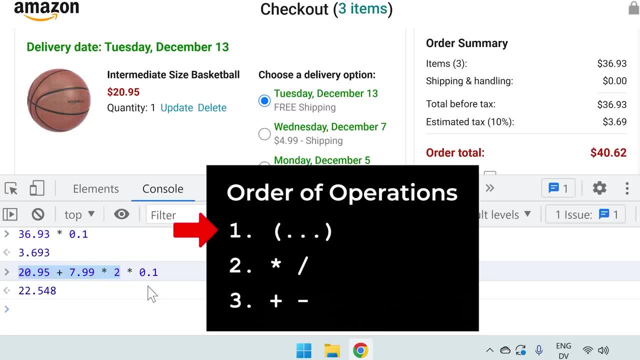 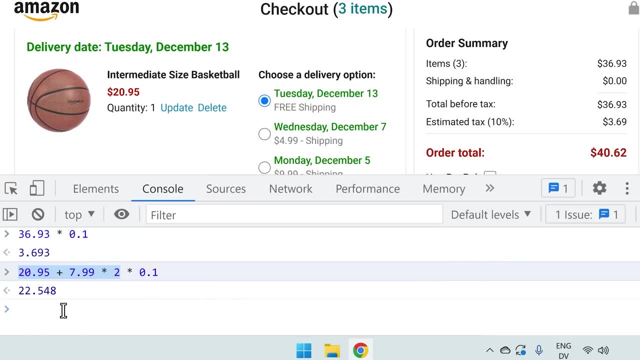 To do this, we can use brackets to control which part of the calculation gets done first. So let's create this calculation again: 20.95 plus 7.99 times 2.. But this time we're going to add brackets around this part of the calculation. 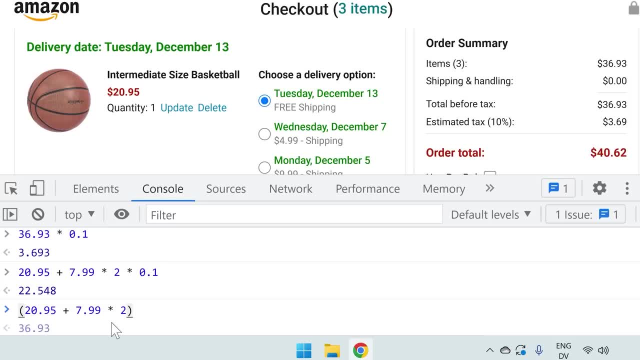 to make sure that this gets calculated first, And then, at the end, we'll multiply it by the tax percent: 0.1.. And now, if we press enter, we will get the same number that we had before. So that's how we use math and the order of operations. 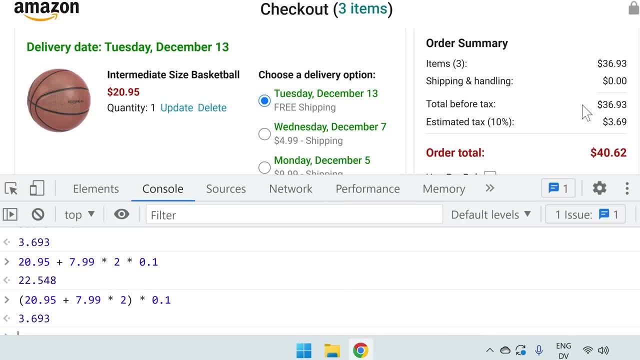 to calculate the numbers in this section of the final project. So don't worry, you don't have to be good at math to learn JavaScript. This is just to show you how math works in JavaScript. In the rest of this lesson we're going to learn some more details about numbers and math. 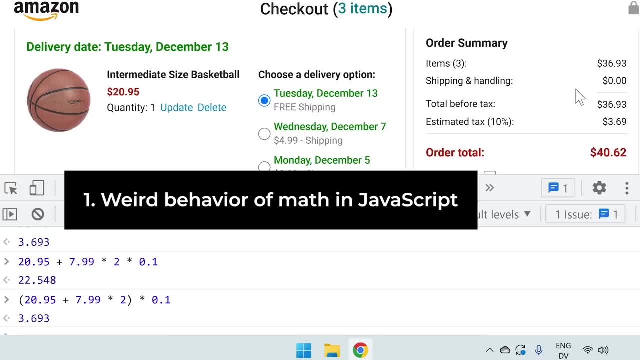 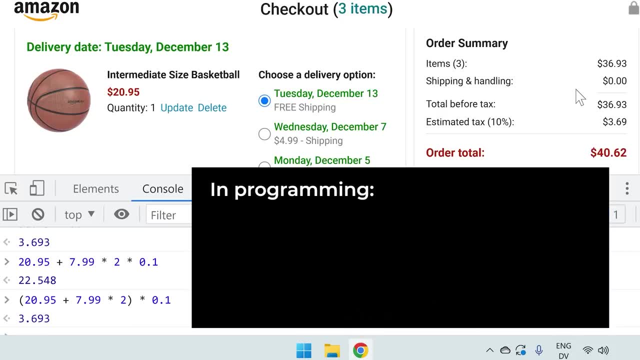 The first detail we're going to learn is a weird behavior of math in JavaScript. First we'll need to learn some terminology In programming. whole numbers like 2, 3, and 4 are called integers. Decimal numbers like 2.2 and 2.5. 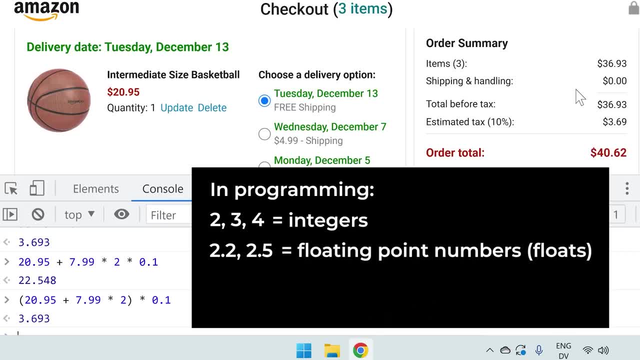 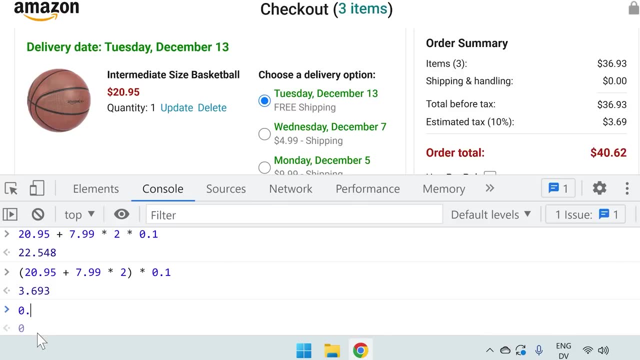 are called floating point numbers or floats, And unfortunately computers have a problem working with floats. For example, if we go back to our console and type the calculation 0.1 plus 0.2 and press enter, it will give us this weird number here. 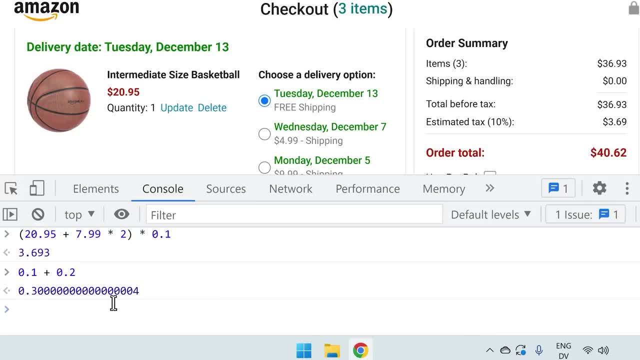 That's close to 0.3, but a little bit inaccurate. So this problem is not specific to JavaScript. Many programming languages also have this problem. The reason this happens is because of how computers store numbers. I'll give a simplified explanation. 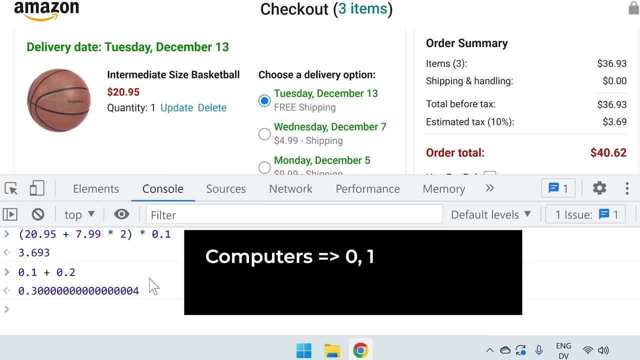 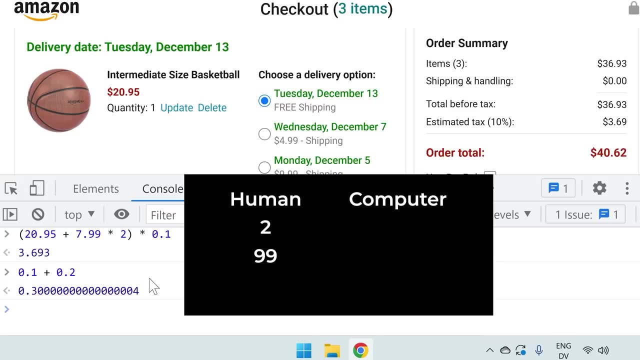 Computers can only store 0s and 1s, while humans can count from 0 to 9. So there's sort of a mismatch between our number systems. For integers this is not a problem. The computer can just use a bunch of 0s and 1s to store it. 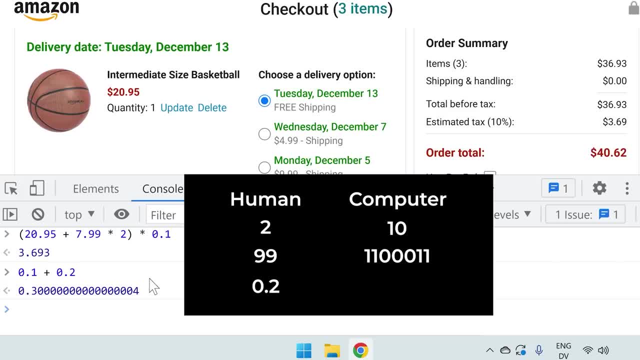 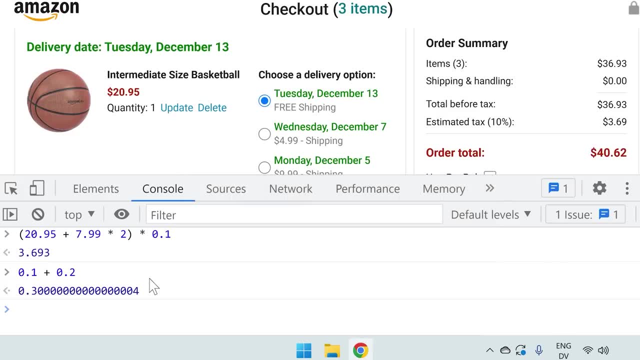 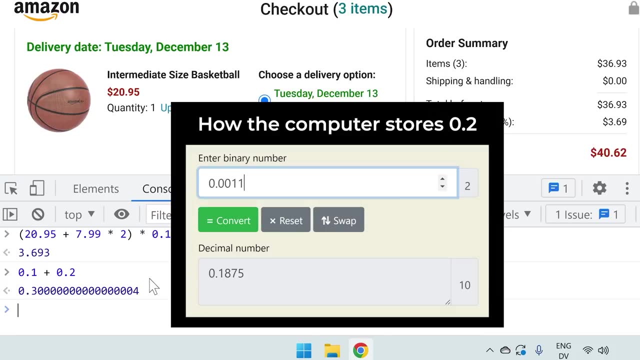 However, for decimal numbers or floats, sometimes the computer can't store the number properly. For example, here's how the computer tries to store 0.2 using only 0s and 1s At the top is what the computer stores. 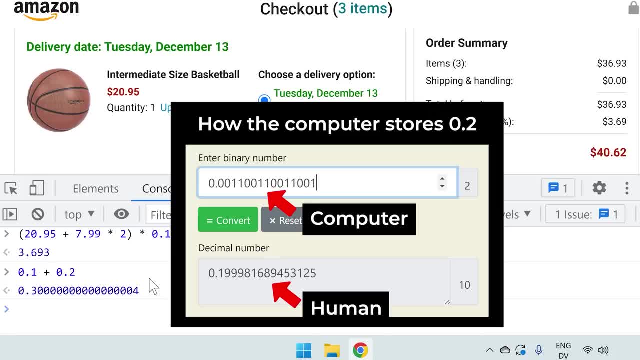 At the bottom is what this is equal to in human numbers. We can see that the computer gets closer and closer to 0.2, but never actually reaches it. And this is why we get these inaccuracies when calculating with floats, Because computers can't store some floats properly. 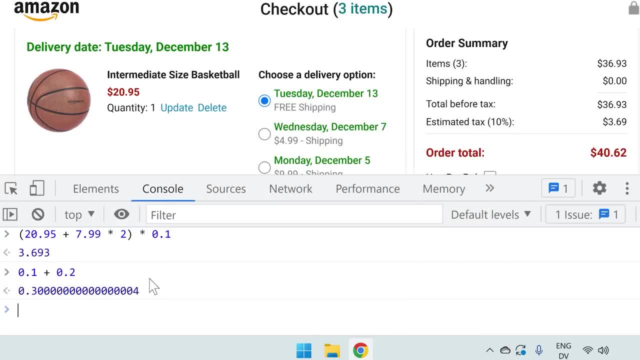 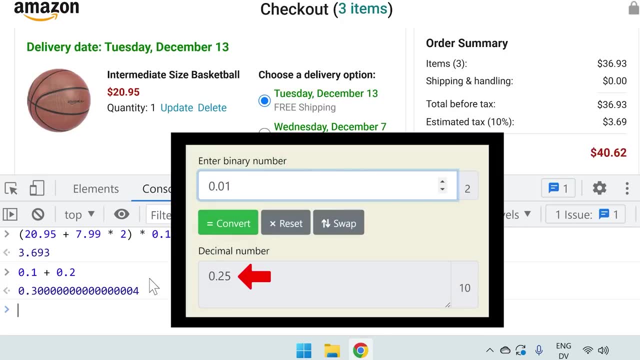 Note that this doesn't happen with all floats. For example, computers can store 0.25 without any problems, So these inaccuracies only happen with some floats, but not all of them. However, when calculating money, we definitely want to avoid any inaccuracies. 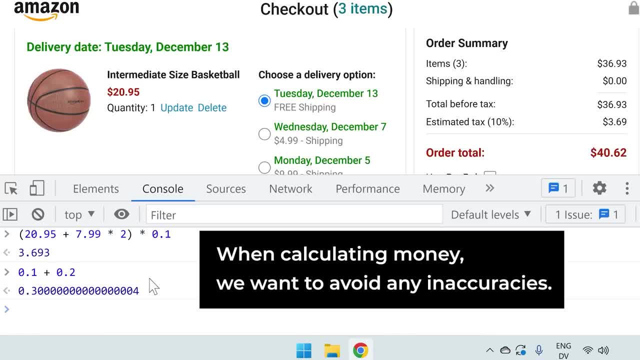 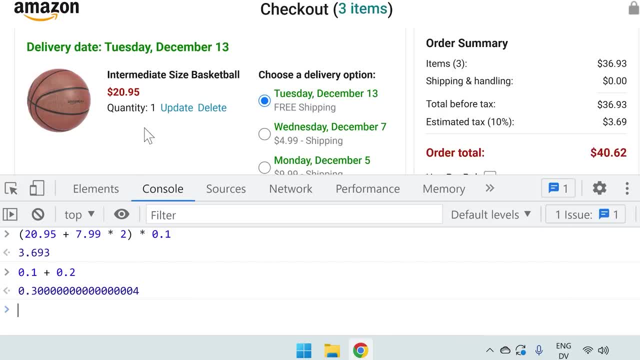 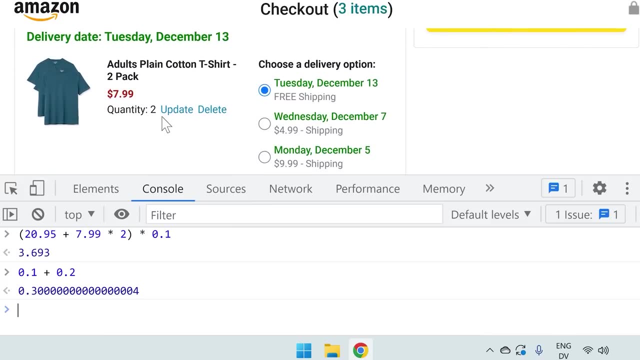 So let's learn how to do that. First, we're going to set up our cart again, So make sure in your cart you have one basketball with free shipping, and this time you have one t-shirt. So we're going to click update. 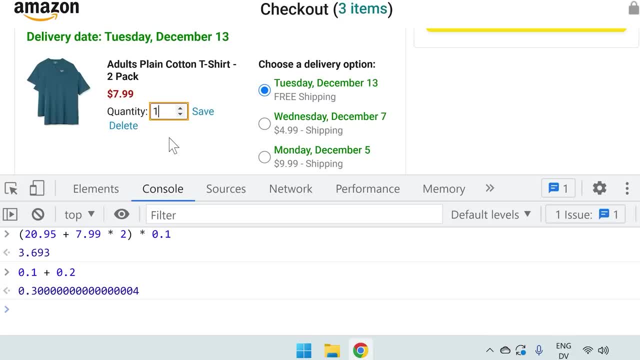 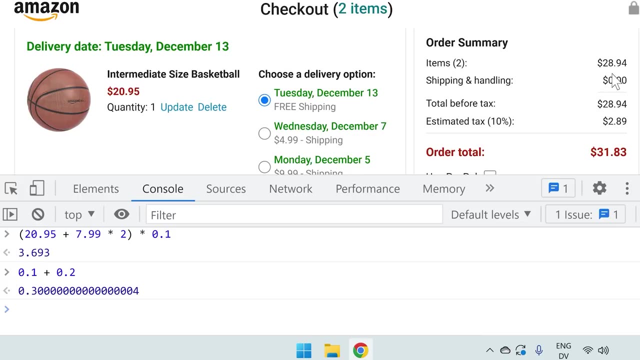 change this to 1, and click save. And this t-shirt also has free shipping. Now let's scroll up and we're going to calculate this number at the top again, which is the cost of the products. Let's go into our console. 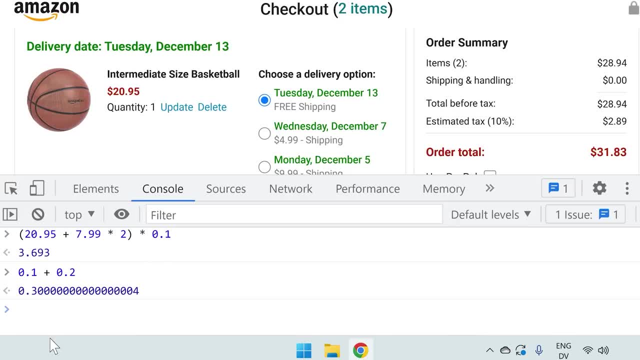 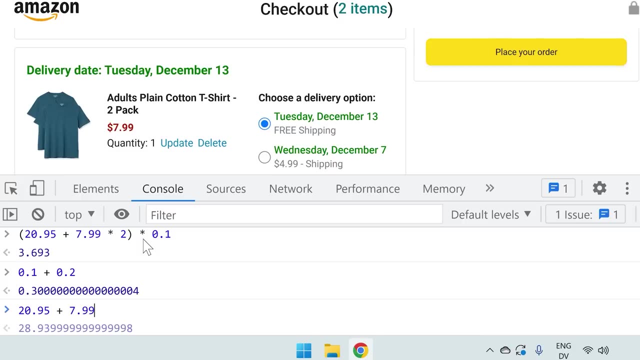 and we're going to add the cost of the basketball- $20.95, plus the cost of the t-shirt, which is $7.99.. If we press enter, calculating with these floats causes the inaccuracies that we saw earlier. So how do we avoid this problem? 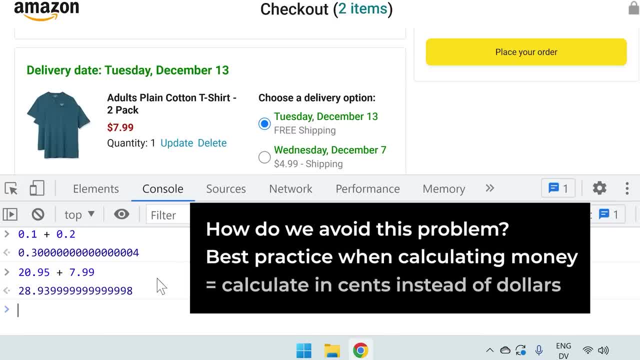 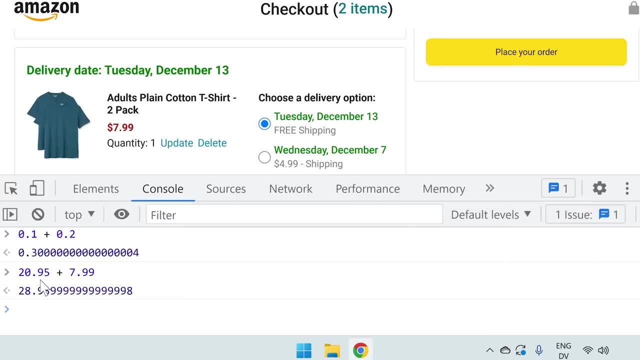 The best practice when calculating money is to calculate in cents instead of dollars. So instead of $20.95, we're going to calculate $2,095, plus $7.99.. Notice, we're not using floats anymore, so we avoid the inaccuracies. 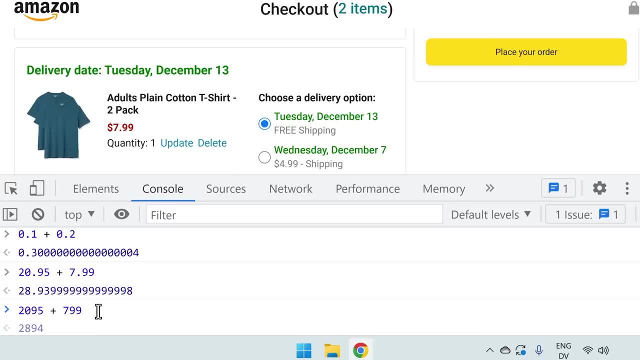 But now this number is in cents, so we need to convert back to dollars. To do that, we'll surround this calculation with brackets to make sure we calculate this first, and then at the end we'll divide by 100, to convert back to dollars. 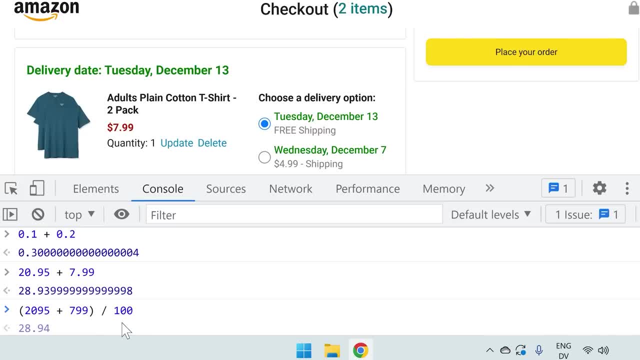 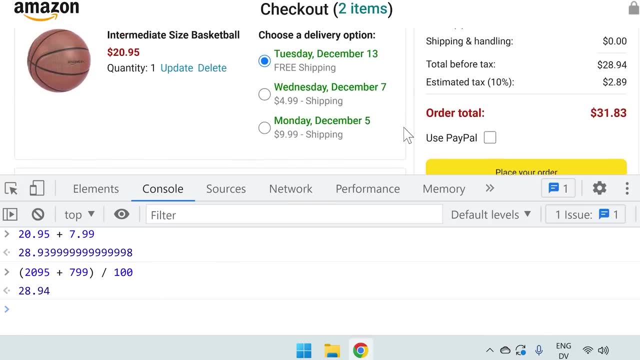 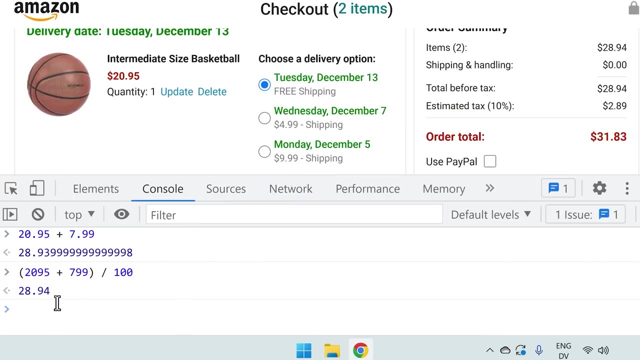 because there are 100 cents in each dollar. If we press enter and scroll up, that's how we get the exact number that we see on the page. So remember, in programming, calculations with floats are sometimes inaccurate and when working with money, 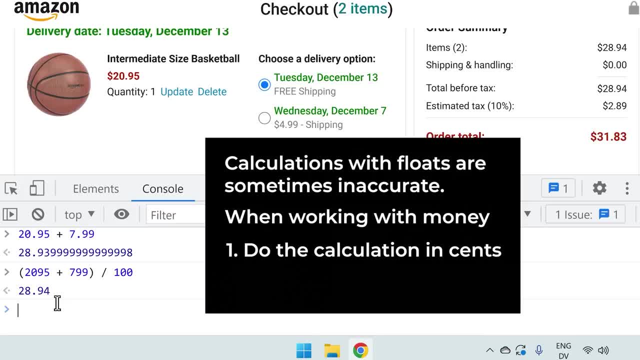 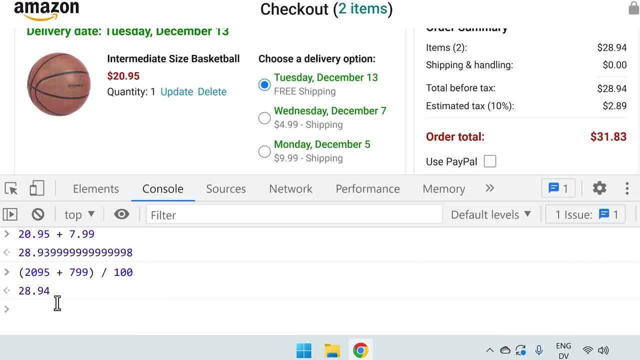 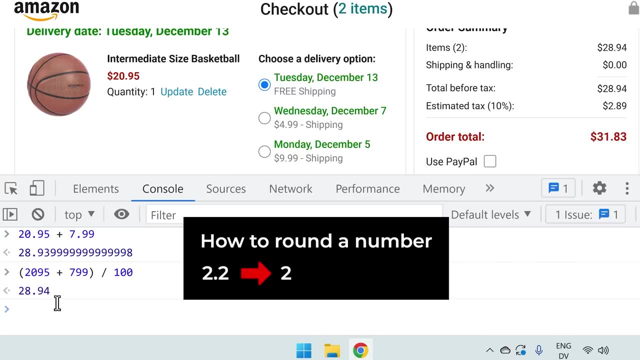 the best practice is to do the calculation in cents and then convert back to dollars at the end. The next detail we're going to learn is how to round a number in JavaScript. Rounding just means taking a number and moving it to the nearest integer. 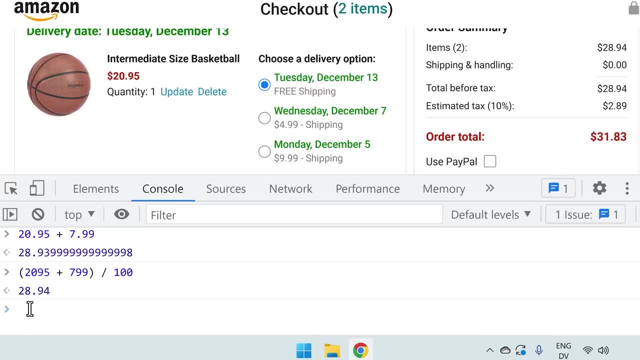 To round a number, we can use this code: capital M, math dot round. open bracket. close bracket. So make sure you use a capital M, because JavaScript is case sensitive. Now, between the brackets, we can put a number that we want to round. 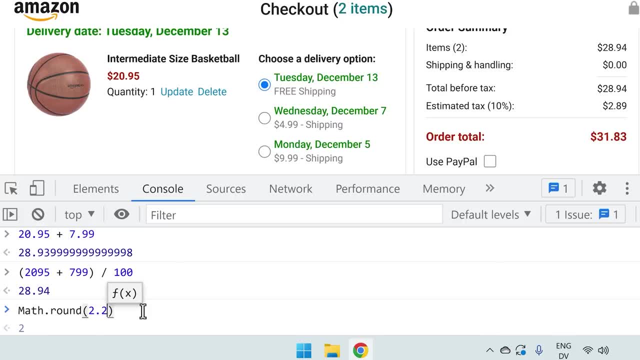 like 2.2.. If we press enter, it will round this number down to 2.. If we do capital M math dot round, open bracket, close bracket and between the brackets we put 2.8 and press enter, it will round. 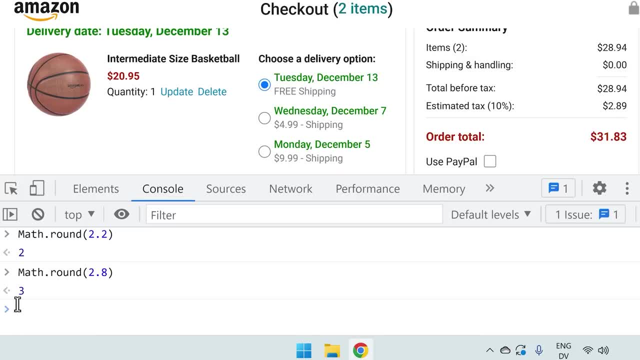 2.8 up to 3.. Now let's do a practical example with math dot round. We're going to calculate the tax again, But this time we're going to round the result to exactly this number on the page. So first, 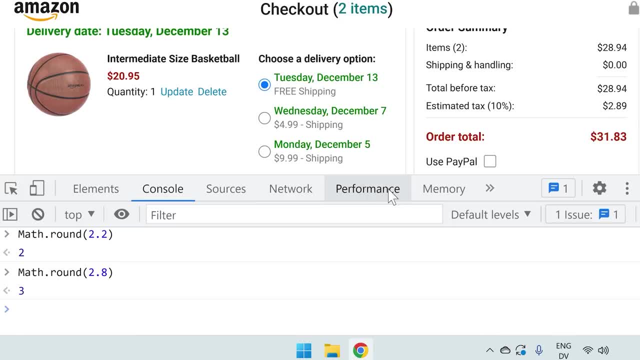 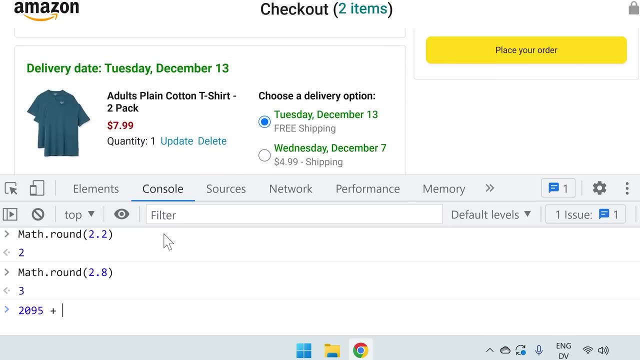 let's calculate the tax. We'll go into our console and add the cost of the products in cents, so 2,095 cents for the basketball and plus the cost of the t-shirt, which is 7.99 cents, and we'll surround this. 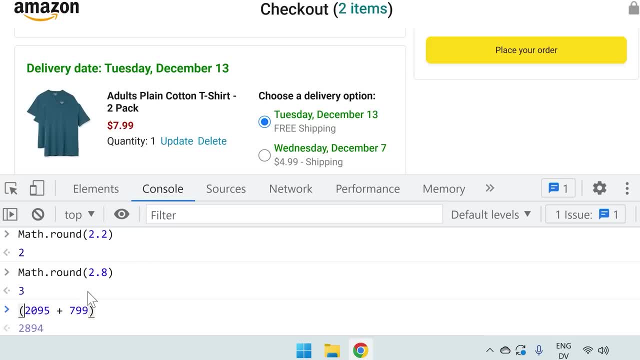 in brackets, To make sure. we calculate this first, And then we're going to multiply this by the tax percent, or 0.1. And finally we'll convert this back to dollars. So let's surround this in brackets as well. 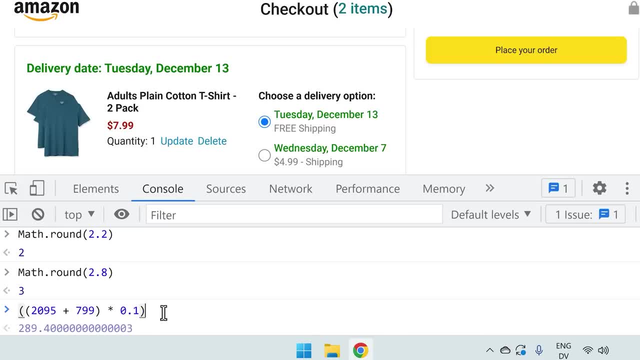 to make sure, we calculate this first and at the end we'll divide by 100 to convert back to dollars. So notice, here we can have brackets inside brackets. In this situation, JavaScript will calculate the inner brackets first and then the outer brackets. 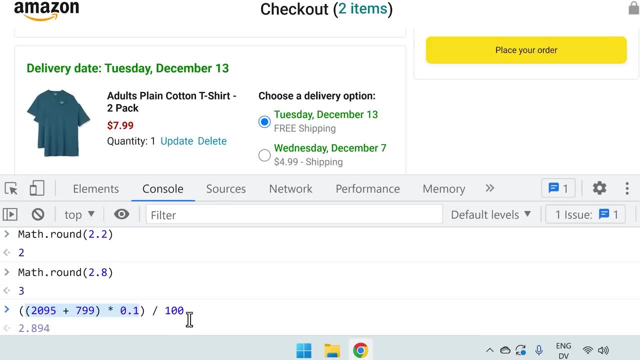 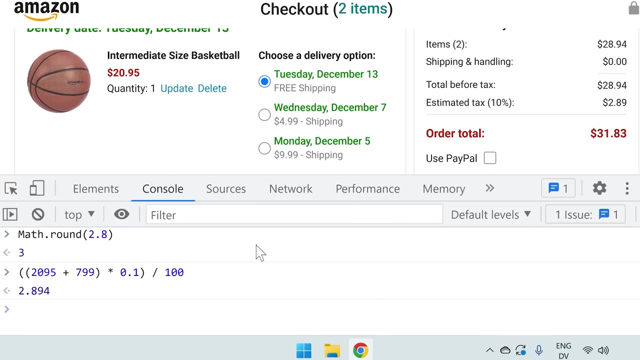 and then everything else. If we press enter, this gives us 2.894, which is close to the number on the page. It's the same amount of money, but our number is more accurate than we need. So now let's learn how to use. 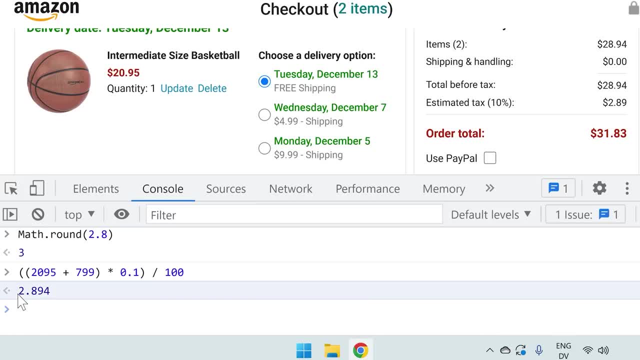 mathround to round this number to exactly 2.89.. First let's create a copy of this calculation, So we'll select it, right click, copy and down here right click and paste. So one thing we might try to do. 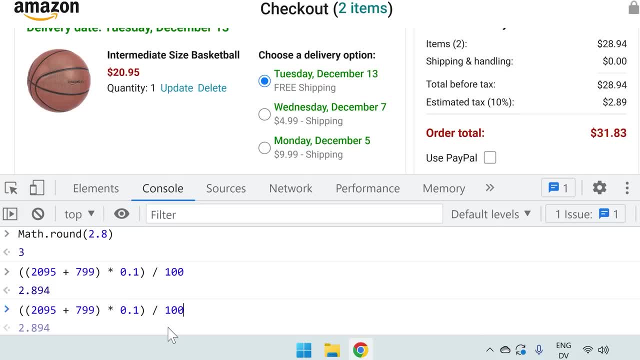 is to round this entire calculation. However, this will round 2.894 to 3, because it rounds to the nearest integer. Instead, what we want to round is this number here, So remember that this number is the result in cents. 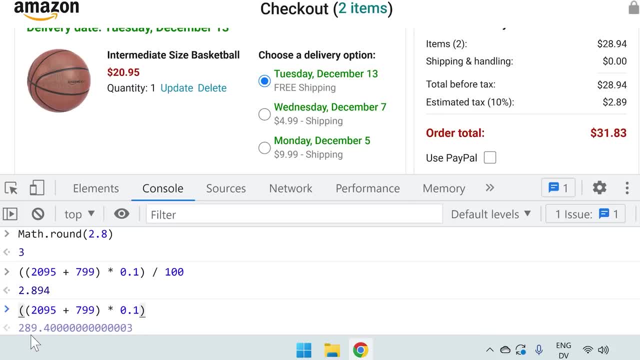 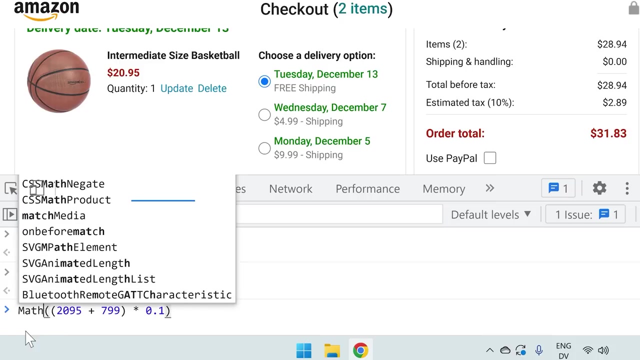 which is 289.4.. If we round this number, it will round down to 289 cents, which is exactly $2.89.. So to round this calculation, at the front we'll type capital, M, math dot round. So we already have. 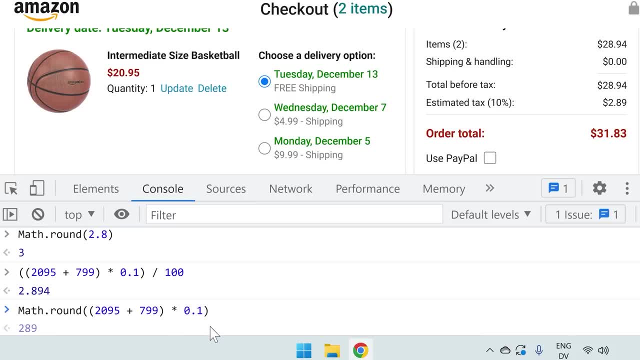 brackets around this, so we don't need extra brackets. So this will round to 289 cents And finally we'll convert this back to dollars at the end by dividing by 100.. If we press enter, that's how we round. 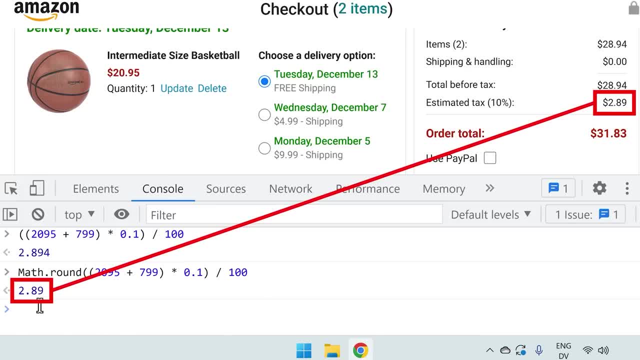 this calculation to get the exact number on the page. So to summarize, we first calculate the result in cents and then we round this to the nearest cent and then at the end we convert back to dollars. Again, don't worry, you don't have to be good. 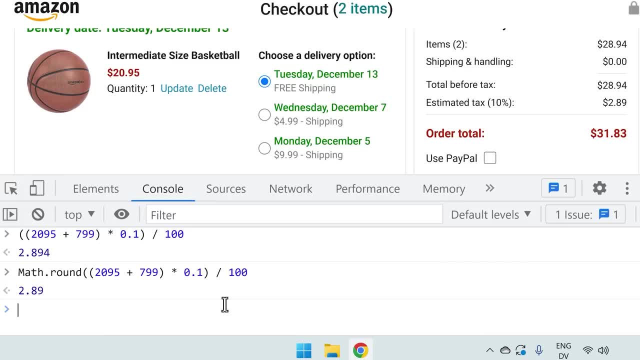 at math to learn JavaScript. These examples are just for learning. Almost all the math we do in JavaScript is more simple than this. I'll give you some exercises at the end of this lesson to help you get more practice. The last thing we're gonna. 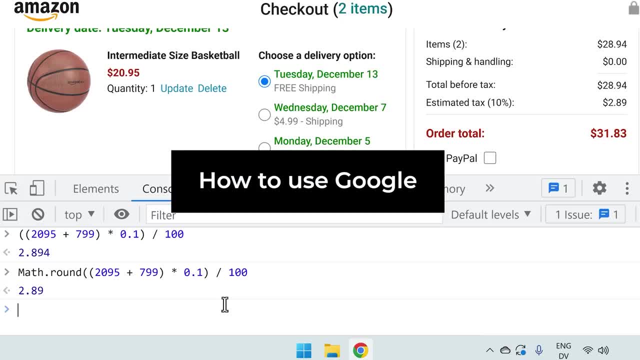 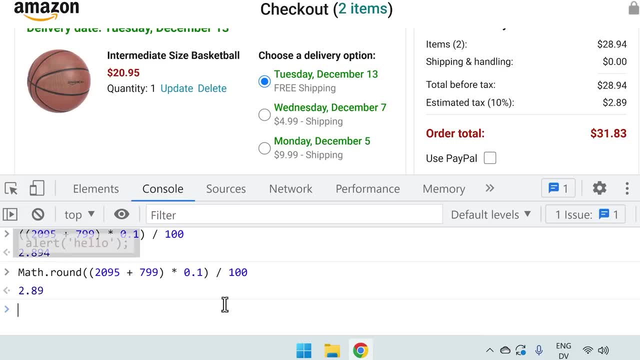 learn in this lesson is how to use Google when you're learning to code. So far, I've been giving you different pieces of code, like alert and mathround. You might be wondering: where do I find this code, These pieces of code? 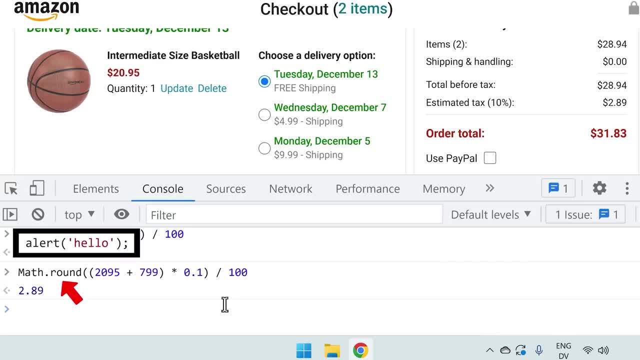 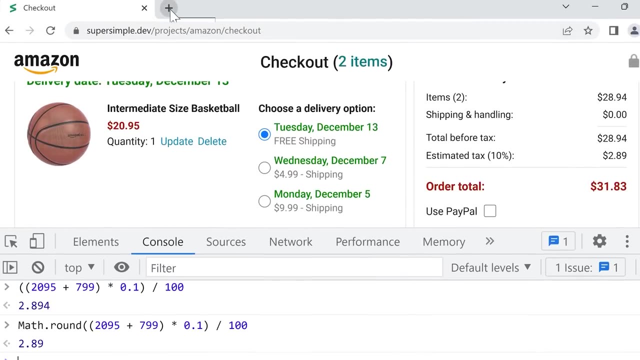 are features of JavaScript And I find this code by searching on Google. So we're gonna learn how to use Google to learn new features of JavaScript on our own. Let's go to our browser and create a new tab at the top, And we'll click here. 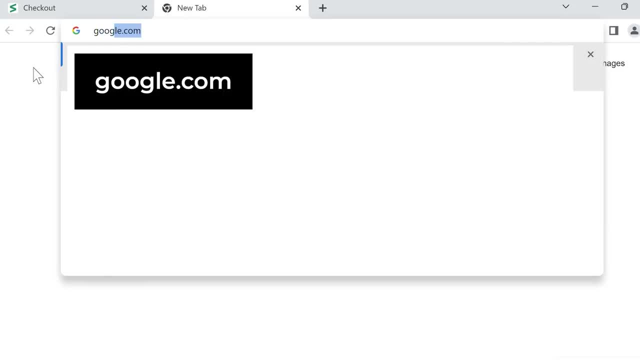 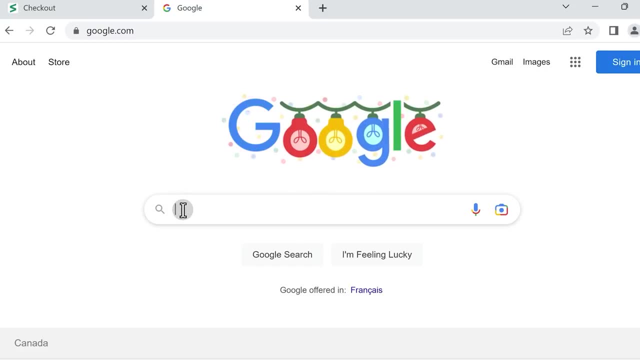 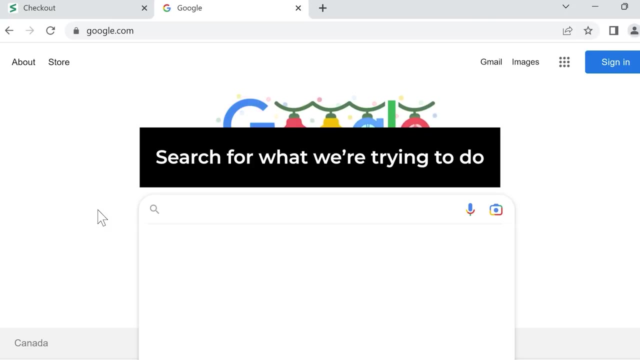 and type google dot com and press enter And we'll search in Google. So the trick to searching in Google is to search for what we are trying to do. For example, if we want to round a number, we would search for JavaScript: how to. 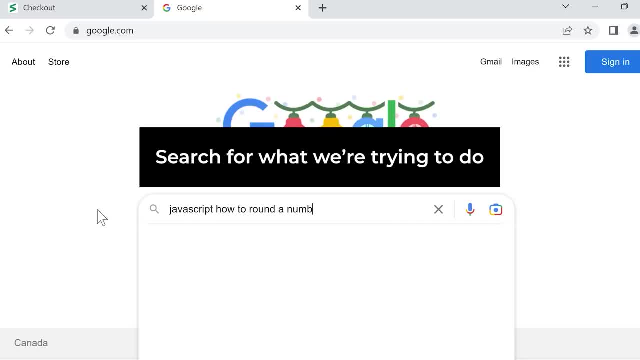 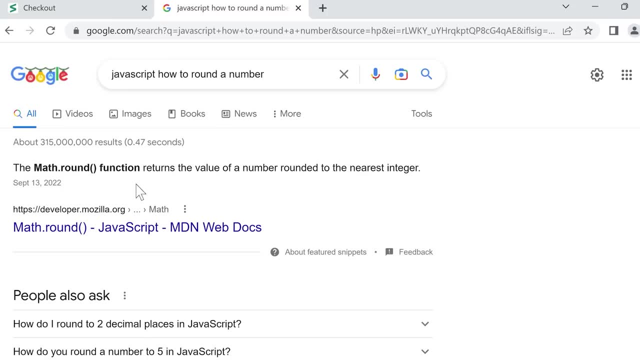 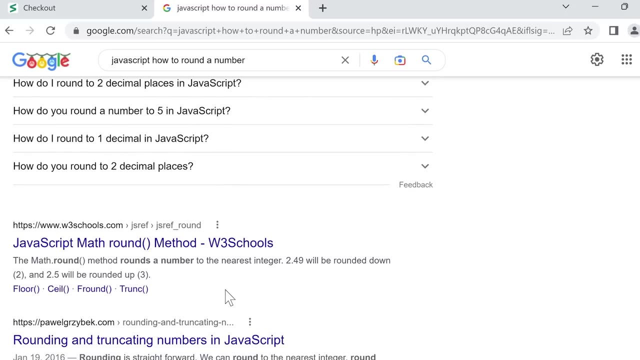 round a number. If we press enter, sometimes you might get the code right away in the first result and sometimes you might have to go into the other results to find the code that you need. In my example I see the code math dot round in the first result. 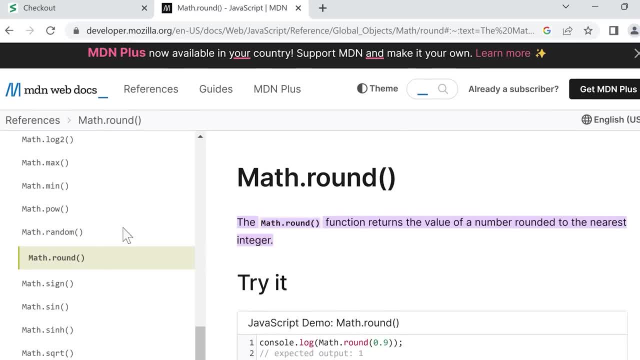 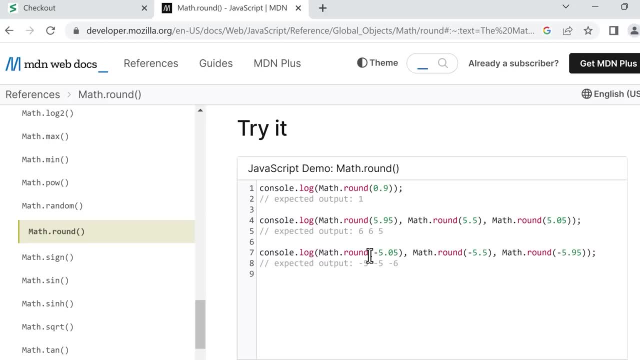 so I can click into this result, read about what this code does and also see some examples of how to use it. One thing to keep in mind is that when you're searching in Google, you might not understand all the code that you get in your 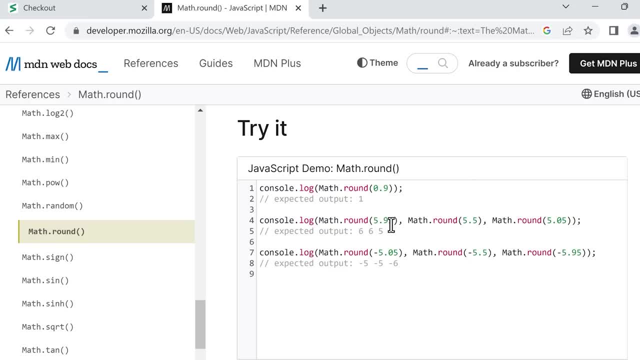 results. For example, here there's a lot of code that we haven't learned yet, And actually that's okay. We just need to look for the pieces of code that look familiar to us, like this part of the code We can then use. 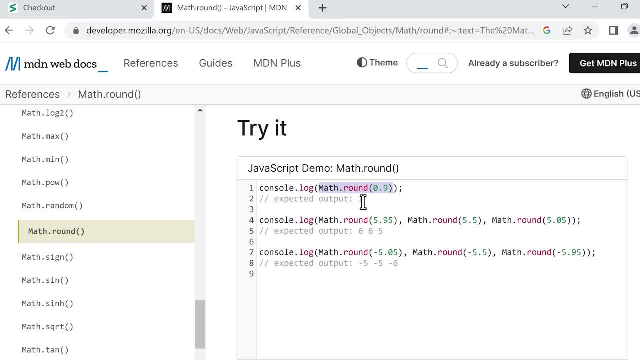 this part of the code in our own code. We don't have to understand every bit of code that we get from Google And, don't worry, as we move through this course, we will understand more and more of this code that we get from Google results. 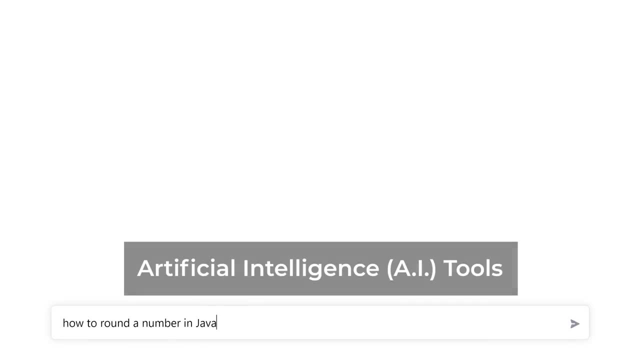 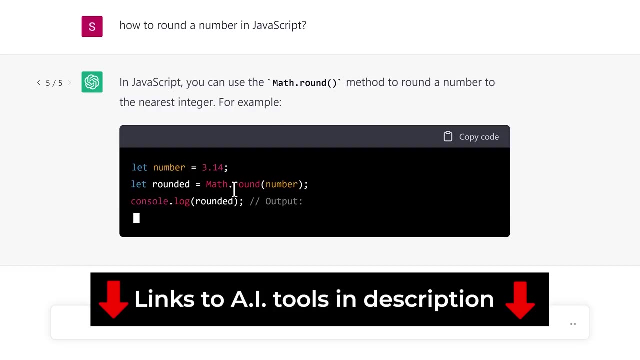 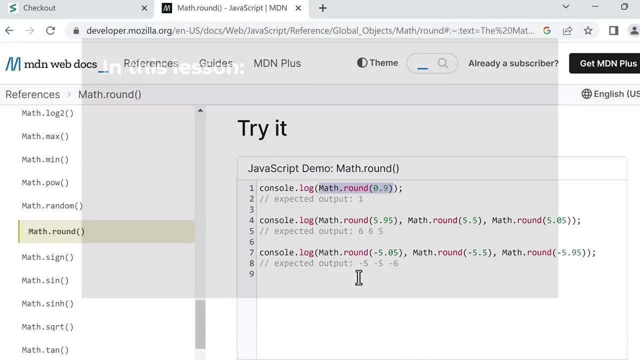 These days, we also have some artificial intelligence or AI tools that can help us search for code. I'll provide links to some of these tools in the video description, And that's the end of this lesson. In this lesson, we learned how to work. 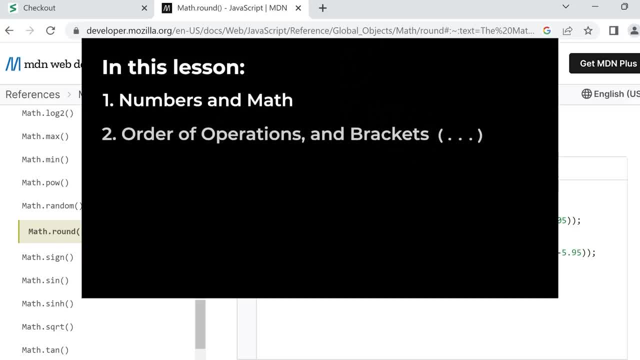 with numbers and math. We learned the order of operations and brackets. We calculated the numbers in the final Amazon project. We learned that calculations using floats can be inaccurate and how to avoid this problem. when working with money, We learned how to round numbers. 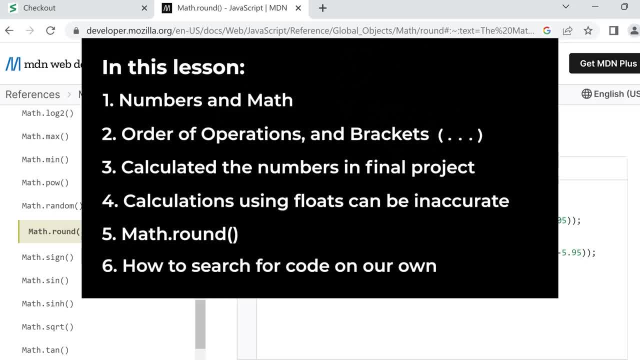 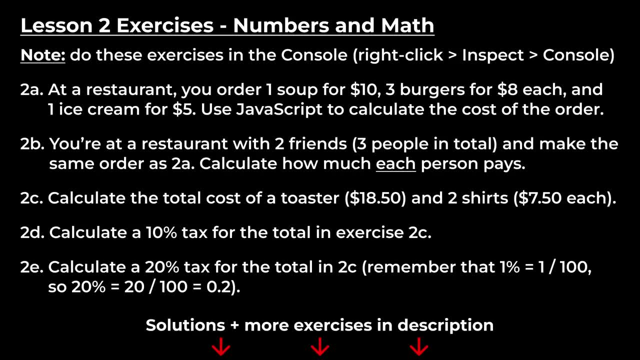 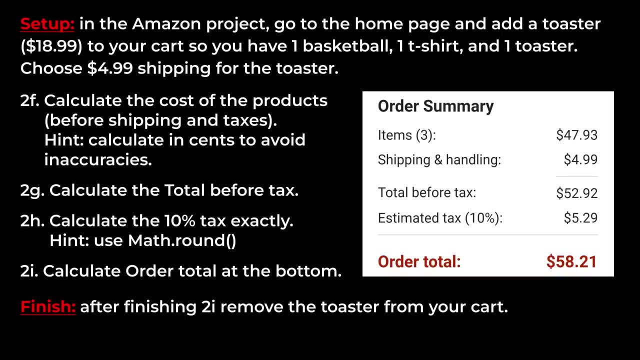 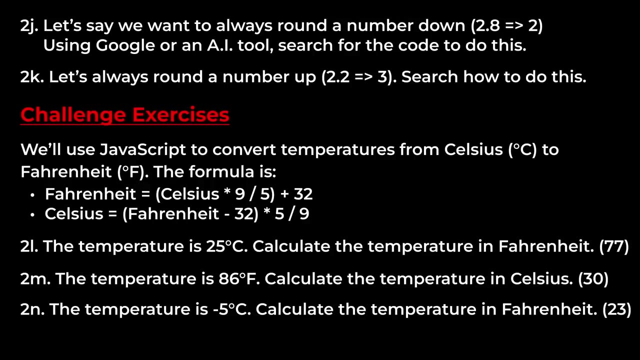 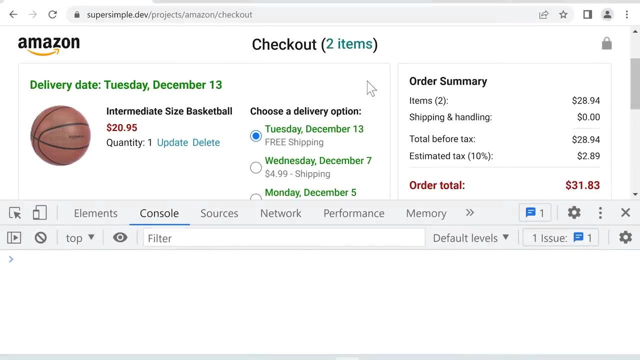 using mathround And we learned how to search for code on our own. Here are some exercises to help you practice numbers and math. In the previous lesson we learned how to work with numbers and math. In this lesson we're going to learn 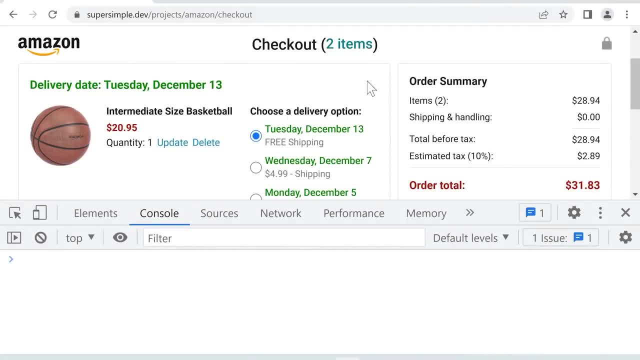 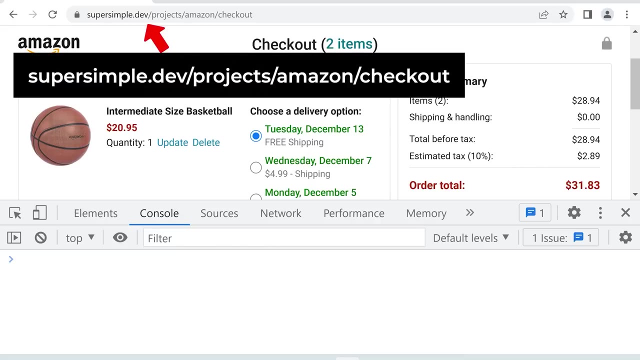 how to work with text And we're going to create the text in this section of the final project. First, make sure you have the final project open and you're on the checkout page. Also, make sure you have your console open on this page. 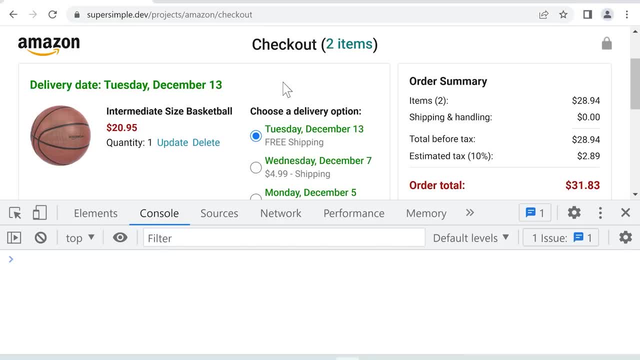 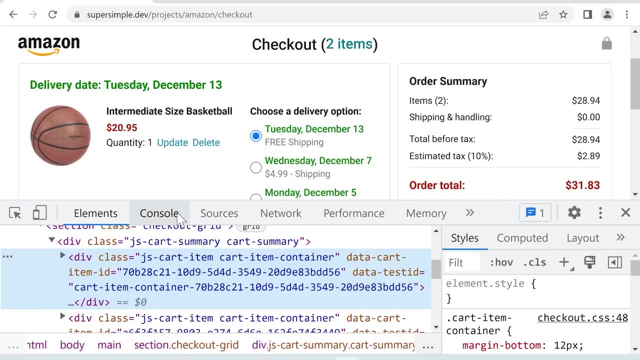 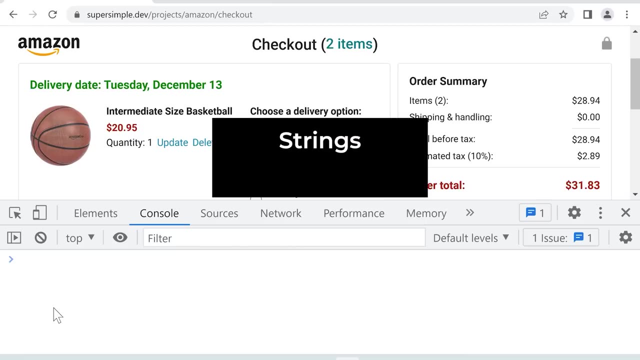 If not, you can go to a blank area, right-click, click, inspect and then click the console. Now we're going to learn a feature of JavaScript called strings. A string represents text. Let's go to our console and create our first string. 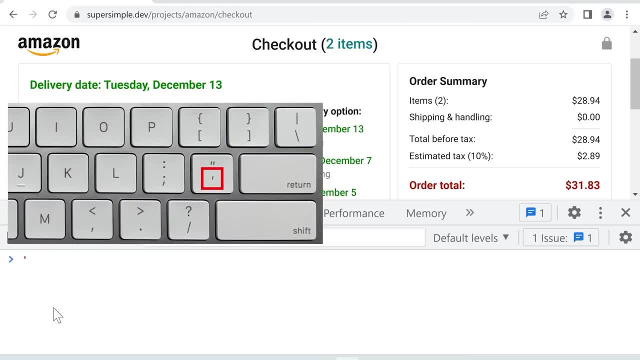 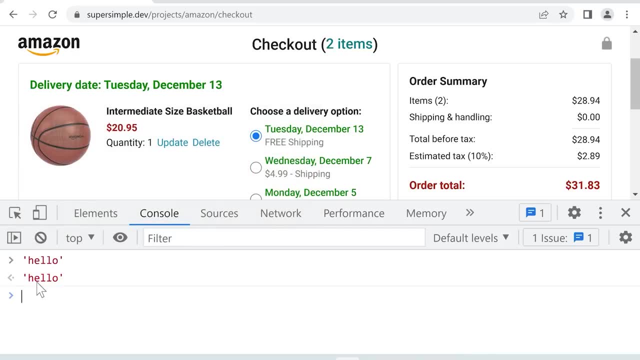 We're going to type single quote hello and single quote and press enter. This is a string and it represents the text hello. And we've actually seen this code before. In the first lesson, the first piece of code that we learned was: 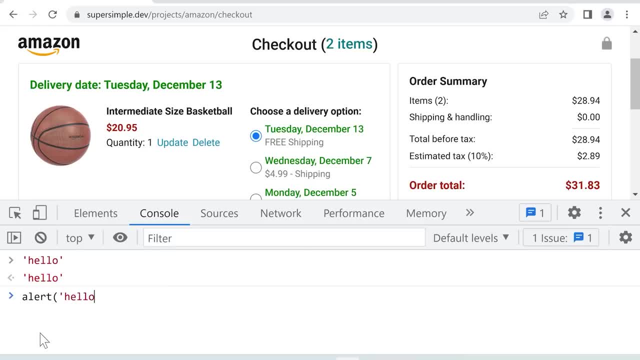 alert. open bracket. single quote: hello. single quote. bracket and semicolon. This code creates a pop-up on the page. If we press enter, it creates a pop-up. Now, inside these brackets, we actually created a string. 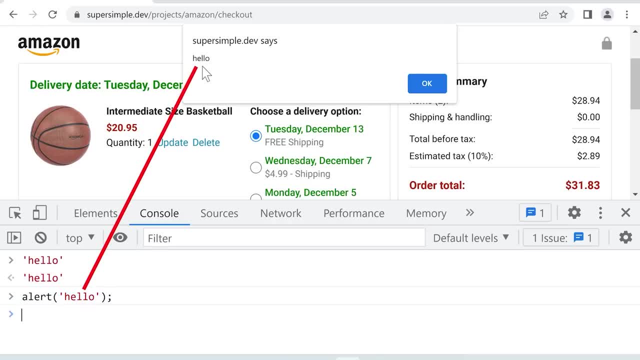 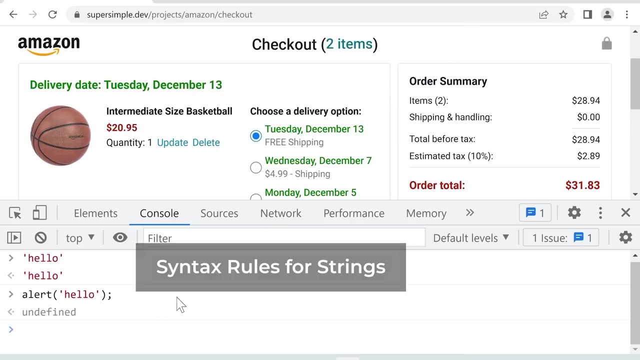 This string is the text that appears in the pop-up. So, as you can see, a string represents text. Let's press ok and now let's learn the syntax rules for strings. To create a string, we just write some text. 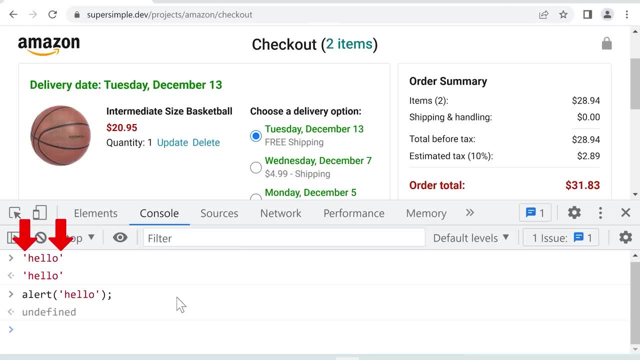 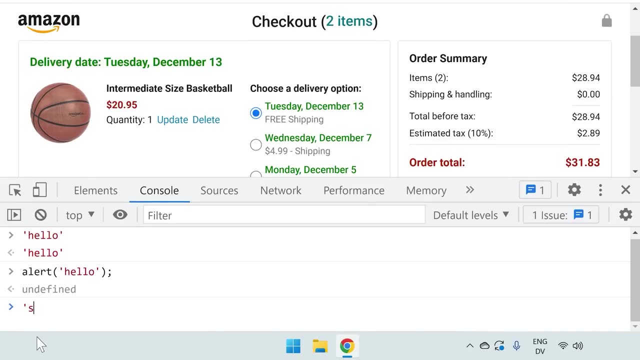 like hello, and then surround this text with single quotes, One at the beginning and one at the end. We can also add strings together. For example, let's type the string sum plus the string text And press enter When we add two. 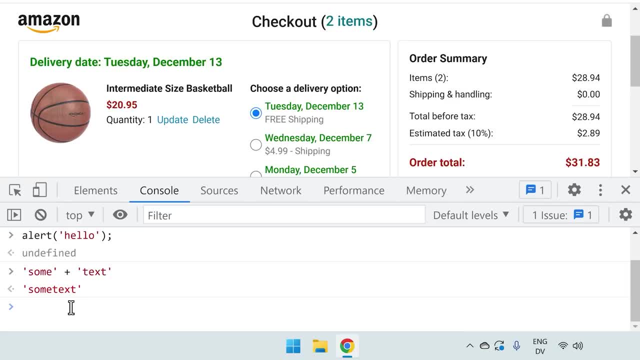 strings. it combines the strings together into a bigger string And this makes sense. We're adding two pieces of text together. We can also add more than two strings at a time. For example, we can type the string sum plus the string more. 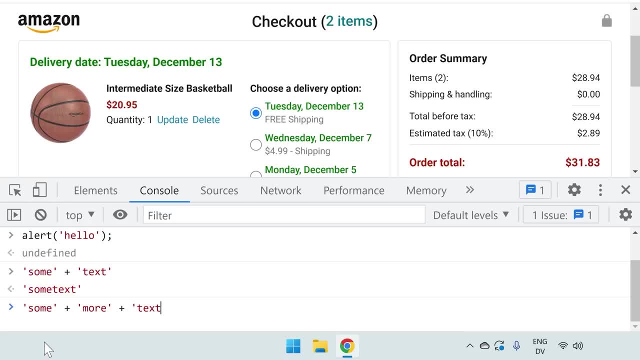 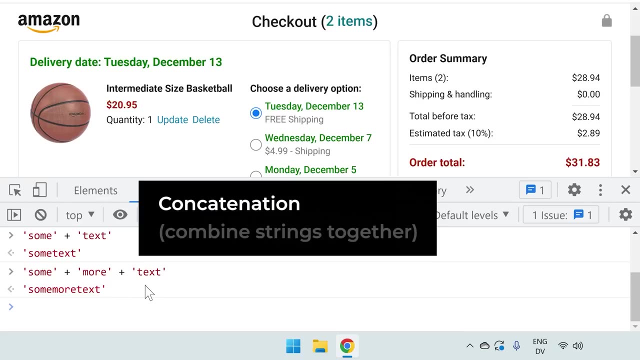 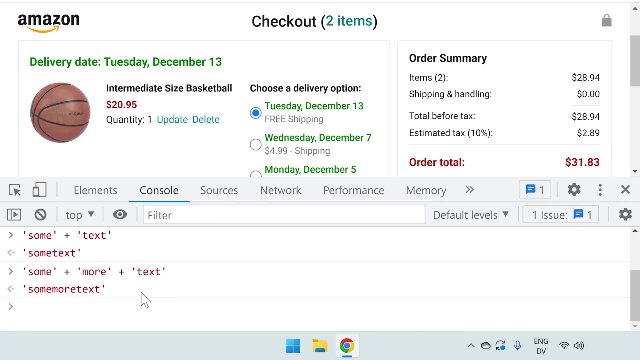 plus the string text. If we press enter, the computer will combine all three strings into one big string. By the way, this is called concatenation, when we combine strings together. Now, in the previous lesson we learned about numbers, Numbers and 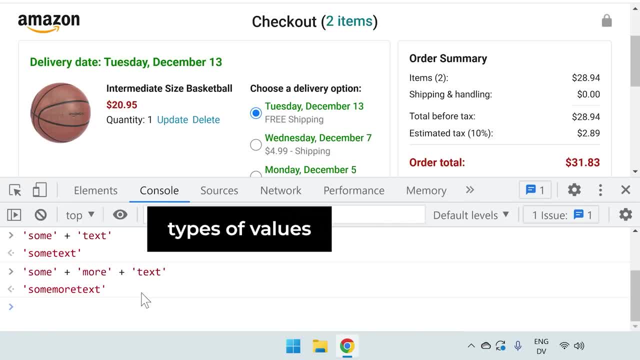 strings are two different types of values in JavaScript. They represent different things And we can actually check what type of value something is using this code: type of, and then space, and then a value like the number two. If we press enter, type of will tell us that 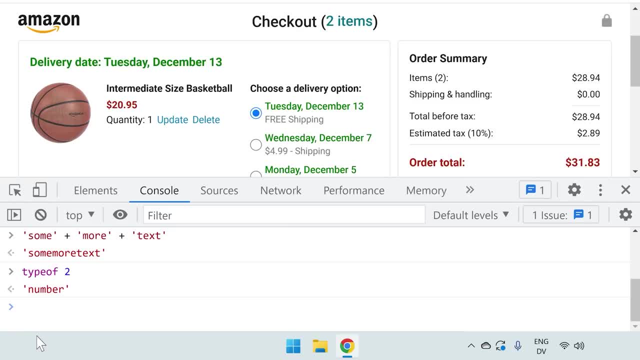 two is a number. If we do type of quote hello quote- and press enter, it will tell us that hello is a string. Now what if we added a string and a number together? For example, let's type the string hello plus the number three. 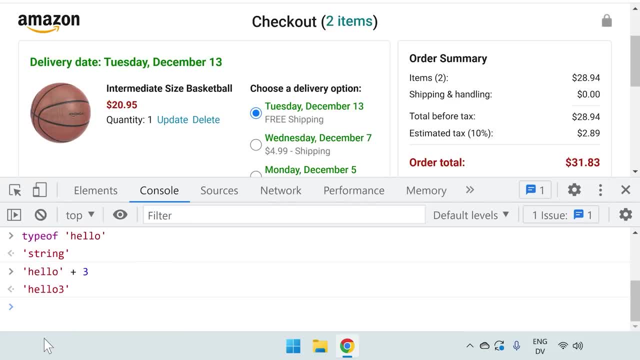 and press enter. So when we add a string and a number, JavaScript will automatically convert this number into a string. So this gets converted into the string hello plus the string three, And then it combines them together into the string hello three. This feature. 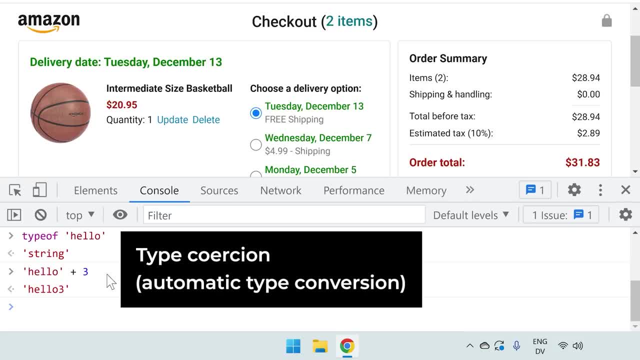 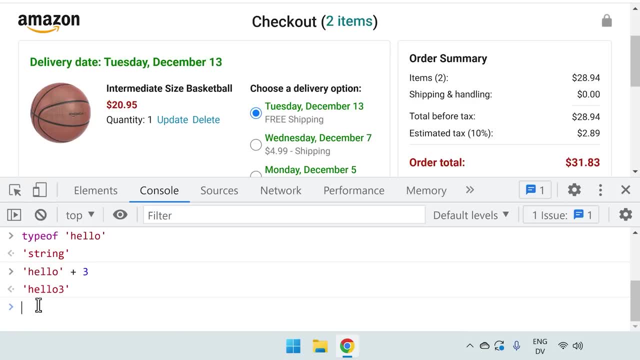 is called type coercion or automatic type conversion. Okay, now that we understand the basics of strings, let's do some practical examples. We're going to use strings and numbers to create the text in this section of the project. First, make sure that in your cart you 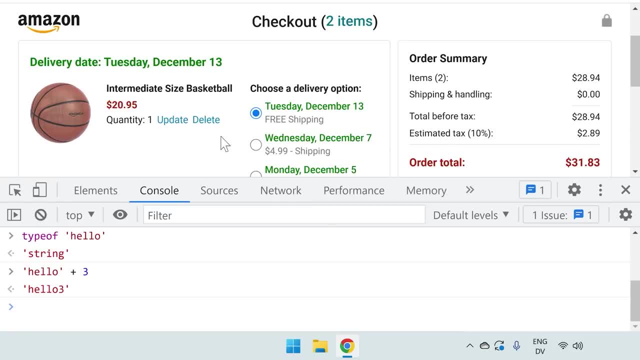 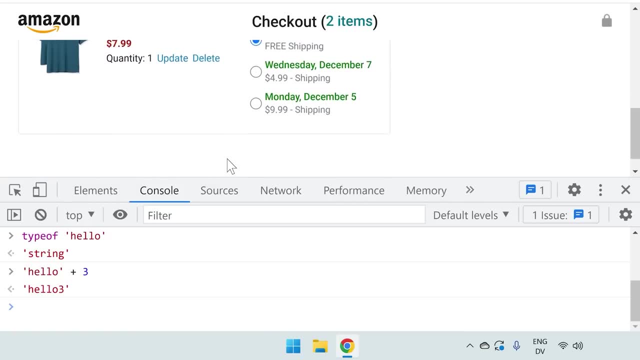 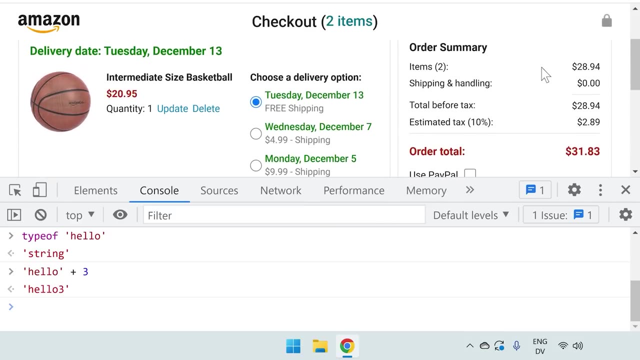 have one basketball with free shipping and you have one t-shirt, also with free shipping, And you have no other products. Let's scroll up and we'll start by creating this text in the top right. So this is the cost of the products, but this time. 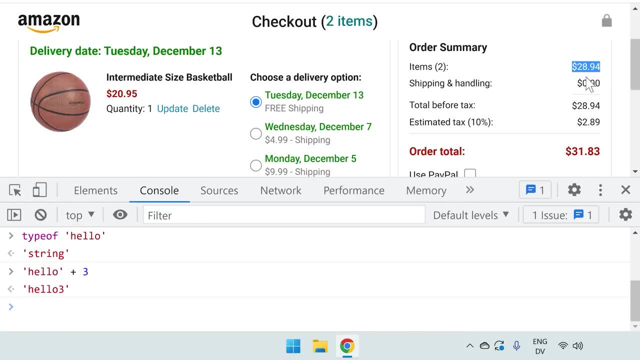 we're going to have a dollar sign, So instead of just a number, this will be text. So one thing we can do to create this text is just type out the string directly like: quote dollar twenty-eight, point nine four, and quote However. 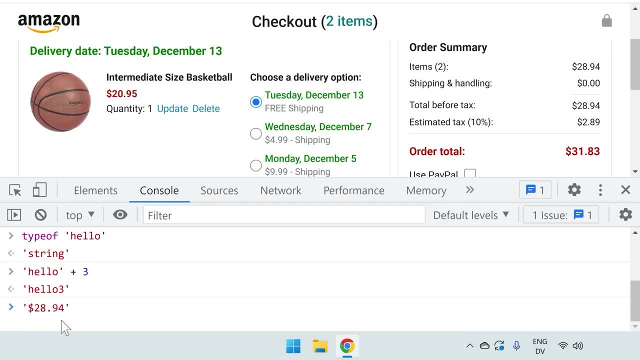 let's actually calculate this number using math. Remember, the advantage of JavaScript is that it's able to do calculations. So instead of typing out twenty-eight point nine four, we're just going to create the string dollar sign plus and we're going to calculate. 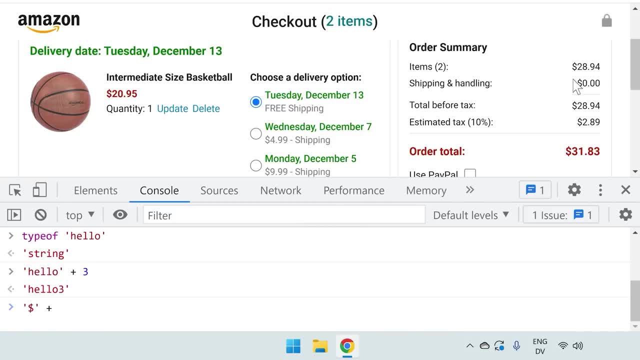 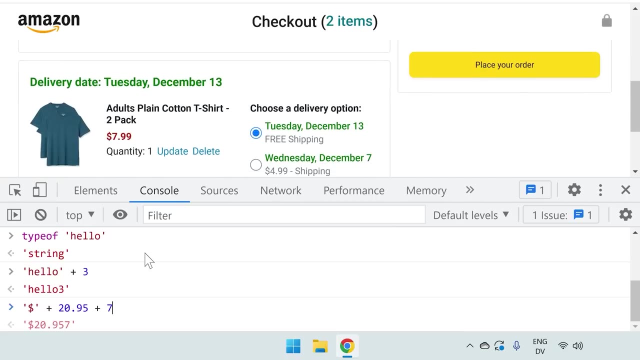 this number using math. So we're going to add the cost of the basketball, which is twenty dollars and ninety-five cents, plus the cost of the t-shirt, which is seven dollars and ninety-nine cents. If we press enter, unfortunately this doesn't look right. 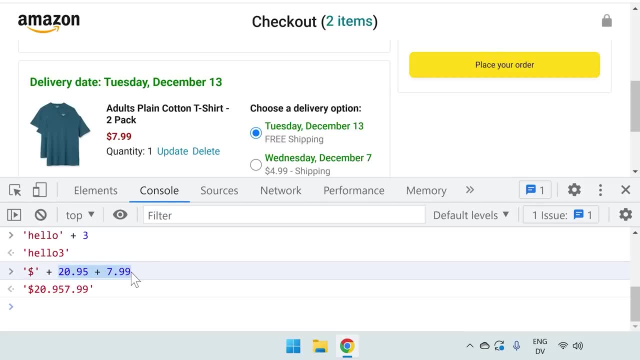 Instead of doing math and adding these two numbers together, it just sort of put the numbers one after another into the string. So why is this happening? JavaScript adds from left to right, So the first step is to add these two values And, as we learned, if we 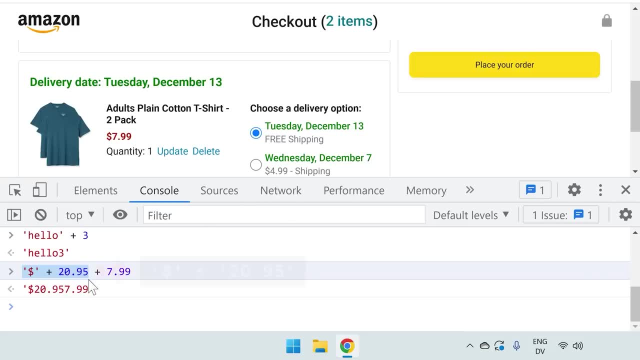 add a string and a number. JavaScript will automatically convert this number into a string, So the result of this calculation will be the string dollar twenty point nine five and quote. The next step is to add seven point nine nine, So it will add seven. 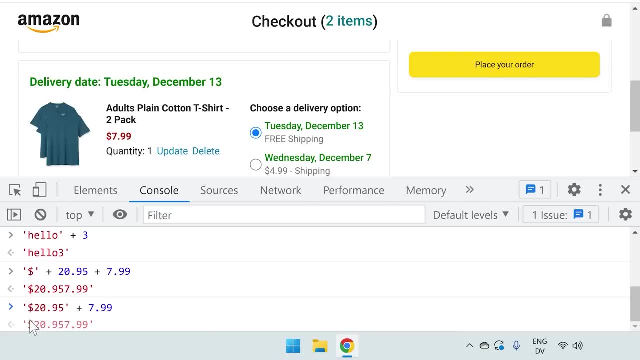 point nine, nine. and now we're adding again a string and a number, So JavaScript will automatically convert this number into a string and combine them together. That's why it puts seven point nine, nine at the end of this string instead of doing math. So what we actually 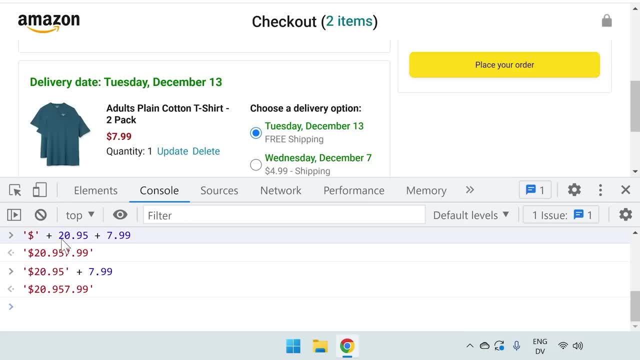 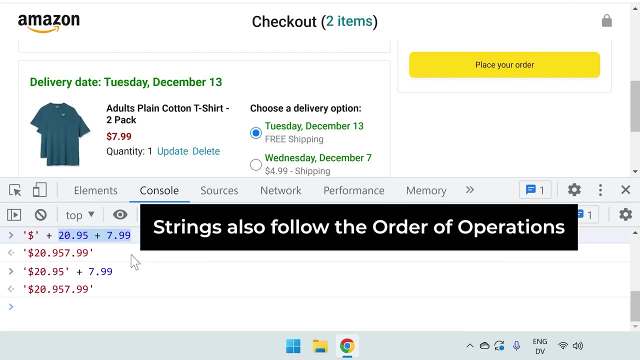 want to do here is to add these two numbers first and then combine the total with the string. So how do we do this? The solution is that strings also follow the order of operations, just like numbers. And remember, in the order of operations we can use brackets. 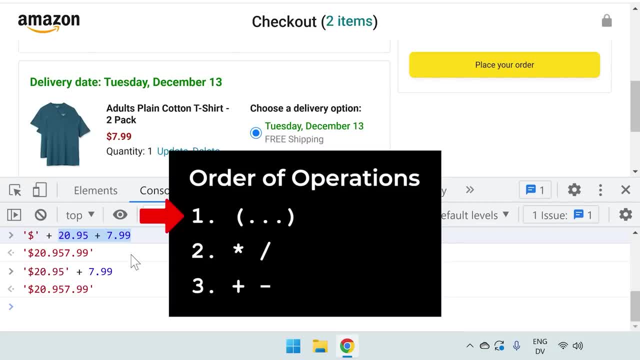 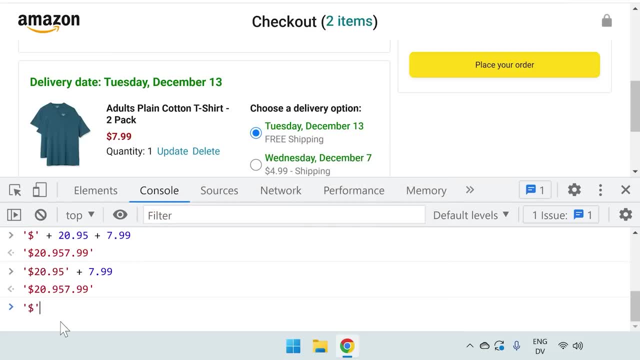 to control which part of a calculation gets done first. So let's type this calculation out again: The string dollar sign plus twenty point nine, five plus seven point nine nine. But this time we're going to add an open bracket and a close bracket around this calculation. 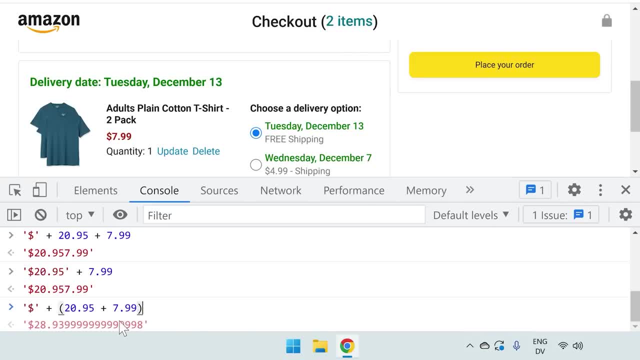 This tells the computer to calculate this number first using math And then combine this result with the string after. If we press enter now, this is doing math and it solves our original problem. Unfortunately, now we have another problem. This math is inaccurate, So remember. 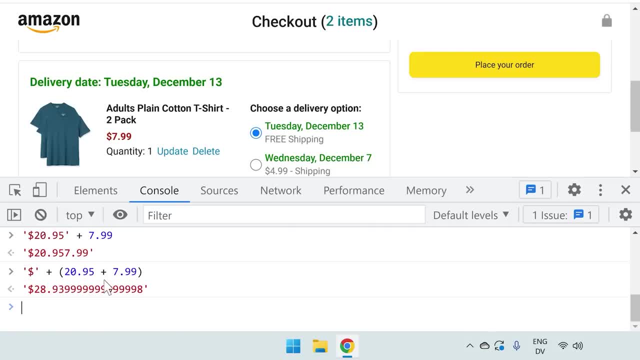 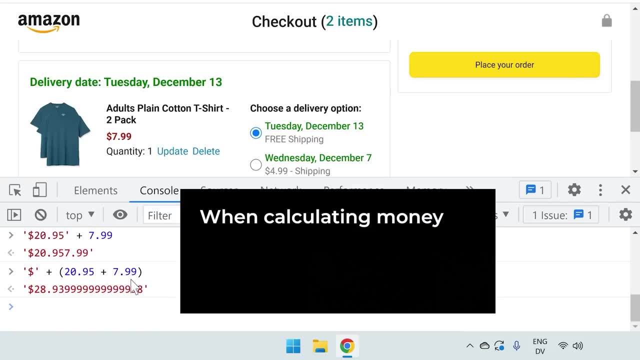 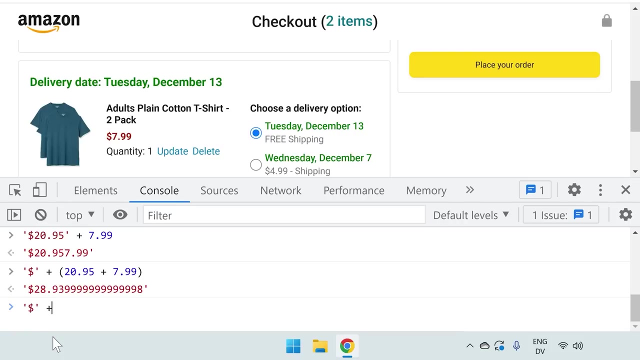 from the previous lesson. doing calculations with floats can sometimes cause inaccuracies, And the best practice when calculating money is always calculate in cents and then convert back to dollars at the end. So at the bottom here we're going to add the string dollar plus open. 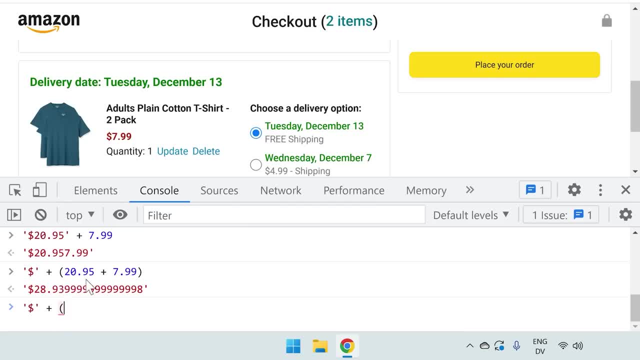 bracket and instead of twenty dollars and ninety five cents we're going to add two thousand ninety five cents plus seven ninety nine cents and close bracket, And then at the end we're going to convert this number back to dollars by dividing by one hundred, If we press enter. 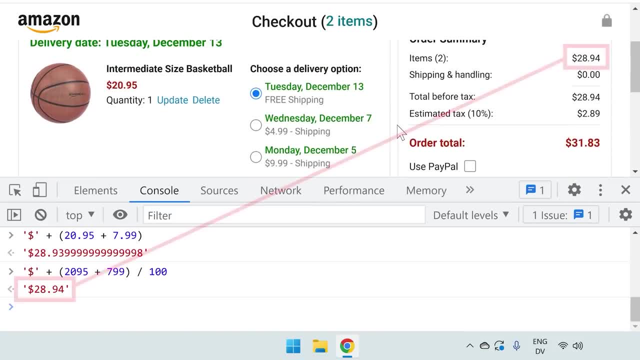 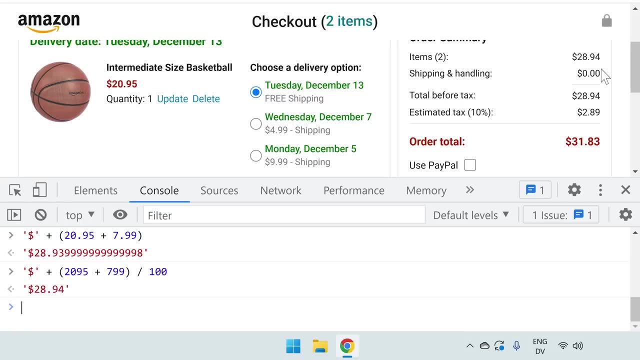 this will give us the text that we see in the final project. Again, strings follow the same order of operations as numbers. Brackets are always calculated first, Multiply and divide are done next and add and subtract are done after, So adding this result. 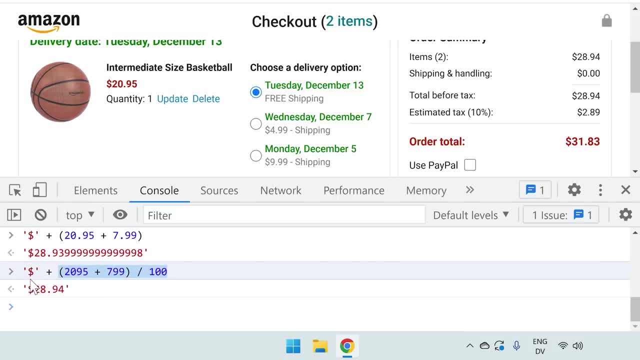 to the string is the last step. Now let's do a more complicated example. Let's use strings and numbers to create this entire line of text, not just the dollar text. To create this, we're going to go from left to right. Let's go back in our console. 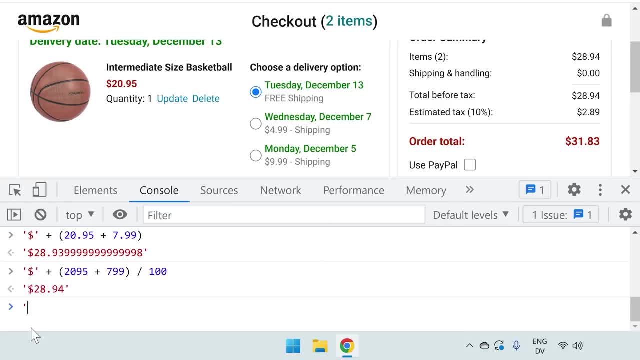 and we're going to start with the string items: open bracket. and here we could just type two and close bracket. but let's actually calculate this number as well, using math. So this number is the quantity, or the number of products in our cart. Let's go back to our console. 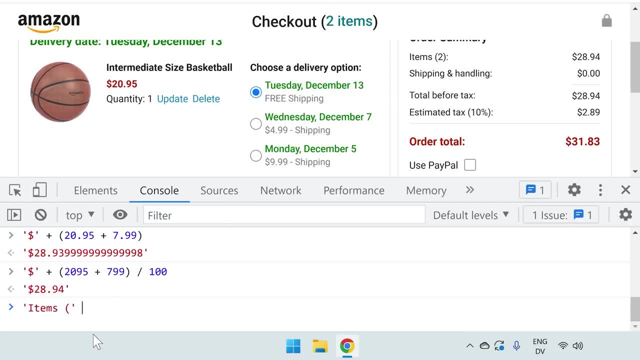 we're going to end the string here and we're going to add and we're going to calculate the quantity. So we have one basketball plus one t-shirt. Again, we run into the same problem as before: This gets calculated first and results in a. 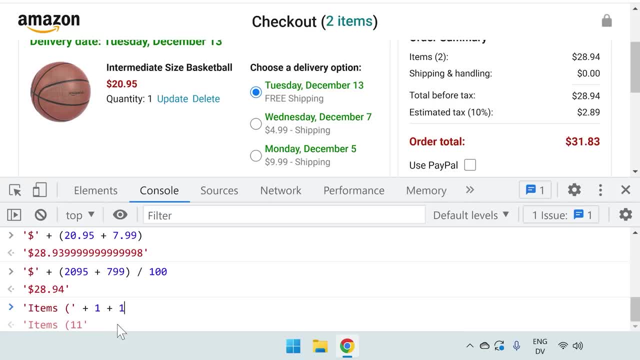 string and then it would just combine the one at the end of the string. instead of doing math To solve this, we're going to use brackets again. So around the one plus one we're going to add open bracket and close bracket. This tells the computer to. 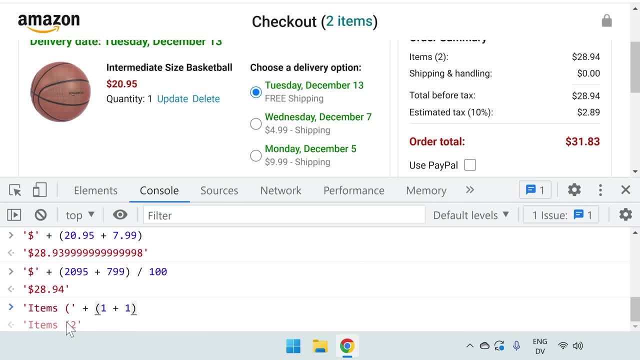 add the numbers first and then combine it with the string. Alright, let's keep going from left to right. We're going to add the rest of the string- quote, close, bracket, colon- and let's just use a space to represent the space between these two. So we'll type. 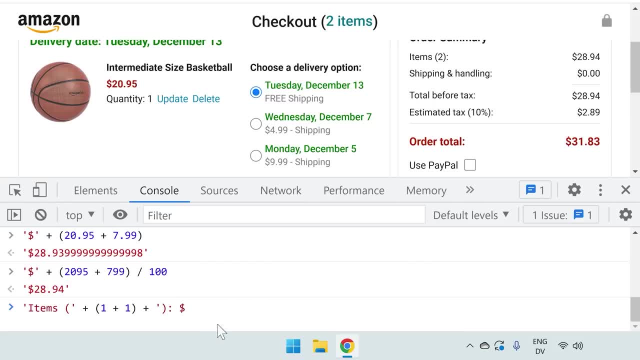 a space dollar sign and then we're going to calculate this number again and add it to the string. So we'll end the string and then plus, and we already did this calculation up here, So we can select this and then right click, copy and here: 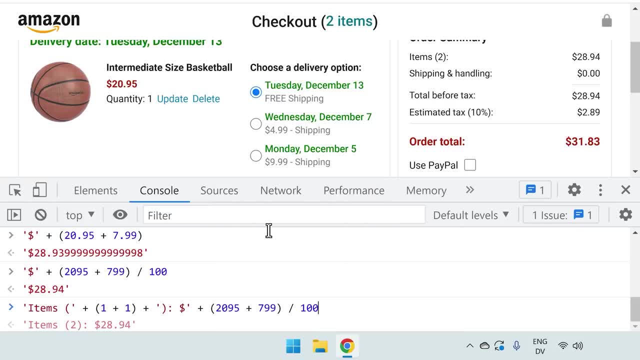 right click and paste and press enter, And that's how we create this first line of text: using strings and numbers. We break up the string into parts, calculate the numbers and then add the parts back together. Alright, now let's take these strings that we created. 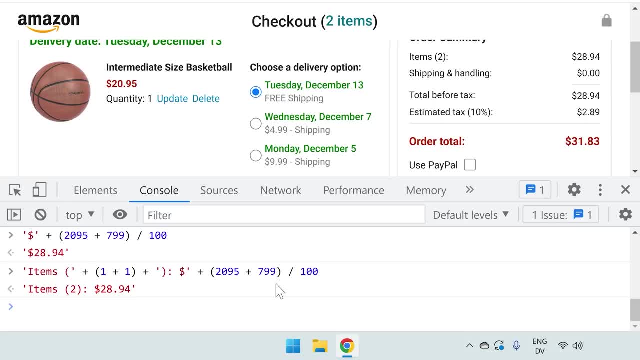 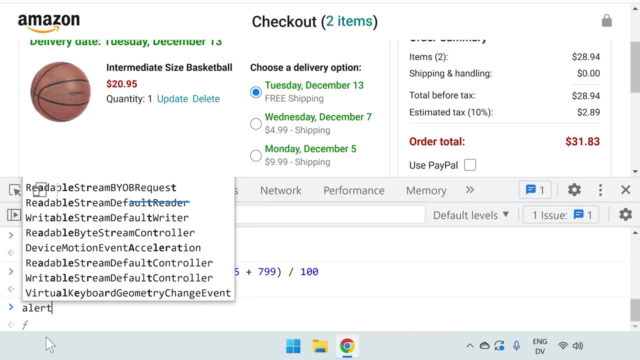 and do something with them. Let's create a popup and display this first line of text inside the popup. We'll go back to our console and type the code for creating a popup: alert- open bracket, close bracket, semicolon- and then inside the popup, we're going to display this string. 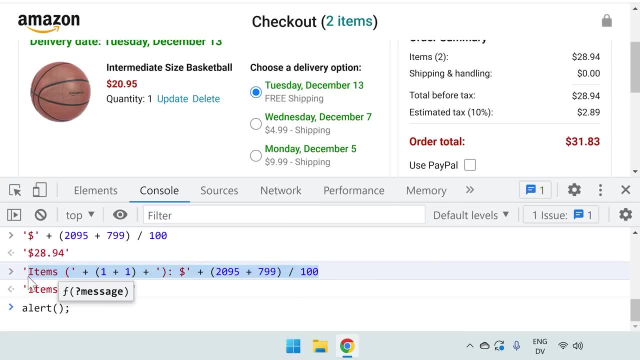 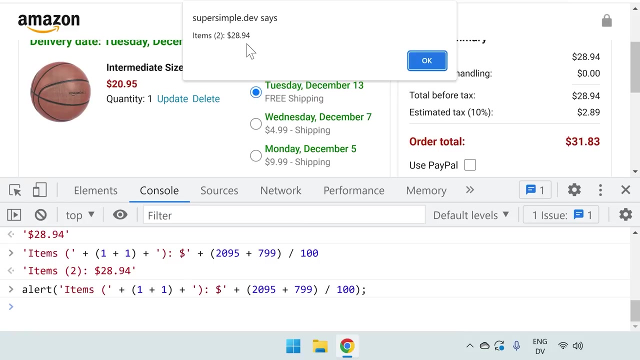 So let's just make a copy of this code. We'll select it, right click, copy and between the brackets, right click and paste. If we press enter, the computer displays a popup with the first line of text of the final project inside. So that's how we use strings. 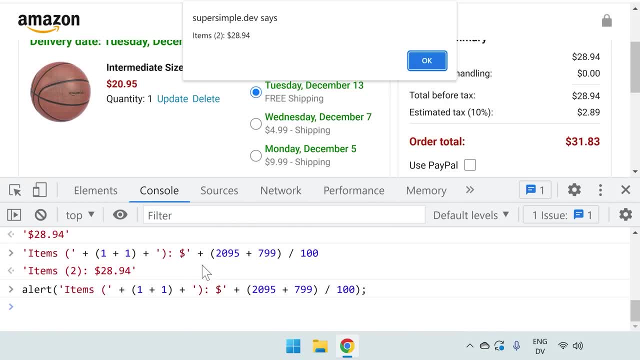 to create the text in the final project, and once we create the strings, we can use them in other JavaScript code. In the rest of this lesson we're going to learn more details about strings In JavaScript. there are actually three ways to create a string. 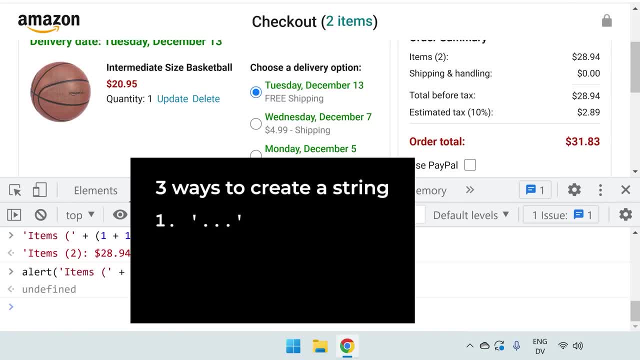 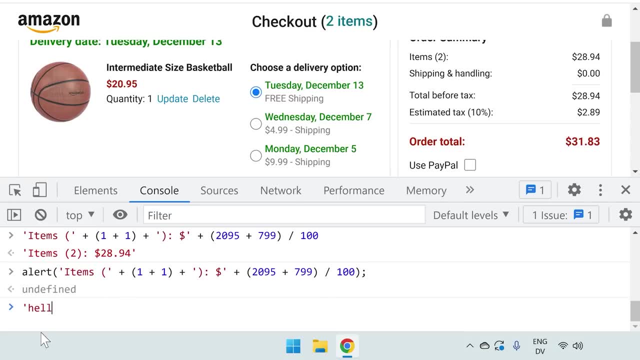 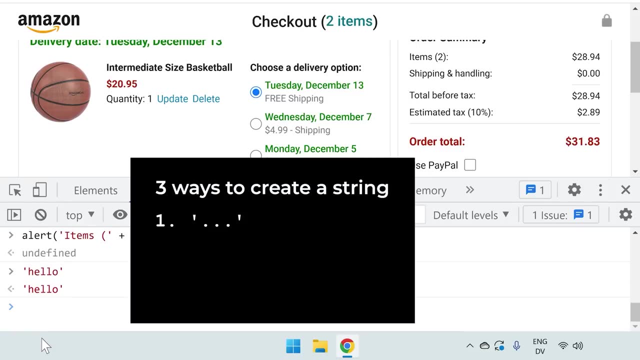 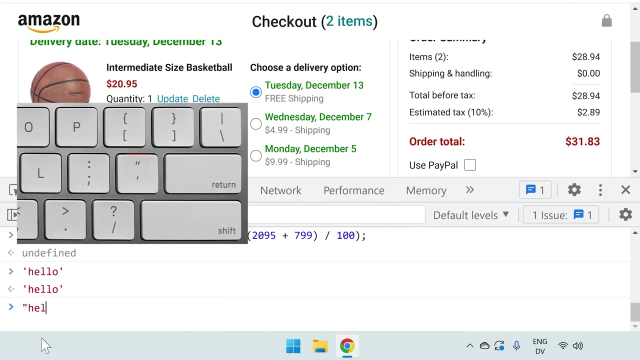 The first way is to use single quotes, which we already learned. For example, we can type single quote, hello and single quote and press enter. The second way to create a string is to use double quotes, For example double quote hello and double quote, and press. 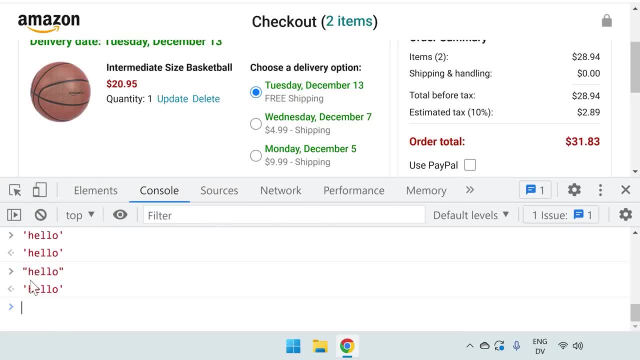 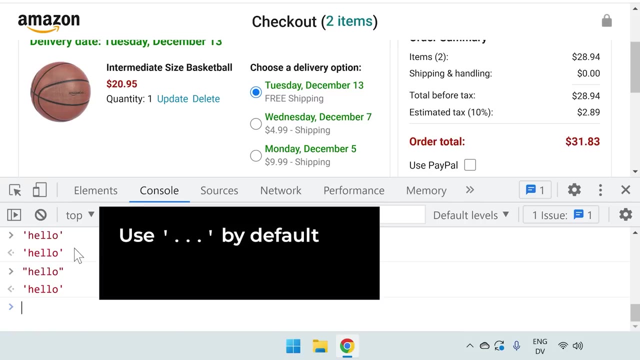 enter. This creates the exact same string as single quotes. So which one should we use to create a string, Single quotes or double quotes? In JavaScript, I recommend using single quotes by default. They're a little easier to read and type. There is one situation. 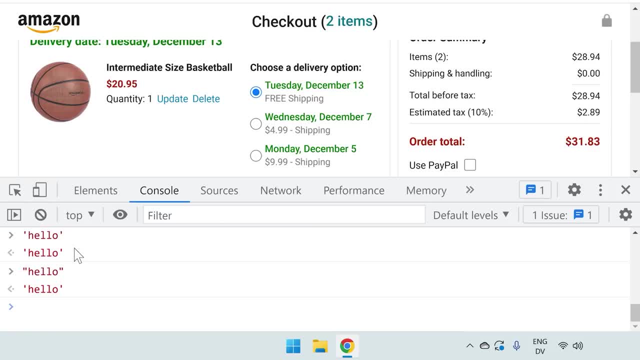 where double quotes might be useful, and that is if we have a single quote inside the string. For example, if we type the string I'm learning JavaScript and single quote and press enter, this doesn't work because there's a single quote inside the string and this single quote will end. 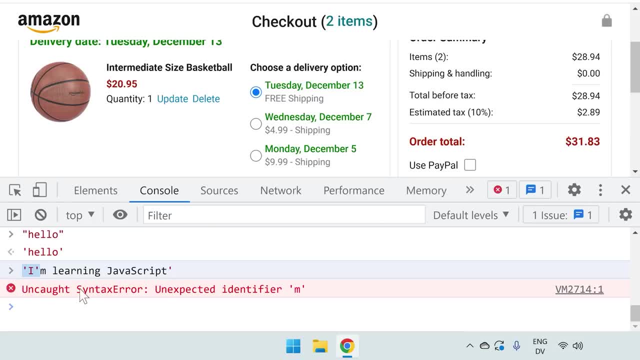 the string early. To solve this, we can create the string using double quotes, For example, double quote- I'm learning JavaScript- and double quote and press enter. So now this works. Because we created the string using double quotes, the single quote no longer has a special meaning and 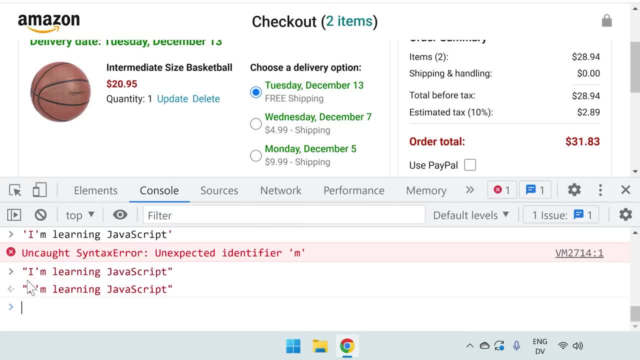 it will no longer end the string early, So this is a situation where double quotes might be useful. Otherwise, we use single quotes by default. Now there's actually another solution to this problem other than using double quotes, And that's by using an escape. 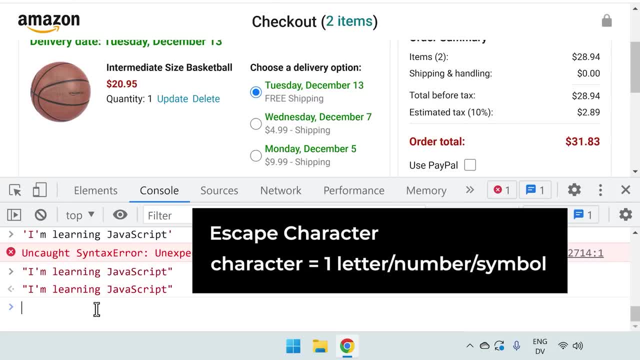 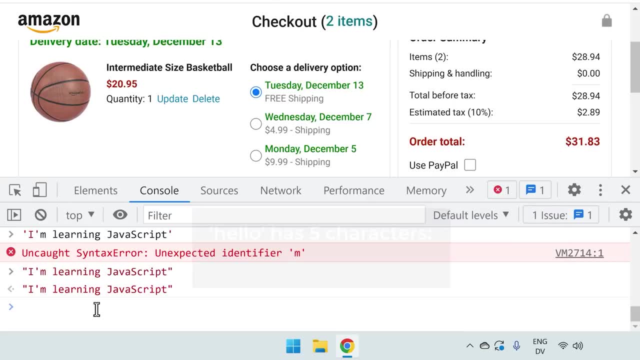 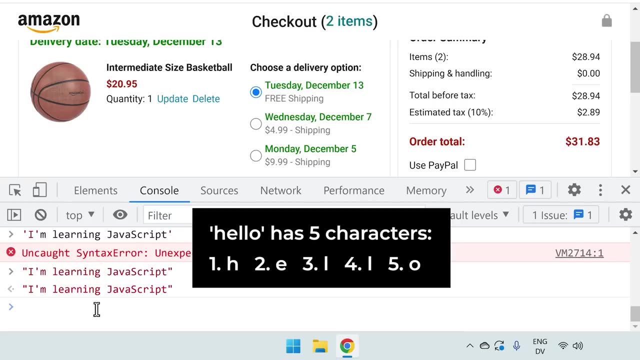 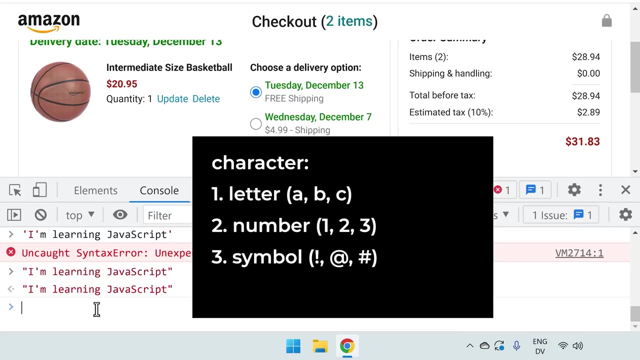 character. So a character is one letter, number or symbol in a piece of text. For example, the text hello has five characters: h, e, l, l? o. A character can be a letter, a number or also a symbol. These are all considered characters. 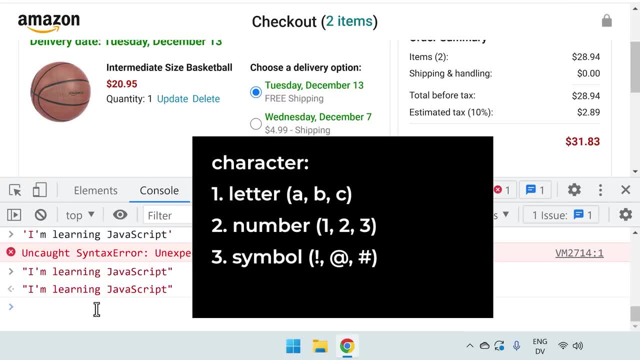 Now, in addition to these characters, we have a special set of characters we can also use in a string, Called escape characters. An escape character looks like this, A backslash, and then another character Like single quote. This combination actually counts as one character. 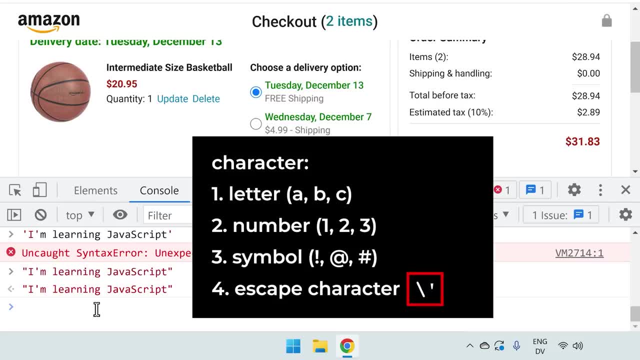 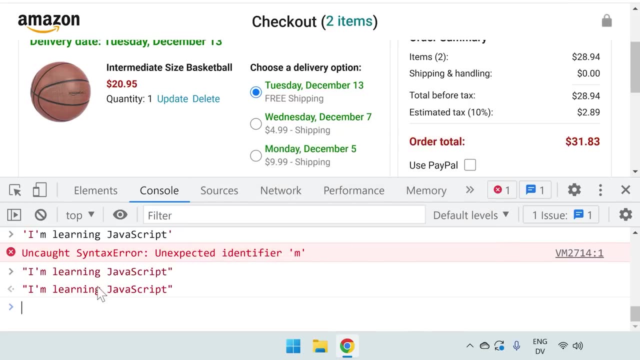 in a string. This character creates a single quote. that is just text. It doesn't have a special meaning and it doesn't start or end strings. For example, we can create this string with single quotes again, So single quote i, and this time we'll use the escape character. 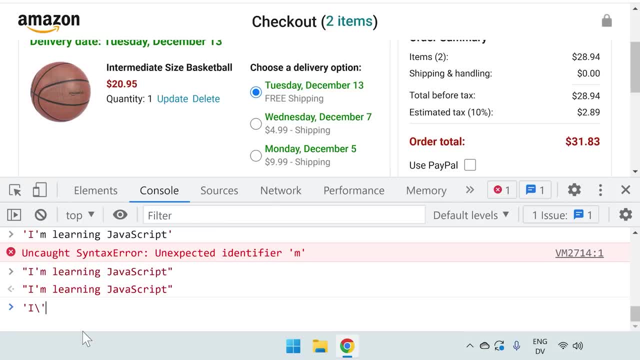 backslash single quote. and then m learning java script and single quote and press enter And now this works because the escape character backslash single quote creates a single quote. that is just text. It doesn't start or end the string. Another escape character, that's: 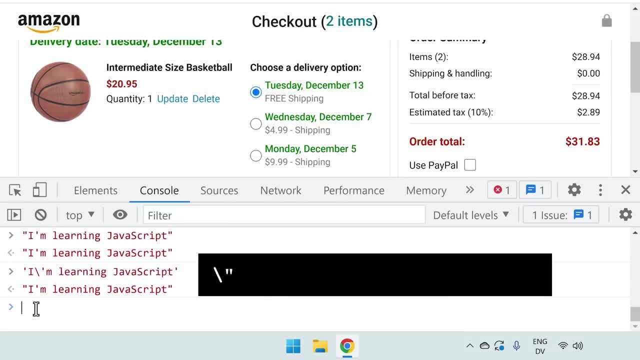 useful to know is backslash double quote. This creates a double quote. that is just text. It doesn't start or end a string. The last escape character we'll learn in this lesson is backslash n. This is called the newline character. This escape character doesn't. 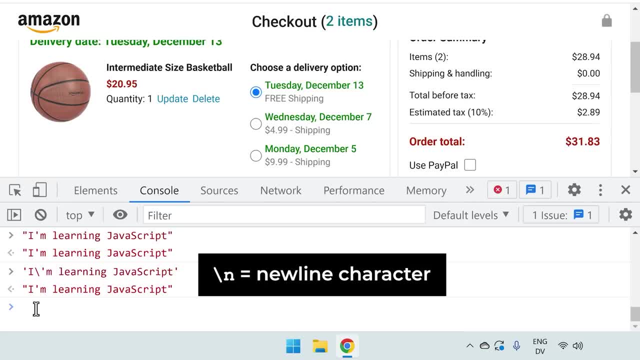 create the letter n anymore. It creates a new line of text. For example, let's create a popup using alert, open bracket, close bracket and semicolon, and then inside the brackets we're gonna create a string sum and then backslash n text and single quote. 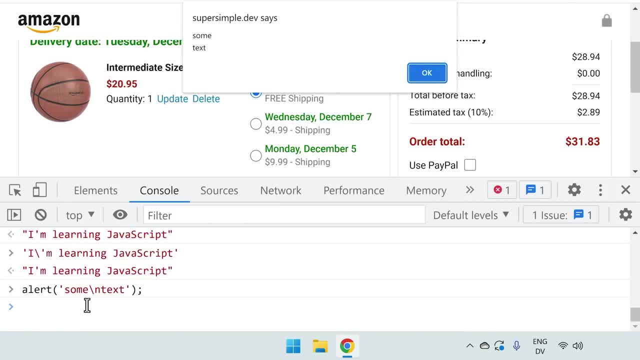 If we press enter, you'll notice that this escape character created a new line of text in the popup And that's why we call this the newline character. So that's how escape characters work. They're a set of special characters that start with backslash and we can use. 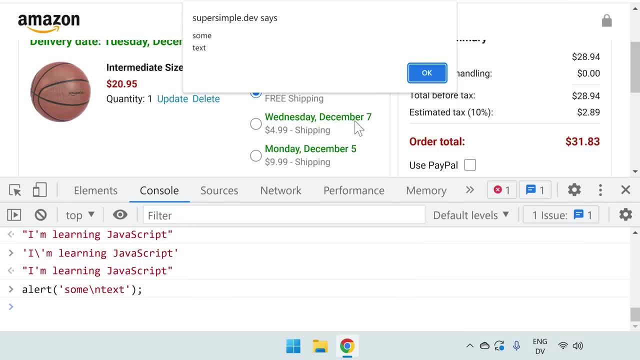 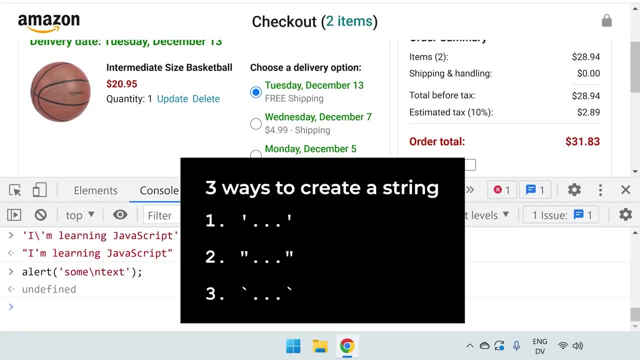 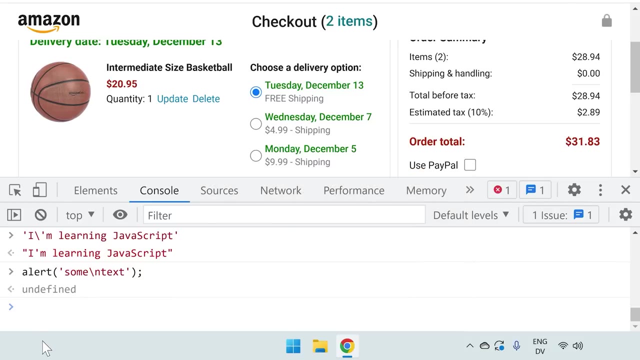 them in a string. Now let's press ok and we're gonna learn the third way of creating a string in JavaScript which is using backticks. For example, let's type in our console and we'll type backtick, hello and backtick and press enter. 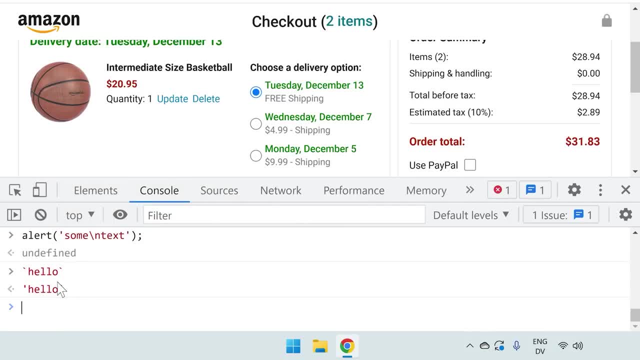 This creates the same string as single quotes and double quotes. Strings created with backticks actually have a name. We call these template strings And they have a name because they have some special features. The first special feature of template strings is called interpolation. 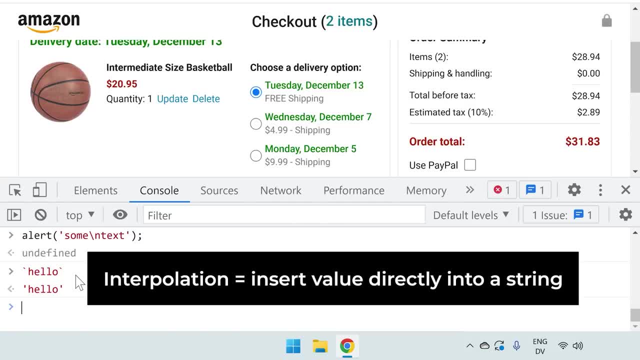 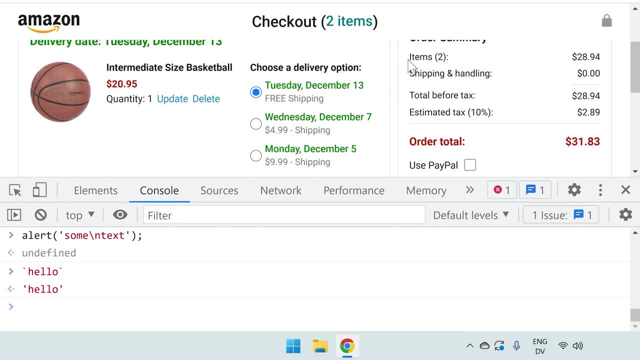 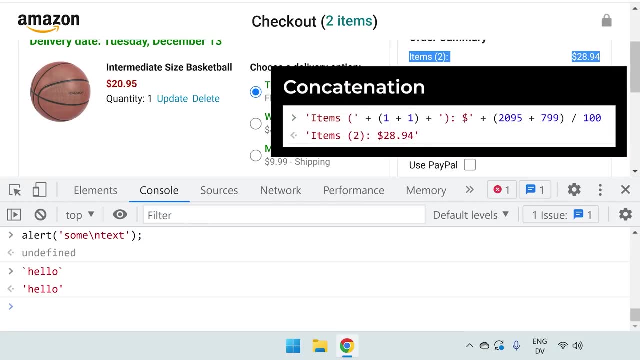 Interpolation lets us insert a value directly into a string, For example. let's say we want to create the first line of text in our project. Earlier in this lesson we created this text with concatenation, which means we broke it up into parts and added them back together. 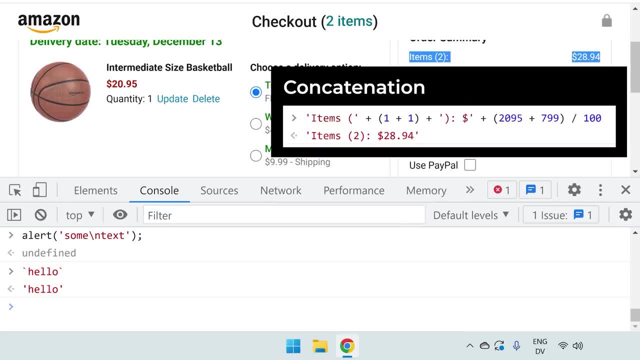 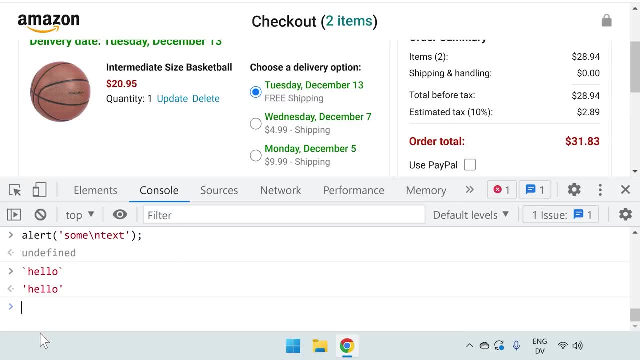 Interpolation gives us a much easier way to do this. We'll go to our console and we'll create this text using a template string, because interpolation is only a feature of template strings. So we'll type: backtick items, open bracket, close bracket and now between these brackets. 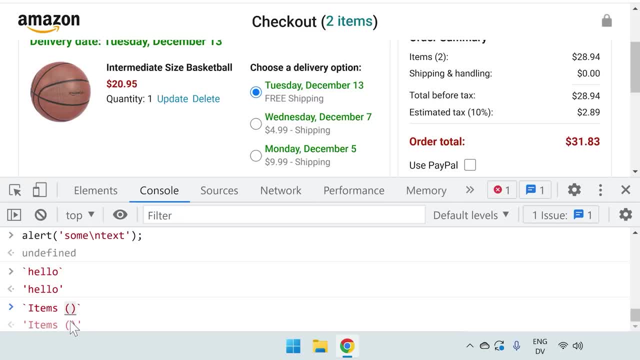 we want to insert the quantity or the number of products in our cart. To insert this with interpolation, we're going to type dollar. open curly bracket, close curly bracket. So this combination of characters allows us to insert values directly into the string Between these curly brackets. 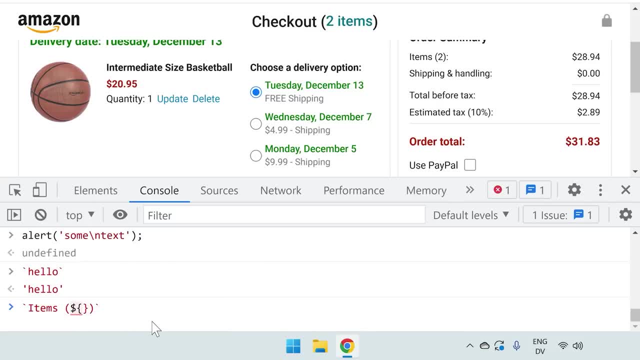 we can calculate the quantity, which is one basketball plus one t-shirt. This will add one plus one, which equals two, and then insert it directly into the string. Let's keep going and create the rest of this line, So we're going to type at the end a colon. 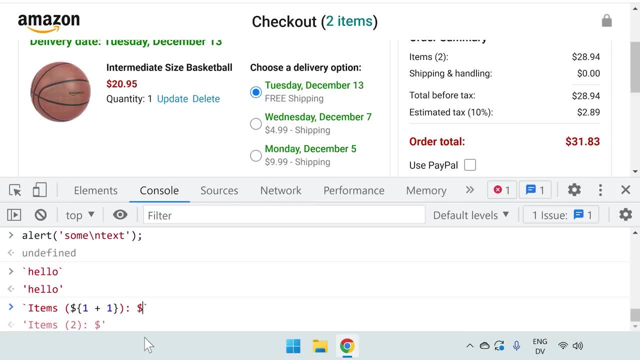 space and dollar. and now we're going to insert another value into the string, which is the cost of the products. To insert another value, we're going to type dollar, open curly bracket, close curly bracket again, And between the curly brackets we're going to calculate. 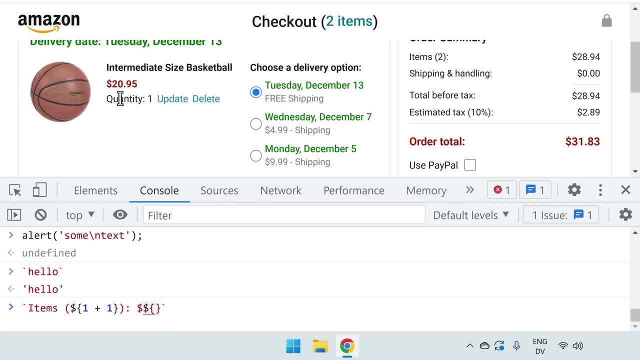 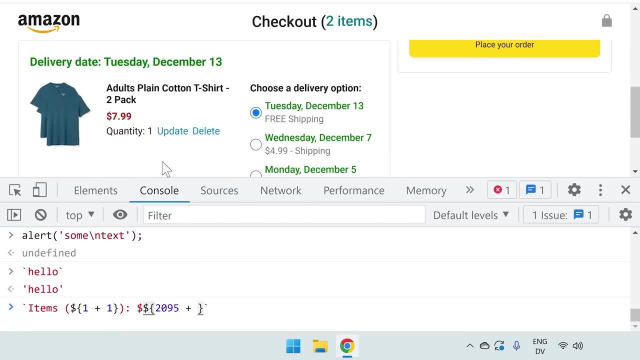 the cost of the products, which is two thousand ninety-five cents plus seven ninety-nine cents, and we'll surround this in brackets to make sure we calculate this first and at the end we're going to convert back to dollars by dividing by one hundred, If we press. 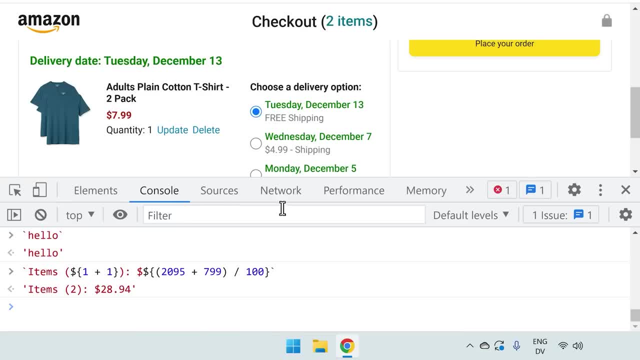 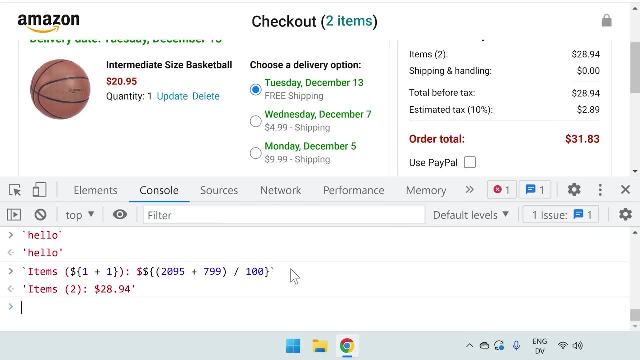 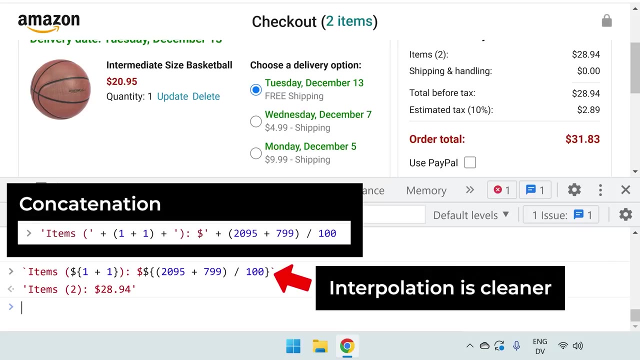 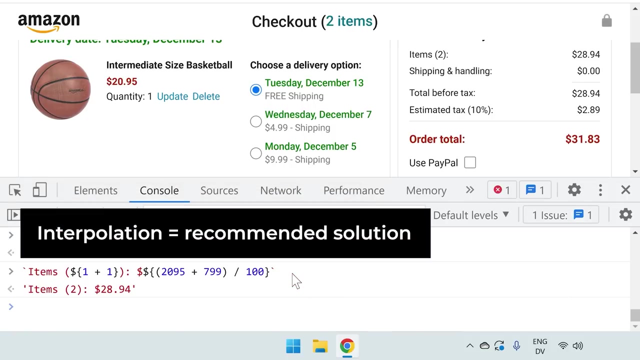 enter. this creates the first line of text again in our final project. If we compare this code, which uses interpolation, to our previous code, which uses concatenation, you can see that interpolation is a much cleaner way of inserting values into a string. So interpolation is the recommended solution. 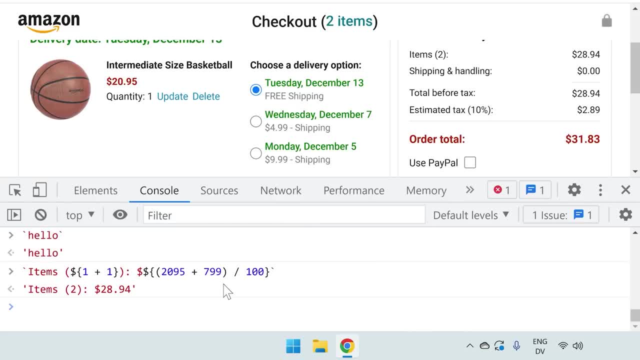 Next template strings have another special feature called multi-line strings. Let's go to our console and we're going to type a back tick sum and then press enter and text and back tick Notice that this string is on multiple lines, so we call this a multi-line string. 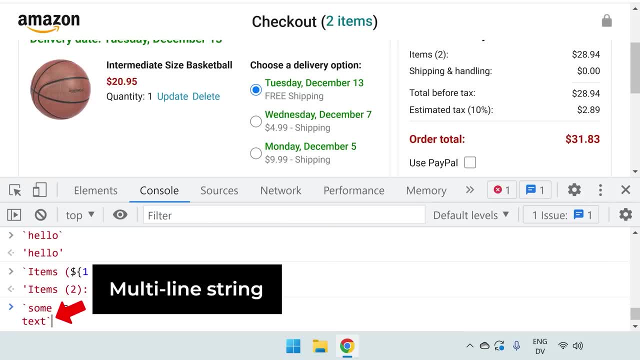 and this feature is only available for template strings. If we press enter, you can see that the new line in the string just creates the new line escape character that we learned earlier. So that's the multi-line string feature of template strings. We're going to use multi-line strings. 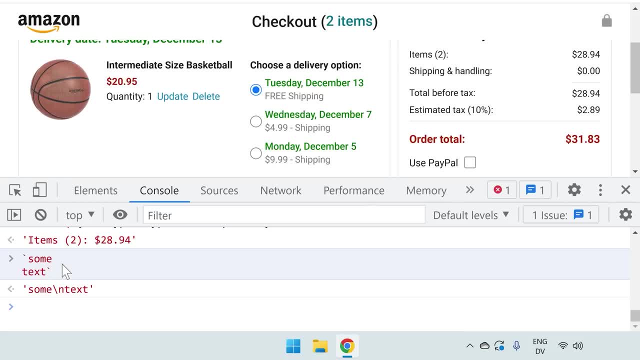 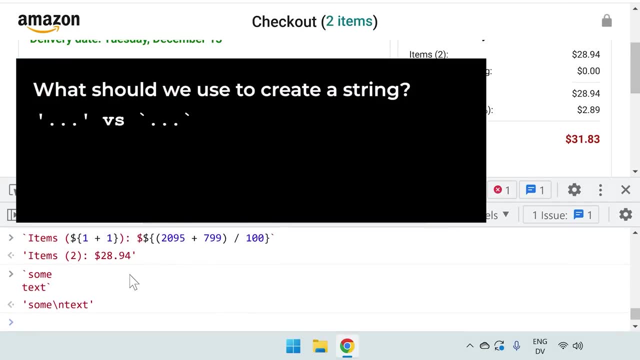 a lot later in this course, but for now I just wanted to introduce you to this feature. Now you might be wondering again: what should we use to create a string, Single quotes or template strings? Even though template strings have more features, I find that most JavaScript code. 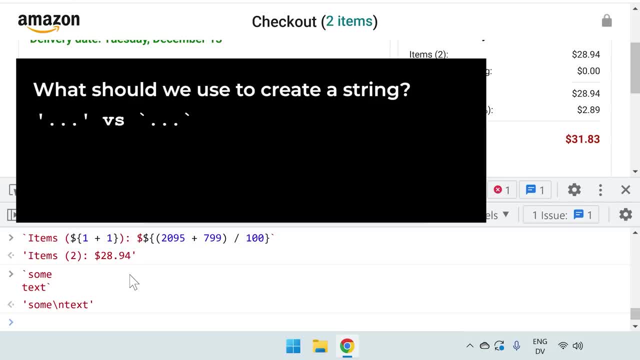 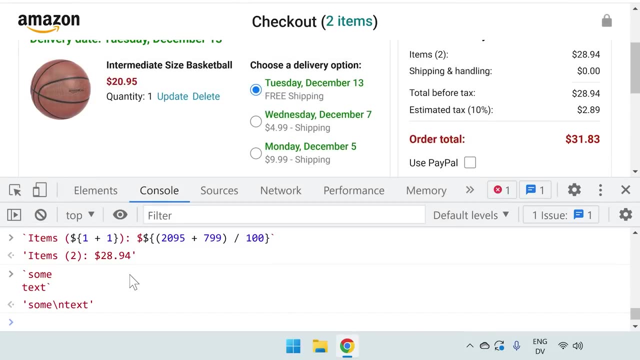 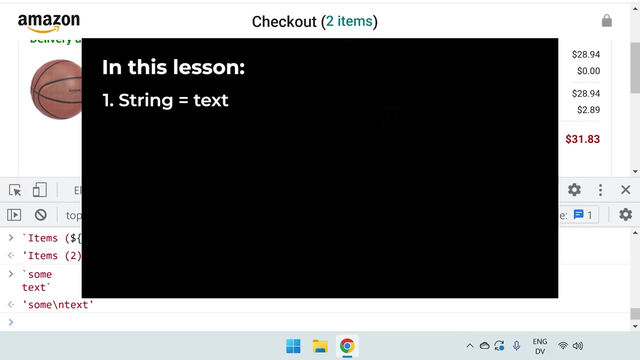 still uses single quotes by default, And if we need to insert a value into the string or type the string on multiple lines, then use template strings. And that's the end of this lesson. In this lesson, we learned about strings. A string represents text. 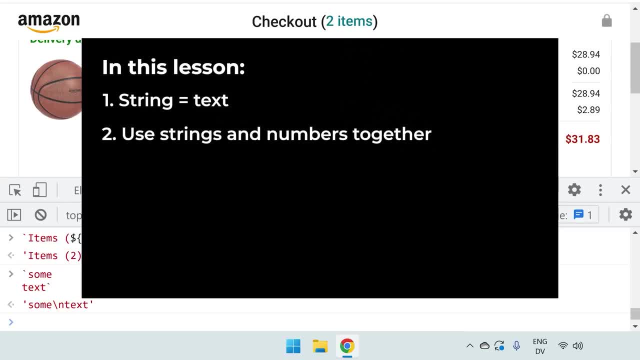 We learned how to use strings and numbers to create the text. in our final project, We learned different ways of creating a string: single quotes, double quotes and backticks, or template strings. We learned about escape characters and we learned two useful features of template strings. 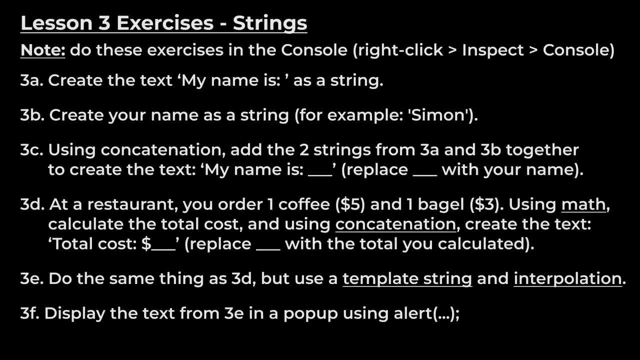 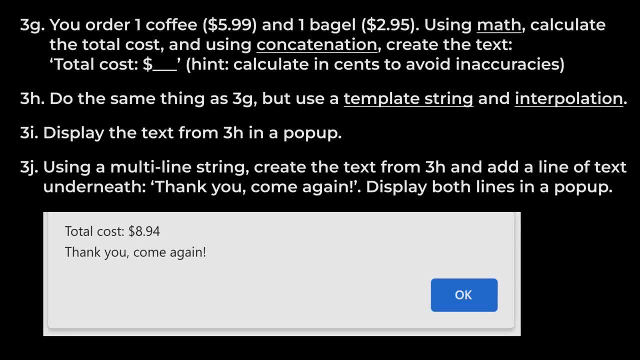 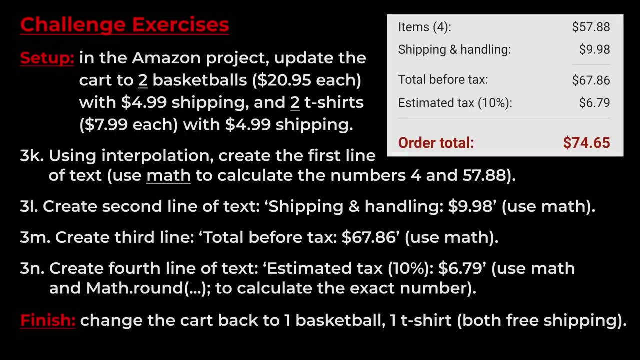 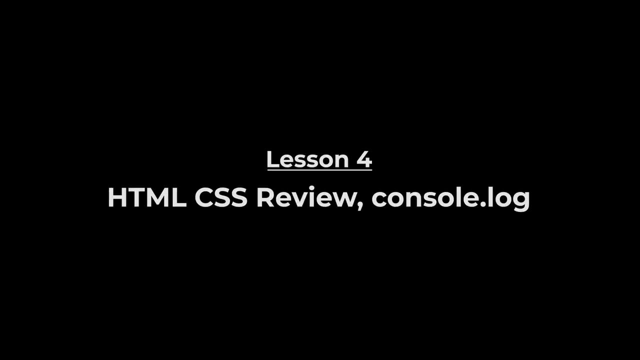 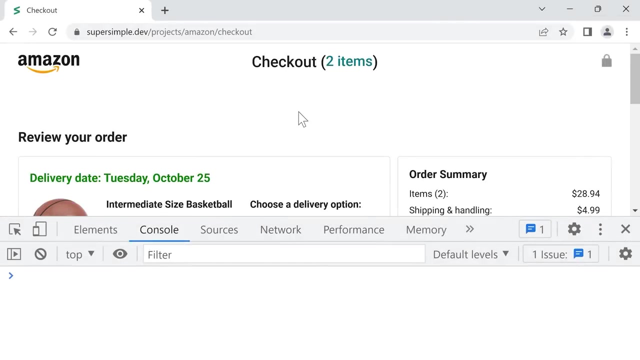 interpolation and multi-line strings. Here are some exercises to help you practice using template strings. So far in this course, we've learned some basic features of JavaScript, like numbers and strings. In this lesson, we're going to learn how to use HTML, CSS and JavaScript together. 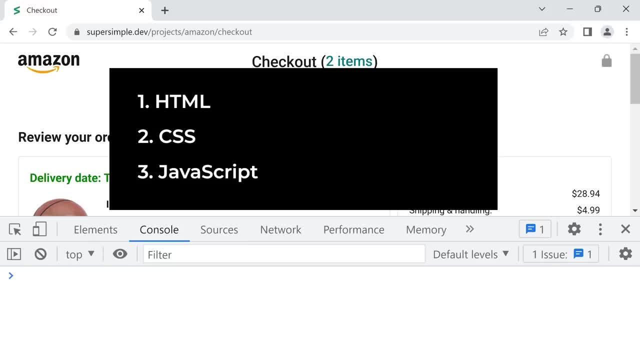 As I mentioned at the beginning of this course, we use all three technologies to build a full website. HTML creates the content of a website, like the buttons and the text. CSS changes the appearance of the website, And JavaScript makes the website interactive, The first thing we're going to do. 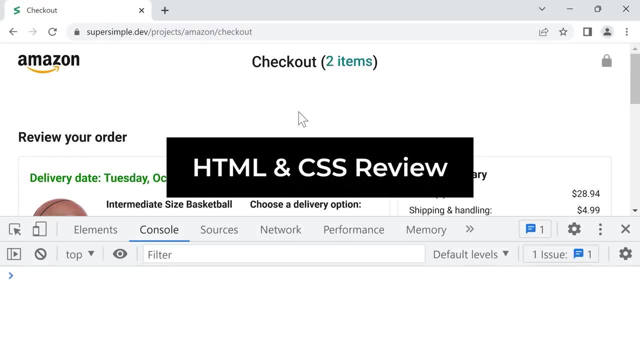 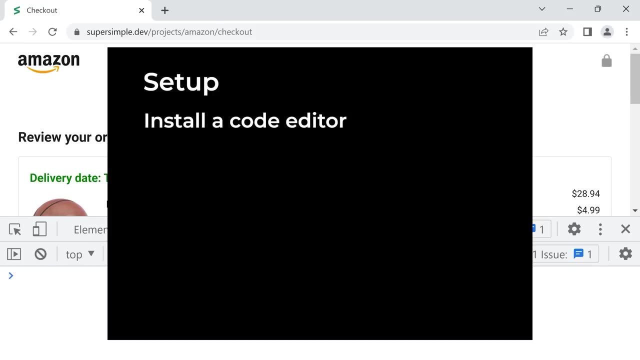 is review the basics of HTML and CSS that we will need for the rest of this course. Now, in order to write HTML and CSS code, we'll need to install another piece of software called a code editor. A code editor helps us write and organize. 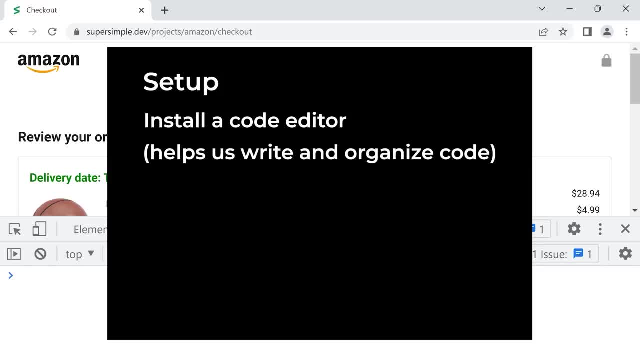 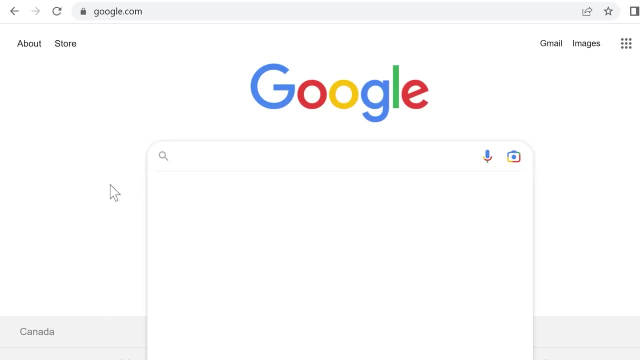 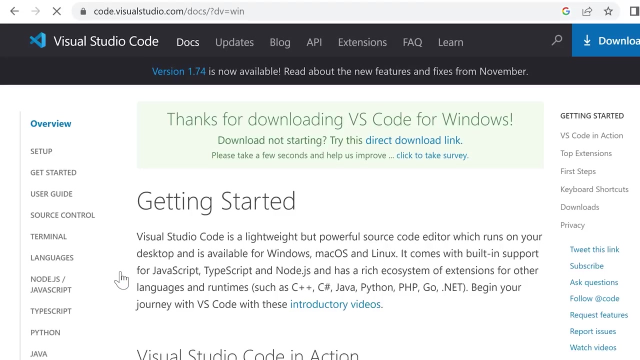 our code. The most popular code editor for web development is called VS Code or Visual Studio Code. To install VS Code, you can go to wwwvscodecom in your browser, search for VS Code, click the result and follow the instructions to download and install. 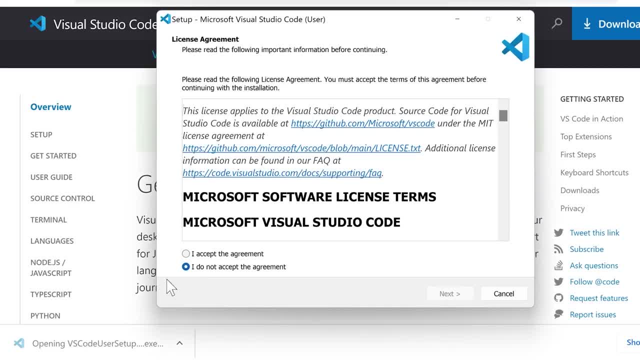 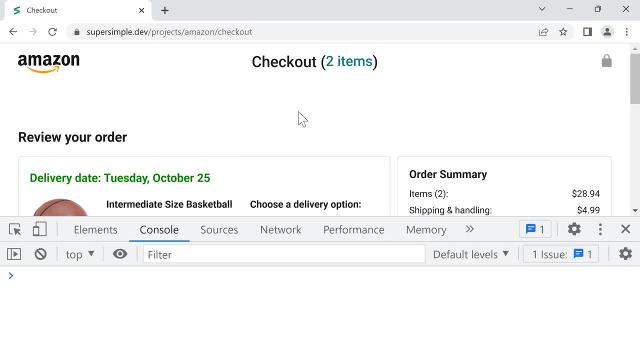 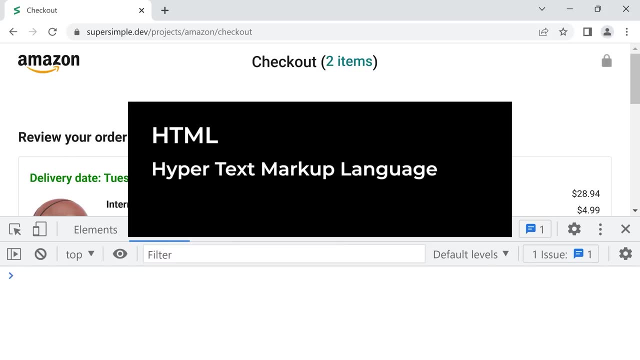 Once we've installed VS Code, we're ready to review the basics of HTML and CSS. We'll start with HTML. HTML stands for Hyper Text Markup Language And, just like JavaScript, HTML is also giving instructions to a computer. Now, unlike JavaScript, we can't use the console. 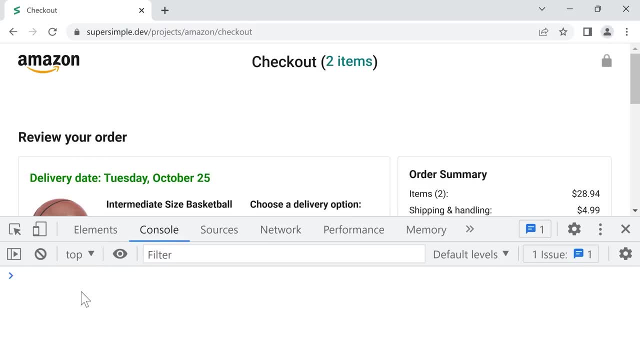 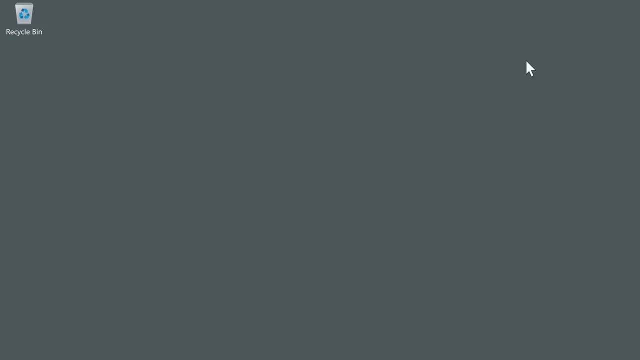 to write and run HTML code. Instead, we write HTML code inside a file using our code editor. Let's do that right now. We'll start by going to our desktop, so I'm going to close my browser to go to my desktop and then we're going to create. 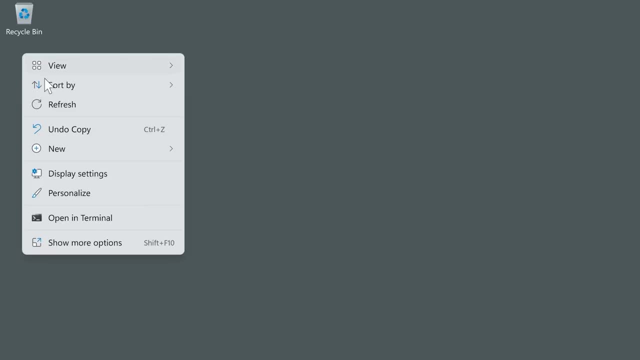 a new folder, So we can right-click New Folder. This folder is going to contain all the code that we write in this course. Let's name this folder JavaScript-Course. Next, we're going to open this folder in our code editor, So let's open. 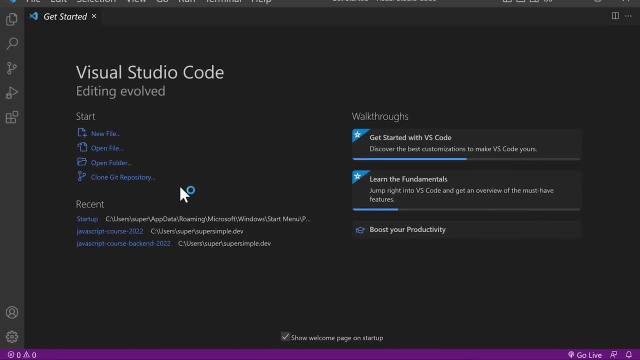 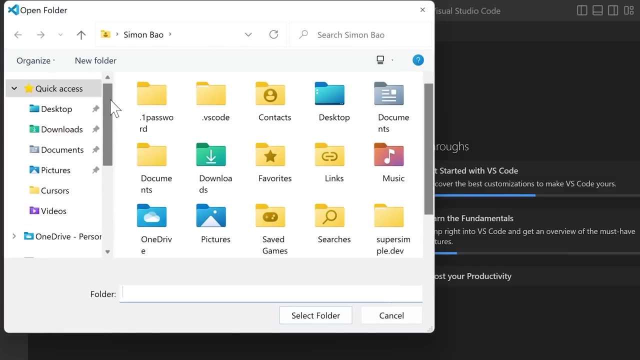 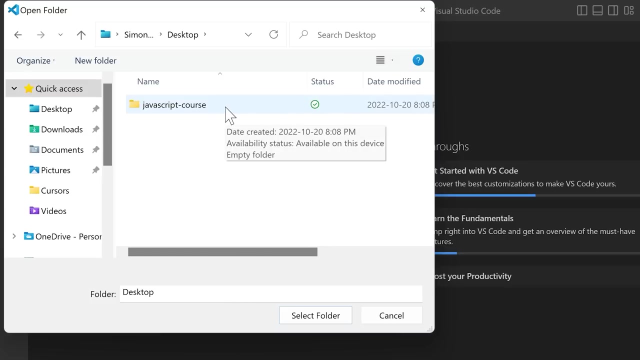 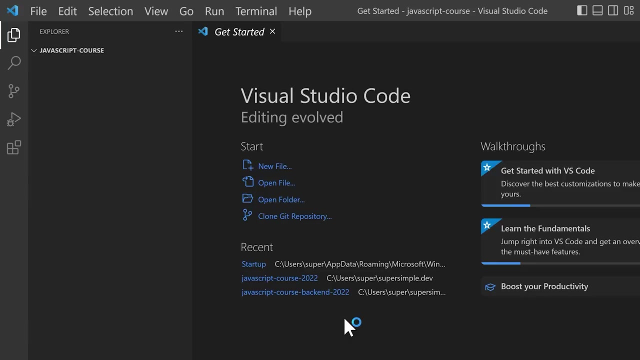 VS Code and then we'll click File, Open Folder and find the folder that we just created For me. it's on the desktop and it's this folder right here, So we're going to select the folder and then click Select Folder. Now we can close. 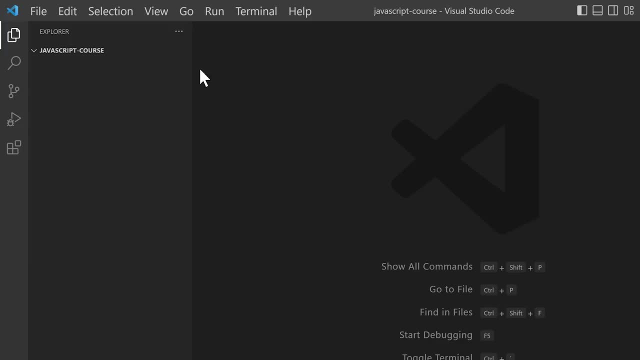 this startup message and we're going to create an HTML file. We're going to click this icon to create a new file and we're going to name this file websitehtml and press Enter. Ending the file name with html tells the computer that this file. 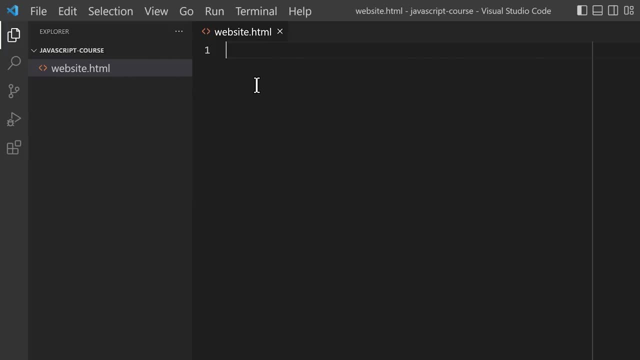 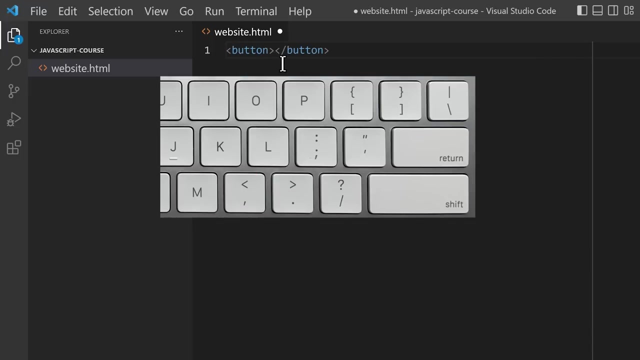 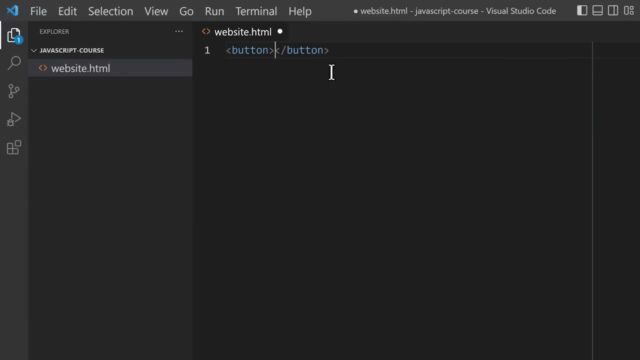 contains HTML code rather than just text. Now let's review some basic HTML code. We're going to type the code button greater than, and we also need to type less than slash button greater than, but our code editor might autocomplete this for us. So this code: 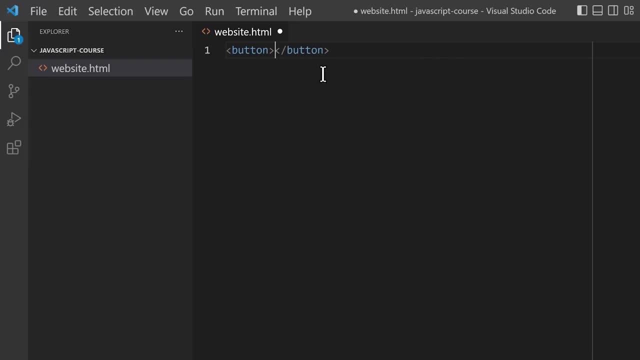 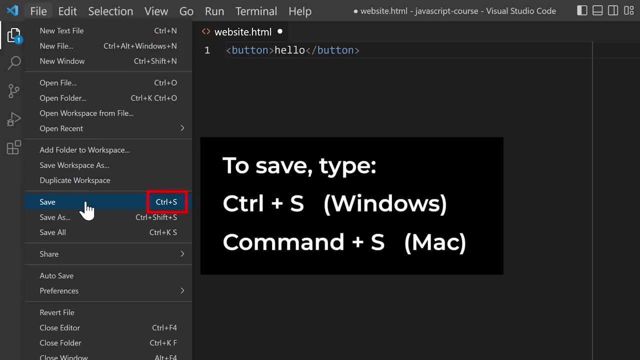 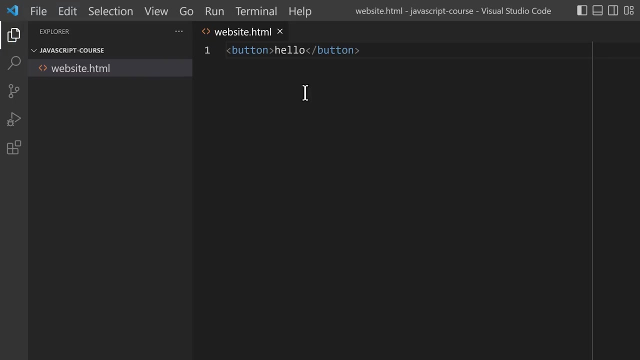 tells the computer to create a button, And inside the button we're going to have the text Hello. Now let's save this file by clicking File Save or by typing Ctrl S on Windows or Command S on Mac: Now to run this HTML code. 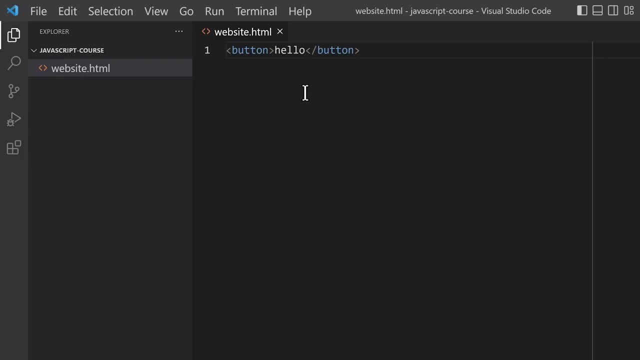 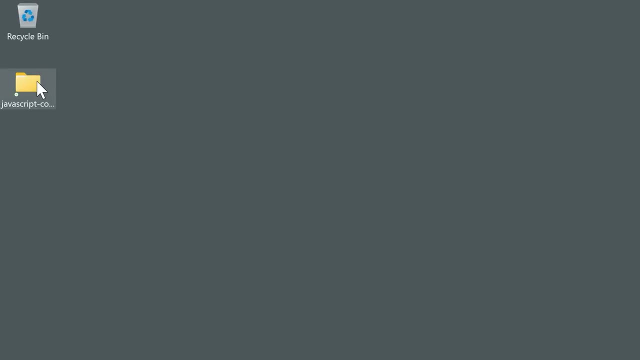 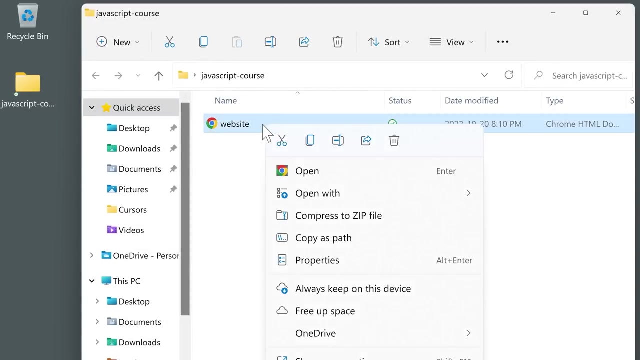 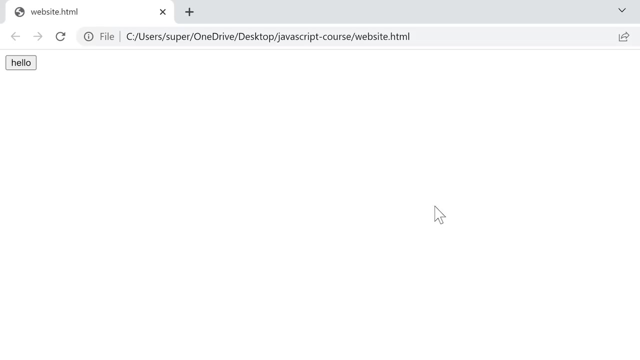 we're going to open this file in our browser. Let's go back to our desktop. We're going to open the folder that we created, Find the HTML file, select it and then right click Open with Google Chrome. As you can see, we have a website. 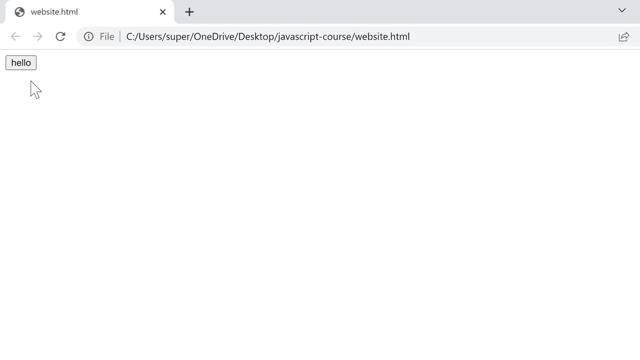 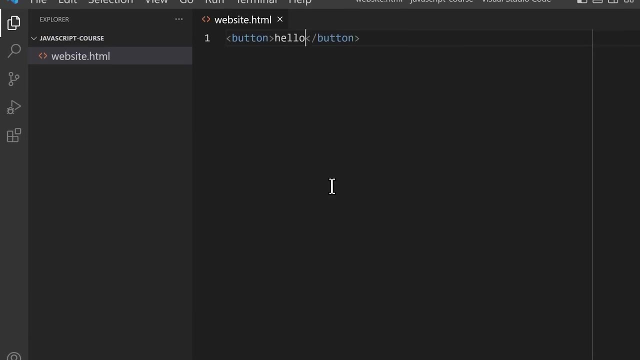 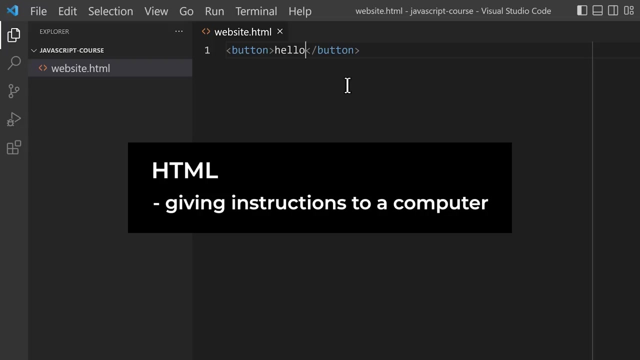 and we created a button with the text Hello inside, And if we look back at our code, that's exactly what we told the computer to do. So, just like JavaScript, HTML is also giving instructions to a computer. Let's review some more HTML code. 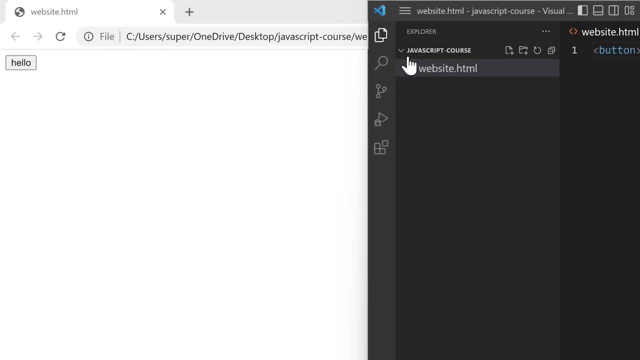 First I'm just going to rearrange my windows here so that it's easy to see the website side by side. Next we're going to click the end of the first line and press Enter to create a new line, and we're going to type the code. 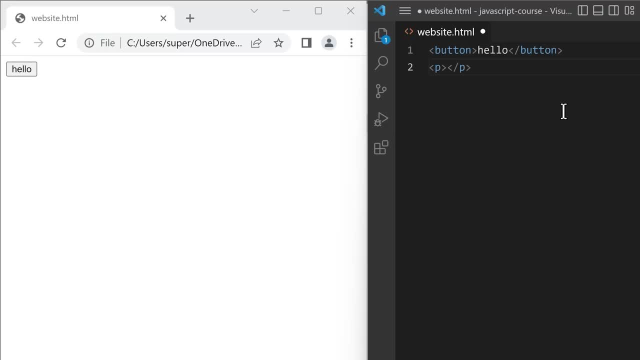 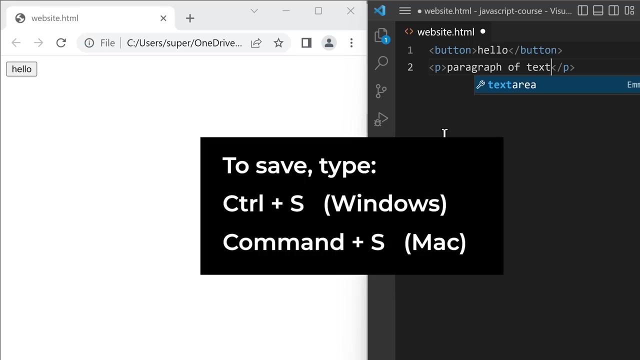 less than p greater than, and we also need to type less than slash p greater than. So this code creates a paragraph And inside the paragraph we're going to put some text. For example, paragraph of text. Now let's save our file by typing control s on windows. 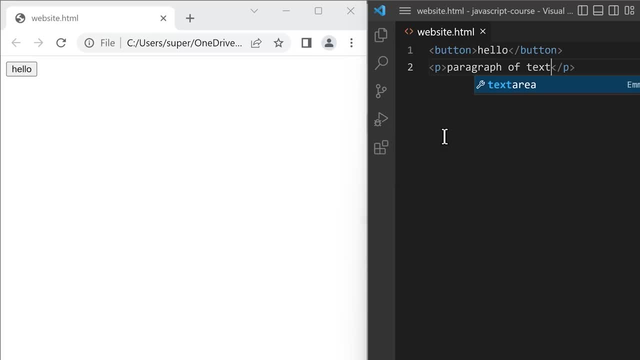 or command s on mac and to update our website to the new code. we're going to go to our website and click refresh or type control r on windows or command r on mac, And now you can see that the computer created a paragraph of text, just like we told it to do. 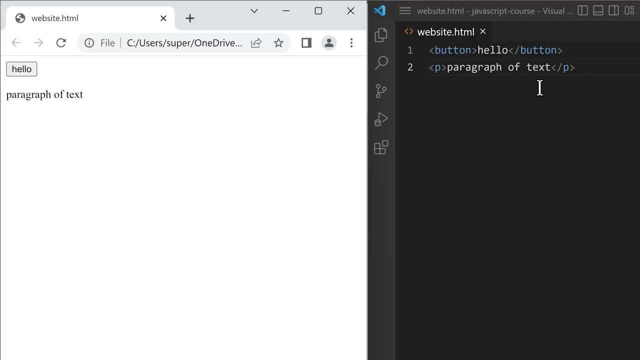 And that's the basics of HTML. The computer reads our code and then follows our instructions one by one. First it creates a button and then it creates a paragraph of text. Now let's review the syntax rules for HTML. Each of these things: 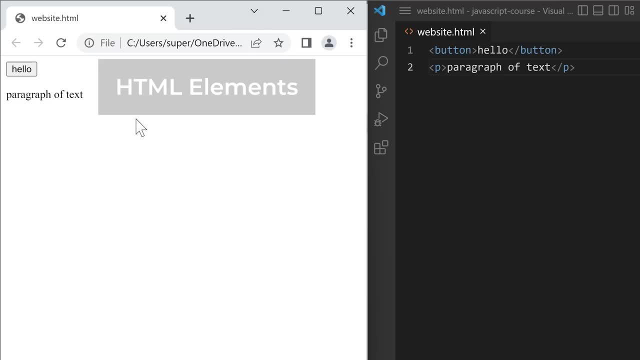 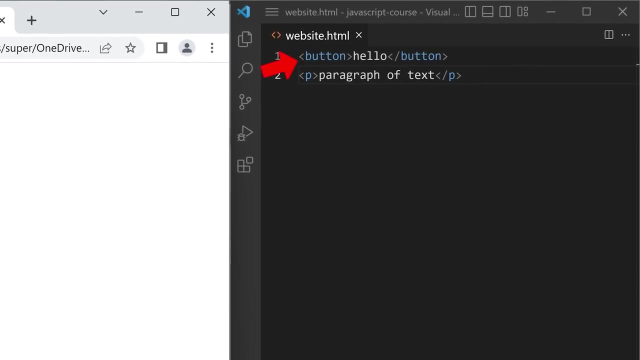 that we're displaying on a webpage. these are called HTML elements. So a button is a type of HTML element and a paragraph is another type of HTML element. To create an element, we start with a less than symbol and then the element name like a button. 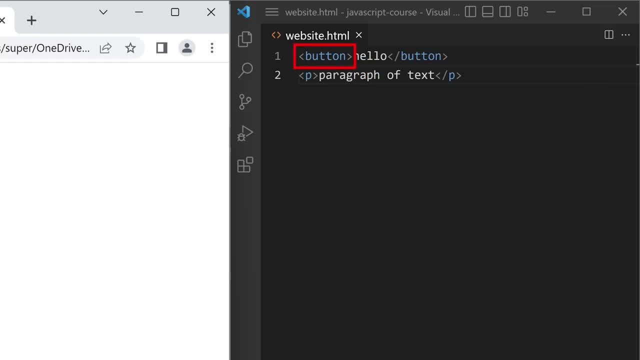 And then the greater than symbol. So this whole thing is called an HTML tag. This tells the computer to create a button element. Every HTML tag needs a matching tag. The matching tag follows the same syntax, except it has a slash in front of the. 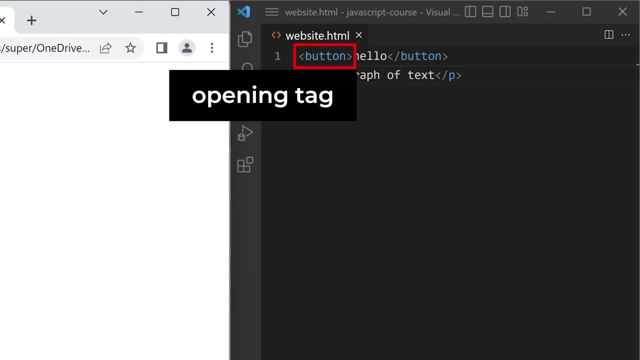 element name. So this is called the opening tag and this is called the closing tag. You can think of the opening tag as the start of the button and the closing tag as the end of the button, And in between we have the contents inside the button. In this case, 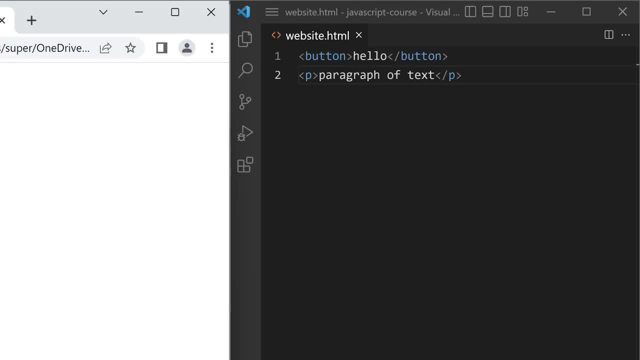 it's the text. hello, In addition to text, we can also have elements inside an element. For example, we can go to our paragraph element and we can add a button inside. So less than button, greater than, and we also need less than slash button. 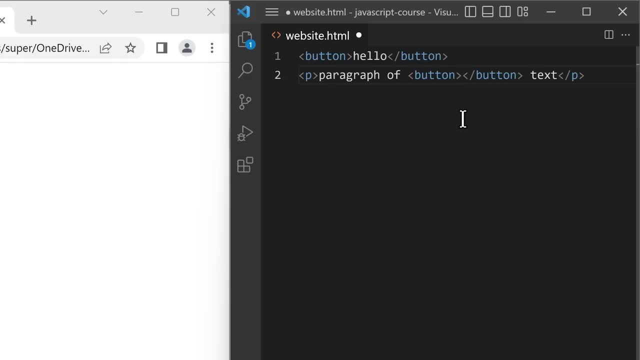 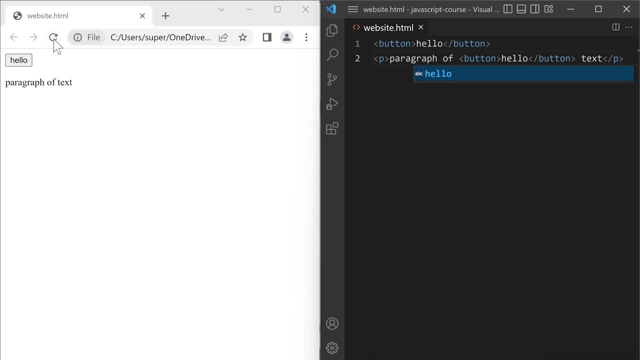 greater than, And then inside the button we'll also have the text hello. If we save this file and refresh the page now, our paragraph element has a button element inside. By the way, this is called nesting, when we have an element inside another element. 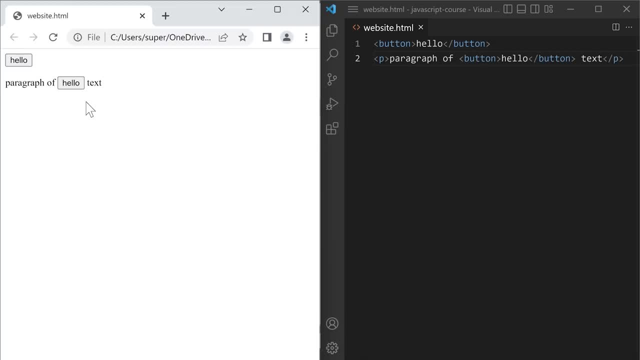 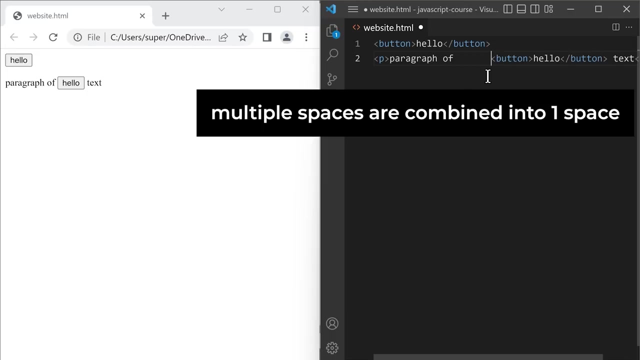 The last syntax rule we have to review is that in HTML, if we have multiple spaces- for example, if we go here and type multiple spaces- multiple spaces are combined into one space on the webpage. So if we save this code and refresh, you'll notice that all. 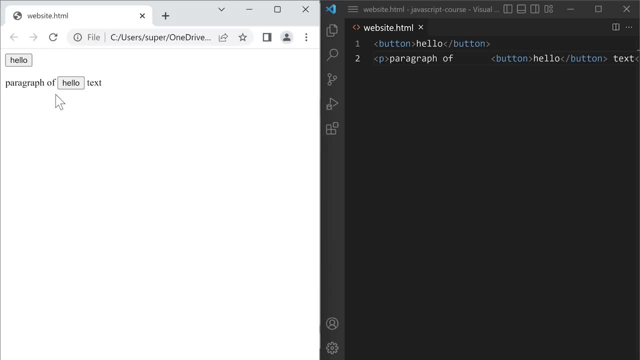 of the spaces that we added only show up as one space on the webpage. In addition, in HTML new lines also count as spaces. So if we go back to our code and we type here and press enter to create a new line and then save and 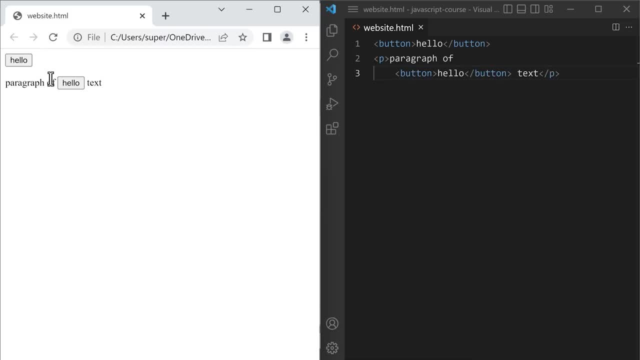 refresh, notice that the new line doesn't appear on the webpage, And that's because this new line here is the same as spaces in HTML, So all of these get combined into one space on the webpage. At first this might seem a little weird, but this feature. 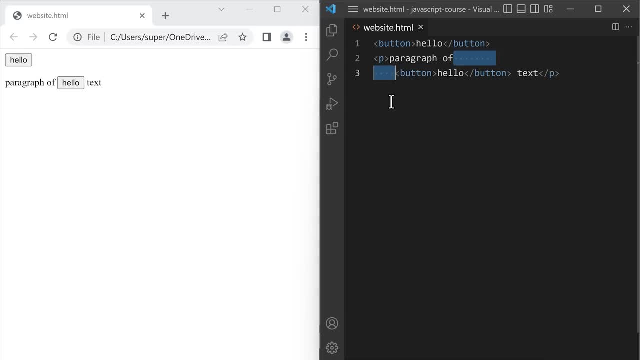 gives us a lot of flexibility when organizing our HTML code. For example, we can go into our code and add a new line here to separate these two elements and make our code easier to read. Another thing we usually do to make our code easier to read is to 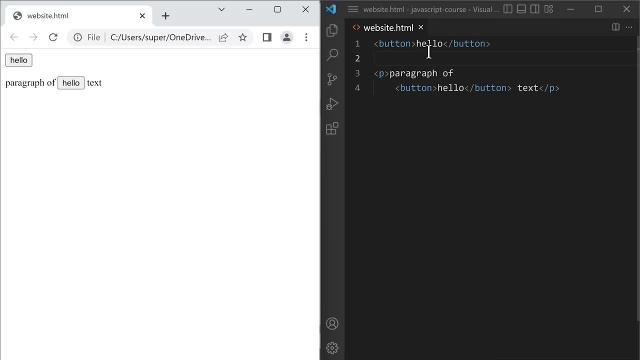 put the contents of an element on its own line. For example, we're gonna type here and press enter, and here and press enter again to put the contents of the button on its own line. Now it's a lot easier to see where this button. 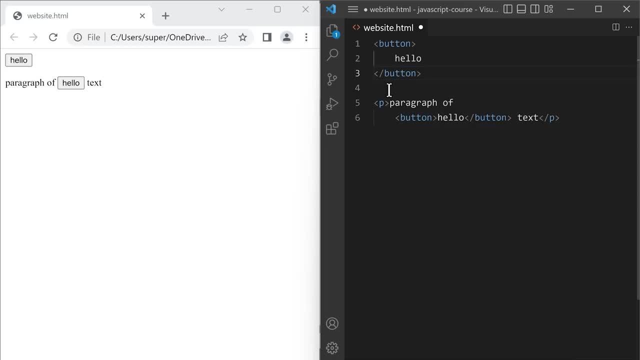 starts and where it ends. We can do the same thing with the paragraph. We can type here and press enter, and type here as well and press enter, and then remove some of the extra spaces to put the content of the paragraph on its own line. 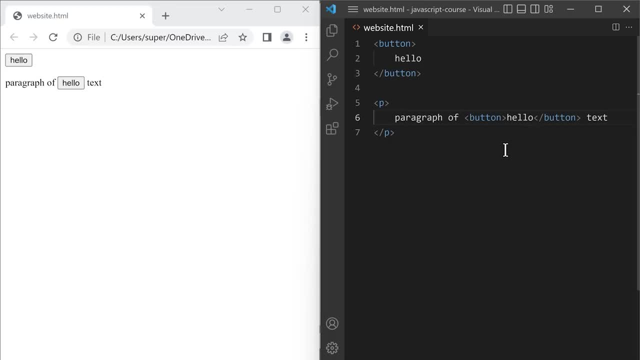 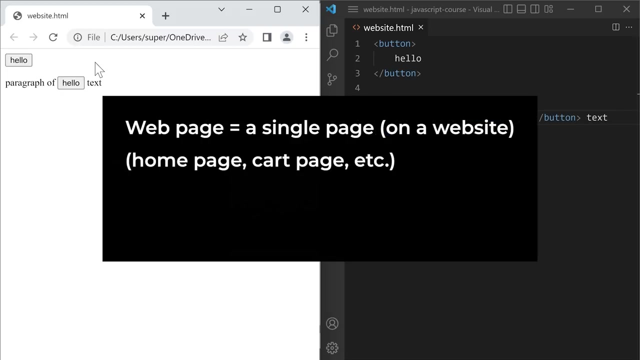 And now, if we save our file and refresh, you'll notice that none of the new lines that we added appear on the webpage. By the way, a webpage is a single page, like the homepage or the cart page Together. we call this a website. 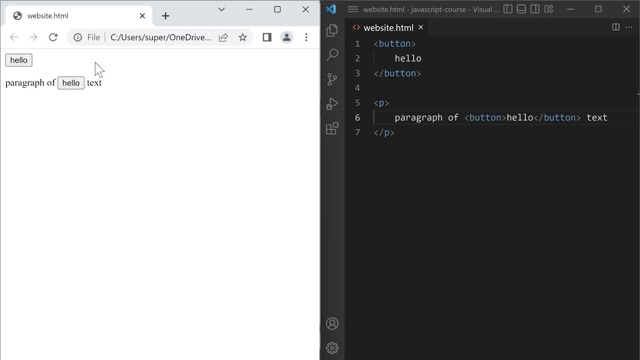 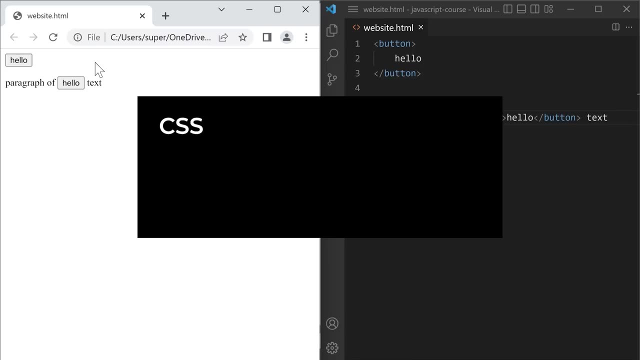 So that's the basics of HTML and HTML syntax. Now let's review CSS. CSS stands for Cascading Style Sheets, and CSS changes the appearance of our website. Let's review some CSS code. We're going to write our CSS code inside our HTML. 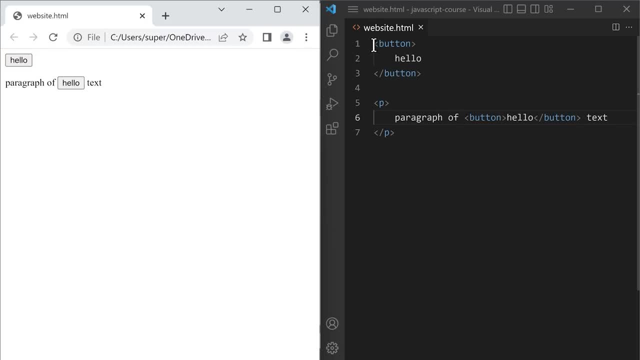 file. First let's type here and create some new lines at the top, and then at the top we're going to create a special HTML element called the style element. So let's type less than, style greater than, and we also need the closing tag. 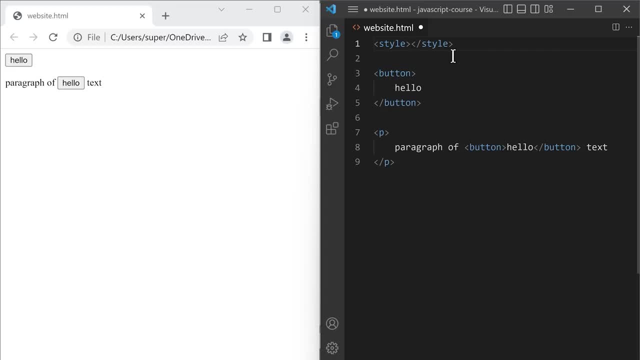 less than slash. style greater than So. the style element is unique because it doesn't appear visibly on the page. Instead, the purpose of the style element is that it lets us write CSS code inside. So inside here, let's press enter to create a new line. 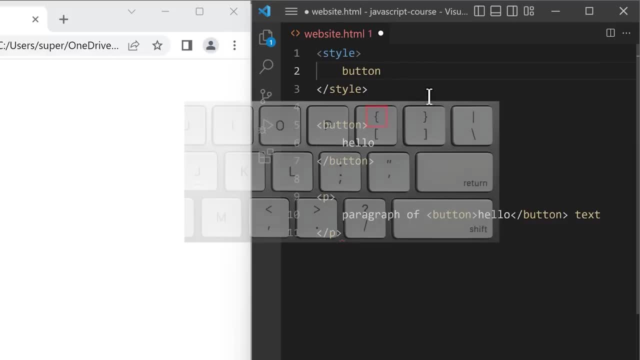 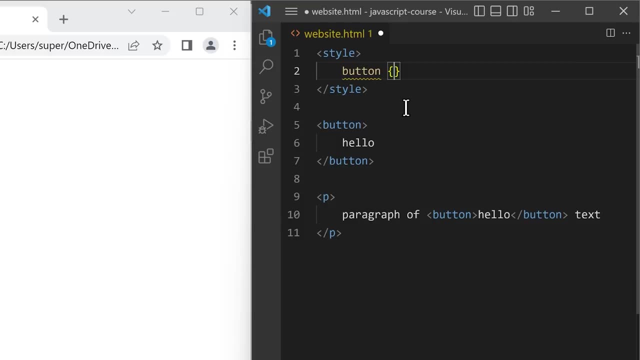 and we're going to type button close and then, inside the curly brackets, we're also going to press enter to create a new line. So this is CSS code and this code tells the computer to change the appearance of all buttons on the page And then inside. 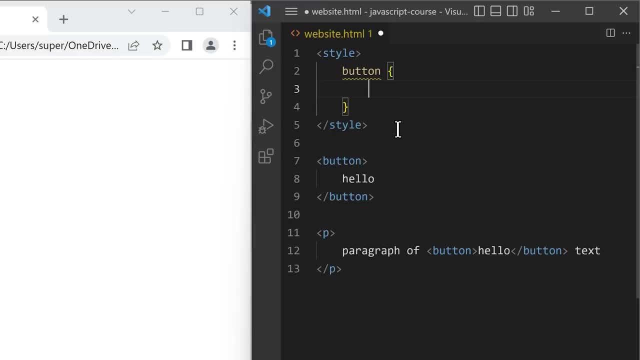 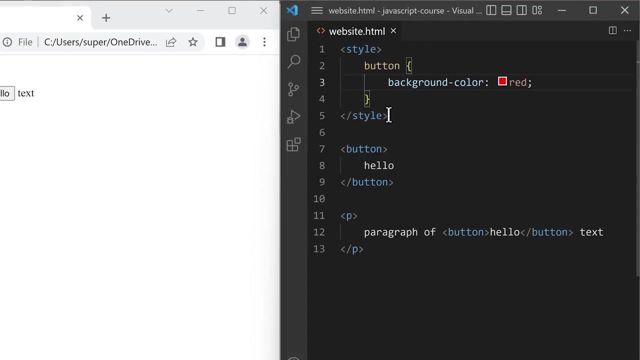 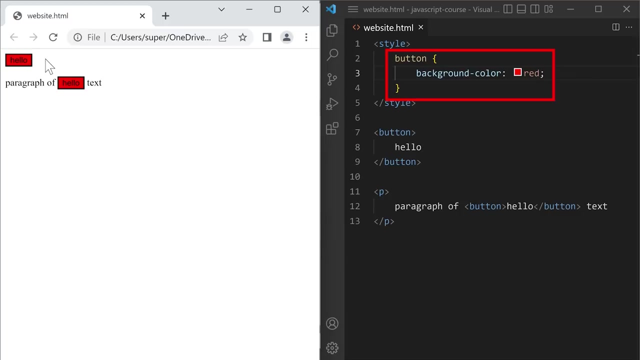 these curly brackets we can tell the computer how to change the appearance. For example, we can type background dash, color, colon, red and semicolon. If we save and refresh, you can see that this CSS code changes the appearance of all buttons on the page. 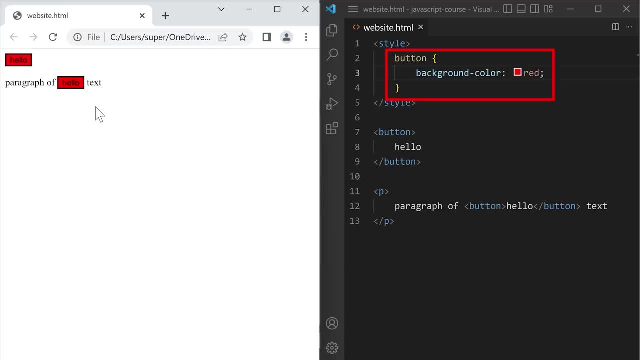 and changes their background color to red. Let's do another example. We're going to go back to our CSS code. We're going to type here and press enter to create a new line and we're going to add color, colon, white and semicolon. 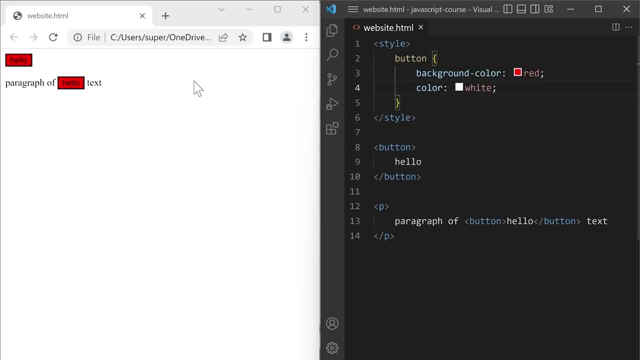 Let's save and refresh. and this CSS code changes the text color of all buttons on the page to white. Let's do one more example. We're going to type the code, border, colon, none and semicolon. Let's save this and refresh. And this CSS code. 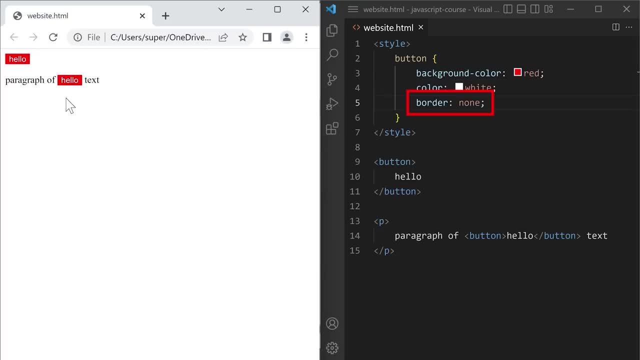 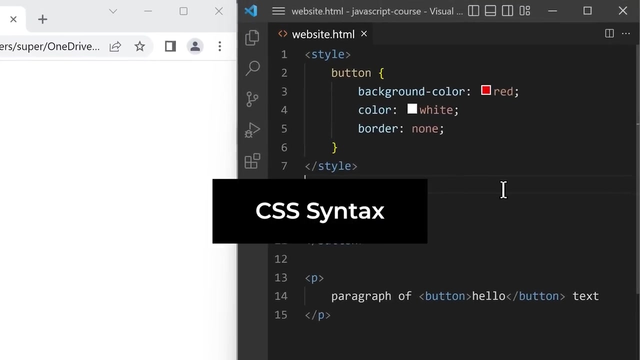 removes the border for all buttons on the page. And that's how CSS works. We tell the computer which elements we want to change and then how to change the appearance of these elements. Now let's review the syntax rules for CSS, This part of the CSS code. 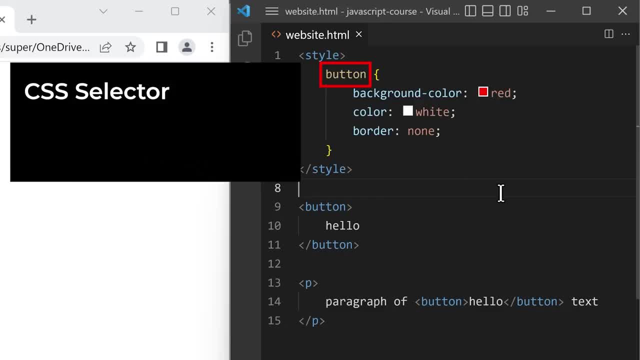 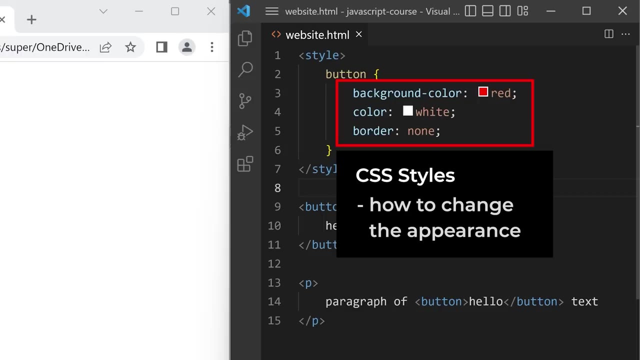 is called the CSS selector. It tells the computer which elements we want to change. In other words, it selects which elements to change. Inside the curly brackets we have some CSS styles. This tells the computer how to change the appearance For each style. the left. 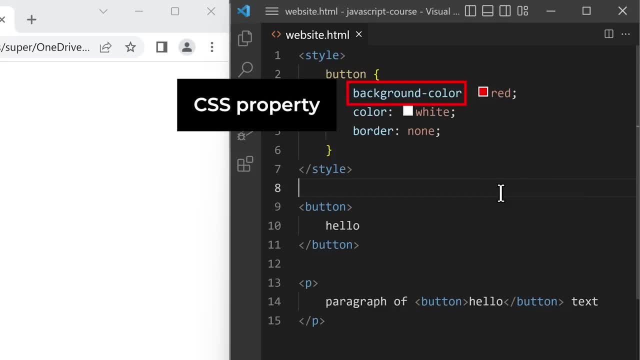 side is called the CSS property. This tells the computer what we're changing. The right side is called the CSS value. This tells the computer what we're changing the property to. For example, this style changes the background color to red. We use a colon. 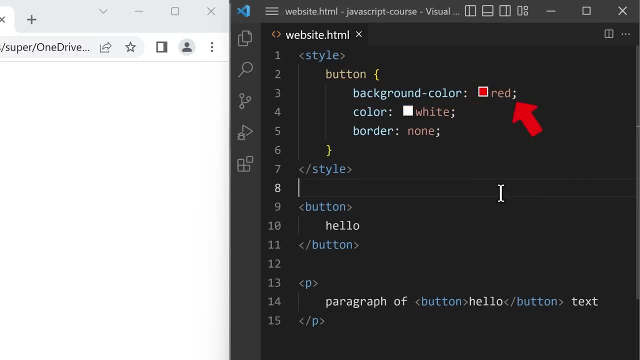 to separate the property and the value, and a semicolon at the end to tell the computer that this is the end of a style. So that's the basic syntax of CSS. We tell the computer which elements we want to change and then how to change. 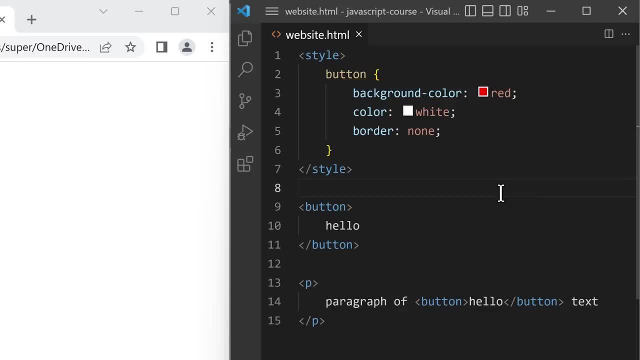 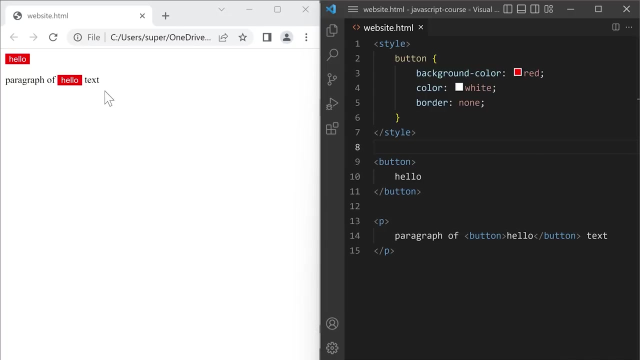 the appearance of these elements. The next thing we're going to review is HTML attributes. Right now, this CSS selector changes the appearance of all buttons on the page. However, what if we only want to change the appearance of this one button and we want to style the other button? 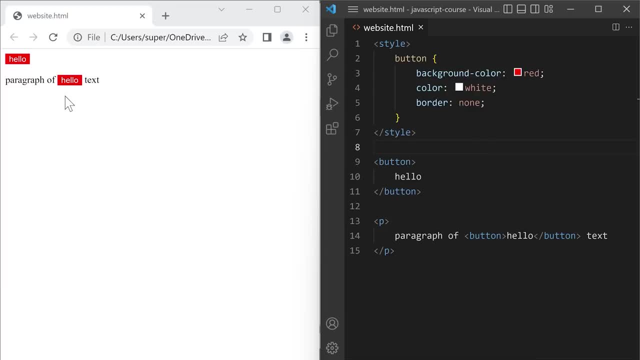 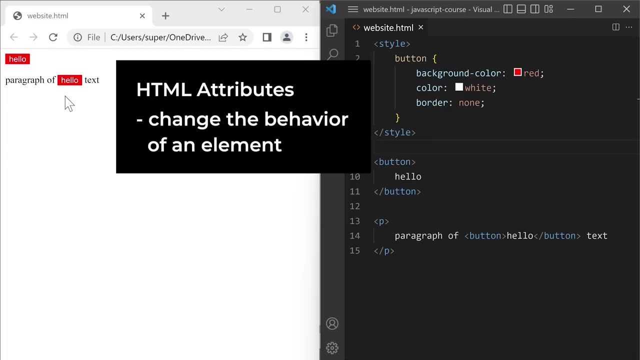 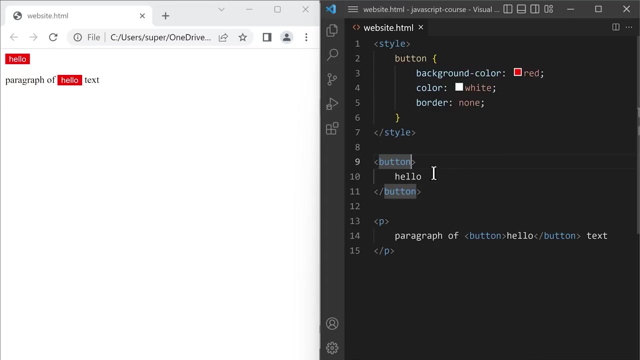 differently. How do we do that? We're going to review a feature of HTML called attributes. Attributes change the behavior of an element. For example, we're going to go to the opening tag of the first button and then here we're going to add an HTML attribute. 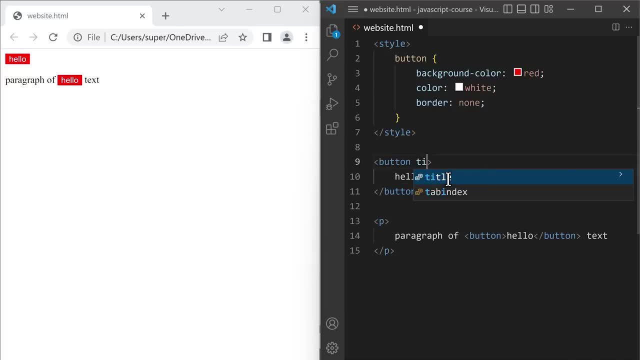 by typing space. title equals double quotes and then in between the double quotes we're going to type tooltip. so this is an HTML attribute and this attribute adds a tooltip to this button. If you're wondering what a tooltip is if we hover over some code in our code editor. 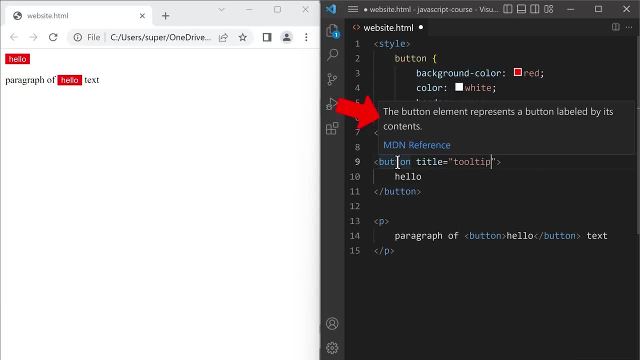 it'll show us this sort of popup with more information. This is called a tooltip: when we hover over something and this shows up. So if we save our file and refresh the webpage, and now we hover over our button, we can see that the HTML attribute added. 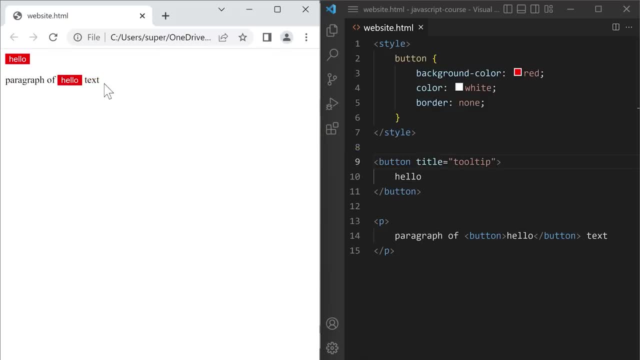 a tooltip to our button and then inside the double quotes is the text inside the tooltip. For example, we can actually change this to good job and if we save and refresh and hover over our button, the text between the double quotes is what shows up in our tooltip. 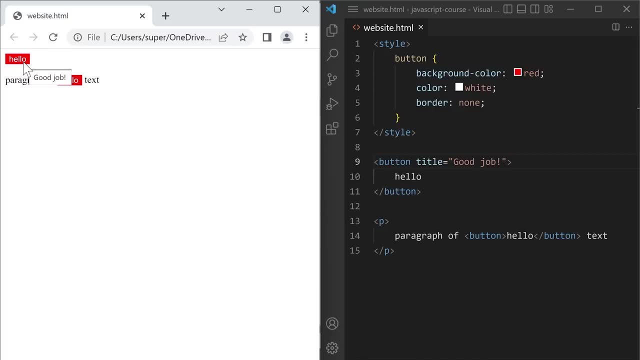 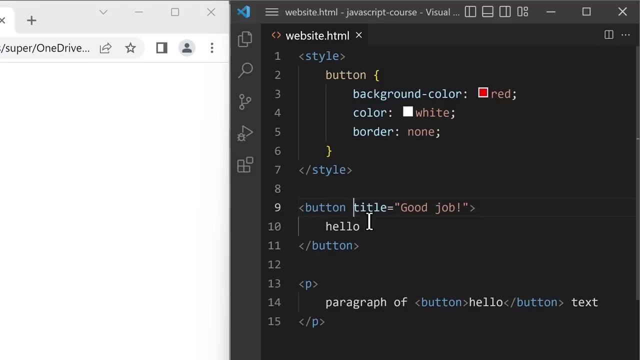 So that's an example of an HTML attribute. Now let's review the syntax rules for attributes. We always put attributes on the opening tag and we add a space between the element name and the attribute to separate them. On the left side is the attribute. 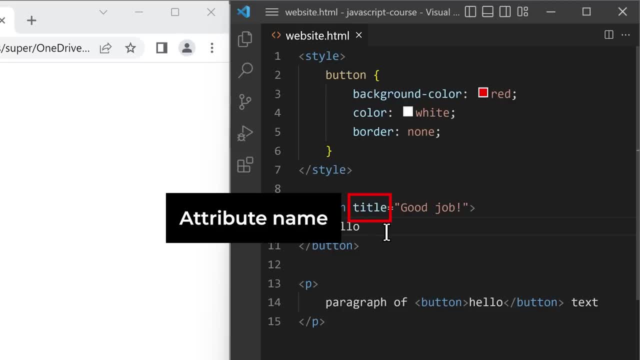 name. This tells the computer what we're changing about this element On the right side is the attribute value. This tells the computer what we're changing this attribute to. For example, here we're changing the tooltip of this element to good job. 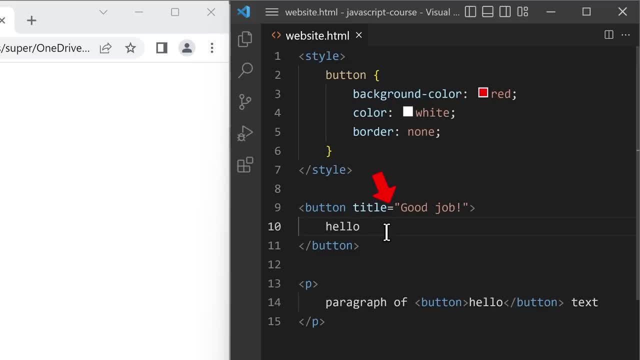 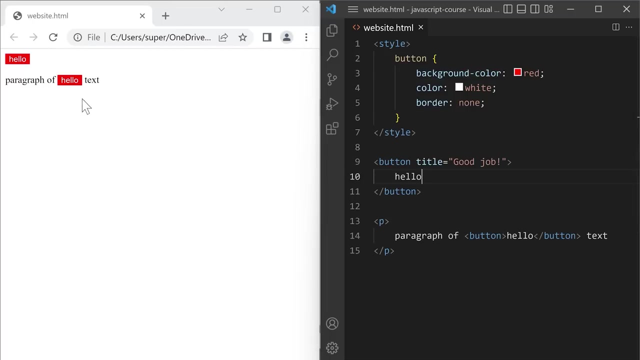 We separate the name and value with an equal sign and make sure there are no spaces around the equal sign, And we surround the value with double quotes. Now let's go back to the original problem. How do we style these buttons differently? We can do this using 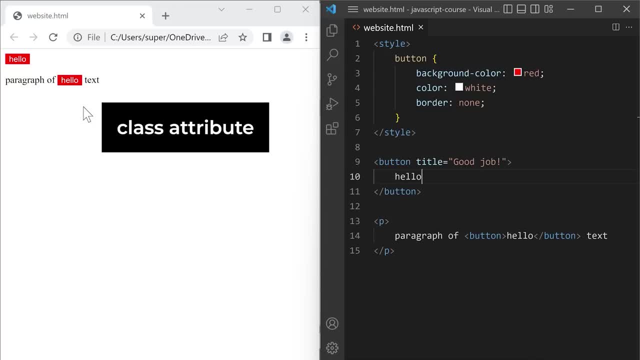 a very important attribute called the class attribute. Let's review that right now. We're going to go back to our button and then here we're going to type space class equals double quotes and then inside the double quotes we're going to type red dash. 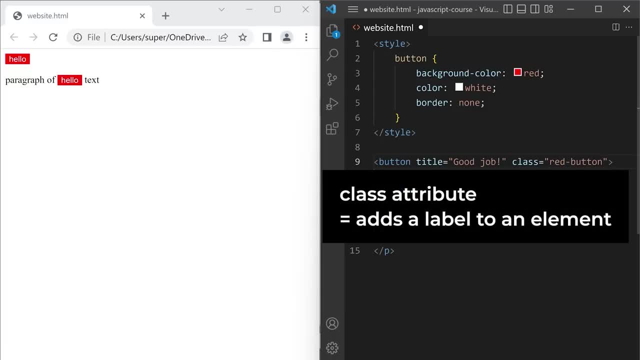 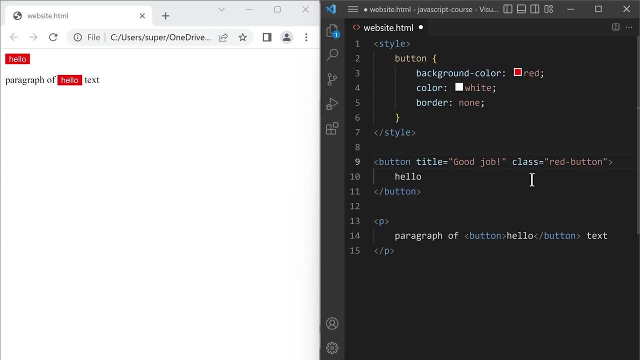 button. So the class attribute sort of adds a label to an element. So here we labeled this button as a red button And now that we labeled this element, we can select it in CSS. To do that, we're going to go to our CSS. 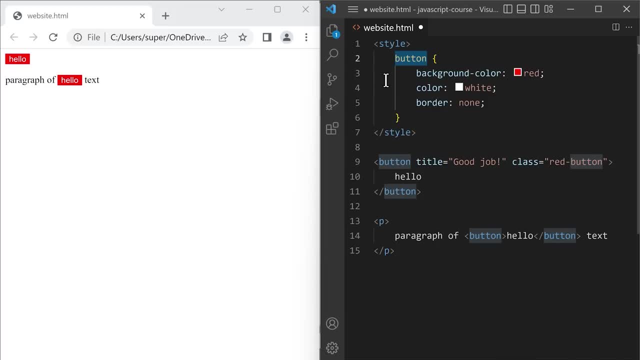 code. We're going to remove the button selector and replace it with dot red dash button. When we start the selector with a dot, this means that now we're looking for a class. So here we're going to look for all elements with the class red. 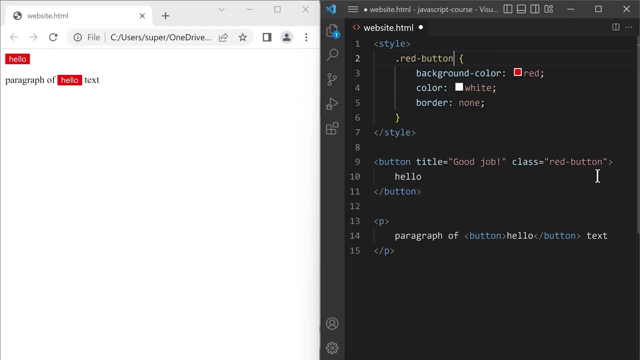 dash button, which is only this element. If we save and refresh now only the elements with the class red button gets these styles. We can also add the same class to multiple elements. For example, we can go to our other button and add the class. 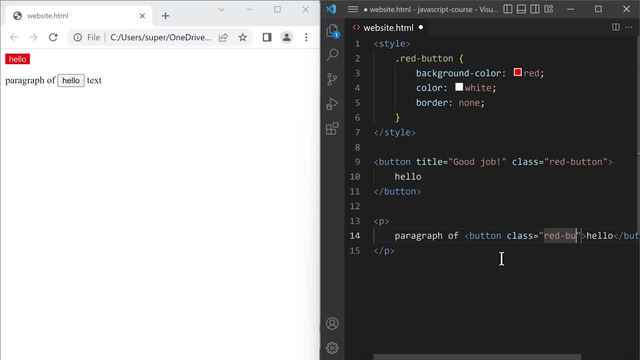 equals red dash button. If we save and refresh now, these styles get applied to both buttons again, because they both have the class red dash button. If we want to style this button differently, we just give it a different class. For example, we can: 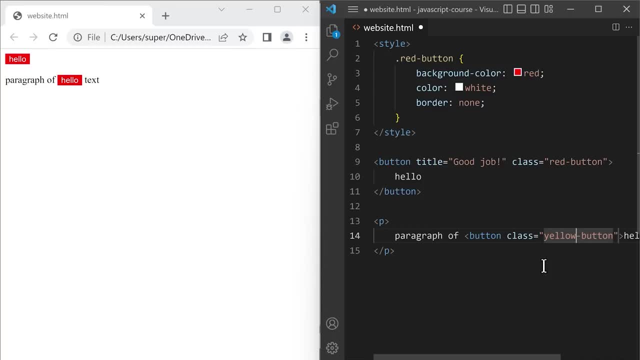 change this to yellow dash button And then in our CSS we can add another selector So we can type: dot. this means we're going to select a class and we're going to select the yellow dash button class. Open curly bracket. close curly bracket. 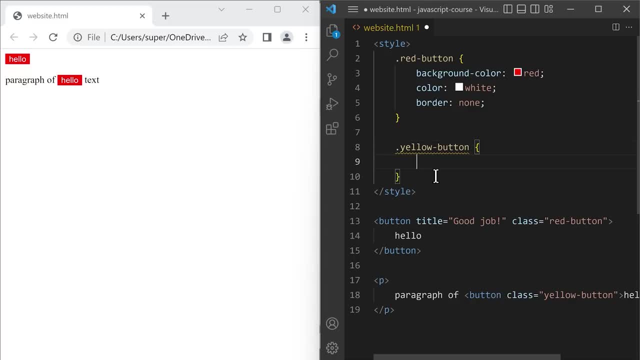 And then inside here we can add some styles for the yellow button, For example background, dash, color, colon, yellow and semicolon. Now let's save and refresh, And that's how we use the class attribute in HTML to modify specific elements. The final thing we need to review: 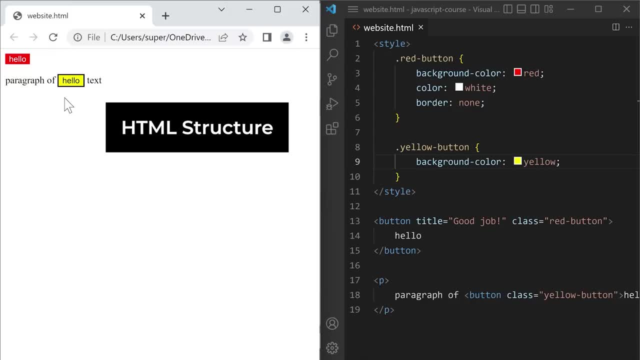 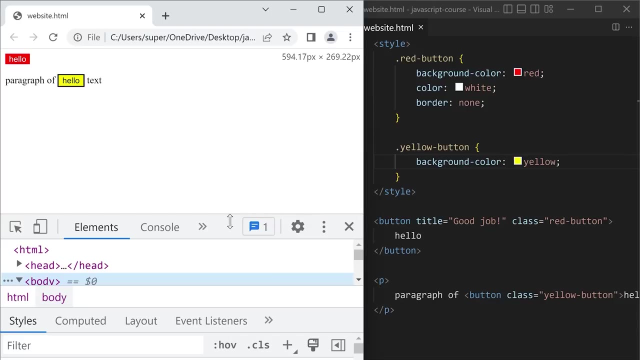 is something called the HTML structure. Let's go back to our website. We're going to find a blank area and then right click and then click inspect. So we already learned about the console tab. Here we can write and run JavaScript code. Now we're going to go to. 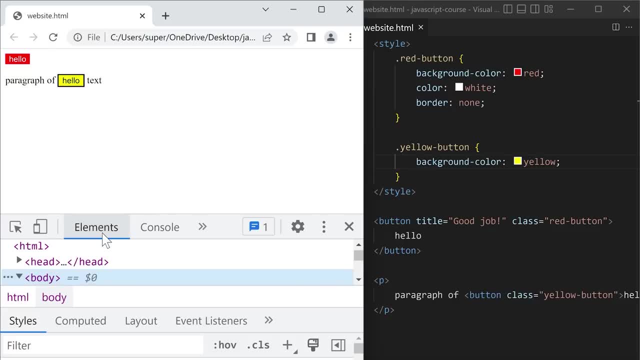 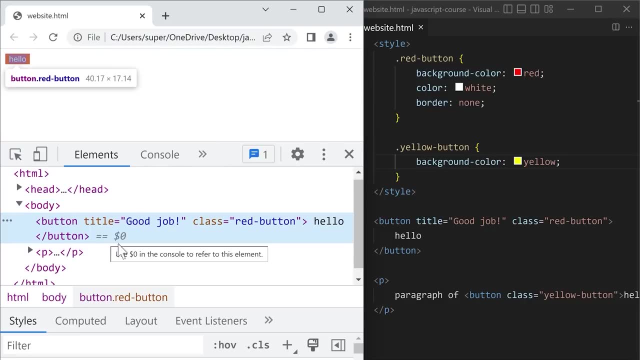 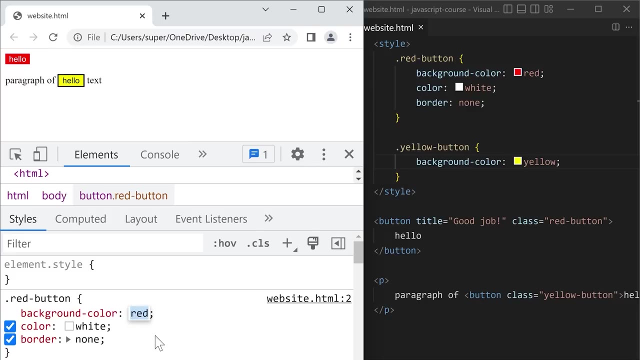 the elements tab, which is for HTML and CSS. So in the elements tab we can see all the HTML on the page as well as all the CSS on the page, And we can play around with the CSS if we want. Now, if we go back to the HTML, 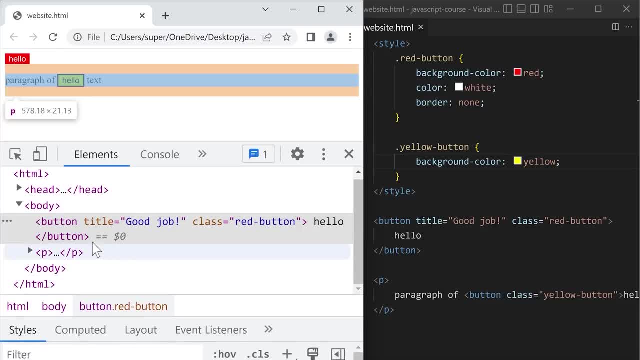 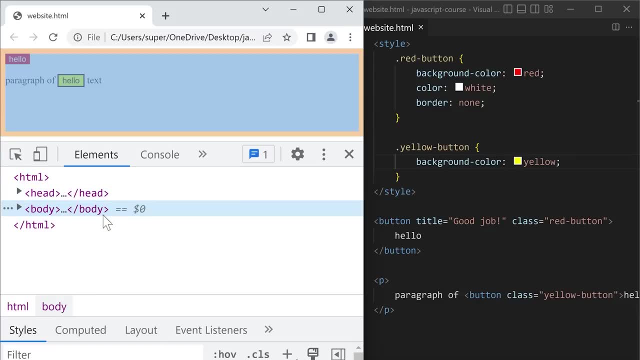 you'll notice that our webpage has some elements that we didn't add before: The HTML element, the head element and the body element. So this is the structure that we're supposed to follow when writing HTML In our code. we didn't. 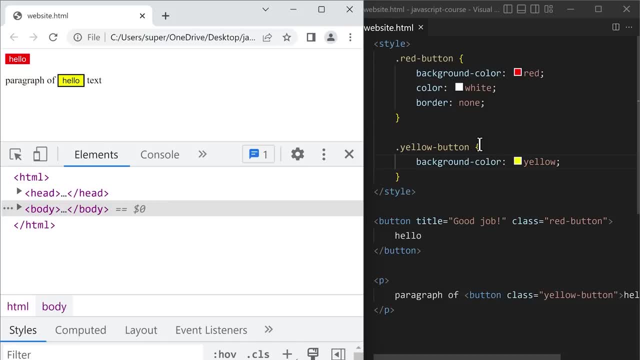 follow this structure, so the browser actually adds it for us automatically. However, it's still best practice to follow this structure in our code, because it gives us access to some more features of HTML. Let's review the HTML structure and add it to our code. 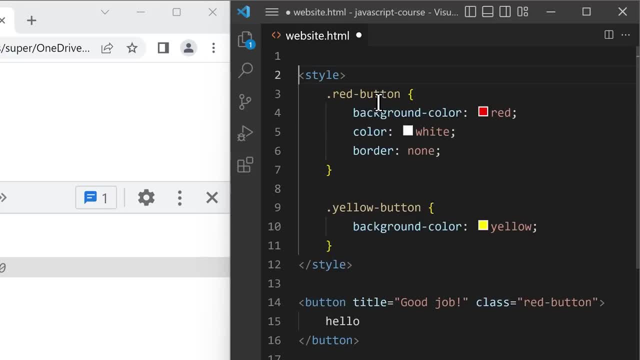 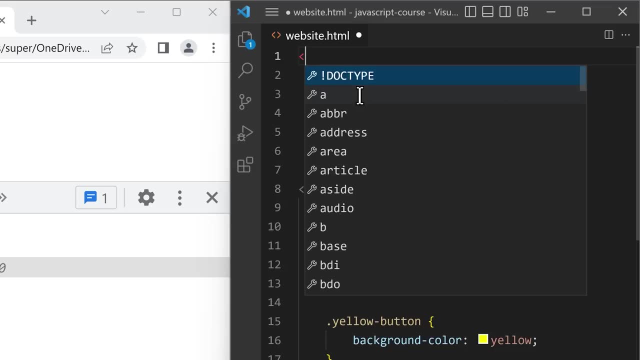 We're going to type up here and we're going to create some new lines, And now every HTML file is going to start with less than exclamation type in capitals and then space. HTML and greater than This is not an HTML element, It's a special line of code. 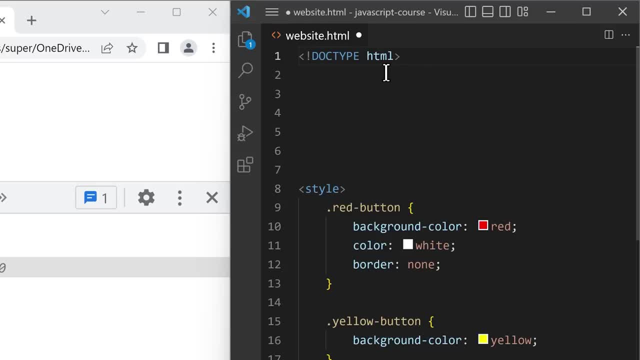 that tells the browser to use a modern version of HTML. If we don't have this, the browser might fall back to an older version of HTML that has less features. Next, we're going to create an HTML element, So less than HTML and greater than. 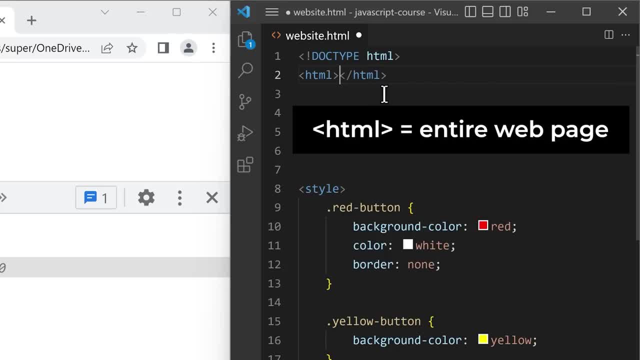 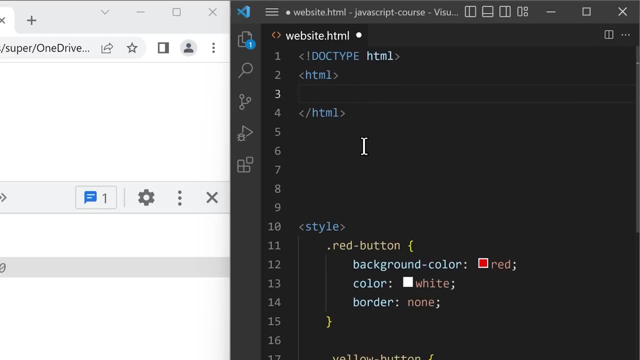 The HTML element represents the entire webpage, So everything on the webpage should go inside this element And then inside the HTML element. we're also going to split it up into two sections: The head element and the body element. So the body element is supposed to contain everything. 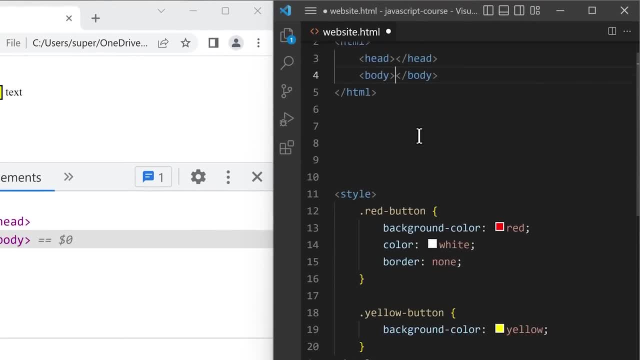 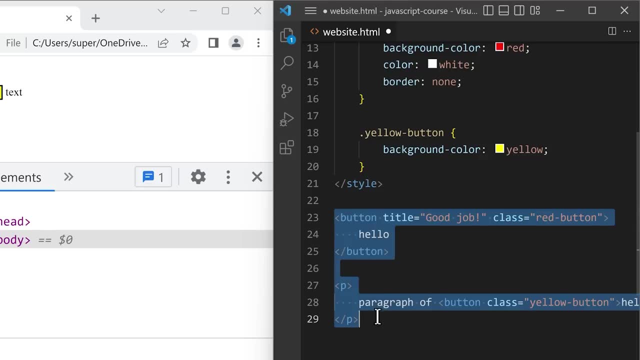 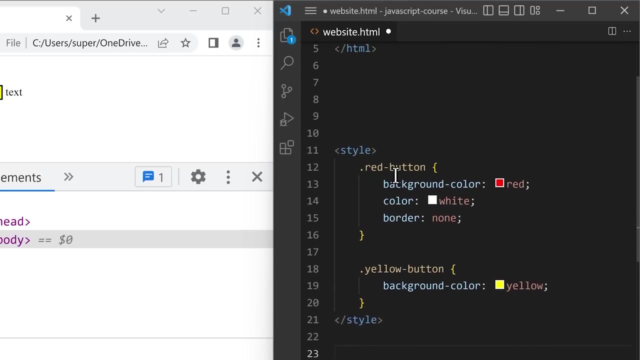 that is visible on the page. In our example, that would be the buttons and the paragraph. So let's actually select this code and we're going to right click and cut, and then, inside the body, we're going to right click and paste The head element. 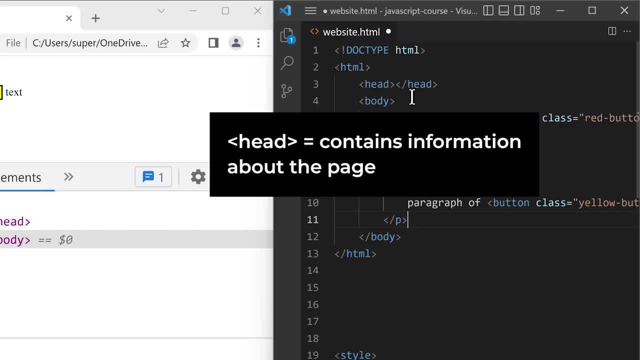 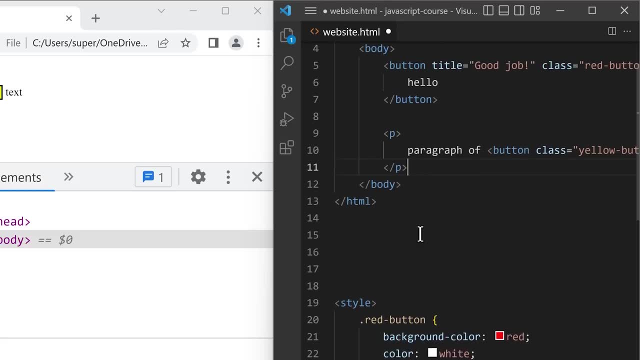 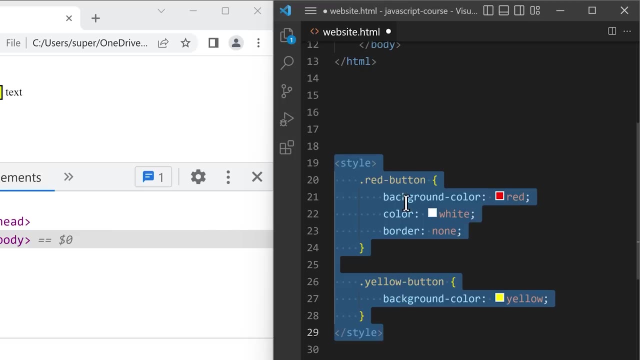 contains information about the page In general. everything that is not visible on the page goes inside the head. In our example, that would be the style element, So let's select this as well. We're going to right click and cut and then inside the head. 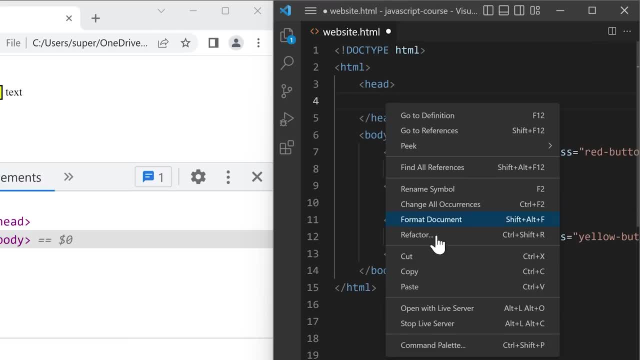 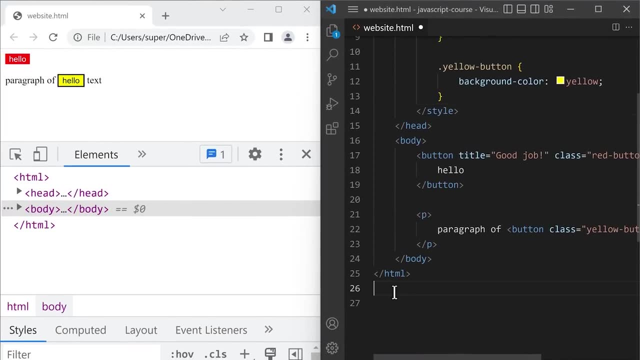 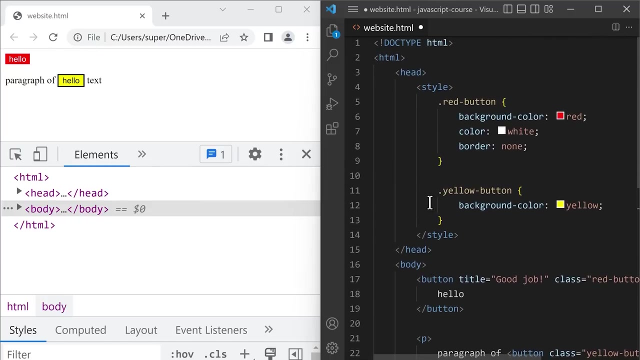 element, we're going to right click and paste And at the bottom, let's just clean up by removing all of the extra new lines. So this is a structure that we're supposed to follow in all of our HTML files, As you can. 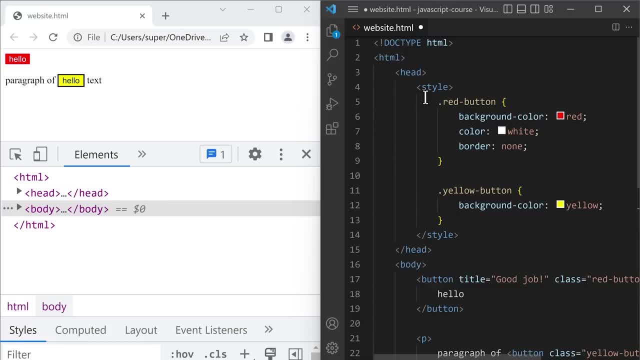 see, this structure uses a lot of nesting, or elements inside elements, to organize our code. Okay, so what are the benefits of following this structure? One benefit is that there are other elements that we can use inside the head. For example, let's type here: 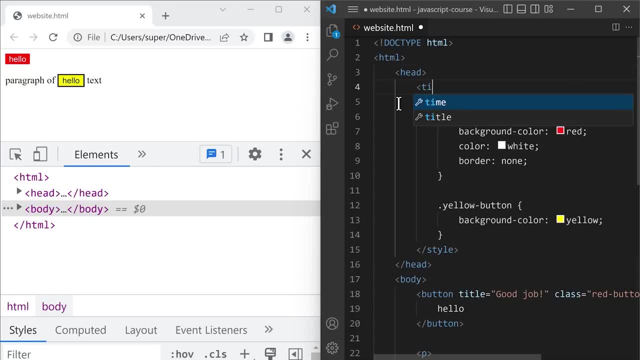 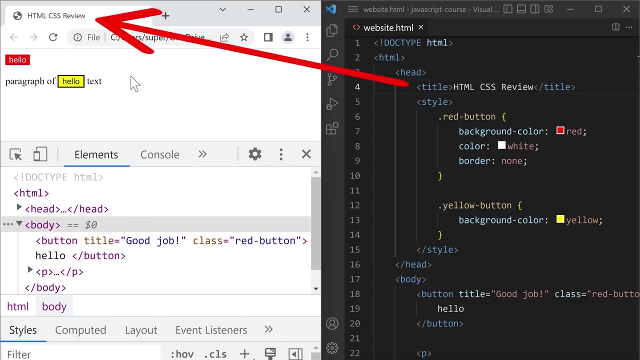 press enter and we're going to add the title element. So the title element sets the text in the tabs. Inside we can type HTML CSS review. If we save and refresh, the title will show up in the tab. So this is an example. 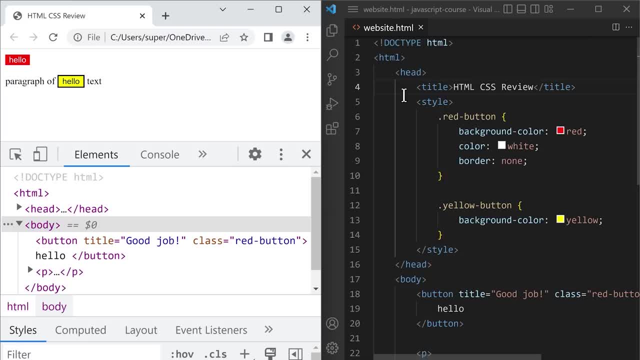 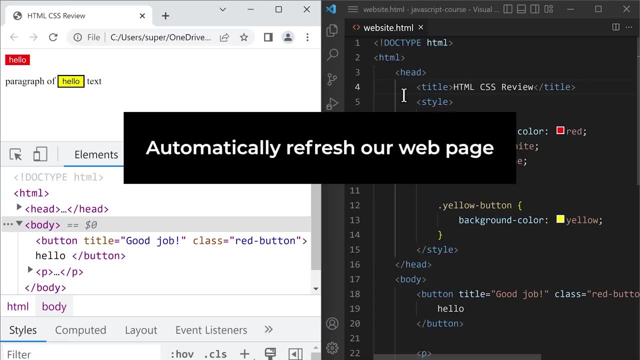 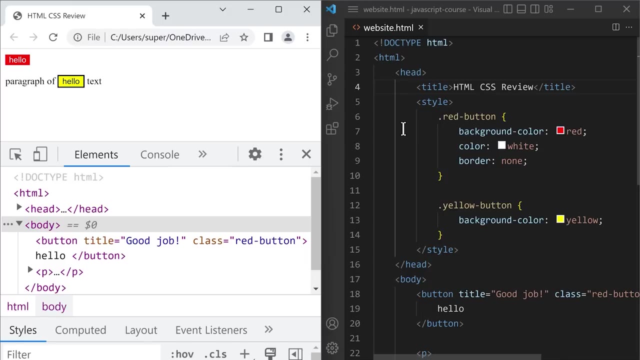 of an element that we can now add in the head. Another benefit that we get from this structure is the ability to automatically refresh our webpage when we change our code. So far, every time we change our code, we have to save and then manually. 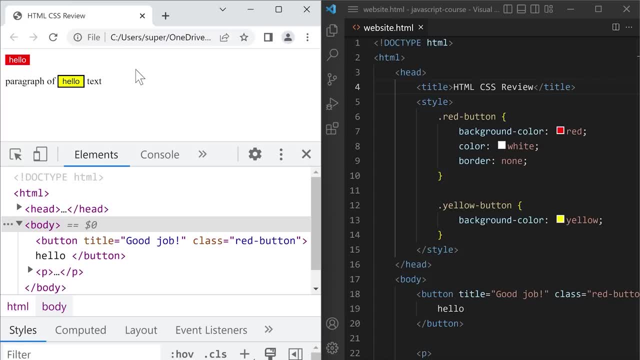 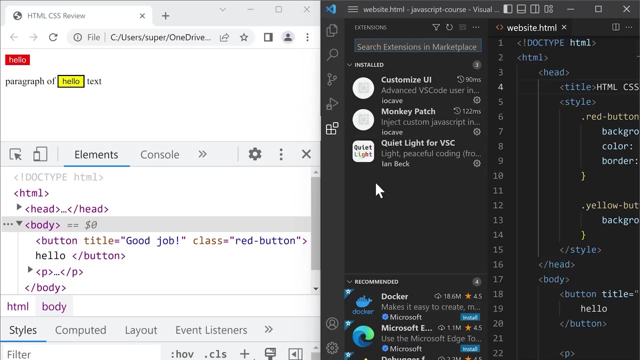 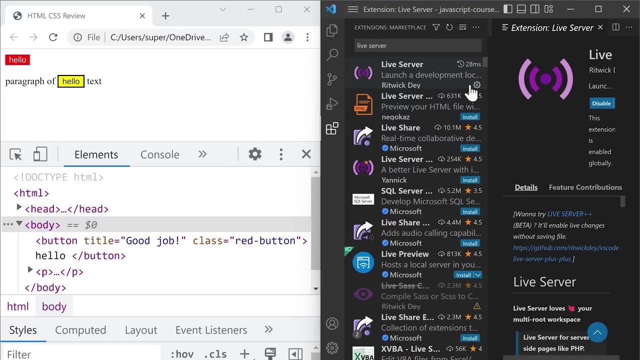 refresh the webpage. We can actually automate this by following the structure and then installing a VS Code extension. So let's click the extension area and we're going to search for the extension live server and click install. Once we have that installed, we're going to change a setting. 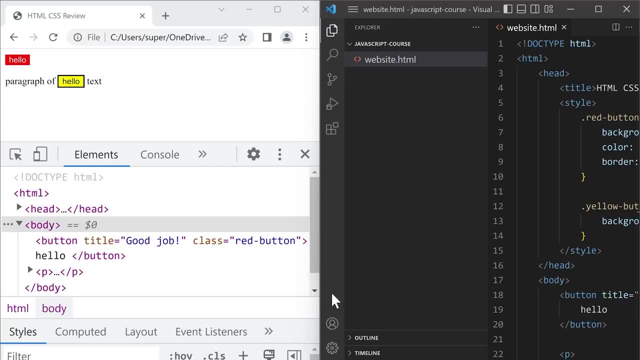 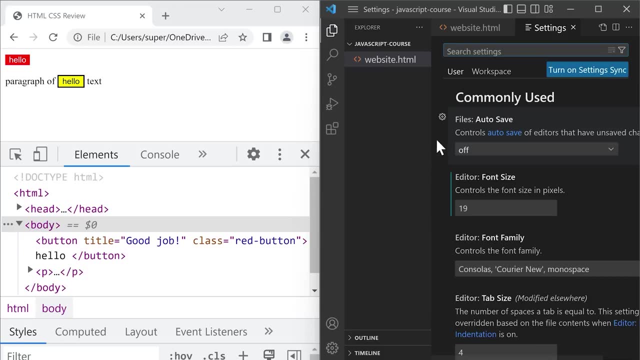 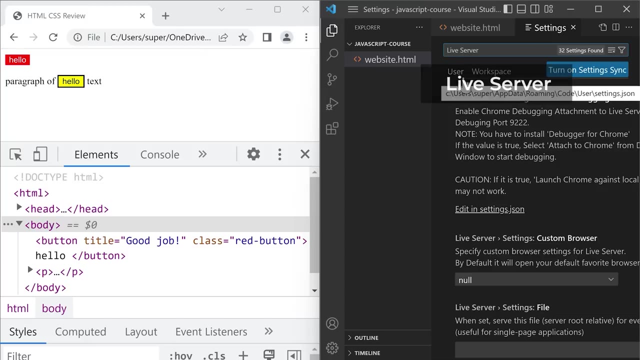 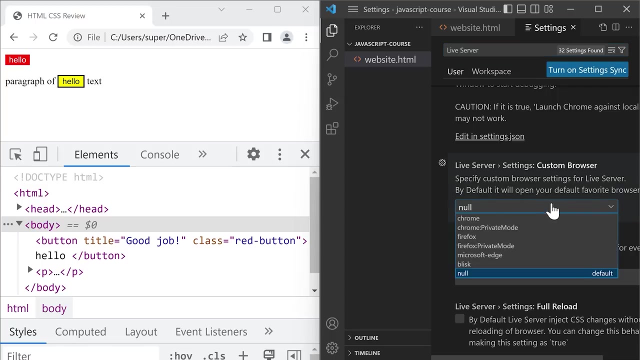 Let's open the settings by clicking this icon in the bottom left and then click settings At the top. we're going to search for live server And we're going to look for a setting called live server custom browser, And we're going to change this to Chrome. 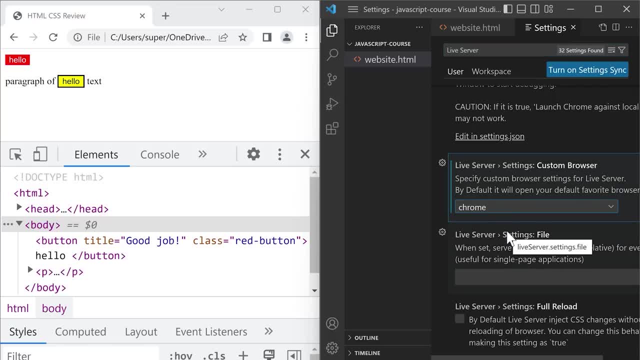 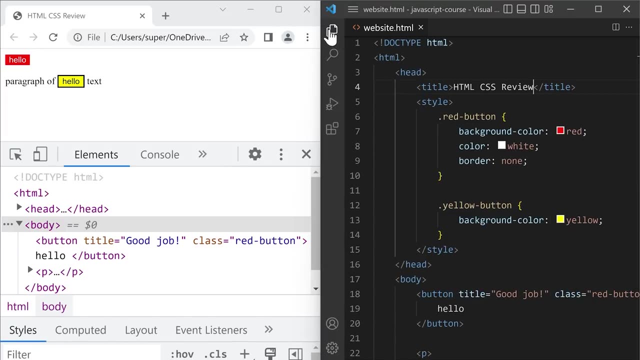 Now, if Google Chrome is already your default web browser, you don't need to do this step, but it's nice to know. Now let's close the settings and go back to our code Next, instead of opening this file directly in the browser, like before, 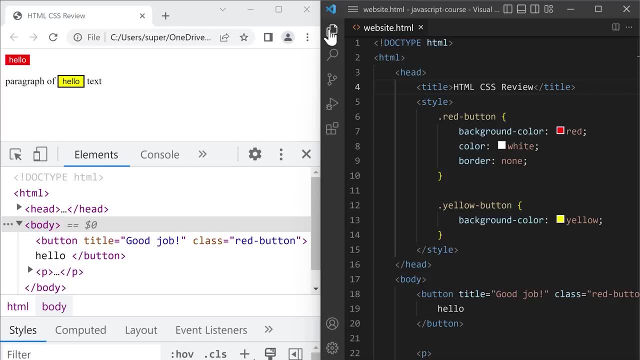 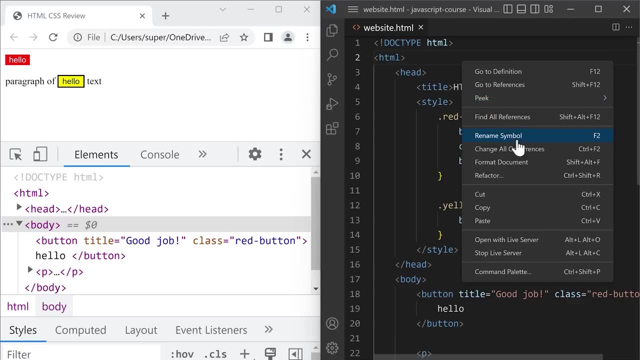 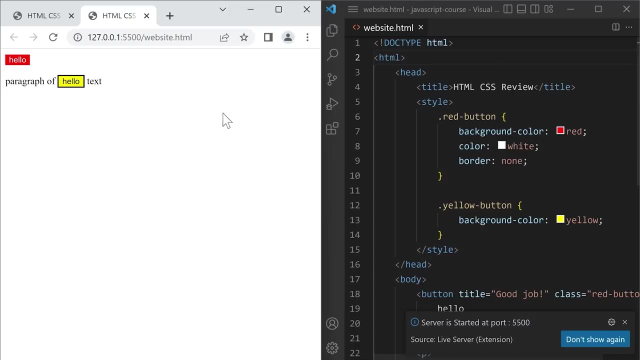 we're going to use live server to open this file. To do that, we're going to right click this file in our code editor and then click open with live server. If we open a file with live server, this web page will automatically refresh. 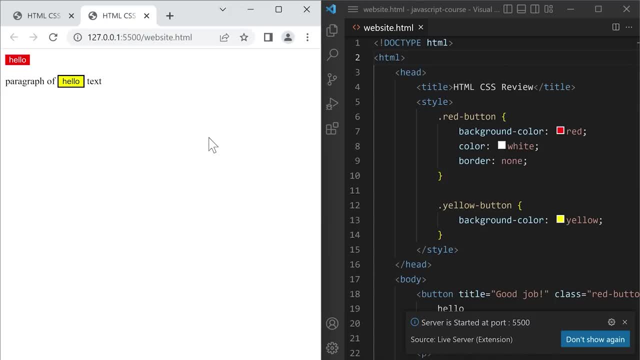 when we change our code. For example, we can go here and change the background color to green. If we save, live server will automatically refresh the web page. So we don't have to do that back and forth anymore. Let's just change it back to red. 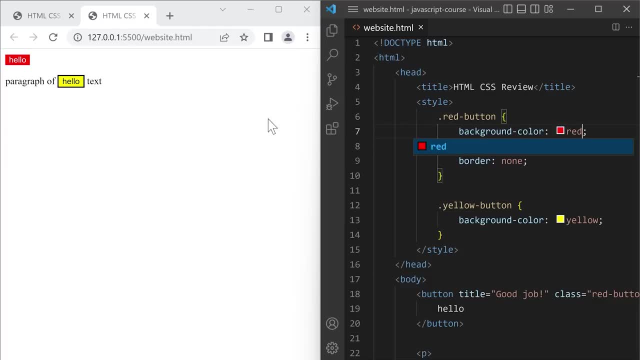 so that the class name makes sense, And save And we can also close the previous tab. So this is the HTML structure. It gives us access to more features of HTML And this is all we need to review about HTML and CSS for now. 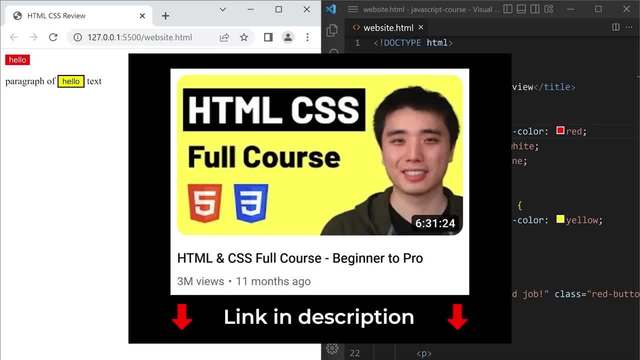 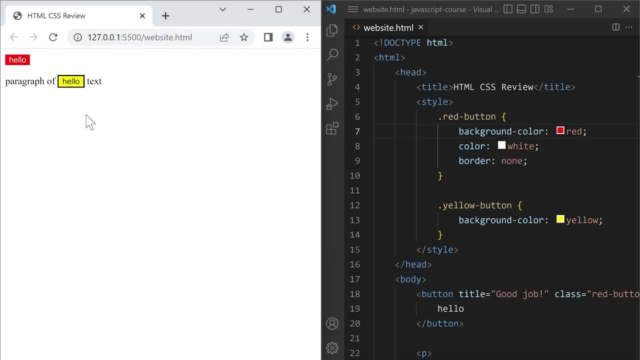 If you want to learn more, you can check out my HTML and CSS full course in the video description. Before we add JavaScript to our website, we're going to review some VS code setup, So you'll notice that many of these lines have spaces at the front. 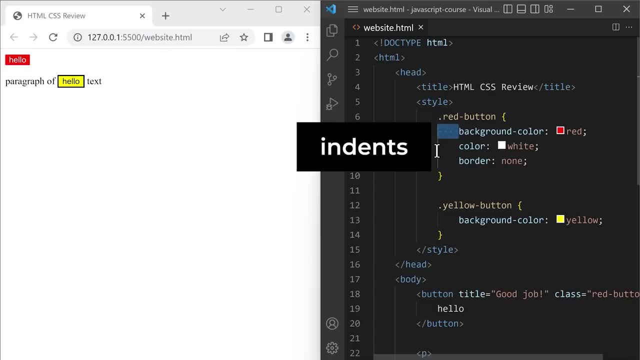 These spaces are called indents, And indents make our code easier to read. For example, we can easily tell that this code is inside the brackets because it has an extra indent in the front. If we didn't have indents, here's what the code would look like. 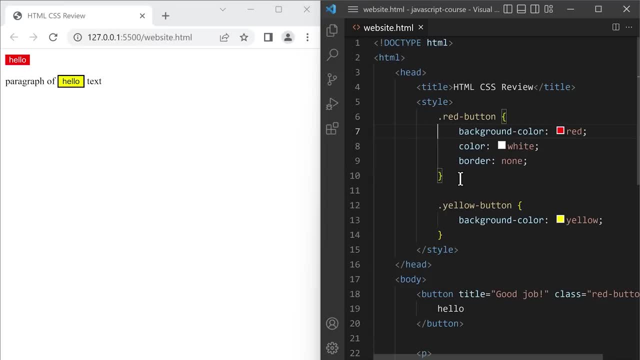 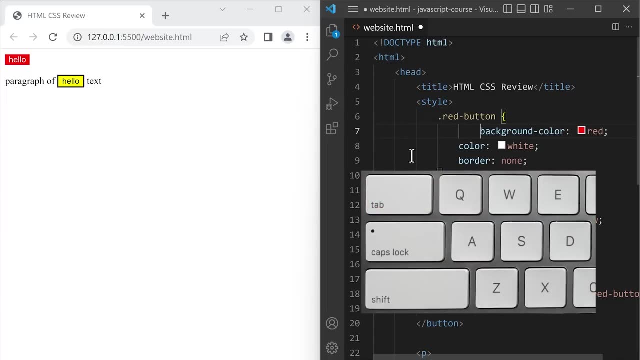 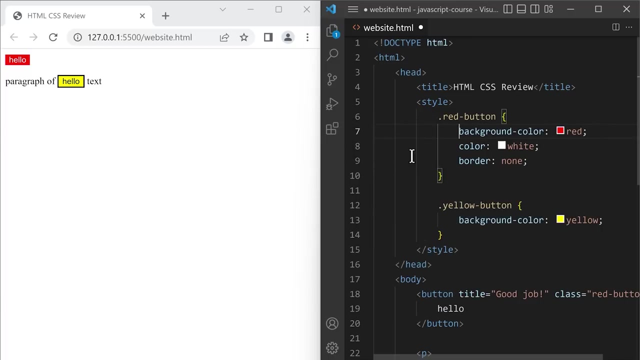 It's a lot harder to read. To add an indent, we can type at the beginning of the line and press tab. To remove an indent, we can press shift tab or just use backspace. Now, by default, VS code uses four spaces per indent. 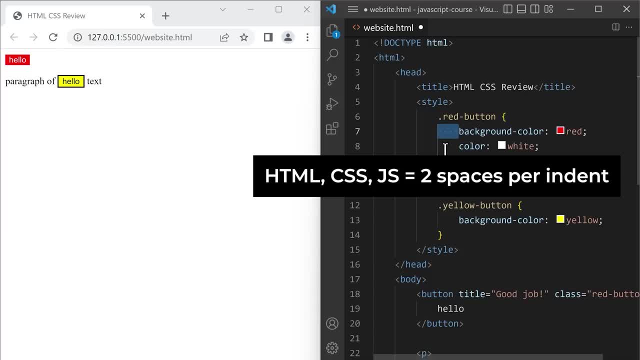 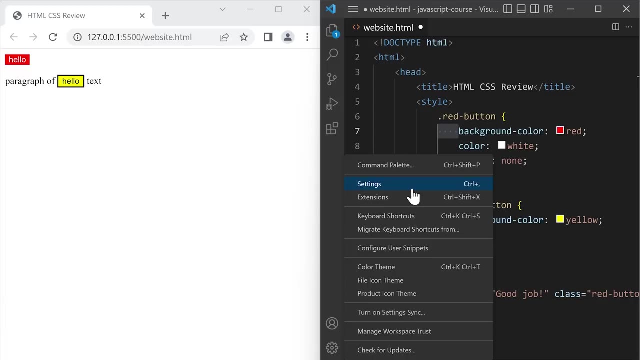 However, in HTML, CSS and JavaScript we usually use two spaces per indent, So we're going to update this setting. Let's go to our settings by clicking this icon in the bottom left and then click settings And at the top. 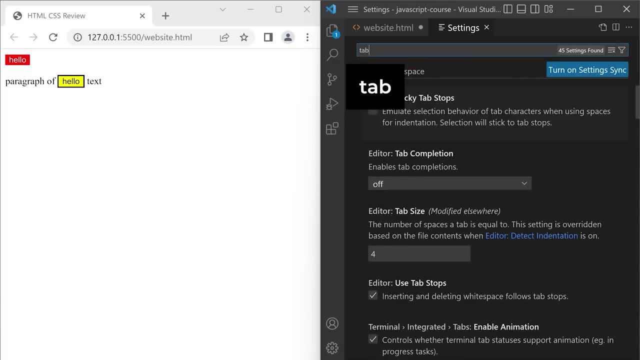 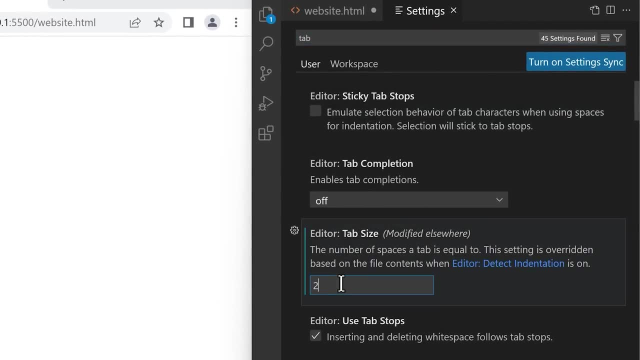 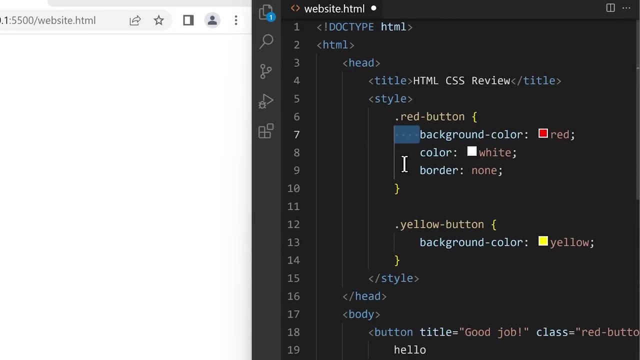 we're going to search for tab And we're going to change the tab size from 4 to 2.. Now let's close the settings and we're also going to change the indents for this file. We're going to go down here and click. 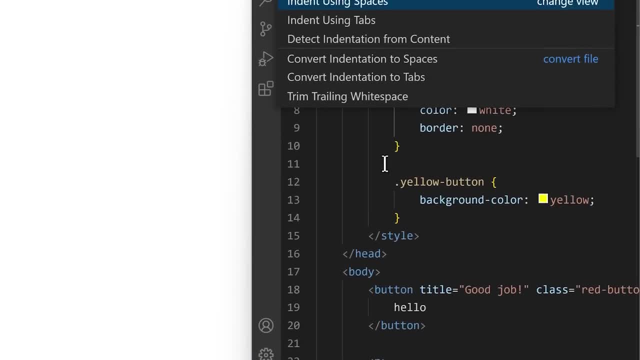 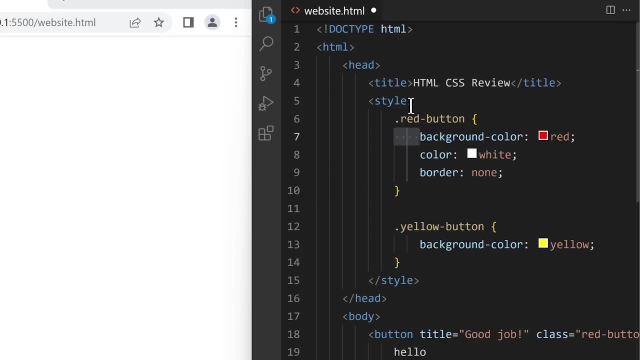 select indent And we're going to choose indent using spaces and then click 2.. And now, if we type at the start of a line and press tab, it will only add two spaces per indent. So let's reformat our code to use two spaces. 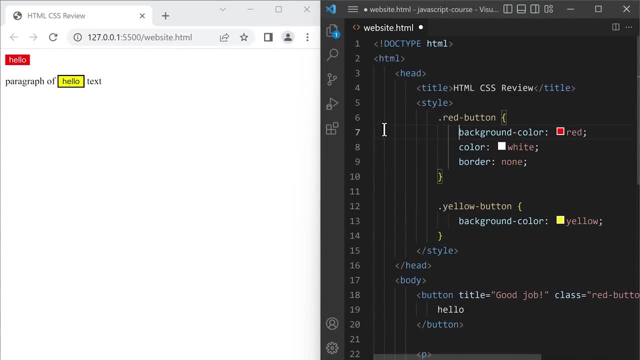 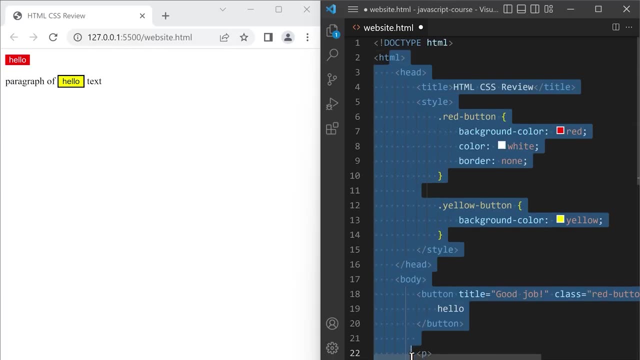 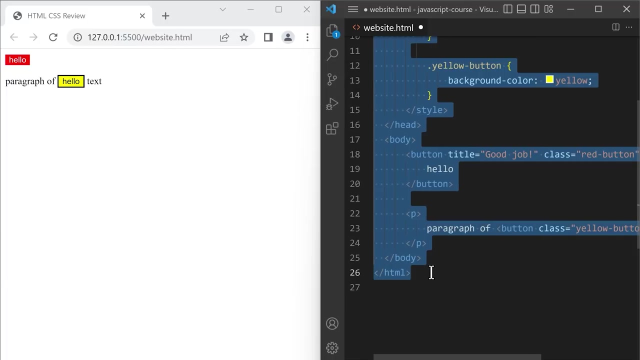 per indent instead of four. First, we're going to remove all the indents in our code. A shortcut for this is to select all of these lines and press shift tab to remove one indent for each line. So we're going to keep pressing. 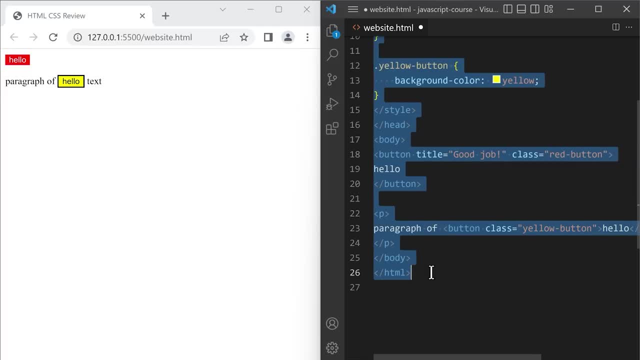 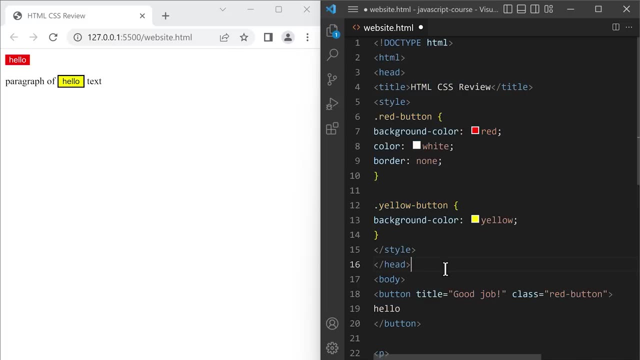 shift tab until we remove all the indents. Next, we're going to add the indents back using a similar shortcut. We're going to select the head element and press tab to add one indent for each line and then select everything inside the head. 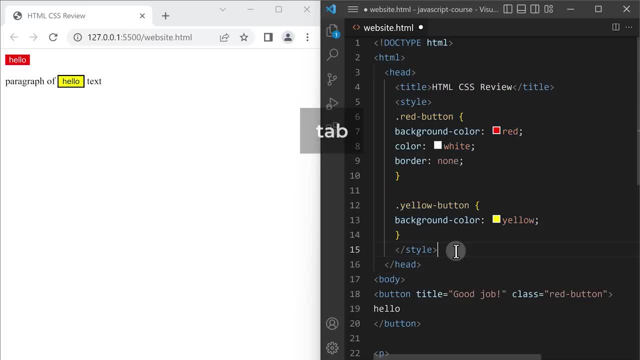 and press tab to add another indent, And then select everything inside style and press tab and then inside each of these brackets we're going to select the lines, press tab and then here, press tab. We'll do the same thing for the body element. 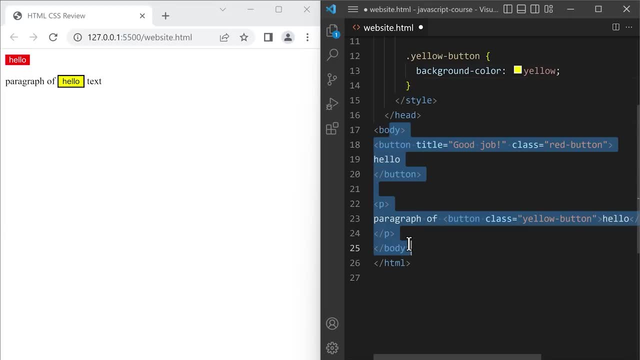 We'll select all these lines and press tab, select everything inside the body, press tab and then inside each of these elements we're going to press tab and press tab. Now, if we save, our website will look the same, because all we did was adjust the indents. 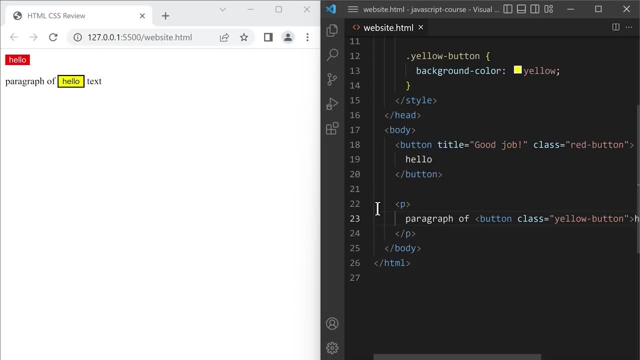 So there's one other setting in VS Code that we're going to set up, which is line wrapping. If you look at this line of code, you can see that it's really long and we need to scroll horizontally to see the rest of the line. 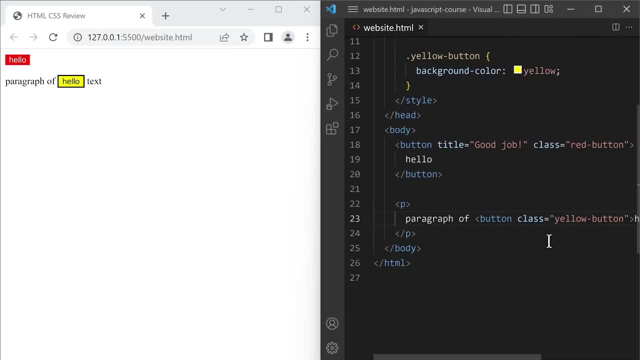 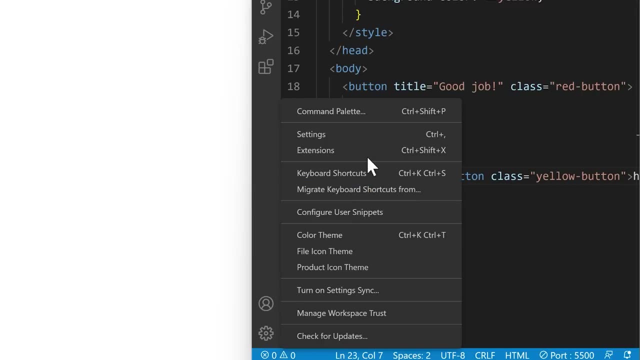 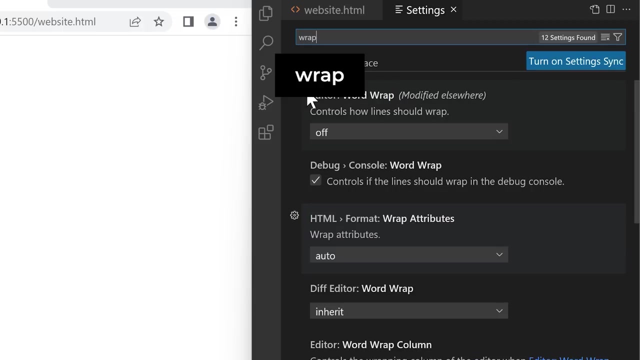 Instead we're going to make this line wrap around. if it gets too long, Let's go back into our settings by clicking here and then click the settings and then up here we're going to search for wrap and we're going to look for editor word wrap. 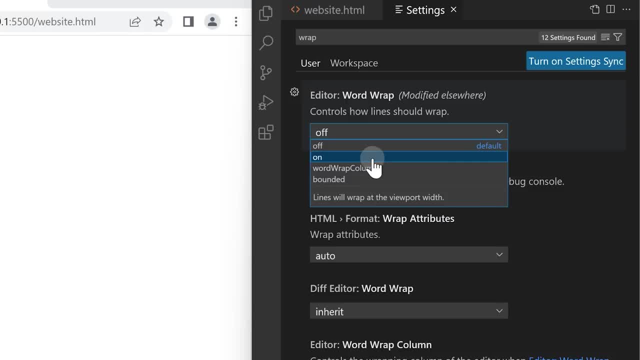 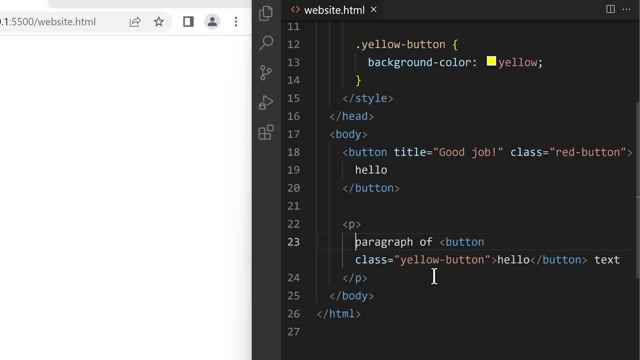 and we're going to turn this on Now. if we close our settings and go back to our code, this line, which is really long, will wrap around to the next line instead of us having to horizontally scroll. So that's the VS Code setup that we need. 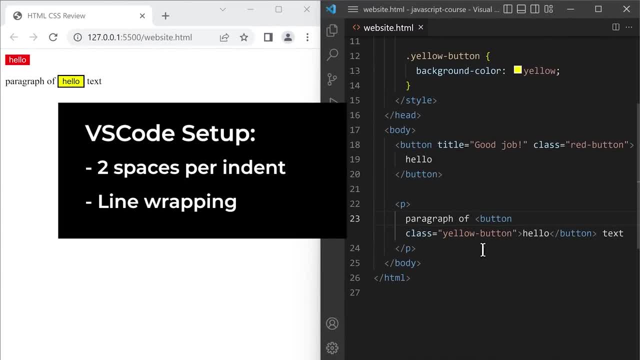 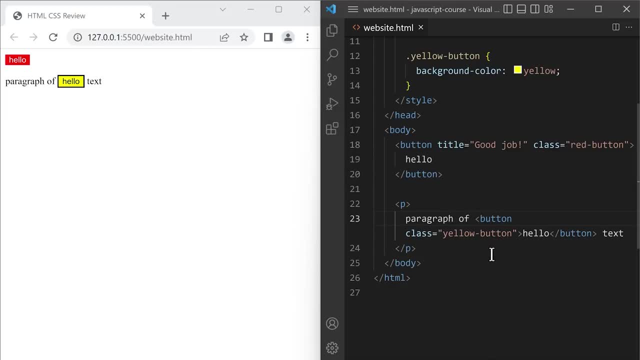 Two spaces per indent and line wrapping. Finally, we're going to add JavaScript to this website, So we learned that we can use the console to write and run JavaScript. Well, there's actually another way to run JavaScript, which is inside an HTML file. 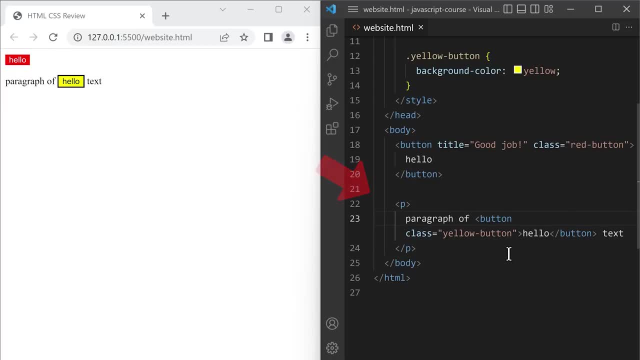 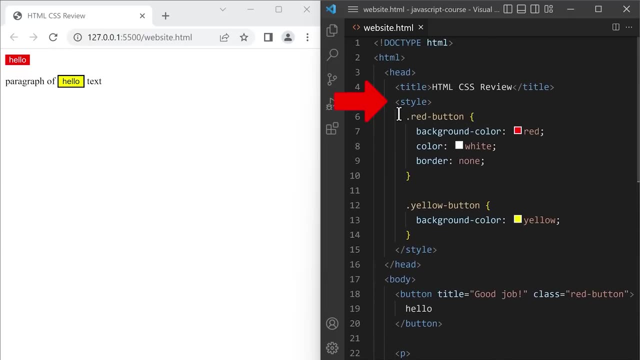 Let's learn how to do that. So we learned that HTML has a special element that runs CSS code, called the style element, while HTML has another special element that runs JavaScript code, and this element is called the script element. So inside our body, at the bottom, 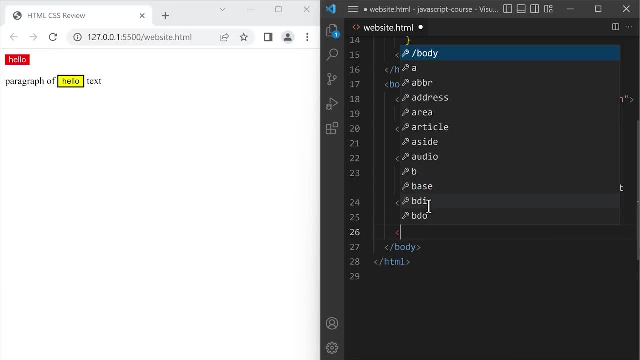 of the body. we're going to add script greater than and the closing tag less than. slash. script greater than, And. inside the script element we can put some JavaScript code. We're going to add the code alert. open bracket, quote- hello quote. close bracket and semicolon. 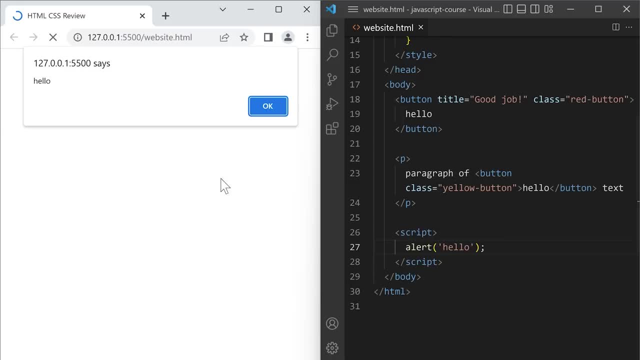 If we save, Live Server will refresh the page, and now you'll notice that the computer now runs our JavaScript code just like it did in the console. It creates a popup with the text hello inside, And we usually put the script element at the bottom of the body. 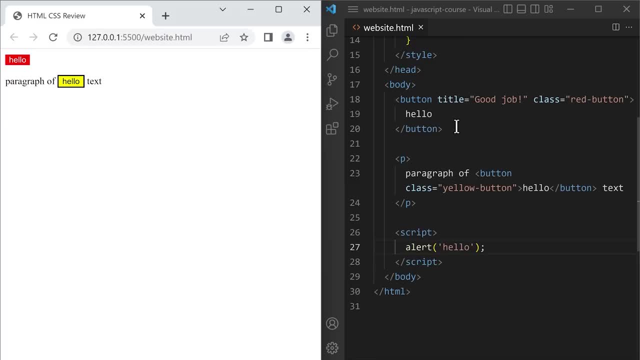 because we want the webpage to be created first, and then we use JavaScript to make it interactive. For the rest of this course, we're going to run our JavaScript code using an HTML file. The console that we used in the previous lessons is more of a way to try out. 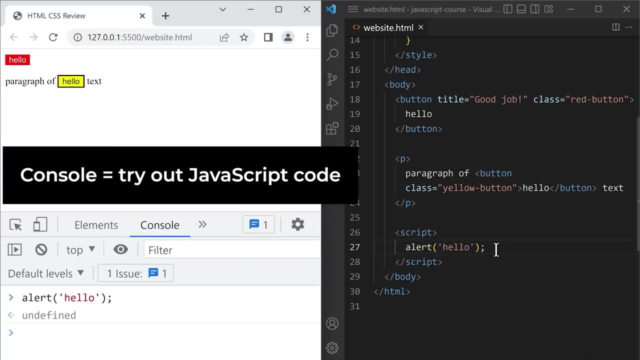 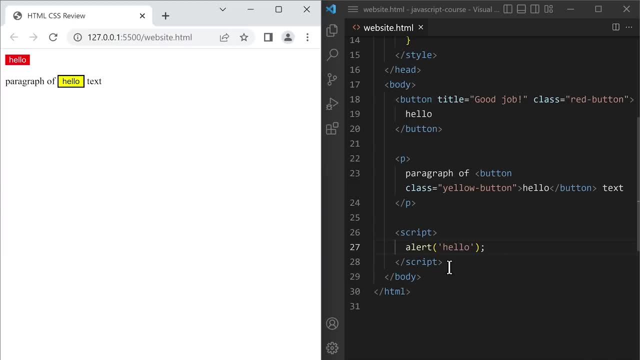 JavaScript code, We wouldn't use the console for a real website. In addition to the script element, we have another way to run JavaScript code inside HTML, And that's by using an attribute. Let's go back to our first button, and here we're going to add: 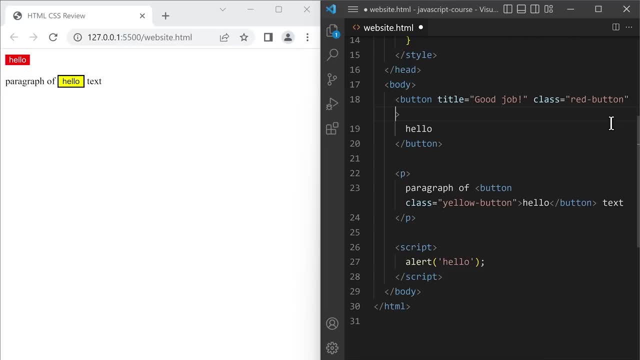 another attribute. We're going to type space and this time we're going to add the onClick attribute equals double quotes, So this attribute will run JavaScript code whenever we click this button. That's what onClick means. Between the double quotes, we can write some JavaScript. 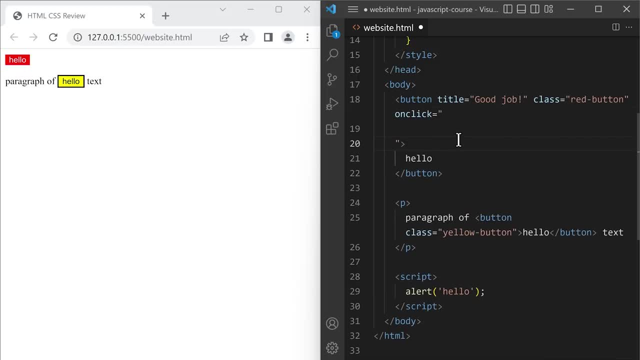 For example, let's press enter, enter. and then here we're going to type: alert- open bracket, quote, good job quote, close bracket and semicolon. Now, if we save, Live Server will refresh the page and run this line of JavaScript code. Let's press OK. 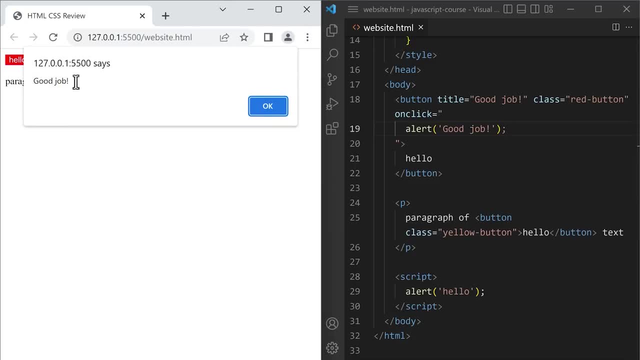 And now, if we click this button, it will run this line of JavaScript code and create a popup with the text good job inside. So those are two places where we can run JavaScript code: The script element and the onClick attribute. The code in the script element. 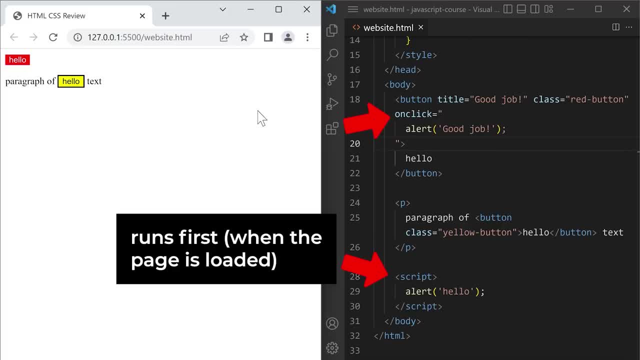 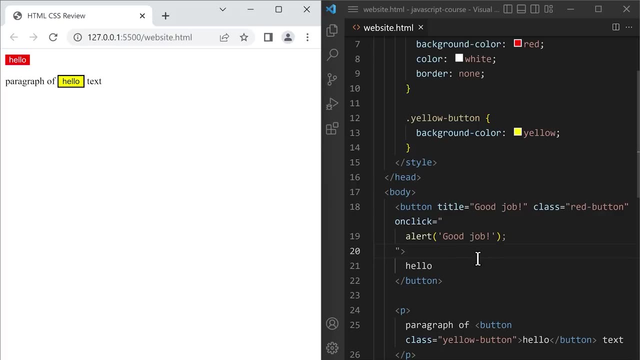 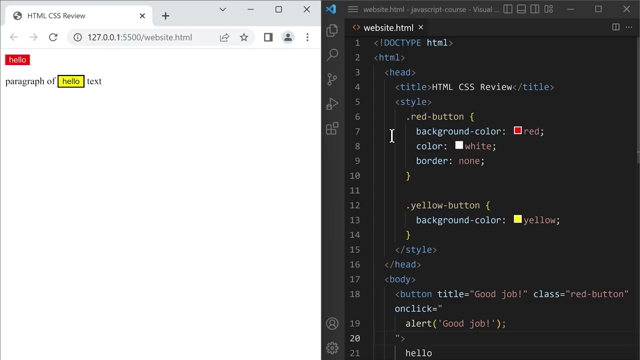 runs first when the page is loaded. The code in the onClick attribute runs after, when we click the button on the page. And that's how we use HTML, CSS and JavaScript together on a website. Notice that everything starts from HTML. HTML first creates the website. 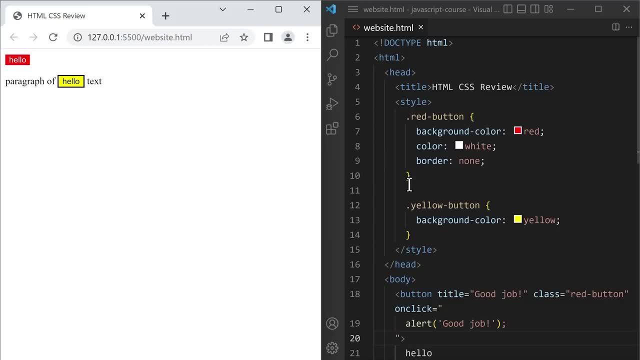 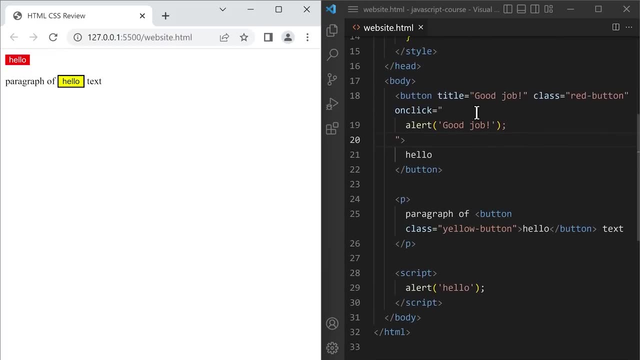 And then, inside the HTML, we can run CSS code to change the appearance and we can run JavaScript code to make the website interactive. Now let's learn some new features of JavaScript that we haven't seen yet in this course. The next feature we're gonna learn: 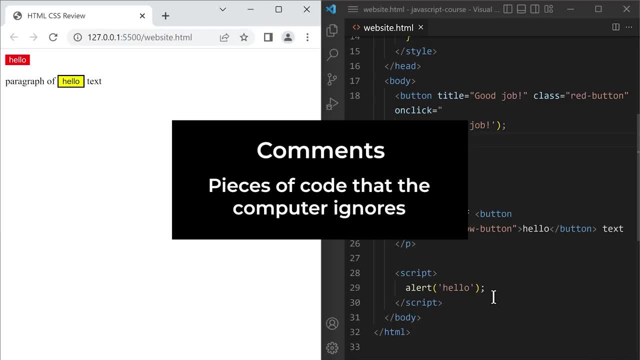 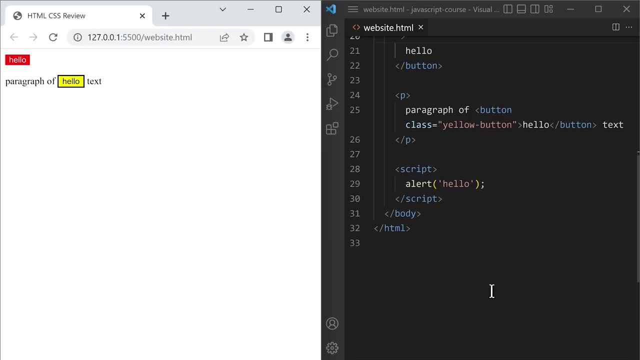 is called comments. Comments are pieces of code that the computer ignores. So let's create our first comment. We're gonna go down to the script element here and type forward slash, forward slash. So this is a comment. Anything after the double slash will be. 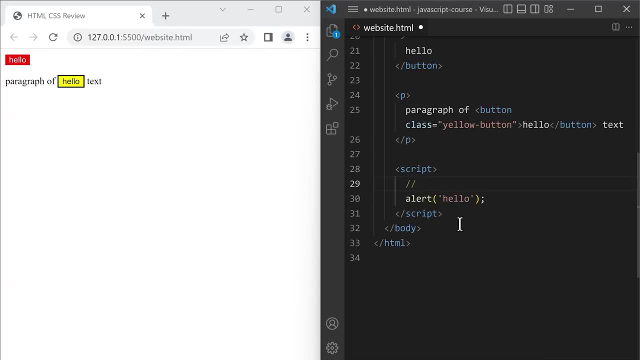 ignored by the computer So we can type anything we want, Like: this is a comment. If we save, it ignores this line and creates the popup in the next line. Now let's close this popup and learn why we use comments. Comments are useful for. 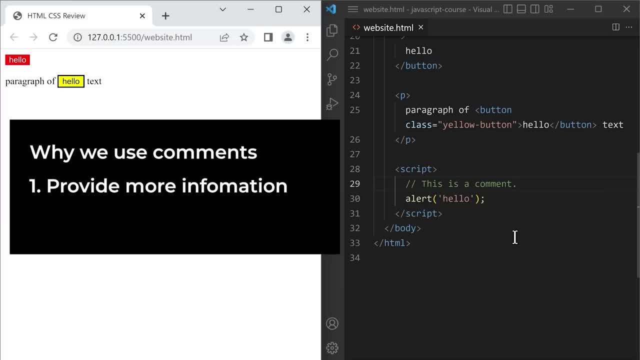 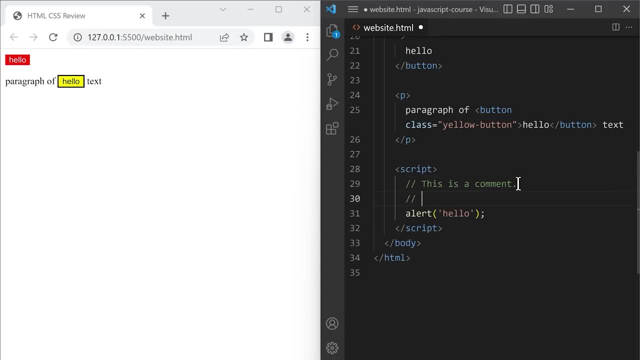 providing more information for people reading our code. For example, we can create a comment above this code. like This code creates a popup, This comment helps others and ourselves understand what this code does. So that's one way we use comments. Another way we use comments. 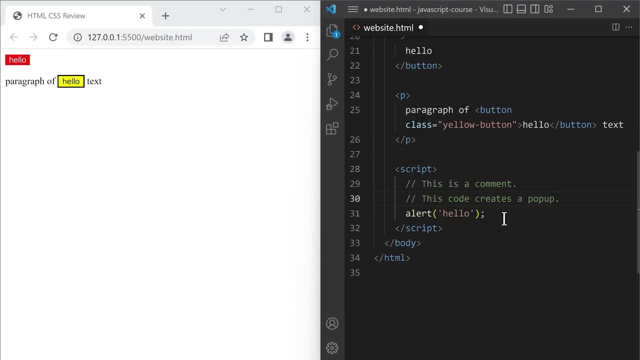 is if we don't want to run some code anymore, but we also don't want to delete it. For example, this code creates a popup every time we refresh the page, And this can be annoying. So I want to stop running this code, but I also don't want to. 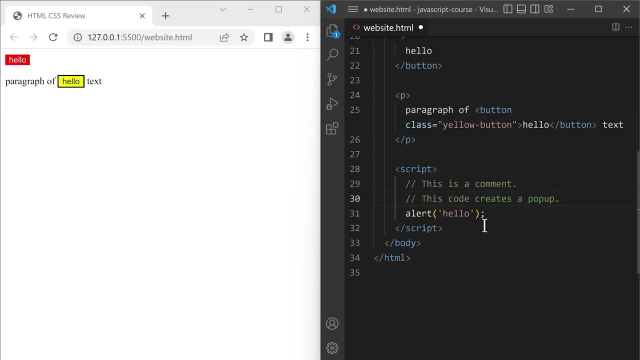 delete it, Because you might want to review this code later. So what we can do here is to add a double slash in front of this line to turn this code into a comment. Now, if we save, the computer will ignore this line of code. 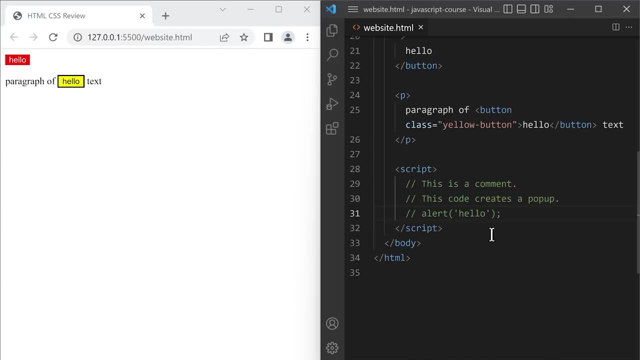 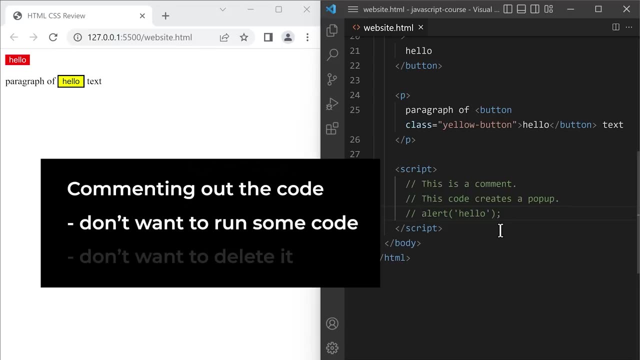 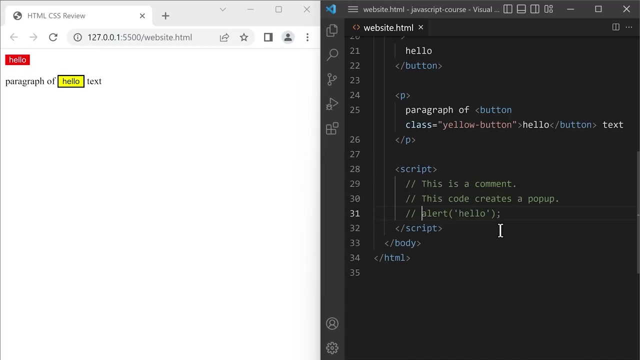 and not create the popup. This is called commenting out the code. It's useful if we don't want to run some code anymore, but we also don't want to delete it for informational purposes. So JavaScript has another syntax for writing comments, And that syntax is: 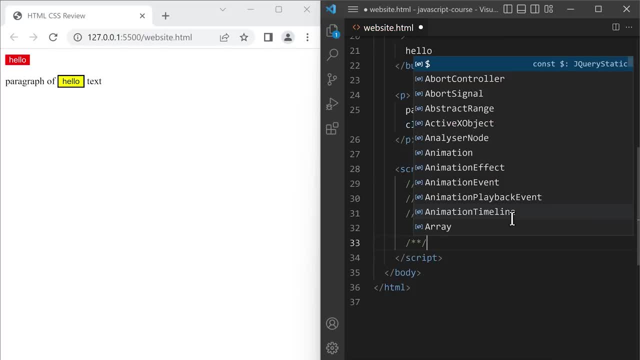 slash star and star slash Here. anything between the stars is a comment. This is called a multi-line comment Because between the stars we can write a comment on multiple lines. For example, we can type multi enter line, enter comment. On the other hand, 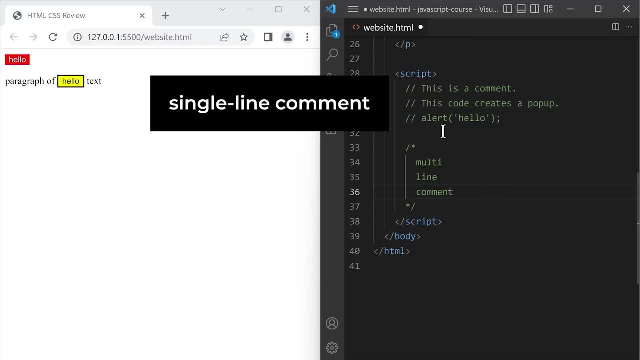 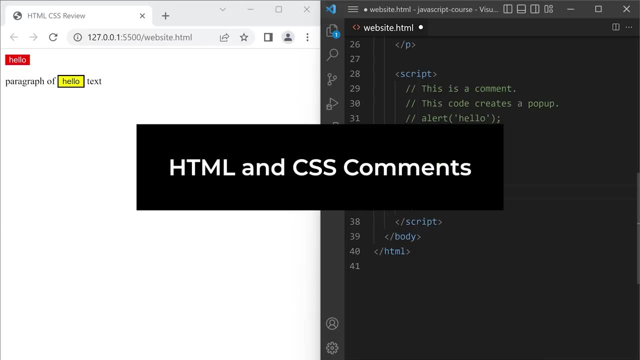 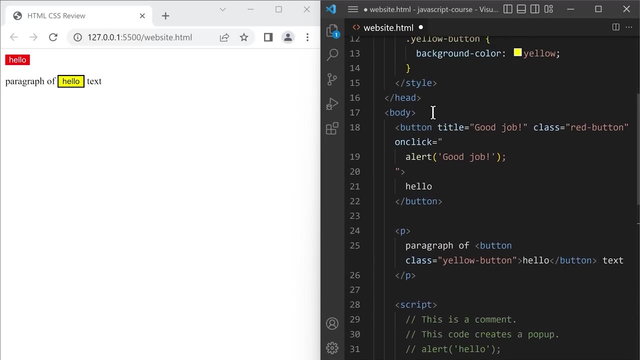 double slash is known as a single line comment. Now, just like JavaScript, HTML and CSS also have comments, But they use a different syntax. If we scroll up to our HTML, here we can type less than exclamation, dash dash, And we also need dash dash greater than. 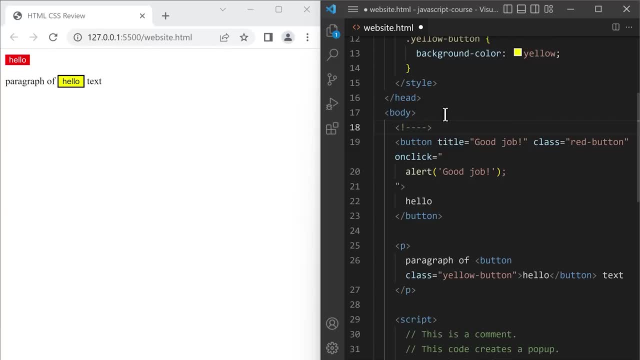 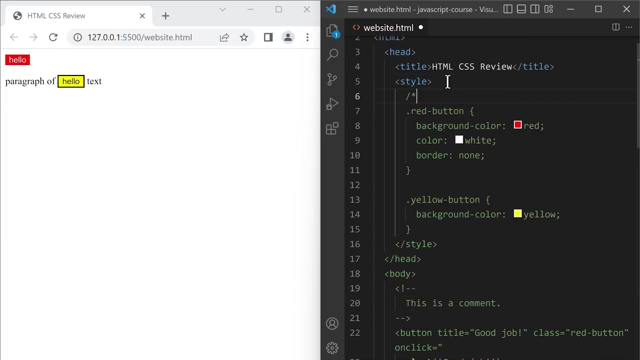 So anything between these double dashes is a comment. For example, this is a comment In C S S. to create a comment, we can type slash, star, star, slash. So it's the same multi-line comment as JavaScript Between the stars. 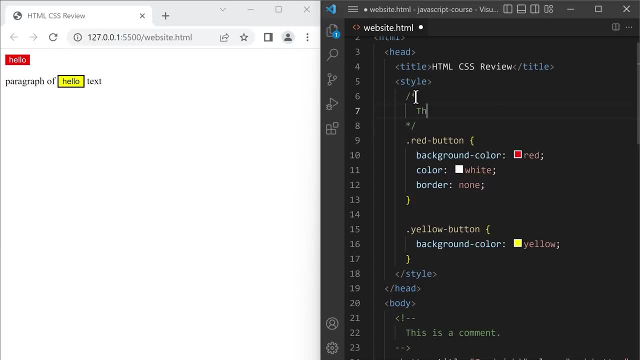 we can add a comment, So this is a comment. If we save our file, nothing changes on our webpage, Because comments are ignored by the computer. The last feature of JavaScript we're going to learn is called console dot log. Let's go back to our code. 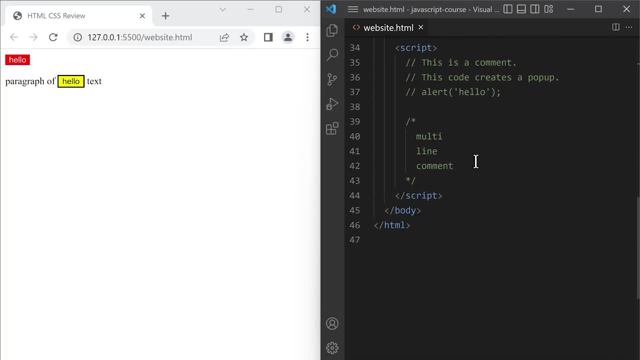 And at the bottom, in the script element, we're going to type the code two plus two. So we learned that this code in JavaScript does some math. However, if we save this file, where is the result of this math? So we might think. 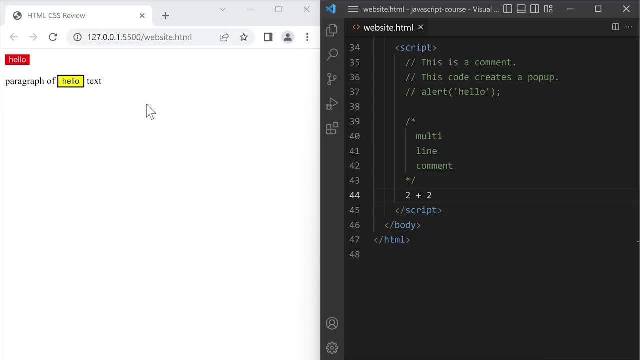 that the result will show up in the console. But if we right click, click inspect and then click the console, you'll notice that the result doesn't show up here either, And that's because before we were running two plus two inside the console. 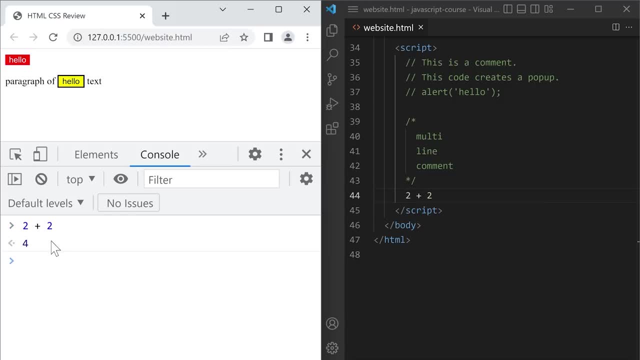 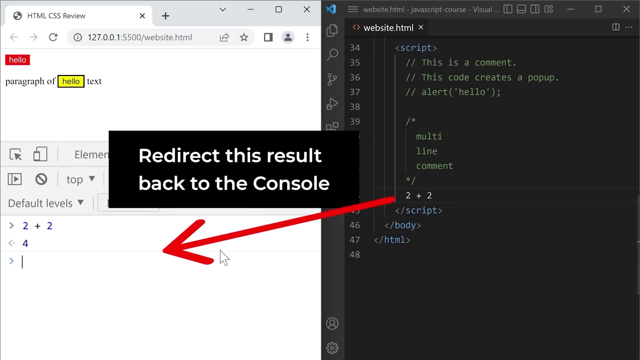 So the result shows up in the console, But now we're not running this code in the console anymore. We're running this code on the webpage. So how do we see this result? The solution is: we're going to redirect this result back to the console. 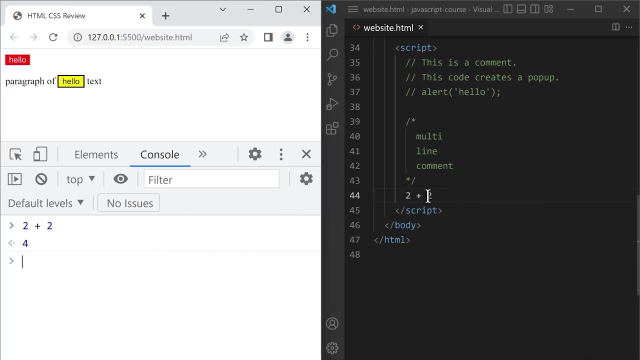 To do that, we're going to use this piece of code: console dot log- open bracket, close bracket and semicolon. Console dot log will display whatever's between the brackets back in the console. So if we move this code between the brackets, so we select this. 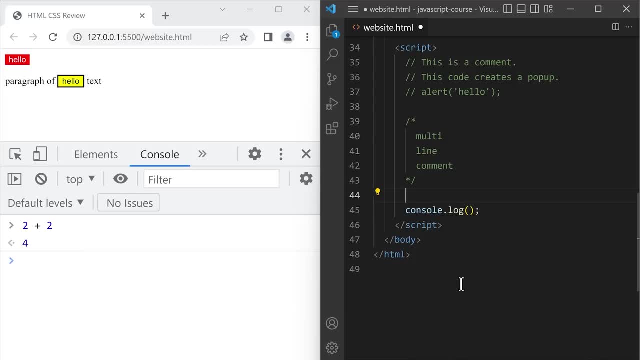 and then right click cut and then, between the brackets, right click paste and save. the result of this code is displayed back in the console, And console dot log works for any code that we learned so far. For example, we can use strings. 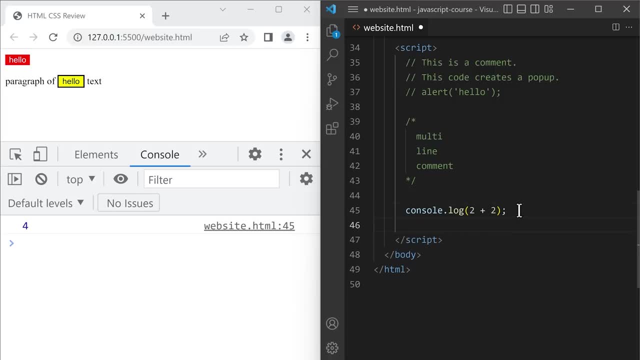 So let's create a new line and type console dot log, open bracket, close bracket, semicolon, and then between the brackets, let's type some strings: Quote, sum quote plus quote text, quote And save this file. 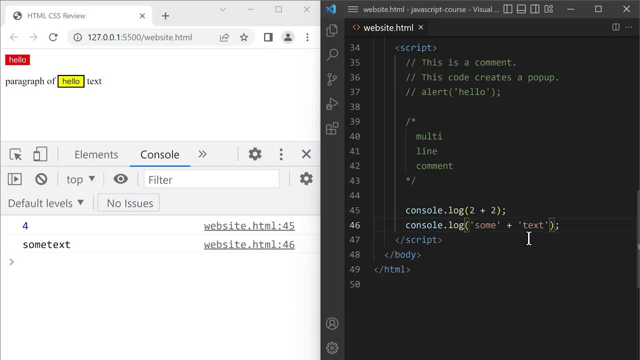 Again, it will display the result of whatever's between the brackets back in the console. So that's how we see the result of JavaScript code that is running in a file. We use console dot log And that's the end of this lesson. 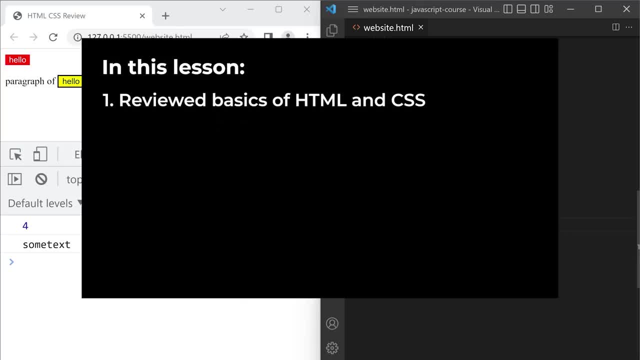 In this lesson, we reviewed the basics of HTML and CSS. We set up our code editor vs code, We learned how to load JavaScript inside an HTML file using the script element and the onClick attribute, We learned how to create comments And we learned how to use 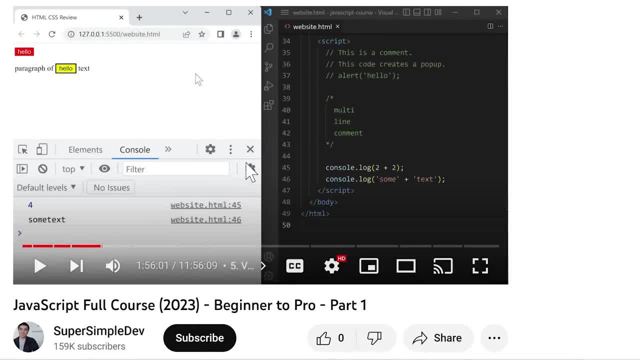 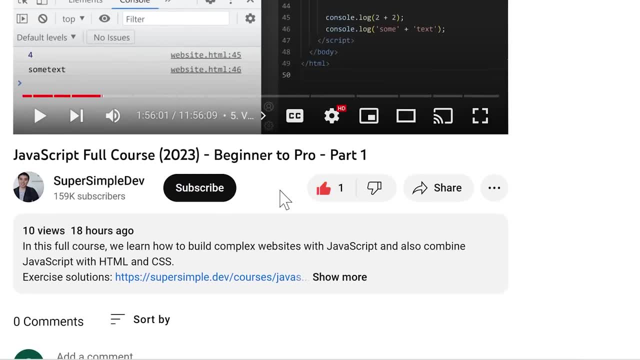 console dot log. Thanks for watching this course so far. If you find this content valuable, you can support this channel by liking the video, clicking subscribe below the video and recommending this course to your friends. Thanks again, and let's continue with the course. 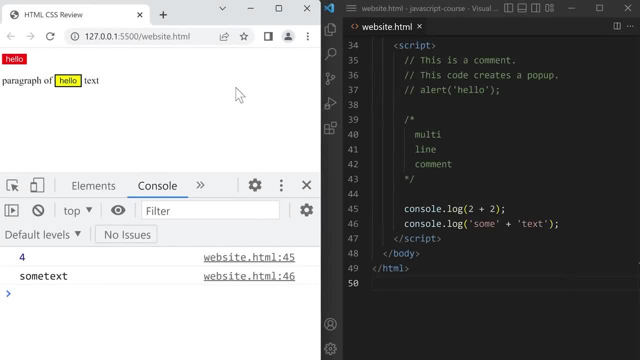 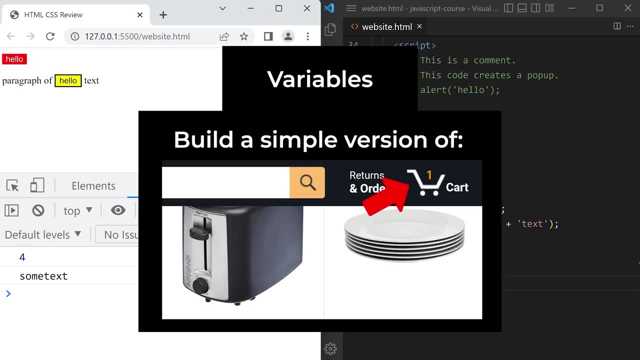 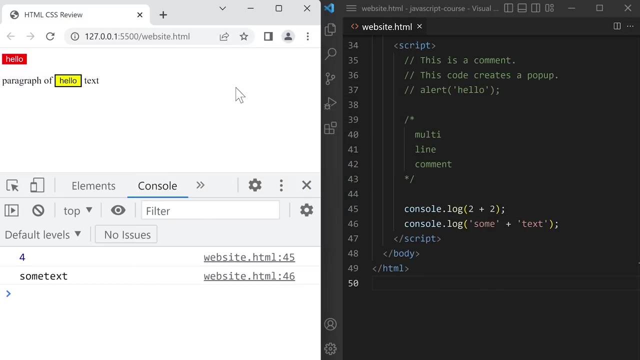 In this lesson we're going to learn the next feature of JavaScript, called variables, And we're going to use variables to build a simple version of the cart quantity feature of the final project. First, let's create a new HTML file just for learning variables. 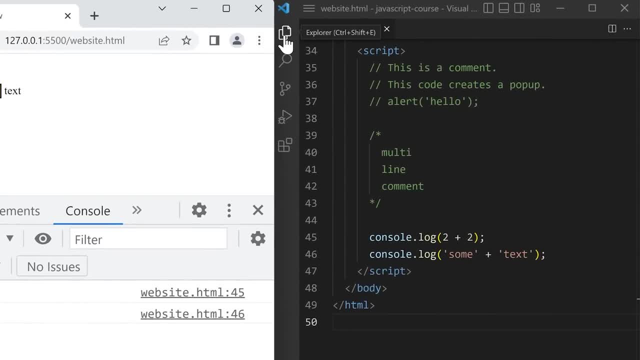 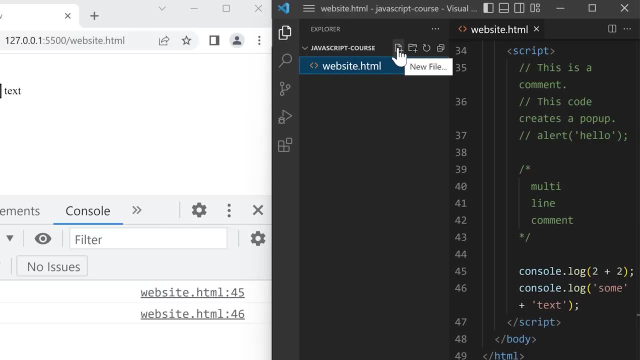 We're going to go to our code editor and click this icon to show our files, and then click this icon to create a new file And we're going to rename this file 05. dash variables, dot html and press enter, So the 05. 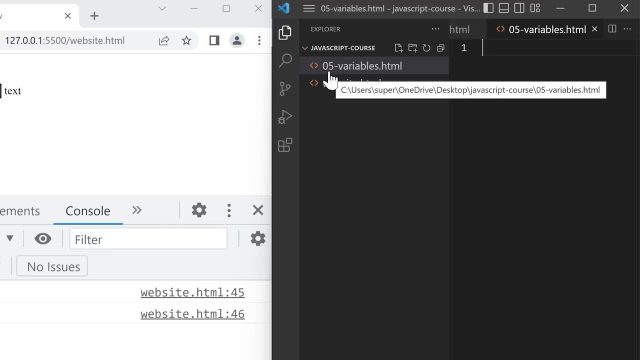 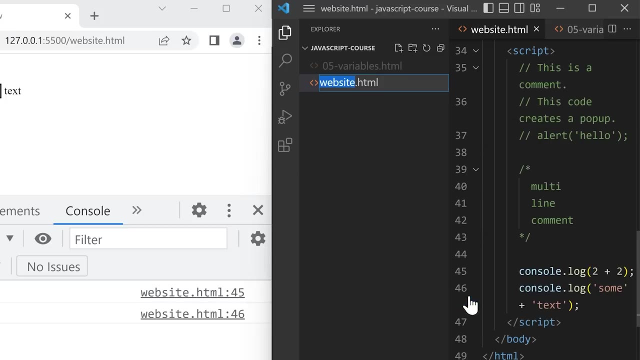 just means that this file is for lesson 5.. Let's also add the lesson number to website dot html. We'll select this file and then right click rename, and then at the front we'll add 04- dash and press enter Next. 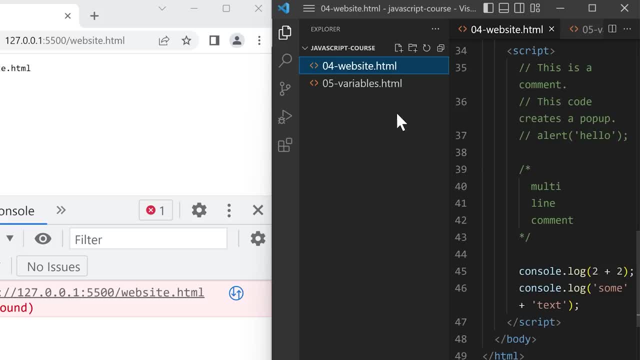 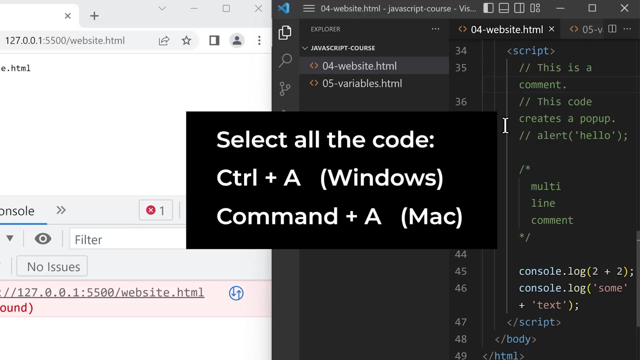 we're going to copy all the code in website dot html to variables dot html. So let's click in this file and we're going to select all of this code by typing control A on Windows or command A on Mac, And then we're going to right click. 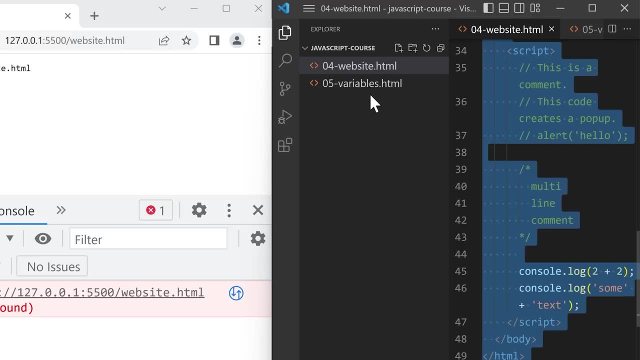 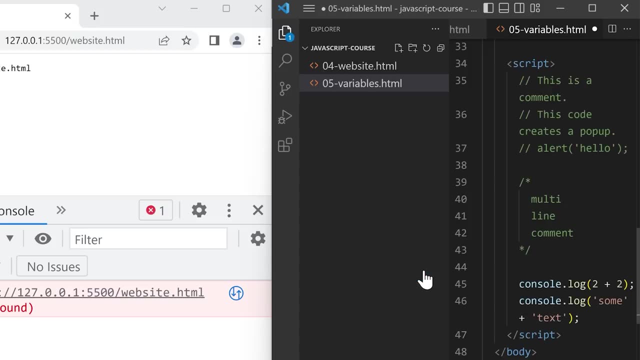 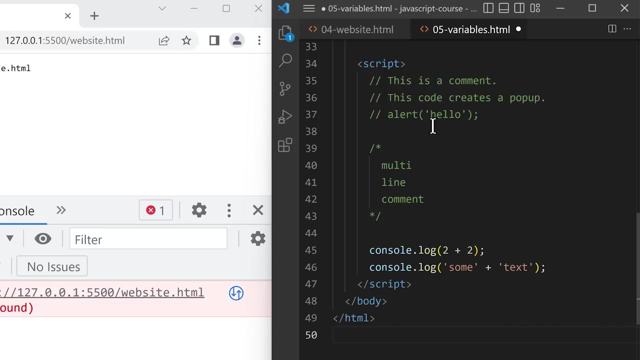 copy and then, inside variables, dot html, right click and paste. Let's click this icon to hide our files for now and we'll prepare this file for this lesson. So let's scroll up to the top, and first we're going to change the title. 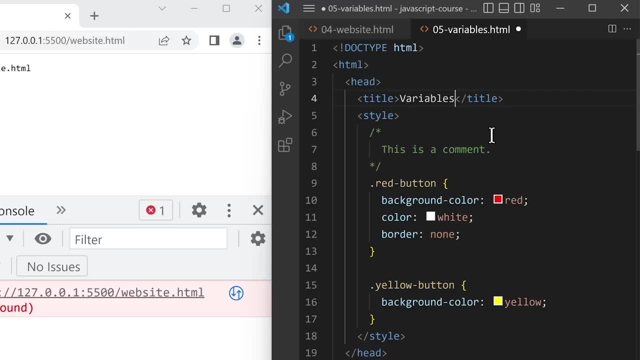 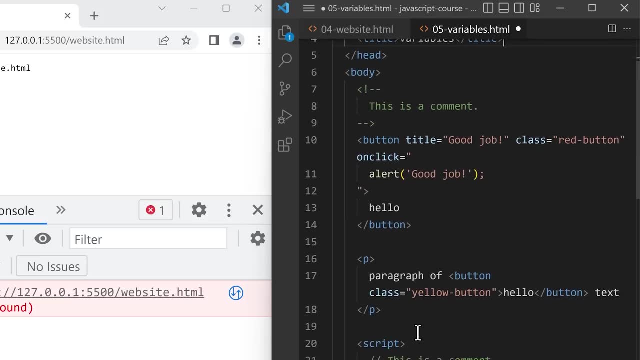 to variables. Next, we're going to delete all the CSS, because we're going to start over, And we're going to delete all the html except for the script element. And let's delete all the javascript from the previous lesson. And finally, let's. 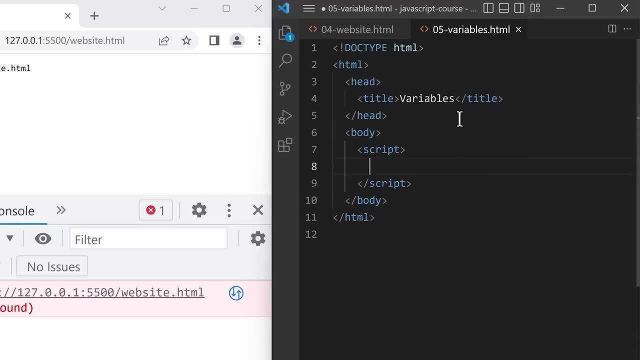 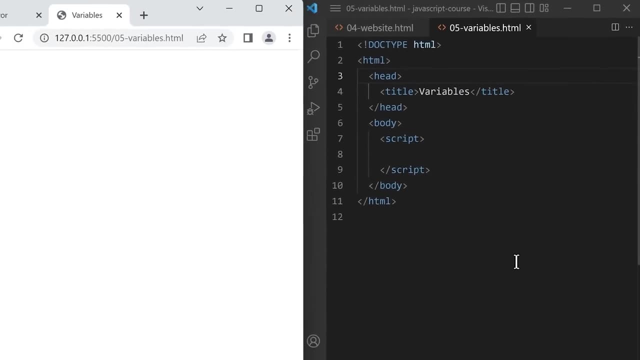 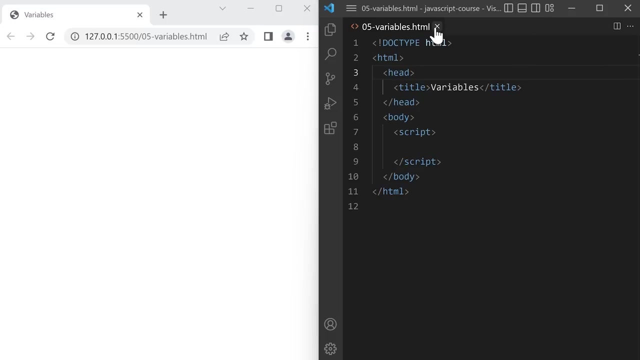 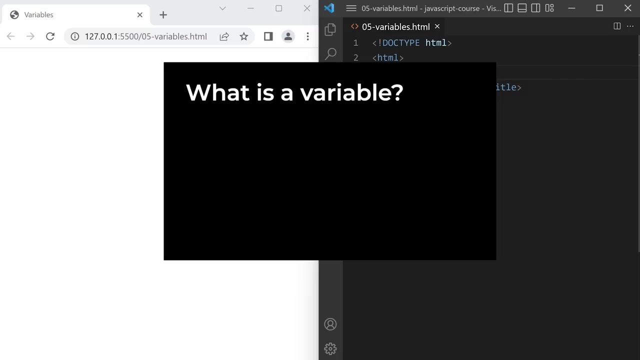 save and we'll open this file in our browser by right clicking and then open with live server. And now we can close the previous tab and the previous code for now. Now we're ready to learn variables First of all. what is a variable? A variable- 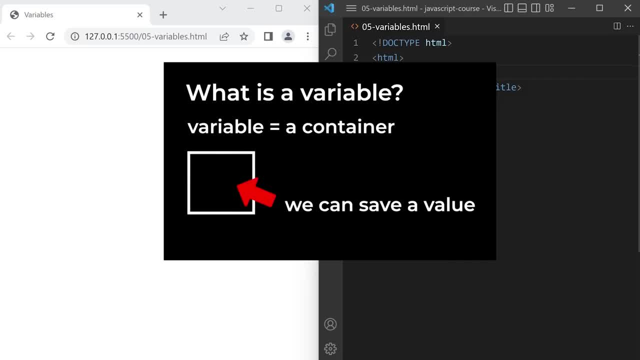 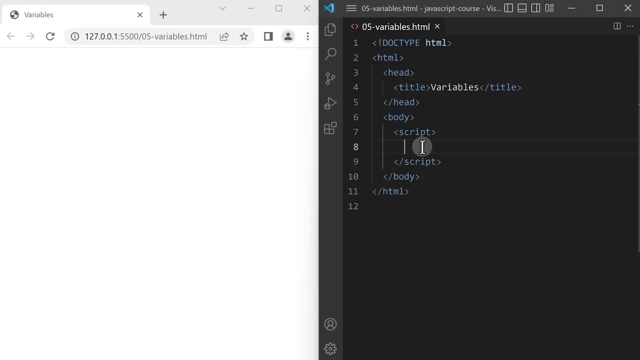 is like a container. We can save a value like a number or a string inside a variable and then use it later. Let's do an example and create our first variable. Inside the script element, we're going to type the code let and space. 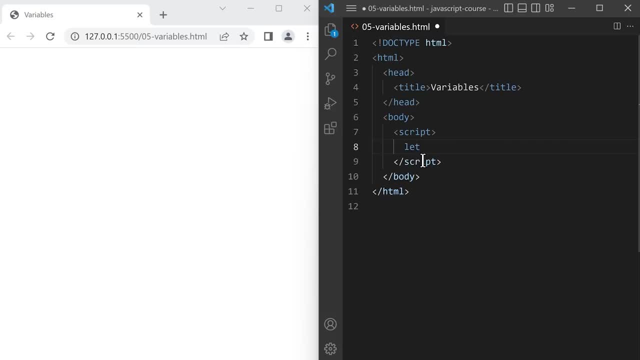 The word let creates a new variable, And now we're going to choose a name for our new variable. Let's name this variable one. So this creates a variable or a container named variable one, And now we can save a value inside this variable. 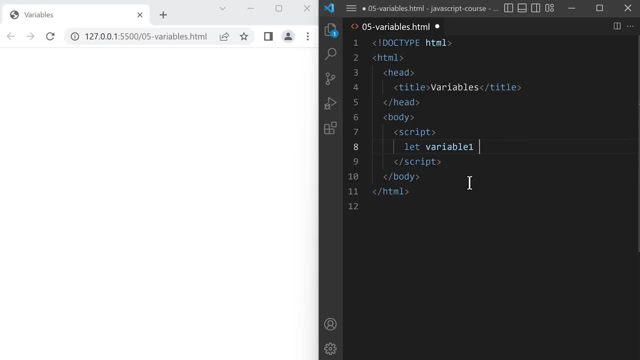 To do that, we're going to type space equals space and then a value like a number or a string. So let's save the number three inside And we'll type a semicolon at the end. So here we use the let to create a new variable. 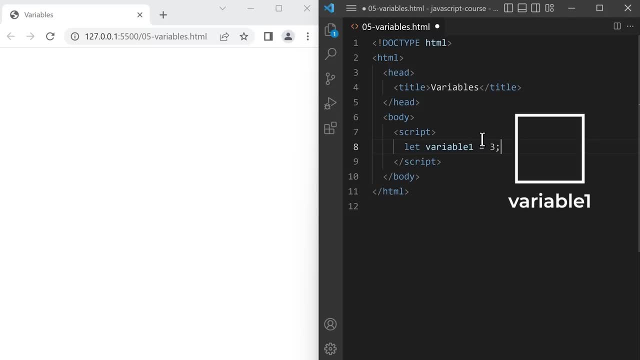 We named this variable variable one and we saved the value three inside this variable. Now that we saved this value, we can use it later. For example, let's type a new line and type the code: console dot. log. open bracket. close bracket and. 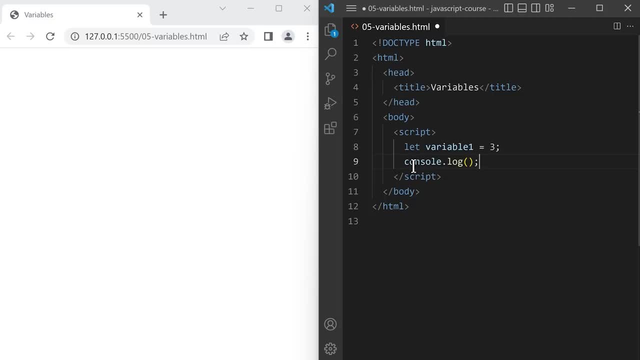 semicolon. Remember from the previous lesson that this code displays whatever's inside the brackets in the console, Or we put a value inside, like the number two, If we save, and then go to our website and open the console. so right click inspect and then click the. 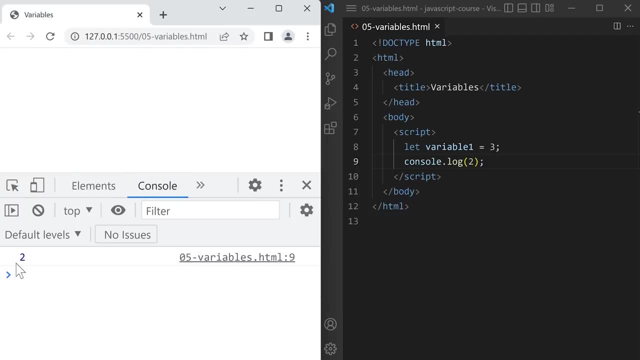 console, we can see that the number two was displayed in the console, So now let's try replacing this value with the variable that we created above. So instead of two, we're going to console dot log variable one. If we save, notice that it now displays three. 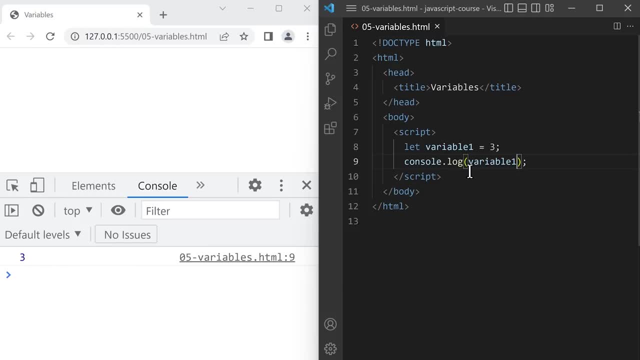 So it's displaying whatever value is saved inside the variable. As you can see, we can save a value inside a variable and then use that variable later on. Let's do another example. We're going to create another variable, So we're going to create some new lines. 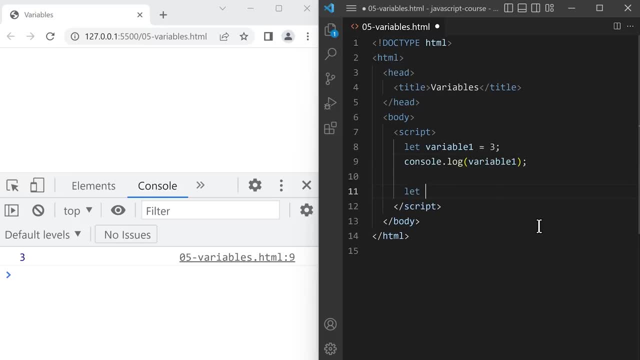 and we'll type let- and this time let's name this variable calculation- And we're going to type space equals space to save a value inside this new variable and this time, instead of just a number, we're going to save a calculation: Two plus 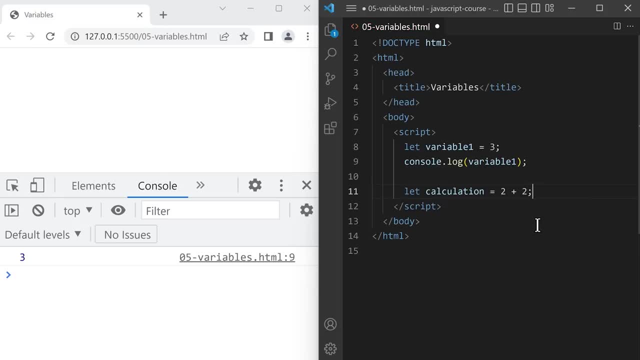 two and semicolon. So this will calculate two plus two and then save the result, which is four, into the variable. If we console, dot, log, open bracket, calculation and semicolon and save, it will show us that the value four is saved inside a calculation. 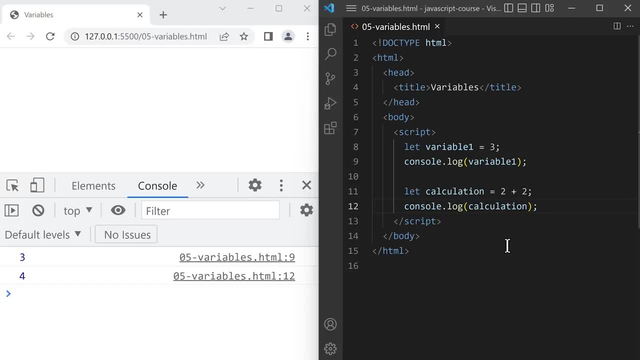 Now let's try this code. We're going to type a new line and then console, dot, log, open bracket and calculation again, and plus two and semicolon. So here we're using a variable inside a calculation. What this does is that it takes whatever value is saved. 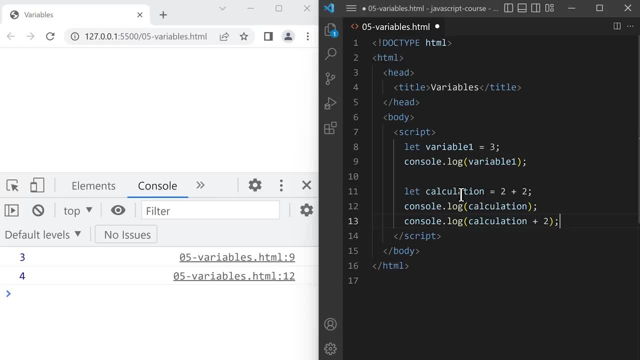 inside the variable- Right now it is four- and then substitutes that value into the calculation. So this will be four plus two, which equals six. If we save, we can see that in the console it displayed six. So we can use a variable wherever we. 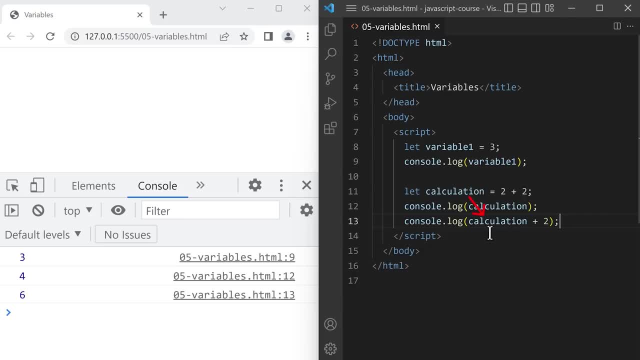 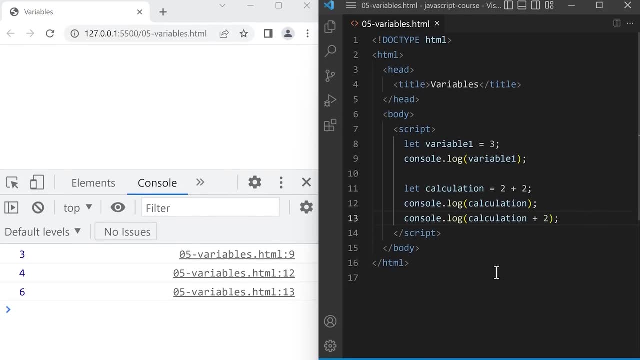 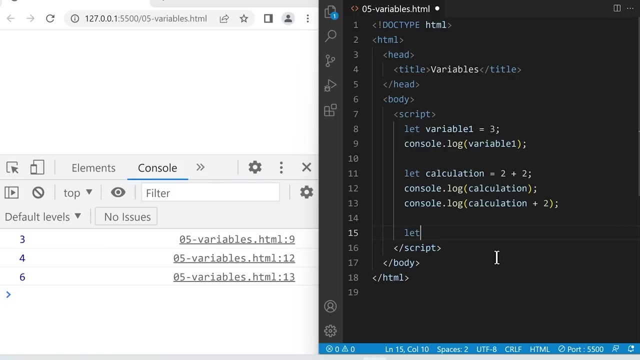 use a value And JavaScript will substitute whatever is inside the variable into the code. Let's do another example. We're going to type some new lines and create a new variable, again using let, and we're going to name this variable result And we're 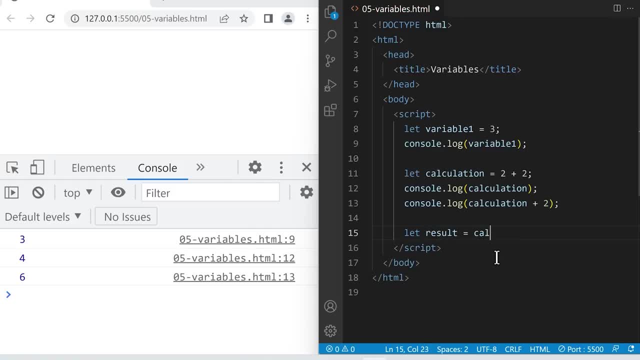 going to make it equal to calculation plus two and semicolon. So this does the same thing as the code before. It will take whatever value is inside calculation, which is four, and substitute it into this code. So we get four plus two equals six. 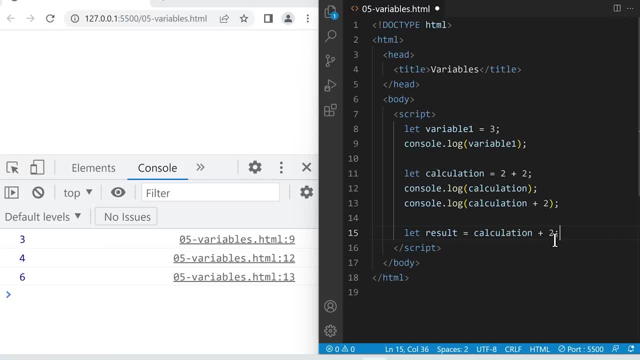 But this time we have an extra step: We're going to save this result, which is six, into another variable. So if we console dot log result and save, we can see that six was saved into the result variable. Again, we can use a variable. 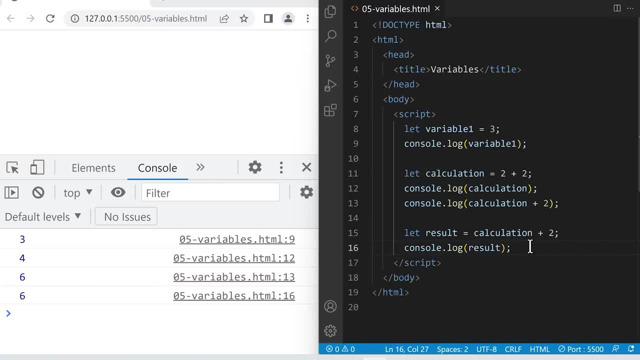 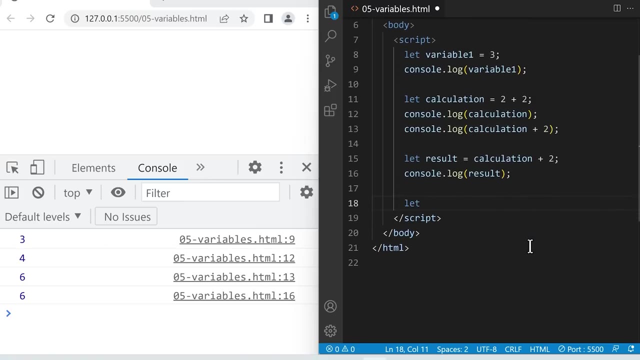 wherever we use a value. Now, in addition to numbers, we can save any type of value in a variable, including strings. For example, let's create a new variable using let and let's name this message, And we're going to save inside this variable a string, this time. 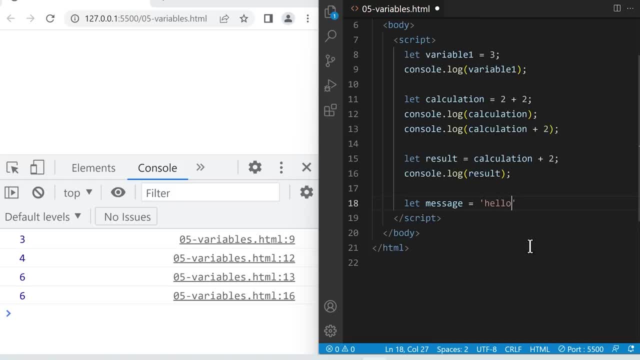 So quote hello, quote and semicolon. Again, we're going to console dot log this variable. So console dot log and message And a semicolon at the end, If we save, it will show us that the string hello is saved inside this variable. 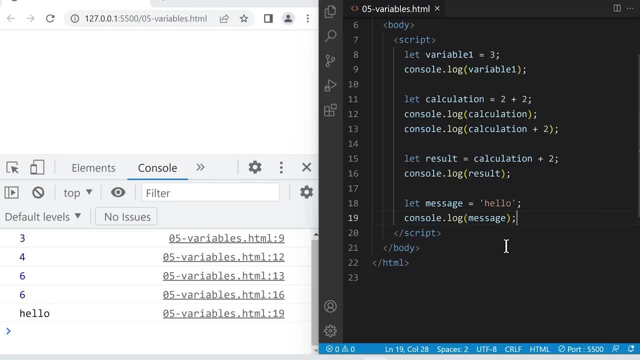 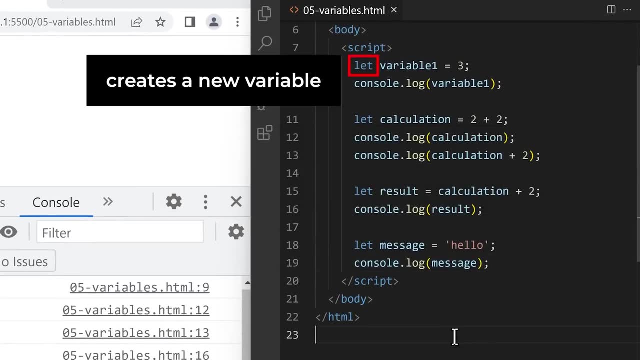 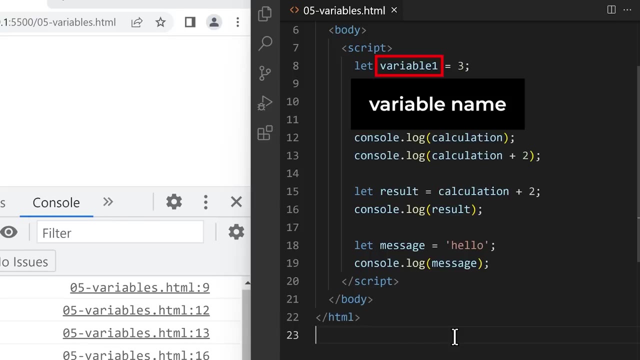 Okay, now that we learned how variables work, let's learn the syntax rules for variables. The word let creates a new variable, And then we give the variable a name. So we can name variables almost anything we want, except for a few restrictions. Number one: 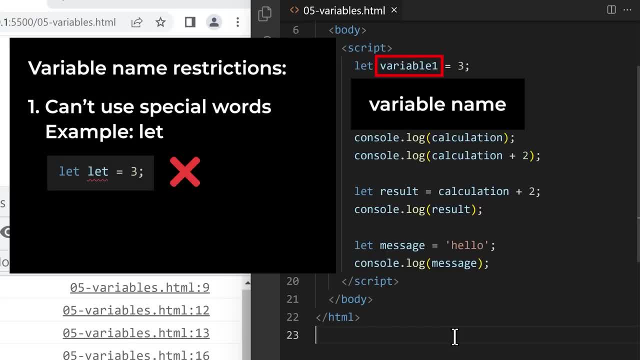 we can't use special words like let as a variable name. That's because let already has a special meaning. in JavaScript It creates a variable, So let is a reserved word. However, we can use let one or let two as variable names. 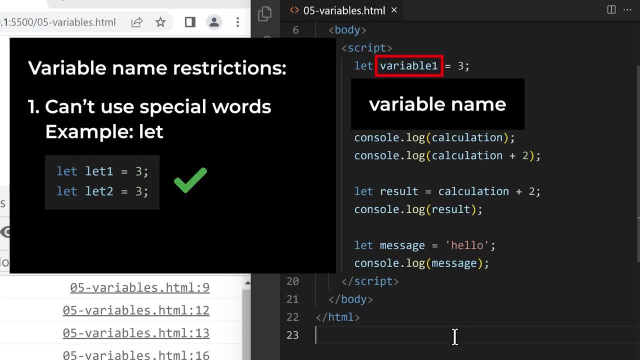 We just can't use let Number. two: we can't start a variable name with a number. If we start with a number, JavaScript will think this is a number instead of a variable name. However, we can use numbers in the middle or the end. 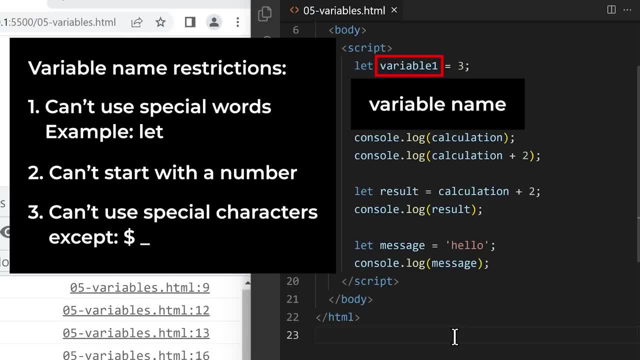 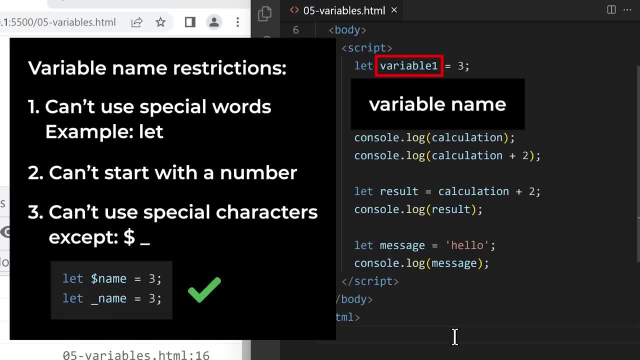 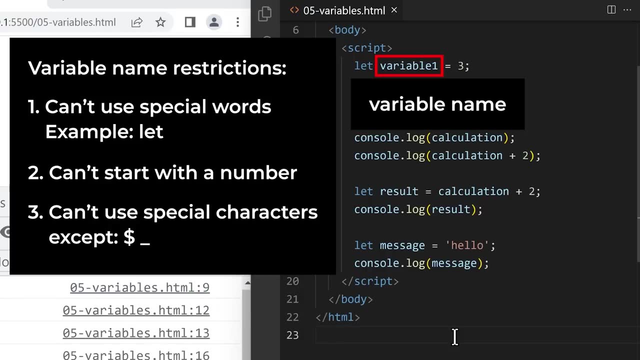 Lastly, we can't use most special characters like these or a space in a variable name. However, there are two special characters we can use Dollar and underscore. So those are the rules for naming variables, And then to save something inside a variable, we just use the. 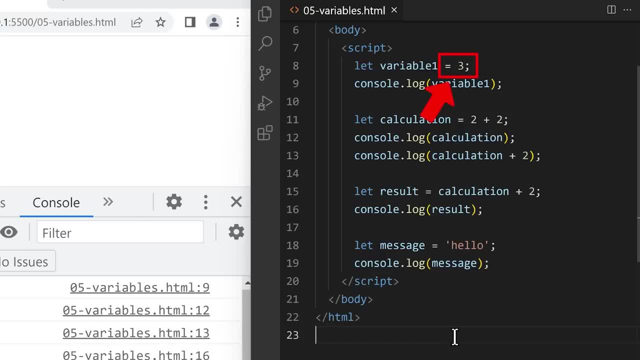 equal sign, and then the value we want to save, And that's it. After we create a variable, we can start using it in the rest of our code. Now there's one last part of the syntax that we haven't learned, which is the. 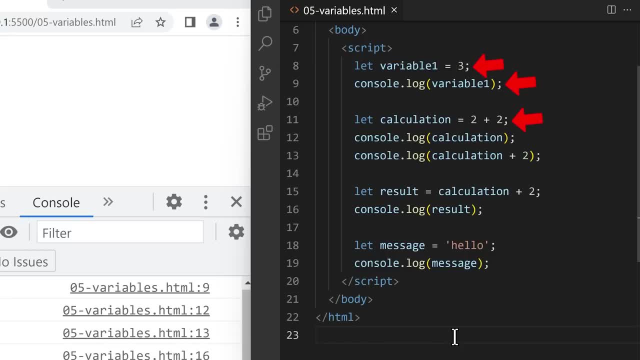 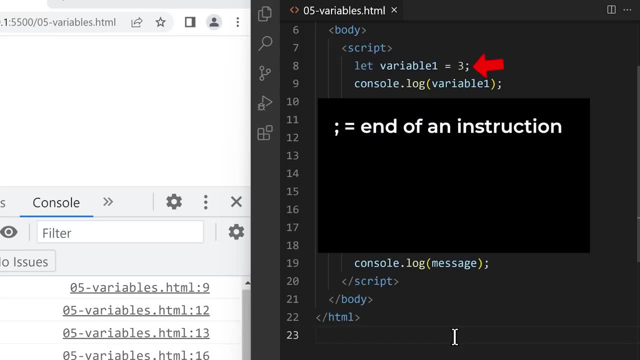 semicolon. We've seen semicolons in many places already. In JavaScript, a semicolon means this is the end of an instruction. It's similar to a period in English. In English, a period means this is the end of a sentence. 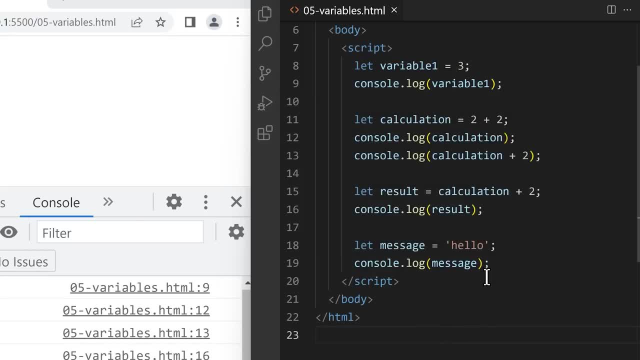 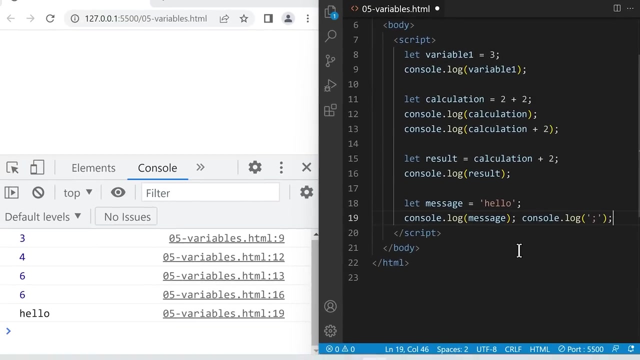 So here this semicolon tells JavaScript that this is the end of an instruction. And now, after this, we can add another instruction Like console dot log, open bracket, and then the string semicolon And a semicolon at the end, If we save. 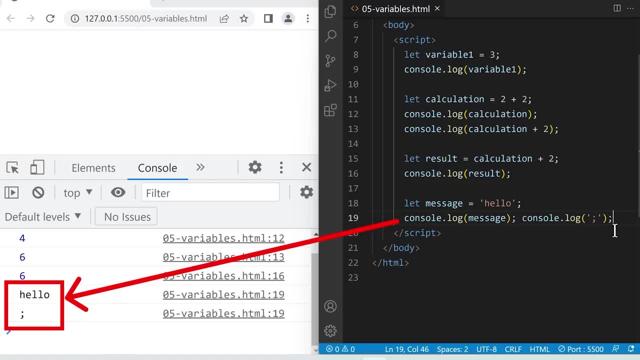 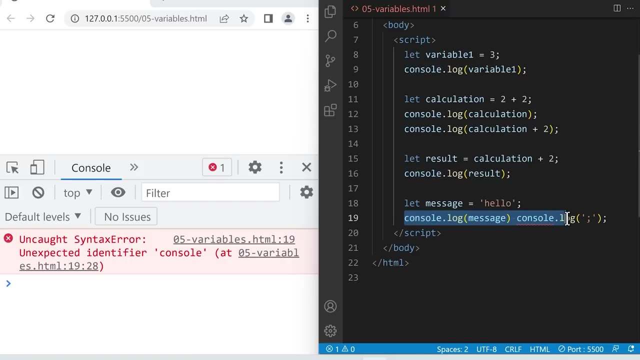 it will run these two instructions one after another without any problems. So if we didn't have the semicolon here and we save, it wouldn't work, Because JavaScript thinks that this entire line is one instruction, So we need semicolons to separate different. 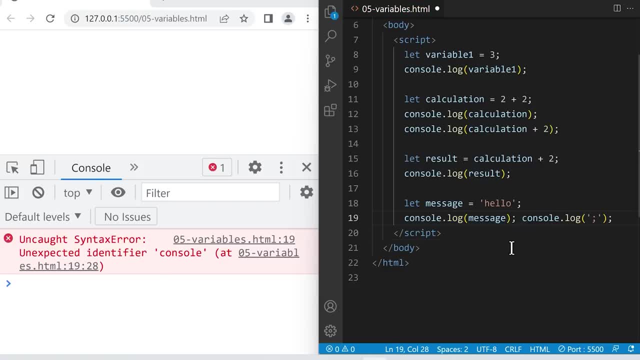 instructions in JavaScript. If we save, everything goes back to normal. So JavaScript is a little special Because it has a feature called semicolon insertion. That means it will try to insert the last semicolon in a line of code automatically, For example. 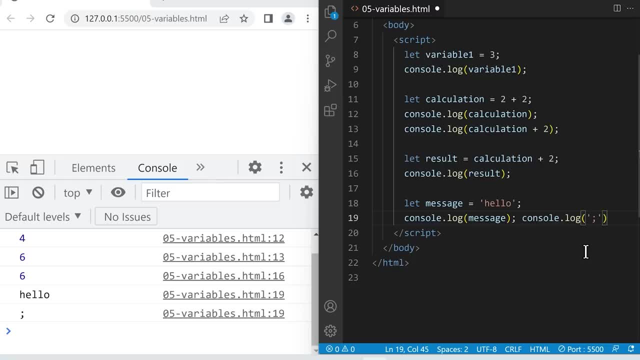 if we removed the last semicolon and save, this code will work without that semicolon, And that's because JavaScript inserts the last semicolon automatically. However, a lot of companies still prefer to use semicolons in their JavaScript code, Because semicolon insertion 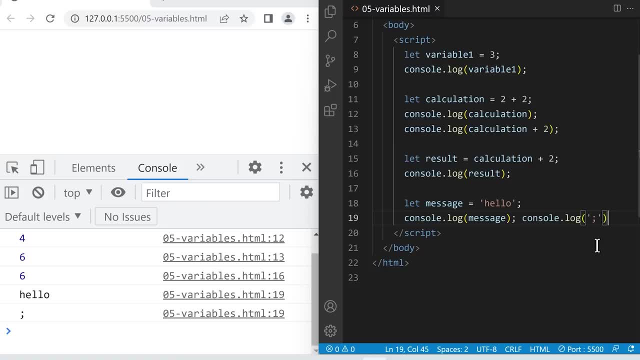 can sometimes put the semicolon in the wrong place. For this reason, we're also going to use semicolons in this course To help you get used to JavaScript code with semicolons. Next we're going to learn how to change the value, that is: 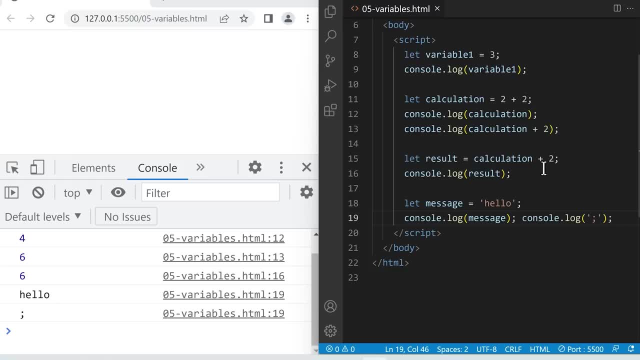 saved inside a variable. For example, here we save the number 3 inside variable 1.. Now we're going to change the value saved inside variable 1.. To do that, we're going to go to the bottom and create some new lines. 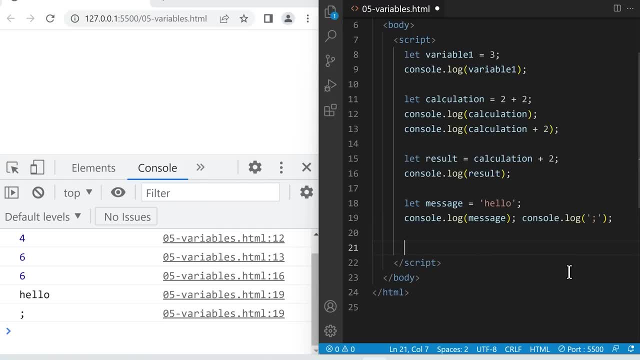 And we're going to type the variable name again, So variable 1.. And now to change the value saved inside, we're just going to type the equal sign And then a different value, Like 5 and semicolon. And now, if we 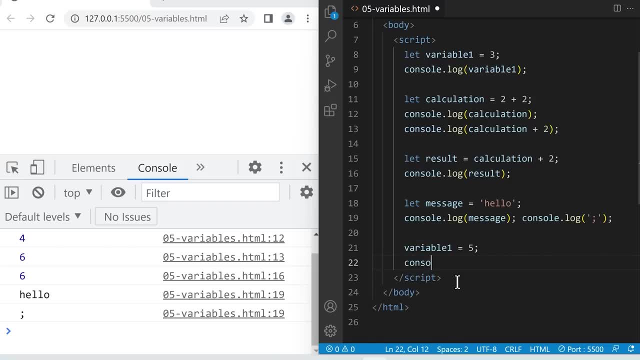 consolelog, this variable, consolelog, variable 1, variable 1 and semicolon and save. it will show us that 5 is now saved inside variable 1.. Notice also that if we scroll up to the top, the first consolelog still displays the value 3.. 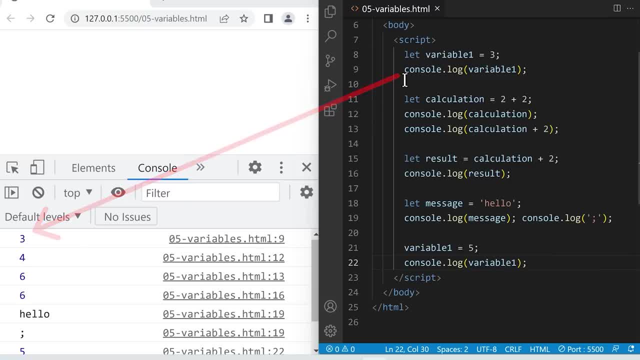 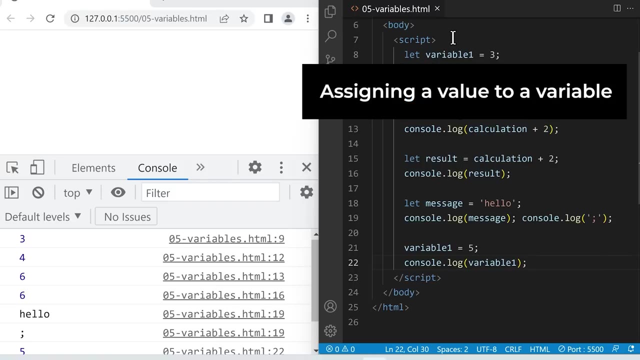 And that's because at this point in the code, variable 1 still contained 3.. We didn't update the variable yet. So when we first saved a value inside this variable- this is called assigning a value to a variable- Then when we change the value inside this variable, 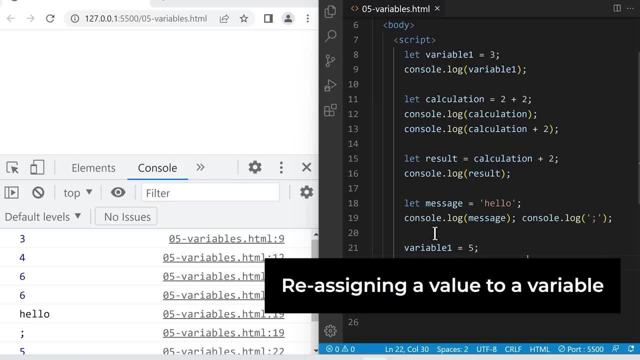 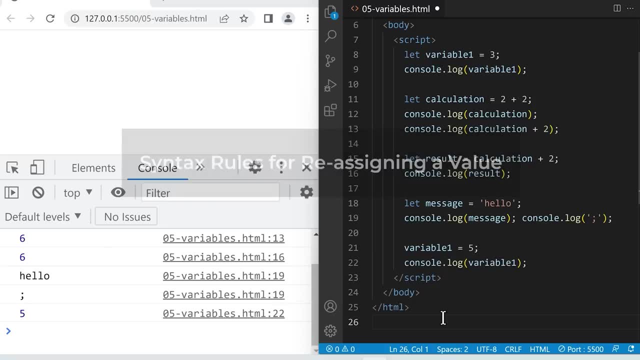 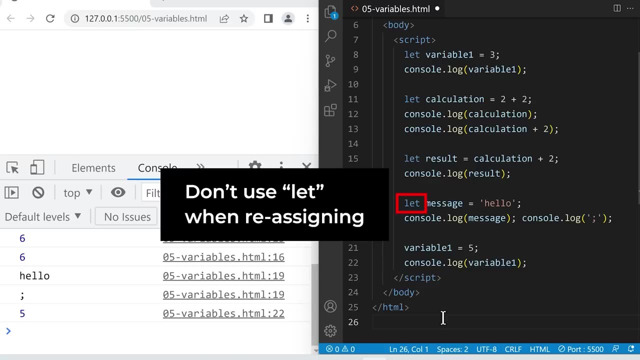 this is called reassigning a value to a variable. Now let's learn the syntax rules for reassigning a value. Notice that we don't use the word let when reassigning. That's because let creates a new variable. So if we 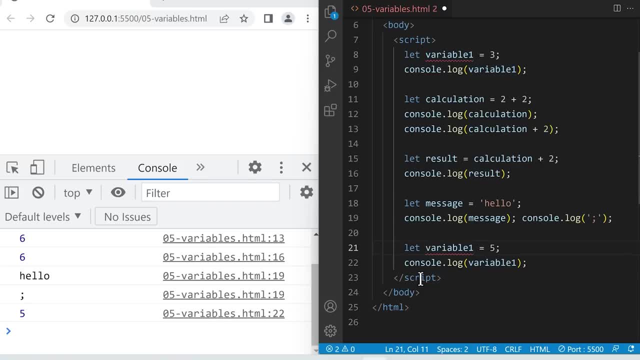 try to use let again. it would try to create a new variable named variable 1.. However, variable 1 already exists and we can't create two variables with the same name, So this would cause an error. Instead to reassign a variable, we just type out: 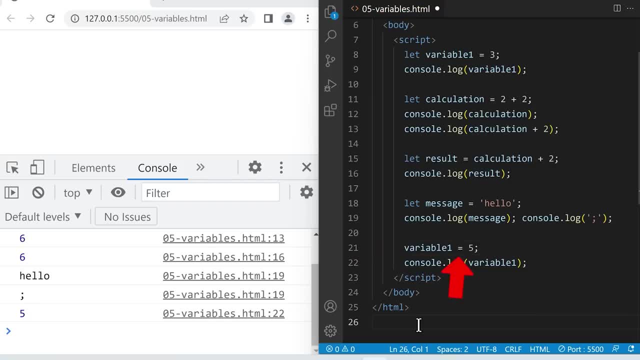 the variable name and make it equal to something else. So that's the syntax for reassigning a variable. Now we're gonna do one last example before working on the project. Let's go to the end of our code. We're gonna type some new lines. 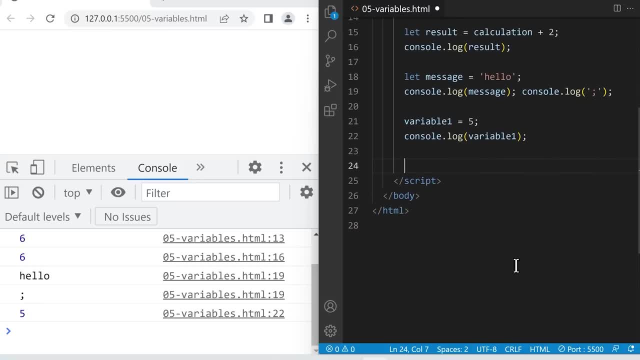 And this time we're going to reassign variable 1 again. So we can reassign a variable as many times as we want. So let's type variable 1 and then equals, and we're gonna type variable 1 plus 1 and semicolon. 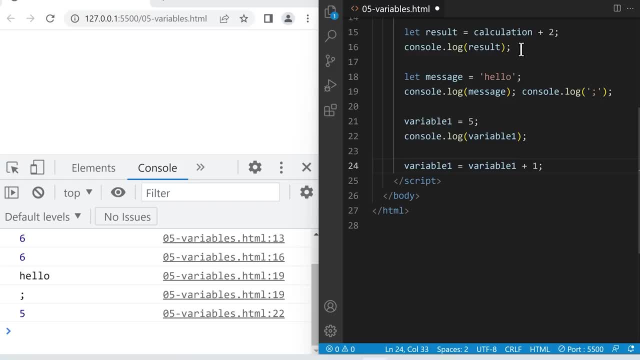 So we learned earlier that we can use a variable inside a calculation And it will substitute whatever value is inside the variable. Here we're also using a variable inside the calculation, but we're using this variable itself. So it's essentially taking this variable, increasing it by 1. 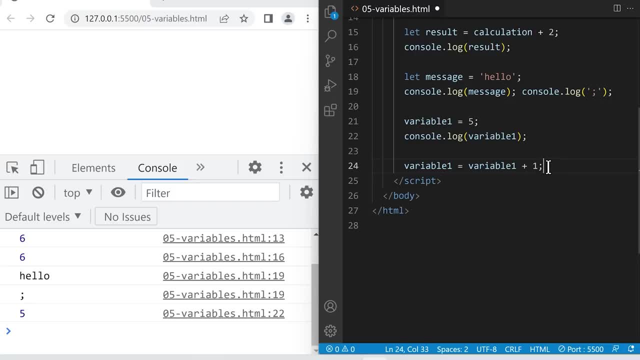 and then saving it back. If we console dot, log this variable, variable 1, and save, variable 1 now contains 6.. So it took the previous value in variable 1, which was 5, added 1 and then saved it back. So this: 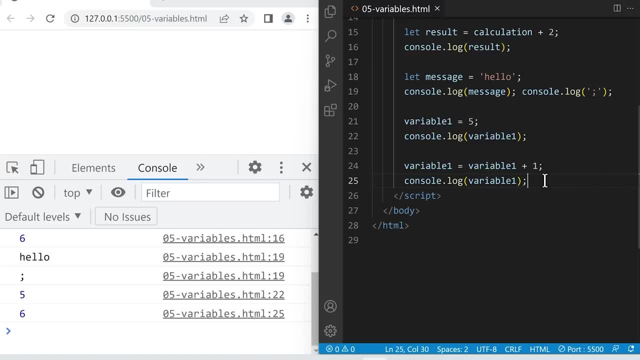 is how we increase the value of a variable by a certain number. Okay, Now that we know how to create and reassign variables, we're ready to work on a project. So I actually prepared a project that we can do for this lesson. 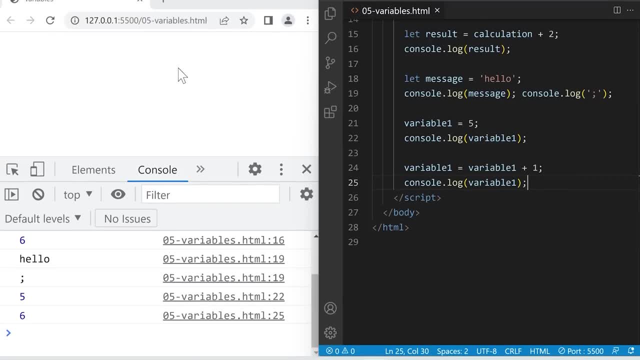 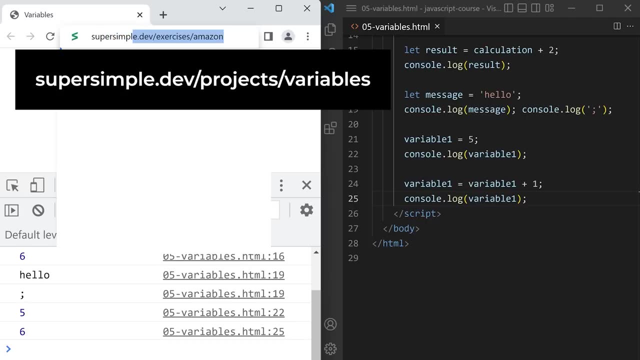 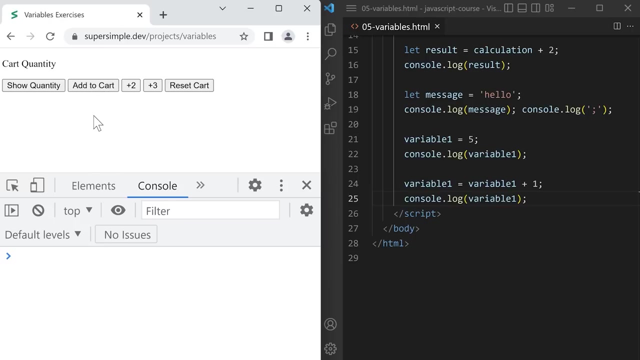 And we can see this project by going to our browser, clicking at the top and typing supersimple dot dev, slash projects, slash variables and press enter. So we're going to work on the cart quantity feature of the final project. So in the final project we have a number in the top right. 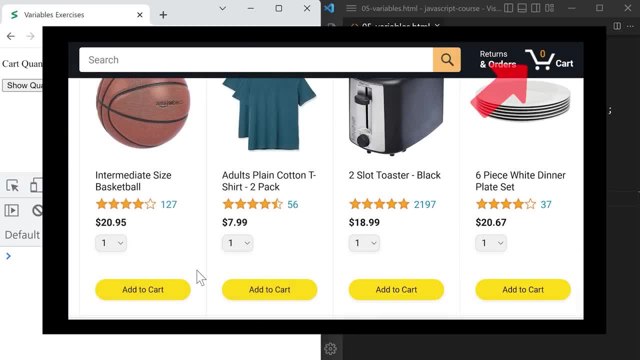 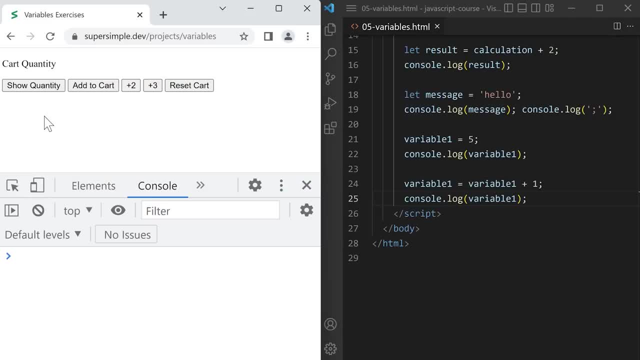 corner that shows how many products are in our cart. When we click the add to cart button, this quantity will increase. So what you see here is a simple version of the cart quantity feature that we can create. right now Let's go over how it works. 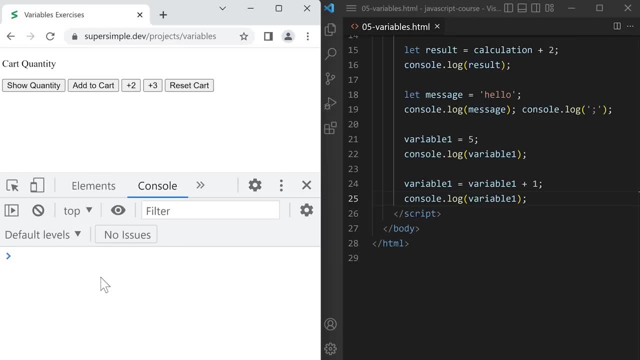 First make sure you have the console open on this page Now, when we click the show quantity button, it will show us that there are zero products in our cart. If we click the add to cart button, it will increase the quantity by one and display. 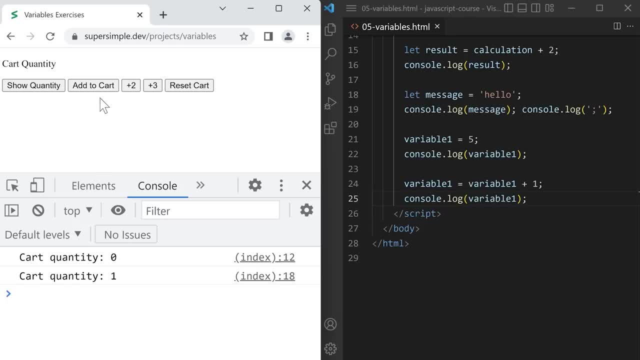 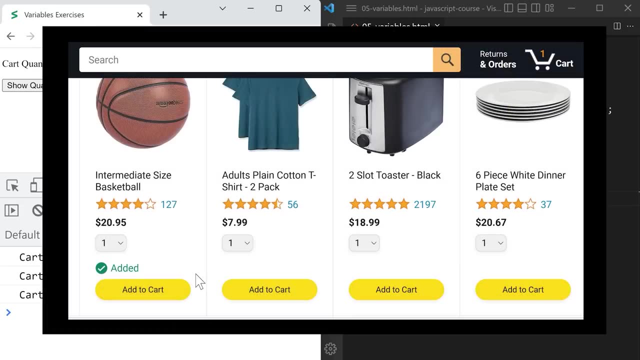 it in the console. If we click add to cart again, it will increase the quantity by one again. Now in the final project, we can also add more than one product at a time using this dropdown. For now, we're going to build a simpler version of that. 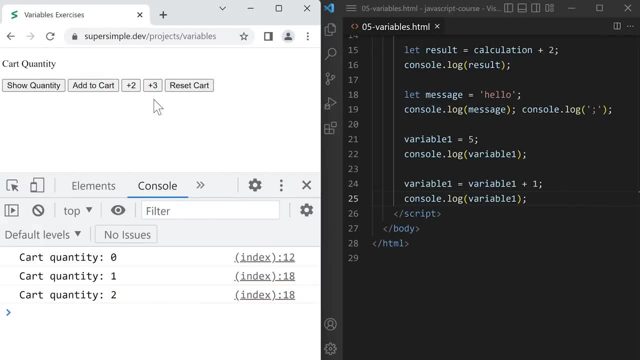 We're going to use the plus two and plus three buttons to add multiple products. So when we click the plus two button, it will increase the quantity by two and display it in the console, And when we click the plus three button it will increase. 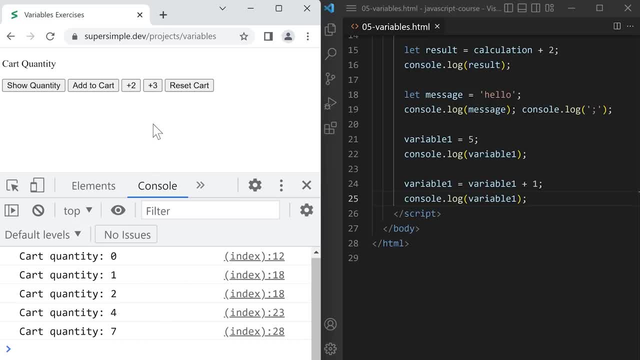 the quantity by three. And finally, when we click the reset cart button, it will reset the quantity back to zero and display this message in the console. So now that we understand how this project works, let's build this step by step. First, let's create a new. 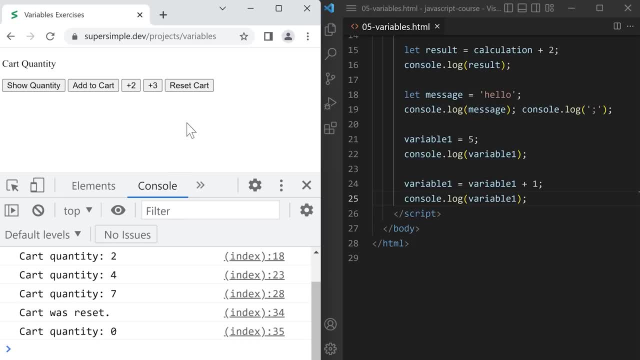 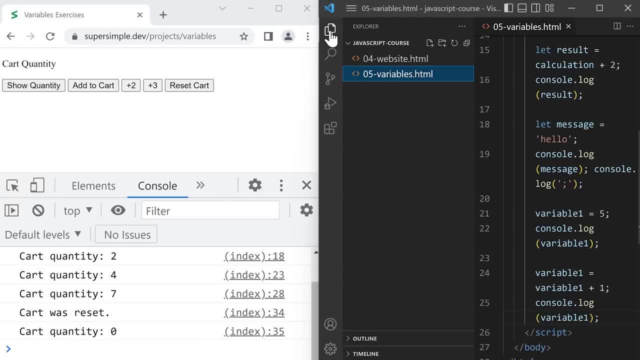 HTML file just for this project. We're going to go to our code editor and click this icon to show our files, and then click this icon to create a new file. Let's name this file: zero five, dash, cart, dash quantity dot html and press enter. 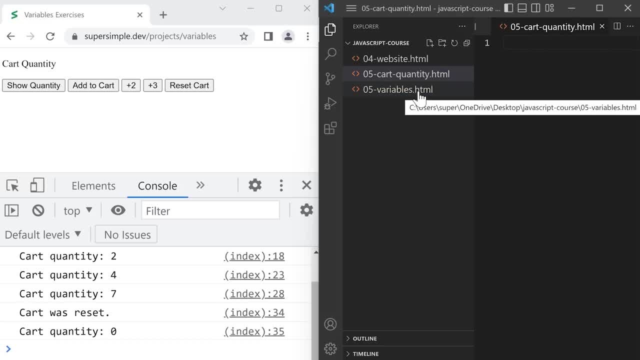 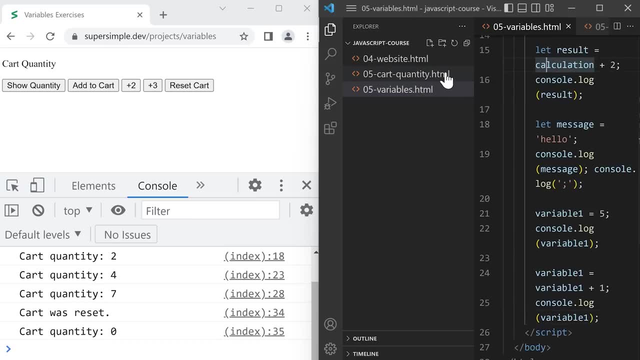 Next, let's open variables dot, html, and we're going to copy all the code here into our new file. Let's type control A on Windows or command A on Mac to select all this code, and then right click, copy and then in our new file. 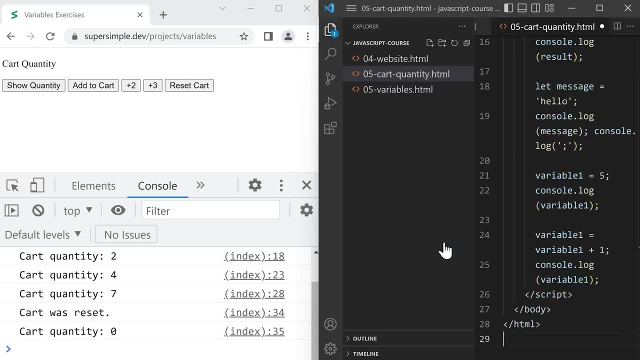 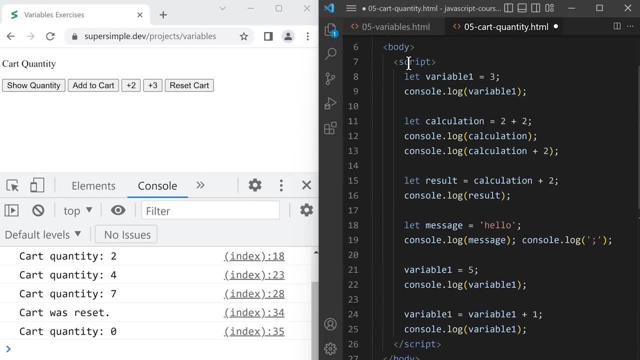 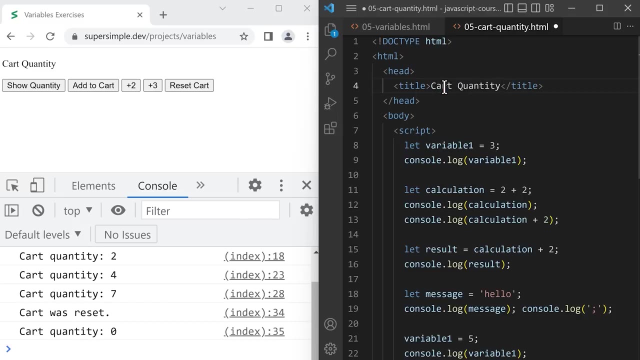 right click and paste. Let's close this for now, and in the new file we're going to change the title to cart quantity and let's remove all of our JavaScript code but keep the script element, because we're going to write new JavaScript code Now. we're ready. 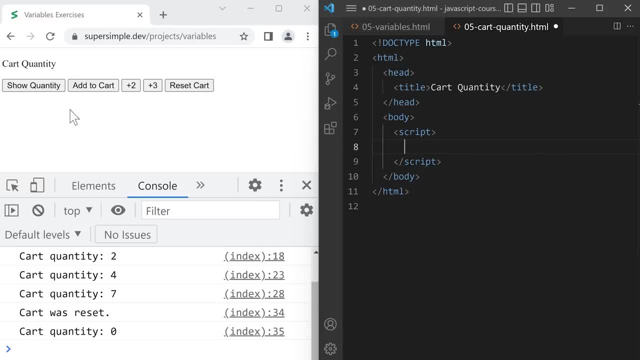 to begin, Let's start by creating these buttons. Let's go to the body element and create a new line and here, as we learned in the previous lesson, we can create a button using this html code: lesson button greater than and the closing tag: lesson slash button. 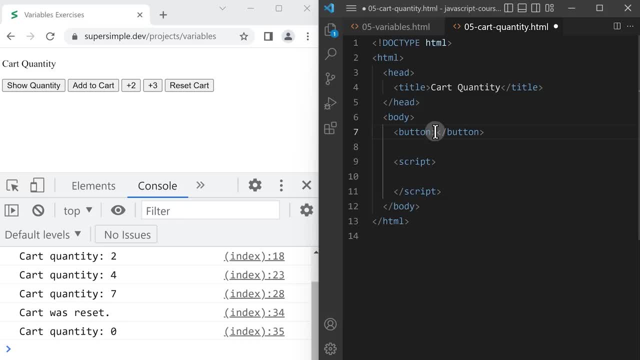 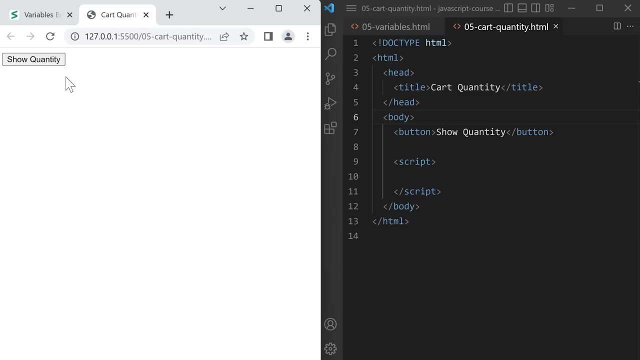 greater than Inside this button. we're going to have the text show quantity and let's save. now let's open this file in live server by right clicking and then open with live server and we can see that we created the first button. now let's create. 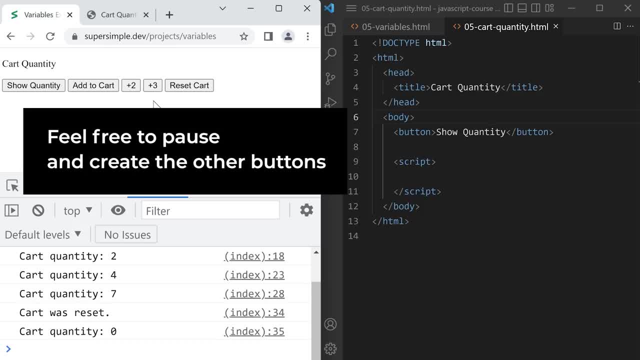 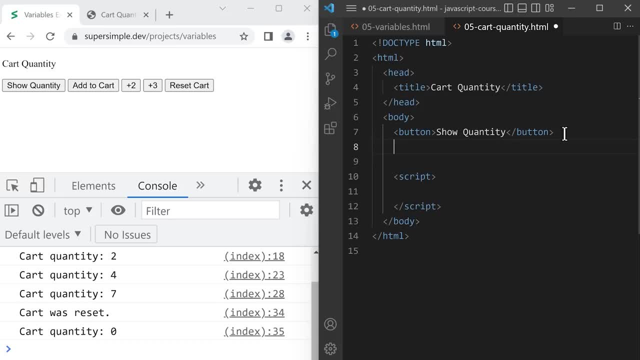 the other buttons here. feel free to pause the video if you want to try it yourself. we're going to go back to our html and create another button. inside this one, we're going to have the text add to cart. let's create another button. this one is going to have the text plus. 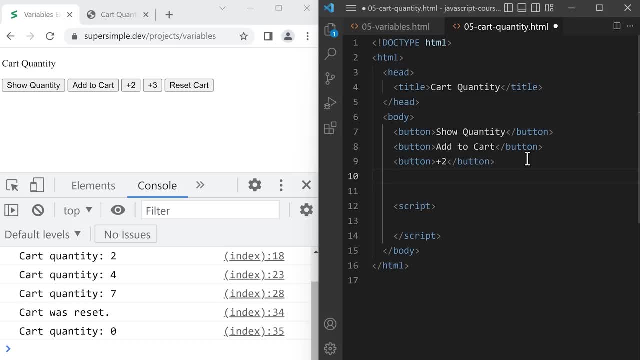 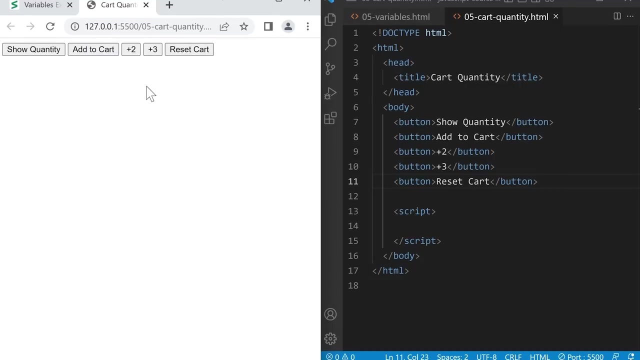 two and we'll create another button. this one is going to be plus three- and finally, we'll create the last button, and this one is reset cart. and now let's save. and if we go back to our tab, we've created all the buttons. now let's make this webpage interactive. 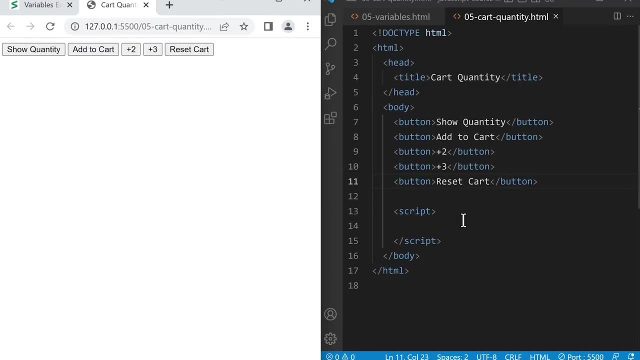 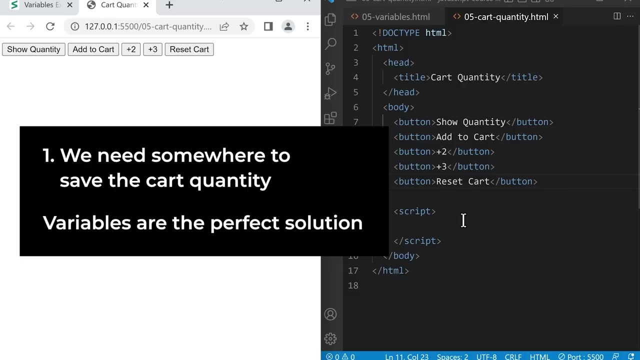 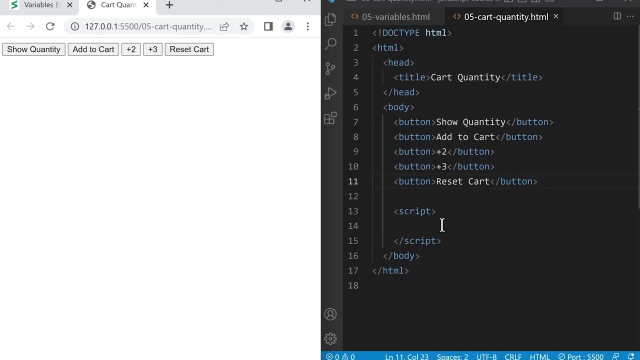 with javascript. first of all, we need somewhere to save the cart quantity. so, as we learned in this lesson, variables are the perfect solution for this. variables: let us save a value. so let's go into the script element and we're going to create a variable by typing. 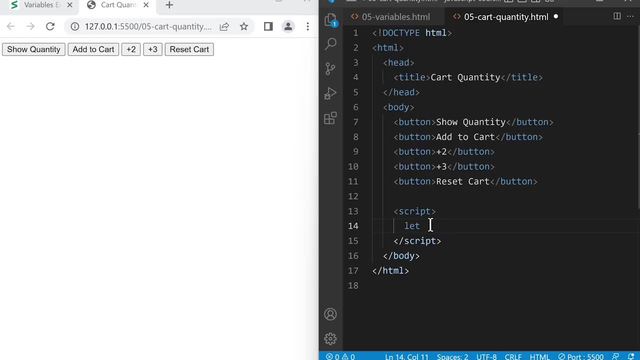 let. and this variable is going to save the cart quantity, so let's just name it cart quantity. so the cart quantity will start out at zero. so we're going to type equals zero and semicolon. next, when we click the show quantity button, we want to display the quantity in the 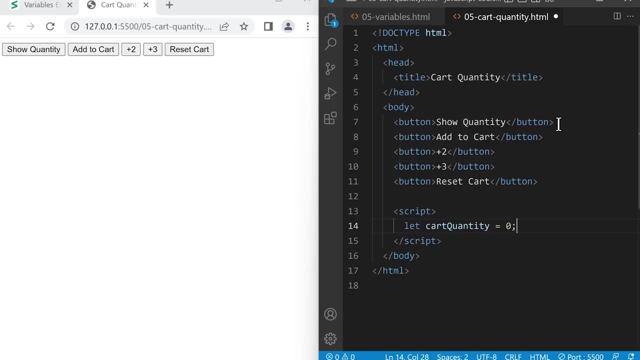 console to do this. we learned a special html attribute in the previous lesson called the on click attribute. so we're going to type in this opening tag here space on click equals and double quotes, so the on click attribute runs some javascript when we click this button and between 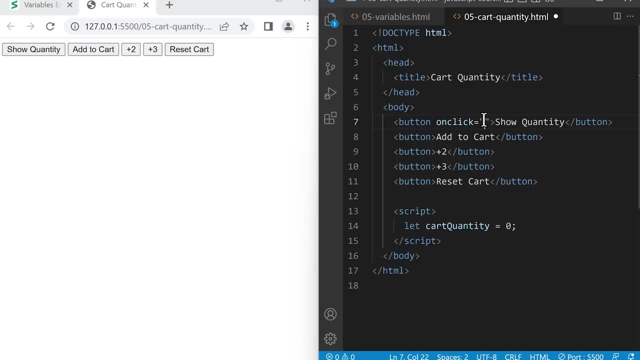 the double quotes. we can write javascript code, so let's press enter, enter. and now, when we click this button, we want to display the cart quantity in the console. so let's type console dot log, open bracket, close bracket, semicolon. and then, between the brackets, we're going to display. 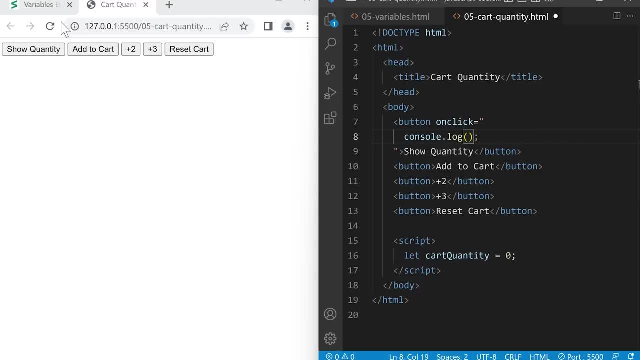 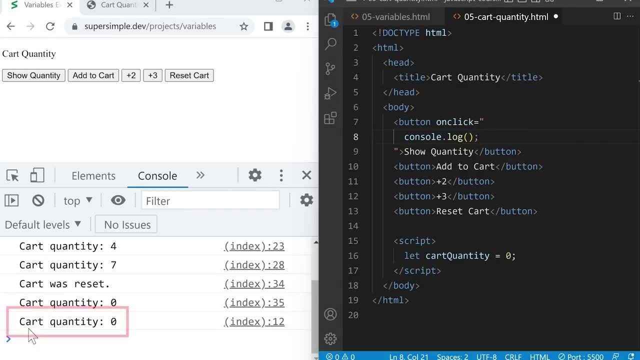 a message. now, if we go back to supersimpledev and we click show quantity, we want to display this message in the console. so in our code, between the brackets, we're going to type the string quote, cart quantity, colon zero. now let's save and go back to our 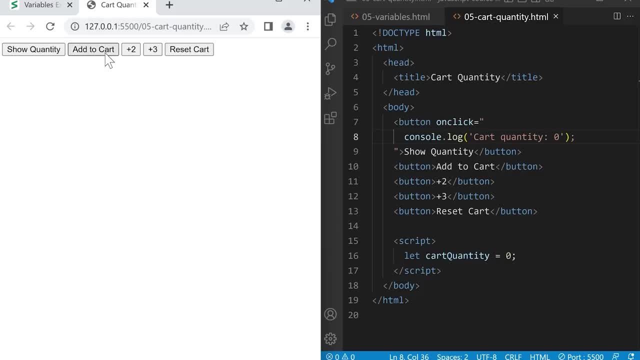 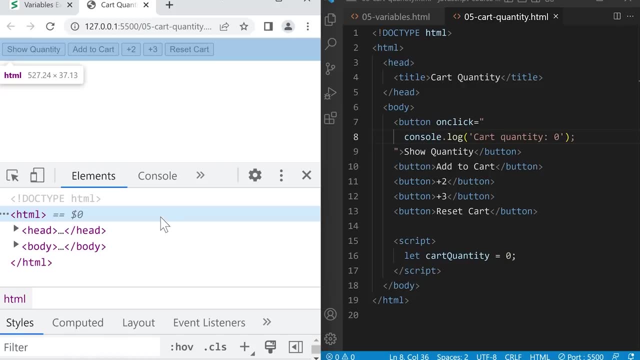 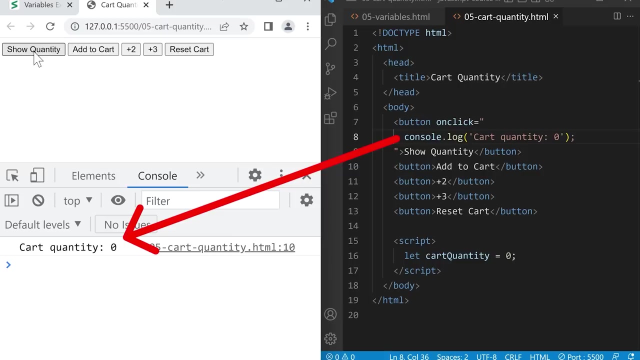 tab to try it out. so we're going to open the console first by right clicking and then click inspect and then click the console, and now, when we press the show quantity button, it should display that message in the console. ok, so we just made our project interactive. however, 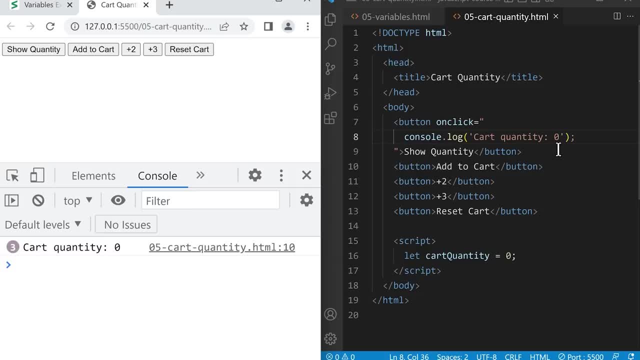 we obviously don't want to display zero every time. we want to display the value inside cart quantity, so we'll need to insert this value inside this string. remember from the strings lesson: when we want to insert a value into a string, we're going to use a template string. 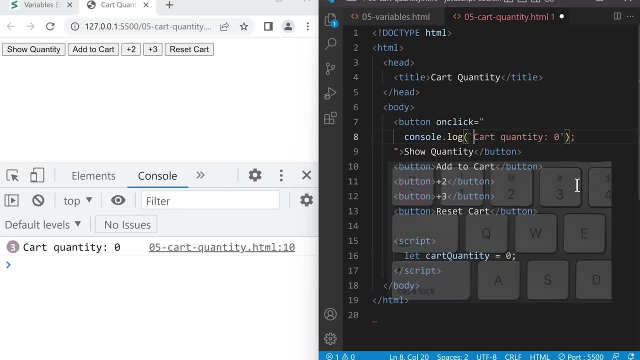 so let's switch the single quotes to back ticks to create a template string. and now, instead of zero, we're going to insert a value using dollar- open curly bracket and close curly bracket, and in between these brackets we're going to insert this variable: cart capital Q. 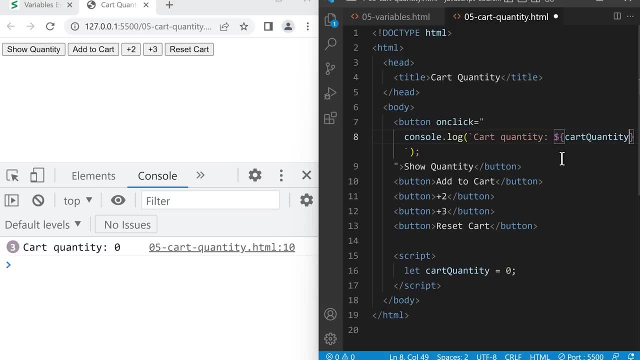 quantity. remember that javascript is case sensitive, so make sure you type the variable name exactly the same. now let's save and click show quantity again. and now it displays the value inside cart quantity in the console. so notice that variables also work with string interpolation. again we can use: 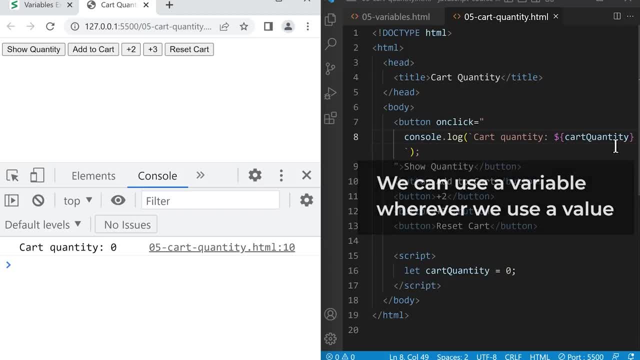 a variable wherever we use a value, and it will just substitute whatever value is saved inside this variable into the code. now let's make the rest of the buttons interactive. so when we click the add to cart button, we're going to add one to this cart quantity and display it. 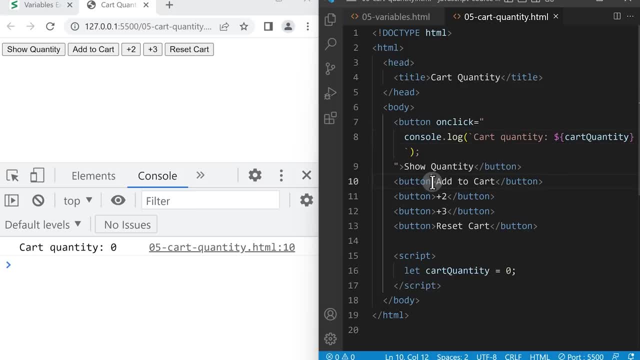 in the console. so again, we're going to type here and type space on. click equals double quotes, and between the double quotes we're going to add javascript. let's also add some new lines here to make our code easier to read. ok, so in the on click attribute, 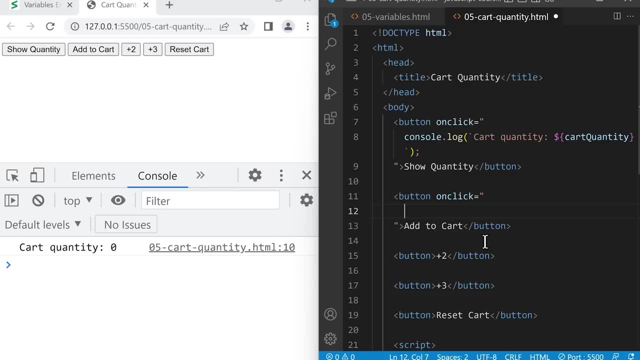 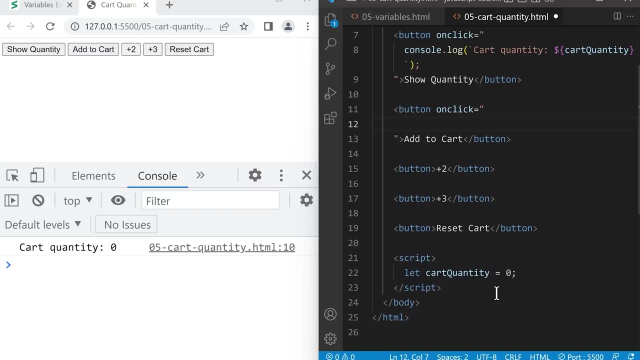 we're going to do two things. the first one is increase the cart quantity by one. we can do that by reassigning the cart quantity variable. so we're going to type just the variable name- cart quantity- and we're going to make it equal to itself. 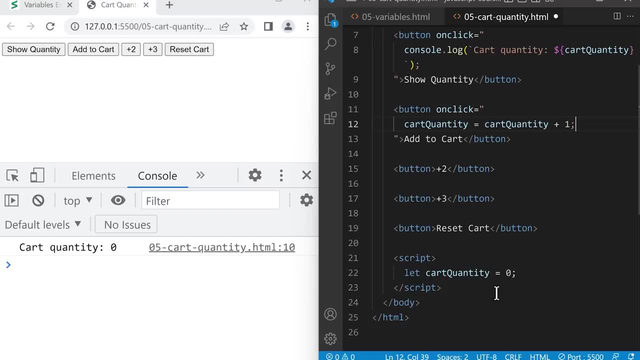 plus one and semicolon. next we're going to display the updated quantity in the console. so let's press enter and we're going to display this message again so we can actually just copy this code. so we'll select it and then right click and copy and then here: 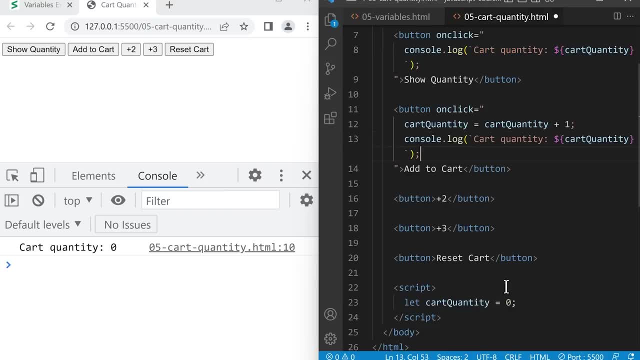 right click and paste. now, if we save and click the add to cart button, we'll see that it increased the quantity by one and displayed the updated quantity in the console. let's press it again to make sure it works. so it increases it by one again and then displays it in the console. 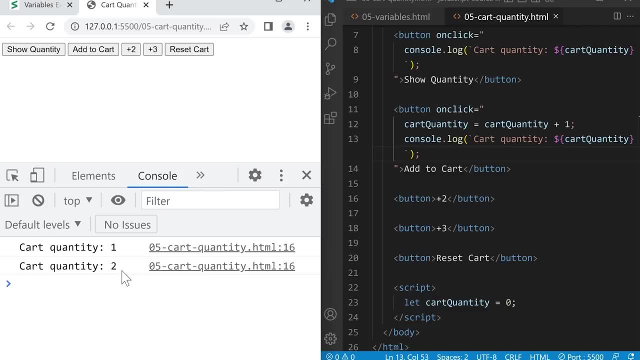 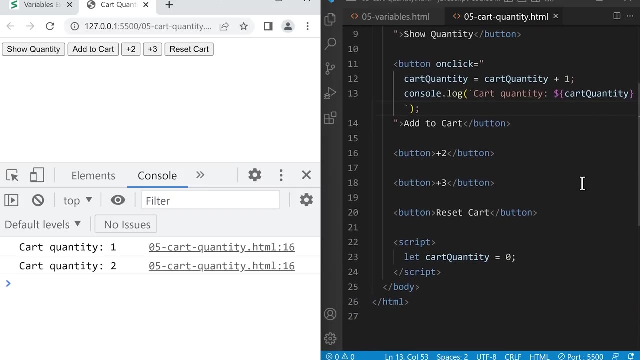 so that's basically how the cart quantity feature works in the final project. first we need a variable to save the quantity and then, when we click a button, we're going to update the quantity. so now let's make the rest of these buttons interactive. feel free to pause the video. 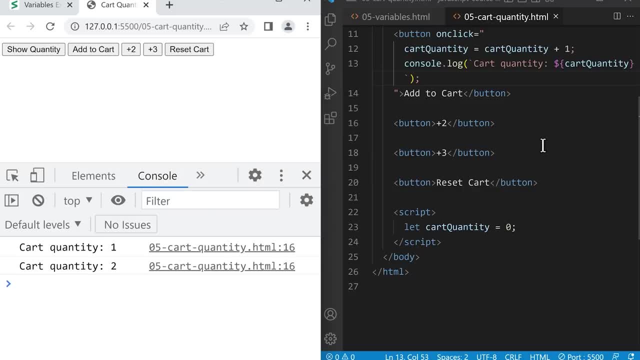 if you want to try it yourself. for the plus two button we're going to add the on click attribute again, on click equals double quotes, and inside we're going to increase the cart quantity by two, so cart quantity, and then we'll just make it equal to itself. 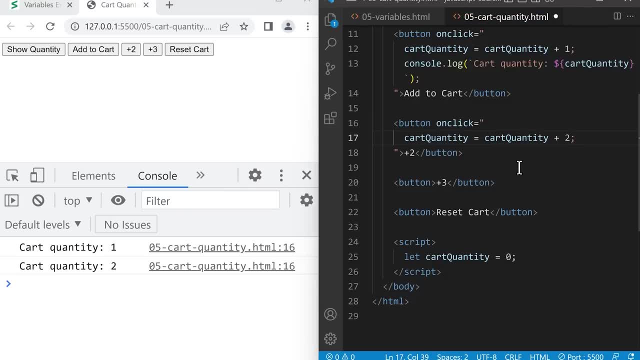 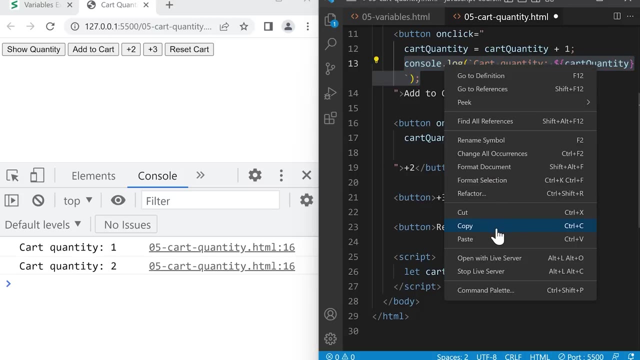 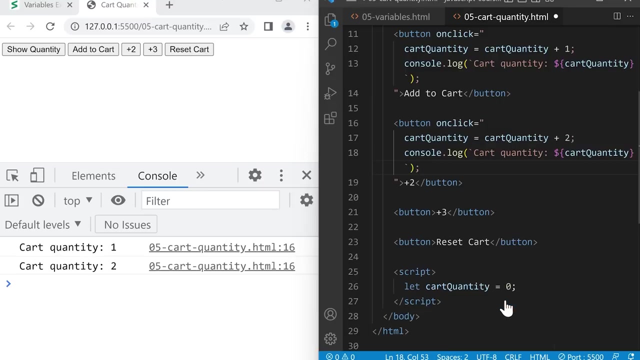 plus two and semicolon. and again we're going to display the updated quantity in the console so we can create a new line and just copy this code. so select it, right click, copy and here right click and paste. let's save and click plus two a few times. 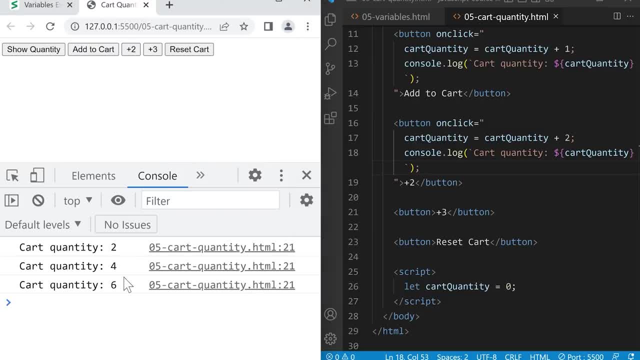 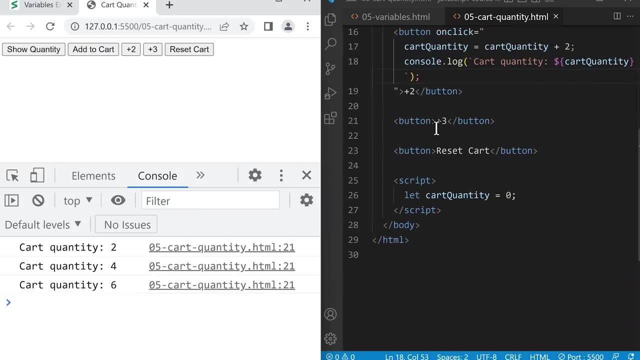 and we can see that it adds two to the cart quantity and displays it in the console. for the plus three button we'll do the same. let's type an on click attribute. click equals double quotes, and here we're going to increase the cart quantity by three. 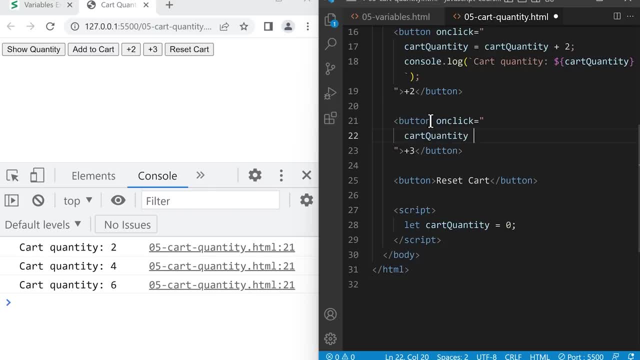 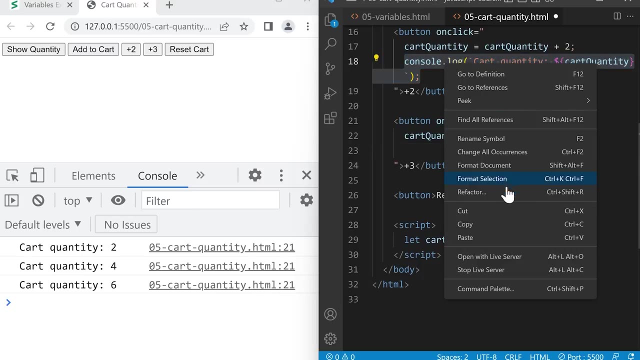 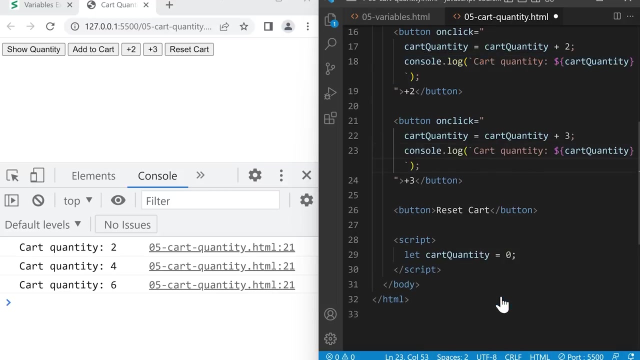 so cart quantity equals itself plus three and semicolon, and we're going to display this in the console again. so we'll select this right click, copy and here right click and paste. let's save again and try it out to make sure it works. so plus three. 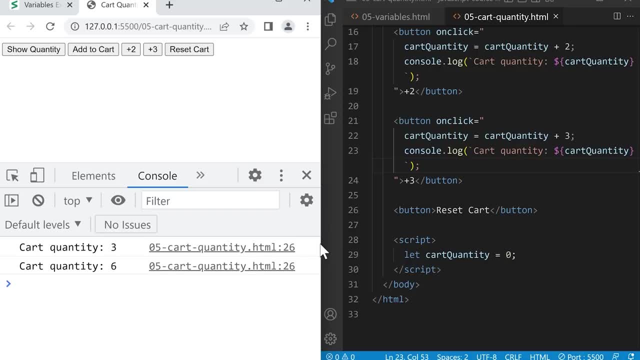 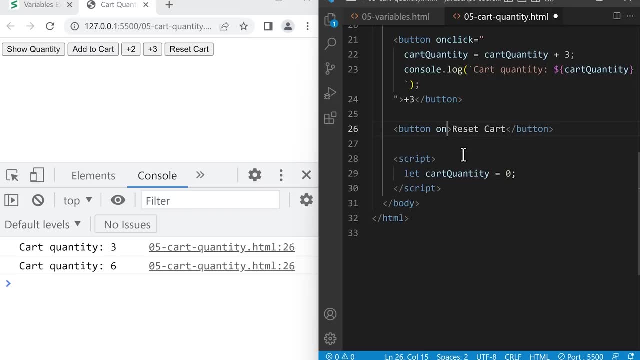 plus three. and finally, let's do the reset cart button. so we'll add the on click attribute again. on click equals double quotes and inside the double quotes we're going to do something a little different this time: instead of increasing the cart quantity, we'll set it back to. 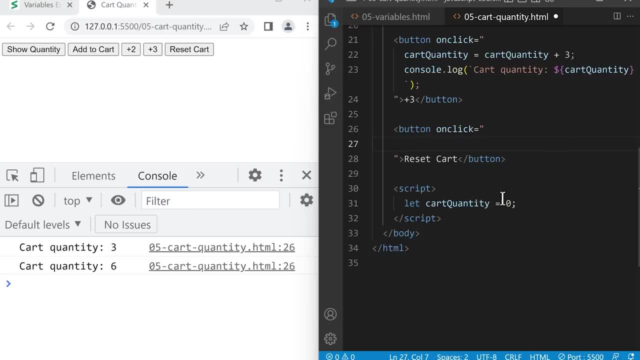 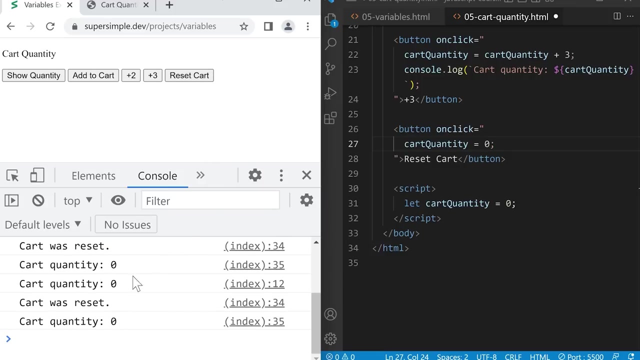 zero. to do this we can just reassign the cart quantity variable- so cart quantity- and just make it equal to zero and semicolon. now, if we go back to supersimpledev and try out this reset cart button, you'll notice that it displays two messages. the first message is: 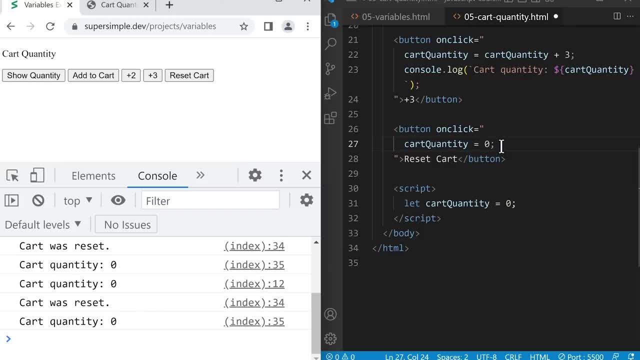 cart was reset. so we're going to display that message in our code. first console dot log and the string cart was reset, and the second message is the same message as the other buttons, so we can just select this and then right click, copy and then here right click. 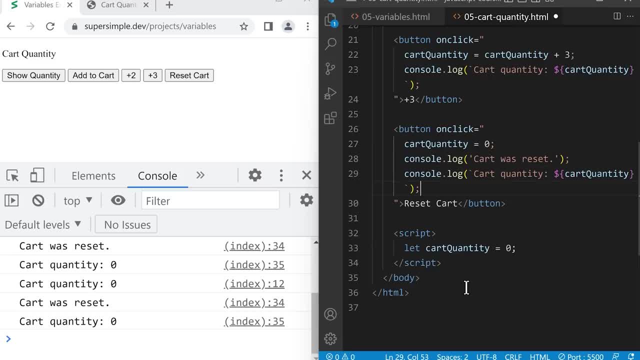 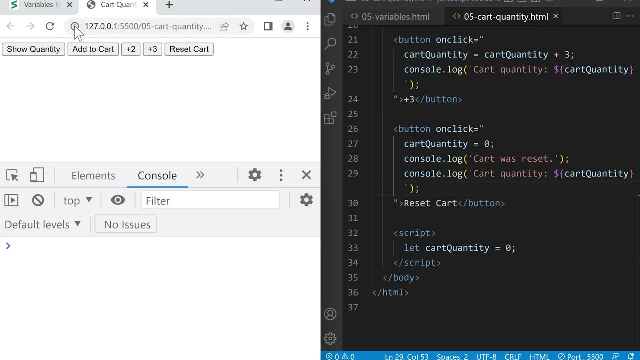 and paste. and now let's save and go back to our tab and give this a try. so the cart quantity starts at zero. when we press add to cart increases by one, this increases by two, this increases by three and when we click reset cart, it'll display: 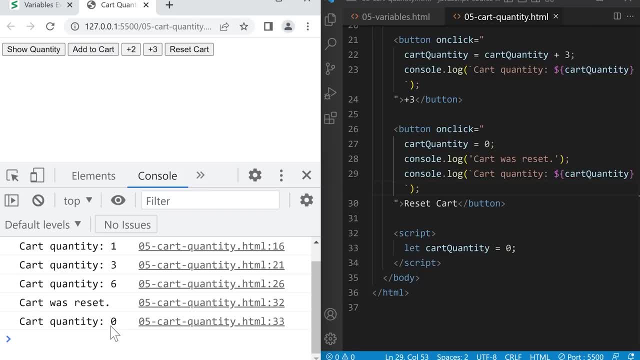 cart was reset and reset the cart quantity back to zero, and that's it. we just created a simple version of the cart quantity feature of our final project, using everything that we learned in this course so far. now we're going to learn some shortcuts for reassigning. 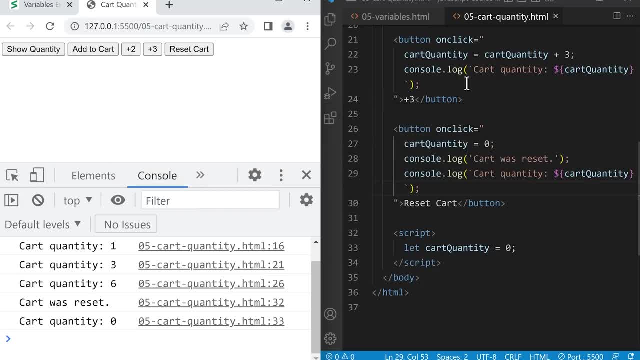 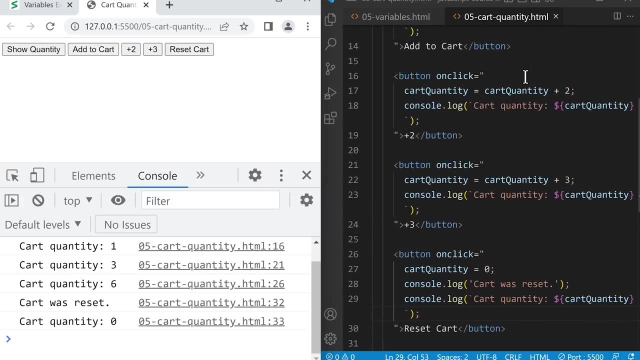 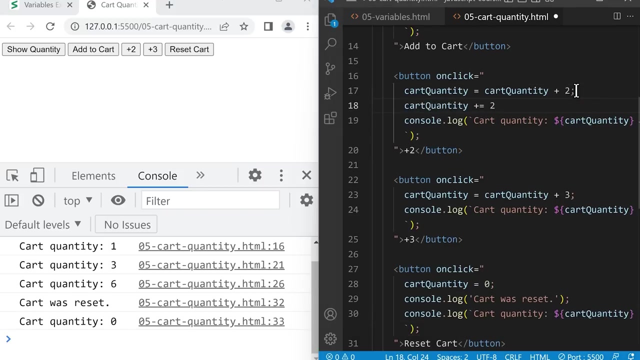 variables. so if we look at this line of code here, we're increasing the value of this variable by two and then saving it back. well, there's actually a shortcut for this, and that shortcut is cart quantity plus equals two and semicolon, so this does the same. 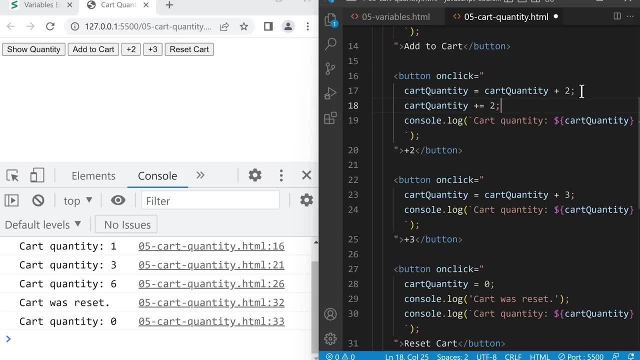 thing as the line above, but it's just shorter. the plus means we're going to add two to cart quantity and equals means we're going to save that result back to cart quantity. so we can actually delete this line and the code will work the same way. 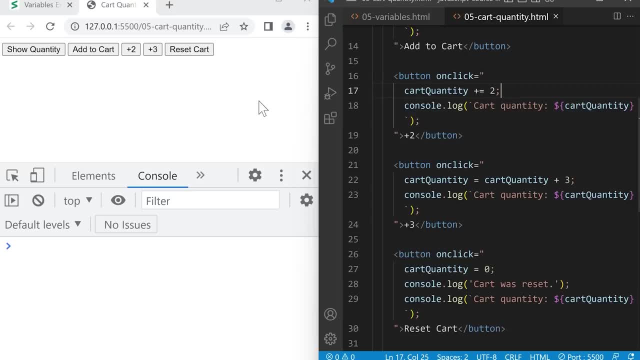 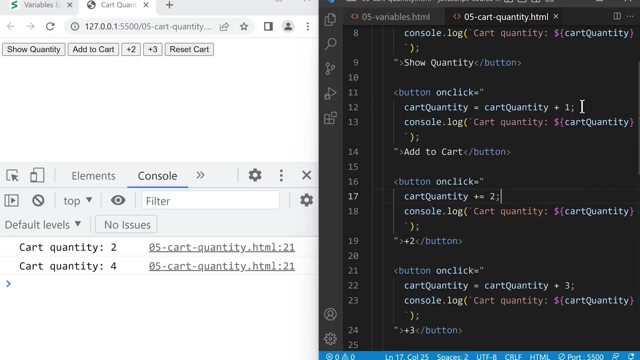 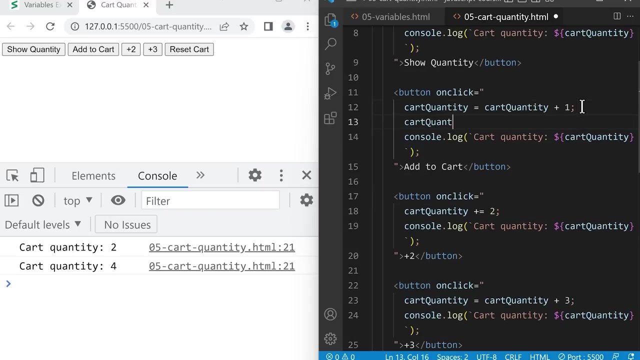 if we save and try it out, it will still add a two and then save it back in cart quantity. let's scroll up and practice by using this shortcut for cart quantity plus one, so instead of this line we can type: cart quantity plus equals one and semicolon. 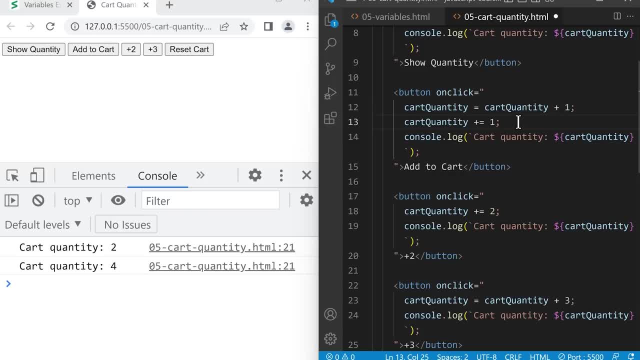 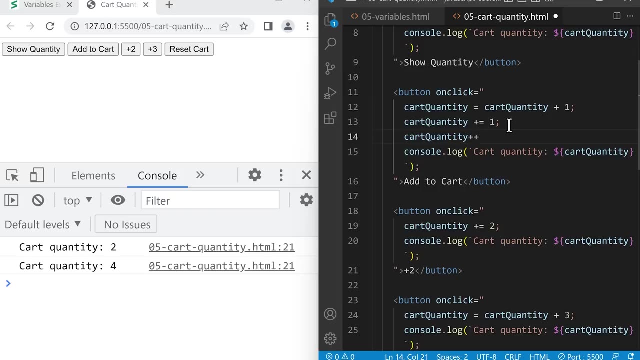 so it turns out that in programming plus equals one is so common that we have an even shorter shortcut for plus equals one, and that shortcut is cart quantity plus, plus and semicolon. so this is the same thing as plus equals one, and all three lines do the same thing. 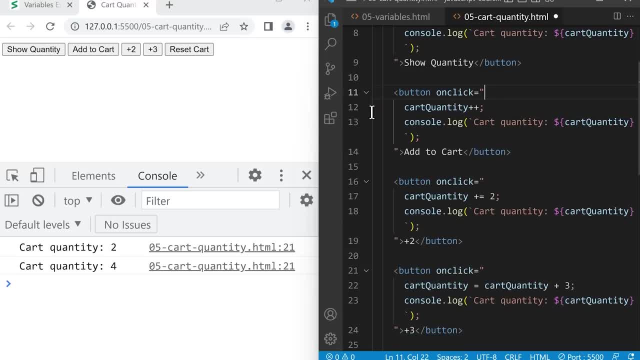 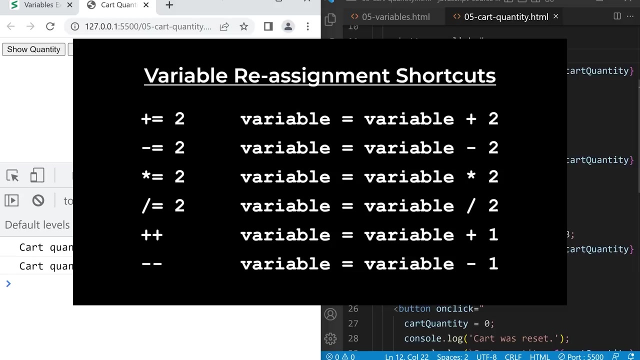 so we can remove these lines and the code will work the same, because it's just a shortcut. if we save, so if we click add to cart, it will add one every time. so those are some shortcuts for reassigning variables. we also have these shortcuts for the other operators. 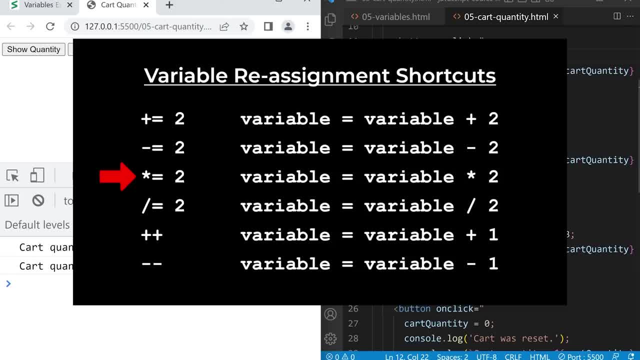 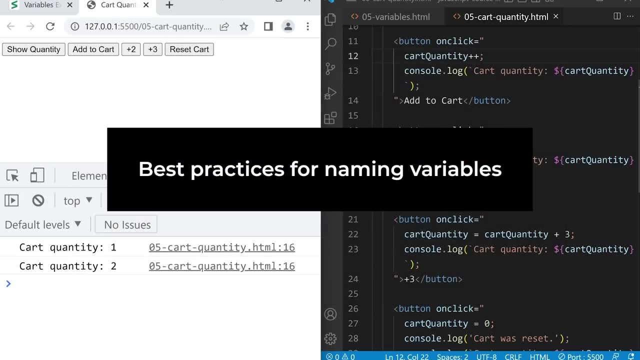 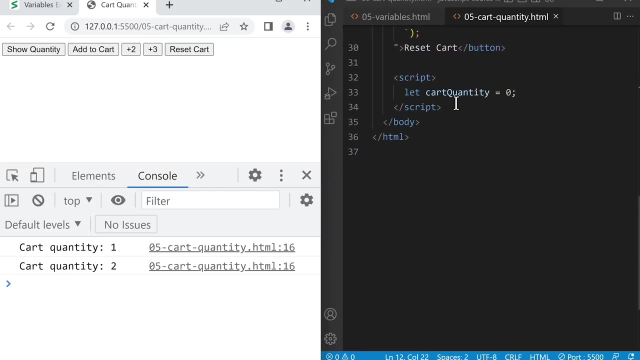 like minus equals, multiply equals, divide equals and minus minus. we'll leave some exercises for these other shortcuts at the end of this lesson. next we're going to learn some best practices for naming variables. so if we scroll down, notice that our variable cart quantity has two words in it. 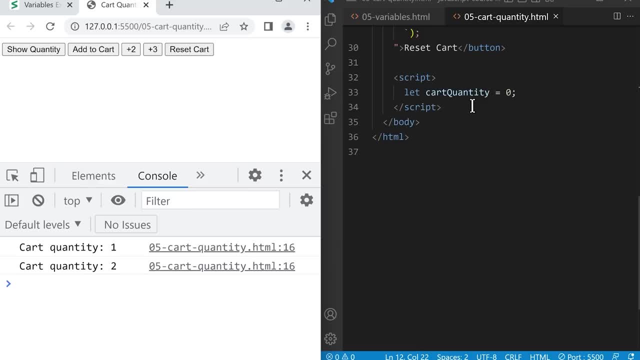 cart and quantity. we learned earlier that we can't have spaces in a variable name, so if we want to have multiple words, we have to combine them together like this. now you might be wondering why we wrote it this way, with a lowercase c and a capital q. 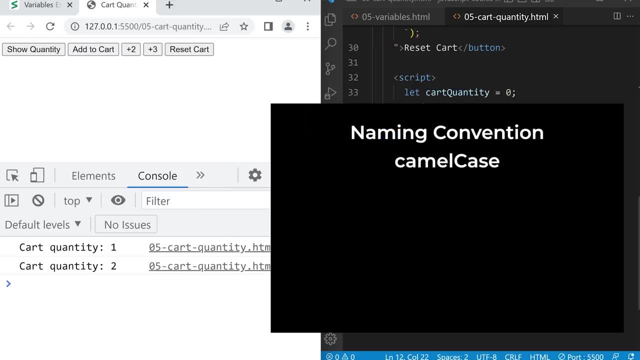 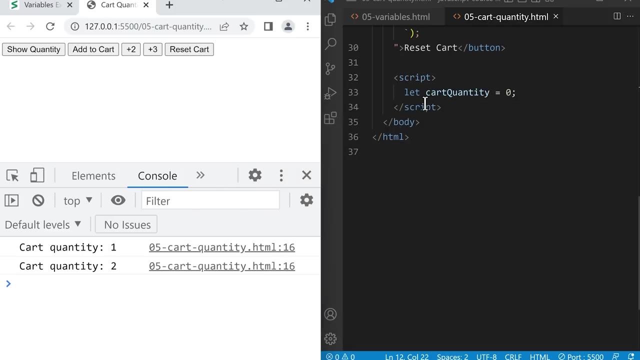 this is actually a naming convention called camel case. in camel case we combine the words together and capitalize every word except the first word. so for cart quantity we capitalize quantity but we keep cart lowercase because it's the first word. camel case is actually the standard naming convention. 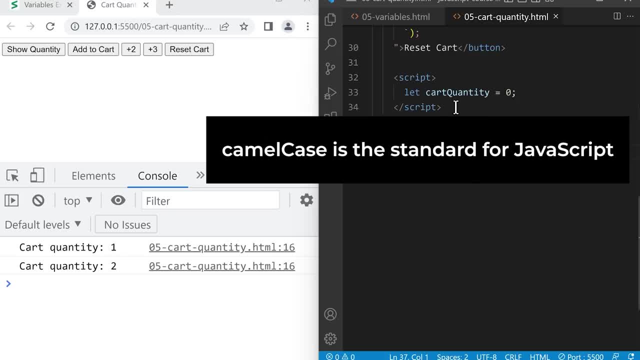 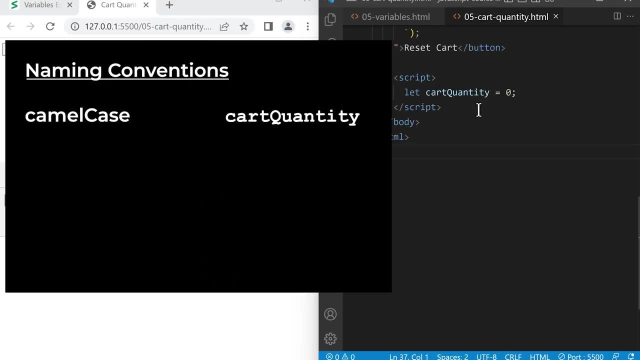 for javascript, all of our variable names should use camel case. now in programming there are other naming conventions that exist. another one is called pascal case. pascal case is the same as camel case, except we capitalize the first word. so for cart quantity, pascal case would be. 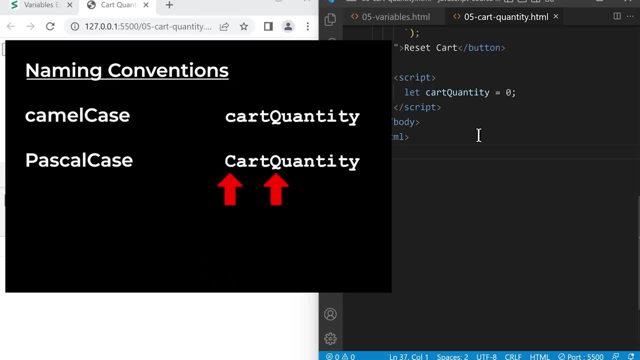 capital cart and capital quantity. in javascript there is one feature where we use pascal case, which we'll learn later in this course. for everything else we use camel case. another naming convention is kebab case. here we keep the words lowercase and combine them with a dash. 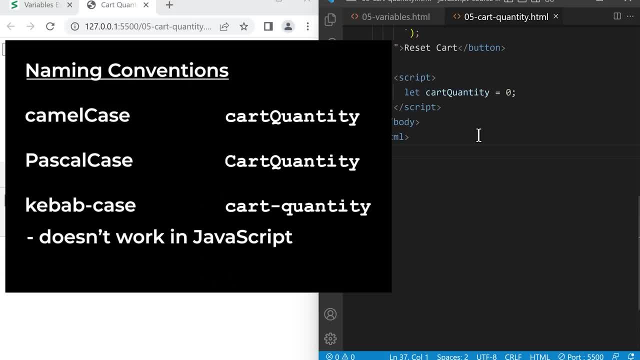 like cart dash quantity. kebab case doesn't work in javascript. it's already a minus symbol. however, we use kebab case in html and css and also in our file names, as you can see here. and finally we have snake case, where we keep the words lowercase. 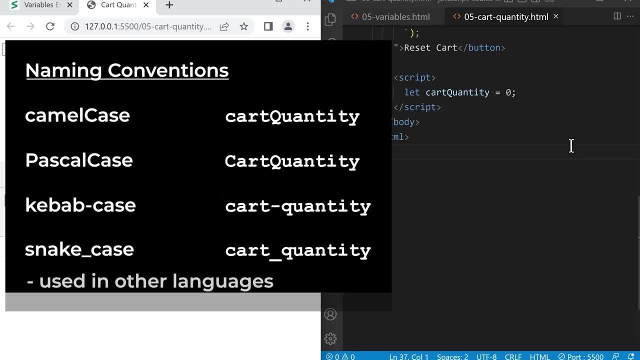 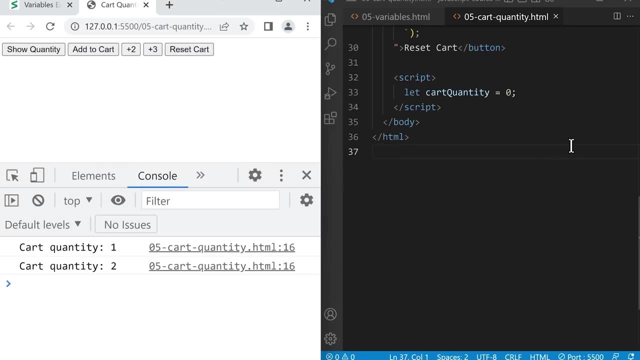 and combine them with underscores. snake case is used in other languages, but it's not really used in javascript, so those are the common naming conventions used in programming. now, one more thing I want to note is that when we name our variables, try to pick a name that is not too short. 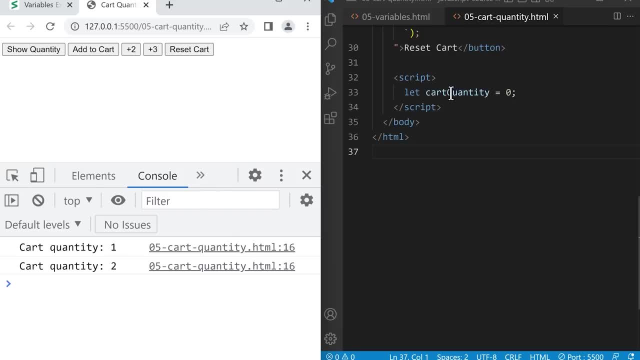 or too long. for example, instead of cart quantity, we could have named this variable c, but this name is too short. it's hard to understand what c means. we could also use a name like this: quantity of products in the cart, but this name is too long. it's hard to read this in the code. 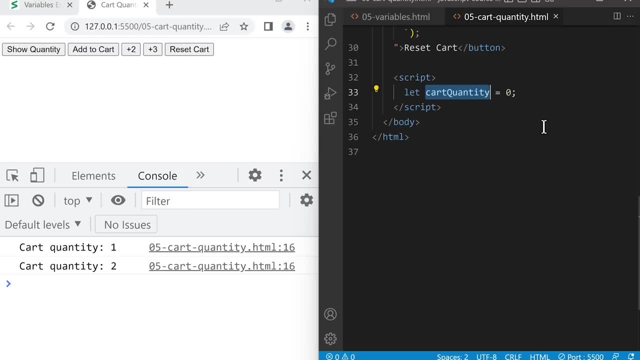 so try to have a balance between a name that is understandable but not too long, like cart quantity. the last thing we're going to learn in this lesson is there are three ways to create variables in javascript. let's go back to our variableshtml file and we're going to learn those three ways. 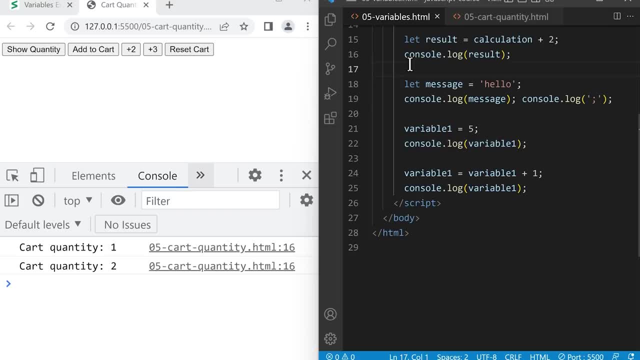 so the first way is to use let, which we already learned. the second way to create a variable is to use the word const, so at the bottom we can type const space and then a variable name like variable 2 and make it equal to 3. so const creates a variable. 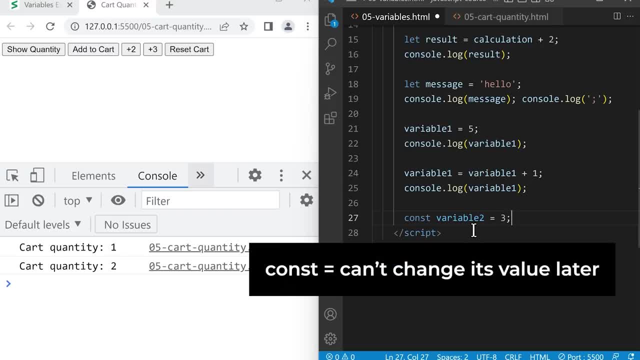 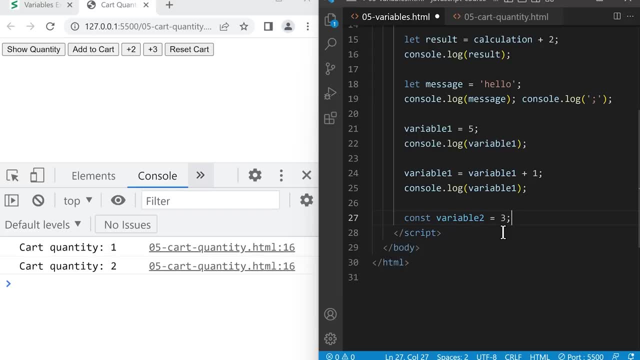 just like let, except we can't change its value later. this value stays constant. that's why it's called const. if we try to change its value, like variable 2 equals 5, and then we save this and we open this file in the browser by right clicking. 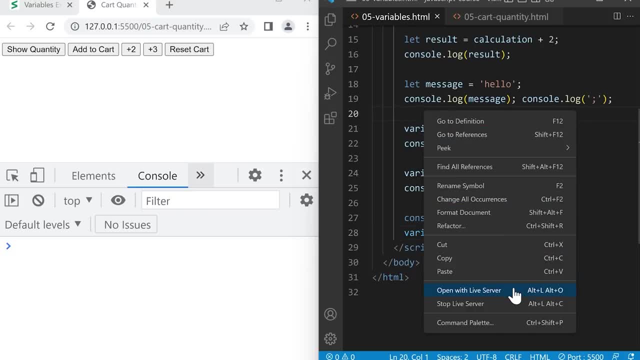 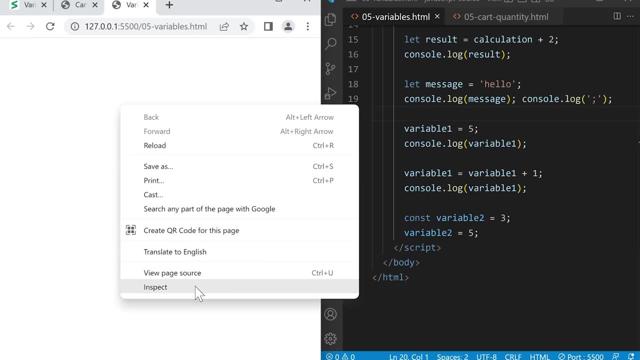 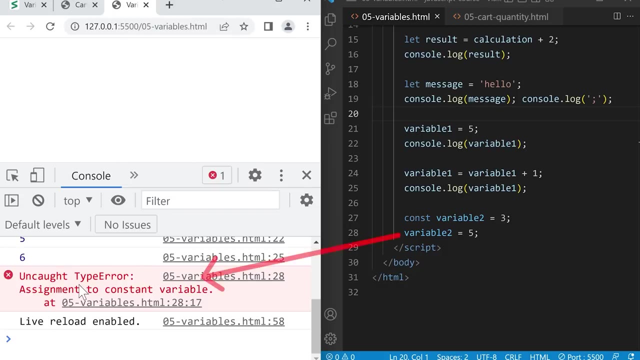 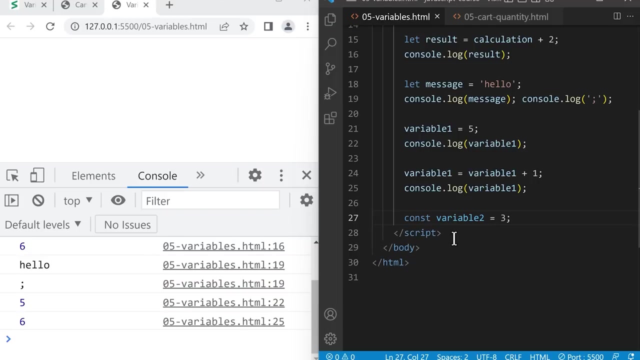 and then open with live server and then the console. so right click inspect and then click the console. it will give us an error when we try to change this variable. so this doesn't work. let's remove this line and save. so why would we ever use const instead of let? 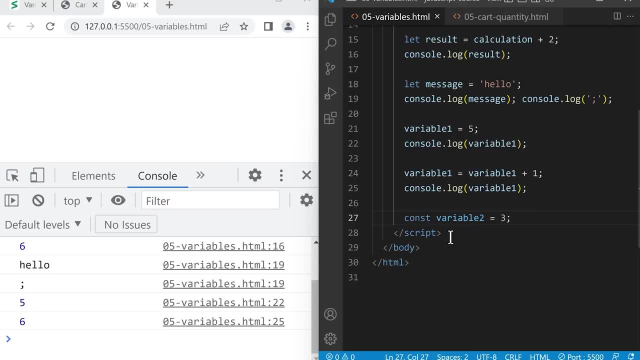 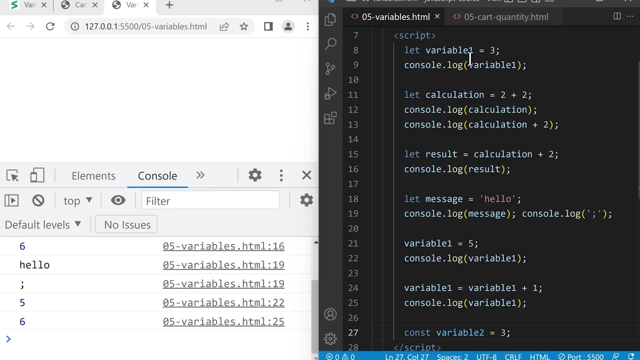 well, const makes our code safer and easier to understand. when we create a variable with const, we know for sure that this variable will always contain 3 for let. however, if we create a variable, it's hard to know what value is inside this variable, because later on we can. 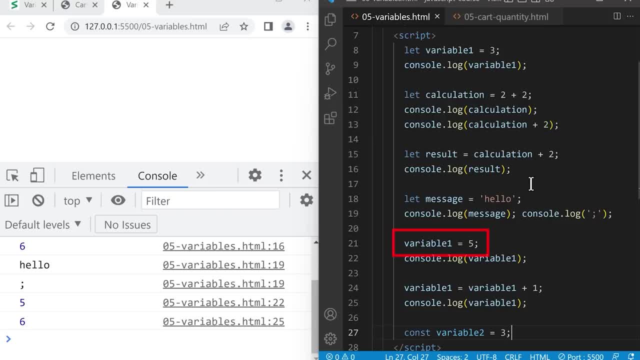 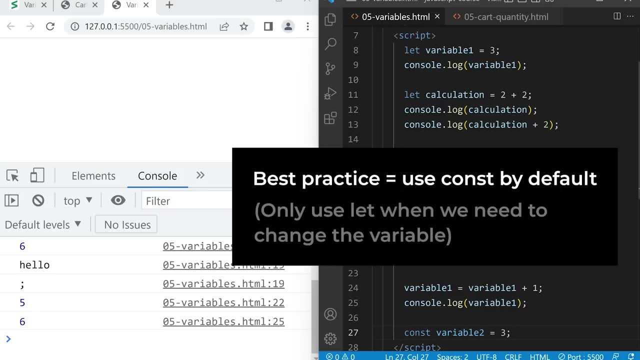 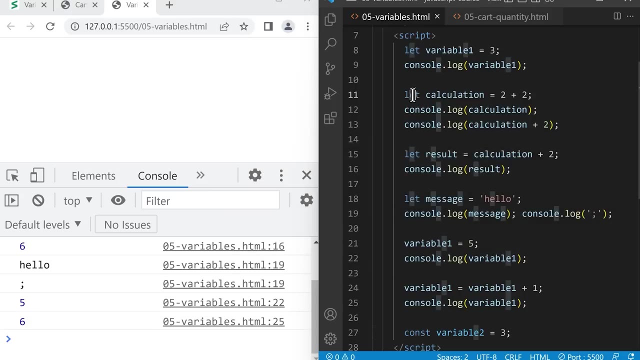 change this value in our code. so, in order to keep our code safer, it's actually a best practice to use const by default and only use let when we know that we need to change the variable. so here it's actually best practice to use const to create this calculation variable. 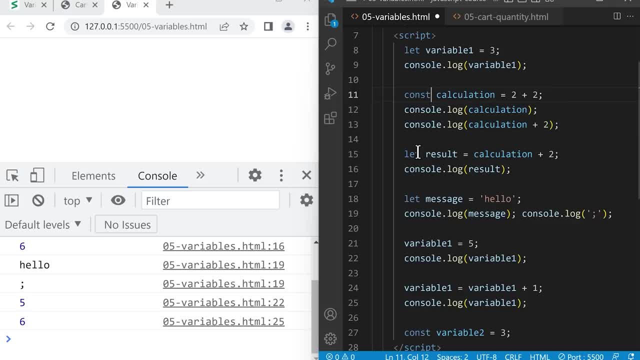 because we're not changing it later. same thing for the result variable and the message variable. now, for variable 1, we have to use let, because we're changing it later in this code. so that's const. it creates a variable that can't be changed later. finally, the third way of. 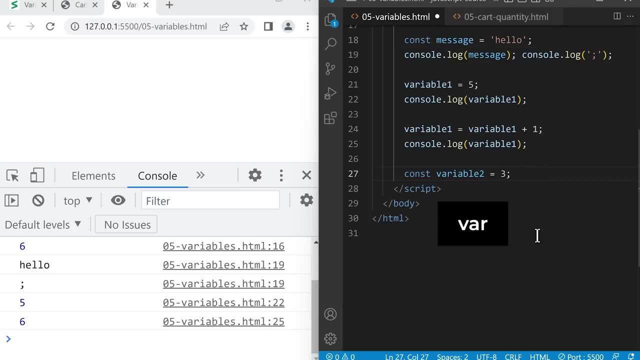 creating a variable is to use another word, var. so at the bottom we can type var space and then a variable name like variable 3 and make it equal to 3. so var creates a variable just like let, and this variable can be changed later. var is actually the original way. 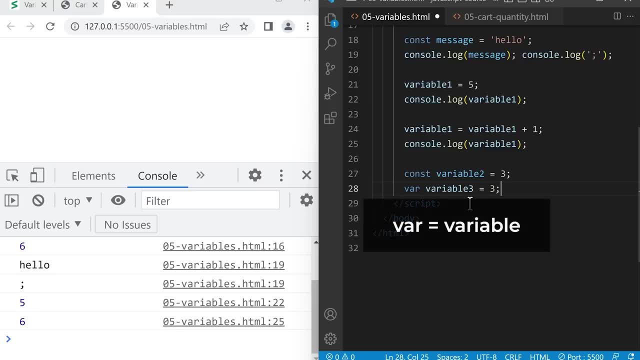 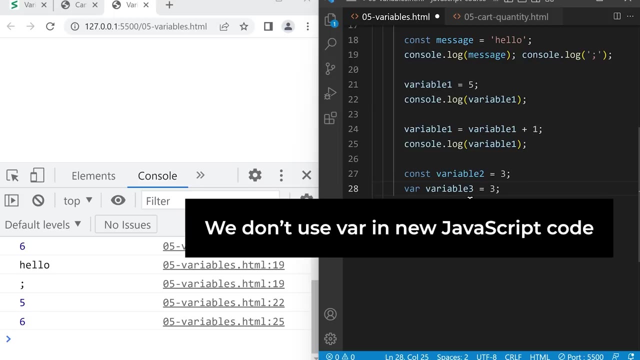 to create variables in javascript. var means variable. however, var has some issues that we'll learn later in this course and because of these issues we don't use var in new javascript code. you might see var in older javascript code, so it's still useful to know. so those are three. 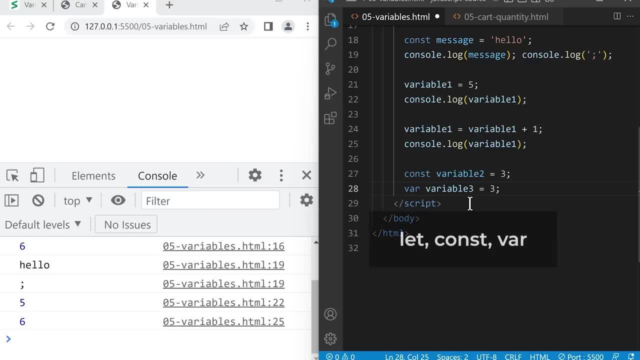 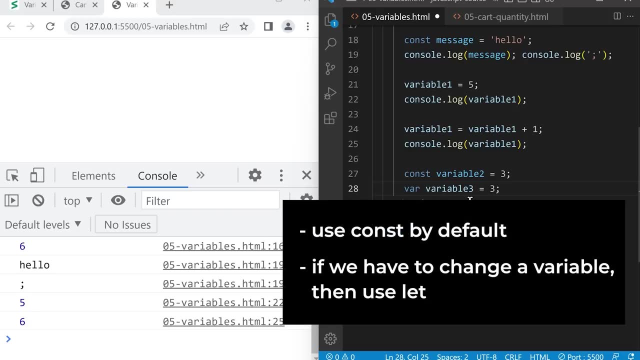 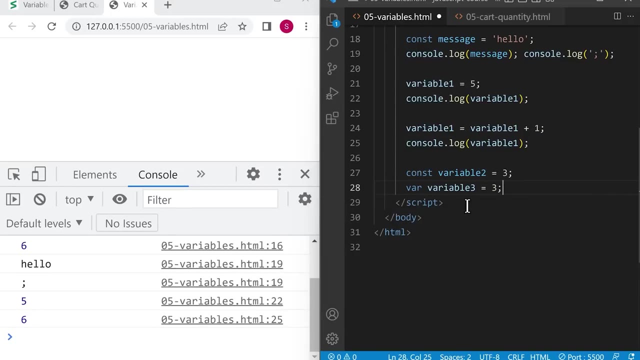 ways to create variables in javascript: let const and var. we use const by default, and if we have to change a variable, then use let. so one more thing we're going to learn is that we can use type of with variables. so remember that type of tells us what type a. 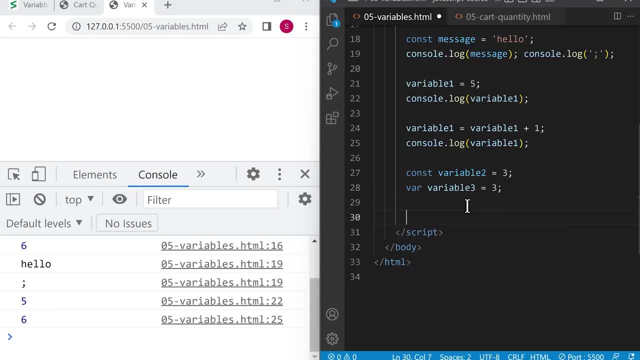 value is. for example, if we wrote console dot log type of 3 and save, type of will tell us that 3 is a number. well, we can actually use type of with a variable. so if we change this to variable 2 and save, type of will tell us the type of. 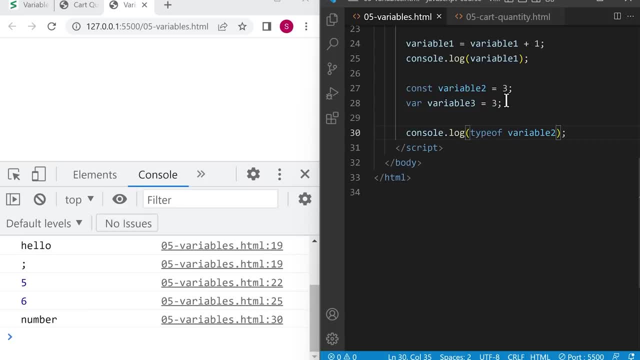 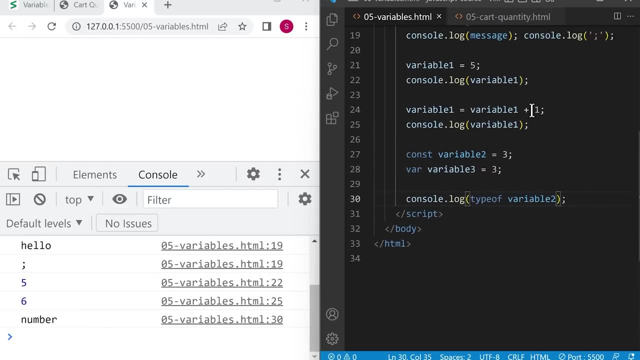 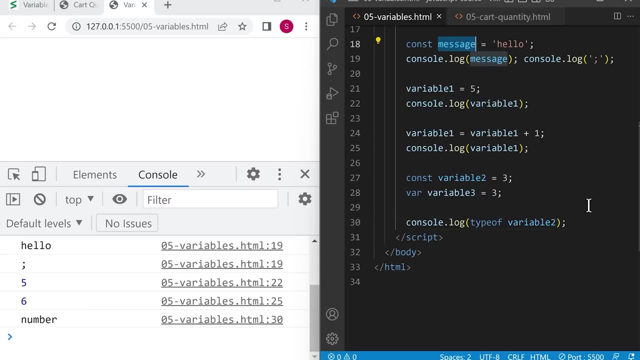 value inside the variable, which is a number, and that's what we see in the console. now let's check the type of this variable message. so message contains a string and if we do console dot log type of message and save, this will tell us that the value inside 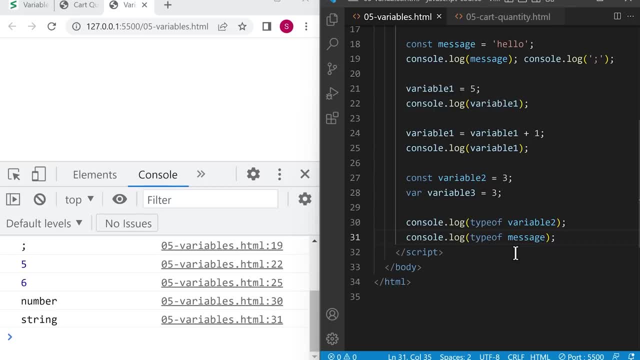 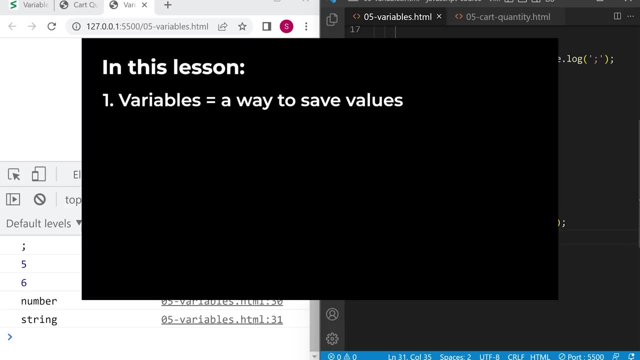 the message. variable is a string, so we can use type of to check the type of value that is saved inside a variable. and that's the end of this lesson. in this lesson we learned about variables, which are a way to save values and use them. later we learned 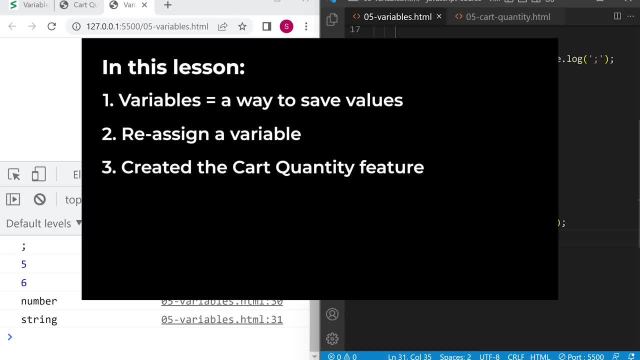 how to reassign a variable. we created the cart quantity feature of the final project. we learned some shortcuts for reassigning a variable. we learned some naming conventions and best practices for variable names and we learned 3 ways to create a variable: let, const and var. 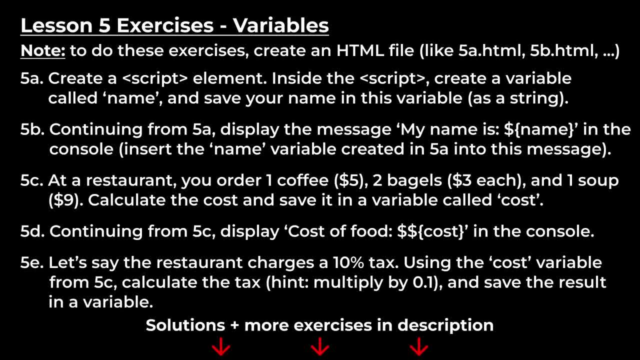 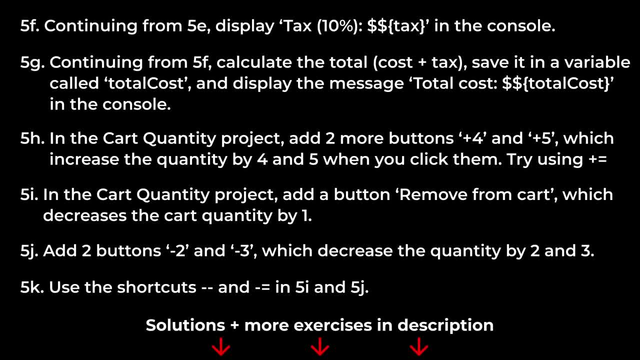 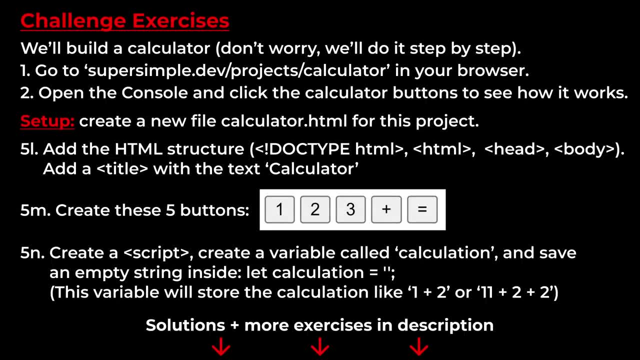 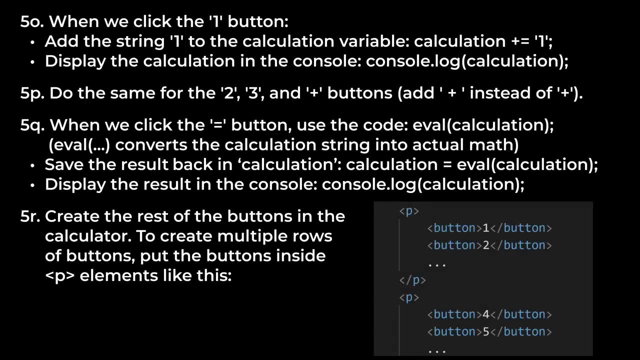 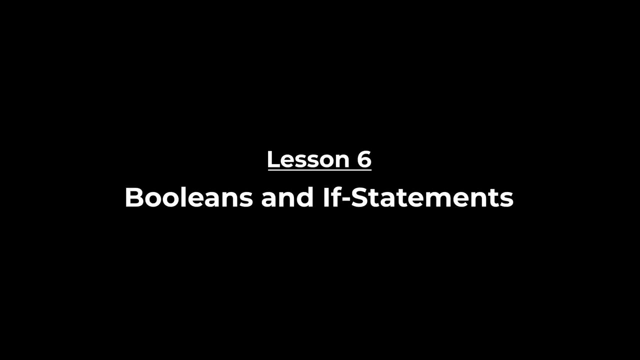 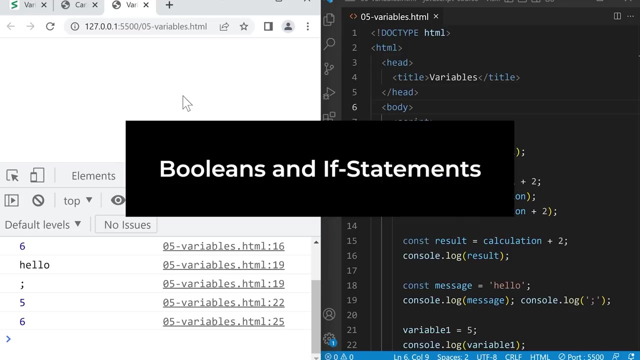 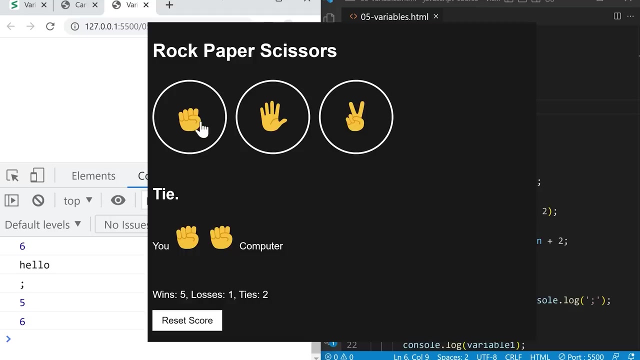 here's some exercises to help you practice using variables. in this lesson, we're going to learn two more features of javascript called boolean and if statements, and we're going to use these features to build this rock paper scissors project. let's start by creating a new html. 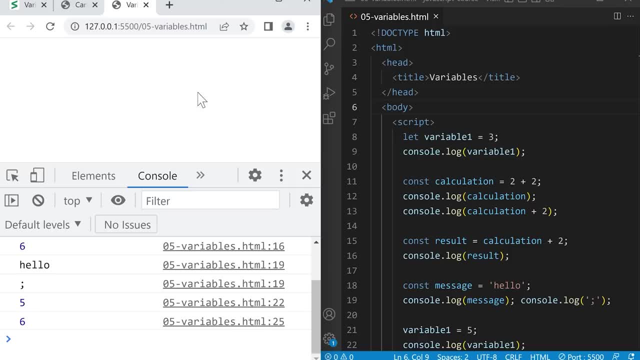 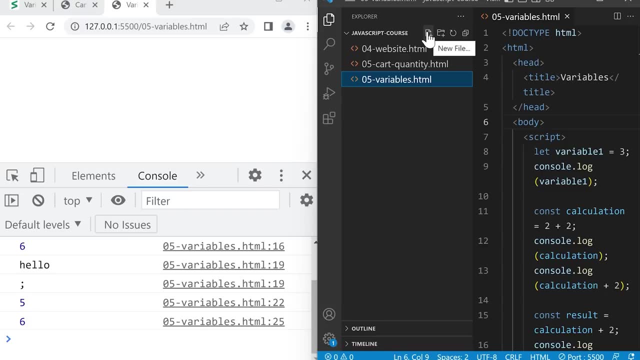 file for this lesson. we're going to go to our code editor and click this icon to show our files, and then click this icon to create a new file. we're going to name this file 06 dash booleans dot. html and press enter. let's open. 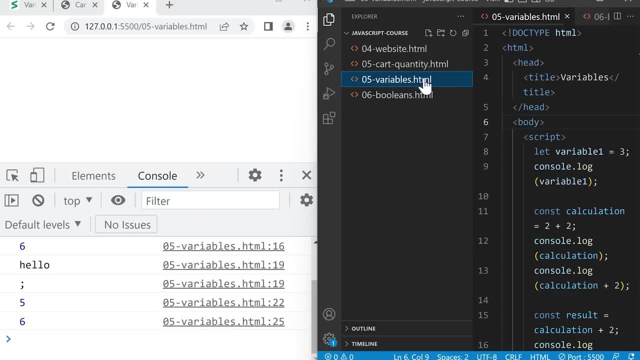 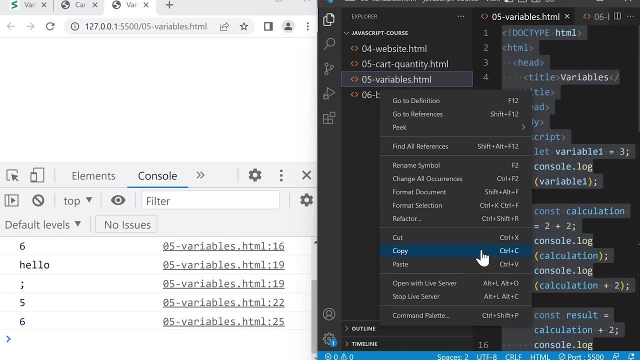 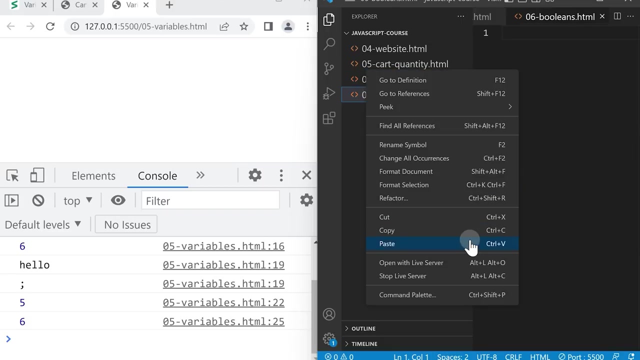 variables dot. html. and we're going to copy all this code into our new file. let's select the code using control a on windows or command a on mac, and then right click, copy and in here, right click and paste. let's close this for now and prepare this file for this. 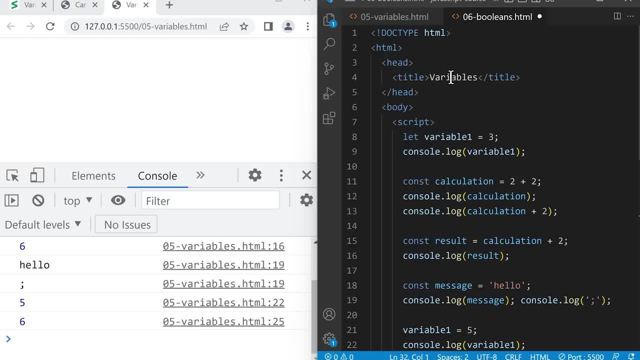 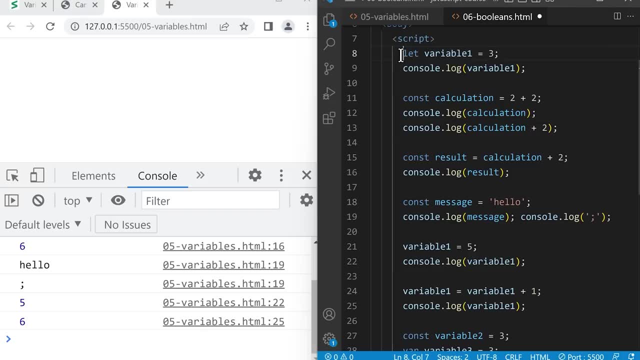 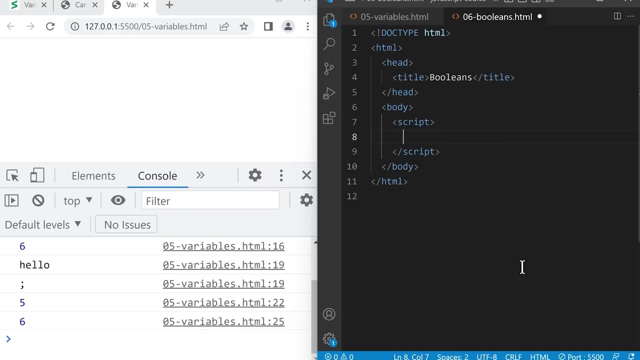 lesson. so we'll scroll to the top and change this to booleans and then remove all the javascript code, but keep the script element. now let's save and open this file in live server by clicking, and then open with live server and we can close the previous tabs. 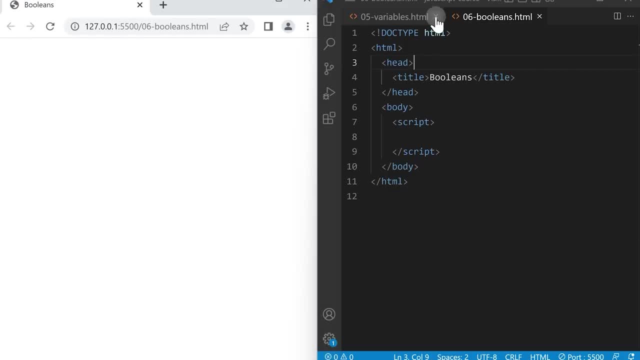 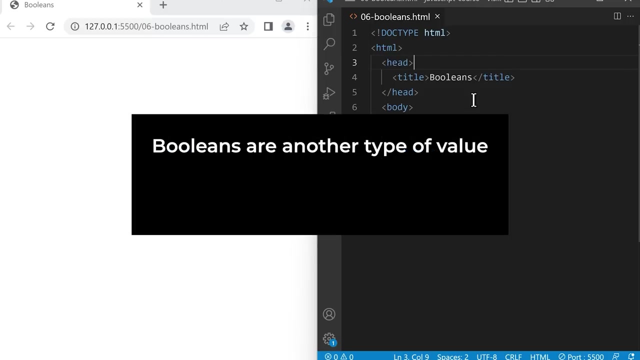 as well as the previous code. for now, we'll start by learning what are booleans. so far in this course, we learned two types of values in javascript: numbers and strings. booleans are another type of value in javascript, but booleans are special because there are only two boolean. 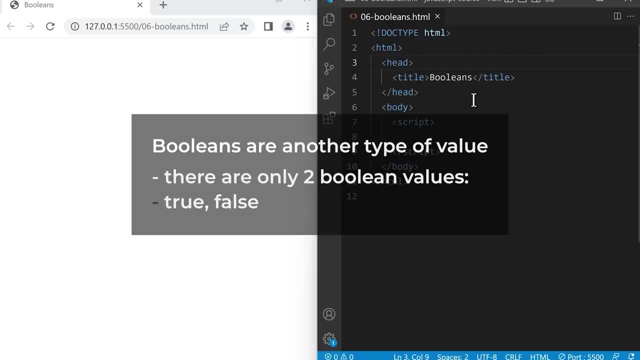 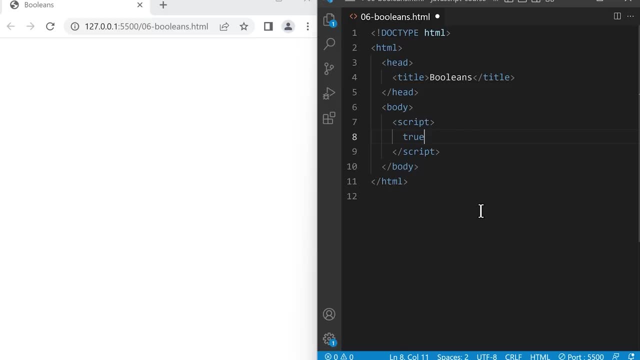 values true and false. let's click in the script element and type true, press enter and type false. so these are the only two boolean values that exist, true and false. so what's the purpose of boolean values? a boolean value represents whether something is true or false, for example in javascript. 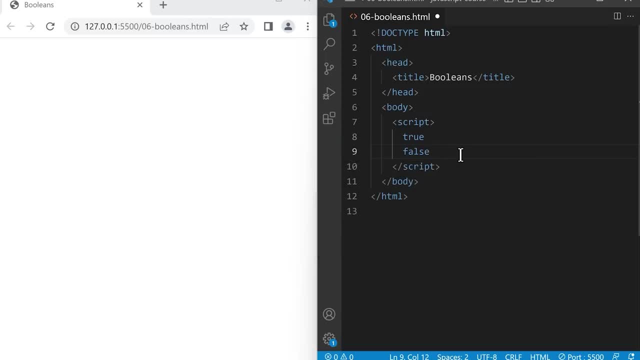 we can compare two numbers. let's create some new lines and type the code 3 less than 5. so this code checks whether the number 3 is less than 5 and of course this is true. so if we consolelog this code, consolelog and save. 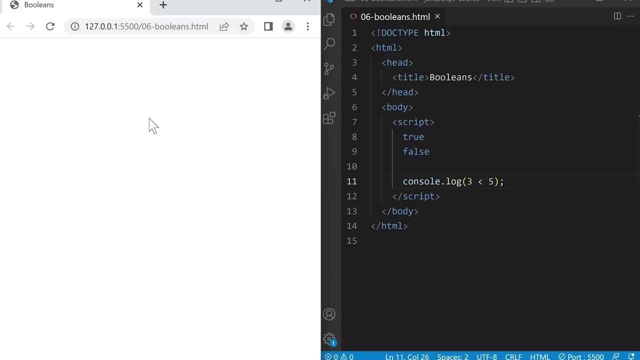 and then go to our website and open the console. right click, inspect and console. it will show us that the result of this code is the boolean value. true, let's try another example. let's delete this less than symbol and replace it with a greater than symbol. so now this code. 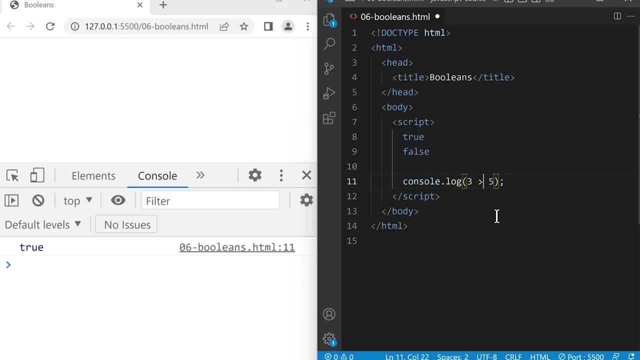 checks whether 3 is greater than 5, and we know that 3 is not greater than 5. so, if we save, the computer will tell us that the result of this comparison is the boolean value false. so, as you can see, a boolean value represents whether something 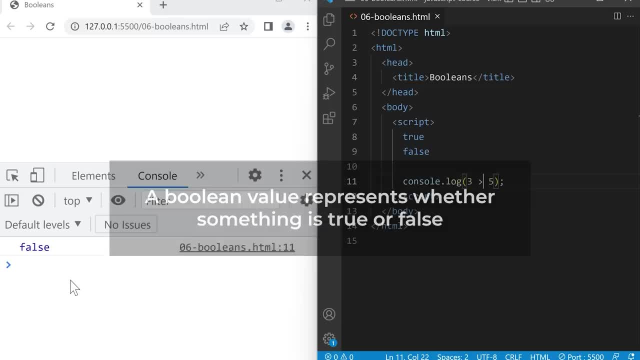 is true or false. now let's learn the syntax rules for booleans. to create a boolean, we just type true or false. note that we don't surround these with quotes like this. if we surround them with quotes, this is now a string, not a boolean. we can use typeof to check. 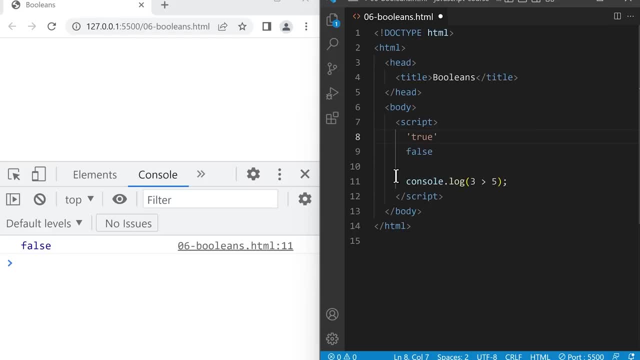 this. so at the front we can type: consolelog type of true. if we save this, will tell us that this is a string. now, if we remove the quotes and save this, will tell us that this is now a boolean. so when creating a boolean, don't put quotes around. true. 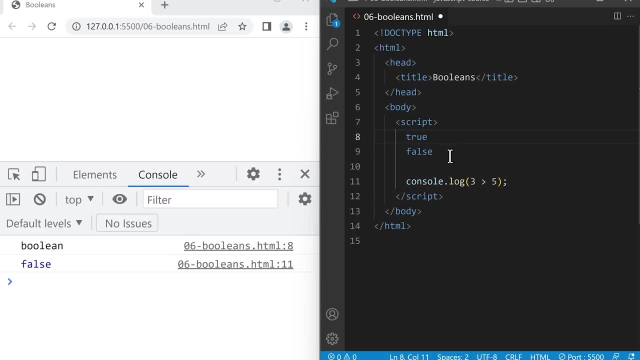 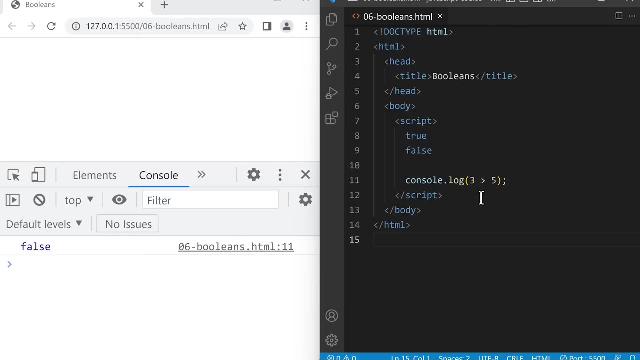 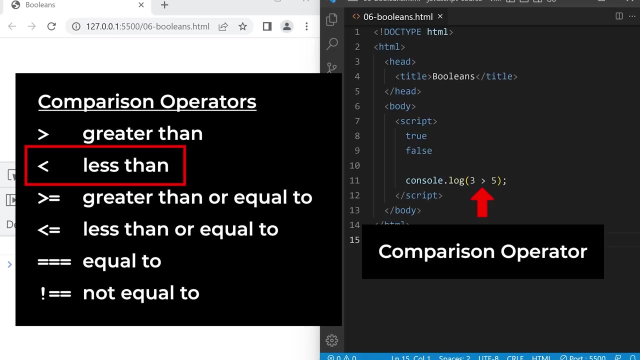 or false. let's save now. one way to create a boolean is to compare two numbers, for example three greater than five. so this greater than symbol is called a comparison operator, and there are many other comparison operators we can use. we saw less than earlier, and we also have greater than or equal. 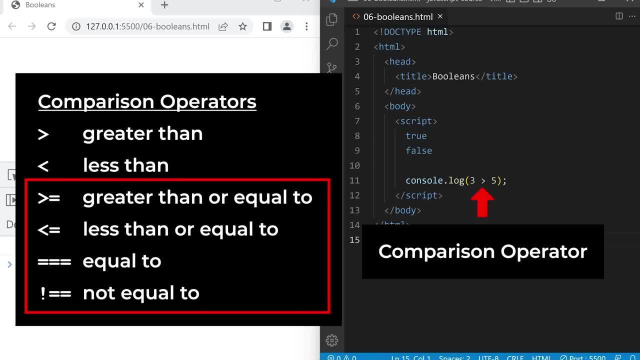 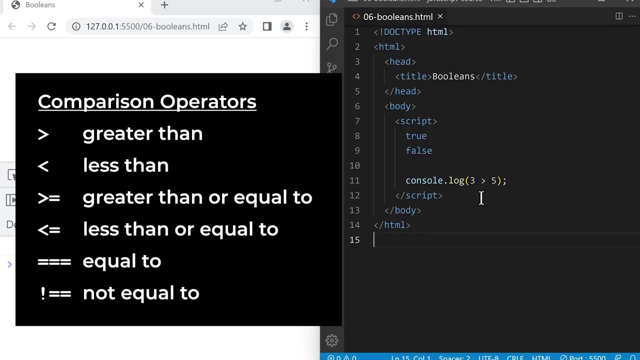 to less than or equal to triple equals, which checks if two values are equal to each other, and- exclamation, double equals, which checks if two values are not equal to each other. now, javascript is a little special because it has two ways to check if two values are equal. 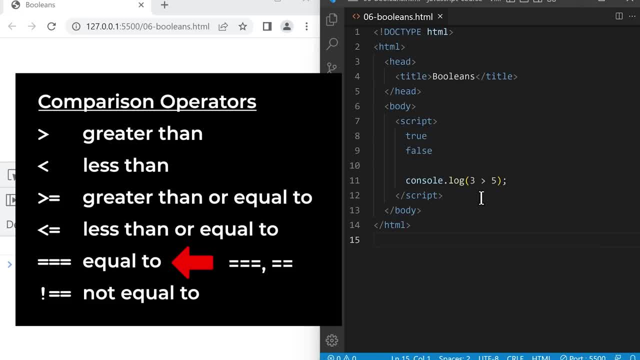 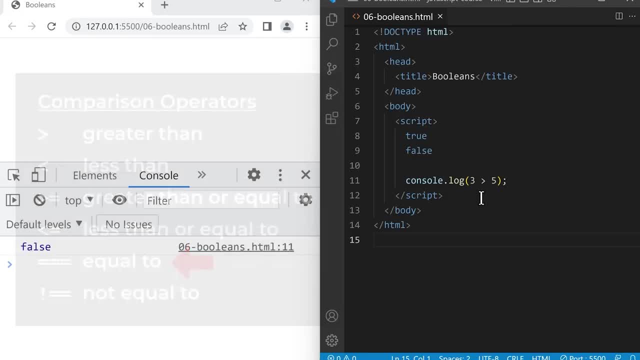 triple equals and double equals. the difference is that double equals tries to convert both values into the same type. for example, in our code, let's create some new lines and consolelog and let's check if the number five is equal to the string 5.00. 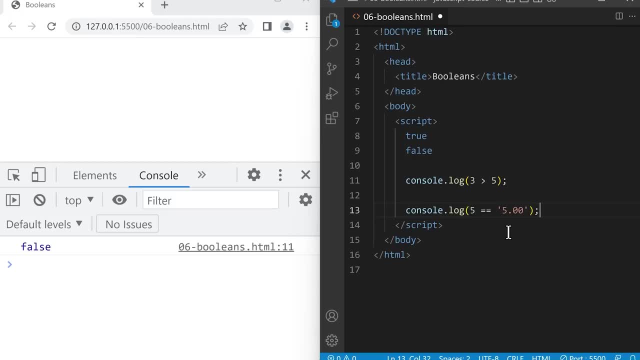 if we save, it will tell us that these two values are equal to each other, even though one of them is a number and the other is a string, and that's because the double equals converts both values into the same type, so converts both of these into the number five. 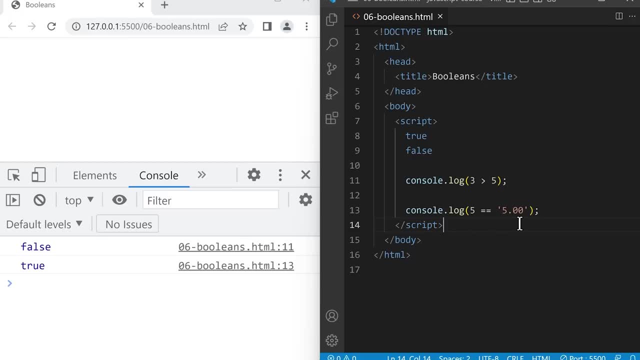 and then compares them. so that's why they are equal. however, this is not a good idea, because this value is a number and this value is a string. it's a piece of text, so they shouldn't really be equal to each other. that's why, in javascript, 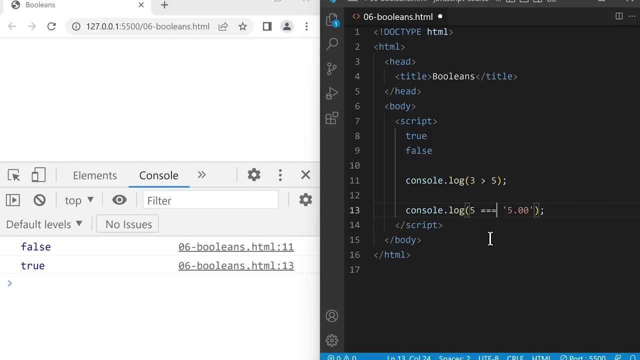 we always use the triple equals to check if two values are the same, so that we avoid the conversion behavior of double equals. so if we save now, it will tell us that these two values are not equal to each other, because one value is a number and the other value. 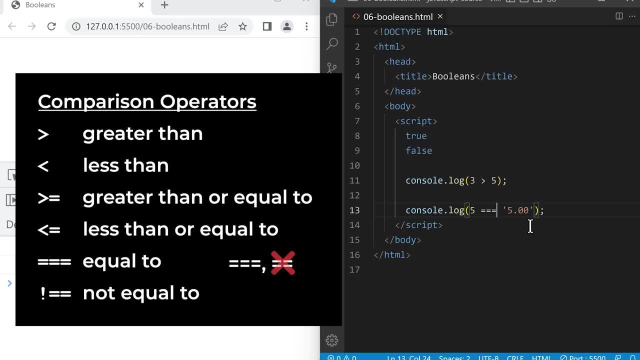 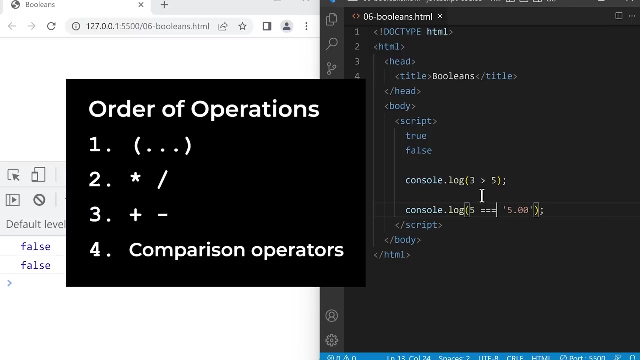 is a string, so this rule also applies to not equal to. in javascript, we always use exclamation double equals instead of exclamation equals to avoid the conversion behavior. alright, so those are comparison operators. in the order of operations, comparison operators have a lower priority than math. so if we did something like: 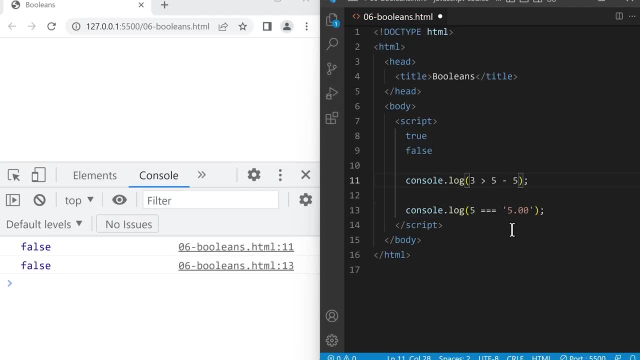 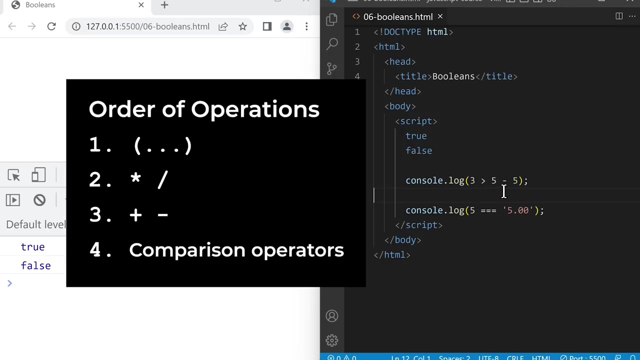 five and then minus five. this would calculate five minus five first, which is zero, and then compare the two numbers. so three is now greater than zero. so if we save the first, comparison will now be true. so comparison operators have a lower priority than math operators. now that we know. 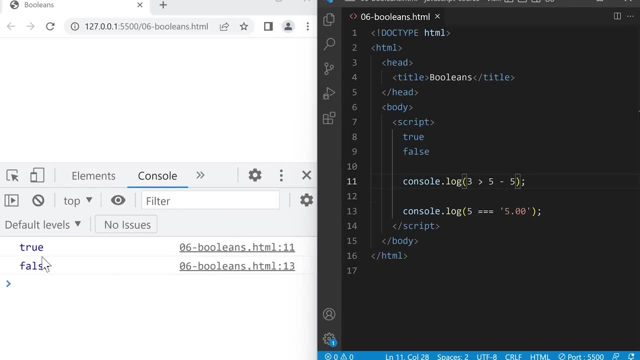 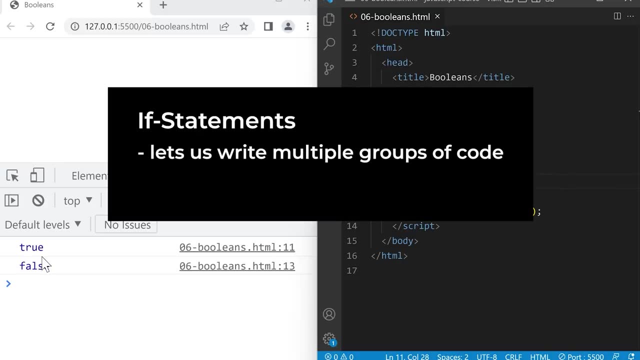 what boolean values are. we're going to combine them with a really useful feature called if statements. an if statement lets us write multiple groups of code and then decide which code to run. let's do an example and create our first if statement. we're going to go to the 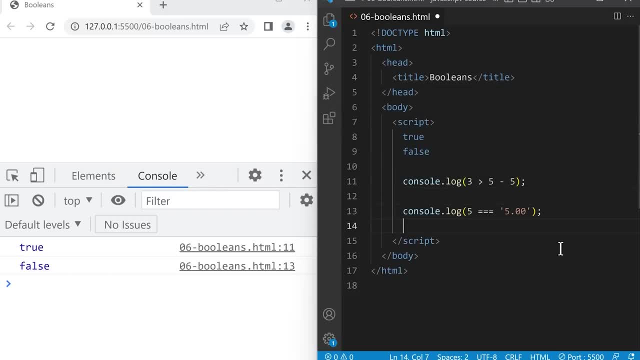 bottom and create some new lines and type if and open bracket, close bracket. and open curly bracket, closed curly bracket. between these round brackets we're going to put a boolean value like true, and in between the curly brackets we're going to put some code to run, for example: 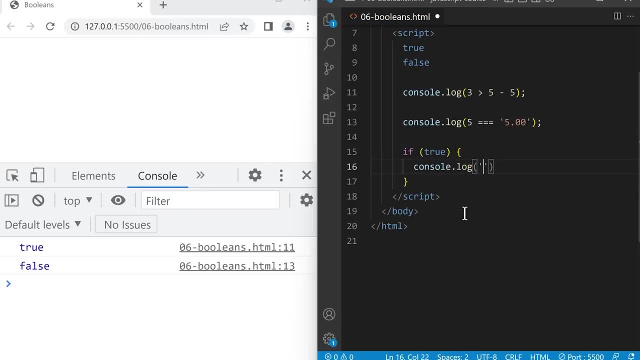 console dot log. hello. so the way that an if statement works is that if this boolean value is true, then we're going to run the code in the curly brackets. if this boolean value is false, then we're not going to run the code if we save the value between the brackets. 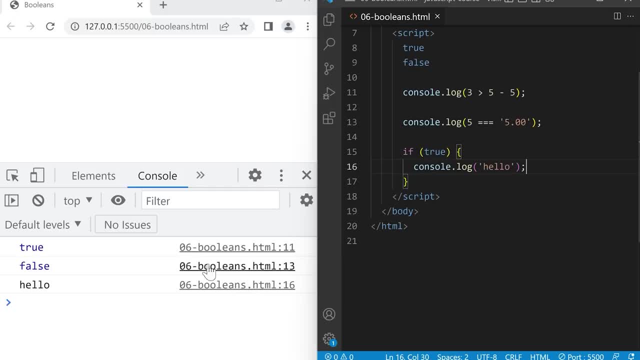 is true. so we're going to run this code and display hello. now, if we change this to false and save, it will not run this code. so an if statement lets us decide whether or not to run some code based on this boolean value. now, if statements have: 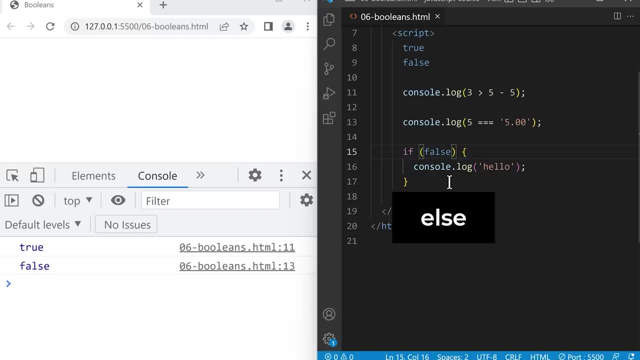 another useful feature called else. let's go to the end of this. if statement and type else: open curly bracket, close curly bracket and then inside these curly brackets we're going to put some different code like console dot log. else the way else works is: if this boolean value is true. 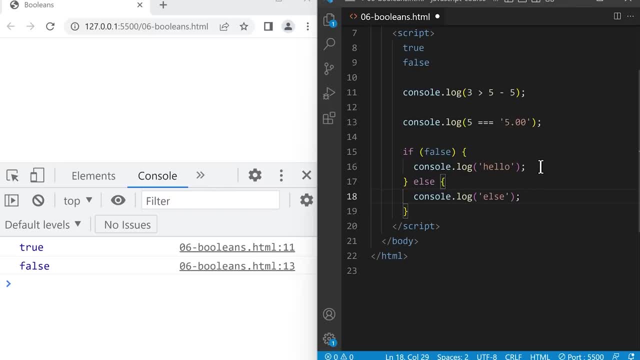 the computer will run this code. otherwise we will run the code inside. else, let's give it a try. we'll change this boolean value to true and save, and because it is true, it will run this code and display hello. now, if this boolean value is false and 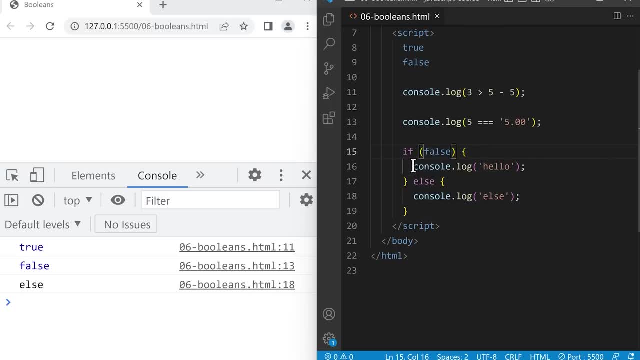 save because it is false, it will not run this code and it will run the code inside else and display else. so using if and else, we can write two groups of code and then decide which code to run. now let's do a practical example. we're going to write some code to: 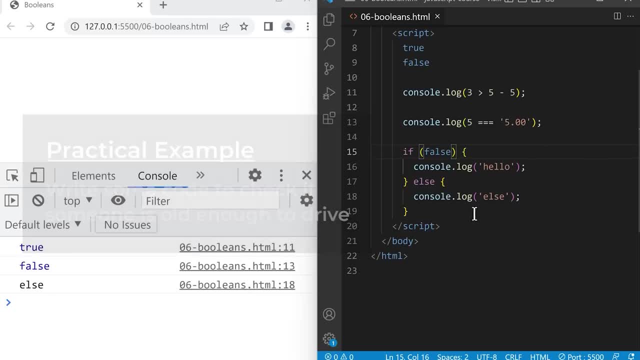 check if someone is old enough to drive. let's go to the bottom and create some new lines and we're going to type if brackets and curly brackets and inside here we're going to compare two numbers. the first number is a person's age. let's pretend we have a. 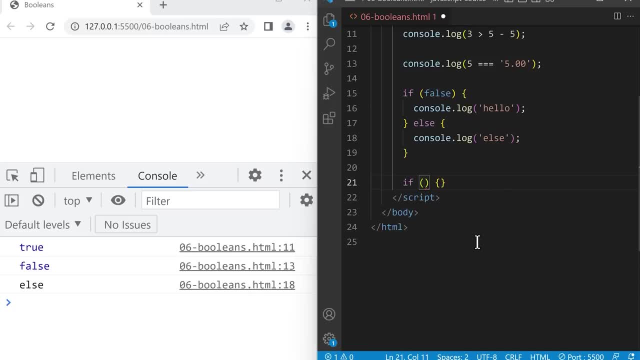 person who is 30 years old. so we're going to type 30, then we're going to check if this age is greater than or equal to the legal driving age. let's pretend the legal driving age is 16. notice that between the brackets we don't. 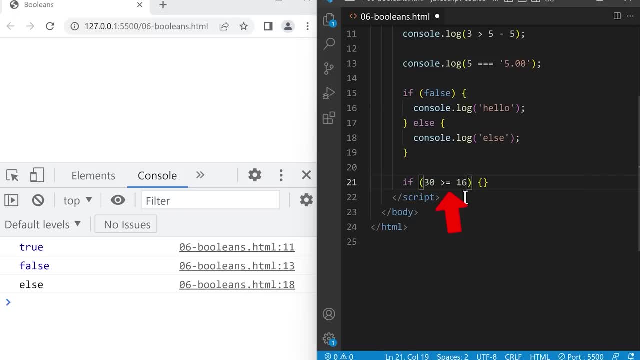 have to just put a boolean value. we can put any code that results in a boolean value. so this comparison results in the boolean value. true, that means the computer will run the code between the curly brackets. so in here let's type console dot log. u can drive. 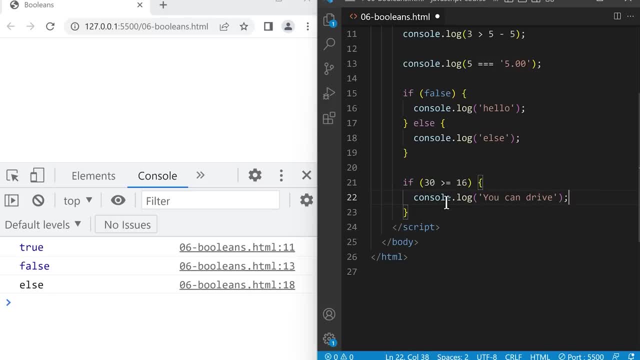 now, if this is not true, let's run some different code. at the bottom we'll type else and curly brackets, and then inside these brackets we'll type console dot log. u can not drive now. let's save, and it will tell me that this person, who is 30 years old, 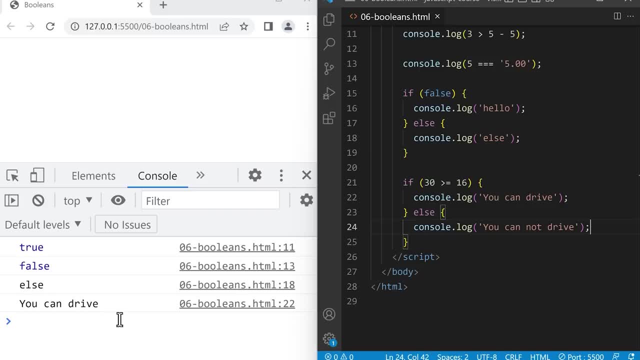 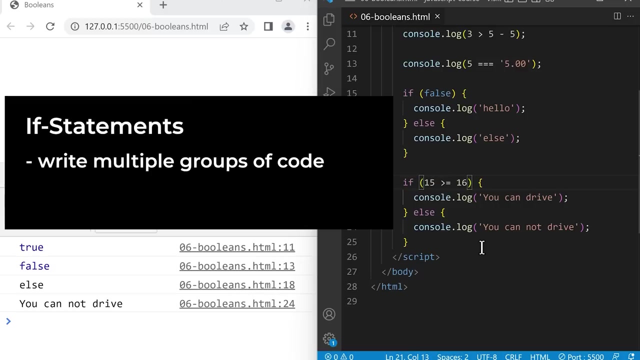 can drive. if we go back and change this to a person that is 15 years old and save, this comparison will result in false, so it will display you cannot drive. so that's how we use if statements. we can write multiple groups of code for different situations and then decide. 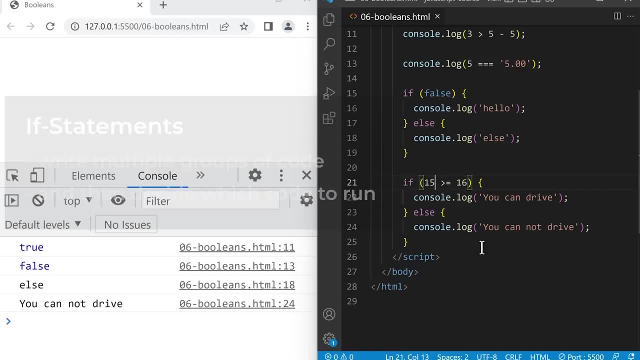 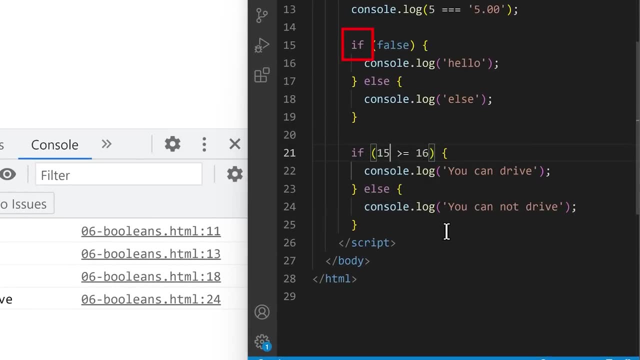 which code to run. now let's learn the syntax rules for if statements. to create an if statement, we type if and then round brackets with a boolean value inside. this is called the condition. if this condition is true, we will run the code inside the curly brackets. we can also: 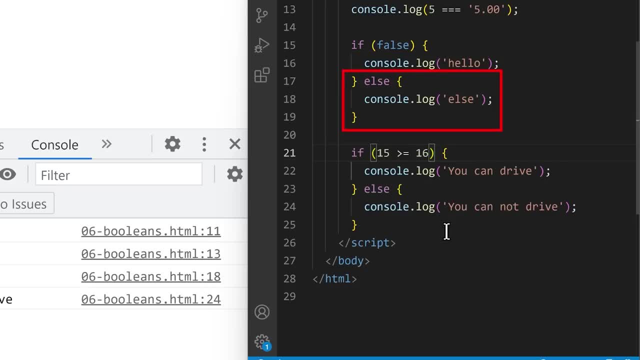 add an else statement. this code will run if the condition is false. the else statement is optional. we don't have to have one. so these curly brackets and the code inside these are called branches because it's like a tree branch. the code is splitting off into two directions. 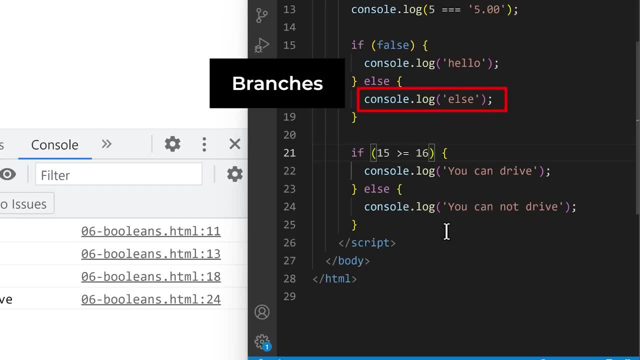 and we either run this code or we run this code. one more thing to know is: in a branch, if we only have one line of code, the curly brackets are actually optional, so we can delete these and the code will still work. however, if we have more than one line of code, 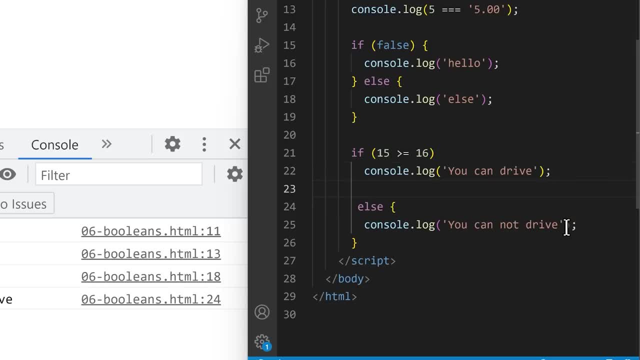 in this branch. for example, if we add another line, console dot log, congrats. now this branch has two lines of code, so the curly brackets are mandatory, so we have to add them back. now we're going to learn another feature of if statements, which is we can have more. 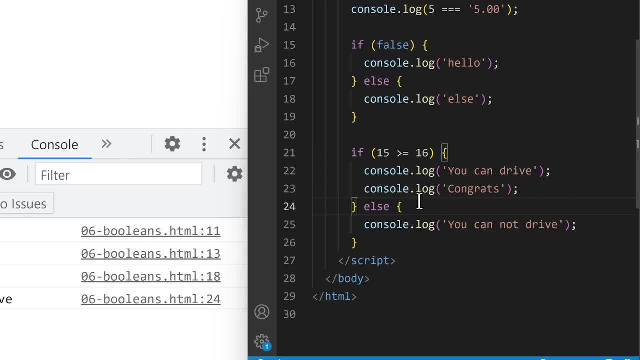 than one condition. for example, we're going to go to the end of this: if branch and type, else if, and then brackets and curly brackets, else if. lets us add another branch to our if statement. between these round brackets, we can add another condition. for example, if a person is almost 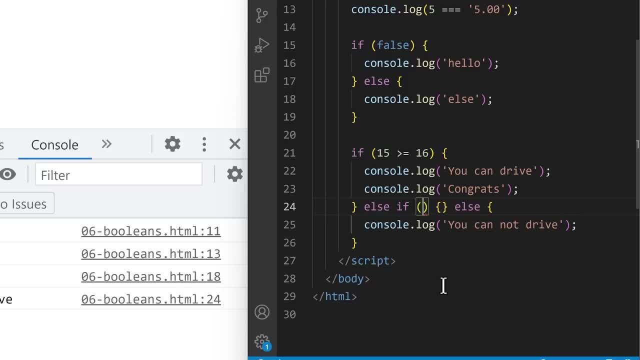 old enough to drive, lets display a different message. so, inside this condition, lets check if this person's age, which is 15, is greater than or equal to 14. so we're checking if they are almost old enough to drive. and now, inside the curly brackets, we're going to display a different. 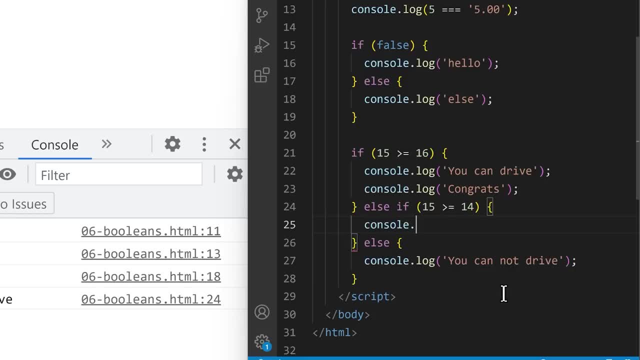 message console dot log almost there. so the way this works is that the if statement checks the conditions one by one. first it checks if this is true. if it is, it will run this branch. then it checks if this is true. if it is, it will run this branch. 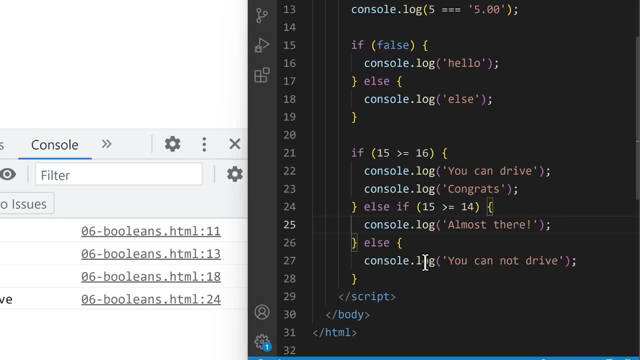 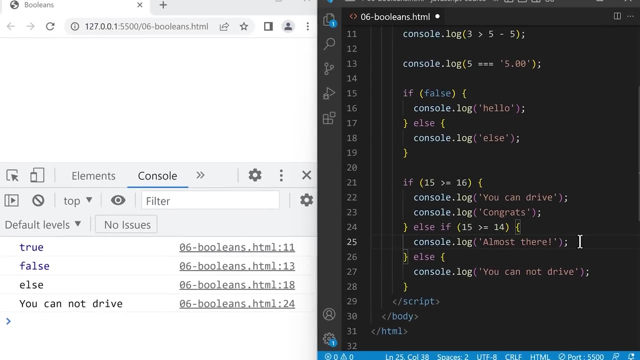 and if none of the conditions are true, it will run the else branch. so here this condition is false, so we're not going to run this code. but now the second condition is true, so we're going to run this code. if we save, we display almost there in the console. 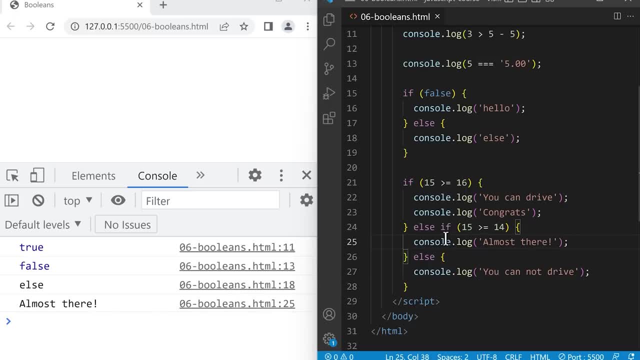 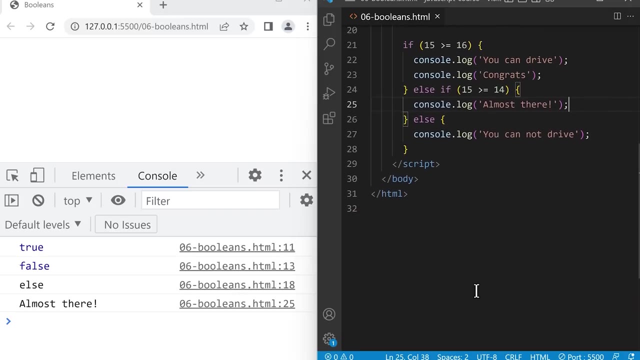 so, using else if branches, we can add as many conditions as we want to an if statement. the next thing we're going to learn is that we can combine if statements with variables from the previous lesson. for example, here we wrote the person's age two times, so we can actually save this age. 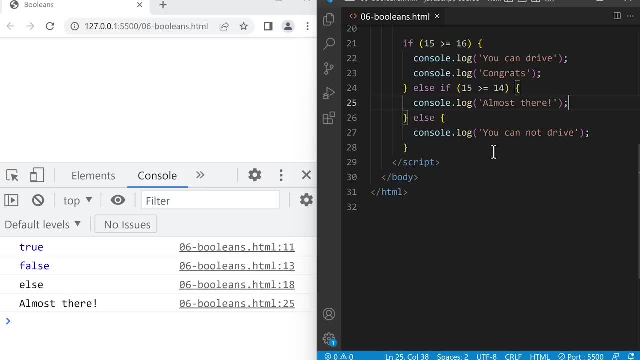 in a variable and then reuse that value. so, above the if statement, let's create a variable using const and let's name this variable age, and we'll make it equal to fifteen. remember, the best practice for creating a variable is to use const by default and only use let. 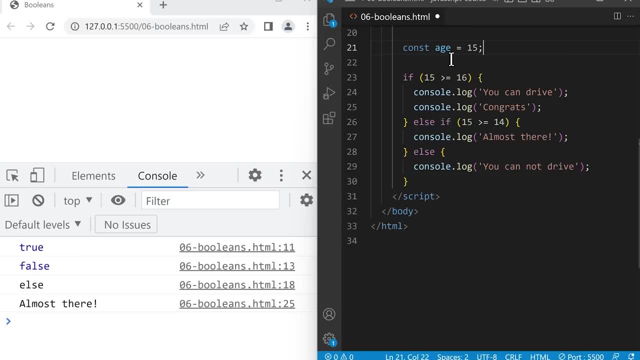 if we're going to change this value later, and now that we saved this number in a variable, we can use the variable inside the if statement. so we'll replace fifteen with age, and here as well, with age. so this will take whatever value is inside the variable. 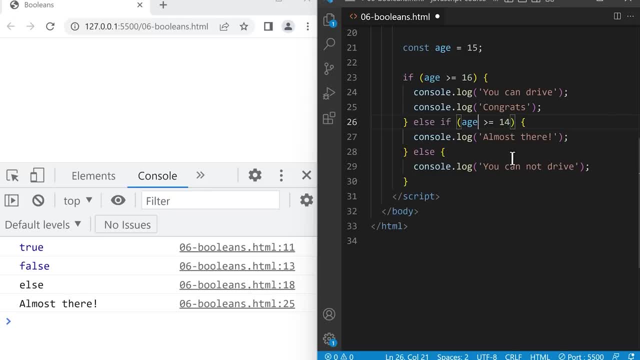 and substitute it into the code. if we save, the if statement works the same way as before and we run this line. okay, now we're ready to use booleans and if statements to do a project. we're going to build a rock paper scissors game. first, let's take 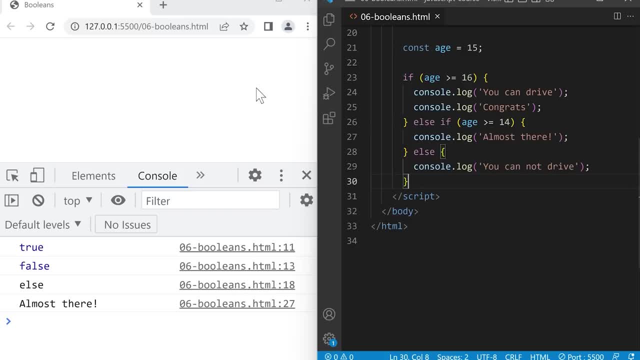 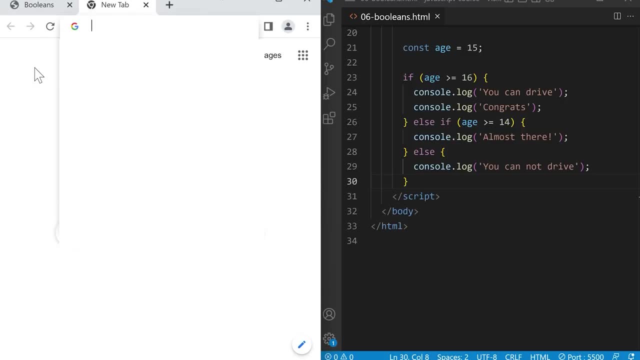 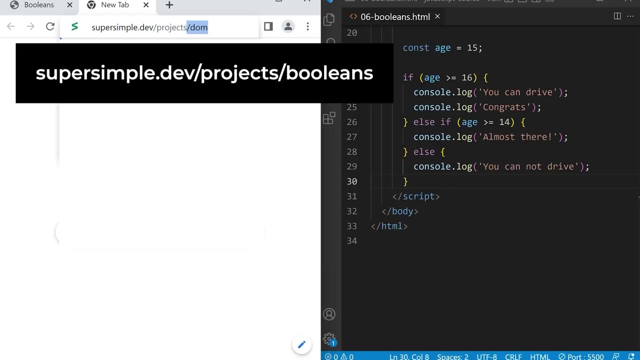 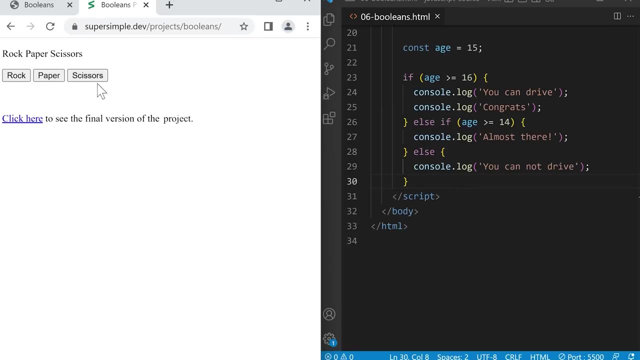 a look at the project. we're going to go to our browser and at the top create a new tab and we're going to type here super simple dot dev, slash projects, slash booleans and press enter. here we can see a simple version of a rock paper scissors game. 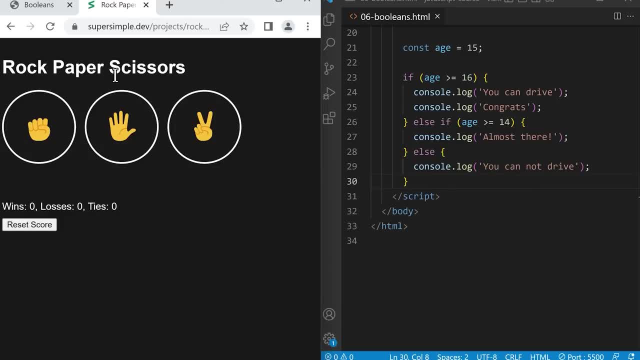 and if we click this link it will take us to the final version of this game. so in this game we can pick a move and then the computer will pick a random move and it will show us the result and we also have a score of how many times we won. 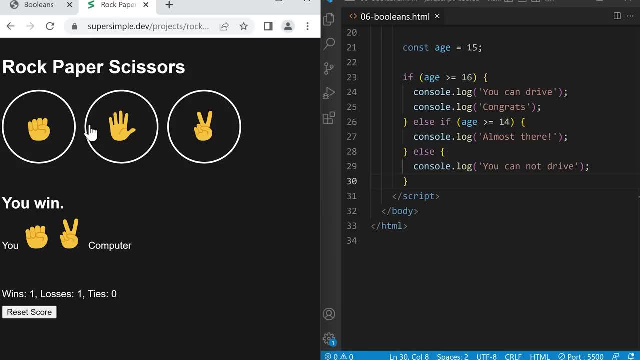 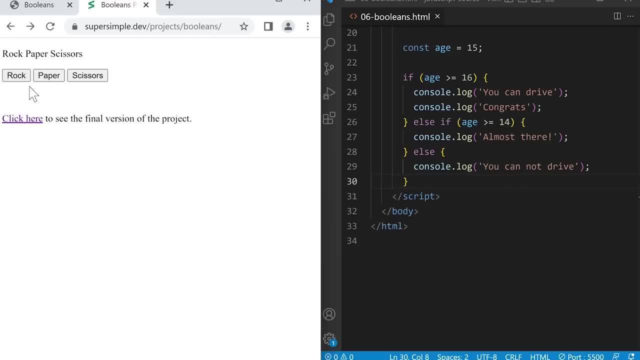 lost and tied. so we're going to build this as we go through the course, but for now, let's go back and we're going to start by building this simple version of the game. so how this simple version works is we click one of these buttons to pick a move. so let's. 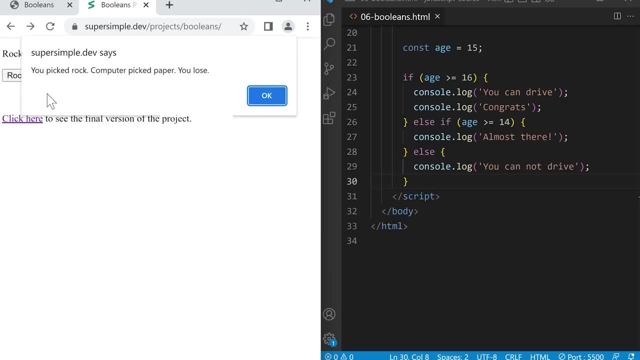 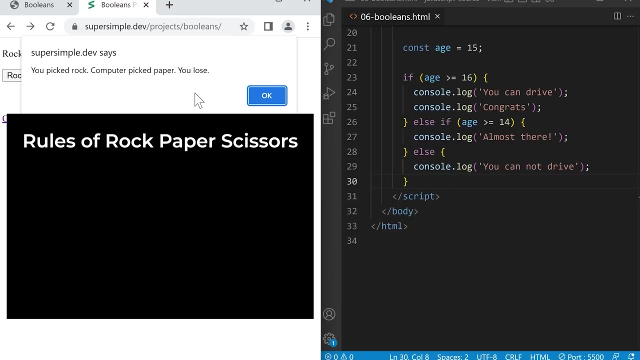 pick rock, then the computer will randomly pick a move- in this case it's paper, but for you it might be different- and it will compare the two moves and display the results in this popup. so the rules of rock paper scissors are: rock beats scissors, paper beats rock. 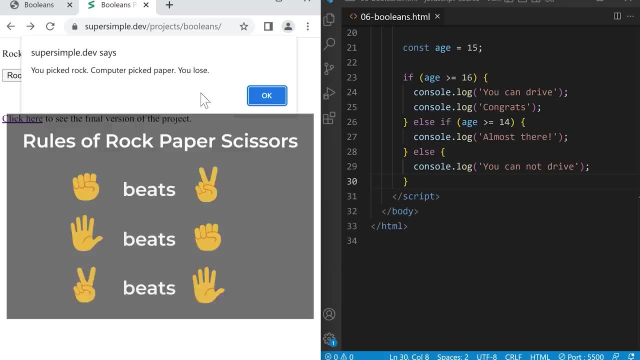 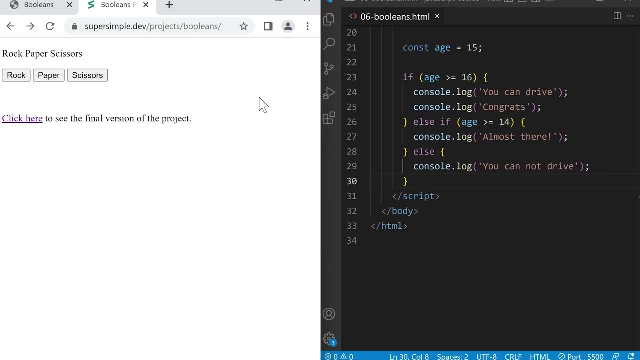 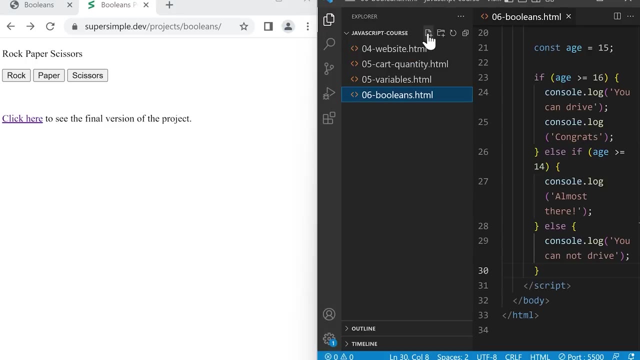 and scissors beats paper. let's press ok and we'll get started on this project. first, we'll create a new html file just for this project. let's go to our code editor and click here and create a new file, and we're going to name this file. 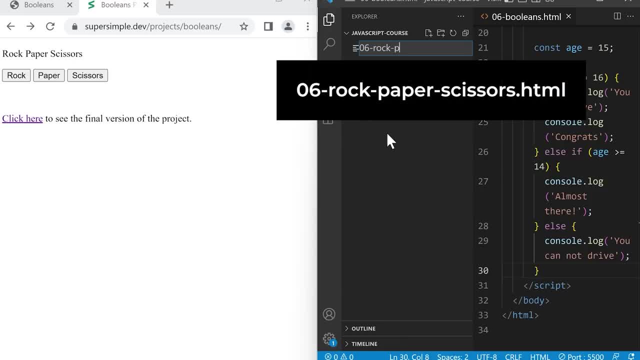 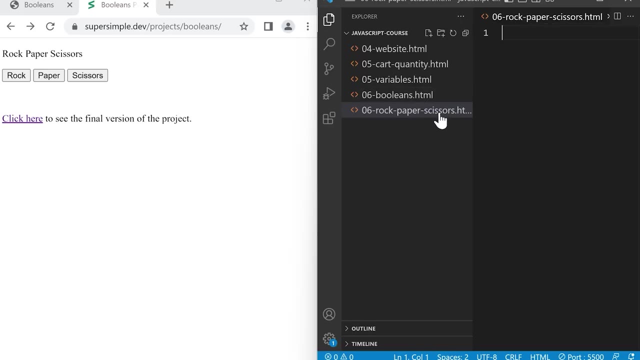 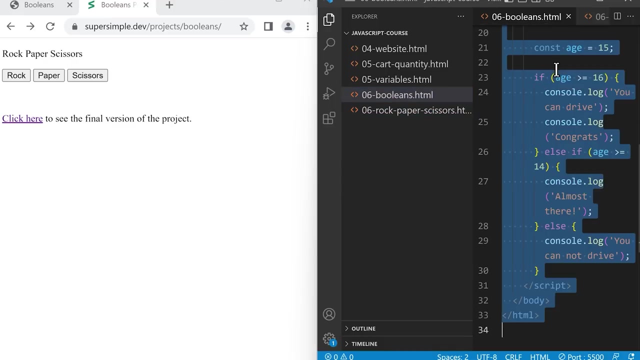 06-rock-paper-scissors- 06-rock-paper-scissors- html and press enter. next let's copy all the code from booleanshtml into this new file. so we'll open this again and then control a or command a to select all the code and then right click. 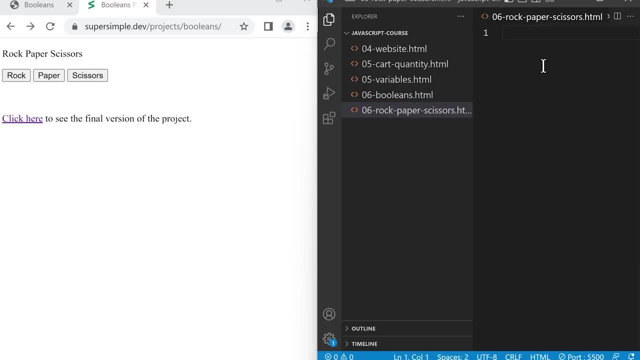 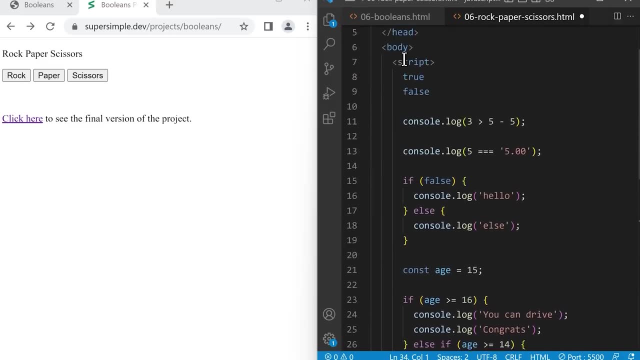 copy and in here, right click and paste. let's close this and prepare this file so we'll change this to rock paper scissors and remove all of the javascript code that we had before. finally, let's save and open this file in the browser by right clicking and then open with live server. 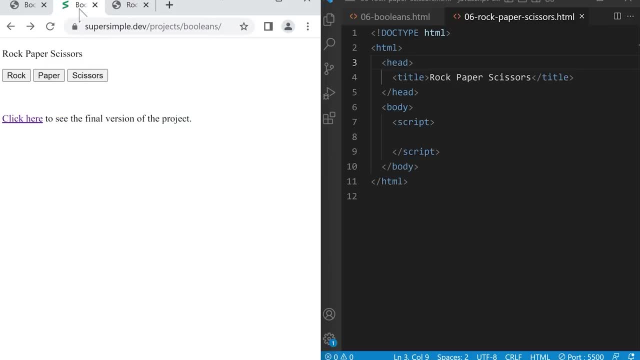 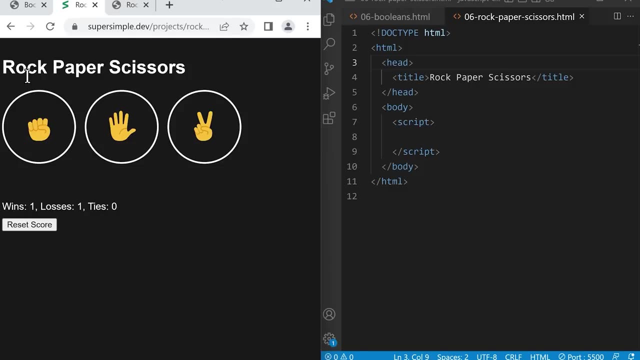 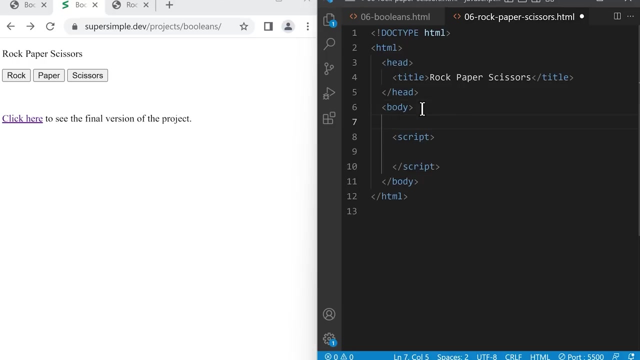 let's take a look at the project again. so we're going to start by creating the text first, because this text is in the final version of the project. so in our html we're going to create a paragraph element for this text. so: less than p. greater than: 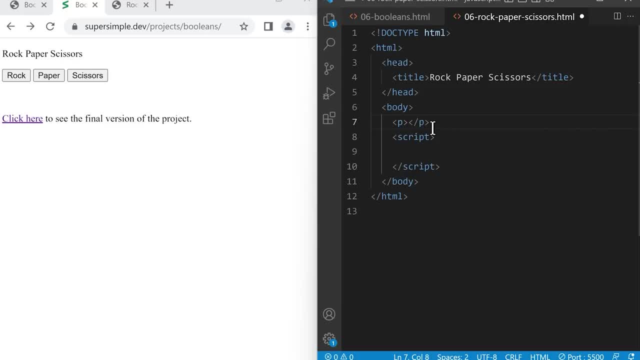 and the closing tag less than slash, p greater than inside our paragraph, we're going to have the text rock paper scissors. next let's create the buttons. so we'll go to our html and create a button and inside this first button we'll have the text rock. 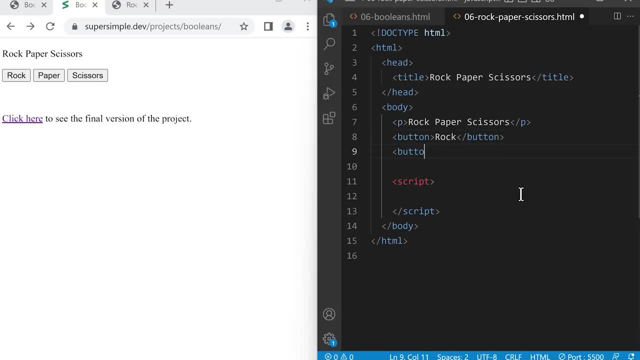 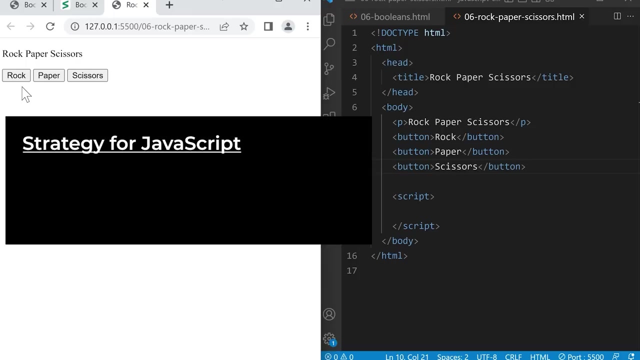 let's create another button. this one will be paper. and we'll create the last button. this one will be scissors. now let's save and check our new tab. and now we created all the elements that we need. next let's make these elements interactive with javascript. so when writing javascript, 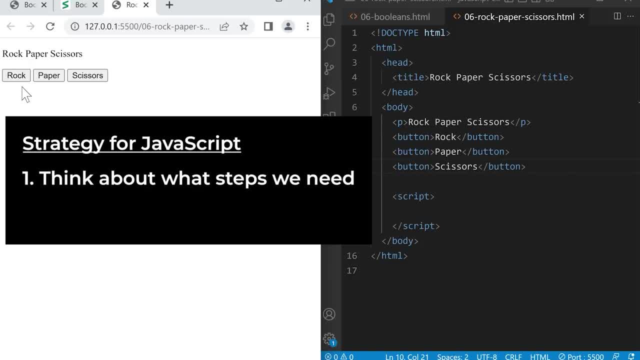 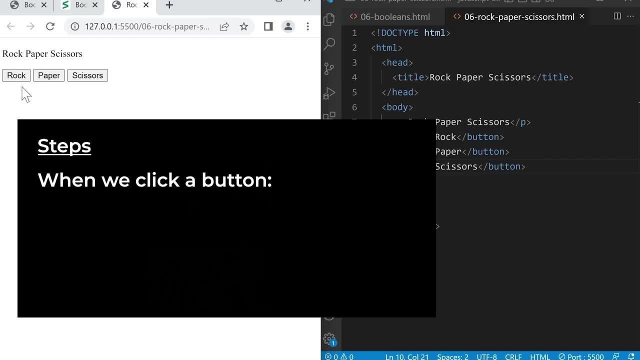 a good strategy is to think about what steps we need to do and then convert those steps into code. so here, when we click a button, the first step is the computer will randomly select a move, and then we're going to compare the moves to get the result and finally, 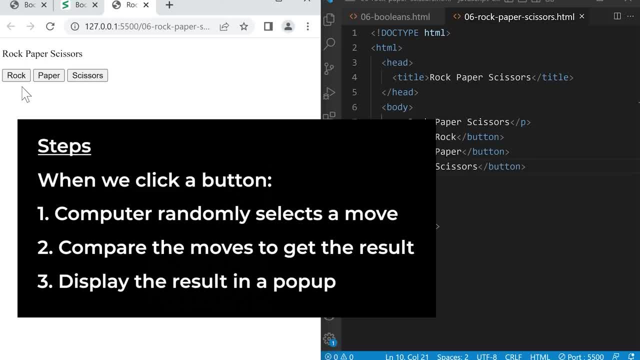 we'll display the result in a popup. by the way, this is called an algorithm. an algorithm is a set of steps to complete a task or to solve a problem. now that we know what steps we need to do, we're going to convert these steps or this algorithm. 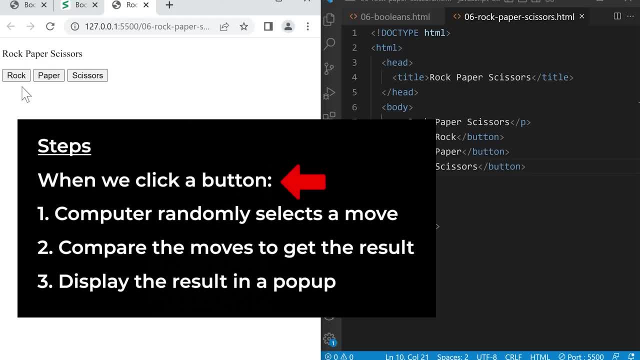 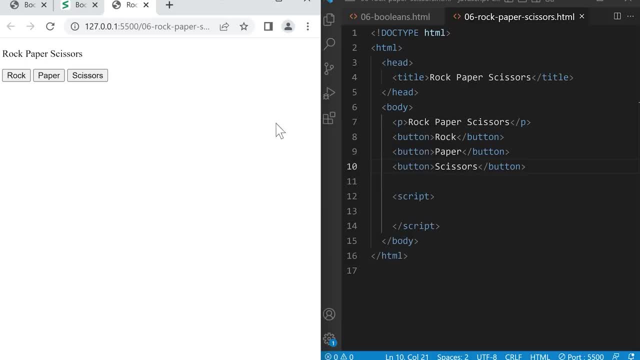 into code. first, we're going to run some javascript when we click these buttons, so let's use the onclick attribute again. we'll go to the opening tag of the button and type: onclick equals double quotes, and then inside these double quotes we can add our javascript. so 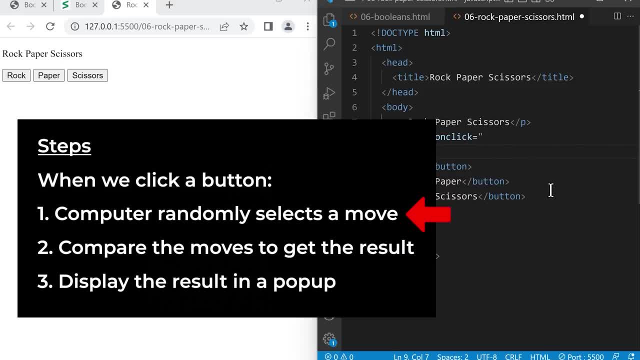 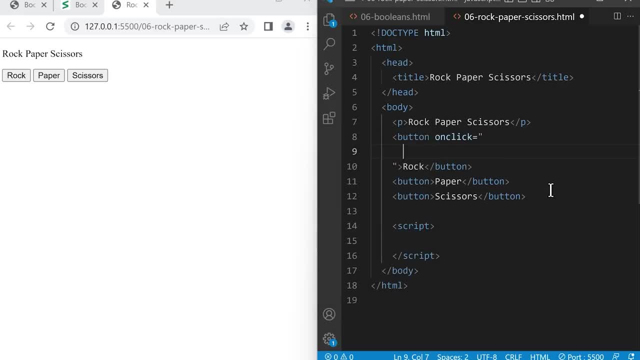 now we have to figure out how to randomly select a move for the computer. to do this, we need to learn a new piece of javascript code. so here we're going to type capital M. math dot. random open bracket- close bracket. math dot. random generates a random number between: 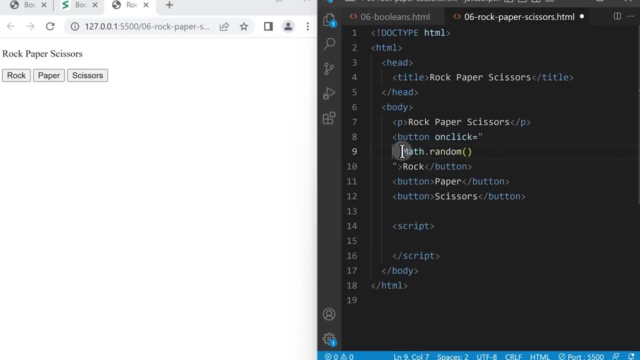 0 and 1. so if we console dot log, this console dot log and save and click this button and then check in our console by right clicking inspect and the console it will display a random number between 0 and 1 if we click this button. 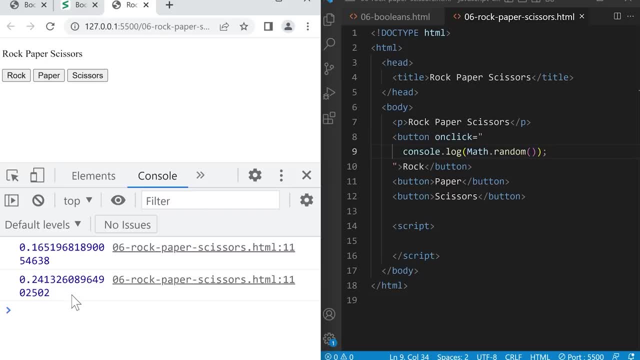 again, it will generate a different random number. so every time we run math dot random, it generates a different random number between 0 and 1. now, to be more precise, it actually generates a number greater than equal to 0 and less than 1. now let's. 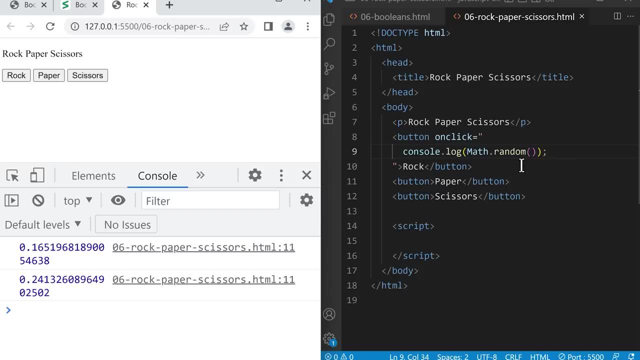 save this random number in a variable so we can use it later. so we'll replace the console dot log with const and then a variable name. let's just name it random capital n, number and then equals. so we saved this random number inside this variable. next we need a way. 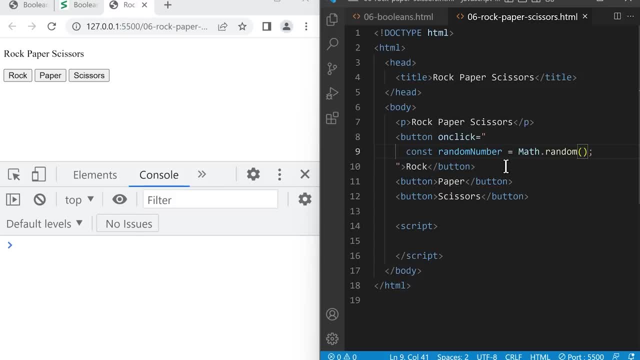 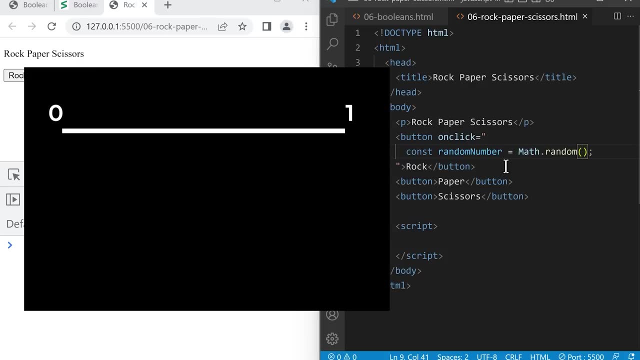 to convert this random number into a move like rock, paper or scissors. to do this, let's imagine the space between 0 and 1 and then divide the space into 3 equal parts. each part represents a move. if we generate a random number and it's between 0. 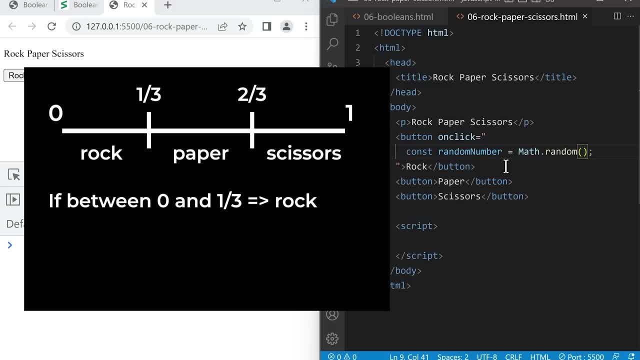 and 1 third, the move will be rock. if it's between 1 third and 2 thirds, the move will be paper, and if it's between 2 thirds and 1, the move will be scissors. this is how we can convert the random number into a move. 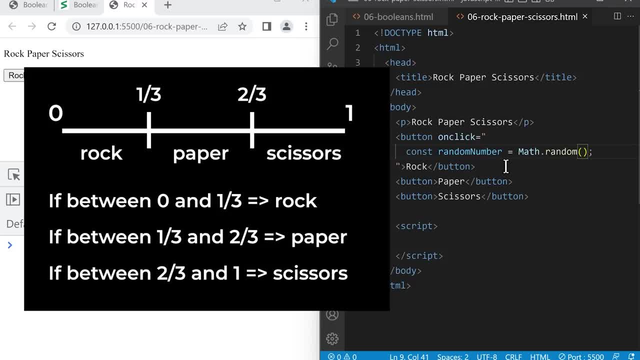 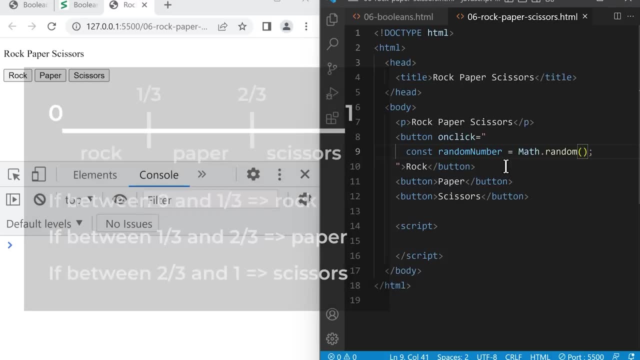 and this will give the computer an equal chance of picking rock, paper or scissors. now let's convert these steps into code, and an if statement is the perfect solution for this. this already looks like an if statement, so in our onclick attribute, let's add some new lines. 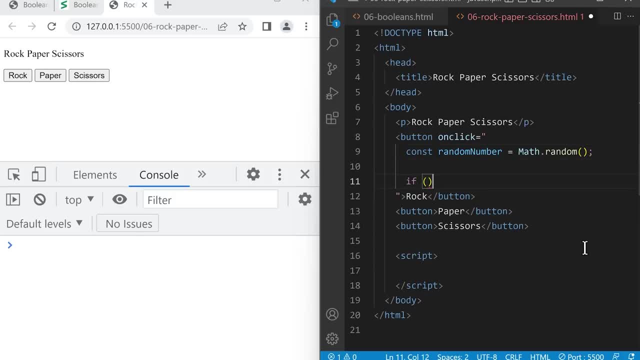 and type if brackets and curly brackets. for this first condition, we're gonna check if the random number is between 0 and 1. third, so let's check if random number is greater than or equal to 0. but in this case we also need to check. 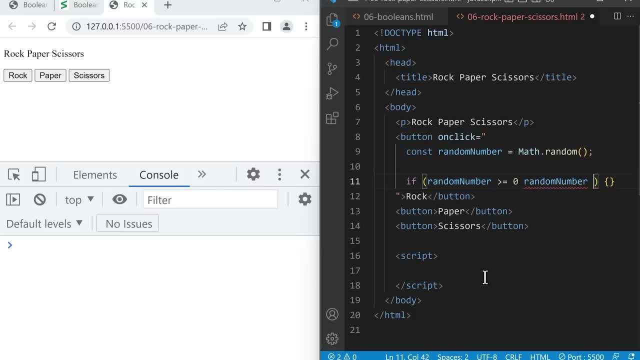 that random number is less than 1 third, because we're checking if the number is between 0 and 1 third. but how do we do this? how do we check that 2 comparisons are both true? to do this, we're gonna learn another type of operator. 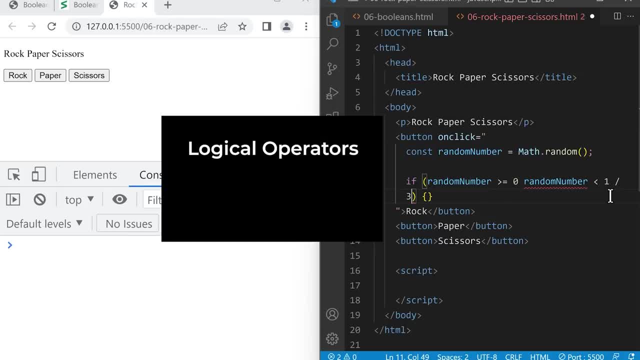 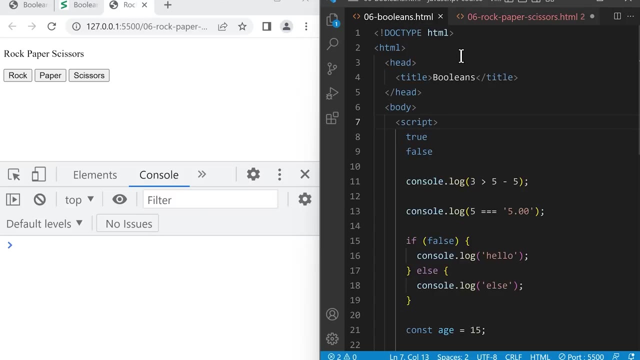 in javascript called logical operators. logical operators: let us combine boolean values, which is what we need to do here. let's go back into booleanshtml and we're gonna learn logical operators. so first let's open the tab for this file and we're gonna comment out all the previous code. 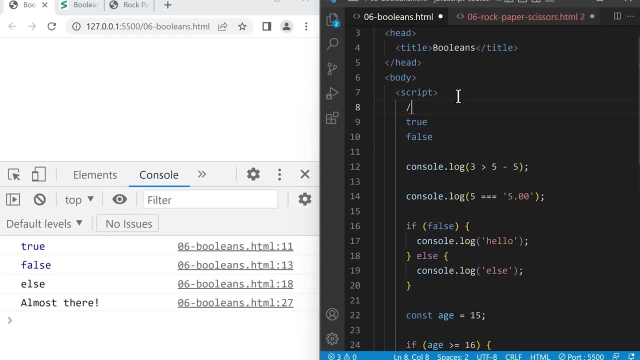 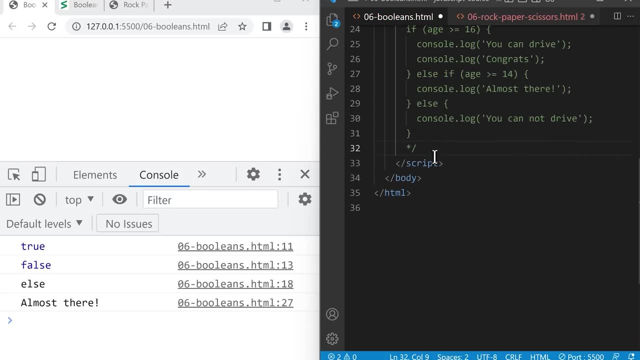 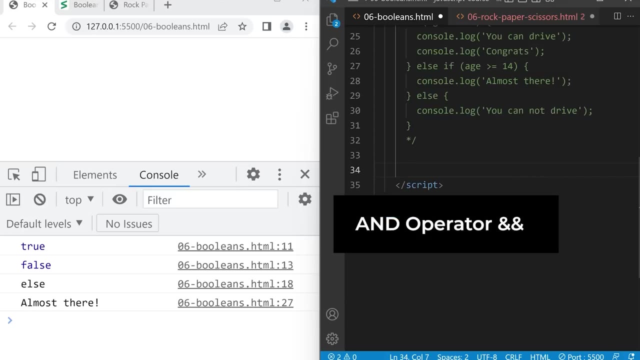 so our console doesn't get too messy. // and then at the bottom, //. now let's create some new lines, and the first logical operator we're gonna learn is called the and operator. let's type console dot log: a boolean value true and another boolean value true. 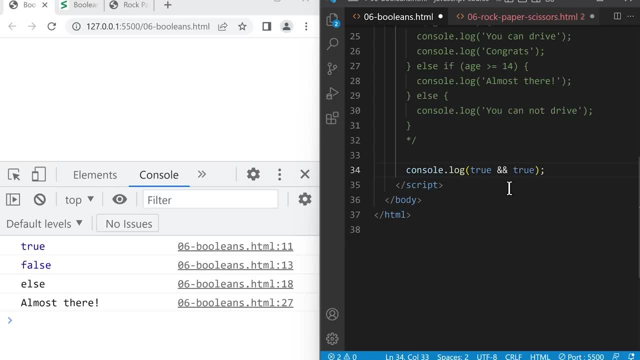 so this is the and operator and it checks if two boolean values are both true. so it checks if the left side is true and the right side is true. that's why it's called the and operator. so here the left side is true and the right side. 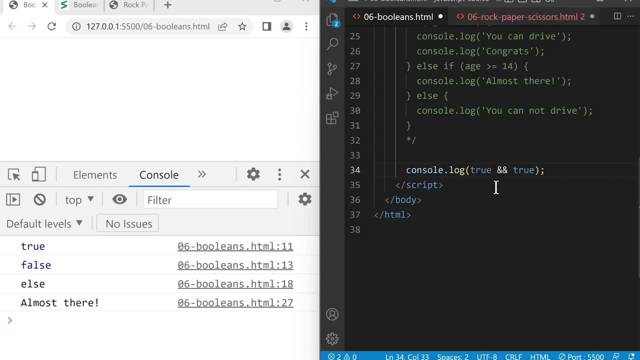 is also true, so the and operator will result in true if we save. this displays true. now if one of these sides is false, for example, if we change this to false now, let's check: is the left side and the right side both true in this case? no, so and. 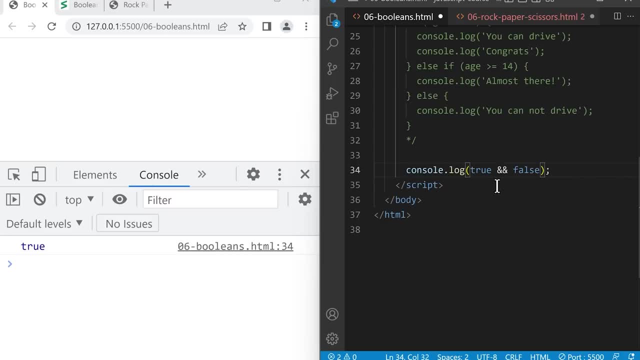 will now result in false. if we save, it now displays false. so that's the logical and and operator. it checks if the left side is true and the right side is also true. so this is exactly what we need for our project. for example, let's create a new line: 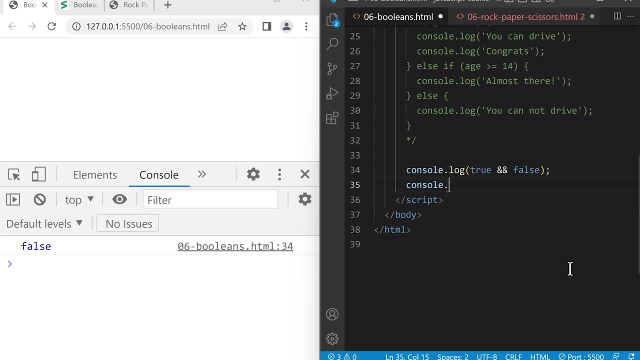 and type console dot log. and let's say that we generated a random number like zero point two and we want to check if it's between zero and one third so we can do zero point two is greater than or equal to zero. and we're also going to check if zero point two 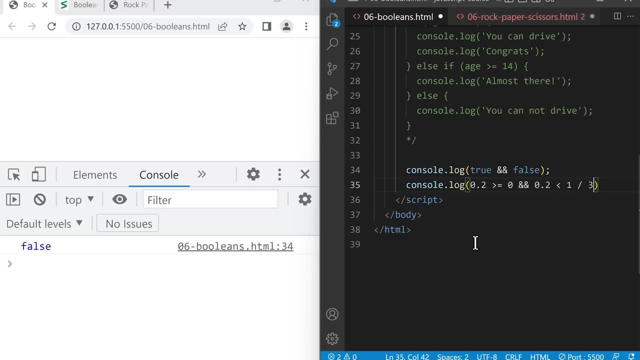 is less than one third. so we're using the logical and operator to check if the left side is true and the right side is also true. so in this example both sides are true. zero point two is between zero and one third. so if we save this whole thing will? 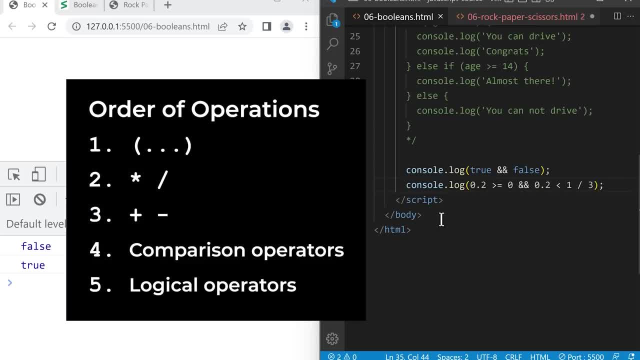 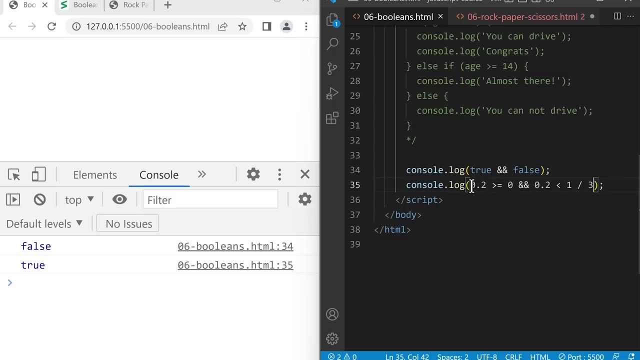 display: true. now, in the order of operations, logical operators like and have a lower priority than math and comparisons. so in this example it will calculate the math first, and then it will calculate the comparison on the left, and then the comparison on the right, and then, at the end, the and. 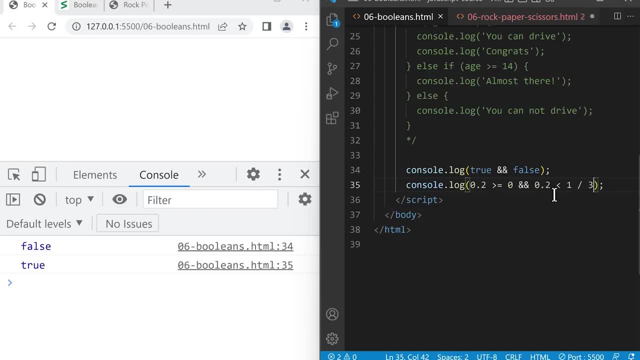 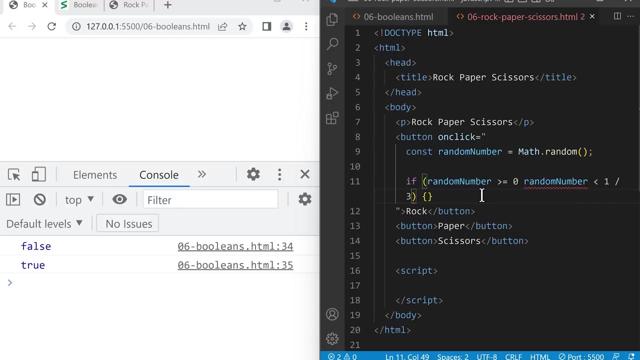 operator checks. if both sides result in true, now let's use the and operator in our project. let's go back to the file for our project and then, inside this first condition, we're going to check if the random number is greater than or equal to zero and at 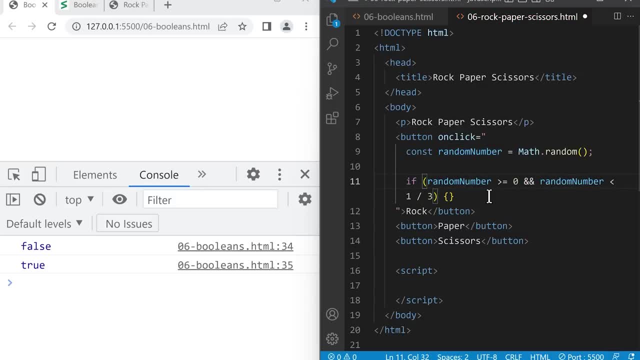 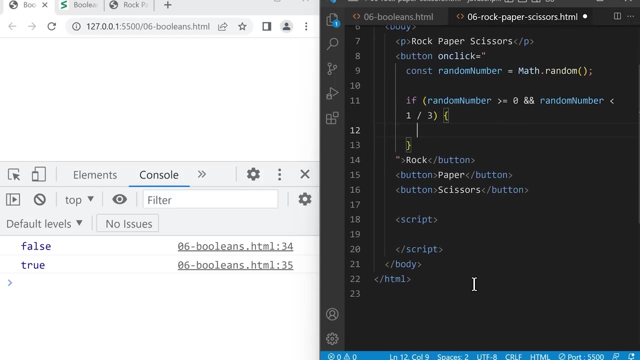 the same time is the random number less than one third. so this is how we check: if a number is between zero and one third, in this case the computer will pick rock. so between the curly brackets let's just type: console, dot, log, rock. let's get some practice and 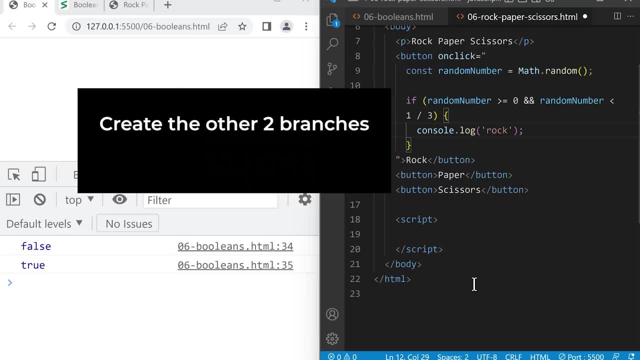 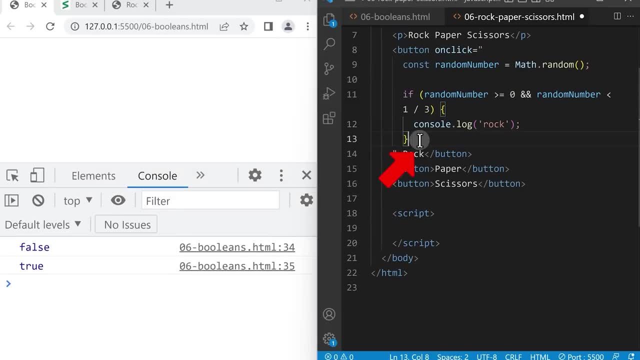 create the other two branches for picking paper and scissors. feel free to pause this video if you want to try it yourself first. so here we're going to type else if to add another branch and then brackets and curly brackets, and in this condition we're going to 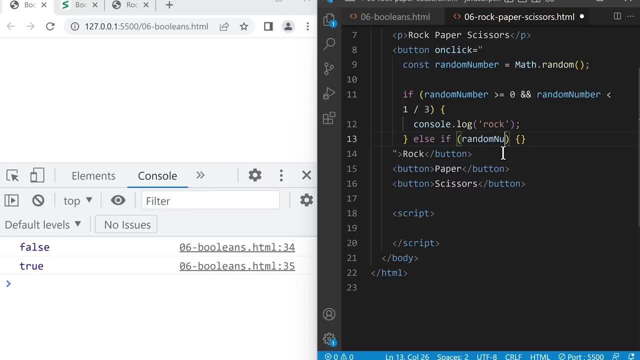 check if random number is greater than or equal to one third and random number is less than two thirds. so if this random number is between one third and two thirds, inside here we're going to console dot log paper and finally, let's create another branch using else if 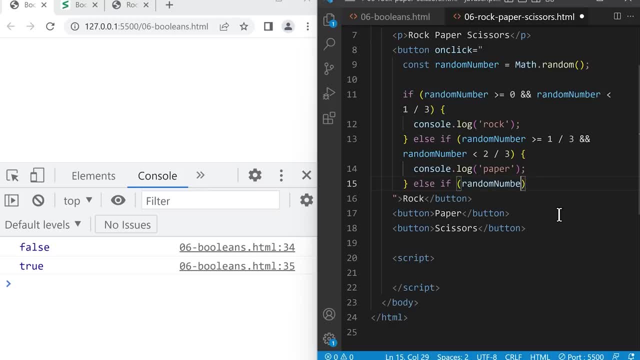 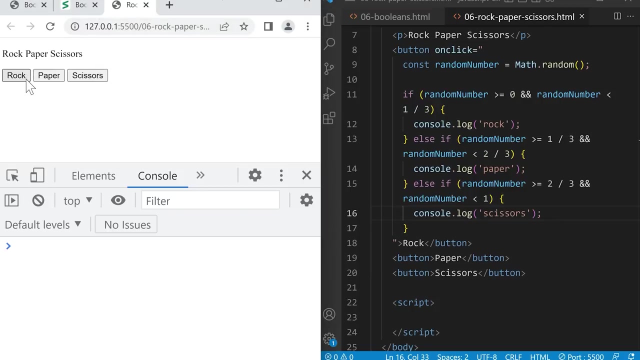 random number greater than or equal to two thirds and random number less than one. and console dot log scissors. if we save and then go back to our rock paper scissors tab and then click the rock button a few times, it will pick some random moves for the computer. 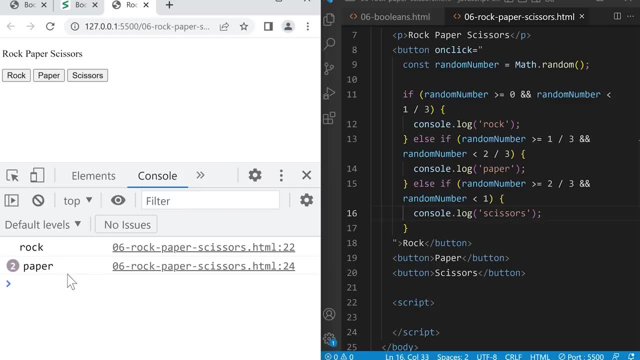 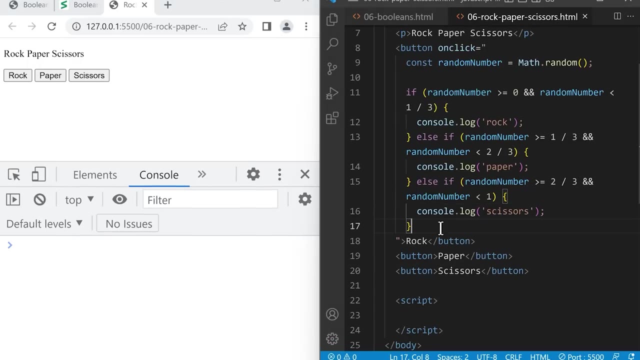 so that's how we generate the computer's move. one thing i want to point out is that i use the less than comparison instead of less than or equal to. i just did this so that the comparisons don't overlap. before we continue in the project we're going to learn. 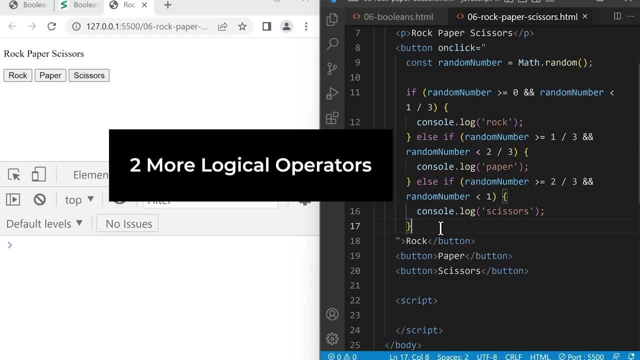 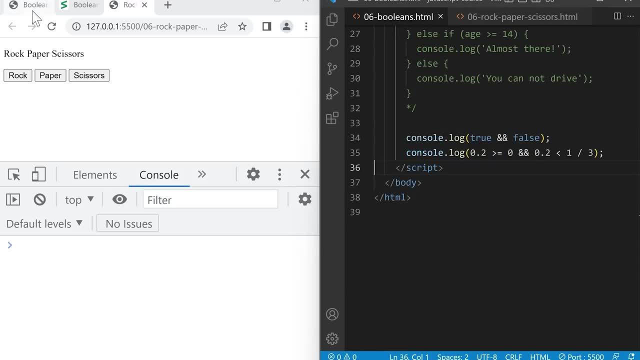 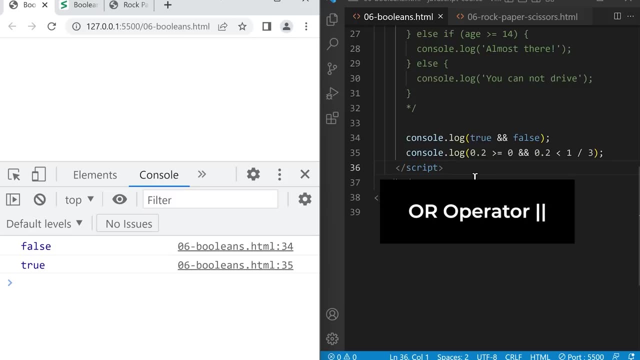 two other logical operators we can use. let's go back to booleans dot html and let's also open the tab for this file. the next logical operator is called the or operator. for example, let's type some new lines and type console dot log true or false. 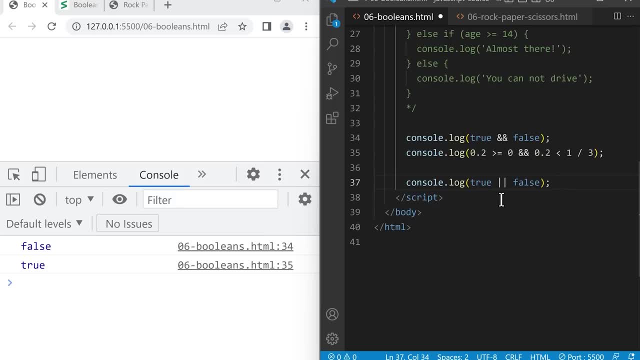 so this is the logical or operator. it checks if at least one side is true. so it checks if the left side is true or the right side is true. that's why it's called the or operator. so here one of these sides is true, so the or. 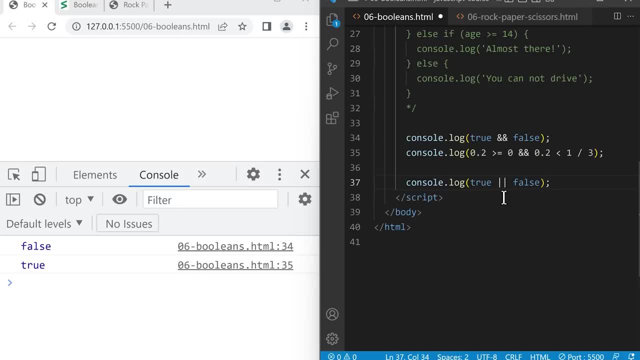 operator will result in true if we save. this displays true. if both sides are true, it will also result in true because at least one side is true. the last logical operator we're going to learn is called the not operator. for example, let's create a new line. 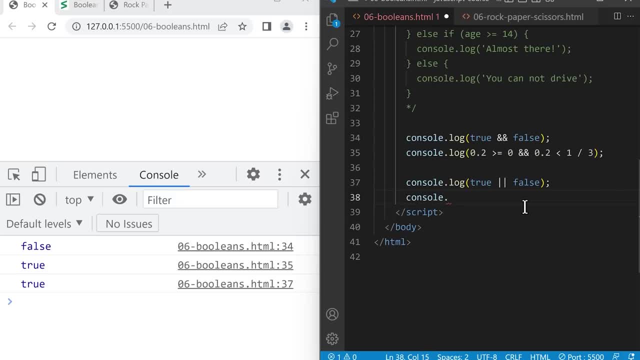 and type: console dot log. exclamation: true. so the exclamation is called the not operator. the not operator only uses one boolean value and it flips it into the opposite value. so if this value is true, the not operator will flip it into false. so if we save, 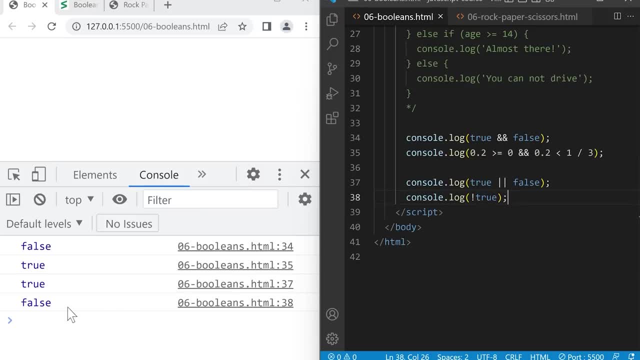 this will result in false. now, if you think about it, if we say that something is not true, that's the same thing as saying that it is false. so that's why this is called the not operator. now, if we change the value to false again, the not operator will flip this. 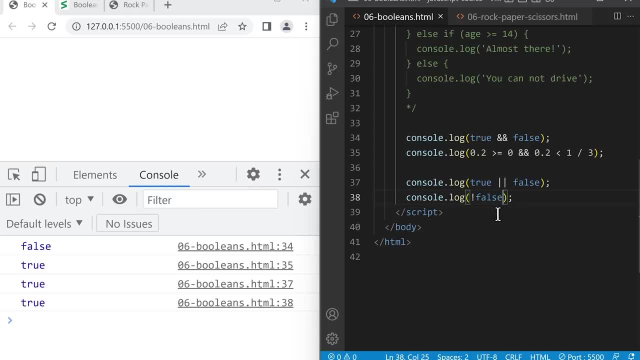 into true. so if we save, this will now result in true. so those are the logical or and not operators. we don't need to use these in our project right now, but I'll leave some exercises for these at the end of this lesson. now let's go back and continue the 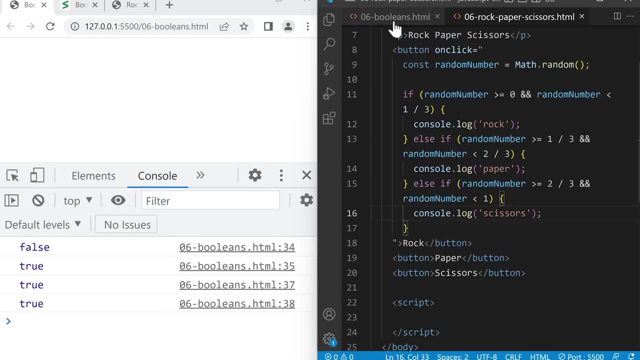 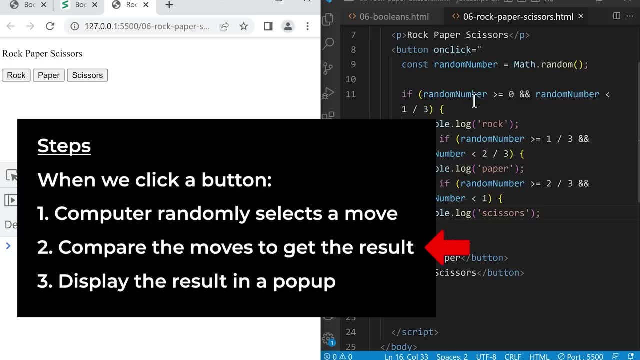 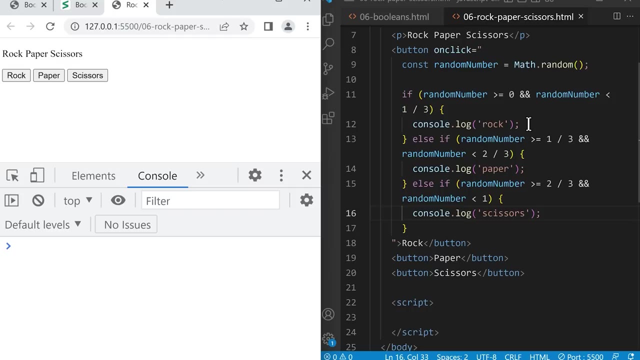 project. let's open the code and open the tab. the next step is to compare the computer's move to our move, which is rock. so first let's save the computer's move in a variable so we can compare it later. so instead of consolelog, we're going to create 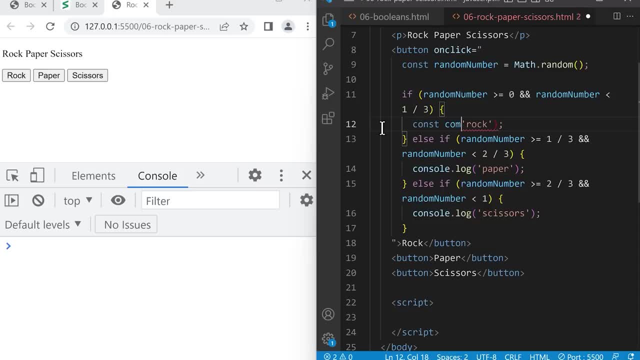 a variable with const computer capital, M move, and make it equal to the string rock. and we'll do the same thing. here const computer move equals paper, and here const computer move equals scissors. and now at the bottom, let's console dot log the computer move variable to make sure that it worked. 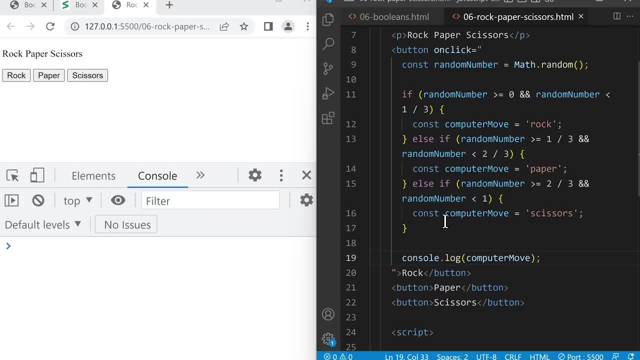 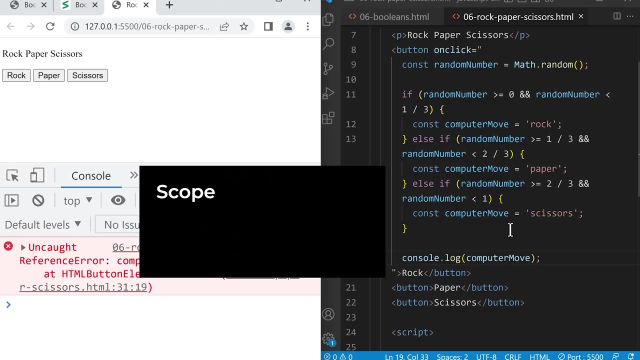 if we save and then click our rock button, unfortunately it gives us an error telling us that computer move is not defined, even though we created it right here. so what is happening here? if statements have a special feature, they create something called a scope. a scope limits where a variable exists. 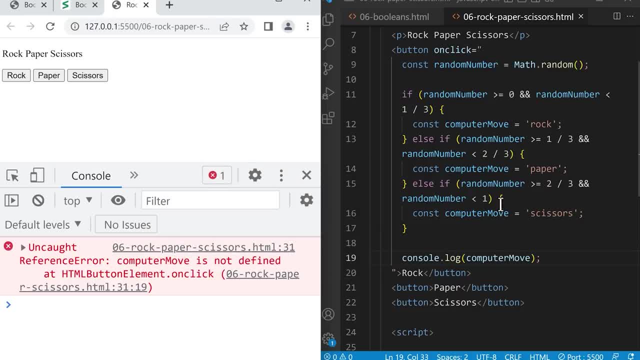 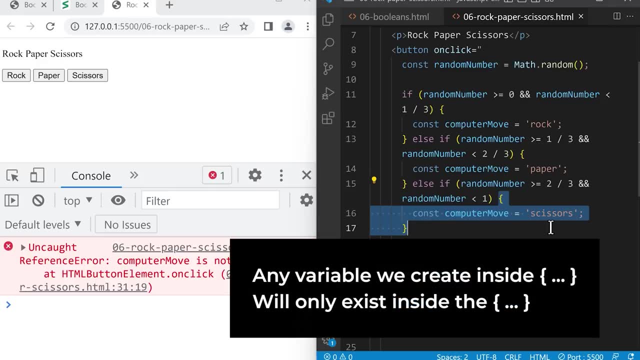 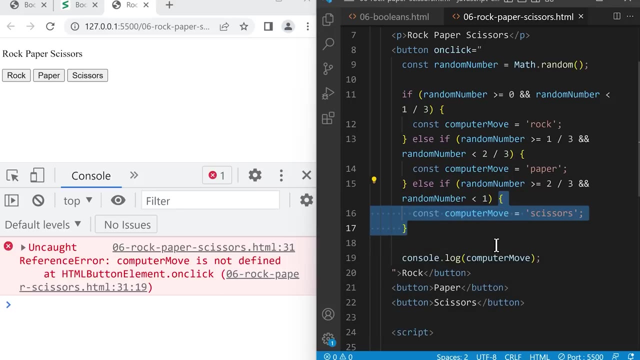 basically, whenever we have these curly brackets like this, any variable we create inside the curly brackets will only exist inside the curly brackets and we can't use these variables outside the curly brackets. so this is called a scope. scopes are a feature of many programming languages and they help us avoid. 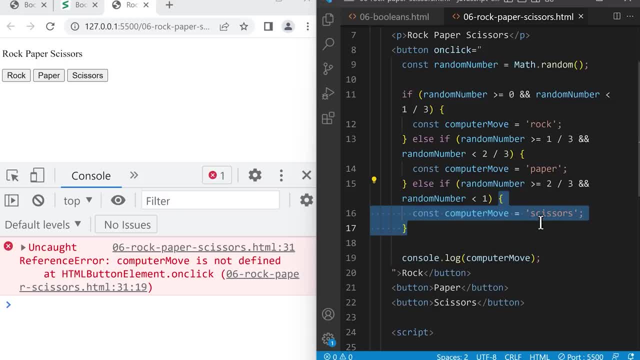 naming conflicts. for example, if I create a variable here called random, number equals 0.5 and this didn't create a scope. so if I delete these curly brackets, this variable name will now conflict with the variable name up here, because we can't have two variables. 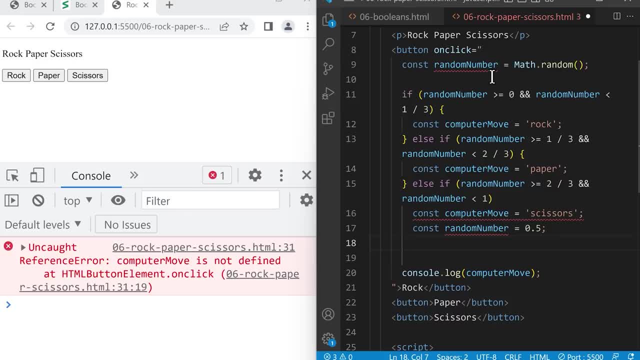 with the same name. so you can imagine that if we didn't have scope and we had hundreds or even thousands of lines of code, we would quickly start to run out of variable names. so by creating a new scope here, all the variable names inside the scope only exist between the curly. 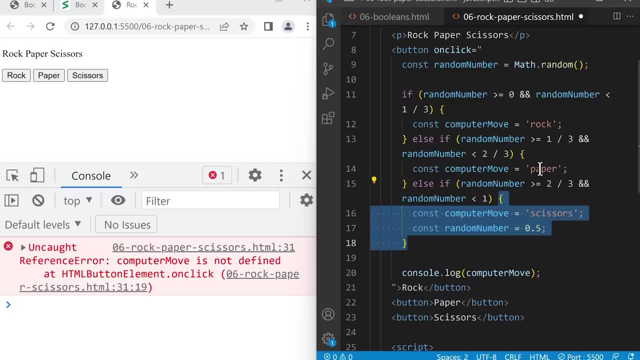 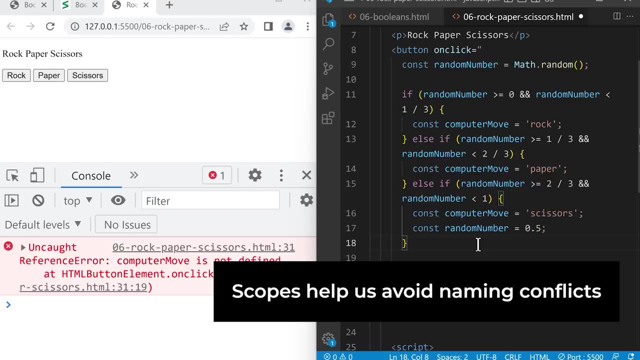 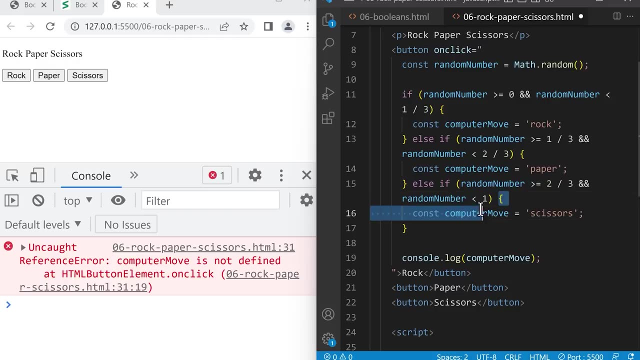 brackets and it won't affect anything outside in the code. so scopes help us avoid naming conflicts. okay, so I'll delete this example and we'll learn how to access this variable outside of this scope. so to access this variable outside of the if statement, we have to create this variable. 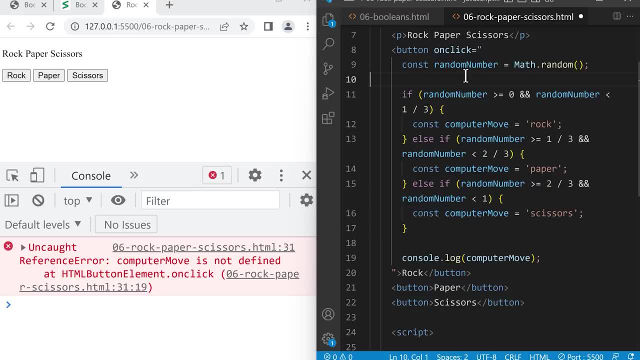 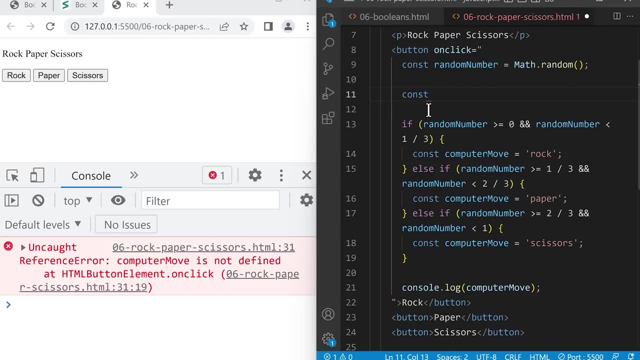 outside of the if statement. so above here we can create this variable const computer move and let's just make it equal to the empty string for now. so this variable was not created inside any curly brackets, so it's accessible from all of this code inside the onClick attribute. 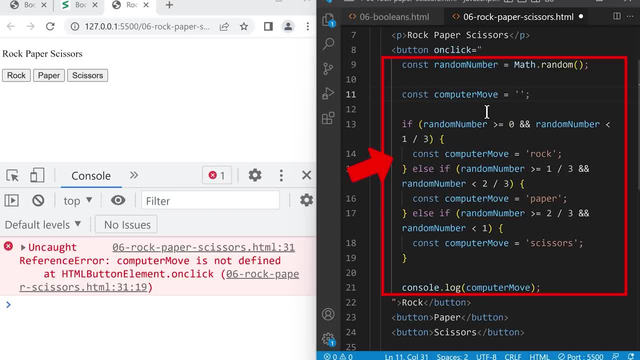 including inside the if statement and then inside the if statement. instead of creating a new variable, we're just going to save the move inside this variable up here, because we can access this variable anywhere else in the code. so instead of using const, we're just going to reassign computer move. 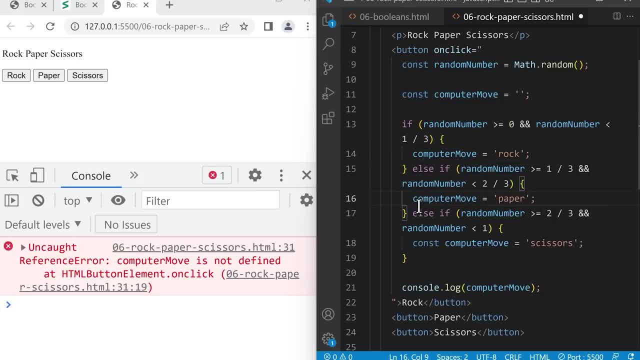 and we're going to remove it here as well, and here as well. and remember, when we reassign a variable we have to switch from const to let. and now, if we save and then click the rock button, we're able to consolelog computer move, because computer move is no. 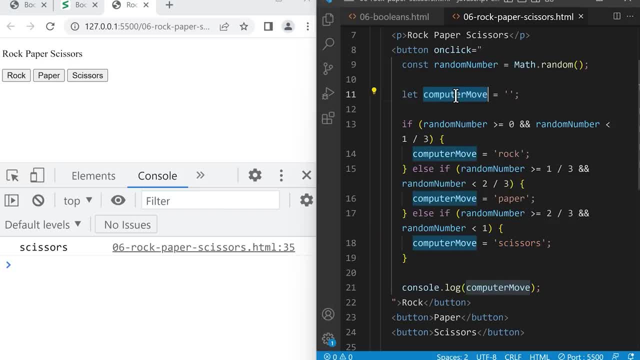 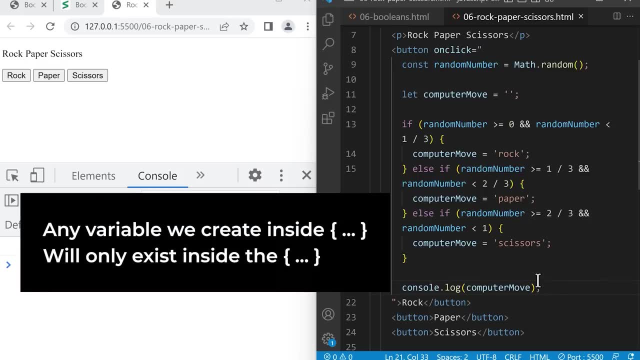 longer inside this scope. it's up here so we can access it in this line of code. so that's how scope works. any variable that we create inside curly brackets will only exist inside the curly brackets. so remember, in the previous lesson we learned a third way of creating variables called var. 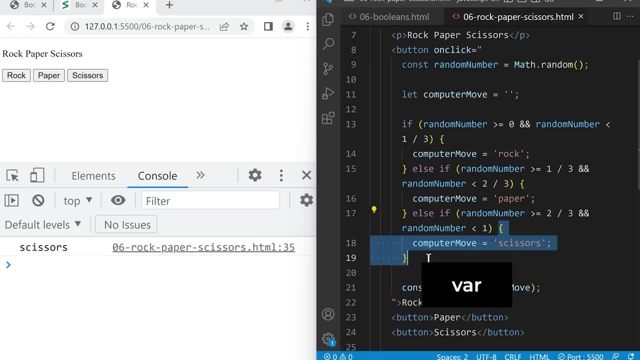 the issue with var is that it doesn't really follow the rules of scope. for example here: if we create a variable with var, like var and random number equals 0.5, this variable will conflict with the variable up here with the same name, even though it's inside a scope. 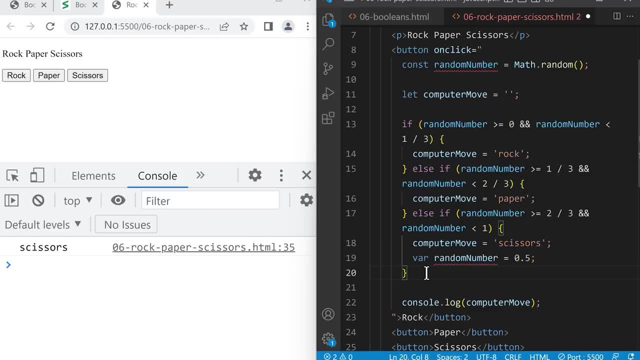 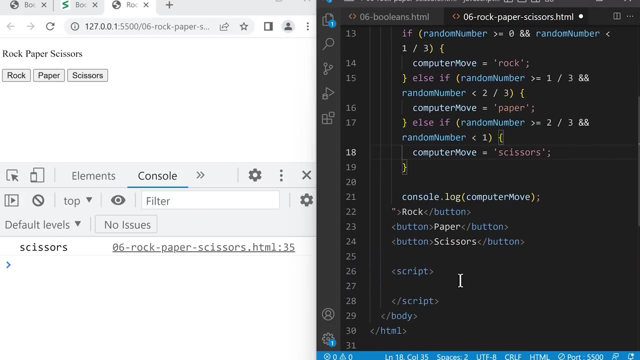 so that's why we don't use var anymore and we just use const and let, because var doesn't really follow the rules of scope. so we can remove this for now and move on to the next step. so we generated a random move for the computer. now we have to compare our move. 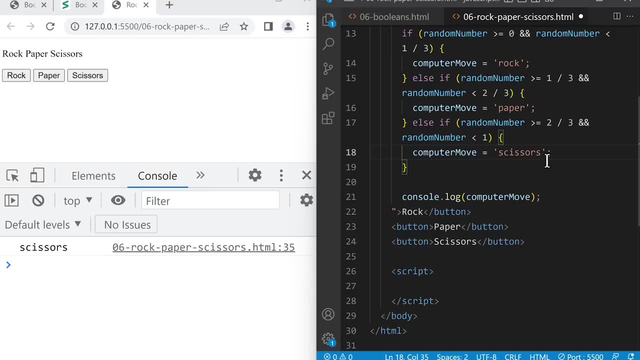 which is rock, to the computer's move to get the result and see who wins. to do that we'll use another if statement. so at the bottom here let's type if and then brackets and curly brackets and then, inside this condition let's check if the computer 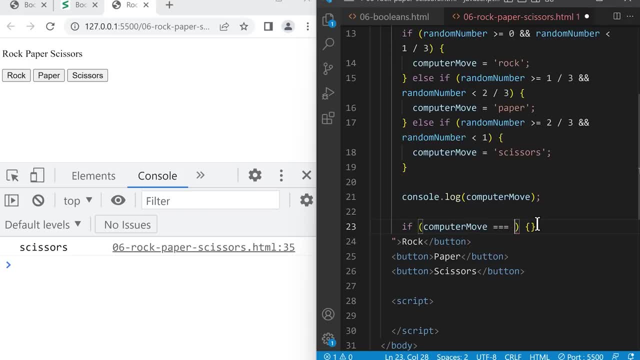 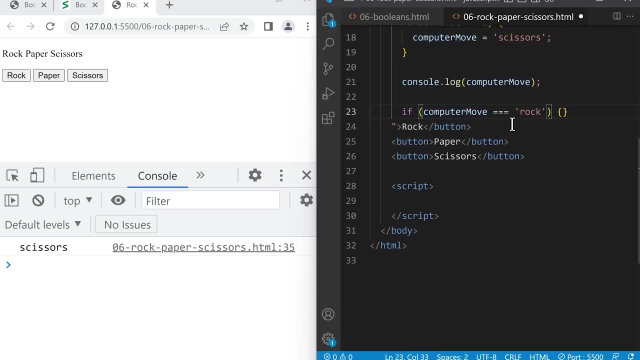 move is equal to rock. so remember, in javascript we always use triple equals instead of double equals to avoid the conversion behavior. and now if the computer's move is rock and our move is rock, then inside the curly brackets the result is going to be a tie, and let's save this string. 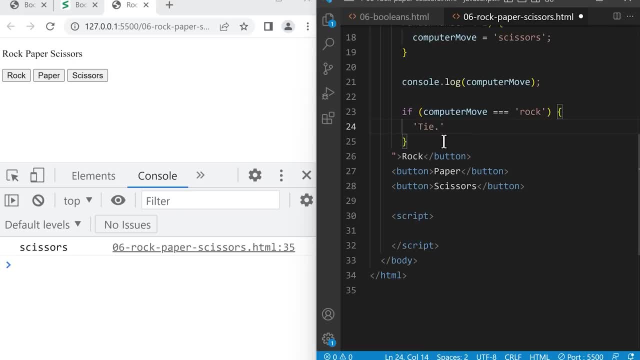 in a variable so we can use it later again. we have the same situation as before. we don't want to create the variable inside here, because then it only exists in this scope between the curly brackets. instead, we're going to create the variable above, outside the if statement. 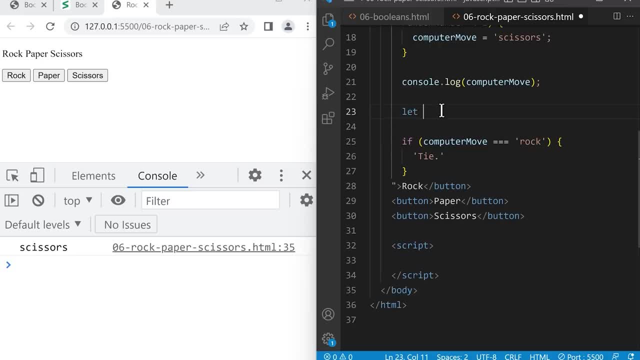 so we'll use let to create this variable, because we're going to reassign it in the if statement. let's name this variable result and just make it equal to the empty string at the top, and then in the if statement, we'll save the result into this variable. 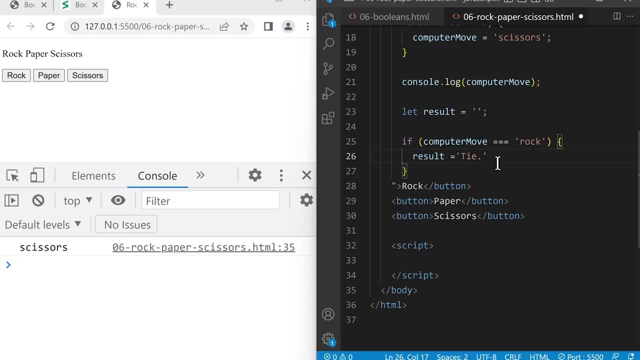 so result equals tie. now let's create the other branches of this if statement. so here we'll add else if brackets and curly brackets, and we'll check if the computer move is equal to paper this time. if the computer move is paper and we picked rock, then we 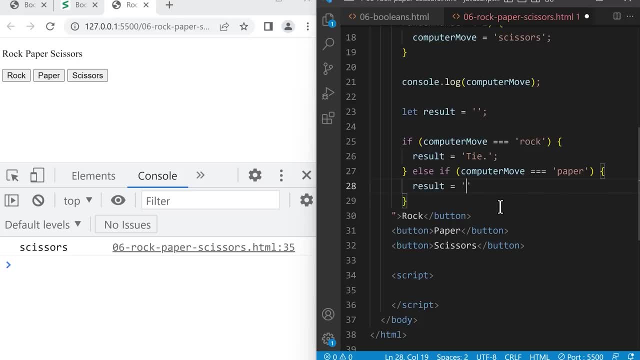 lose, so the result is equal to you lose. and finally we'll add another else: if brackets and curly brackets, and we'll check if the computer move is equal to scissors. and if the computer picked scissors and we pick rock, the result is that you win. so that's. 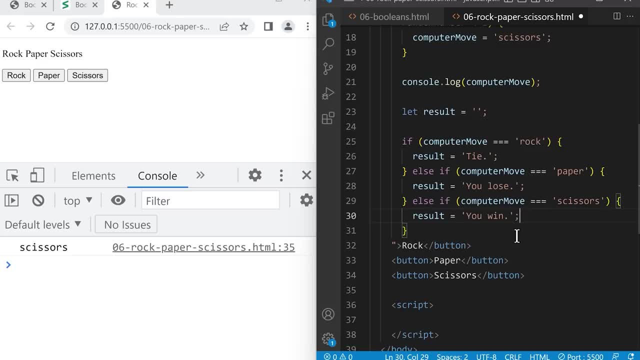 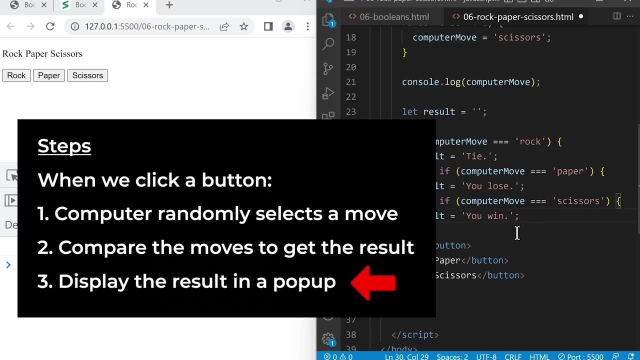 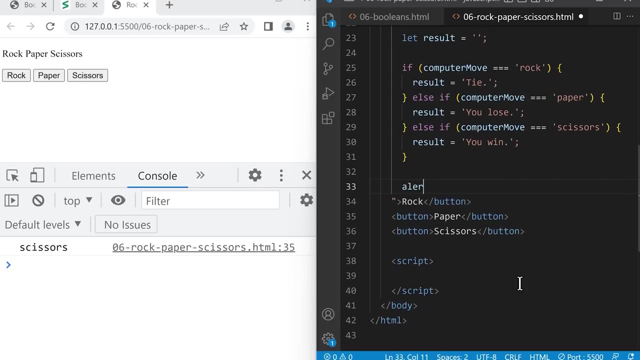 how we compare our move to the computer's random move using an if statement. the last step is to display this result in the popup. so at the bottom let's create a popup using alert- open bracket, close bracket and let's go back to super simple dev to see the message in the popup. 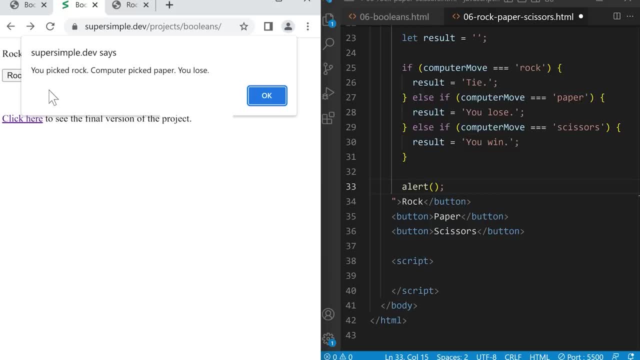 so we'll click this and in the popup it shows our move, the computer's move and then the result, so we can actually just copy this right click, copy and then in here right click and paste. so obviously the computer is not going to pick this move every time and this is not going to. 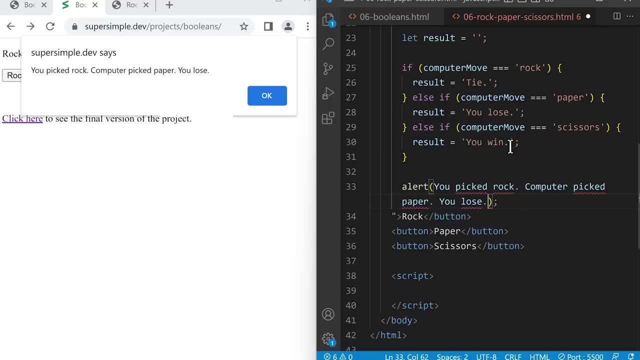 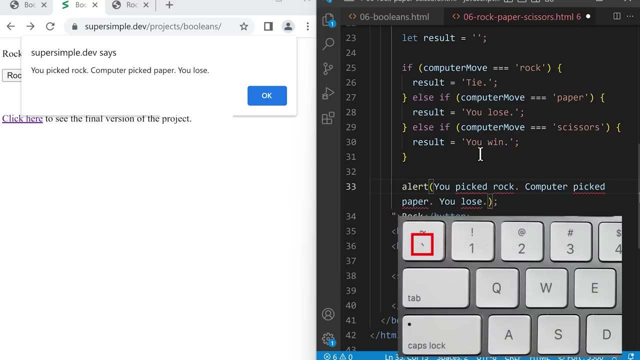 be the same result every time. instead, we want to insert computer move into here and we want to insert result into here. so, because we want to insert values, we're going to turn this into a template string using backticks, and now, instead of paper, we're going to insert a. 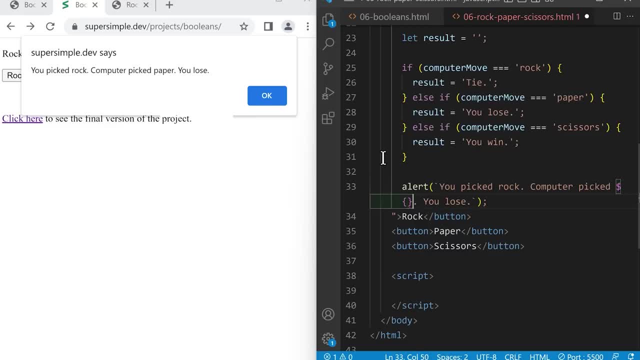 value using dollar and curly brackets and we're going to insert the variable computer move and instead of this text, every time we're going to insert the variable result. and now, if we save and we can click ok to close this and go back to our tab and click. 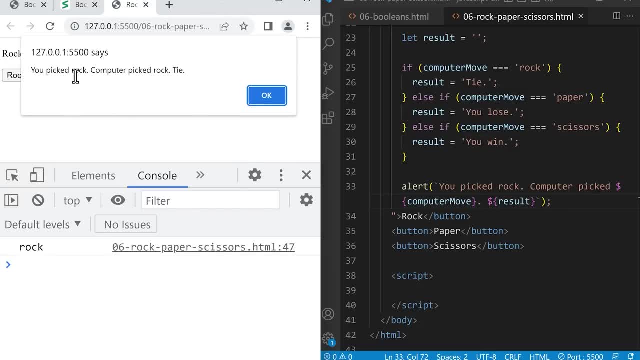 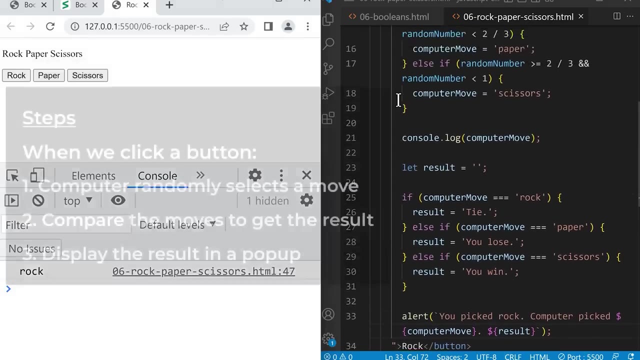 the rock button. we're going to pick rock, the computer will pick a random move and it will show us the result in a popup. so that's how we create this simple version of rock paper scissors. in our code we did things step by step. first, we generated a random number. 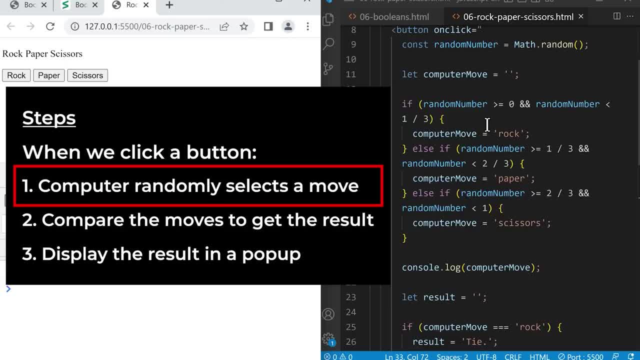 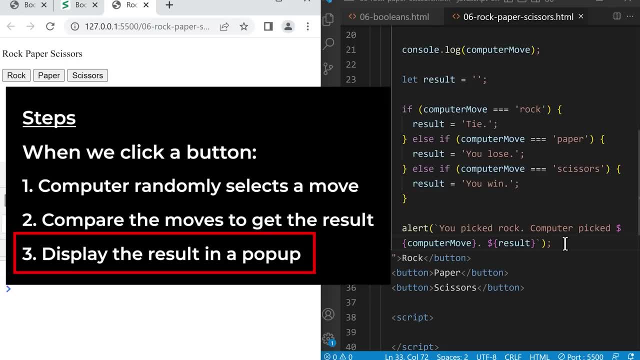 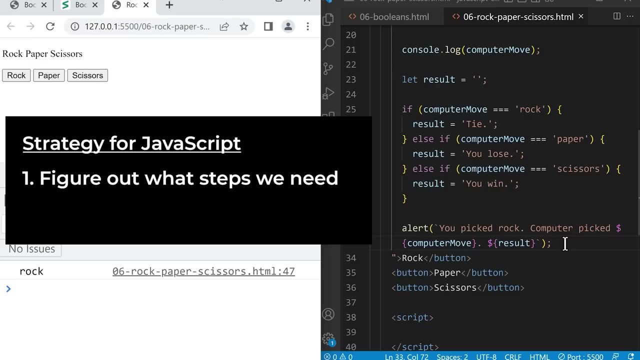 we converted it into a move for the computer and then we compared our move to the computer move and we displayed the result in a popup. so, as you can see, when we're writing javascript, we first figure out what steps we need to do. this is called an algorithm. 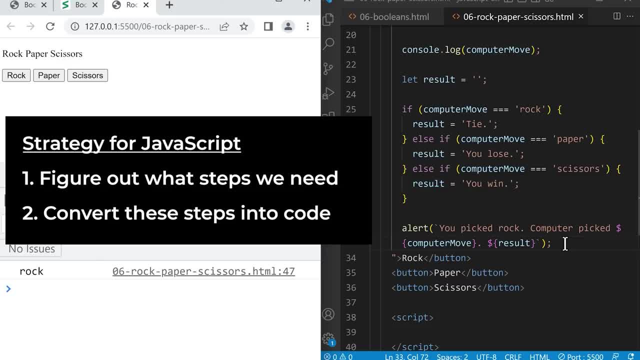 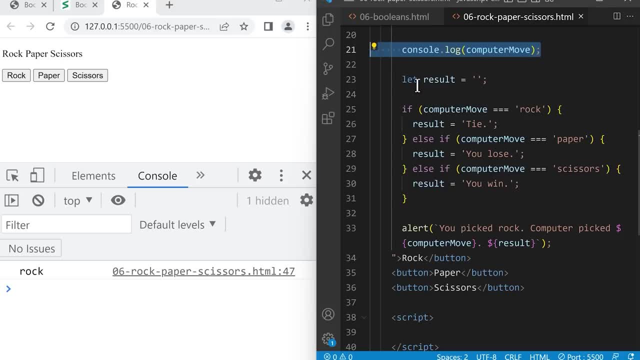 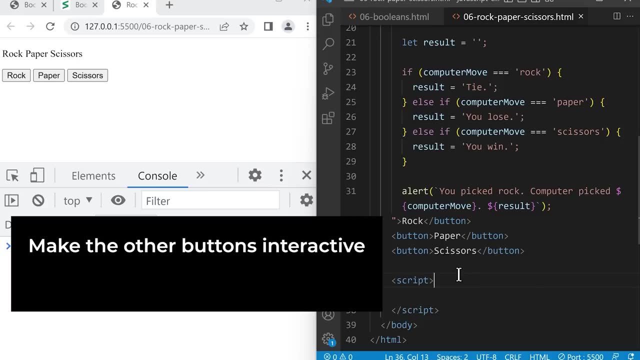 and then we convert these steps or this algorithm into code. so now we can actually remove this consolelog because we don't need it anymore, and the last step is to make the other buttons here interactive. so feel free to pause this video if you want to try it yourself first. 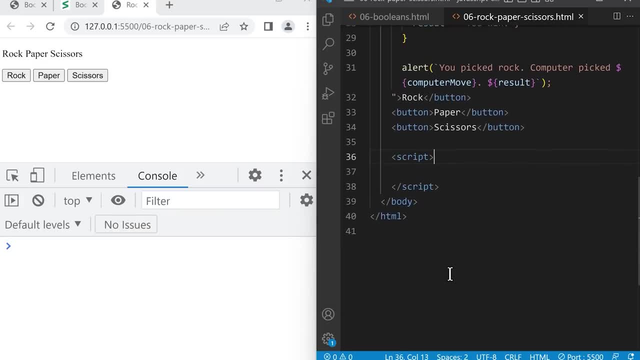 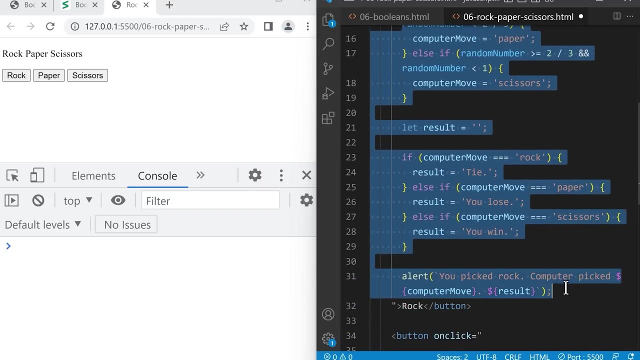 for the paper button. let's add some new lines to make it a little easier to read, and again we'll add the on click attribute and then inside here we can actually make a copy of all the javascript we wrote, so we can select all of this and then 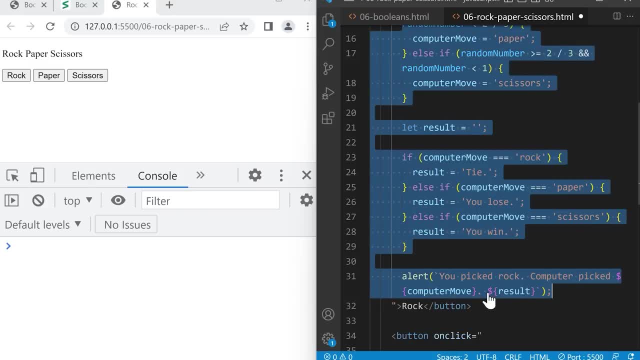 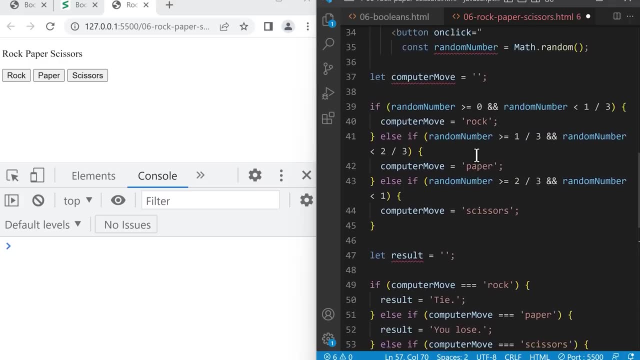 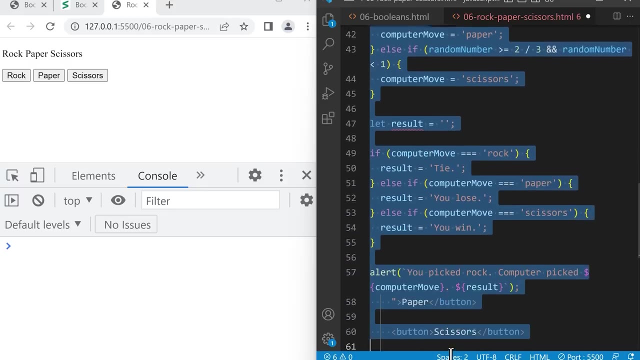 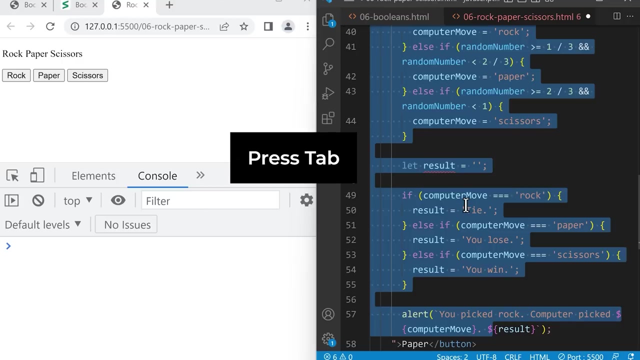 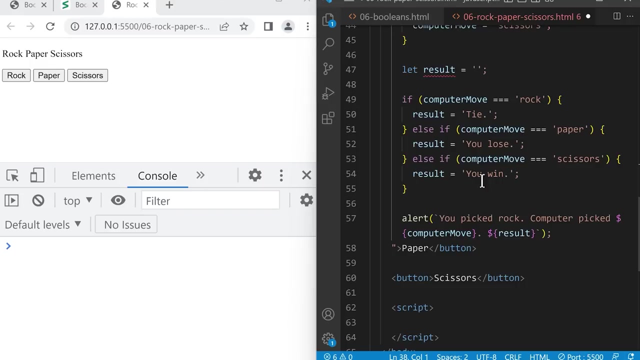 right click, copy and then in here right click and paste. if the formatting doesn't look right, we can select all of these lines and press tab to add indents until the formatting looks good. the one thing we have to change here is that now we picked paper, so 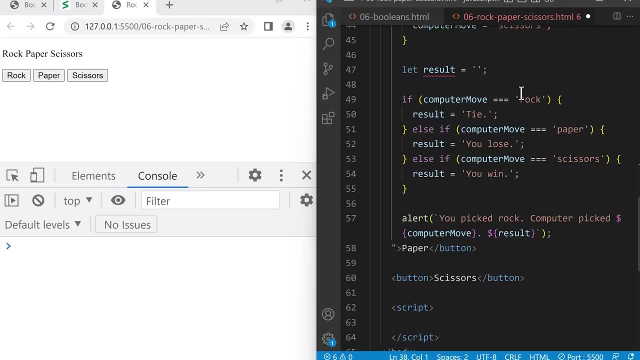 the result is going to be different. if the computer picks rock and we pick paper, that means you win. if the computer picks paper now, it means that we tie, and if the computer picks scissors, that means you lose. and here we'll also change: you pick rock to paper. 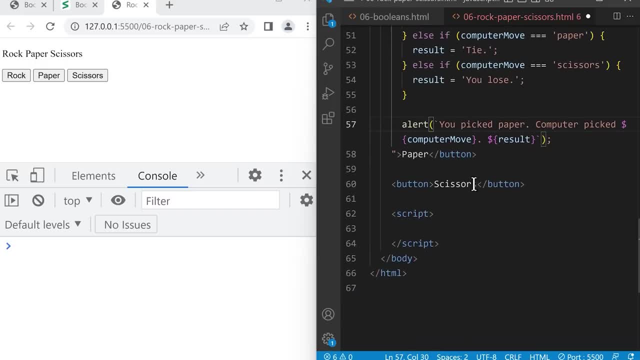 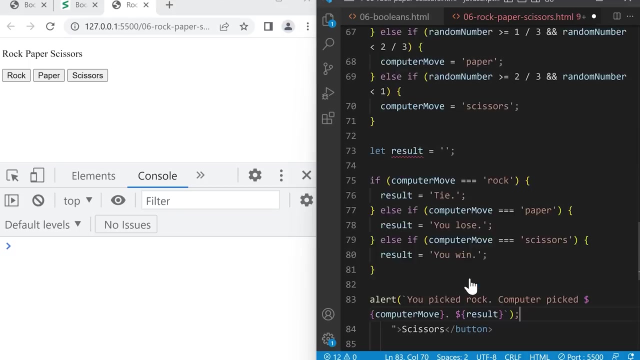 and that's it. the last step is to make the scissors button interactive. so again on, click equals double quotes, and then we'll make a copy of the code. so i already have it. so just right, click and paste and then again select the code that we need to fix the formatting for. 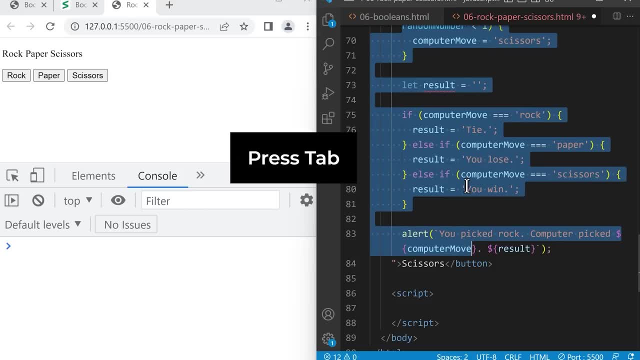 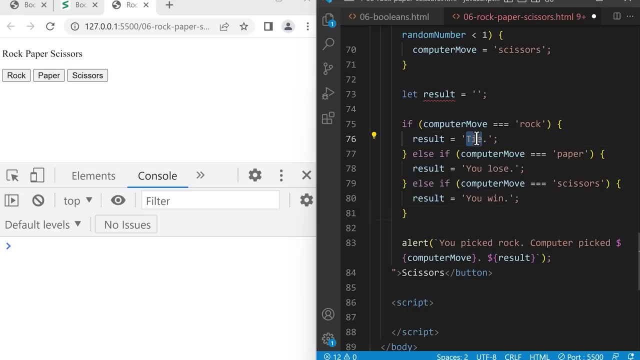 and press tab, and here we pick scissors. so if the computer picks rock, then the result is you lose. if the computer picks paper, the result is you win. and if the computer also picks scissors, the result is a tie, and we'll change you: pick rock to scissors. 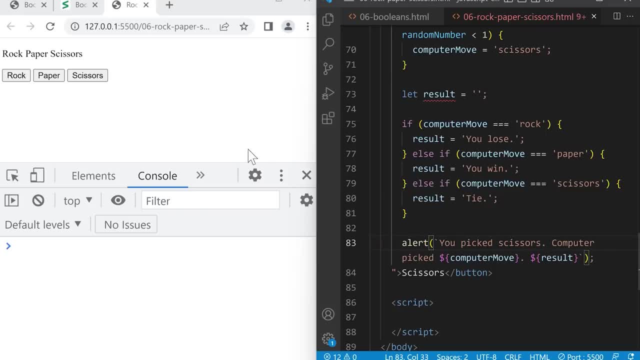 now, if we save and try out our game, if we click rock, we're going to pick rock- computer picks a random move and it will show us the result here. let's press ok and try paper: this also works correctly. let's press ok and click scissors, and this also works correctly. 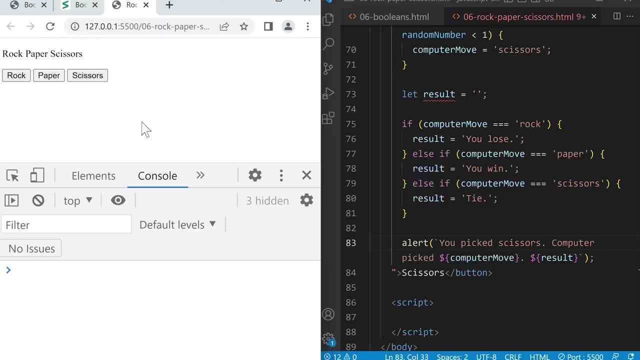 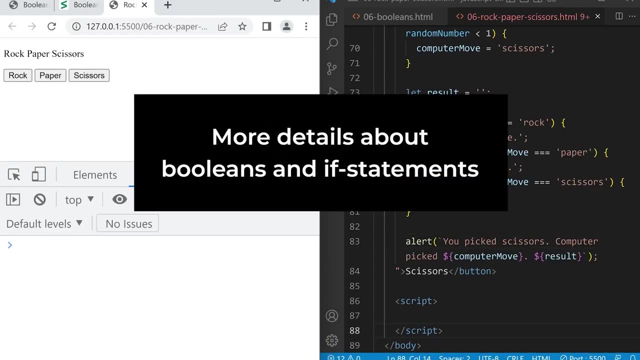 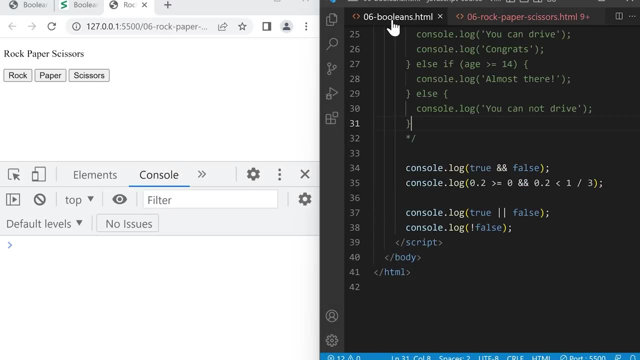 and that's it. we just finished creating a simple version of this rock paper scissors game. in the rest of this lesson we're going to learn more details about booleans and if statements. let's go back to booleans dot html and open the tab for this file. 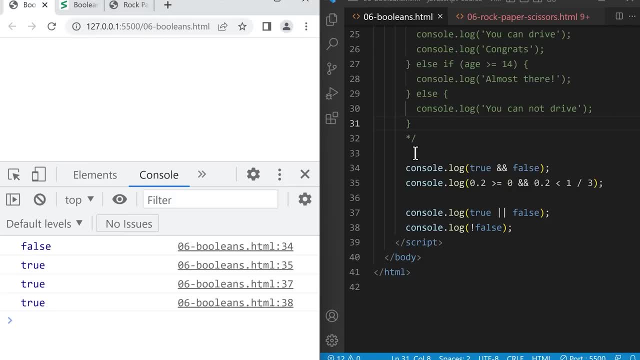 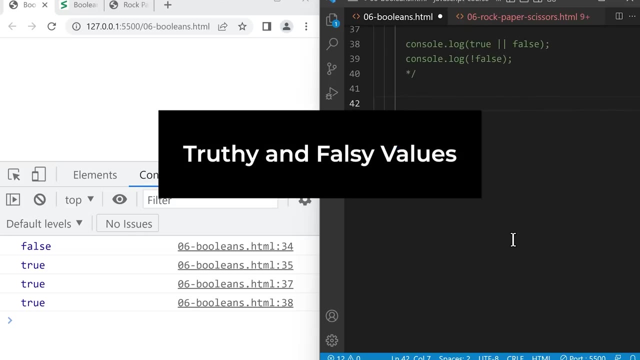 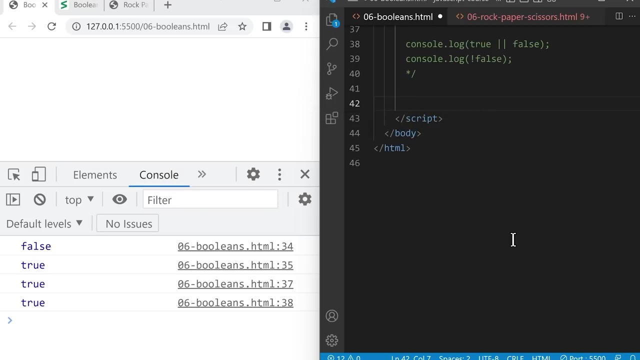 and let's comment out the previous code using slash, star and star slash and create some new lines. the next thing we're going to learn is called truthy and falsy values. so if statements don't just work with boolean values like true and false, they actually work with. 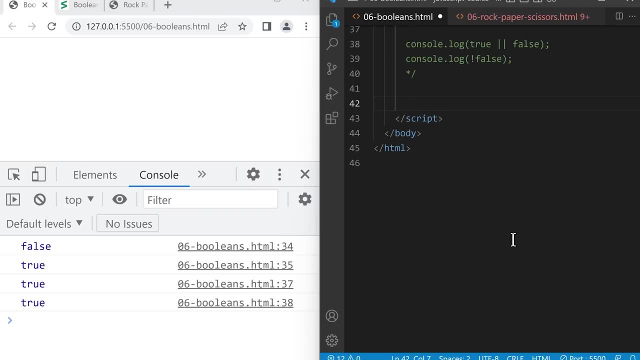 any type of value, including numbers and strings. for example, let's type if brackets and curly brackets, and inside this condition, instead of putting a boolean value, we're going to put a number like five, and then inside the curly brackets, let's console dot log the string truthy. 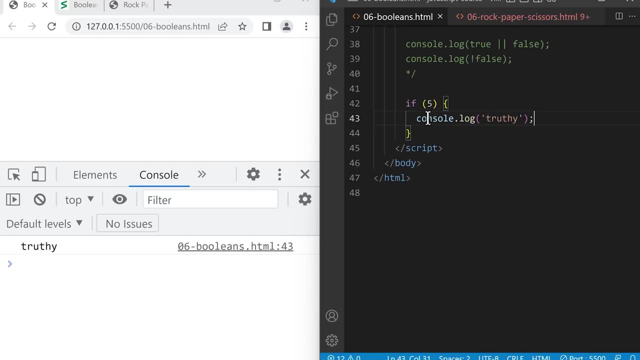 if we save the number five behaves just like true. it causes the if statement to run this code. so we call this value a truthy value because it behaves just like true. now let's change this value to a different number- zero. if we save the number zero, 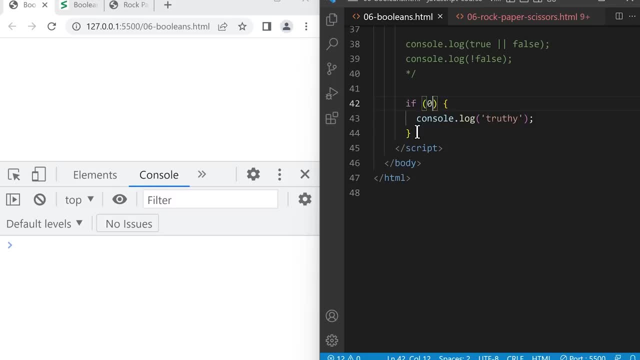 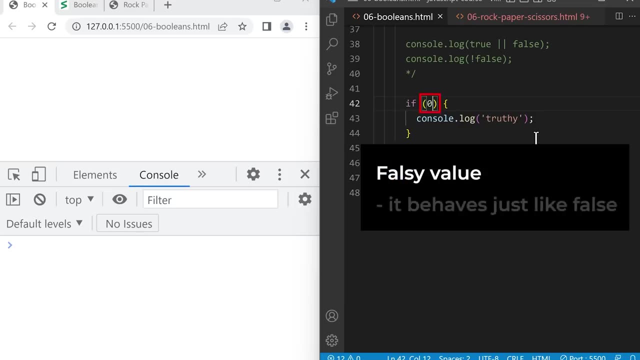 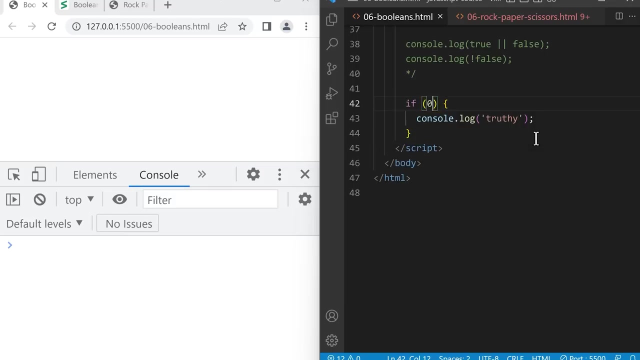 behaves just like false. it causes the if statement to not run this code. we call this value zero a falsy value because it behaves just like false. so how do we know if a value is truthy or falsy in javascript? the list of falsy values. 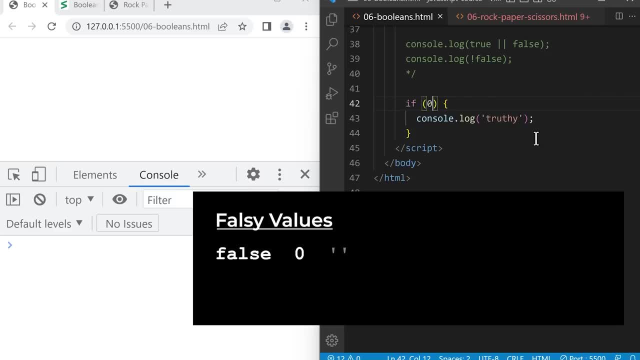 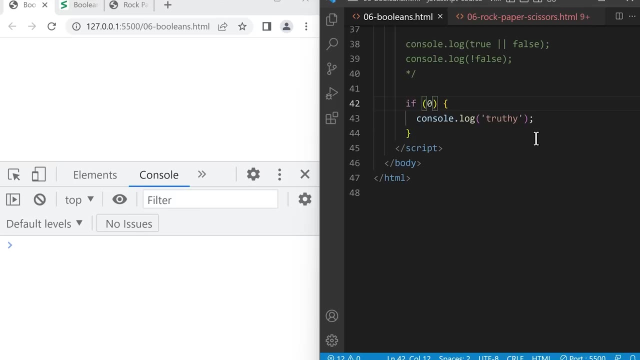 are false. remember zero, the empty string nan undefined and null. any value that is not on this list is a truthy value. so why do we use truthy and falsy values? one way we use them is like a shortcut in our code. for example, let's create: 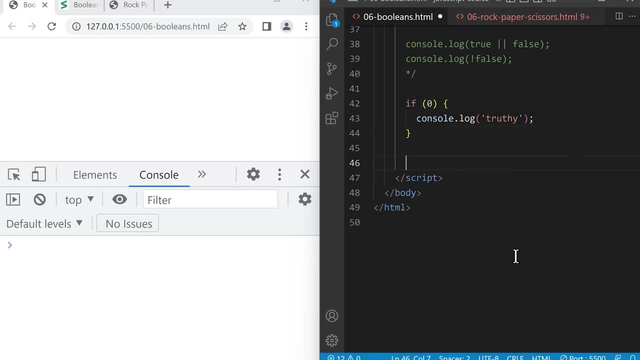 a variable at the bottom using const, and let's call it cart quantity and make it equal to five. next, let's create an if statement, if brackets and curly brackets, and inside the curly brackets let's type console, dot, log. the string cart has products. now let's say that we 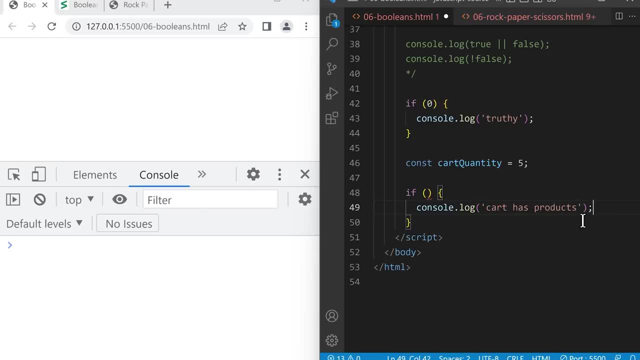 only want to display this message. if our cart has products usually inside this condition, we would check if cart quantity is greater than zero. but now, instead of doing this comparison, we can actually just type cart quantity and it will behave the same way if the cart quantity is not zero. 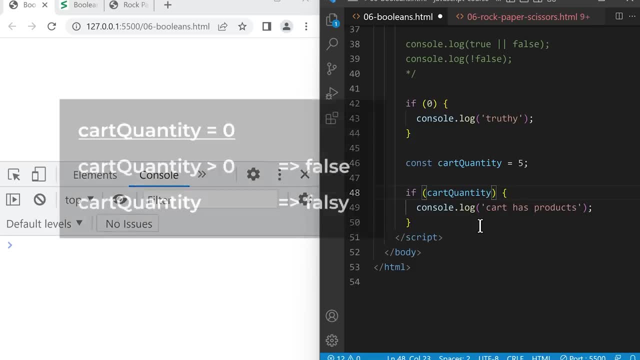 they will both behave like true. if the cart quantity is zero, they will both behave like false. so here, the cart quantity is five, which is a truthy value. if we save, this causes the if statement to run this code. as you can see, instead of doing comparisons, we can. 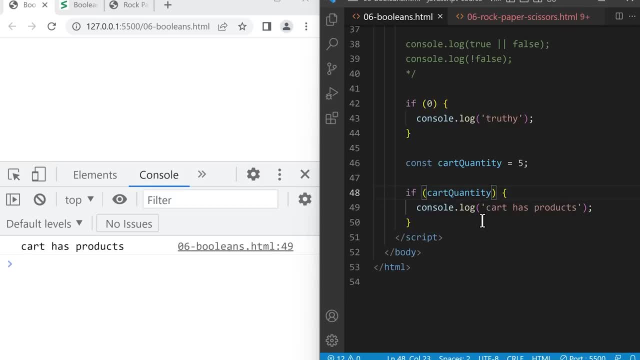 use truthy and falsy values as shortcuts. truthy and falsy values also work with logical operators. for example, if we console dot log, the not operator and the number zero. zero is a falsy value, it behaves just like false, so the not operator will flip it into true. 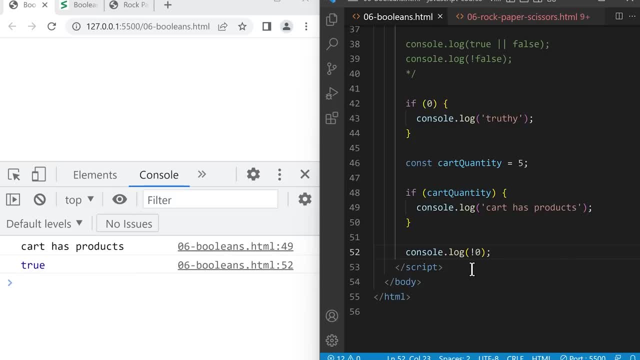 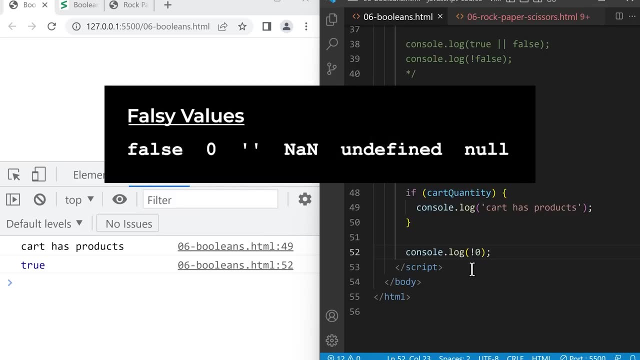 if we save, this will display true. now that we understand truthy and falsy values, let's go over the list of falsy values, because there are some that we haven't learned yet. we already learned false zero and the empty string, the next falsy value. 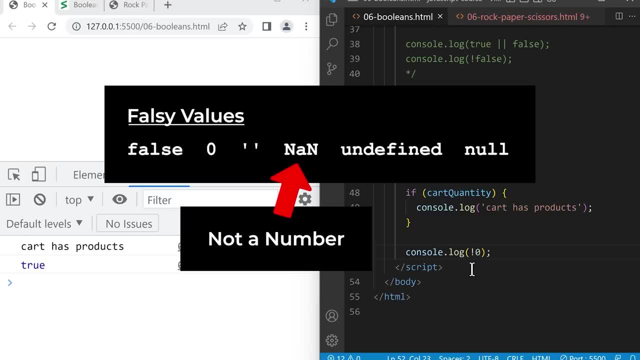 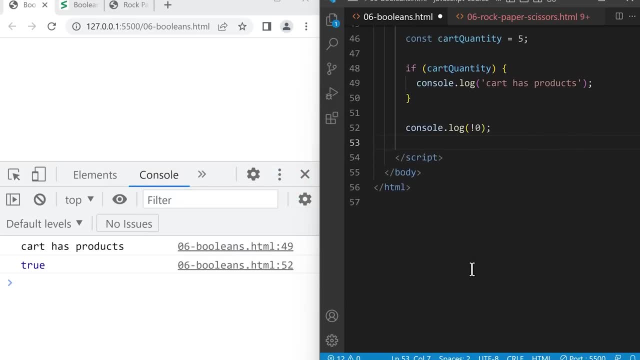 is nan, which means not a number. we get nan if we do some invalid math. for example, at the bottom let's type console dot log the string text divided by the number five. so obviously this is not valid math. if we save, javascript will tell us that the result of this 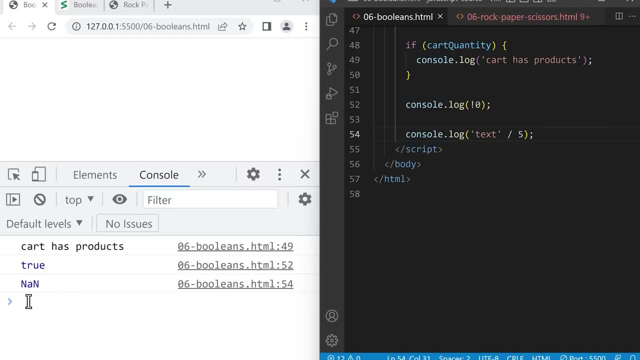 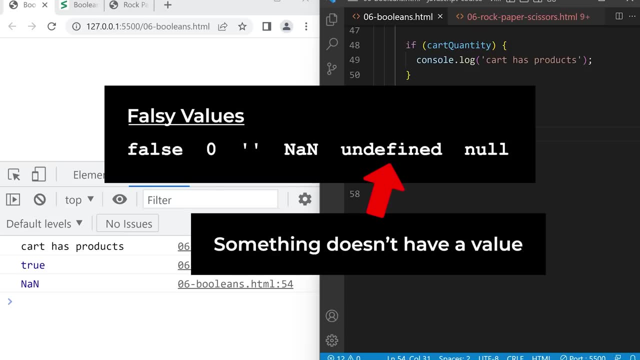 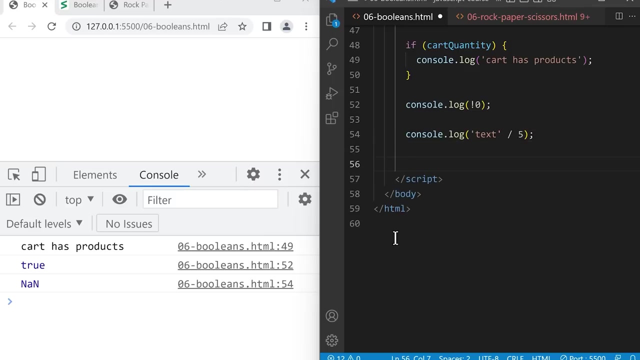 calculation is not a number or nan. the next falsy value is undefined. undefined represents that something doesn't have a value. for example, at the bottom, if we create a variable with let variable one and we don't give it a value, and then we console dot log this. 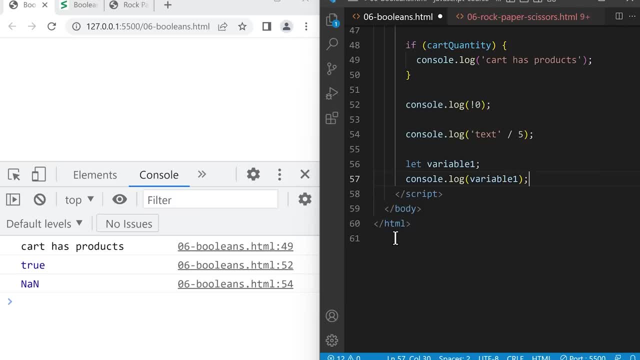 variable and we save, it will show us that variable one contains the value undefined. so undefined represents that this variable doesn't have a value. one thing to note with undefined is that we can only use this syntax with let. we can't use it with const. if we really want to use this with const. 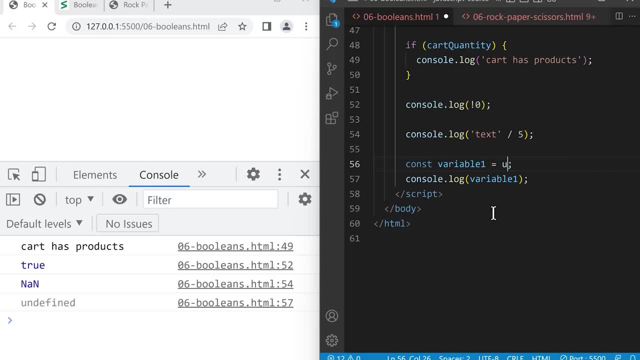 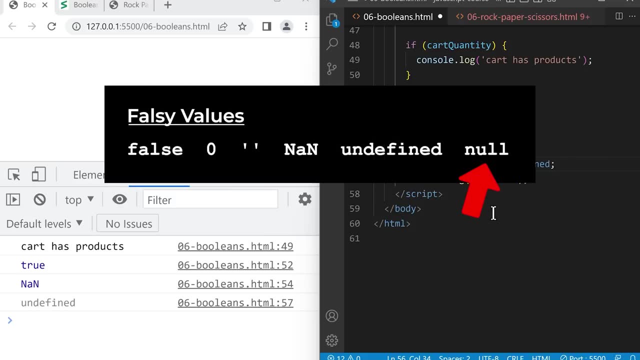 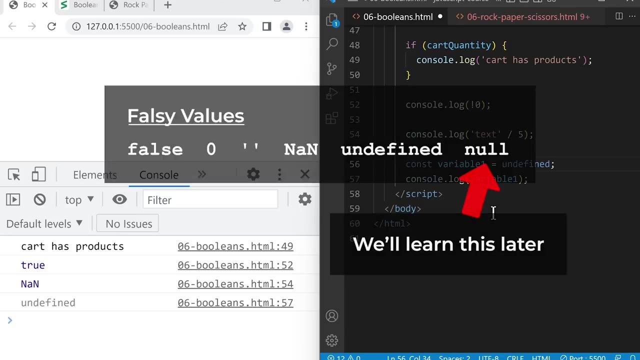 we have to type out equals undefined directly. the last falsy value is null. we'll need some extra knowledge to understand null, so we'll learn about null later in this course. the last thing we're going to learn in this lesson are some shortcuts for if statements. 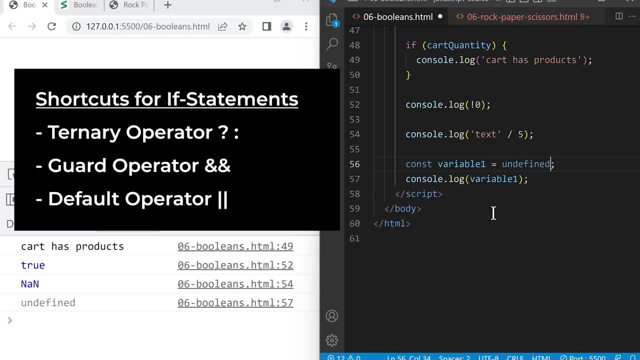 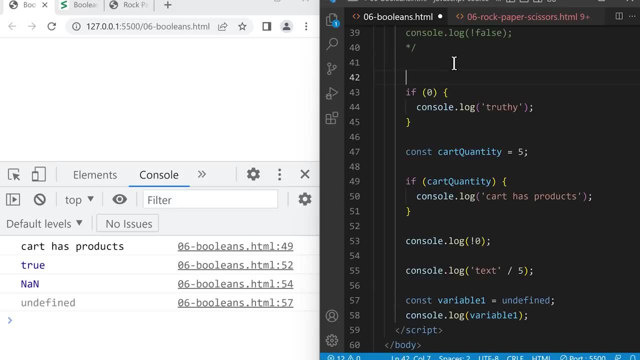 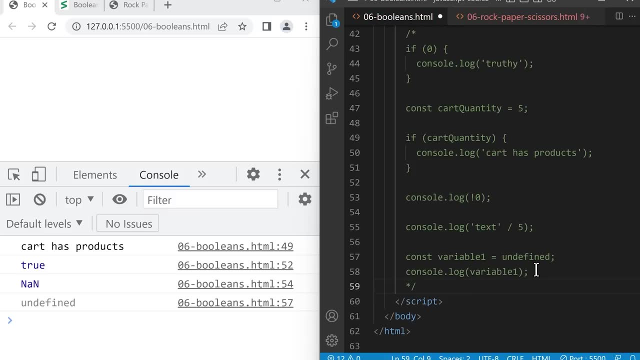 called the ternary operator, the guard operator and the default operator. first let's comment out this code so our console doesn't get too messy: slash, star. and then at the bottom star, slash and let's scroll down and we'll start by learning the ternary operator. 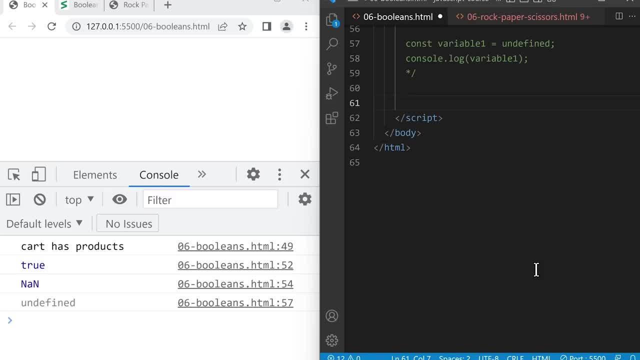 we're going to type a boolean value like true, and question mark another value, for example the string truthy, and then colon and another value like the string falsy. so this is the ternary operator. this is similar to an if else statement. the first value is like the condition. 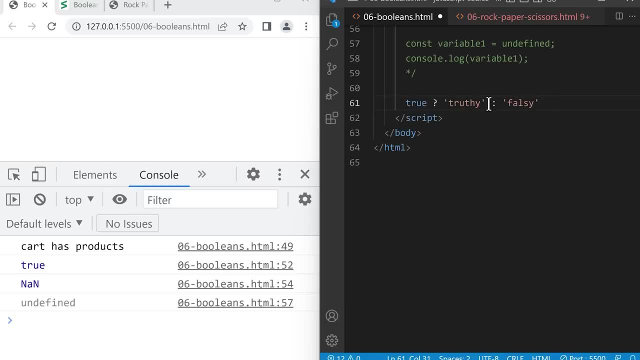 if it's truthy, the result of this code is the value after the question mark. if the first value is falsy, the result of this code is the value after the colon. so you can think of the question mark as the if branch and the colon as the else branch. 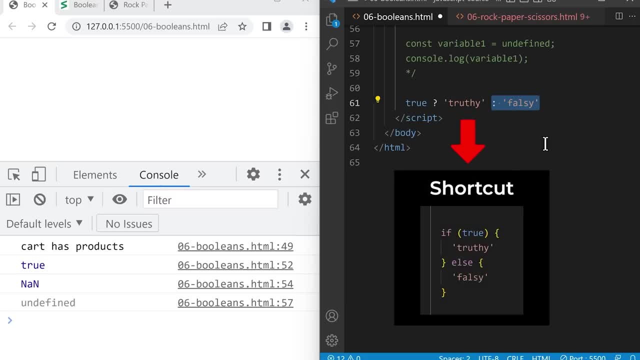 this is sort of like a shortcut for an if statement like this. now, an advantage of the ternary operator over an if statement is that we can save a ternary operator in a variable. so at the front we can do: const, result equals. and now if we? 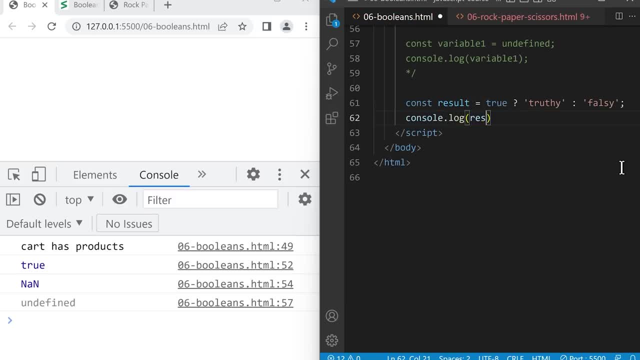 console dot, log the result and save. the first value is true, so the value after the question mark gets saved in the variable. as always, we can use truthy and falsy values instead of just true and false. so here, if we change the first value to a falsy value, 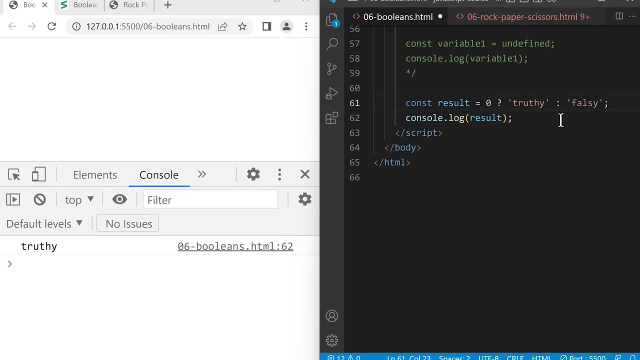 like zero. this will cause the value after the colon to get saved inside the variable. if we save, that's exactly what happens. so this is the ternary operator. it's sort of a shortcut for an if else statement like this: the next shortcut is called the guard operator. 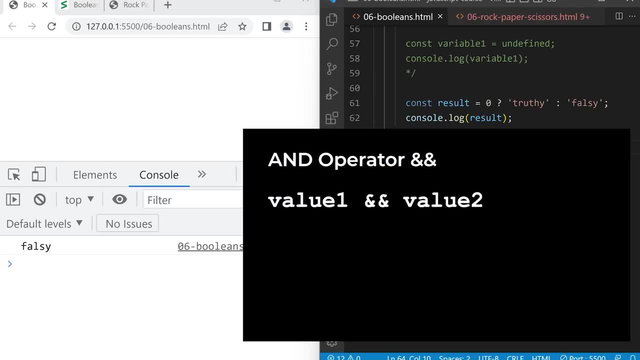 earlier in this lesson we learned the and operator, which checks if two sides are both truthy. the and operator has a special feature. let's say we have an and operator and the left side is false. in this situation we already know it's impossible for both sides to be truthy. 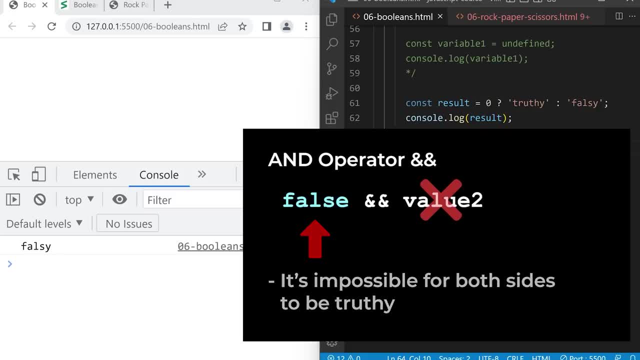 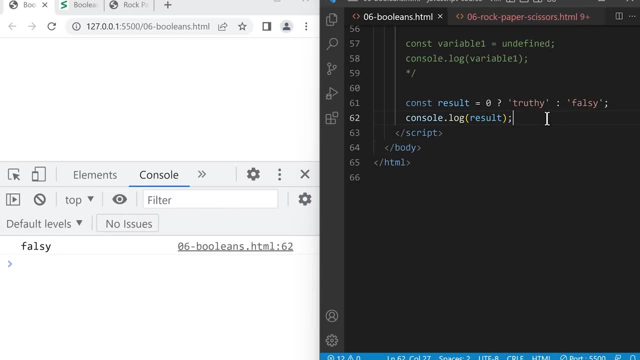 so we don't even need to check the right side. so the and operator actually stops early and doesn't even run the code on the right. this is called a short circuit evaluation. for example, let's go into our code and create some new lines and we'll type: 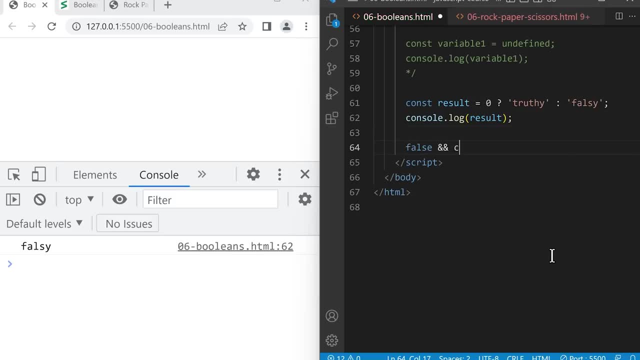 false and console dot log hello. if we save. the left side is falsy, so the and operator stops early or short circuits and it doesn't even run the code on the right. so, as you can see, we can use the value on the left to block or guard. 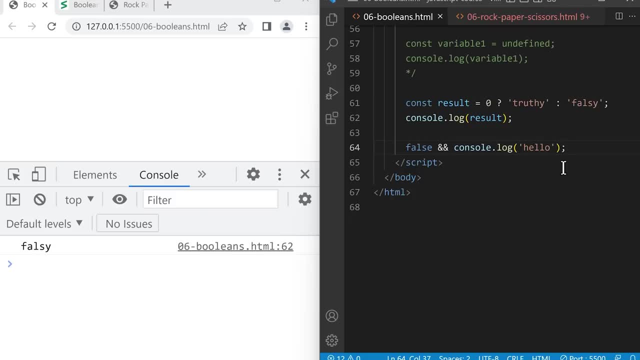 the code on the right. so when we use the and operator like this, we call it the guard operator. this is sort of like a shortcut for an if statement like this and, just like the ternary operator, we can save the guard operator in a variable, for example. 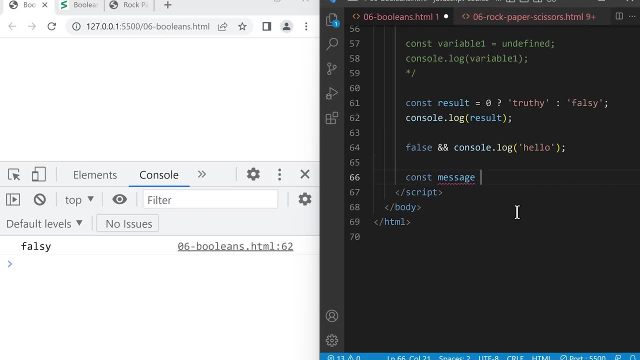 let's create a variable const message and make it equal, false and the string hello. if the first value is falsy, the guard operator will stop early and the result will be the first value. if we console dot, log this message and save the value, false will be saved. 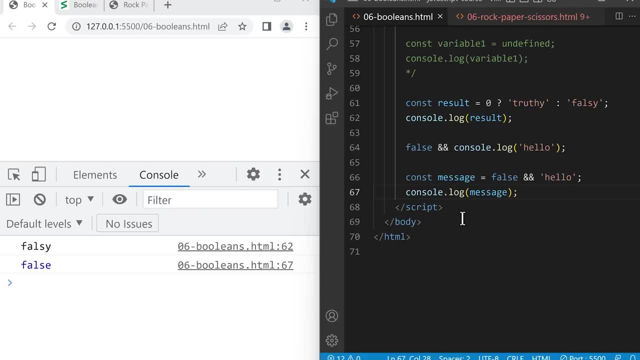 inside this variable. now let's change this value to a truthy value, like the number five. now it will not stop early and it will give us the second value. as the result, if we save the string, hello is now saved inside this variable. this is sort of like a shortcut. 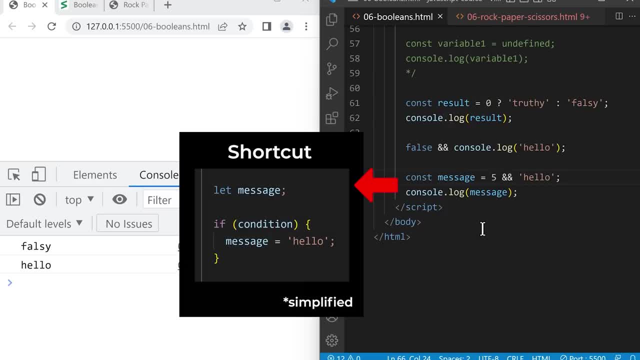 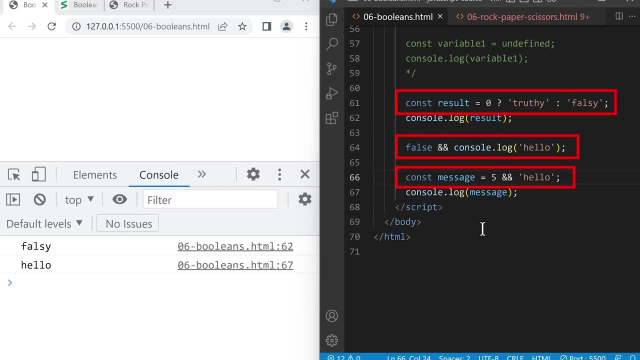 for an if statement like this, so don't worry if it's a bit confusing. all of these are just shortcuts for an if statement. they're sort of like an if statement that we can write on a single line. the last shortcut is called the default operator, which is similar to the guard. 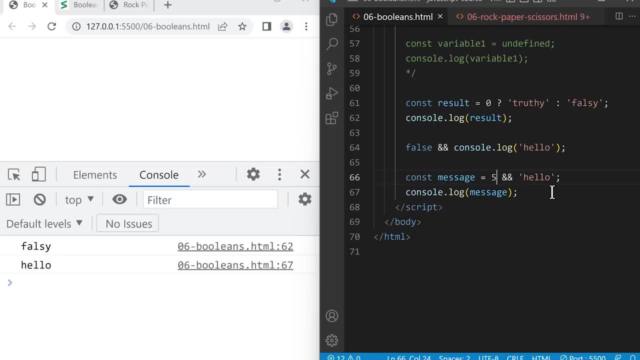 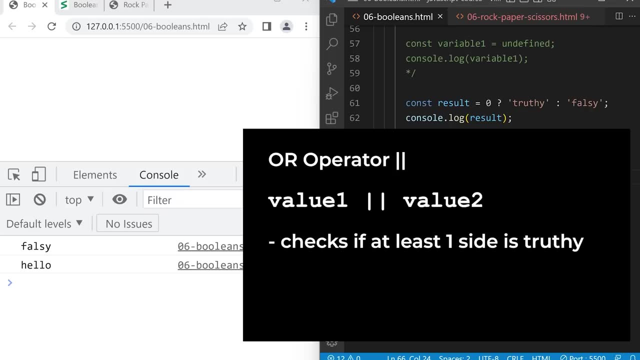 operator but uses or. earlier in this lesson we learned the or operator, which checks if at least one side is truthy. let's imagine we have an or operator and the left side is true. in this situation, we already know the result of the or operator because the left side 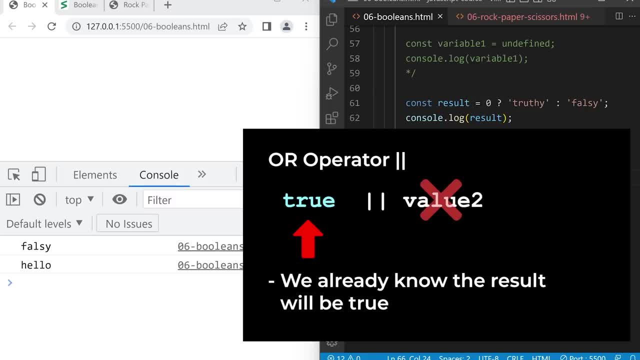 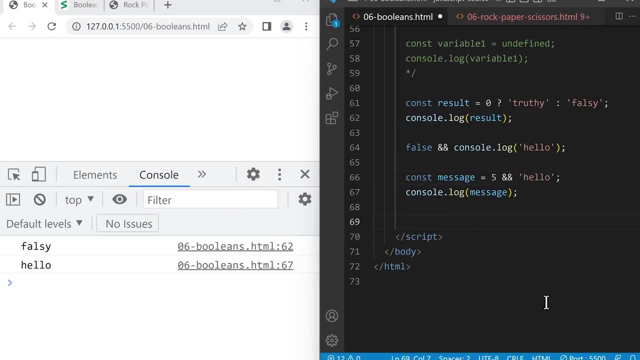 is already truthy, we don't even need to check the right side, so the or operator also stops early or short circuits if the first value is truthy. for example, let's create some new lines and let's say that in our final amazon project we can choose a current. 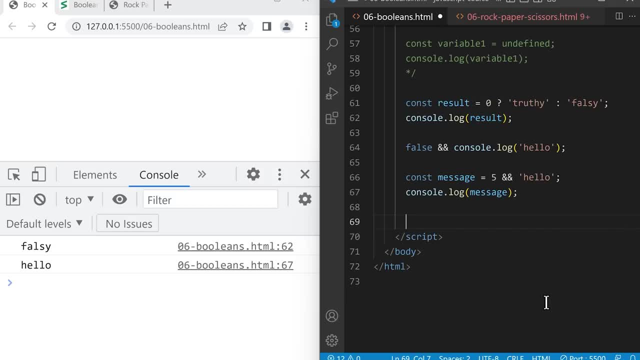 c to pay for our order. let's create a variable with const currency and make it equal to the string eur or euros. now let's say that choosing a currency is optional. if we don't choose a currency, we'll use a default value of usd. 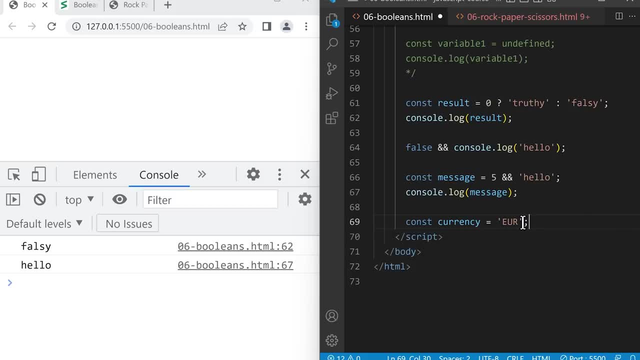 or united states dollars to create a default value. we can go to the end and type or the string usd. so here the left side is truthy. so the or operator will stop early and it will result in the value on the left. if we console dot log the. 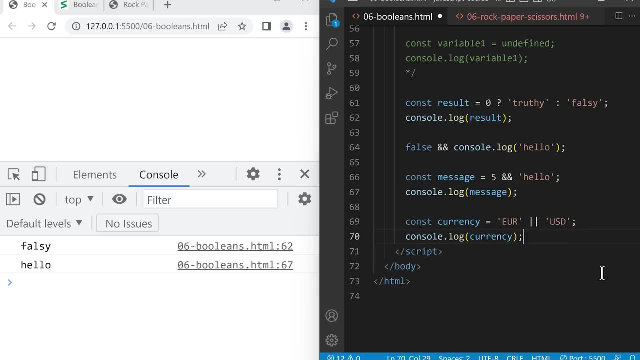 currency and save, it will display euros. now let's say that we didn't choose a currency because it's optional. so let's go here and we're going to change this currency to undefined. now the left side is falsy, so the or operator does not short circuit. 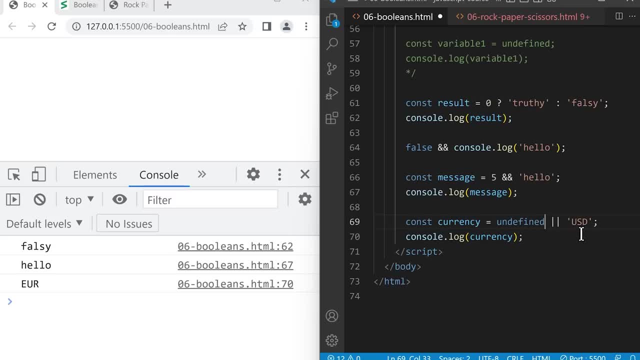 it will continue and the result will be the value on the right. if we save now the string usd is saved inside currency. as you can see, we can use the or operator to set a default value. so when we use the or operator like this, we call it the default operator. 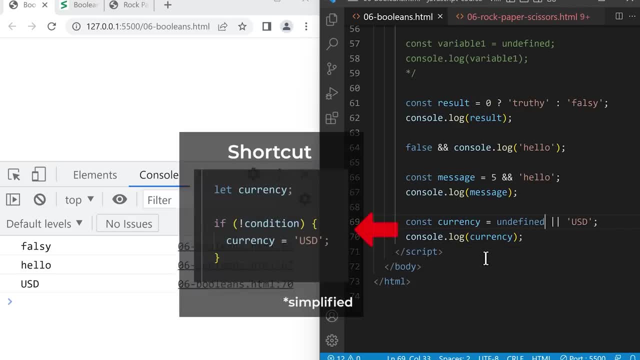 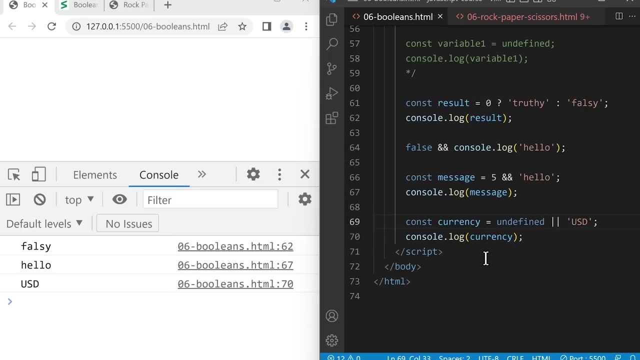 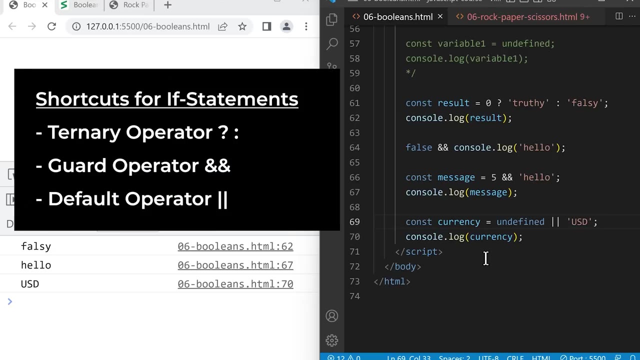 the default operator is sort of a shortcut for an if statement like this. so, don't worry, remember that everything that we learned in this last section are basically some shortcuts for if statements. we don't have to use them, but they can save us some typing and that's the end of this lesson. 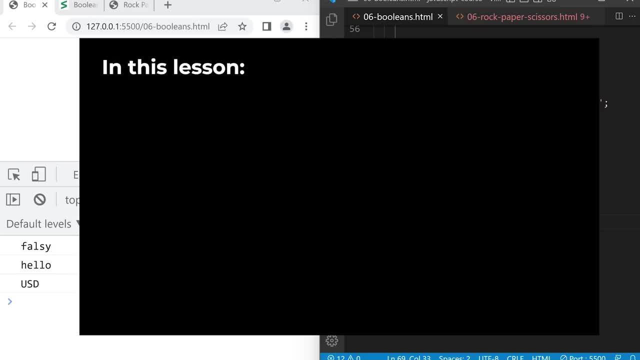 in this lesson we learned about booleans and if statements. boolean values represent whether something is true or false. we learned how to use if statements to make decisions in our code. we learned how to use comparison and logical operators. we learned about algorithms and we created a simple version of. 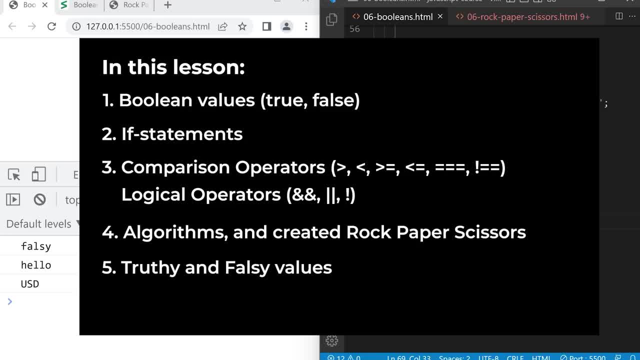 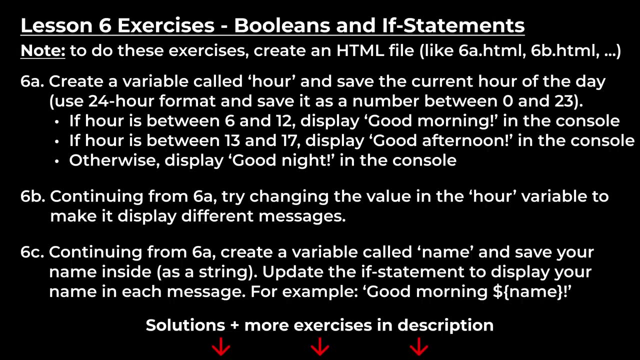 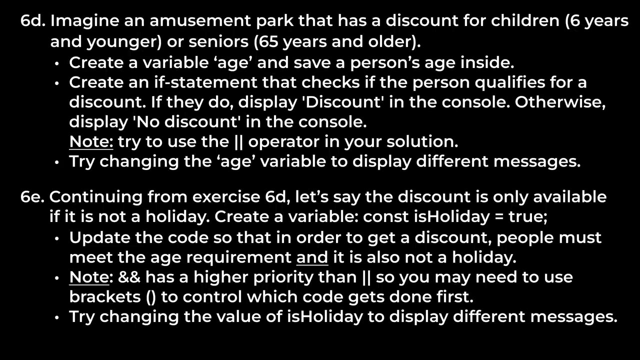 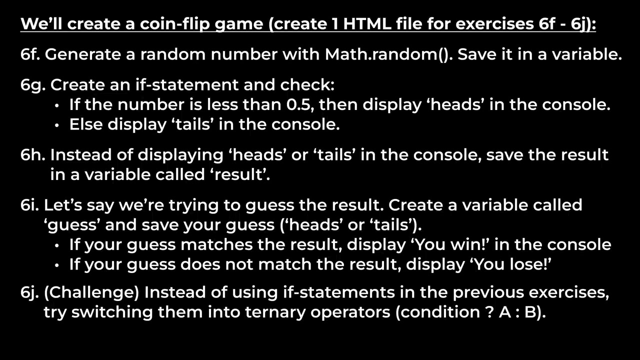 rock paper scissors. we learned about truthy and falsy values, and we learned some shortcuts for if statements, the ternary operator, the guard operator and the default operator. here's some exercises to help you practice booleans and if statements- dem怄. in this lesson we're going to learn. 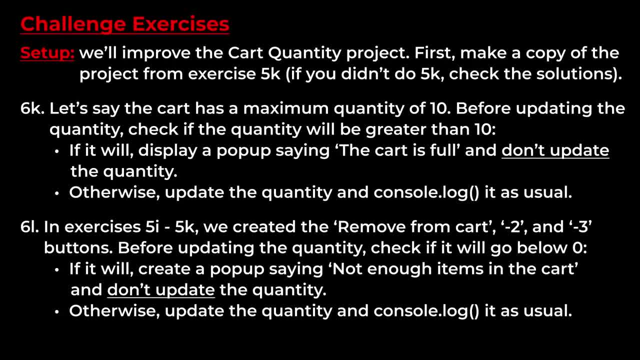 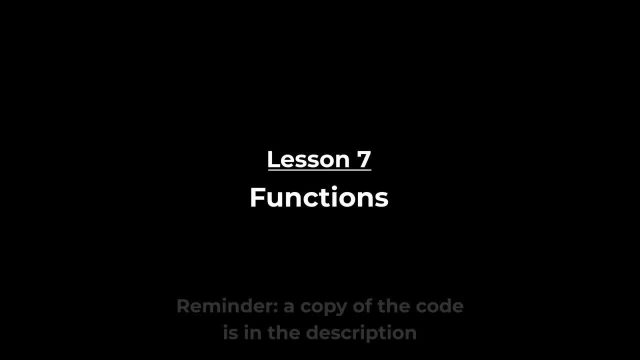 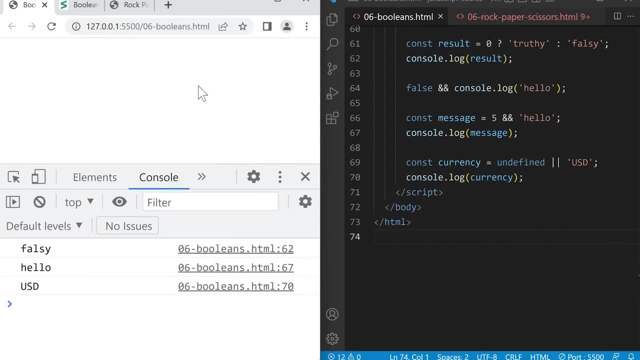 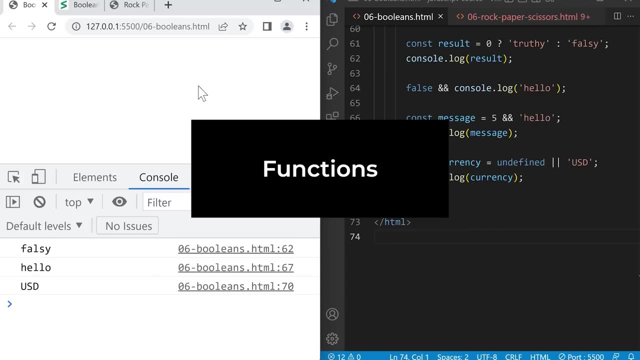 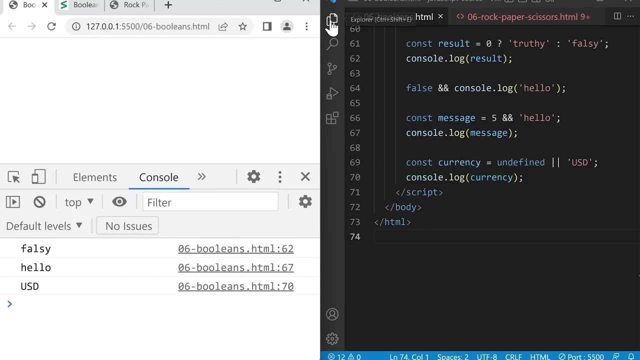 the next feature of javascript called functions, and we're going to use functions to improve our rock paper scissors. we're going to increase the number of aż, our rock-paper-scissors project. First, let's create a new file for this lesson. We'll go to our code editor and create a new file and let's name this file. 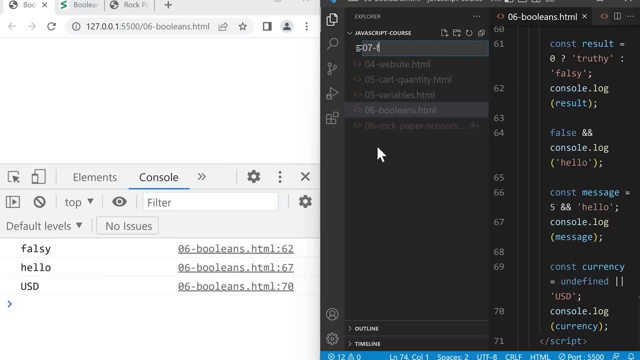 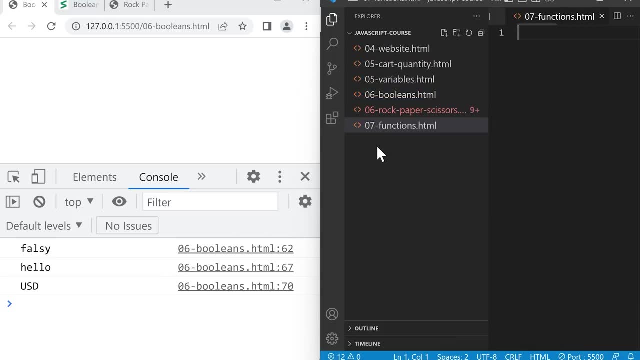 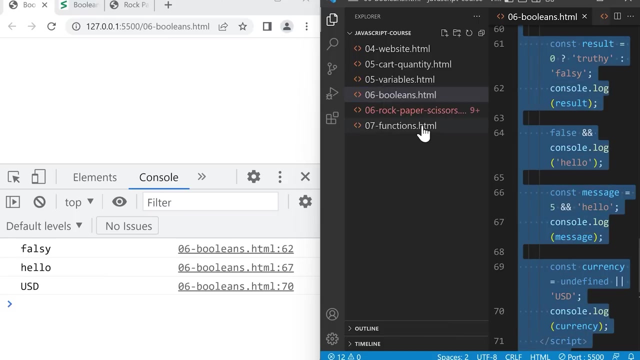 07-functionshtml and press enter. Next let's copy booleanshtml to functionshtml. So we'll click this file and then select all this code using Ctrl A or Command A, and then right-click, copy and in here, right-click and paste. 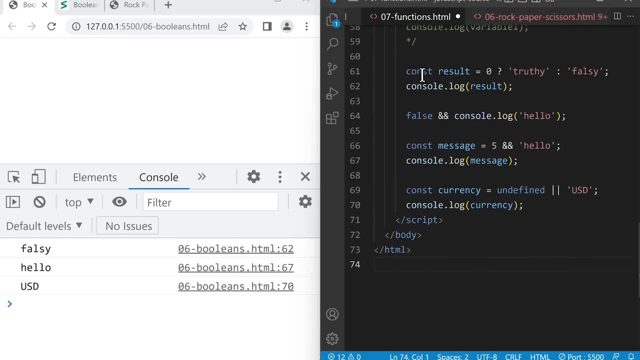 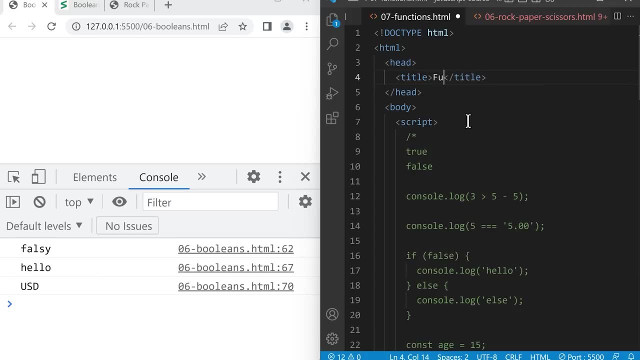 And we'll hide our files and prepare this file for this lesson. So at the top we'll change the title to functions and we'll remove all the code in the script element And let's save And we'll open this file in live server by right-clicking open with live server. 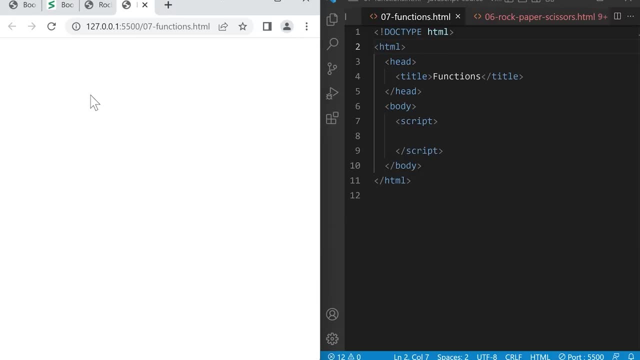 and we're going to open the console as well. So right-click inspect and then click the console, And finally we can close the previous tabs as well as the previous code. Okay, now we're ready to learn functions. First of all, what is a function? 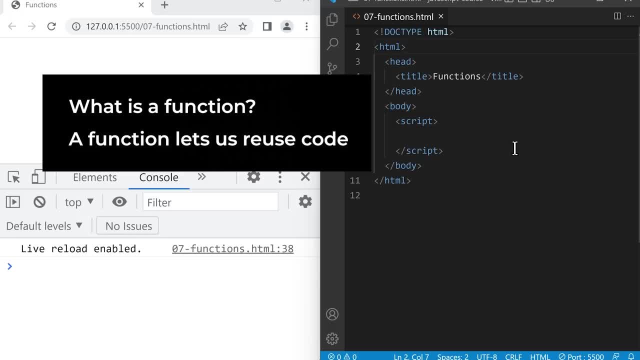 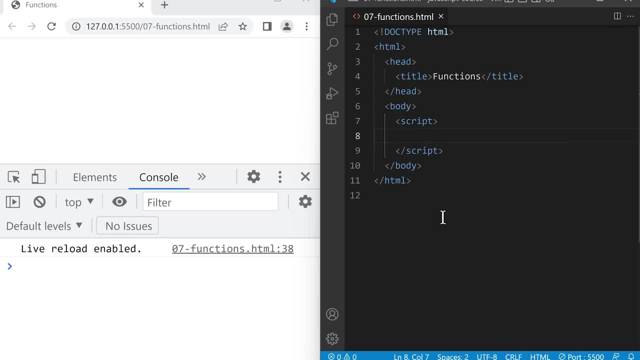 A function lets us reuse code. Let's create our first function. We're going to go to the script element and type the word function and space. So this creates a new function, And then we're going to give a name to our function. 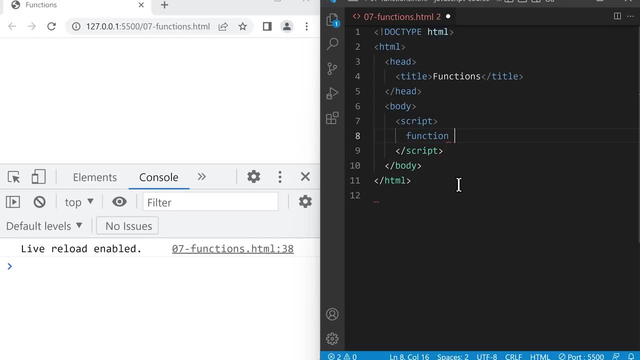 We can name it almost anything we want, but for now let's just name it function one. And then we're going to type round brackets and curly brackets. Then, inside these curly brackets, we're going to create a new line and we're going to type: 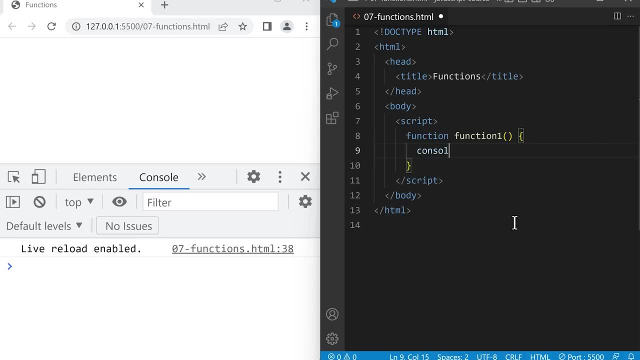 some code. So console dot log And the string hello, And we'll also type console dot log, two plus two And save. So this creates a function. Now let's learn how to use this function. We're going to type at the bottom the function name. 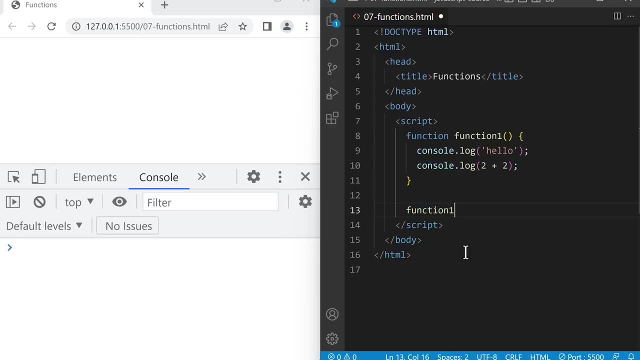 So function One And then open bracket, close bracket and semicolon. When we type the function name with brackets, this will run the code inside the function. If we save, notice that it runs the code inside the function and displays the two lines in. 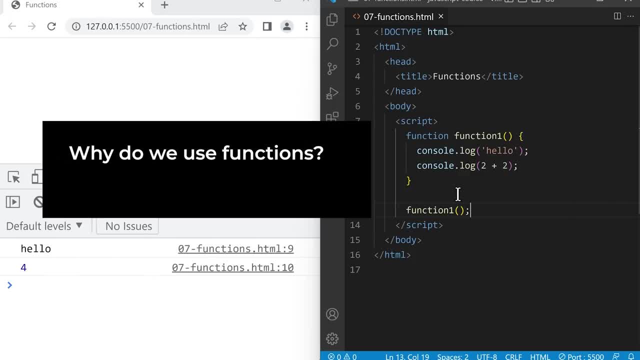 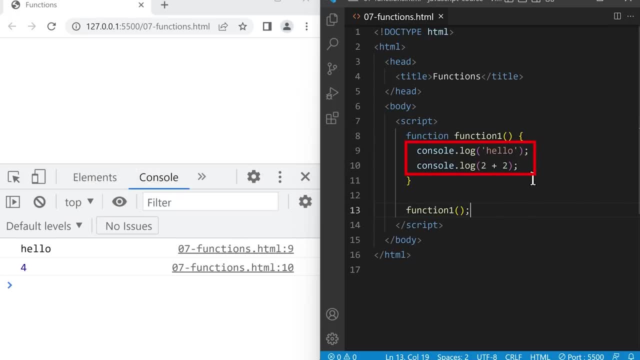 the console. So why do we use functions? A function lets us reuse code. So if we wanted to run both these lines of code again, all we have to do is type the function name again with brackets. So function one and brackets again. 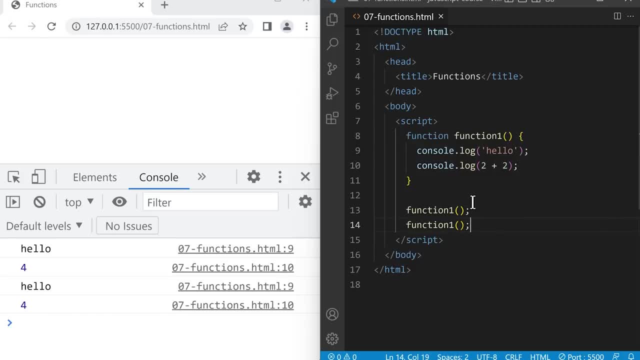 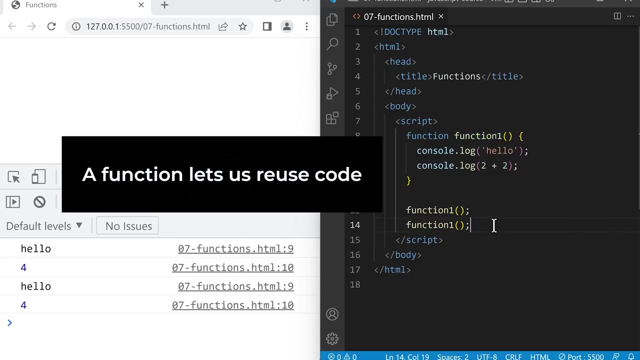 If we save this, will run the code inside the function two times And we can reuse this code as many times as we want by typing the function name with brackets. So that's what a function is. It lets us reuse code. Now let's learn the syntax rules for functions. 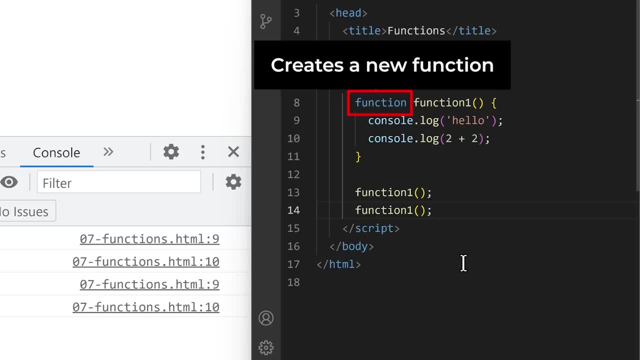 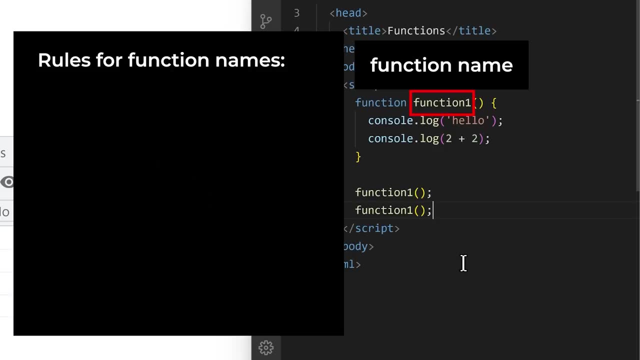 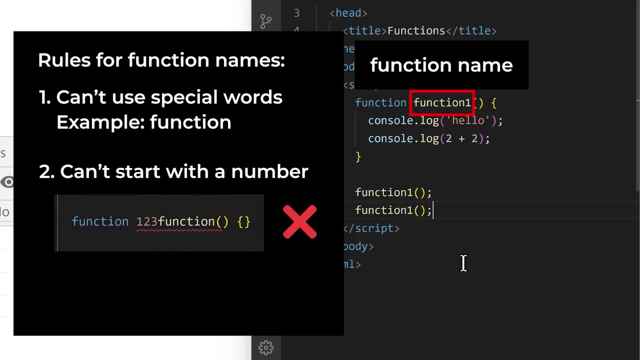 The word function creates a new function, And then we choose a name for our function. The rules for function names are the same as variable names. We can't use special words like function. We can't start with a number And we can't start with a number. 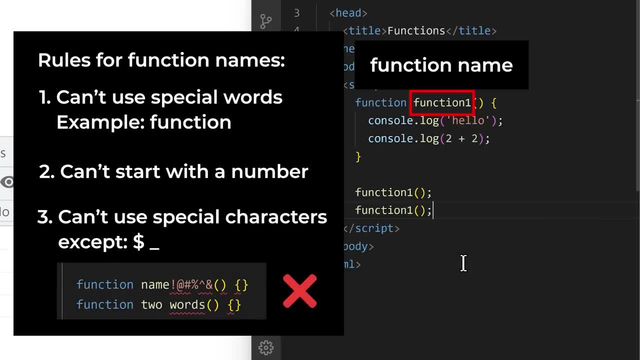 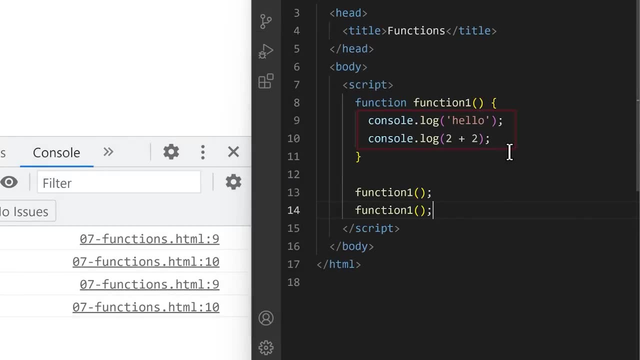 And we can't use special characters, Although dollar sign and underscore are allowed, And just like variable names, the best practice is to use camel case for function names, And inside these curly brackets we put the code that we want to run when we use the function. 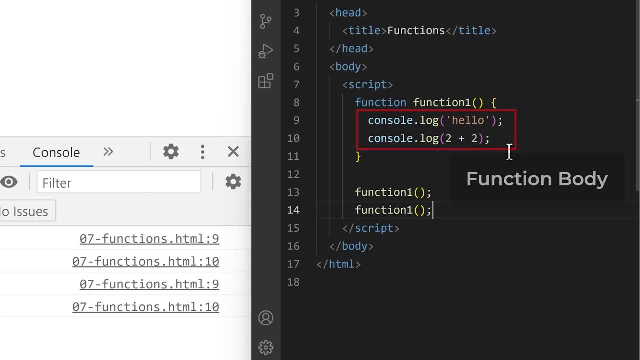 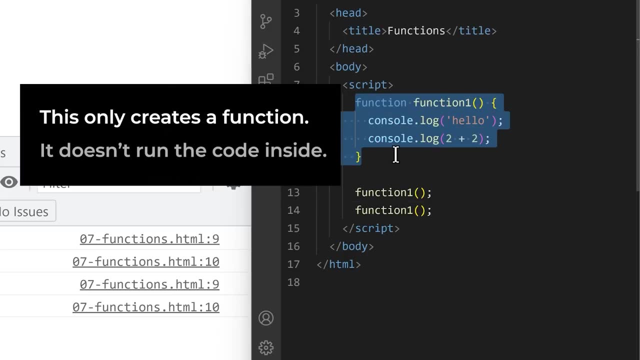 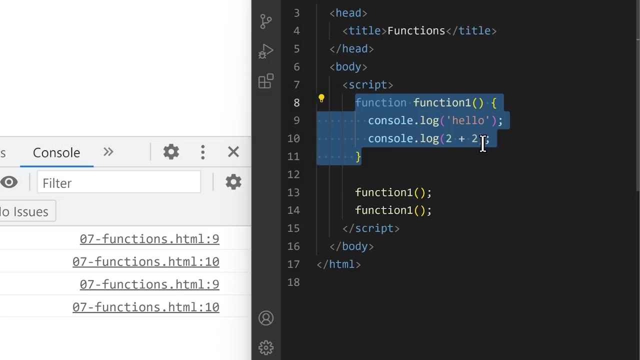 This is called the function body. Now, one very important thing to remember is that this code only creates a function. It doesn't run the code in the function or do anything else. In order to actually run the code, we have to use the function like below: 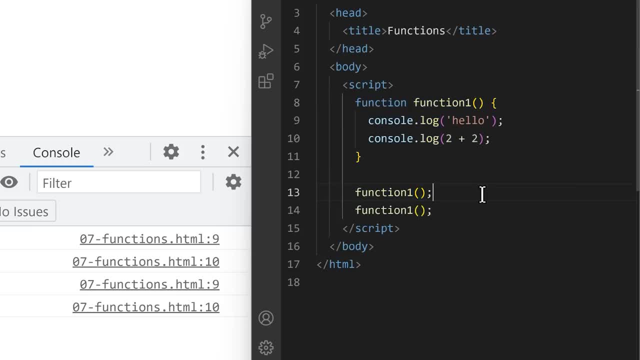 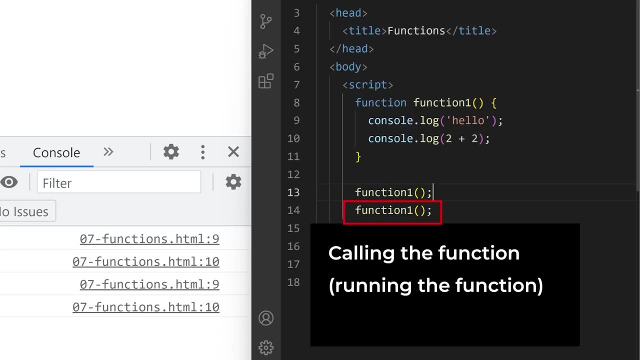 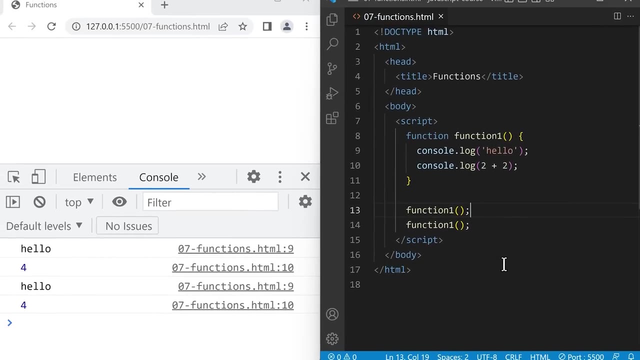 By typing the function name with brackets. This is known as calling the function. It's also known as running the function or executing the function. Now that we learned the syntax rules for functions, let's do a practical example. We're going to use functions to improve the code of our rock paper scissors project. 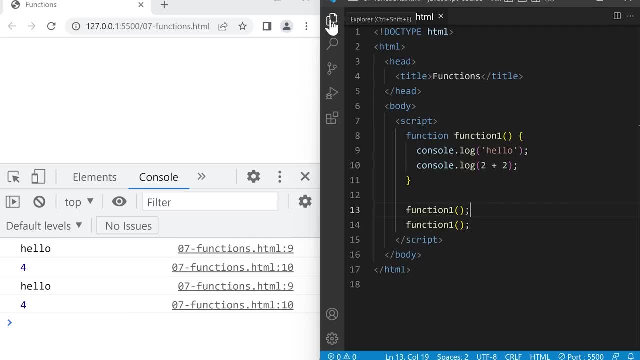 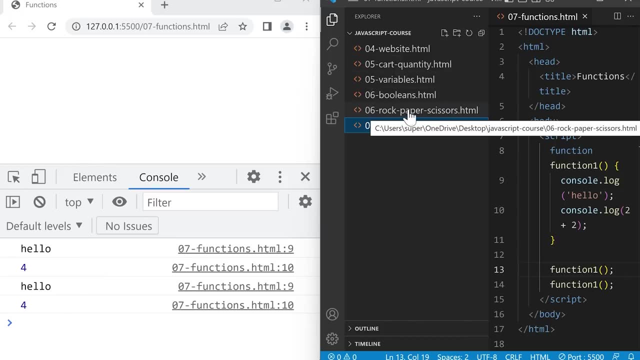 First let's click here to show our files, And we're actually going to make a copy of the project just for this lesson. So we're going to right click this file, Copy, And then, at the bottom, right click and paste. 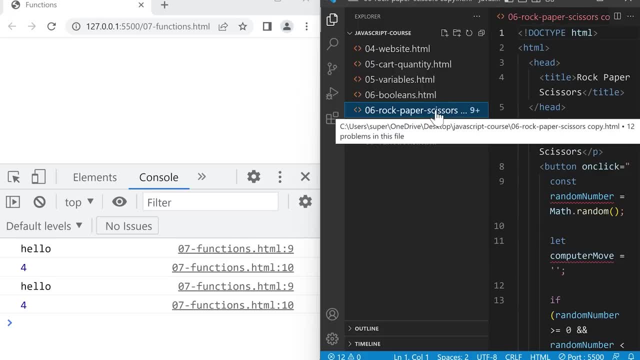 And we're going to rename this file. So right click Rename, Remove copy at the end And then at the beginning we'll change this to 07.. And press enter. Next, we're going to open this file in live server. 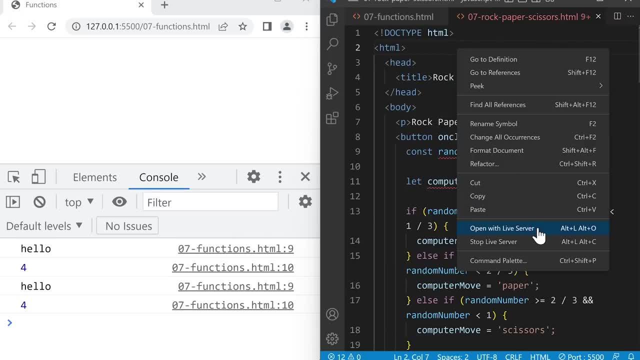 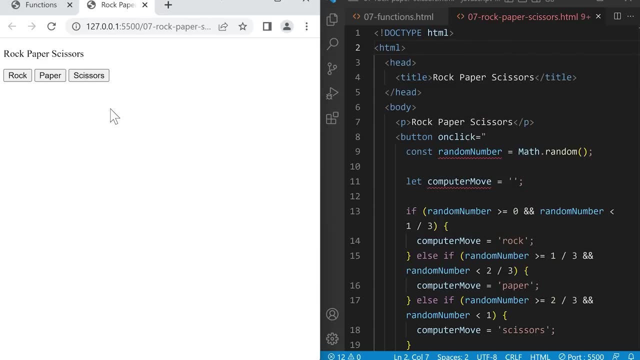 By right clicking And then open with live server And let's also open the console on this page. We'll right click Inspect And then click the console. Alright, Now if we look at the code for generating a computer move. 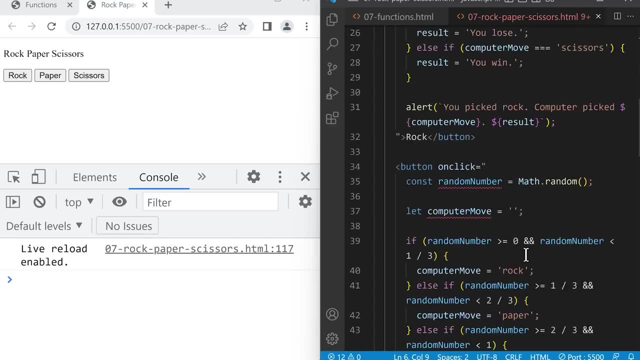 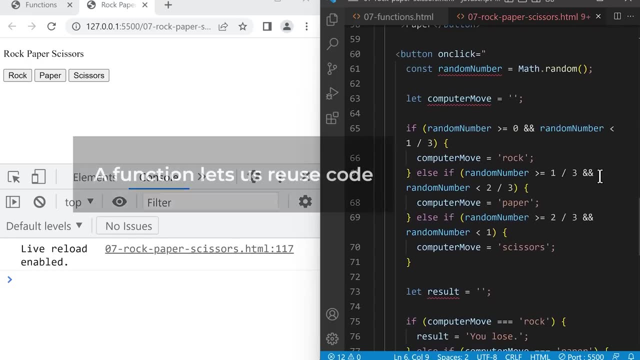 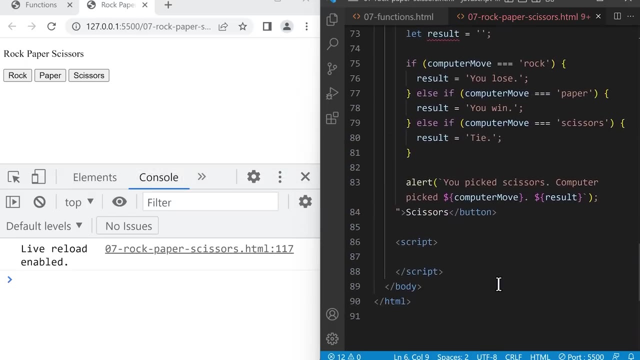 you'll notice that this code is the same for all three buttons. So this is a perfect situation to use a function, Because a function lets us reuse code. So let's scroll down to the script element And we're going to make a function here. 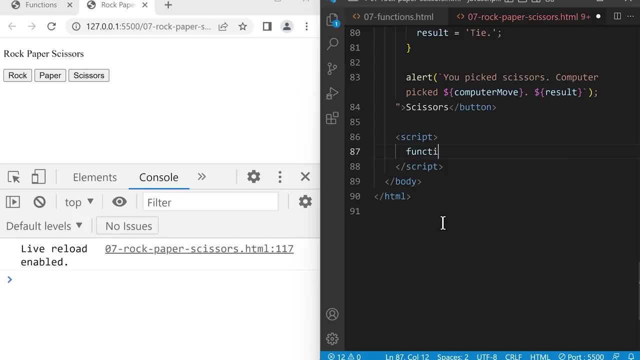 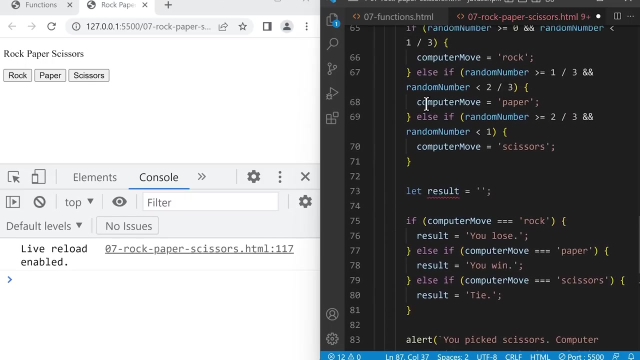 So let's type function and then a function name. Let's name this function pick, computer move, And then brackets and curly brackets. So one recommendation for function names is to use a verb or an action in the name, Such as pick. So next we're going to move all the code for picking a computer move into our new function. 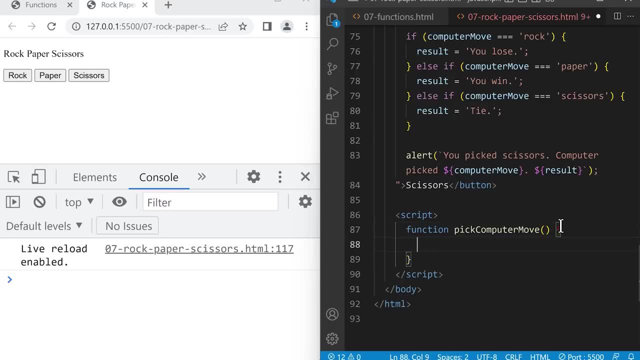 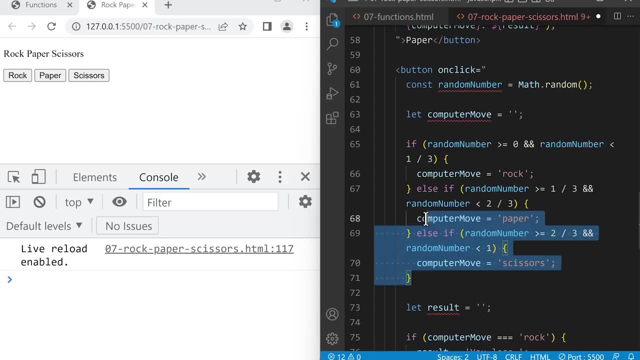 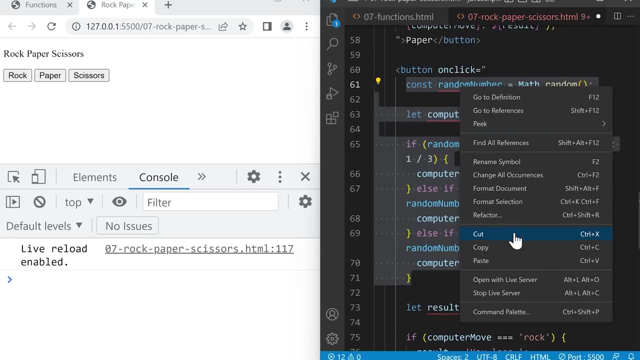 So let's create a new line here And we'll scroll up to the scissors button because it's the closest one, And we'll select all of this code for picking a computer, move And then right click, Cut And inside the function. 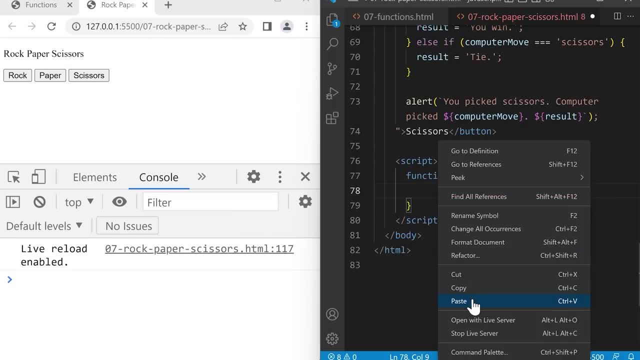 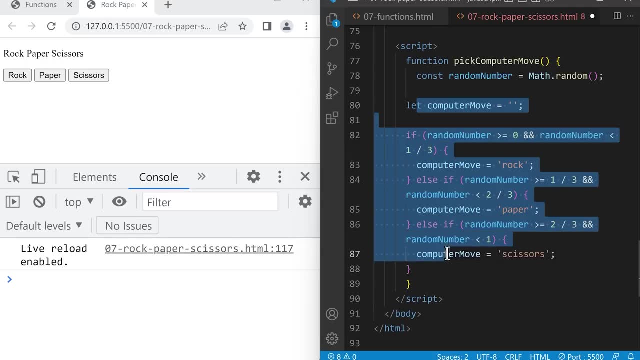 Right click And paste. If we need to fix the formatting, we can select these lines and press tab to add indents. So the reason we created this function is because remember that the script element runs when the page is loaded, So we want to make sure that we create the function first. 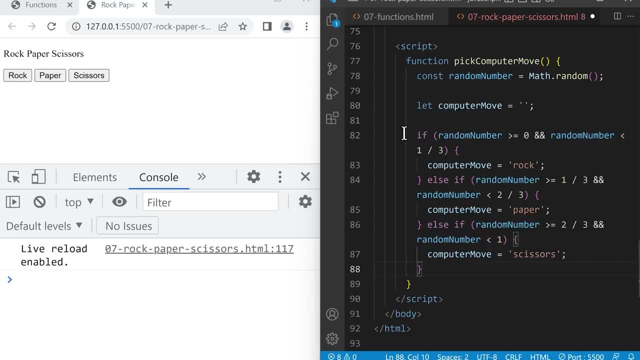 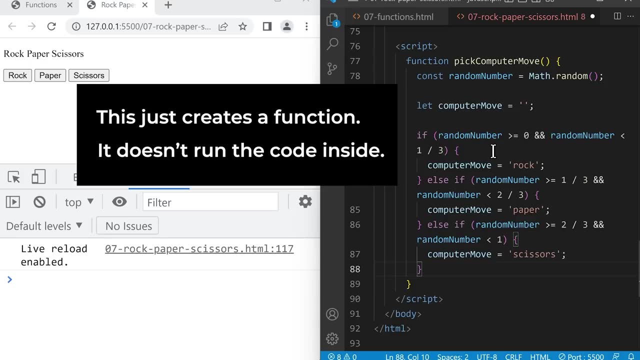 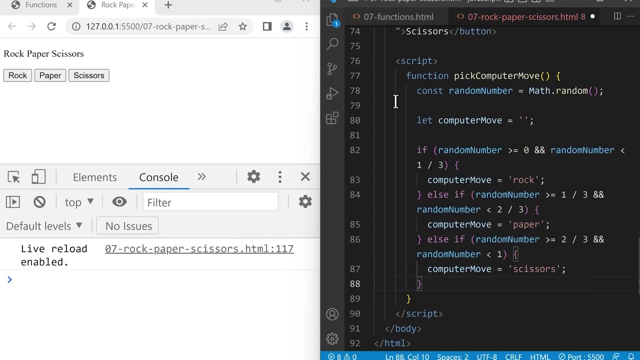 And then we use it in the buttons after Now. remember: this code just creates a function. It doesn't actually run the code inside. To run the code inside, we're going to call this function. So let's scroll up to the scissors button. 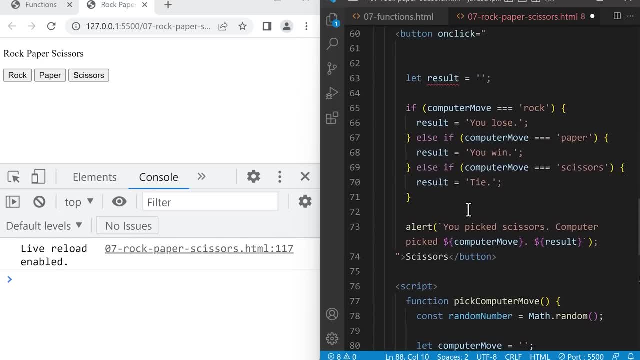 And we're going to call this function by typing the function name: pick computer move, open bracket, close bracket and semicolon. If we save and then click the scissors button, Unfortunately it now gives us an error saying computer move is not defined. Now this might seem weird. 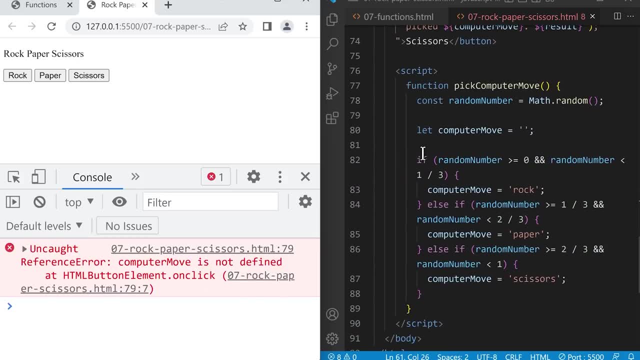 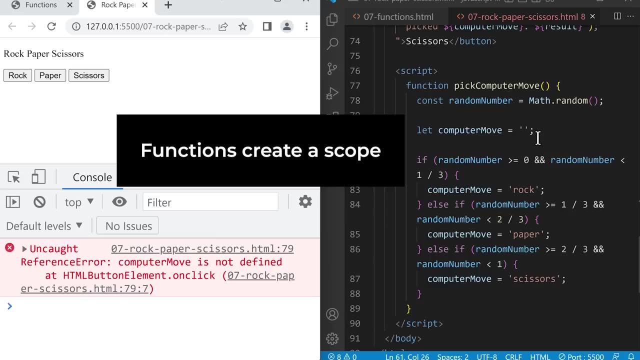 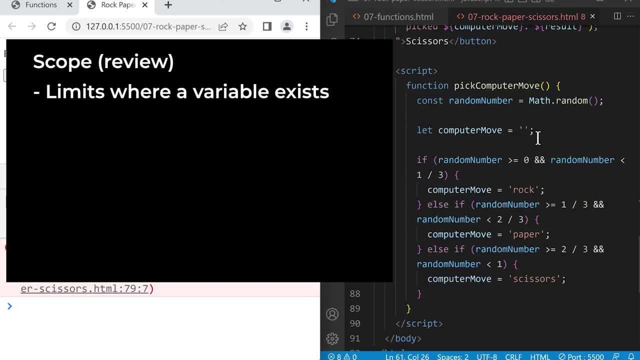 Because down here we actually create the computer move. So what's going on? The reason this happens is because functions create a scope. In the previous lesson we learned about scopes, which limit where a variable exists. We learned about if statements and that if statements create a scope. 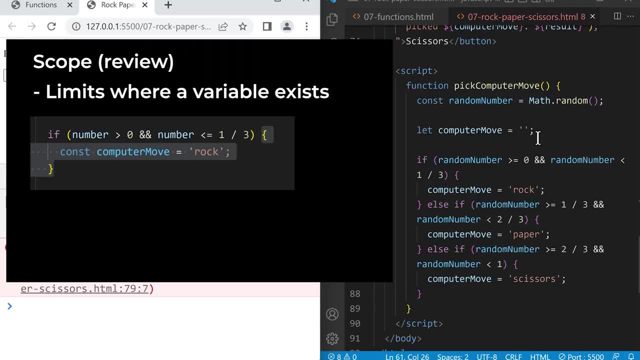 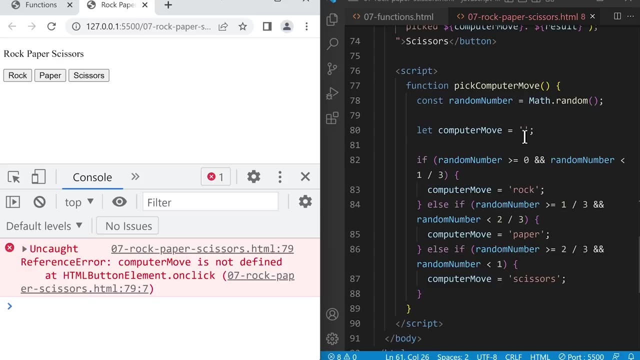 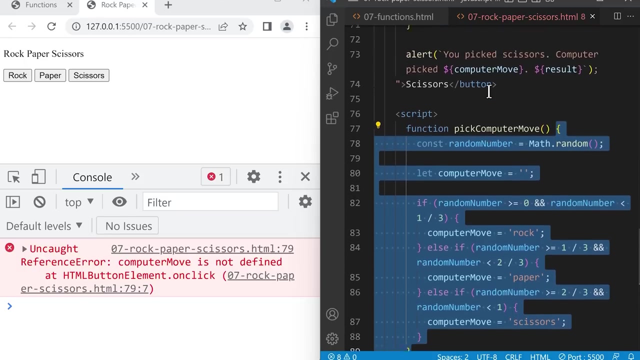 between the curly brackets. This means that any variable created between the curly brackets only exists between the curly brackets. Functions also create a scope. Any variable that is created between these curly brackets only exists inside the curly brackets And we can't use it outside the curly brackets. 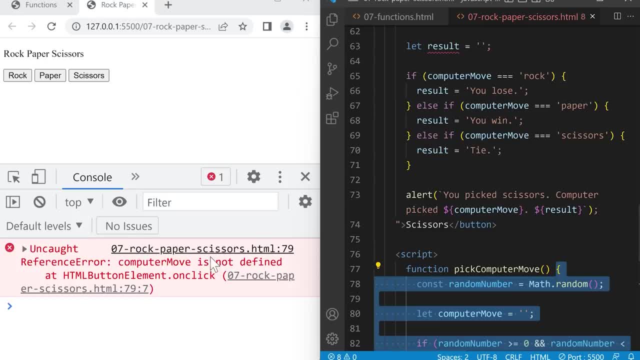 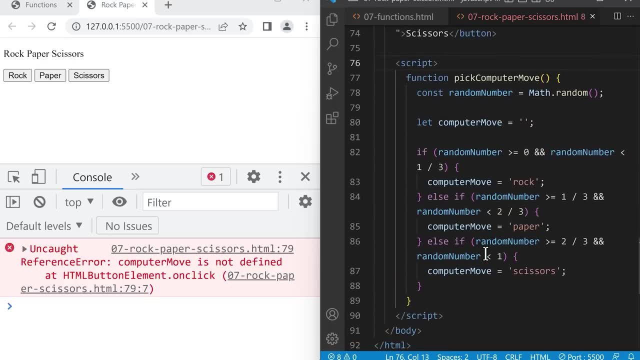 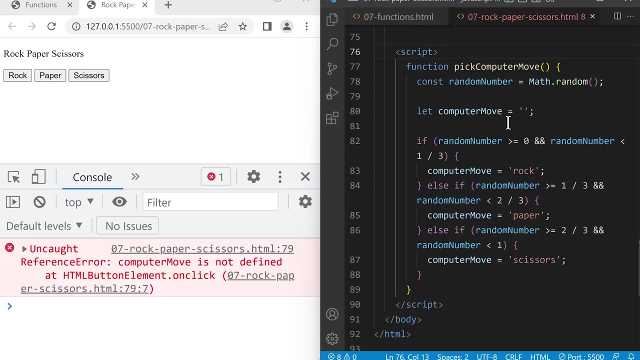 like we do here. So that's why we're getting this error. So how do we solve this problem? Remember that with if statements, we solve this by creating the variable outside of the if statement. like this, We can use a similar solution with functions. 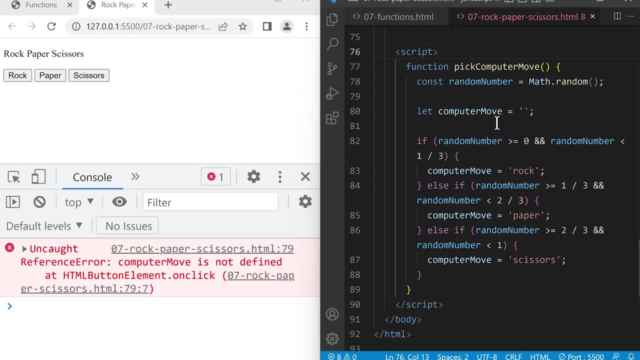 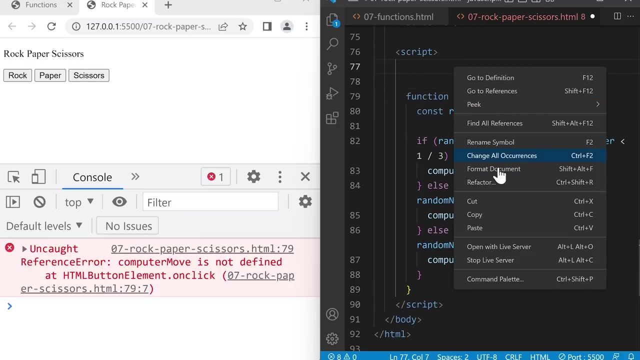 To make this variable exist outside the function, we just have to create it outside the function. So let's select this code: We're going to right-click and cut and remove these lines And then, outside the function, we're going to right-click and paste. 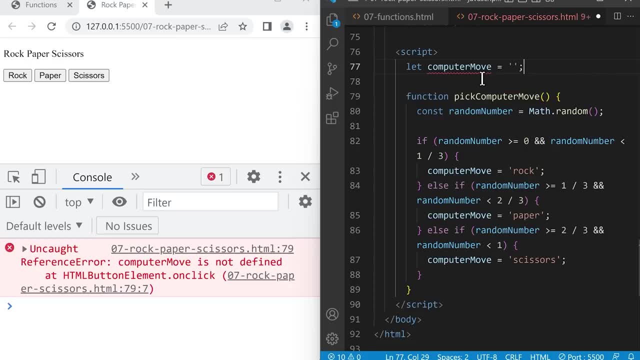 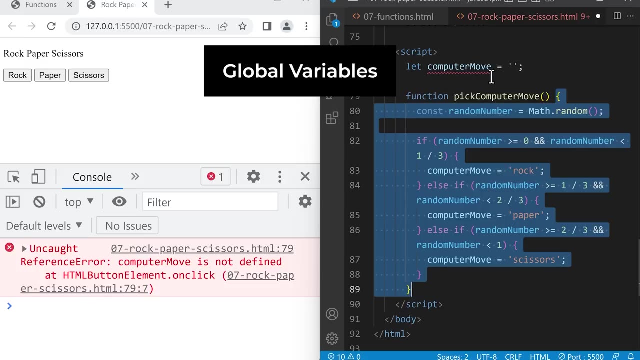 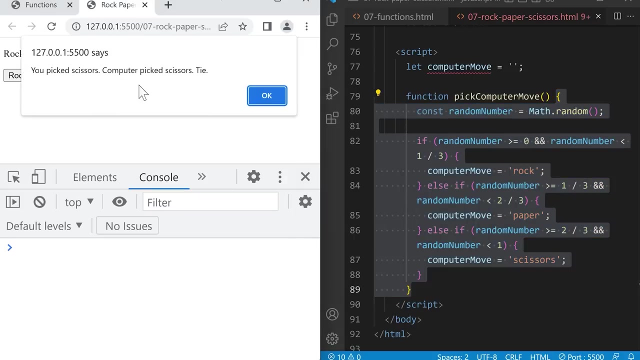 So now this variable is no longer inside the function's scope And it can be used anywhere else in the code. So variables like this that can be accessed anywhere are called global variables. If we save and now click the scissors button, everything is working again. 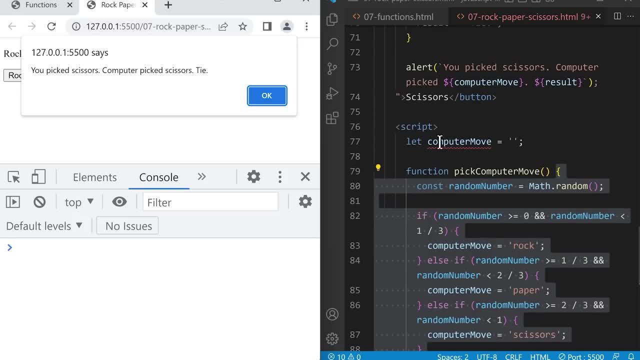 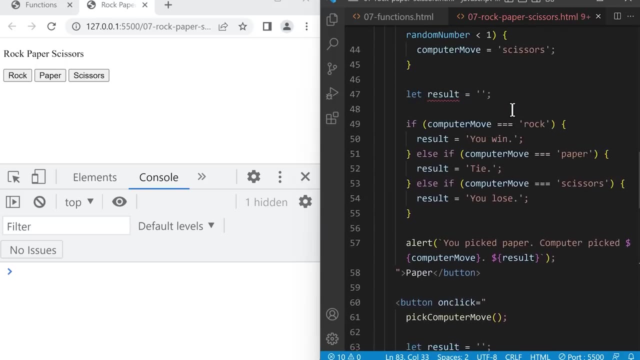 Because this code above can now access this variable. Now let's press OK And let's use this function to reuse this code, So we'll scroll up to the paper button And now, instead of all this code again, we're just going to remove it. 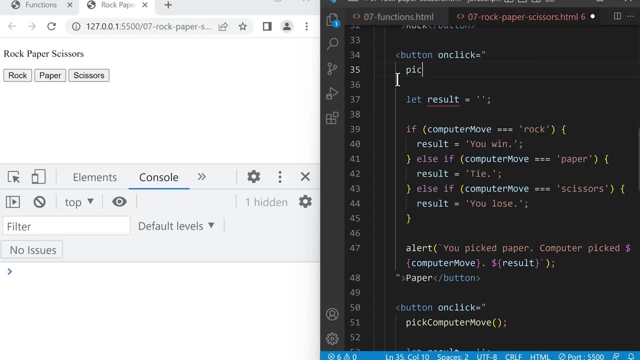 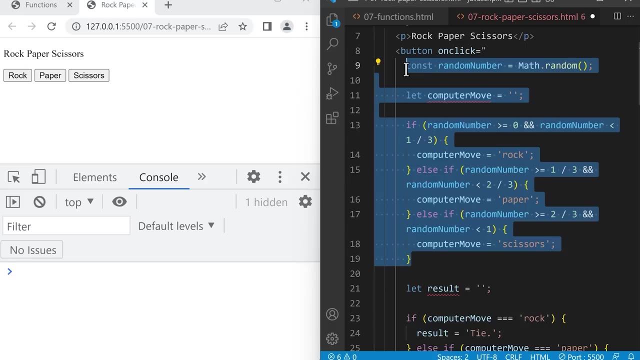 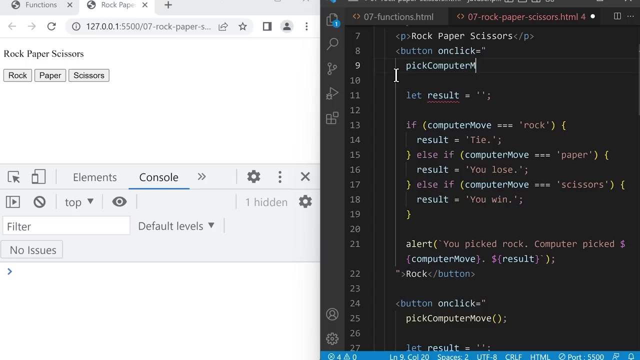 and call the function pick- computer move- open bracket, close bracket, semicolon, and also with the rock button We'll select all this code and remove it and just call the function pick- computer move brackets and semicolon. Now, if we save and click the rock button, 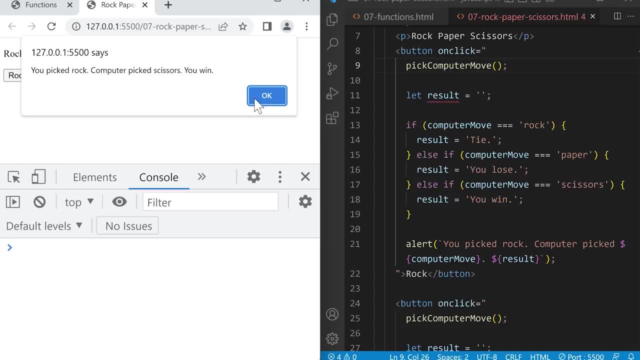 it works just like before. We'll press OK and click the paper button. It also works just like before. So, as you can see, functions, let us reuse code, And they make our code a lot cleaner by removing all the duplication that we had. 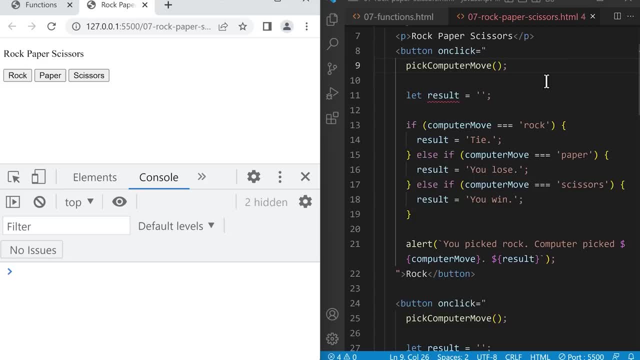 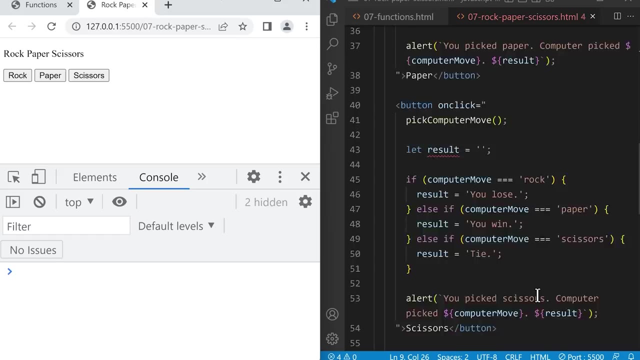 Another benefit of removing duplication is that before, if we ever wanted to update the code for picking a computer move, we had to update it in three places in each of the buttons, But now, if we scroll down, we only have to update it in one place. 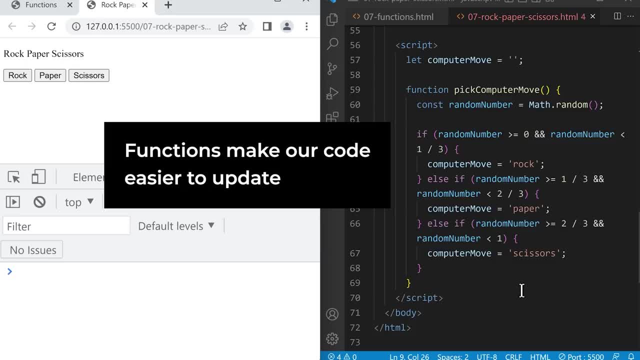 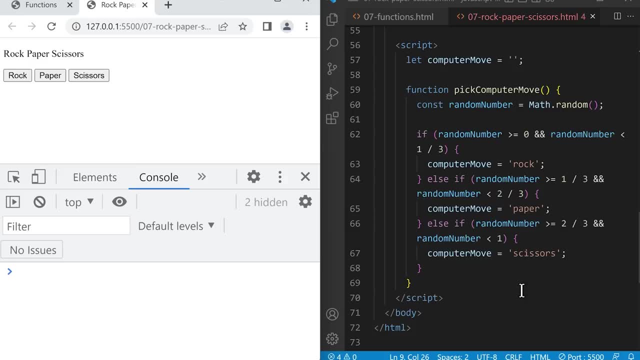 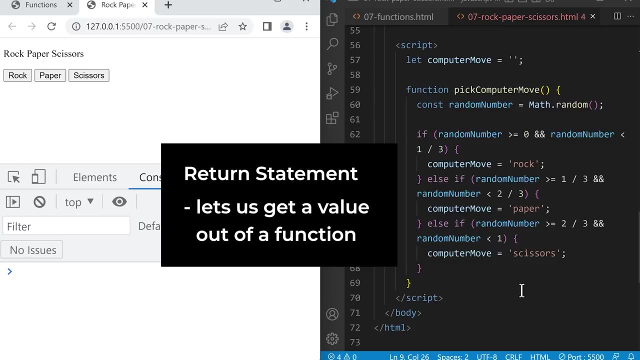 inside this function. So functions also make our code easier to update in the future. Next, we're going to learn a feature of functions called a return statement. A return statement lets us get a value out of a function. So at the end of this function, 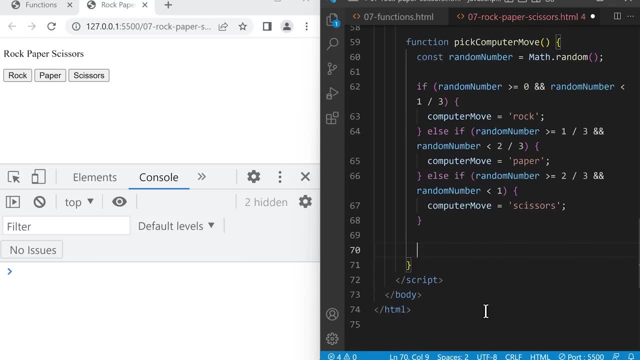 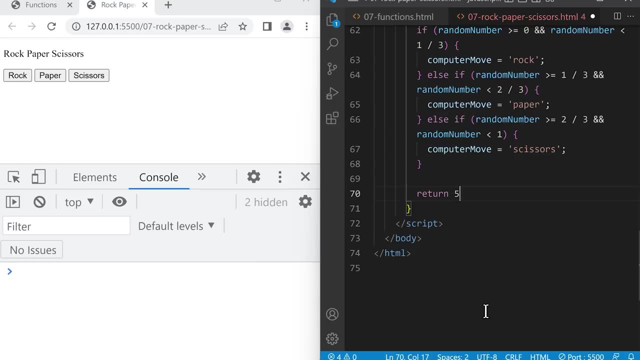 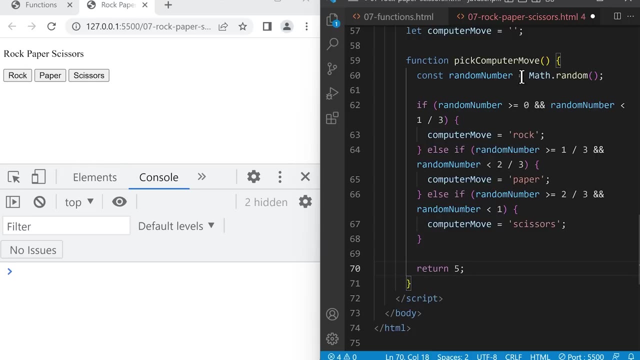 let's type some new lines And we're going to type return and then a value like the number 5 and semicolon. Now, whenever we call this function, it will result in a value: the number 5.. So up here, 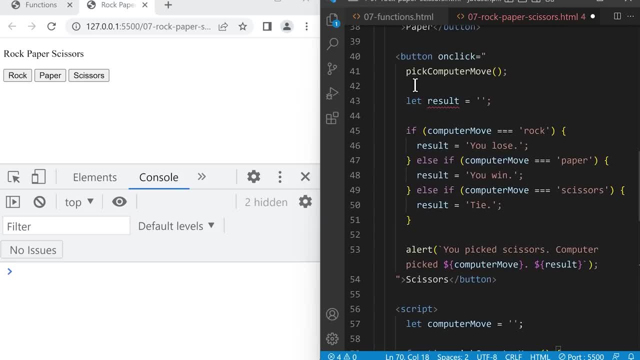 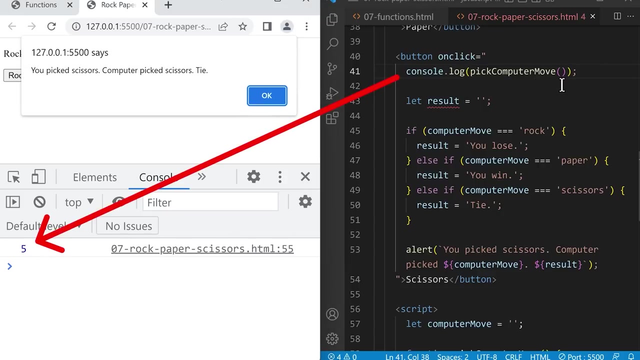 when we call this function, this will result in the number 5.. So we can actually consolelog this consolelog And then save and click the scissors button And it will show us that calling the function now results in the number 5.. 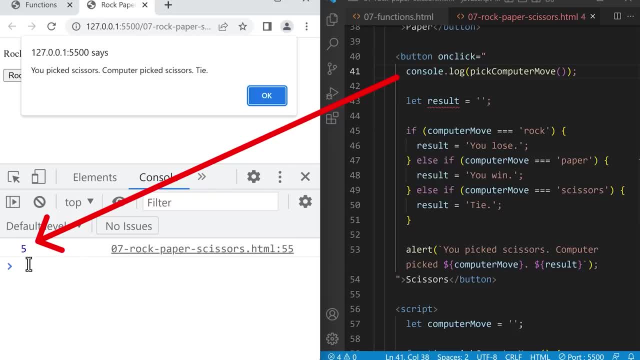 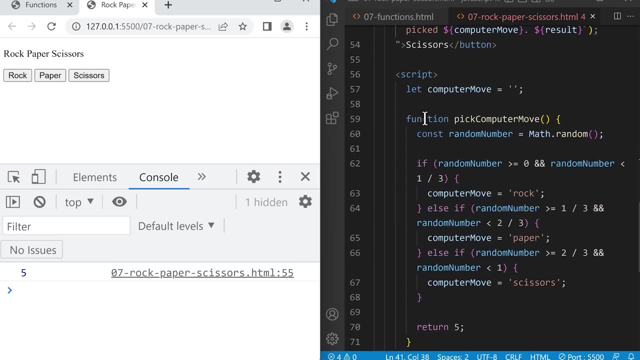 And we display it in the console. So that's how a return statement works. It lets us get a value out of this function. Let's press OK and do another example. We'll scroll down and this time let's change this value to the string rock. 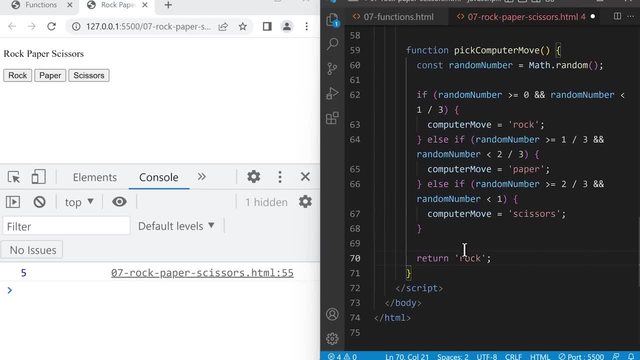 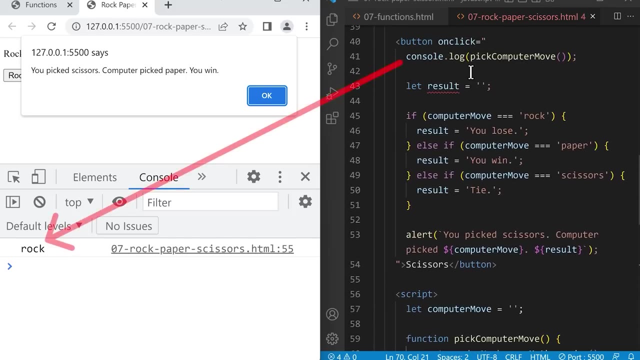 Now, whenever we call this function, it will result in the string rock. If we save and then click scissors and scroll up here, calling this function now results in the string rock And then we display it in the console. So now let's press OK. 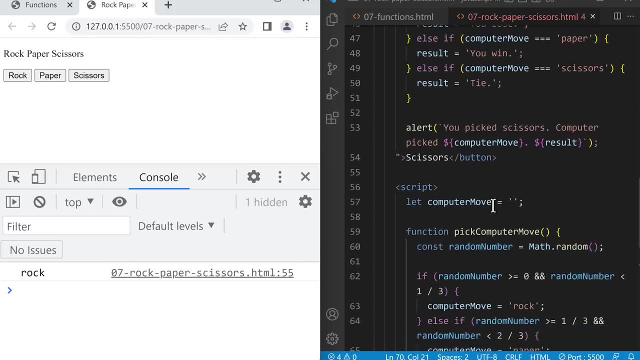 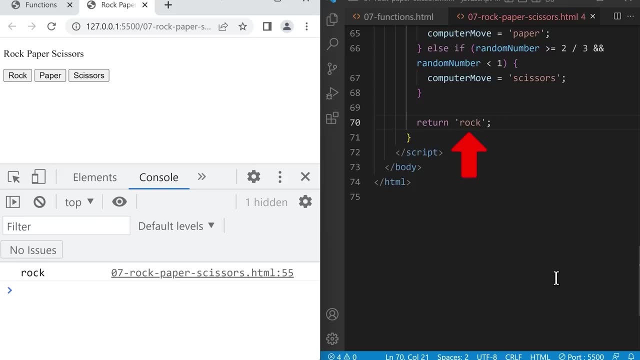 and we'll learn the syntax rules for a return statement. So we just have to type the word return and then a value, And it will get this value out of the function. Now, instead of just a value, we can also return a calculation or a variable. 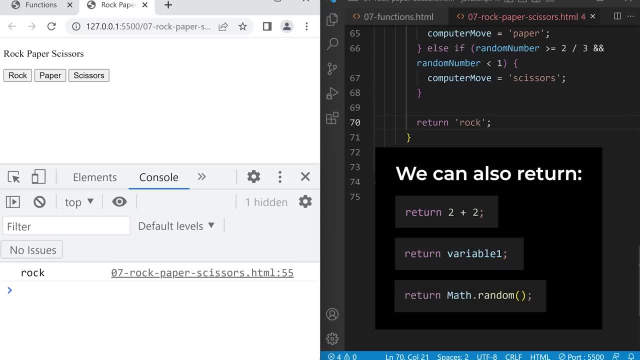 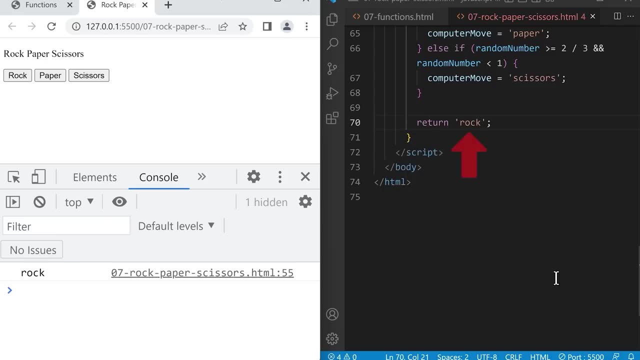 or anything that results in a value. So this is known as returning a value from a function, And this value is known as the return value. We also don't have to return anything from a function If a function doesn't have a return statement. 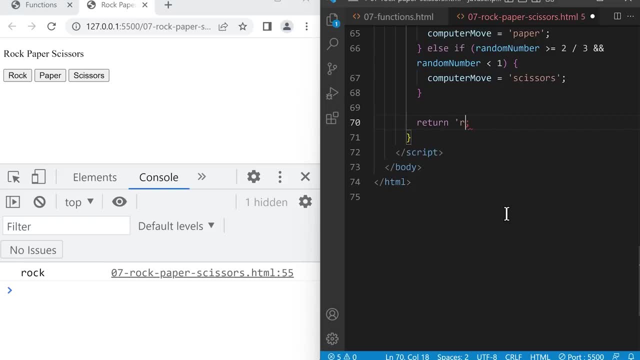 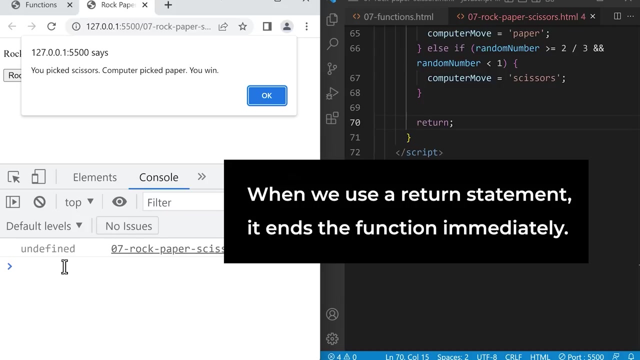 or we return without a value, like this, this will return the value undefined. So if we save and then click scissors again, the function will return undefined. And lastly, when we use a return statement, it ends the function immediately. So after the return statement. 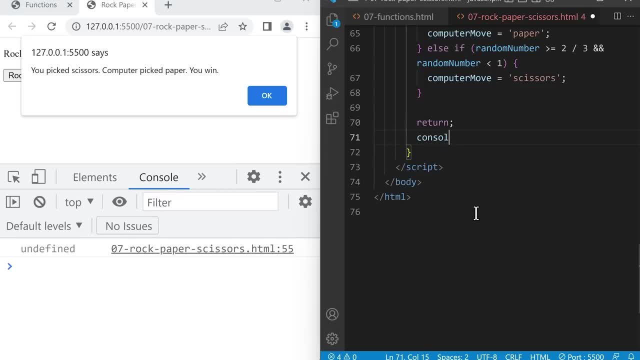 if we type consolelog the string after and press OK here and save this file and then click the scissors button, notice that it doesn't run this code And that's because once we return the code returns back to where we called the function. 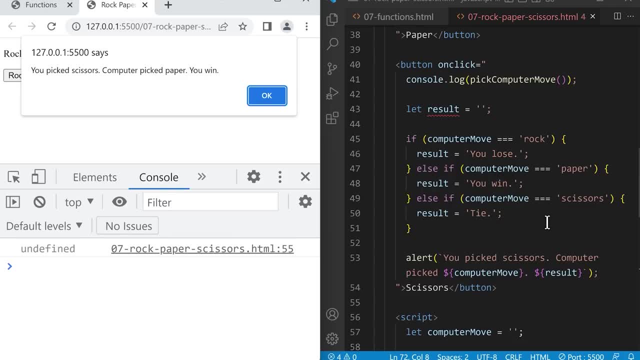 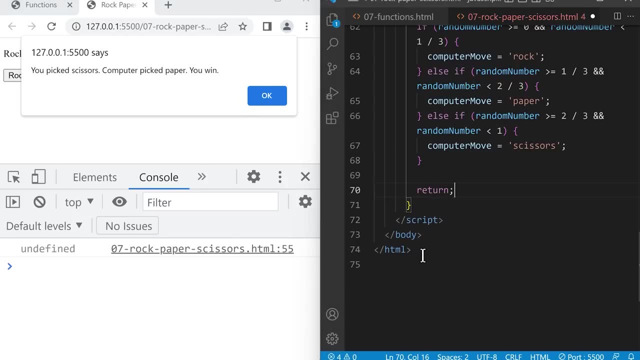 That's why it's called a return statement, So it's not going to run anything after the return, So we can remove this code and press OK. So now that we understand return statements, we're going to learn a better way of getting the computer move. 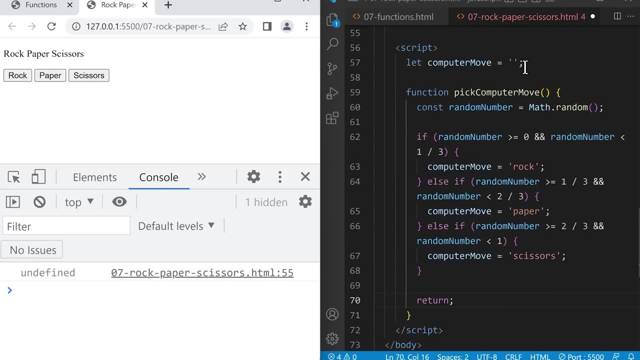 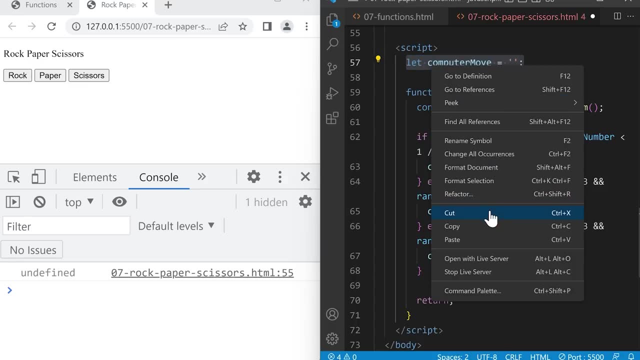 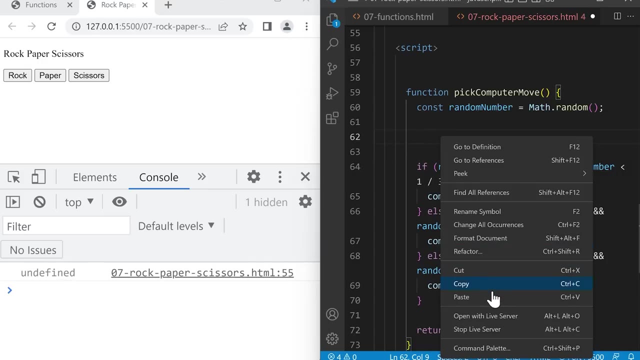 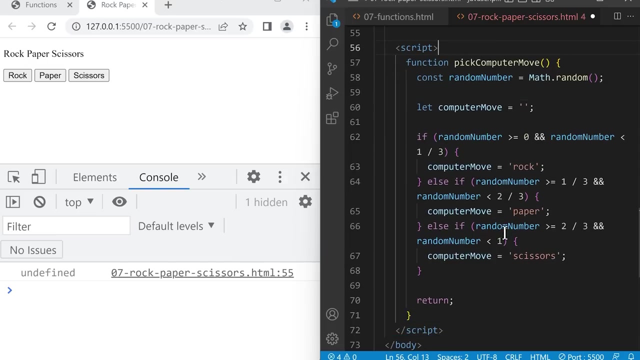 out of this function. So first let's actually move this variable back into the function, So we'll right click and cut, and then in here right click and paste and delete these lines. So now we're back to the original problem. How do we access? 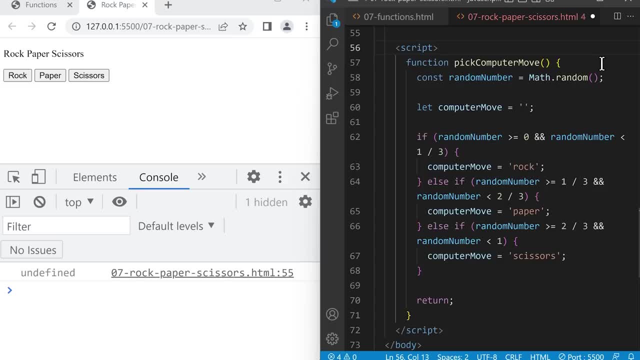 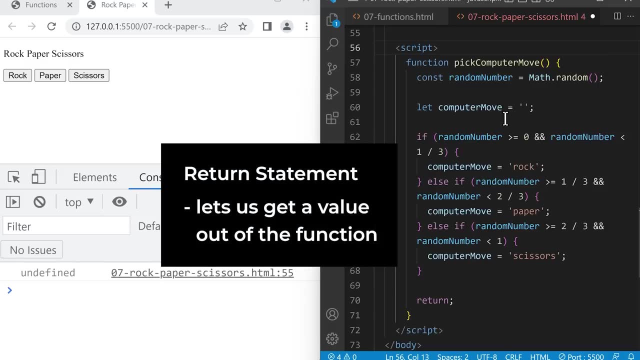 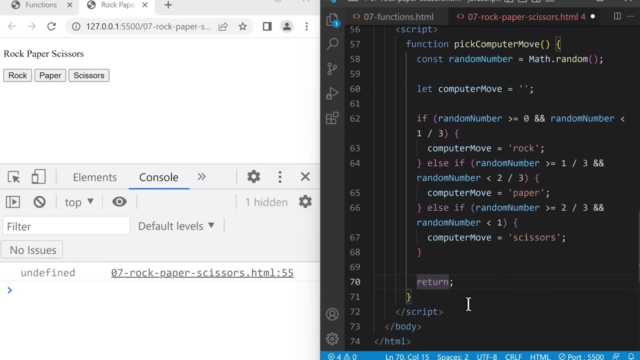 computer move outside of the function. So another solution is to return this variable Because, remember, a return statement lets us get a value out of the function. So down here we're going to return the computer move. So this will take whatever value. 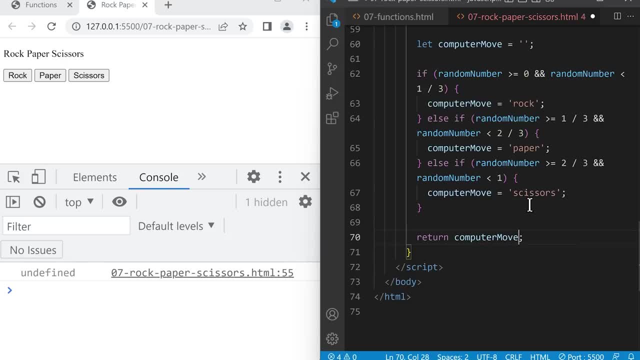 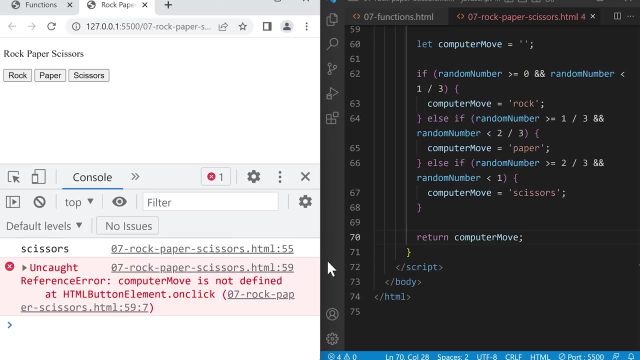 is saved inside computer move, which is one of these values, and return it out of the function. If we save and then click the scissors button, we were able to get the move scissors outside of this function. So what happened here is that we returned. 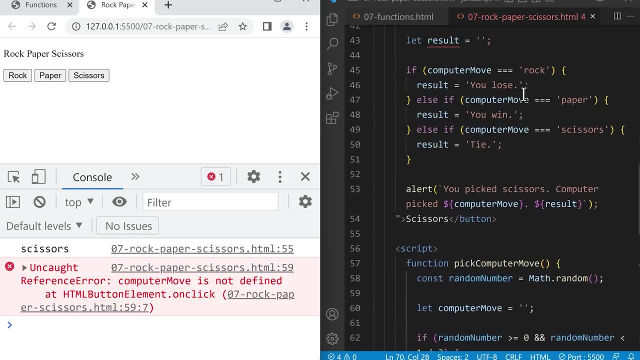 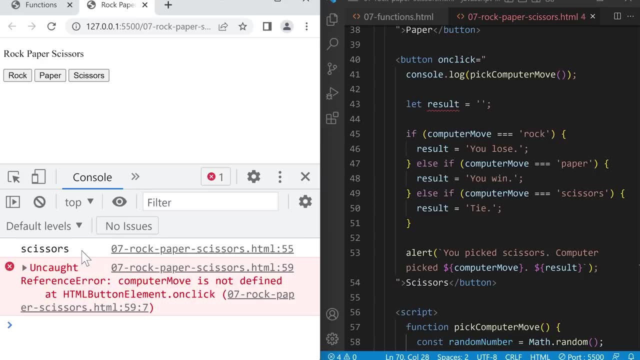 this move and then up here we took the move and displayed it in the console to get scissors. So that's another way of getting the computer move out of a function using the return statement. However, now we're back to this problem with computer move. 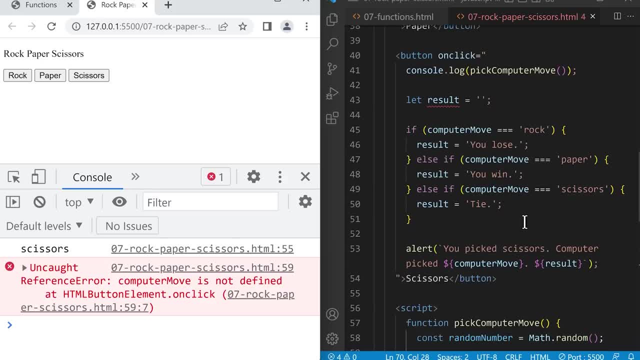 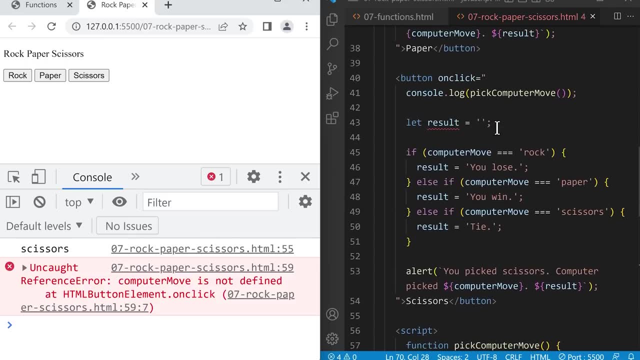 not being defined Because we moved it back into the function's scope. So let's scroll up and remember that this return value is just a value. We can use it like any other value. For example, we can consolelog it or we can also. 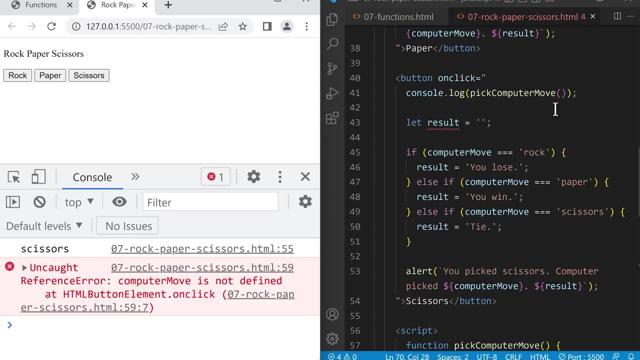 save this in a variable. So let's do that right now. We're going to remove this and create a new variable with const and let's just name this variable computer move to match what we used down here And we'll use equals to save. 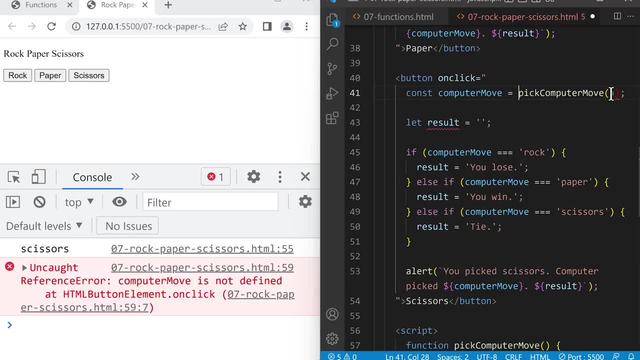 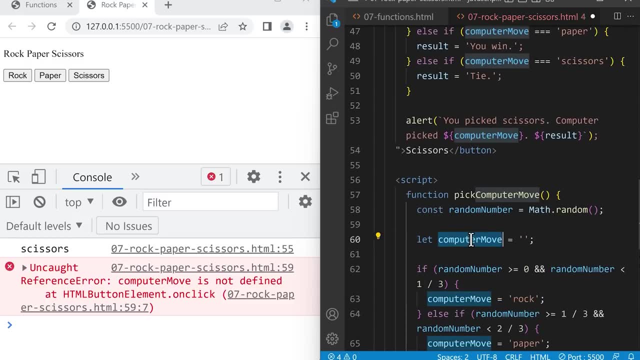 the return value inside this variable. So note that even though we use computer move here as well as here, there are different variables. This one is inside the function's scope, So it prevents it from conflicting with variables outside the function's scope. That's one of the 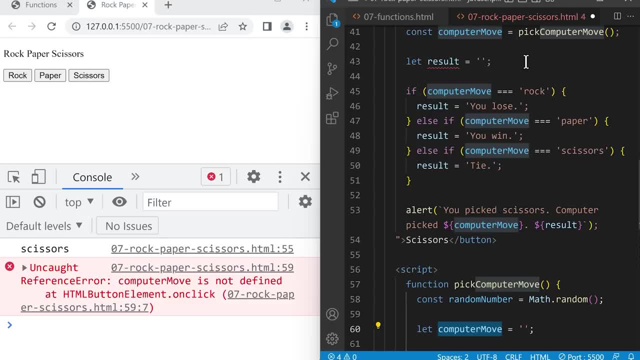 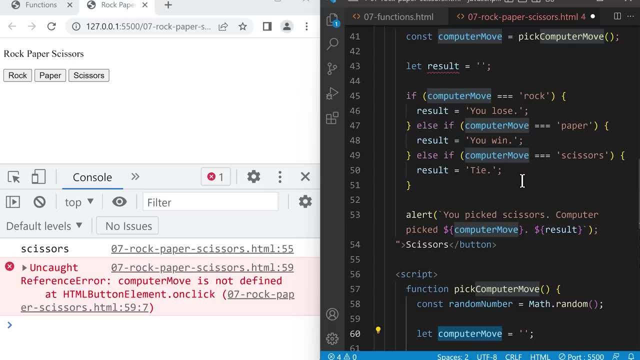 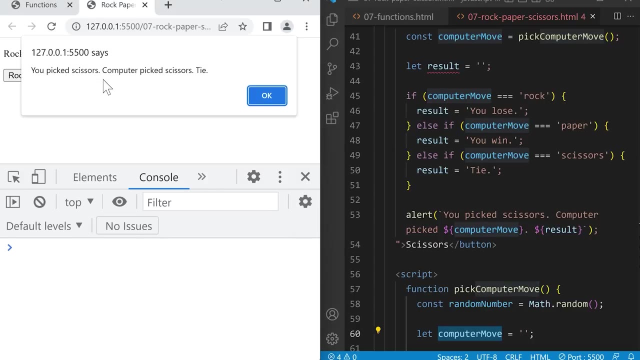 main benefits of scopes. So now that we saved the return value into this variable and we're using this variable here, the code should now work. If we save and click scissors, everything is back to normal And let's press OK. So don't. 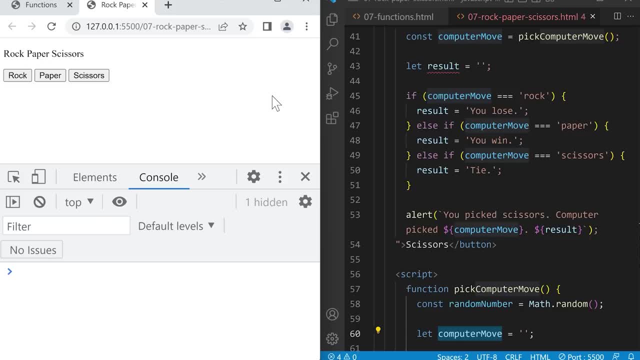 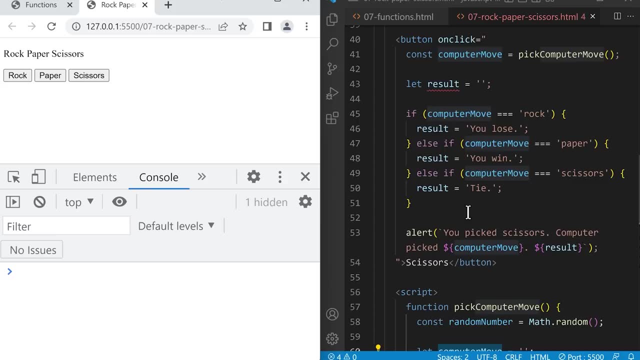 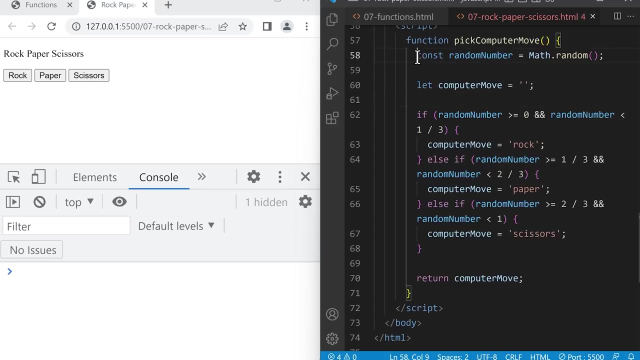 worry. functions can be a little confusing at first, because the code is no longer simply going from top to bottom. When we click this button, we're going to run this function, So the code is going to jump down here And then it's. 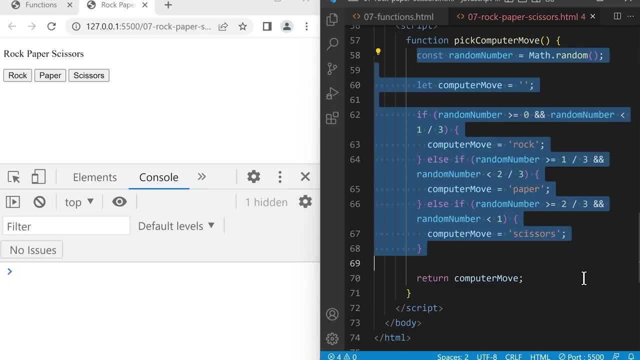 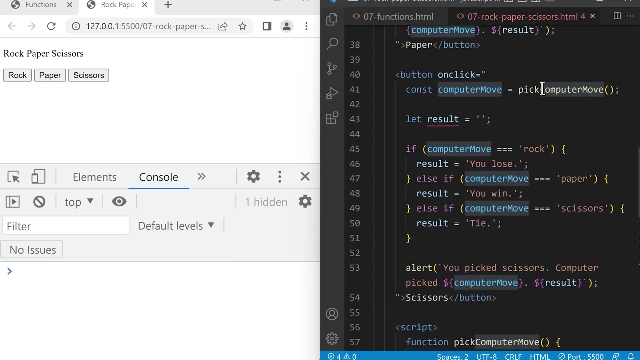 going to run all of this code from top to bottom. At the end we're going to return whatever is inside computer move, back to where we called this function. So we're going to return value into a new variable, computer move, And then use. 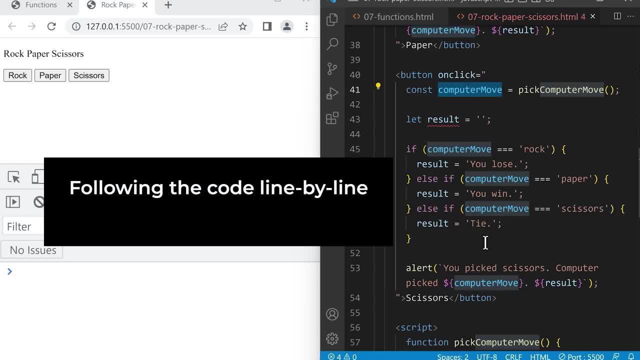 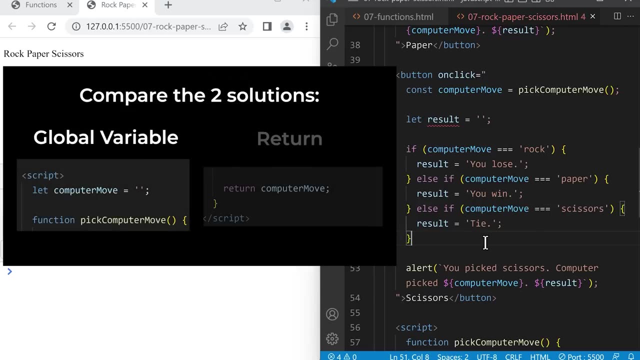 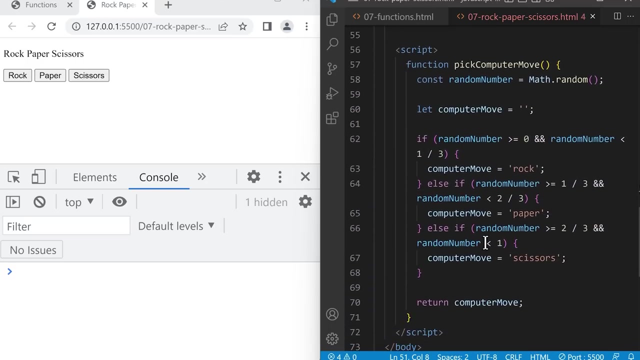 computer move down here. So following the code line by line like this is called tracing the code. It's a useful technique to understand exactly what the code is doing. Now let's compare the two functions. So returning a variable like this is actually preferred. 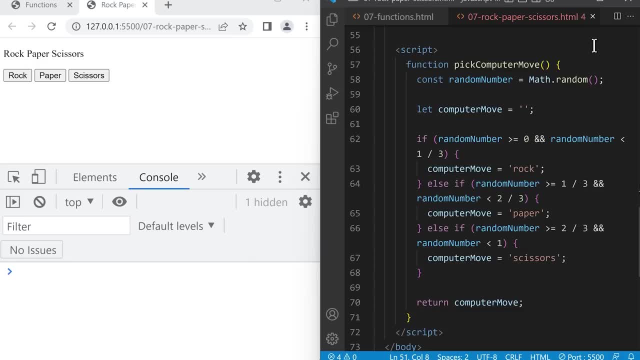 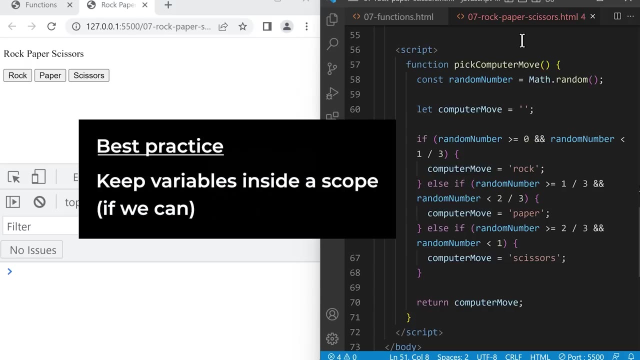 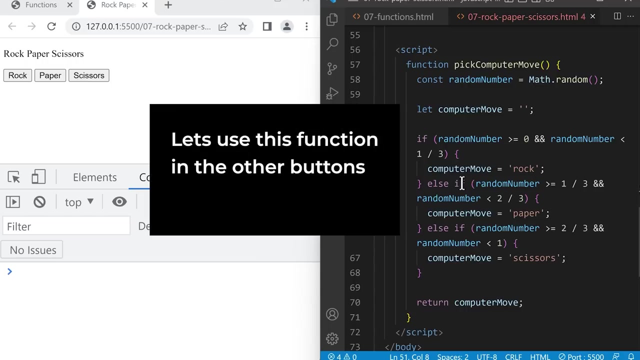 over using a global variable, And that's because a scope can help us prevent naming conflicts, So all the variables inside here will not conflict with anything outside the scope. So generally, it's a best practice to keep things in order and use this function in the. 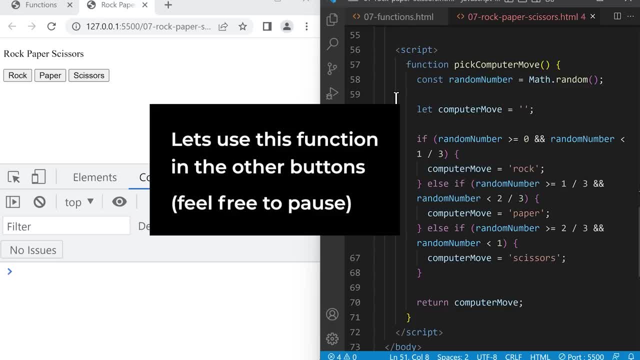 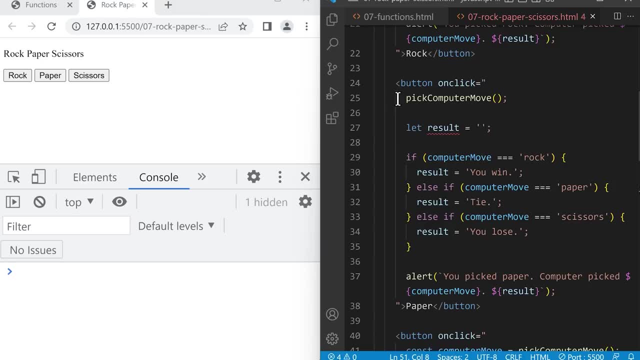 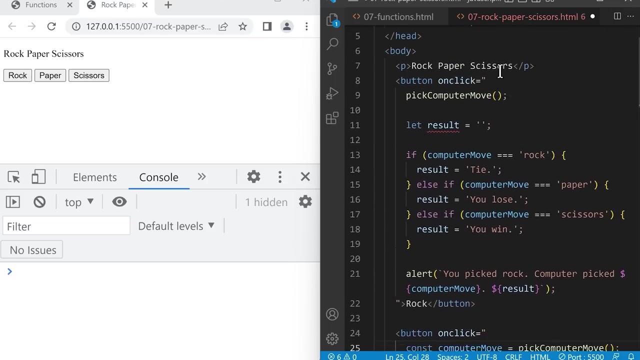 other buttons. Feel free to pause the video if you want to try it yourself first. So we'll scroll up to the paper button And then here we're going to save the returned computer, move into whatever is returned, Make it equal to whatever is. 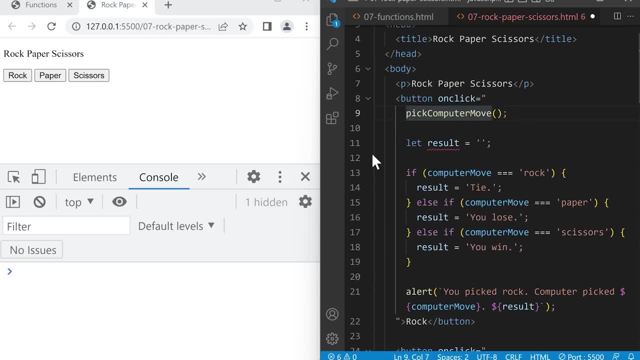 returned. And then same thing for the rock button. We're going to save the return value in a variable const. computer move equals. If we save and click the rock button, this also works And let's press OK. So that's how we. 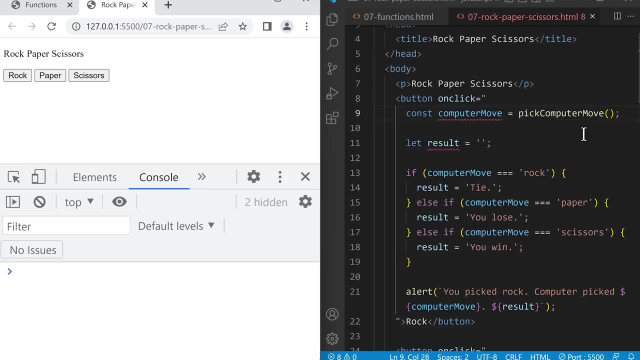 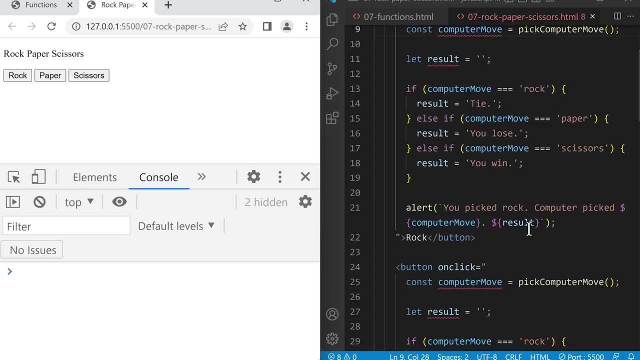 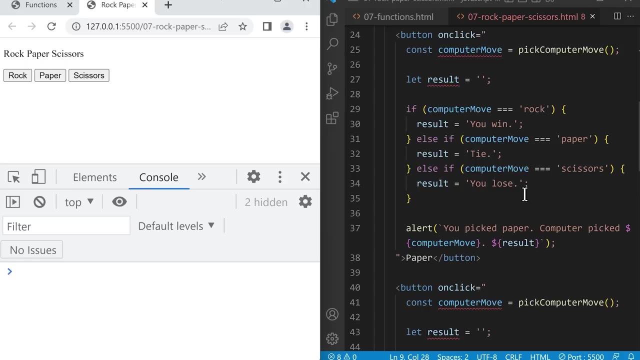 use a return statement to take advantage of the benefits of scope. Next, if we look at the rest of this code, where we compare our code with the message that we display, So we can actually use functions here as well to reuse code that. 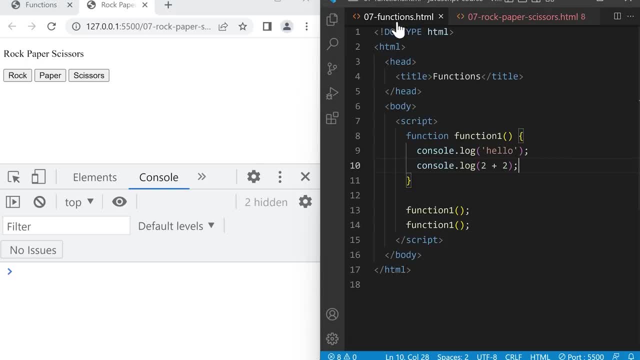 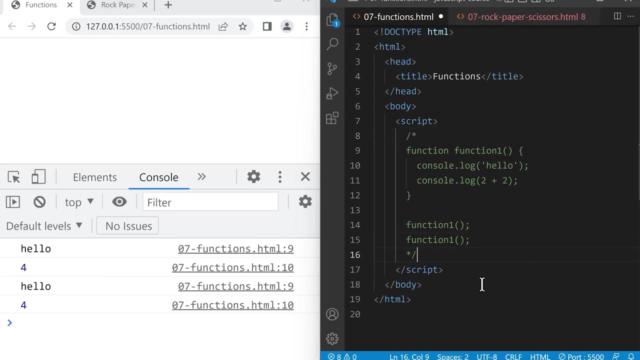 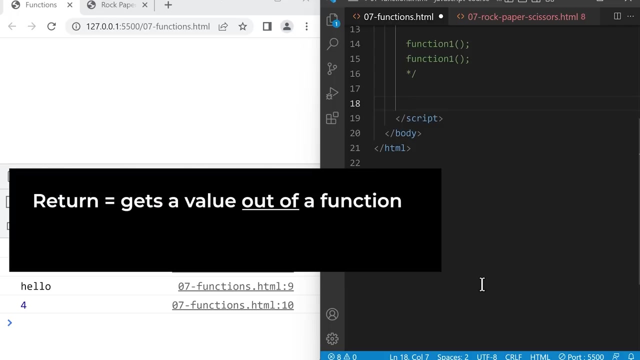 has small differences. To do this, we're going to need another feature of a function, which is a return statement. So let's do an example. Let's say that we have a function called return statement. So let's do an example. 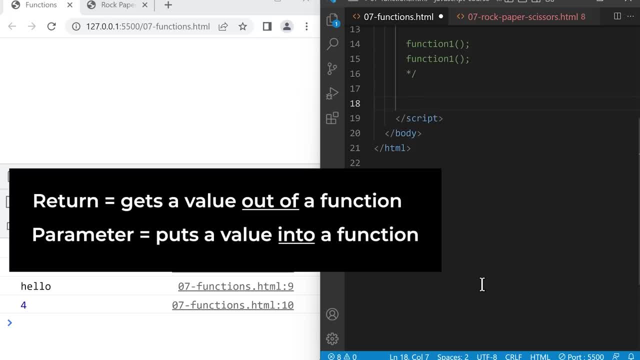 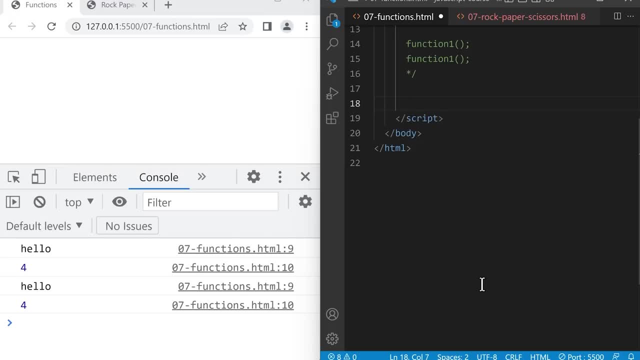 Let's say that we are working on the final Amazon project and we need to calculate the tax for our order. Let's create a function to calculate the tax, So function, let's name it: calculate tax brackets- 1,000 cents or. 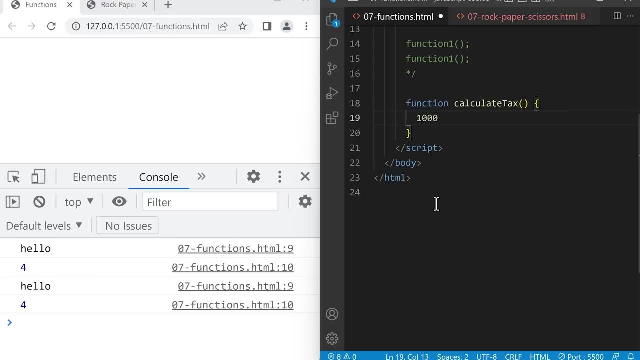 $10, and the tax is 10%. To calculate the tax, we can do 1,000 times 0.1,, which is 10%. Let's also display this number in the console, So at the bottom of the screen. 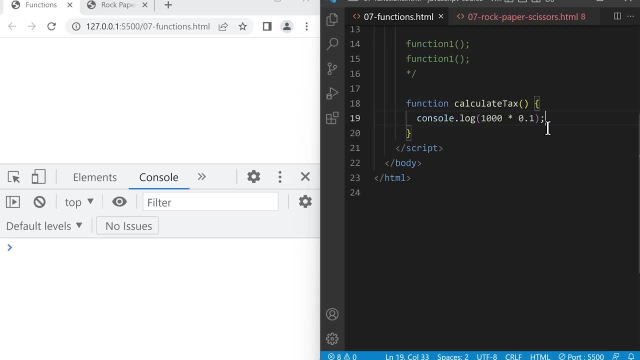 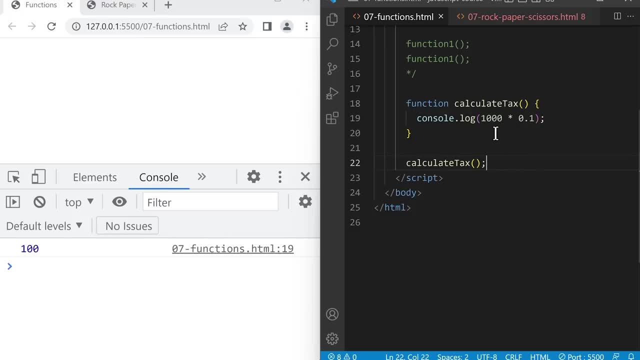 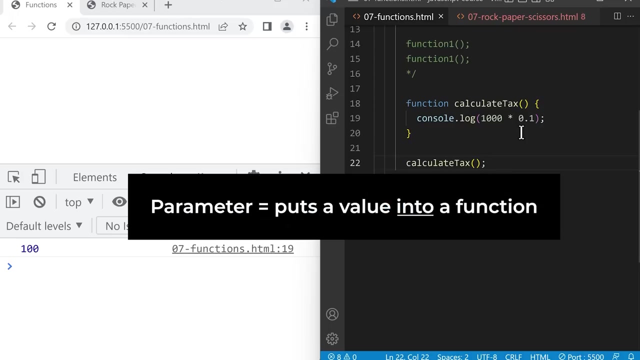 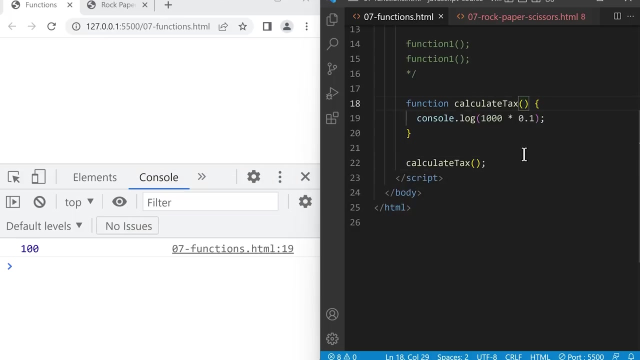 right now, this function only calculates the tax for $1,000.. What if we want to calculate the tax for a different amount? How would we calculate the tax for $1,000?? Let's take a look at the first parameter we need. 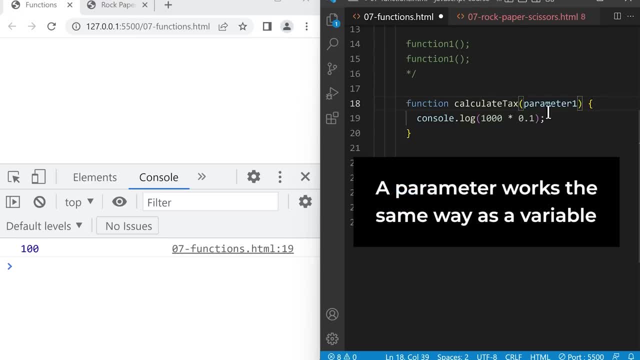 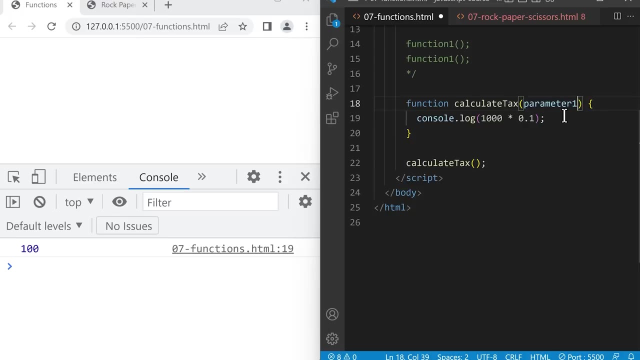 to calculate the tax for $1,000.. So let's finally create our first parameter. So inside this function we're going to put a value, For example $2,000.. This will save this value into this parameter. And now 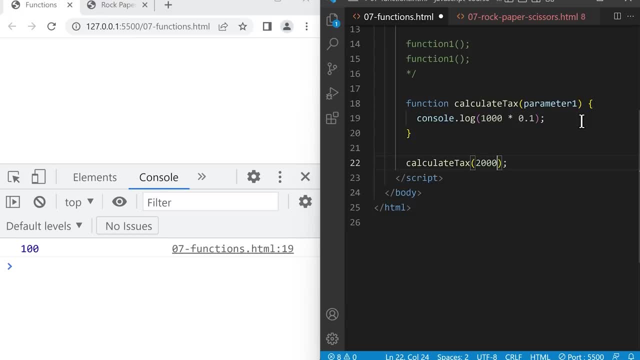 we can use it just like a variable. So let's take parameter 1. And it will take whatever value is inside parameter 1, in this case $2,000, and substitute it into the code. If we save, it will save. 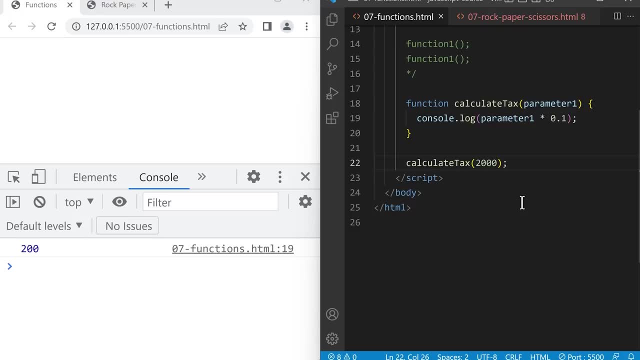 a different value into the parameter. For example, let's create a new line and call the function calculate tax, And this time we're going to save the value as $500.. So, as you can see, a parameter lets us put values into. 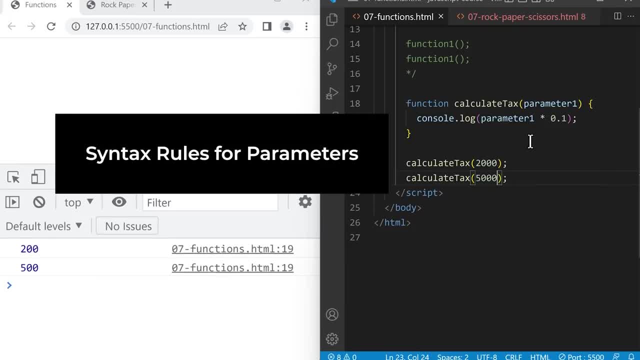 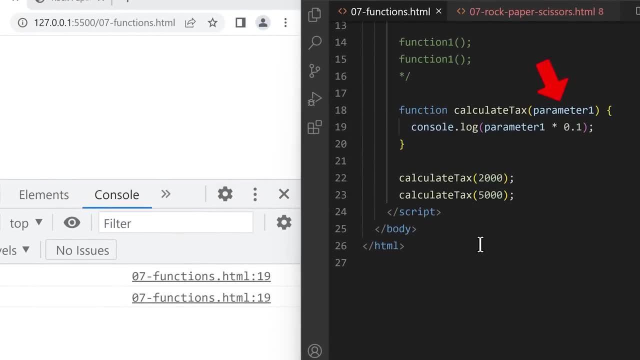 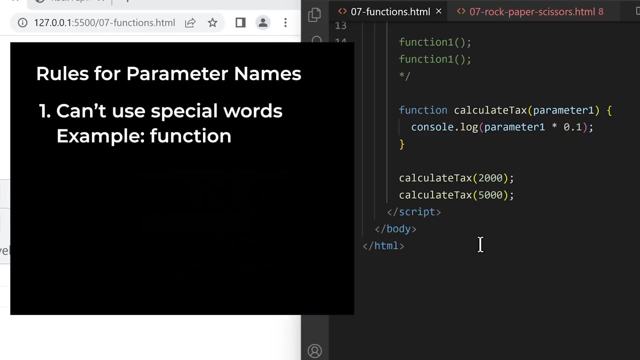 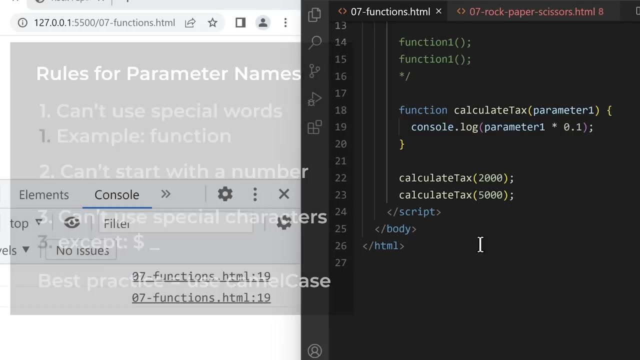 a function, And this allows our function to work with any value. Now let's learn about variable names. We can't use special words, we can't start with a number and we can't use special characters other than dollar sign and underscore. 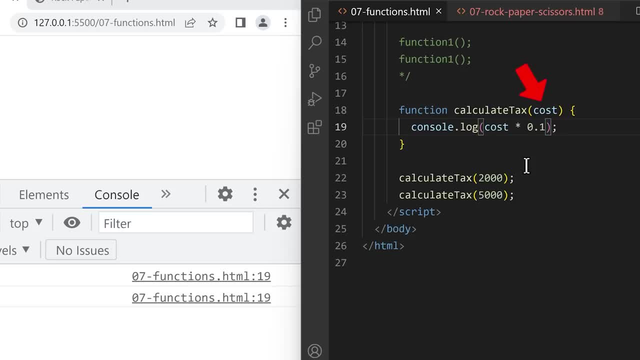 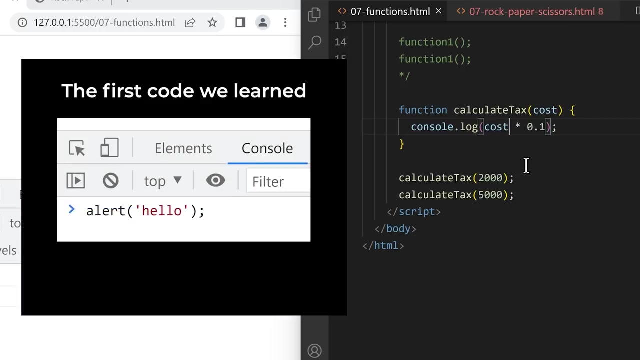 And the best parameter. we usually say: this function takes a parameter. If this parameter should be a number, we say this function takes a number. When we put a value into a parameter, we put a number into a number, So we can use this. 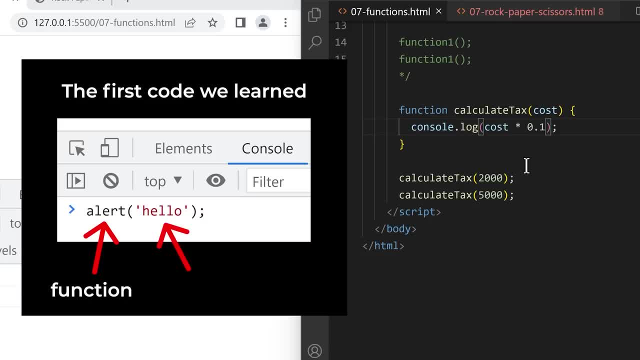 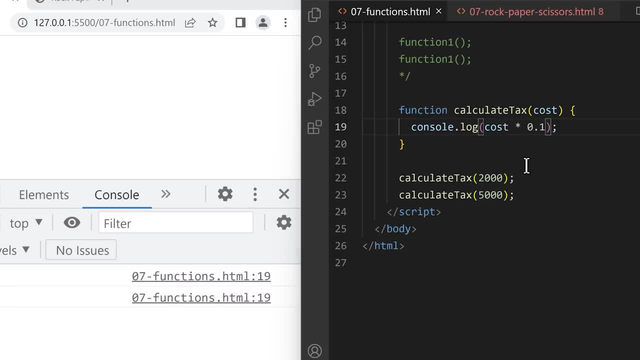 parameter to put a number into a number. So we can use this parameter. to use this parameter between the curly brackets. We can't use it outside the function. Next, a function can actually have more than one parameter. For example, right now. 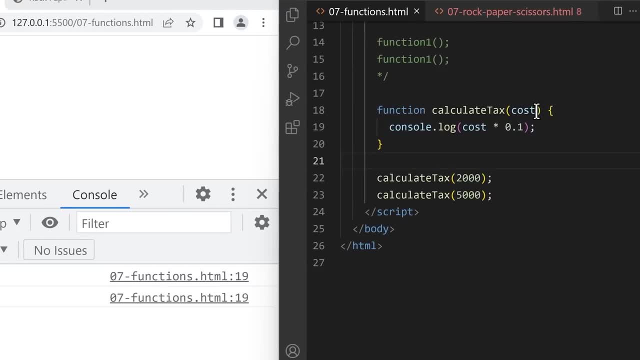 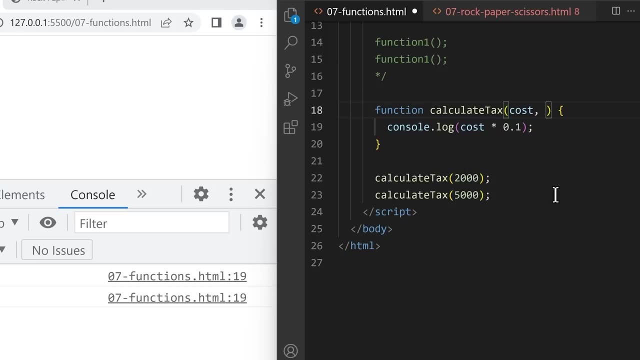 our value is 0.2.. So we can put a number into the second parameter by typing after the first parameter a comma and then another parameter name. Let's name this value 0.2, or a 20% tax, So the 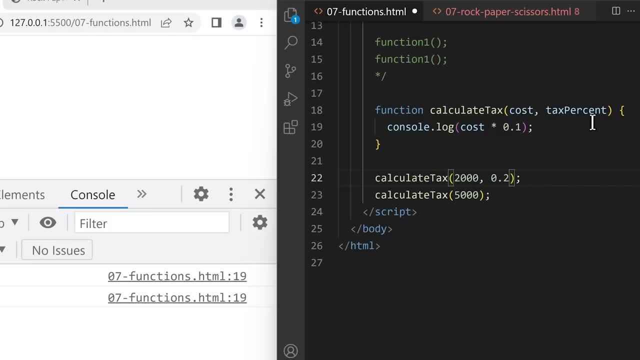 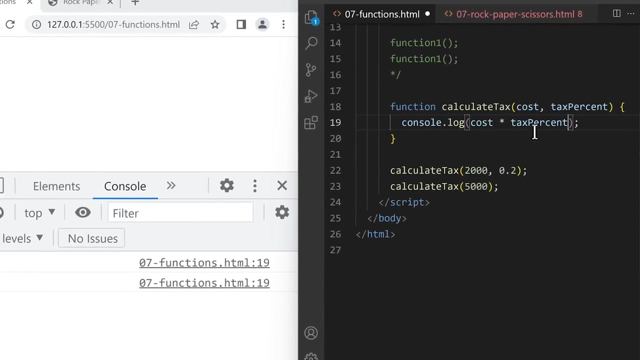 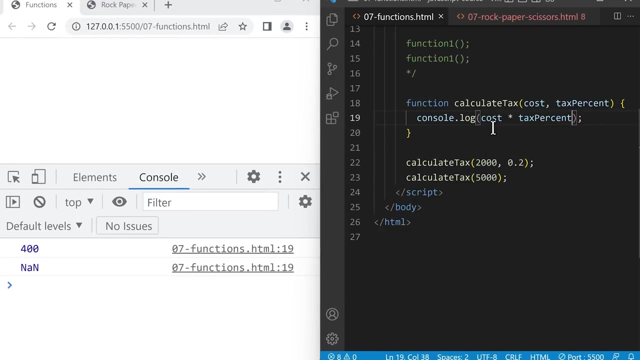 first value gets saved in the first parameter and the second value gets saved in the second parameter, And now we can put whatever value is inside tax percent into the code. If we save this first line will multiply 2000 by 0.2. 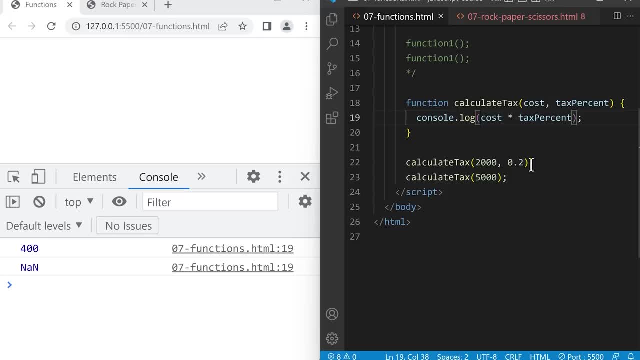 and give us 400 cents as the result. If we don't save a value into the parameter, the parameter will get the value undefined. So here, if we consolelog the second parameter, tax percent, and save, it will get the value in the. 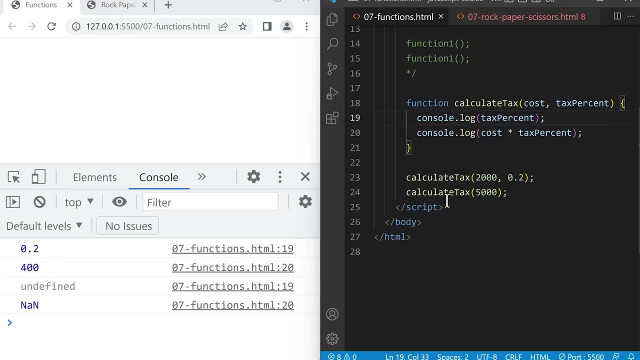 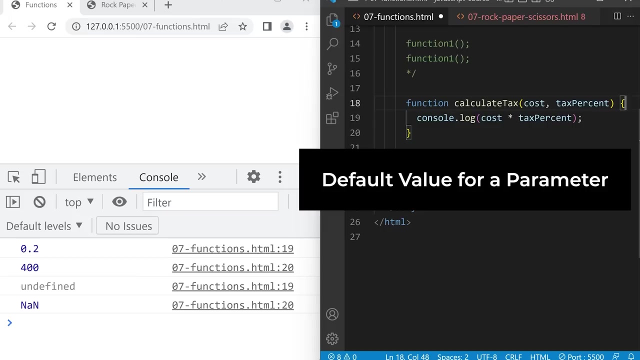 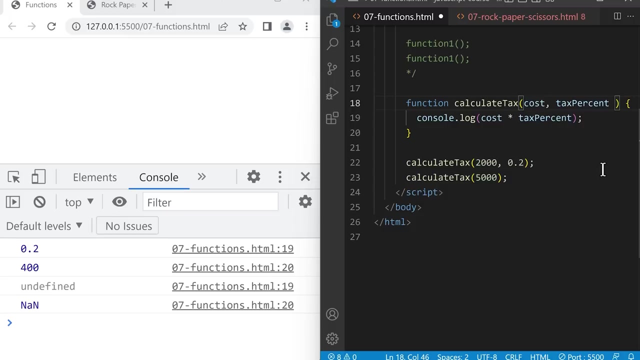 second line. And then multiplying the cost times undefined is not valid math. So we get the result: nan or not a number. So now let's look at the default value for the parameter. To set a default value, we can just type after the: 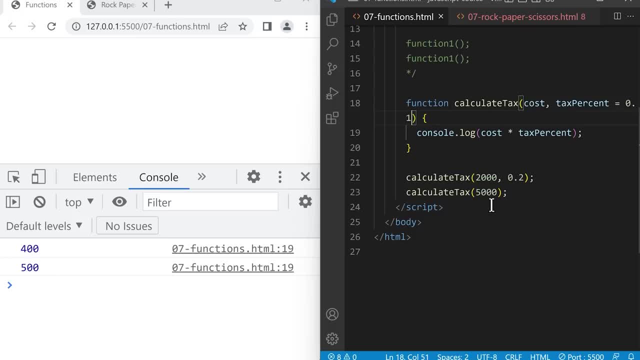 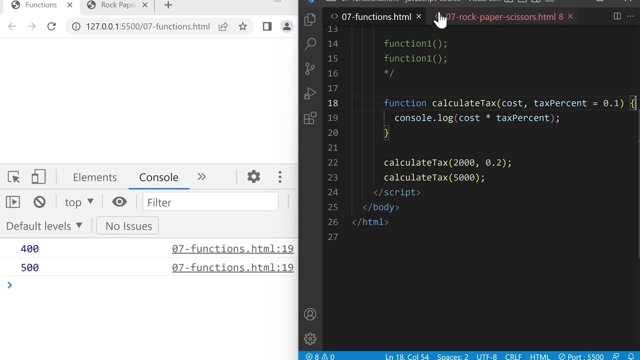 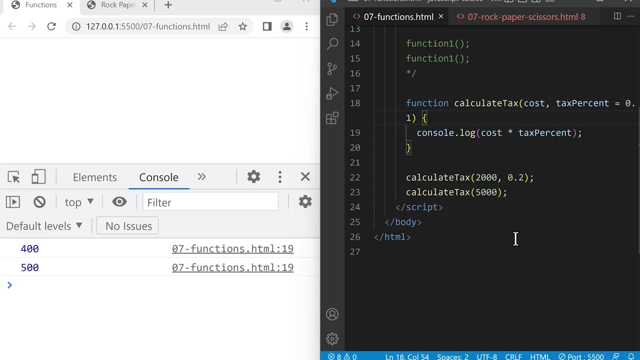 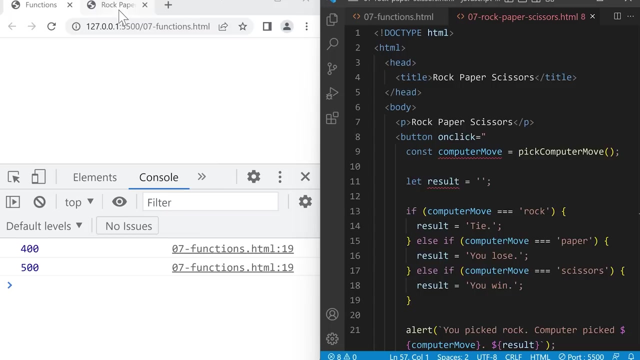 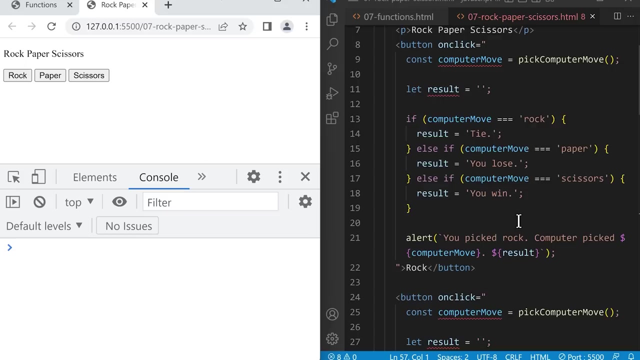 parameter and then add equal sign and a default value like this. So that's how we add a default value for a parameter. Alright, now that we learned parameters, we're going to go back to the rock paper scissors project and we're going to 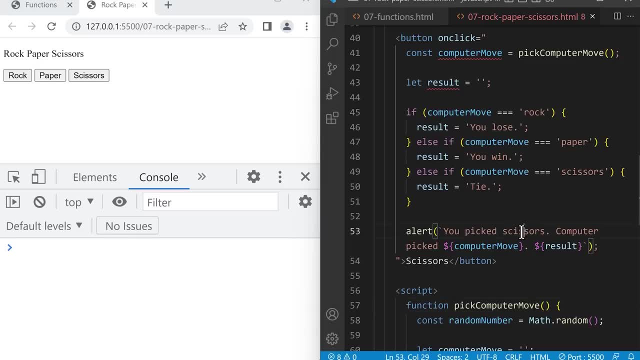 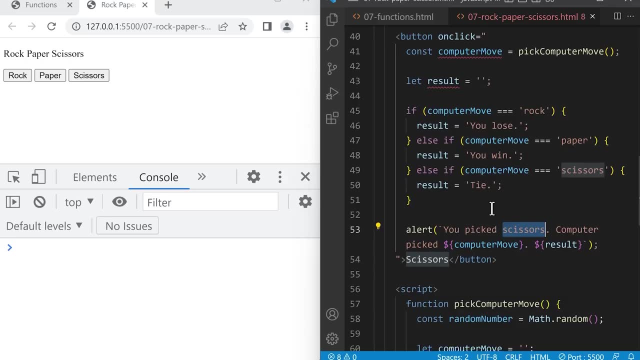 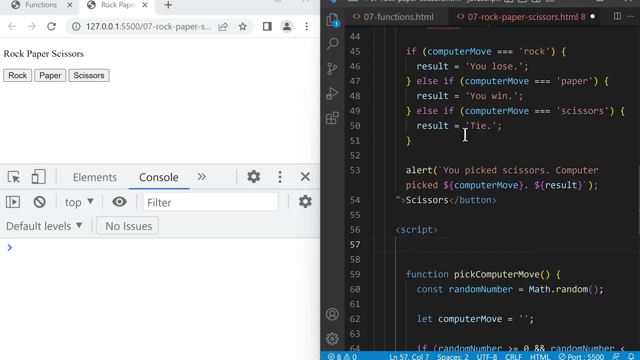 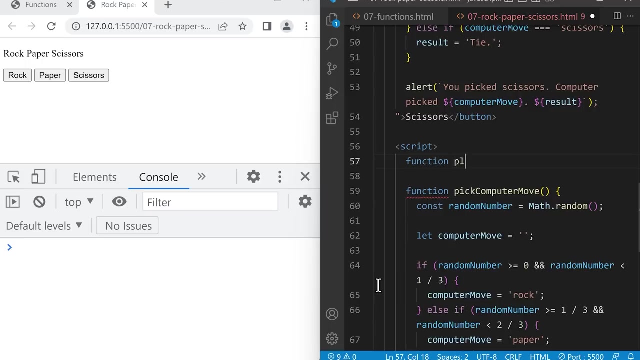 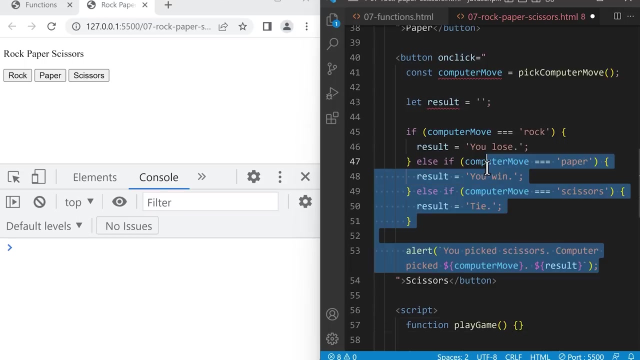 create a new function to reuse all of this code. We'll type function and let's name this function: play game. So now we have a game: brackets and curly brackets. Next let's move all of this code inside the function so we can reuse. 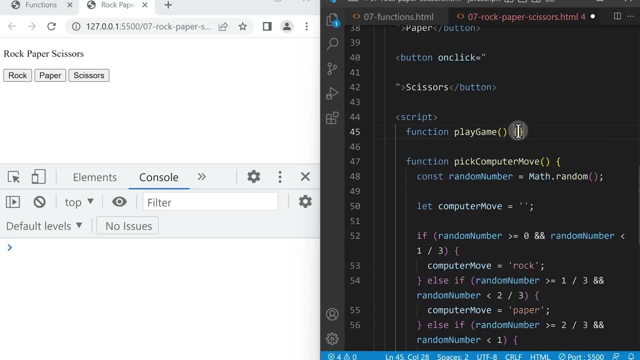 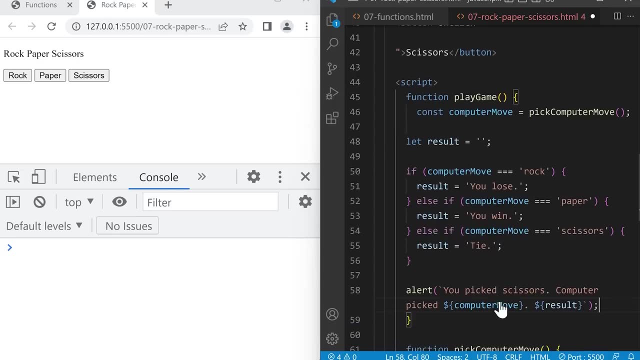 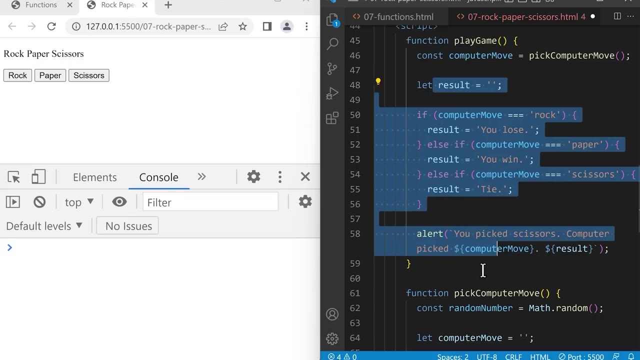 it. We'll select this code and then right click, cut and inside the new format we can select these lines and press tab. So the value that is different for each button is the move that we picked. So we're going to save a value into. 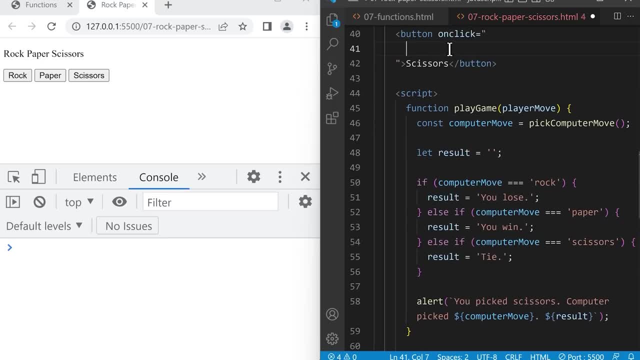 this parameter. So inside our scissors button we're going to call this function and run all this code. So let's type play game and call it move and type the string scissors. So, as we learned, this will save scissors into player move. and now we can. 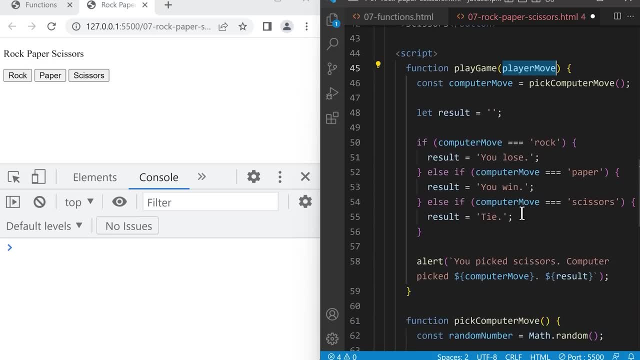 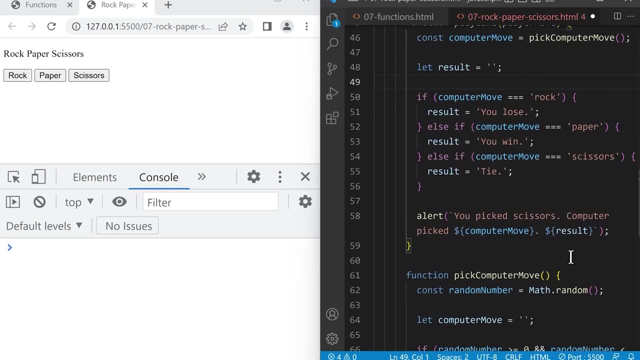 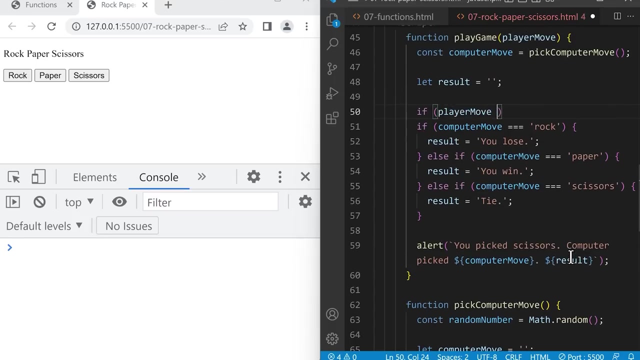 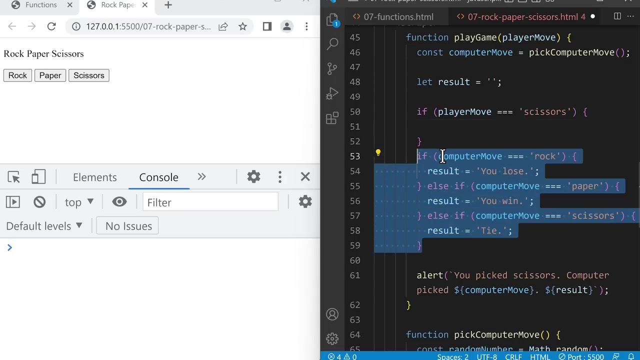 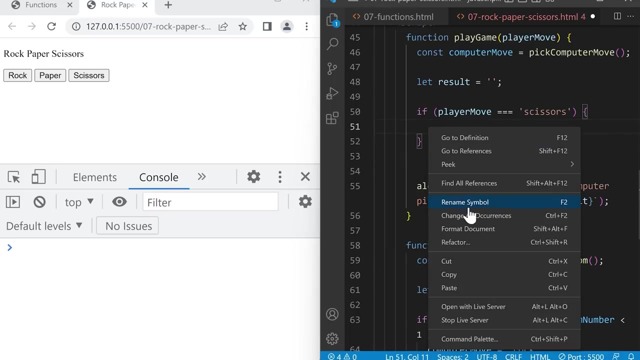 use player move just like a variable in the function. Now let's put this in an if statement So we'll type: if player move equals scissors and curly brackets Inside this if statement. we're going to put this code inside another if statement And 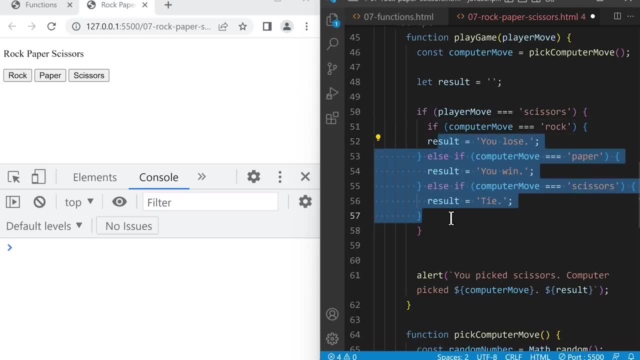 we did this because this code only makes sense if the player move is scissors. And finally, let's modify the code that displays the message. So here, instead of displaying scissors every time, we're going to display whatever is saved inside player move. So we'll 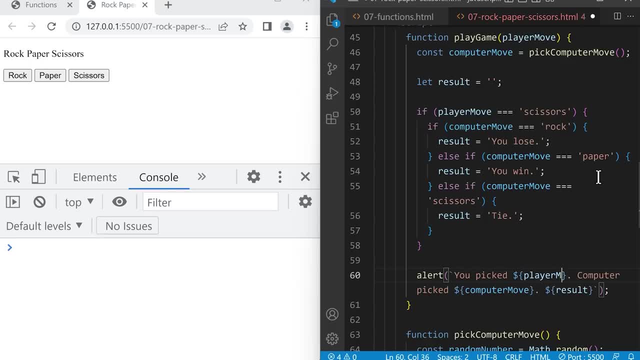 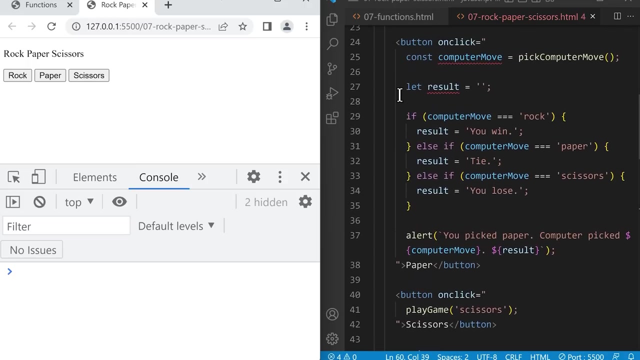 replace it with dollar. open curly bracket, close curly bracket And we're going to use the move scissors button And you'll notice that it works. We display the move scissors and we calculated the result correctly. Let's press ok and we're going to. 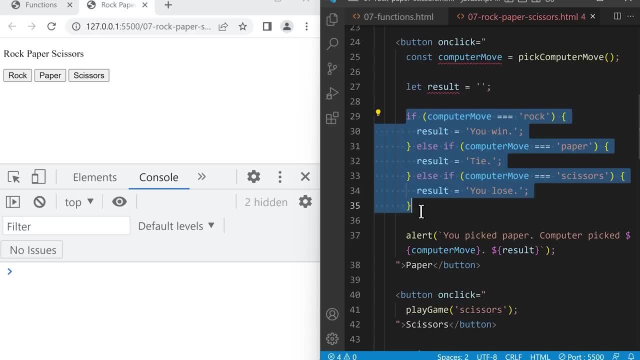 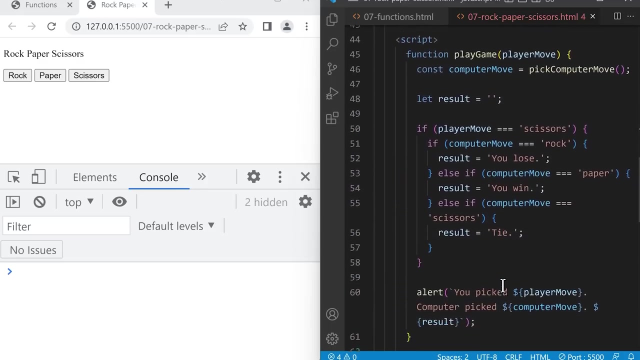 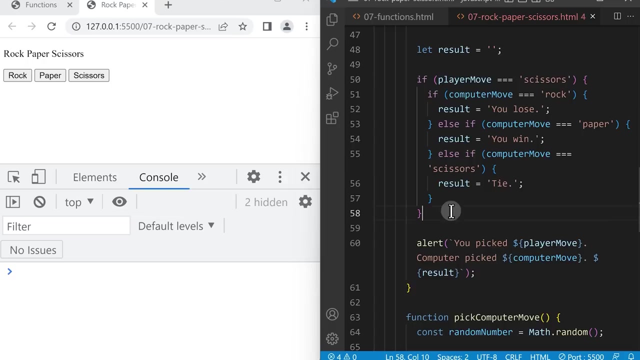 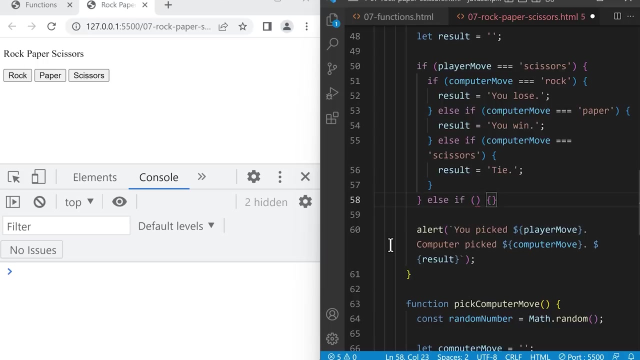 use a different if statement to calculate the result. So let's actually copy this into the function We're going to right click, click, copy and then inside the function we're going to create another branch. if the player move is paper. So inside this condition, 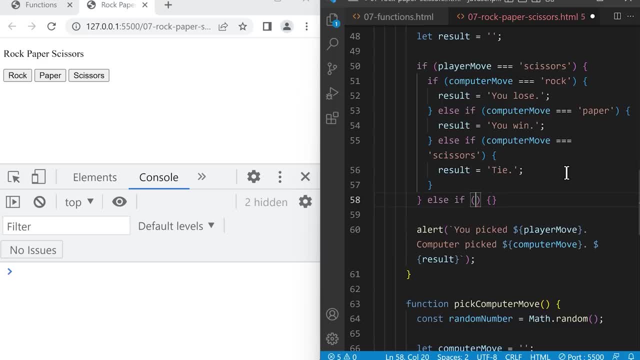 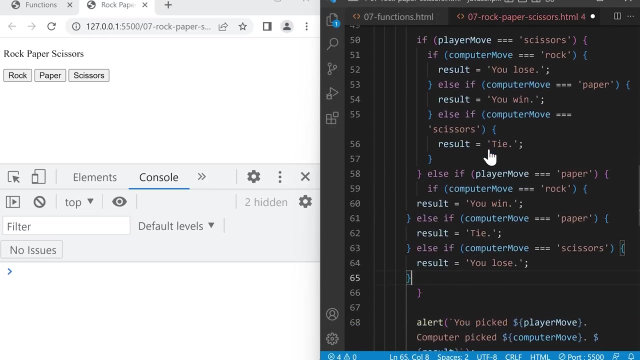 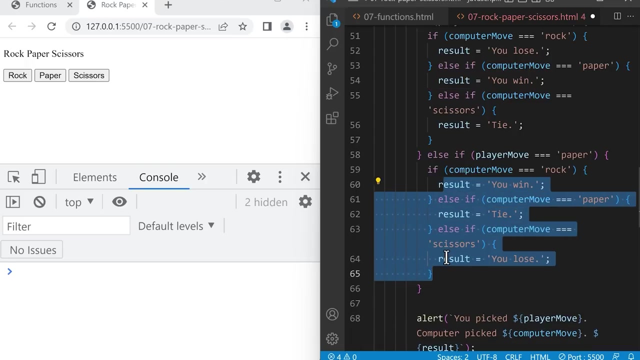 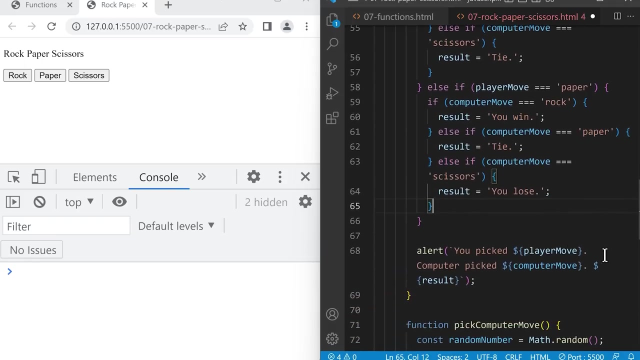 we're going to check if the player move is equal to paper this time, And then inside these curly brackets we're going to paste the if statement we copied earlier. So now we have the code that determines the result for paper Down here. we don't. 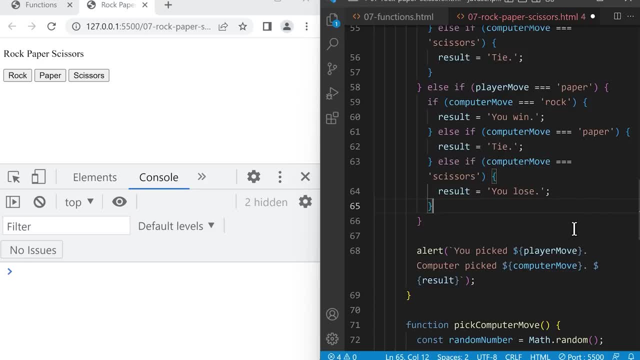 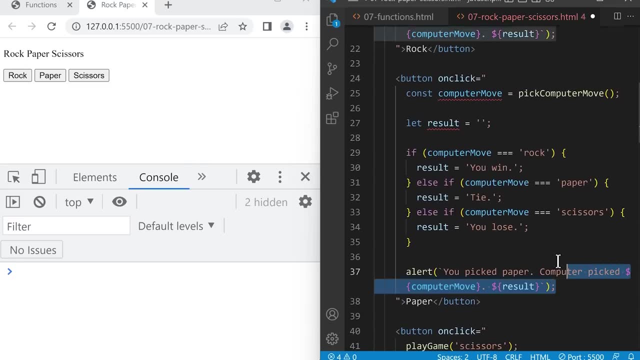 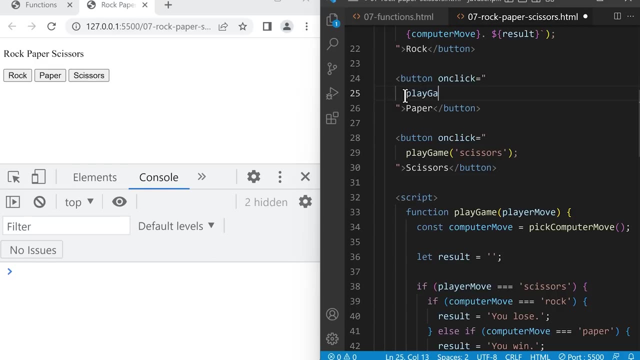 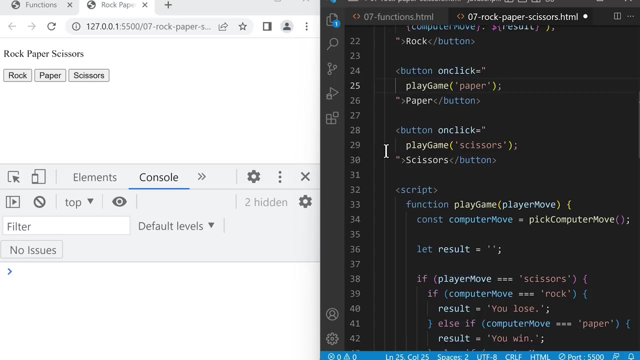 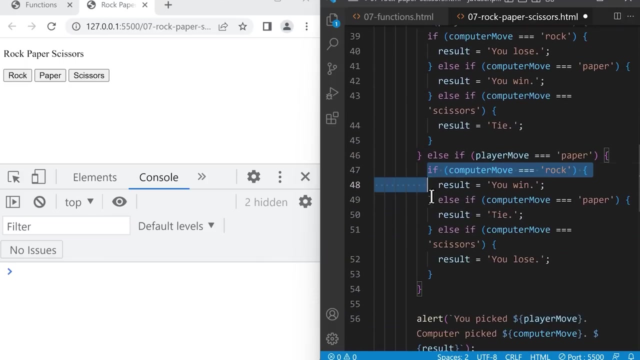 need to modify this code because we're always displaying whatever is inside player move. Finally, we click play game and we're going to pass paper inside. So now paper will get saved inside player move and it's going to run this if statement instead. If. 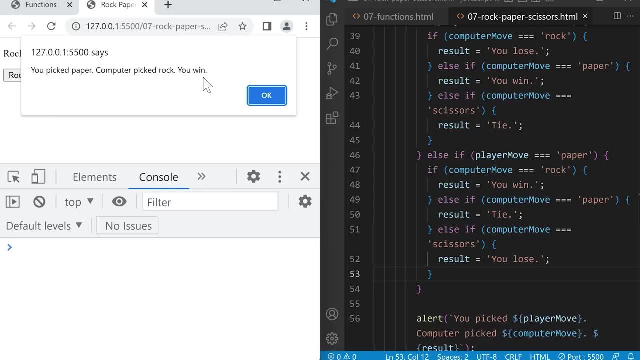 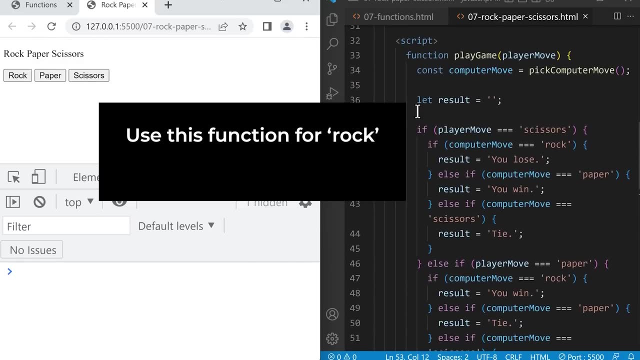 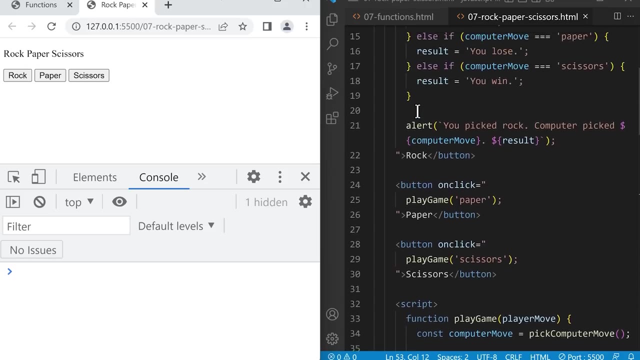 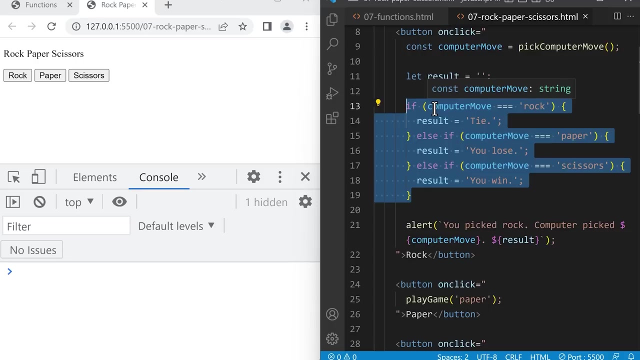 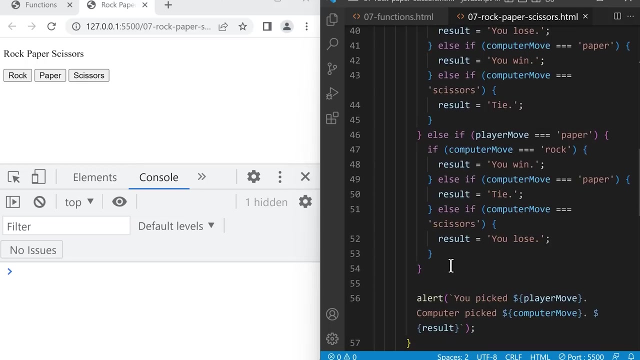 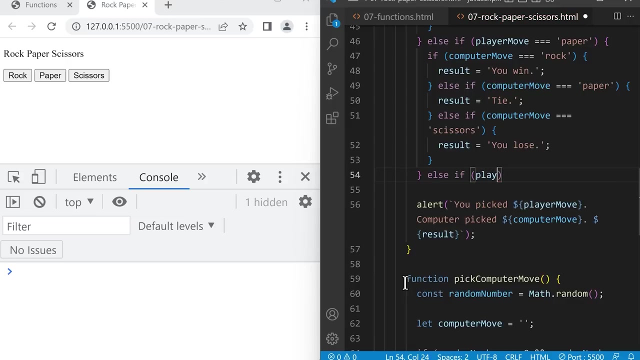 we want to do this. we need to copy this if statement into the function. So let's right click copy and then inside the function. we need to copy this if statement inside the function. Let's create a branch for rock, else if player move is equal. 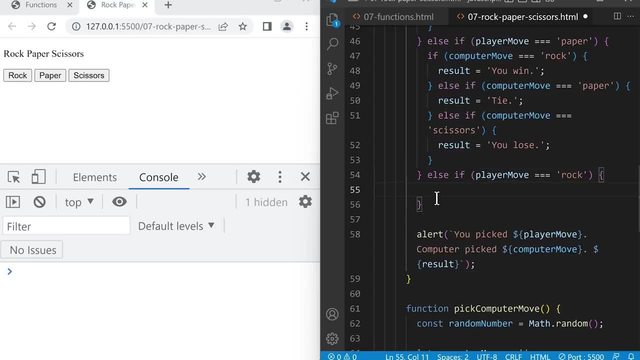 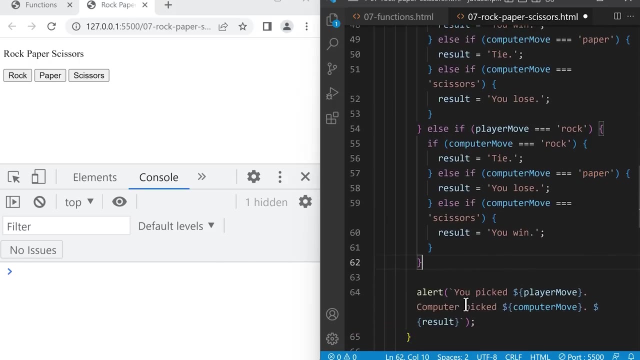 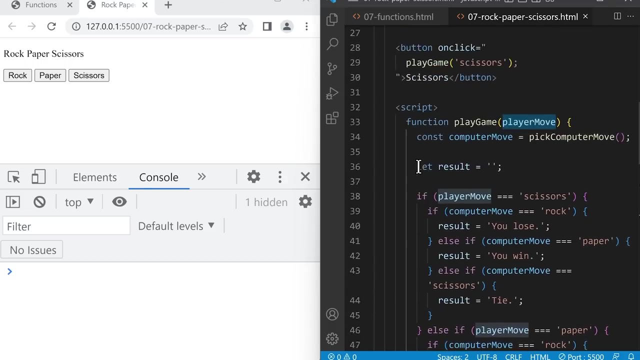 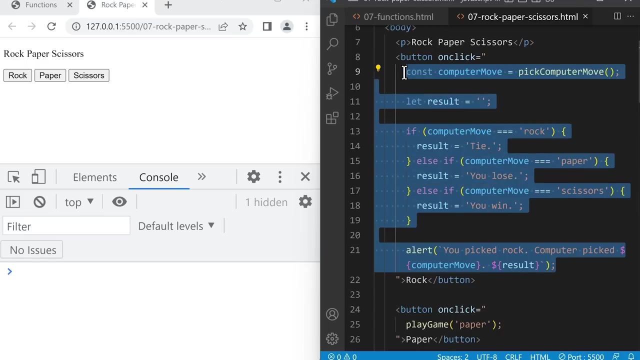 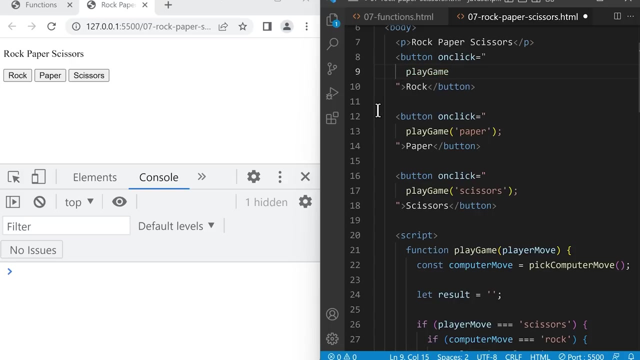 to rock and then curly brackets and inside here we're going to right click and do the same thing we did with string rock and we're going to remove it and just call our function instead play game brackets, and then inside we'll have a function called rock. 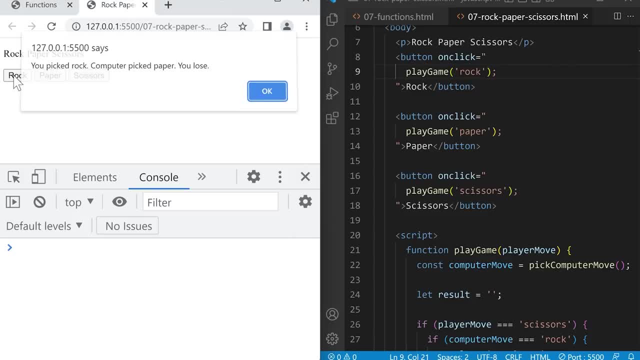 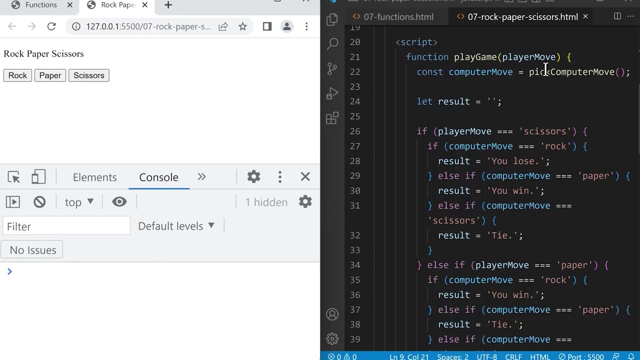 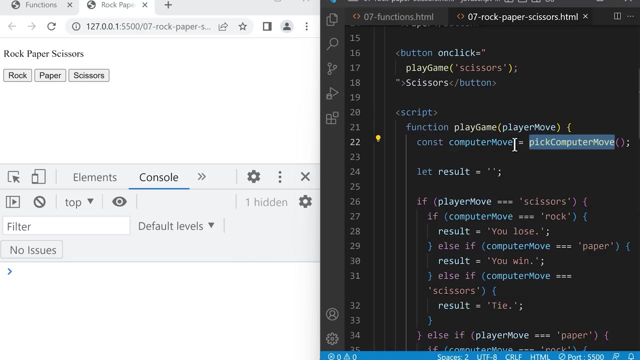 now let's save and click the rock button. so I picked rock, the computer picked paper and we calculated the result correctly. let's press ok. so lastly, notice that inside a function we can call other functions. let's go through the code step by step so that: 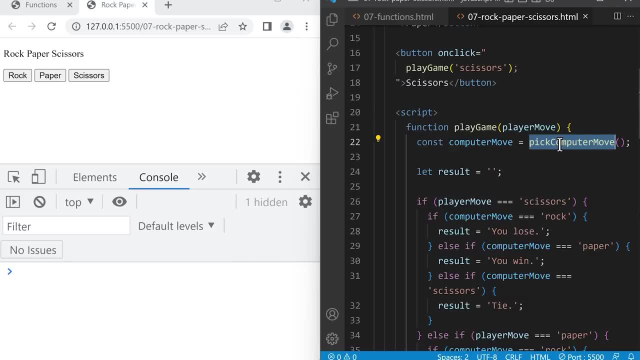 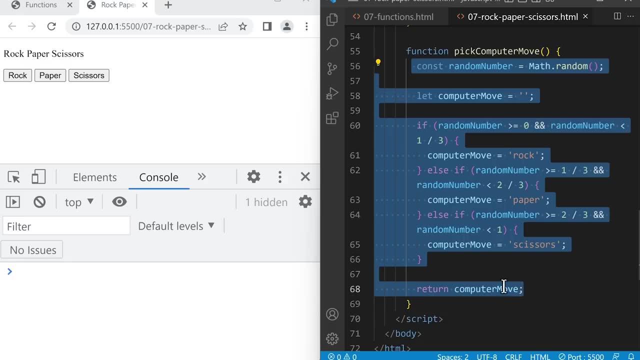 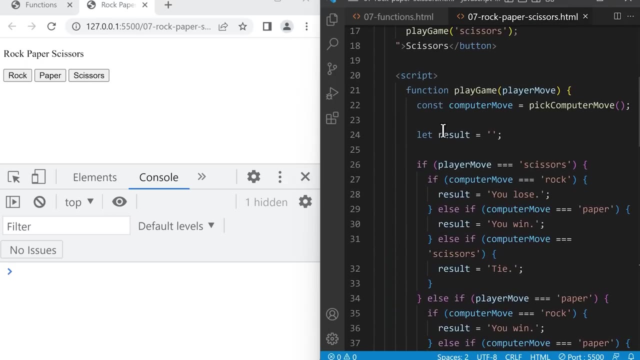 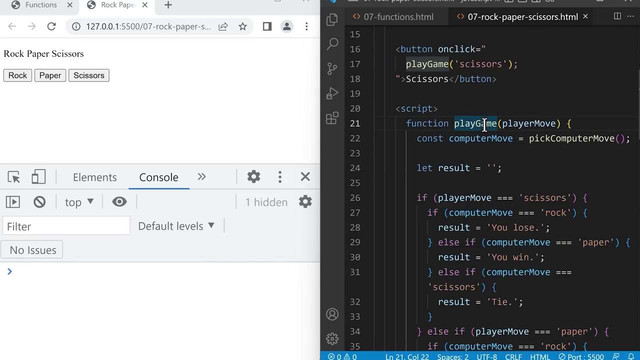 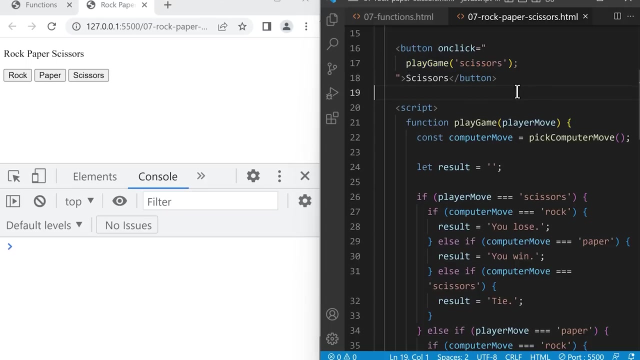 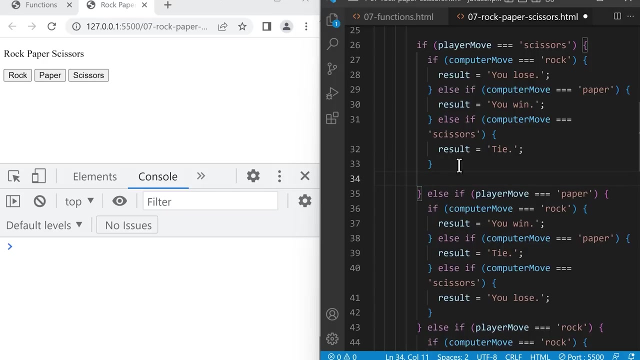 we understand how it works. so here, when this function returns, we're going to return back to where we called it and then keep going and run the rest of the code, and then, when the play game starts, we're going to add some new lines to this, if 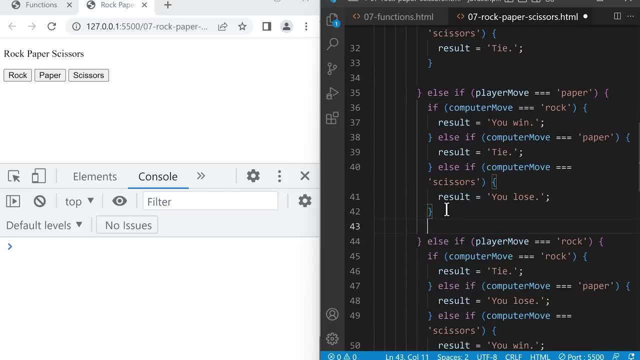 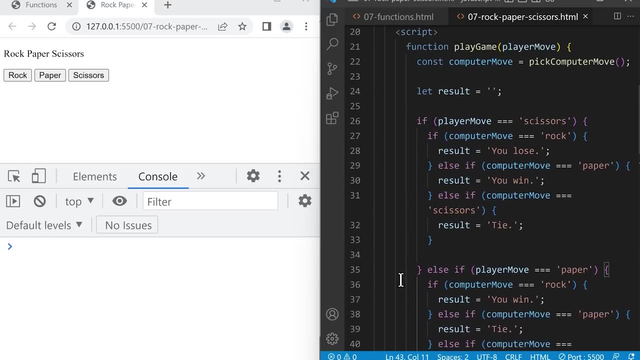 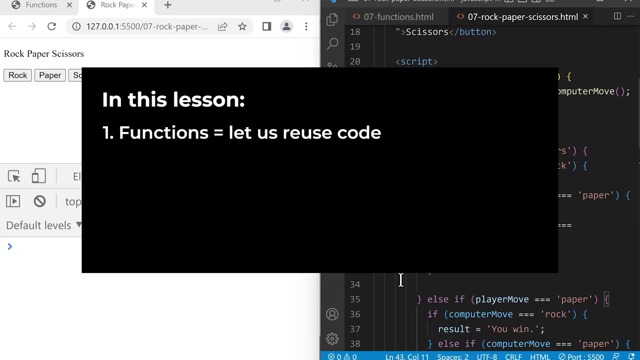 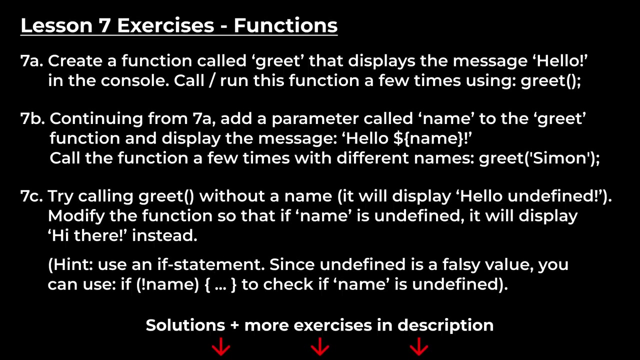 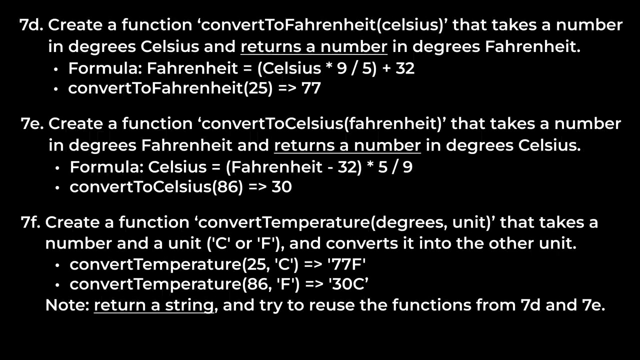 statement to separate the branches and make the code a little easier to read and save. and let's scroll up. we learned how to get a value out of a function using return. we learned how to put values into a function using parameters and we learned how to create. 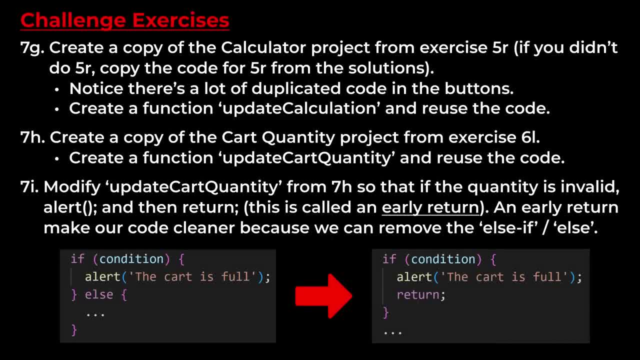 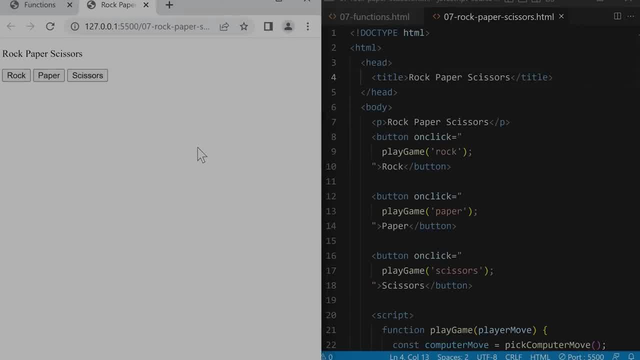 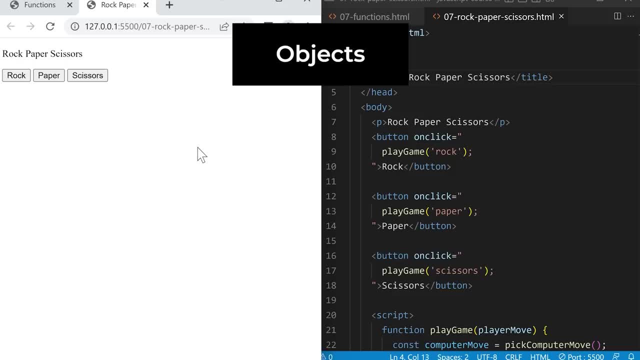 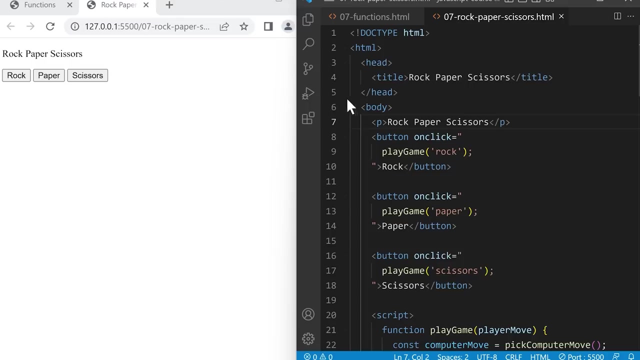 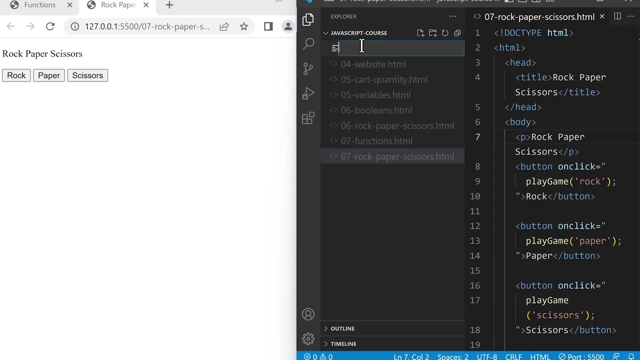 a value in javascript. in this lesson, we're going to learn another type of value in javascript called objects, and we're going to use objects to create a new file. for this lesson, we'll go to our code editor and click this icon and then click this icon. 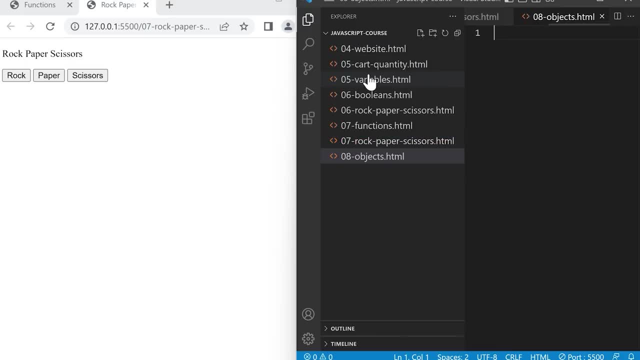 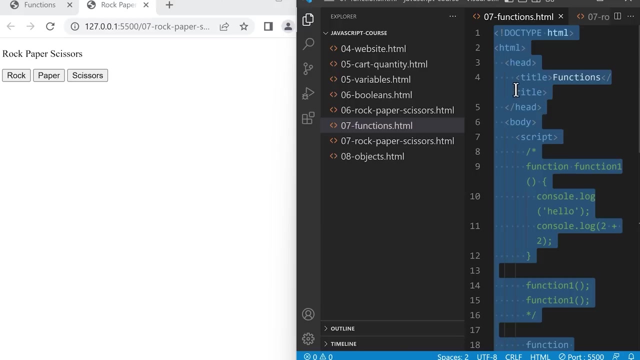 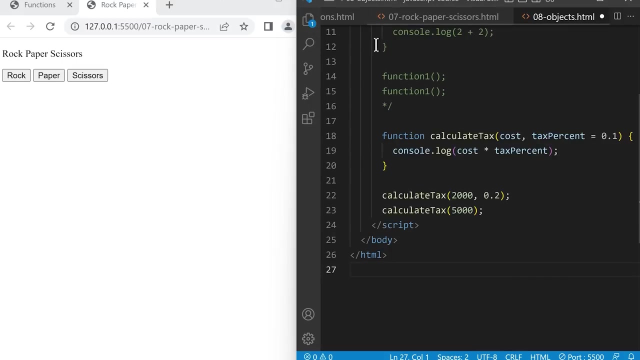 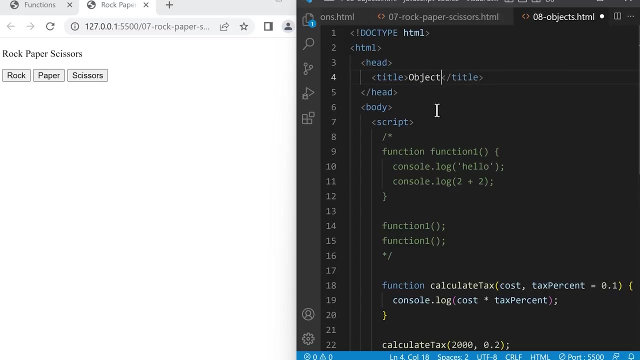 to create a new file and we'll name this file to objects dot html. so we'll type here and press control a or command a to select the code and then right click, copy and in here right click and remove all the code in the script element. finally, 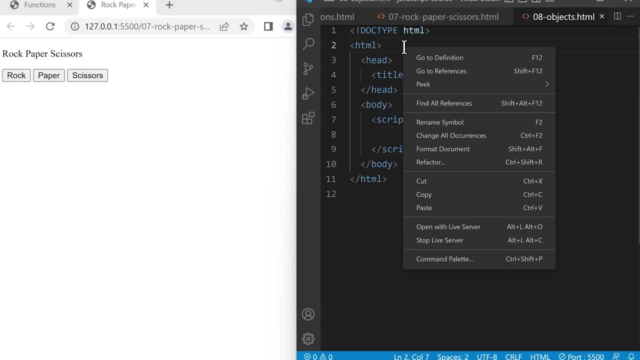 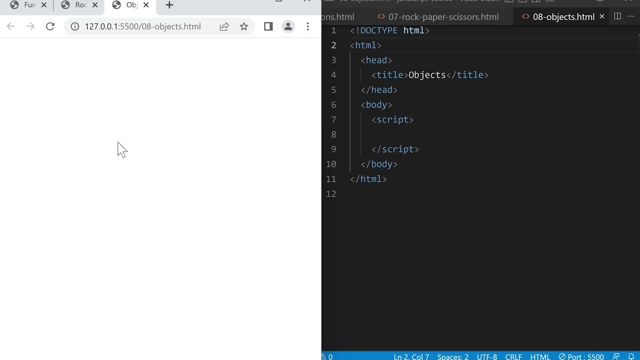 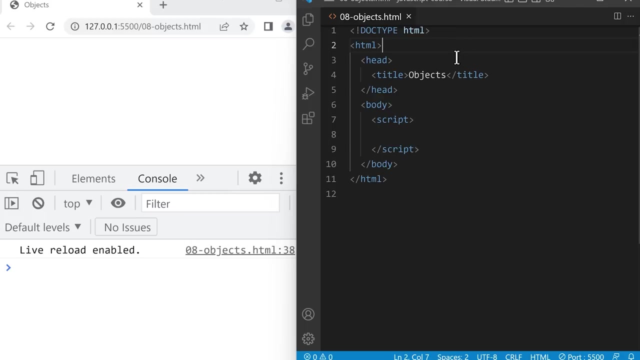 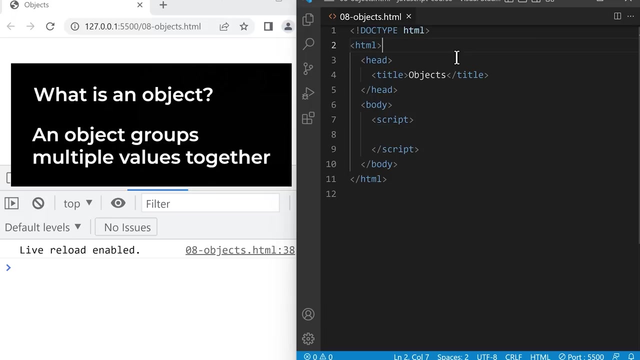 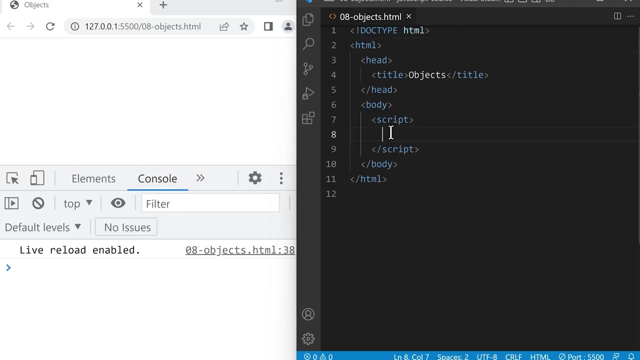 let's save and open this in live server by right clicking open with live server and let's also open the script. let's close our previous tabs and also the previous code, and now we're ready to learn objects. so what is an object? an object groups multiple. 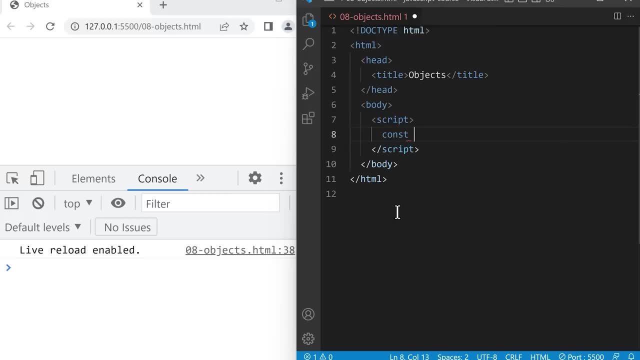 values together and we'll name this variable product and make it equal to open curly bracket, close curly bracket and semicolon. so this is an object. inside this object we can add a comma and then price colon and another value like the number 1090. so inside 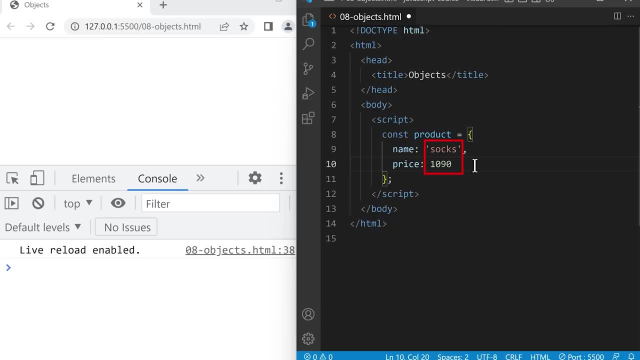 our object. we just added two values. so at the bottom here we have the product and save and it will display both values into the console. so, as you can see, an object lets us group multiple values together. so, for example, let's type an enter and console dot. 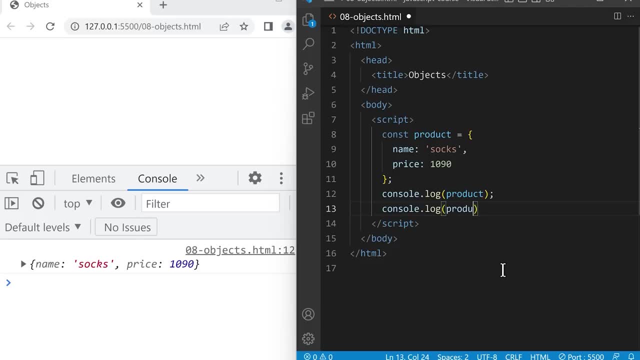 log. we're going to type the object product and then a dot and then a property like name. so dot name will display the string socks in the console. let's do another example and we'll access this second value using the property price. so we'll type enter: 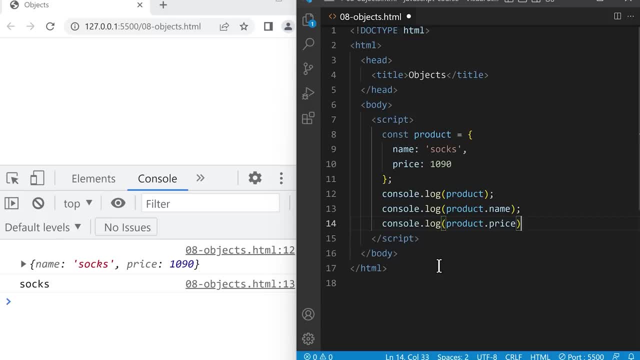 console dot log the value. so this will access the value associated with price, which is 1090. if we save, that's what gets displayed in the console. now we can also use the property to make it equal to something else, like the string cotton socks. so this: 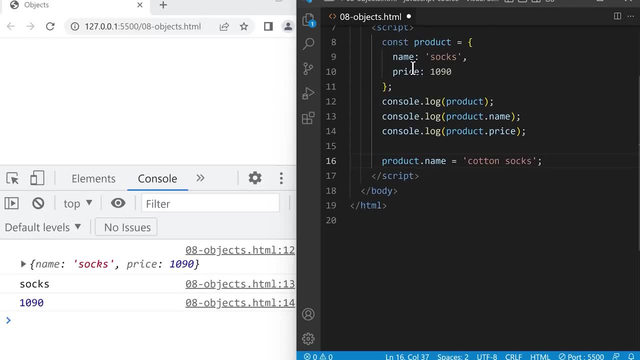 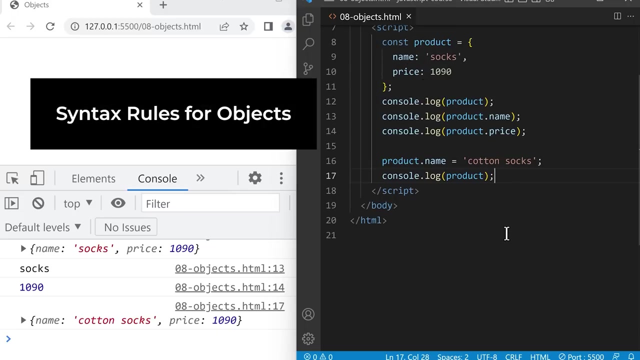 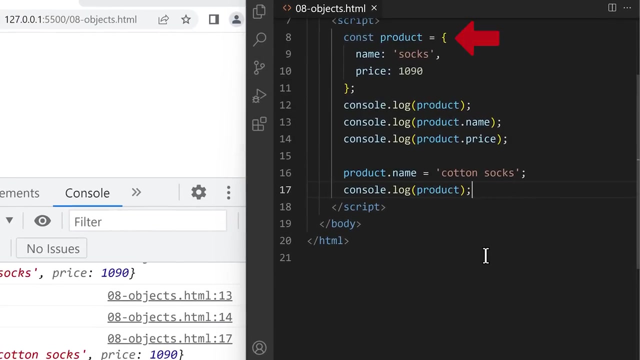 code will change the value associated with the name property to cotton socks. so that's how an object works. we group multiple values together and then we can access or change these values using the properties on the left. now let's learn the first step. we start with an. 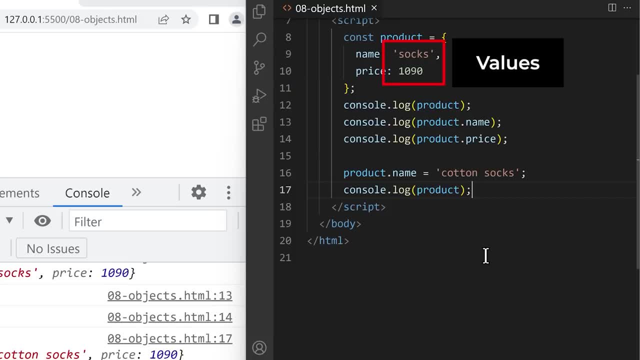 open curly bracket and end with a closed curly bracket inside the object. we can put multiple values. for each value- the code on the right side of the object and we separate them with a comma. to access a value inside the object, we type the object's name and 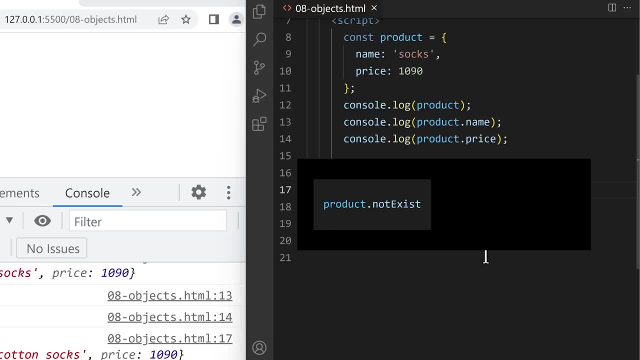 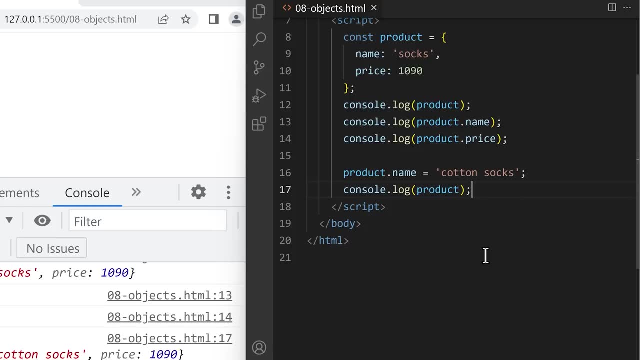 then dot and dot to define the value, but the value will be undefined. to change a value in an object we can use the dot notation again. so product dot name and just make it equal to productnewProperty and make this equal to something like the boolean value. true, 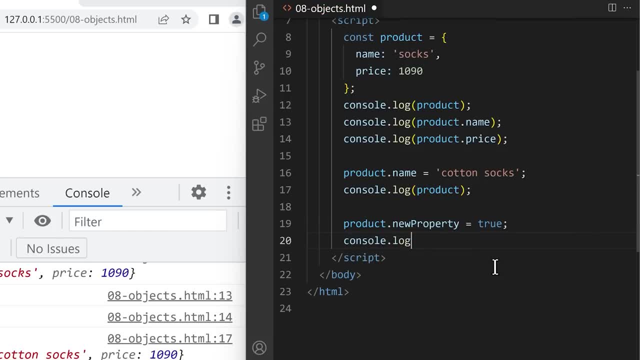 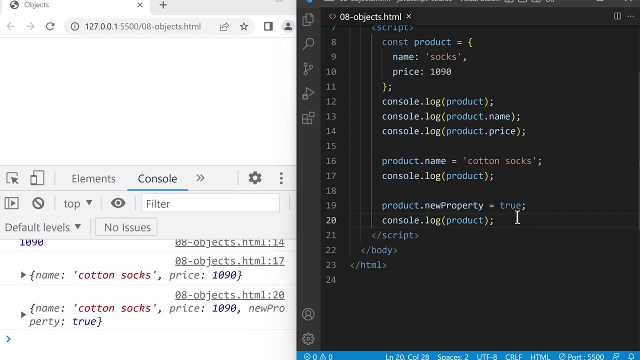 If we consolelog the product again and save, it will add this value to the object along with the new property. We can also remove a value from an object by typing delete and then the object, product dot and then the property we want to delete like newProperty. 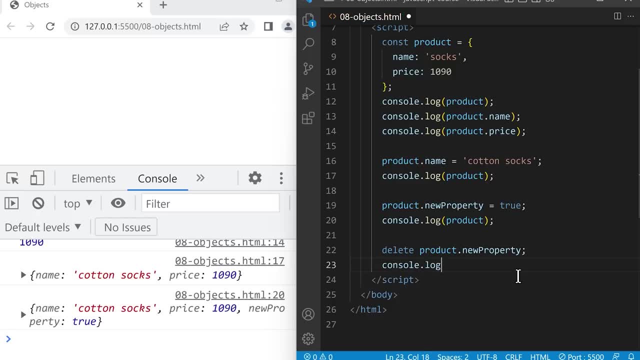 If we consolelog the product again and save, This code will delete newProperty from the object And, lastly, notice that an object is just another type of value. We can save an object inside a variable and we can also consolelog objects. 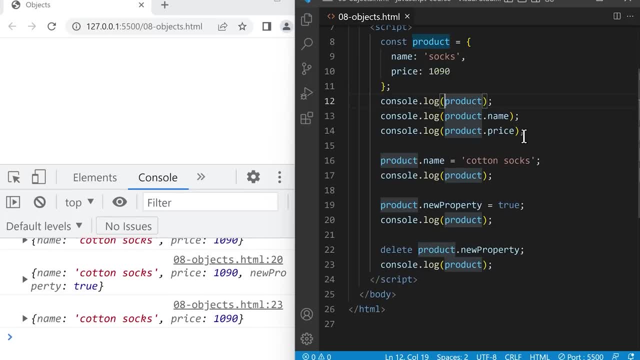 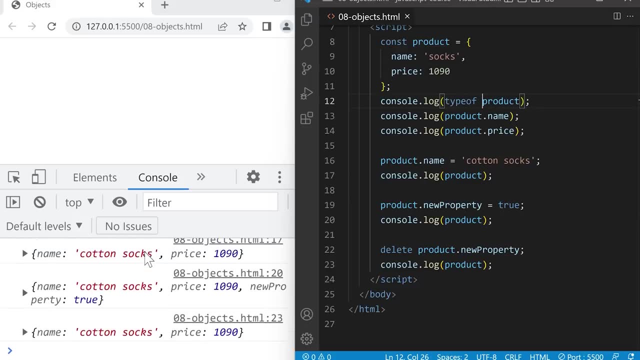 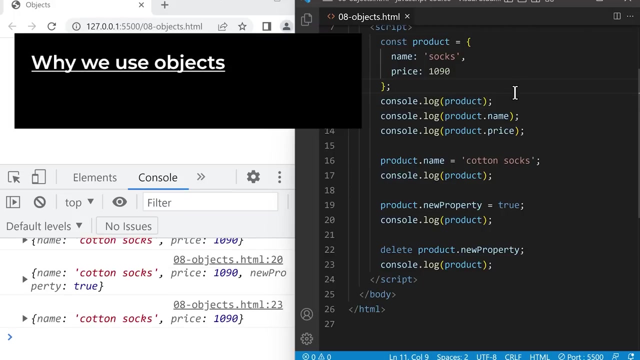 If we check the type of this value- so type of product- and save And scroll up in the console, It will tell us that product is an object. So let's remove this and save, And now we'll learn why we use objects. 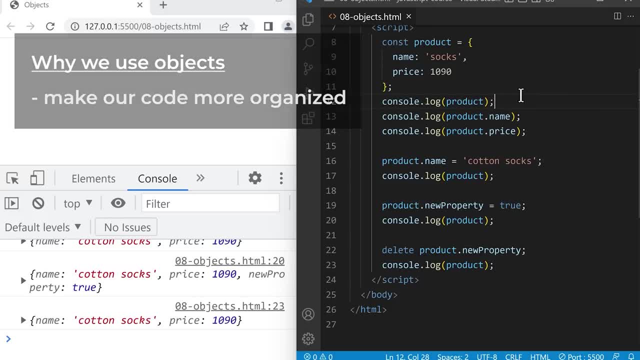 So objects make our code more organized. Instead of creating a bunch of variables for the product's values, like the name and the price and other details, Let's group all these related values together into one object. Objects also allow us to use multiple values together. 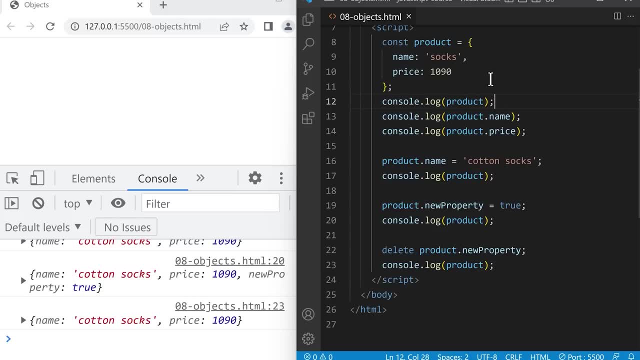 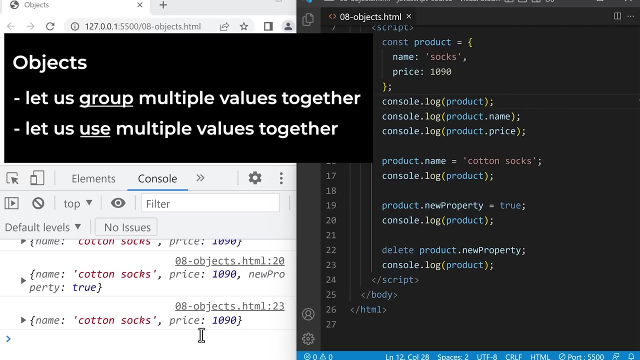 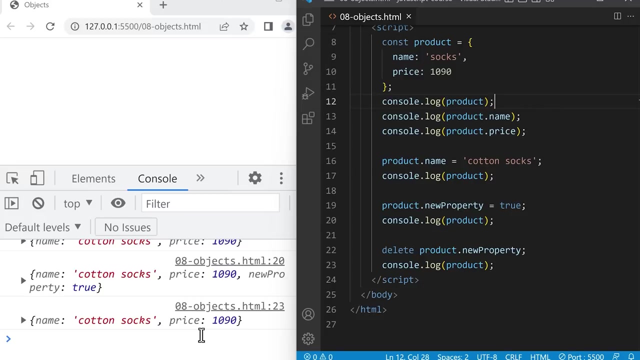 Instead of consolelogging each of these values individually, we can just consolelog the whole object and display all the values at once. So, objects, let us group multiple values together and let us use multiple values together. Next, let's do a practical example with objects. 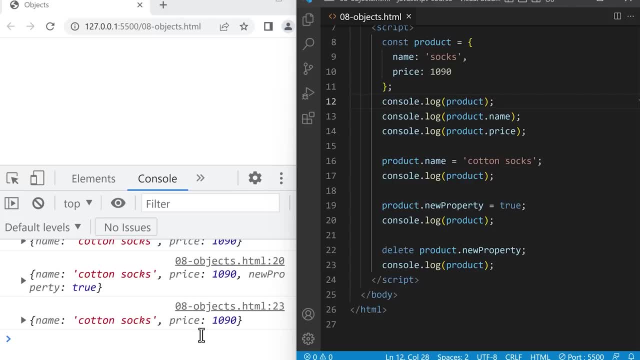 We're going to add a score to our Rock Paper Scissors game, So I've actually prepared a project we can use for this lesson. To see this project, we're going to go to our site and then create us a new tab. 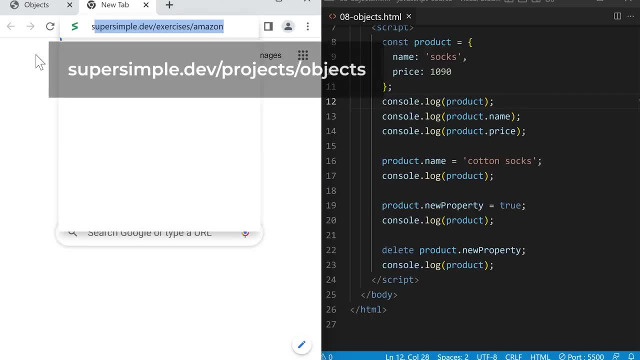 And then up here we're going to type supersimpledev/fnh projects, slash objects and press enter. So this is our simplified rock-paper-scissors game again, except in this project, when we play the game, it's also going to keep track of a score. 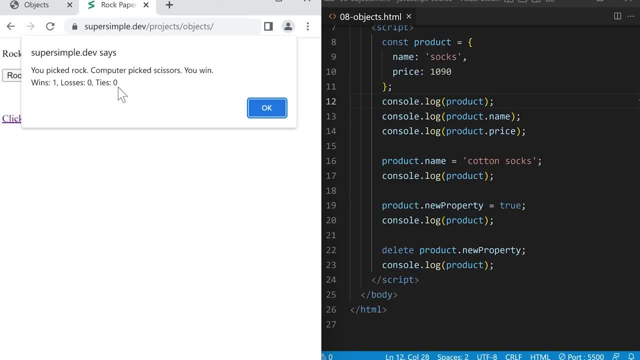 So how many times we win, lose and tie. And also if we click OK, we have a reset score button. So if we play the game a few times and add to our score and then click the reset score button, this will reset the score back to zero. 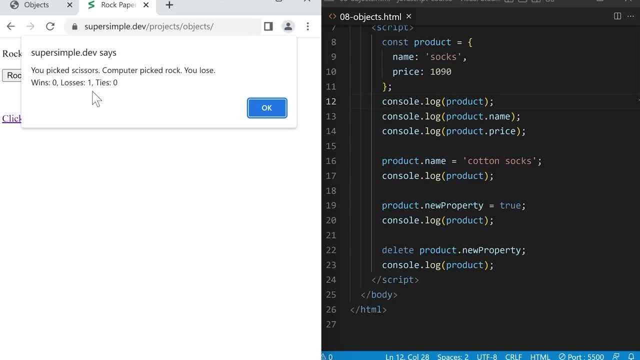 So if we play the game again, the score starts from zero again. So we're going to learn how to use objects to create a score. So let's create this feature, Let's press OK And first let's create a copy of our project, just for this lesson. 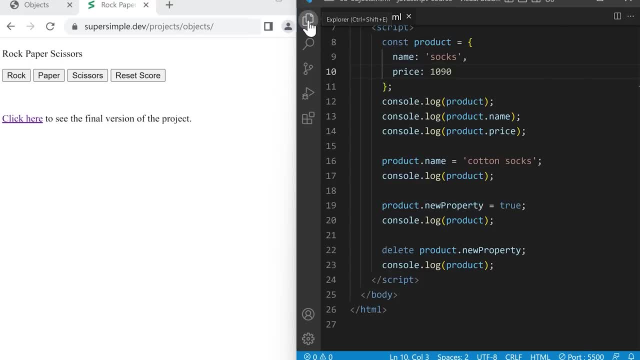 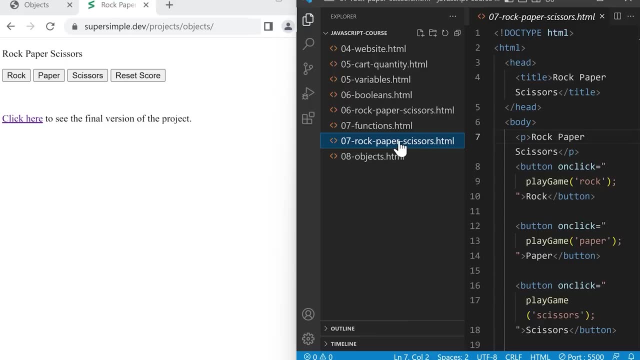 We'll go to our code editor and click this icon to show our files and we'll make a copy of the rock-paper-scissors project from the previous lesson. So we'll right-click and copy and down here, right-click and copy. 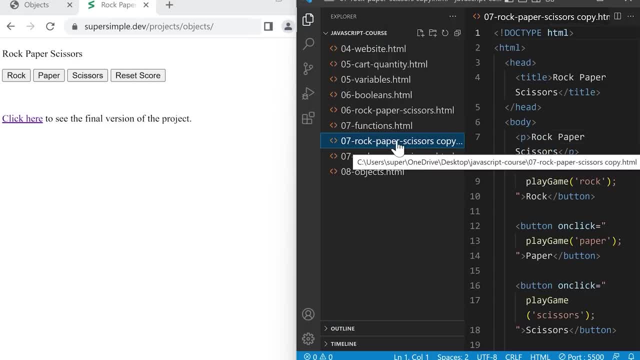 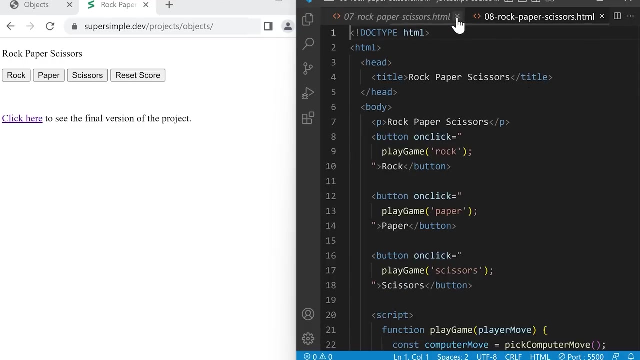 And paste And we'll right-click and rename this file. We'll remove the copy at the end and at the front we'll change this to 08, and press enter. Now let's hide these files and we can close the 07 file for now and let's open this in. 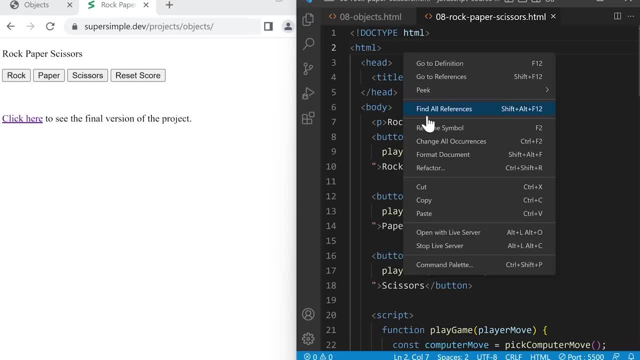 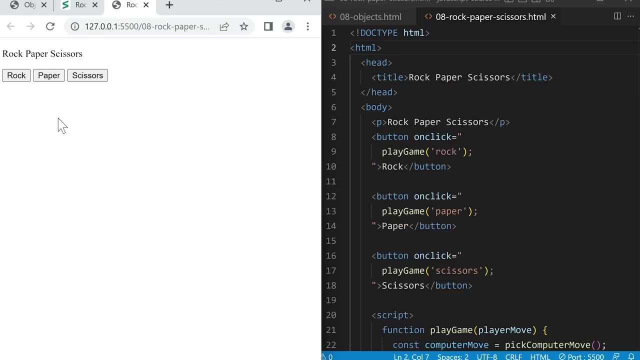 live server By right-clicking And open with live server. Let's also open the console on this page. So right-click, inspect and the console Alright. now let's go into our code and add a score to our game. 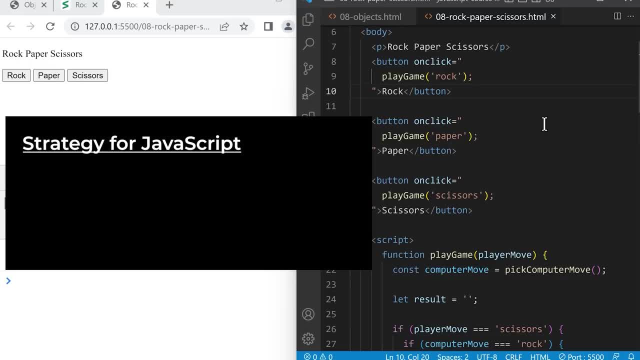 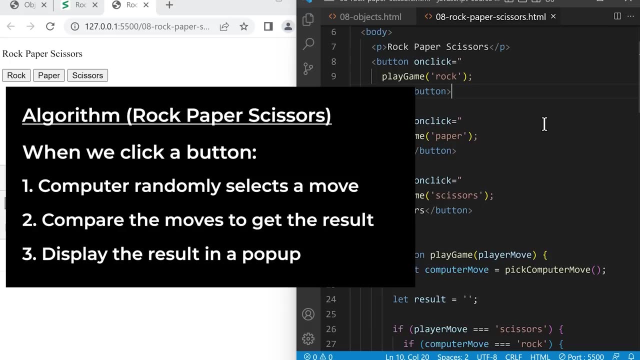 So remember, when writing JavaScript, a good strategy is to think about what steps we need to do- This is called an algorithm- and then convert those steps into code. So we already had an algorithm for the rock-paper-scissors game. Let's update this algorithm to include the score. 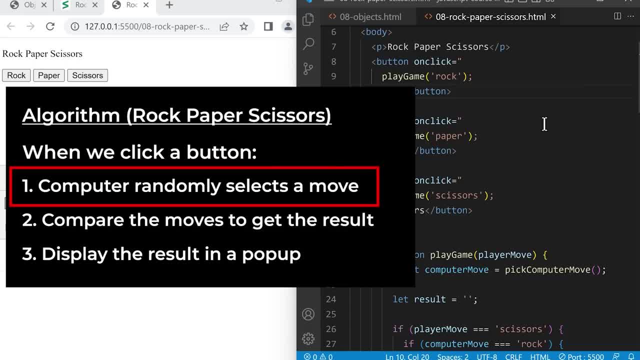 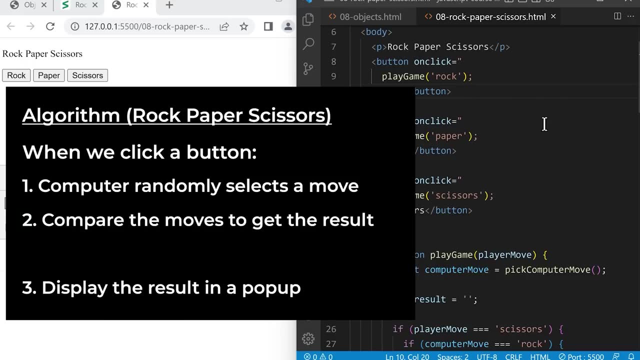 So first, the computer randomly selects a move. This step will stay the same. Number two: we're gonna compare the moves to get the result. This step will also be the same. But now We're gonna add an extra step. After getting the result, we're gonna update a score. 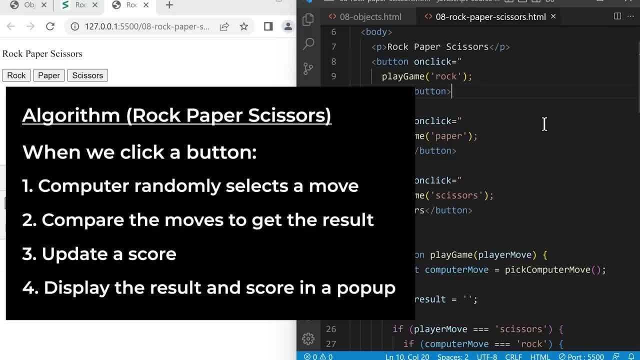 And finally, we'll display the result and the score in a popup. Now let's convert these updated steps, or this algorithm, into code. The first thing we need to change is we added a third step. We're going to save and update a score. 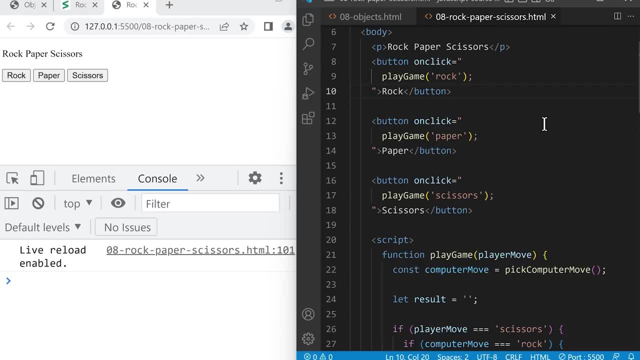 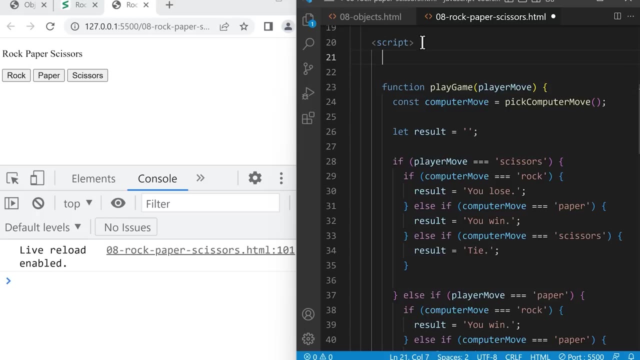 So first we need somewhere to save our score. So one place we can save it is inside a variable. Let's go to our script element And at the top we're going to create a variable for our score using Const Score and make it equal to an object. 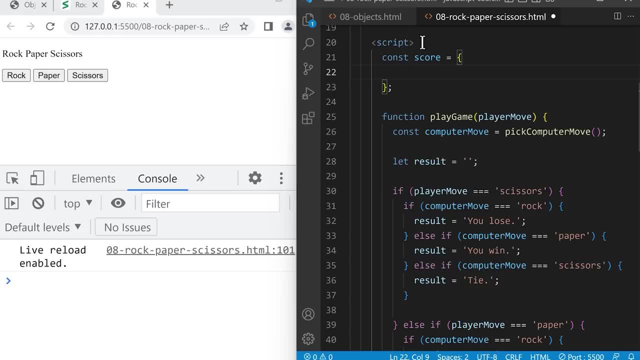 And inside this object we're going to have the property wins. So this will keep track of how many wins that we have. We'll type colon and the number zero, because the score starts at zero, and then a comma and then another property losses. 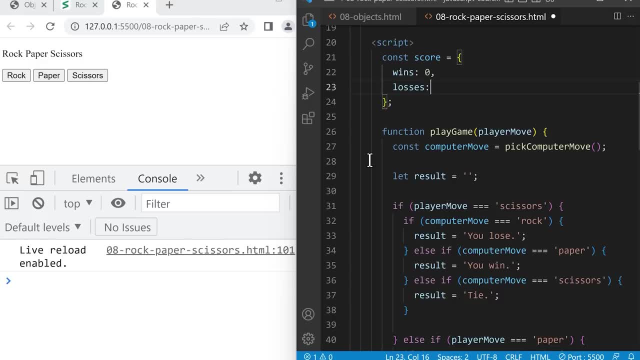 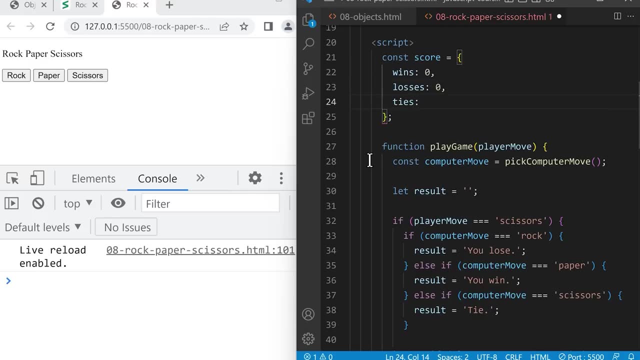 This will be how many losses we have. and then colon and zero, and then another comma and ties colon and zero. So we use an object here because these values are related to each other. You could use separate variables, but we're using an object for convenience. 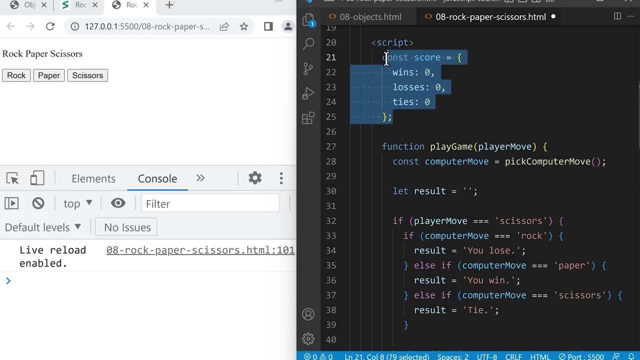 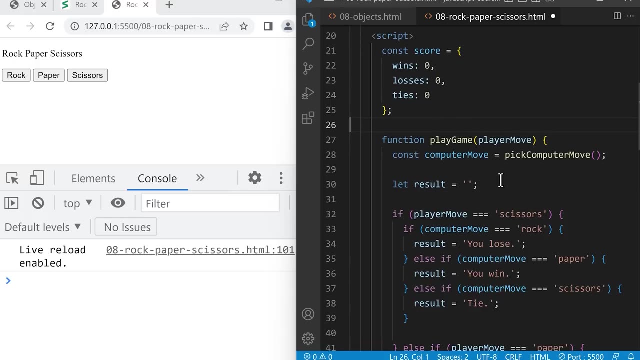 Another thing you'll notice is that we're creating this variable outside of a function and outside of a scope, And that's because every time we make a move, we need to update the score from last time. So, in order to save the score, 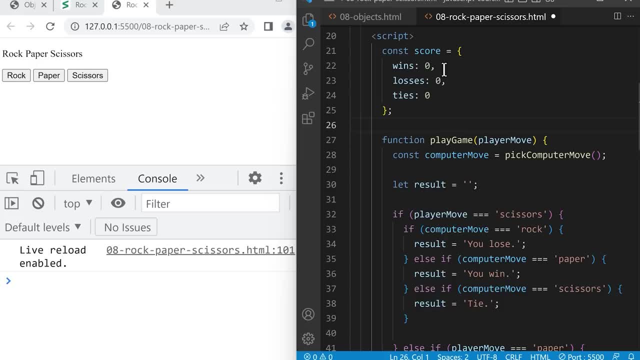 we're going to update the score from last time. We need to keep it outside the function. If the score was inside the function, the function would create a new score every time, which is not what we want. So, in this situation, in order to save a score from last time, 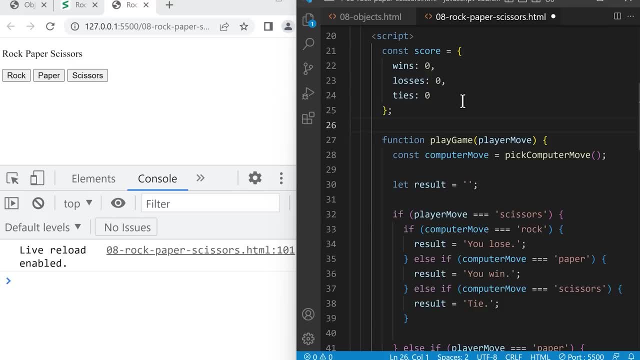 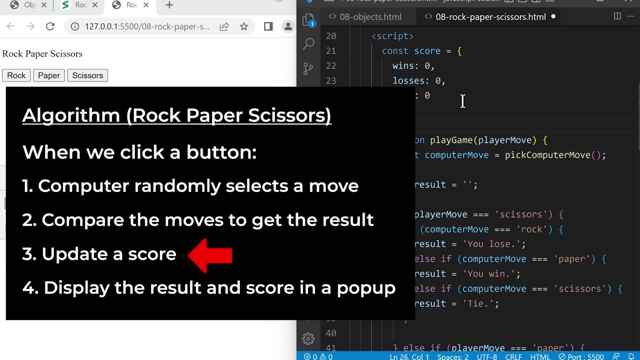 we're going to keep this variable outside. Now, every time we play the game after we calculate the result, we're going to update the score, So let's go ahead and do that. So let's scroll down to where we calculate the result. 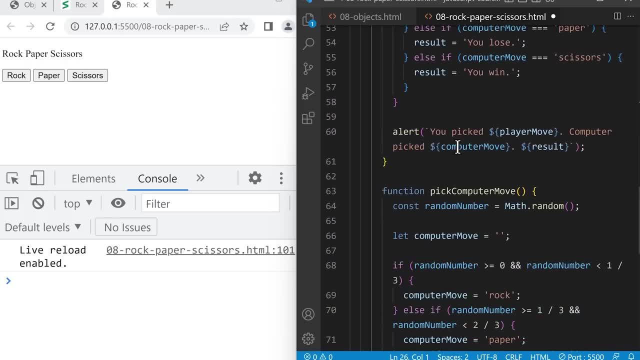 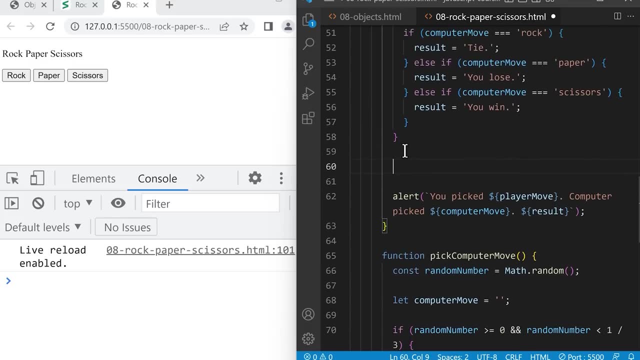 which is here And then below it we're going to type some new lines and type the code for updating the score. So we can do that with an if statement. So we'll type if brackets and curly brackets And inside the condition. 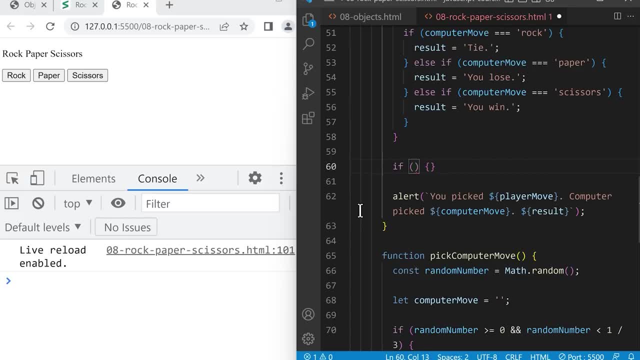 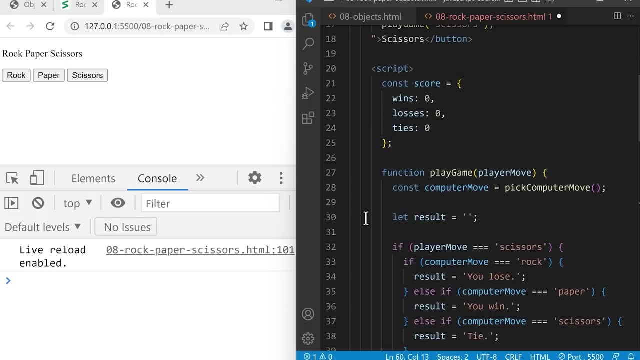 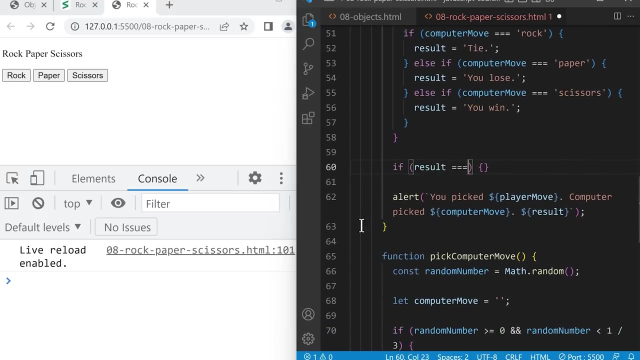 we're going to check if the result is a win. If it is a win, we're going to update the wins property and increase it by one. So, down here, if the result is equal to the string, you win and make sure that this string. 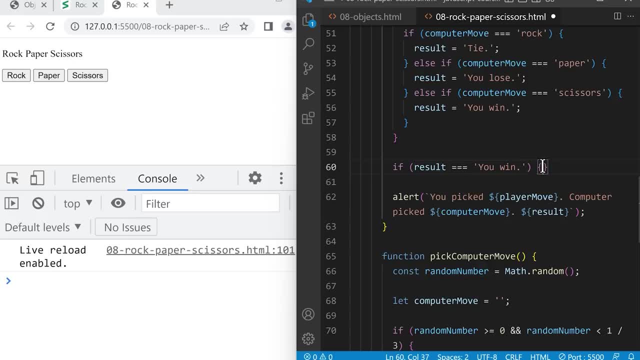 matches the string up here inside the curly brackets. we're going to update scorewins And we'll make it equal to itself plus one. So this is how we increase the wins property in the score object by one. Now remember from the variables lesson: 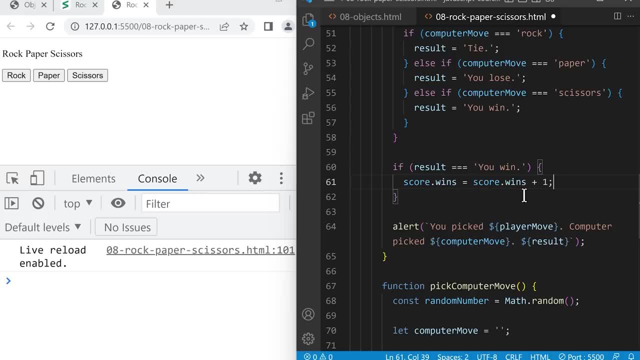 that we have a shortcut for increasing something by one, And that shortcut is: plus equals one. Next, let's add another branch to this. if statement for the other two results, So else if brackets and curly brackets. And in the second condition we're going to check if 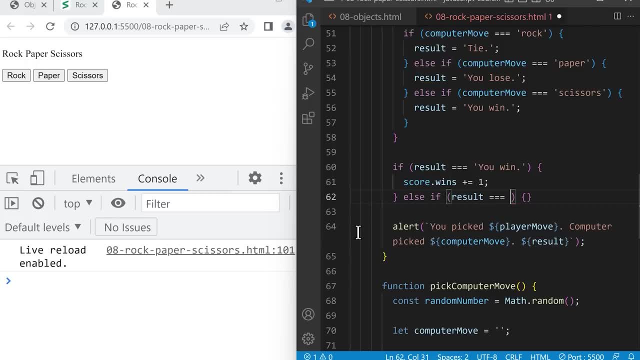 result is equal to the string you lose And make sure this string matches the string up here. So if the result is you lose, we're going to update scorelosses property and increase it by one. So plus equals one. And finally, 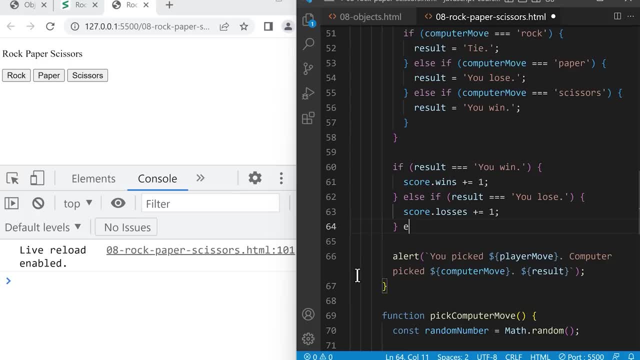 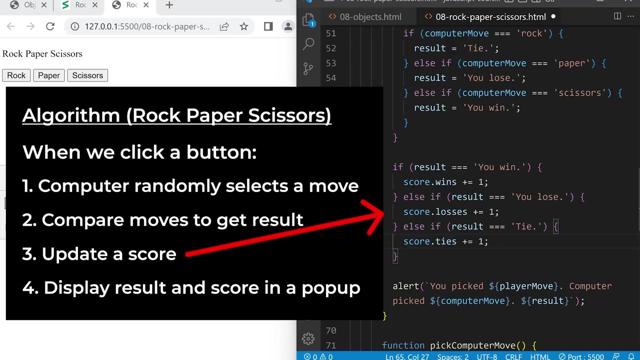 we'll check if the result is a tie. Else, if brackets and curly brackets result equals to the string tie And here we'll update score. dot ties plus equals one. So we converted this step in the algorithm to code. The score starts at zero. 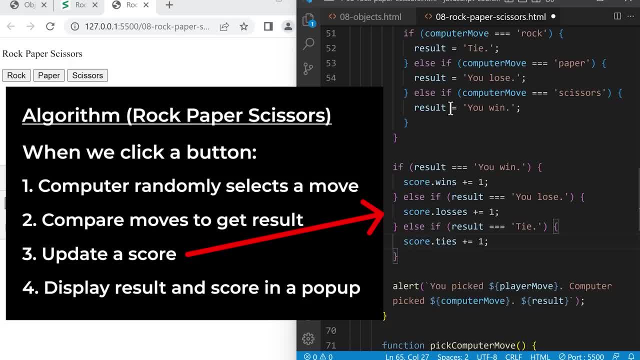 And every time we play the game, after we calculate the result, we're going to update the score using this code. Now let's convert the last step into code. We're going to display the result and the score in the pop-up at the end. 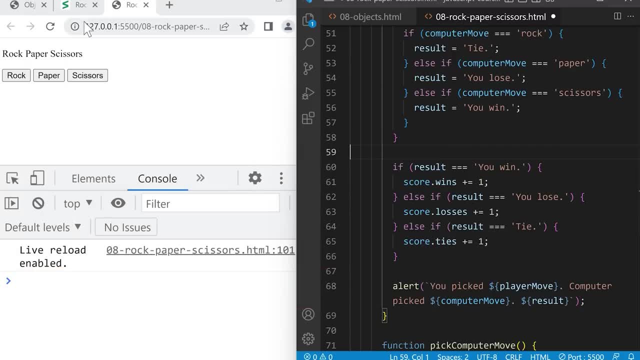 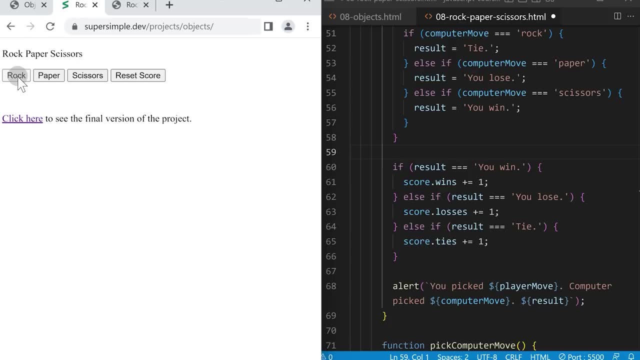 So let's actually go back to the supersimpledev project and we'll see what the pop-up looks like. We'll click one of these buttons and in this pop-up, on the second line, we display the score. So in our code, 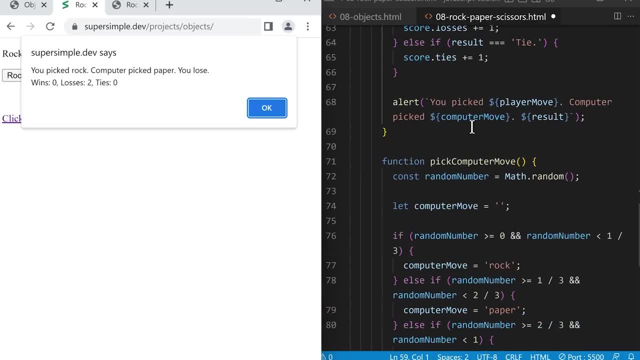 this is the code that displays that pop-up. So how do we add a second line to the pop-up? Remember that template strings have another special feature called multi-line strings, So we can type at the end of this template string and press enter to add another line. 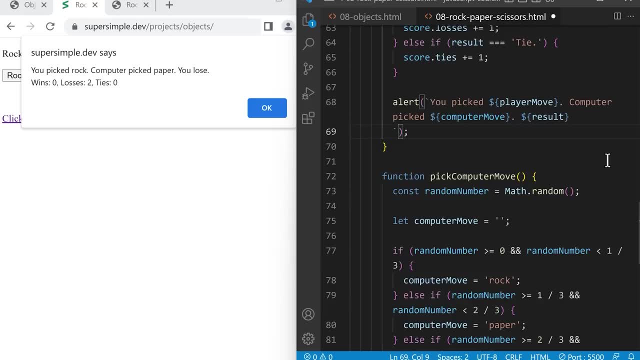 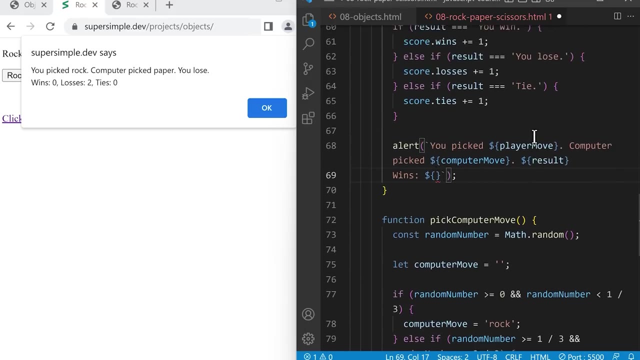 to this string. So here we can type wins colon, and we're going to insert a value using dollar: open curly bracket. close curly bracket. and here we're going to insert the number of wins that we have, which is score, dot wins. So we'll type: 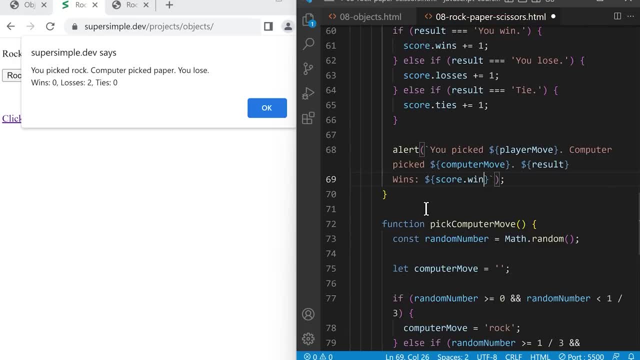 score dot wins. Next we're going to show the number of losses that we have. So after this let's type a comma and losses colon and insert another value. Here we'll insert score dot losses and finally we'll type a comma. 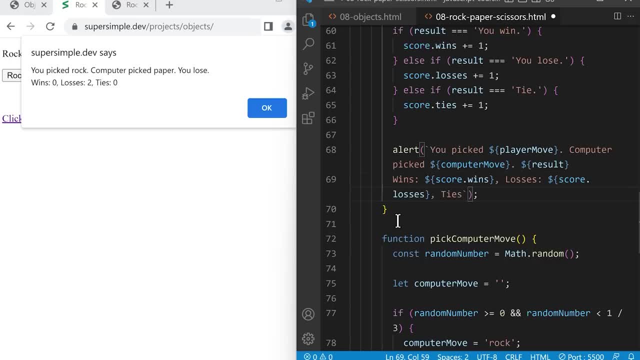 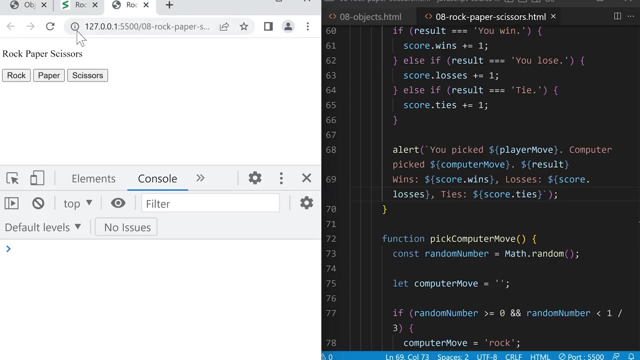 and we'll display ties colon and insert a value, score dot ties- And this will display our score in the pop-up. So let's save this and give it a try. We'll click OK and then go back to our tab and play the game. 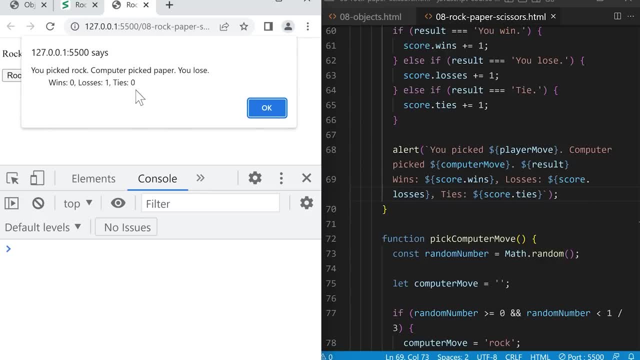 So now on the second line, we will display the score. One small issue here is that we have a lot of spaces on the second line, So these spaces correspond to the spaces here. When we use multi-line strings, these extra spaces will show up. 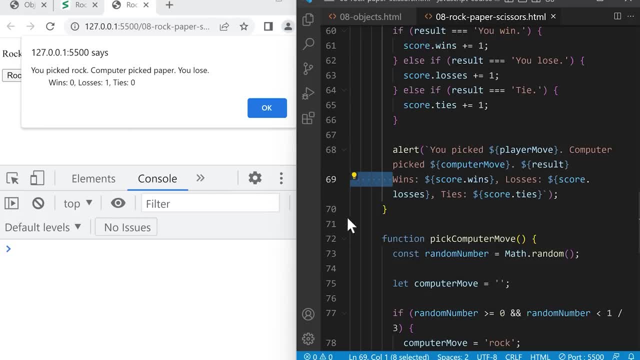 in the pop-up. So to remove these spaces, we can just remove them in the code like this: Now, if we save, press OK and play the game, it will show our score on the second line without those extra spaces at the front. 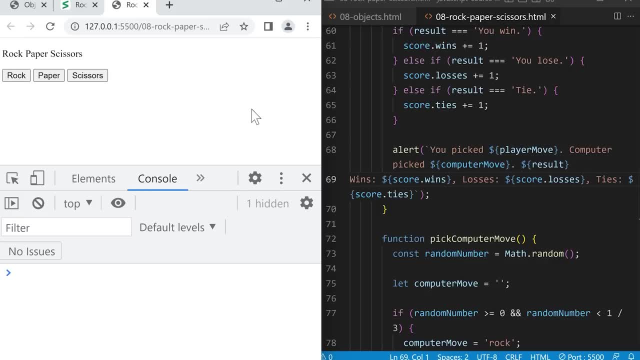 Let's press OK. We're going to add one more feature to this project. If we go back to supersimple dot dev, we have a reset score button which will reset the score back to zero when we click it. Let's add this button. 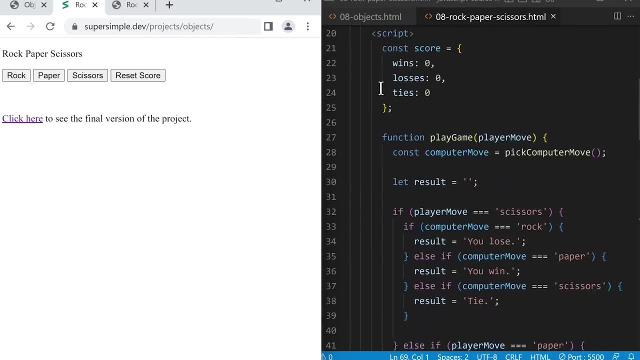 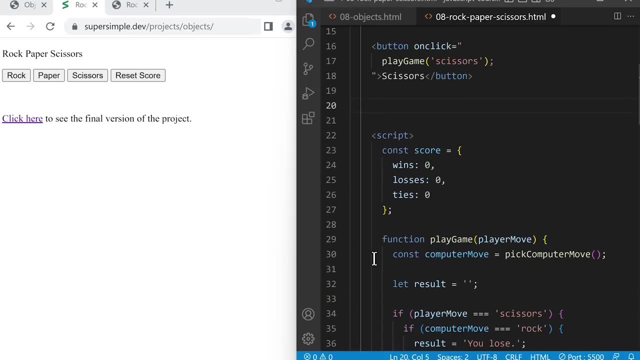 in our project. So we'll scroll up and inside the HTML we'll add a button with the code less than, button greater than, And inside the button we'll have the text reset score. And now, when we click this button, we'll run. 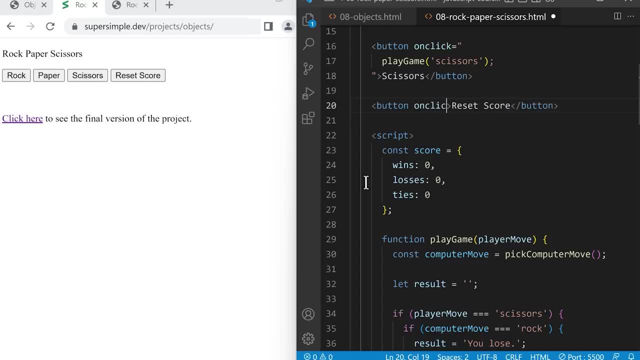 some code using the onClick attribute equals double quotes, and then in here we're going to write some code to reset this score back to zero. So one way we can do it is because this score is an object. we can use dot notation to change. 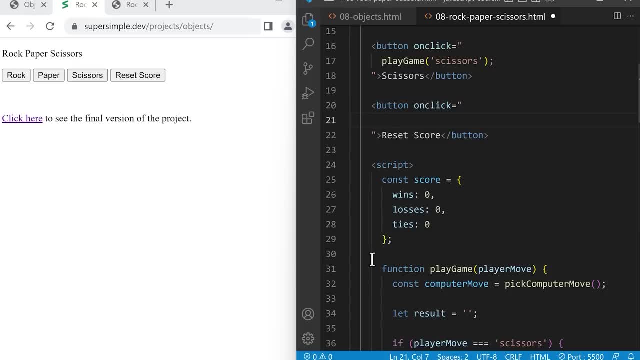 everything back to zero. So we can type score dot wins and make it equal to zero. We'll also type score dot losses and make it equal to zero, And finally, score dot ties and make it equal to zero. Now let's save and go. 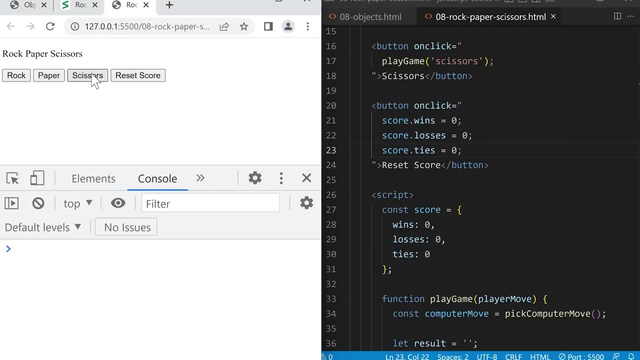 back to our tab and play the game a few times To get a score. let's press OK and press reset score and then play the game again And you'll notice that the score started from zero again. So that's how we create the reset. 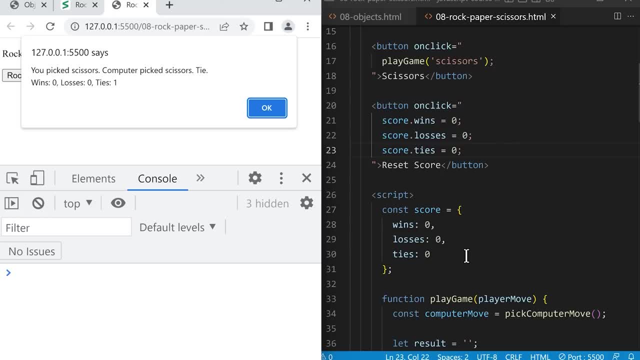 score button. We just set all of these properties back to zero And that's it. Now let's add a score feature to our rock paper scissors project using an object to save the score. Let's press OK and we're going to learn more. 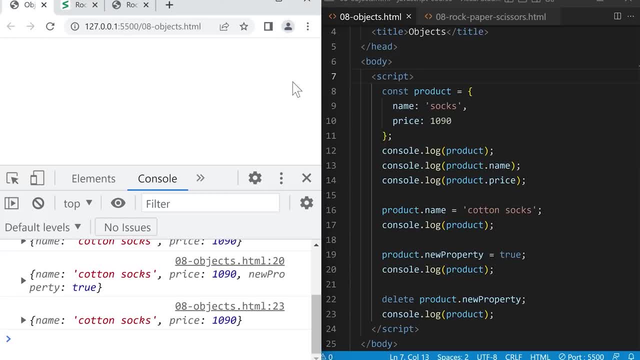 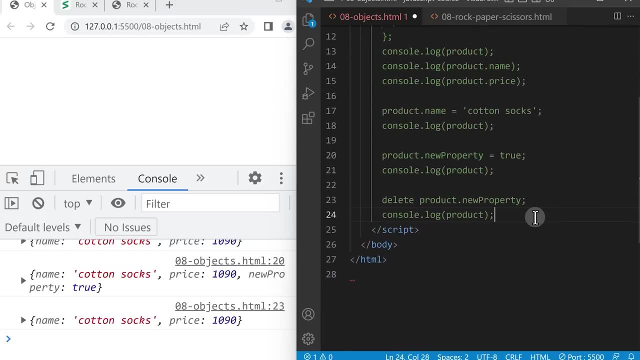 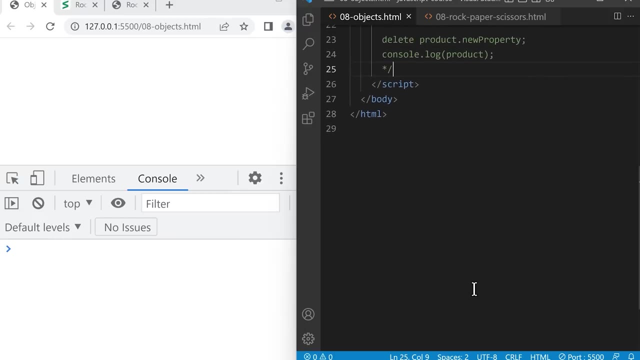 details about objects. Let's go back to objects, dot html, and at the bottom star slash and save. Now let's scroll to the bottom and we'll do some setup. So first let's create a variable with const. we'll name it product to and make. 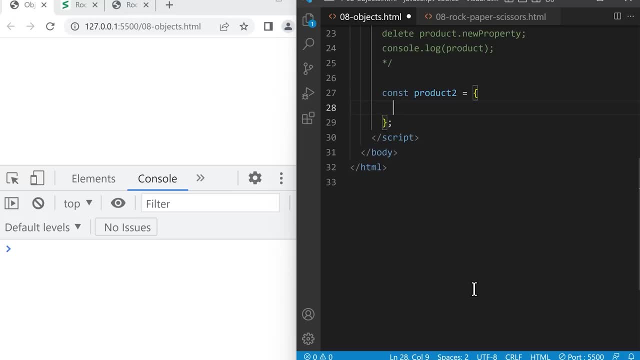 it equal to another object, Inside colon and the string shirt and we're going to console dot log this object. So console dot log product to and save. So the next detail we're going to learn about objects is another way to access values, For example. 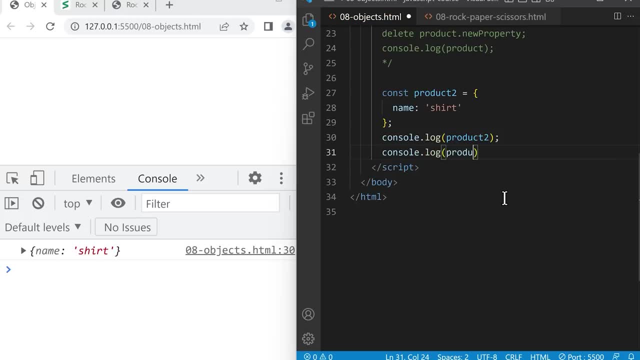 console dot log product to dot name. This will access the value associated with the name property. In JavaScript we have another way of accessing values inside objects, which is using square brackets. So console dot log product to, and this time we'll type square brackets. 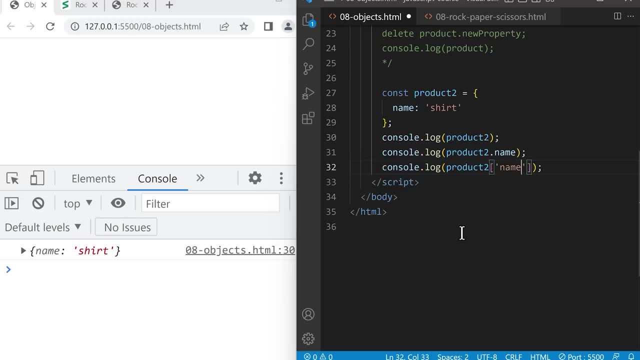 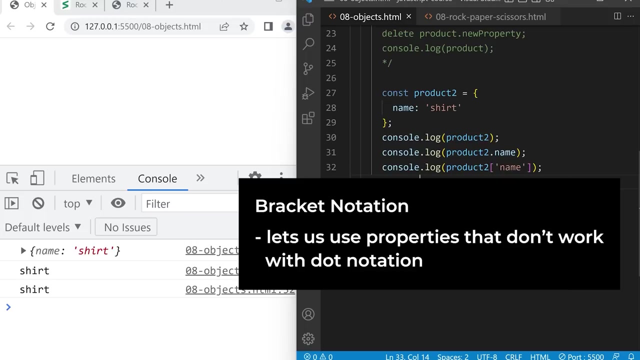 And then inside the square brackets, we'll have a string with name. So this is the name property. If we save these two lines of code, both access the string shirt which we see here. So when do we use the bracket notation instead of the values? 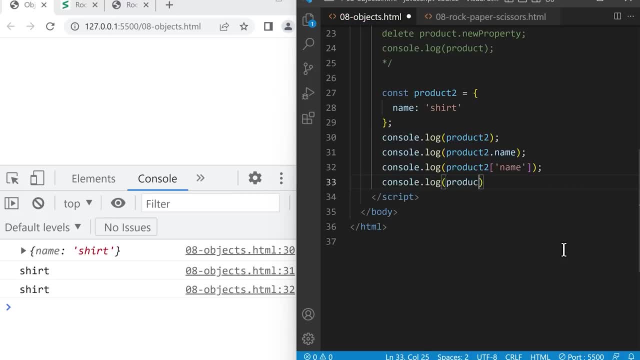 of product, and we do the same with the dot array. So we print this data and it is a dot and we also have the dot, and So in order to use a property like this, we have to use bracket notation. So we're going to replace the dot with square brackets and turn this into a string. 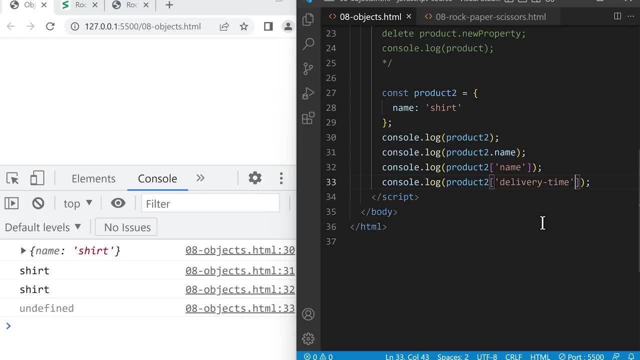 Now, if we save, it no longer gives us an error And because delivery time does not exist in the object, we get the value undefined. So using bracket notation, we can also add values to the object when we create it. So here we can add a comma and we'll add another property using bracket notation and 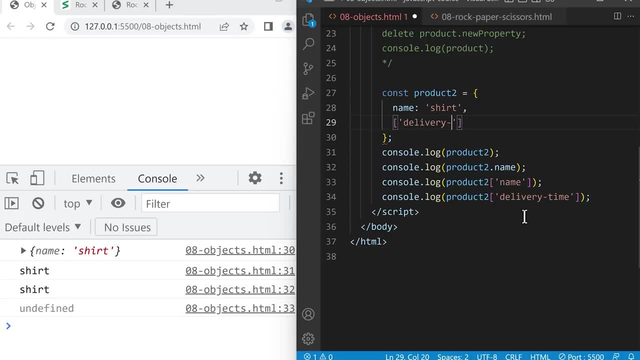 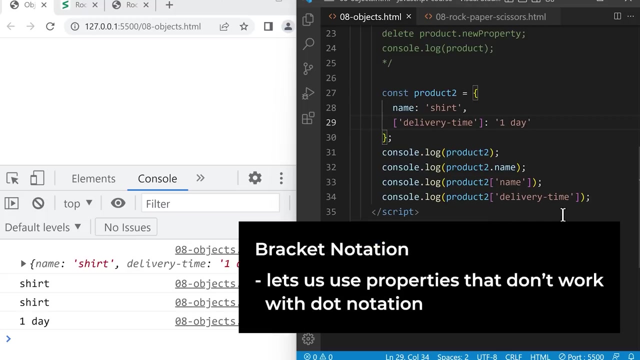 a String frm Delivery – time And a colon frm, Delivery frm, and then a value like the string: one day, If we save this, lets us add a delivery dash time property to this object. So, as you can see, bracket notation, lets us use properties that. 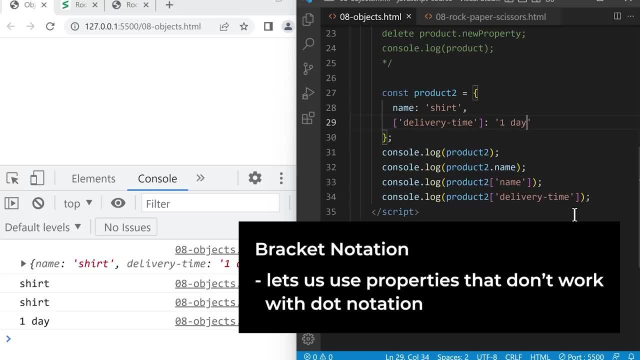 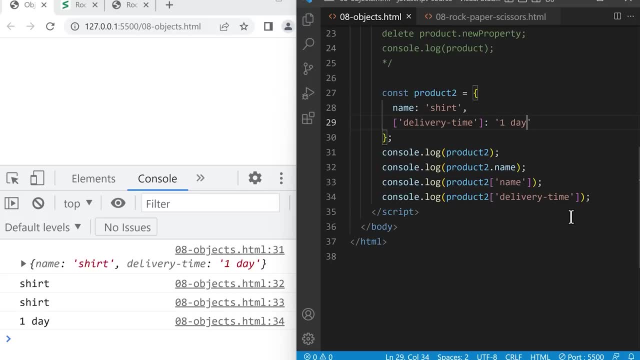 normally don't work with dot notation. Another feature of bracket notation is that between the brackets we don't just have to use a string, We can use a variable, a calculation or anything that results in a value. So you might be wondering which one should we use: dot notation or bracket. 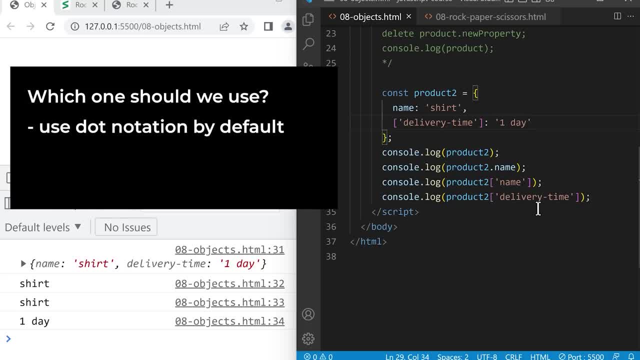 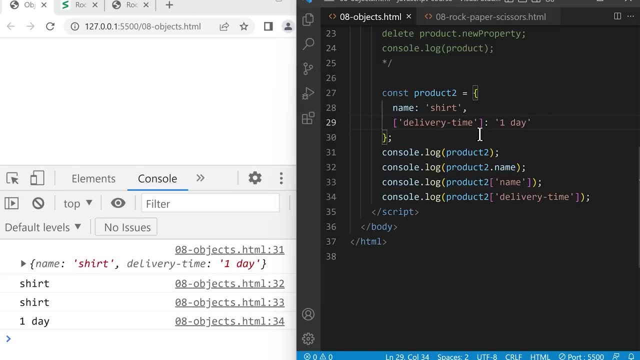 notation. We usually use dot notation by default because it's shorter and easier to read, But if we need to use properties that don't work with dot notation, then we use bracket notation. Now, a shortcut here is when we create the object. if we only have a string between the 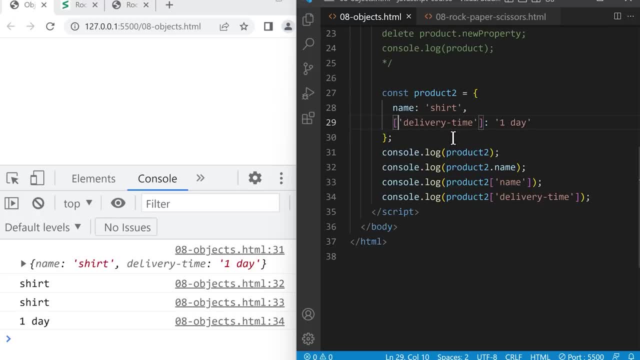 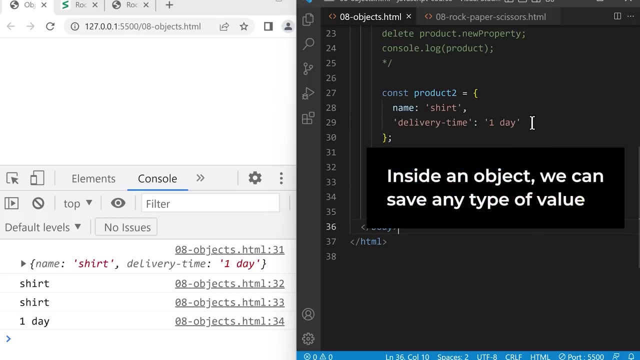 brackets. the brackets are actually optional, So we can just type this: If we save, the code will still work. Okay, the next detail we're going to learn is that inside an object, we can save any type of value. So this is what we're going to do. So we're going to save any type of value. So this: 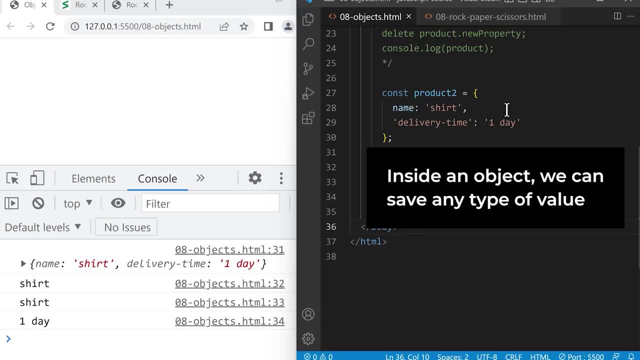 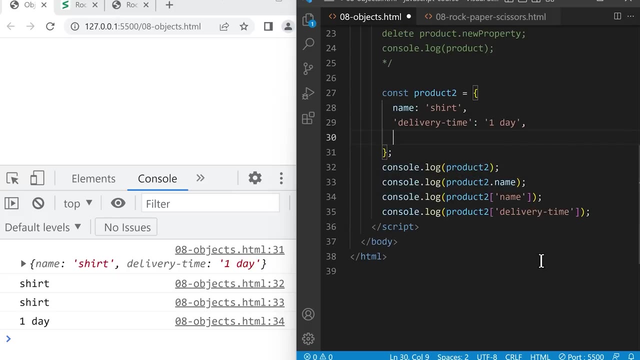 includes numbers, strings, booleans as well as other objects Because, remember, objects themselves are also values. For example, we can type a comma and add a property called rating colon and then an object: Open curly bracket. Close curly bracket. Inside this inner object, we 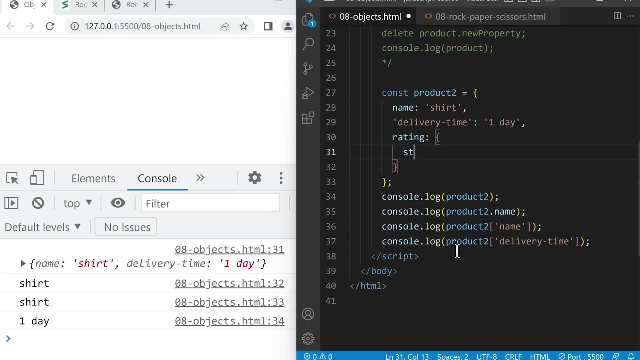 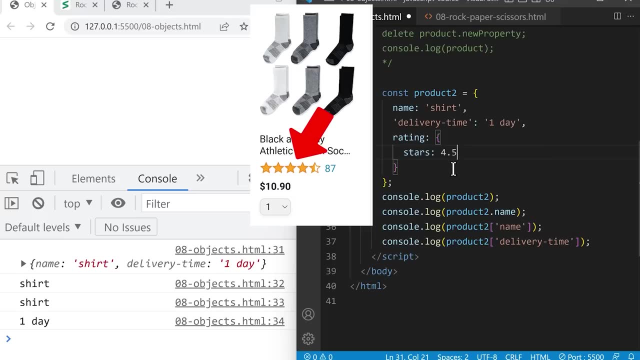 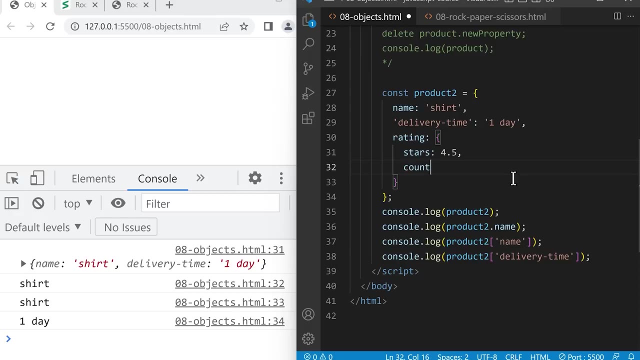 we can add more properties like stars, colon 4.5.. This is how many stars a product has, and then a comma and a property called count, colon 87.. This is how many ratings a product has. So this is called a nested object. 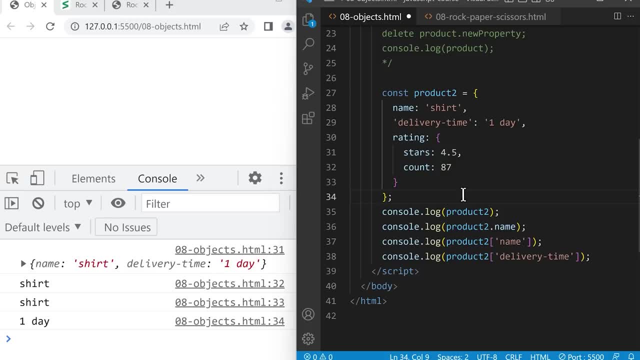 or an object inside an object. We can use nested objects to make our values more organized. So, inside the product, the number of stars that it has and the number of ratings that it has are both related to a rating, So it makes sense to group them together further. 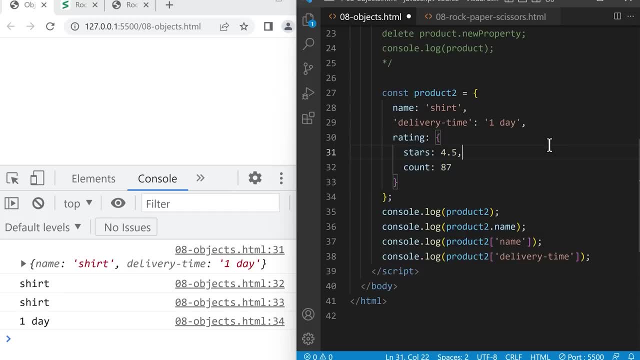 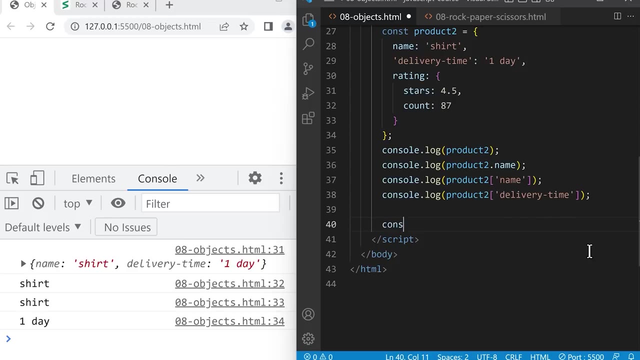 inside the product. Now, to access values inside the inner object, we just use the dot notation or bracket notation multiple times. For example, at the bottom we can type consolelogproduct2.rating. This will get the value associated with rating, and this is an object. 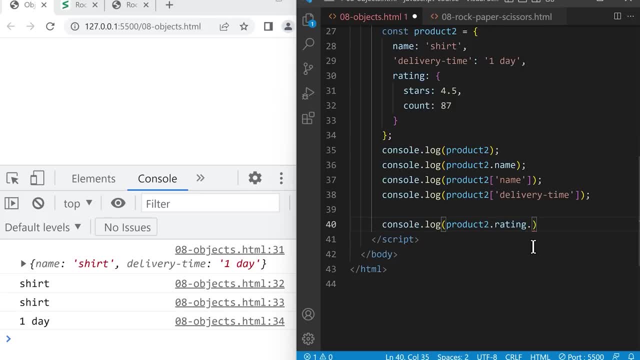 So we can use the dot notation notation again count. So this will get the count inside the rating object, which is this value right here. So if we save, it will display 87.. And finally, another type of value we can put in an: 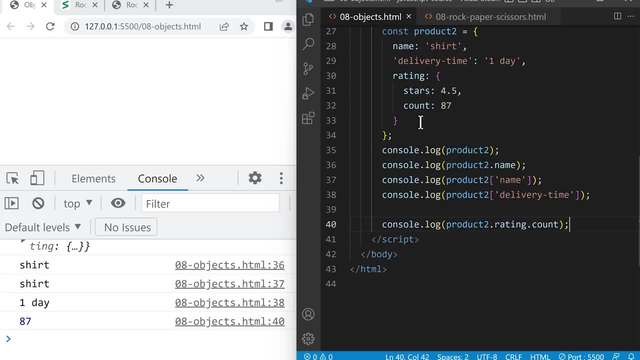 object is a function. So in this object let's type comma and another property, fun, colon, and we're going to create a function here. So let's type function and we'll name the function function one brackets and curly brackets, And then inside the function we're going to have some JavaScript. 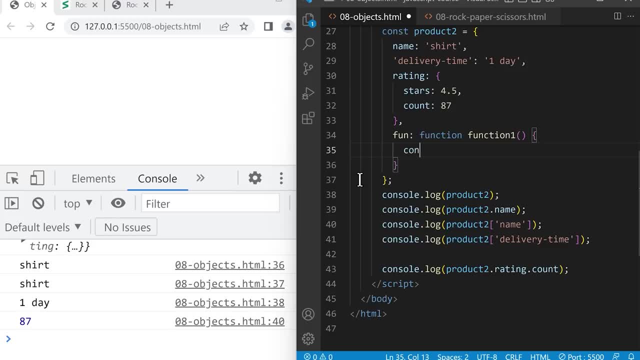 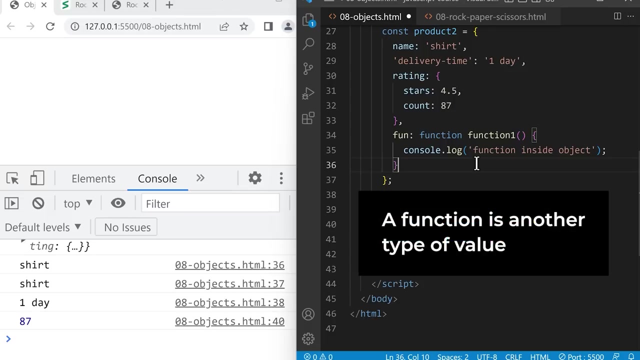 code Like usual. So consolelog: the string function inside object. This saves a function inside the object And this works because a function is actually just another type of value in JavaScript. But we'll learn more about this feature of functions later in this course. 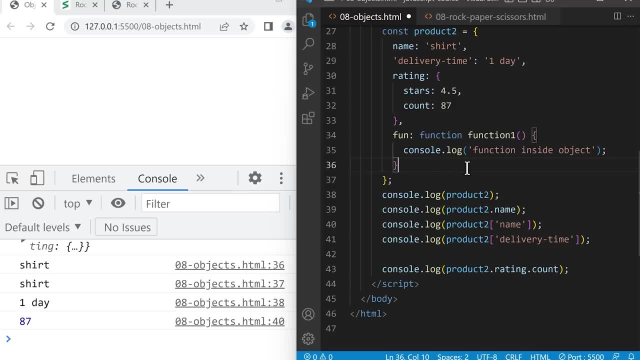 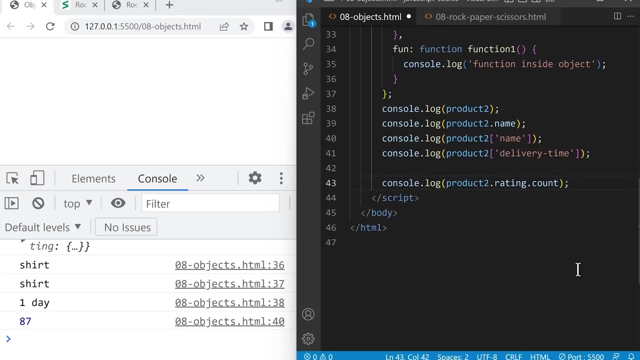 For now just know that functions are also values and we can save them in an object. To access this function we can use the dot or bracket notation as usual. So at the bottom we can type the object product two and then a dot and then the. 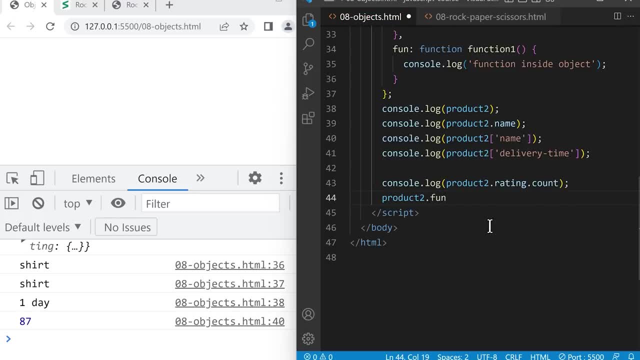 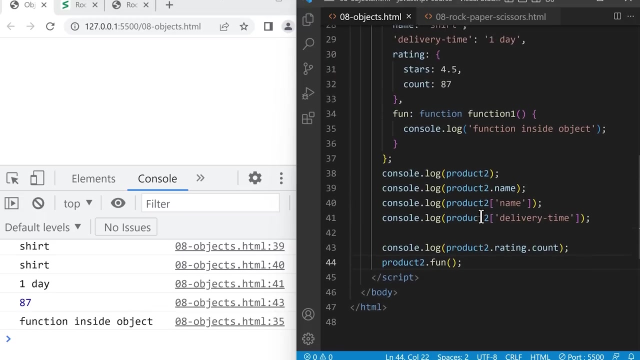 property fun associated with the fun property, which is a function, and because this is a function we can call it as usual, using brackets. if we save this will run the function here and it will display function inside object into the console. so when we save functions inside an object, this is called a method and we've 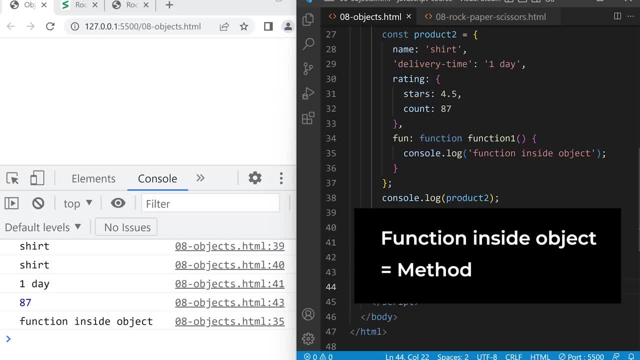 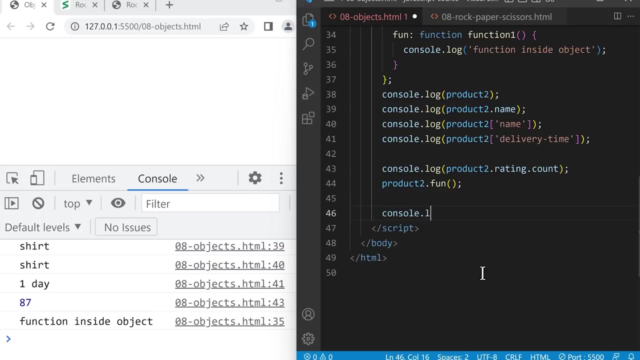 actually been using methods this whole time. console dog is actually a method. consul is an object provided by JavaScript and log is a function that is saved inside the console object. if we go to the bottom and type content: consolelog, type of console and save, this will confirm that console is just an object. 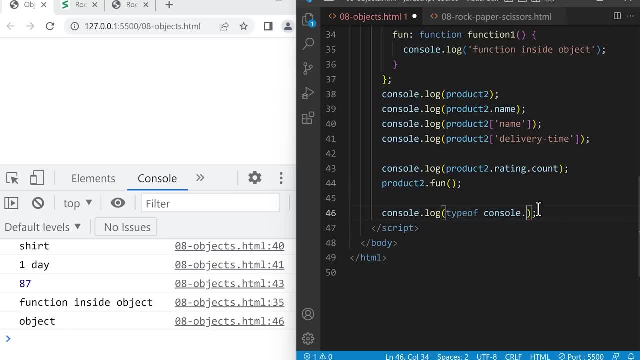 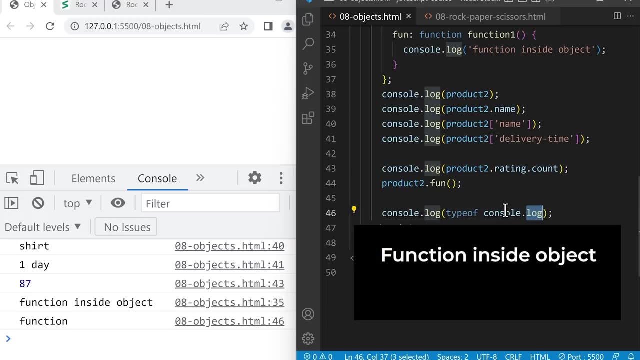 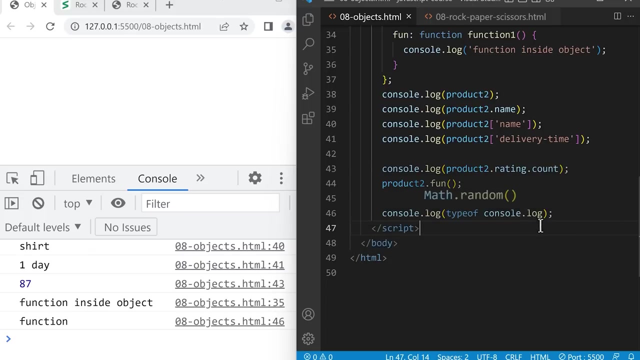 And if we change this to consolelog and save, this will show us that consolelog is a function. So log is a function that is saved inside the console object, So we call this a method. Another example of a method is mathrandom, which we used in the rock-paper-scissors project. 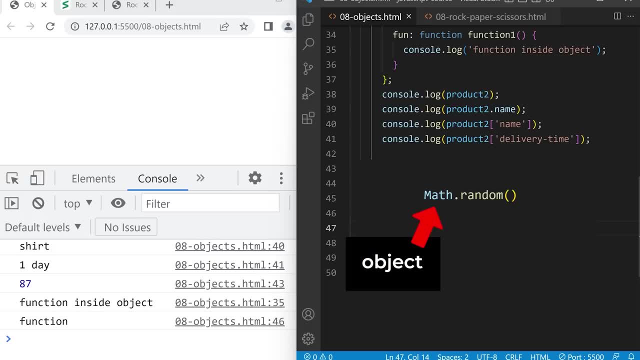 Math is also an object provided by JavaScript, and random is a function saved inside the math object, So we call mathrandom a method as well. So we've actually been using objects and methods all throughout this course, and now we understand all the code that we've been using so far. Next we're going to learn 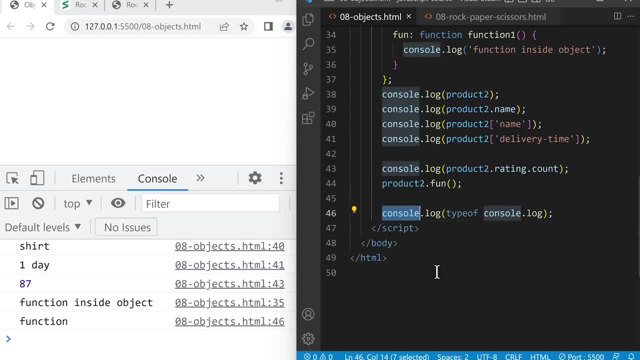 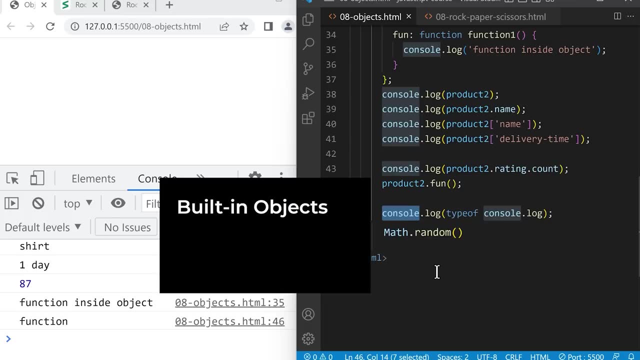 about built-in objects. So the console object and the math object are known as built-in objects because they are built into the language. They are provided by the language. We're going to learn about built-in objects and we're going to learn about built-in objects. 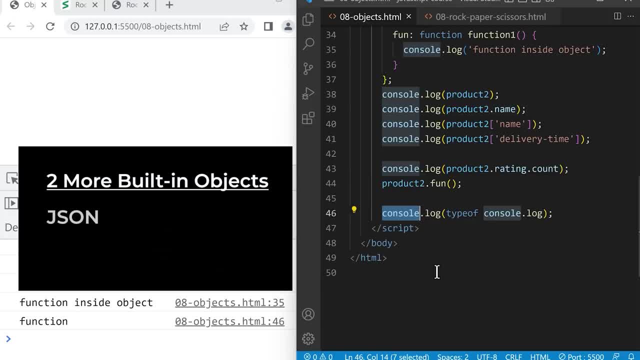 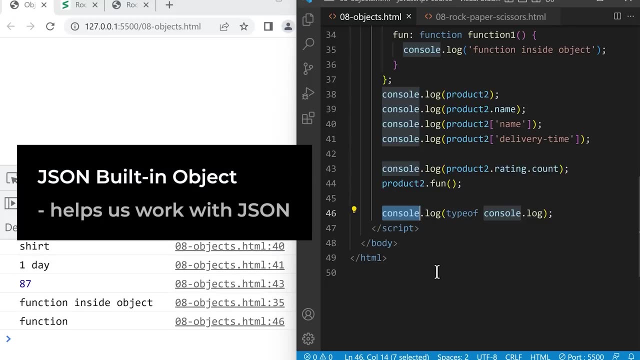 We're going to learn two more built-in objects called JSON and local storage, and we will use these objects to improve our rock-paper-scissors project. Let's start with the JSON built-in object. This object helps us work with something called JSON. JSON stands for 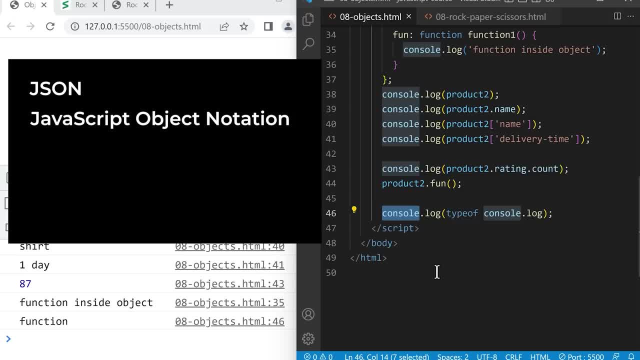 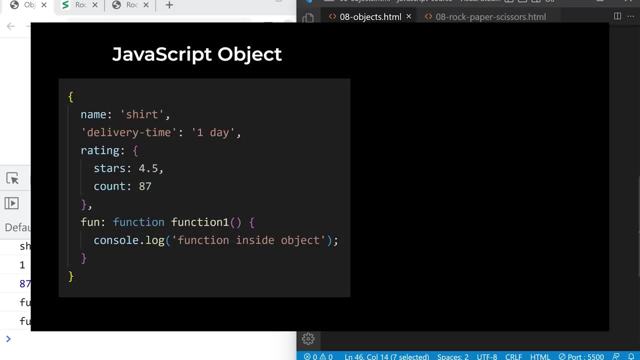 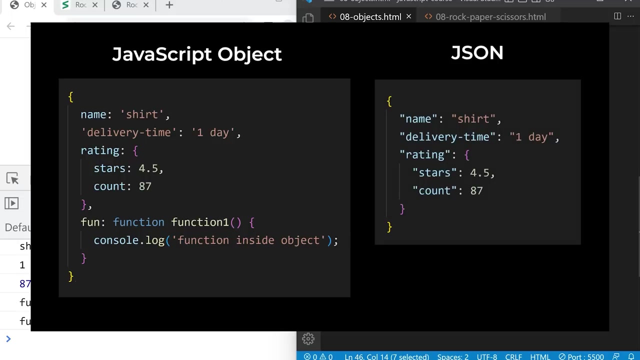 JavaScript Object Notation. The easiest way to understand JSON is it's basically a syntax. It's a similar syntax to a JavaScript object, but it has less features. For example, the code on the left uses JavaScript Object Syntax and the code on the right uses JSON. 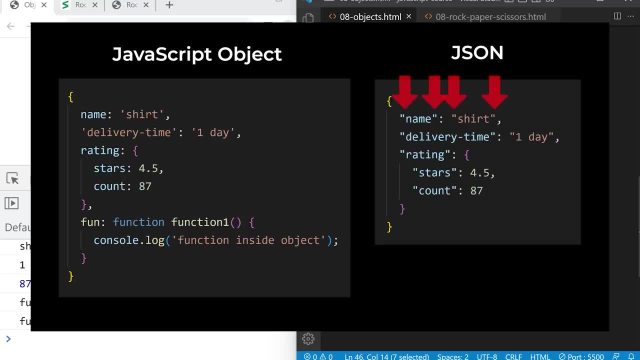 Syntax. So one difference is that all properties and strings must use double quotes in JSON. JSON does not support single quotes. Another difference is that all properties and strings must use added quotes. So one difference is that all properties and strings must use mia'ts. 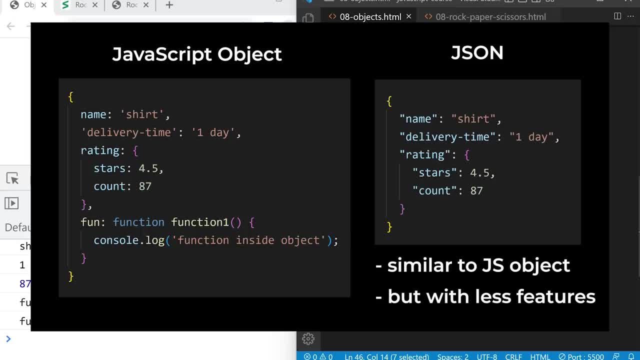 and the other difference is that JSON does not support functions. So, as you can see, JSON is basically a syntax that's similar to a JavaScript Object Syntax, but with less features. So why would we use JSON syntax instead of a JavaScript Object Syntax, A JavaScript 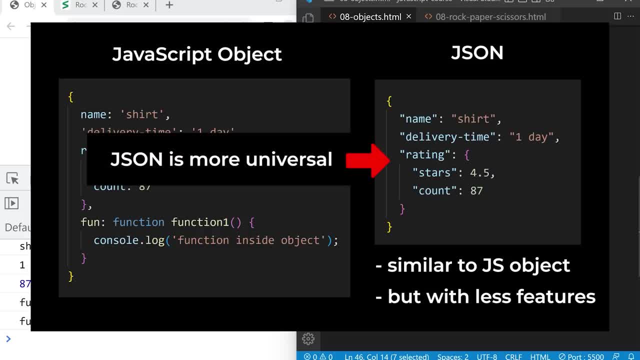 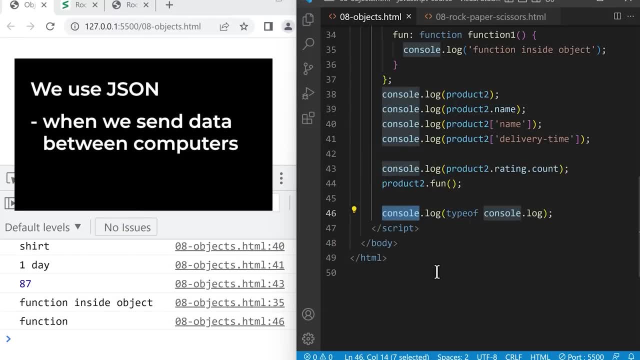 by almost every programming language, So JSON syntax is more universal. For this reason, we use JSON when we send data between two computers that might use different programming languages. We'll learn how to do this later in the course. We also use JSON when we store data. We'll learn how to store data in this lesson. 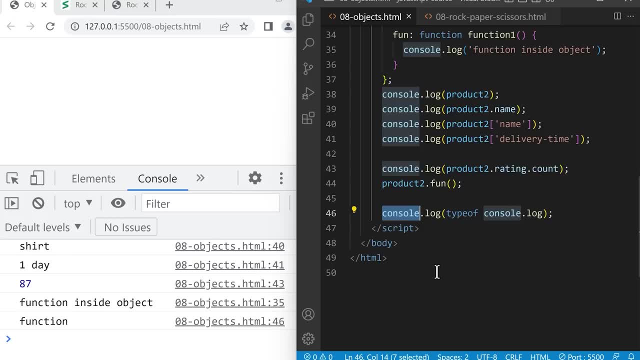 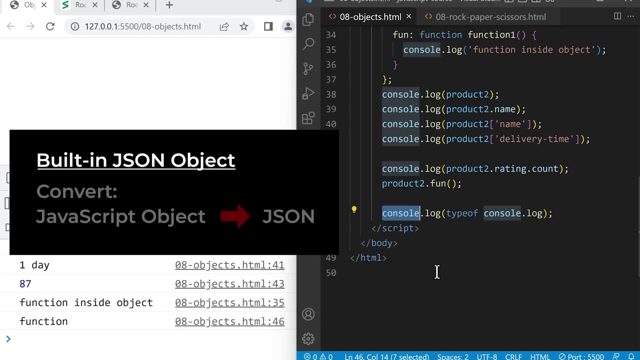 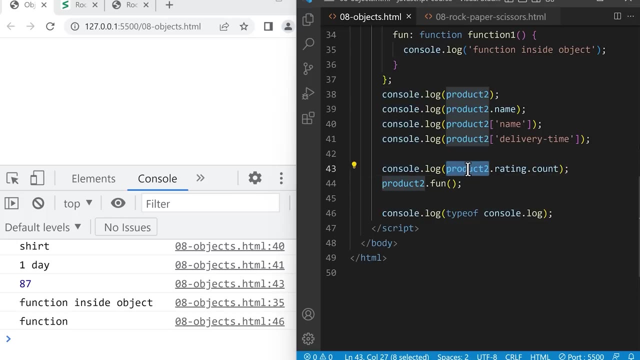 Now that we understand what JSON is, let's learn about the built-in JSON object. The JSON object helps us convert a JavaScript object to JSON. For example, let's convert our object product2 to JSON. So we'll create some new lines and we'll type the JSON object dot stringify. 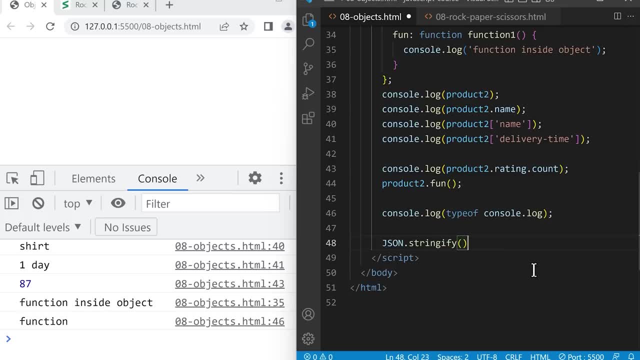 And open bracket, close bracket. So stringify is a method of the JSON object, So it's a function that is saved inside this object And we can call this function using brackets. Between the brackets we can give it a JavaScript object we want to convert. 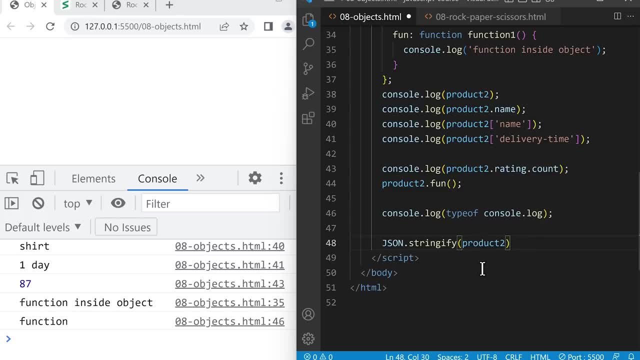 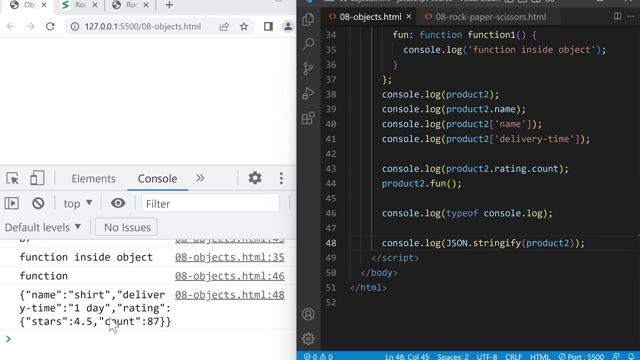 Like product2.. This will convert the object into JSON. So now let's console dot, log the result And save, And in the console it will display the product using JSON syntax. If we scroll up, you'll notice that the function that we saved in the object 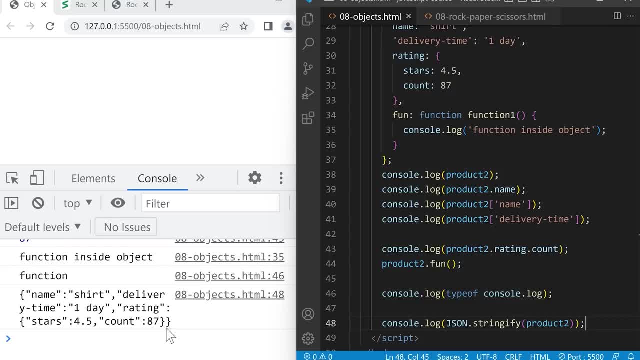 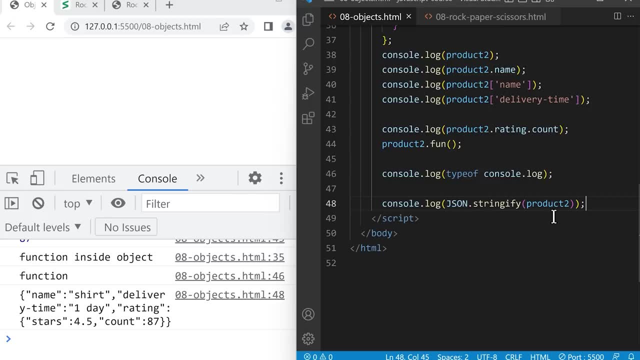 is not inside the JSON, And that's because JSON does not support functions. Now let's go ahead and convert our string to JSON. So one thing to note about stringify is that it actually results in a string. So at the front, if we type type of and save, it will tell us that the result that it gives is actually. 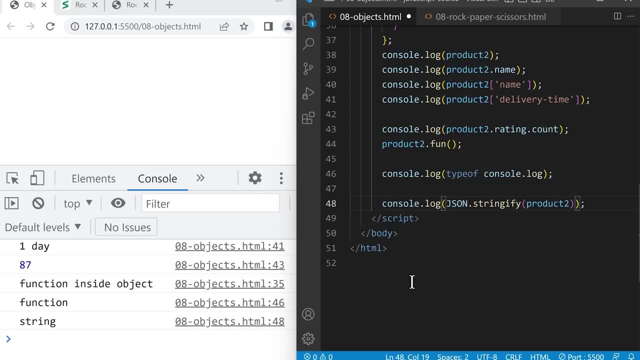 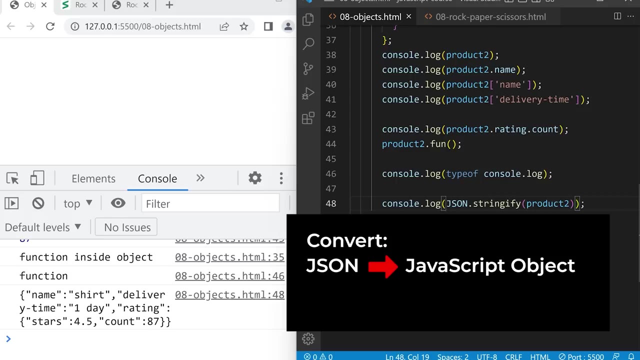 a string. So if we remove this and save now, this JSON string is ready to be sent to the client, to another computer or to be saved in storage. Next let's learn how to convert the other way, from a JSON back to a JavaScript object. 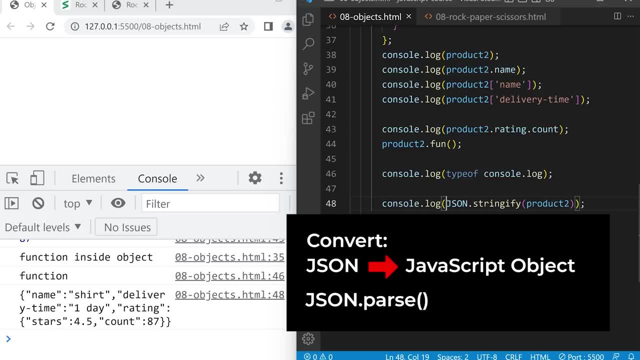 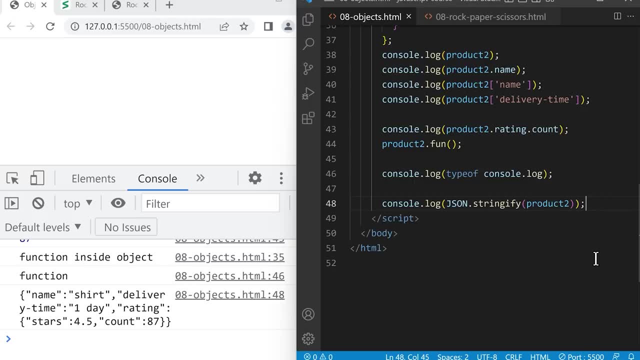 To do that we'll use another method in the built-in JSON object called JSONPars. At the end we'll type JSONPars and brackets, And between the brackets we can put a JSON string that we want to convert. 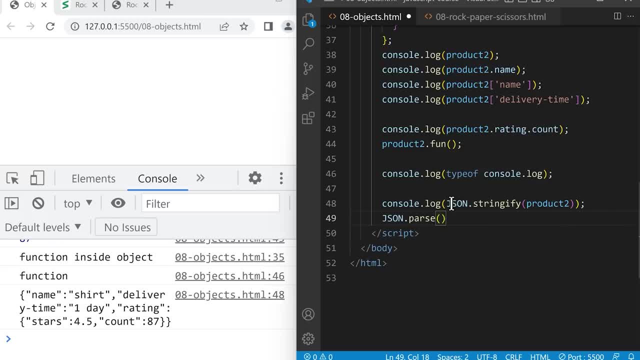 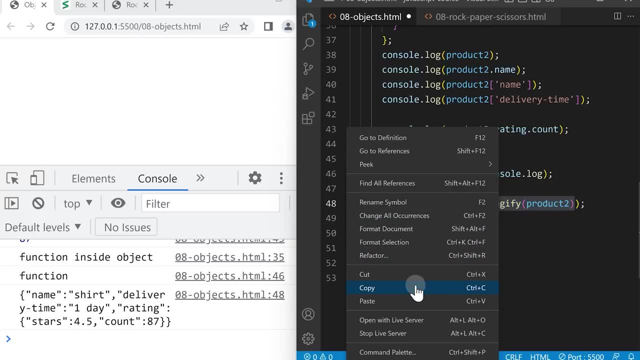 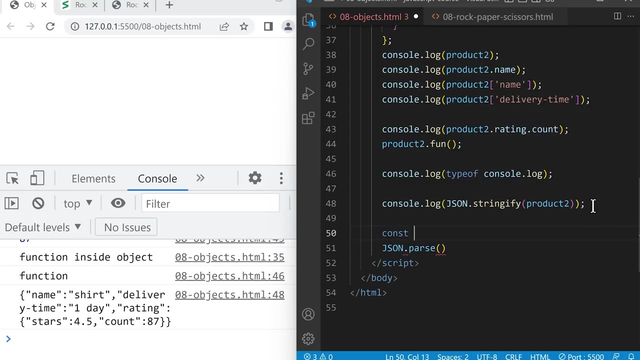 So we actually have a JSON string up here, So let's just make a copy of this. We'll select it, right-click copy and let's create an extra variable to make it more clear const JSONString and make it equal to right-click and paste. 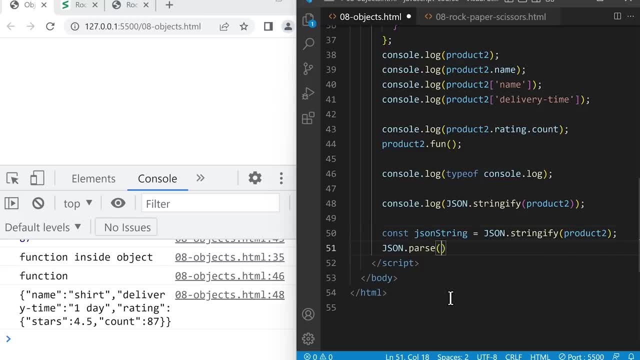 And now let's convert this JSON string back into an object by putting it into Pars And finally we'll consolelog this result. So consolelog And save, And JSONPars will turn the JSON string back into a JavaScript object. 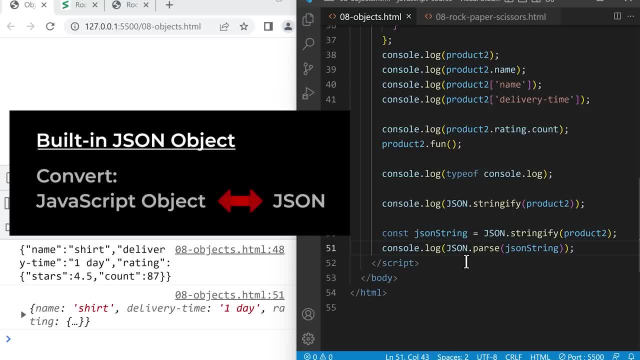 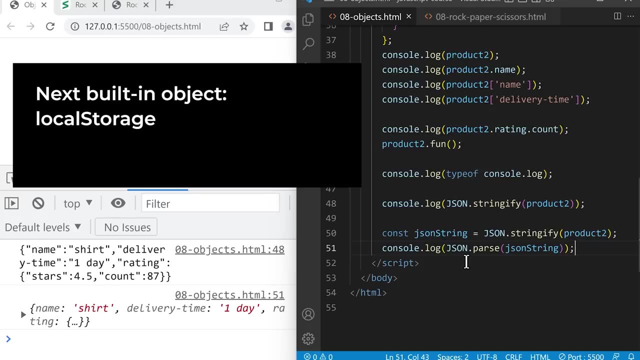 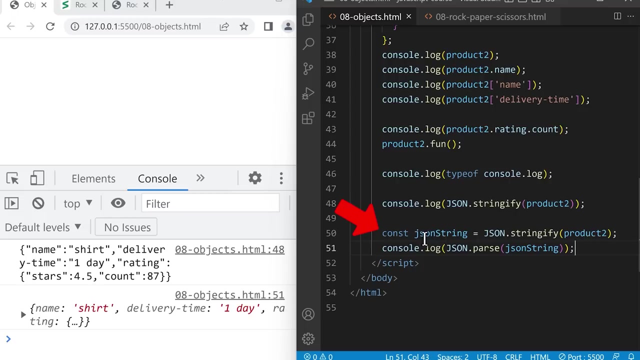 So that's the built-in JSON object. It helps us convert back and forth between a JavaScript object and JSON. Now we're going to learn the next built-in object, called local storage. Local storage is used to save values more permanently. So far, we've been saving our values in variables. 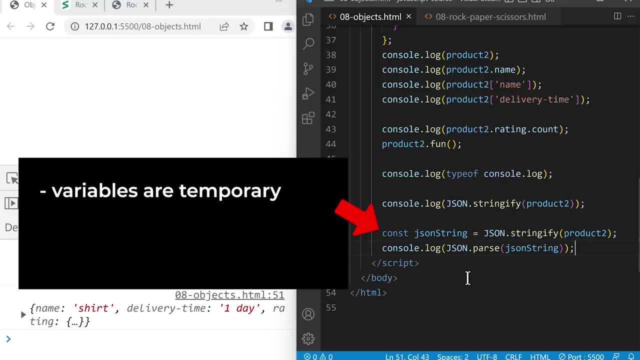 However, variables are temporary. They only exist on the current page. If we refresh the page or close the page, all the variables are deleted. For example, if we go back to our rock-paper-scissors project And open the text editor. 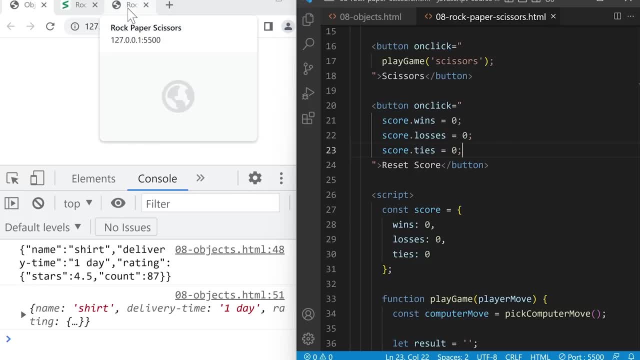 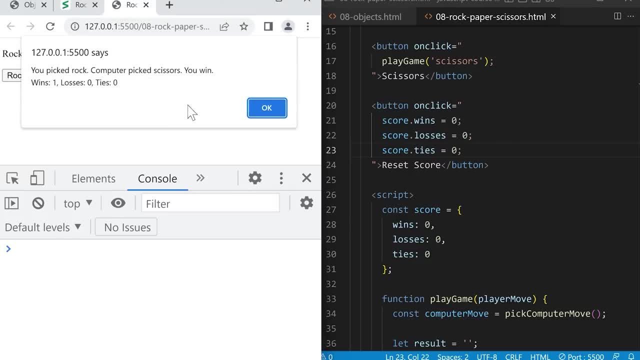 But we can see that we've already saved our values. So let's open the tab for this project And we play a few games And play it again. So we have two games And we refresh the page. Notice the score starts from 0 again. 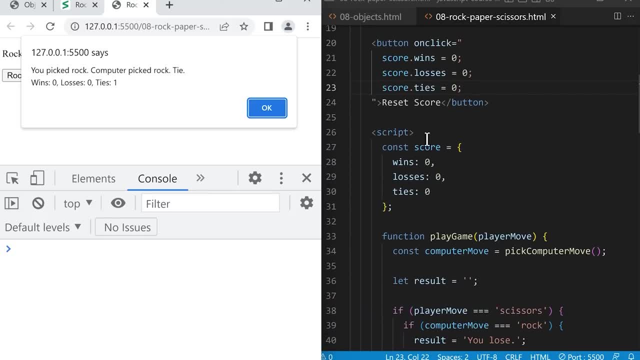 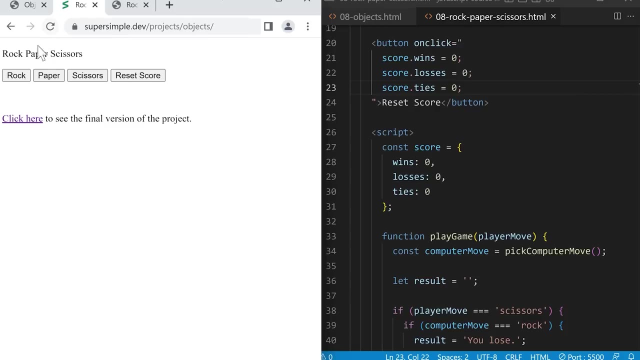 And that's because when we refresh the page, all of these variables are deleted And the score gets reset back to zero. If we press OK and go to supersimpledev and we refresh the page and we play the game, notice that the score doesn't start from 0. 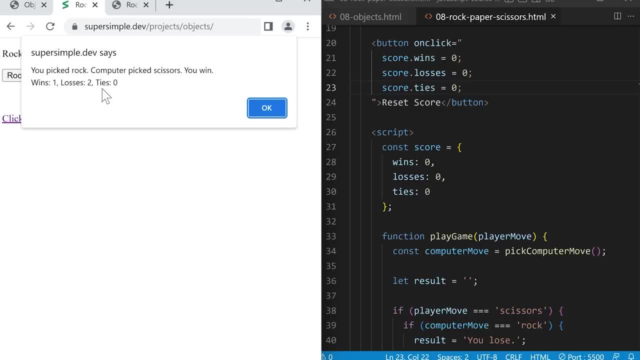 It starts from the previous score, even though we refreshed the page, And that's because this project saves the score in local storage And local storage doesn't get deleted when we refresh the page. Now let's learn how to use local storage in our project. 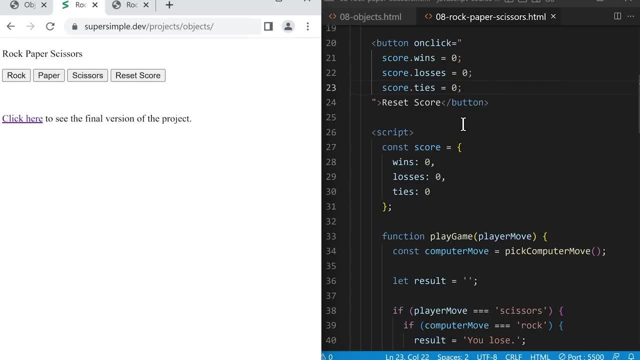 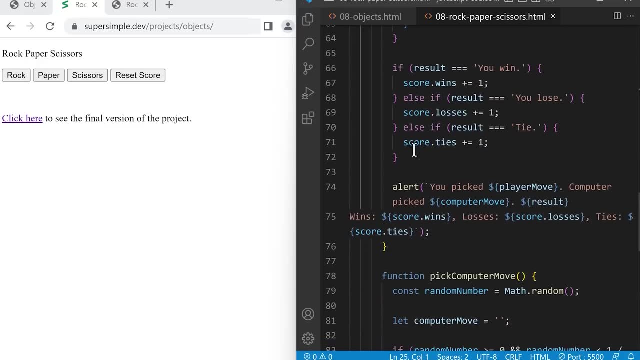 Let's press OK and we'll go back to our code and we'll scroll down to where we update the score. So here, after we update the score, we're going to save it in local storage. But first let's learn how local storage works. 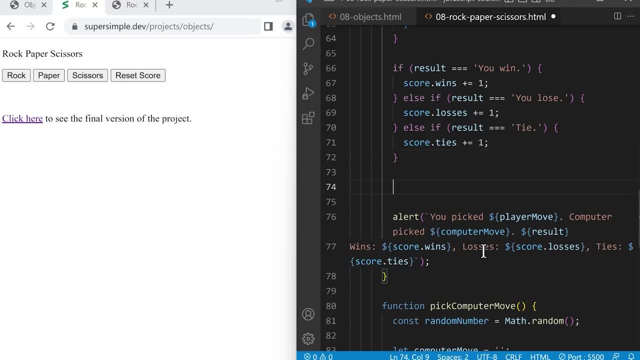 So at the bottom here we're going to type the local capital S storage object To save a value inside local storage. it has a method called setItem, So we can type dot, set, capital I, item and brackets because this is a method or a function saved inside the object. 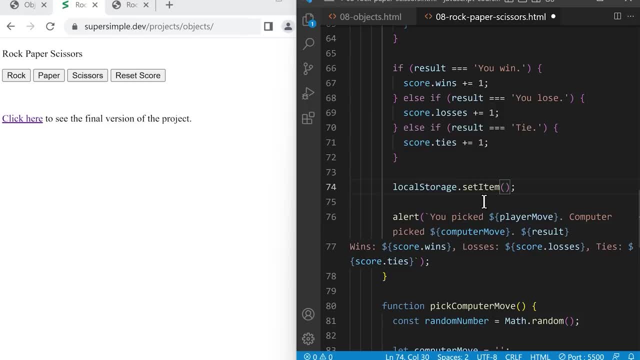 And we're going to give two strings to this. The first string is a name. This is how we're going to access the value that we save later, So let's use the string message as the name And we'll type a comma. 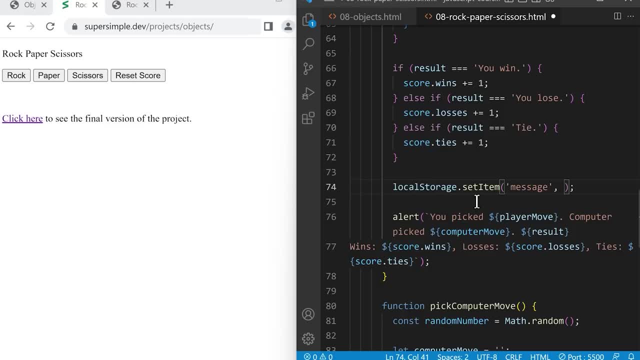 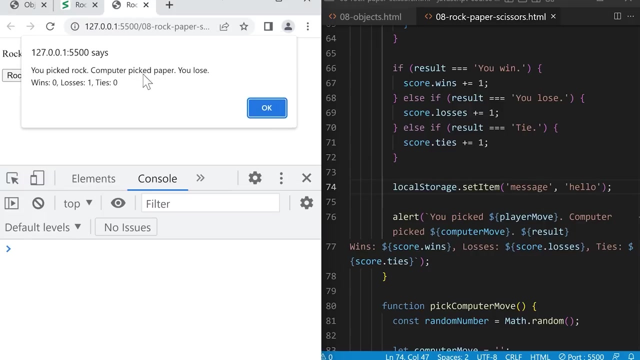 And then we'll type the value that we want to save into local storage. So local storage only supports strings. So let's save the string hello. So inside local storage. if we save and then go back to our tab and play the game, it will. 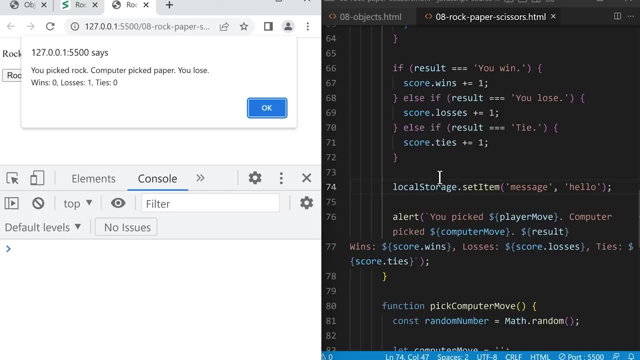 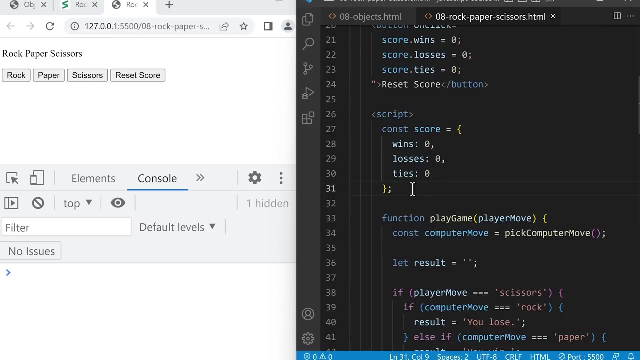 run all this code and save this string into local storage. Now let's learn how to get this string out of local storage. We'll press OK And we'll scroll to the top, And when we first load the page, We're going to get that value out of local storage by typing. 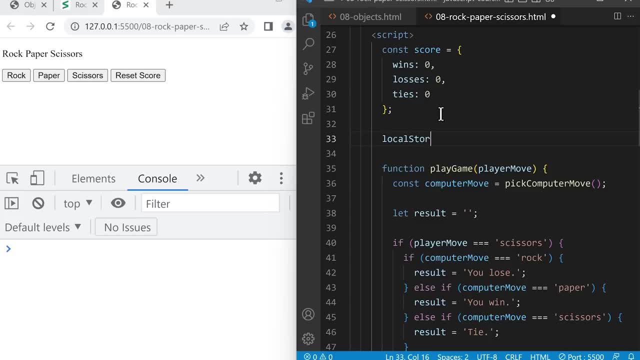 local capital S storage dot get item this time and brackets. So the get item method gets a value out of local storage And we're going to give it one string. So this string is the name that we used earlier, which was message. So we'll type this string: message. 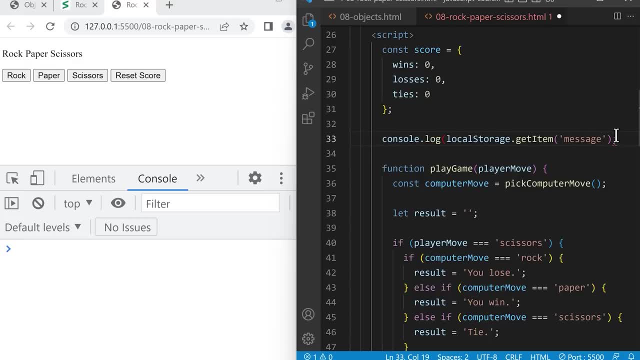 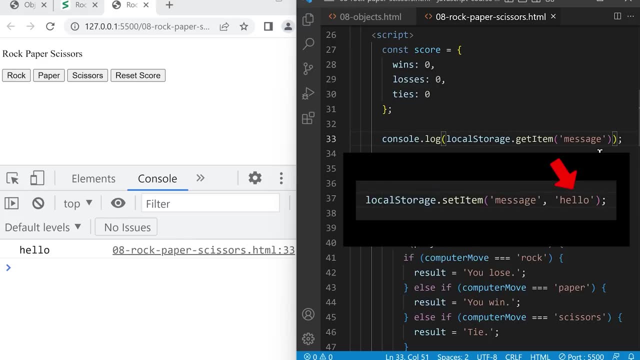 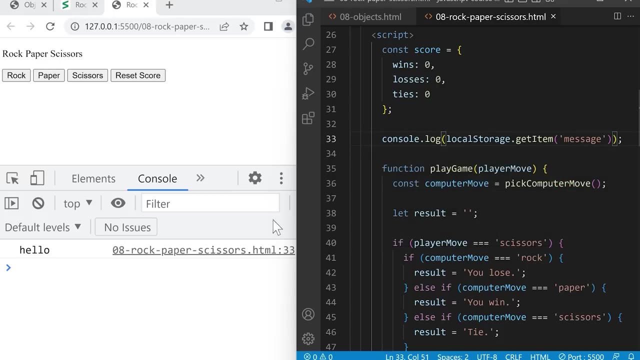 Now let's console dot log this result. So console dot log and a bracket at the end and save. It will get the value that we saved earlier out of local storage. So we saved the string hello And that's exactly what gets displayed in the says. 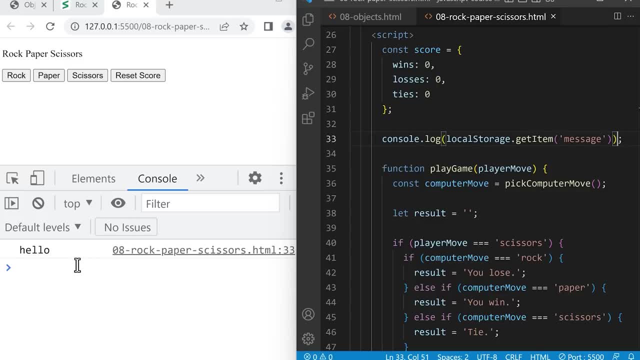 It's going to use the abra in the console, So, using local storage, we were able to get the value that we saved earlier, even though we refreshed the page. Now let's save our score into local storage so it doesn't get reset when we refresh the page. So let's scroll to the bottom. 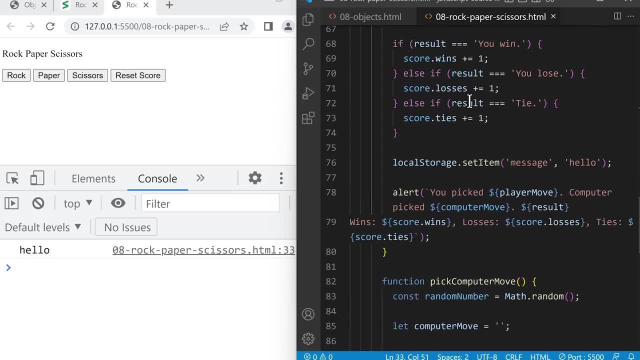 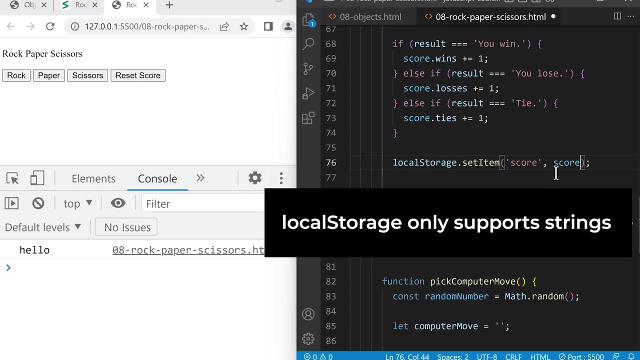 And instead of using the name message, we're going to use the name score to save our score. And instead of the string hello, we're going to save the score object. Now, one problem here is that local storage only supports strings, So we need to convert our object into a string. 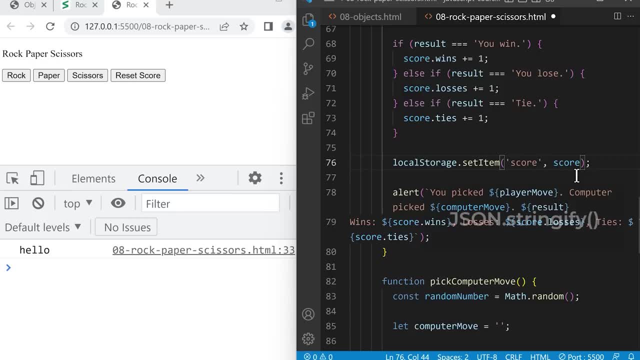 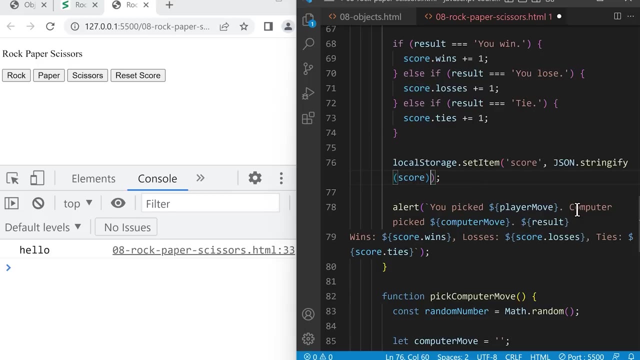 And we actually learned how to do this earlier Using jsonstringify. So at the front we can type jsonstringify and then brackets around the score, And this will convert the JavaScript object score into a json string And then it's ready to be saved in local storage. So if we save this and then play the game, 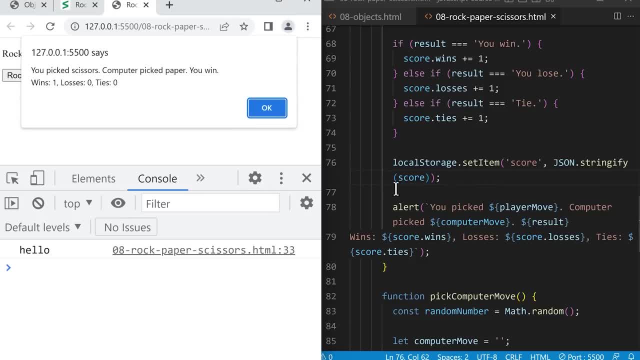 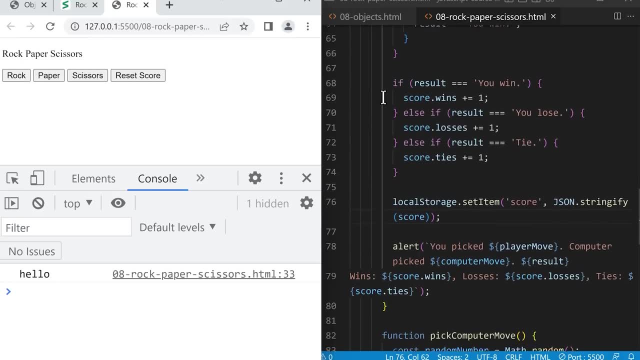 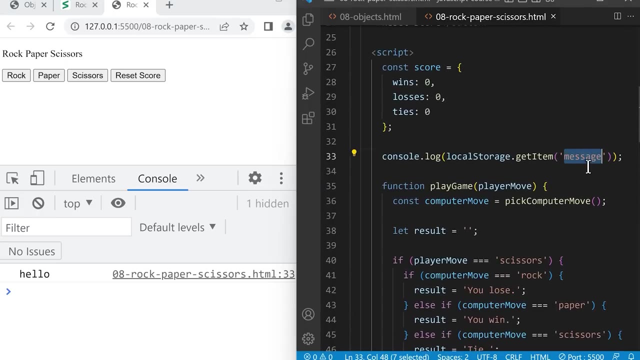 it will run this code and save our score into local storage. Now let's press OK And then scroll up to the top, And now, instead of getting the message, we're going to get the score out of local storage. If we save Now, when we load the page we're able to get the score that we saved from last time. 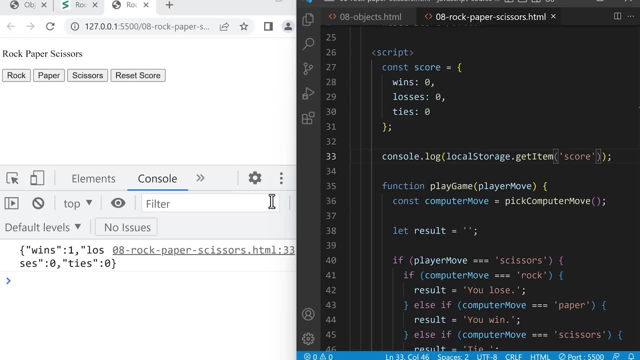 as a jsonstringify. The last step is, instead of resetting the score to zero every time, we're just going to use the score from local storage. Before we do that, remember that this is just a string, So we need to convert this back to an object. We also learned how to do this earlier using jsonparse, So at the front. 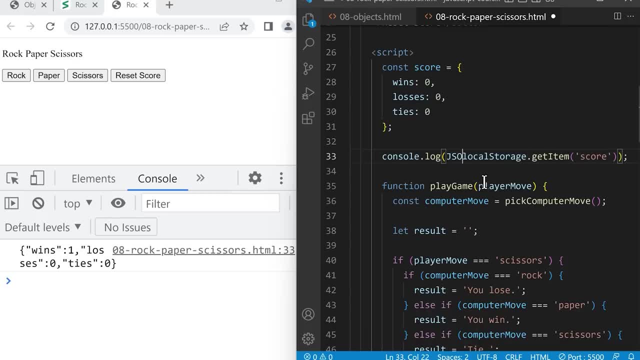 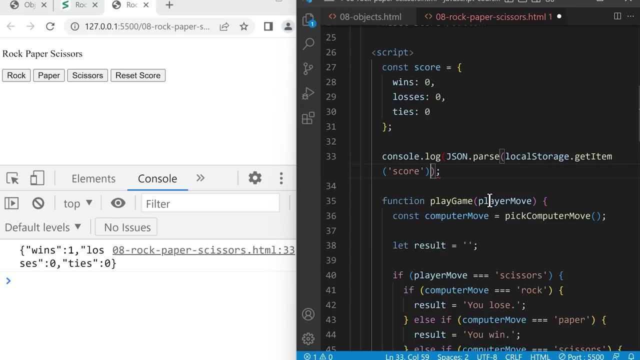 we can type jsonparse and then open bracket and at the end a close bracket And it will convert this back to an object. If we save, it will convert the score from a json string back to an object. So now we can use it up here. So instead of doing this, we'll remove it. 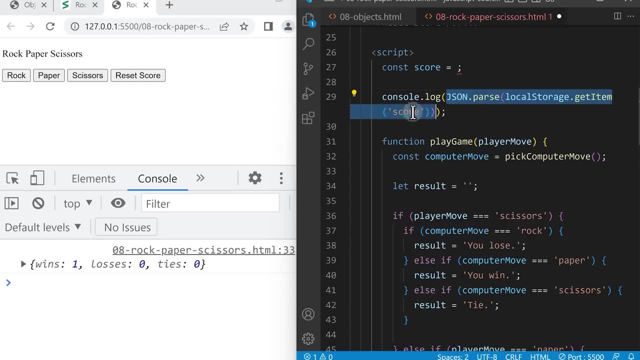 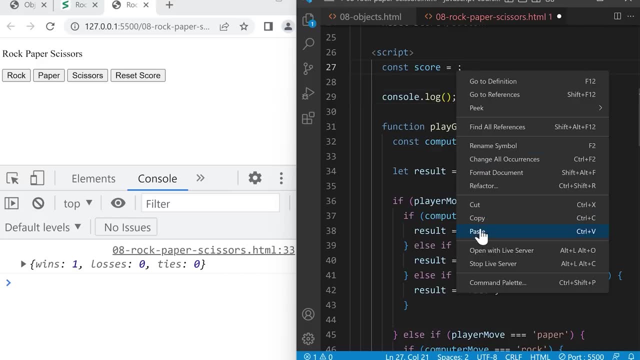 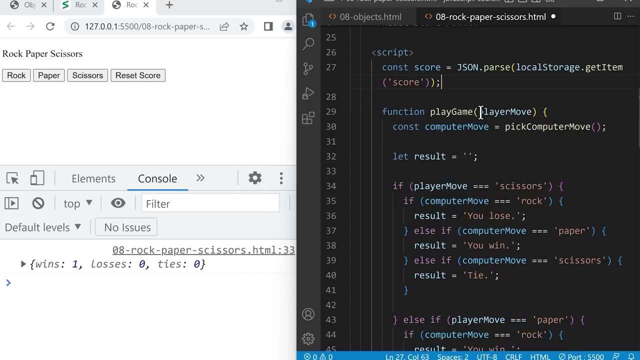 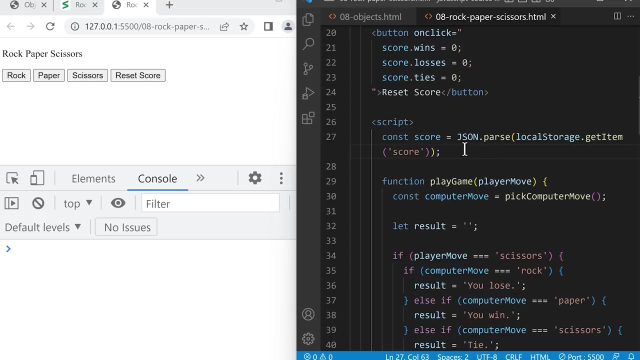 And replace it with this code. So right-click, cut And then here right-click and paste And we'll remove consolelog And save. So now when we load the page, it will load the score from local storage If we play the game. 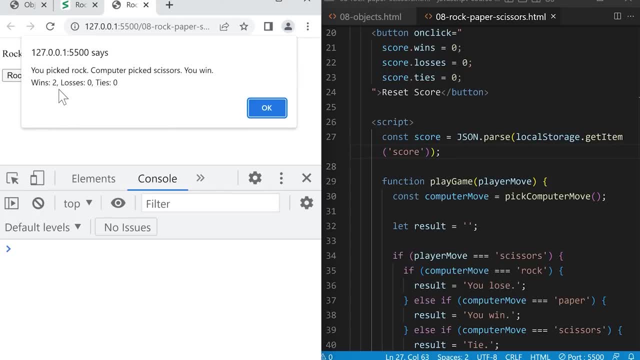 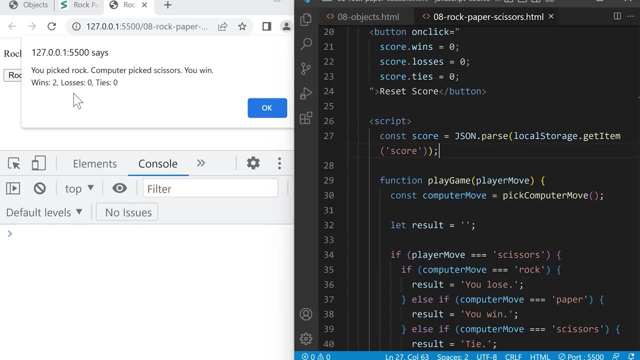 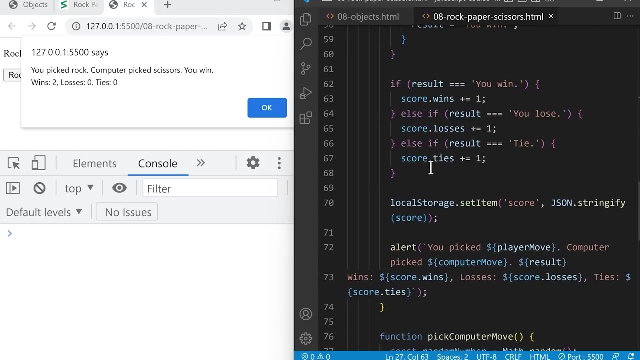 Notice that the score doesn't start from zero. It starts from the score that we had last time, Sur計. Let's review what we did step by step So far. we've already added a score and Livest 그렇ец. When we update our score in this code. after we update the score, we'll save it in local storage. 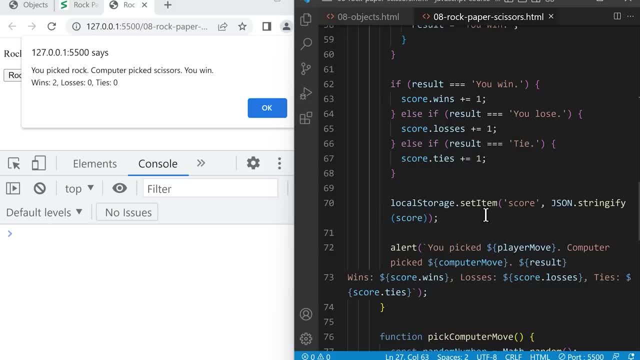 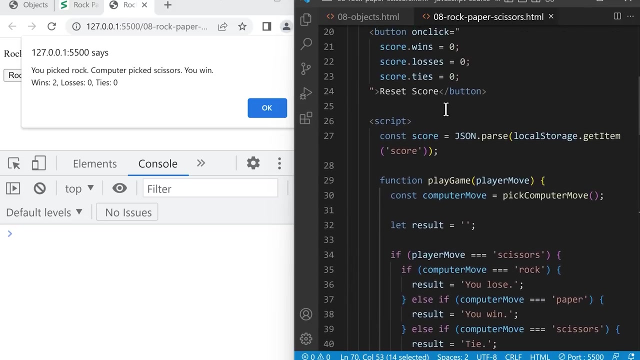 using localStoragesetItem. Now, local storage only supports strings, so we have to convert our score object into a JSON string using JSON dot stringify and then, after we've saved this into local storage, when we load the page up here, we're going to load the score that we just saved from local storage using local storage dot. 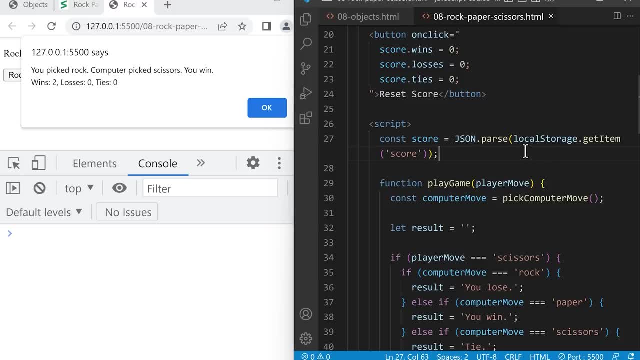 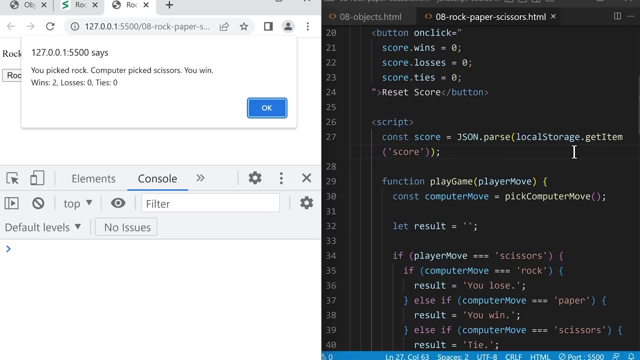 get item and the score was saved as a JSON string, so we need to convert it back into an object using JSON dot parse. so that's how we use the JSON object and the local storage object to save our score more permanently. let's press OK. and the last feature we're going to add is when we click the reset score button. 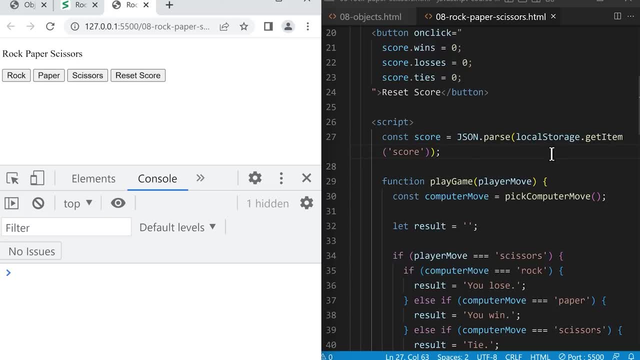 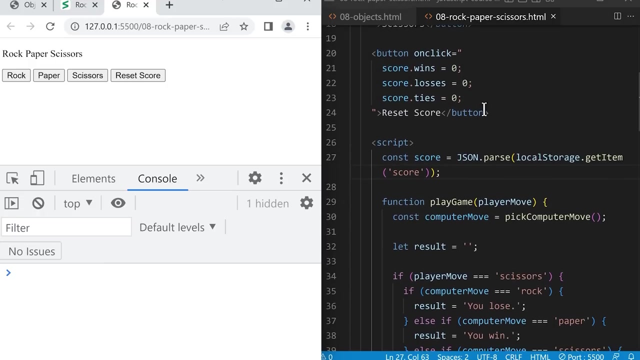 we also need to remove the score from local storage. otherwise if we press reset score and refresh and then play the game, it would just grab the old score from local storage. so reset score doesn't really work here. let's press OK and fix this issue. so here in the reset score button at the end we're going to remove the. 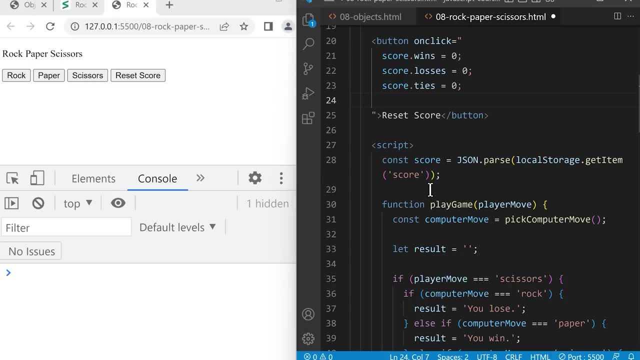 score from local storage. so we'll type local storage and then a method called dot, remove item and brackets, and between the brackets we're going to tell local storage which value we want to remove. so we're going to remove the score. so we'll type the string score if we save and we click the reset button. 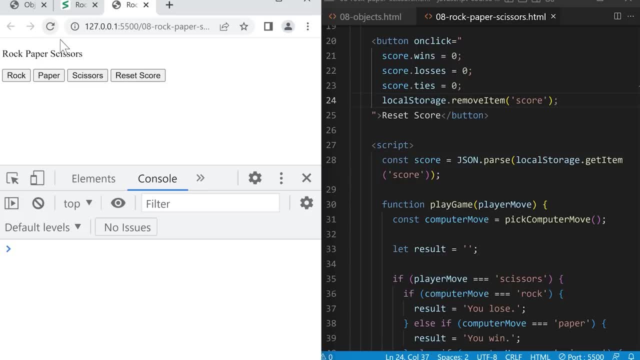 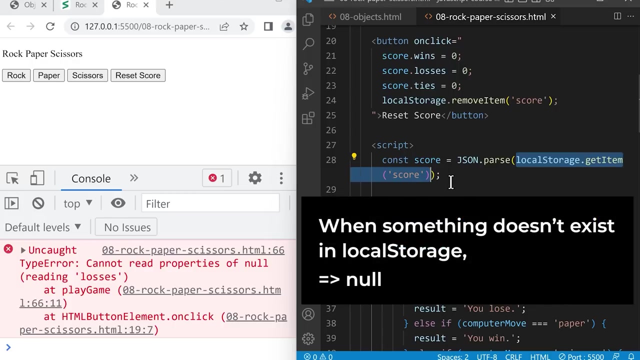 and then we refresh the page and try to play the game again. unfortunately, it now gives us an error. so what is happening here? so remember that we remove the score from local storage. so now, when we load the page, this actually doesn't exist. when something doesn't exist in local storage, it's going. 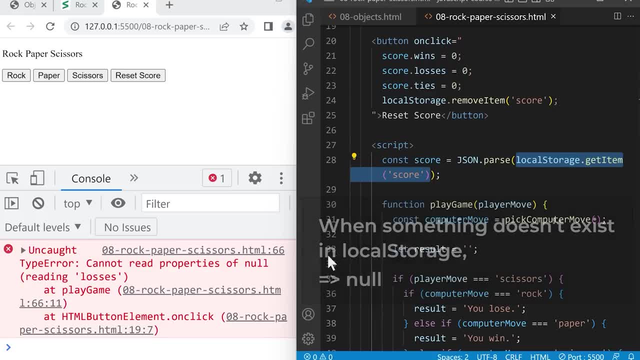 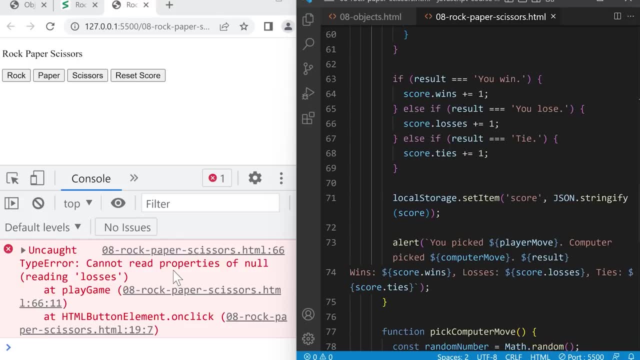 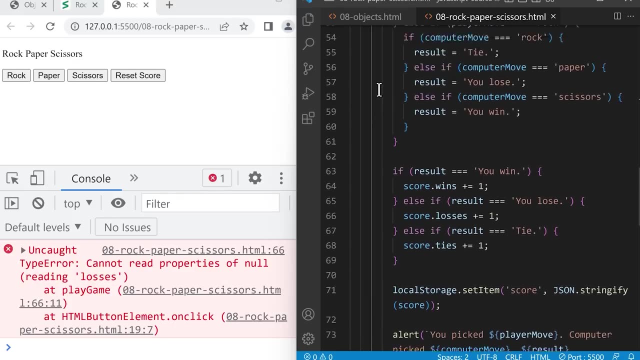 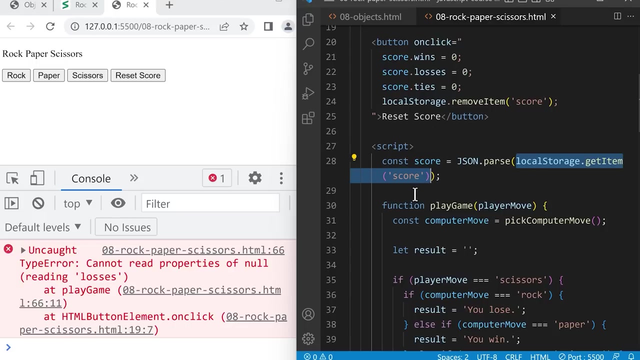 to give us a value called null and at the bottom, if we try to access any property on null, it will give us an error. so that's what we see here. so how do we solve this problem if we scroll up? one way to solve this problem is that if there is no score in local storage, we're 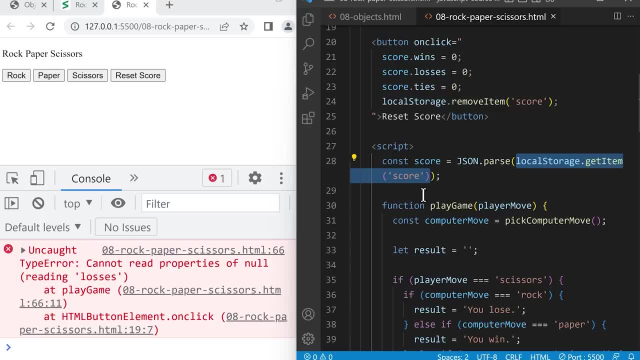 going to give it a default value. let's look at how we can do that. so after this line, we're going to check if the score is null. we can do that using an if statement, if brackets and curly brackets, and we'll check if score is equal to null. and if it is equal to null, we're going to 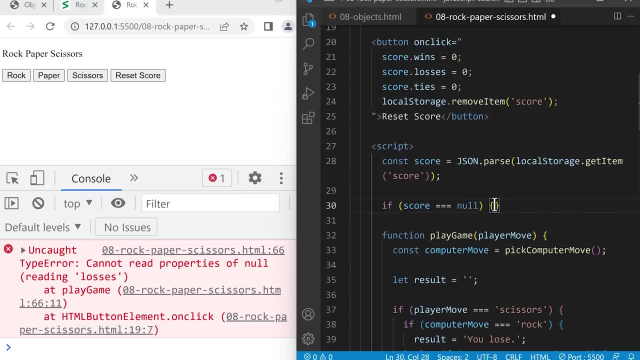 give this a default score. so inside the curly brackets we'll just make the score equal to the default object we had earlier, which was wins zero and then losses zero and ties zero. and remember, if we need to reassign a variable, we have to change it from const to let. 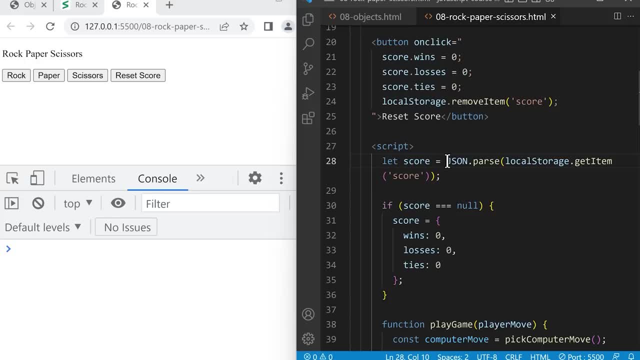 if we save, the score will be null because we removed it earlier and now this will give it a default score, so everything should work as before. if we play the game, you'll notice that the score starts from zero or this default score, and everything is working again. so that's how we create the score feature in the Rock Paper. 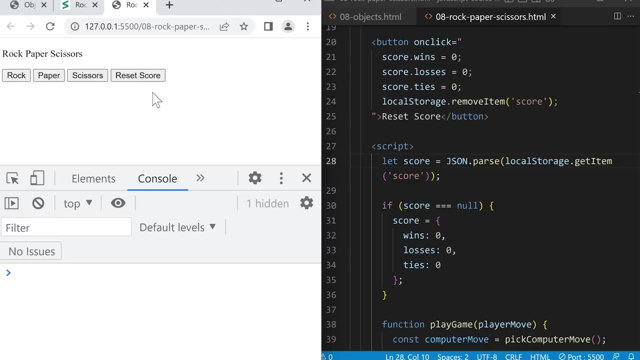 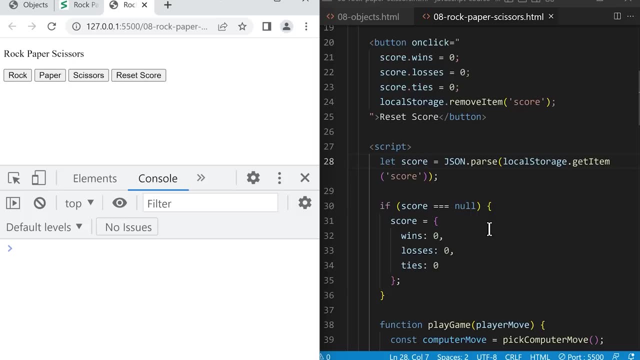 scissors project, as well as the reset score feature. next, we're going to use some shortcuts to code. So these shortcuts are things that we learned in the Booleans lesson. So remember that null is a falsy value. That means it will behave just like false. So 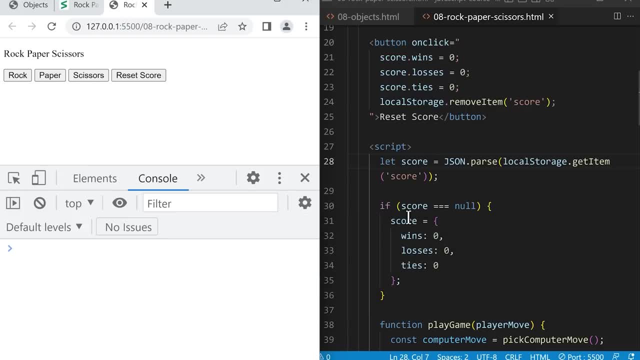 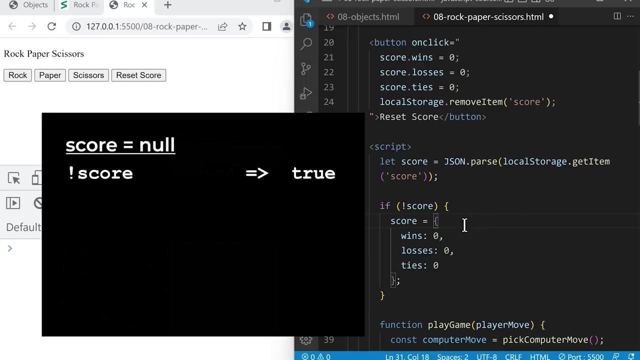 a shortcut we can use here is: instead of checking if the score is equal to null, we can also remove this and check if notScore. So notScore does the same thing as checking if it's null. If the score is null, notScore will flip it into true, So both of these will. 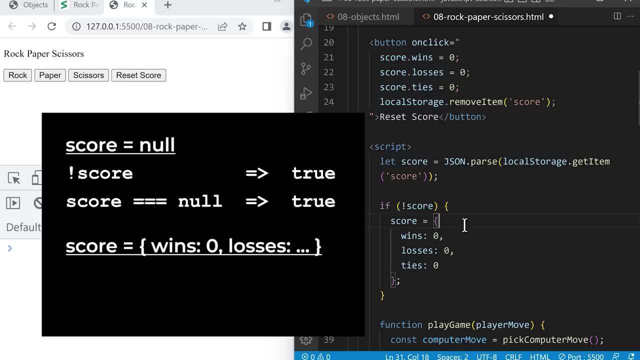 return true. If the score exists, it's an object. then both of these will return false. So instead of checking if a value is equal to null, we can just use the not operator as a shortcut. Now, also from the Booleans lesson, we have an even shorter shortcut for. 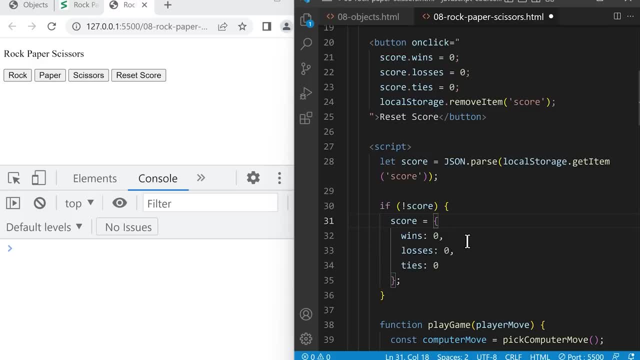 doing this. So notice here that this code basically sets a default value if the score doesn't exist. In the Booleans lesson, we learned a technique called the defaultValue. The defaultValue is a default operator, which is exactly what we need here. So on this line, 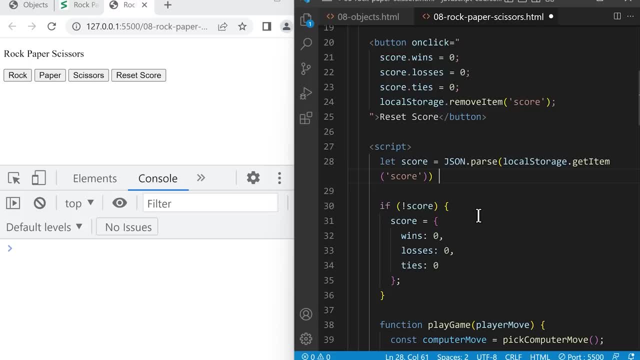 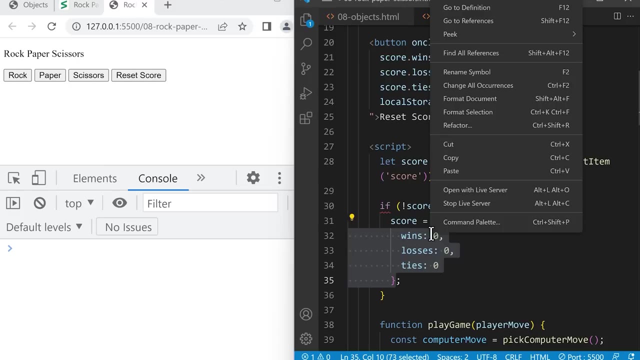 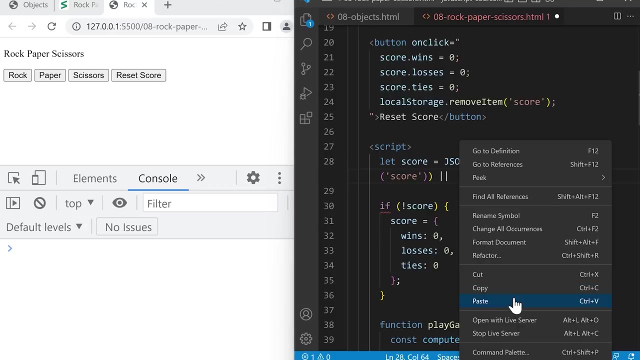 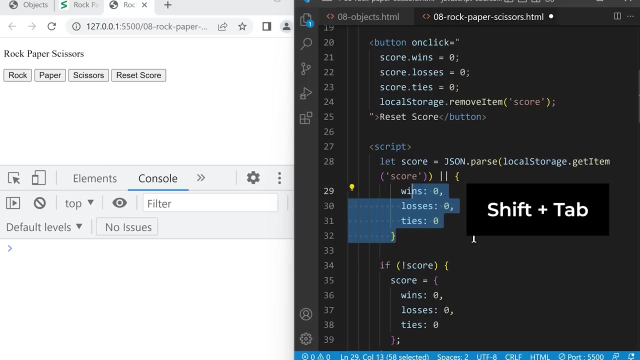 we can remove the semicolon and type OR and then a defaultValue. So we want our defaultValue to be this object, So let's select it and then right-click copy and then here right-click copy And I'll select these lines and press Shift-Tab to remove an indent And I'll add a semicolon. 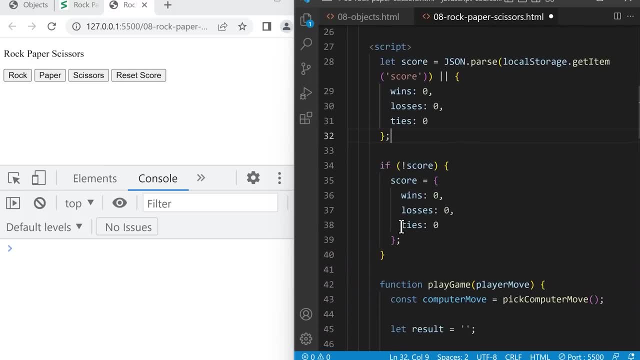 back at the end. So the way that the default operator works is that if the left side is truthy- so in this case we have a score- it will use the left side. If the left side is falsy, or in this case the score is null, then we will use the right side as a default. 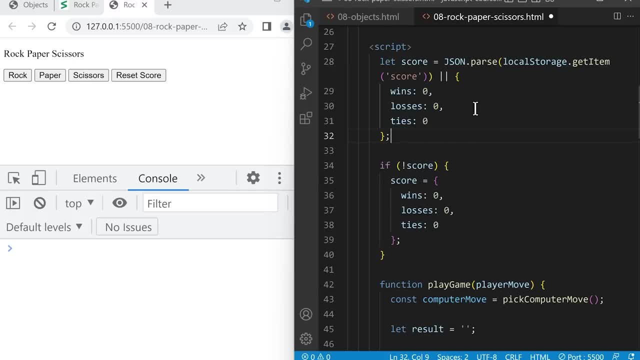 value. So this does the same thing as this code below, but it's just a shortcut. So now let's comment out this code using slash star and at the bottom, star slash. So we'll leave it here just for reference, And then save And we're good to go. So now let's go back. 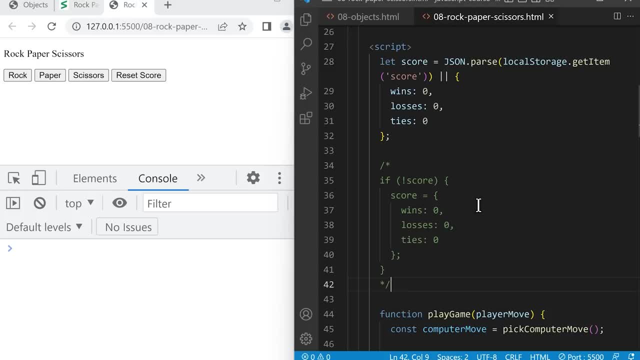 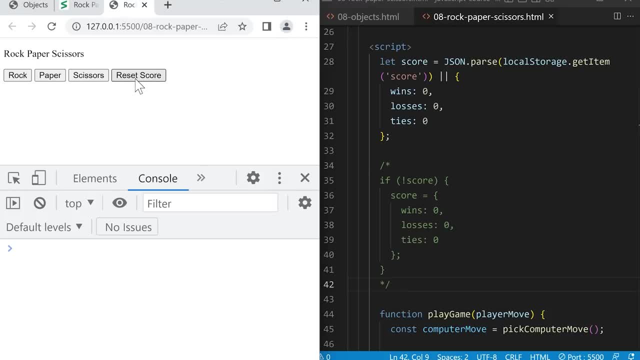 good to go. So now we're good to go. So now we're good to go. So now let's go back to the Booleans lesson. And if we hit save, and if we click reset, score again and refresh and play the game, it will still work. So this is a perfect situation to use the default. 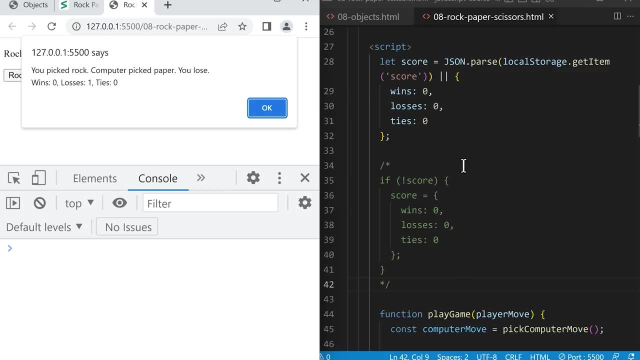 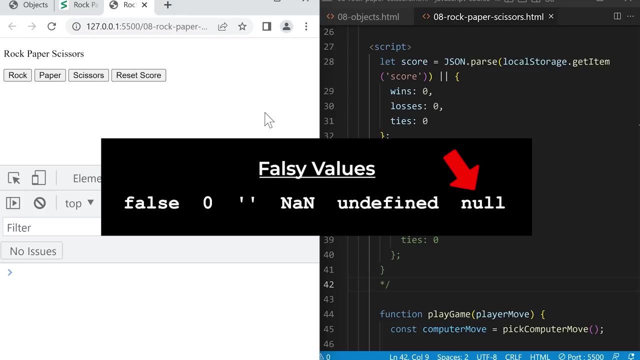 operator to simplify our code, So let's press OK, And that's all we're gonna do for this project in this lesson. Now let's move on and learn more details about objects. The first thing we'll learn is the value null, So null is one of the falsy values in JavaScript. 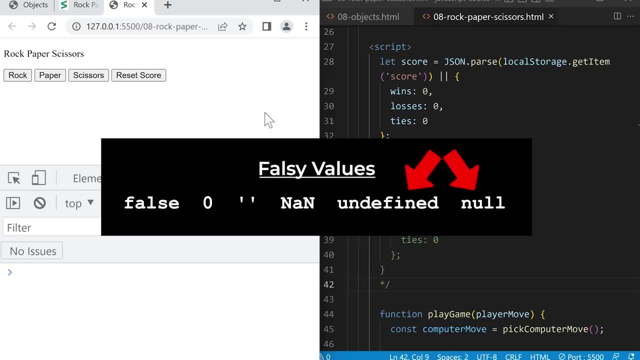 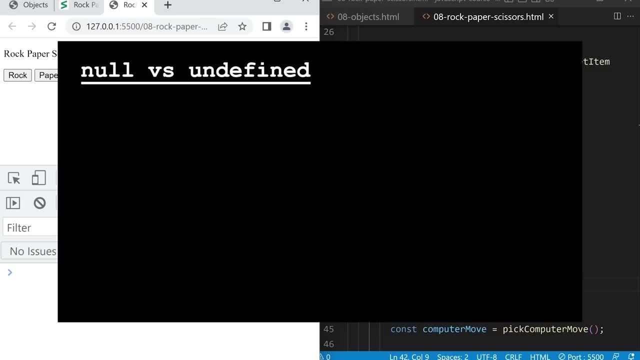 It's similar to the value undefined. They both represent that something doesn't have a value. So what's the difference between null and undefined? We use null when we intentionally want something to be empty, For example. in the previous lesson we learned that if a function has parameters, we can. 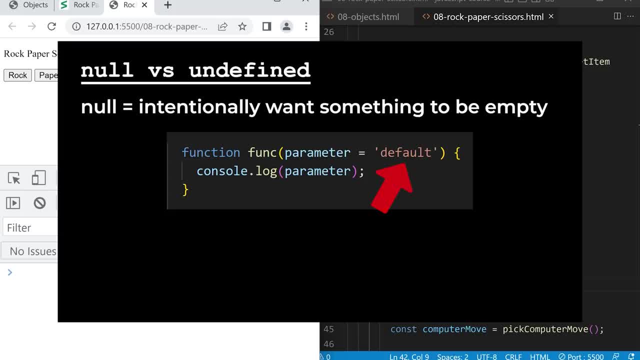 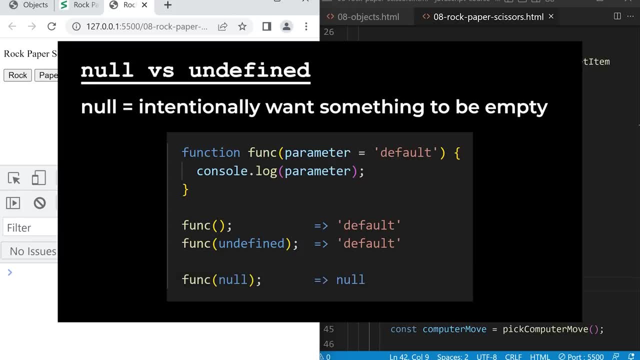 give the parameter a default value. If the parameter is undefined, it will use the default value. However, if we set this parameter to null, it will not use the default value and it will just use null. So null means we intentionally want something to be empty. 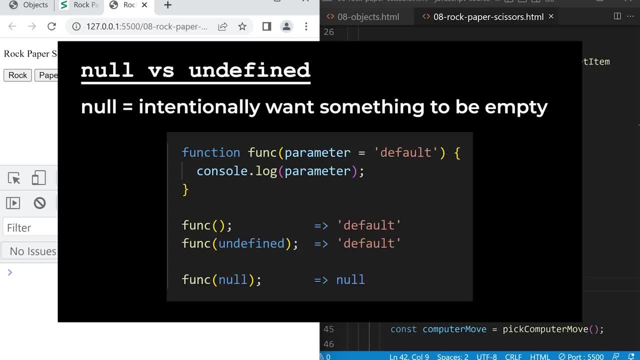 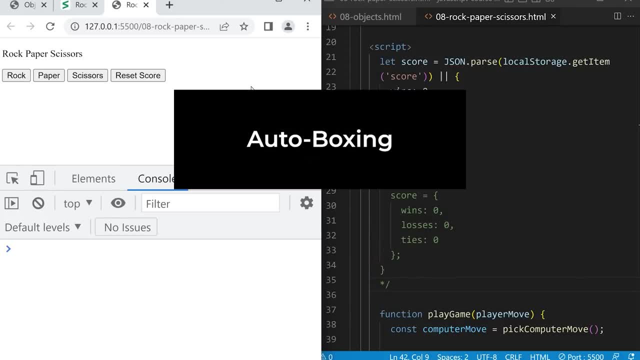 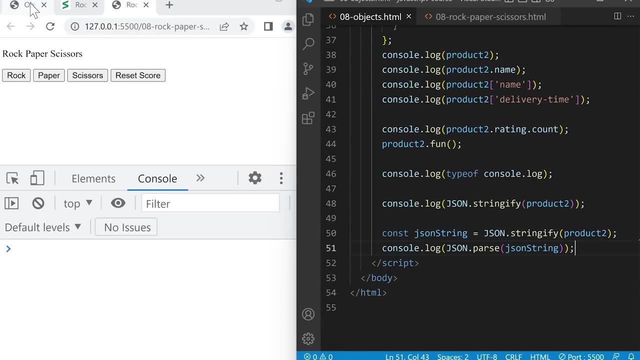 In most cases, though, null and undefined work the same way. Okay, so the next detail about objects we're going to learn is called auto-boxing. Let's go back to objectshtml and open the tab for this file. Let's also comment out the previous code. 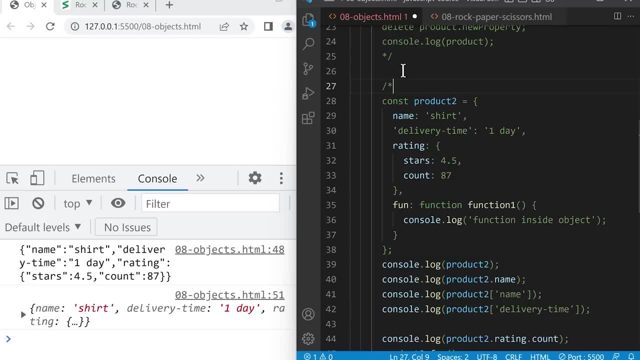 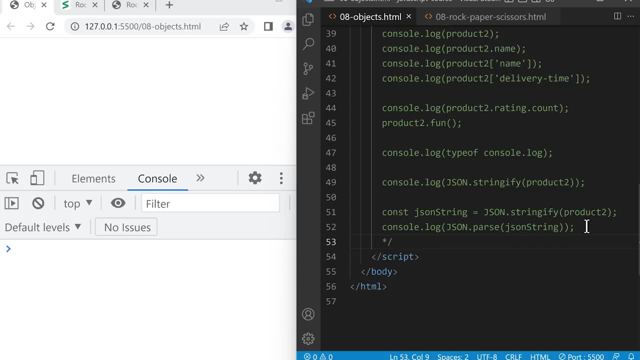 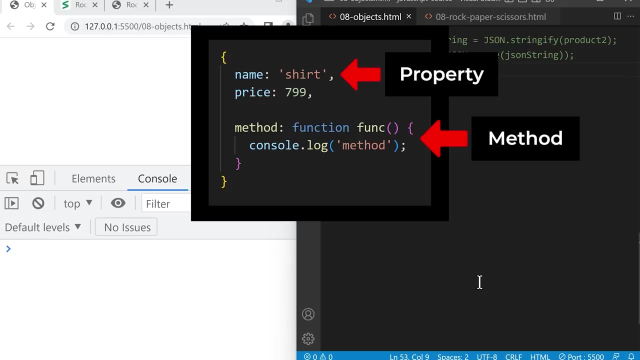 So our console doesn't get too confused. The main thing we're going to do is change the name of our object to messy, So slash star. and at the bottom star, slash and save. So let's scroll down. We learned in this lesson that objects can have properties and methods. 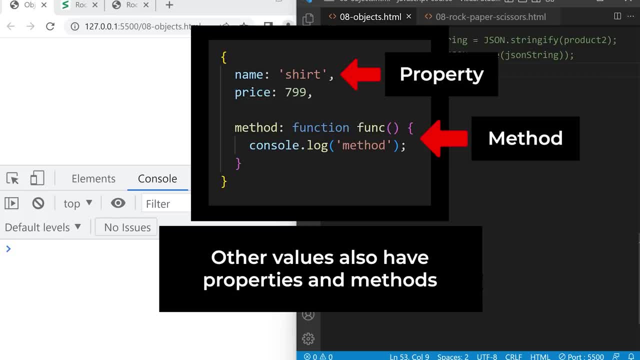 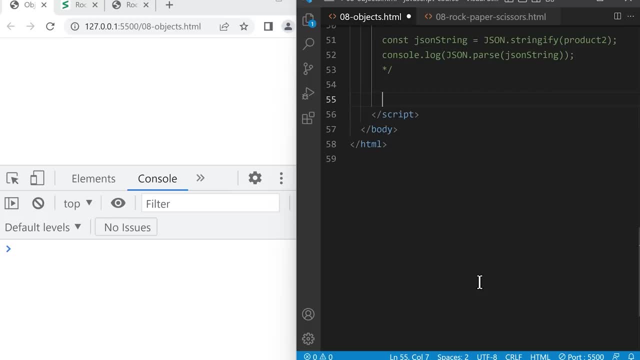 So you might be surprised to learn that other values also have properties and methods. For example, at the bottom We're going to type consolelog the string hello and then the dot notation and a property called length. So strings can also have properties. 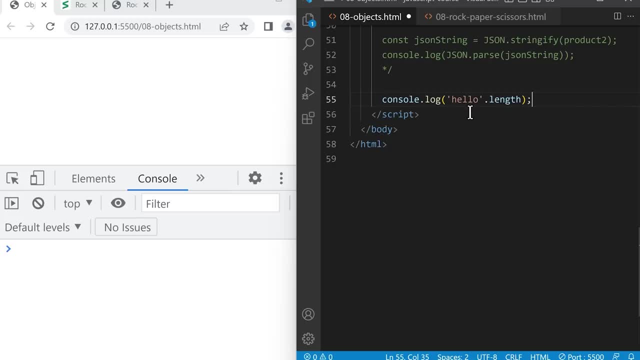 The length property tells us how many characters or letters are in this string. So hello has five letters. So if we save, the length property will be five. Here's another example. We'll type consolelog the string hello and then the dot notation and a method: this: 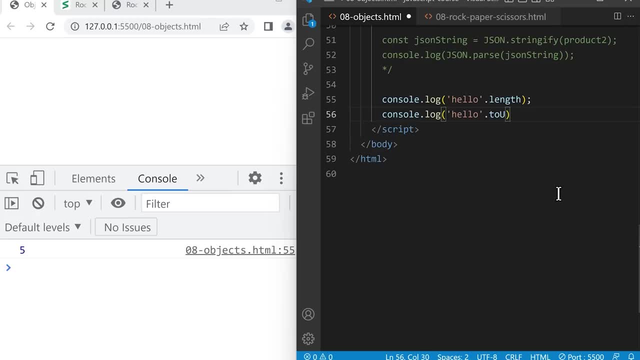 time To capital U, upper capital, C, case and brackets. So this string, It also has a method called toUpperCase And this method gives us a copy of the string with all letters capitalized or in uppercase. If we save, it will give us hello in capital letters. 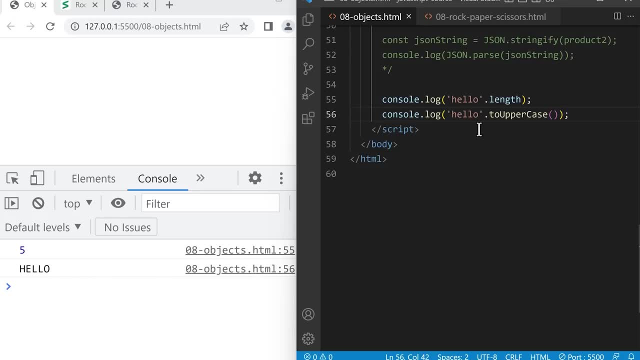 So, as you can see, simple values like strings can also have properties and methods. So now you might be wondering: These are strings, not objects. How can strings have properties and methods? The answer is that JavaScript has a special feature called autoboxing. 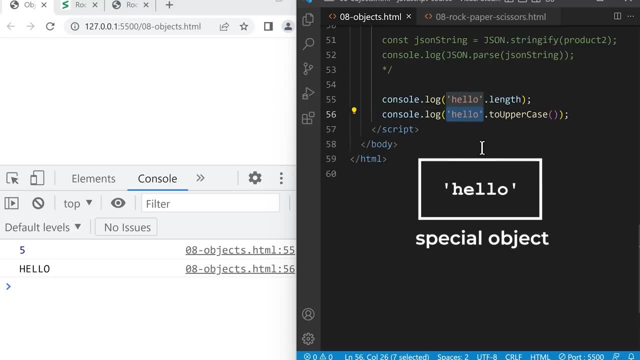 JavaScript automatically wraps this string in a special object first, And this object has the property length and the method toUpperCase, So this is done automatically. We don't see the special object That's wrapped around this string, So this feature is called autoboxing. 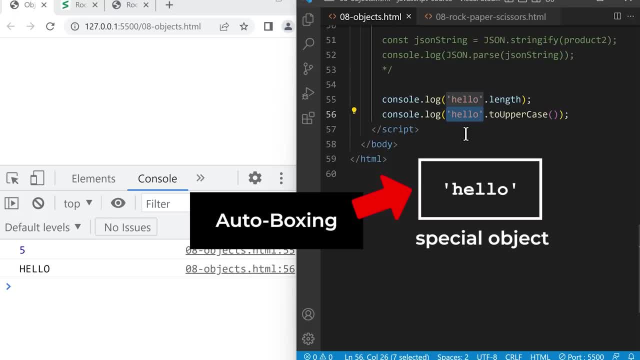 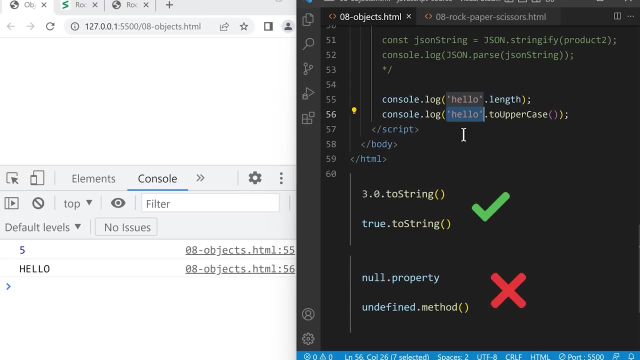 Because JavaScript automatically wraps this string in an object like a box, So autoboxing also works with other types of values like numbers and booleans. The only thing is that autoboxing does not work with null and undefined. It would just give us an error. 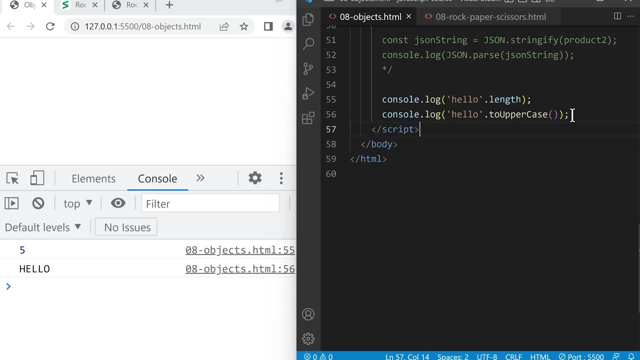 The last detail we're going to learn about objects is a really important detail, And that is: objects are references. To demonstrate, let's create a new variable with an object, So const object1, and make it equal to an object. Inside this object, let's have a property message, colon, object. 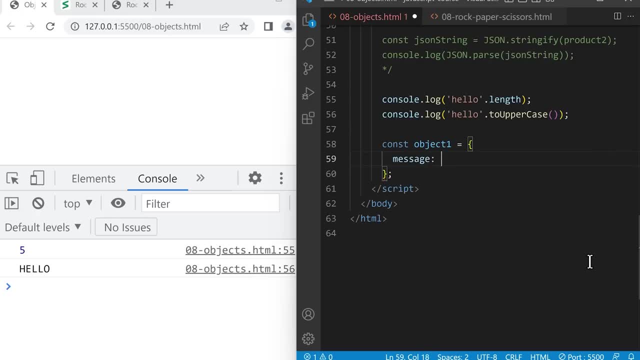 And we're going to call it object, And we're going to call it object And we're going to call it object And the string hello. So you might think that when we create an object like this, we create a value that has. 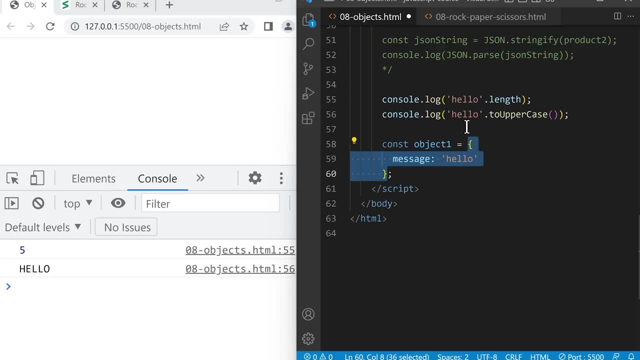 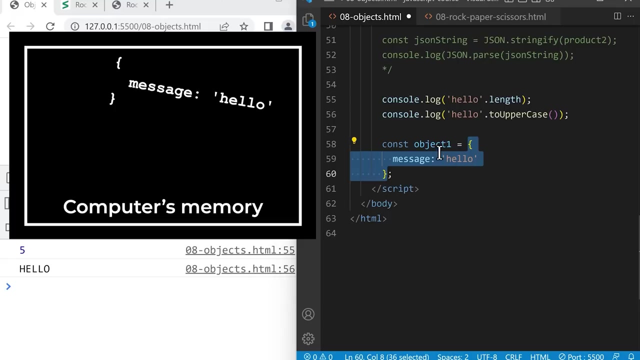 other values inside and we save the whole thing in a variable. However, this actually works a little differently. When we create this object, the actual value is created somewhere in the computer's memory, And this variable actually just gets a reference That points to that location in the computer's memory. 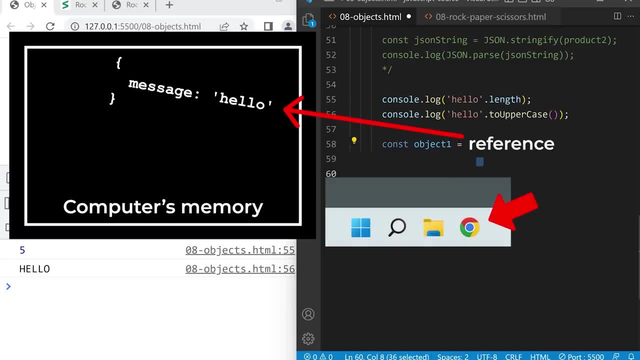 This is like a shortcut on your computer. A shortcut points to where the actual file or folder is. So there's no way to actually see this reference. But just know that this is a reference And the object is somewhere else in the computer's memory. 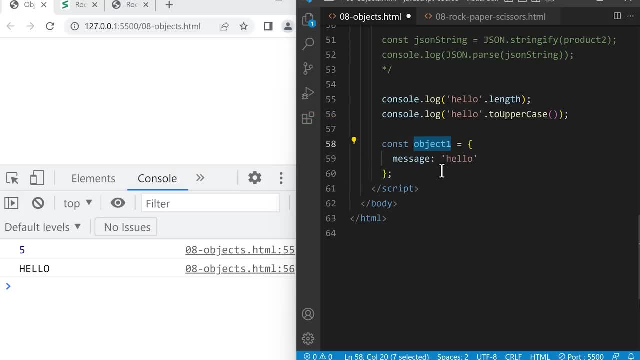 So the reason it works this way is to make the language more efficient. For example, Let's create a new variable. Below this line, we can create a variable const and call it object2.. And make it equal to object1.. 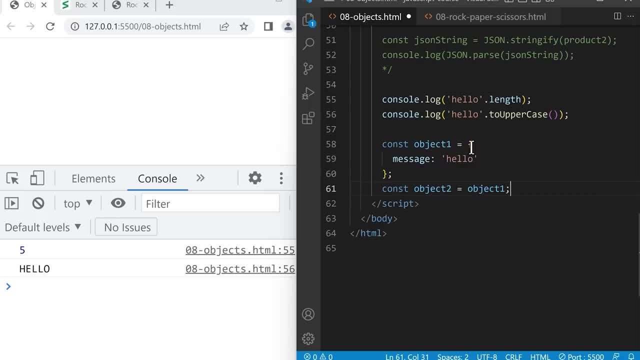 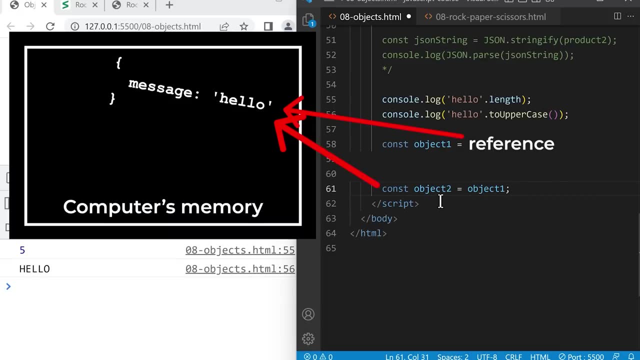 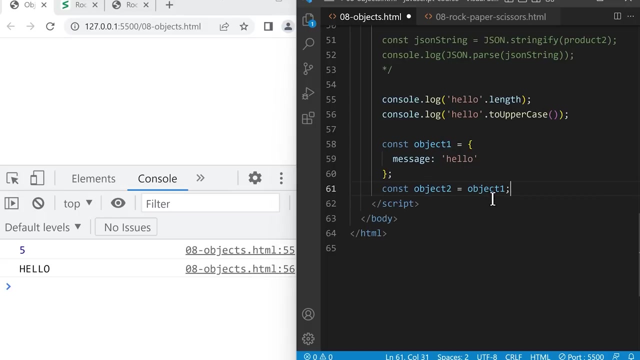 So this code doesn't actually make a copy of the object, It just makes a copy of the reference that points to the object. So this makes the language more efficient, Because if we had a really big object, A really big object here, It's not good to copy the entire object over and over again. 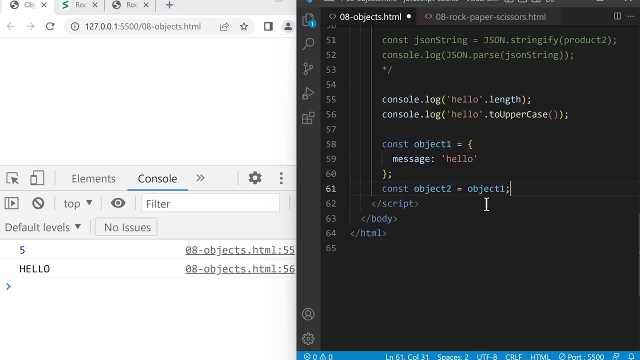 Instead, JavaScript just copies the reference, which is much faster. This is called copyByReference. Now that we learned that objects are actually references, Let's learn some interesting behaviors of references. So at the bottom here, We're going to change the property message in this object. 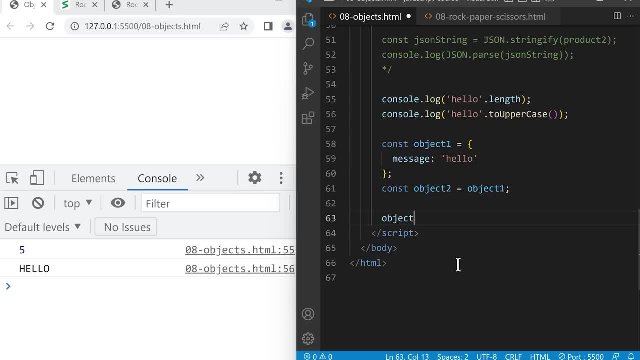 We can do that By typing the object object1.messageProperty And make it equal to something else Like the string goodJob. And now If we consolelog object1.. So if we do this, Go to the left And we'll do this. 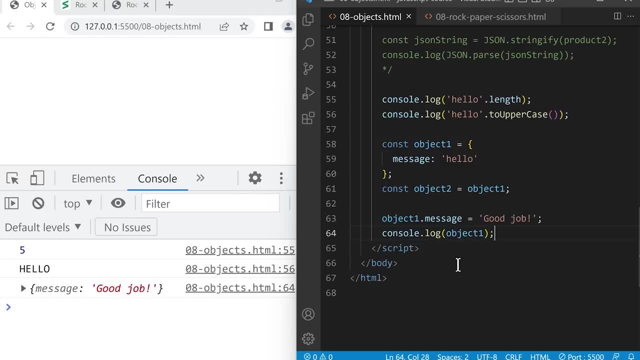 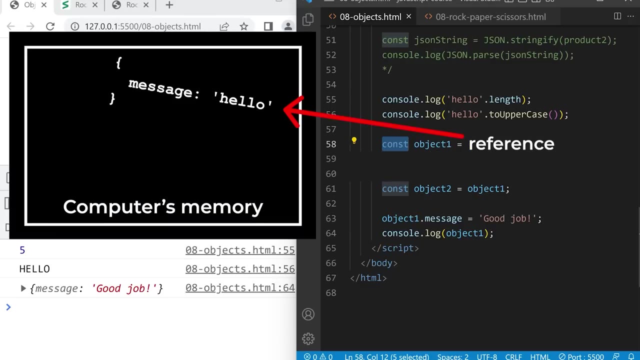 and save, Notice that we were able to change the message property even though we created object 1 with const, And that's because this variable just contains a reference that points to the object. So const prevents us from changing the reference in the variable, but it doesn't prevent us from reaching. 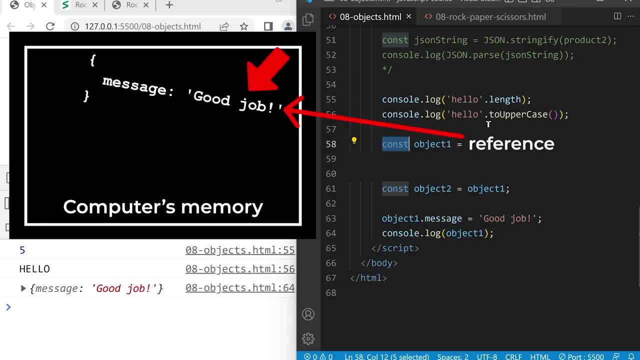 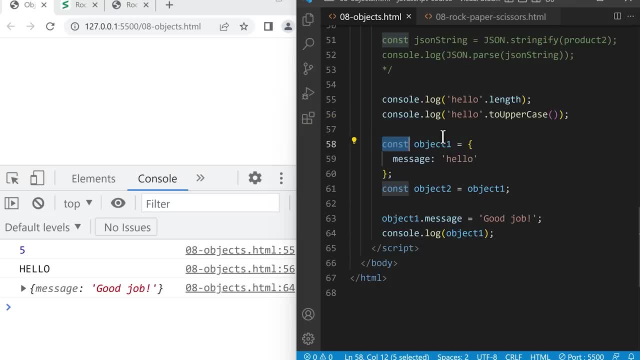 into the reference and changing the object that it's pointing to. So just be careful when you're working with objects. Even though we use const, we can still change the values inside the object. Another interesting behavior is that on this line, we're not actually copying the object into this variable, We're 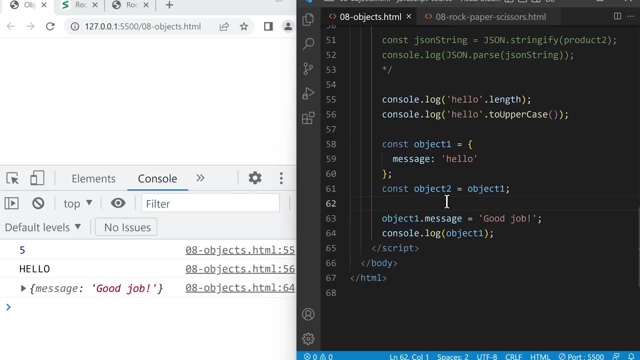 copying the reference. So object 2 actually has the same reference as object 2.. So object 2 has the same reference as object 2.. So object 2 has the same reference as object 1.. They actually point to the same object in. 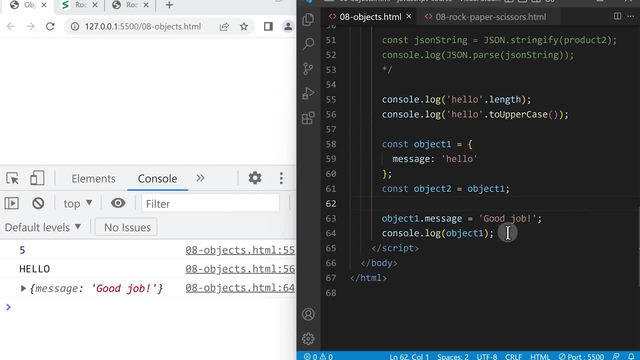 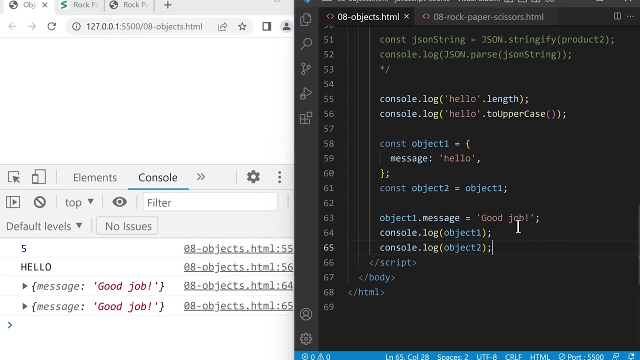 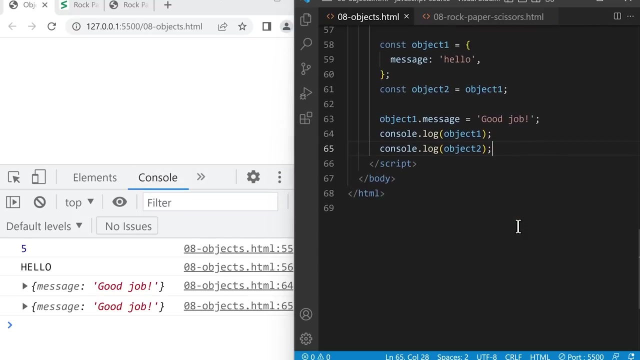 the computer's memory. So at the bottom, if we type consolelog, object 2 and save, you'll notice that for object 2, the message property was also changed, even though we only changed object 1.. The last interesting behavior is is that we can't compare objects directly. For example, let's go to the 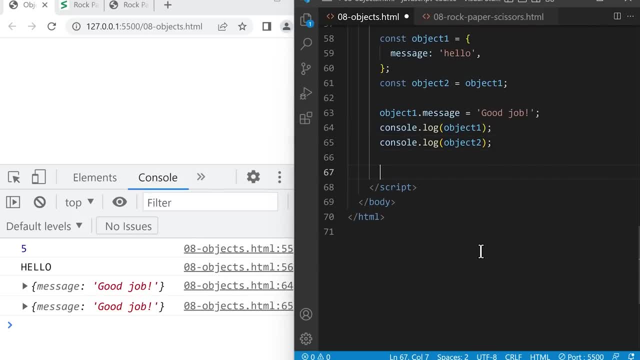 bottom and we'll create a new object using const object 3 and we'll make it equal to an object And then inside we're going to have these same values as object 1.. So we'll have the property message- check, career- And the value. 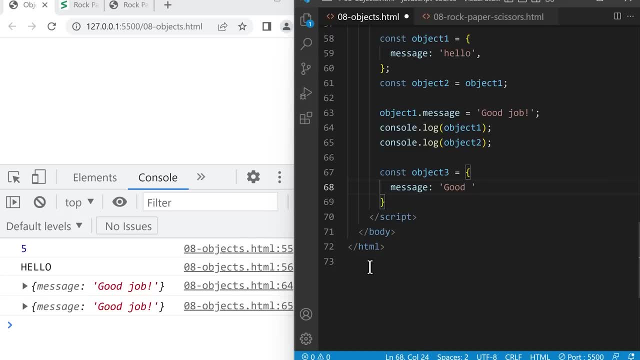 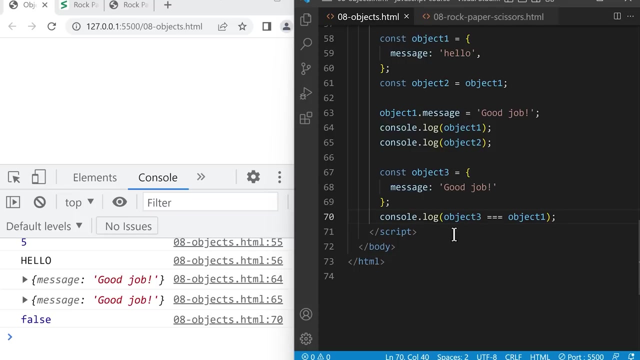 is the string. good job. so now let's try comparing object three to object one. so here we'll type console dot log and check if object three is equal to object one. if we save, it will tell us that these two objects are not equal to each other, even though they have the same values inside. and that's because. 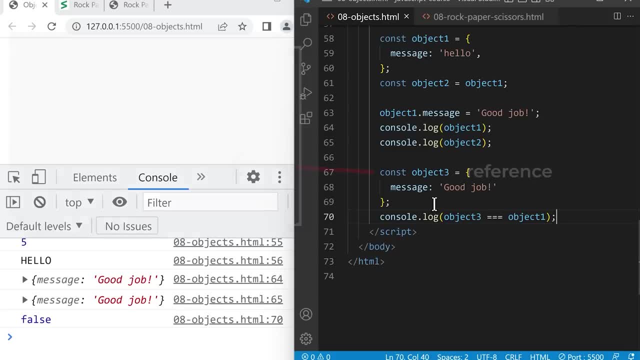 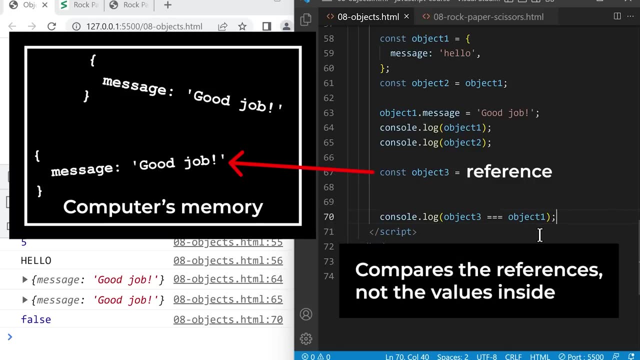 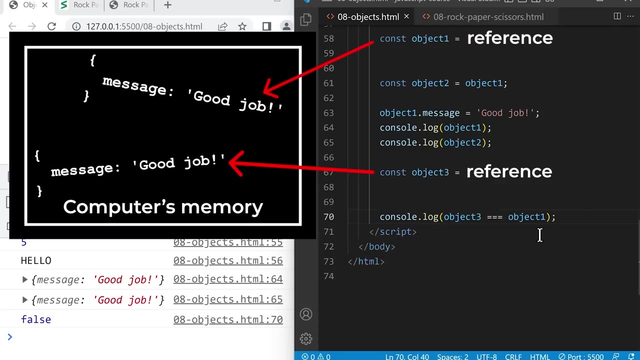 remember, objects are references, so object three also contains a reference and this code compares the references and not the values inside the object. so because object three is equal to object one, it will tell us that these two objects are is a different reference than object one. that's why this code results in false. 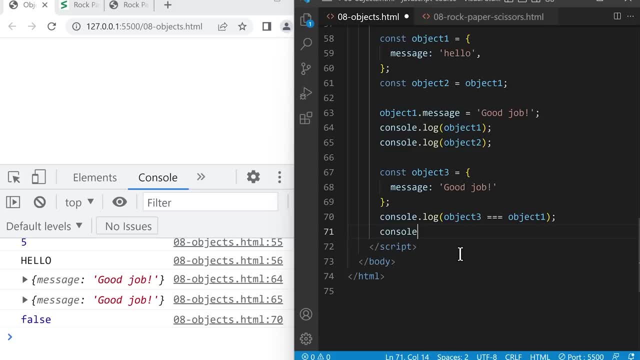 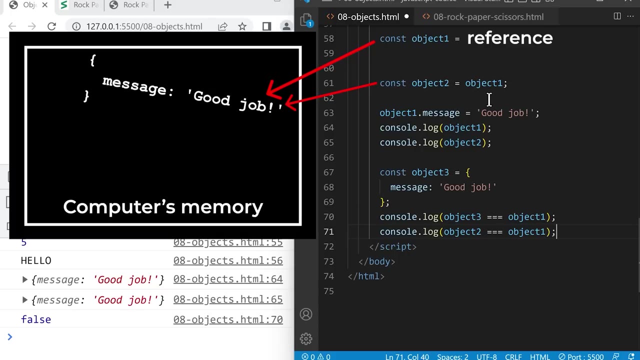 if we did console dot log and we check if object two is equal to object one, object two has the same reference as object one. it points to the same object in the computer's memory. so if we save, this will tell us that these two variables have the same reference. 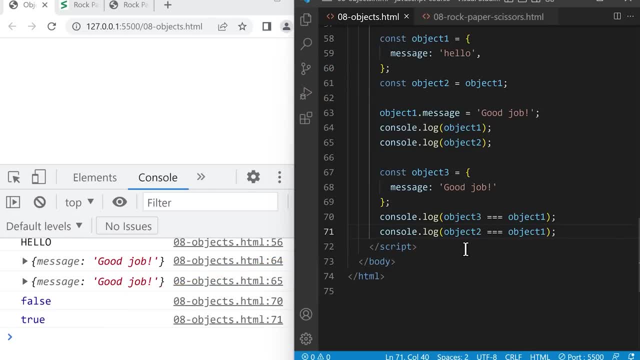 so just remember that when you're comparing two variables that contain objects, you're actually comparing the references, not the values inside. if we want to compare the values inside, we would do that manually by checking the message property against this message property. so don't worry, object references are a little confusing at first, but the more you work with it, the more you just 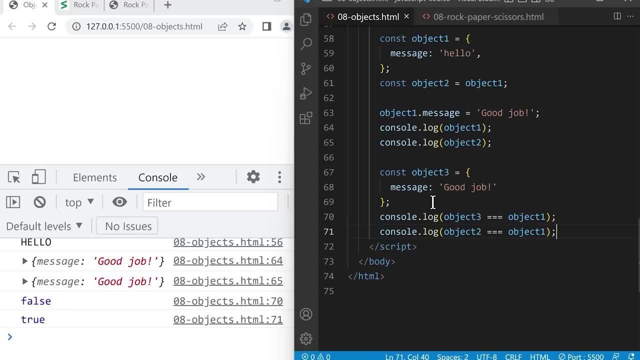 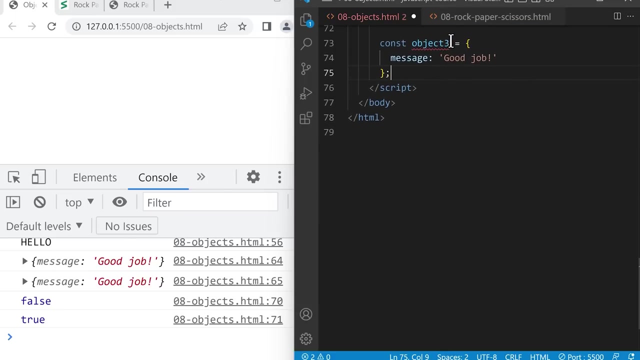 get used to it. the last thing we're going to learn in this lesson are some shortcuts for objects. so first let's make a copy of object 3.. we'll select the code and right click- copy, and then at the bottom we'll scroll down and right click and paste and let's rename this variable to object 4.. so now let's say that we 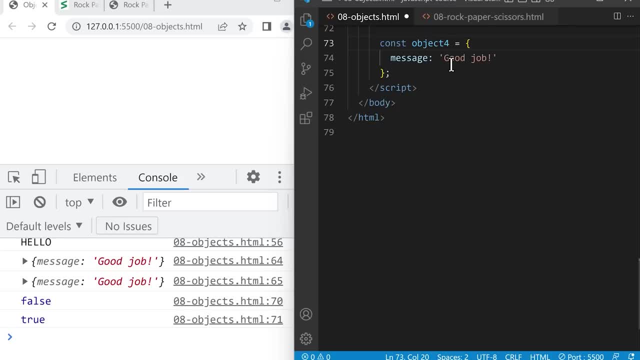 want to get the message property out of this object, we can do that by typing object 4, dot message. and now let's also say that we want to save this in a variable also called message. so at the front we'll type const message and make it equal to this value. 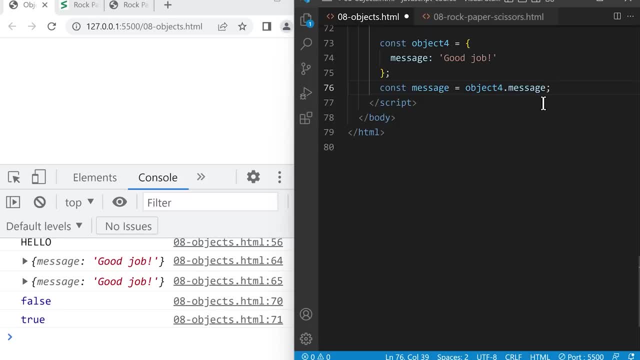 so now, if the variable name and the property name are the same, we actually have a shortcut for this. to use a shortcut, we're going to type const and curly brackets. so we're going to type const message and make it equal to object 4.. so this shortcut is called destructuring. this will take the message property out of object 4. 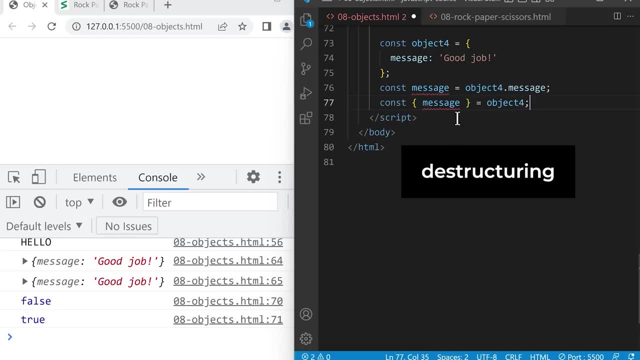 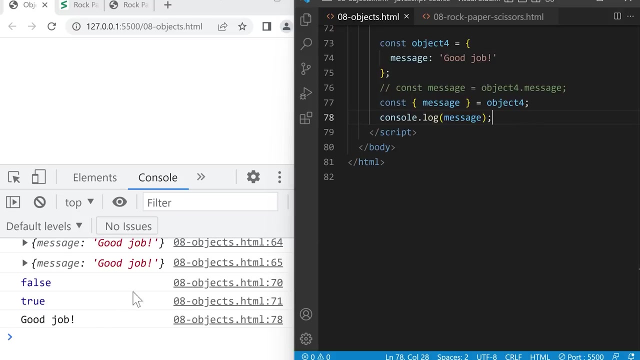 and save it in a variable called message. so this line of code does the same thing as the code above. so let's comment out this line using double slash and we'll just keep it for reference. so at the bottom, if we type console dot, log message and save, it will display good job. so the 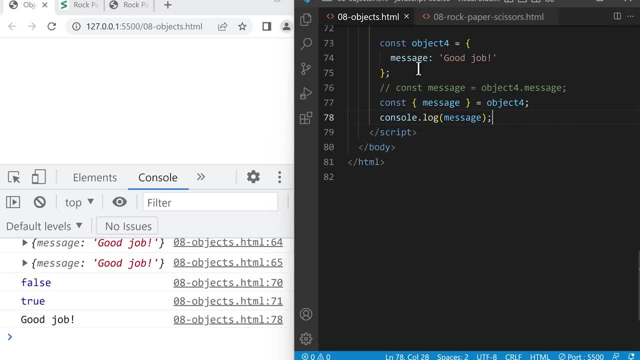 destructuring shortcut took the property out of the object and saved it in this message variable. next, we can use this destructuring shortcut for multiple properties. for example, let's add another property to this object using comma and we'll add a price property, colon 799.. and now we can take the price property out of this object by typing after message a comma. 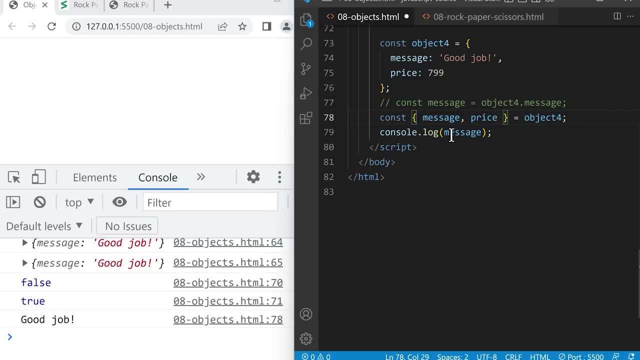 and price. so this will take the price property out of the object and save it in a variable called price. if we console, dot, log the price and save, it will display 799. so that's the destructuring shortcut. it's an easier way to take properties out of an object. 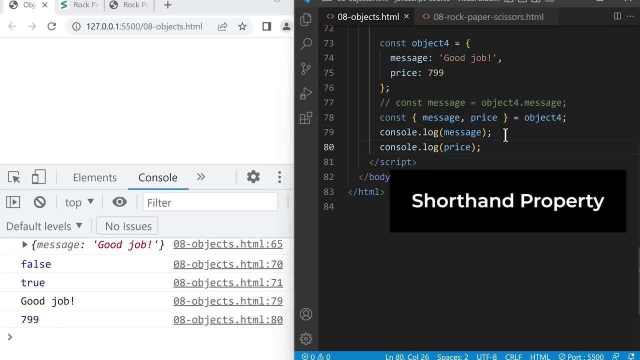 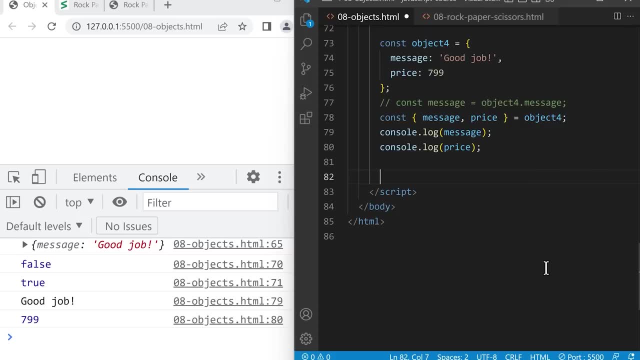 the next shortcut we're going to learn is called the shorthand property. so at the bottom let's create some new lines and let's say we want to create a new object. so we'll type const and let's name this object 5 and we'll make it equal to an object. 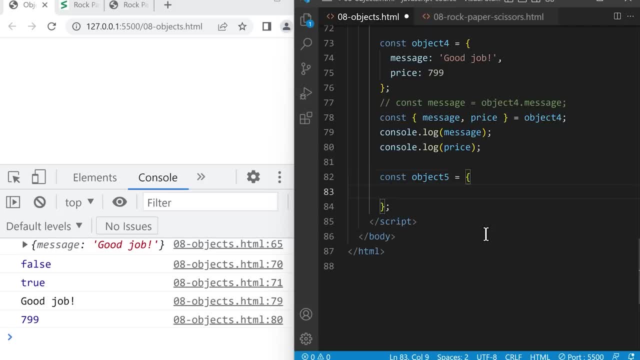 and inside this object. let's say we want to create a message property, so we'll type message colon and for the value let's type the variable message. so what this does is that it takes whatever is inside the message variable and substitutes it into this code. so at the bottom, if we consolelog object five and save. 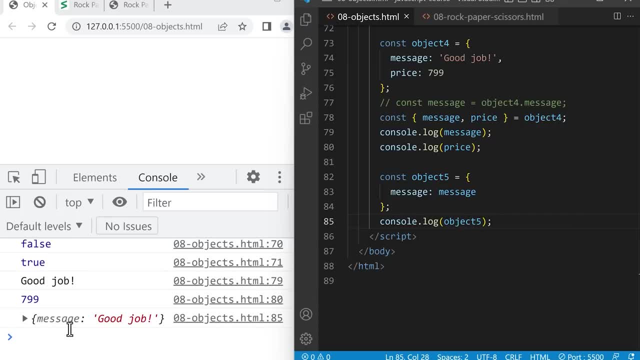 this object will have a property called message And the value is whatever is inside the message variable, which is good job. So now we actually have a shortcut for this code. If the property and the variable name are the same, we can actually just type it out once like message. 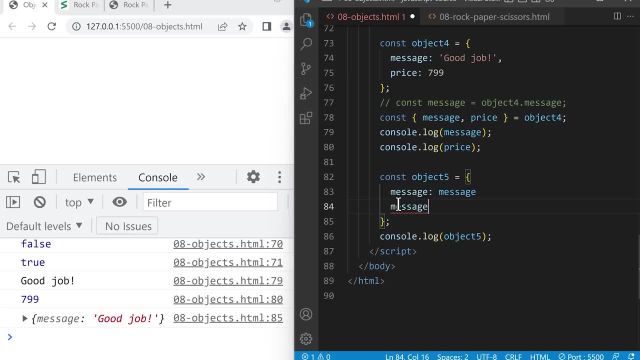 So this code does the same thing as message, colon message, And this shortcut is called the shorthand property. So if we comment out this line using double slash and save, you can see that this shortcut creates the same object that we had before. The last shortcut we're going to learn is called the shorthand method. 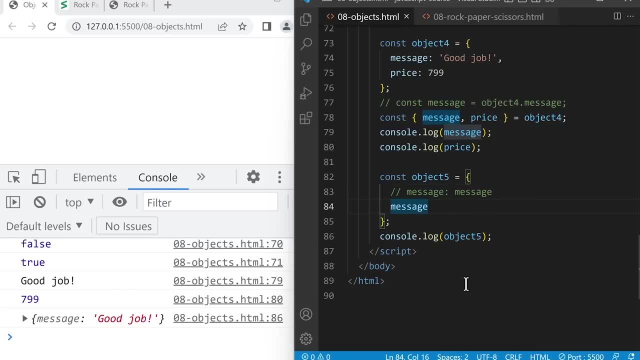 So at the end let's create a new property, comma, and we're going to say: and let's name it method, colon, and we'll save a function in this property. So we'll type function and let's name it function1, brackets and curly brackets. 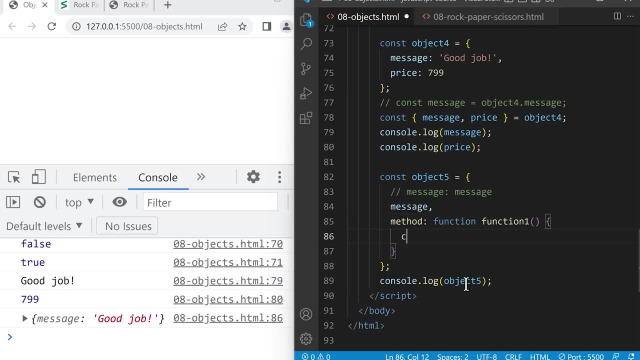 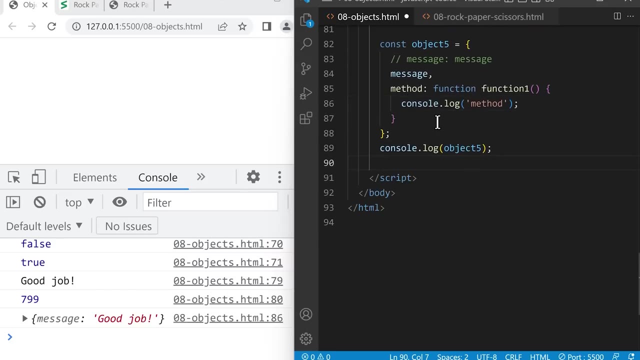 And inside this function, let's consolelog method. And now here at the bottom, let's run this function by typing object5.method. So this will access this function and we'll run it by typing brackets. If we save, this will run the code in the function and display method in the console. 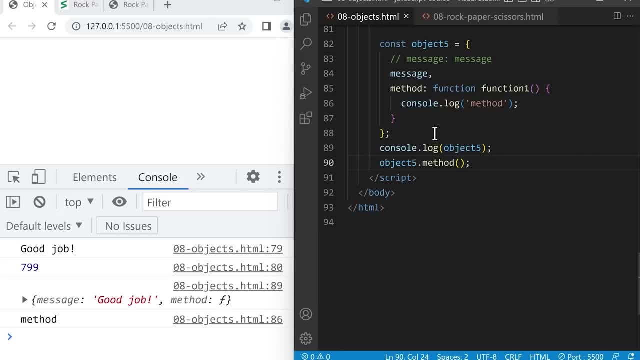 So we actually have a shortcut for writing this. So at the bottom we can type method again and just type brackets and curly brackets: consolelog string method. So this code does the same thing as the code above. So these brackets will create a function, just like here. 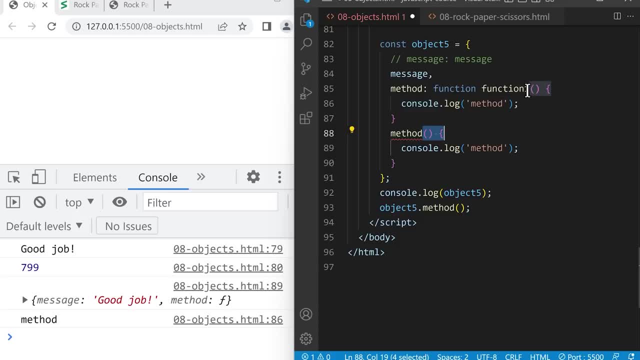 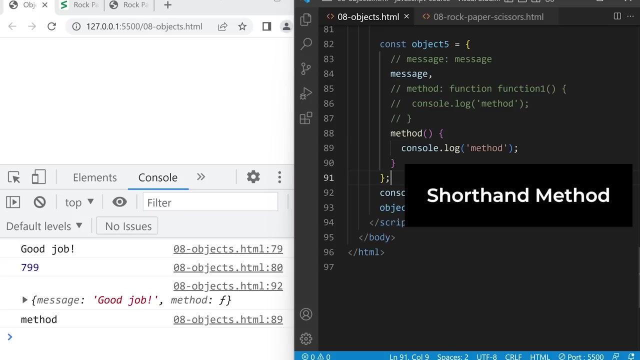 So this function name is actually not needed. So if we comment out these lines of code and save, it will still display method in the console because this is a shortcut for these lines of code. So this shortcut is called the shorthand method syntax. And that's the end of this lesson. 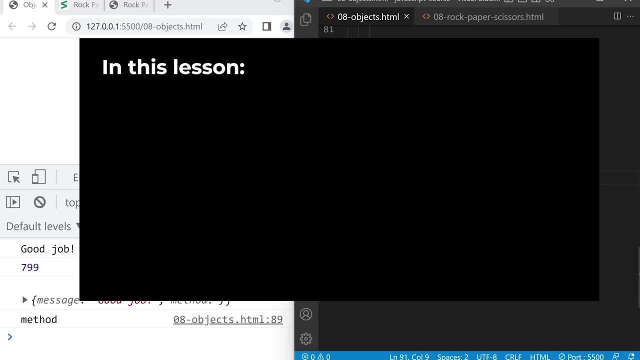 In this lesson we learned another type of value called objects- Objects group related values. together We added a score to our rock-paper-scissors game. We learned about built-in objects and used the JSON and local storage objects to save our score more permanently. 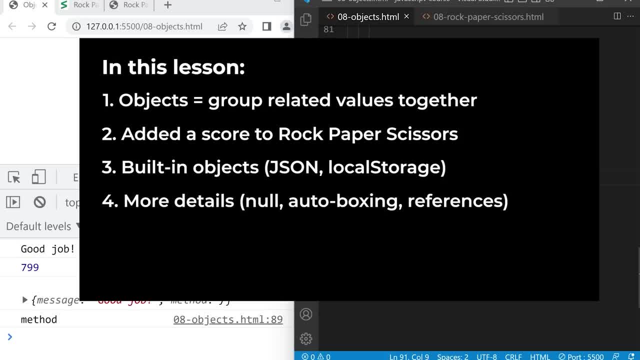 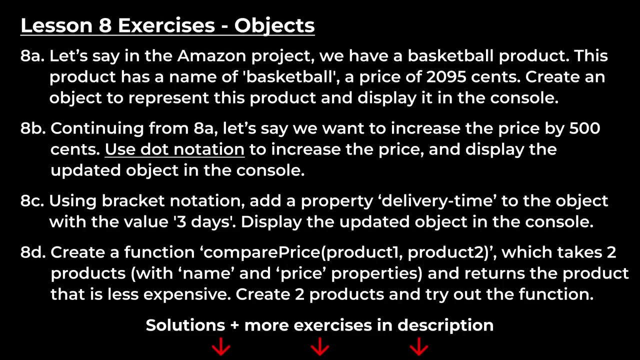 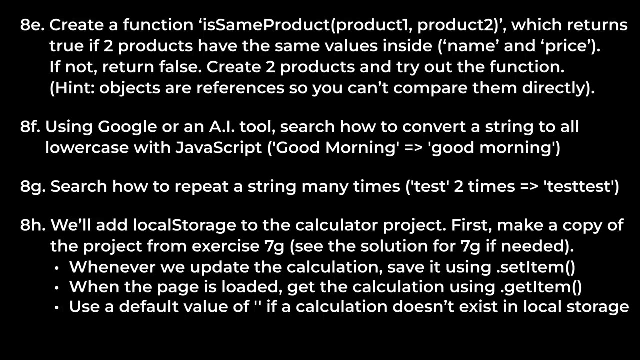 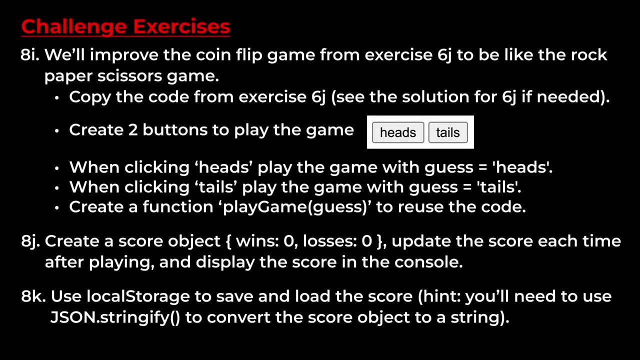 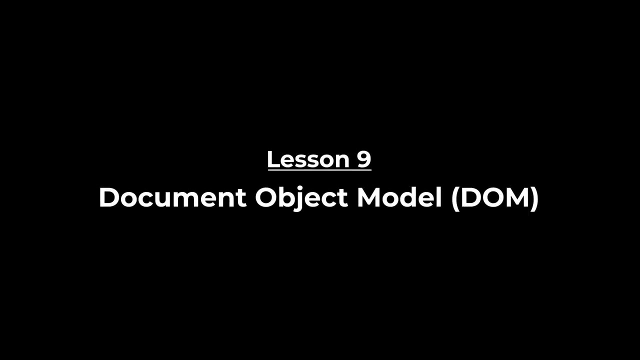 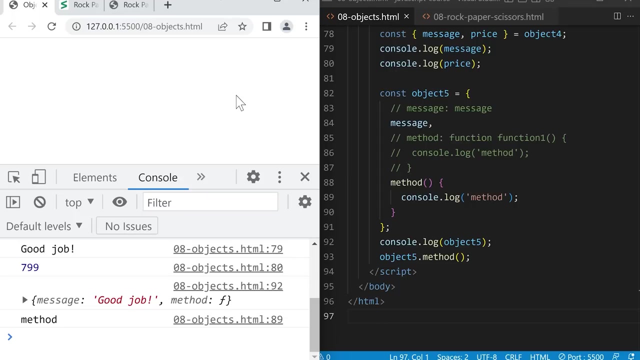 We learned more details about objects like null, autoboxing and references, And we learned some useful shortcuts like destructuring shorthand properties and shorthand methods. Here are some exercises to help you practice working with objects. In this lesson, we're going to learn one of the most important features of JavaScript. 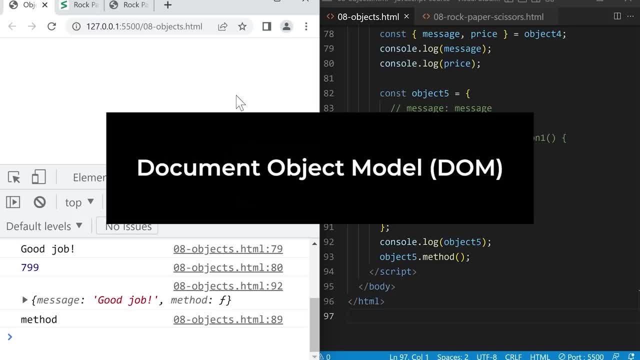 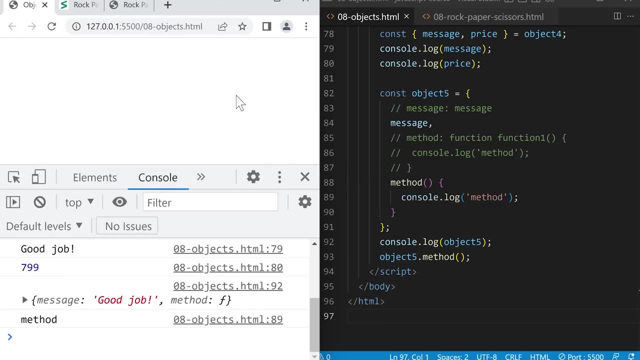 called the Document Object Model or the DOM, And we're going to use the DOM to improve our rock-paper-scissors project. So first we'll create a new file for this lesson. Let's go to our code editor and click this icon to show our files. 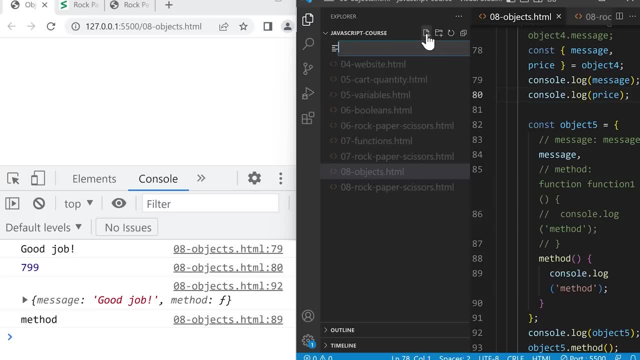 And then click this icon to create a new file, And then click this icon to show our files, And then click this icon to create a new file, And then click this icon to create a new file And we'll name this file 09-DOMHTML. 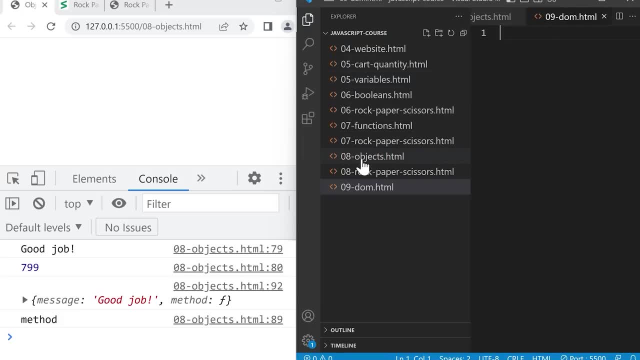 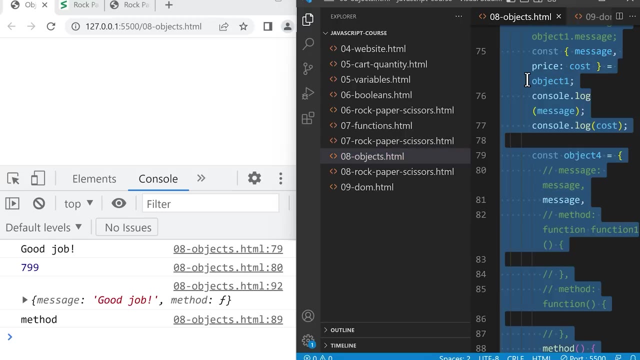 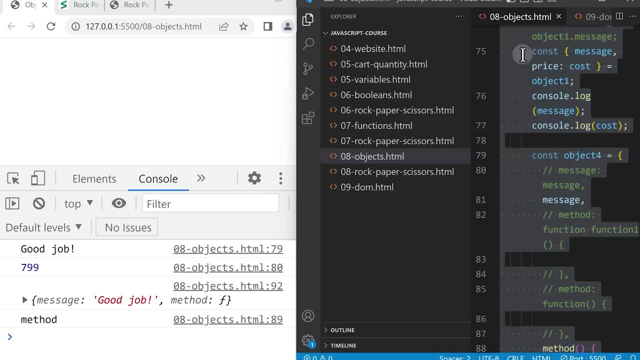 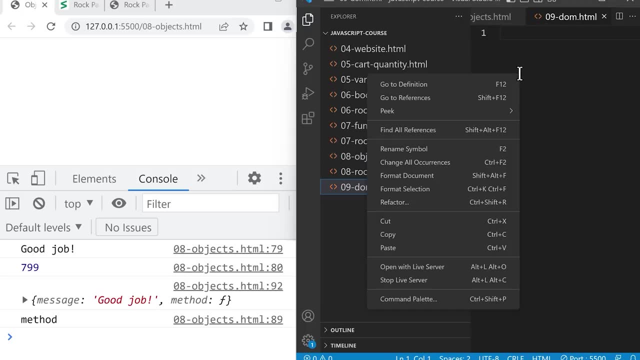 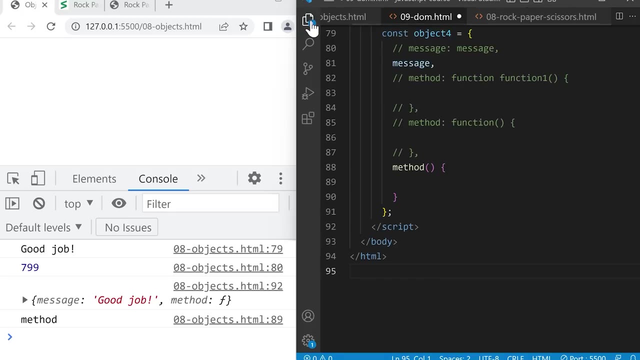 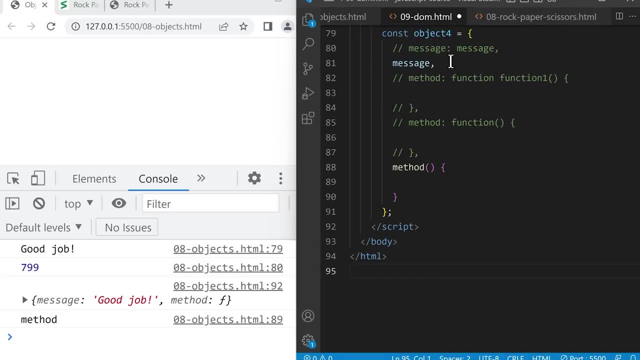 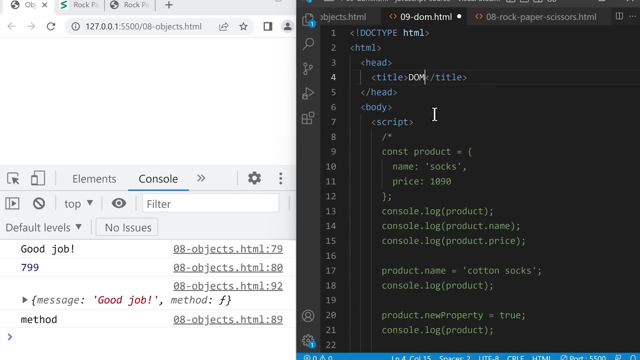 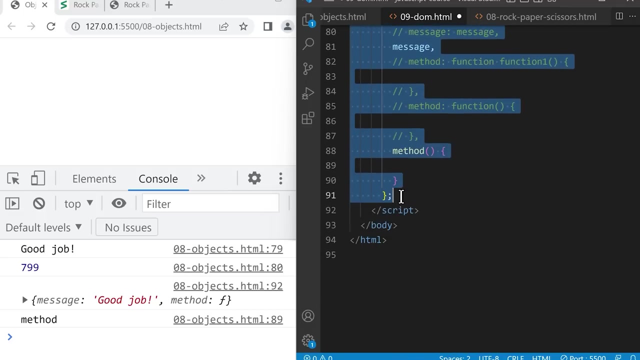 and we'll prepare this file for this lesson. So let's scroll to the top and we'll change the title to DOM and let's delete all these files. and we'll change the title to DOM and let's delete all these files. Now let's save this file. 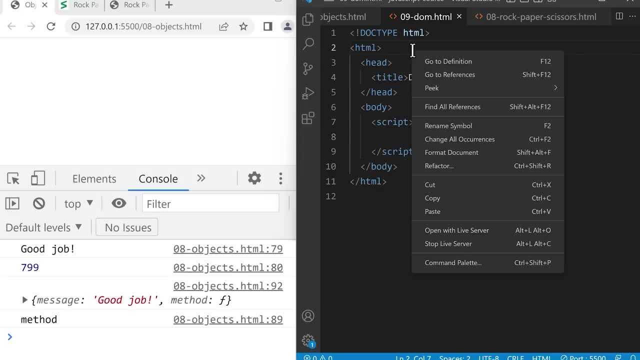 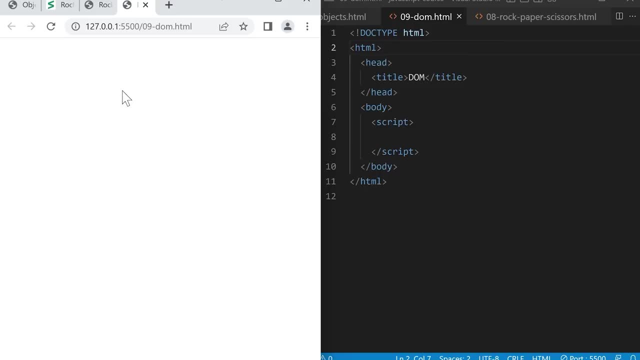 and we'll open it in the browser by right-clicking Open with Live Server And let's also open the console on this page. We'll right-click, click Inspect and then click the console, and then click the console, And now we can close the previous tabs as well as the previous code for now. 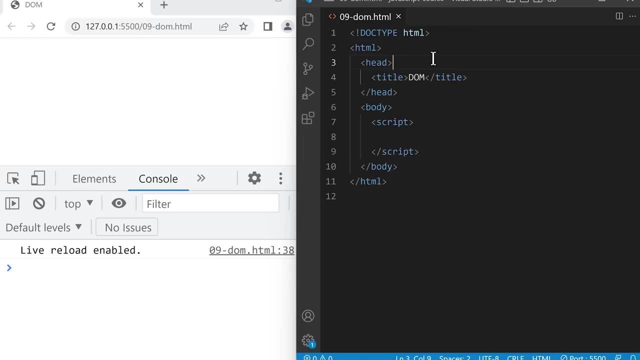 And for this lesson we're going to do an extra step in the setup. Inside the body we're going to create a button. So here let's type the code less than, button, greater than, And inside the button we'll have the text hello. 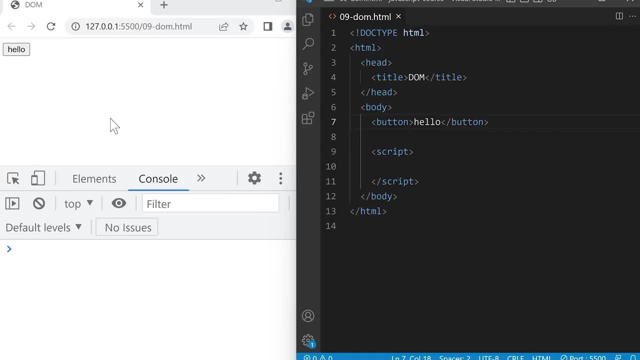 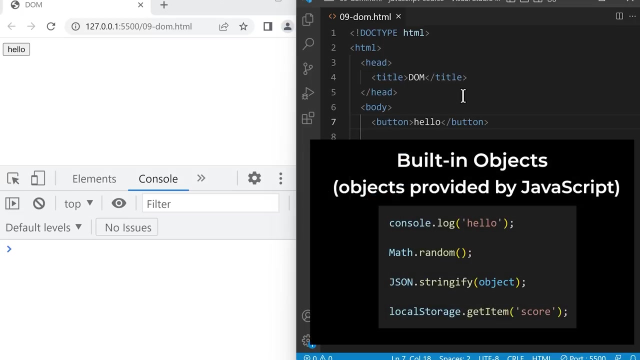 Now let's save, and we should have a button on the page, And now we're ready to learn the document, object model or the DOM. In the previous lesson we learned about objects, which group multiple values together. We also learned about built-in objects, which are objects that are provided by. 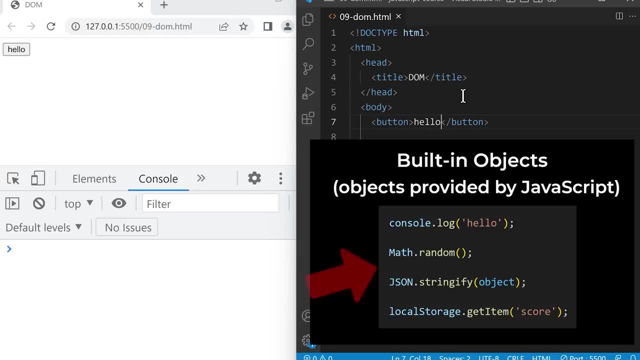 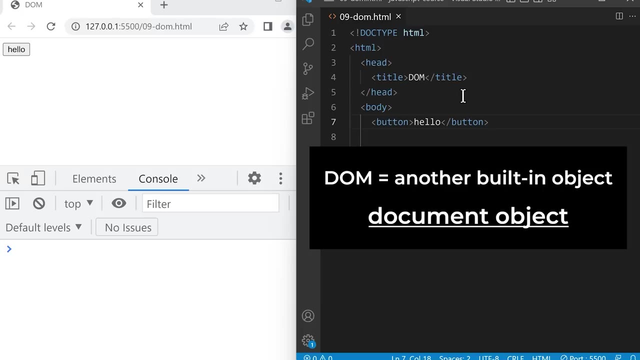 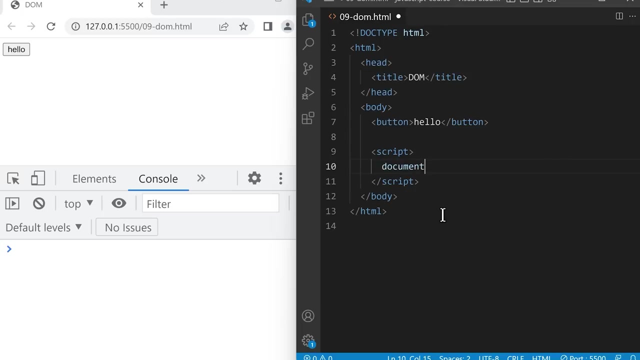 JavaScript. Some examples of built-in objects are console math, JSON and local storage. The DOM is another built-in object called the document object. So let's go to our script element and we're going to type document. So this is a built-in object provided by JavaScript. 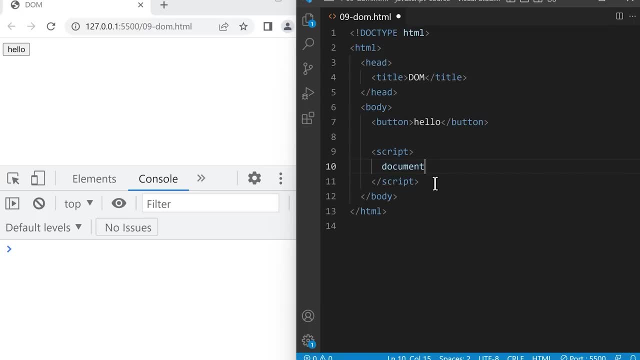 And we've actually seen this document object before. In the first lesson, one of the first pieces of code that we learned was document dot, body dot, inner capital. HTML equals the string hello and semicolon. So this code removes everything on the page And replaces it with the text hello. 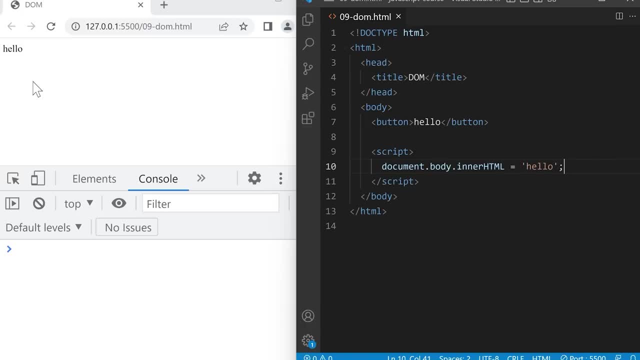 If we save, it will remove the button and just put hello. And now that we learned objects in the previous lesson, we can fully understand this syntax Document. here is a built-in object And this is the dot notation. This means we're accessing a property of the document. object. 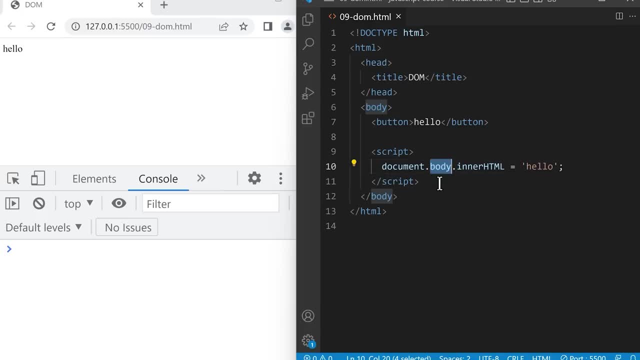 Called body. Now body is also an object, So we can use the dot notation again to access a property of the body object called inner HTML. And finally we use an equal sign to change the inner HTML property to the string hello. But as you can see, there's something very special about the inner HTML property. 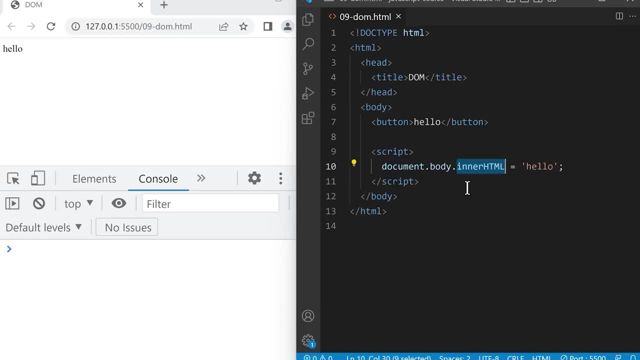 It's that it's not just a dot. It's that it's a dot Right. It's that it's just an XML property. When we change this property, it also changes the web page. So this document object and the web page are linked together. 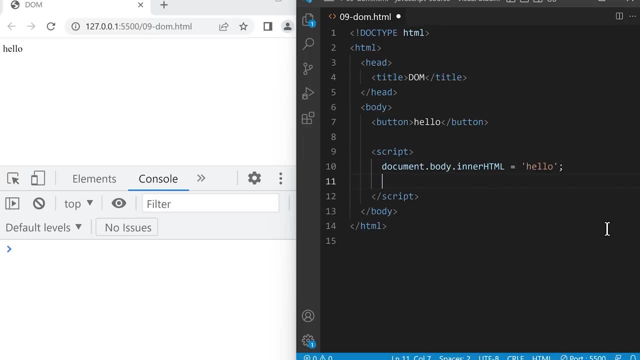 Let's do another example. We'll go to the end here and press enter and we'll type the document object again And we'll use the dot notation again. And this time let's access the property and we'll change the title property using an equal sign. 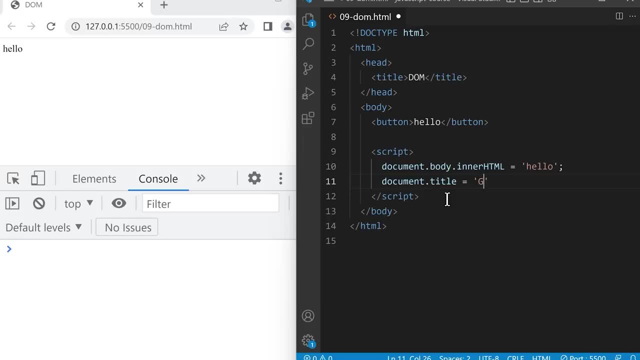 and we'll change it to the string. good job. If we save, changing the title property will also change the title at the top of the tabs here. So now this says good job Again. as you can see, the document object is linked to the web page. 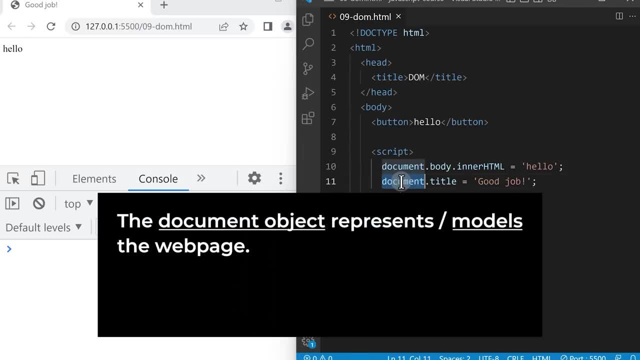 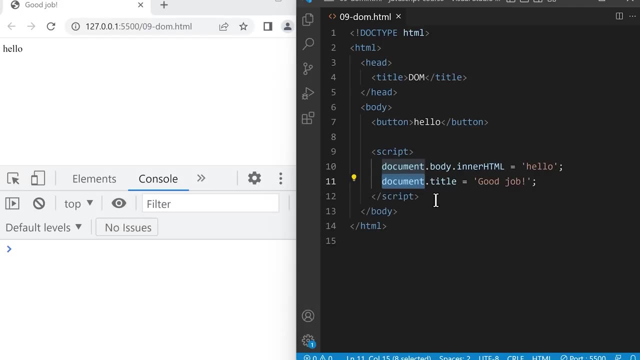 So from these examples, it shows us that the document object represents or models the web page, And that's why we call this feature the document object model or the DOM. Now that we know what the DOM means, let's learn the syntax rules for this. 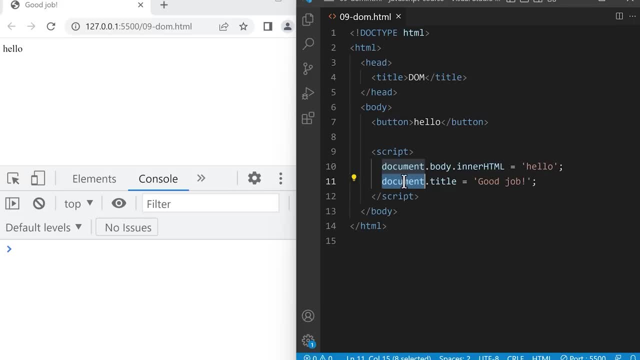 So the DOM is just this built-in document object, And this object works the same way as any other object. It contains properties like body and title that we can access using the dot notation. Now, the special thing about the document object is that it is linked to the web page. 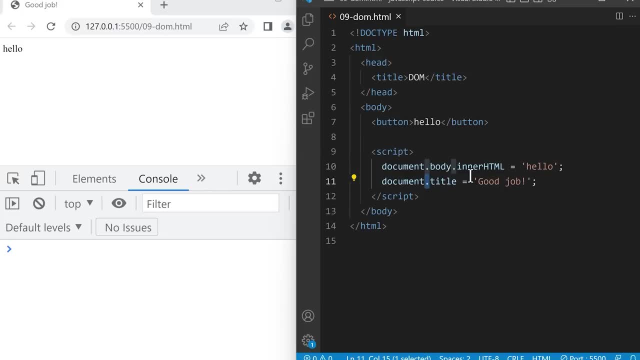 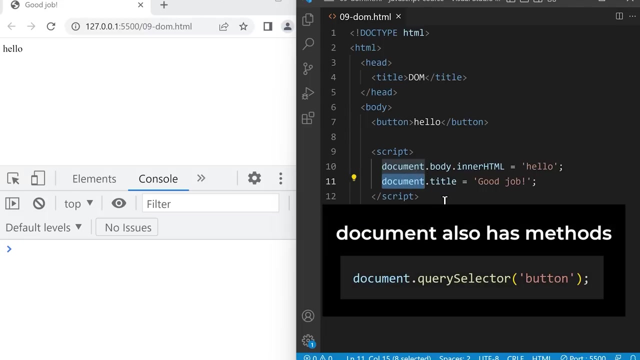 That means if we change certain properties in this object, it will also change the web page. Now, in addition to properties, the document object also has methods we can use, And we'll learn about them later in this lesson, Now that we understand the syntax of the document object, 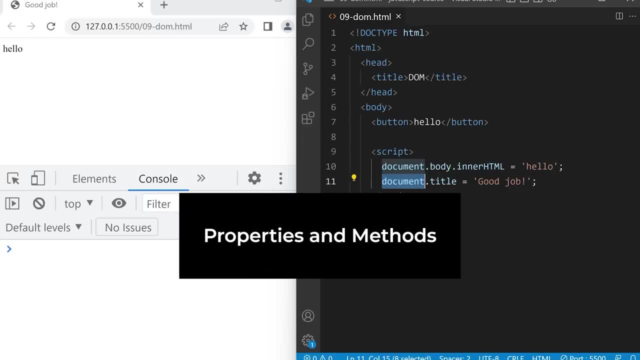 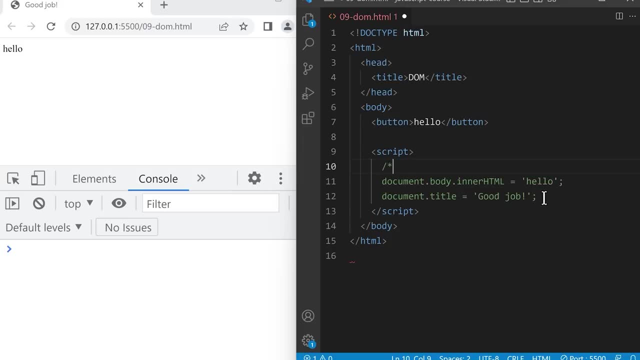 let's learn about the properties and methods we can use. First, let's comment out this previous code using slash, star, star, slash, And we'll create some new lines at the top. So the first property we're going to learn is called documenttitle. 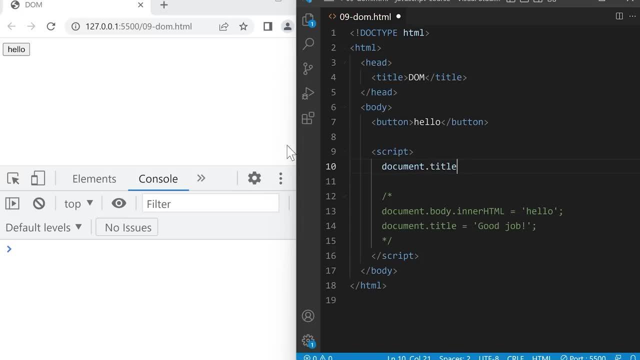 So this property will give us the title at the top of the tabs here. So if we consolelog this property, consolelog and save, this will give us the text at the top, which is DOM, and that's what gets displayed in the console. 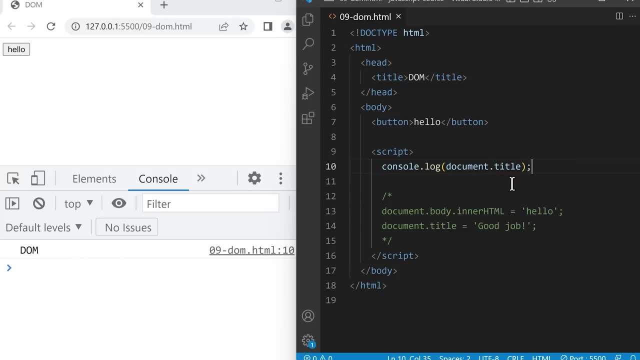 If we change the documenttitle property it will change the text at the top of the tab. So here, if we type documenttitle and make it equal to the string changed and save, now the title at the top of the tab will be changed. 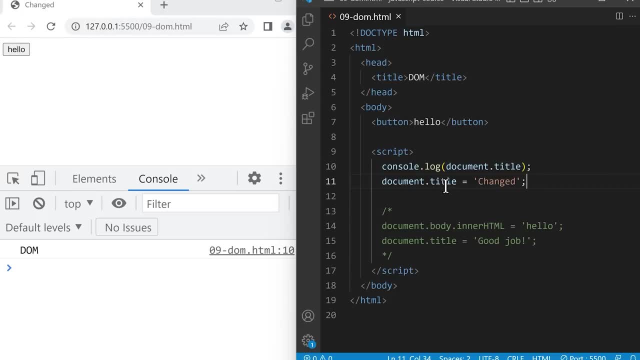 So, as you can see, the title property is linked to the title at the top of the tab. We can use it to get the title and we can also use it to change the title. Next, we're going to learn another property called. 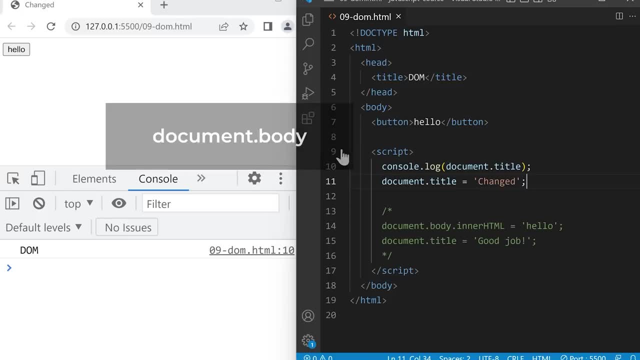 documentbot. So let's go into our code and let's type documentbody. Now documentbody is a very special property, So this will literally get this body HTML element and put it inside our JavaScript. So let's actually consolelog this. 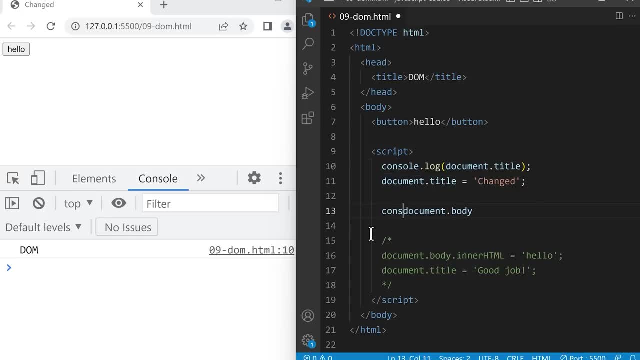 to see how it works, consolelog and then close, bracket and save And inside the console it will tell us that documentbody is the body HTML element And if I hover over this it will tell us that it is exactly the body on our page. 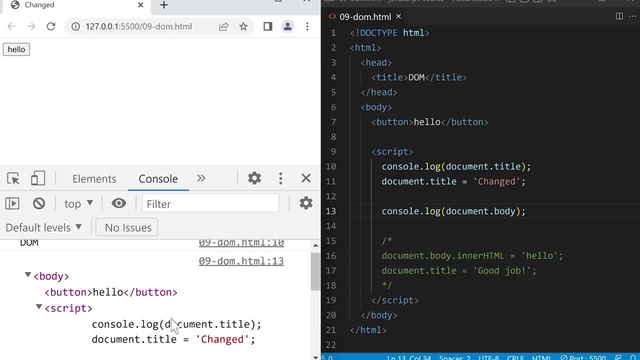 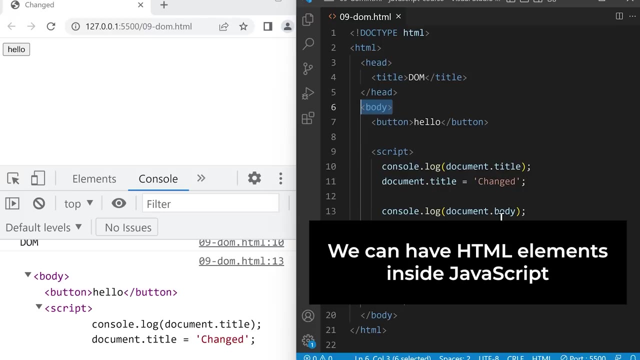 If I expand this, we can see that this code is exactly the code that we have here, And this shows us one of the most important features of JavaScript: We can have HTML elements inside JavaScript. The document object or the DOM combines JavaScript and HTML together. 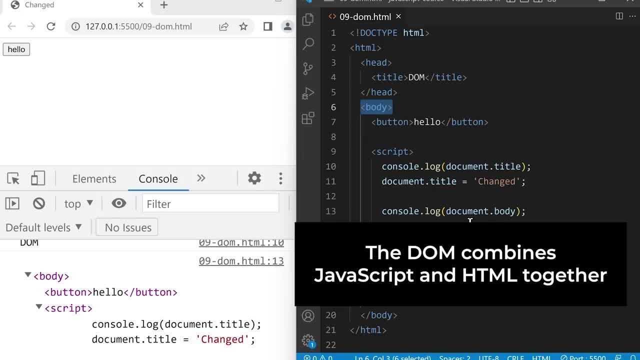 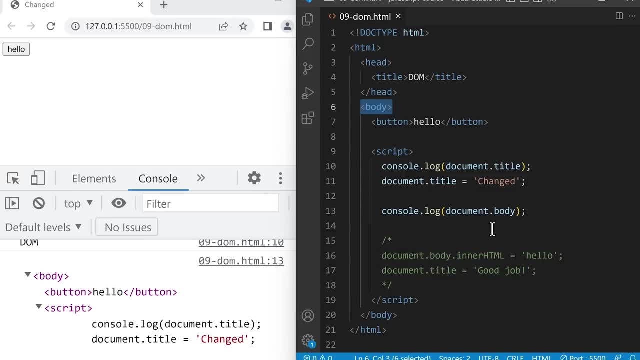 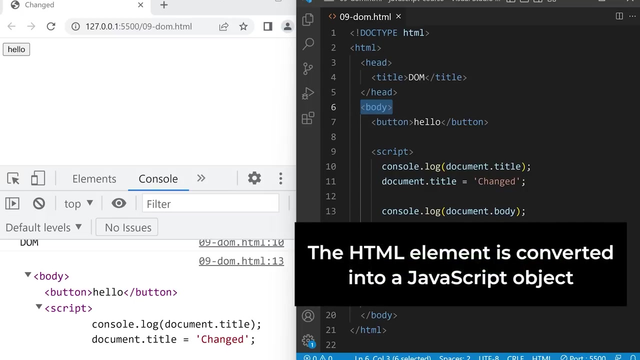 and it gives JavaScript control of the web page. Okay, So now that we have an HTML element inside our JavaScript, what can we do with it? A really important thing to know is that when an HTML element is inside our JavaScript like this, the HTML element is converted into a JavaScript object. 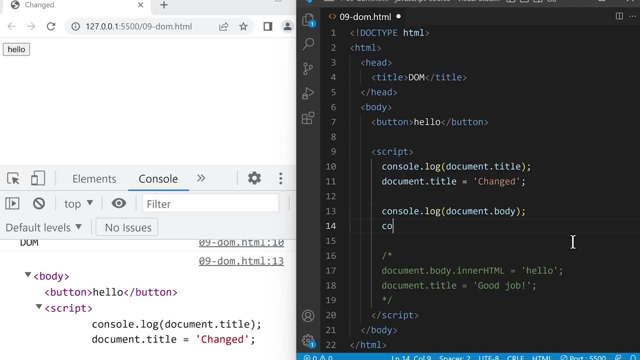 So, for example, if we do consolelog type of documentbody and save, it will tell us that the body HTML element is just an object when it's inside JavaScript. So, just like any other object, this has properties and methods we can use. 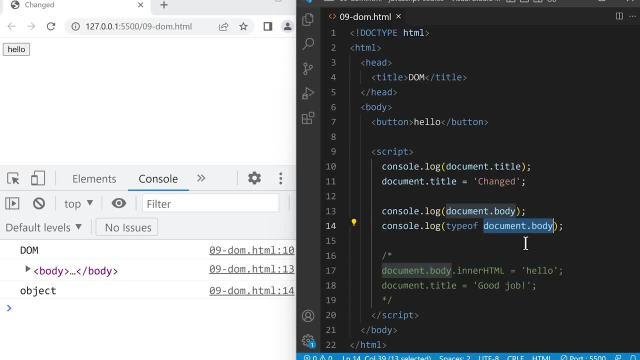 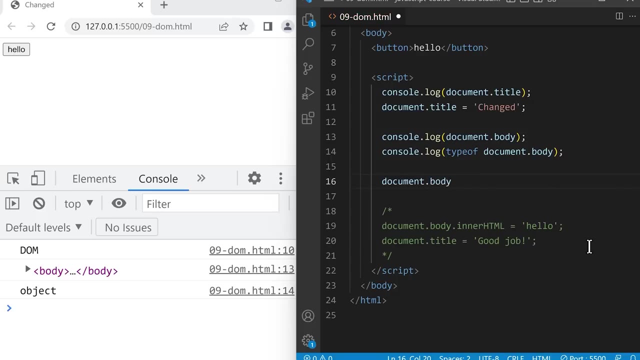 So one useful property of the body element is innerHTML, which we saw earlier. So down here let's type documentbodyinnerHTML. So the innerHTML property controls all the HTML inside the body. That's why it's called innerHTML. So if we access this property, 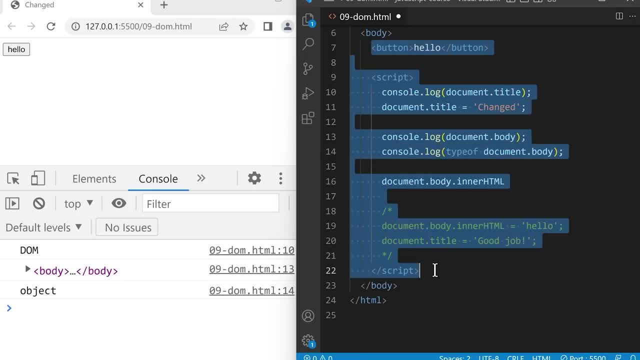 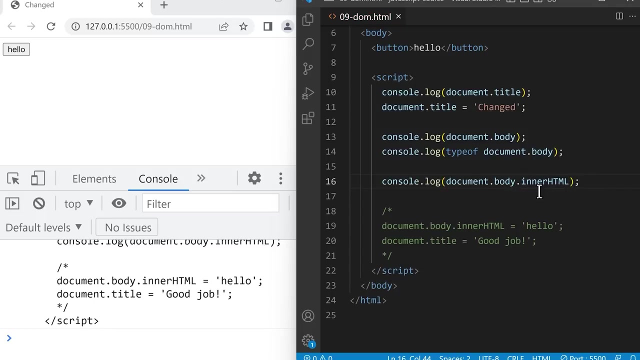 it will give us all the HTML inside the body. So let's consolelog to confirm, consolelog and save, and innerHTML will give us all of this HTML inside the body element And if we change the innerHTML property it will change the HTML. 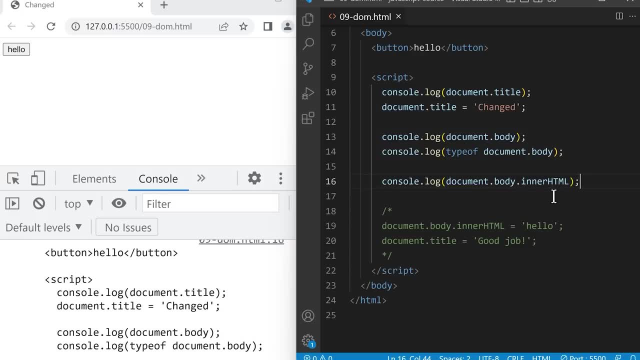 inside the body element. So let's create a new line and we'll type documentbodyinnerHTML and we'll change it to the string changed. So this will replace all of the HTML inside the body with the text changed. If we save, that's exactly what it does. 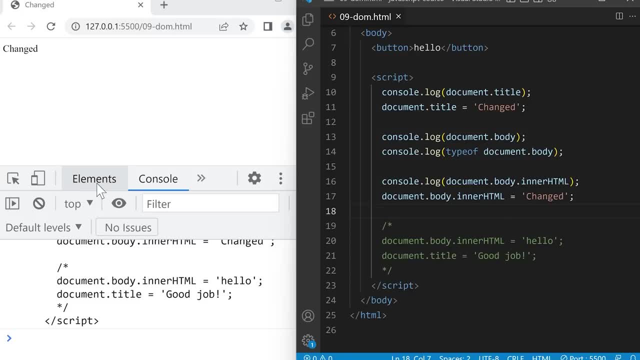 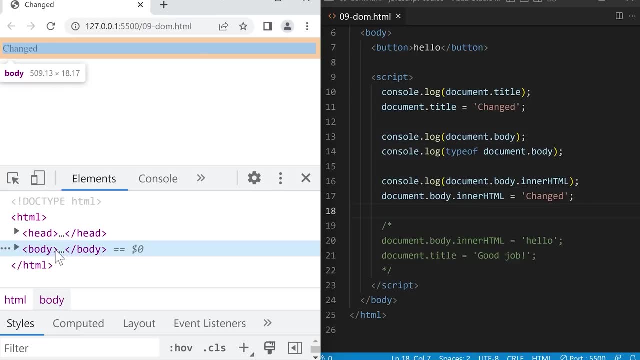 And we can actually confirm this by going into the elements tab. So this tab is for HTML and CSS. We can find the body element, expand it and you can see all of the HTML that we had before was replaced with changed And don't worry about this part. 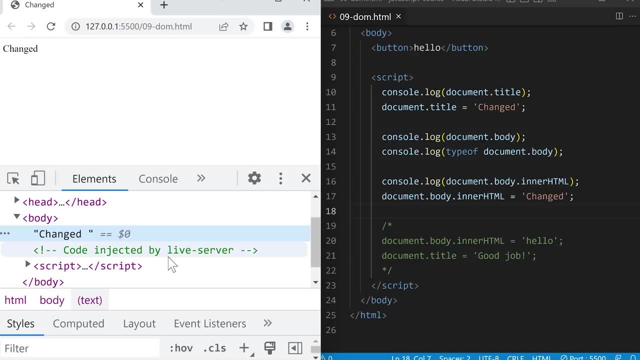 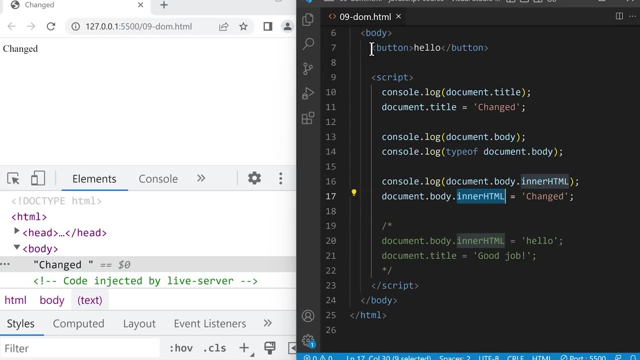 this part is just added by live server after. So this shows that innerHTML gives us control of all the HTML inside the body. We can get this HTML and we can also change this HTML. Now, another feature of innerHTML is that we can replace: 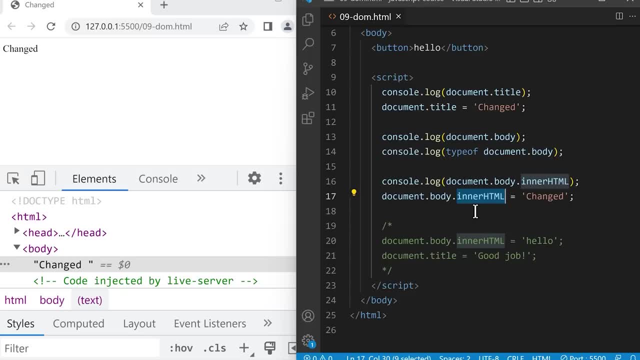 this HTML with new HTML code, not just text. So, for example, instead of just text, we can replace it with a code: less than button greater than, And also less than slash button greater than. So this is HTML code for creating a button. 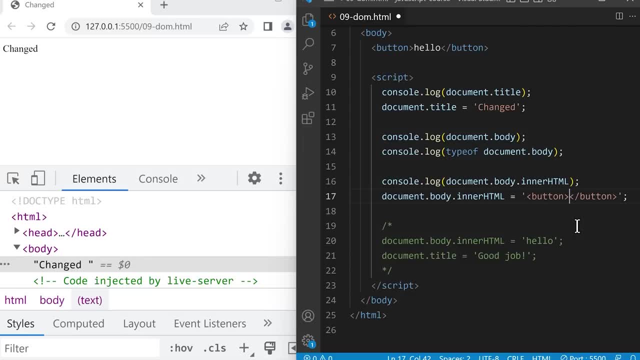 And inside the button let's put the text: good job. And now this code will replace all the HTML inside the body with this new HTML. If we save, it removes all the previous HTML and this new HTML creates this button. So, using this innerHTML property. 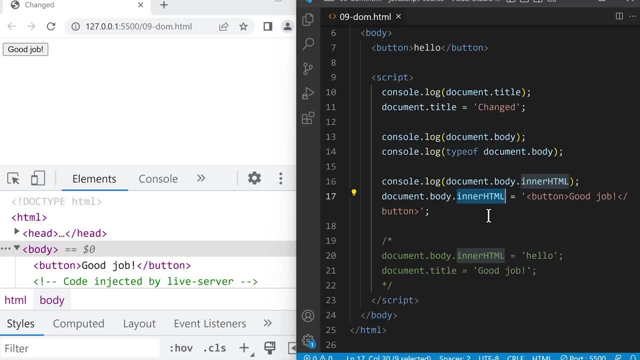 JavaScript can replace the HTML inside the body to whatever we want. We have full control of the web page. Alright, now we're going to learn a method of the document object that we can use As a reminder. a method is a function that is saved. 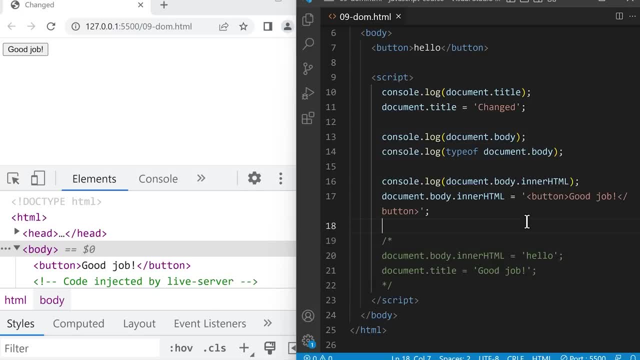 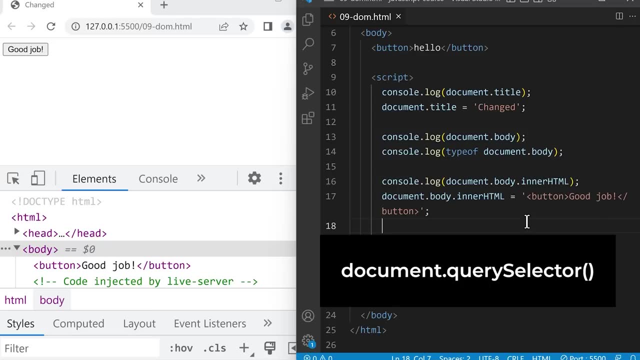 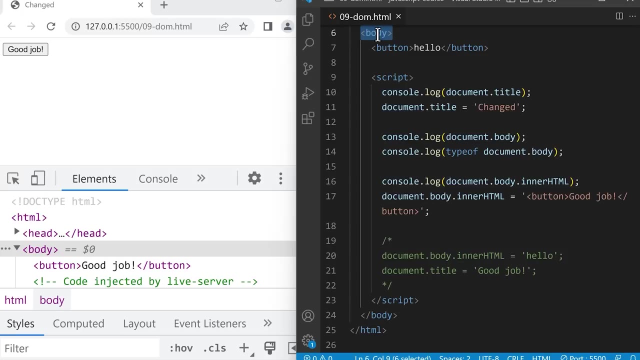 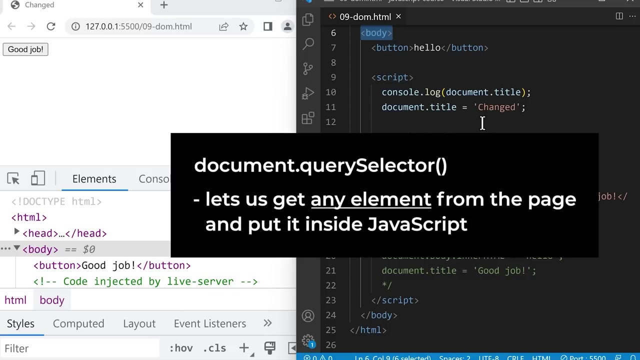 inside an object. So we're going to learn a very important method called documentquerySelector. We just learned that. documentbody lets us get the body element and put it inside our JavaScript. DocumentquerySelector lets us get any element from the page and put it inside our JavaScript. 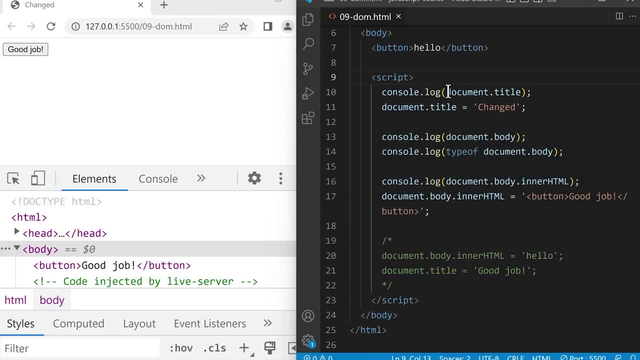 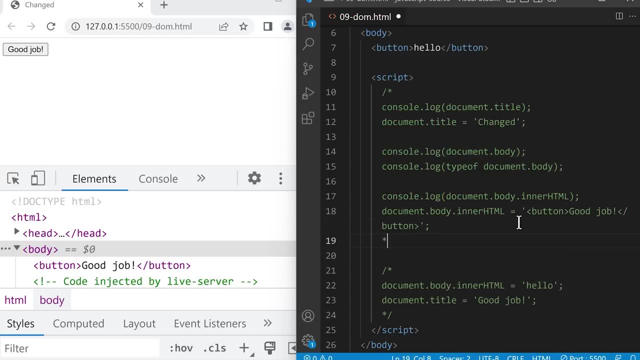 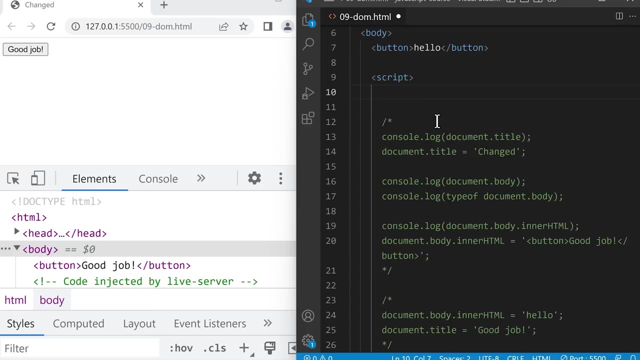 Let's give it a try. So first we'll comment out the previous code using slash, star and star slash. Let's create some new lines at the top And let's type documentquerySselector and brackets. So documentquerySelector- lets us get. 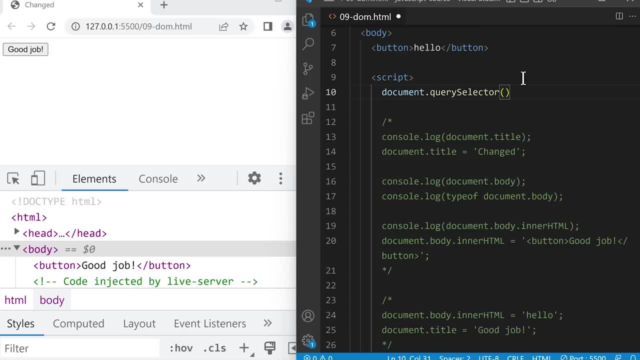 any element from the page and put it inside our JavaScript. Between these brackets we're going to put a string. This string tells JavaScript which HTML element to get from the page. So if we type button, this will get the first button element from the page. 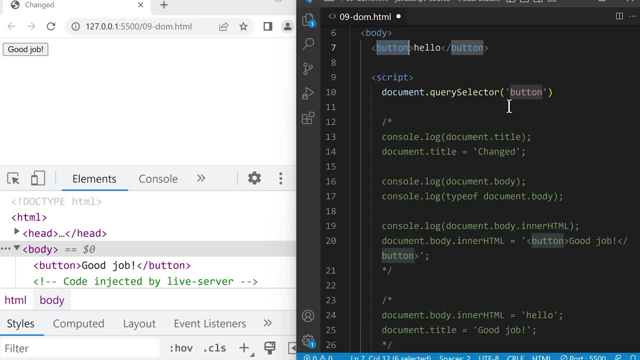 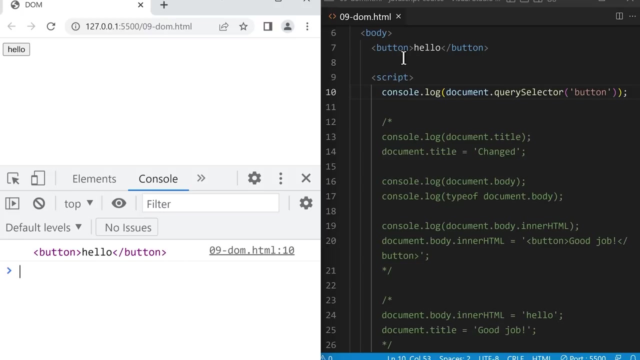 and put it inside our JavaScript. So let's consolelog this to confirm. consolelog this to confirm. So if we close bracket and save and let's go back to our console Now, it will tell us that documentquerySelector got this button element and put it. 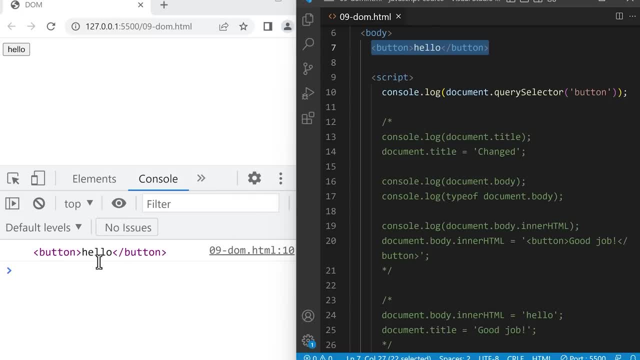 inside our JavaScript, which you can see in the console, And if I hover over this button element, it will tell us that it is exactly the button on the page. So that's what documentquerySelector does: It can get any element from the page and put it. 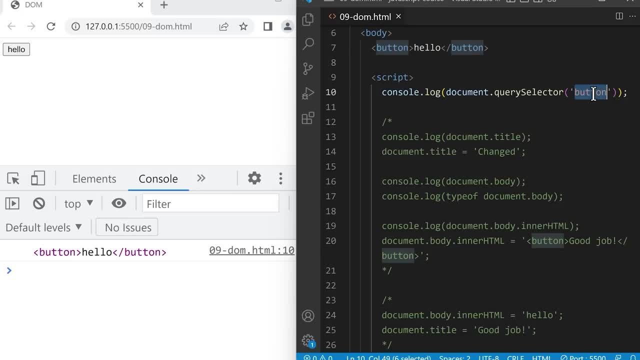 inside our JavaScript. This string tells it which element to get. If we type button, it will get the first button element from the page. If we type body, this will now get the first body element from the page. So it will do the same thing. 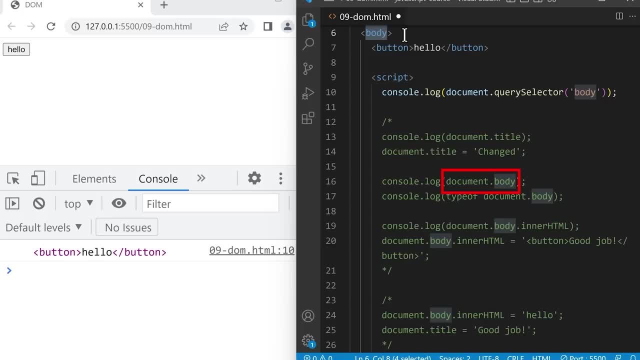 as documentbody. But for now, let's just change this back to button as an example and save. So remember, when an HTML element is inside JavaScript, it's just a JavaScript object. So this button element is also just an object and it has. 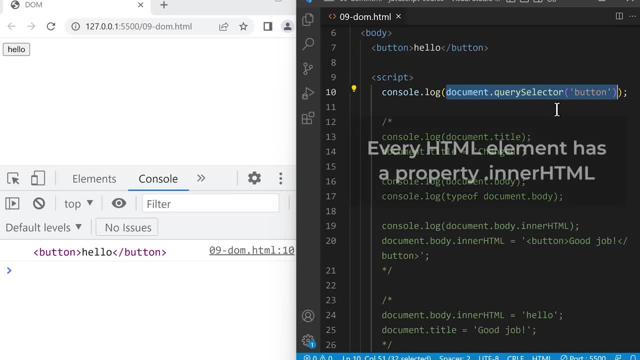 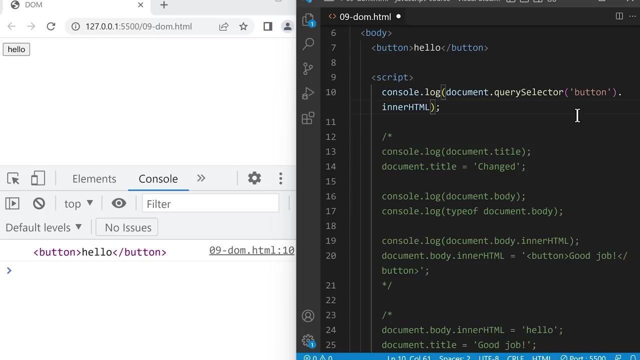 properties and methods we can use. Every HTML element actually has a property called innerHTML, which lets us control the HTML inside the element. So for this button element, let's type at the end innerHTML, and this will give us the HTML inside the button. 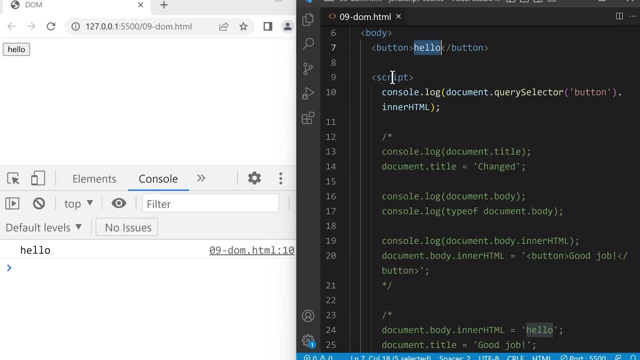 If we save, it will give us hello, And again, if we change the innerHTML property, it will change the HTML inside the button. So let's make a copy of this code. We'll select it and right-click, copy and down here. 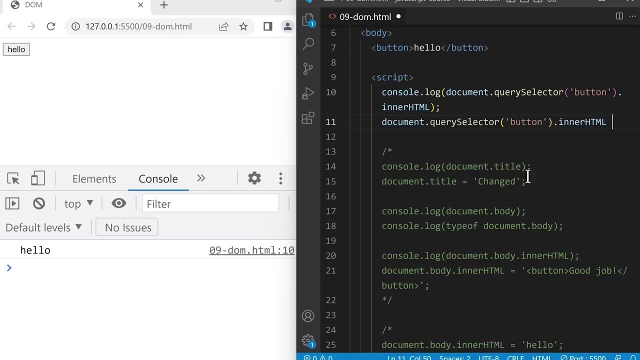 right-click and paste And here we have the innerHTML property using an equal sign and the string changed. So this will only change the HTML inside the button which is here to changed. If we save, we'll see that we can actually. 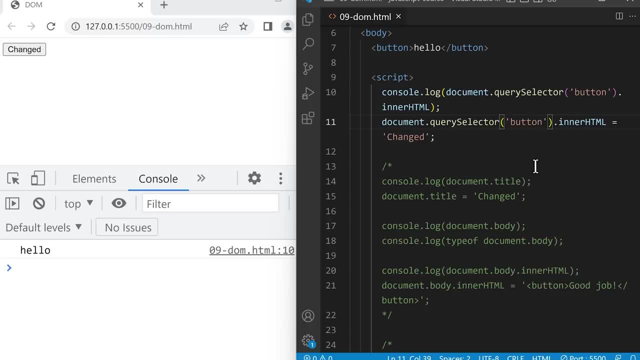 put it on multiple lines So we can type documentqueryselector and then put innerHTML on a separate line to make it easier to read And we can get any element from the page, put it inside our JavaScript and then we can control the. 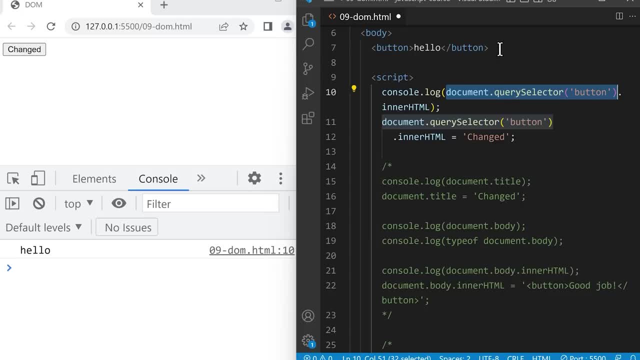 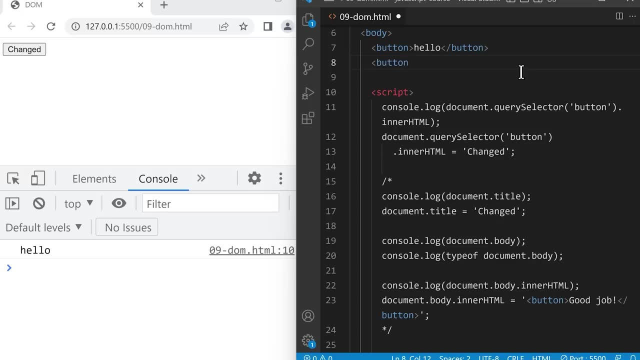 HTML inside that element And this allows us to only have the text second button and save. So now we have two buttons on the page, But documentqueryselector will only get the first button on the page. How do we do that? Let's. 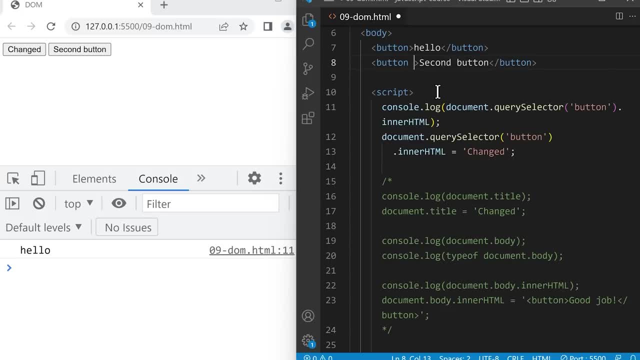 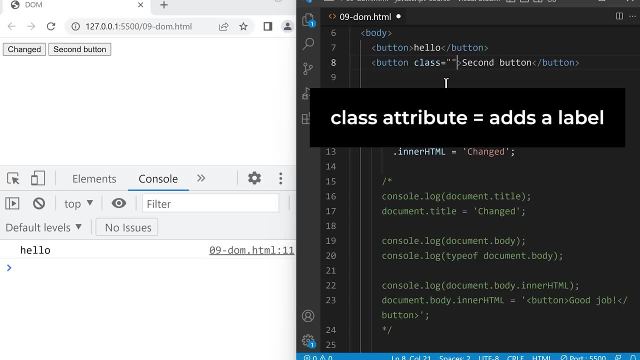 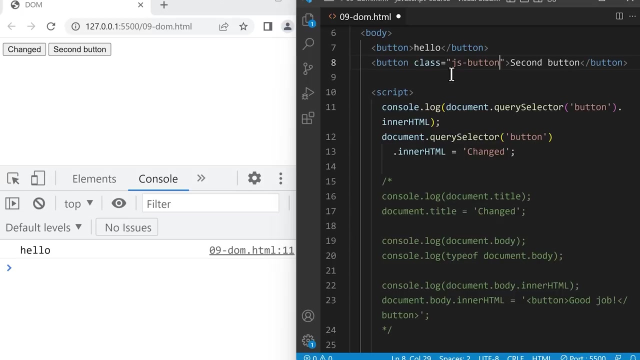 look at the class attribute. So in the opening tag we're going to type space. class equals double quotes, So the class attribute sort of adds a class to the class So we can select it using documentqueryselector. So at the bottom here. 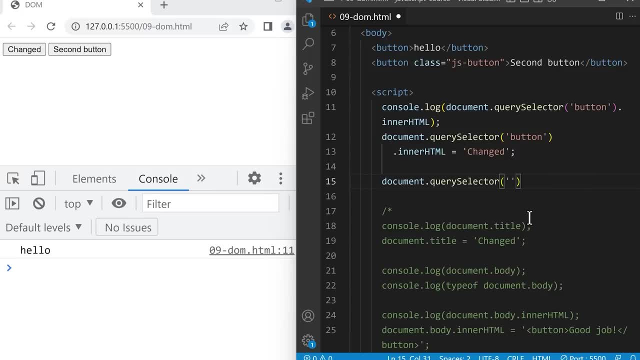 we'll type documentqueryselector again and brackets and we'll type a string inside and in the class rather than an element name. So we're going to look for the class js- button And now documentqueryselector will select an element with the class. 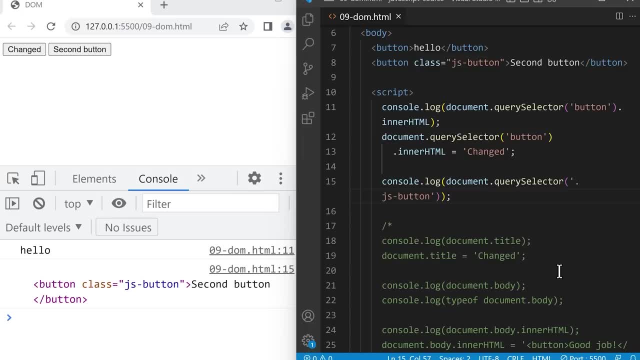 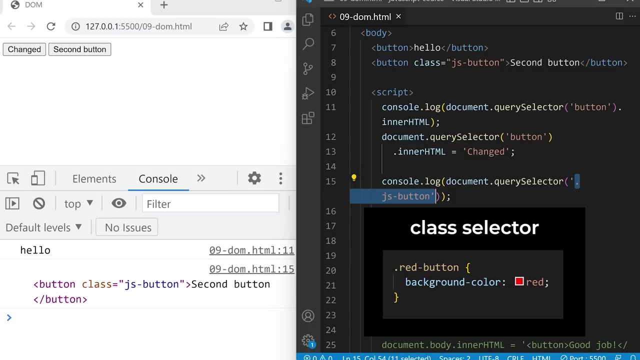 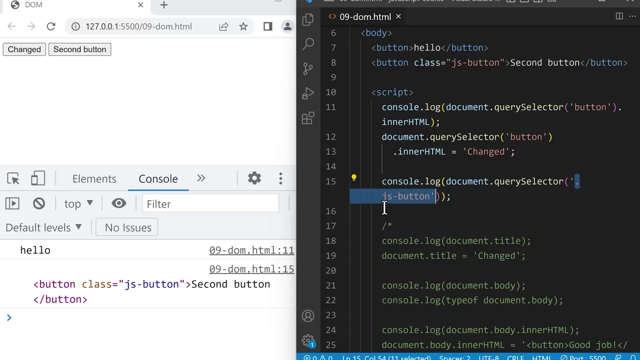 js- and save. And now you will see that this code gives us the second button on the page. So, using a class attribute and then starting with a dot in queryselector, we'll be able to use this string to style elements with a specific. 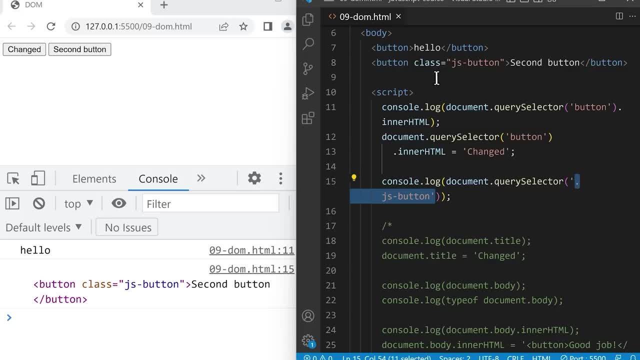 class. In fact, anything we use in CSS can also be used in this string And also this second button is also just an object And, remember, objects are values and we can save them inside a variable. So instead of consolelog. 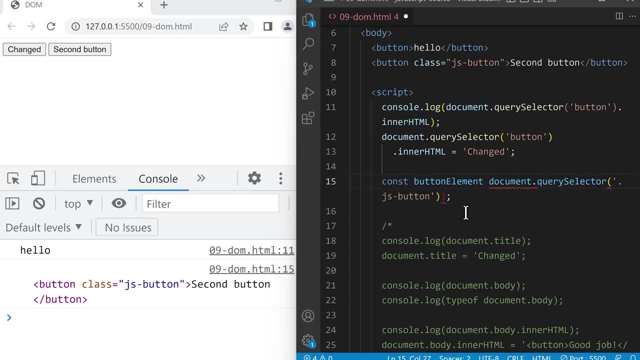 let's create a variable using const with element or lm to make it clear there's an HTML element inside this variable And finally we'll type an equal sign to save this element And we can remove this extra element and save it. It will. 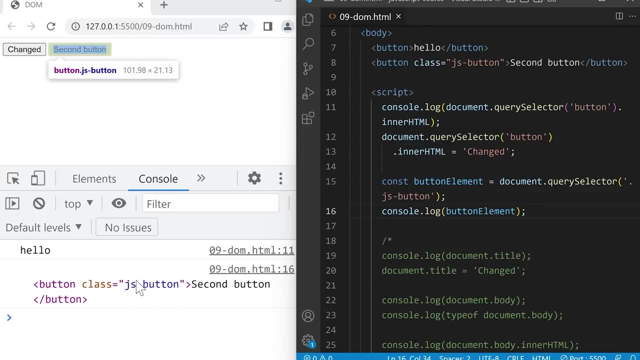 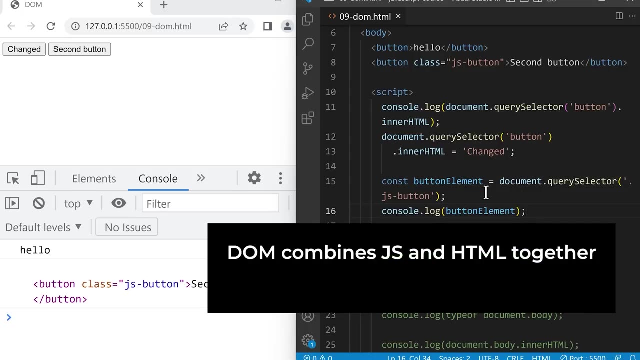 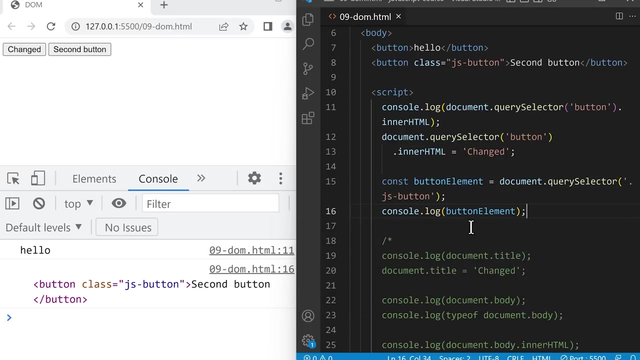 tell us that the second button was saved inside this variable. So, using the DOM, we can get HTML elements from the page. put it inside the page. Alright, now that we learned how to use the DOM, let's do some practical examples. 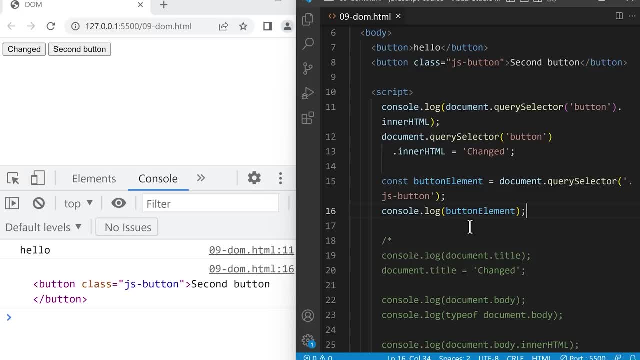 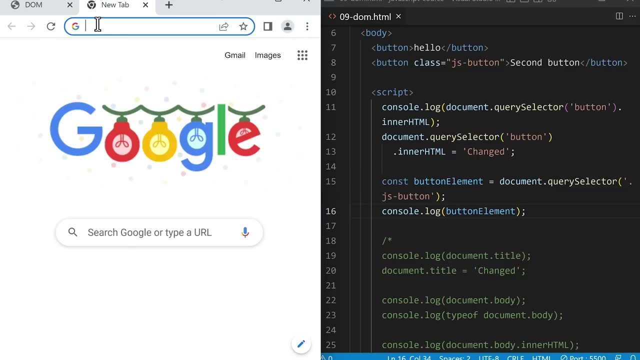 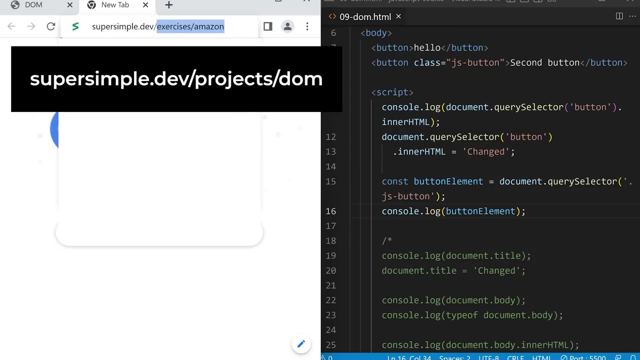 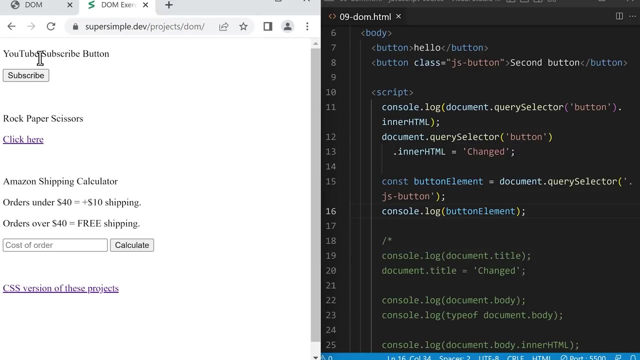 So I've actually prepared some projects that we can do for this lesson. To open these projects, we'll go to our website slash projects, slash DOM and press enter On this page. we'll be working on three projects: The YouTube subscribe button. 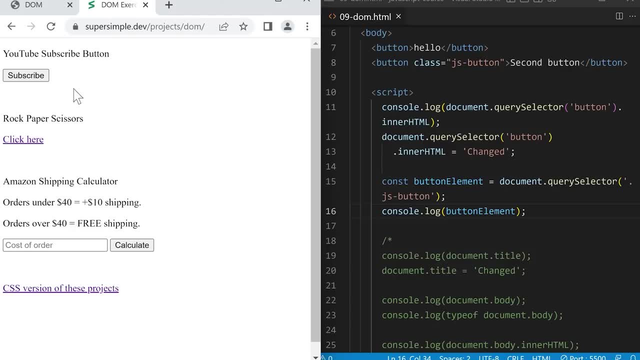 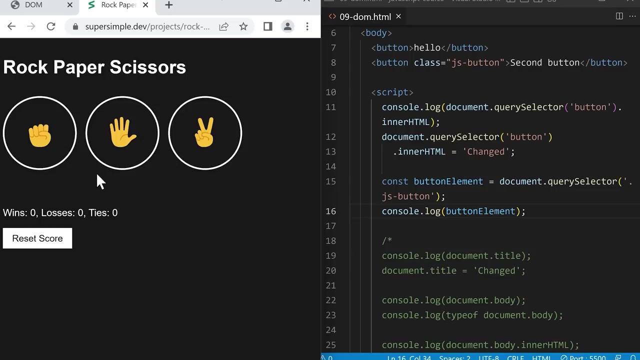 the rock paper scissors project we've been working on for a long time, And in the next lesson we're going to use CSS to style these projects and make them look nice, And you can preview that by clicking on these icons. But for this, 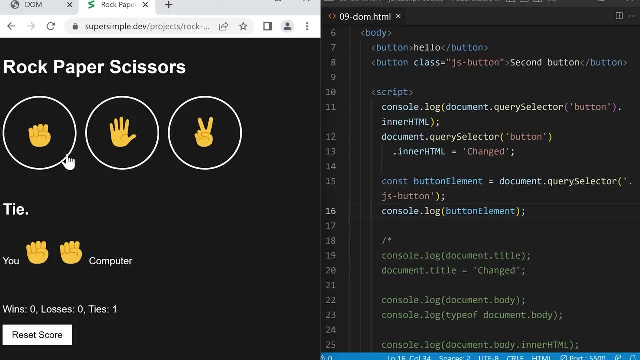 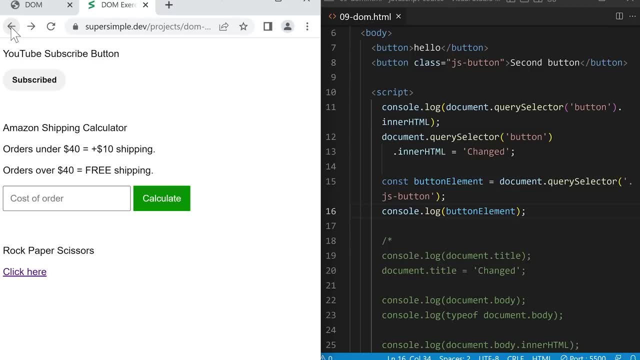 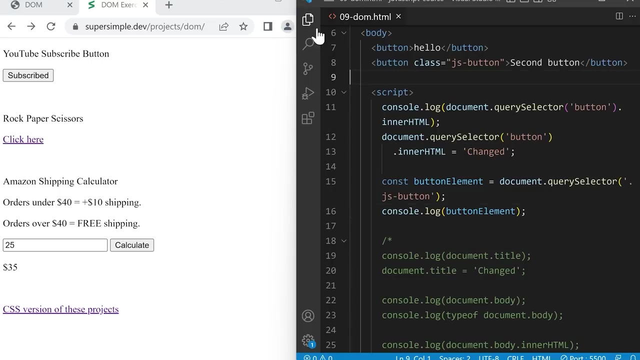 lesson. we're only going to focus on the functionality and not the styling. So let's go back to the projects. We'll click back and click back to create a new file just for these projects. We'll go to our code editor and click. 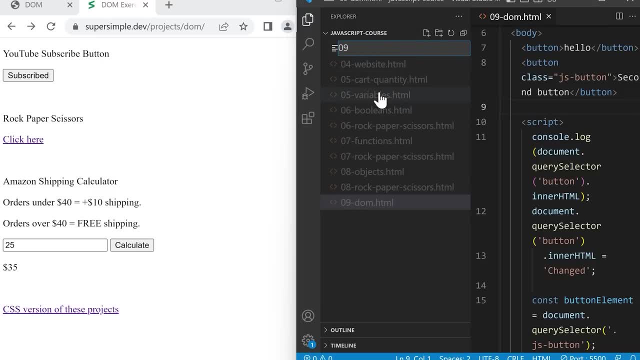 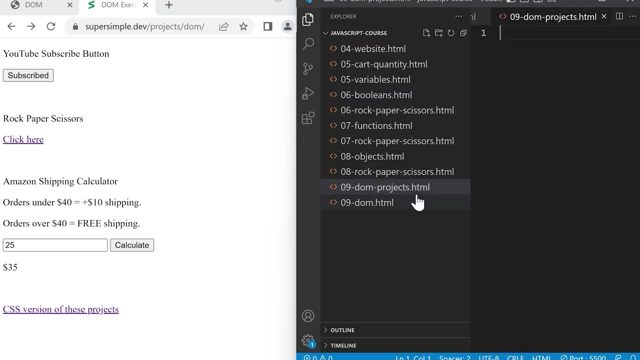 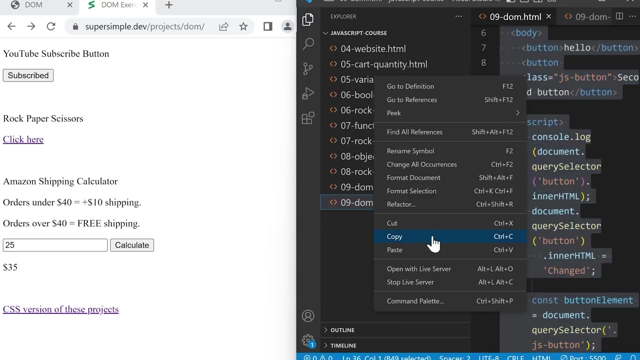 this icon and then click this icon to create a new file. Let's name this file: copy domhtml into this file, So we'll open it and then click in here and type control a or command a to select the code, and then right click copy. 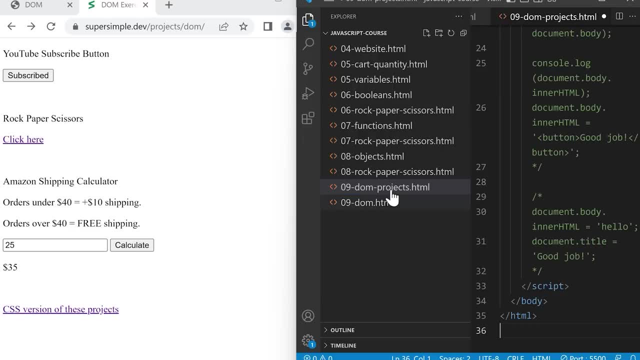 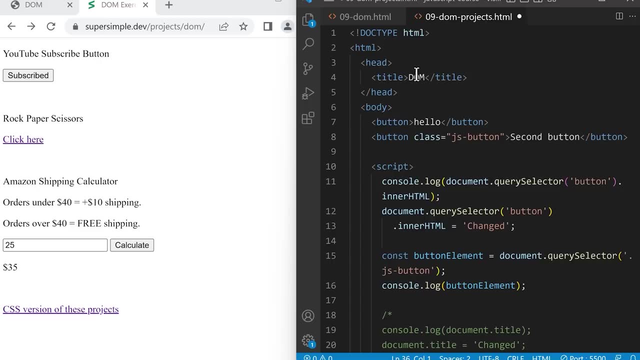 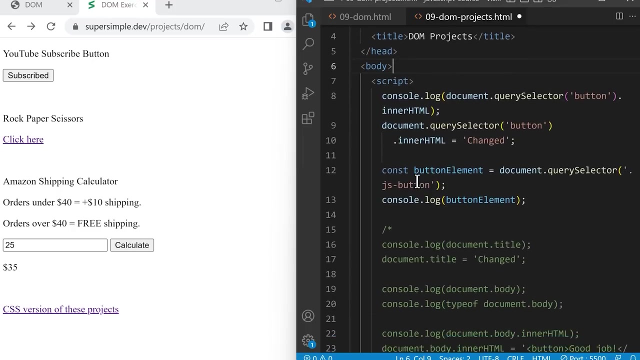 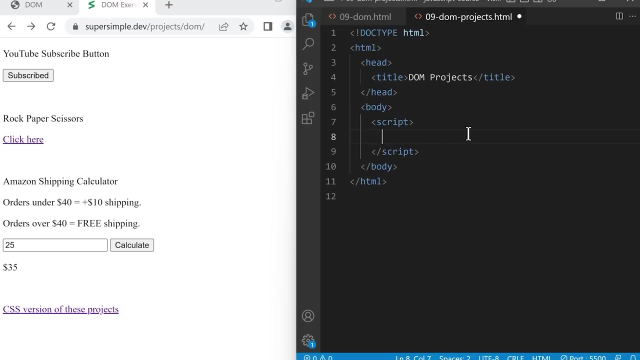 and in here, right click and paste. We'll save this file. so let's scroll up and we'll change the title to dom projects and let's remove our html, but keep the script element and we'll also remove the html from the html and let's 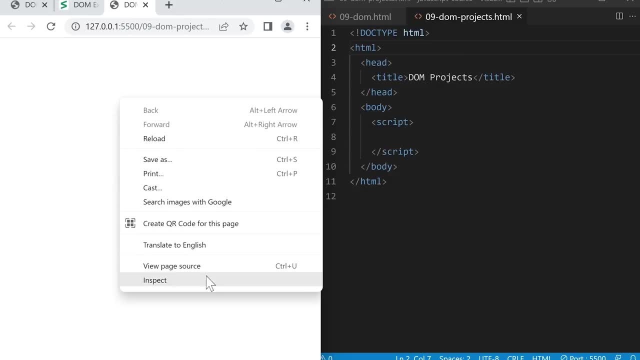 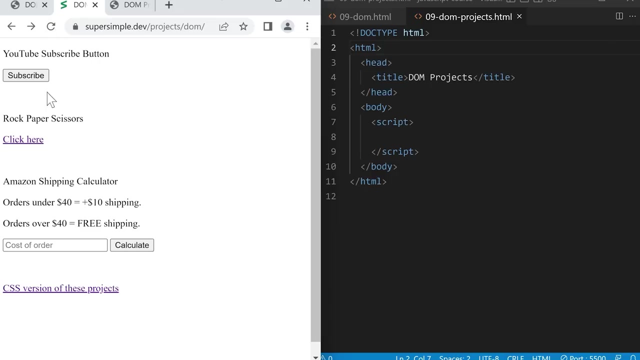 open the console, just in case. Right click, click, inspect and then click the console. Alright, we're ready to start with the projects. Let's change to get it back to normal and when we click this button it will change to subscribed. First, let's 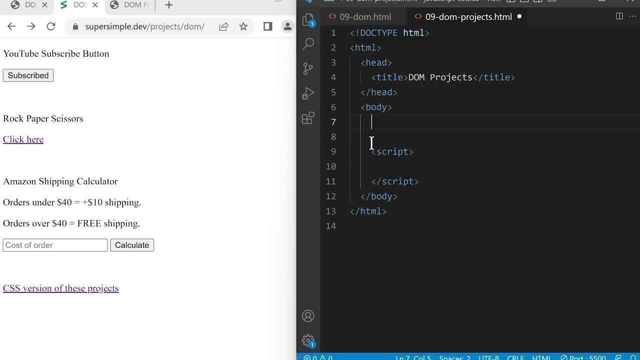 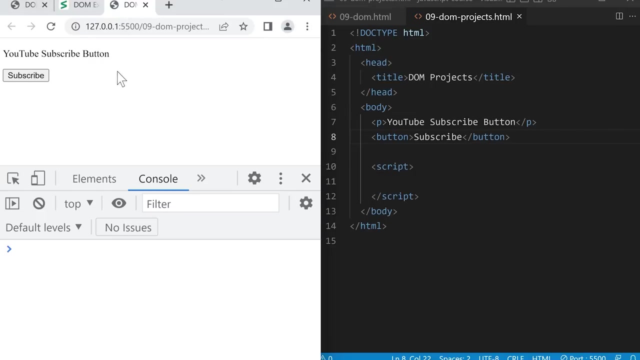 create the html elements for this project. We'll go back to our tab and we'll have the text youtube subscribe button. And now let's create the button. So on the next line we'll type less than, button, greater than, and we'll have the. 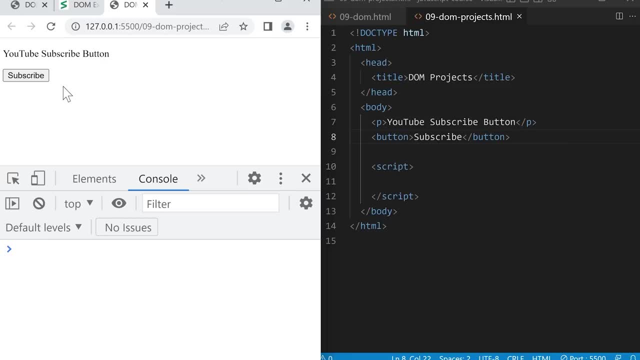 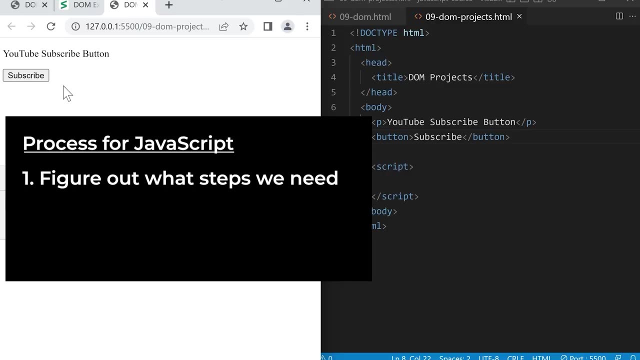 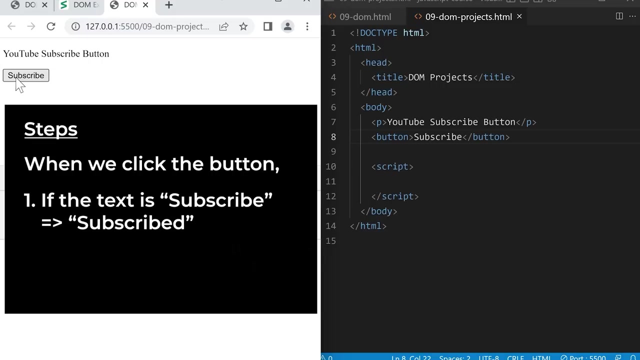 html elements that we need. So now let's make this interactive with javascript, And remember we have a process for this. First, we'll figure out what steps we need. to subscribe, We'll change it to subscribed. Otherwise, we'll change it back. 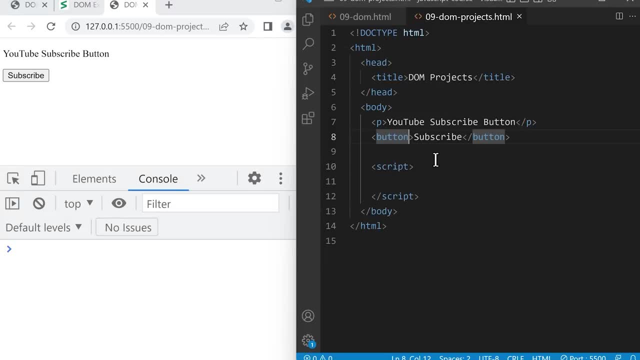 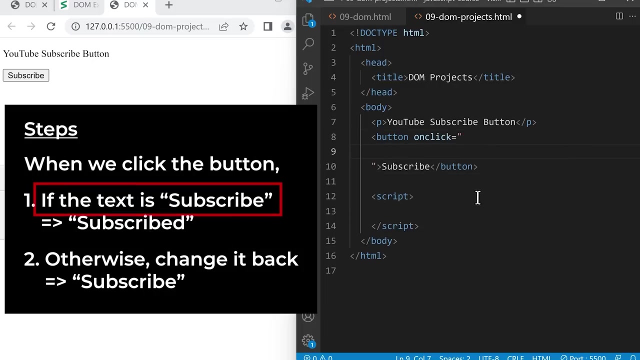 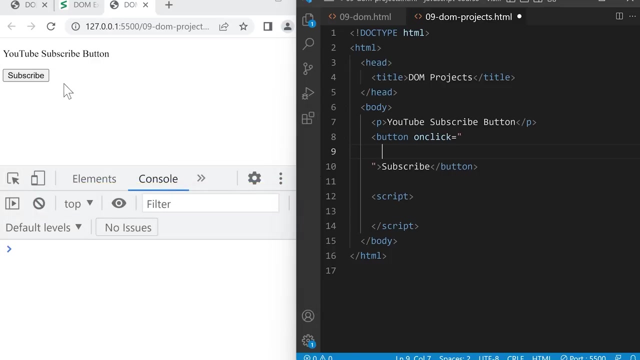 Now let's convert these steps into code. Let's go to our button element and we're going to get the text inside the button, And we learned how to do this earlier. We can use document dot query selector to put this button into our javascript. 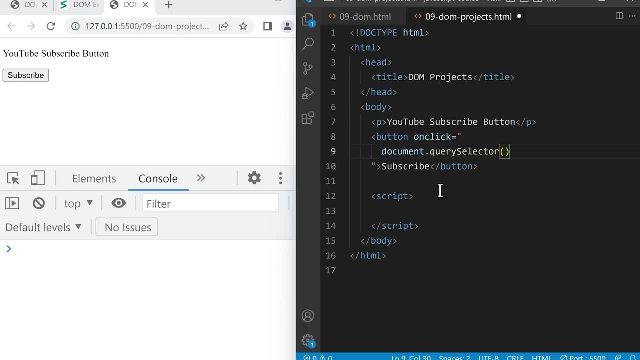 and add a string And, as we learned, we're going to use a class attribute to select this specific button. So in the opening tag let's add a class attribute and inside document dot query selector, we're going to type a dot to select a class. 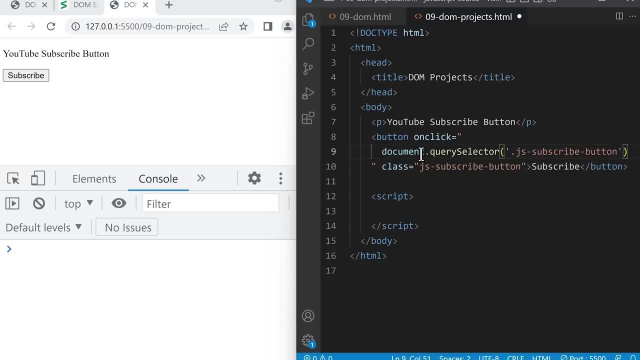 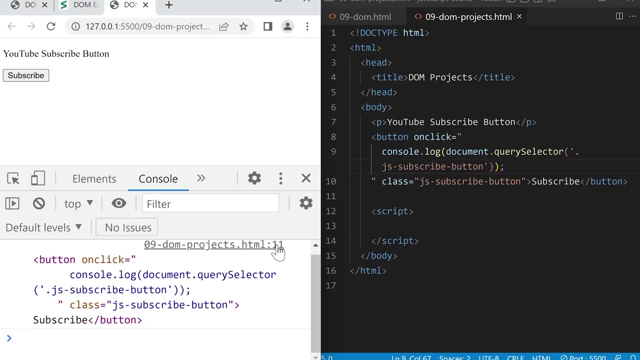 and we're going to select the class js dash, subscribe, dash button. And now let's click our button and it will show us that document dot query selector. got the button on the page. So now let's save this button in a variable. so let's 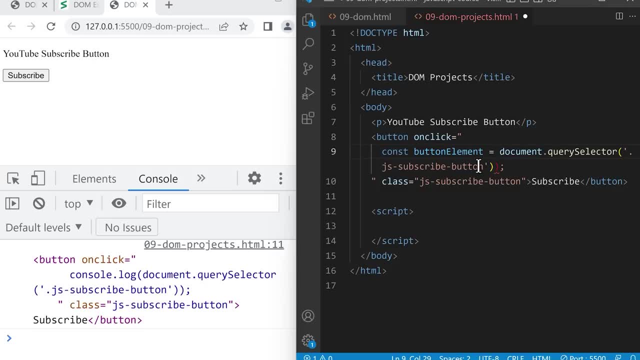 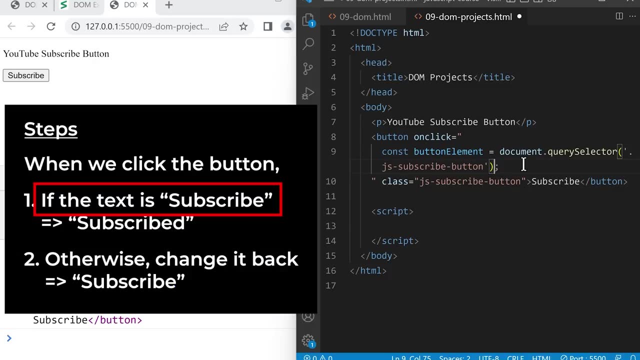 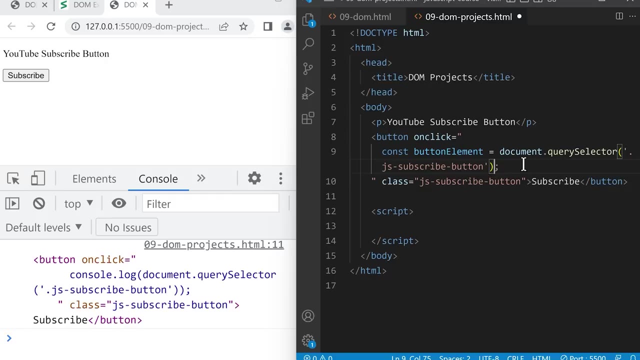 make it equal to this result. So now that we have the button inside our javascript, we're going to check if the text inside the button is subscribe. To check the text inside this condition, let's get the text inside the button So we'll type. 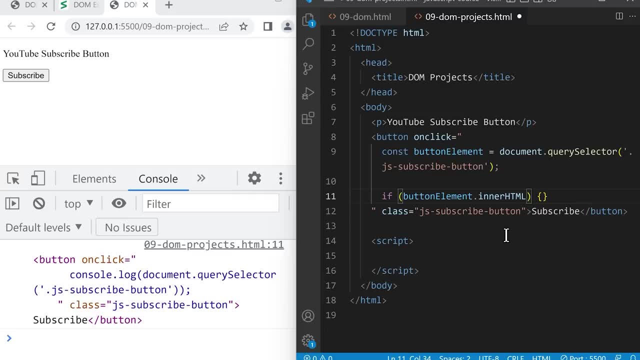 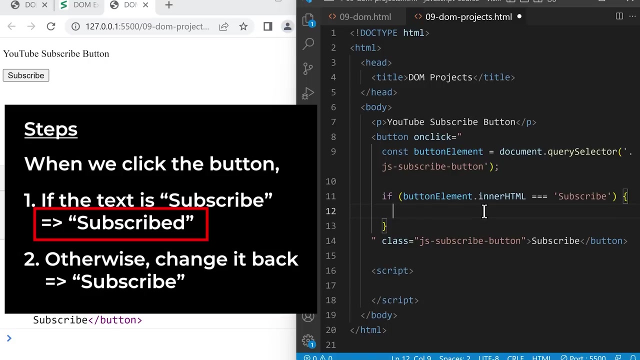 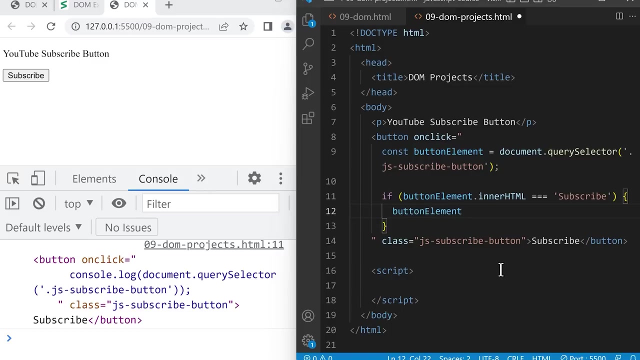 button element: dot- inner capital html. and we're going to check if it's equal to subscribe. Now, if it is equal to subscribe, inside the curly brackets, we're going to change the text in the button to subscribed. So let's type the code. button element. 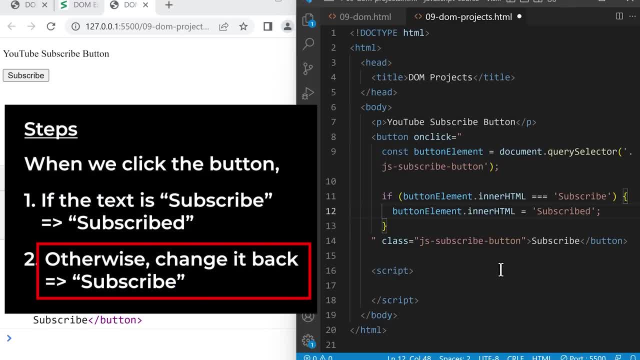 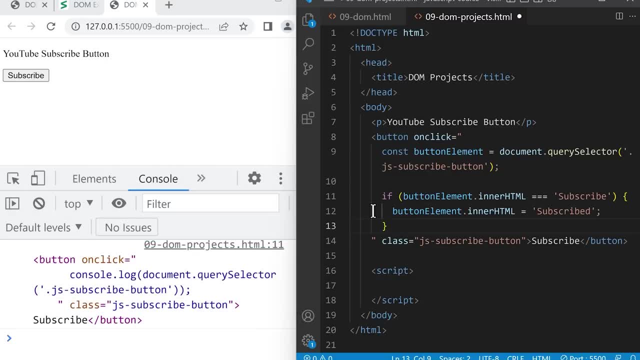 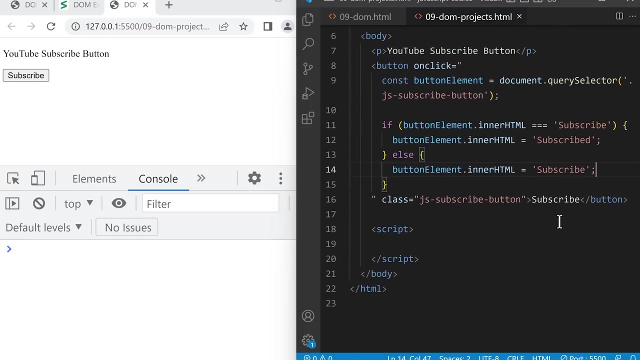 dot inner capital html inside the button element dot inner capital html and we're going to change the text back to subscribe. So let's type button element: dot inner capital html and make it equal to the string subscribe and save Now, before you try out this, 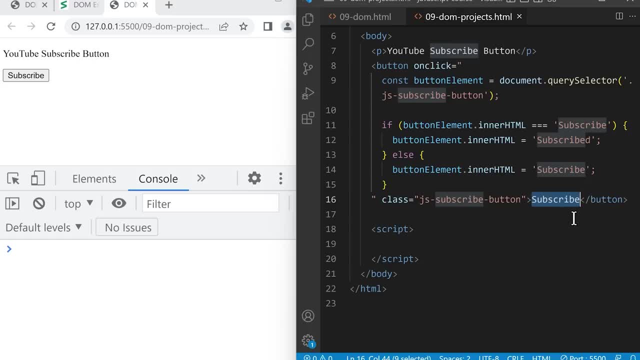 project make sure that the text inside the button has no spaces or spaces. it will change to the text subscribed. If we click it again, it will go back to the original text. So that's how we create the subscribe button project using the DOM. So 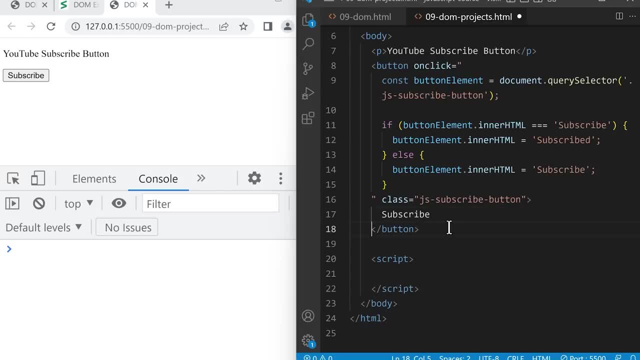 now let's go back to our project and click the button again. You'll notice that it no longer changes the text, And that's because now we have a bunch of spaces around this text And these spaces are not in the text. So what? 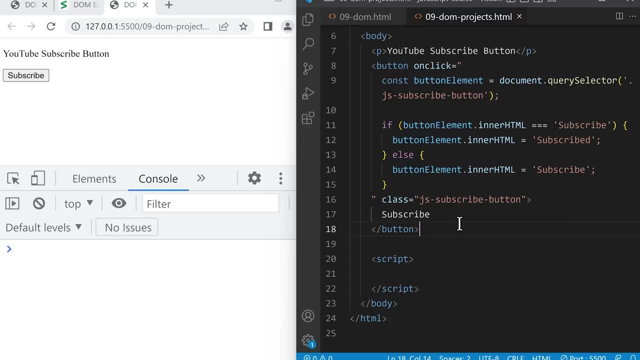 do we solve this problem when there are spaces around our text? To solve this, we're going to use a different property of an HTML element. If we save and go back to our project and click it again, it'll start working again. So that's. 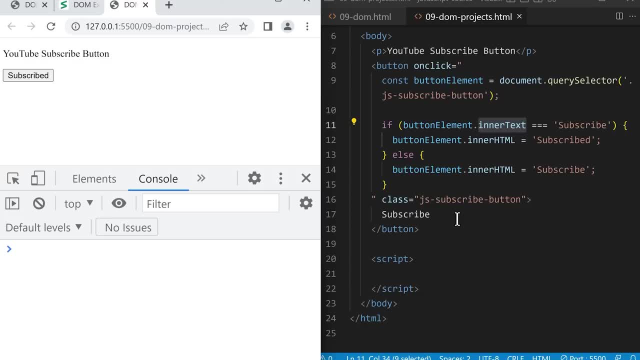 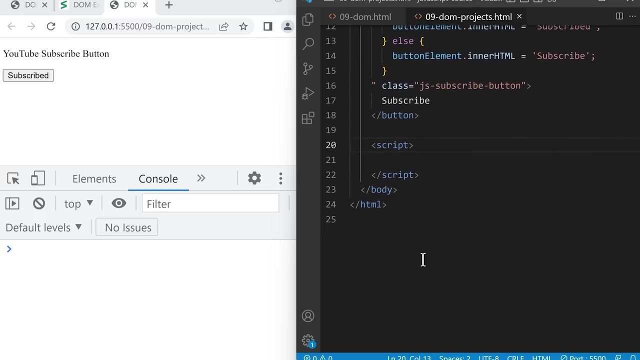 the inner text property of an HTML element. Let's see how to make our code cleaner. Right now, we're mixing HTML and JavaScript together, So to make our code cleaner and easier to read. we're going to do this by using the function subscribe. 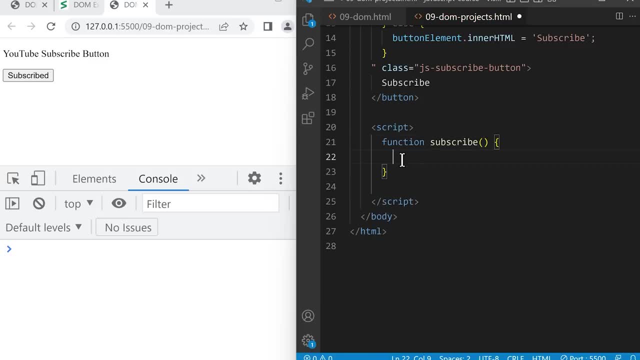 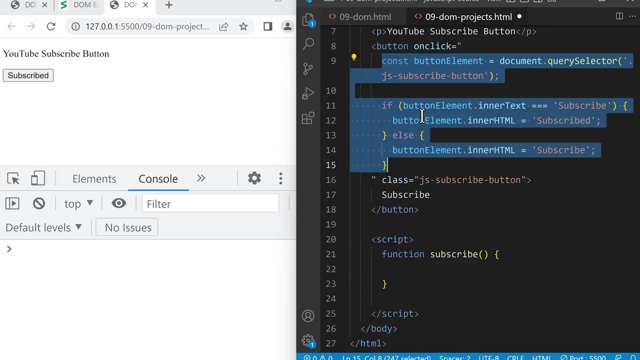 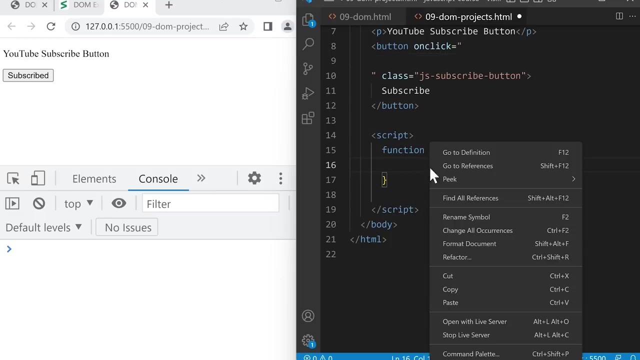 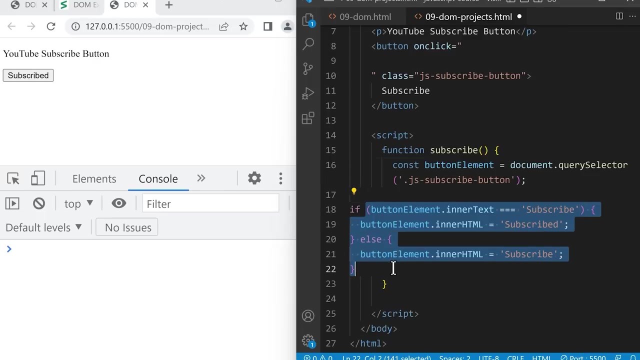 brackets and curly brackets, And inside these curly brackets we're going to move all of this code. So let's select this code To fix the formatting. we can select these lines and press tab a few times. And now that we have this function, 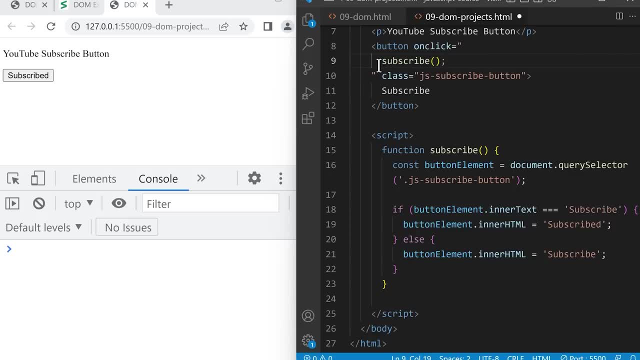 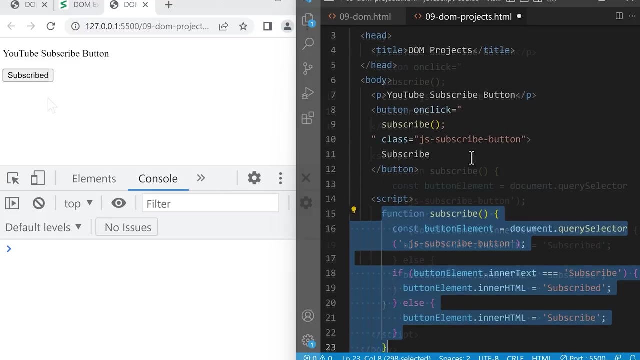 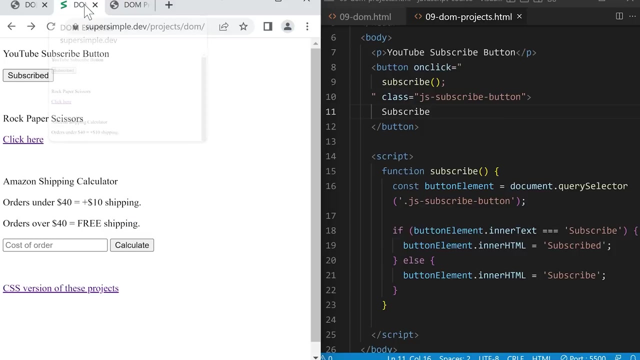 we're going to go to the on click attribute and we'll see that our code is cleaner because we grouped all the JavaScript code at the bottom And we're no longer mixing as much HTML and JavaScript together. Now let's look at the next version. 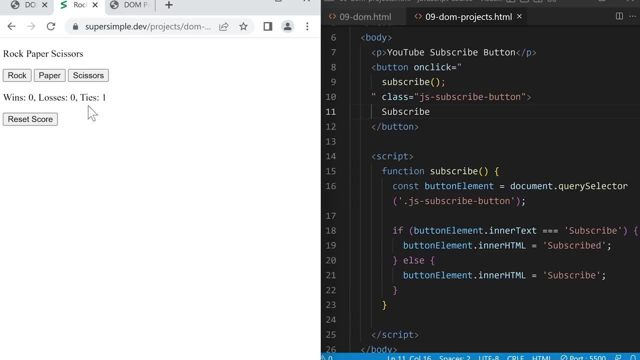 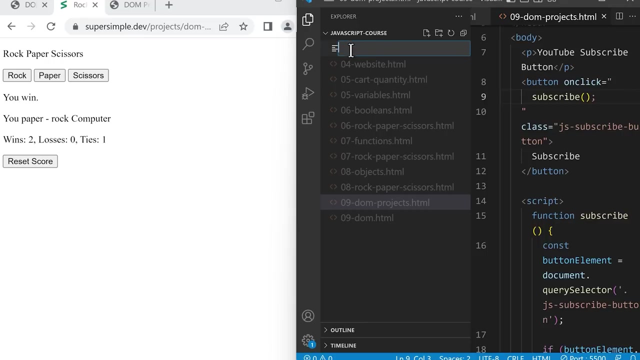 of this project, So you'll notice a few changes here. The first change is that we're going to show the score on the page instead of the screen, So let's create a new file for this rock paper scissors game for this lesson. So 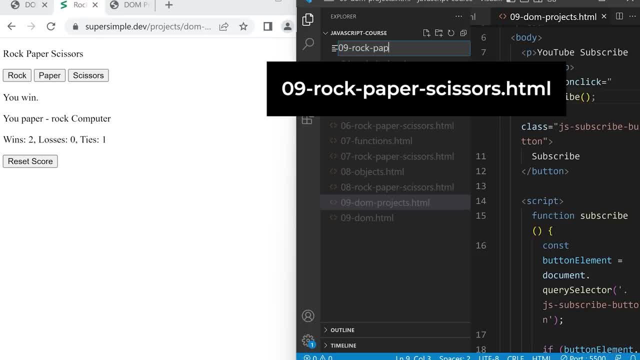 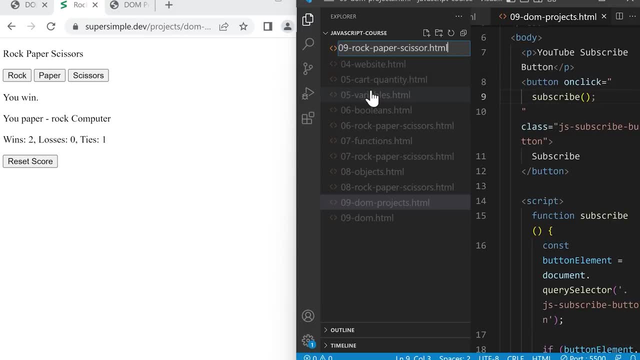 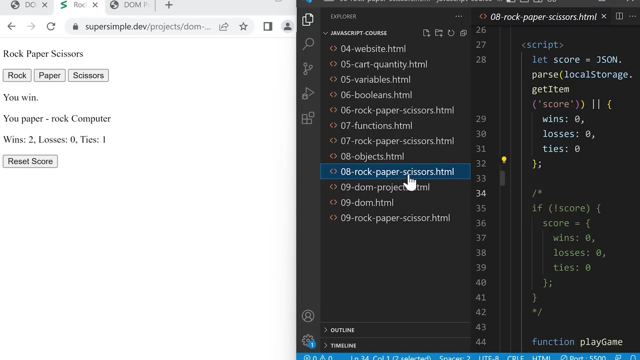 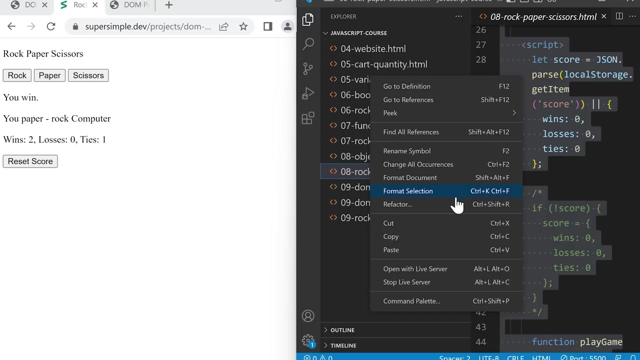 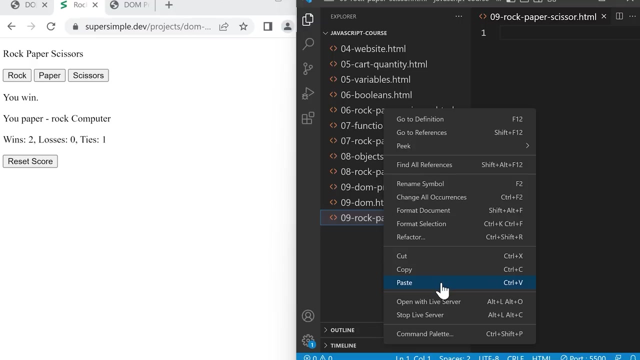 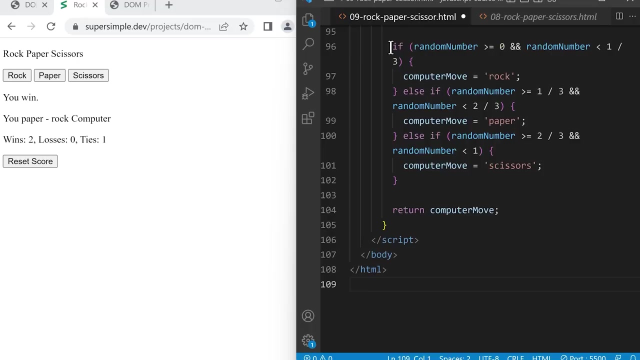 let's go to our code editor and we'll click this icon and enter. And let's copy the previous rock paper scissors which is here. We'll click here and type Ctrl A or Command, A Right click, copy and here right click and paste. 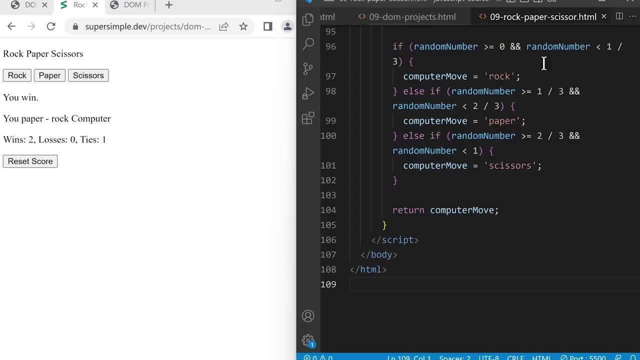 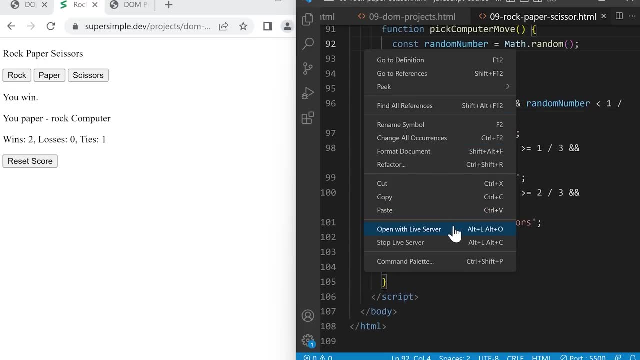 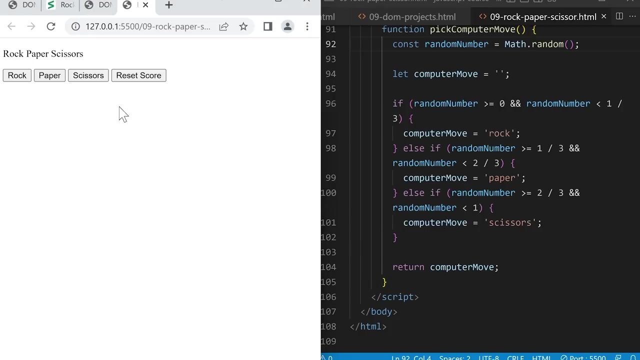 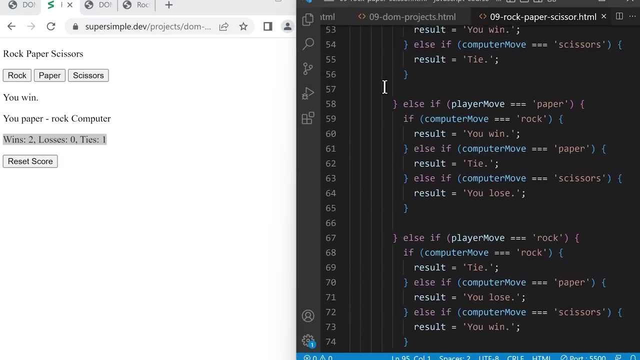 We'll close 08 rock paper scissors and finally, we'll open this in the browser by right clicking: open with live server. Now we're ready to begin the second project. So let's put the score. So let's create an HTML element for this. 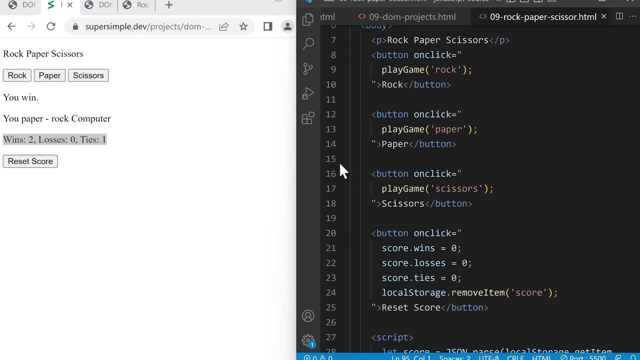 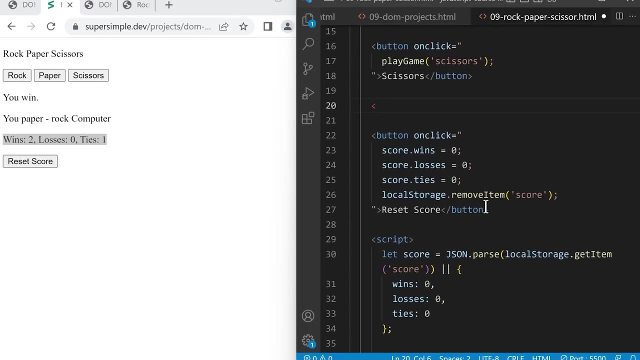 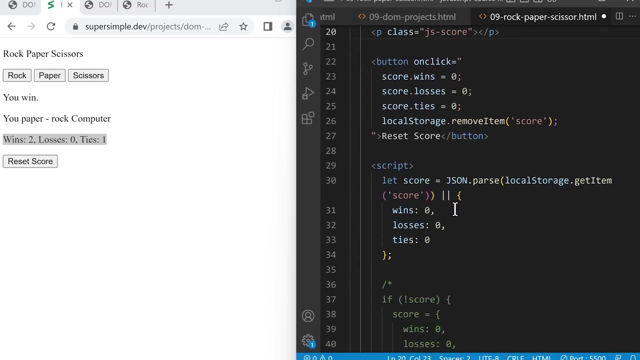 We'll scroll up to our HTML, which is here, And after the scissors button, let's add a paragraph element in our JavaScript. So in the opening tag we'll type space: class equals double quotes, js dash score. Now that we have a class, let's. 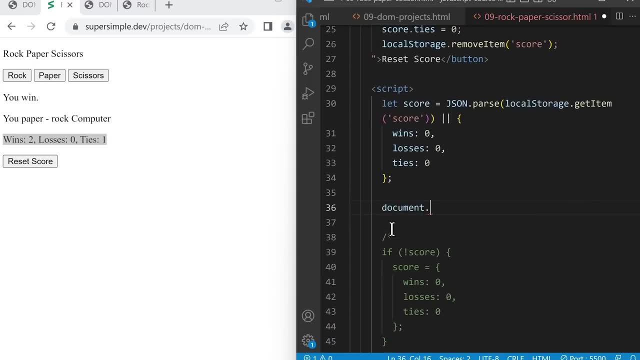 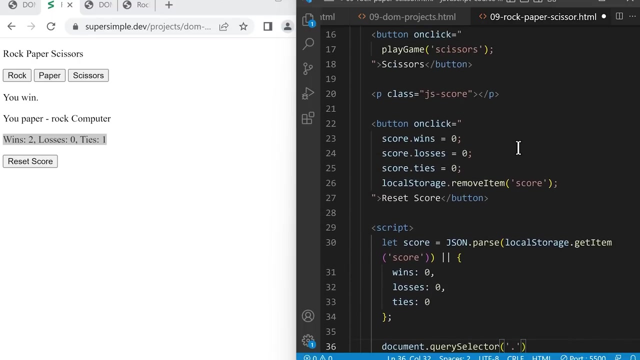 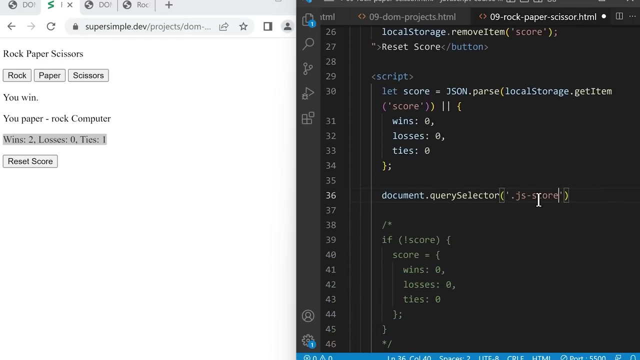 get this element in our JavaScript. So we're going to type a dot and we're going to select the class: js dash score. So js dash score. So this will get the paragraph element from above and from below. To do that we can use: 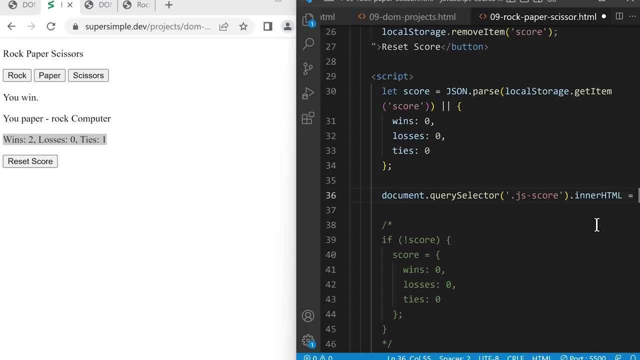 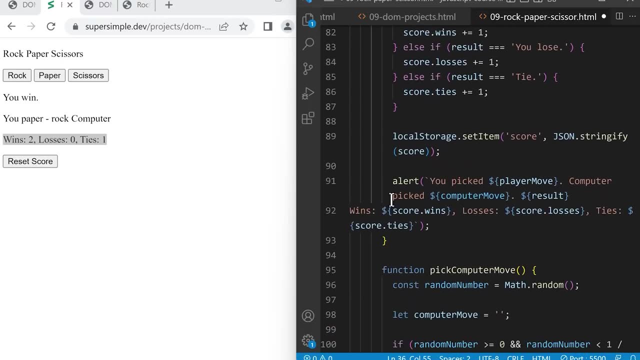 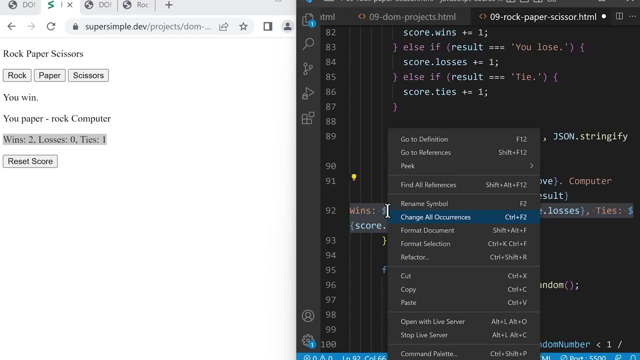 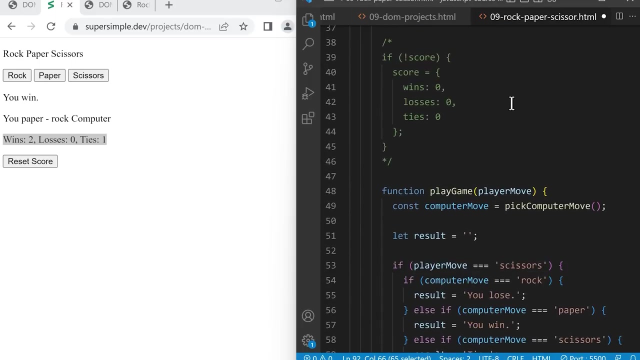 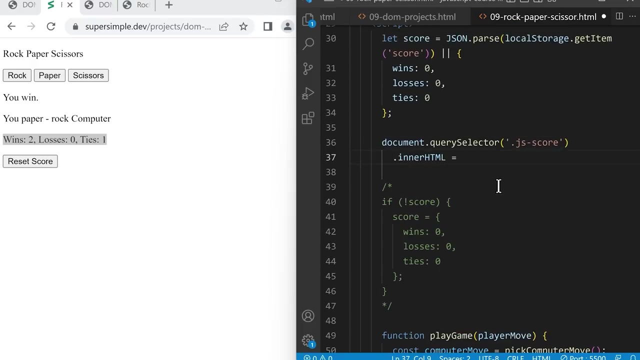 inner HTML, dot. inner capital HTML, and we'll make it equal to the score. If we scroll down, we actually create the popup to here and I'll actually put this on a separate line to make it easier to read. And now, here we're going to. 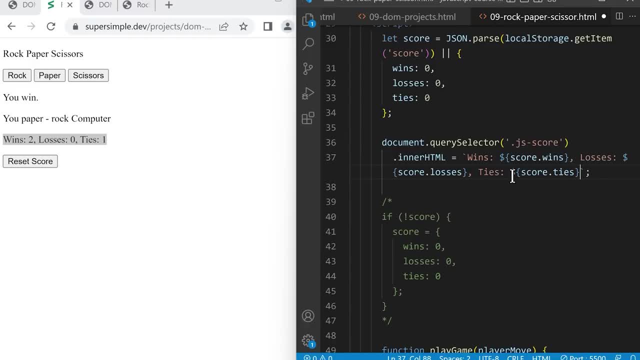 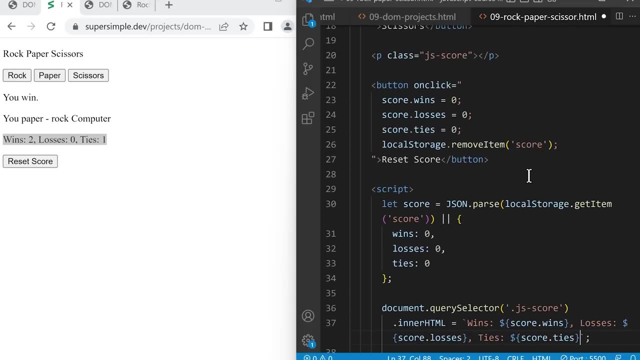 type a string using back inside this element, So inside this paragraph. If we save and then go back to our tab, you can see that now it displays the score on the page. Now, before we move on, I want to point something out with HTML. 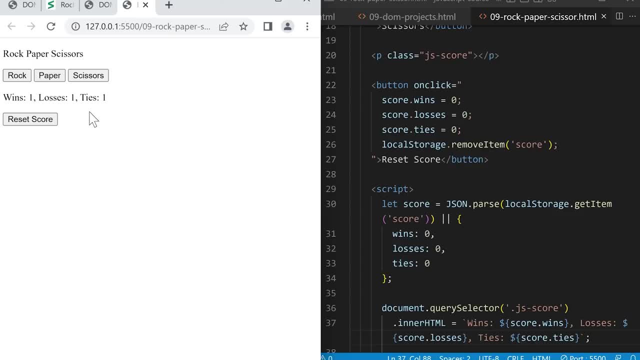 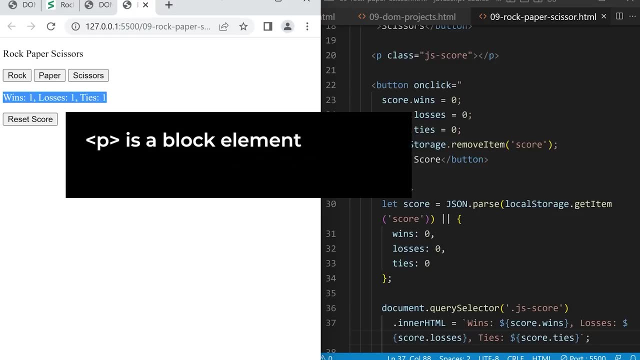 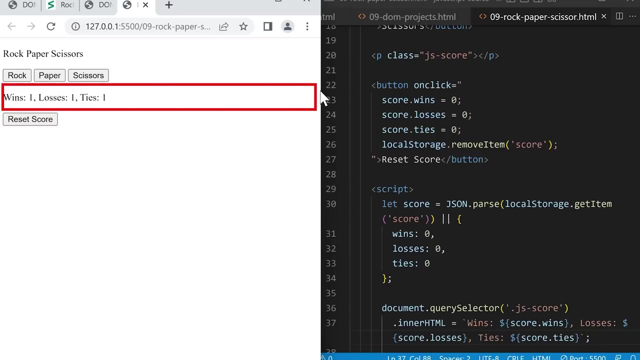 So what determines if an element appears beside something or below something? So the paragraph element here is known as a block element. A block element will always take up an entire line by itself, So this is why we get this layout here. So this is. 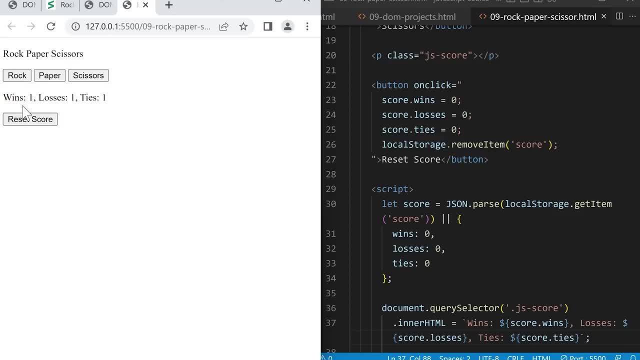 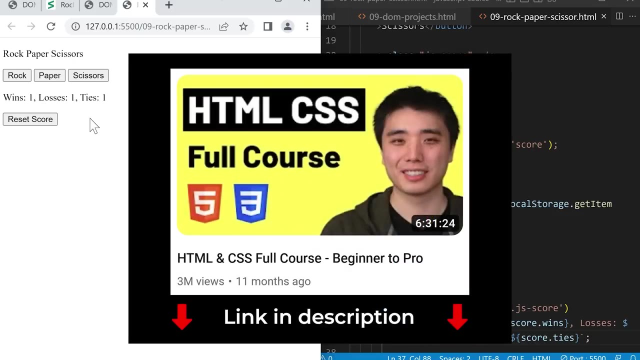 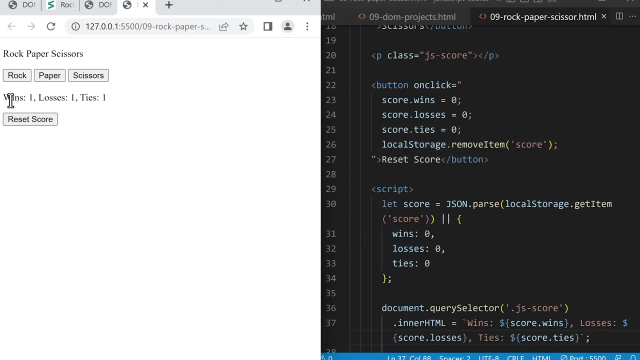 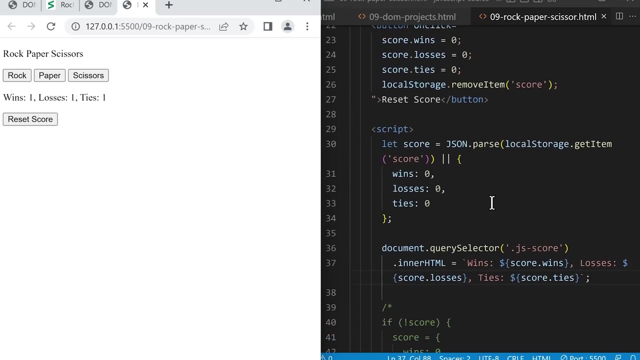 just a short review of layouts. If you want to learn this in more detail, you can check out the description below. Alright, the next feature we're going to do is, if we play the game, we also want to update the score Right now, if 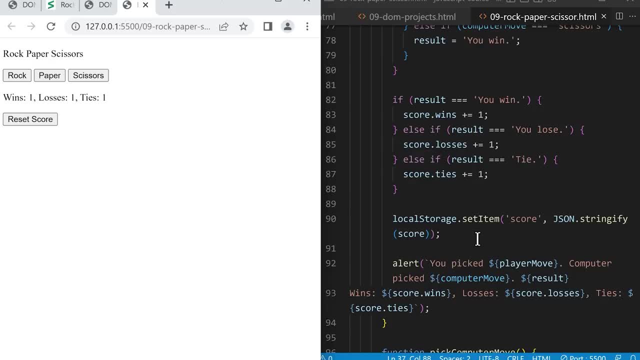 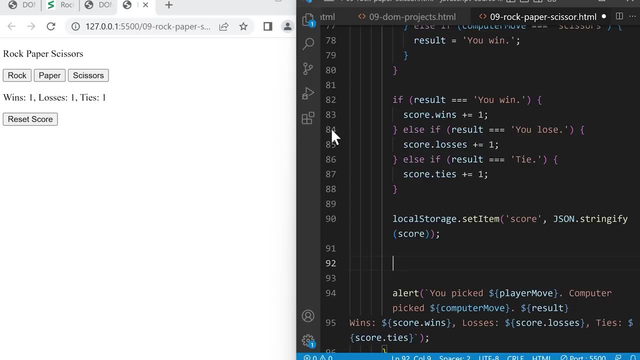 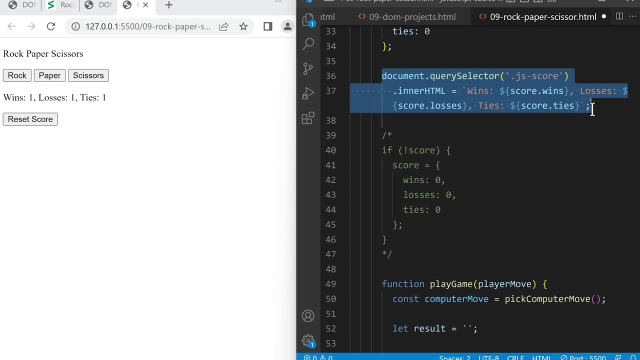 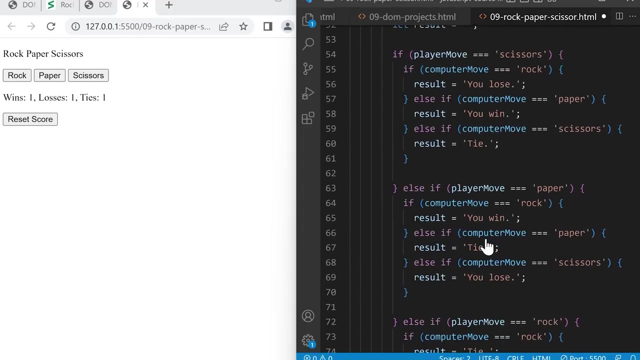 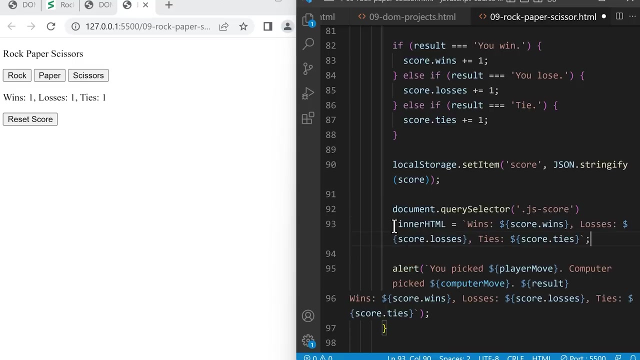 we play, it doesn't change anything because we're going to update the score on the page, So we can actually use the same code that we used above, which is here. So let's make a clean up of the score by clicking on the game tab. 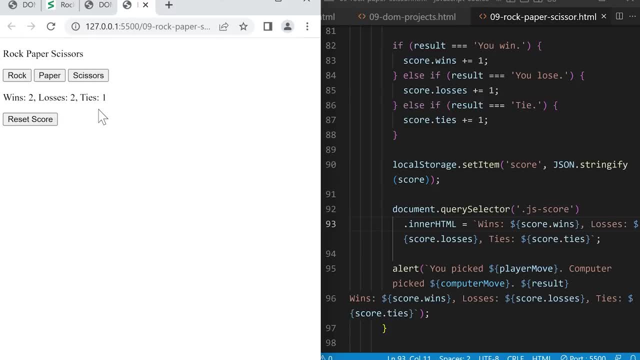 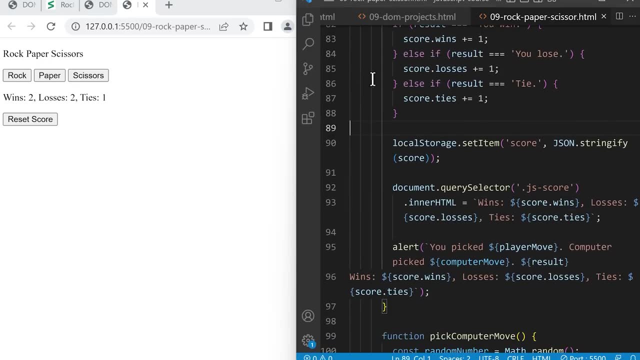 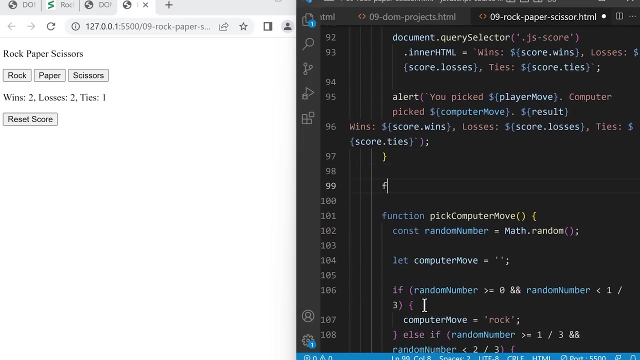 at the front, If we save and then try out our game, we'll click a move, press ok. so at the bottom here let's create a function using function and we'll call it update score element brackets and curly brackets and we'll move this code into. 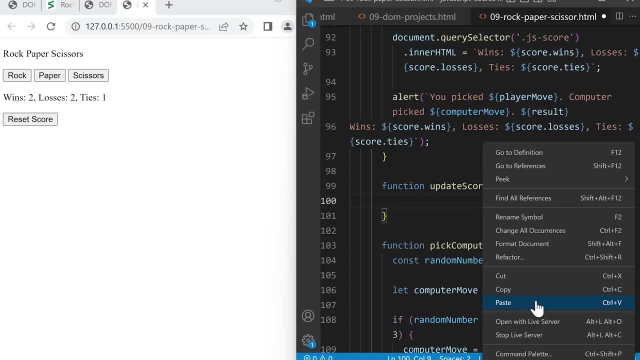 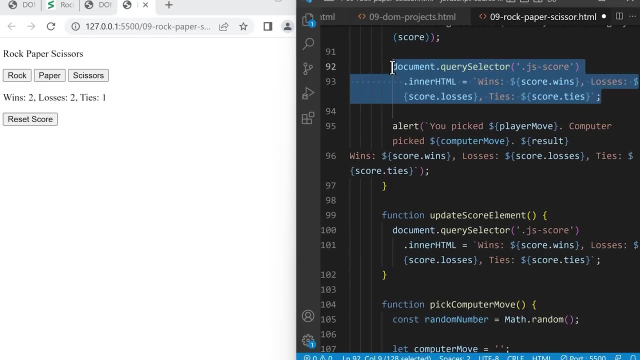 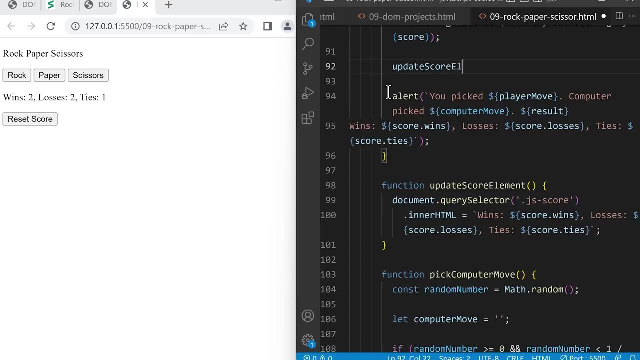 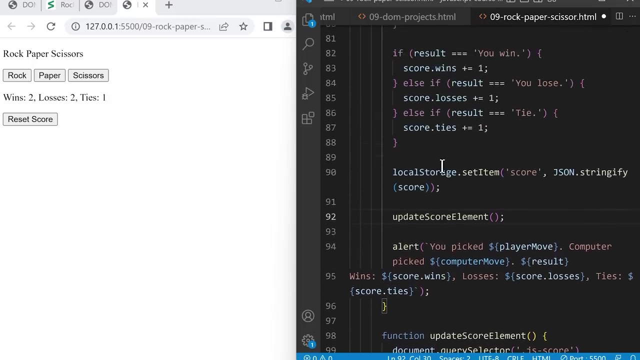 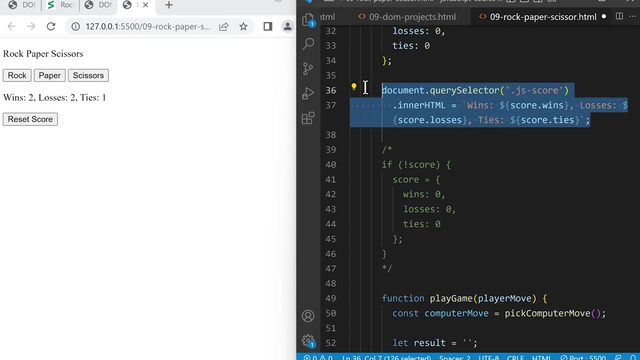 the function here right click and paste. and now, instead of writing this code multiple times, we're just going to call the function update score element and brackets. this will run, so let's scroll back up and instead of typing out all this code again, we can just use: 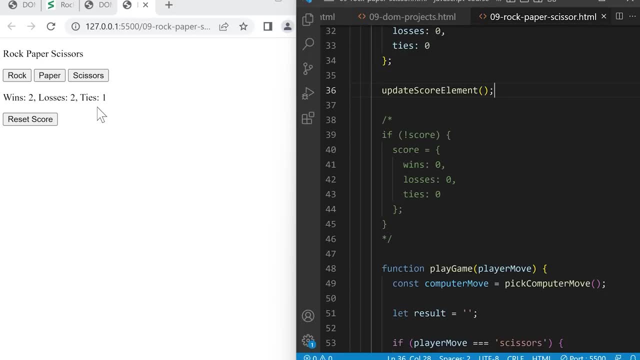 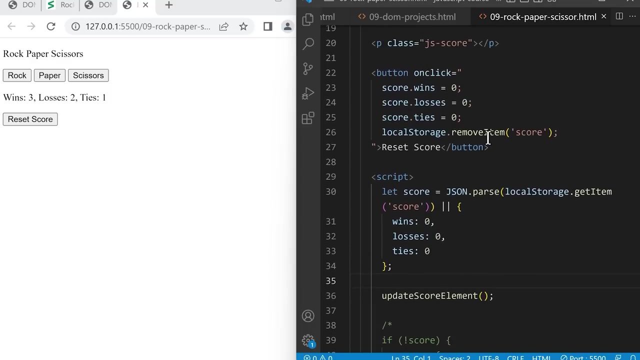 our function: update score element and brackets. now let's save it and let's go into our code and let's go to the reset button, which is here, and after we reset the score, it doesn't actually update it, so let's go ahead and reset the score. 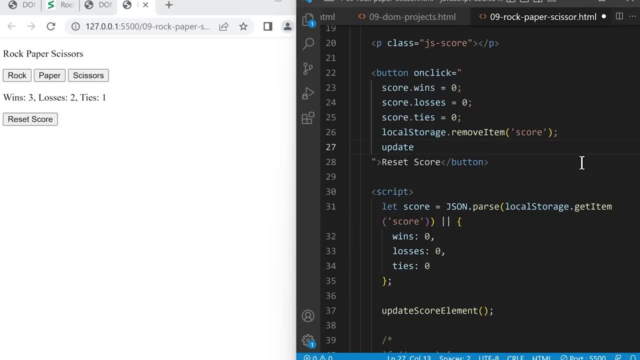 we're going to call that function again: update score element and brackets if we save. and now let's play the game and press ok, so we have. now we've finished the score. let's go back to super simple dev and play the game. and now we're. 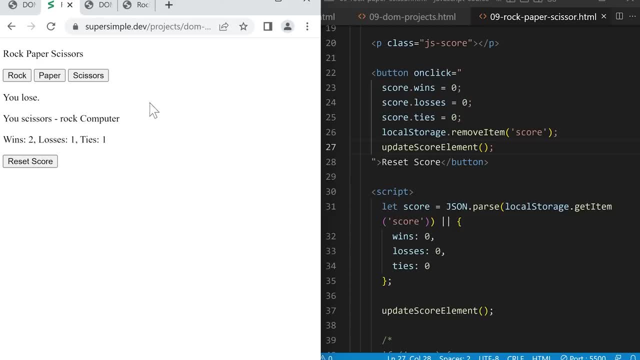 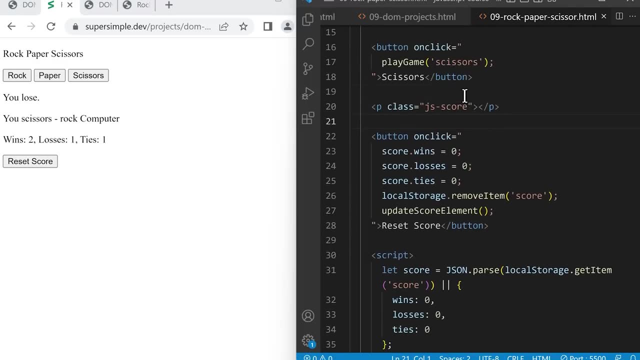 going to work on this section. we're going to show the result and the class we're going to add. a less than p greater than this is going to be the result. so let's give it a class of js dash result and let's create another paragraph. 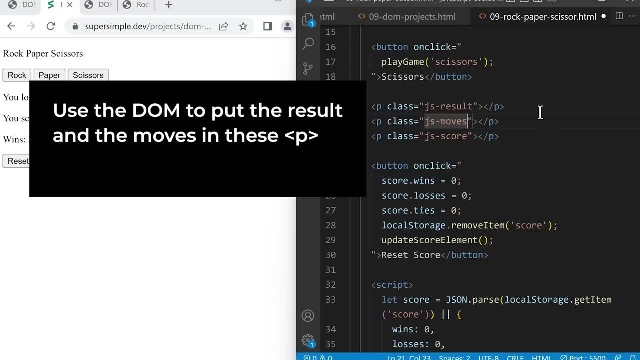 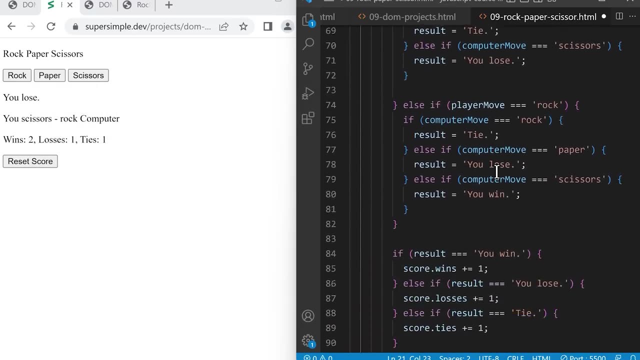 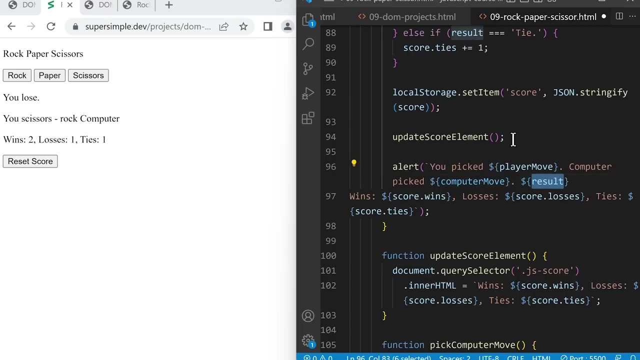 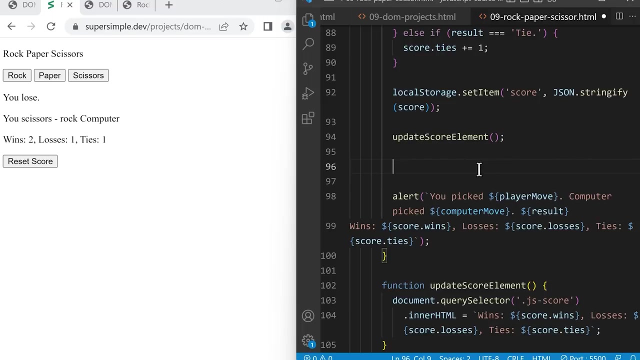 with the result and the moves. now let's use the dom to put the result and the moves in these paragraphs. feel free to pause the video if you don't want to pause the video. now we're going to add the result to this paragraph, so we'll. 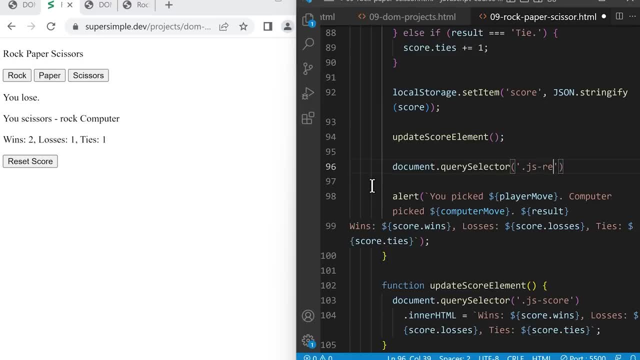 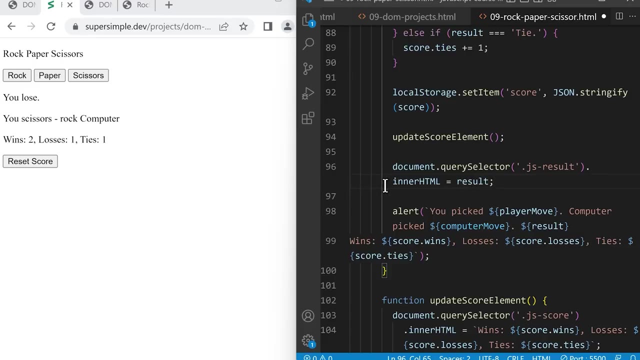 type: document dot query selector, brackets and a string and we'll type a dot and we'll change this to result. and now let's also display the moves. so we'll type some new lines and document dot query selector, again brackets and a string, dot, m, l, and make. 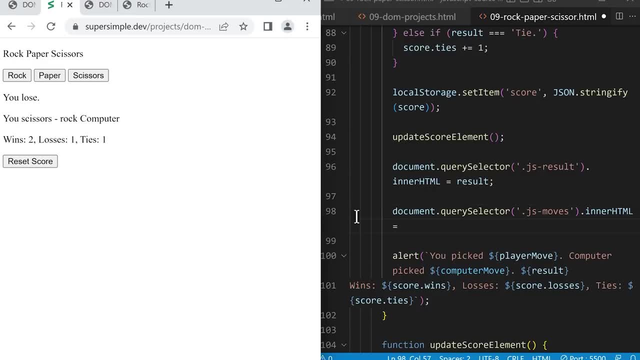 it equal to this text right here. so let's type a template string, because we're going to insert our moves inside the string, and we'll type u and we'll insert the player move, dollar curly brackets, player move. and so dollar curly brackets again, and computer move. 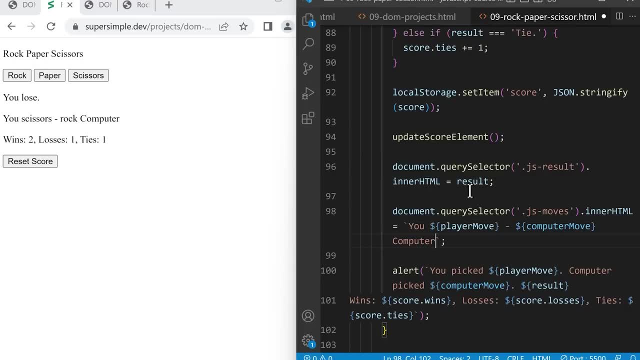 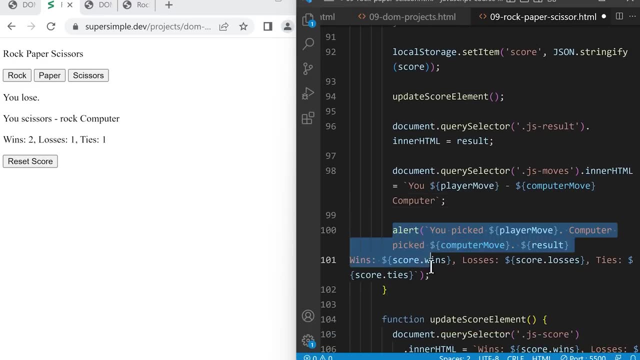 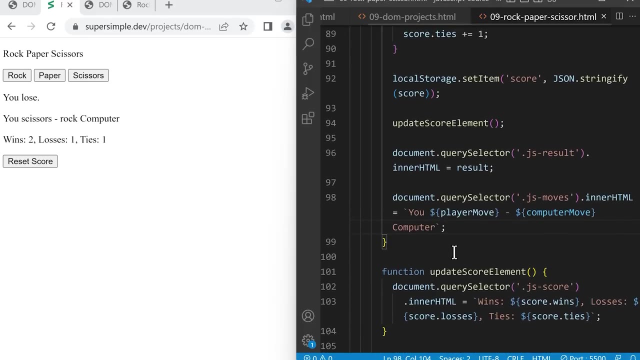 computer at the end. so now that we're displaying everything on the page, we don't need this pop-up at the end. so we can actually delete this pop-up. alright, let's go ahead and play our game now. it will show the result and the moves that 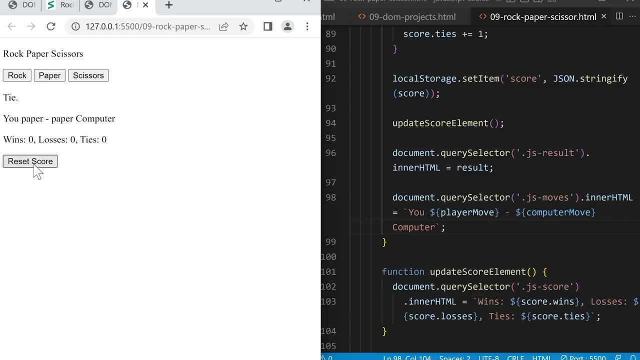 we picked on the page instead of in a pop-up. let's play it again to make it look like a pop-up. so let's move on to the third and final project. we'll go back to supersimpledev and we'll click back to go back. 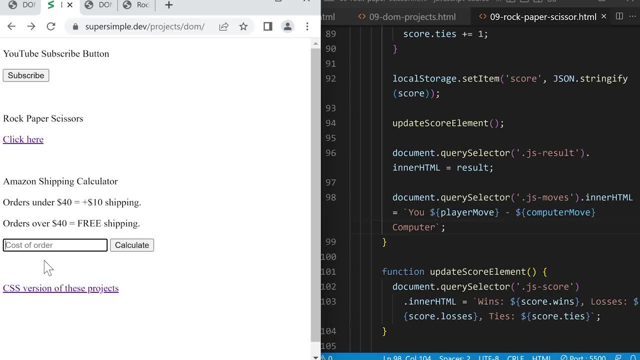 to our projects and if the order is under $40- for example $25- and we click calculate, it will add $10 of shipping and display the total down here. but if we type a cost that is less than $10, we'll see that the $10 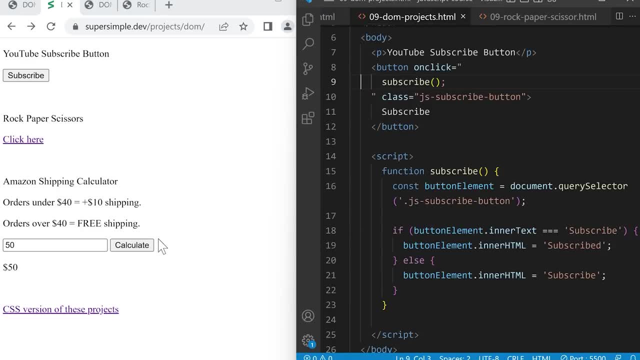 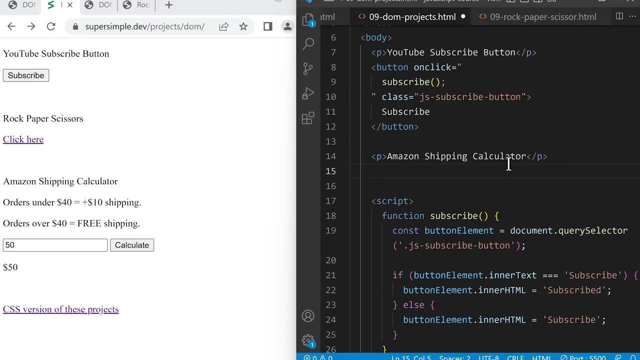 is less than $10. so let's go back to our project file and we'll start by creating the html elements. so let's create this text box. so the html element for a text box is called input, so we'll type less than input, greater than so. 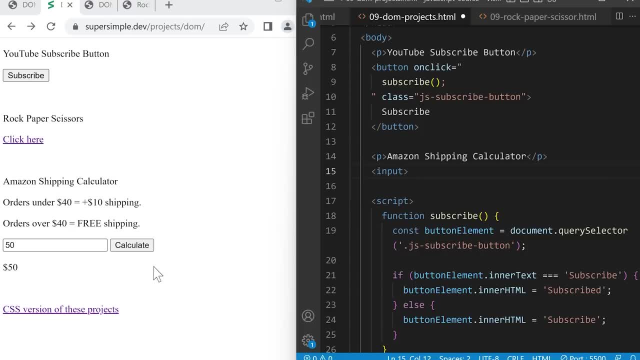 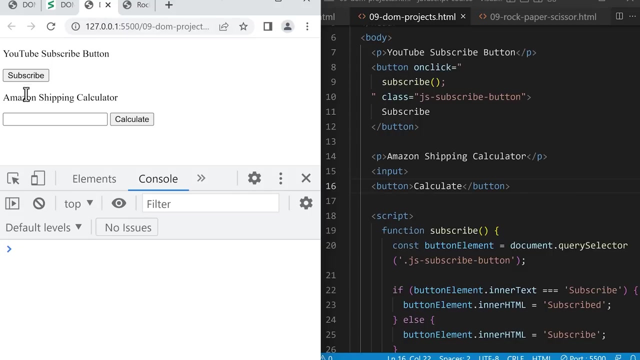 the input element is special button, so here we'll create less than button, greater than calculate. now let's save and open the tab for this file, which is right here, and we have the text box and we have this gray text. so this is called a placeholder to. 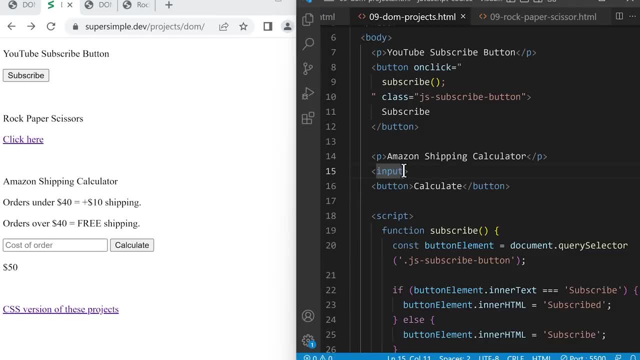 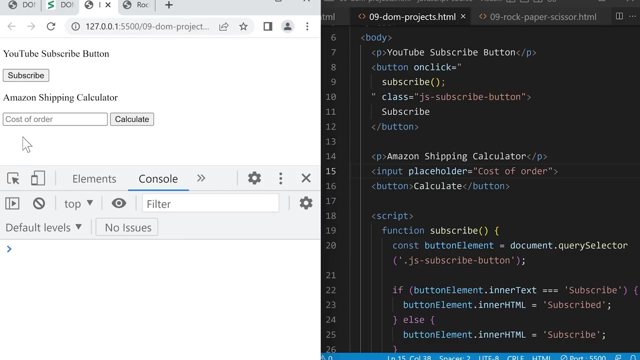 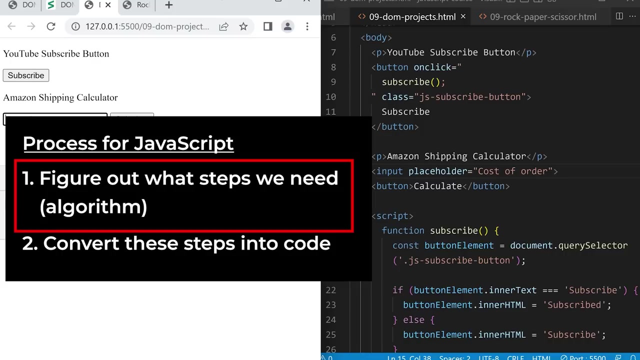 add a placeholder to a text box. we're going to use the placeholder attribute, so we'll put the text we want as the placeholder, which is cost of order, and save now if we go back to our project, we now have a placeholder we'll need to add. 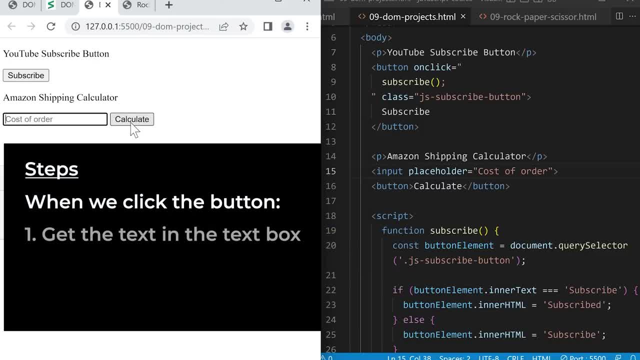 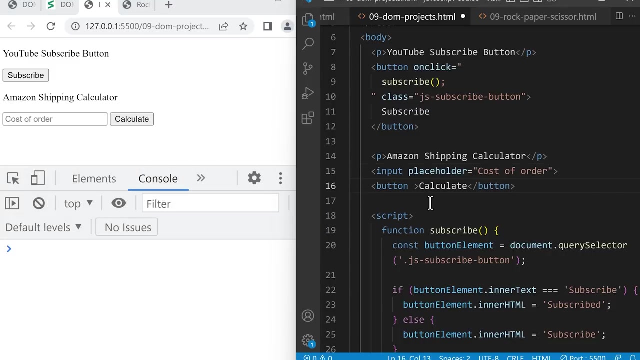 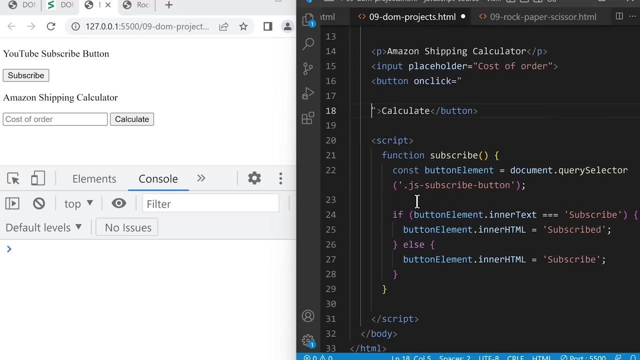 a placeholder to our page, so we'll add a placeholder to our page. now we need to add a placeholder to our page, so we click on And inside here let's also create a function to separate our JavaScript code like we did before. So in the script we're going to create a function function and let's name it: calculateTotal brackets and curly brackets. 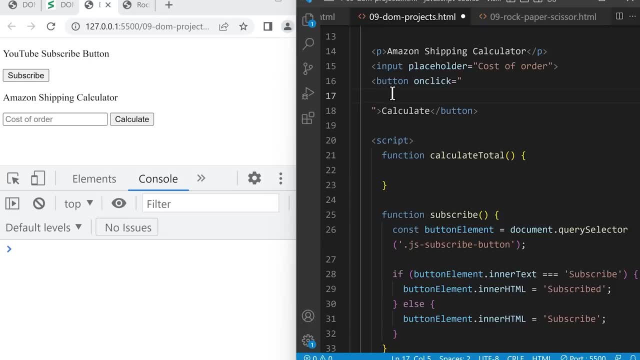 And inside onClick we're just going to call the function So calculateTotal brackets. The next step is to get the text inside the text box. So first let's get this input element and put it inside our JavaScript. To do that, we can use documentquerySelector again. 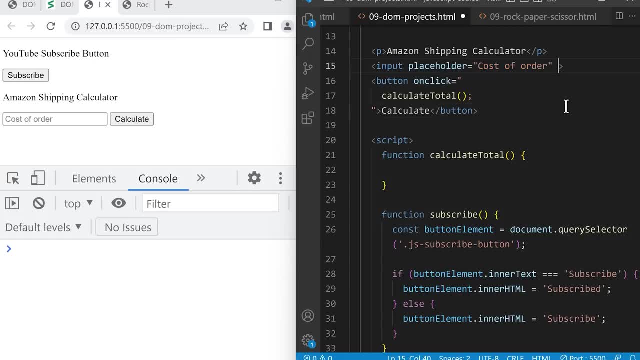 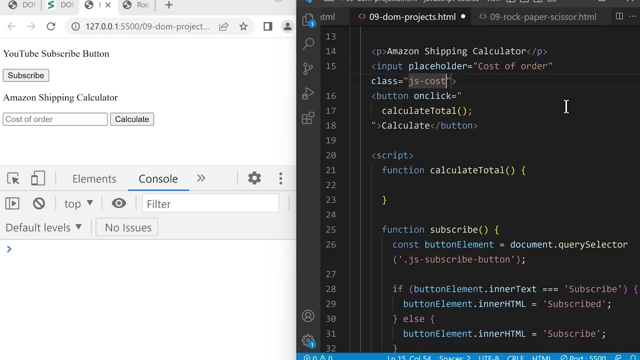 So we'll add a class to this input so we can select it. Class equals js-cost-input. And then inside our JavaScript we'll use documentquerySelector- brackets and a string and a dot, And this class class js-cost-input. So this code will get the input element and put it inside our JavaScript. 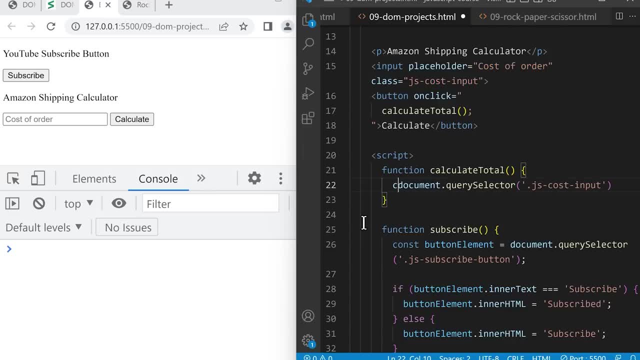 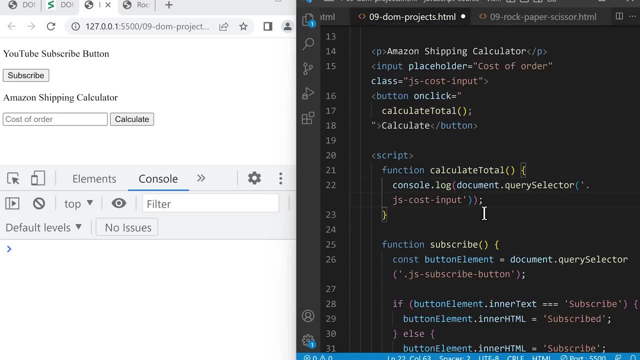 Let's confirm by consolelogging the result And save. And now, when we click the calculate button, It will give us the input element from the page. Let's save this input element in a variable so we can use it later. Instead of consolelog, we'll use const. 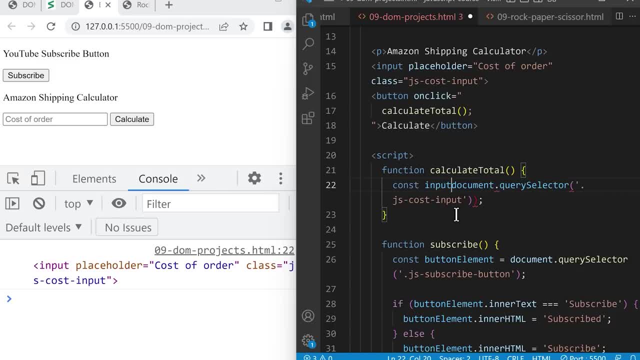 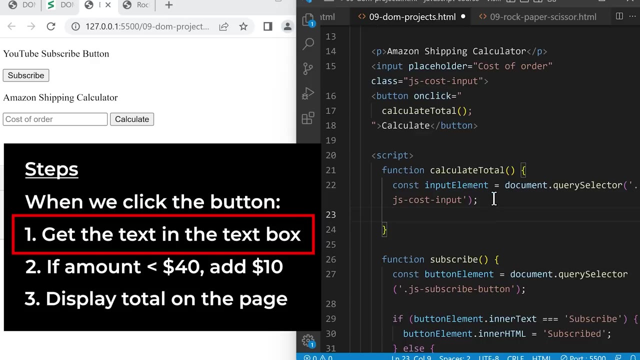 And we'll name the variable inputElement And make it equal to this element And remove the extra bracket, And next we need to get the text inside the input InputElement. So so far in this lesson we've been using the property innerHTML to do this. 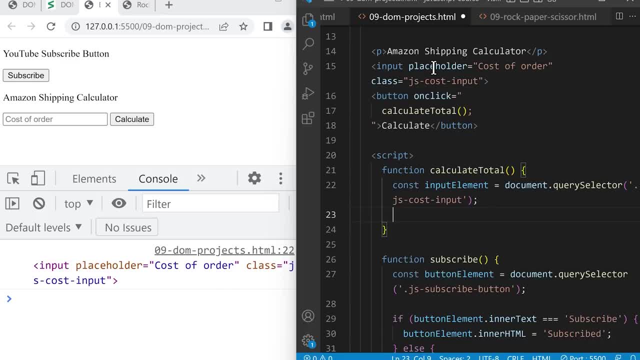 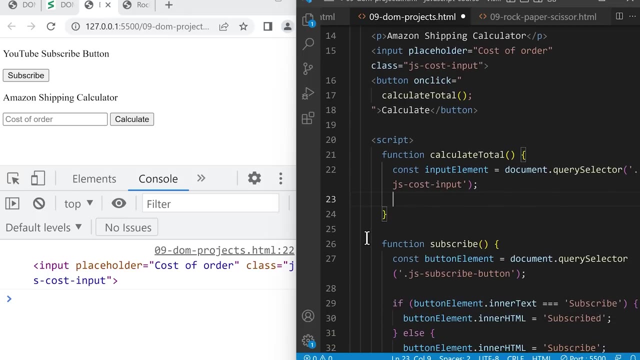 However, for inputElements you'll notice that there is no HTML inside. So for inputElements we're going to use a different property called value. So at the bottom here we're going to type inputElement. This is how we get the text inside a text box. 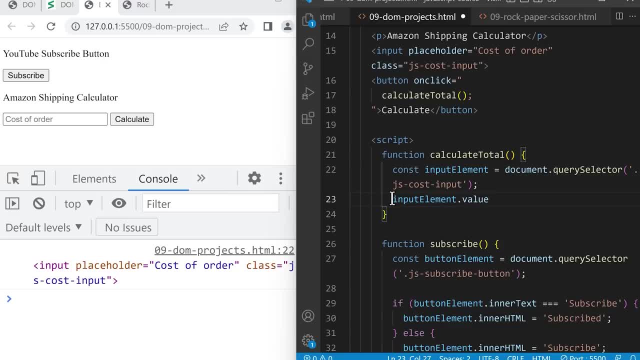 So let's consolelog this to confirm that it works. So we'll consolelog And save. And now let's type something in the text box Like 50. And click calculate, And inputvalue will give us the text inside the text box. 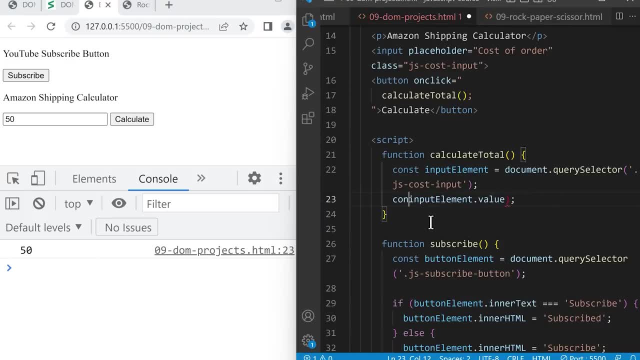 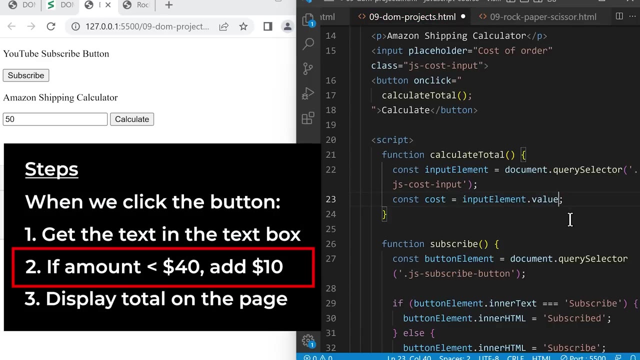 Let's save this text in a variable so we can use it later. Const, And we'll name the variable cost And make it equal to the text in the text box. The next step is to check if this cost is under $40.. 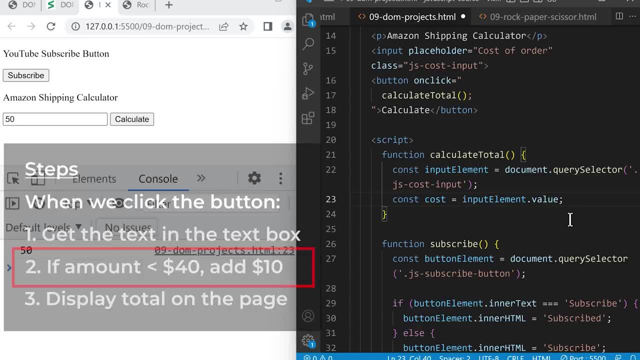 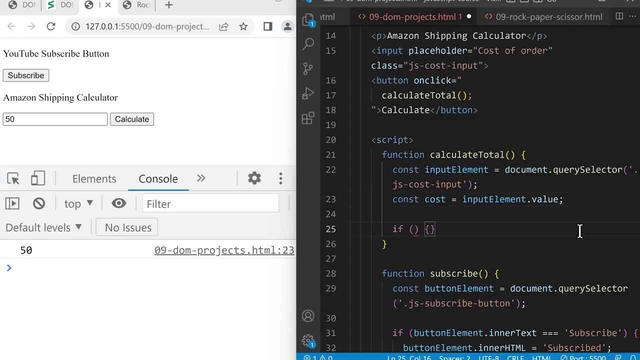 If it is, We'll add $10.. So down here let's type if brackets and curly brackets And inside the condition we'll check if cost is less than 40. And if it is inside the curly brackets we'll do. cost equals itself plus $10 of shipping. 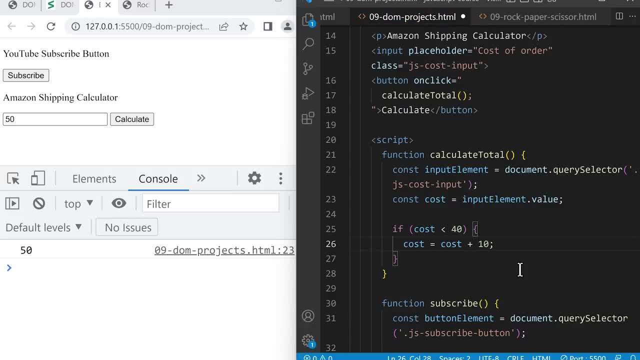 And if it is inside the curly brackets we'll do. cost equals itself plus $10 of shipping. And remember, when we change a variable we have to switch from const to let. And finally we're gonna display the total cost on the page. 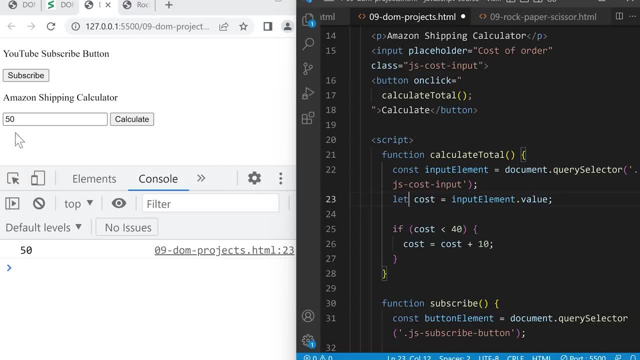 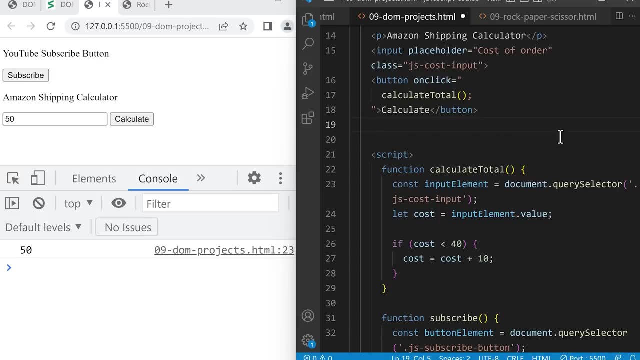 So let's create a paragraph where we can display the cost. So down here we'll create a paragraph. less than p, greater than, Let's give it a class, give it a class js-total-cost. And now, inside our JavaScript, let's use documentquerySelector, brackets and string. 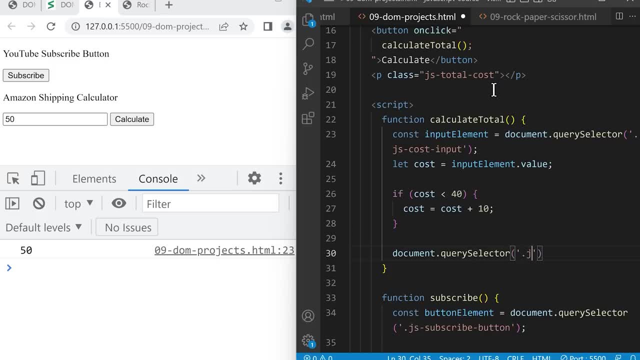 and we'll type a dot and the class js-total-cost And we're gonna put the cost inside the paragraph. We can use dot inner capital HTML and make it equal And let's use a template string. So back ticks and we'll have a dollar. 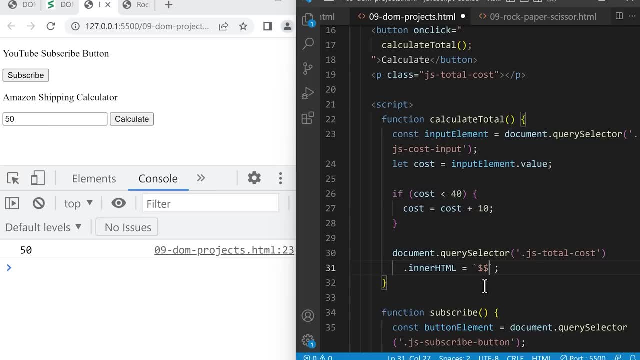 and we're gonna insert the cost using dollar and curly brackets cost. Now let's save and try out this project. So first we'll type a cost that is over $40, like 50. If we press calculate, we're not gonna add $10 of shipping. 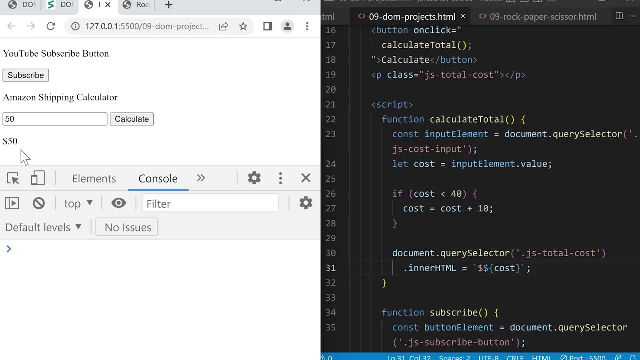 and we'll display the same total on the page. Now let's try a number under $40, like 25, and press calculate, And this number doesn't look right. It's saying that we have to pay $2,510.. So what's going on here? 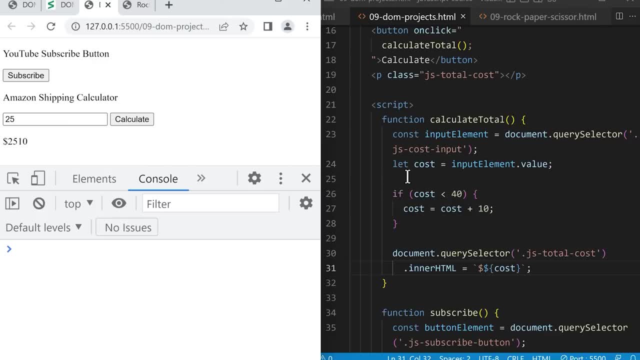 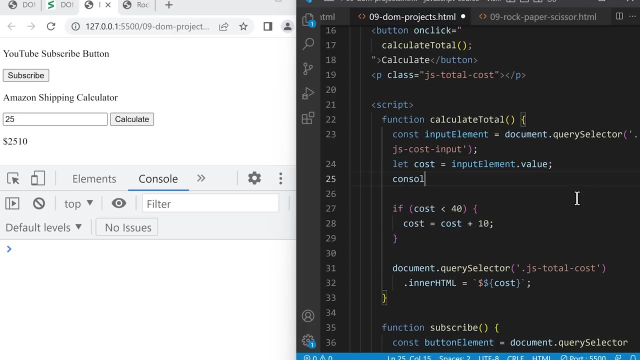 Let's go into our code and let's use consolelog to figure out what's wrong. So first let's consolelog the cost to make sure that we're getting the right number from the text box. So down here, consolelog And save. and then let's type 25 again and press calculate. 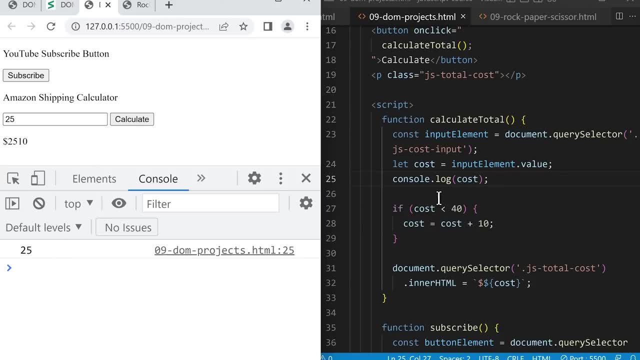 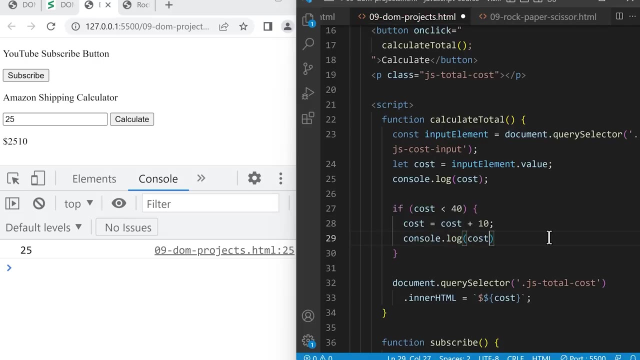 And it will give us 25.. So we're getting the correct text from the text box. Now let's consolelog down here to see if the math is working. So we'll type consolelog cost and save And save. and let's try 25 again and calculate. 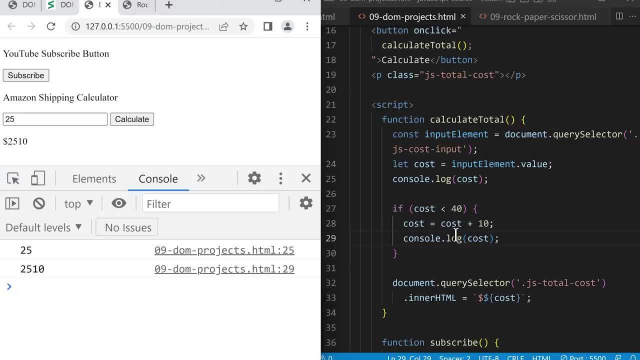 And down here, when we add 10,, this is where things go wrong And it results in 2,510.. So it's not doing math properly here. So let's check if cost is a number to make sure that it's doing math. 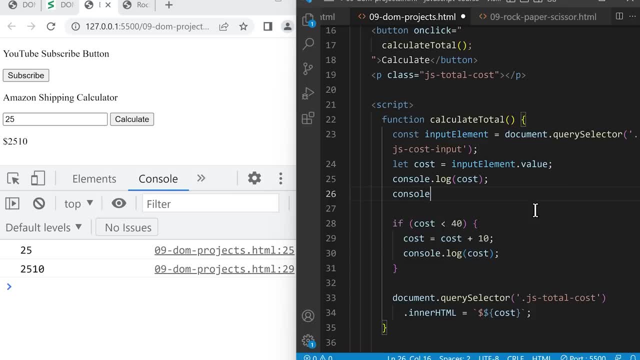 So here we'll type consolelog- costlog. So let's try this consolelog- the type of cost and save. So let's type consolelog the type of cost and save. Let's type 25 again and calculate, And aha, it's telling us that the cost is a string. 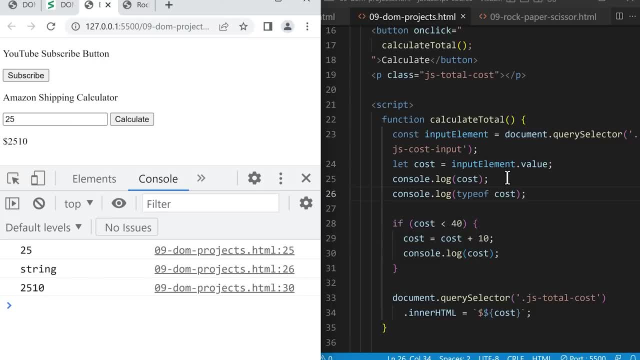 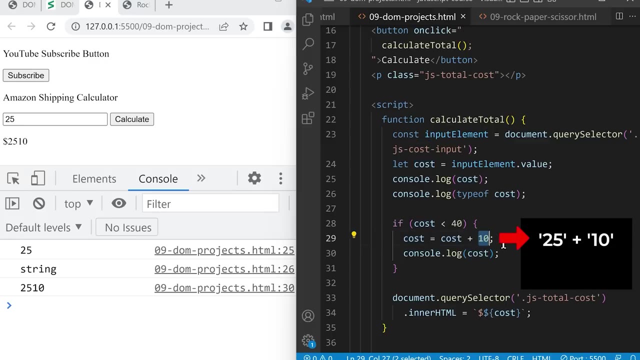 So this is actually not a number, It is a string. that's why it's not doing math. So remember from the strings lesson. So remember from the strings lesson: When we add a string with a number, JavaScript will automatically convert this number into a string. 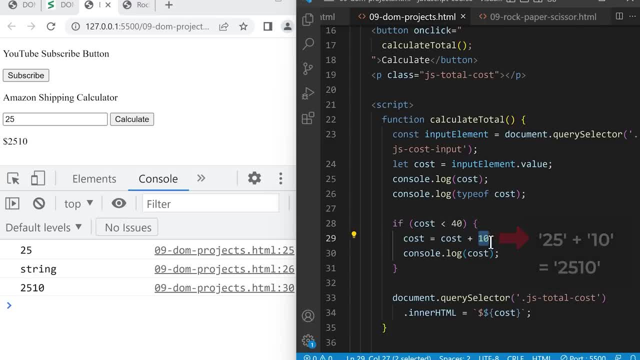 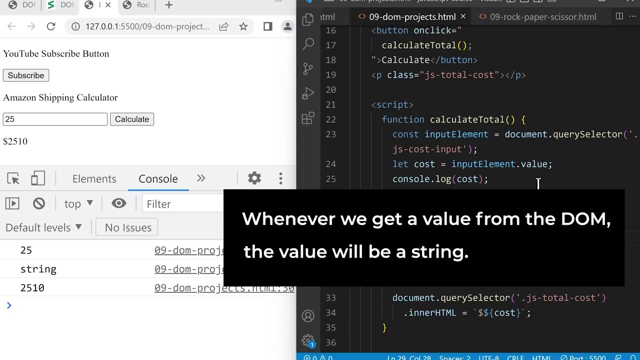 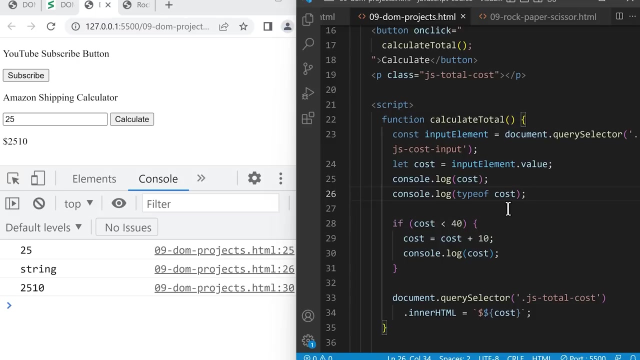 and combine them together. That's why it just combines 25 and 10 here. This is called type coercion. So whenever we get a value from the DOM like this, the value will be a string. So in order to do math, we have to manually convert this string into a number. 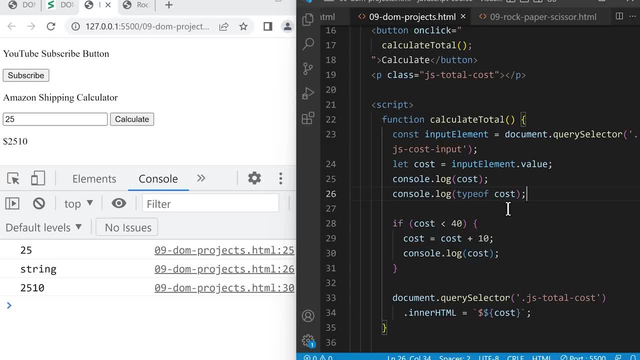 To do that, JavaScript has a built-in function called number. So before this code we're going to type capital, N, number, open bracket and close bracket. So the number function takes whatever's between the brackets and manually converts it into a string. 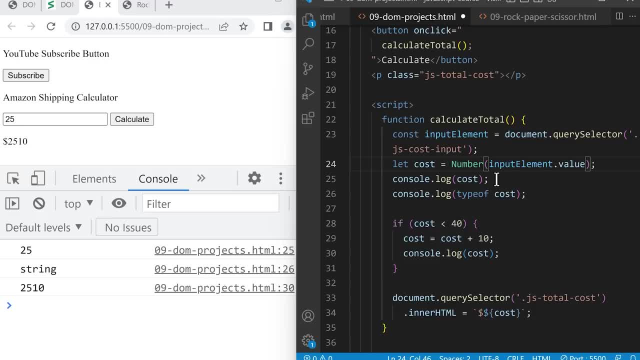 It manually converts it into a number. So now, if we save and we type 25, and press calculate, the cost is now a number and it will do the math properly and give us 35. So remember, whenever we get a value from the DOM, 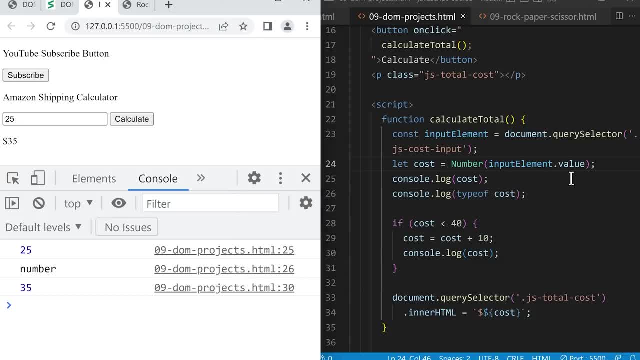 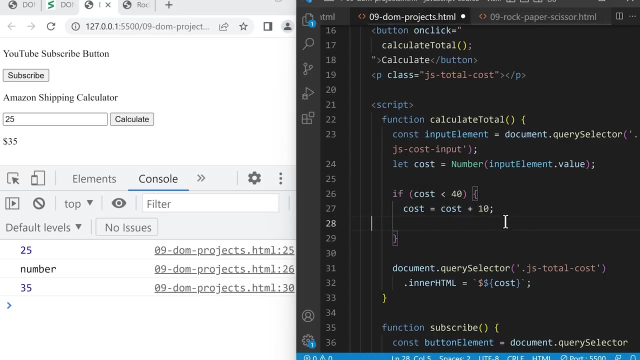 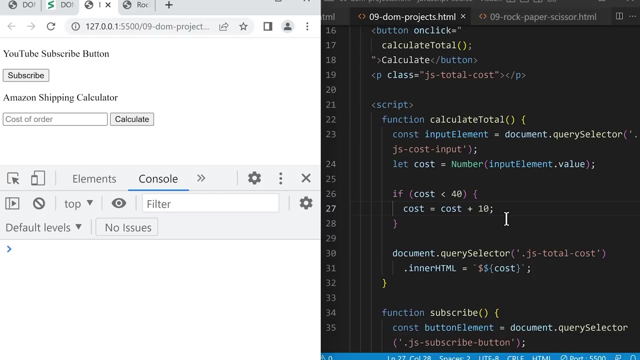 the value will be a string, So if we want to do math with it, we have to manually convert this value into a number first. So now let's remove the consolelogs that we used to figure out this problem And save. Okay, we're going to add one more feature to this project. 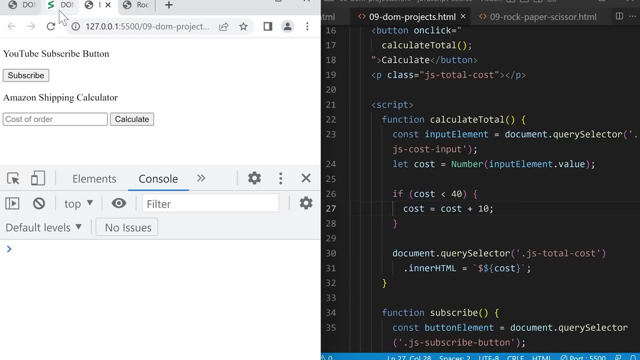 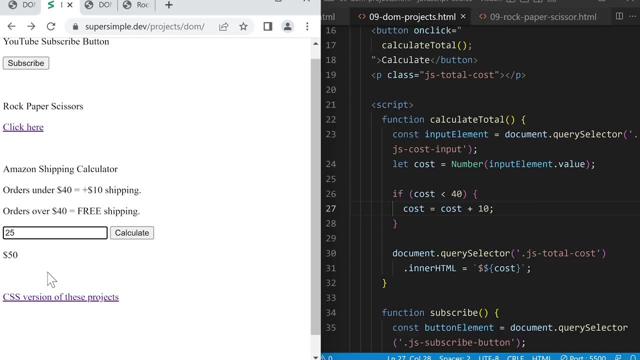 Let's go back to supersimpledev and inside the text box we're going to type 25, and press enter. So pressing enter will also calculate the total and display it on the page. So let's learn how to create this feature. 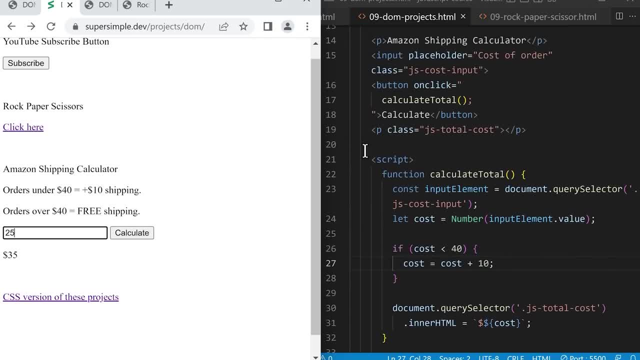 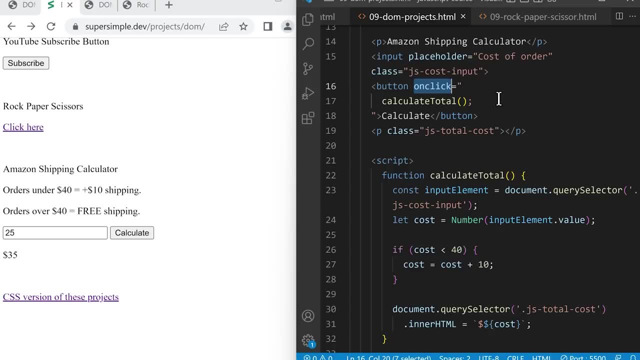 So, if we go back to our code, so far in this course we've been using the attribute onClick, which runs some JavaScript. when we click an element, HTML has another attribute we can use, called onKeyDown, which is a variable that we can use to create an element. 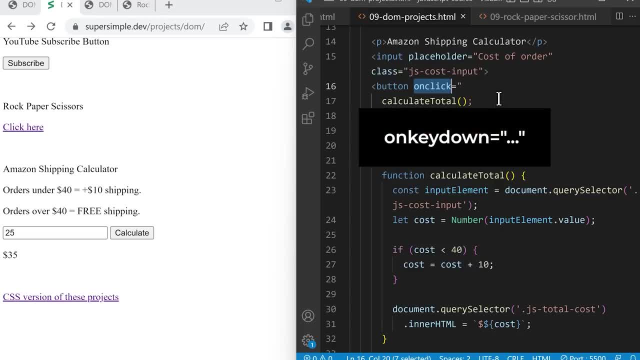 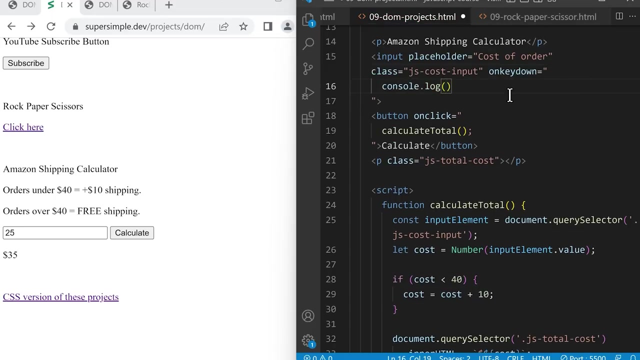 HTML has another attribute we can use, called onKeyDown, which runs JavaScript when we press a key down on our keyboard. So inside the input this time let's add the attribute onKeyDown equals double quotes. and then inside here: consolelog. 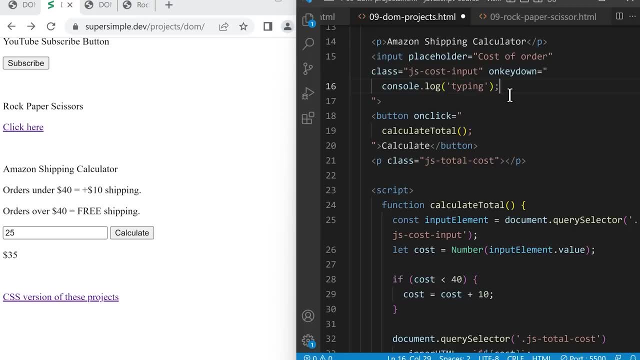 and the string typing. So now, every time we type a key down, every time we type in the input, it will consolelog this message. Let's save it and give it a try. We'll go to the tab for this file. 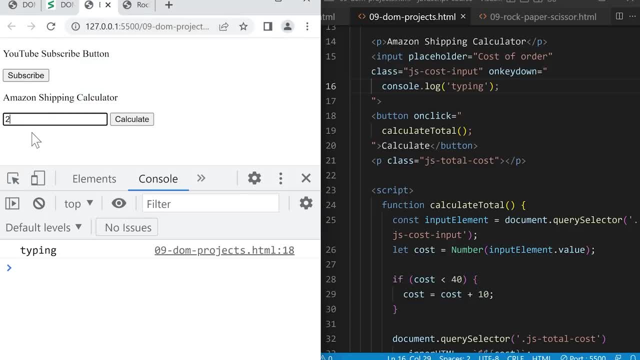 and then inside the text box we'll type some numbers And you can see that every time we type something, it will run this code and display this message. So that's how we do something when we type in an element. So clicks and key downs are known as events. 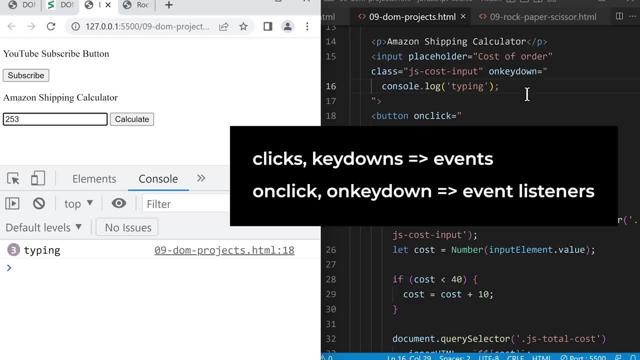 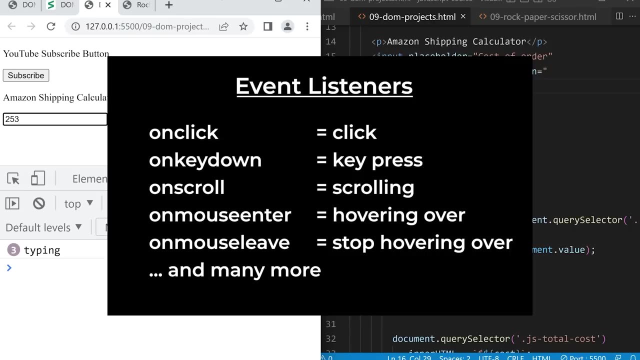 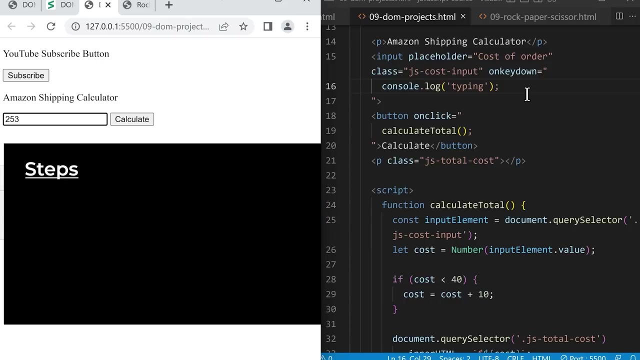 OnClick and onKeyDown are known as event listeners. They check for events and runs JavaScript when those events happen. Now, in addition to clicks and key downs, there are many other events we can listen for in JavaScript. Okay, so now let's figure out what steps we need to do. 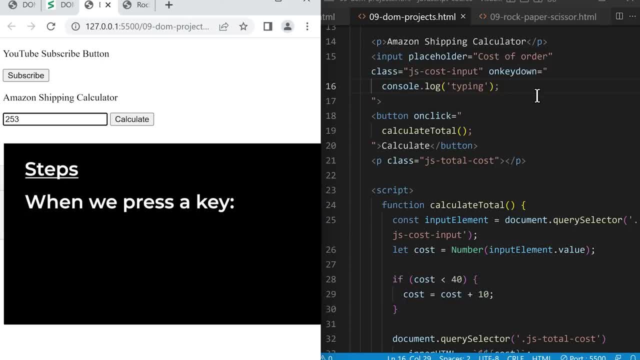 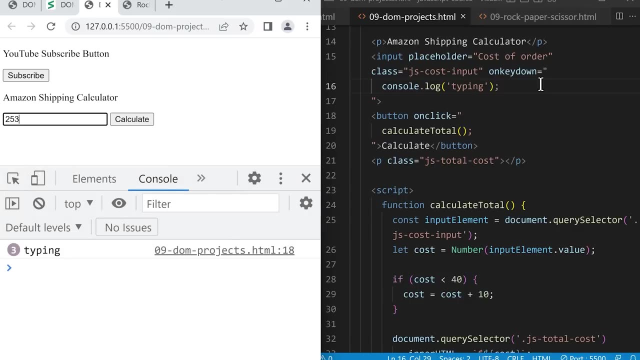 for this project. When we press a key down in the text box, we're gonna check if the key is the enter key. If it is, we'll do the same thing as the calculate button. So how do we know what key we pressed? 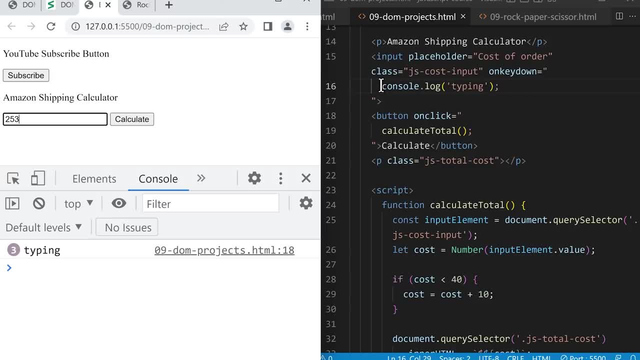 Inside onKeyDown, we're actually given a special object called event. So instead of this string, let's remove it and we'll consolelog event. So this is an object that's provided to us by JavaScript and it contains information about the event. 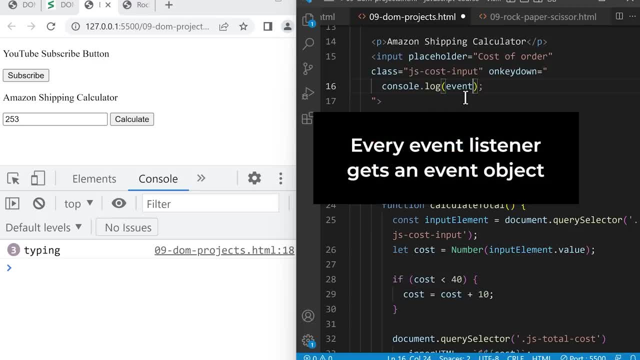 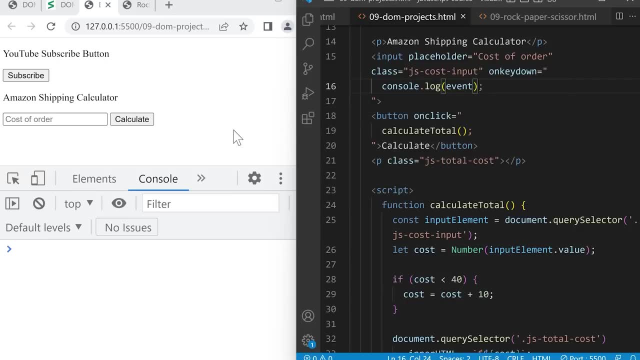 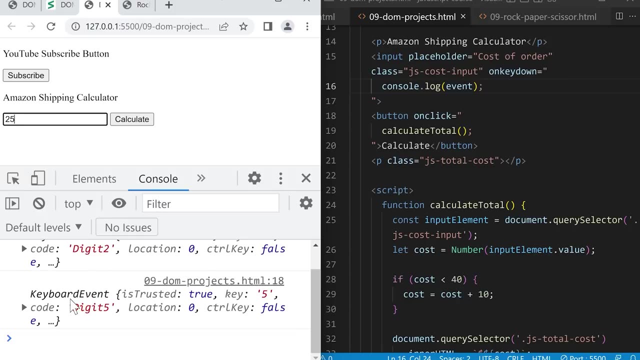 Every event listener, including onClick, also gets an event object. If we save and type in this text box it will show us that event is this object And inside the object it has a bunch of information, including the key that we typed. 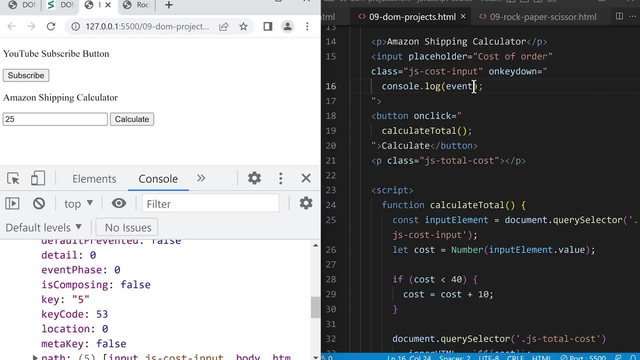 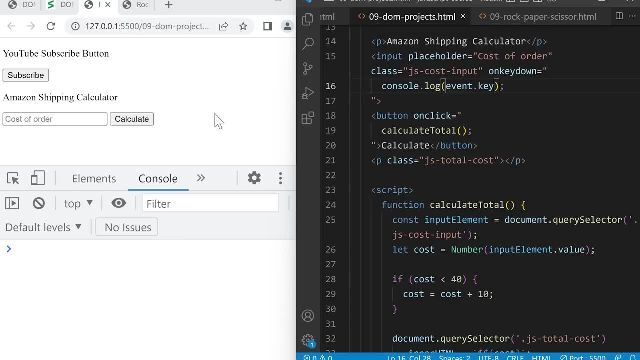 So here let's use the event object and we'll get key and save. So now inside this text box, if we type something, it will tell us the key that we pressed, And if we press enter, it will tell us that the key. 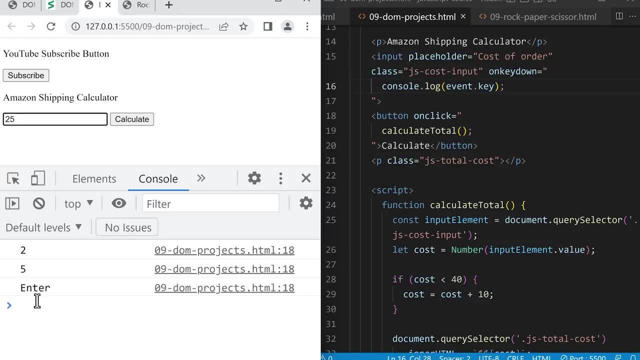 that we pressed is the event object, And if we press enter, it will tell us that the key is the event object. It will tell us that the key is enter. So the next step is to check if the key is enter. 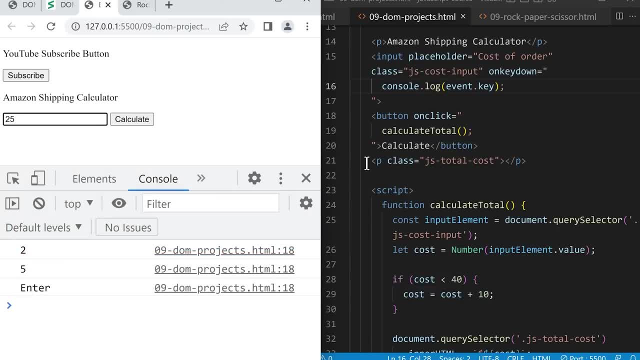 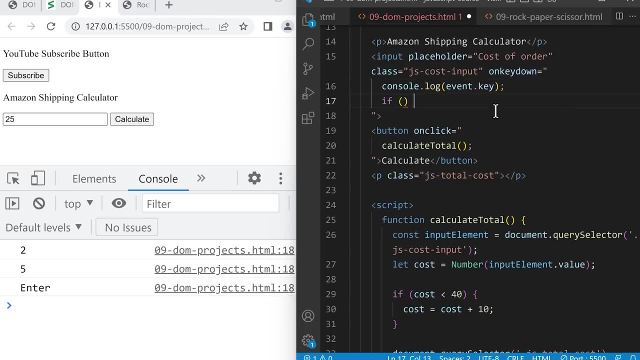 And we can do that using an if statement. So in our code we'll type a new line if brackets and curly brackets, and inside the condition we'll check if eventkey is equal to the eventkey And inside the condition we'll check if eventkey. 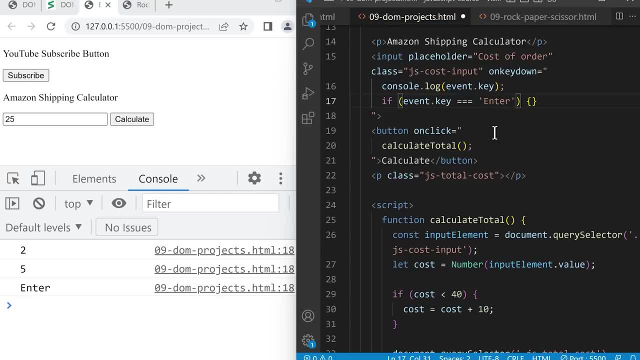 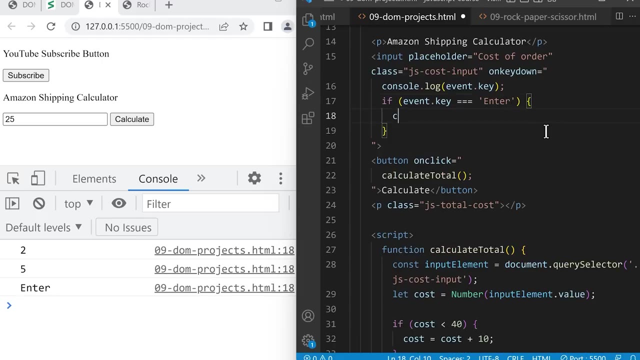 the string enter if it is equal to enter. we're going to do the same thing as the calculate button, so we can actually just use this function again inside the curly brackets. we'll type calculate, total and brackets and save. so now let's go back to our project. 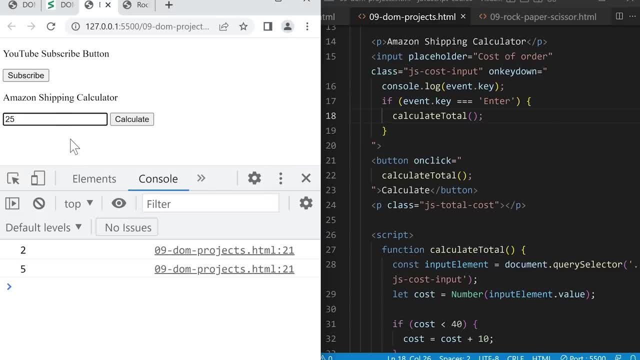 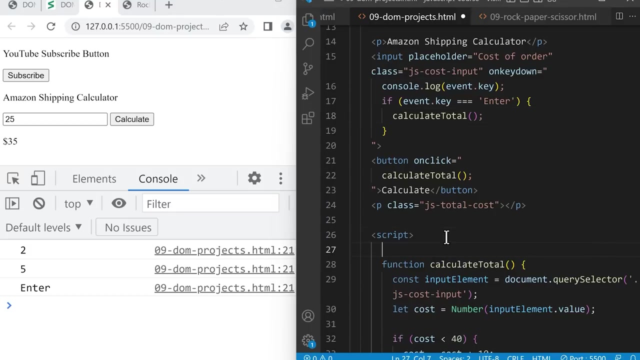 and type 25, enter and it will calculate the total and display it on the page. so that's how we create this keyboard feature of this project. lastly, let's clean up our code and move this into a function like the rest of our code. so, inside the script element, let's create a new function using 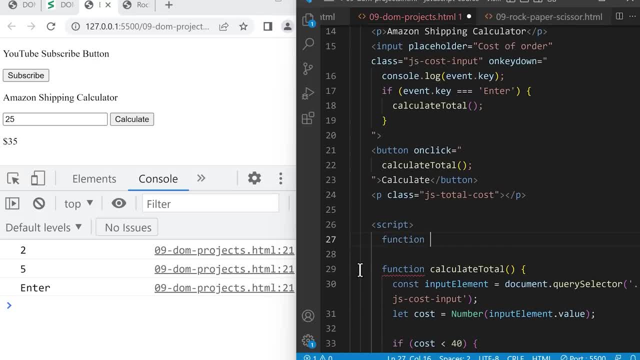 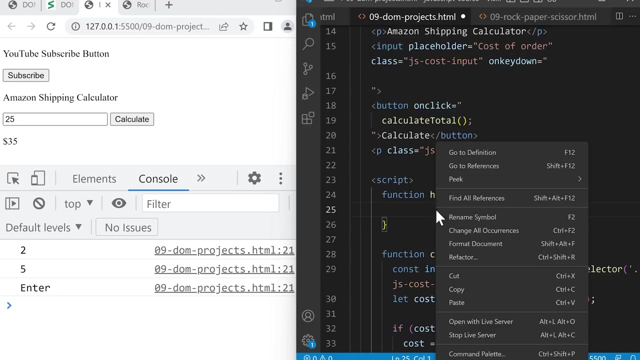 function, function, function, function, function, function, function and we'll name it: handle, cost, key down brackets and curly brackets and let's move this code into the function. we'll select it: right click, cut and in here, right click and paste. if we need to fix the formatting, we can select these lines: 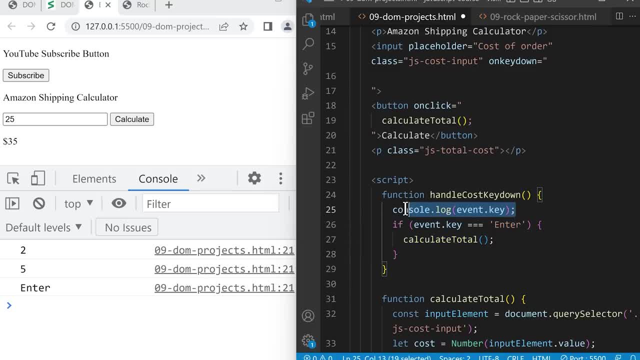 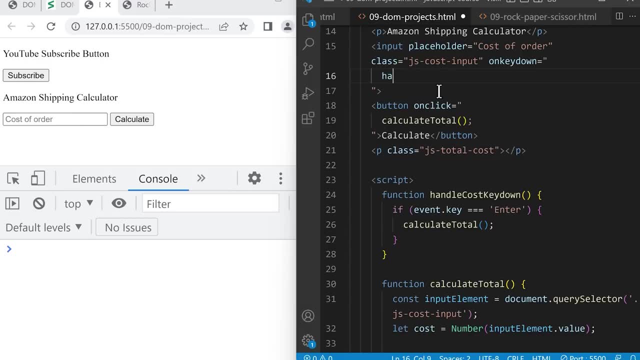 and we can go ahead and create a new function and press tab and let's remove this consolelog. and now up here we're going to call this function: handle cost, key down and brackets. now the last thing we have to do is that event does not exist inside this function, so we have to put the event object into the function. 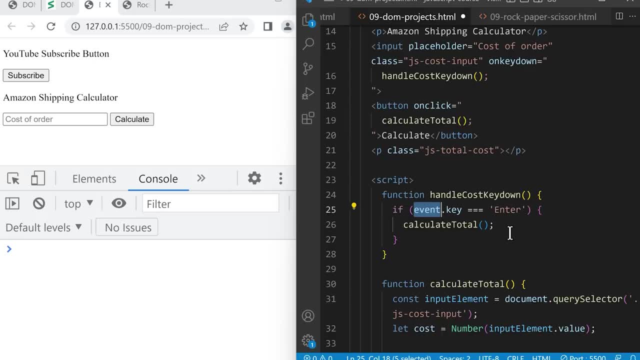 function. And remember, to put a value into a function we can use a parameter. So between these brackets we can create a parameter called event. And now to save something inside this parameter, we're going to go up to these brackets and type event. This will take the. 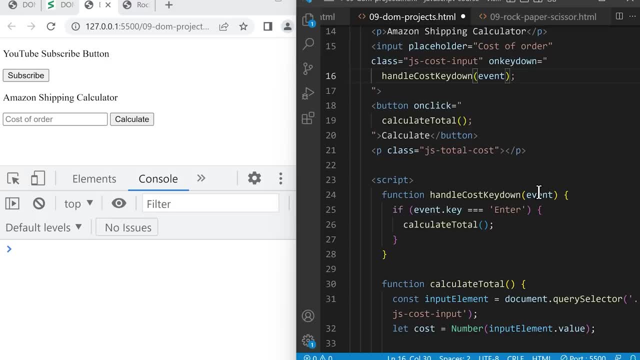 event object and put it inside the function where we can use it just like a variable. So now, if we save and try out the project 25, enter, so this still works. And now we've finished all three projects in this lesson, So in the rest of this lesson we're going. 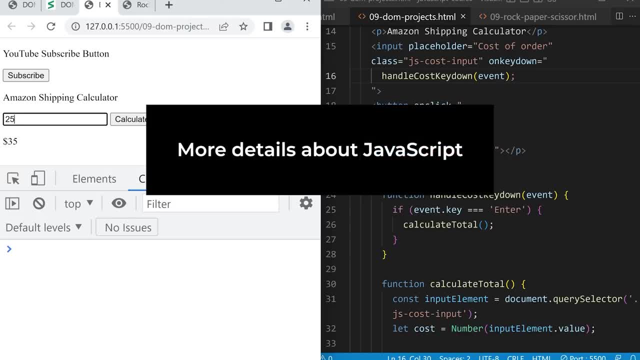 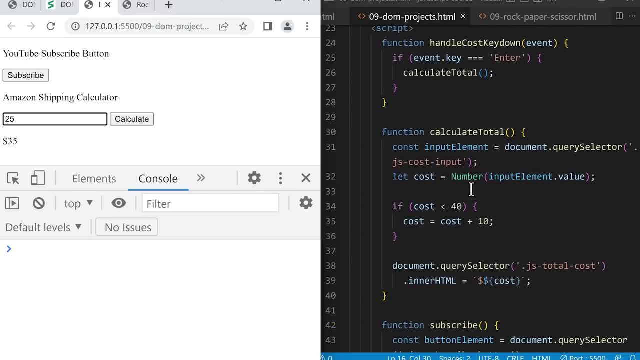 to learn some more details about JavaScript. In the last project, we learned how to manually convert a string into a number using the number function. We can also convert the other way, from a number to a string. So let's go to the top of the. 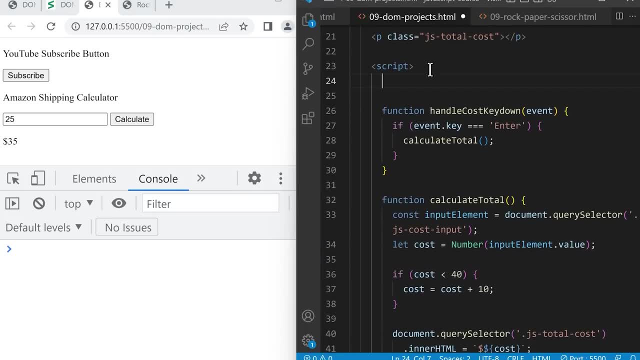 script element And we can type capital, S, string and brackets. So the built in string function will convert a value into a number. And yes, now we know the cost of constant string fixing. Between the brackets we can put a number like 25, and this will convert the number into these string 25.. The next: 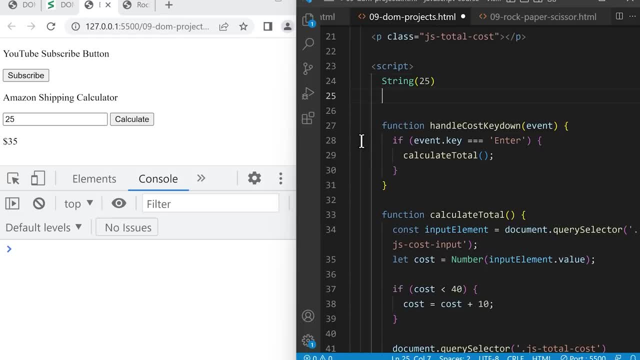 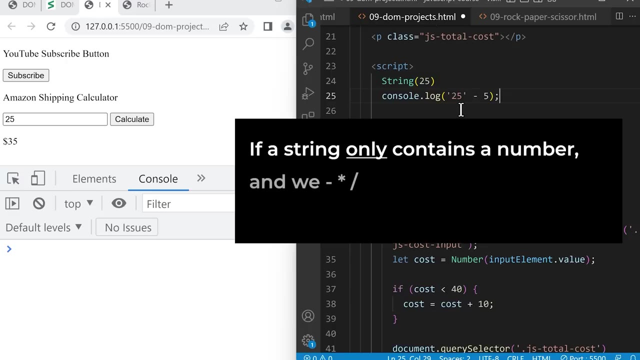 detail we're going to learn is a special behavior of strings. So below this line we can type consolelog: the string 25 minus 5.. So if a string only contains a number and we subtract, multiply or divide, JavaScript will automatically convert this string into a number. 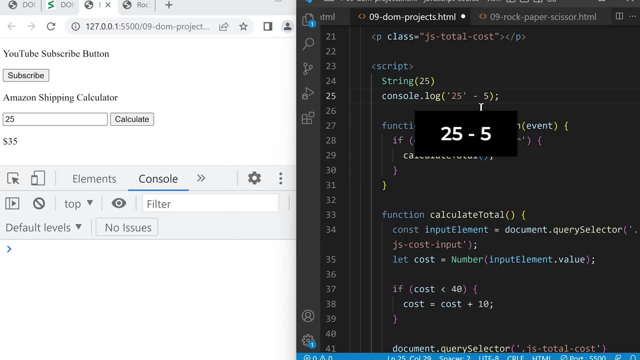 So this gets converted into the number 25 minus 5. And if we save, it will do math and give us 20.. So this is another example of type coercion or automatic type conversion. However, it's not recommended to do math with strings like this, because adding works. 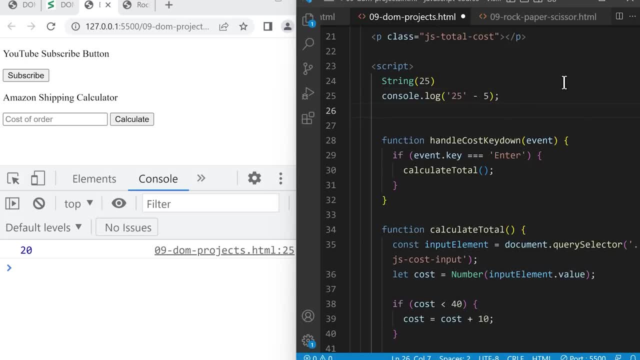 differently. For example, on a new line let's type consolelog the string 25 plus 5. And save. This will convert the number into a string and combine them together into 255.. So because adding strings works differently, the best practice is always do math using. 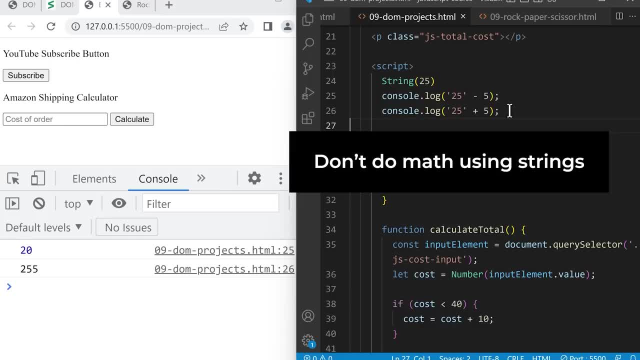 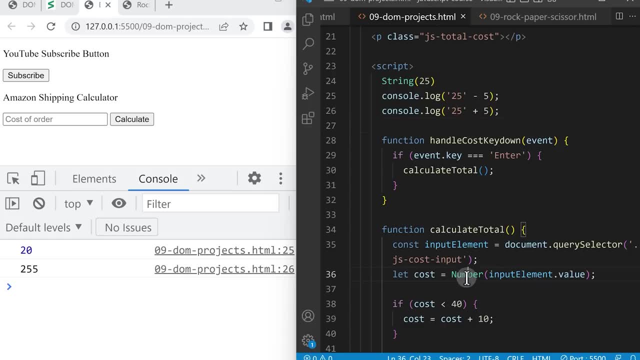 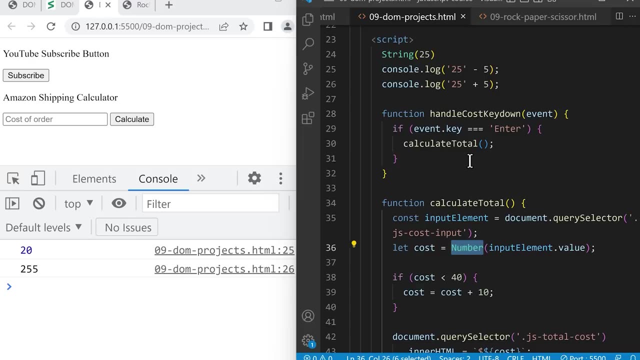 numbers. don't do math using strings. If we need to, we can manually convert the string into a number using the number function, like we did here. The last thing we're going to learn in this lesson is another built-in object called. 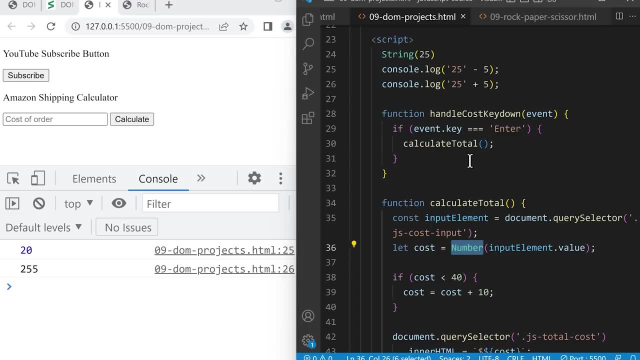 the window object. So in this lesson we learned about the document object. The document object represents the web page. The window object represents the browser. So let's go into our script element and try it out. Below this we'll type window. 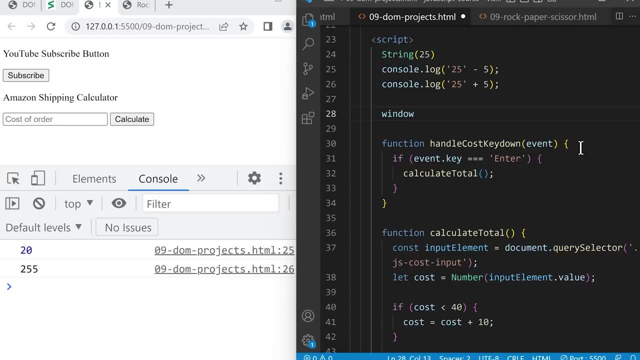 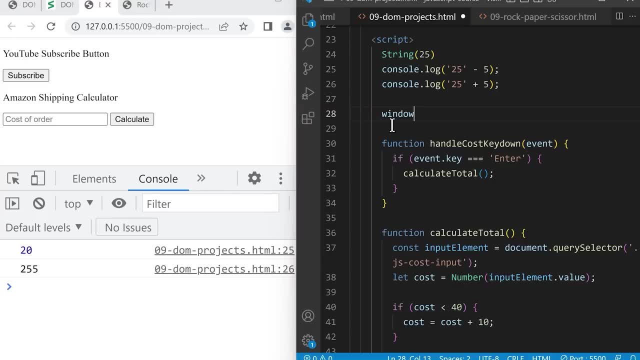 So let's think What's inside the browser? Well, the web page is inside the browser, So the document object is inside the window object. That's what I arms Sign into. End of memorization. End of it document. this will give us the same document object that we've been using in. 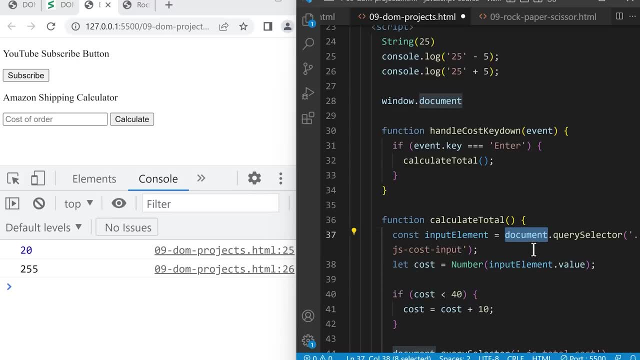 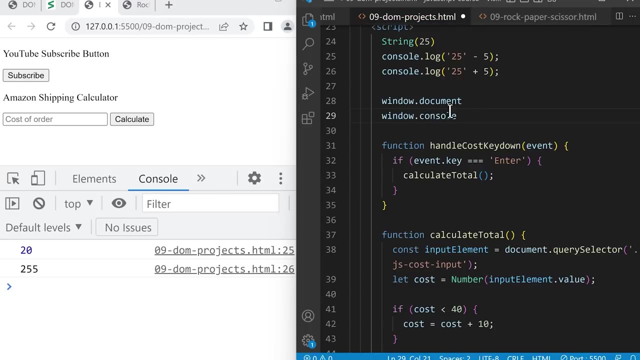 this lesson. so what else is part of the browser? well, the console is also part of the browser. so here, if we type window dot, console, this will give us the same console object we've been using in this course. so we can actually do console dot, log and the string window and save, and this will do the same thing as console. 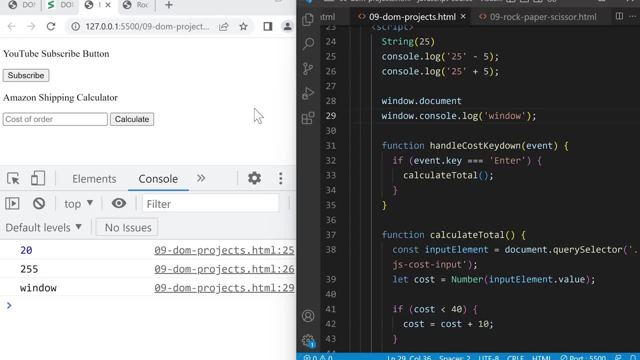 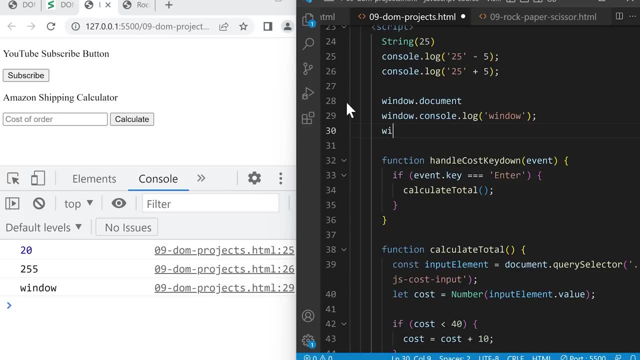 dot log. what else is part of the browser? well, pop-ups are also part of the browser. so if we type window, Oh dot alert, This will give us the same alert function that we've been using in this course to create pop-ups. However, you might have noticed that we never type window dot document. 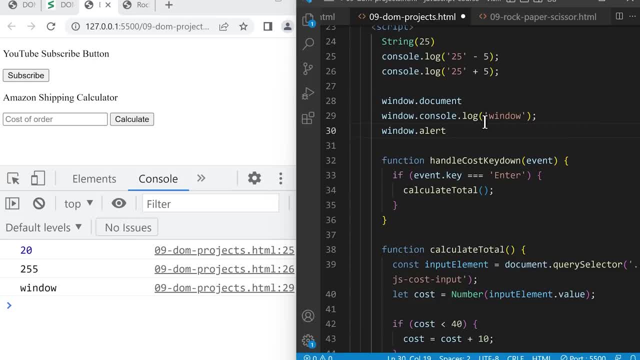 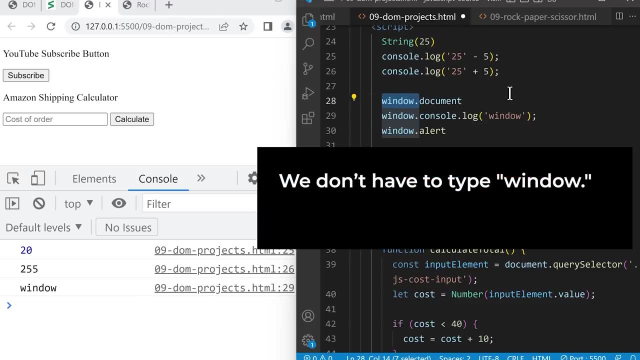 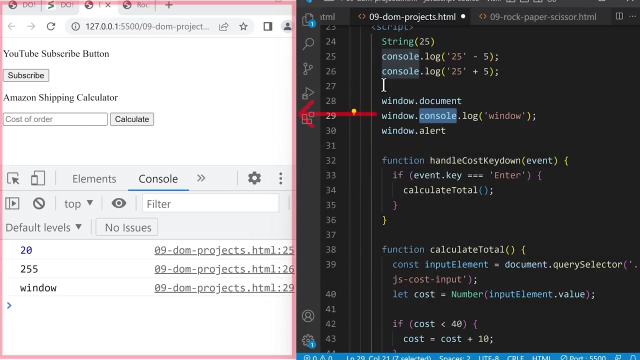 or window dot, console, dot, log. And that's because the window object has a shortcut. We don't have to type window dot at the front, We can just type document or console and JavaScript will automatically add window dot at the front for us. So window is a built-in object. that 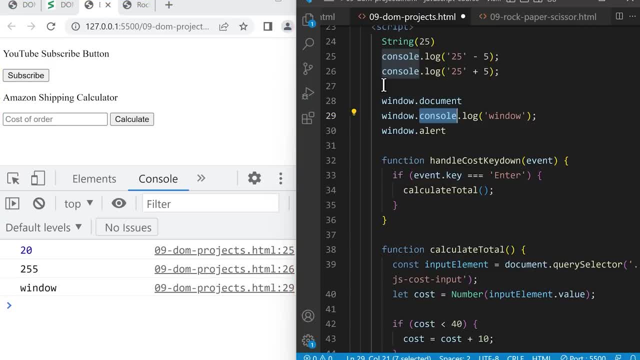 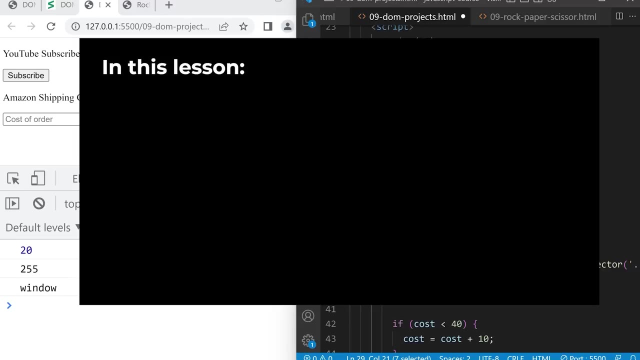 represents the browser. We don't have to type out window dot ourselves, because JavaScript adds it for us automatically. But it's still nice to know how this works behind the scenes. And that's the end of this lesson. In this lesson we learned about the document object. 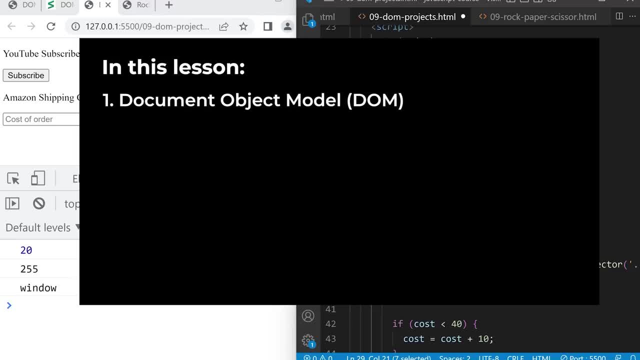 model or the DOM which allows JavaScript to fully control the web page. We learned how to use document dot query selector to get elements from the web page and put them inside our JavaScript. We learned how to use inner HTML to modify the HTML inside an element. 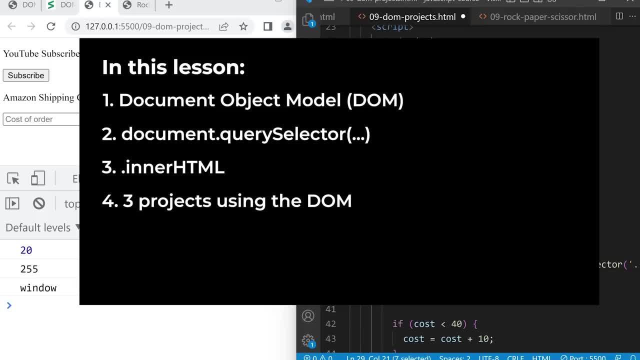 We will see you in the next lesson. We worked on three projects using the DOM, We learned how to make elements interactive with the keyboard using on key down, And we learned some more details about strings, as well as the window object which represents the browser. Here are some exercises you can do on your own. 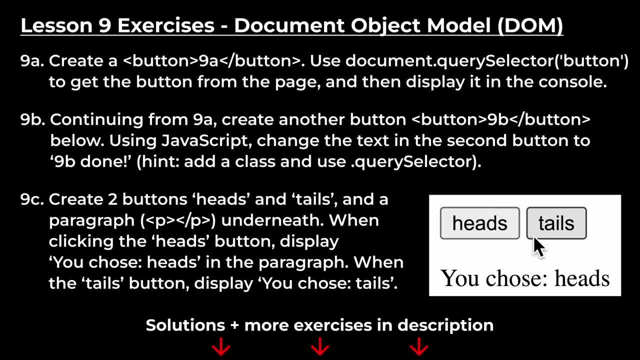 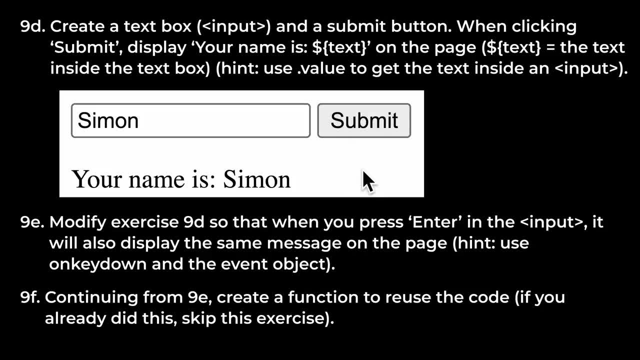 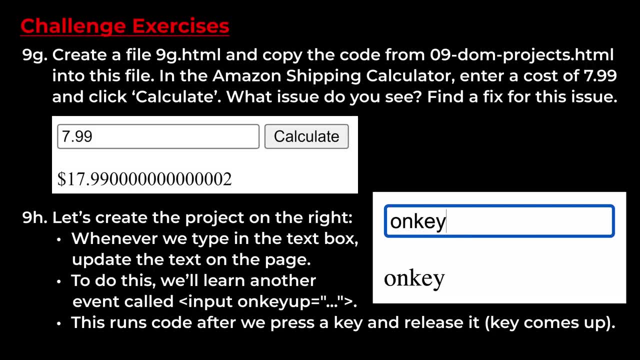 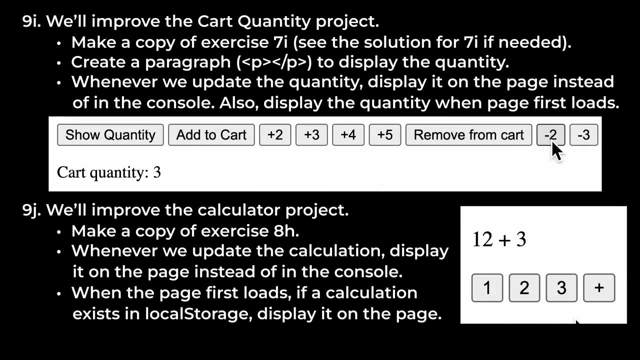 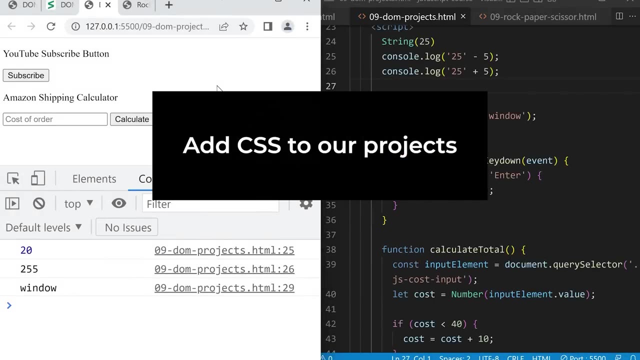 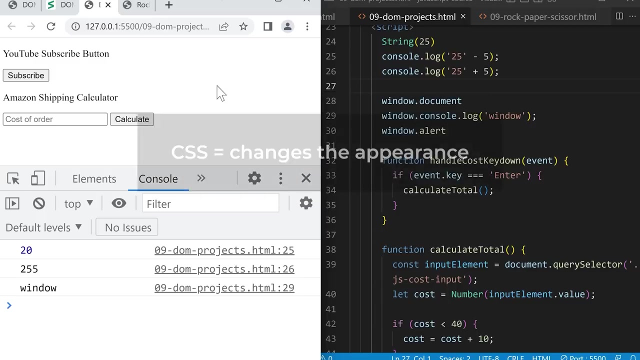 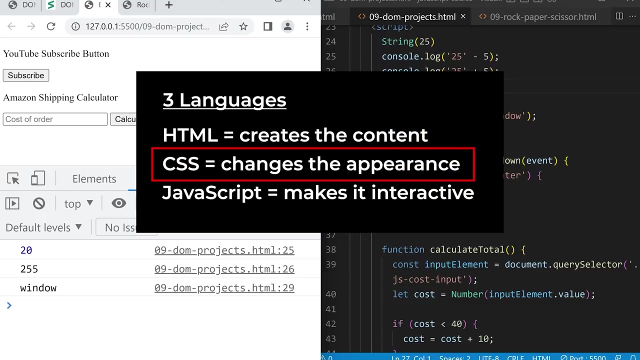 to practice using the DOM In this lesson. we're going to add CSS to all of our projects And we're going to finish our rock paper scissors project. CSS is a different language that changes the appearance of our website. It's one of the three languages that we use to create websites. 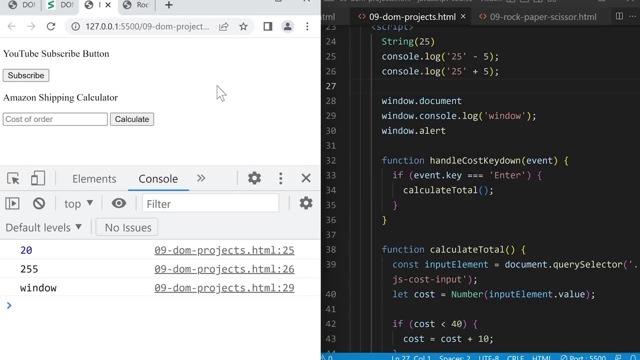 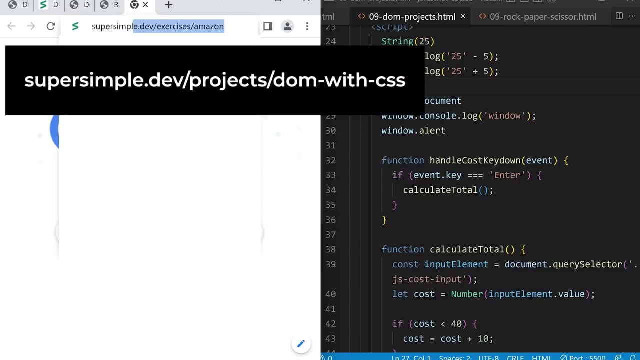 So first let's look at the projects we're going to work on in this lesson. We'll go to our browser and create a new tab at the top, And here we're going to type supersimpledev- slash projects, slash- dom-with-css, and press enter. 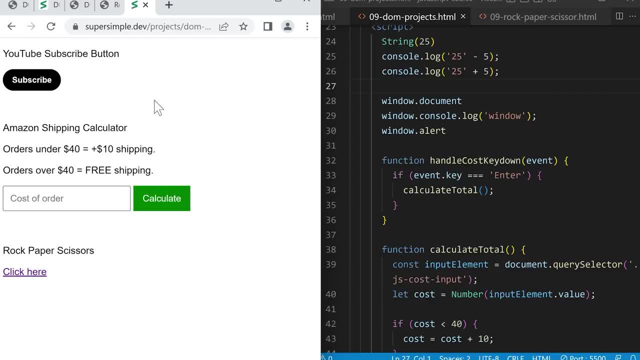 So these are the same three projects we created in the previous lesson, except this time we're going to add CSS to make these projects look nice. Let's start by creating a copy of the project's HTML file from the previous lesson. We'll go to our code editor and click this icon to show our files. 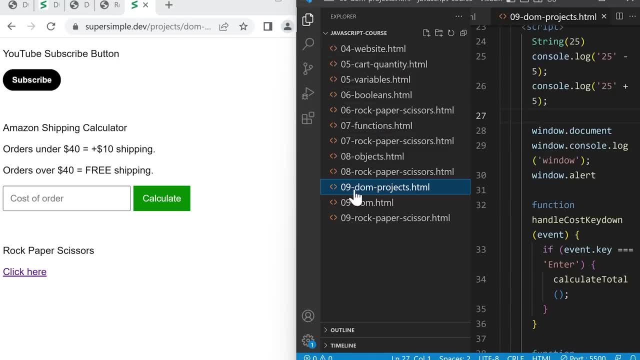 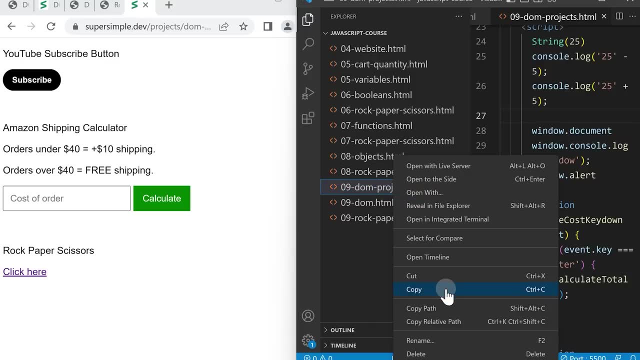 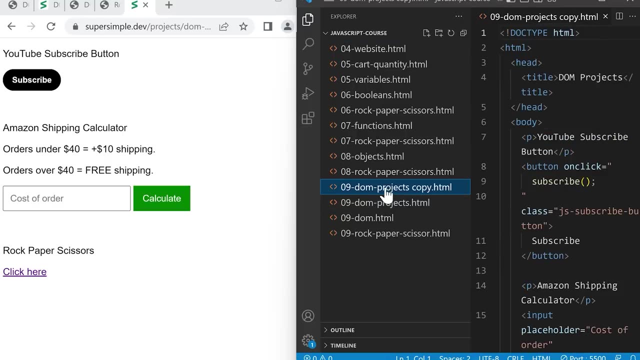 And then here we're going to select 09-dom-projects, We're going to right-click, copy And down here, right-click and paste And let's rename this file by right-clicking rename. At the end we're going to remove copy. 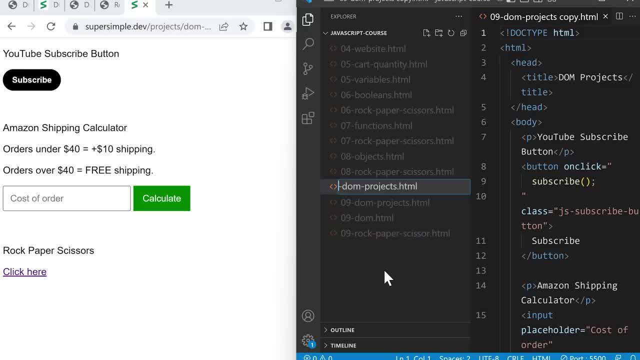 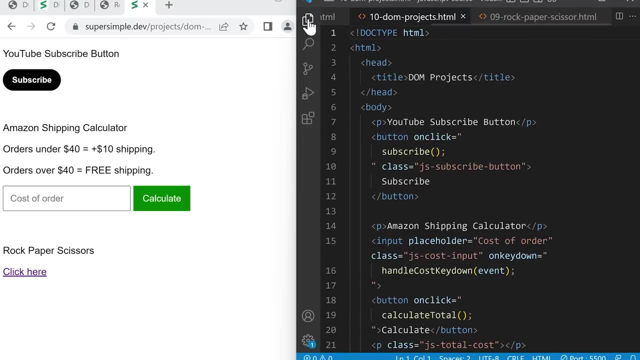 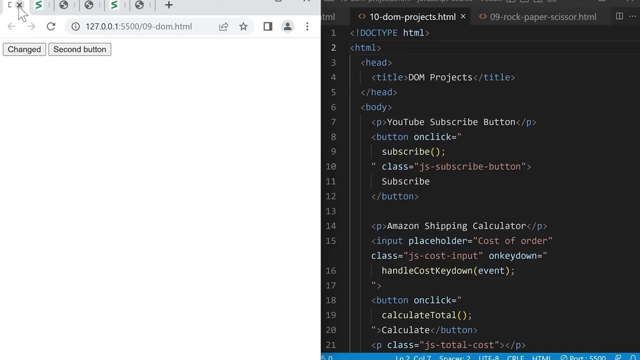 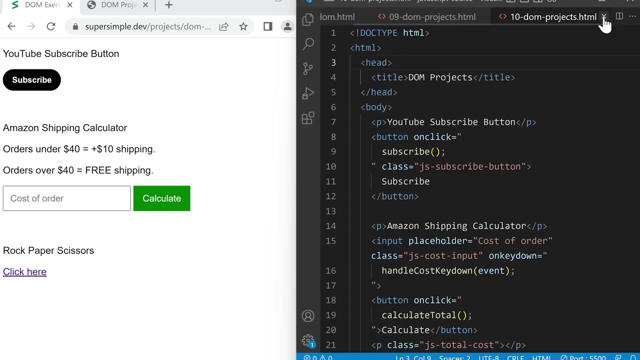 And at the beginning we're going to change it to 10 and press enter. Now let's hide our files And we're going to open 10. dom-projects in the browser by right-clicking: open with live server. Now we can close our previous tabs, as well as the previous code from lesson nine, which is this file and these two. 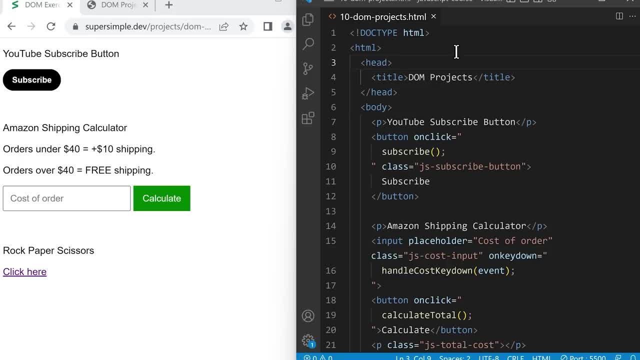 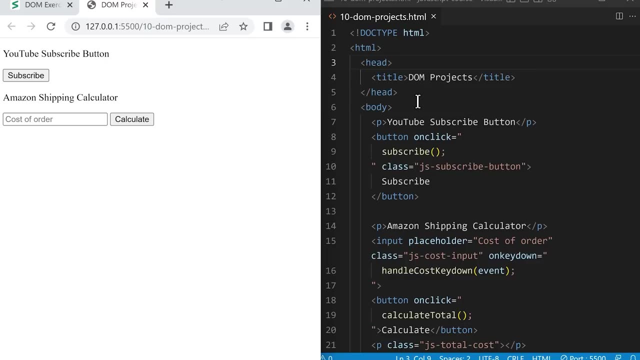 And now we're ready to add CSS to our projects. We'll start with the YouTube subscribe button. Let's go to the tab for our project And we're going to style this button first. So we reviewed CSS in lesson four And one of the ways we can write CSS code is using the style element. 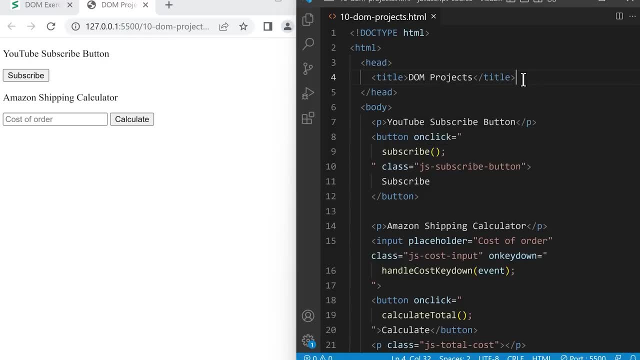 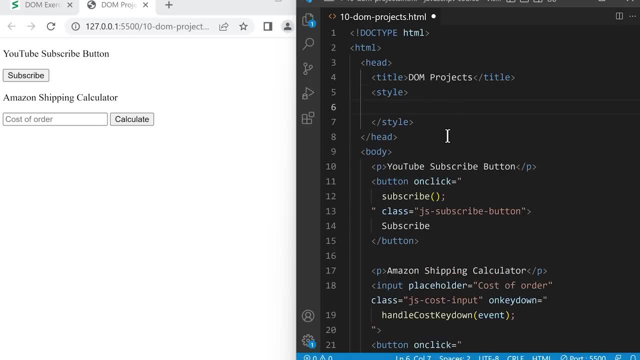 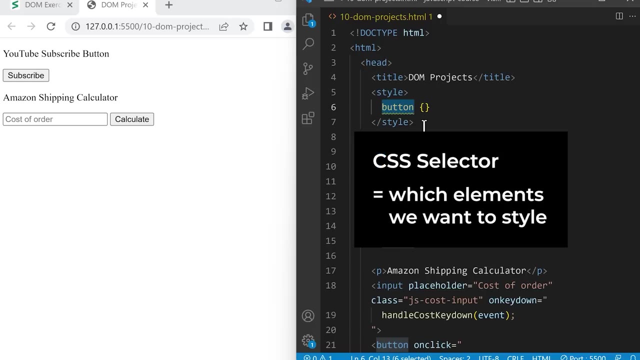 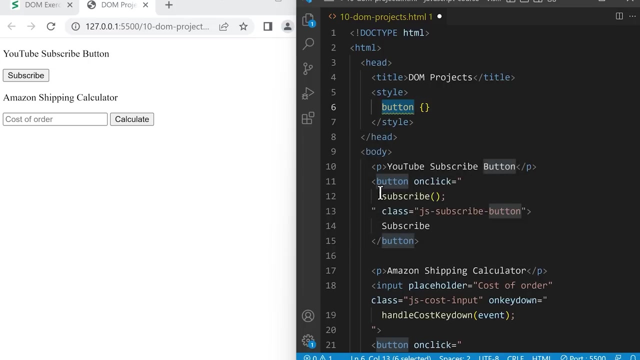 So inside here we're going to write button open, curly bracket, close curly bracket. So the code in front of the brackets is called the CSS selector. This tells the computer which elements we want to style or change the appearance. So button will style all button elements on the page. 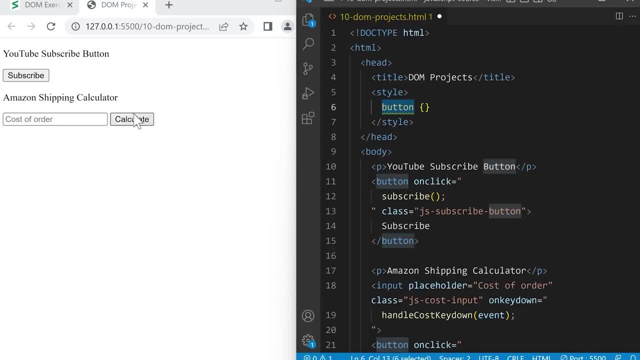 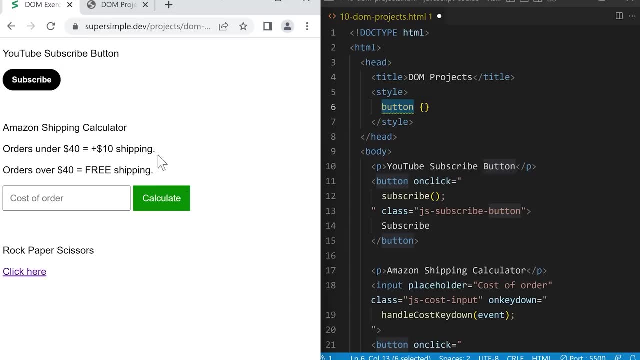 But in this situation we only want to style the subscribe button, Because the calculate button will be styled differently. So to style a specific element we can use the class attribute. So if we look at our button currently, it already has a class of JS subscribe button. 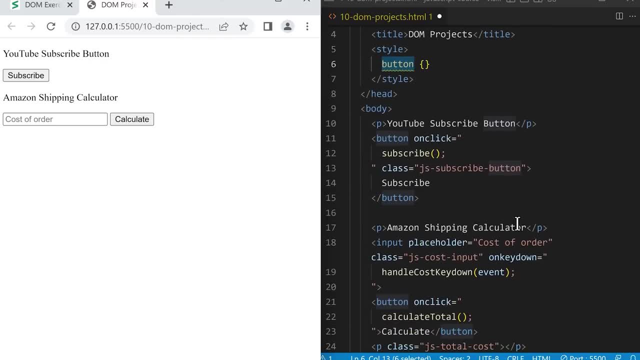 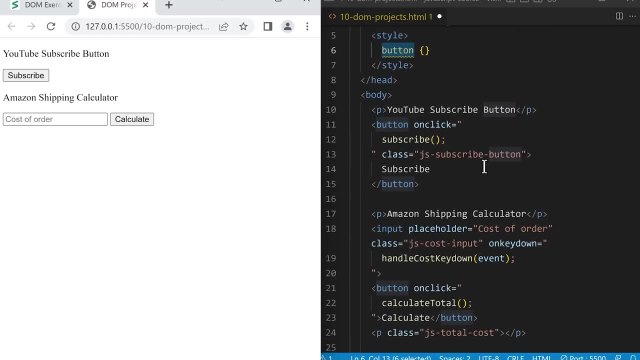 But this class is being used by our JavaScript. A good practice Is to add a different class that will be used by CSS, So an element can have multiple classes. We just separate them with a space. So inside this class attribute we're going to type space and add another class. 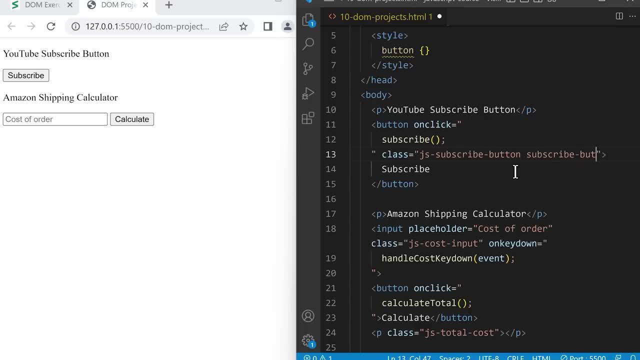 Subscribe dash button. Now this element has two classes and we're going to use this second class in our class, In our CSS. so to style a specific class, we're going to remove button and we're going to type a dot. So starting with a dot means we're going to style a class rather than an element name. 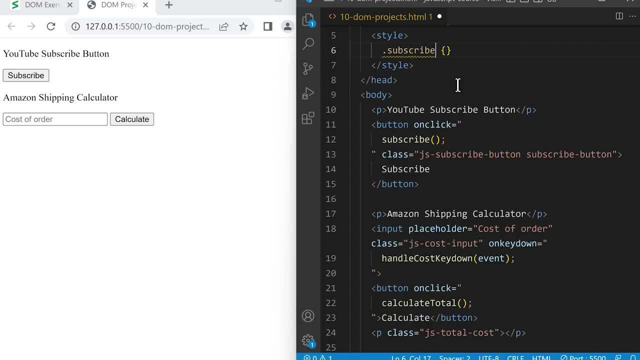 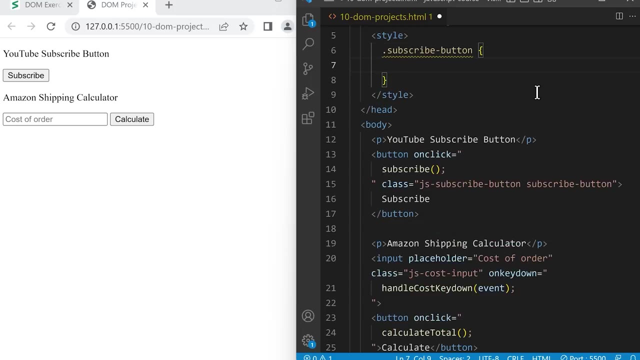 So we'll style the class subscribe dash button, which is this button right here and now, inside these curly brackets, we're going to tell the computer how to style this button. For example, border, colon, none and semi-colon. 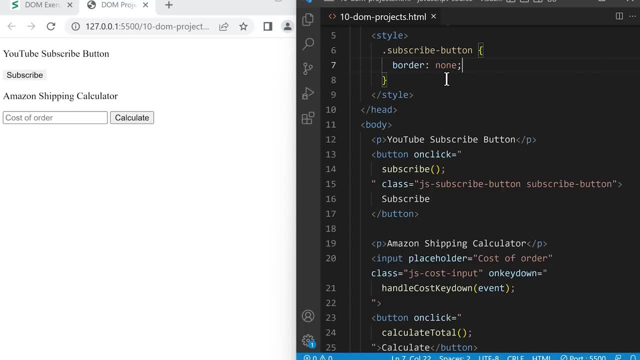 If we save, this will remove the border from the button, So it no longer has a border like this button. So that's how we style a specific element with CSS. We add a class to the element And then inside CSS, we start with a dot and the class. 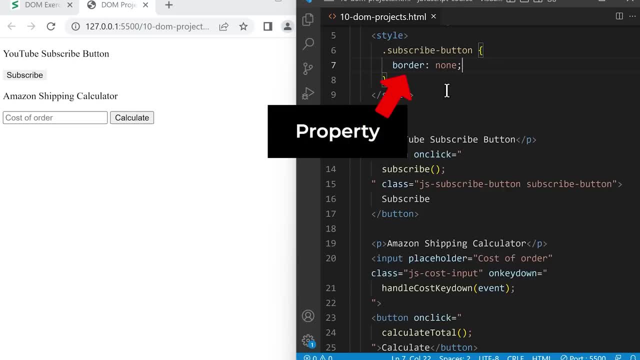 And between the curly brackets, the code on the left is called the property. This tells the computer what we want to change. On the right is called the value. This tells the computer what we want to change the property to. We separate the property and value with a colon and we end the whole thing with a. 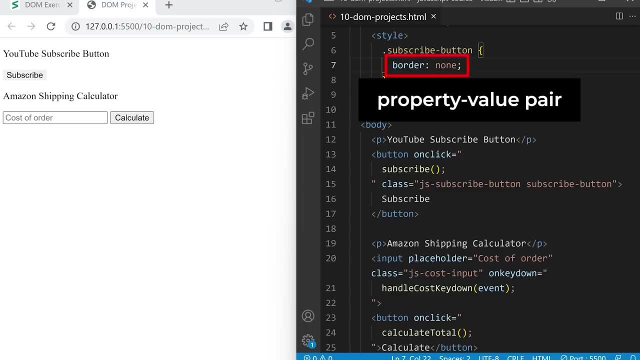 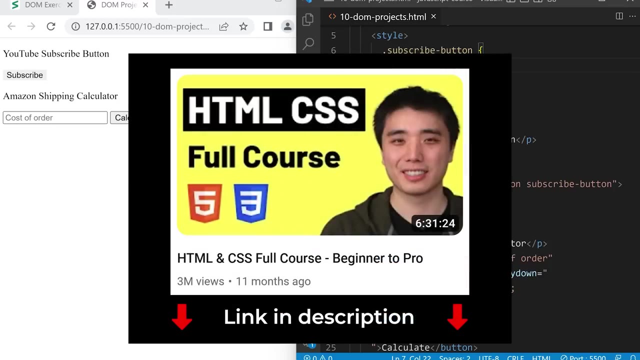 semi-colon, So this is also called a property-value pair. As a reminder, this is just a review of CSS. If you want to learn CSS in more detail, you can check out my HTML and CSS full course in the video description. 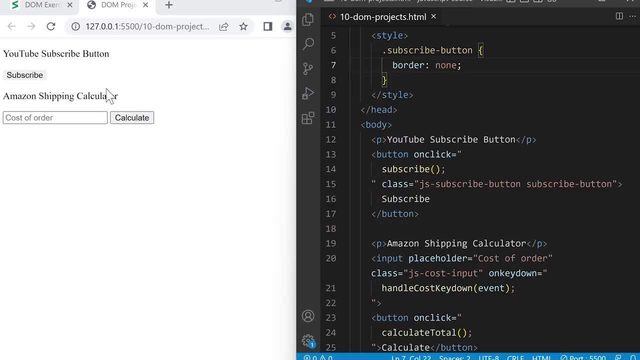 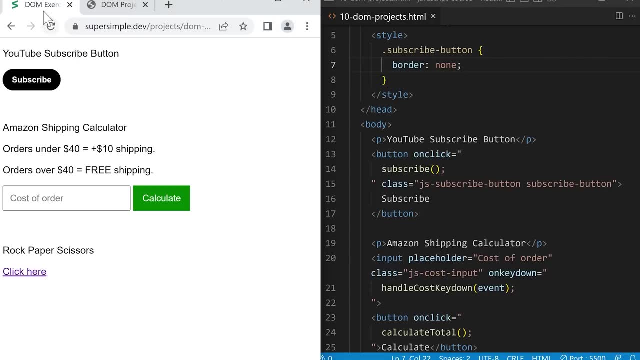 So we just added one style to this button. We're going to add more styles so that it looks like our final design. To make this easier, I'm going to rearrange my windows And I'm going to put the final design at the bottom and then our project at the top. 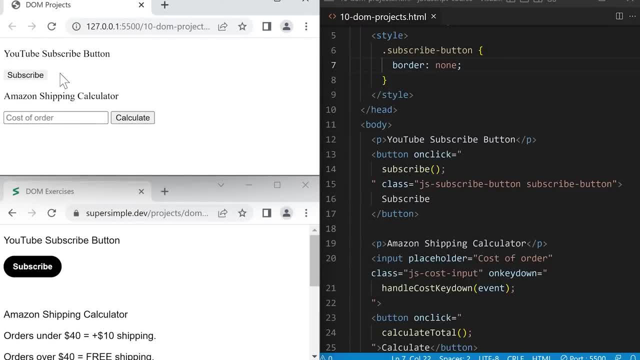 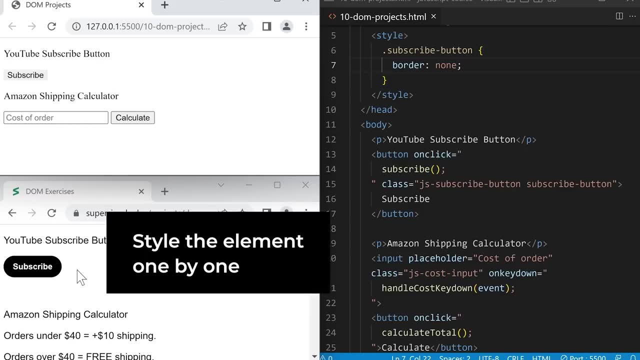 This will make it easier to compare the two designs. Next, to make it look like the final design, we're going to style our element one by one. Let's go back to our code and press enter, And next let's change the back-end. 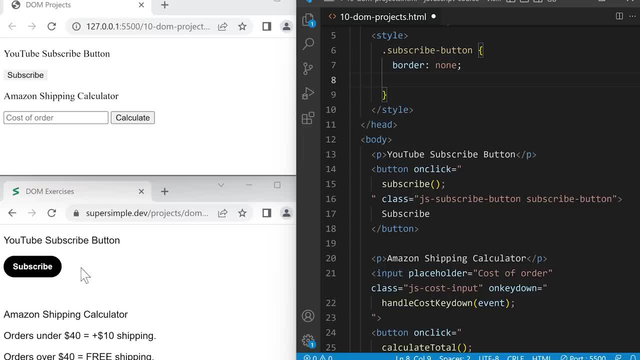 We're going to change the back-end. We're going to change the background color to black. To do that, we'll type background dash, color, colon black and semi-colon and save. Now our button has a black background. Let's keep going, one by one. 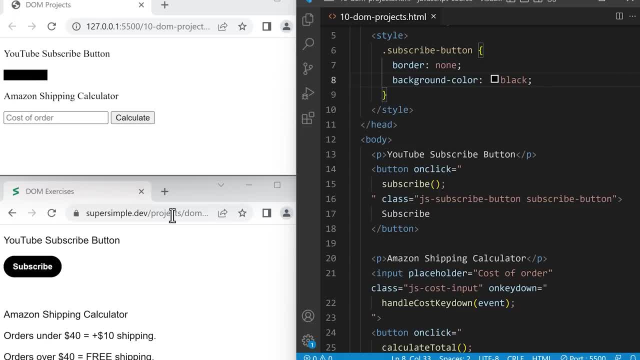 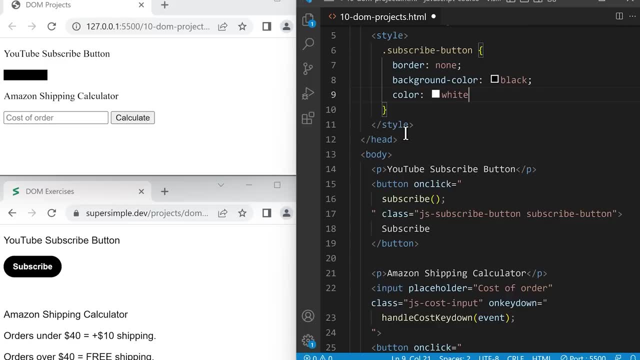 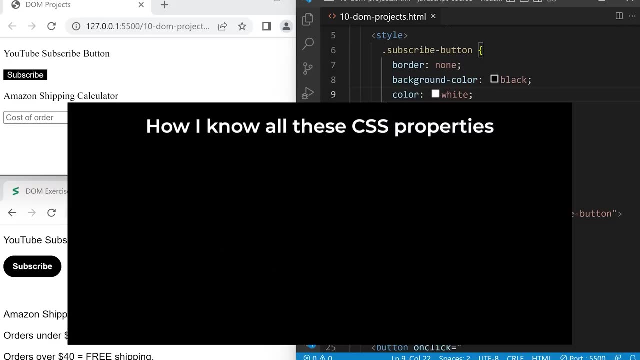 We'll change the text color to white next. So in our code we'll type color, Color, colon, white and semi-colon and save. Now if you're wondering how I know all these properties, you can usually find them by searching in Google. 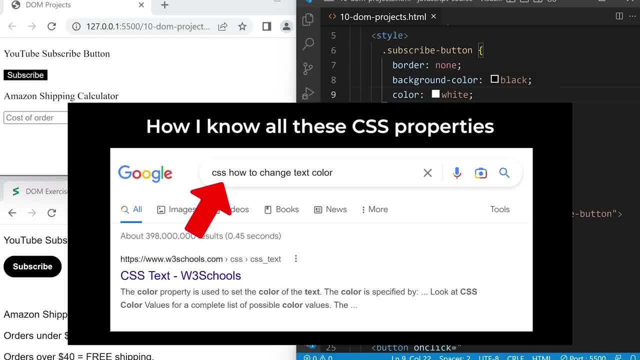 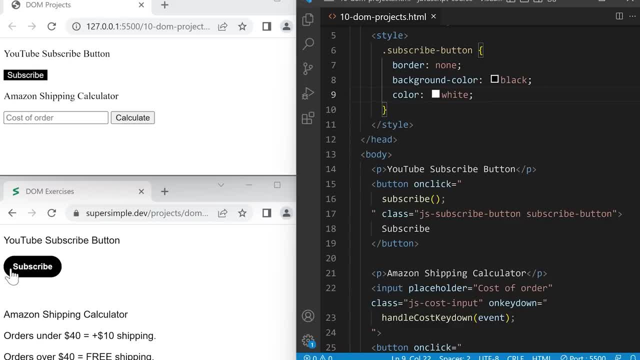 Just make sure you search for what you are trying to do. Let's keep going one by one. The next thing we'll change is we're going to add spacing on the inside of the button In CSS. we're going to add spacing on the inside of the button. 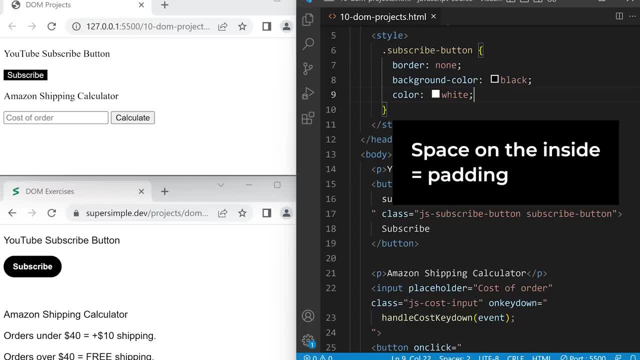 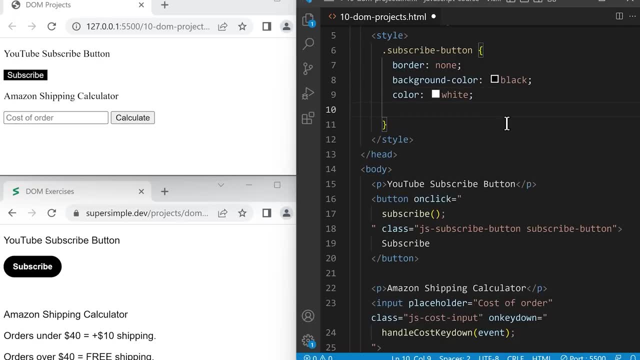 In CSS, space on the inside of an element is called padding, So we'll create a new line and we'll use the property padding-top colon 10px and save. So this will add space on the inside of the element called padding at the top of 10px. So we'll add space on the inside of the element called padding at the top of 10px and save. So we'll add space on the inside of the element called padding at the top of 10px and save. So we'll add space on the inside of the element called padding at the top of 10px and save. 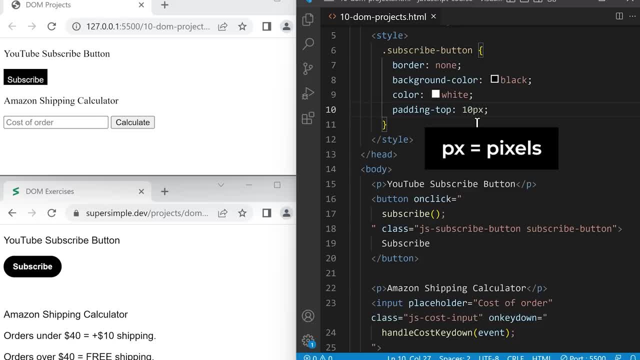 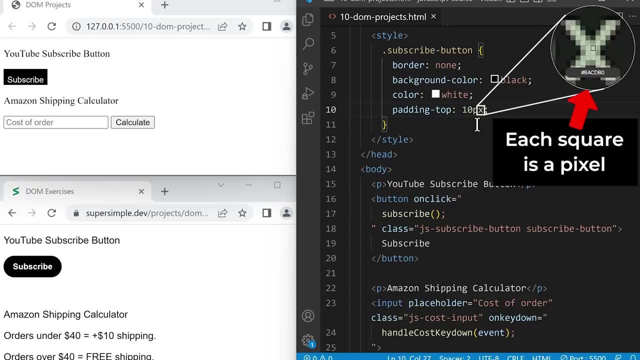 So the px here means pixels. A pixel is a unit of measurement in computers. Your screen is made up of many small little squares. Each of these squares is called a pixel. So a pixel is the smallest thing that you can have on your screen. 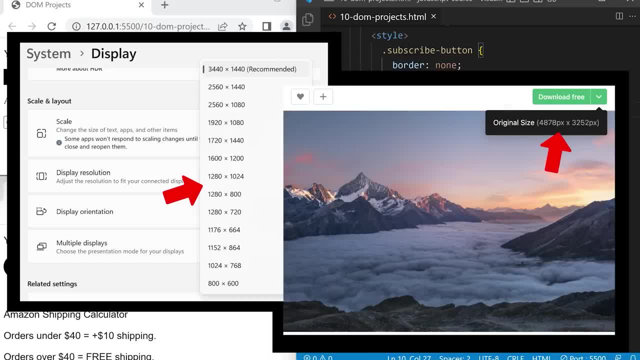 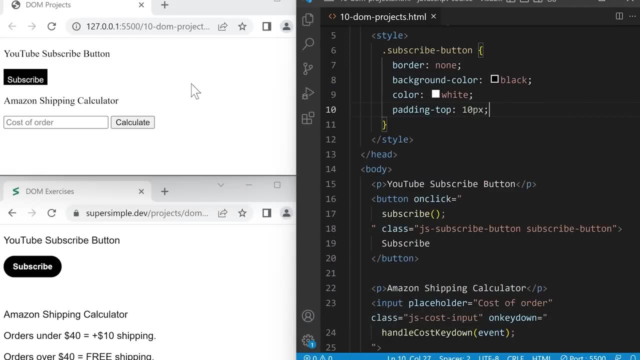 Screen sizes are measured in pixels. Images and video sizes are also measured in pixels. The more you work with pixels, the more you'll get used to how big a pixel is. So in this example, 10 pixels is equal to this amount of space. 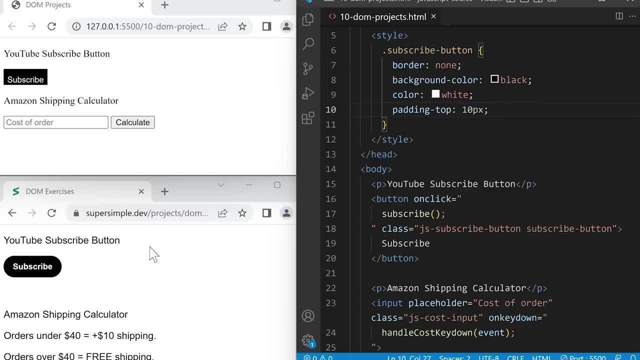 And it looks pretty close to the final design, So let's keep going. We'll add space on the inside of the element at the bottom this time, So we'll create a new line and type padding-bottom. We'll add space on the inside of the element at the bottom this time. 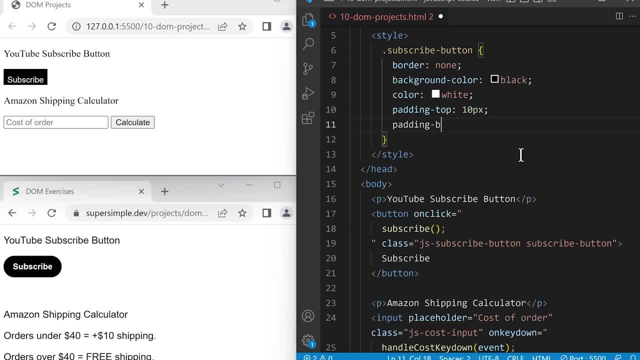 So we'll create a new line and type padding-bottom. Screen sizes are measured in pixels. Screen sizes are measured in pixels. Screen sizes are measured in pixels. colon 10px again and save and that adds space at the bottom of the element of 10. 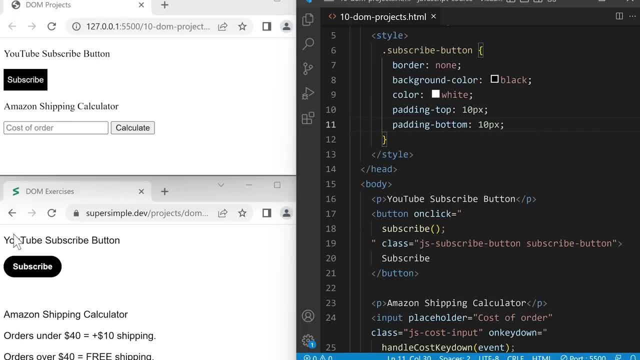 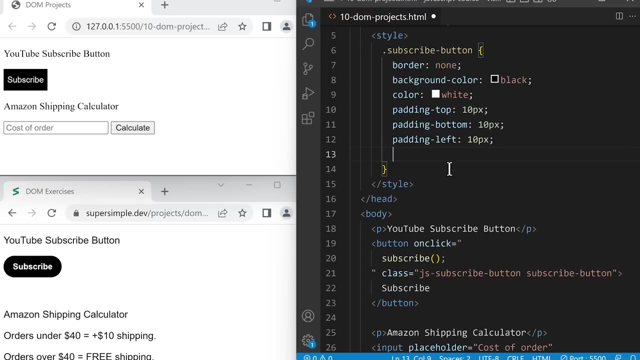 pixels. next, let's increase the space on the left and the right. we'll go into our code and add padding dash left colon- 10 pixels and padding dash right colon- 10 pixels. let's save and it added some extra space on the left and right, but I 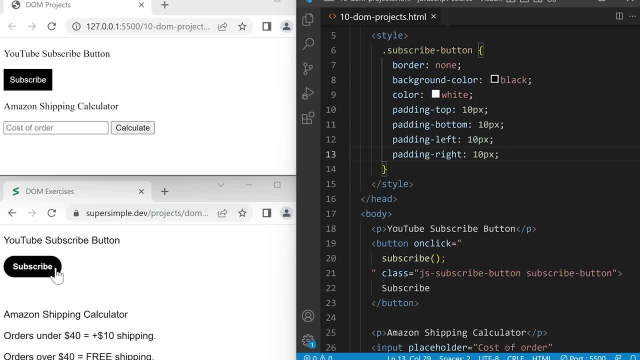 think our final design has a little more space on the left and right, so let's go back and increase our padding. so instead of 10 let's try 15 on both sides, so we'll save. and now the spacing looks close enough to the final design. so in CSS it's normal to do some trial and error to get the styling right. 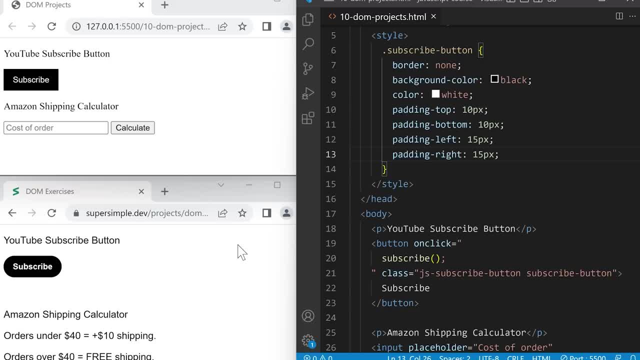 let's keep styling this one by one. next, we'll make the text thicker. you can see that the text is thicker and the spacing is a little bit more or bold. so let's go into our code and to change the thickness of the text we'll use the property font, dash, weight, colon, bold. let's save and that will make our 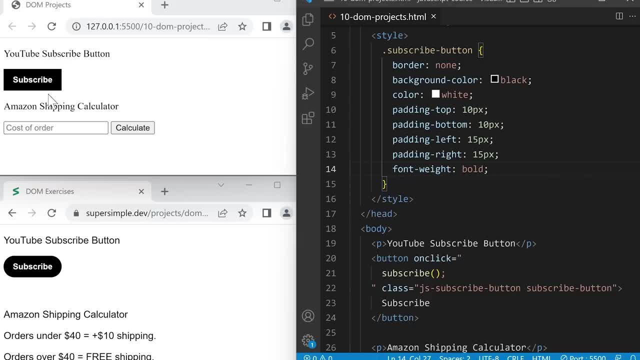 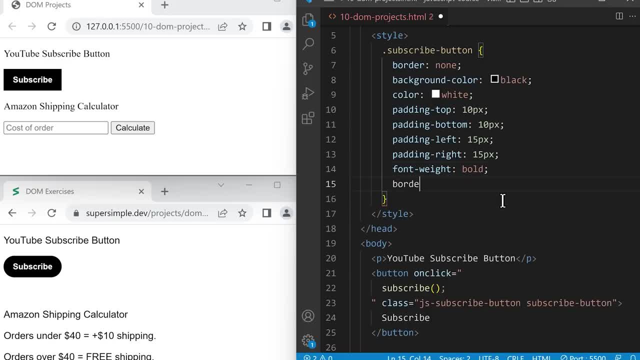 the property for making the corners round is called border dash radius and we'll make it colon 5 pixels. let's save and you can see that it made our corners around. so the pixels here tells the computer how round we want the corners to be. the higher the pixels, the more round it will get. 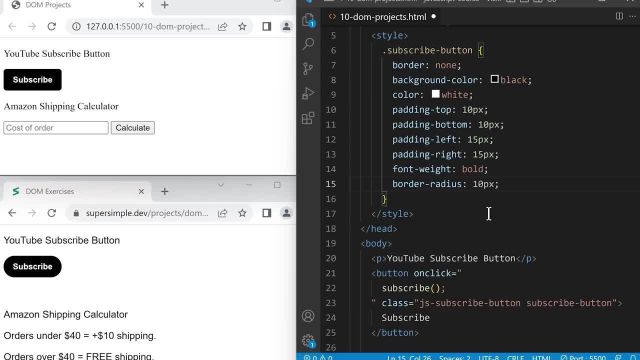 so if we change this to 10 pixels and save, it will make the corners even more round. so let's change this to something really big to make it completely round. we'll change this to 50 pixels and save, and now our button is completely round. the last style we're gonna add is in the final design. if we put our mouse on the 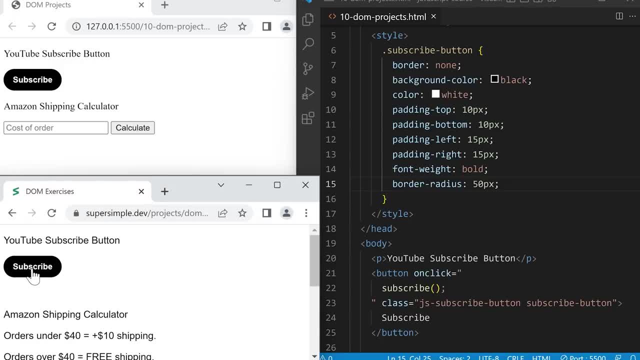 the final design. if we put our mouse on the the button, it turns into this hand icon. so we call this a pointer and we're going to do the same thing in our project. so let's go to our code and to create that pointer icon we're going to use the property cursor colon pointer. 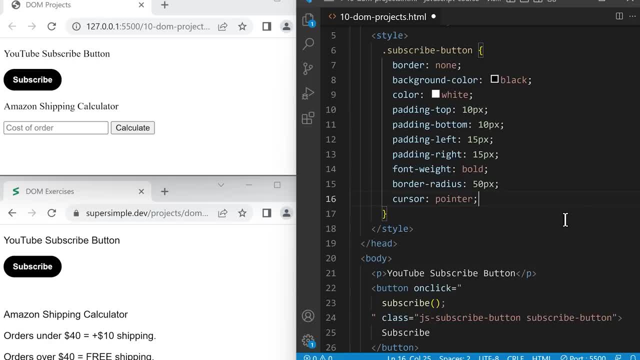 and let's save and put our mouse over the button and you'll notice it turns into this hand pointer icon. and that's it now. our subscribe button looks like the final design. next let's click the subscribe button. you'll notice that it only changes the text. but if we click the final design, it also changes the. 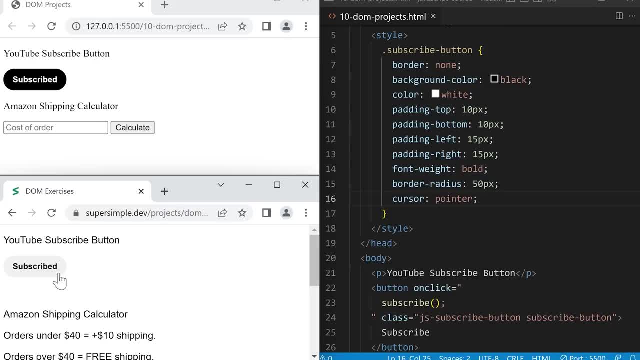 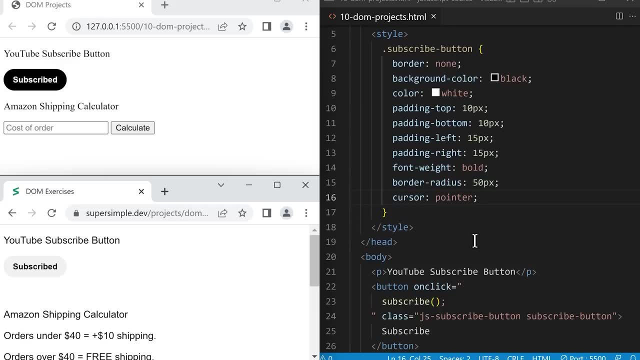 background color and the color of the text. so we can see that the text is and the text color. so we're going to learn how to change the CSS when we click a button. let's go back to our code and this time we're going to scroll down. 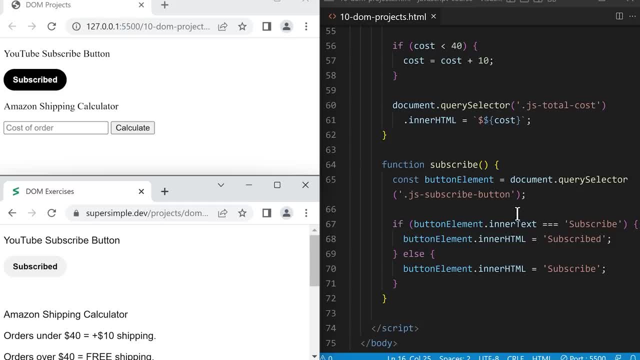 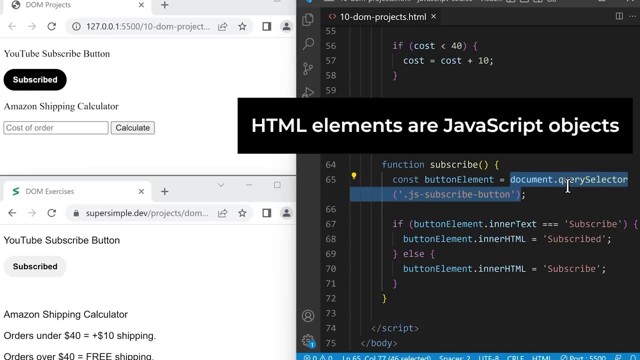 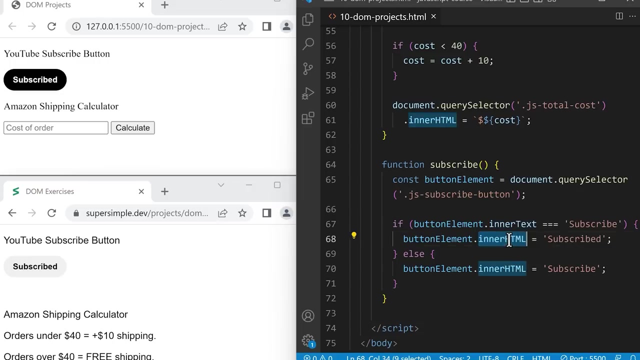 to our JavaScript, which is here. so we learned in the previous lesson: we can get HTML elements from the page and put them inside our JavaScript, and we also learned that these HTML elements are just JavaScript elements, so we can get CSS to add them in our code and the user can also get CSS and CSS also have. 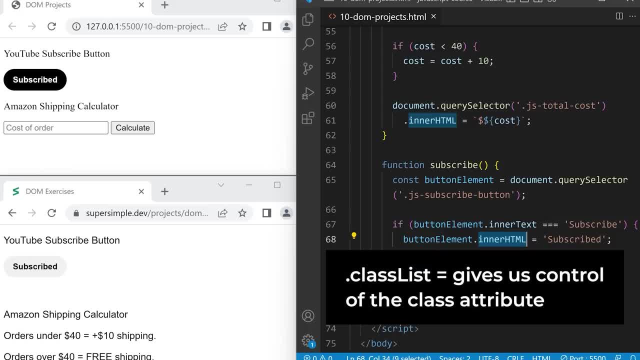 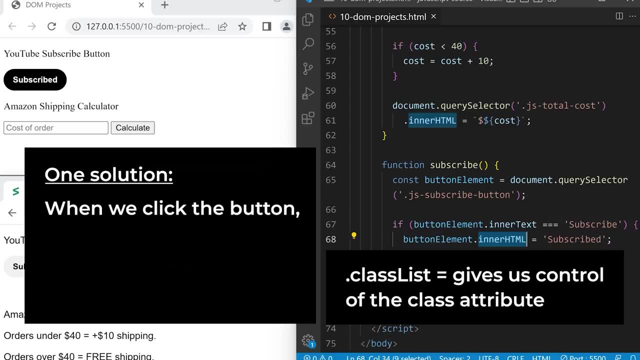 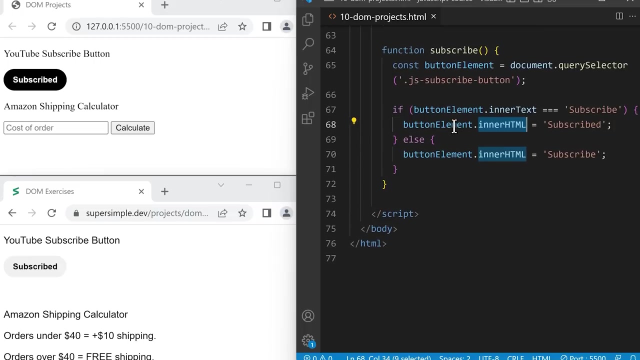 objects and they can have properties like inner text and inner HTML. every element has another property we can use, called class list. class list gives us. So let's see how we do that in our code. We'll scroll down to the subscribe function And when we click the button and make the button subscribed, 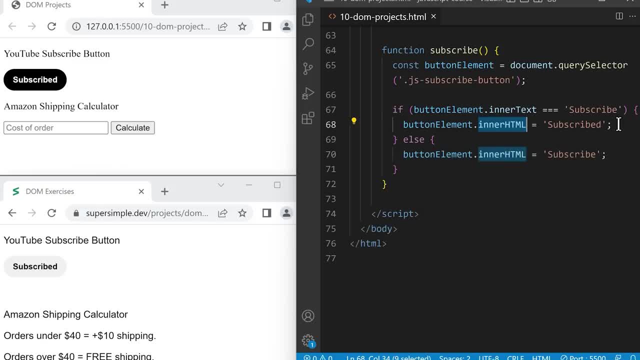 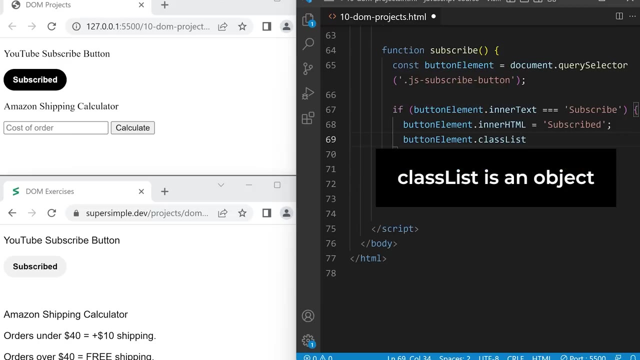 we're also gonna add a class, So let's create a new line and we'll type buttonElementclassList. So classList itself is an object, which means it has properties and methods we can use. One method is called add, which adds a class to an element. 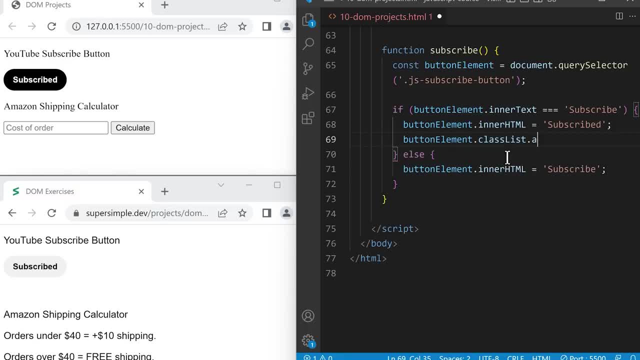 So after this, let's type add. And now inside these brackets we're gonna put a string. So this string is a class that we want to add. when we click this button, Let's add a class called is-subscribed and save. 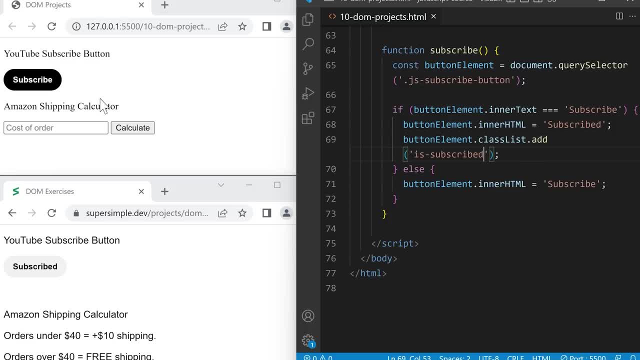 So now, every time we click this button, it will add a class to the button called is-subscribed. Let's give it a try. First we'll right click on the page and then click Inspect, And we'll go to the Elements tab. 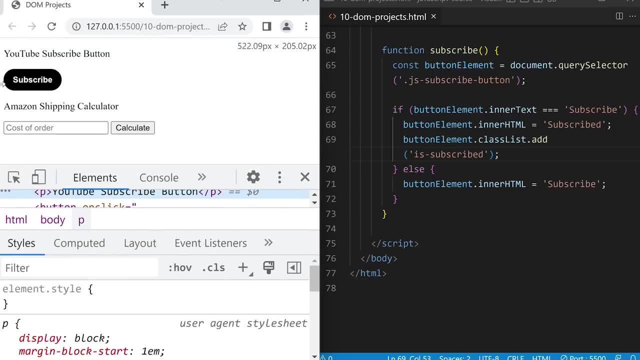 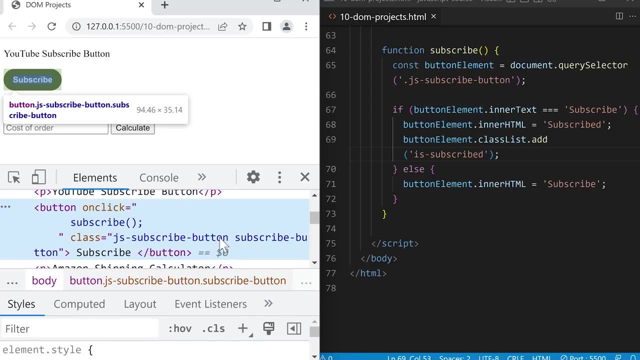 And I'll rearrange my windows so you can see it. And then, inside the HTML, pay attention to the class of the button. Now, when we click the button, it's gonna add an extra class called is-subscribed. So that's what this line of code does. 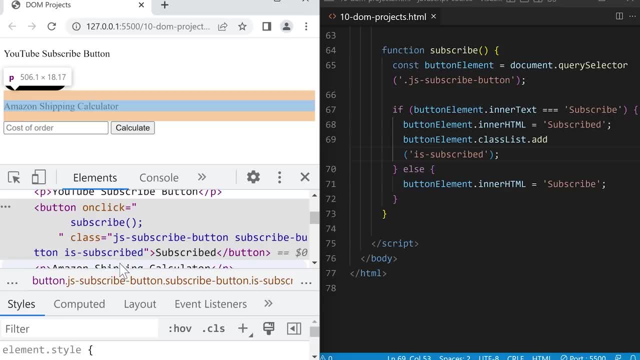 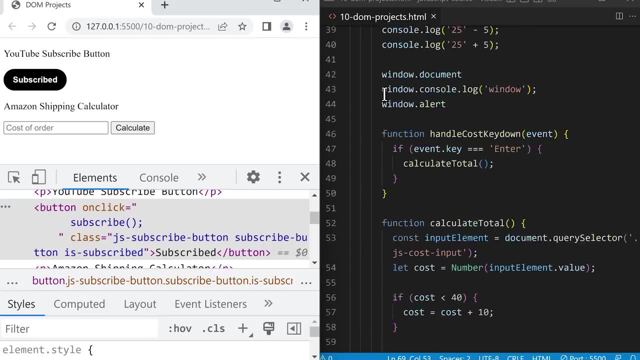 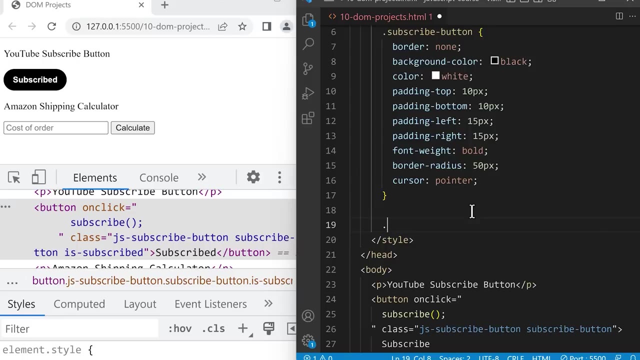 And now that this button has the is-subscribed class, we can style it in our CSS. So let's go back to our code and we'll scroll up to our CSS And here we'll type: to style a class And we'll style the class is-subscribed. 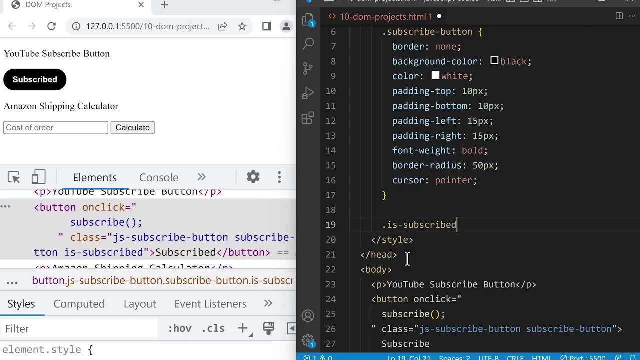 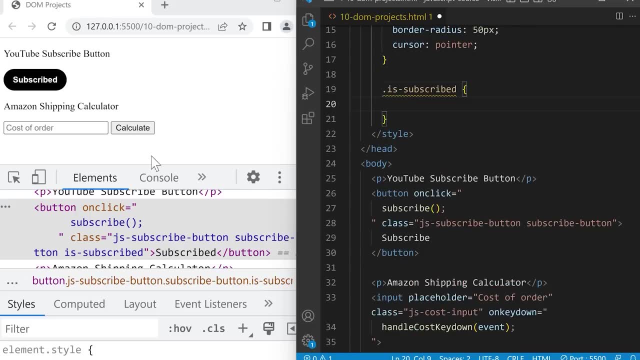 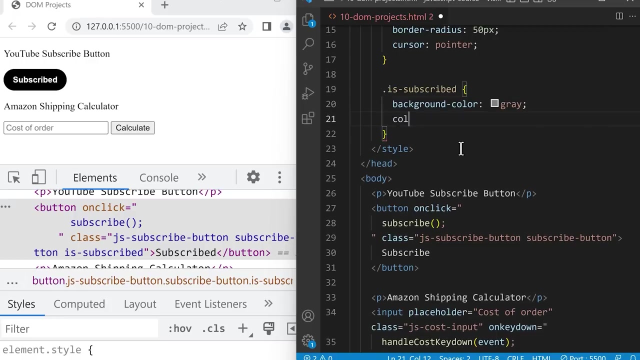 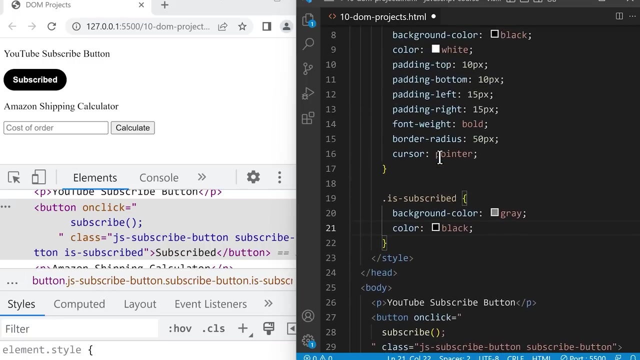 is-subscribed and curly brackets. And now, inside these curly brackets, let's change the background color to gray and the text color to black. Background-color: gray And then color colon: black, And make sure to type these styles below the subscribe button: styles. 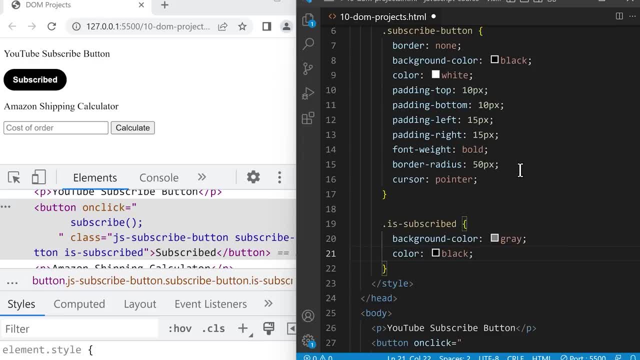 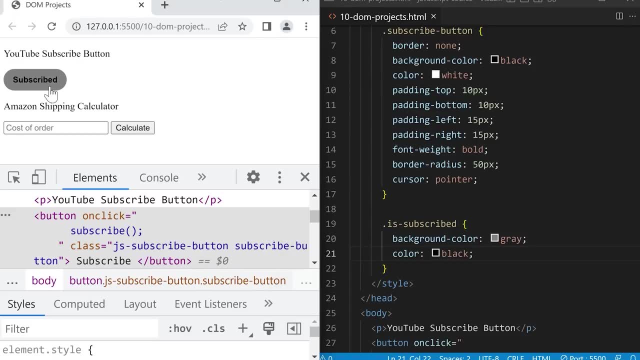 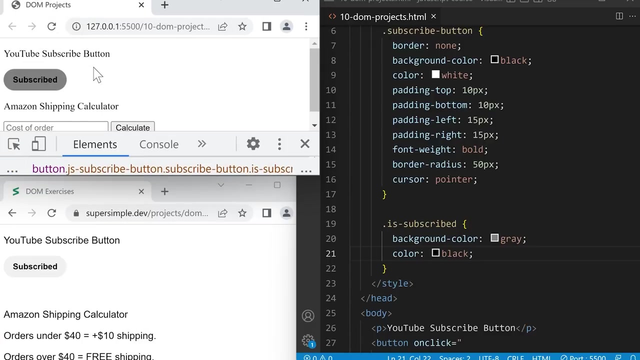 so that these styles will override the styles above. save and then click our button. it will add the is subscribed class and now this button will get our new styles that we added here. so that's one way to change the css when we click a button. all right, now i'm gonna move this back to the top and notice that our background color 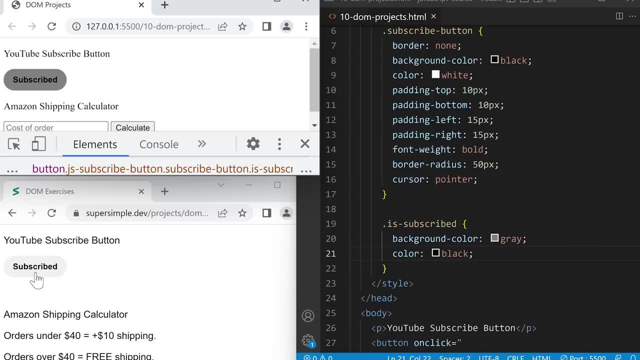 is different from the final design. the final design uses a much lighter gray, so how do we get this exact color? to do that, we're going to open the elements tab again. so on this page we're going to right click, click, inspect and then click the elements tab and i'll rearrange my windows so we can see it. 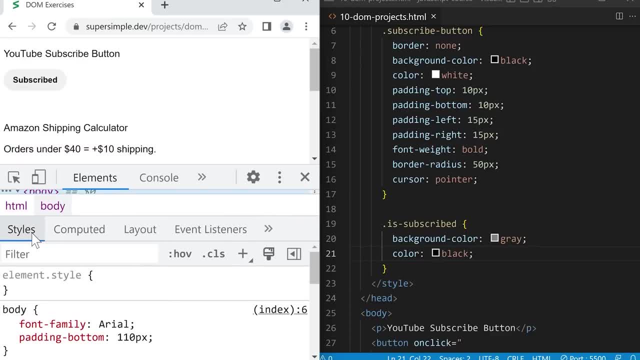 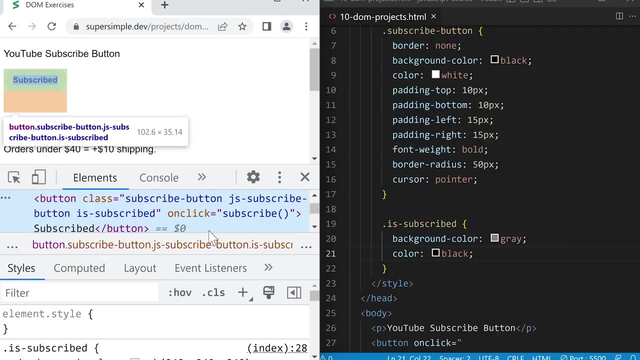 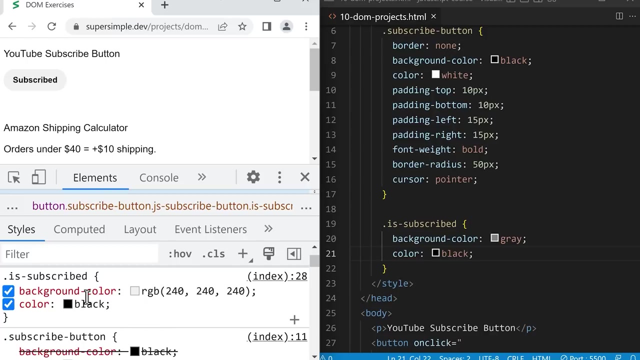 here. so in this section, in the style section, we can see the css that the element has. so first let's actually find this button, which is right here, and we'll click it, and here it will show us the css that this button has and it will show us the background color. 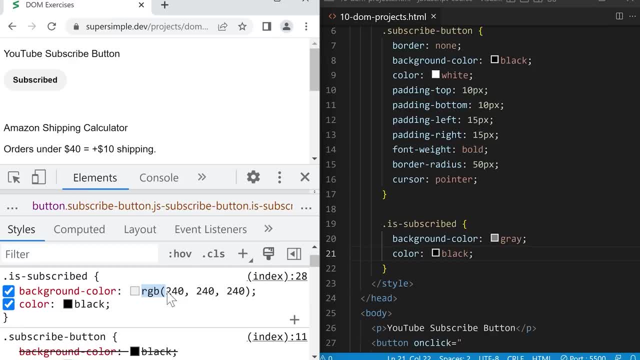 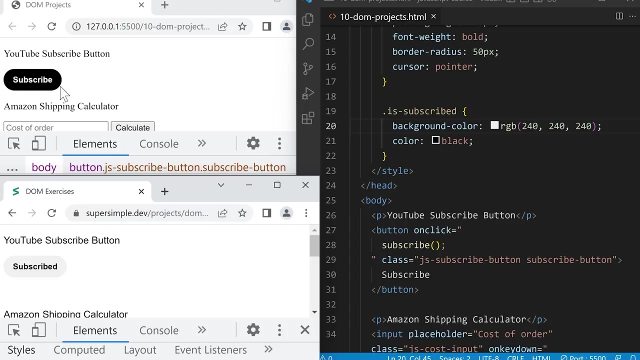 that we should use. so let's make a copy of this color and we'll put it into our code. right click, copy and here we'll remove it and right click and paste. now let's save and go back to our project and try it out, and now we get the exact same color. 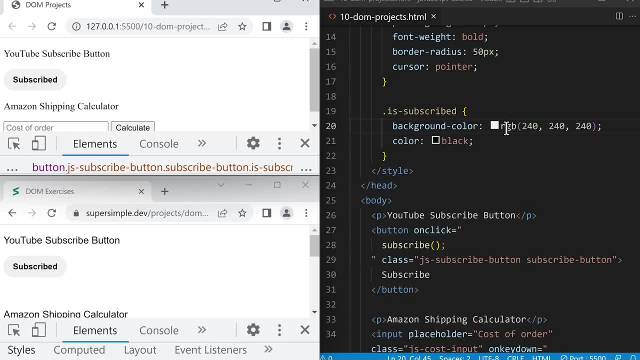 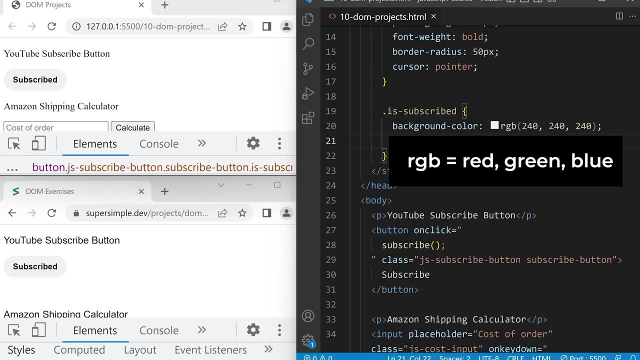 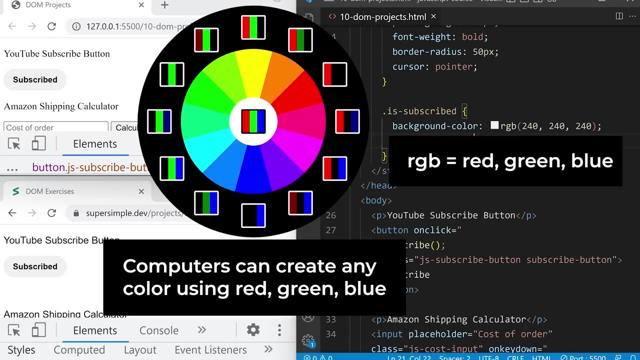 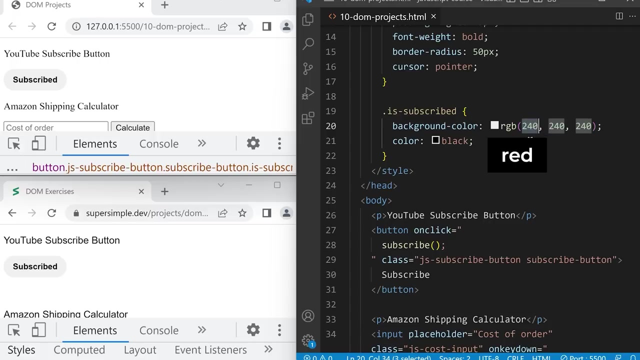 as the final design. so, by the way, this color is known as an rgb value. rgb means red, green and blue, and computers can create any color using a combination of red, green and blue. so the first number here is how much red we want in our color. the second number is how much green we want and the third number is how much. 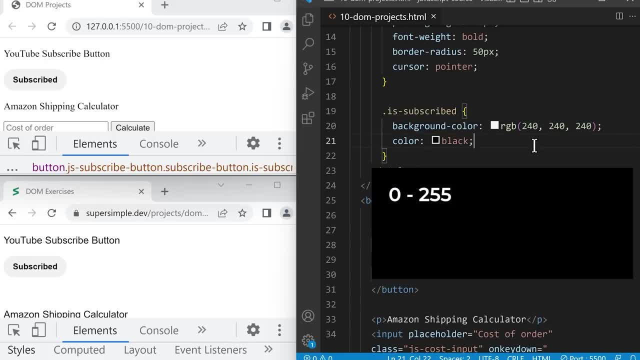 blue, we want from 0 to 255. 0 means less color and darker, 255 means more color and lighter. so this color here uses 240 for all of the colors, so it's close to 255 and will give us a very light gray color. 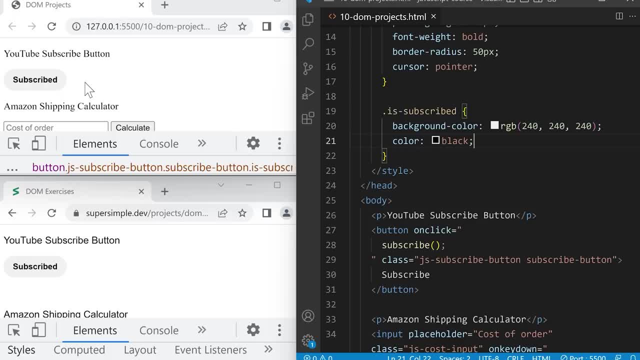 that you see here. next, if we go back to the final design and we click our button again, it will change back to the original style. so we're going to create this feature in our project as well. so one way to do this is when we click the button again. we can remove this class. so let's scroll down to the bottom. 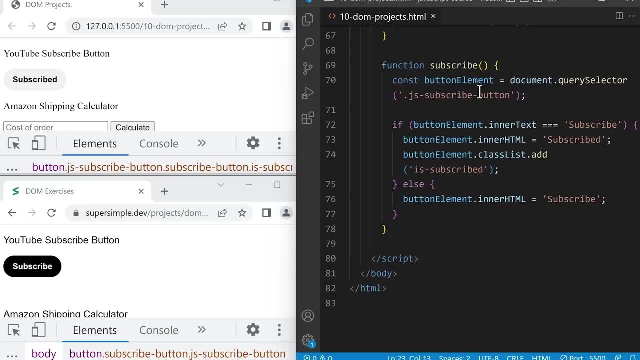 to the subscribe function and when we click the button and we change it back to subscribe, we can remove this class. to do that, class list has another method we can use, called remove. so let's create a new line and we'll type button element dot class capital l list. 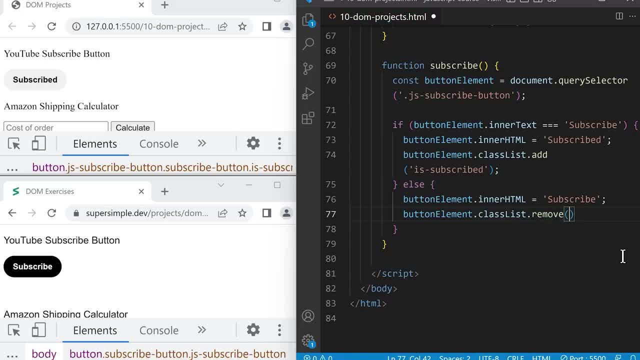 dot remove and brackets. so this does the opposite of dot add: it will remove a class from this element. so inside the brackets we'll type a string and the class we want to remove, which is, is dash sub scribed and save. now let's try out our project. 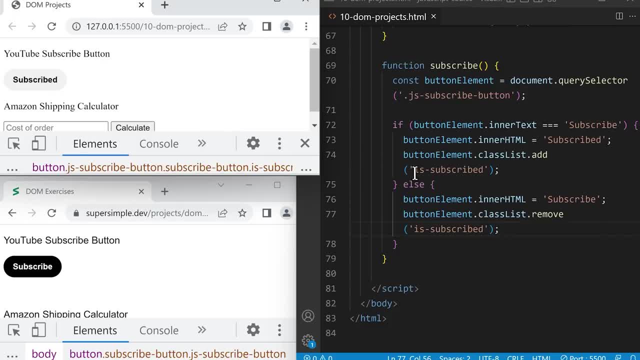 click the button, it will get the class is subscribed and get the extra styles. and now when we click the button again, it will remove the class and it will remove the extra styles. so notice here that when we add a class we just type the class name, we don't type a dot. 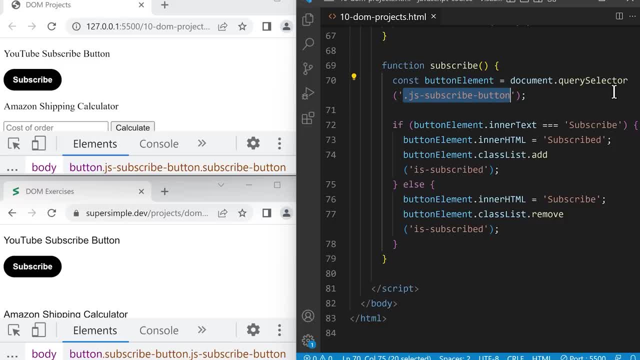 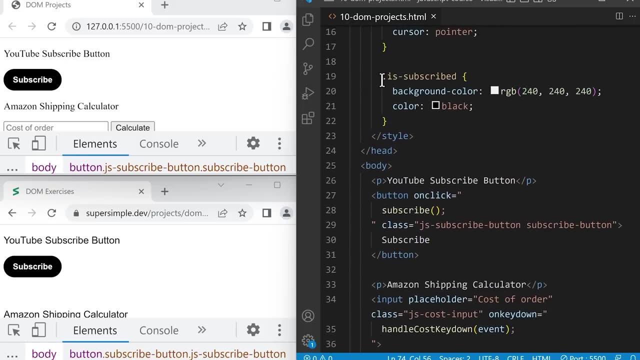 and the class name, like we did for query selector. typing a dot only makes sense in query selector. next, we're going to style the text on the page. let's scroll up to our css and one thing we can do is to style all the paragraph elements on the page using this code: p and curly brackets. however, we're going to use a better solution. 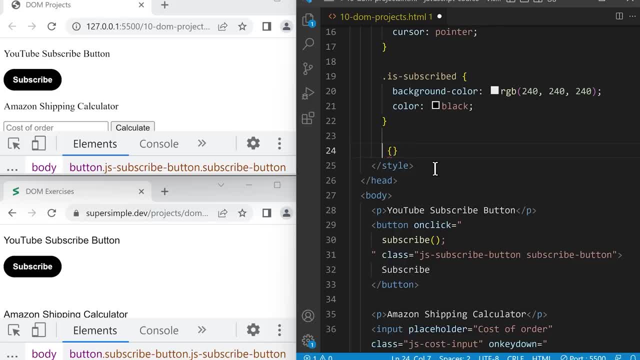 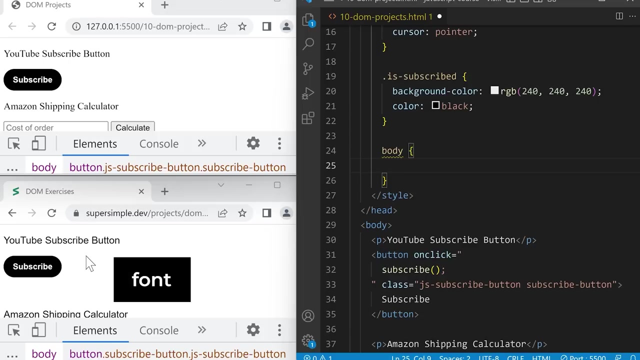 instead of styling all the paragraphs, just going to style the body element. When we change the text in the body element, it will change the text in the entire page. So inside these curly brackets, let's change the text here. So we're going to use a different style of text. This is called a font. To change the font. 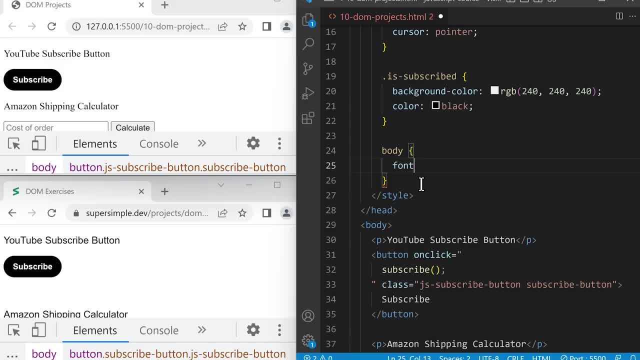 we're going to use this property Font dash, family colon and we'll change it to Arial, which is what I used in the final design. So let's save and this will style all the text inside the body and change the font to Arial, And a good practice is to write any styles for the 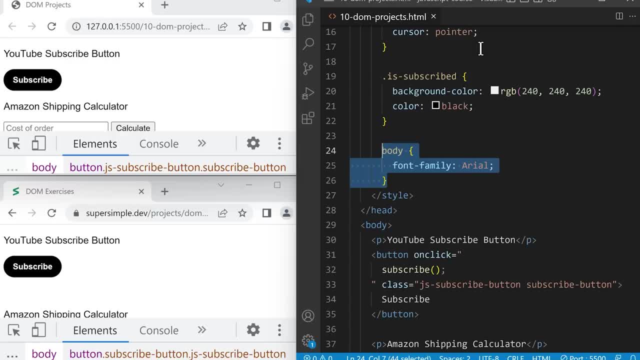 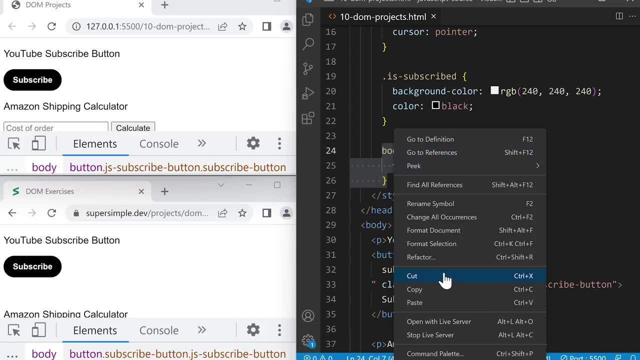 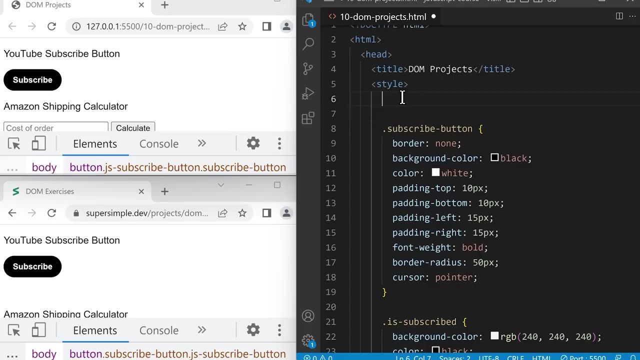 body and change the font to Arial, And a good practice is to write any styles for the body at the top, So if we need to, we can override it later. So let's move these to the top. We'll right-click, cut and then, up here, create some new lines and right-click and paste. 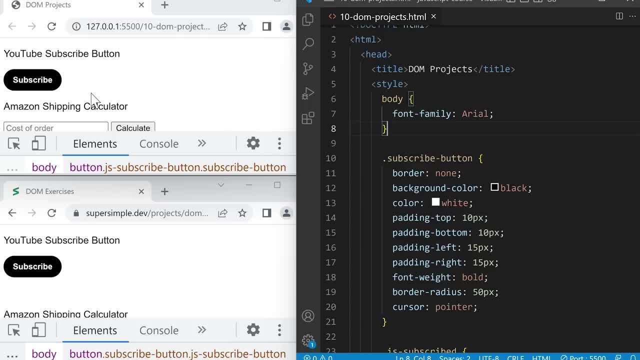 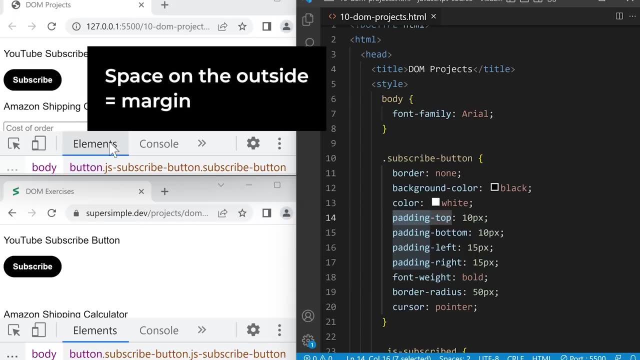 And we're going to add one more style before moving on. Let's add some space between the subscribe button and the second project. So earlier we learned that space on the inside of an element is called padding, Space on the outside of an element is called margin. So inside our subscribe button, 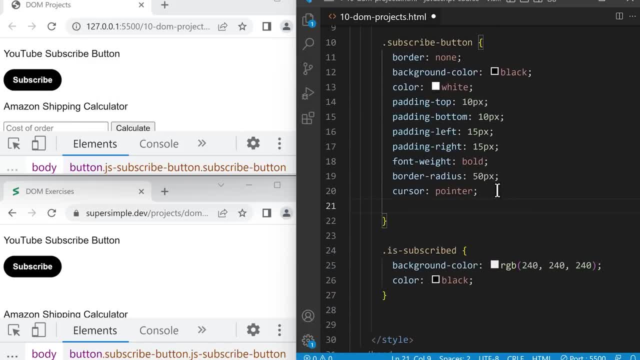 at the bottom, let's add a property called margin dash bottom colon 30 pixels, And so if we want to add aี่ grade now, we'll put in a special object to thepolish toolbar, So this will add space on the outside of the element at the bottom of 30 pixels. 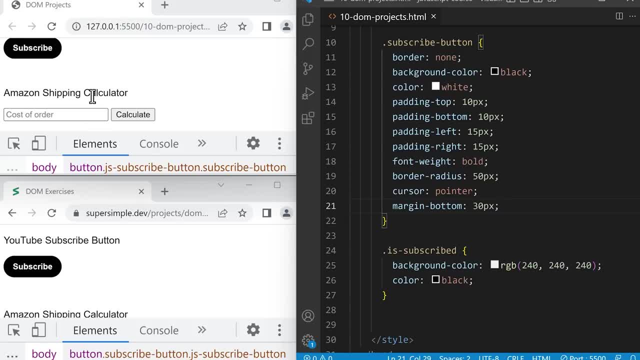 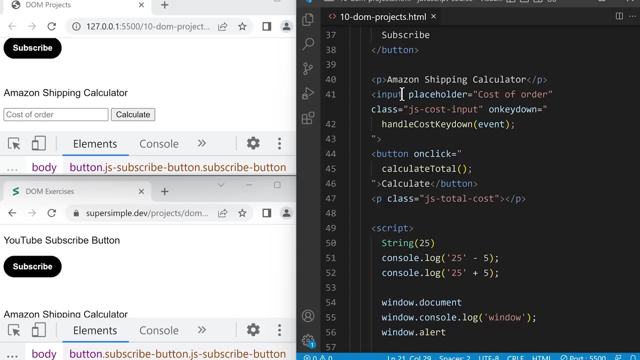 Now let's move on and style the Amazon shipping calculator with CSS. Again, we'll add a class to these elements and then style them in our CSS. Let's scroll down to the text box, which is the input element. Let's type, and we'll click on Way Narrow, and let's we're going to label it3.7.2,. 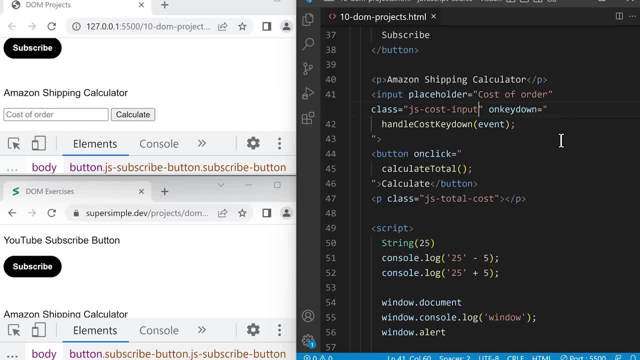 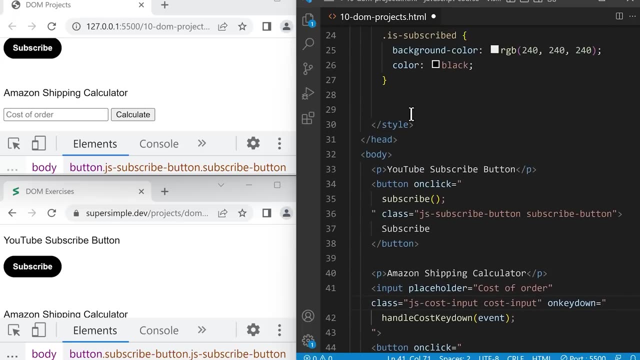 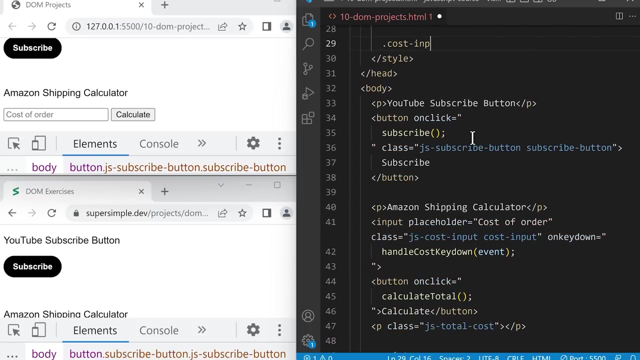 And we're going to add another class by typing space And let's use the class cost-input, And now we're going to style this in CSS. So let's scroll up And here we'll style the class using cost-input and curly brackets. 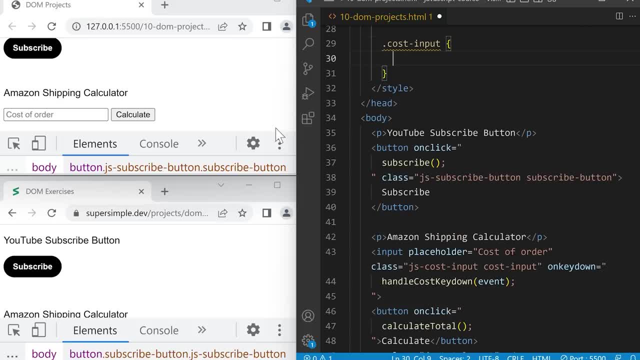 And inside. we'll style this one by one. Let's look at our final design and see what styles we need. So first let's change the text size, Because our text is a little smaller than the text here. So to change the text size we're going to use font-size colon and let's try 15 pixels. 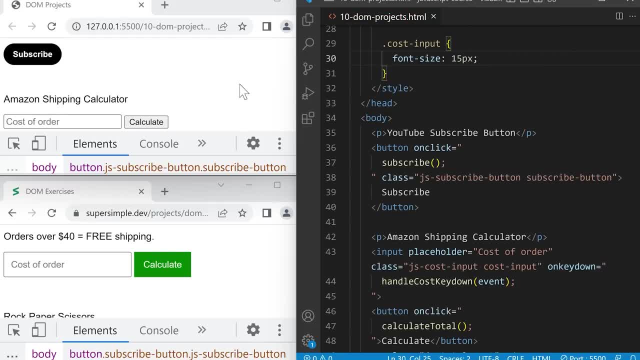 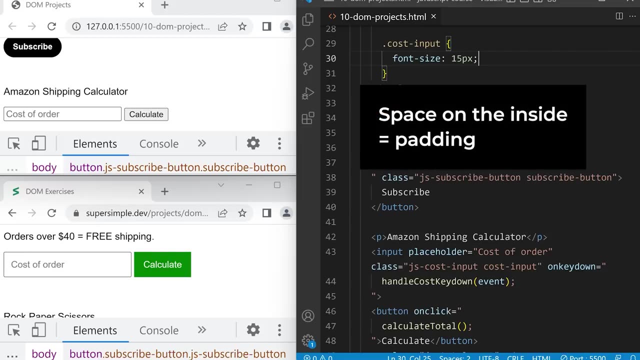 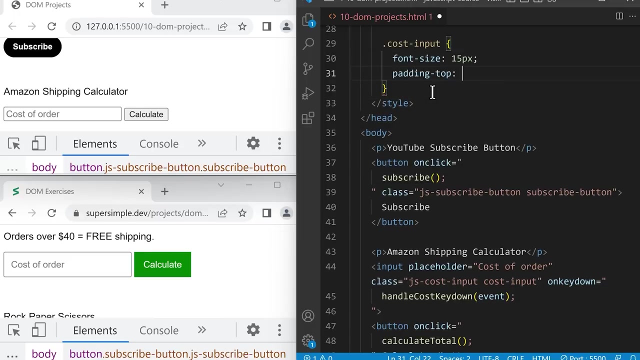 And save. And now our text looks close enough to the final design. Next, let's add some space inside the text box. So remember, space inside an element is called padding, So we're going to type padding-top of 10 pixels. 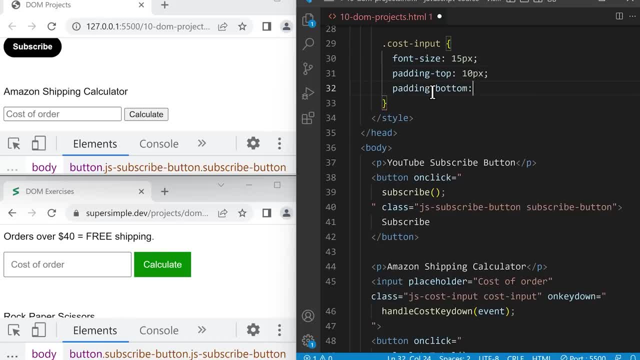 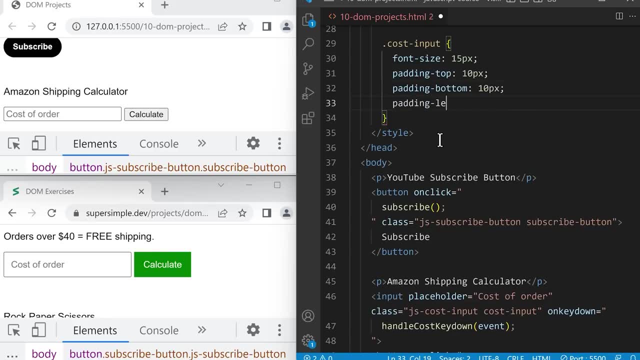 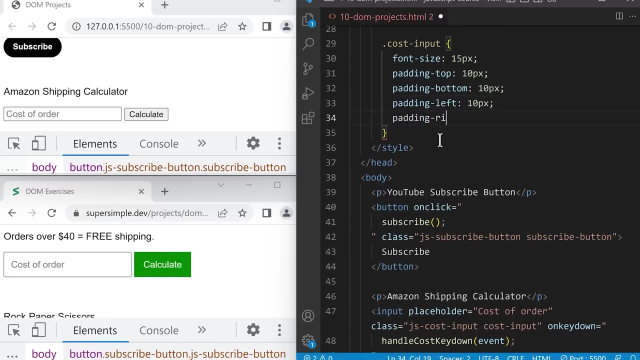 Padding-bottom Also 10 pixels, And let's add padding to the left- 10 pixels- And padding-right of 10 pixels, So this will add space on the inside of our text box in every direction. If we save Now, it looks just like this: 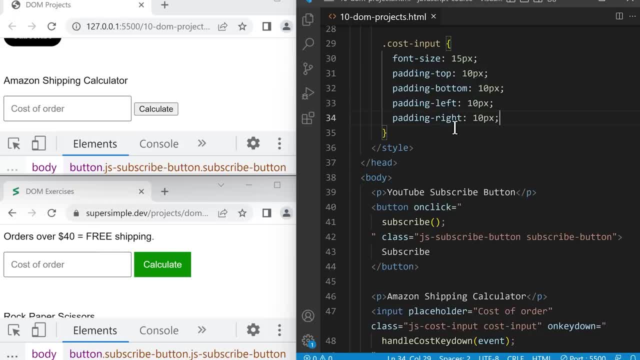 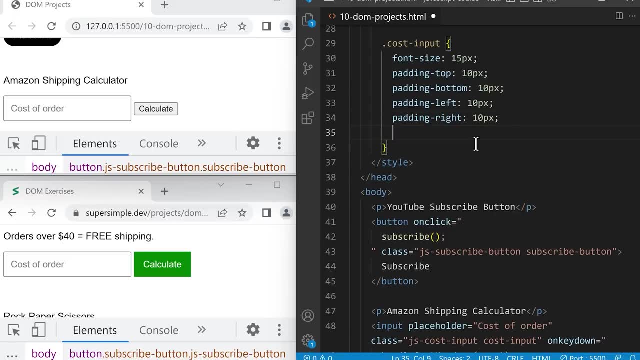 It looks like the final design. Now I'm going to show you a shortcut for padding that will save us some typing. So if we create a new line, we can actually use a property called padding And colon and then type 10 pixels. 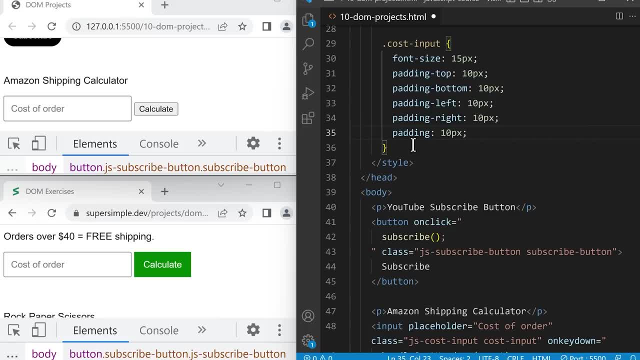 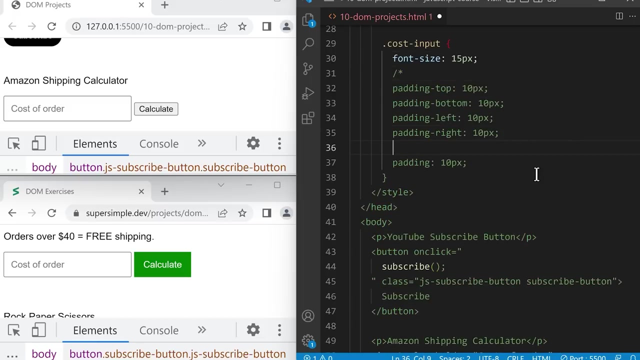 This padding property lets us add padding on multiple sides at once. If we type one value here like 10 pixels, it will add 10 pixels to every side. so this line does the same thing as these four lines above. so let's actually comment this out using slash, star and star slash and save. 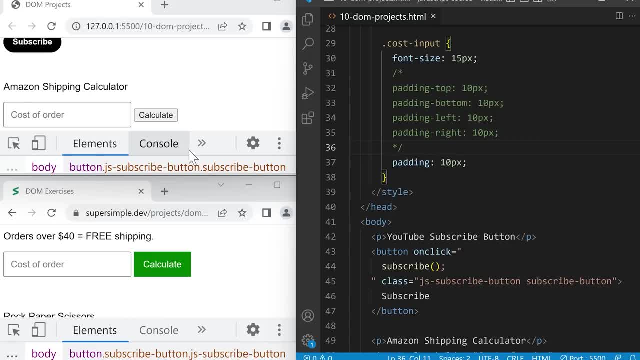 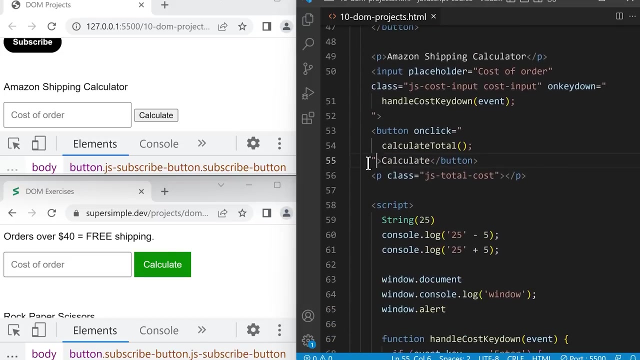 and you can see that this one line of CSS did the same thing as the other four lines of CSS, so this shortcut can save us some typing. next, let's move on and style the calculate button again. we'll add a class to this button so we can style it. so in this button, let's add a class. 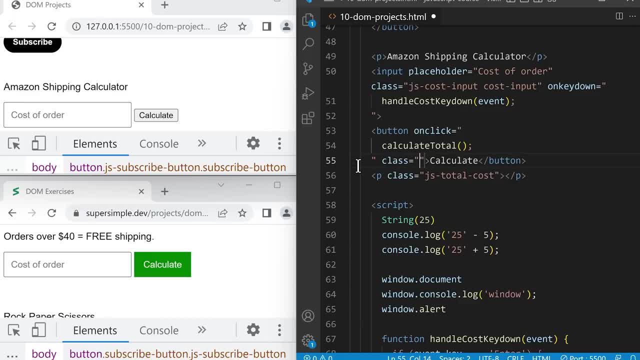 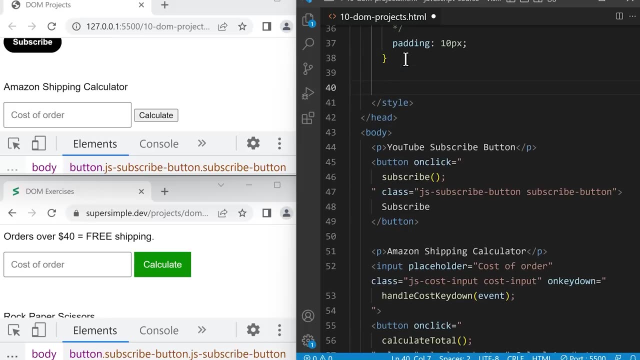 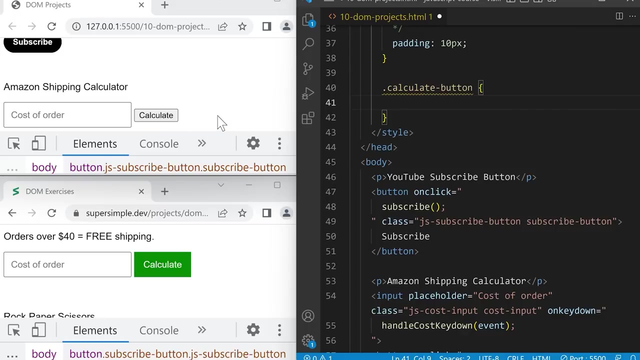 attribute class equals calculate dash button. now let's style this in our CSS by scrolling up, and here we'll type dot- calculate dash button and curly brackets, and inside these curly brackets we're going to style this button one by one. so let's start with the background color. so we'll type background: dash color, colon. 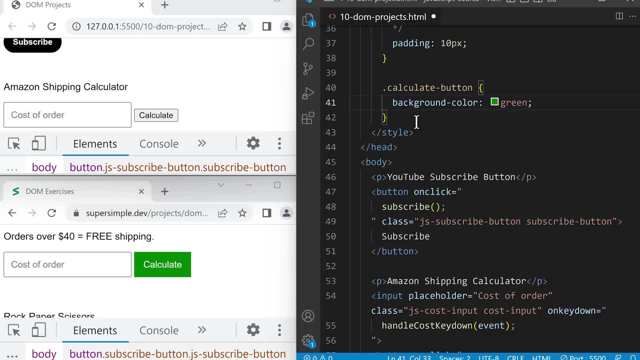 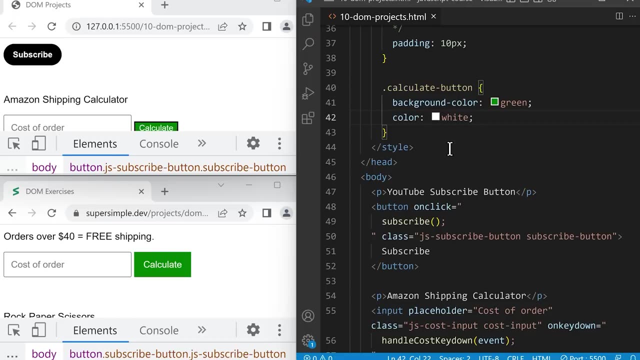 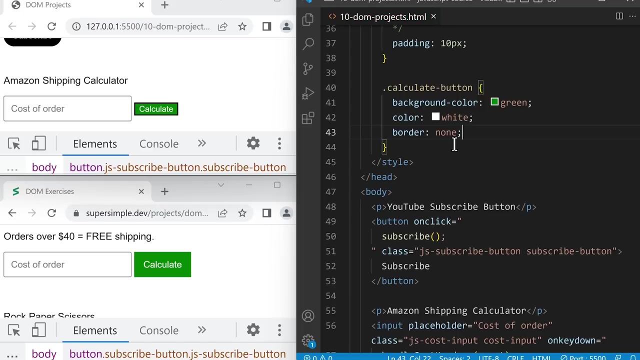 green and semicolon and save. next let's change the text color to white, so we'll type color colon white and save again. okay, let's keep going and we'll remove the border around this button, so we'll type border colon none, save. next let's make our text a little bigger, like in the final design. 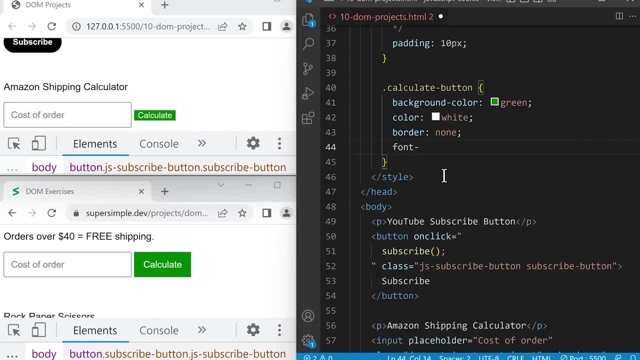 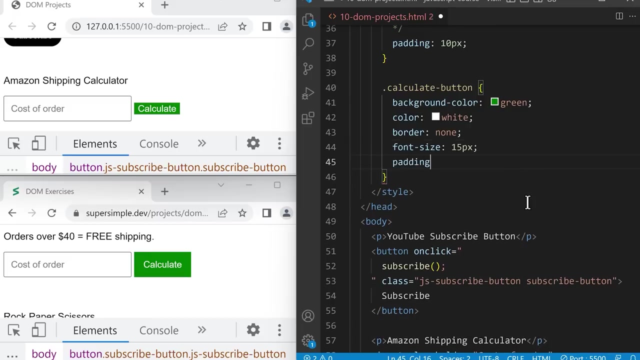 so we'll type font dash size and make it 15 pixels and save okay. so now let's add the space on the inside of the button. so we're going to use this shortcut again. we'll type the padding property colon, and this time we're going to give it two values separated. 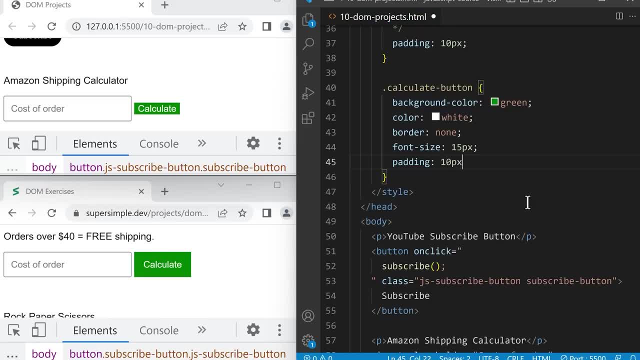 by spaces, 10 pixels and maybe 50 pixels, so it's easier to see what this does. so when we give two values to padding, the first value is the vertical padding, so the top and bottom. the second value is the horizontal padding, or left and right, if we save. 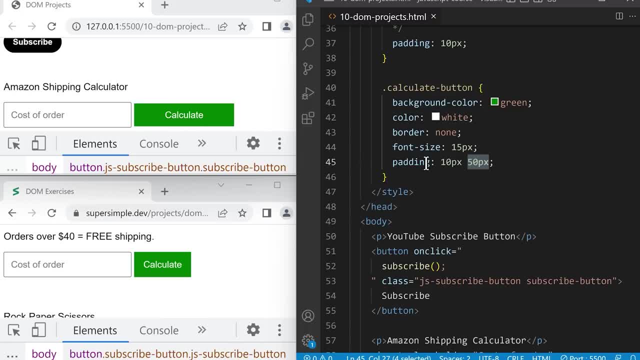 so you can see that the left and right has a lot of padding, which is 50 pixels. so now let's make this match our final design. so instead of 50 pixels, let's bring it down to 15 pixels and save. okay, so that looks pretty close. 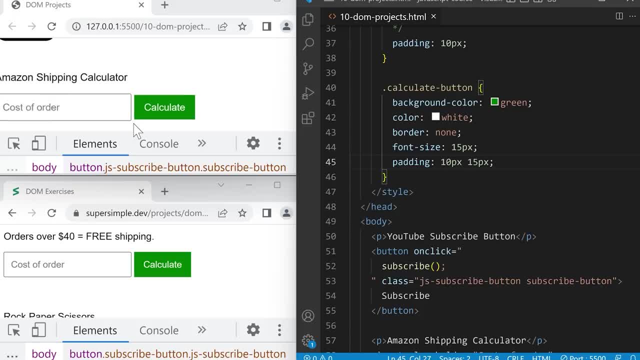 let's also increase the padding on the top and bottom so that the text box and the button line up with each other, like in the final project. so let's change the vertical padding to maybe 12 pixels and save. the last thing we'll style for this project is when we put our mouse over the 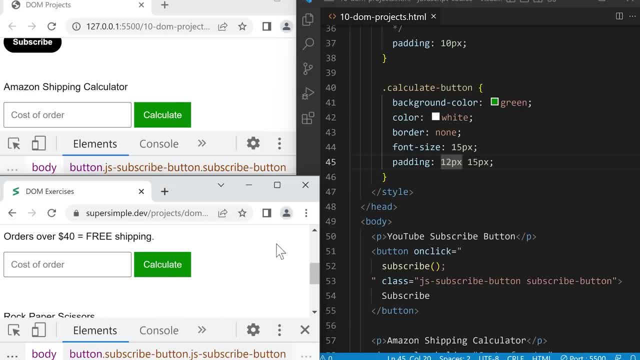 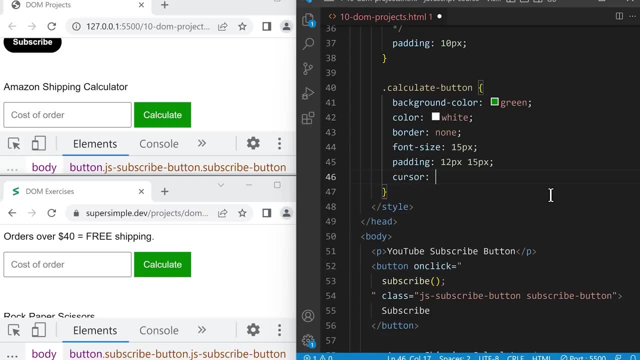 button, it turns into the pointer icon. so to create this we're going to use the property cursor colon pointer and save and give it a try. and that's it. we just finished styling the Amazon shipping calculator. so now let's give this a try. we'll type 25 in the text box and press calculate and at the bottom it will add ten dollars of. 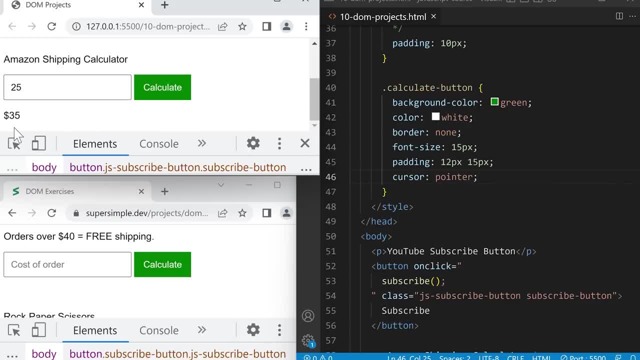 money and show 35 dollars. finally, we're going to style the last project in this lesson, which is the rock paper scissors project, and this will finish the project. let's go back to supersimpledev and we'll scroll down on this page and then click this link to show the final design for. 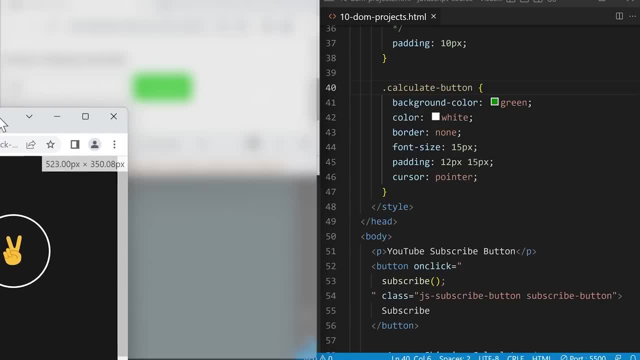 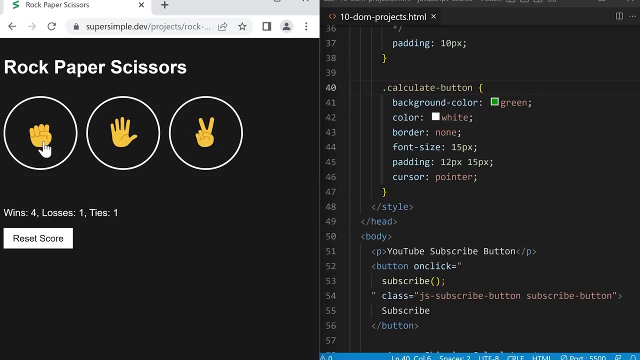 rock paper scissors. so I'll rearrange my windows so we can see this, and we're going to change the buttons to these nice big icons for each of the moves and when we click a move it will show the result in bold and show an icon of the move that we 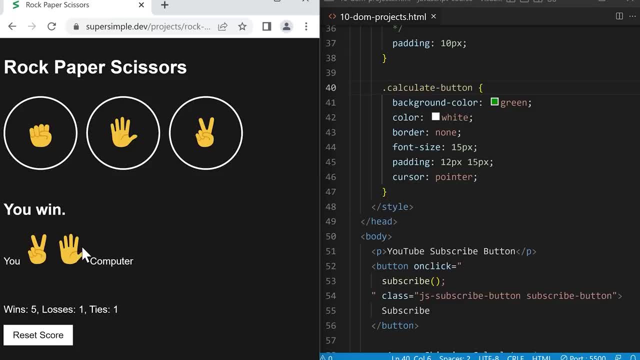 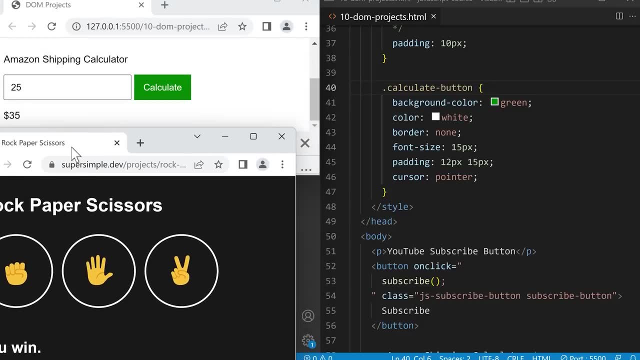 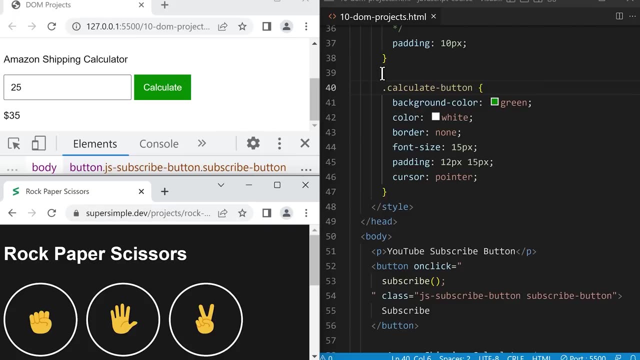 picked and the move that the computer picked. so we're going to make this project look really nice. now let's get started. I'm going to rearrange my windows back, so we have it at the bottom. let's create a copy of the rock paper scissors project for this lesson. 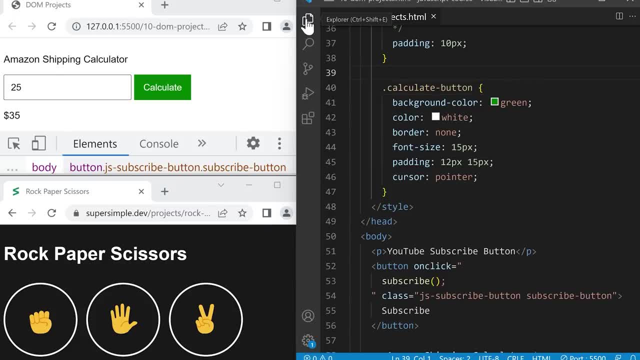 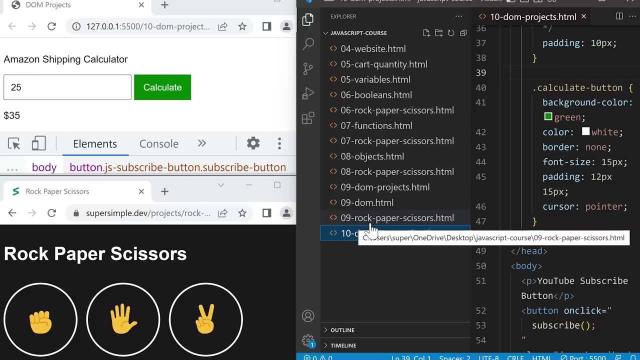 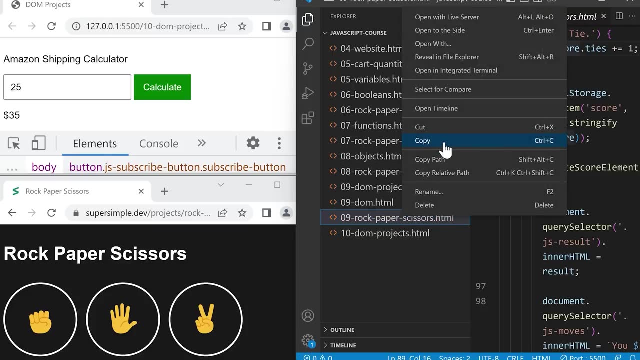 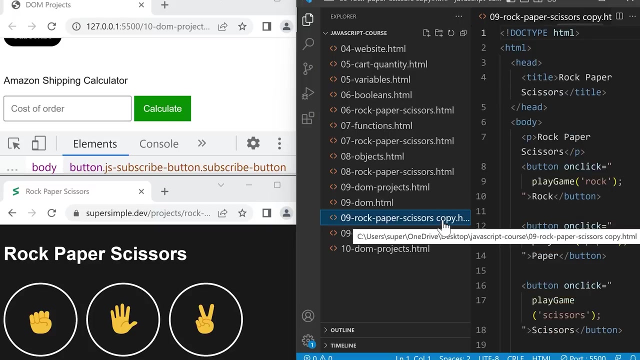 we'll go to our code editor and click here to show our files and we're going to make a copy of 09 dash rock paper scissors. so let's click this file and then right click, copy and down here right click and paste and we'll rename this file by right clicking rename. 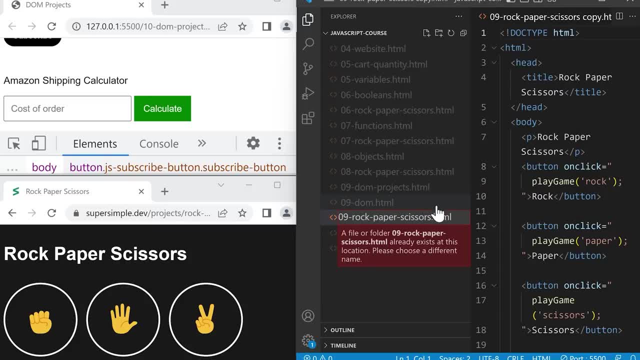 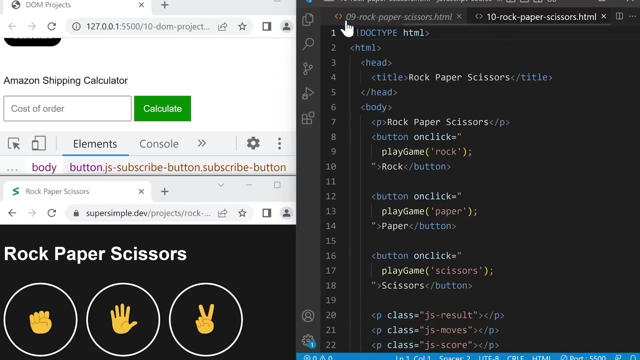 and at the end we'll remove copy and at the beginning we'll change it from 9 to 10 and press enter. now let's click here to hide the files and we can close the 09 file. and let's open the 10 rock paper scissors file in the browser. So we'll right-click and then open with. 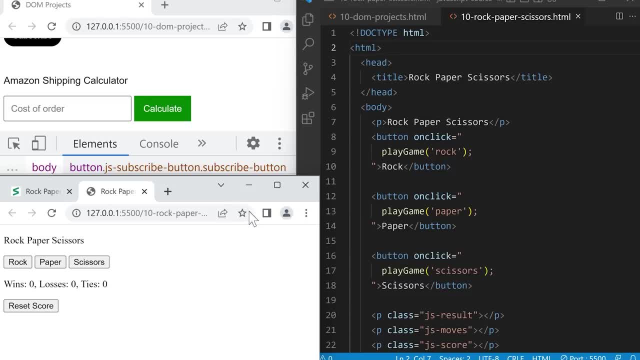 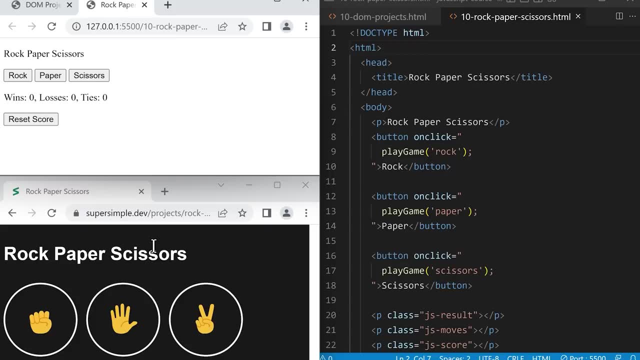 live server And I'll move this tab to the top here so we can see it side by side. So let's start by styling the body. We want to make the background color of the entire page this dark gray color. We'll go into our code and let's create. 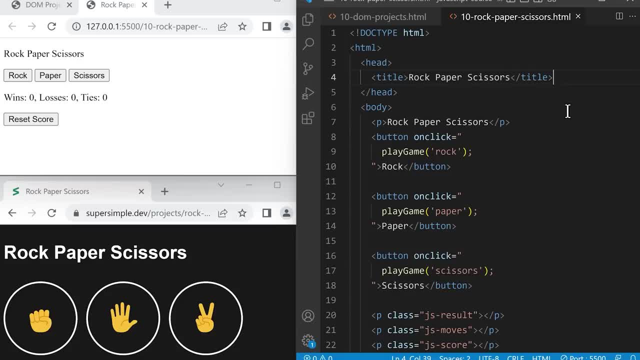 a style element so we can write some CSS. Inside the head let's type less than, style greater than. And then inside here we're going to style the body, so we'll type body and curly brackets. Now, inside here we're going to change the background color, so background dash, color, colon, and we're going to 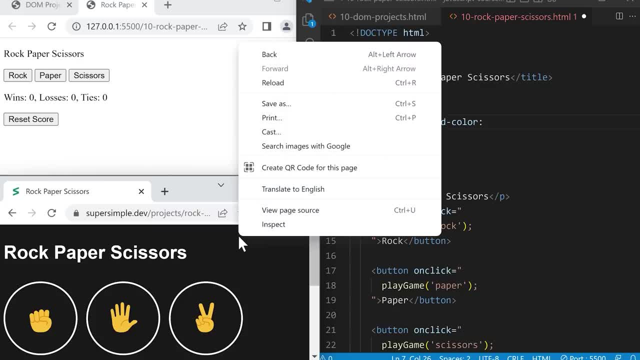 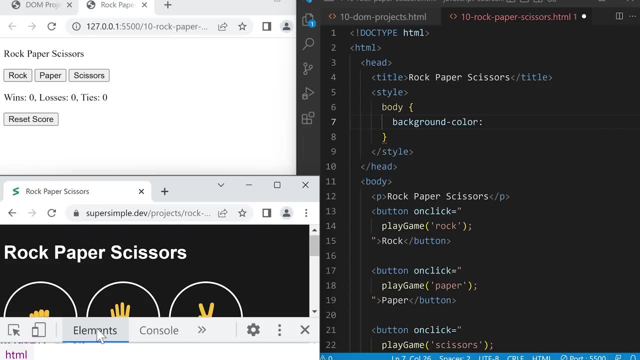 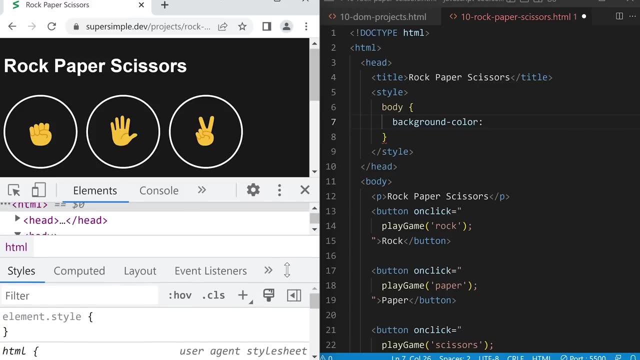 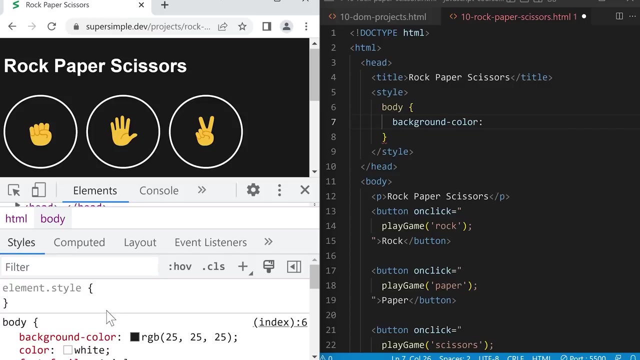 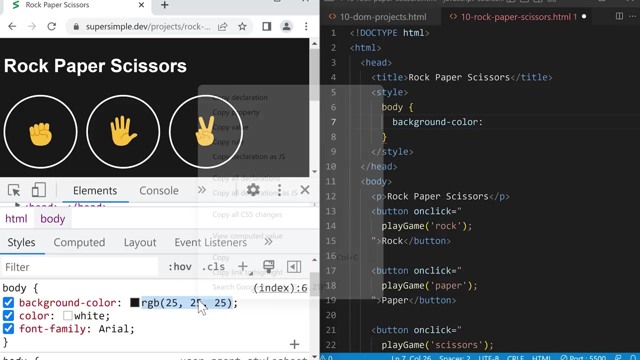 get the color that we see here by right clicking, click inspect, and then go to the elements tab and i'll rearrange it so we can see it. and then here we'll find the body element and click it and in this style section we can find the background color that we need. so let's select this and right click copy. 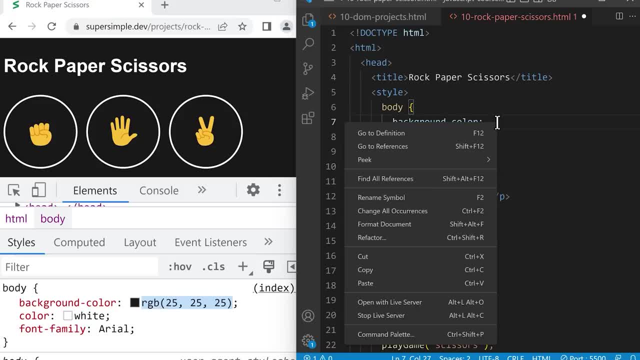 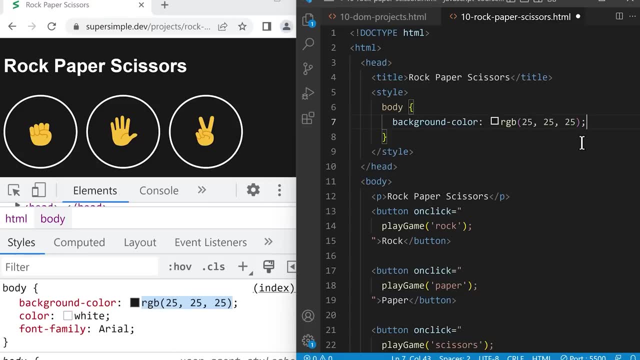 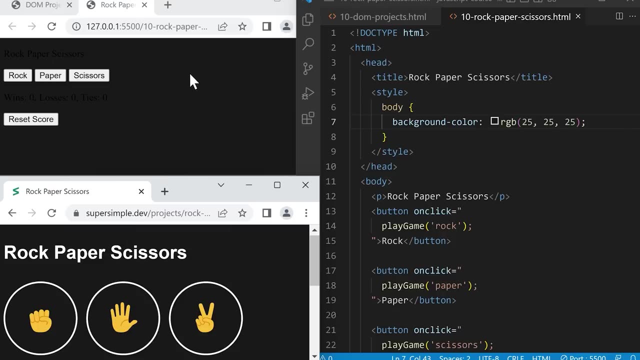 and in here right click and paste and a semicolon at the end. let's save. and i'll move this back to the corner. and now our project has the same background color as the final design. next let's make the text color white. so in our css we'll use the color property and colon white and semicolon and save. 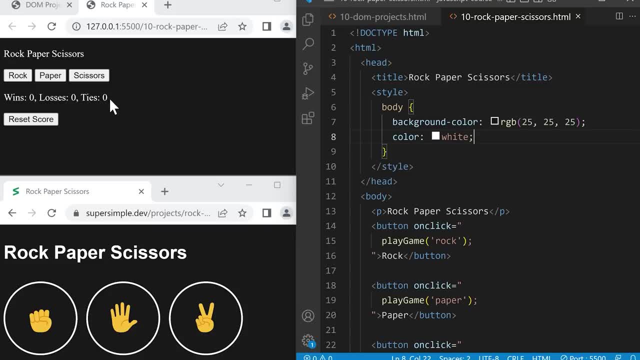 that will make our text white. next, let's change the style or the font of this text. we'll type font dash, family, colon, ariel, which is what the final design uses, and save all right. now let's style these elements one by one to match the final design. we'll start with this. 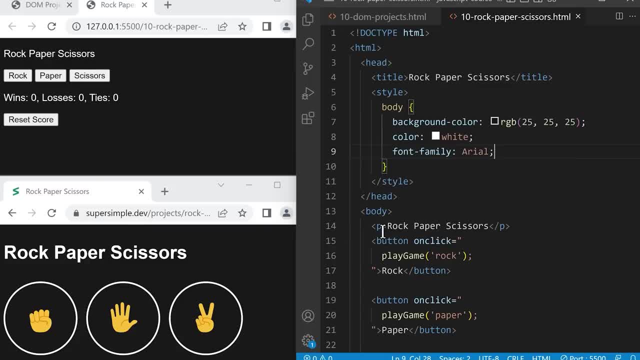 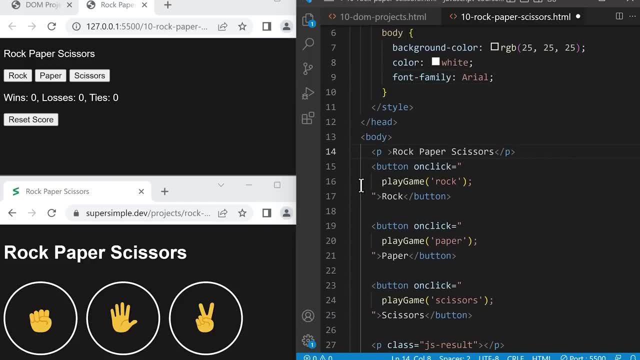 paragraph at the top, so inside the paragraph element let's add a class so we can style it in css we'll add class equals. let's call this the title and then in our css we can style this class by starting with a dot and then title and curly brackets. 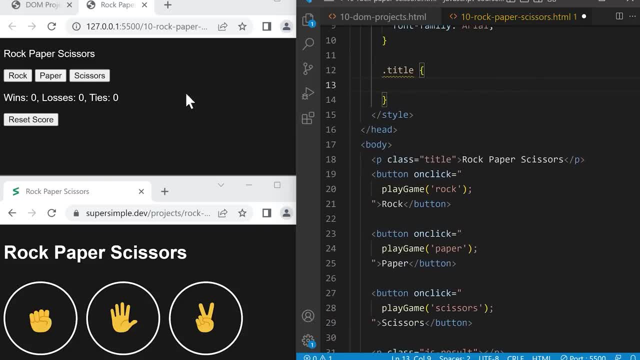 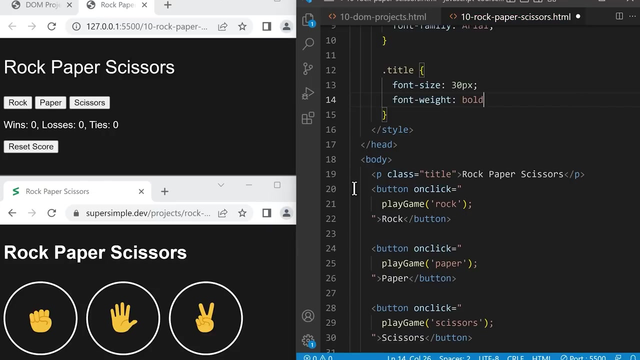 so let's make our title really big, like the final design. we'll change the font dash size, colon- 30 pixels, and save so that looks close enough. next, let's make the text bold in our css. we'll use font dash weight, colon bold and save. now let's move on to styling the buttons. 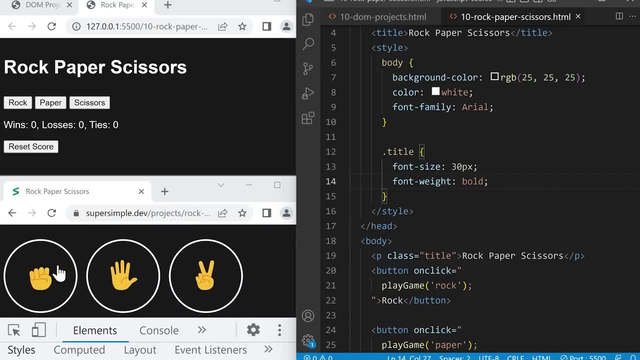 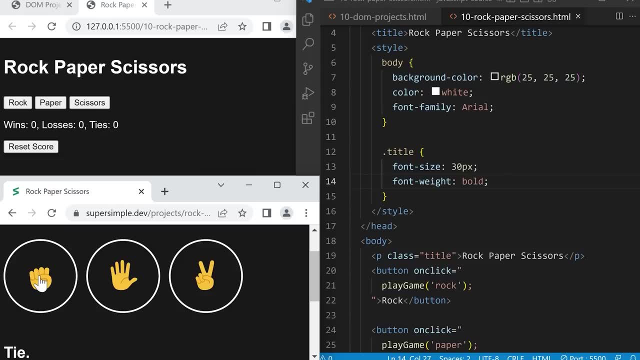 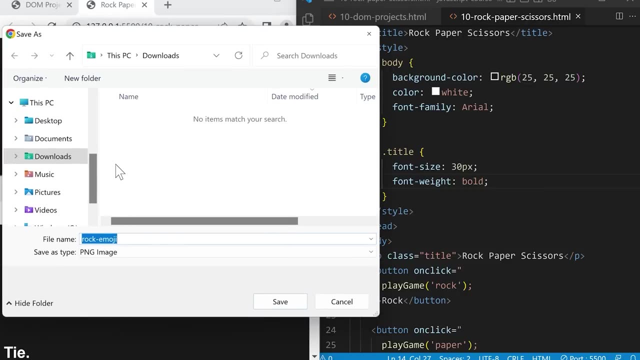 so first we're going to need these images in our project, and i'll show you how to get them. we'll put our mouse over the rock image and we'll right click and we'll click save image. and now we're going to find the folder that contains all of our 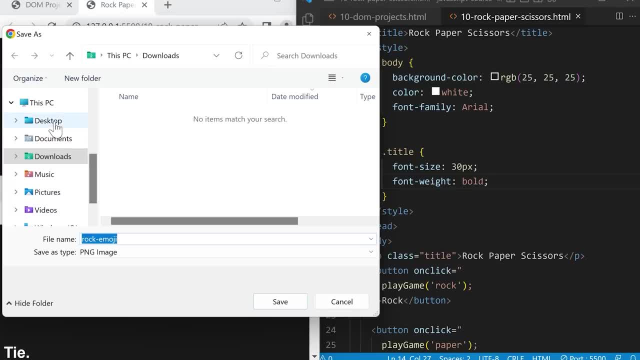 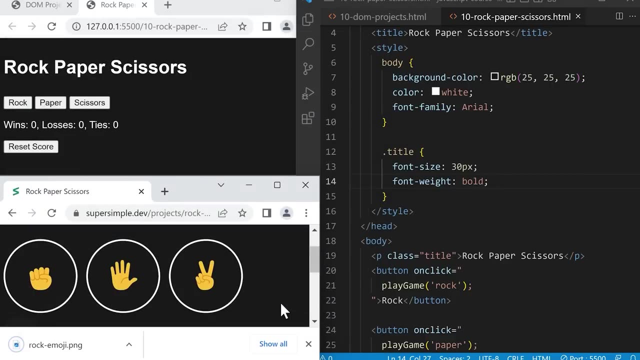 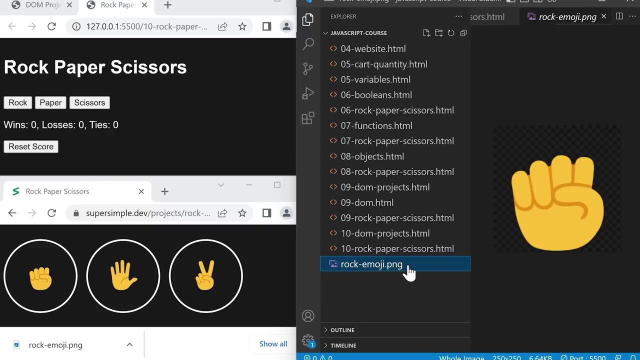 code. so for me it's on the desktop and it's this folder right here. so i'll double click this folder and then leave the file name as the default, rock dash emoji and click save. and now in our code editor, if we click here, we should be able to see the rock image. let's do the same with the paper. 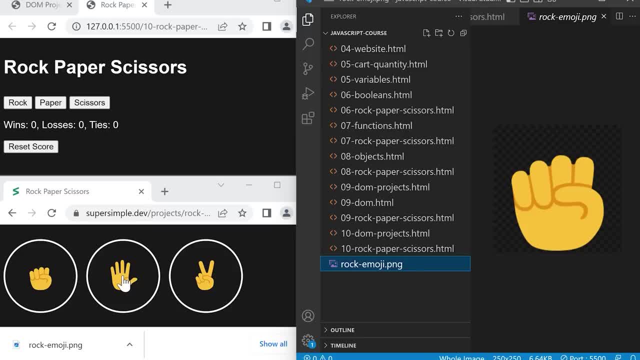 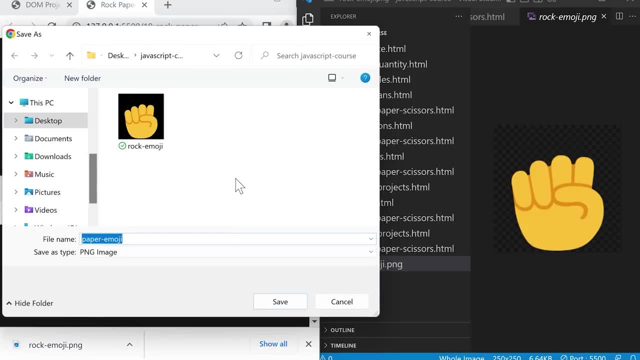 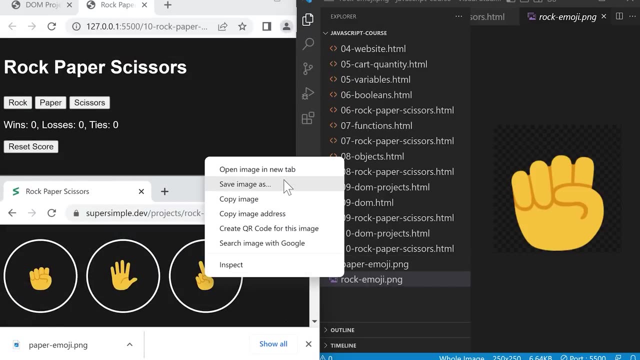 and scissors image, so we'll hover over it, right click, save image, and, in the same folder that contains our code, we're going to save the paper image. and finally, right click, save image and we'll save the scissors image. all right, now that we have these images in our code editor, let's learn how to load them onto the page. 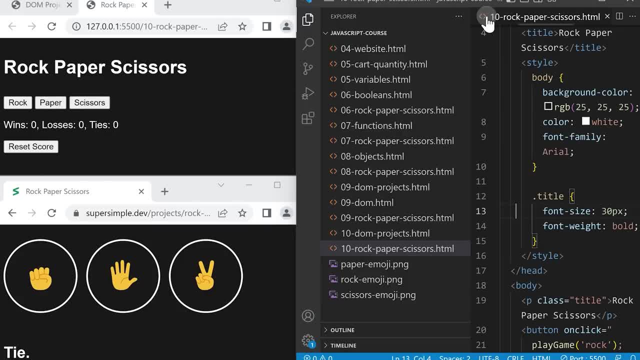 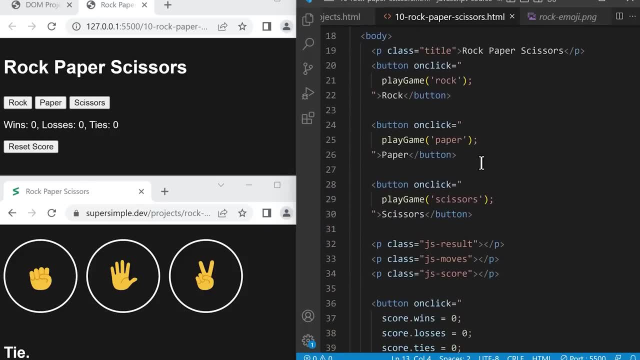 so we can do this using an html element. so we'll go back to our html code and we'll scroll down and inside the button we're going to add an image element. so let's type less than img and greater than so. this is the image html element. it loads an image. 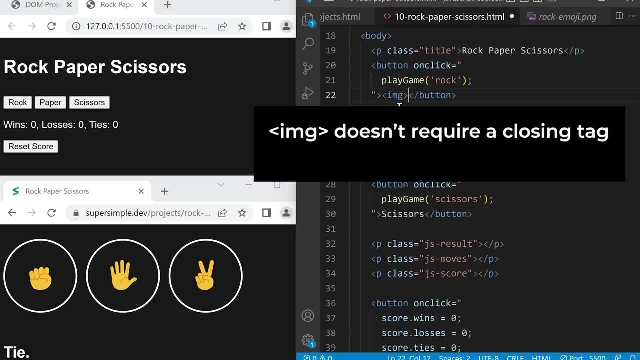 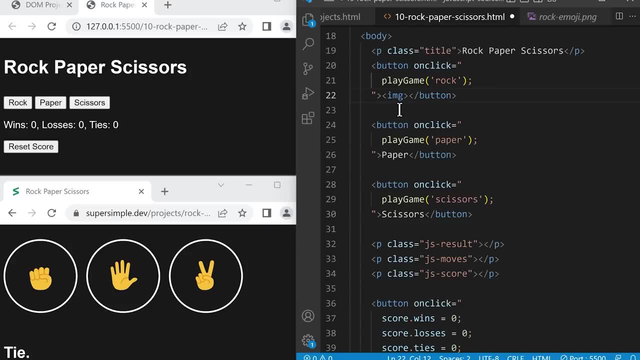 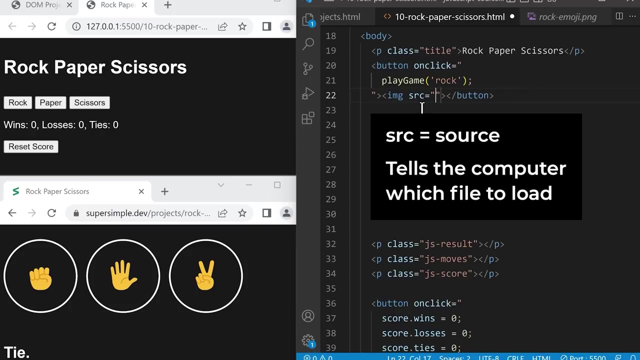 onto the page. so if we click on that image element, it loads and it loads, and so this image element doesn't require a closing tag. this is called a void element. now to load an image, we're going to add an attribute to this element called src. so src stands for source. it tells the computer which file. 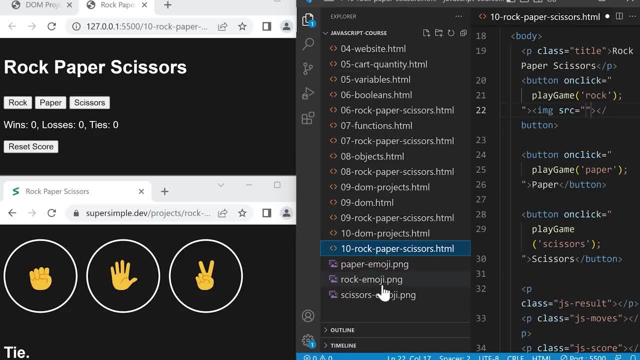 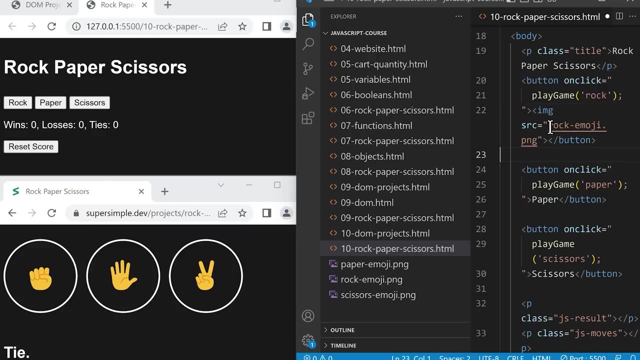 or image to load. so let's look in our project. Inside the source attribute we'll type rock-emojipng. So what this does is it will look for the file with this name beside the HTML file, and it finds it right here and it will load it onto the page. 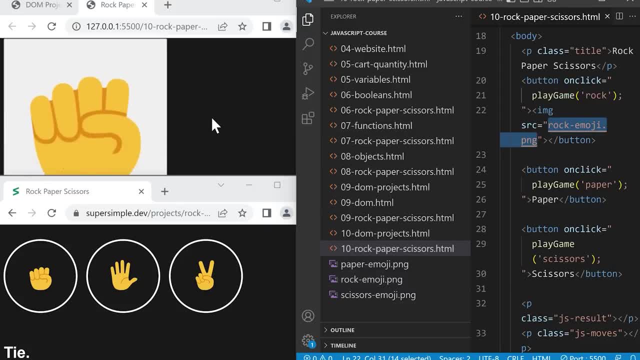 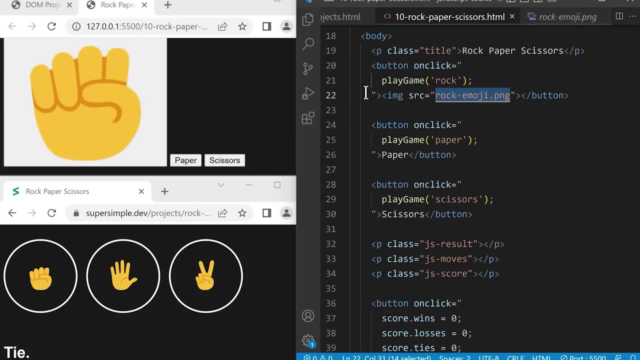 If we save now inside our button, it loaded the rock image Right now. this image is too big, so let's use CSS to decrease the size of this image. We'll hide the files and let's give a class attribute to the image element so we can. 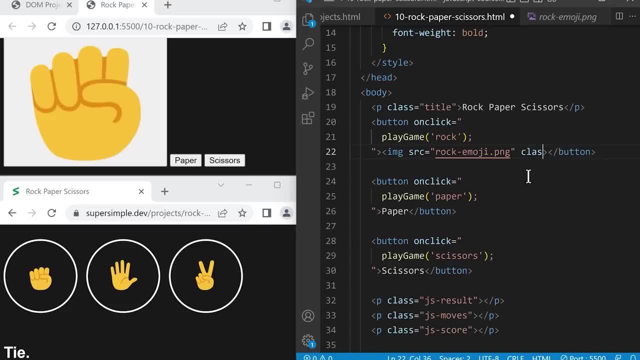 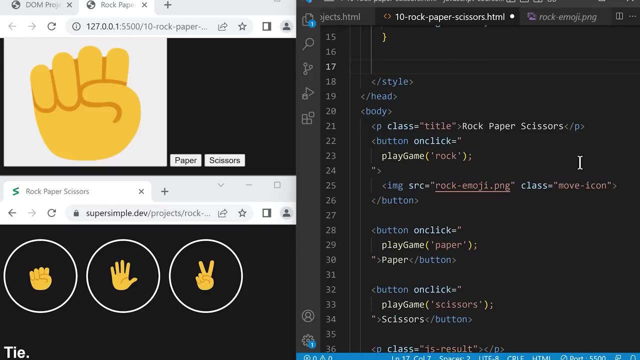 style it. So we'll type: class equals And let's call this a move Move dash icon. And I'm also just going to add some new lines to make the code a little easier to read. So we'll scroll up to the CSS and we're going to style this class using dot move dash. 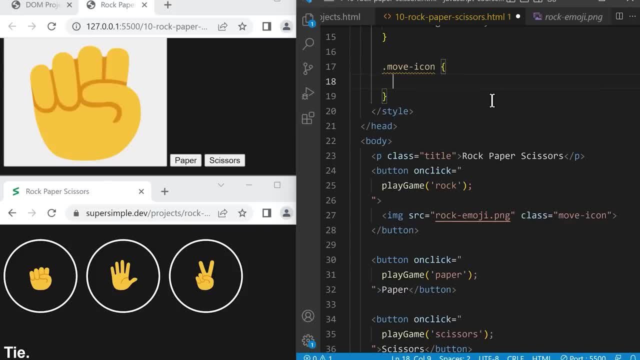 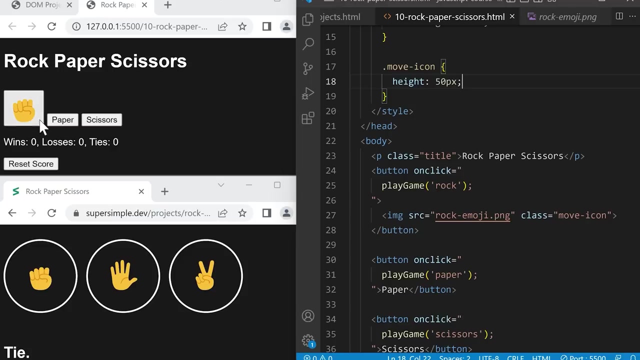 icon and curly brackets. And let's decrease the height of this image. We can use the property height, colon and a pixel value- 50 pixels And save. So this will make the height of this image 50 pixels And it will also resize the width automatically so that the image keeps its shape. 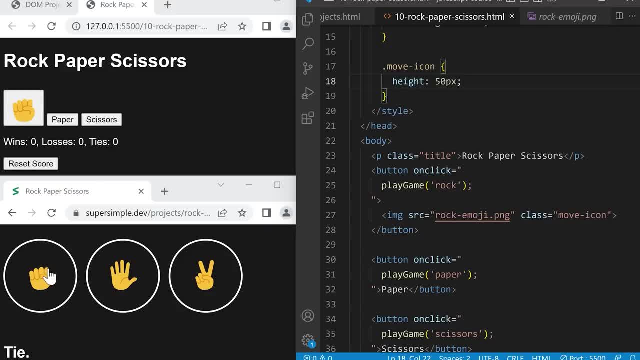 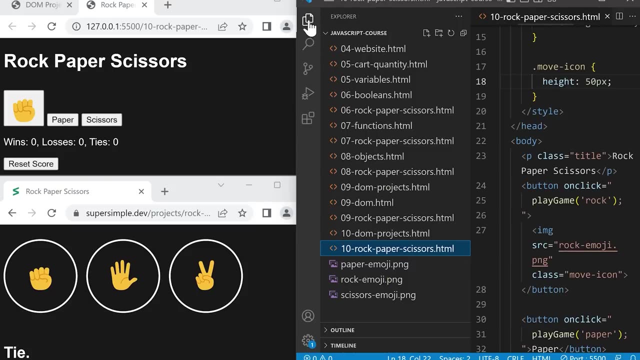 So this size looks pretty close to the final design, So we can move on, Okay. Another feature of the source attribute is that we can put our files into folders. So let's open the files by clicking here And let's say that we want to organize all of our images into a folder. 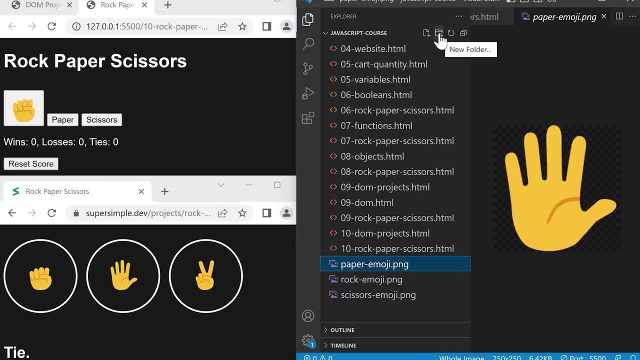 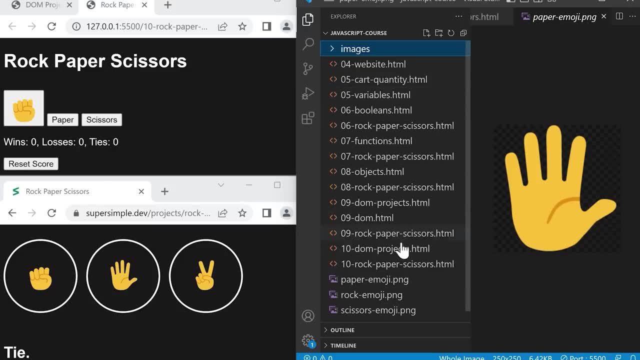 So we're going to create a folder by clicking this icon And let's name this folder images, And we're going to drag this, Okay. Okay, So we're going to drag these images into this folder And drag this in here. 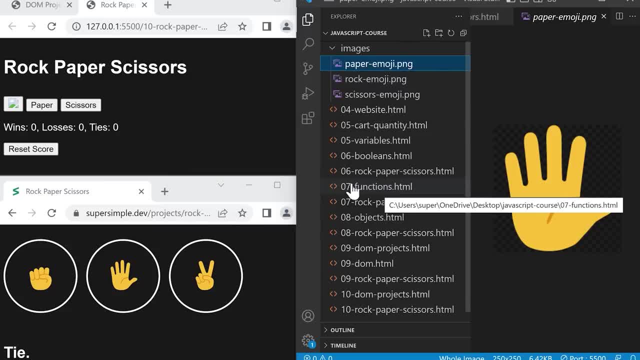 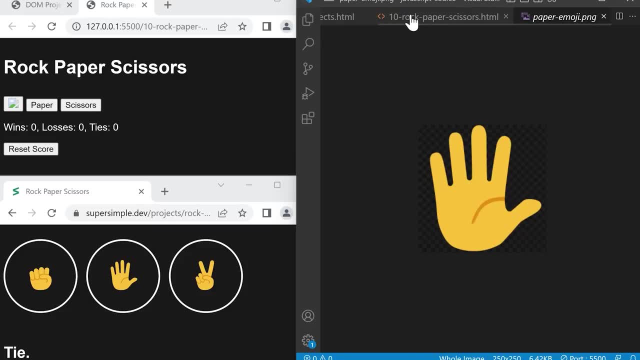 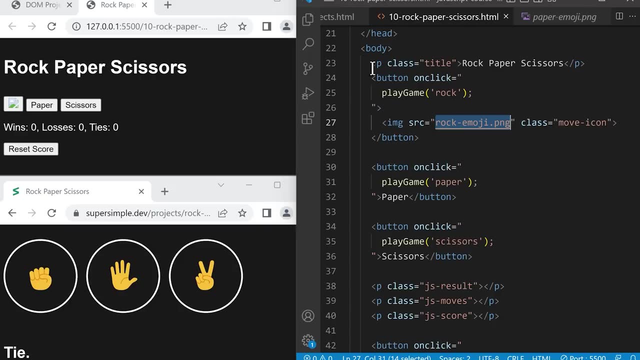 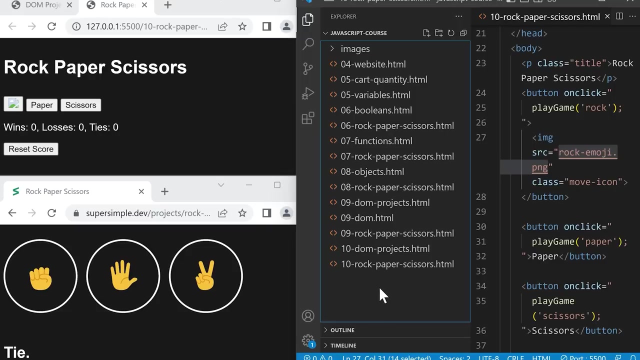 And in here. Now, unfortunately, you can see that the image doesn't load anymore, And that's because, if we look at our code, source tells the computer to look for this file beside this HTML file. Okay, Okay, So now there is no file called rock-emojipng, because we put it in a folder. 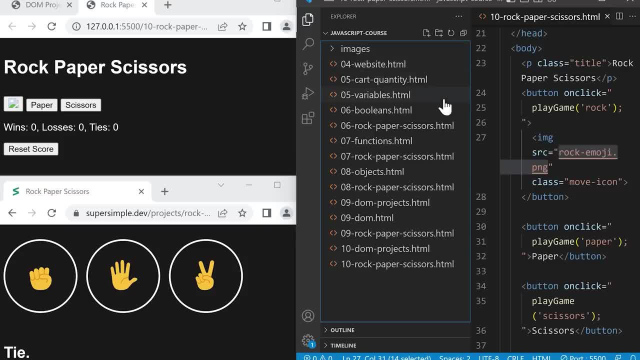 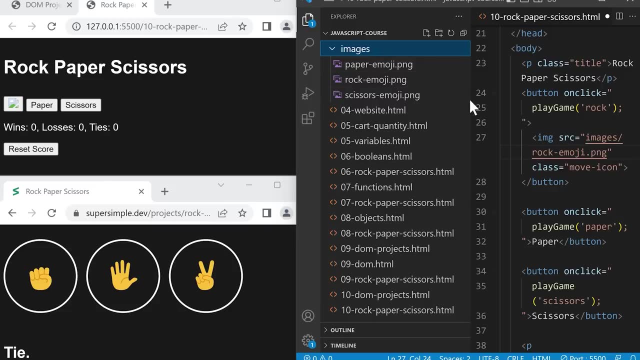 So to tell the computer to look inside this folder, we're going to type the folder name at the start, which is images, And then we're going to type a slash to go into the images folder and then look for this file, which is right here. 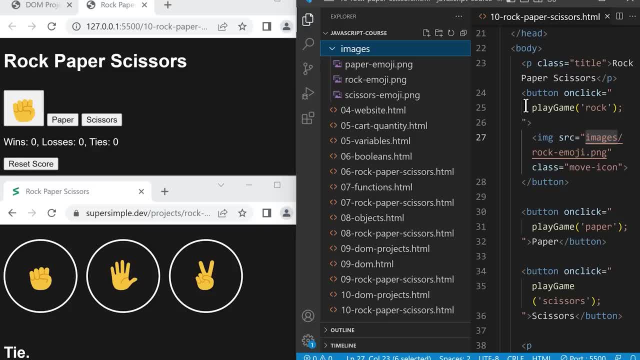 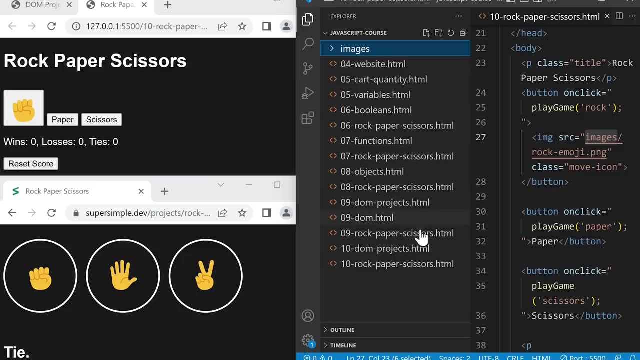 Okay, So if we save, the computer is now able to find this image and load it onto the webpage. So this feature is called file paths. We can tell the computer to look for a folder beside the HTML file, like images, and then. 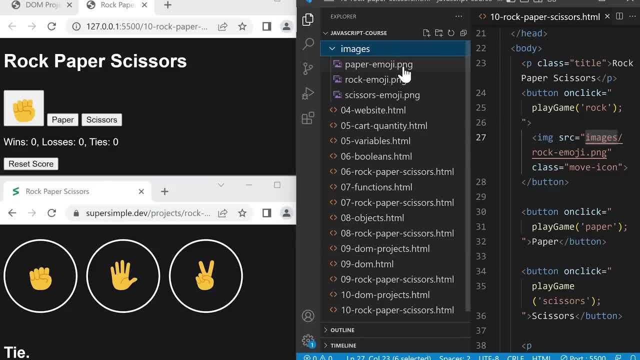 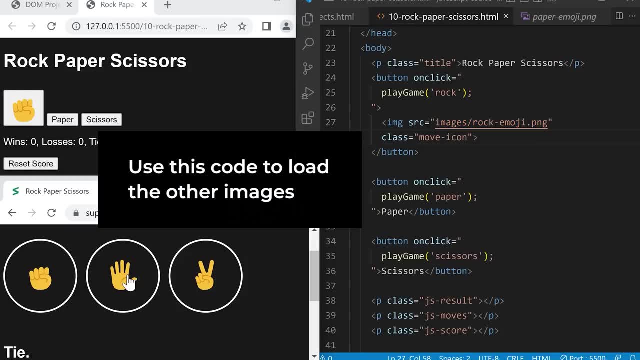 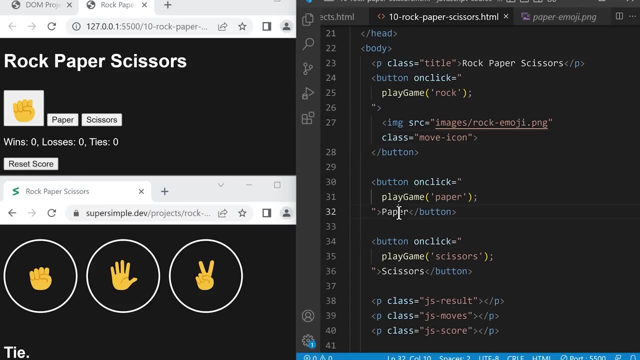 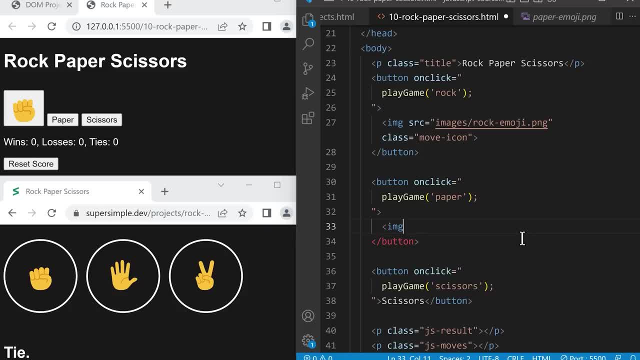 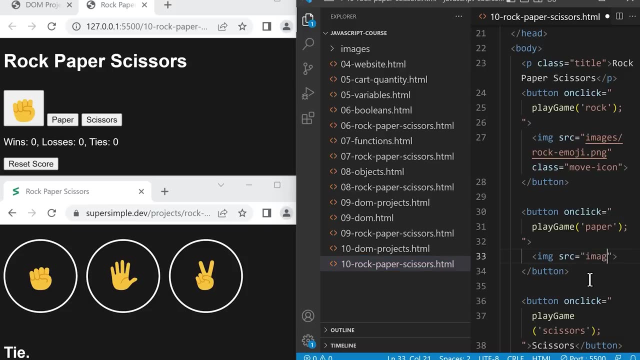 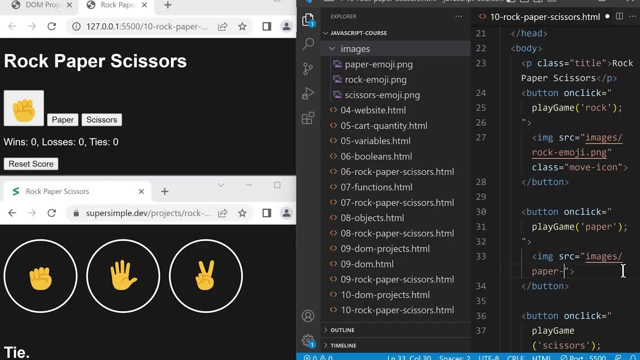 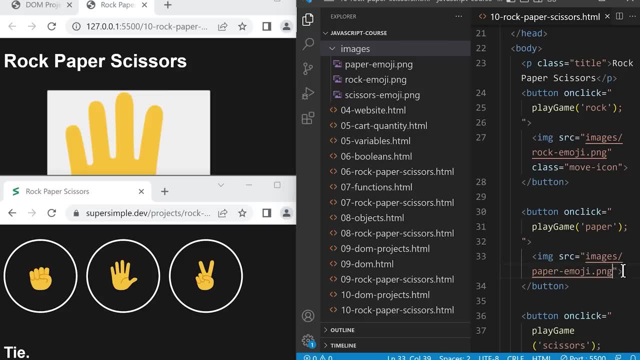 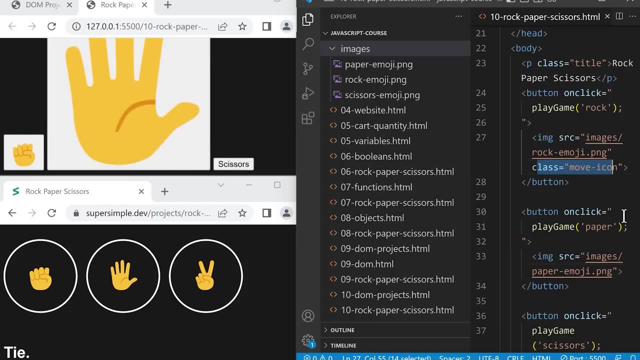 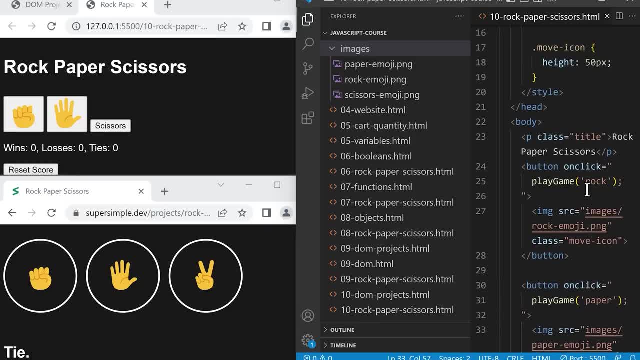 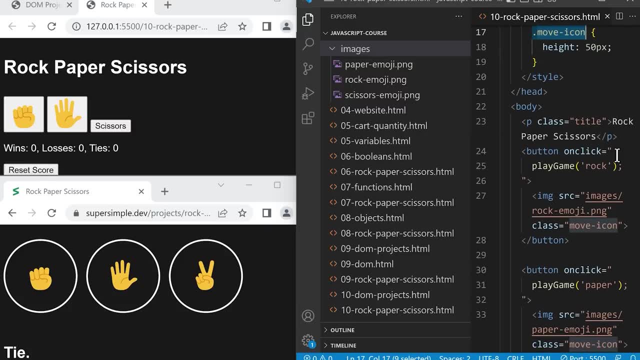 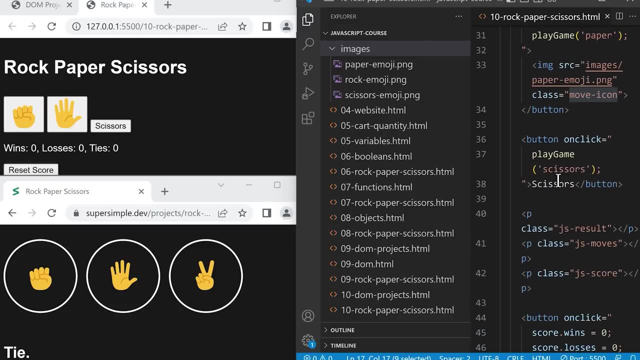 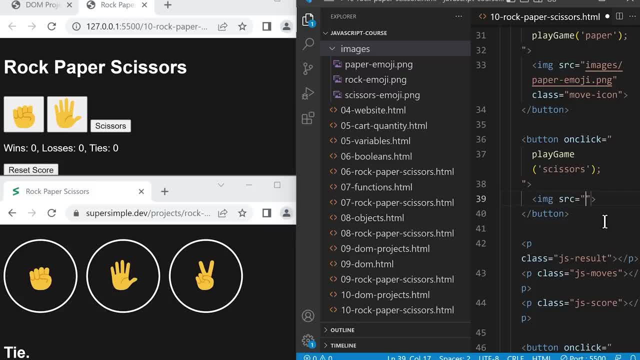 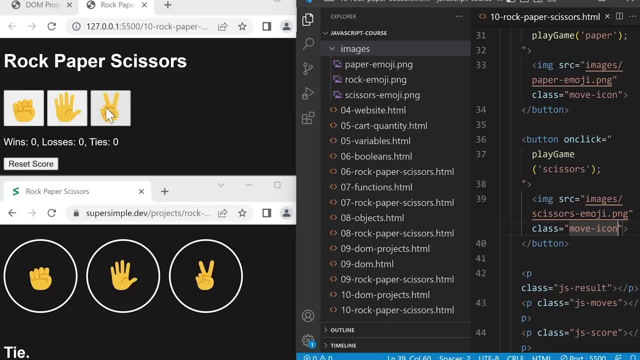 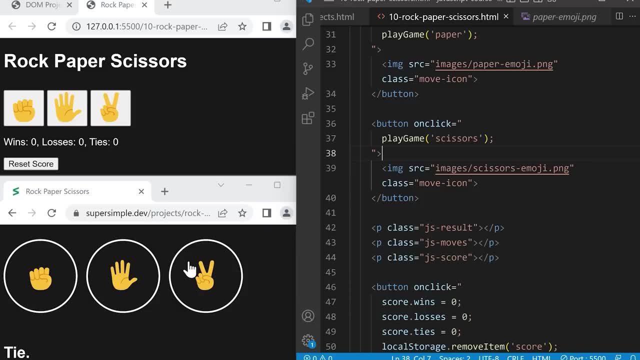 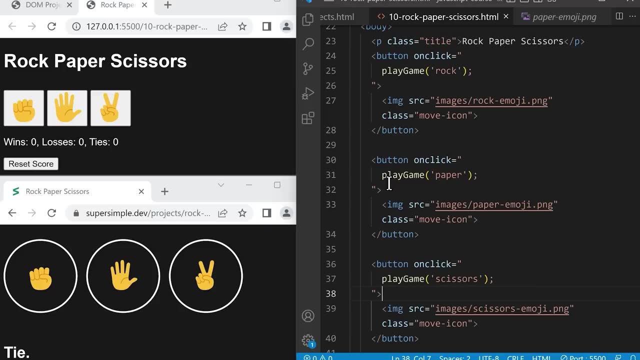 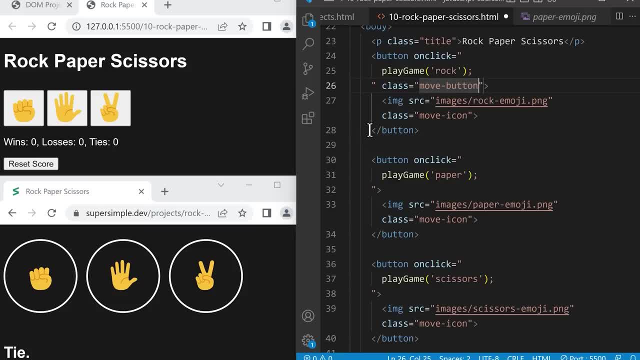 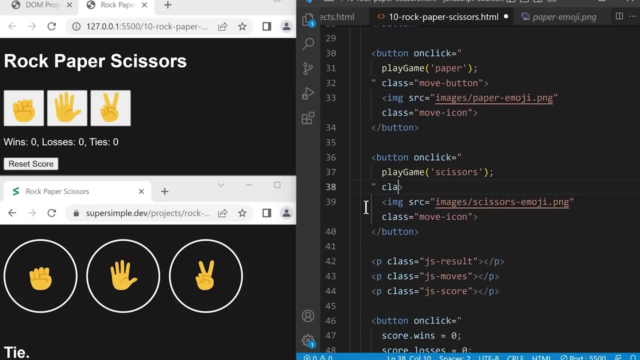 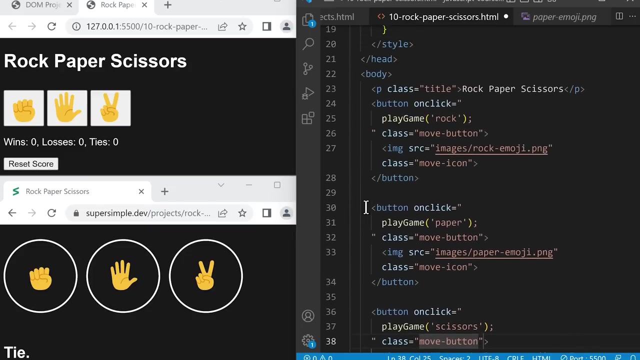 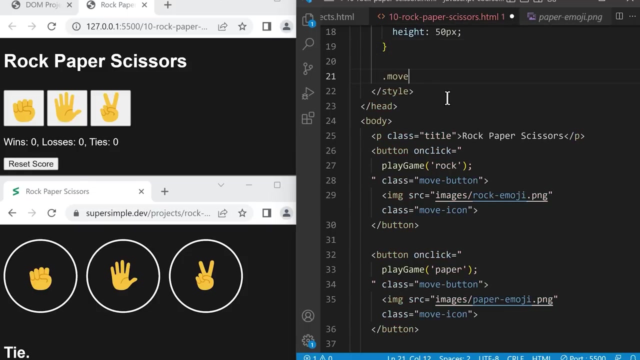 Okay, Okay, Okay, Okay, And for this button we'll add the same class- class equals move-button- as well as for the third button: class equals move-button. Now let's scroll up to our CSS and we're going to style this class using move-button. 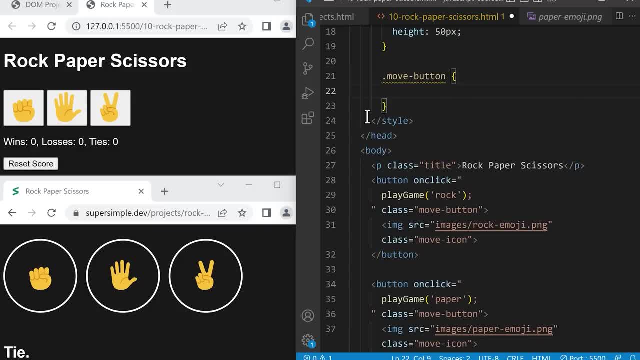 So first let's change the background color to match the background color of the page. So we'll use background-color colon and we'll use a special value called transparent, And this will make the button see-through. If we save now, these buttons are see-through. 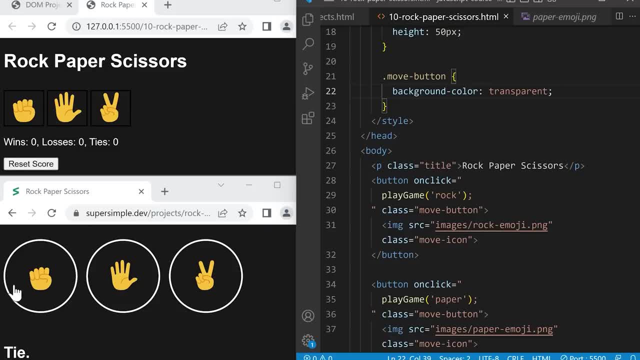 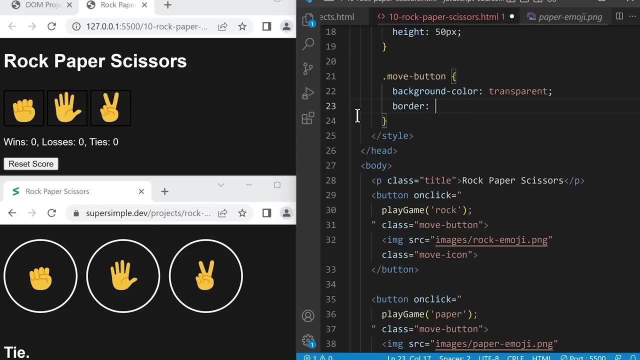 Okay. Next let's add this white border to our buttons. So we'll use the border property colon, and we're going to give it three values. The first value is our border width, or how thick the border is. Let's use one pixel for now. 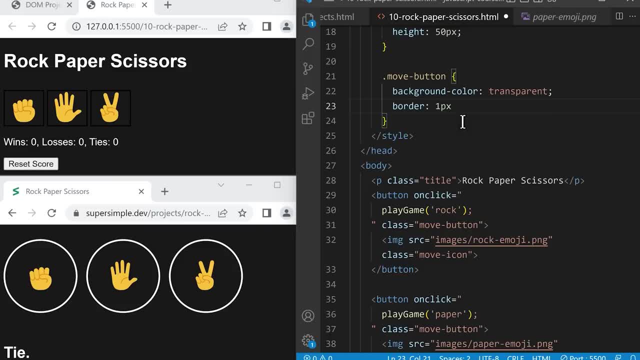 The second value is the border style, and we'll use solid Because it's a solid border. Other values we can use here are dotted or dashed. And the third value is the border color, So we're going to use white And semicolon at the end and save. 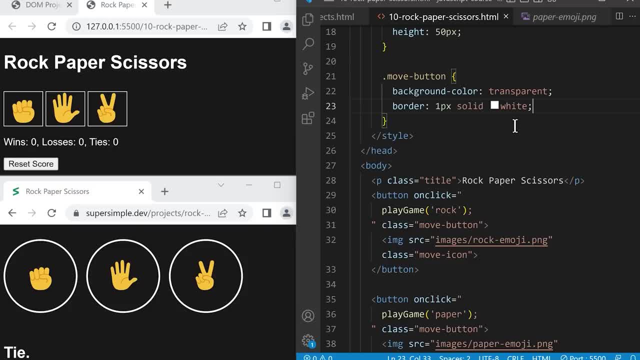 And that will add a border. So let's make our border a little thicker. like the final design, We'll change this first value, Which is the border width, to three pixels And save. Okay, So that looks pretty close. Now let's change the size of our buttons. 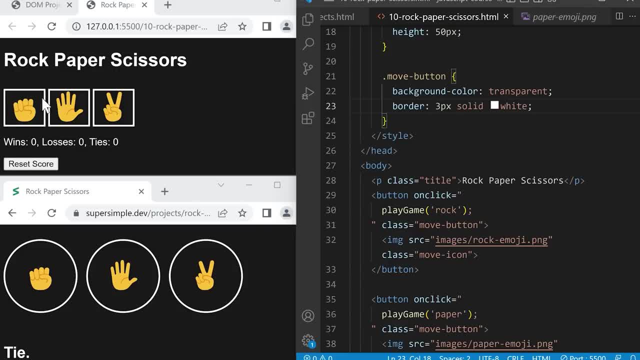 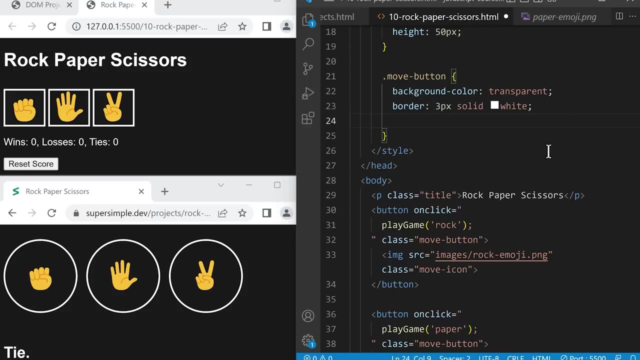 Usually we use the padding to add space on the inside of an element, But in this case our images have different sizes, So we're going to use width and height to set an exact size. So in our CSS We'll type Width. 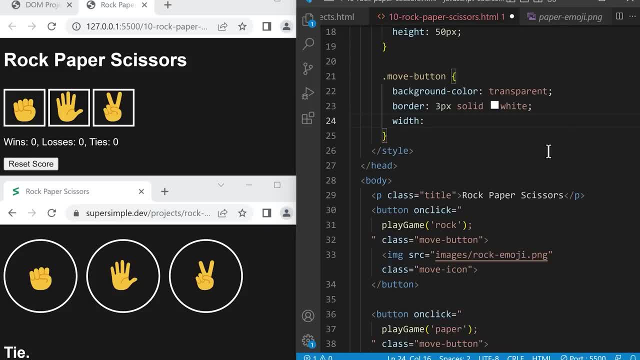 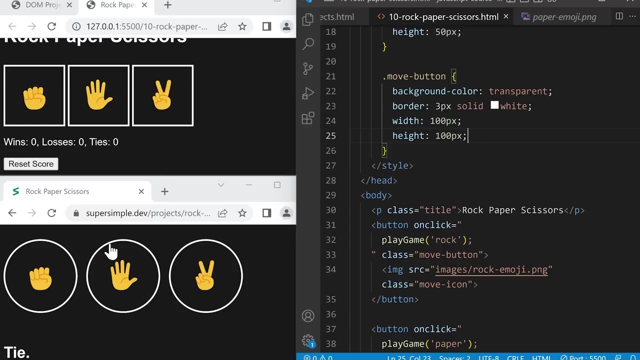 Colon And let's make it a hundred pixels And height And also one hundred pixels And save So it looks like our final design is a little bigger than what we have here. So let's increase the width and the height. So let's try one hundred twenty pixels. 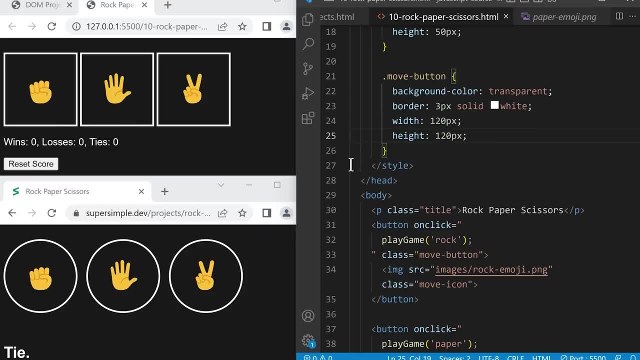 And save There we go Alright. so that looks pretty close. Now let's make these buttons round, And the property for that is called border-radius colon. and to know how much we need to make it round, we can set it to half of the width or the height. 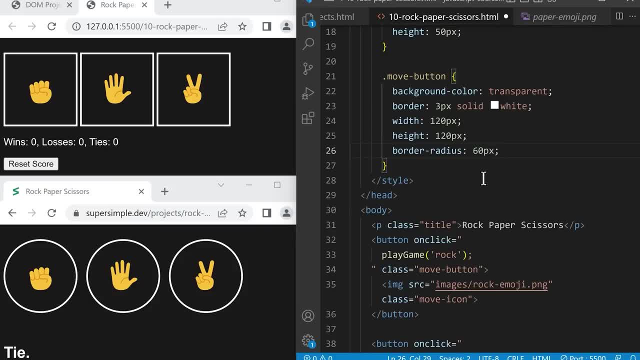 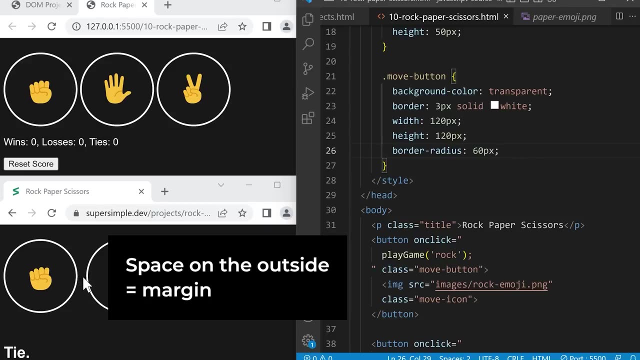 So we'll set it to 60 pixels And save. Okay, so it's coming along really well. And lastly, we're going to add some space between the buttons, So remember that space outside of an element is called margin, So let's add some margin on the right. 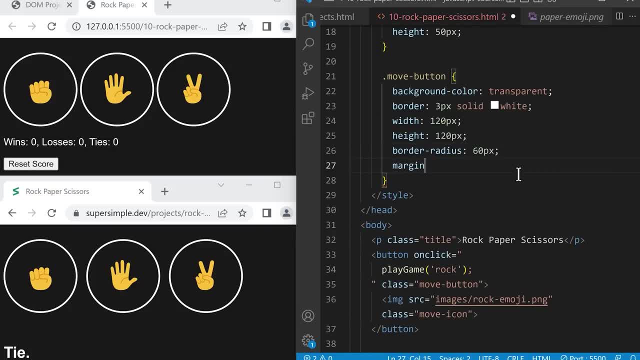 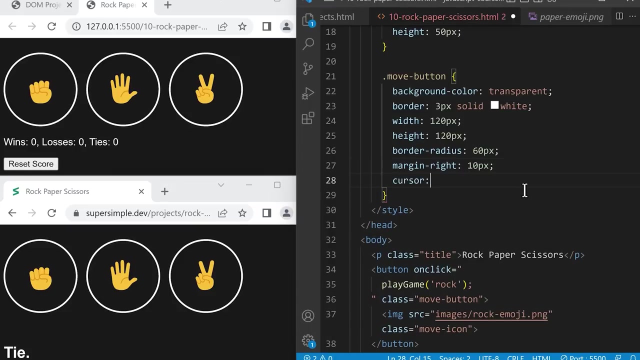 So we'll type margin-right colon, margin-right And maybe 10 pixels And save, And finally, when we put our mouse over the button it turns into a pointer. So the property for that is cursor colon pointer. 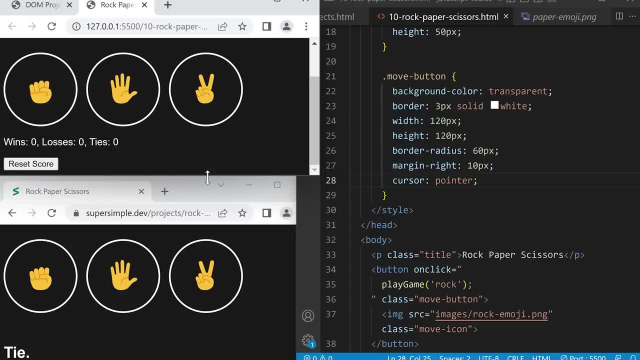 And save, And now our buttons match the final design. So let's keep moving And let's style the next part of the project, which is the result and the moves. If you don't see this here, you can just play the game. 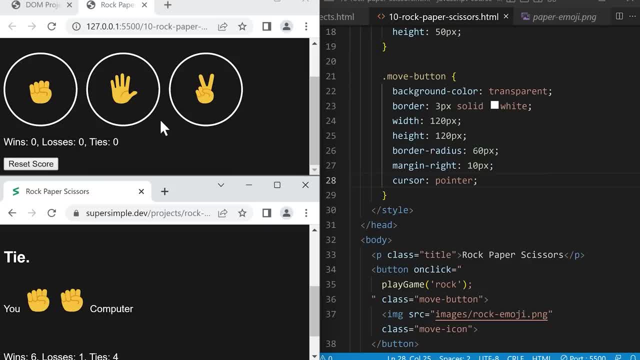 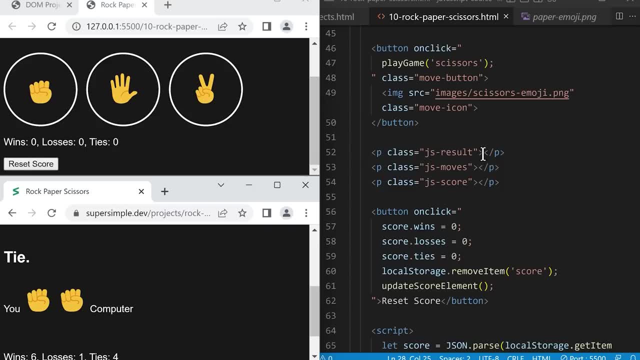 And it'll give us a new result. So, to make this easier to style, we're going to go into our code, We're going to find the result, which is here, And we're going to add some fake results. like you win. 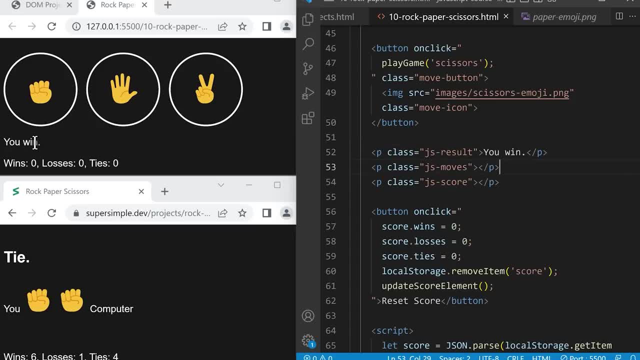 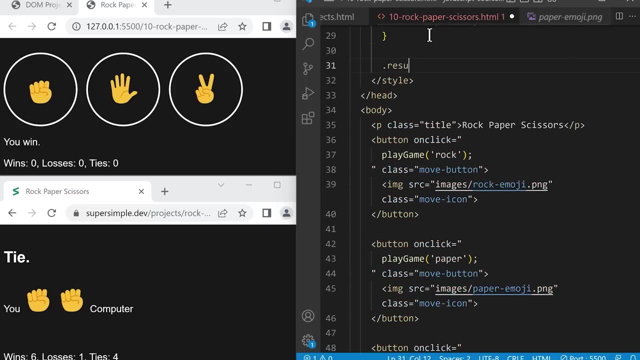 Save. And now we have this result And we're going to style it, So let's give this a class of result. And then in our CSS, we're going to style the class: dot result and curly brackets, So let's make the text bigger. 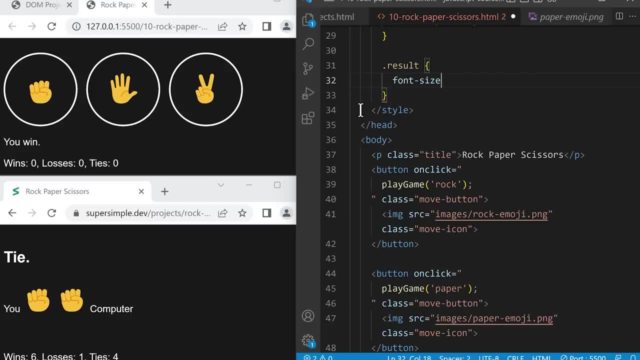 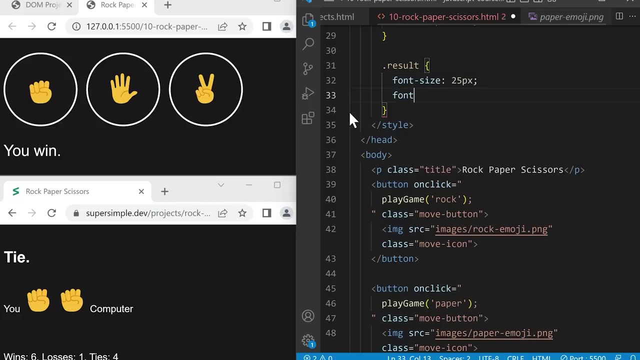 We're going to use font-size colon And maybe 25 pixels And save. OK, that looks pretty good. Let's make the text bold, So we use font-weight colon bold And save. And finally, we're going to add extra spaces between this and the buttons. 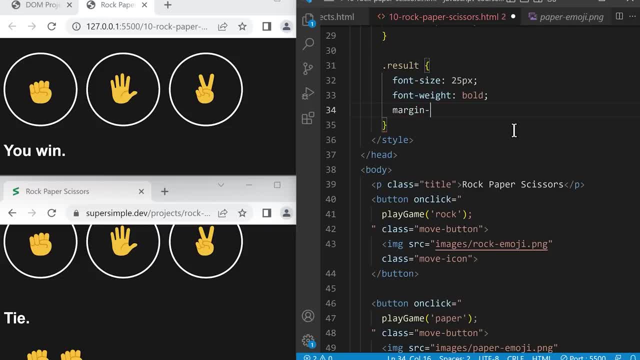 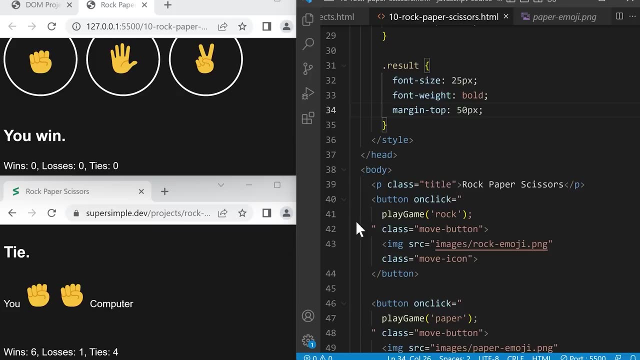 So we'll add margin, DASH, top And maybe 50 pixels And save OK, So I think that looks close enough. Now let's style the moves And again we'll scroll down And we're going to add some fake moves in here. 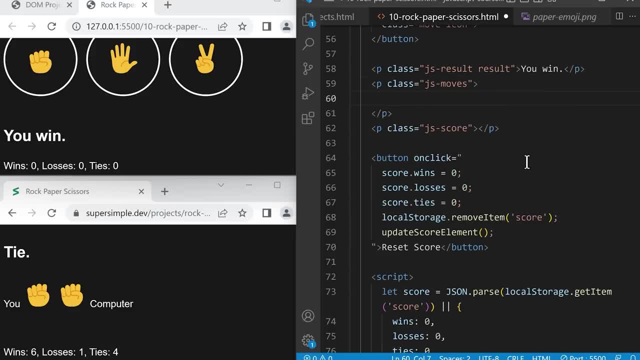 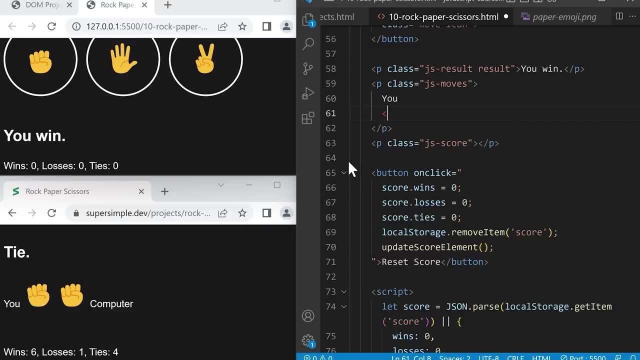 So it's easier to style. So we'll type you And then an image. OK, So let's use the less than image and the source attribute And let's just load the rock image and the scissors image for the computer. So to load the rock image we'll look inside the images folder. 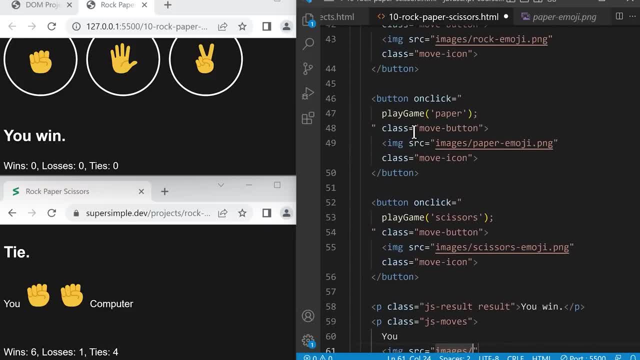 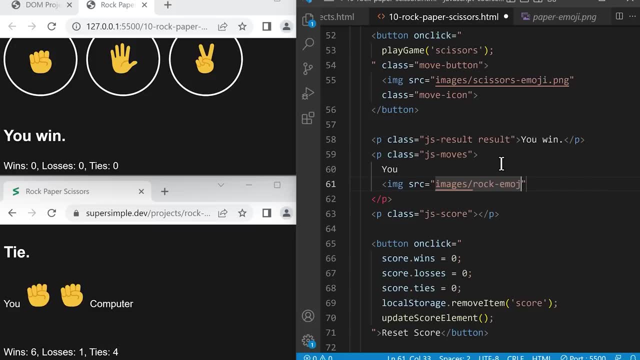 slash to go into the folder and then rock-emojipng. So rock-emojipng, OK, OK, And we'll add another image Less than image. Source Equals Images. Slash These scissors emoji, Scissors Dash. 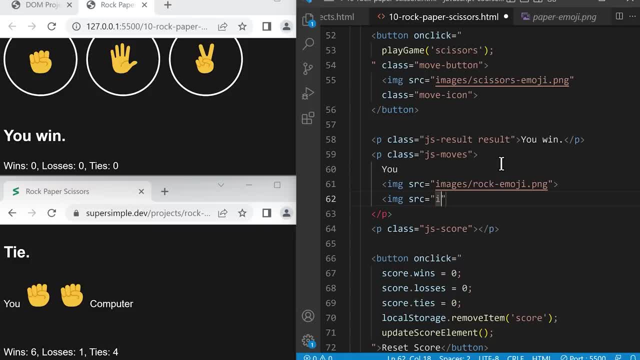 Emoji Dot. PNG And greater than. And finally, the text Computer And we'll add another image. Less than Image. Source Equals Images. Slash These scissors. emoji Scissors, Dash Emoji Dot. 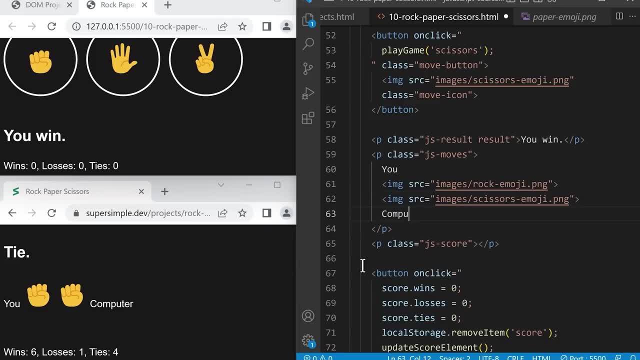 PNG And greater than Let's save, and this will create some results, although the images are really big, So we can use the class move icon to resize them to be the same size as the buttons. So for both of these images let's add the class move dash icon. 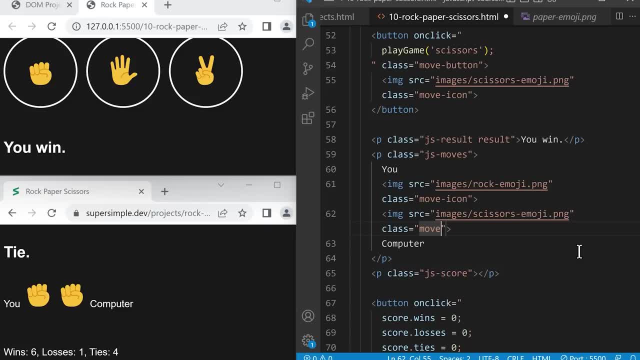 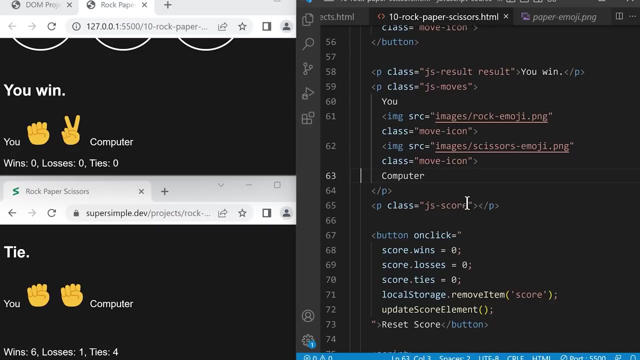 And here as well. class equals move dash icon And save, And now our images look good. Next, let's style this score section. So the only thing we need here is to add spaces between these two. So in this score element, let's add a class of score. 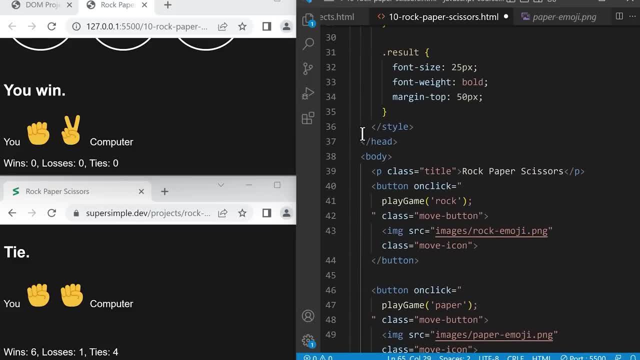 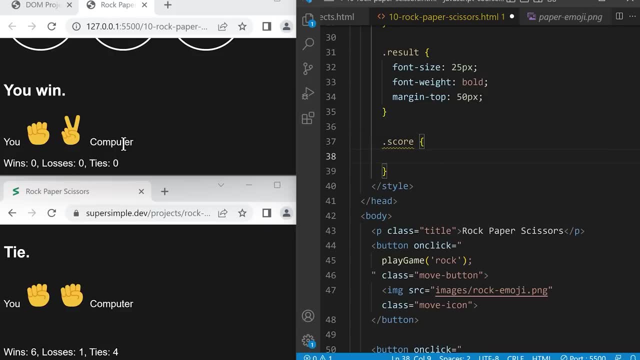 And we'll scroll up and style this element using dot score brackets and let's add some margin at the top. So margin, dash, top colon 50 pixels and save and let's compare it And it looks like our final design has a little more spacing than this. 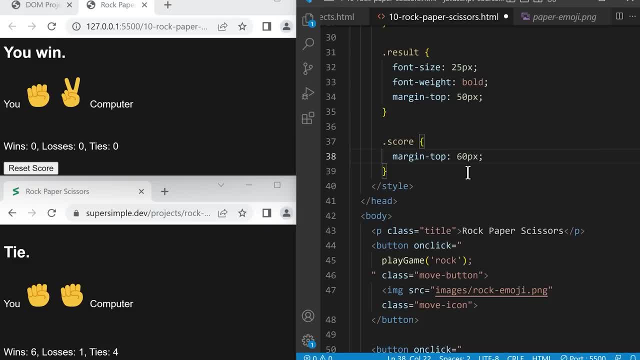 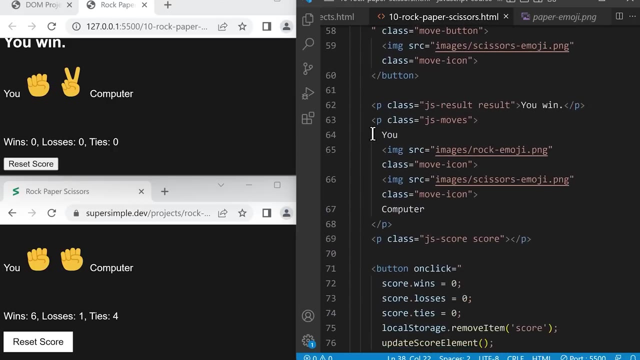 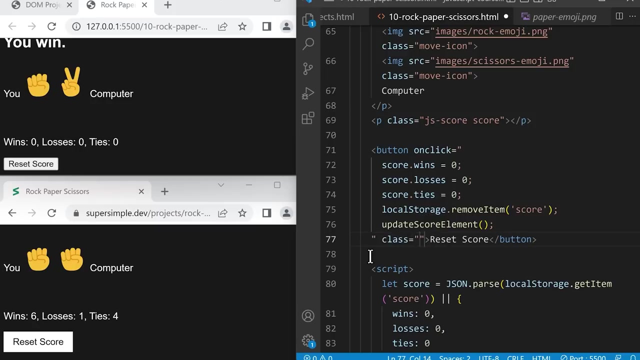 So let's change this to 60 pixels and save, And that looks close enough. And finally we'll style the reset score button. So let's go back to our HTML. We'll add a class to this button. So here class equals reset. dash score, dash button. 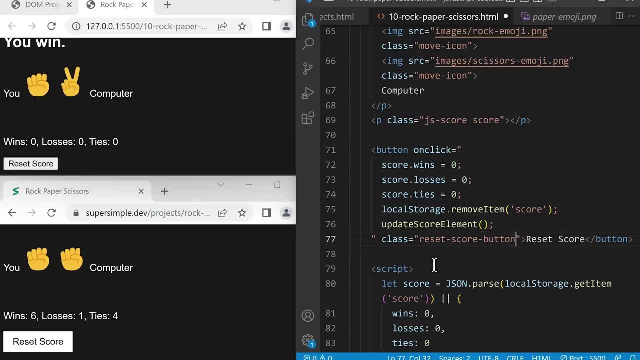 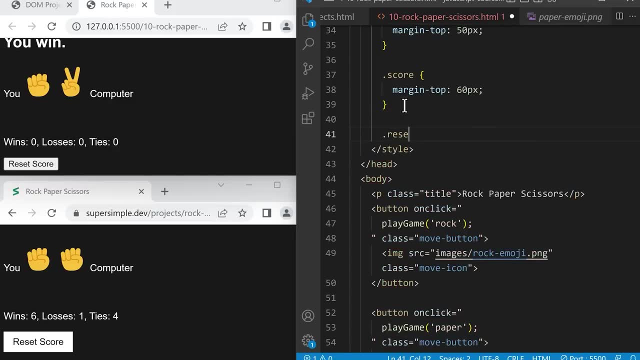 And we'll add a class to this button. So here class equals reset dash score dash button. So at the top we'll type dot reset dash score dash button, curly brackets And we'll make the background color white. So background dash color: colon white. 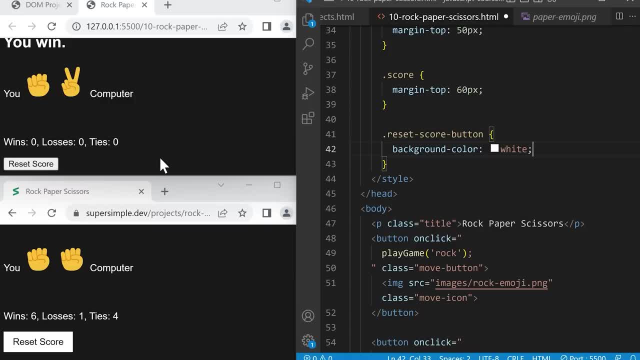 And let's also remove the border from our button And we'll add a class to this button. And we'll add a class to this button And let's also remove the border from our button. And let's also remove the border from our button. 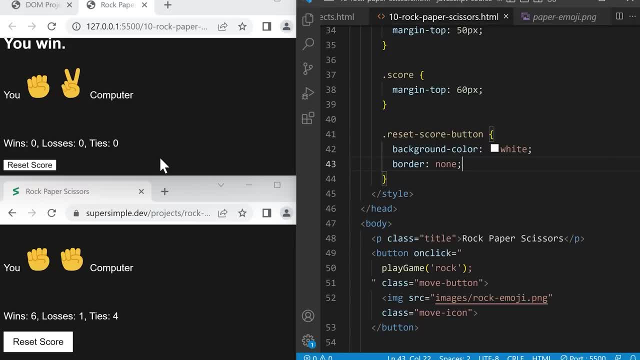 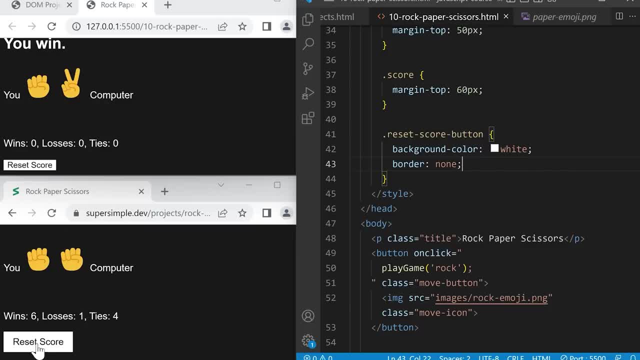 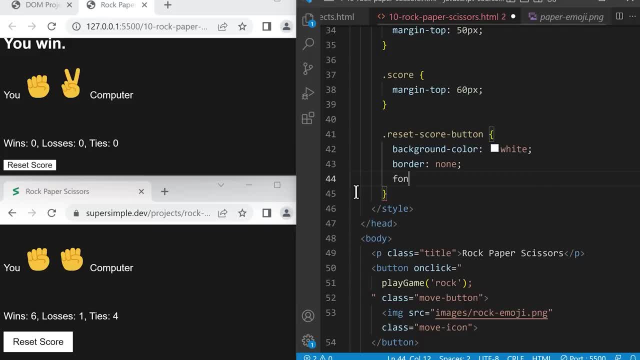 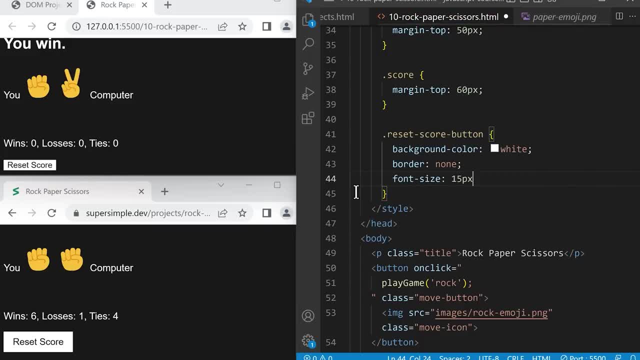 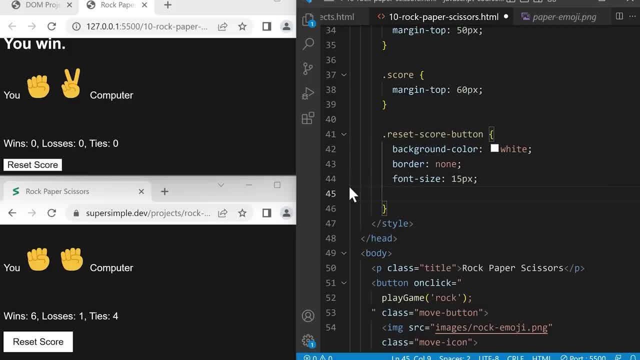 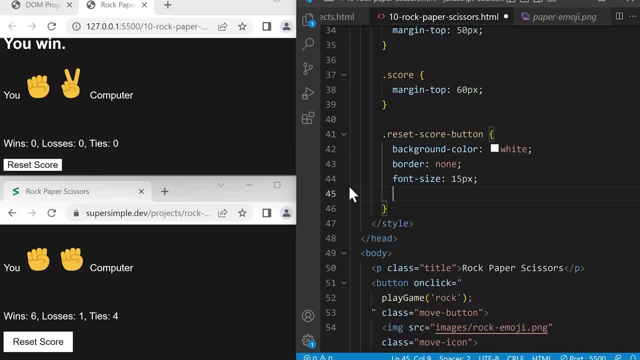 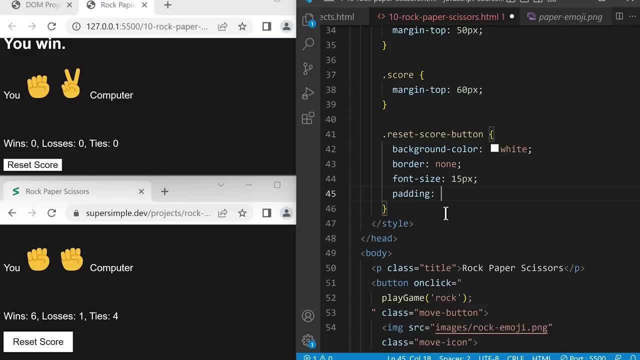 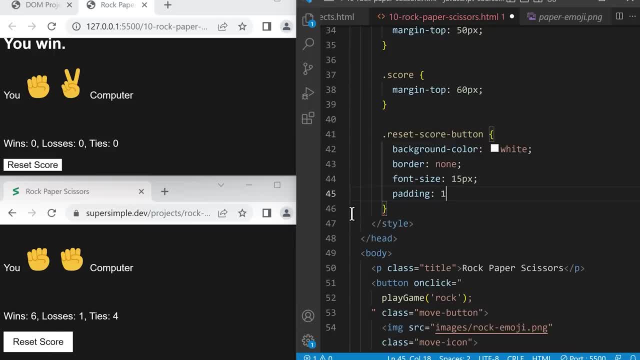 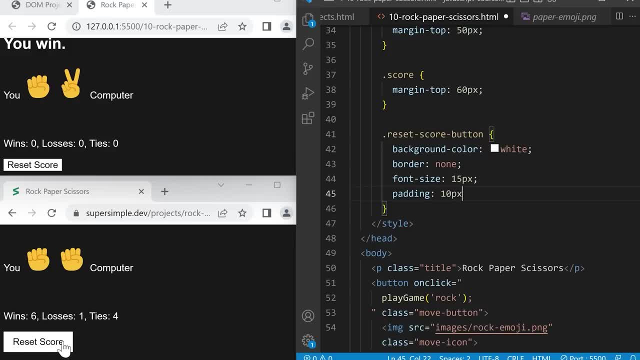 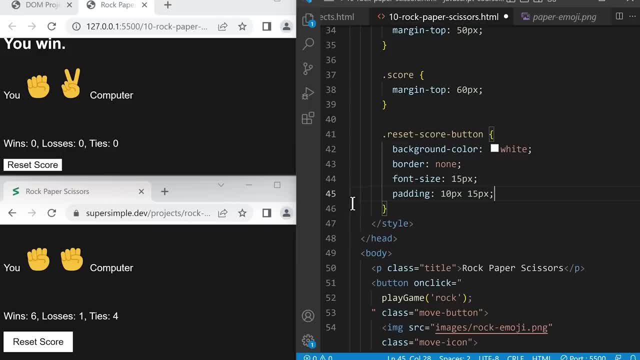 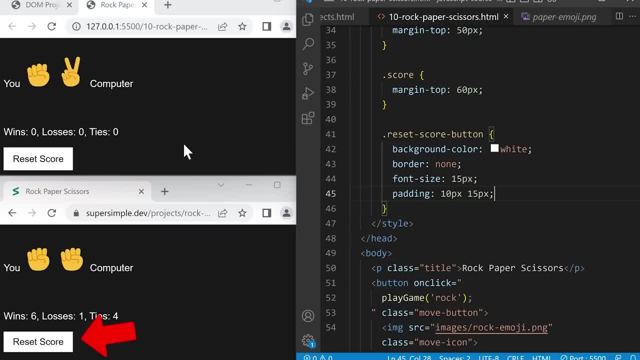 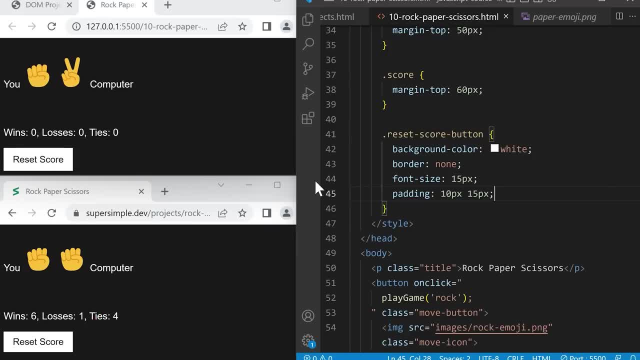 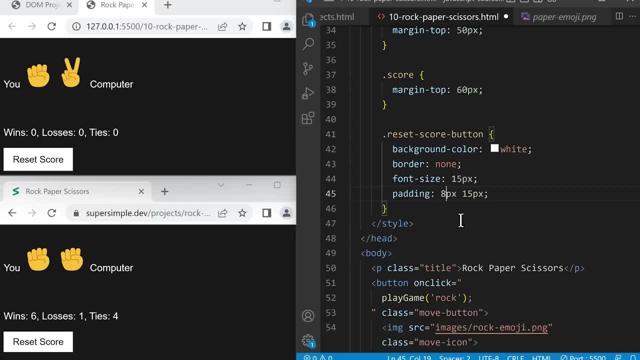 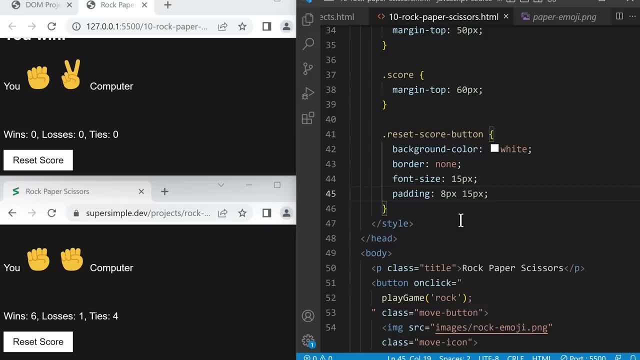 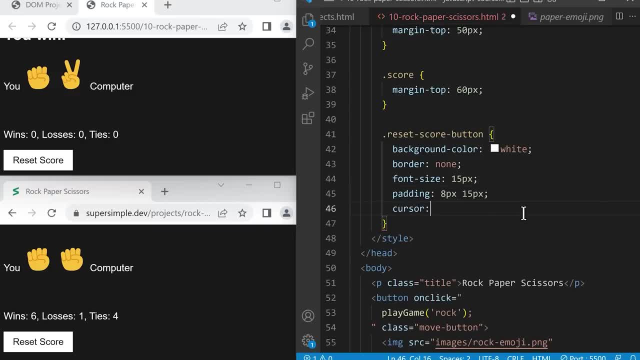 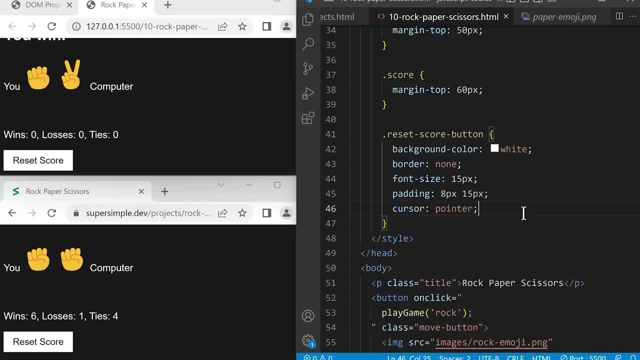 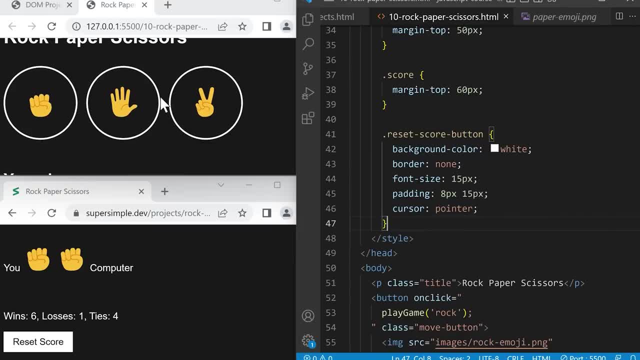 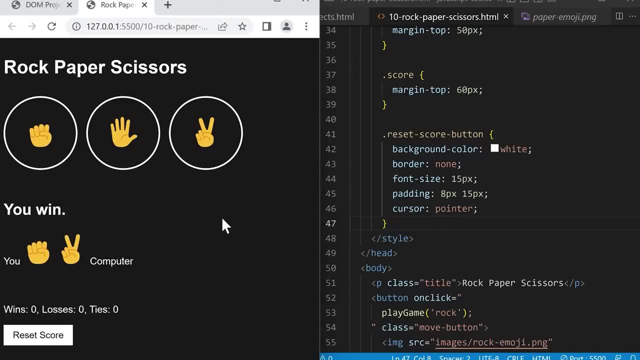 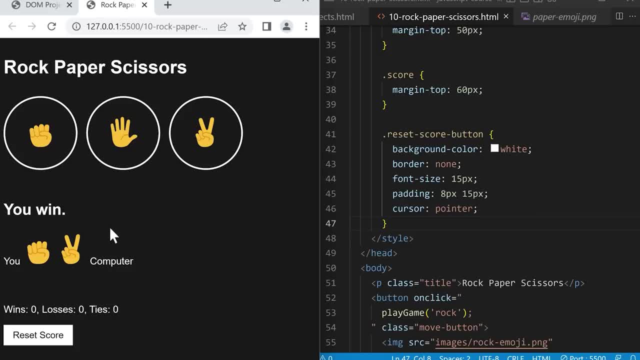 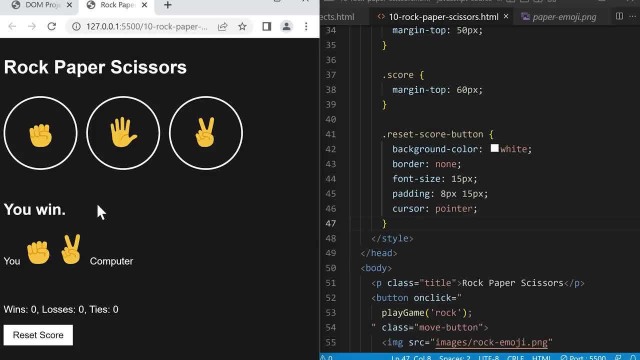 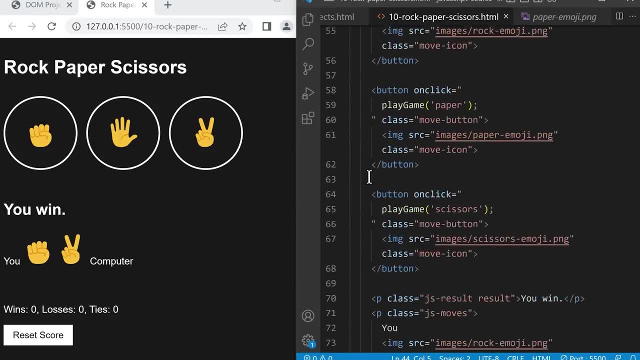 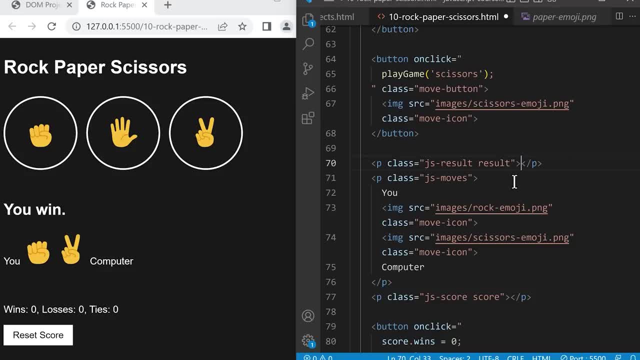 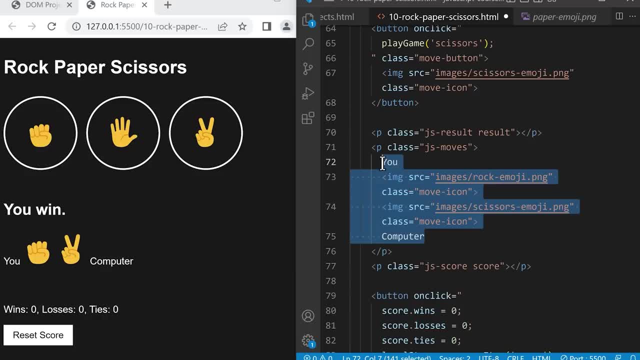 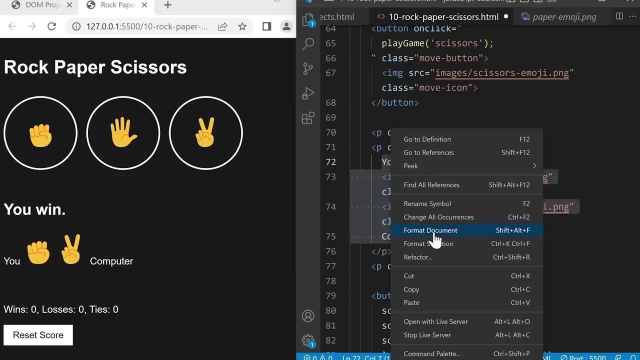 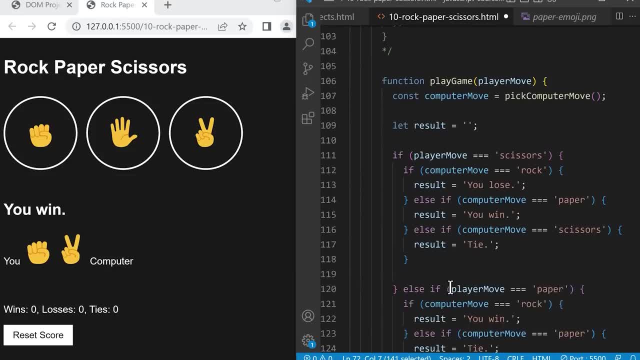 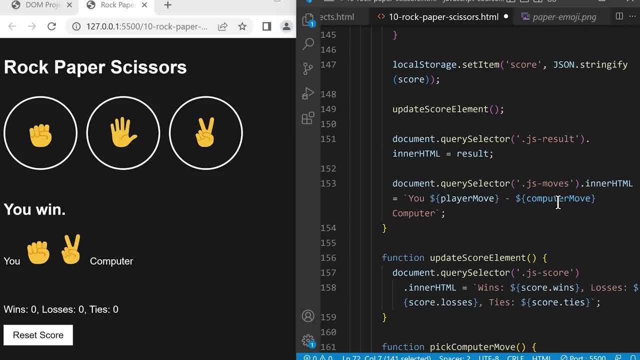 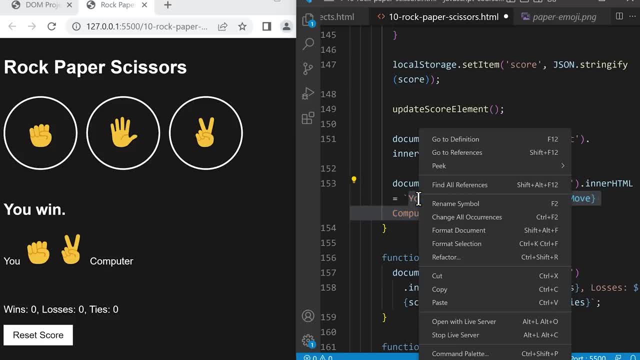 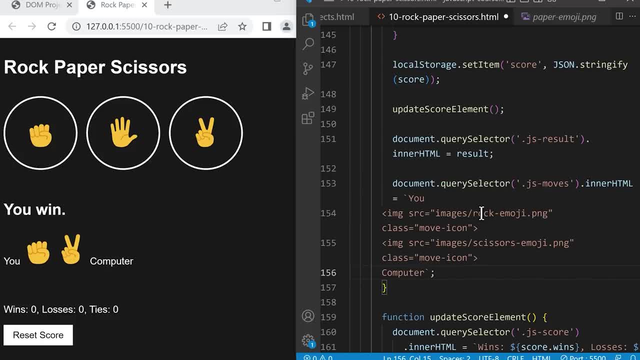 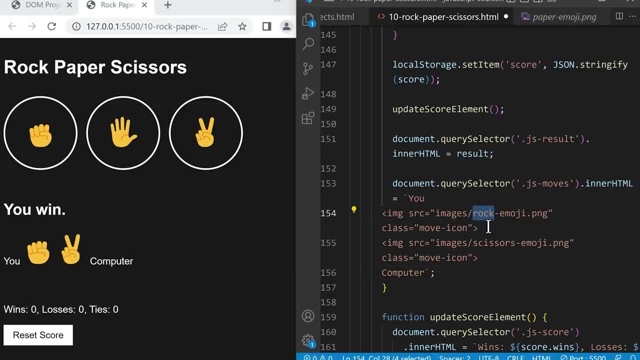 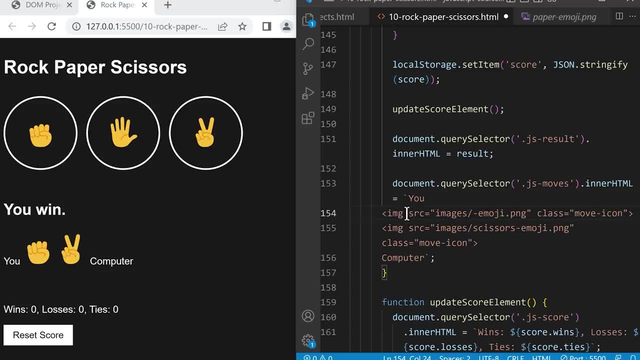 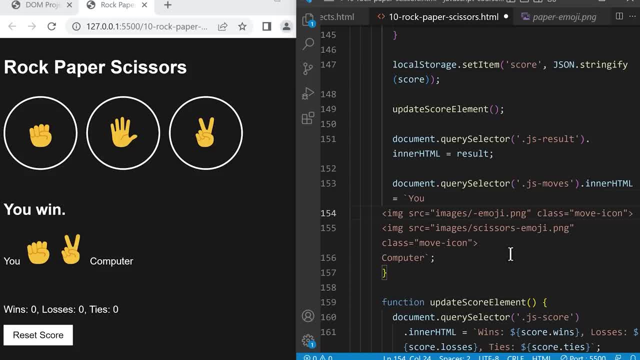 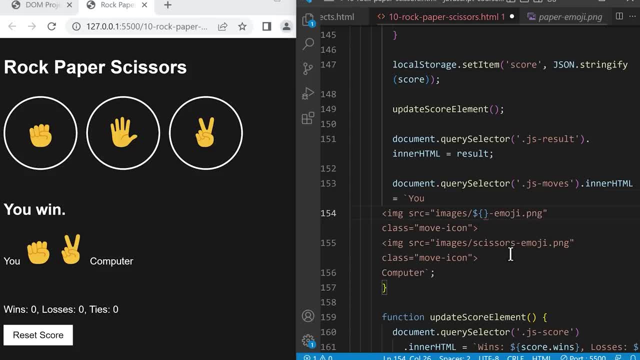 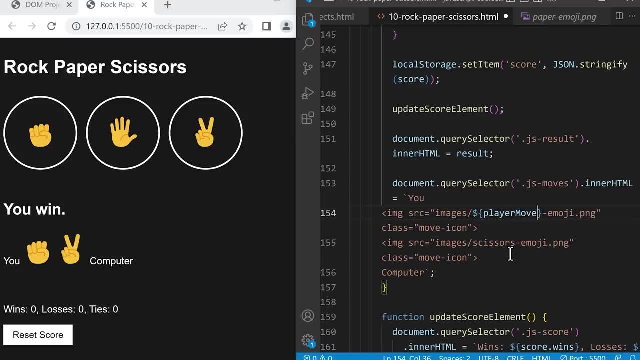 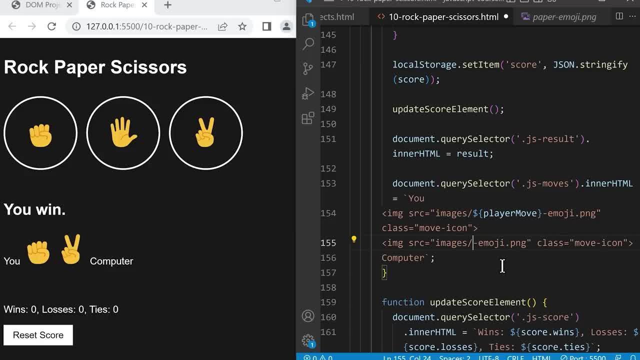 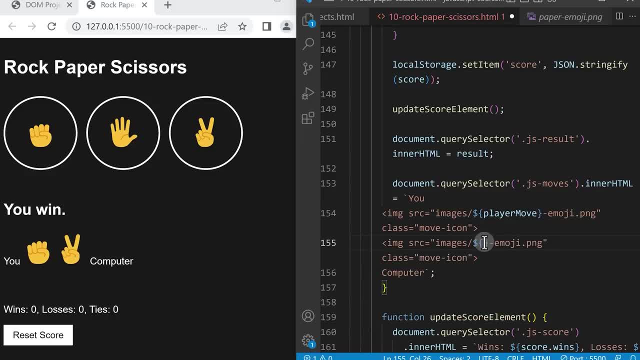 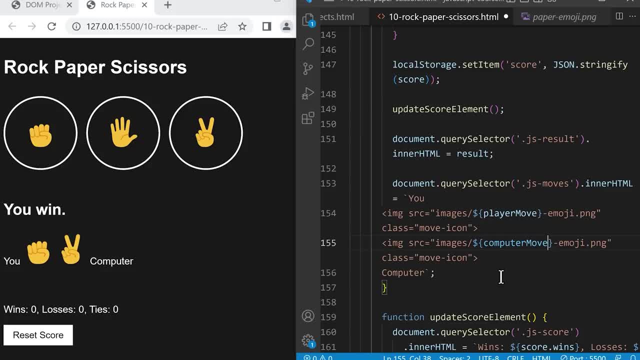 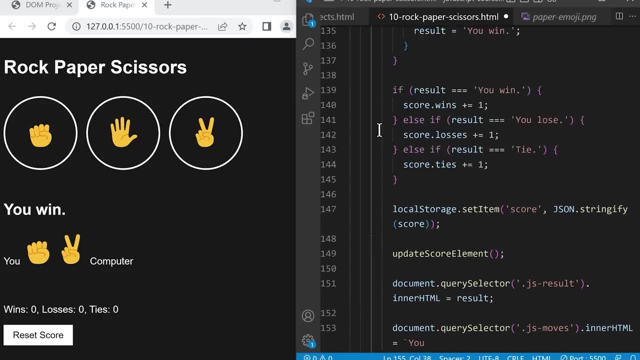 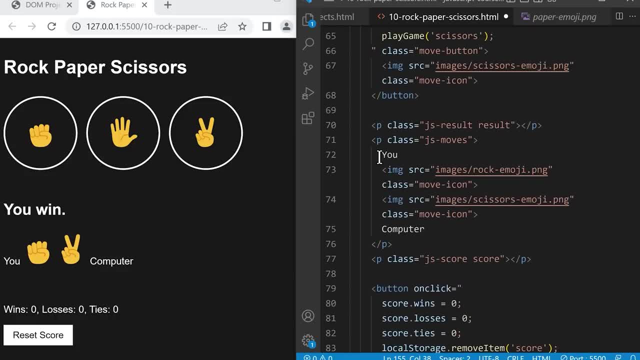 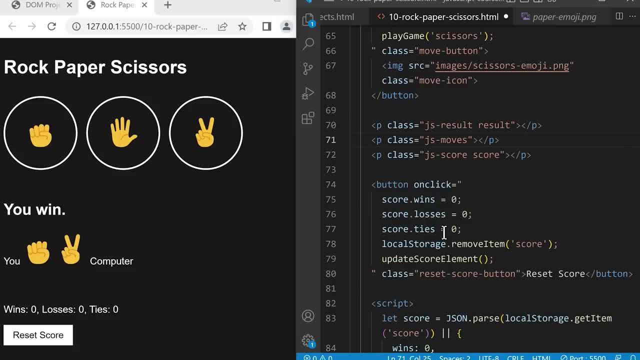 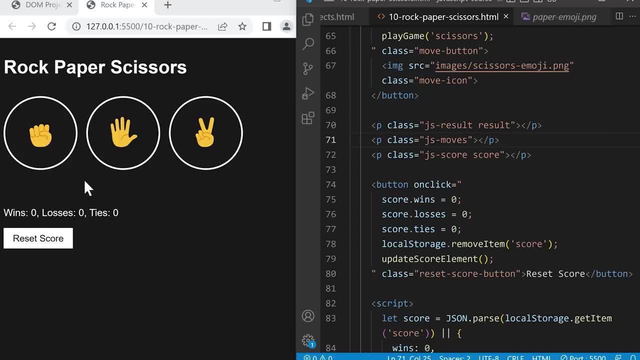 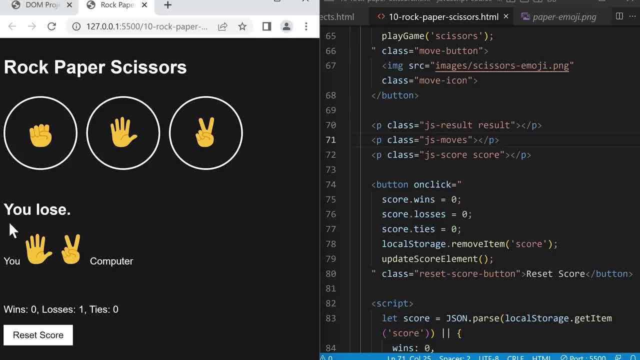 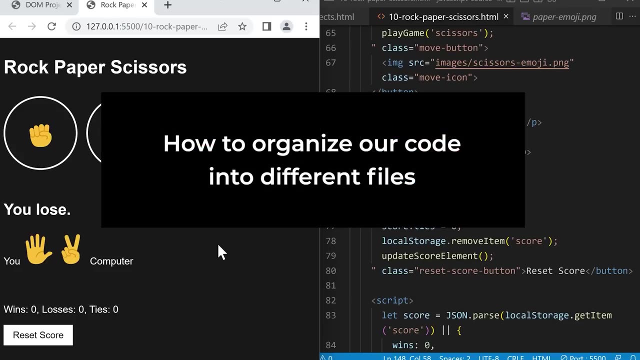 And when we click a move, it will show us the result and also show us the moves that we picked. And that's it. We finished the rock-paper-scissors project. The last thing we're going to learn in this lesson is how to organize our code into different files. 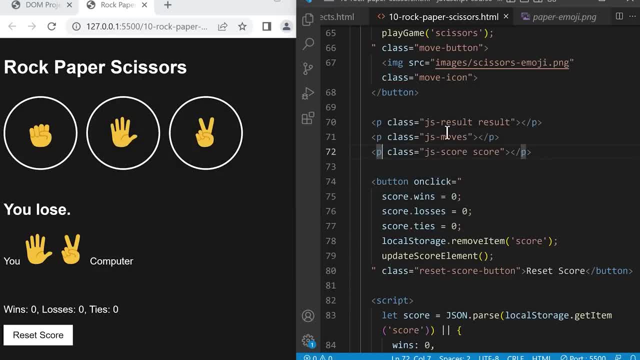 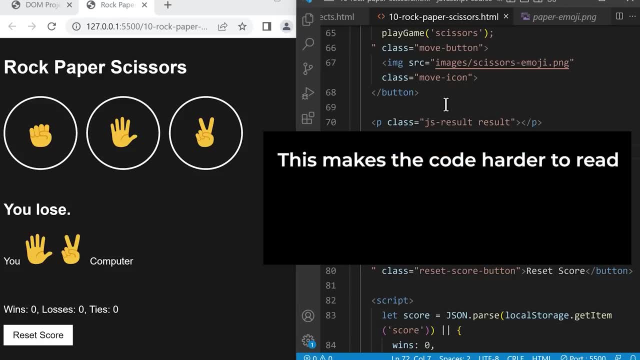 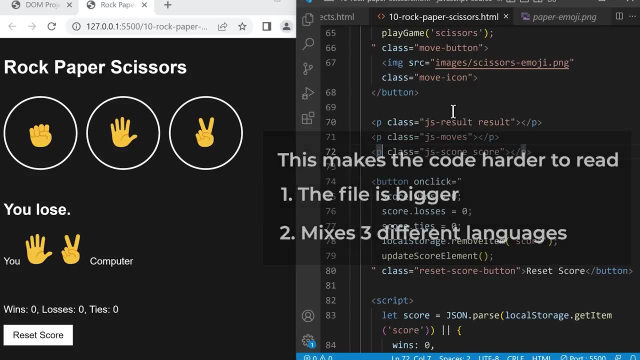 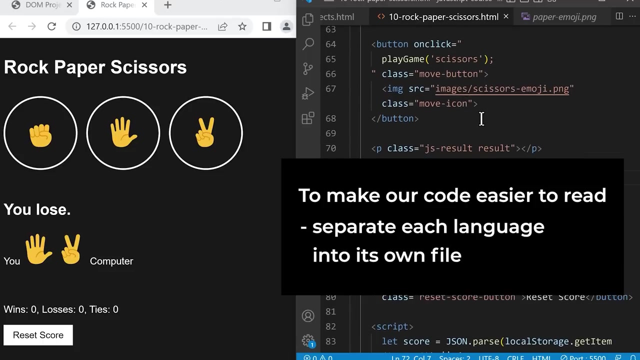 So notice that right now, all of our HTML, CSS and JavaScript is in one HTML file, And this makes the code harder to read, because the file is bigger and it mixes three different languages. To make our code more organized and easier to read, we're going to separate each language into its own file. 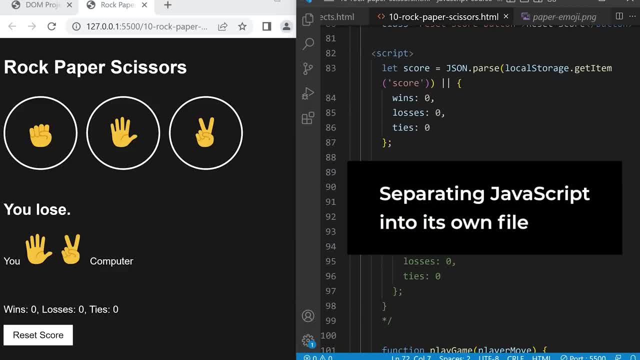 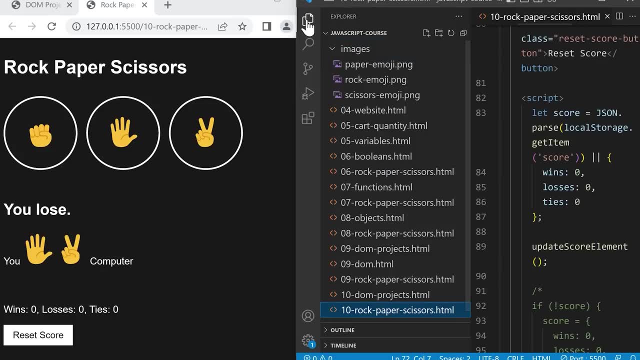 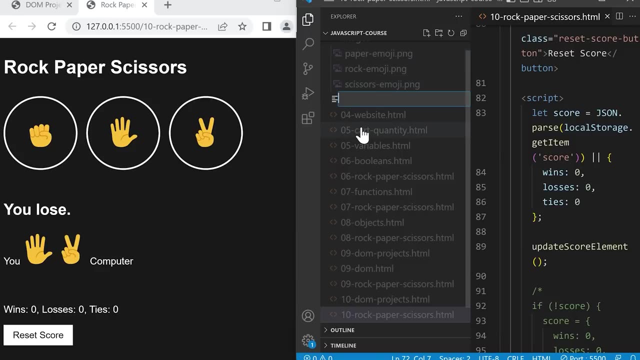 So let's scroll down and we'll start by separating our JavaScript into its own file. We'll click here to show our files And then click this, And then we'll click this icon to create a new file And we'll name this file 10-rock-paper-scissorsjs and press enter. 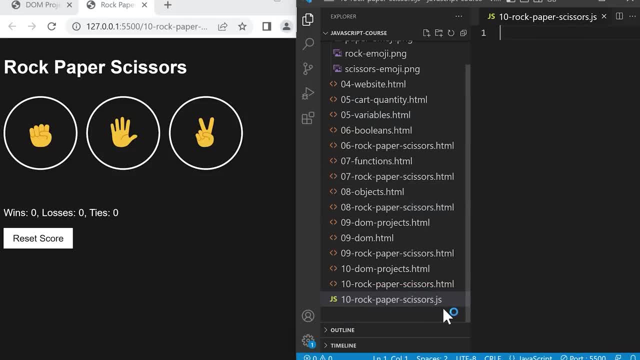 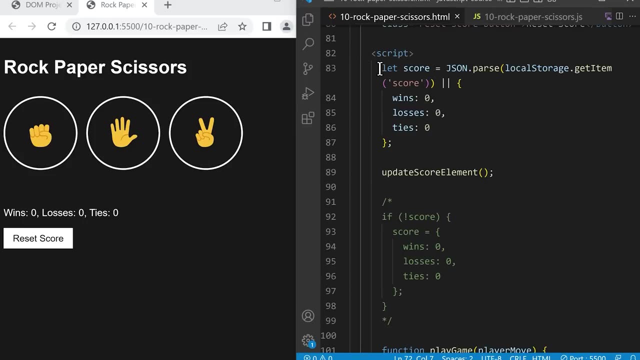 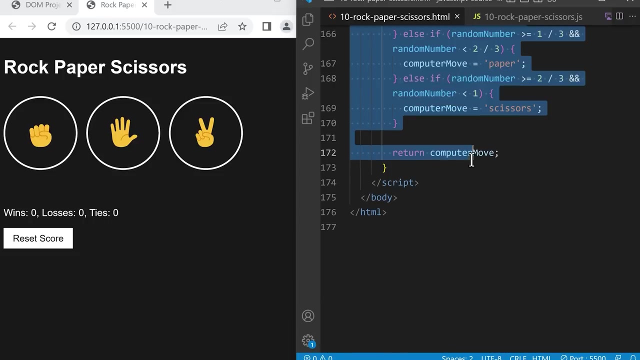 So when we end a file with js, it tells the computer that this file contains JavaScript code, not just text. Now let's go back to our HTML file and we're going to move all of this code into the JavaScript file. So we'll select this code and then we'll right-click and copy and inside the JavaScript file we'll right-click and paste. 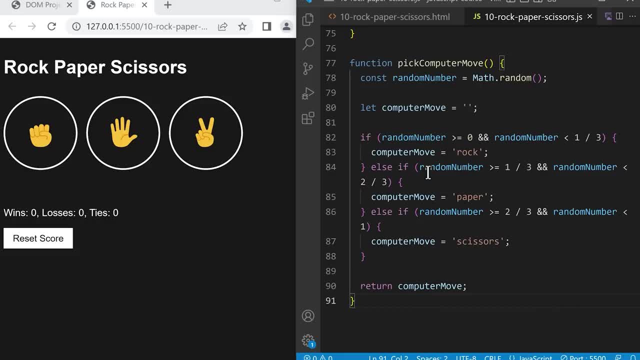 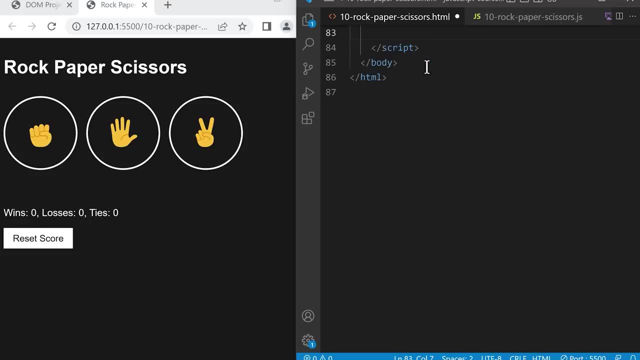 Now let's save And we'll go back to the HTML file And we can delete all this JavaScript code, And now we're just going to load our JavaScript file onto the webpage. To do that, we can use an attribute of the script element called src or source. 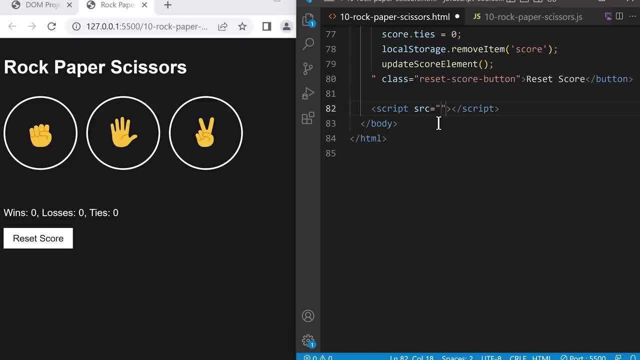 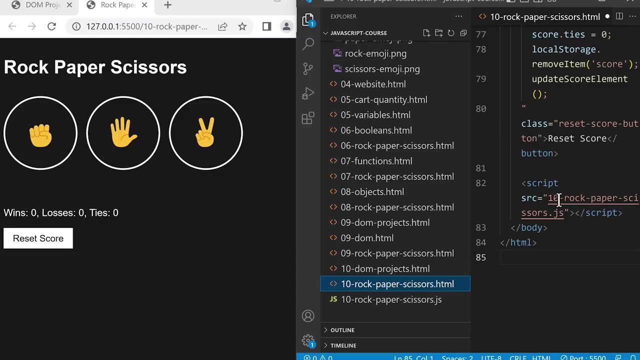 So we'll make it equal. And this Does the same thing as the image element. It tells the computer which file to load. If we type 10-rock-paper-scissorsjs, this will look for a file called 10-rock-paper-scissorsjs beside our HTML file, which is this file here? 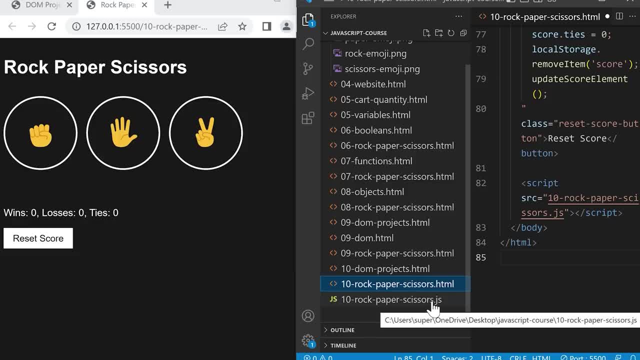 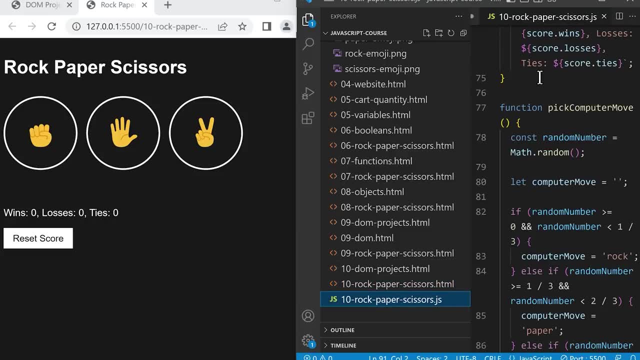 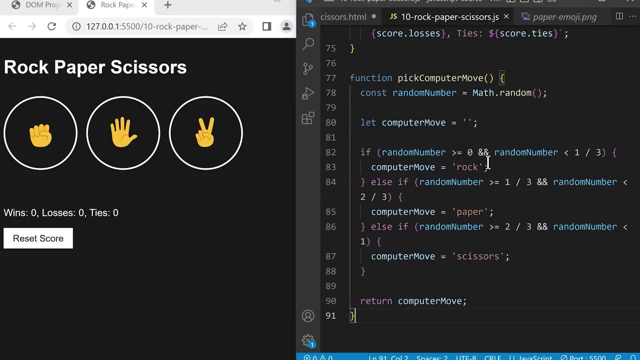 And it will run all the JavaScript Inside this file. So it does the same thing as before, except now our JavaScript code is in its own file, And this makes our code cleaner, Because each file only contains one language And each file also contains less code. 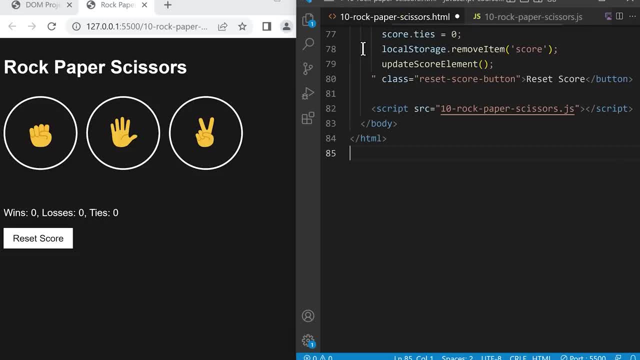 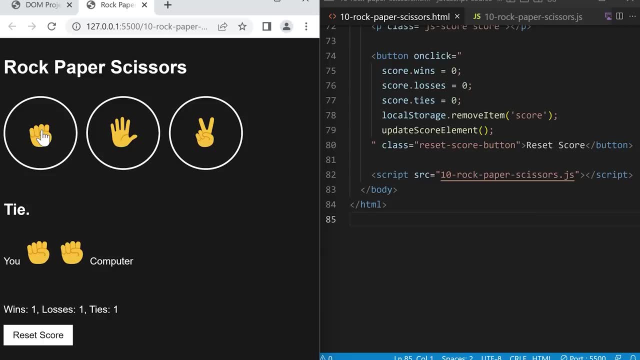 Now let's go back to the HTML file And save, And you'll notice that our project Works the same way as before. We just organized our code better. Another feature of the source attribute is that it also uses file paths, So we can put this JavaScript file in a folder. 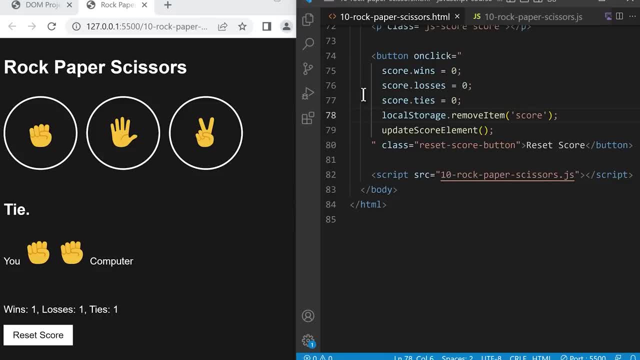 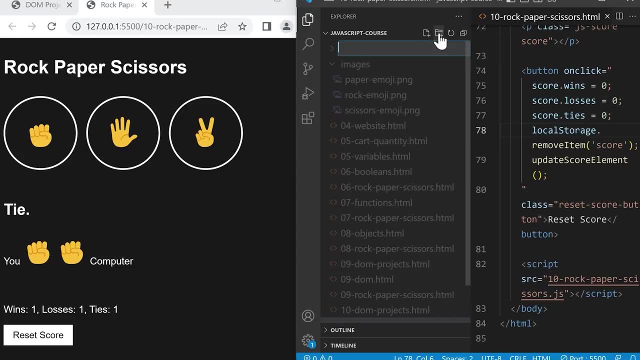 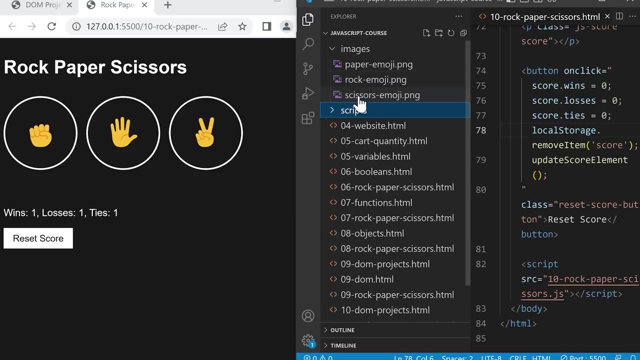 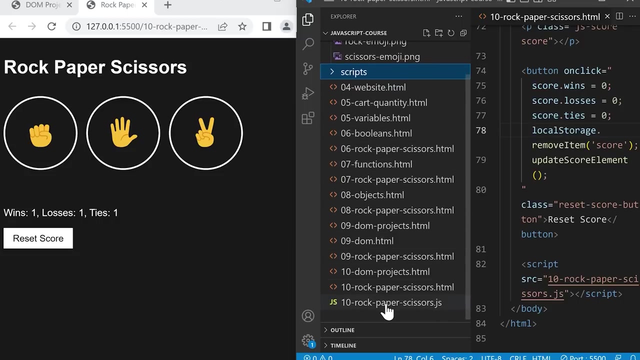 And we'll be able to find it. For example, let's show our files And let's create a new folder by clicking this icon And let's name this folder Scripts, So this folder will contain all of our JS files, So we can drag this file into the folder. 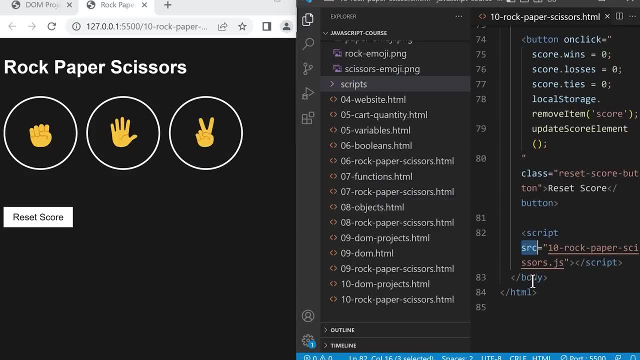 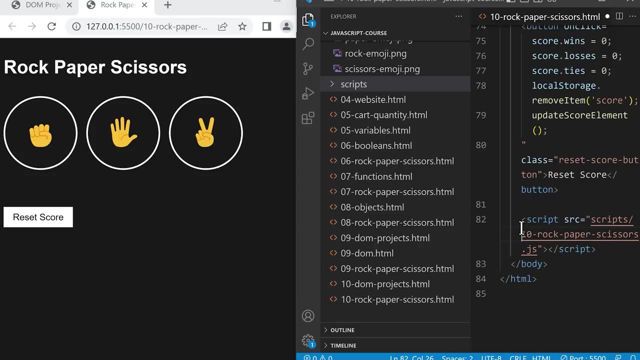 And now we can locate it using the source attribute By typing the folder name, which is scripts, And then a slash To go inside this folder and look for this file, And it will find this folder And it will find it right here. 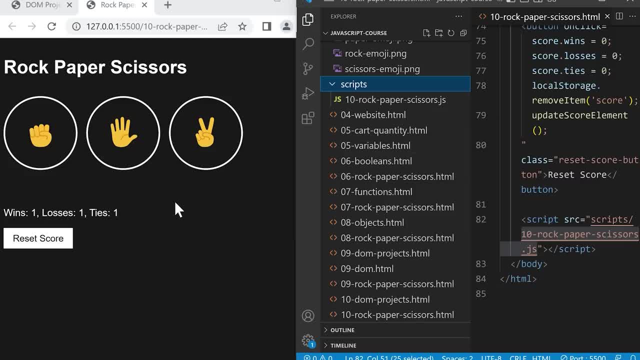 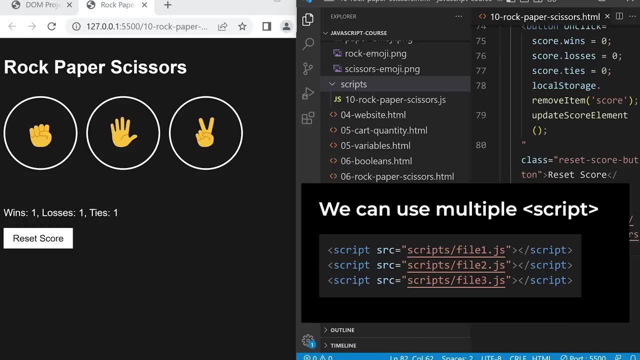 If we save, Everything works as normal. Another feature is we can use multiple script elements. This lets us split our JavaScript into multiple files And then load them all onto the page From top to bottom. Next we're going to learn how to separate our CSS. 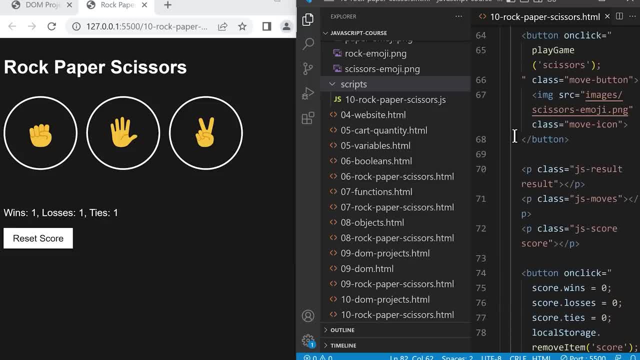 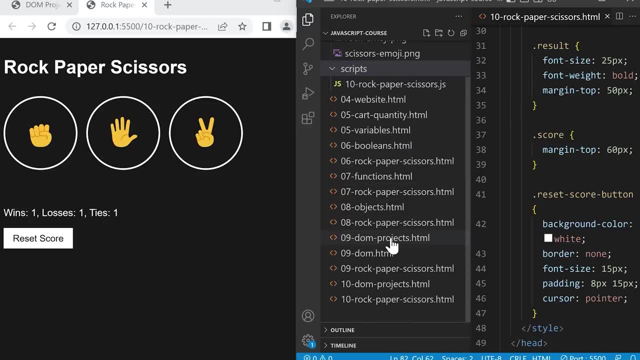 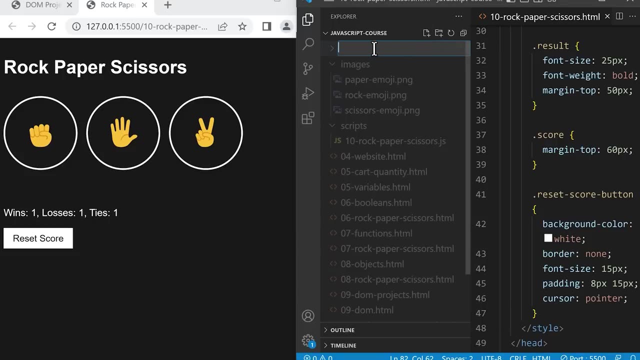 Into its own file. Let's scroll up to our CSS So we can do the same thing with CSS. So let's click the HTML file And let's create a new folder, And we'll call this folder Styles, And press enter. 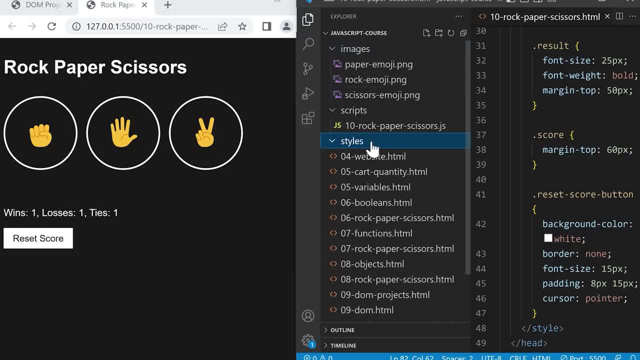 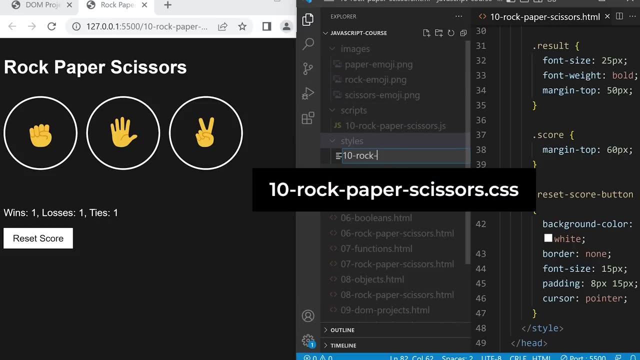 So this folder will contain all of our CSS code. Let's click the folder And we'll create a new file. And we'll create a new file By clicking this icon And let's name this file: 10-rock-paper-scissorscss. 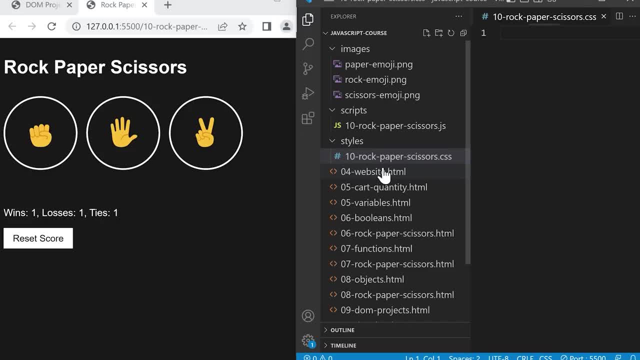 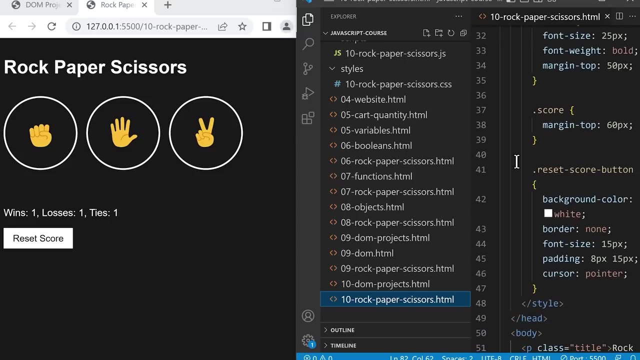 And press enter. So ending the file with css Means this file contains CSS code And now we can go back to our HTML And move our CSS Into its own file. So let's select all this code And then right click. 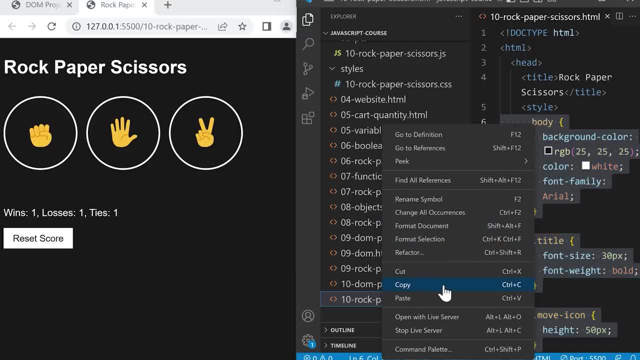 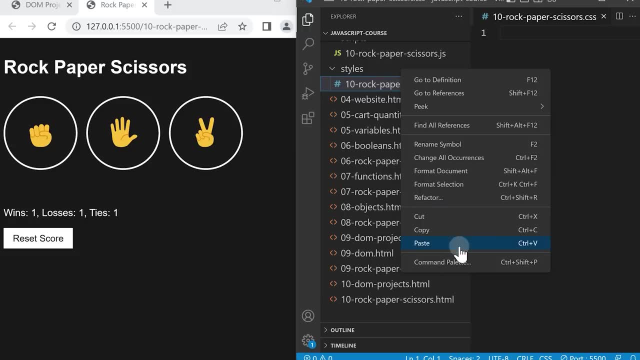 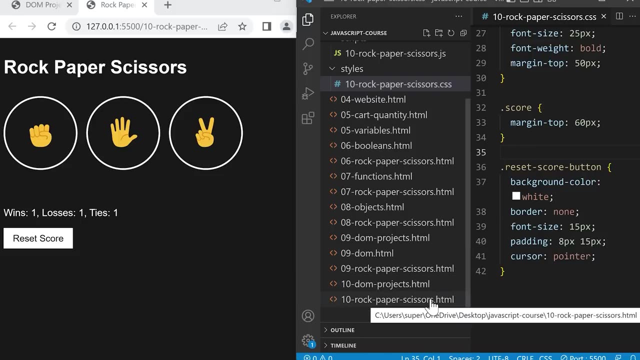 Copy And in here Right click And paste And save this file And save this file. And save this file. Now let's go back to our HTML. Now let's go back to our HTML And we can remove this code. 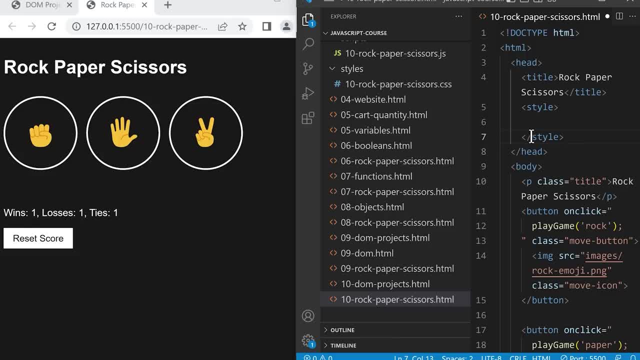 And we can remove this code And we'll learn how to load our CSS file. And we'll learn how to load our CSS file Onto our website. So we're not going to use the style element for this. So we're not going to use the style element for this. 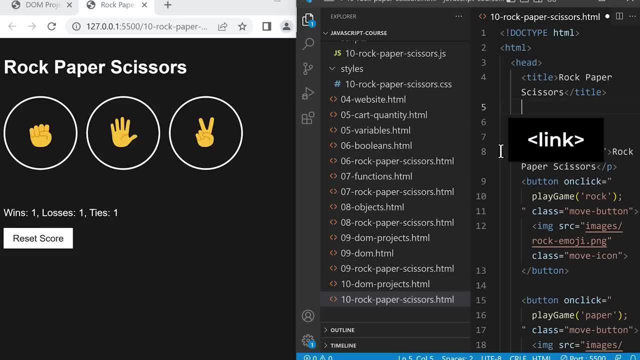 We're going to use a different element Called the link element, So we'll type Less than Link, Greater than, And the link element doesn't require a closing tag. This is another void element. This is another void element. This element uses two attributes. 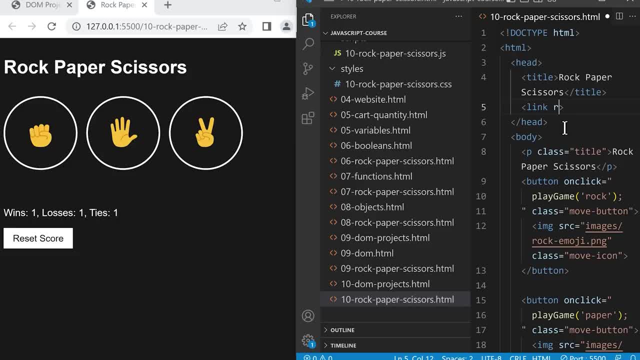 The first attribute Is called R-E-L. R-E-L means Relation. This tells the computer what type of file We're loading. So we're going to set this attribute to Style sheet. This means we're loading a CSS file. 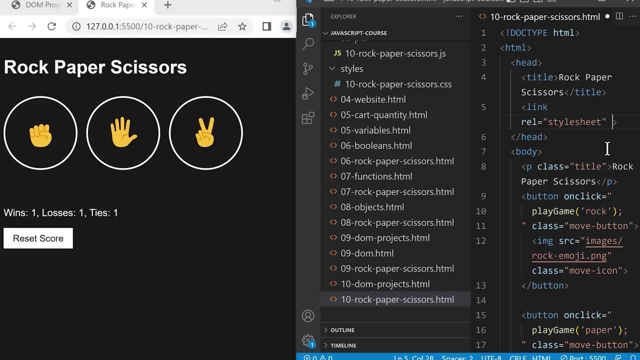 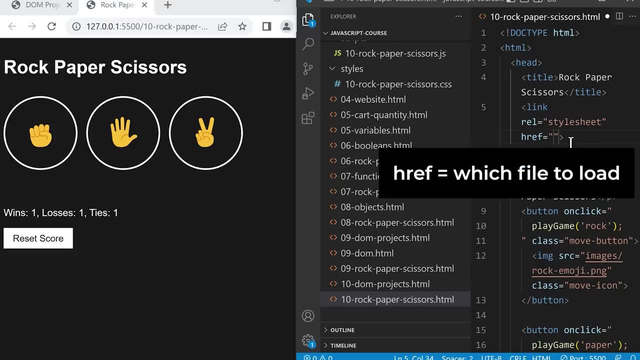 This means we're loading a CSS file And then we'll add a second attribute Called href. Called href, so href tells the computer which file we want to load. so this also supports file paths. so we can type the styles folder. this will look for a folder beside the html, called styles, which. 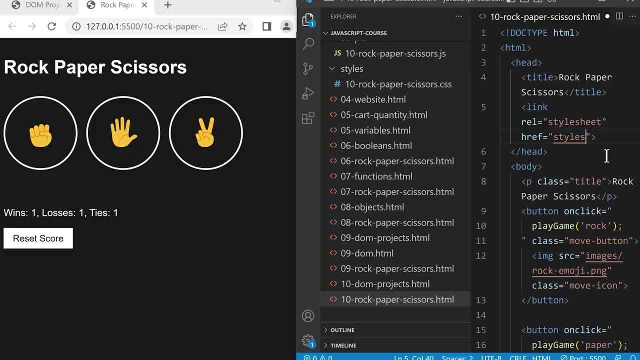 is this one right here, and then we'll type slash to go inside the folder and look for this css file, which is 10 dash rock, dash paper, dash scissors dot css. so this will load all the css inside this file and apply it to our page. so it does the same thing as before, except we separated each language. 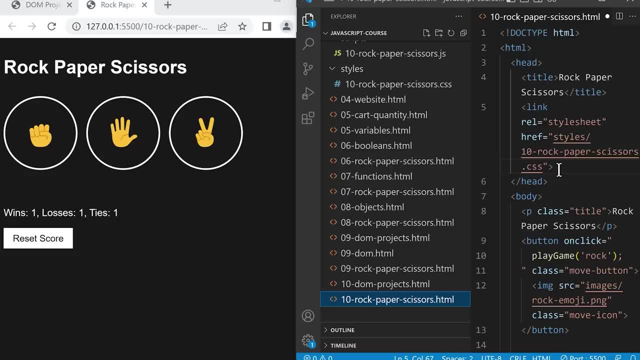 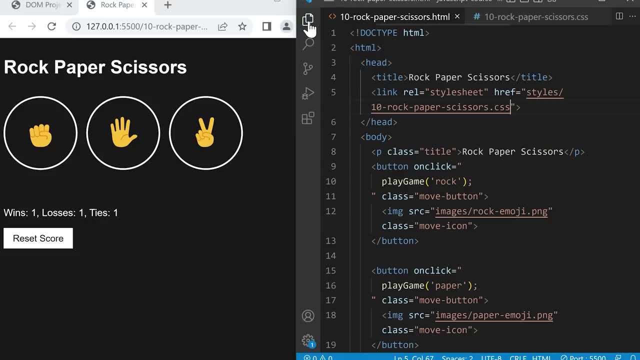 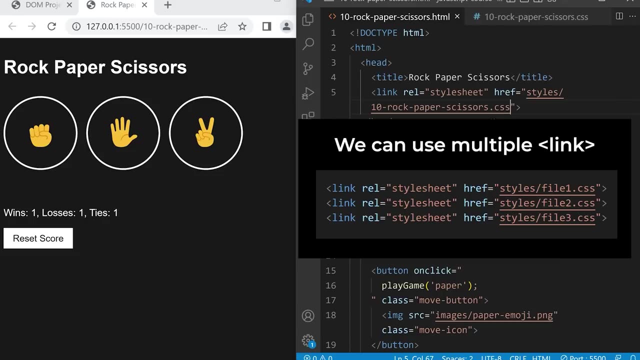 into its own file. if we save, everything still works. you can also use multiple link elements to load multiple css files and all the styles get applied. and just like the script element, we can also use multiple link elements to load multiple css files. so that's how we separate our code into separate files. 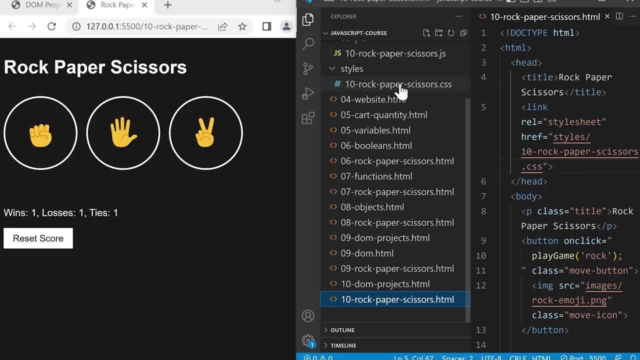 using the script element and the link element. it makes our code a lot easier to read, because each file contains one language and it contains less code. and that's the end of our給feldt-sthod test And that's the end of this lesson. 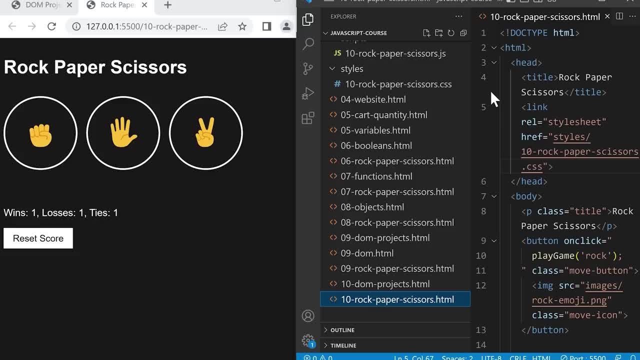 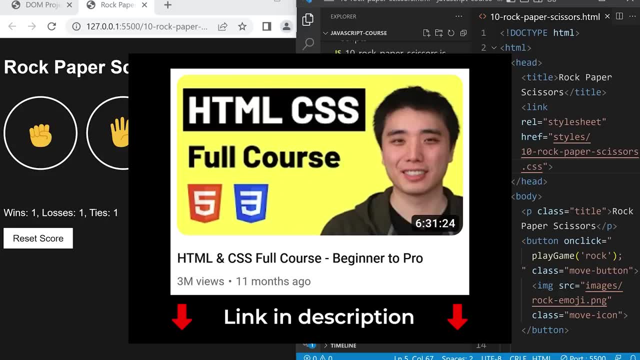 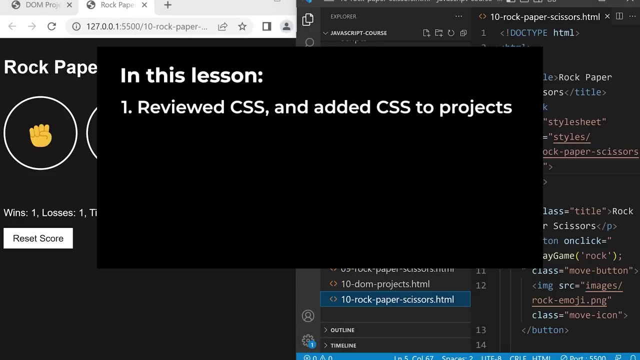 As a final reminder, the CSS we learned in this lesson is just a review. If you want to learn CSS in more detail, you can check out my HTML and CSS full course in the video description. So in this lesson we reviewed CSS and added CSS to all of our projects. 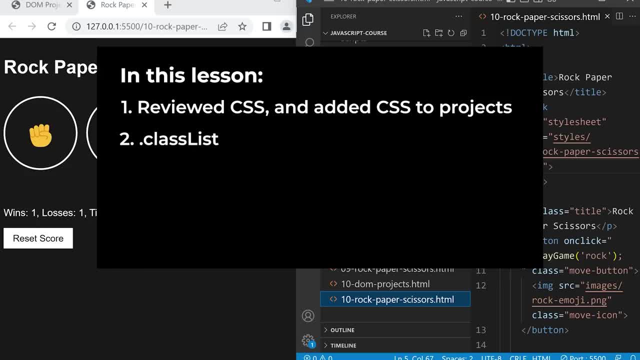 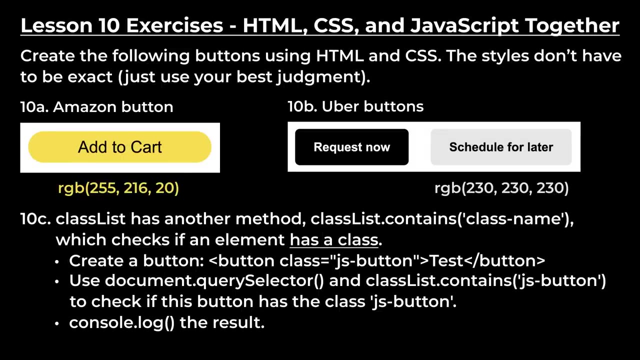 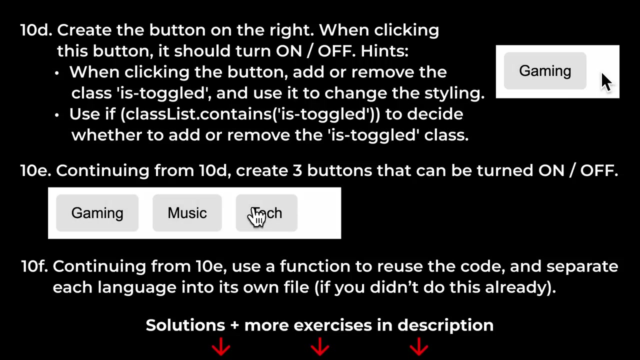 We learned about the class list property, which lets us control the class attribute of an element. We finished our rock-paper-scissors project and we learned how to organize our JavaScript and CSS code into separate files. Here are some exercises to help you practice using HTML, CSS and JavaScript together. 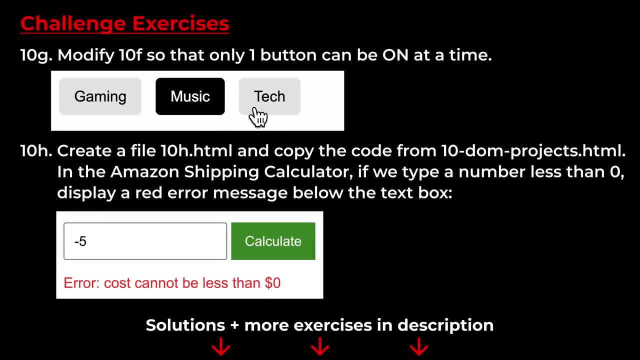 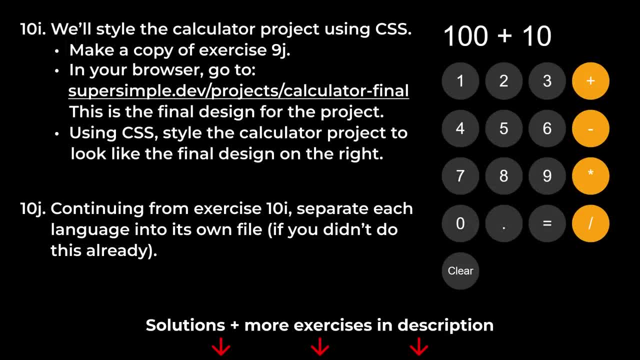 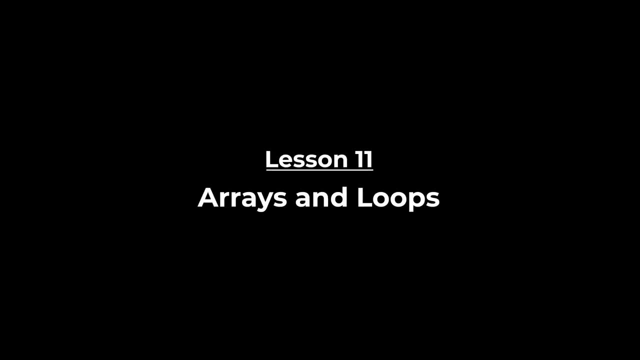 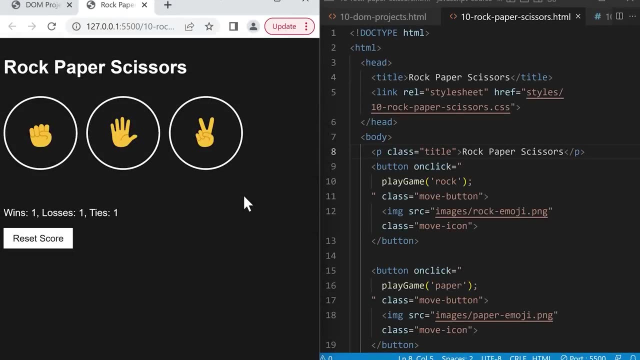 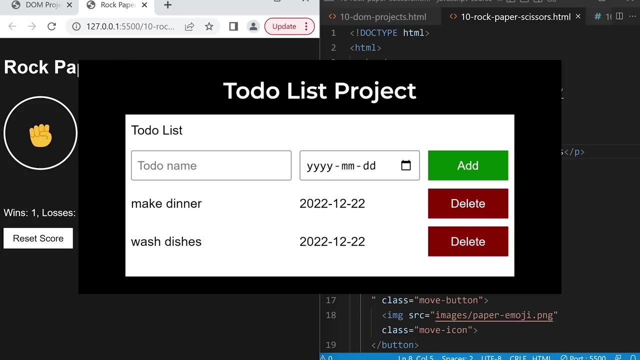 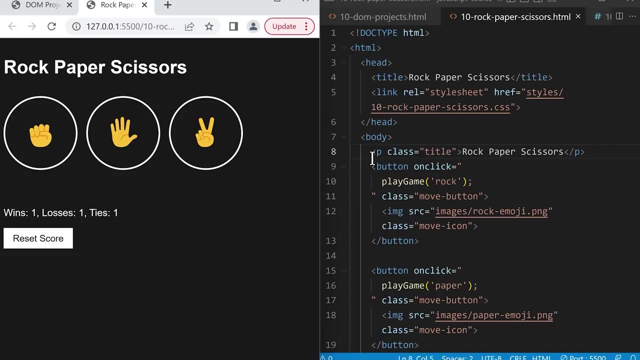 In this lesson, we're going to learn two more features of JavaScript called Arrays and Loops, And we're going to use these features to create this script. First, let's create a new file for this lesson. We'll go to our code editor and click up here to show our files. 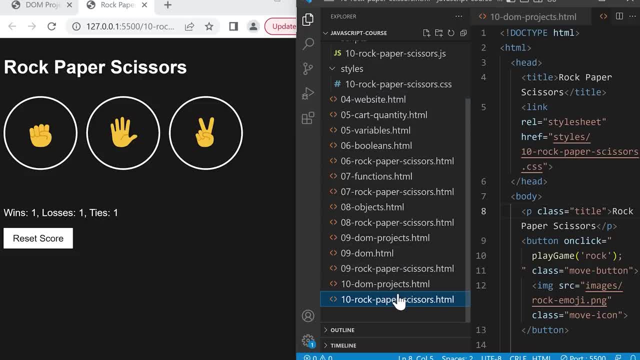 And this time make sure you have one of these HTML files selected so we don't create the new file in one of these folders. So now we're going to click this icon to create a new file and we're going to name this file. 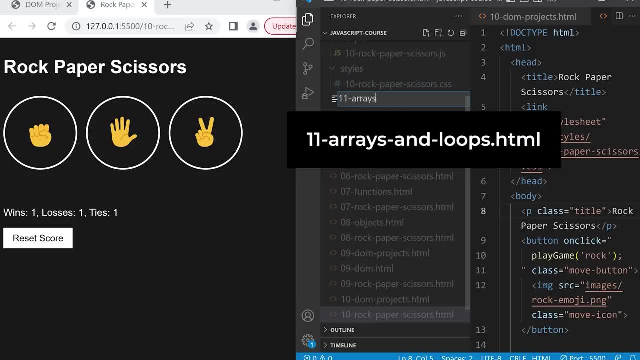 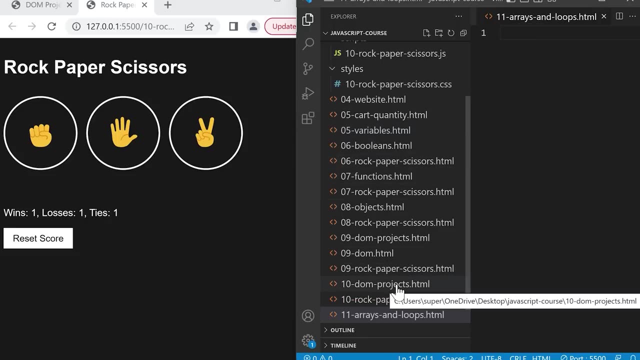 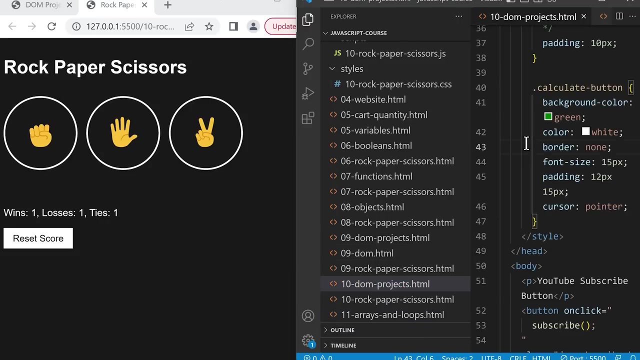 11-arrays-and-loopshtml and press enter. Now let's copy the previous lesson into this file. So we'll click on 10 DOM projects and we'll type here and type Ctrl A or Command A to select the code. 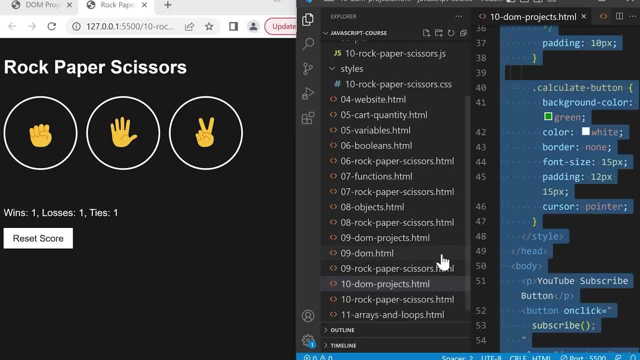 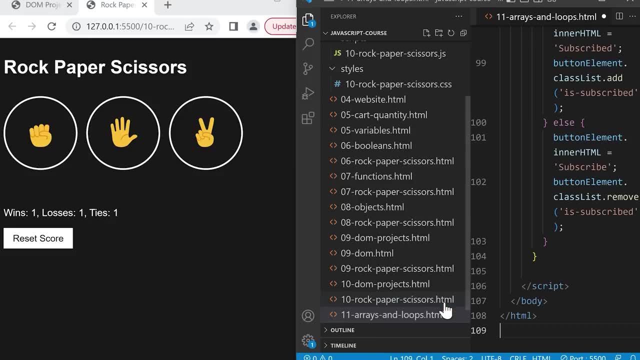 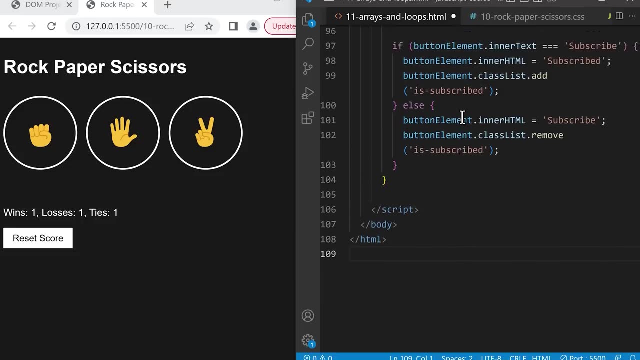 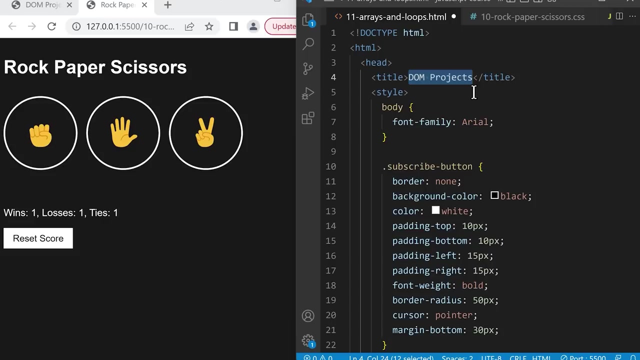 And then right-click copy and in here, right-click and paste. Now let's hide our files and we'll prepare this file for this lesson. So we can scroll to the top and we'll change the title to Arrays and Loops. 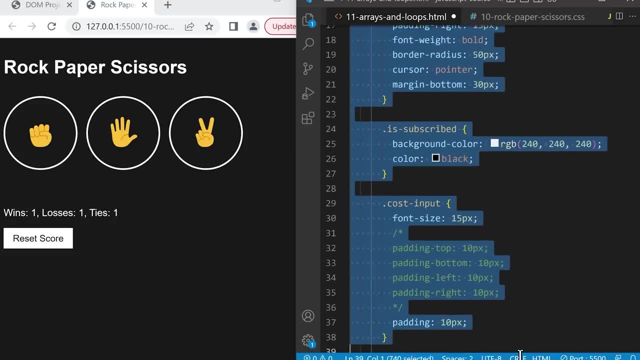 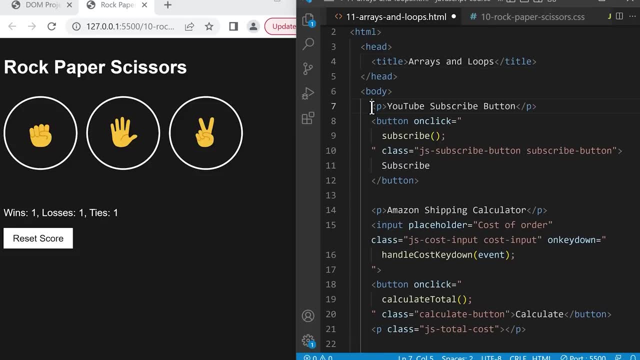 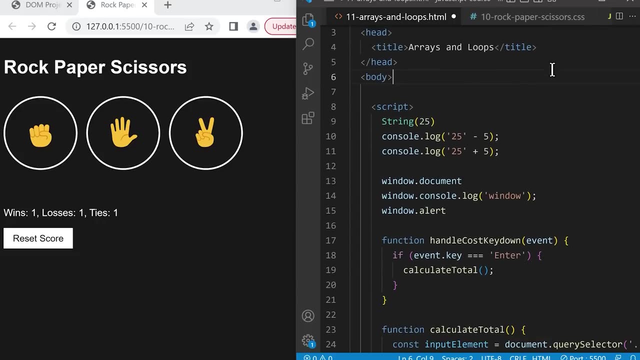 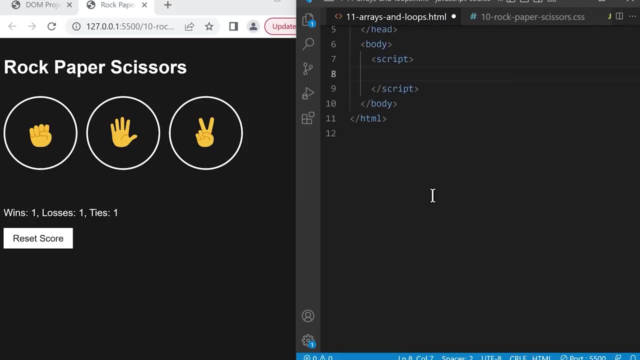 And let's remove all of the CSS, And we'll also remove the HTML, which is right here, And we'll remove all the JavaScript. Now let's save And we'll open this file in the browser. In the browser, by right-clicking. open with Live Server. 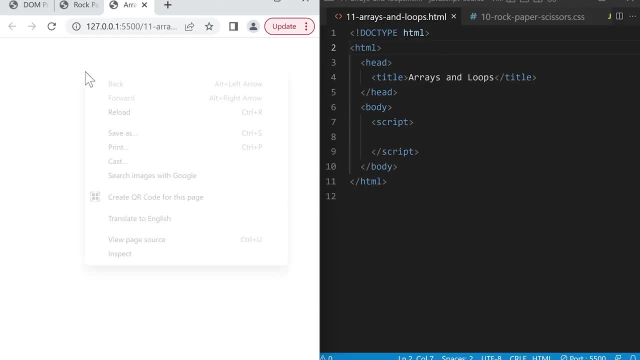 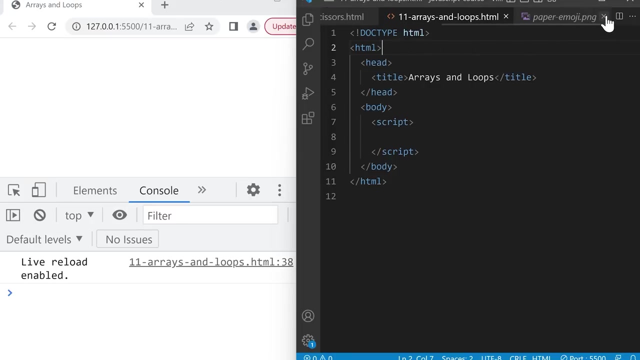 And let's also open the console. So we'll right-click, click Inspect and click the console, And now we can close the previous tabs and the previous code for now, until we just have the lesson 11 file. Now we're ready to learn arrays. 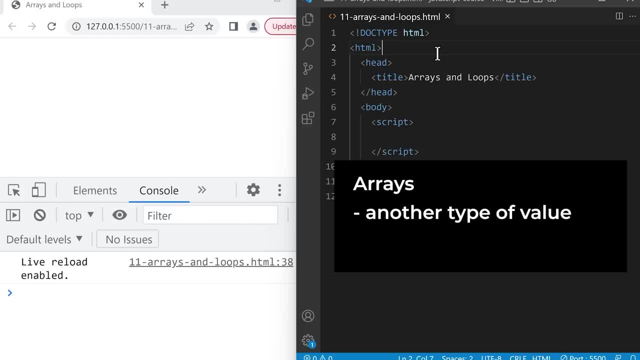 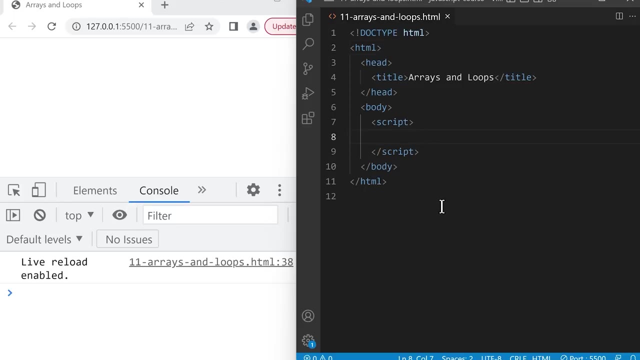 An array is another type of value in JavaScript And it represents a list of other values. So let's do an example and create our first array. We'll go into the script element and we're going to type open square bracket and closed square bracket. 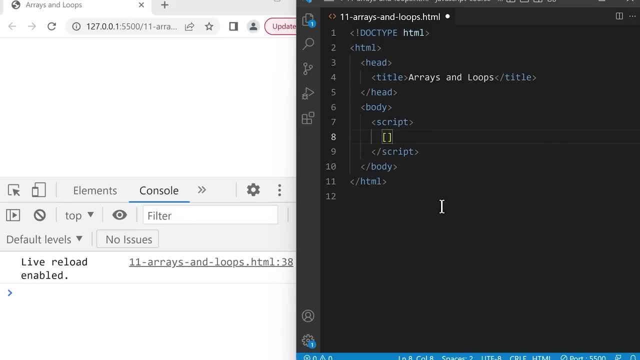 And inside the square brackets We'll type open square bracket. We'll type a value like the number 10.. And then we'll type comma and another value like the number 20.. And then comma again and a third value like the number 30.. 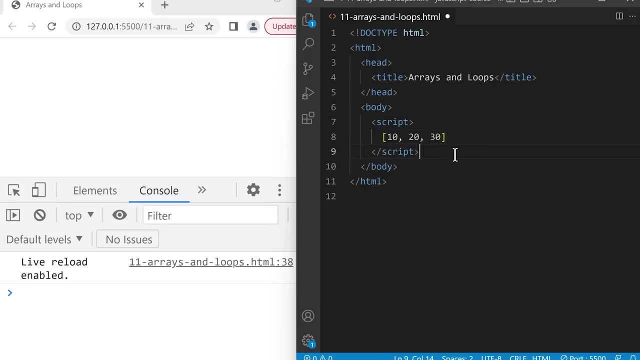 So this is an array And it represents a list of three numbers: 10,, 20, and 30.. Now arrays themselves are also arrays, So let's do an example. So we have a list of a number And there are also values, which means we can save them in a variable. 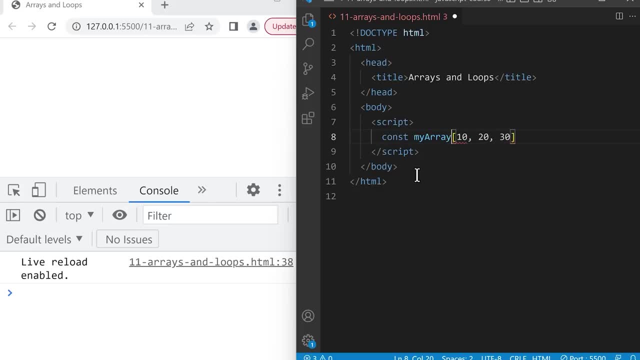 So at the front we can create a variable using const and let's name it myArray, And we'll make it equal to this array And we'll add a semicolon at the end. So now we created a list of values. 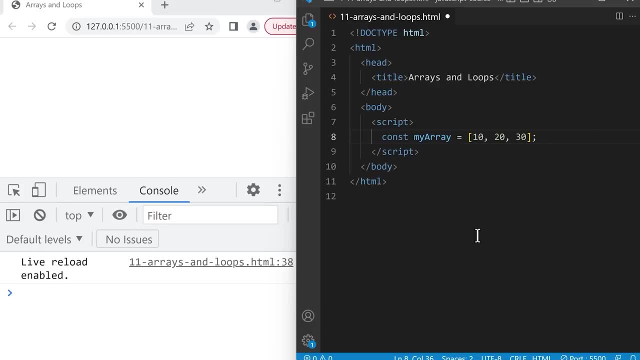 And we saved this list in this variable. Let's create a new line and we'll consolelog myArray and save And it will display the list of values in the console. So that's basically what an array is: It's a list of values. 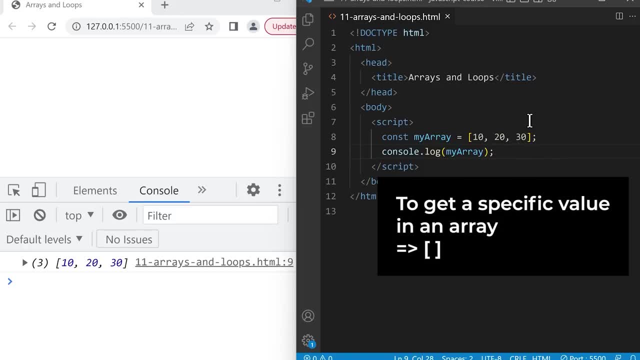 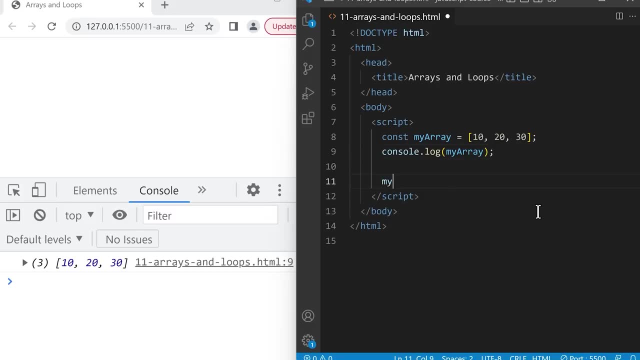 Now, to get a specific value in an array, we can use square brackets. So let's create a new line and we'll type myArray and square brackets. Inside these brackets we'll put a number like 0.. This number represents the position in the array. 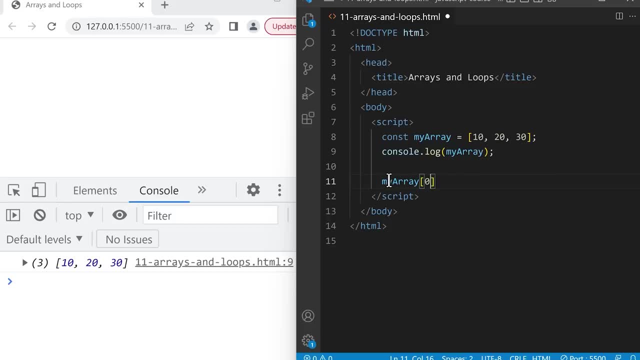 So 0 means the first value. If we consolelog this code and save myArray square bracket 0, gives us the first value, which is 10.. And that's what's displayed in the console. Now, if we change this to 1,, 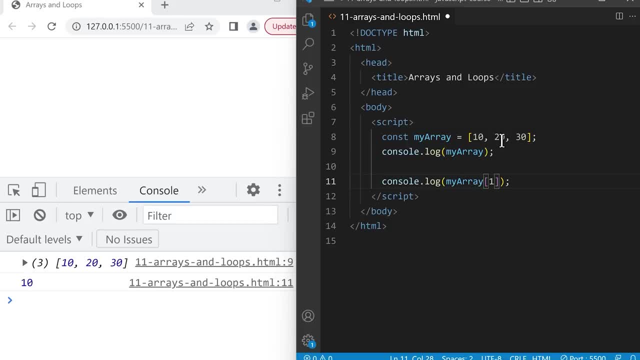 this will get us the second value in the array, which is 20.. If we save, it displays 20.. So this number represents the position In the array. 0 is the first value, 1 is the second value, 2 is the third value, and so on. 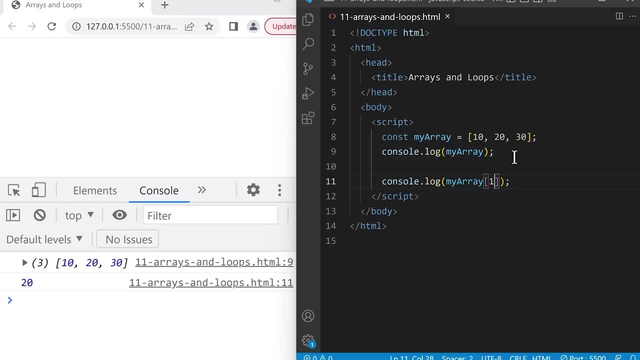 We can also change a value in an array, also using square brackets. So let's create a new line and we'll type myArray- square brackets. And let's say we want to change the first value. So we'll type 0 for the first value and we just make it equal to something else like 99.. 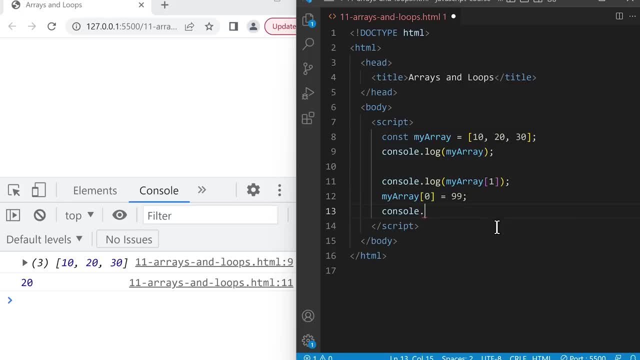 Now, if we consolelog myArray again and save, you can see that this changed the first value to 99.. So that's basically how arrays work: We can access a value inside an array and we can also change a value inside an array. 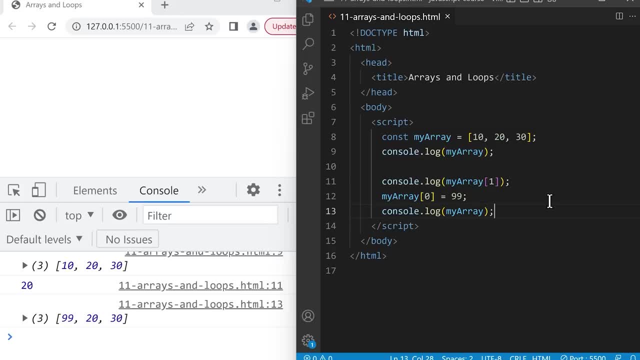 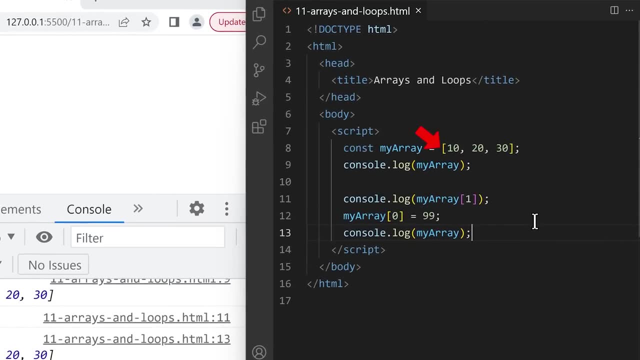 Now that we understand the basics of arrays, let's learn the syntax rules. To create an array, we start with an open square bracket and we end with a closed square bracket. Inside we can put a list of values and we separate each value with a comma. 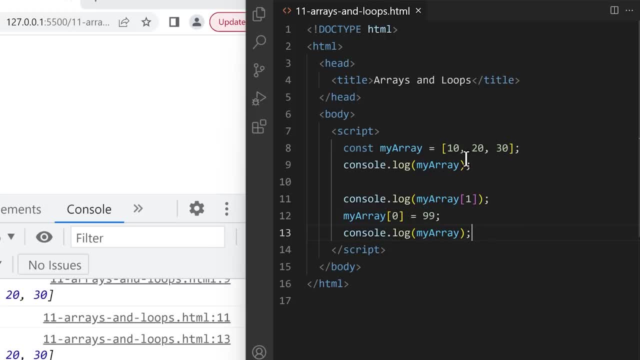 We can also write an array on multiple lines like this: We just put the new lines after the comma. Now, to get a value inside an array, we can use square brackets and a number like 1.. This number is called the index. 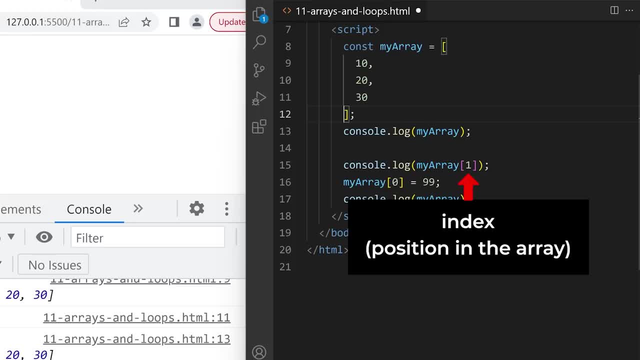 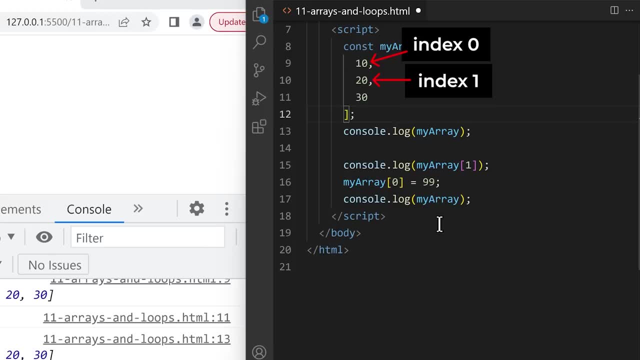 It represents the position in the array that we want to get. So the first value is index 0.. The second value is index 1.. Third value is index 2, and so on. Notice that the index starts as 0.. This is called a zero-indexed array. 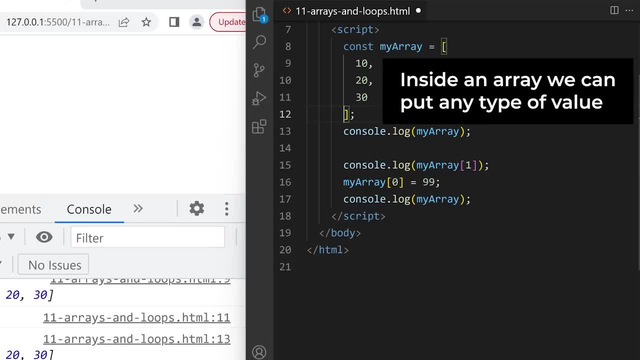 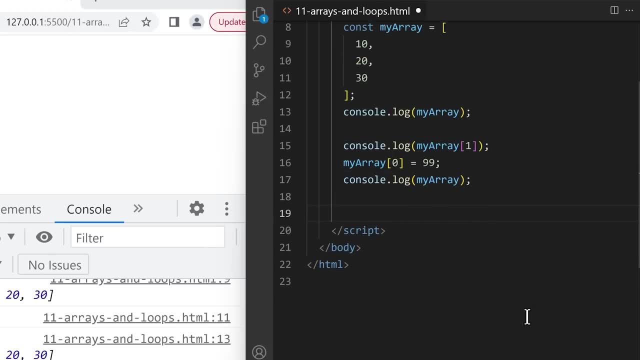 Now, inside an array, we can put any type of value. For example, let's create a new line and we'll create a new array using square brackets, and inside We can put the number 1, and then comma, and we can also put a string like hello. 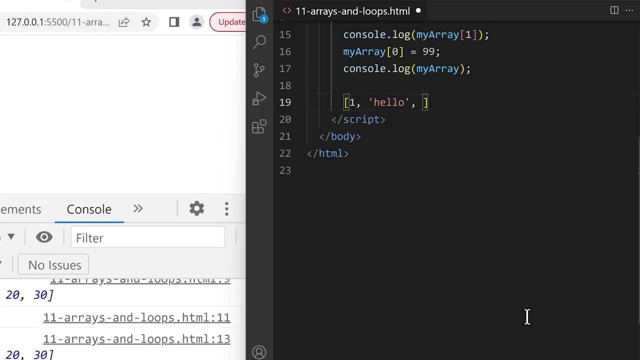 and another comma, and we can put a boolean value like true and another comma, and we can even put an object like curly brackets, name, colon, socks. Now an array itself is also a value. That means we can save arrays in variables like this, or even save it in an array. 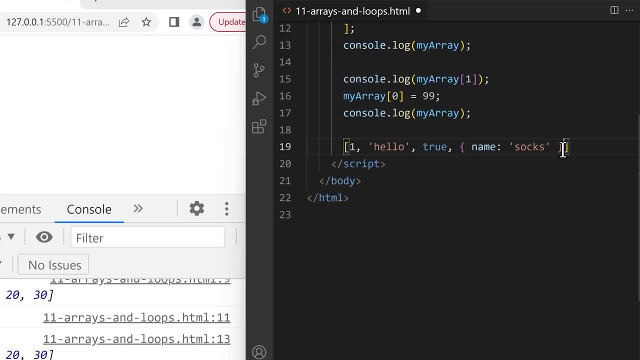 For example, in this array we can add an array inside like 1, comma 2.. Next, arrays have a weird behavior When we try to check the type of an array. So on a new line let's type consolelog type of, and then square brackets 1, comma 2,. 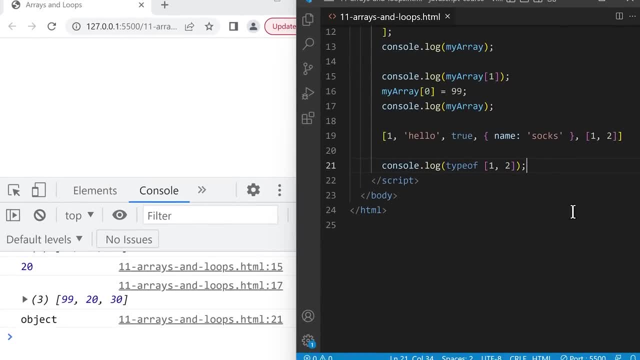 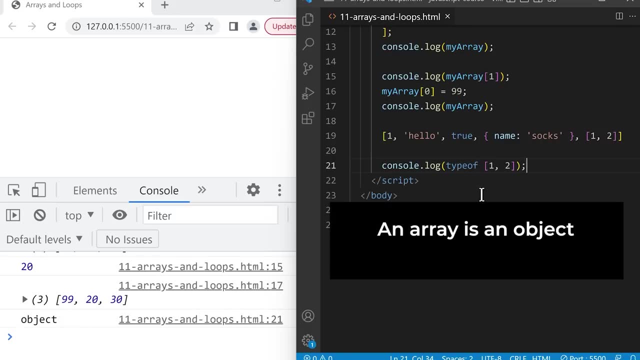 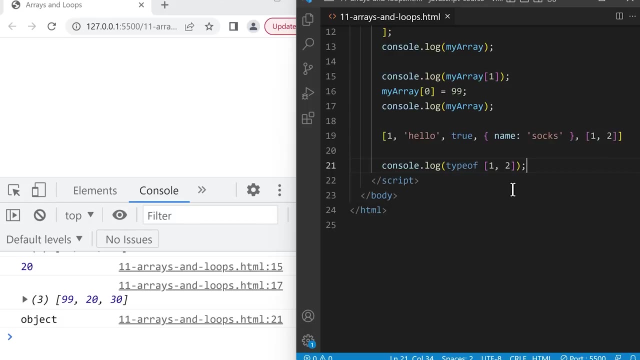 and save. This will tell us that an array is an object, And that's because an array is actually an object, But it's just a special type of object. If we want to check if something is specifically an array, we can use this code. 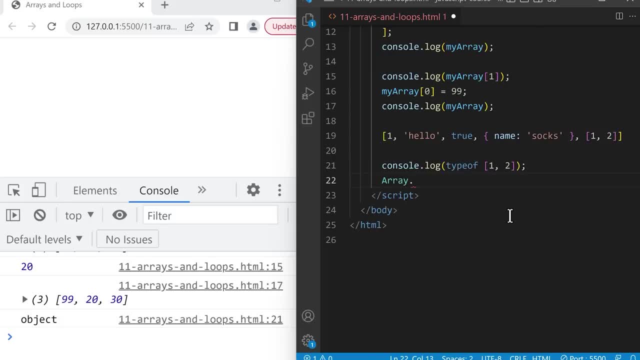 Capital. A array dot is array brackets And inside the brackets we'll put an array, like square brackets 1, comma 2.. So this will check If this value is an array. If we consolelog this result and save, it will display true. 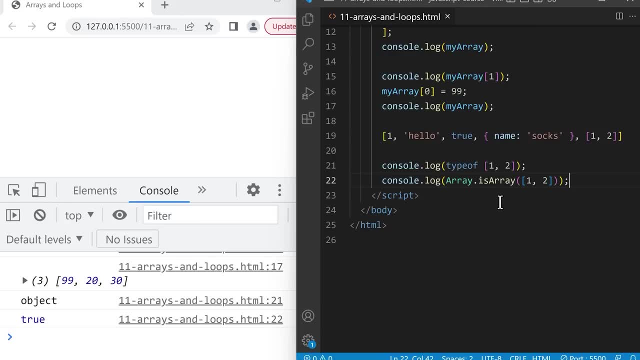 And finally, because arrays are just a type of object, they also have properties and methods we can use. So one useful property is called dot length. So we'll type console dot log my array dot length. This will tell us how many values are in the array. 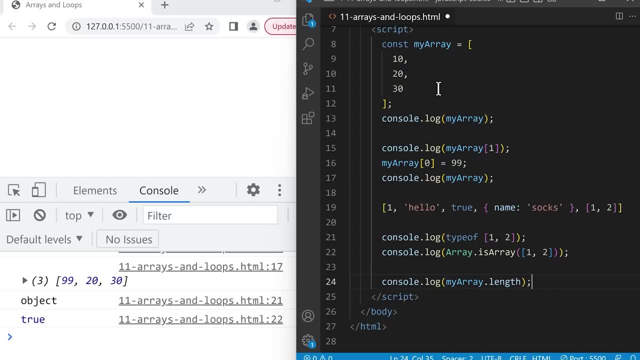 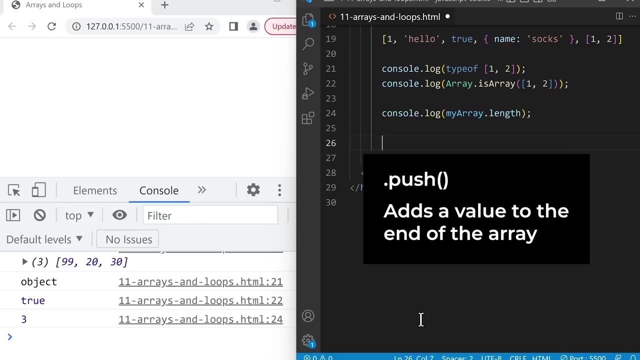 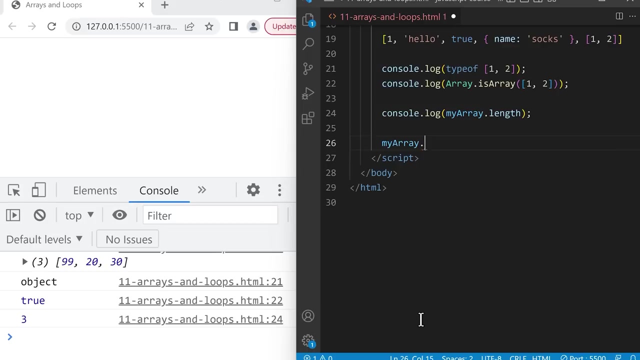 So my array has three values, So if we save it will display three. Next we'll learn a useful method of an array Called dot push. This adds a value to the end of the array. If we did my array dot push 100, this will add 100 to the end of my array. 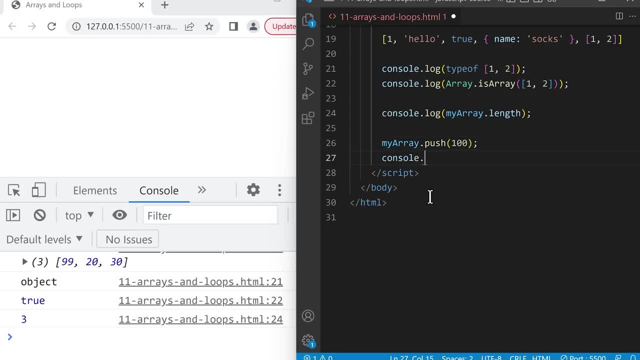 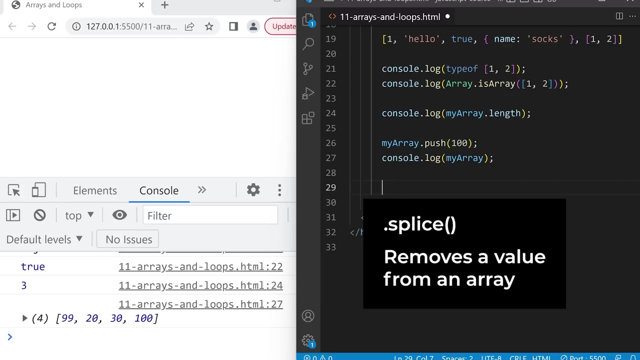 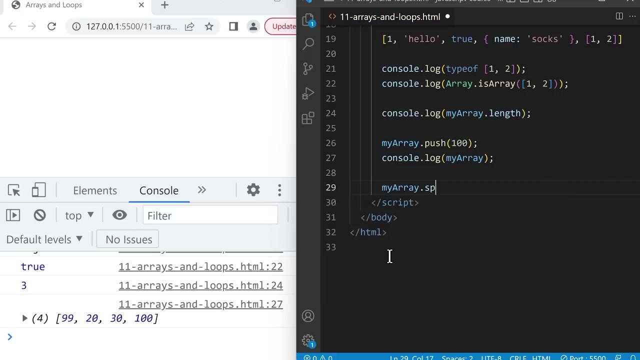 If we console dot, log my array And save, You can see that 100 was added at the end. The last method we're going to learn for now is called dot splice. This removes a value from an array, For example, my array. dot splice and brackets, and a splice takes two numbers. 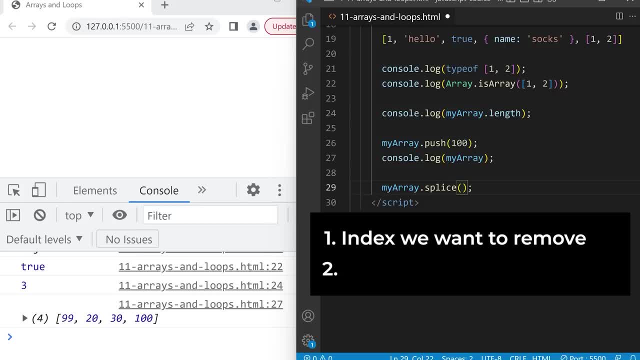 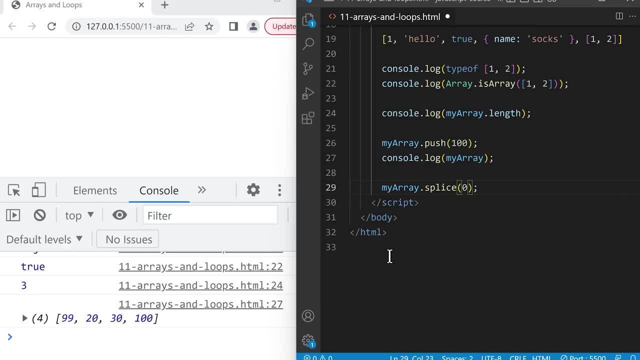 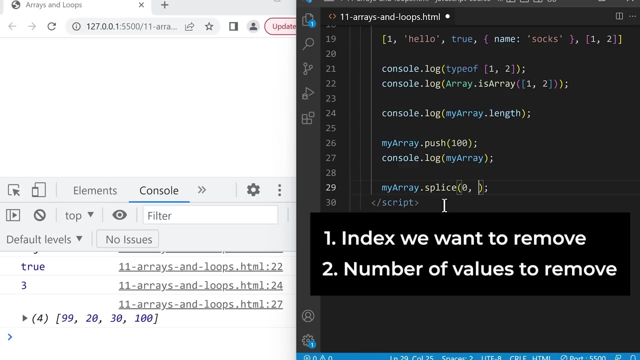 The first number is the index that we want to remove. So let's say we want to remove the first value, which is index 0.. The second number we give to splice is the number of values we want to remove. If we give it 1, it will remove one value at index 0. 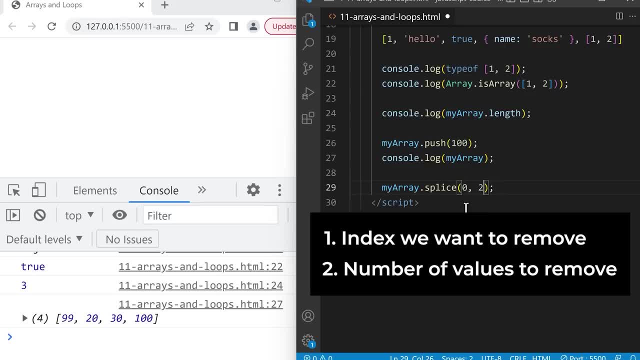 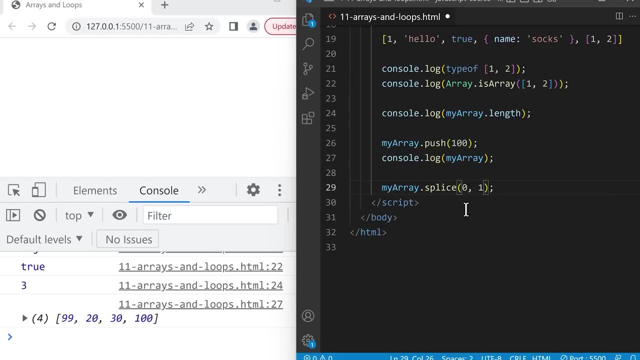 If we give it 2, it will remove two values, starting at index 0.. So for now, let's just remove one value And let's create a new line and console dot, log my array and save. You can see that splice removed the first value from the array, or index 0,, which was 99. 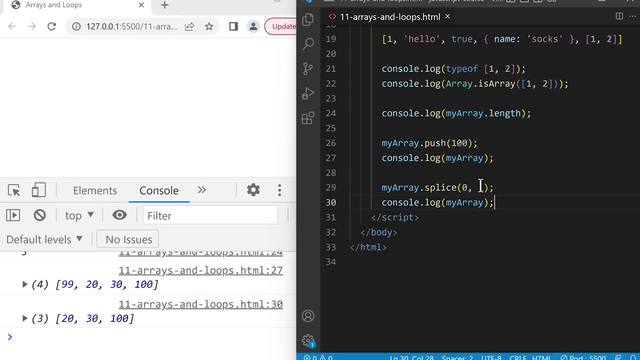 All right, Now that we understand the basics of splice, Let's move on to the next step, To understand the basics of arrays and the syntax rules. let's do some practical examples. So I've prepared a project we can do for this lesson. 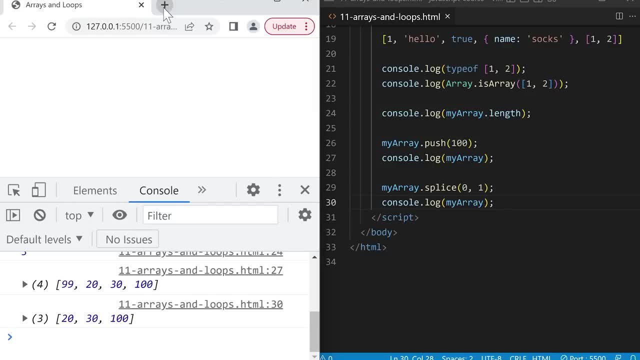 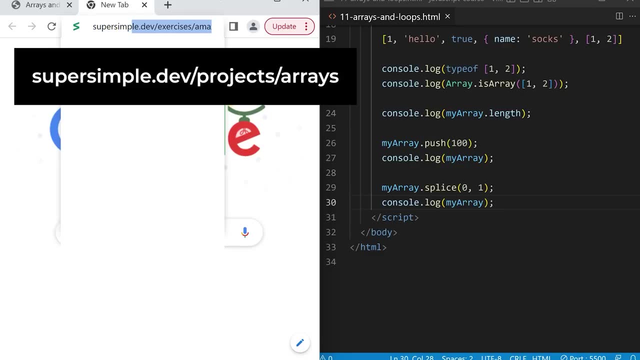 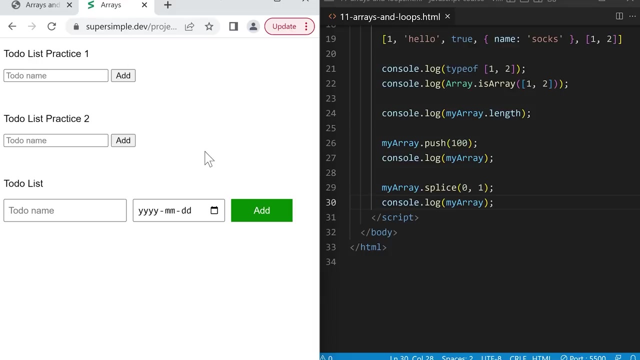 We'll go to our browser, create a new tab at the top And here we'll type super simple: dot, dev, slash projects, slash arrays, Then press enter. So this page contains the to-do list project we're going to create in this lesson. 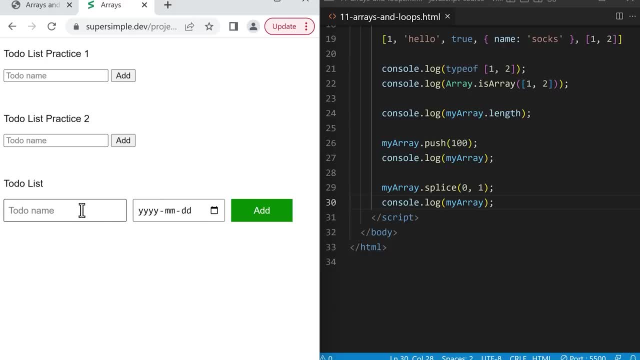 So down here is the final version of the project. We can type a name for our to-do, like make dinner, Give it a due date, And then click add And it will add it to our list. We can add another to-do. 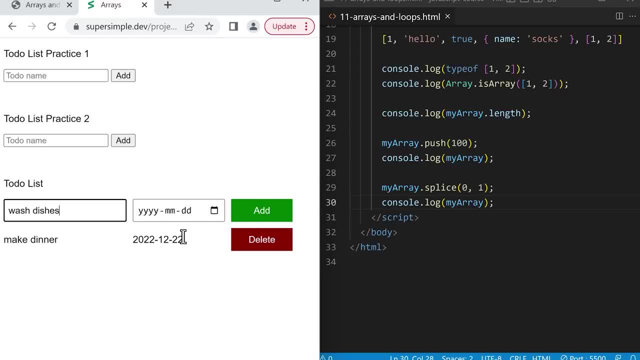 Like wash dishes, And then select a due date And click add again And it will add another to-do to our list And each to-do also has a delete button So we can delete it when we're finished the task. So this is the final version of the project. 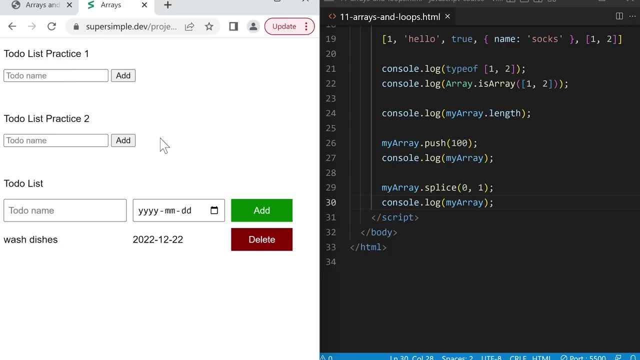 And these two up here are simpler versions of the project that we're going to use to work our way through. So let's start with the first project up here. We're going to open our console by right clicking, Click inspect And click the console. 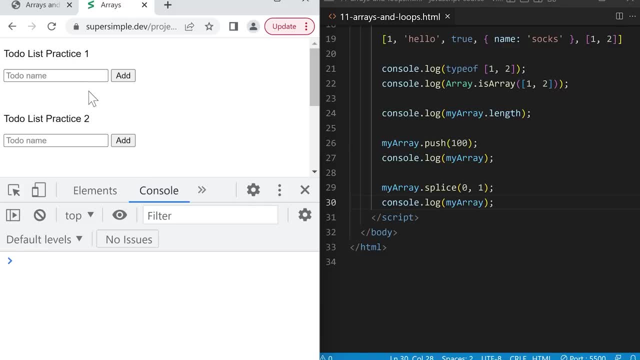 And the way this first project works is we can type a to-do in this text box, Like make dinner, And when we click add, It will add the to-do to an array And display it in the console If we type another to-do. 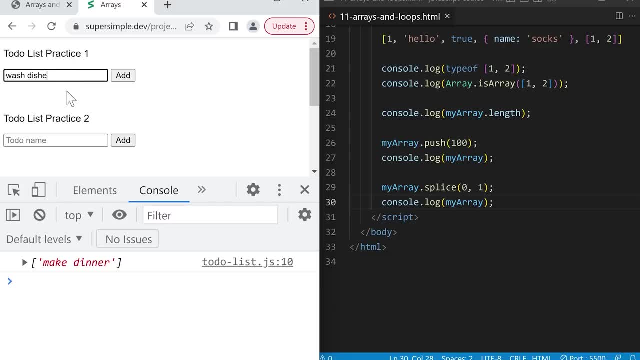 Like wash dishes And click add. It will add it to the array And display it in the console. So let's create this project. We'll start by creating a file for this project. We'll go to our code editor And click up here to show our files. 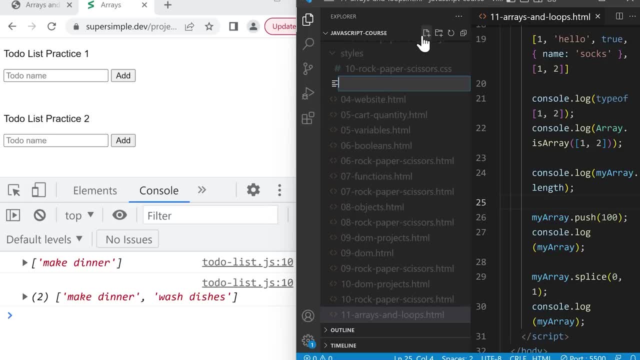 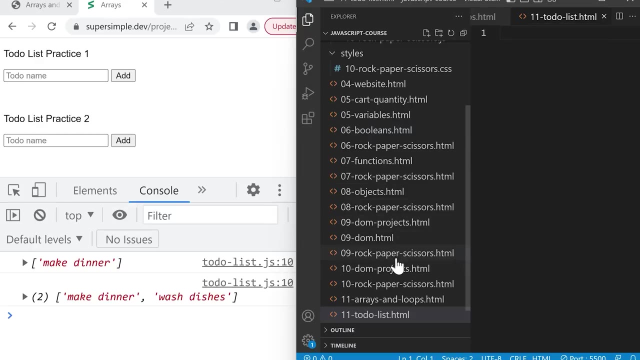 And click this icon to create a file, And we'll name this 11-todo-listhtml, And press enter. Now let's copy the code from arraysandloopshtml. So we'll click here Control-A or Command-A And then right click. 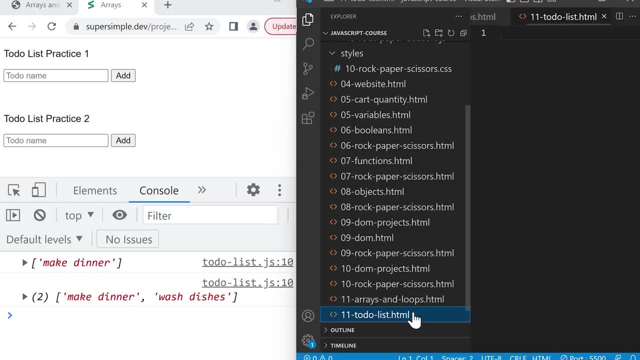 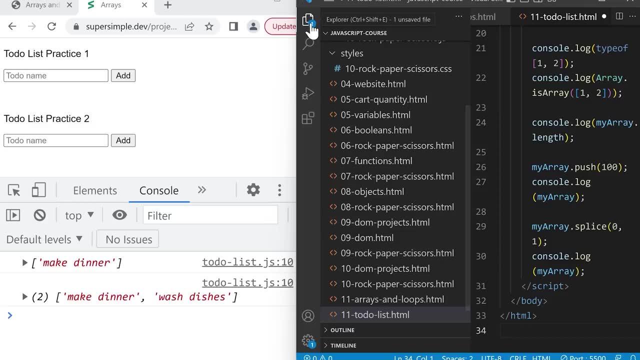 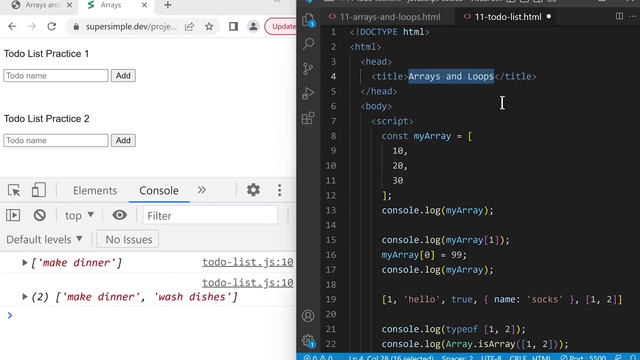 Copy And down here, Right click And paste, And let's close this for now. We'll scroll up And change the title To to-do list And remove all the JavaScript code And this time, Instead of writing all the JavaScript in here, 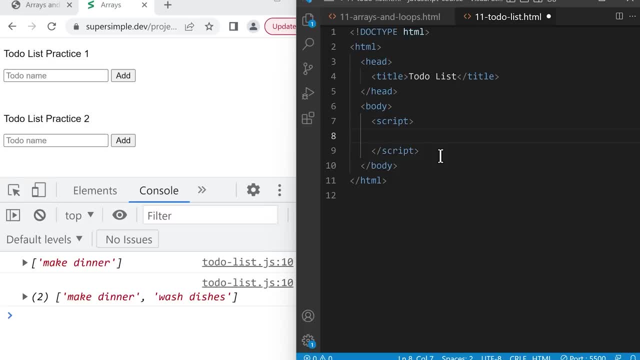 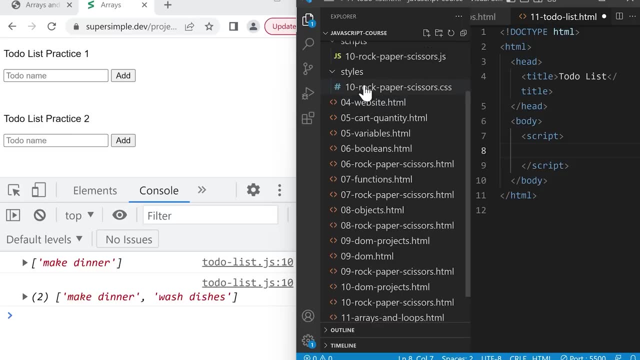 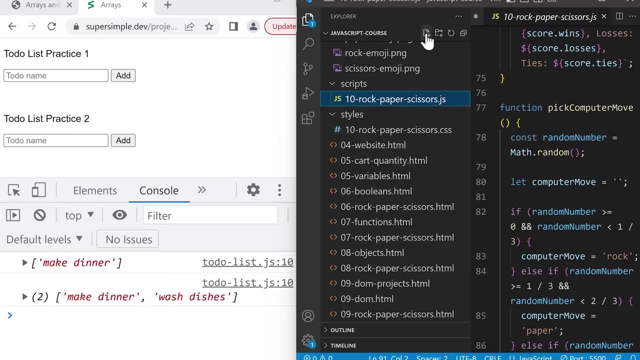 Let's actually put the JavaScript in a separate file, Which we learned in the previous lesson. So we'll open our files again And this time We'll go to our scripts folder, We'll click this JS file And we'll click this icon. 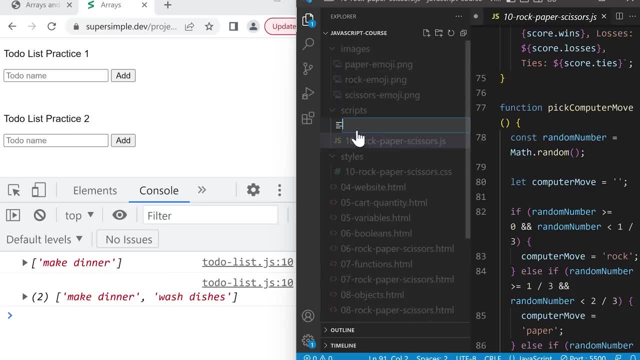 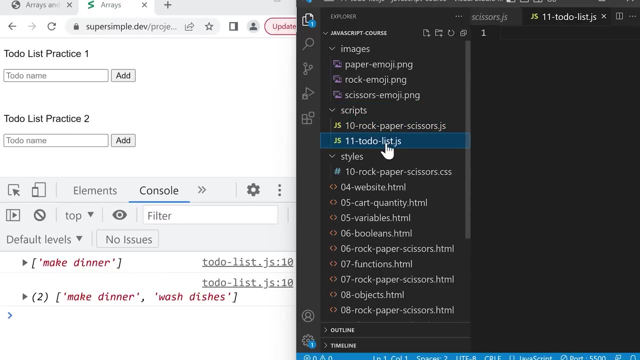 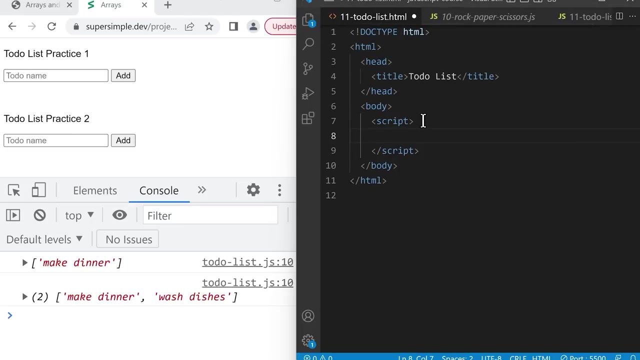 To add a new file to this folder And let's name it 11-todo-listjs And press enter. Next We're gonna load this file Into our HTML file, So let's open this And in the script element: 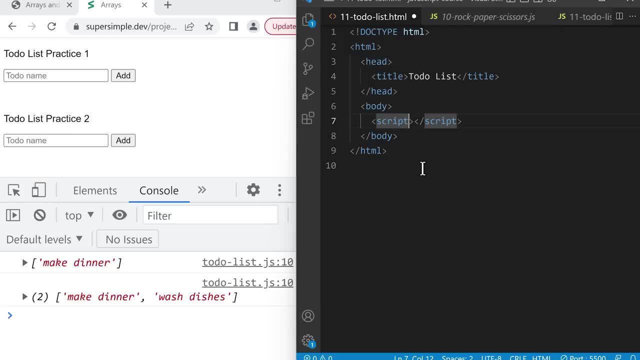 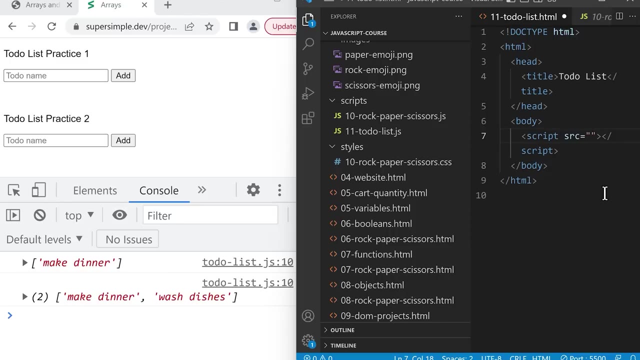 We can remove the spaces And we're gonna add an attribute Called src Equals And we're gonna load the JavaScript file That we just created, Which is inside the scripts folder. So we'll type Scripts And then a slash. 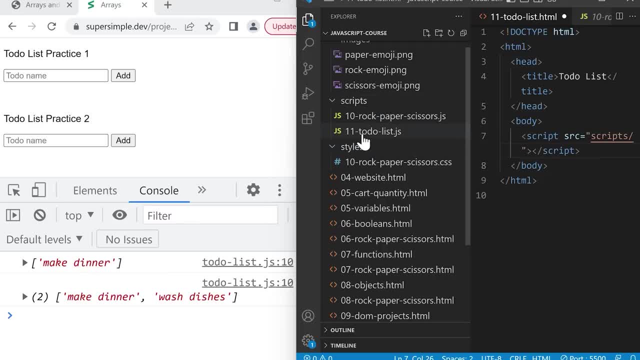 To go into this folder And we'll load the file 11-todo-listjs And save. So now I'm gonna drag this file Down here So I can see Both the HTML And JavaScript At the same time. 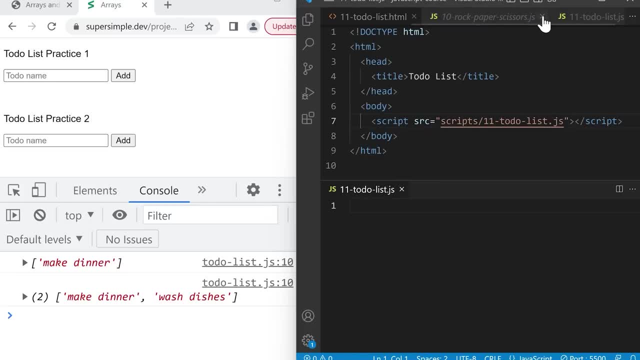 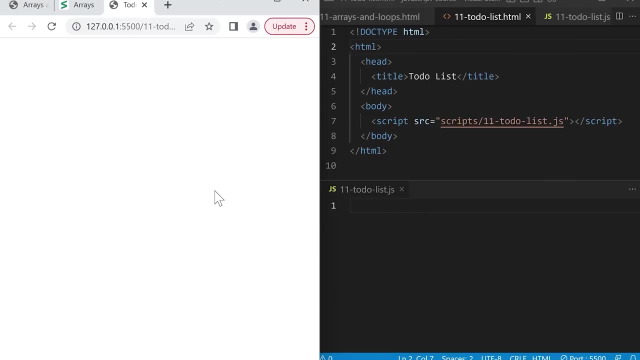 Close this for now, And I can close the other code For now as well. And finally, Let's open this in our browser, So we'll right click Open with Live server And let's also open The console on this page. 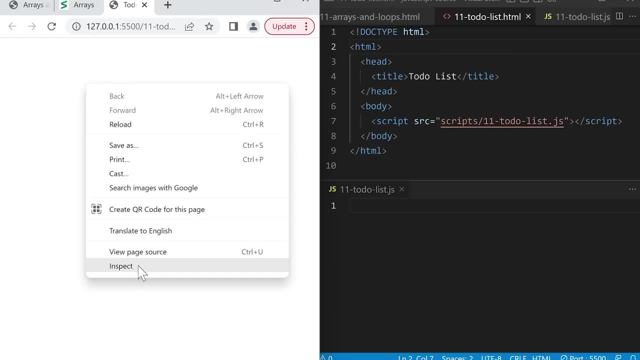 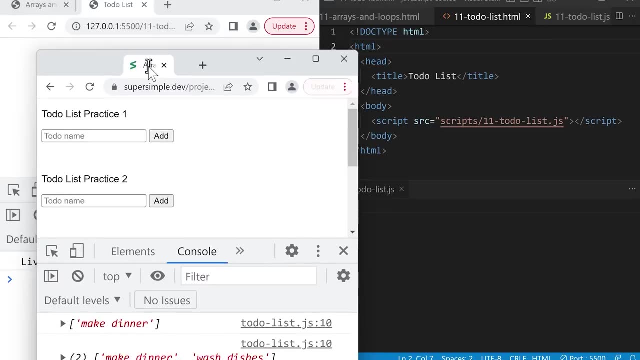 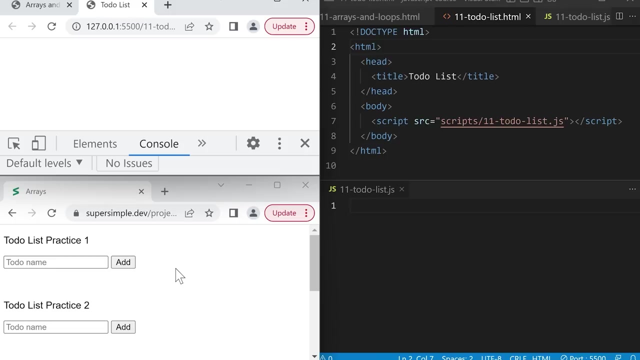 Right click, Click, inspect And click the console. Now, one more thing I'm gonna do for this video Is I'll rearrange my windows So that we can have The final design at the bottom. Let's start By creating the HTML. 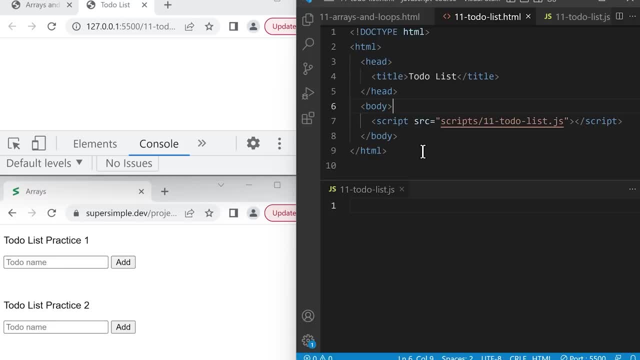 Elements. Let's go to the body And we'll actually create A paragraph element To start. Inside the paragraph, We'll put the text To do List. Next, Let's create The text box. So, to create a text box, 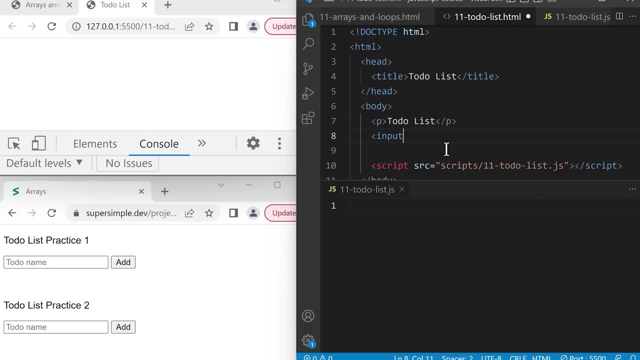 Less than Input. Greater than- And we'll add A placeholder To this text box. Place Holder Equals To do Name. Finally, Let's add This button. So, on A new line, Let's type: 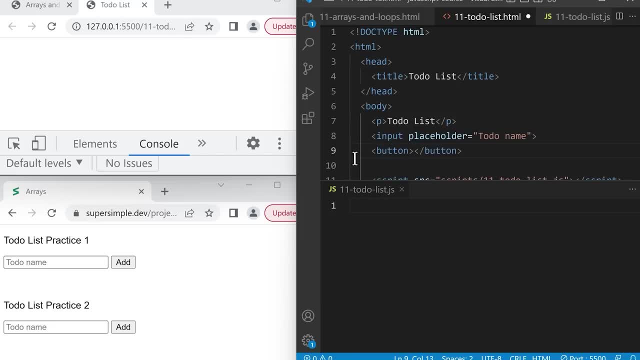 Less than Button, Greater than, And. inside the button We'll have the text Add. Now let's save, And this creates All the HTML elements That we need. Next Let's write. So first We're going to create. 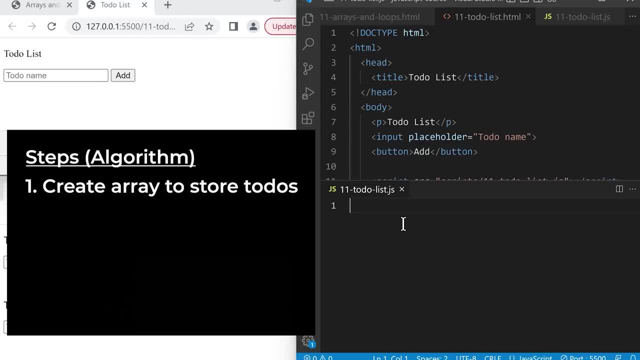 An array To store Our to do's And then, When we click The add button, We're going to get the text From the text box And add it To our array And finally We'll console Log. 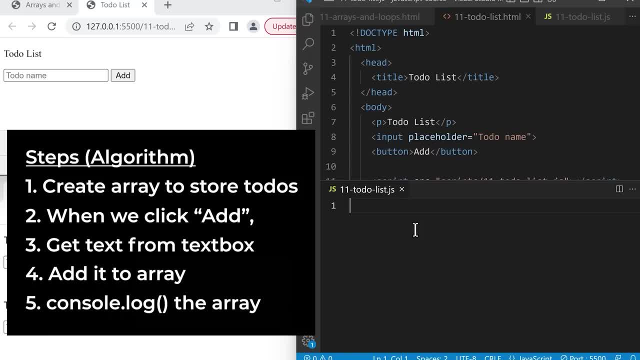 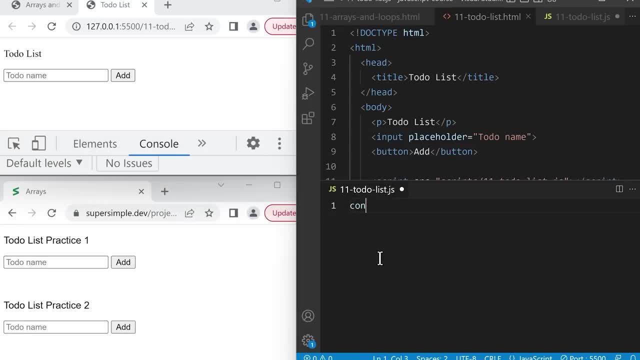 The array. Now let's convert These steps Into code. Let's create A new array, First Using Const. Let's Name it To do List And we'll make it Equal To Square brackets. 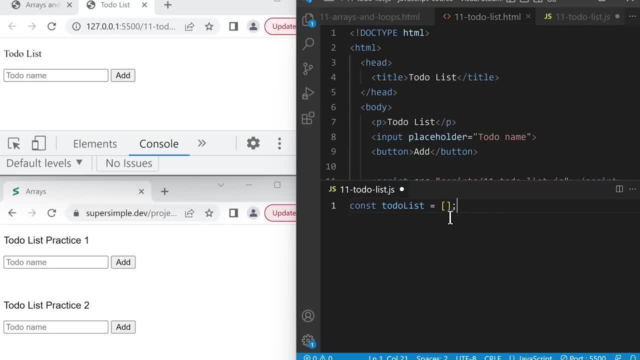 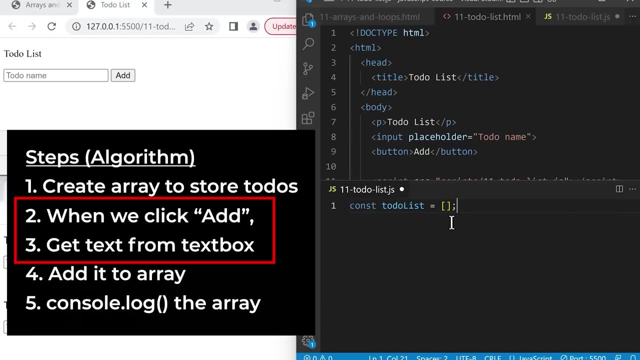 So this Is an array With no values Inside. We also call this An empty Array. Next, When we click The button, Let's get the value From the text box. So let's go To our button. 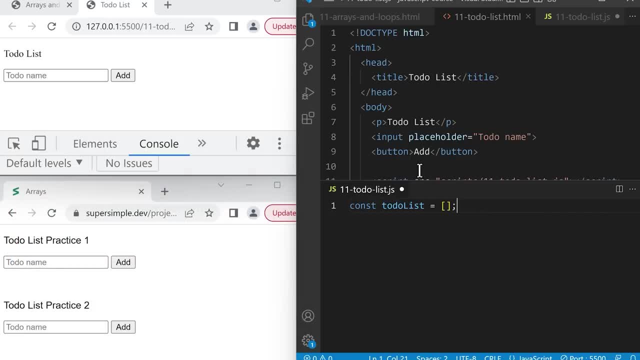 And add An On Click Attribute To Our Array Attribute And then Inside Here, Let's create A function For this. So down Here, Let's create A Function. We'll name it. 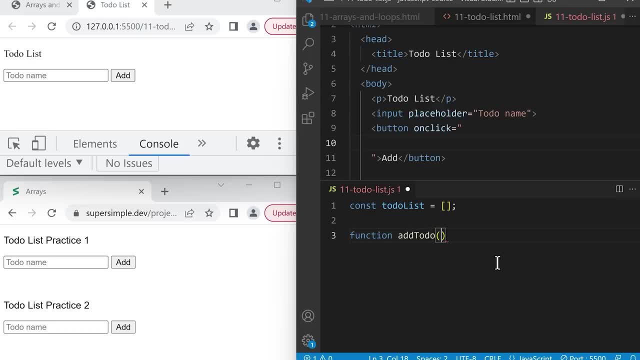 Add To do Brackets And Curly Brackets And then Inside The On Click Attribute, We're just going to Call This Function: Add Brackets. The Next Step. 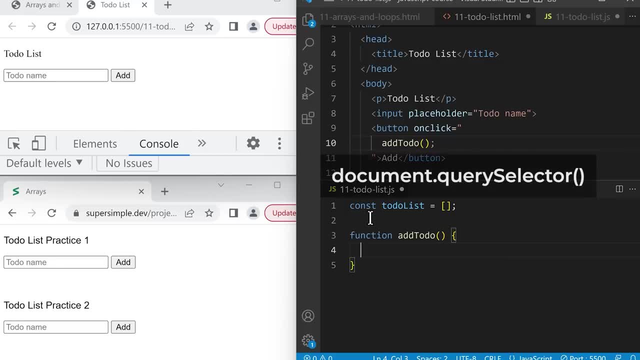 Is To Get The Text In The Text Box. We Can Do That Using Document Query Selector. So To Use Query Selector, We're Going To. 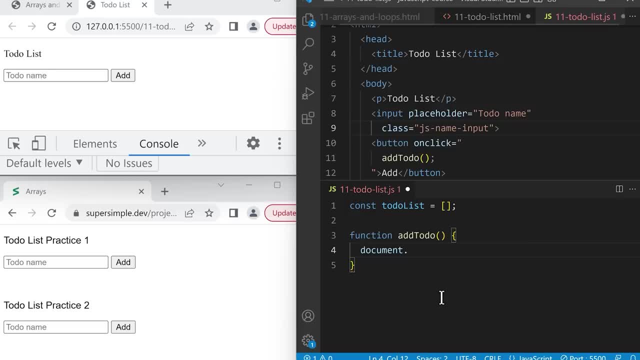 Add Document: Dot Query Selector, Brackets And A String And We'll Type A Dot To Get A Class And We'll Get This Class J. 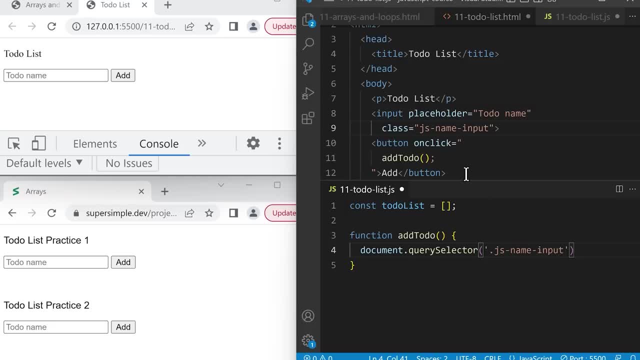 S Dash Name, Dash. Input As And Put It Into Our JavaScript. And Now Let's Save This In A Variable. So At The Start, Let's. 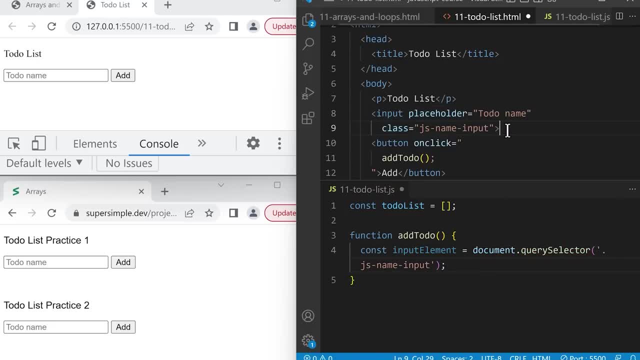 Type: Const Input Element And Make It Equal To This Result Of The Input Element Called Value. So Down Here: Input Element, Dot Value, And Let's 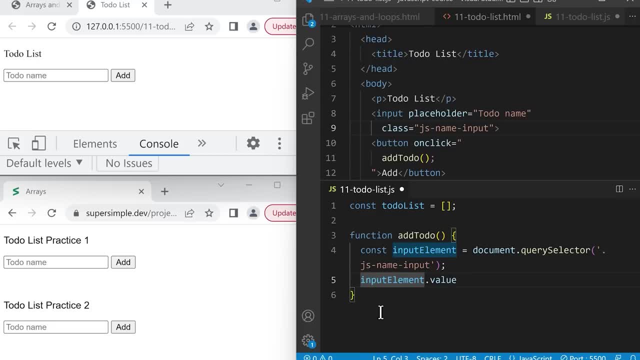 Save The Value In The Text Box In A Variable So We Can Use It. Before We Continue, Let's Console Dot Log The Name To: 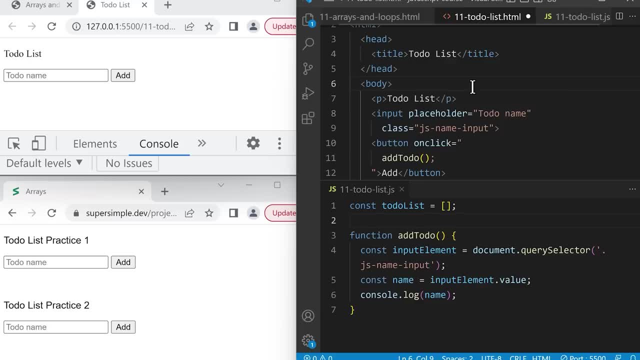 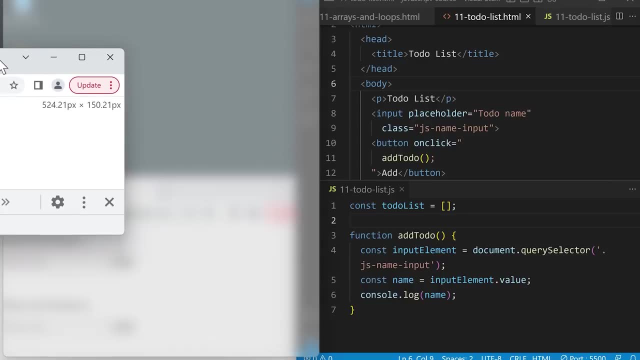 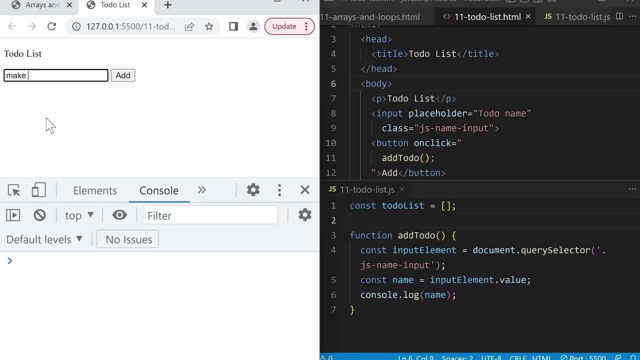 Check If This Is Working. So Let's Save This JavaScript File And Let's Also Save This HTML File. We'll Go Click Add. It Will. 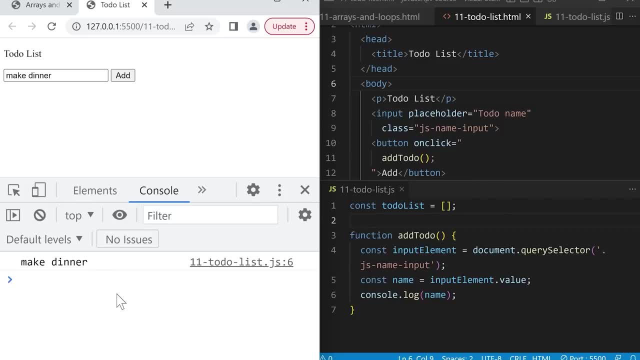 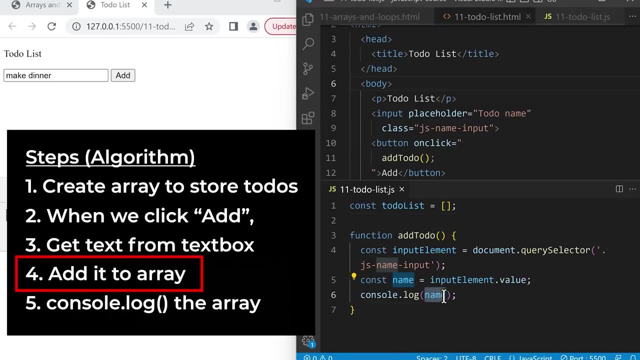 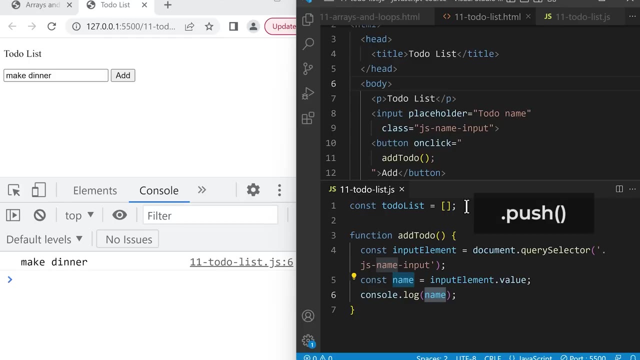 Get The Text From The Text Box And Then Display It In The Console. Okay, So It's Looking Good So Far. The Next Step Is: 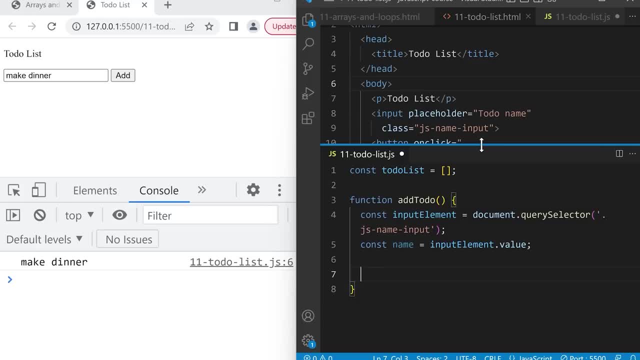 Now And At The Bottom We're Going To Type Our Array, To Do List, Dot, Push Brackets And Then, Between The Brackets, We're Going. 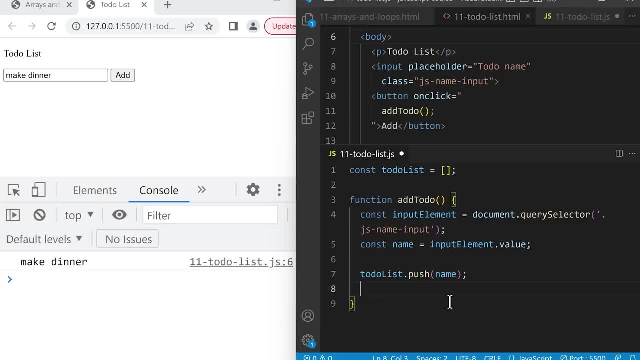 To Add Our Name Here To Do List And Save. Now Let's Give It A Try Or Type Make Dinner In The Text Box And 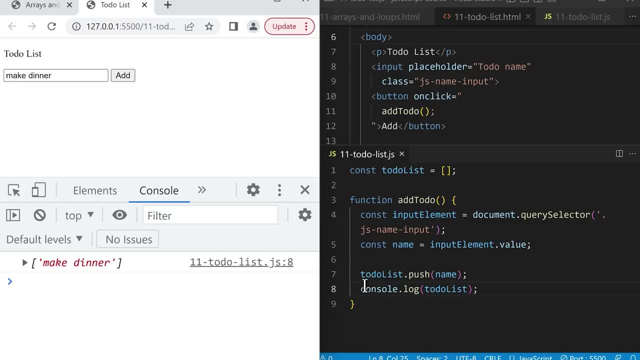 Click Add. It Will Take This Text, Add It. Let's Add Another. To Do, We'll Type Wash Dishes And Click Add Again. It Will. 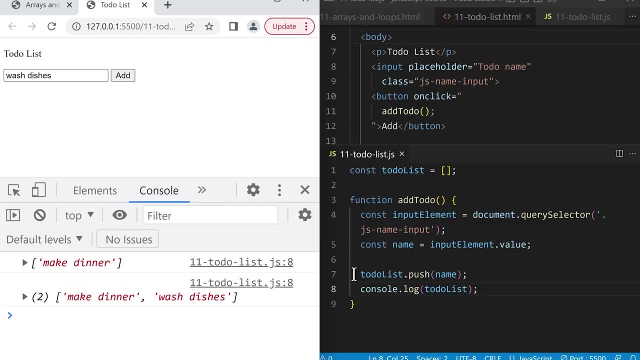 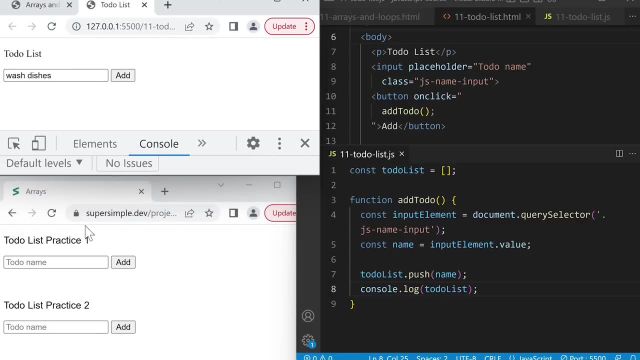 Get The Text In The Text Box And Then Add It To The Array In The Text Box And Click Add. It Will Reset The Text. 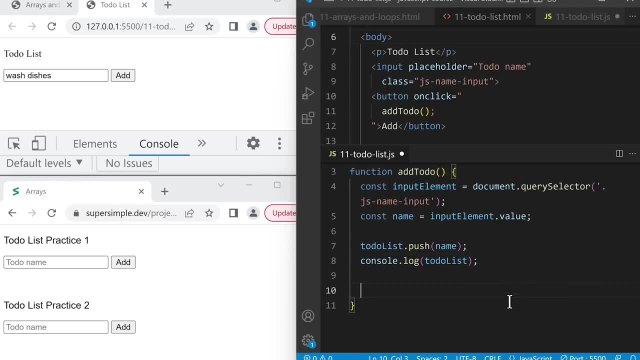 Box To Do That. Let's Go Into Our Code And We'll Create Some New Lines. And Remember That We'll Type Input Element Dot Value. 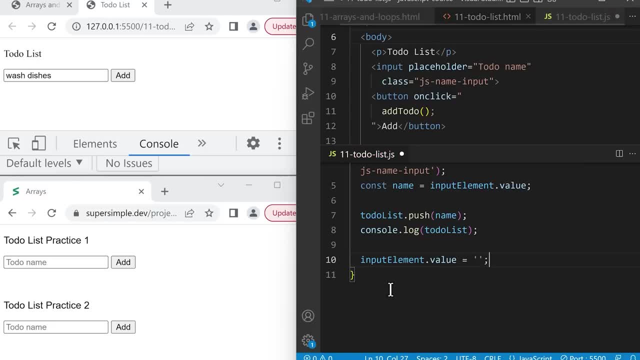 And Change It To The Empty String. So This Will Make The Text In The Text Box Become Empty If We Save And Add To The 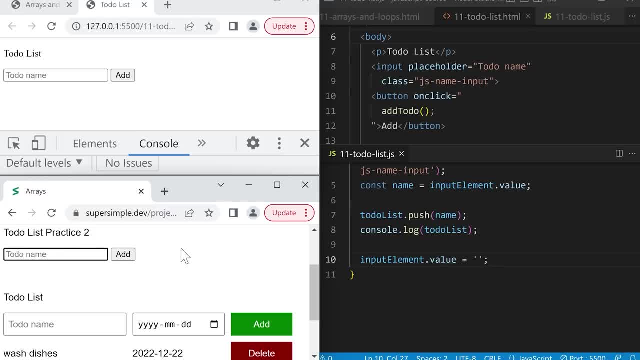 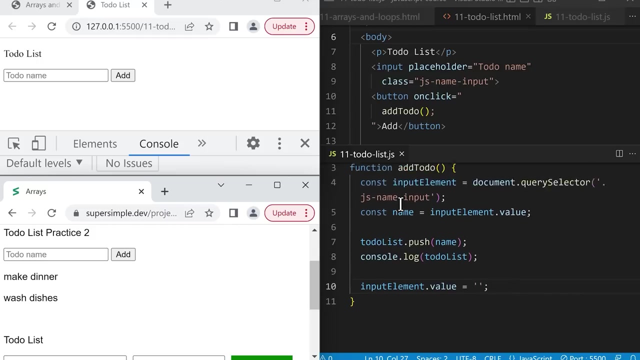 Second Version Of The To Do List. So Here, When We Type Something In The Text Box Like Make Dinner And Click Add, It Will Actually. 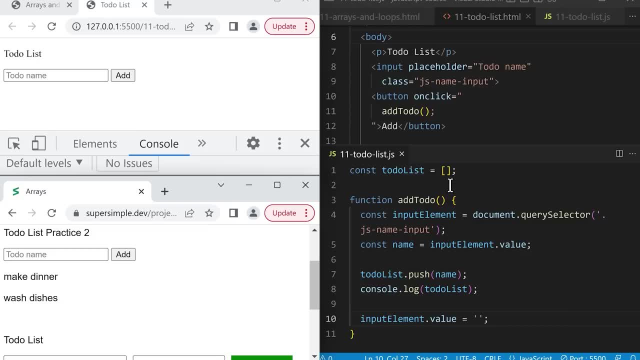 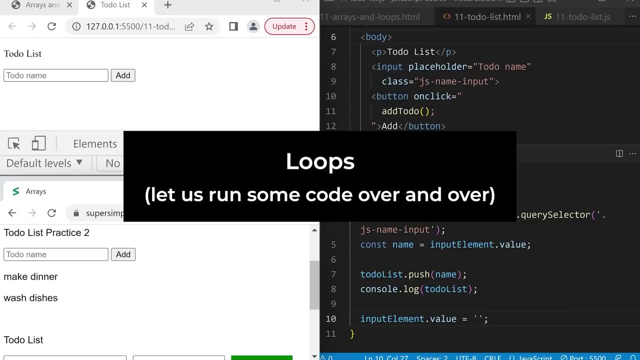 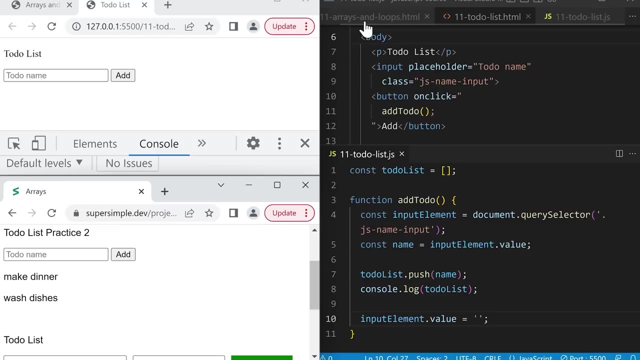 Display Each Value On The Page. To Do This, We're Going To Learn Another Feature Of JavaScript Called Loops- Loops. Let Us Run Some. 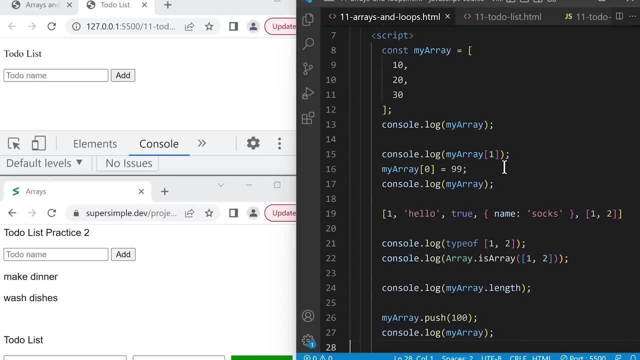 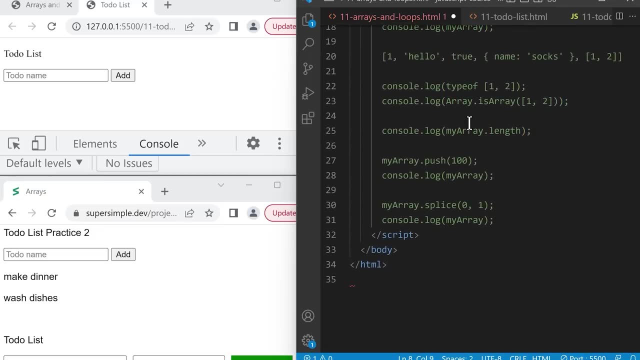 Code Over And Over Like A Word By Typing Slash, Star And At The Bottom Star, Slash. Let's Scroll Down And We'll Create Our. 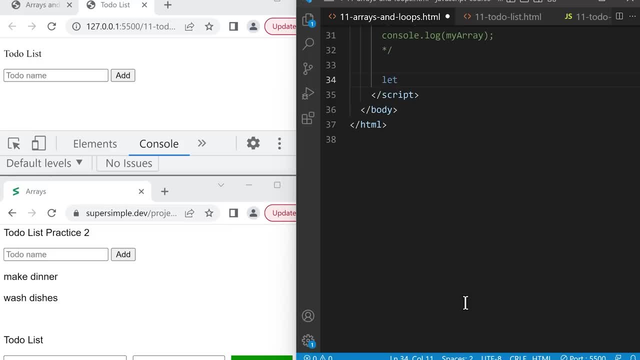 First Loop. We'll Start By Creating A Variable Using The Word While, And Then Brackets And Curly Brackets, And Then Inside These Curly. 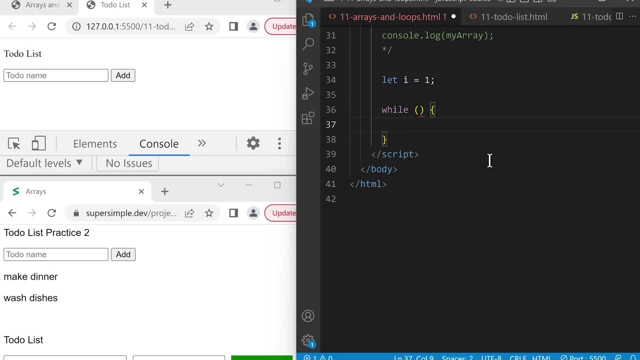 Brackets. We're Going To Put Some Code That The Computer Will Run Over And Over Just Now. Obviously, We Don't Want To Loop This. 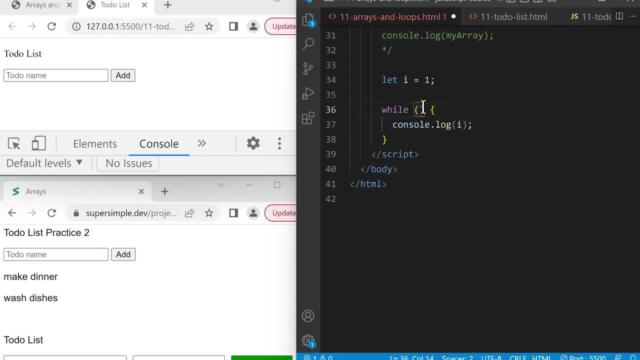 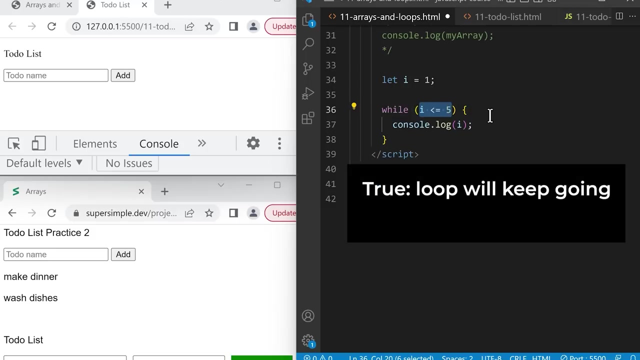 Forever. So How Do We Get This Loop To Stop? We Can Do That Using The Round Brackets Up Here Inside That. If This Code 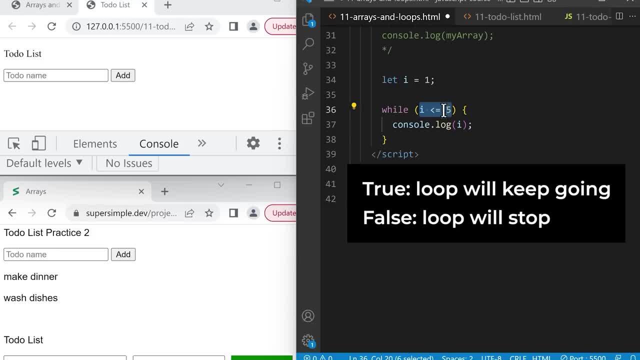 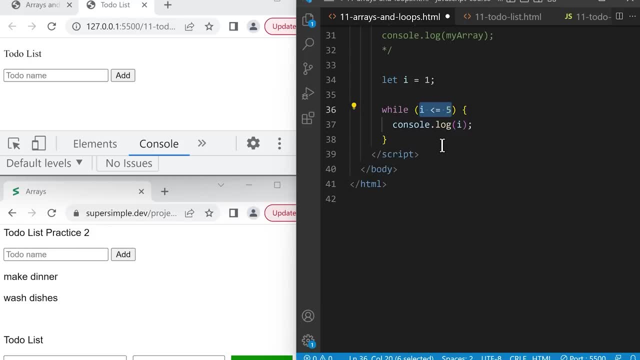 Results In True, The Loop Will Keep Going Over And Over. Once This Results In False, The Loop Will Stop And It Will Go To Loop. 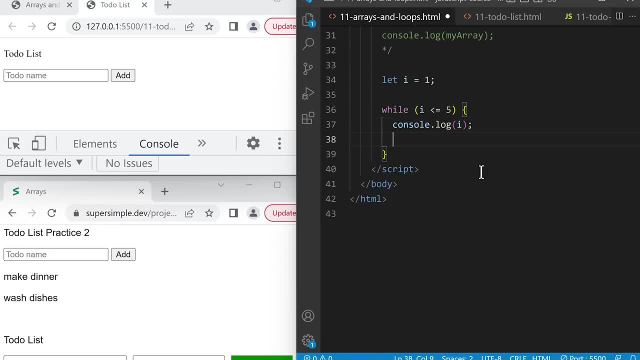 The Answer Is Inside This Loop. We're Also Going To Update This Variable I, So We'll Type I And We'll Make It Equal To. 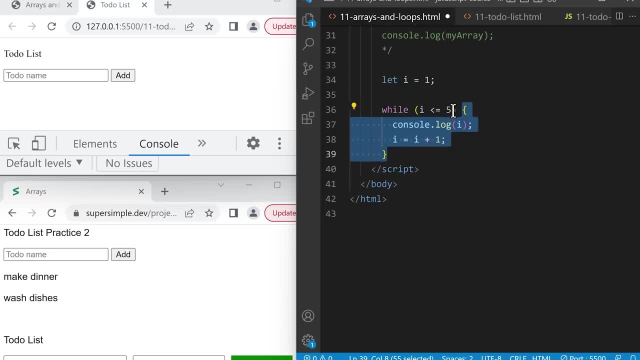 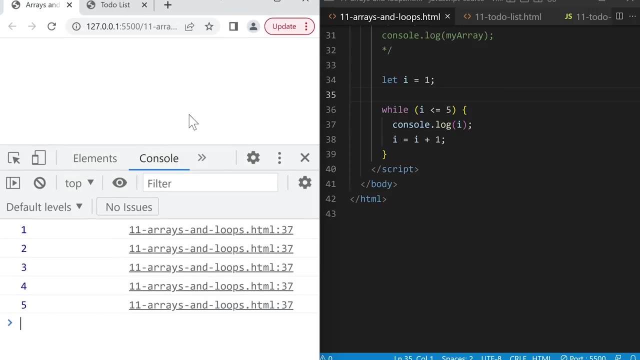 Itself Plus One. So It Will Stop The Loop If We Save And Then Go Back To The Tab For This File And I'll Rearrange. 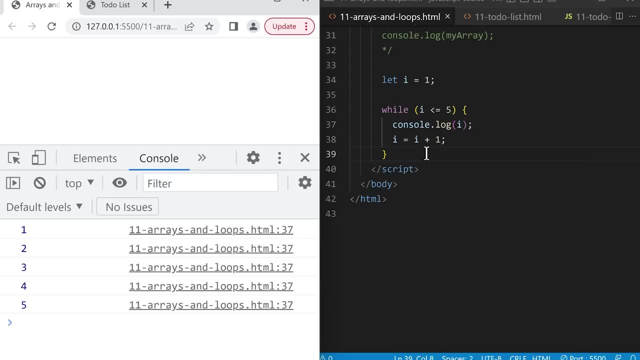 My Windows So We Can See The Console And We Make It Equal To One And Then We Do A Loop. So If This Condition Is, 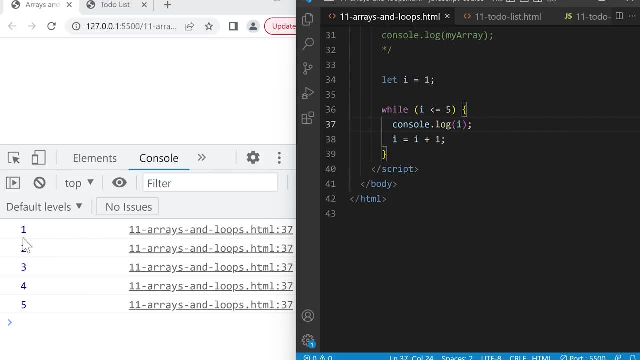 True. The Computer Will Keep Running This Code Over And Over. This Code To Is Less Than Or Equal To Five. This Is True, So We're. 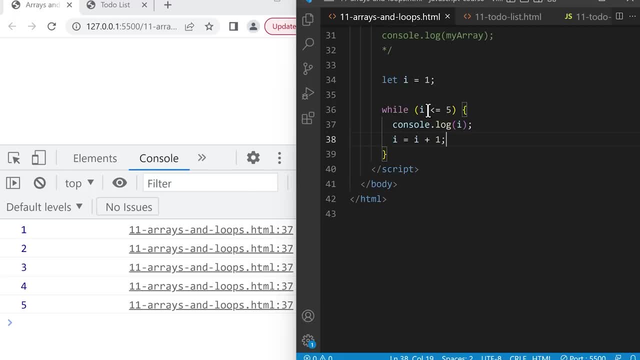 Going To Run This Code Again. This Time I Equals To, And We Display It To Six. Once I Is Six, This Will Become False. Which? 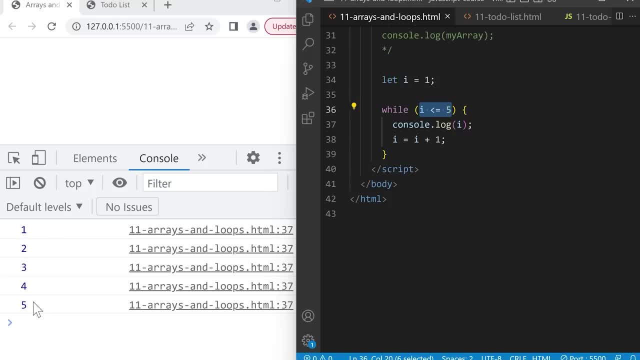 Will Cause The Loop To Stop And Then We Go To The Next Line. So That's Why It Just Like A Loop As Soon As 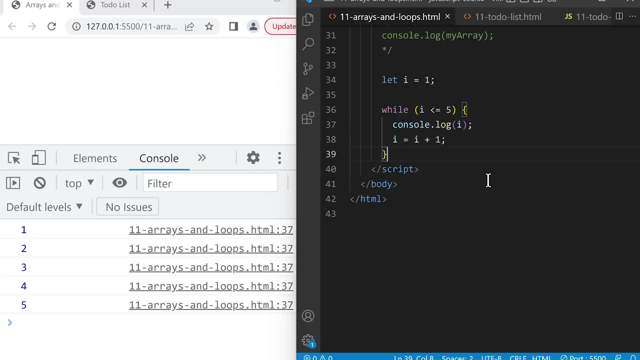 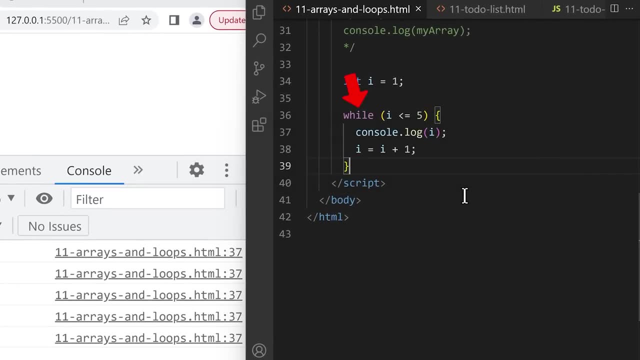 This Condition Is False. It Will Stop The Loop. Alright, Now That We Understand How A While Loop Works, Let's Learn The Code Inside The 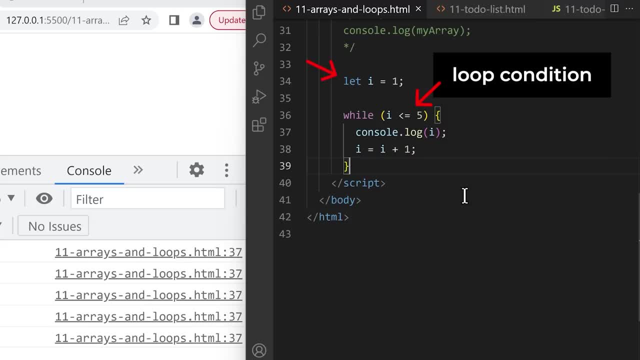 Curly Brackets Is Called The Loop Body. The Variable I At The Top Is Called The Loop Variable. Every Time We Loop, We're Going. 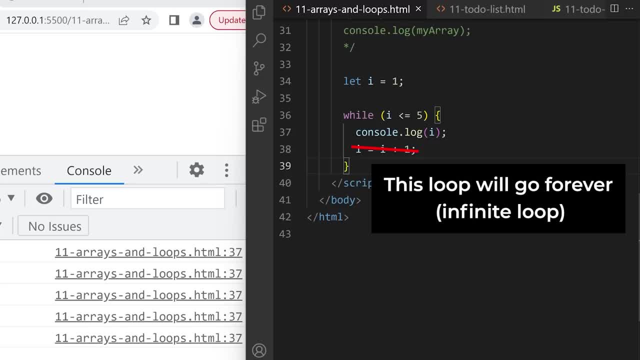 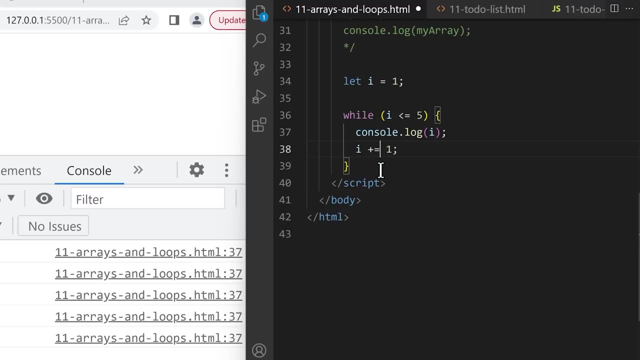 To Increase. This Is Known As An Infinite Loop. Now, Remember That I Equals, I Plus One Has A Shortcut. Instead Of This, We Can Just. 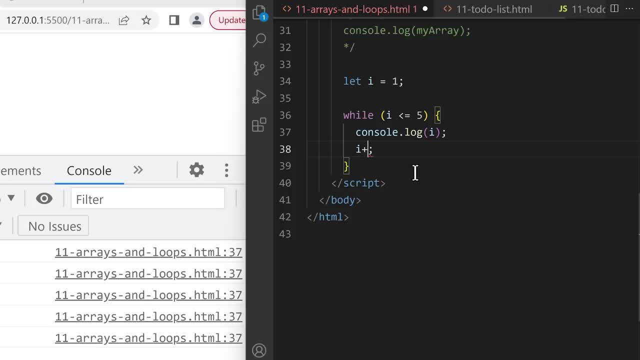 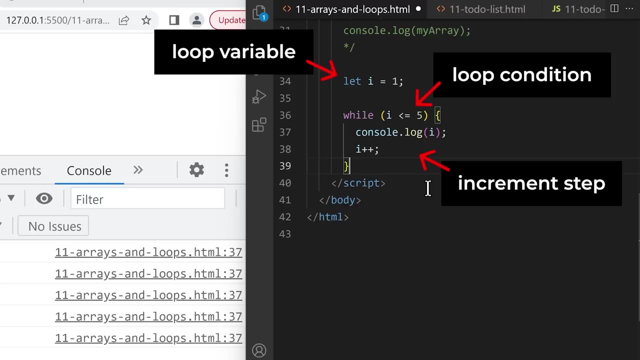 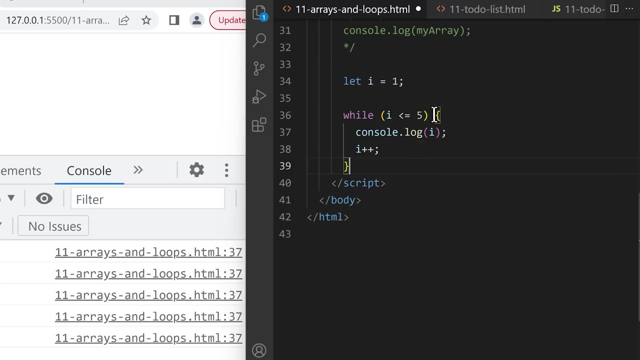 Do I Plus Equals One, So This Will Increase The Value Of I By One Every Time, Just Like Before. So Those Are The Three Major. 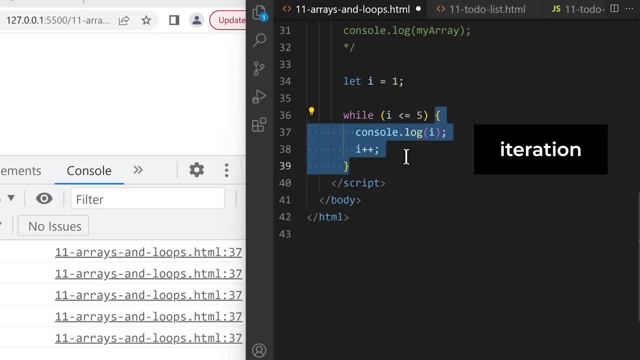 Parts Of A Loop, The Loop Variable. The Value Is Five Times. And, Lastly, Loops Create A Scope- Any Variable That We Create Between These. 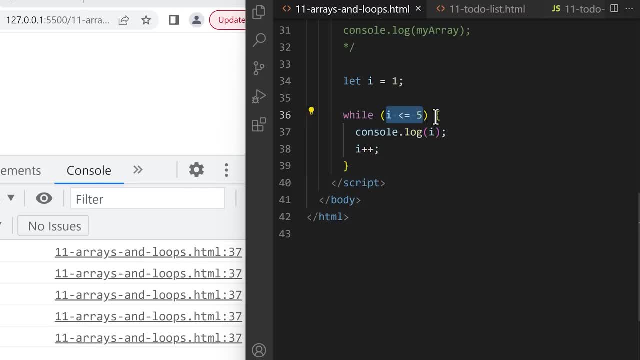 Curly Brackets Will Only Exist Inside The Curly Brackets. So That's A Bracket And A Line. So In JavaScript There's Actually Two Types. 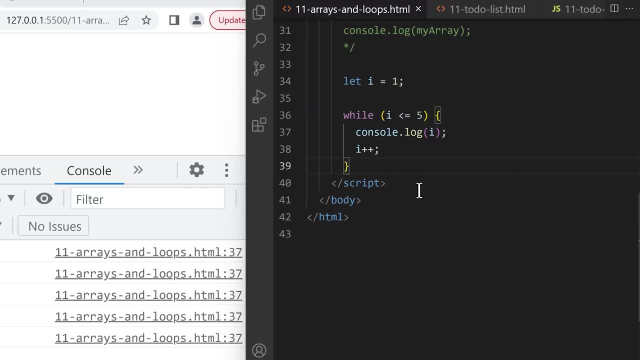 Of Loops. The First Type Is A While Loop, Which We Just Learned. Now We're Going To Learn Another: Curly Brackets Inside These Brackets. 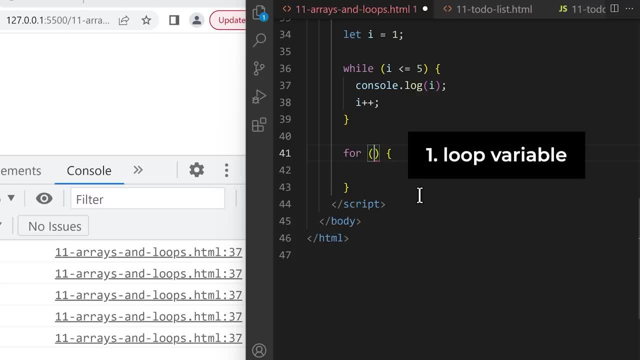 We're Going To Type Three Pieces Of Code. The First Piece Of Code Is The Loop Variable, Which Is The Same Thing As This Line. 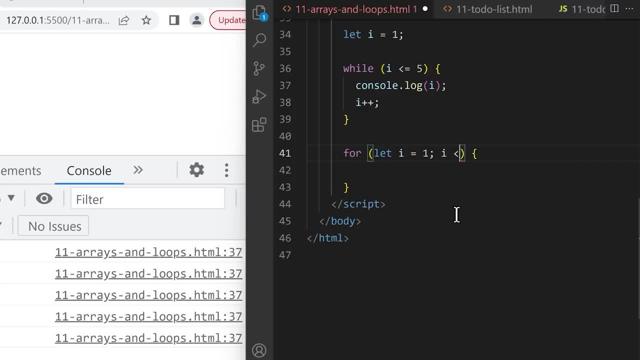 So Here We'll Type I Less Than Equal To Five, And Then Semicolon And Space, And The Last Piece Of Code Is The Increment. 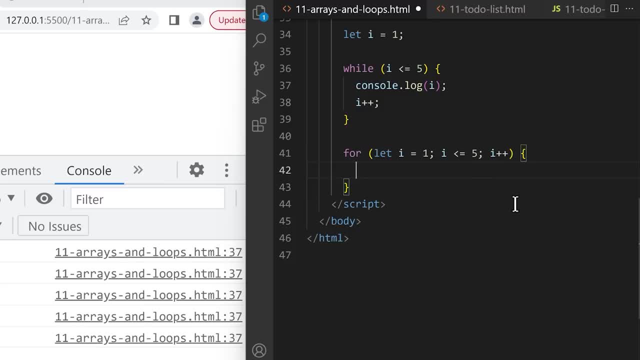 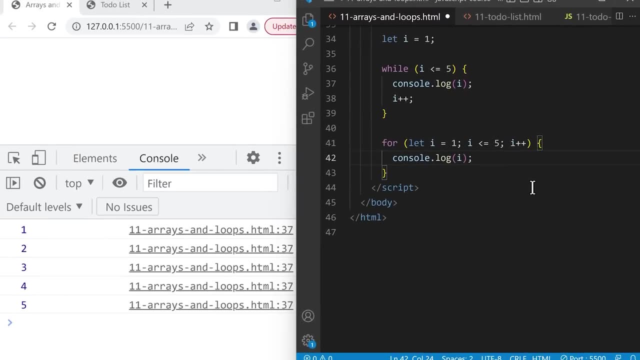 Step, Which Is This Line, Console, Dot, Log I And Save. So This For Loop Does The Same Thing As The While Loop Above It Counts. 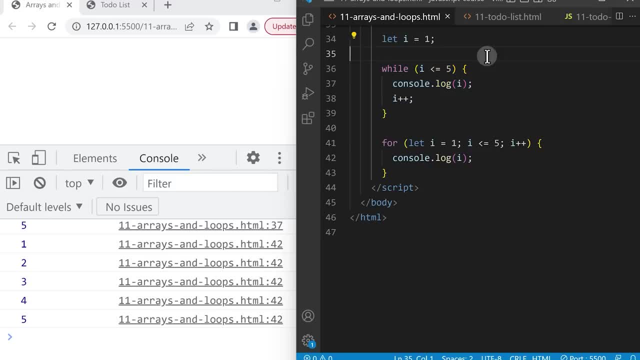 From One To Five, And If We Look Separately, We Group All Of Them Together At The Top. So This Loop Works The Same Way. 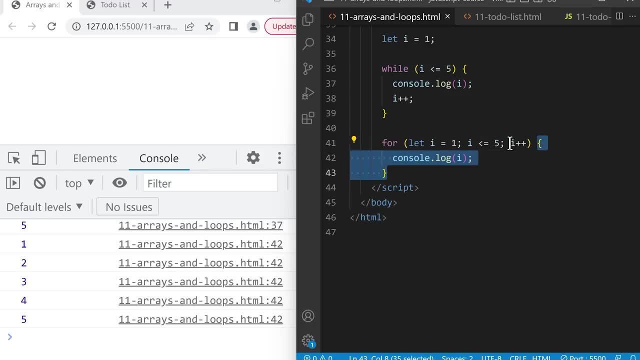 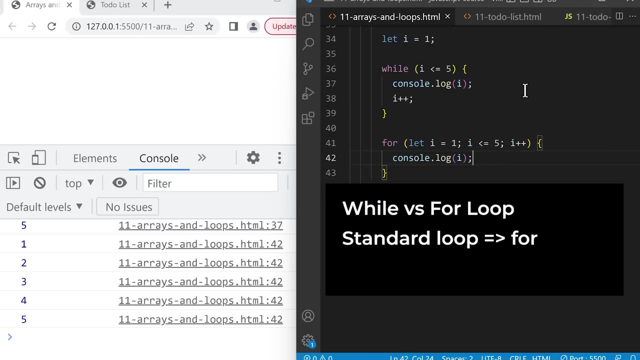 First We Create A Loop Variable And Then, As Long As This Do, A Loop. Which One Should We Use If We're Doing A Standard? 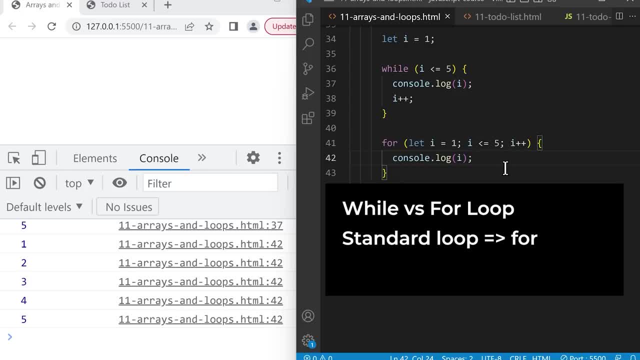 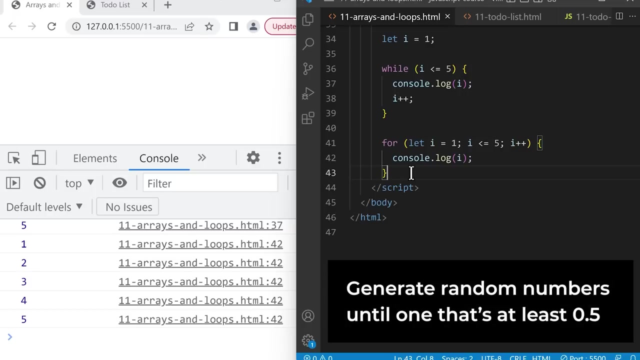 Loop For Example. It Has A Loop, Variable A Condition And An Increment Step Every Time. So What's An Example Of A Non Standard Loop. 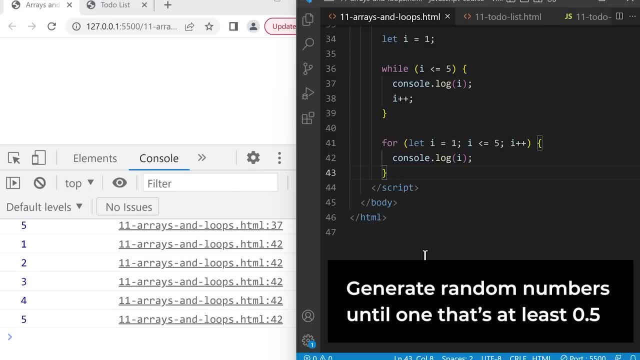 Let's Say We Want To Generate Random Numbers Until We Get A Number That's At Least 0.5.. To Create This, And Then We'll: 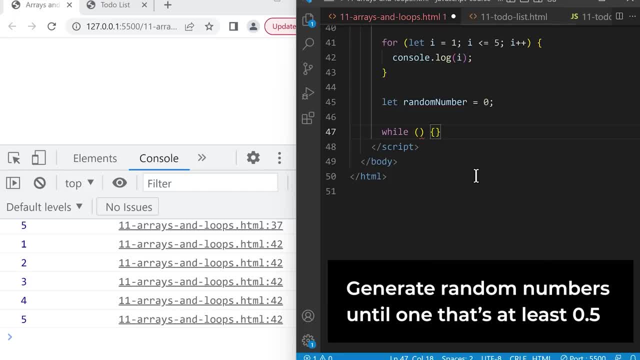 Do A While. Loop Brackets And Curly Brackets Now Inside The Loop Condition. We Want To Keep Running This Loop Until Random Number Is. 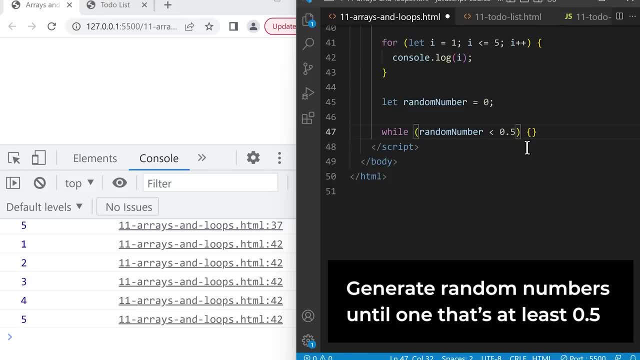 At Least 0.5.. And Then, Inside This Loop, We're Going To Generate A Random Number Between 0. And 1. And Then Save It. 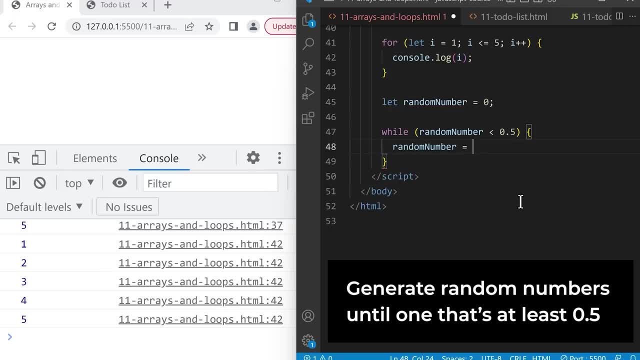 In The Variable Up Here. So We'll Type Random Number If This Random Number Is Less Than 0.5.. It Will Keep Generating Random Numbers. 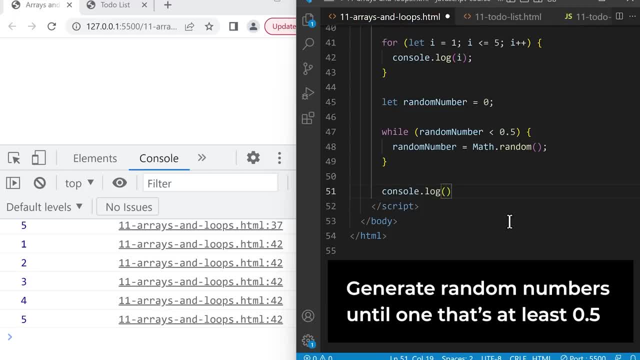 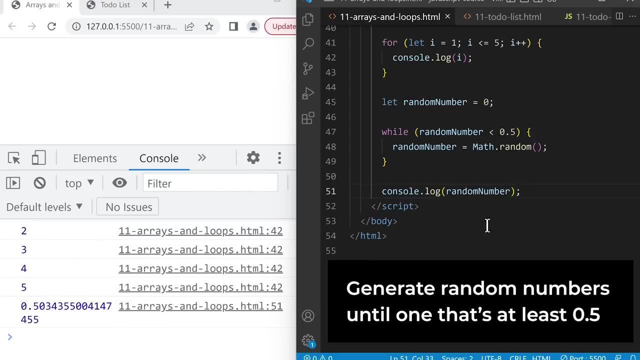 Until We Get A Number That Is At Least 0.5.. So, At The Bottom, If So, Notice That This Is A Non Standard Loop. 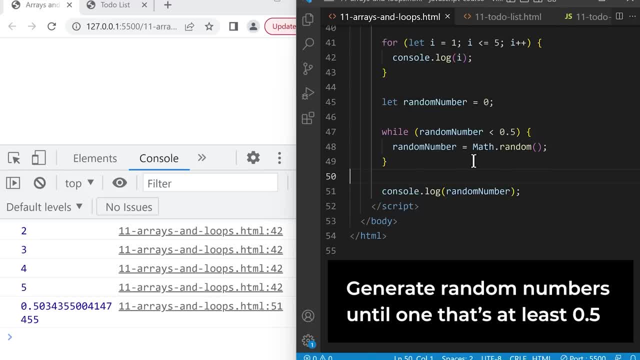 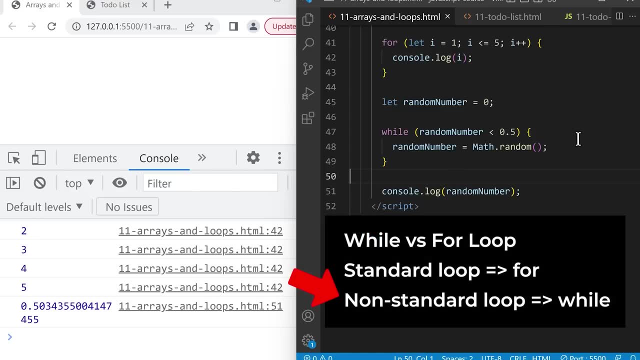 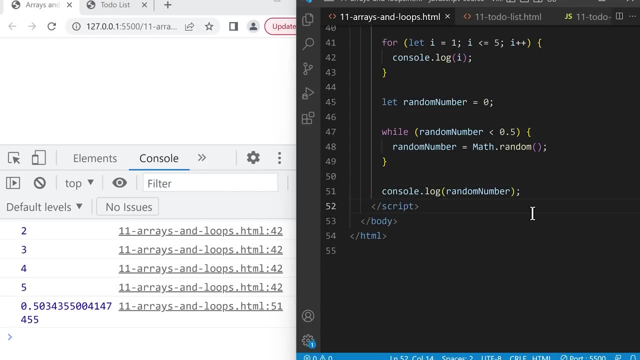 It Doesn't Really Have A Loop Variable That We Increase Every Time, And It Also Doesn't Have The Increment Step. Let's Do Some Practical. 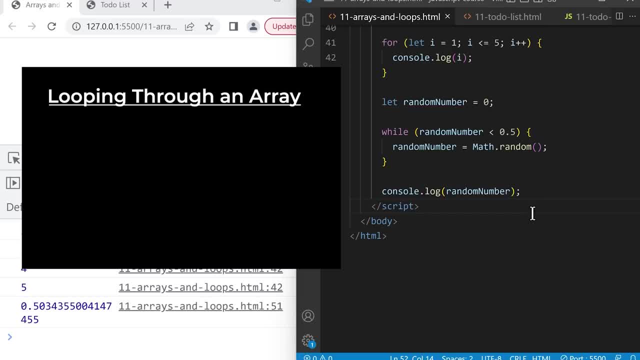 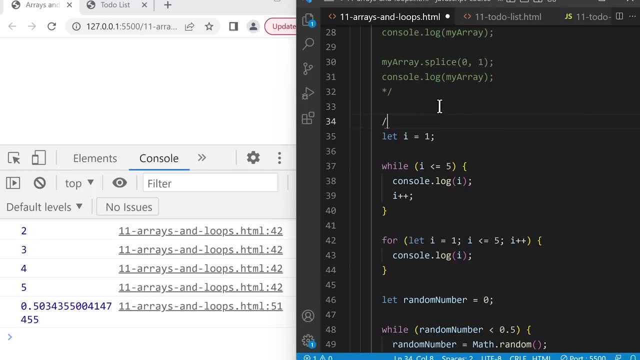 Examples: We're Gonna Learn A Technique Called Looping Through An Array. This Means We're Gonna Go Through Each Value Of An Array One. 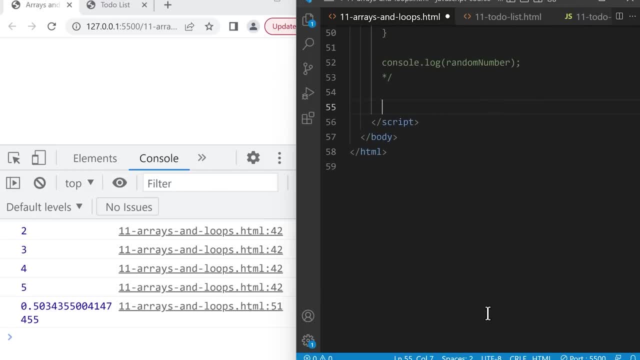 By One We Create An Array Of Strings, So We'll Create A Variable Const To Do List Equal To An Array And Inside This Array. 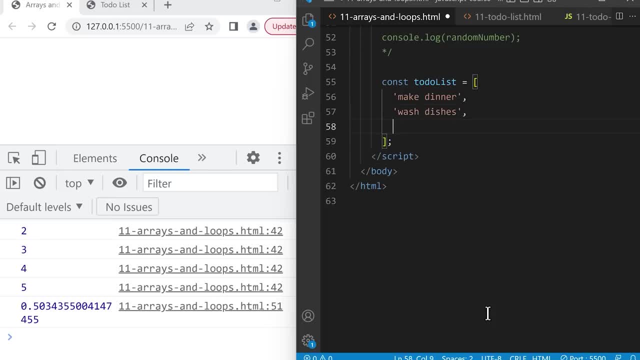 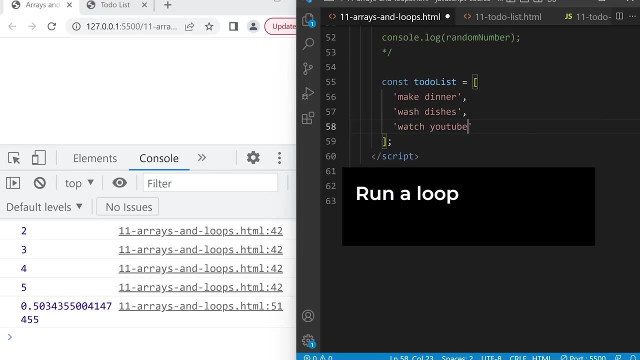 We'll Have The String Make Dinner Another YouTube. Now Let's Take Each Value In This Array And Display It In The Console. To Do That. 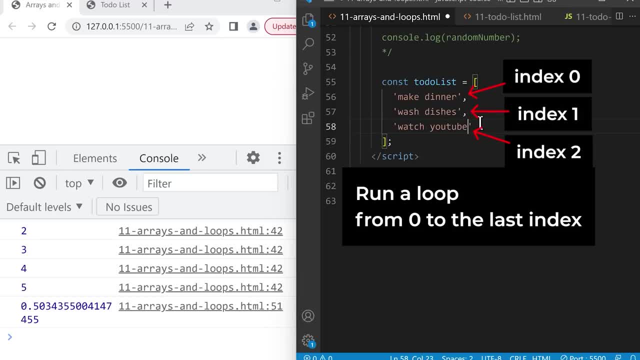 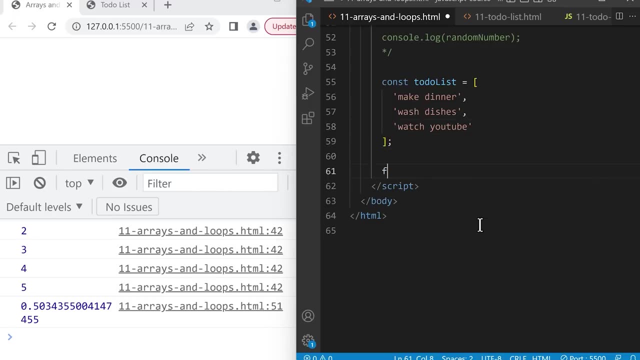 We're Gonna Run A Loop, And This Loop Is Gonna Count The Value, And So On. So Below This, Let's Type For Brackets. 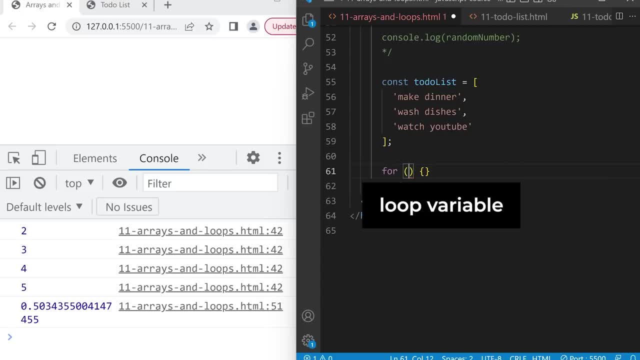 And Curly Brackets. Inside These Brackets We're Gonna Create The Loop Variable. So Here We're Gonna Count Condition, So We'll Keep Looping. 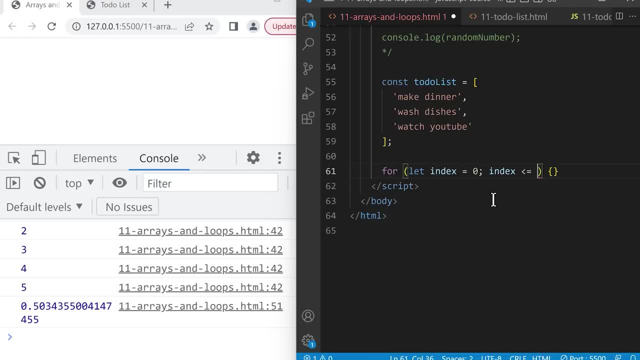 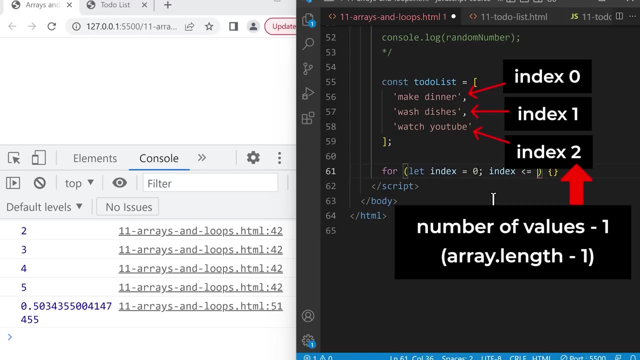 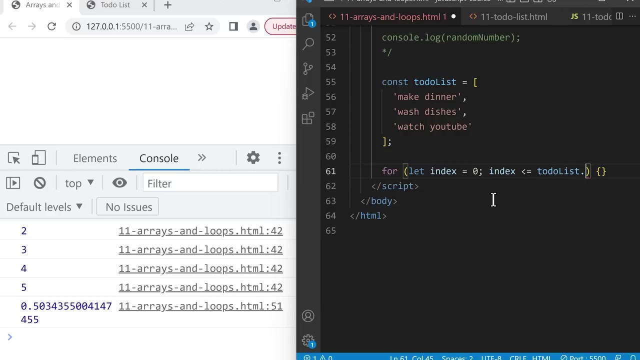 As Long As The Index Is Less Than Or Equal To The Last Index. So Remember That The Index Starts From Zero. This Means The Length. 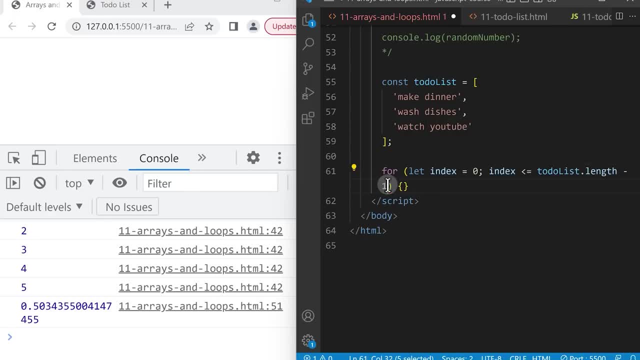 Minus One, And Here We'll Add Another Semicolon And We'll Add The Increment Step, Which Is Index Plus Plus. So We'll Increase It. 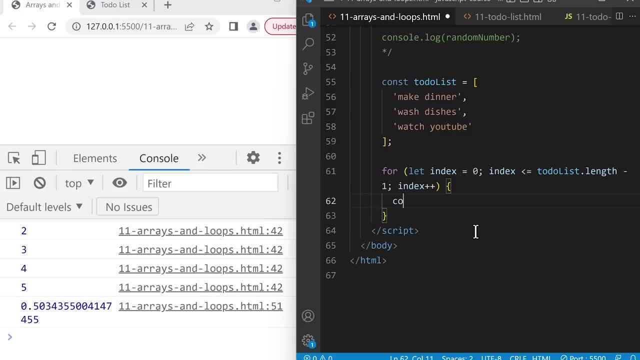 By One Every Time We'll Log This Index And Save, So This Will Count From Zero To Two, Which Is Exactly All The Indexes In. 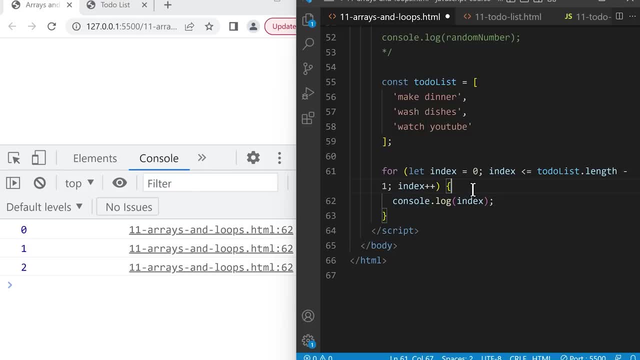 This Array And Now Using This Index List And Then Square Brackets And Between The Brackets Index, This Will Take Whatever The Index Variable Is. 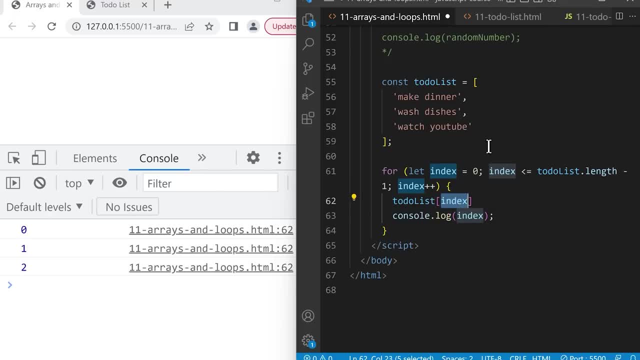 An Access That Index In The Array. So If The Index Which Is The Second Value, And So On. So For Now, Let's Save The 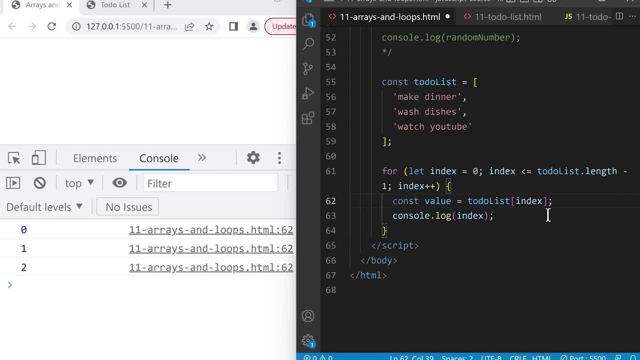 Value In A Variable Using Const Value And Make It Equal To. To Do List Bracket. Get The Value At Each Index And Then Display Each. 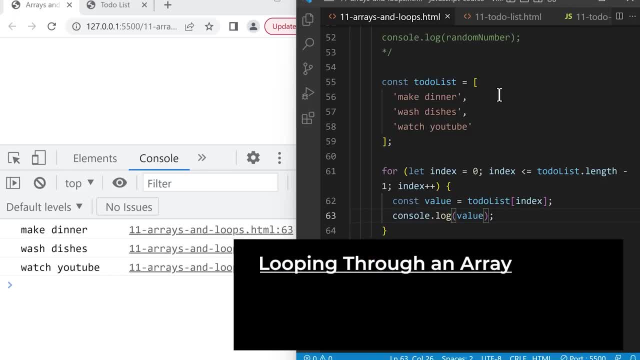 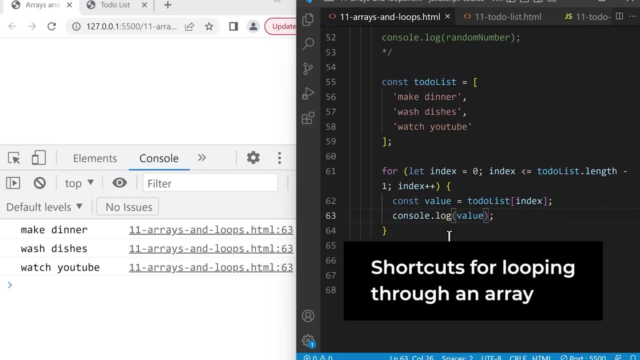 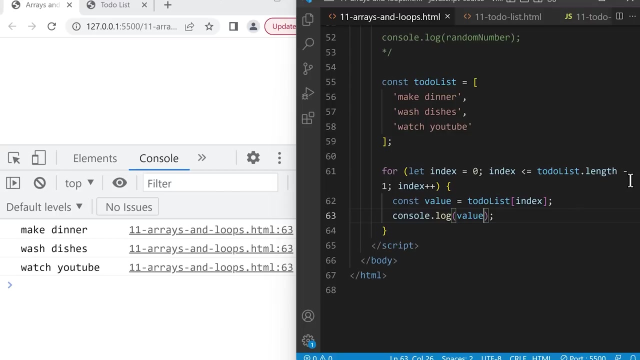 Value, Which Is What We See In The Console. So This Technique Is Called Looping Through An Array. We, Instead Of Checking If Index Is, 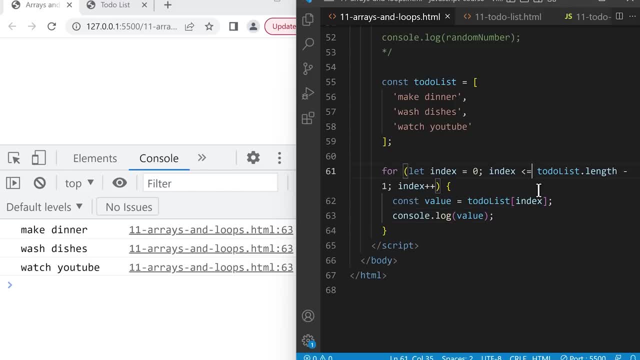 Less Than Or Equal To To Do List Dot Length. We Can Shorten This To Index Less Than To Do List Dot Length Instead Of. 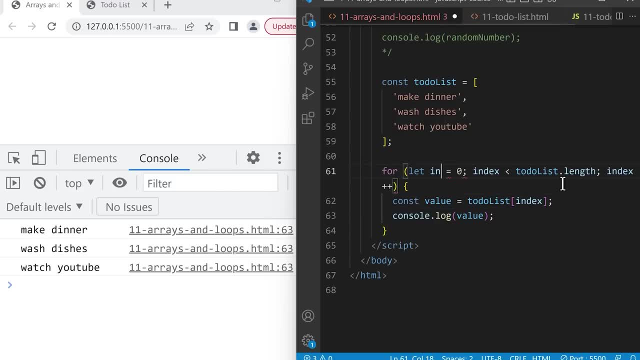 Naming The Loop Variable Index. We Can Shorten This To I, And We'll Shorten This As Well And This As Well, And That's Why. 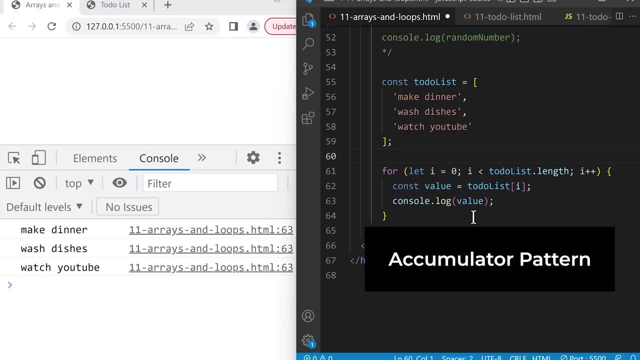 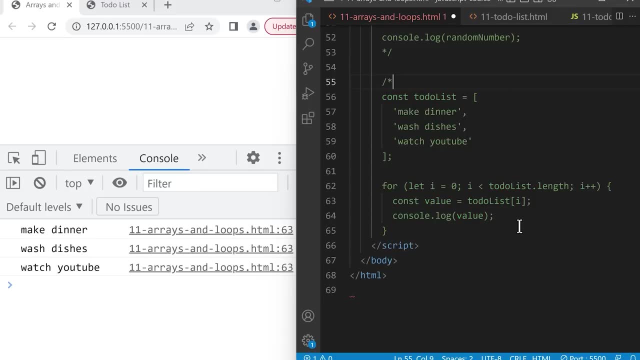 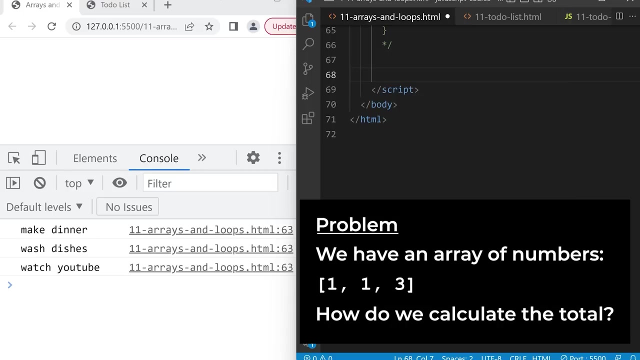 We Often Name Our Pattern. So First Let's Comment Out The Previous Code Using Slash, Star And Star Slash. And At The Bottom Let's Say: 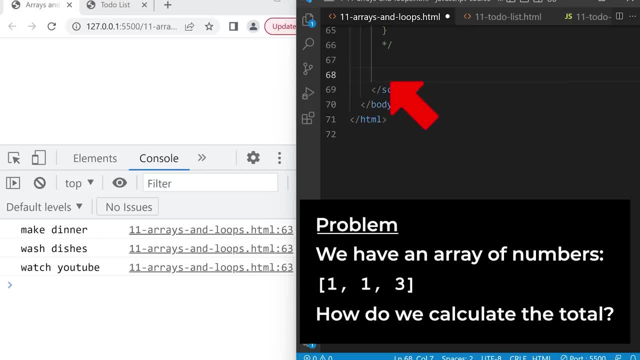 We Have An Array Of Numbers Like This, Const Nums, Equals, Array, And Then The Numbers One, One And Three, And We Want To Calculate. 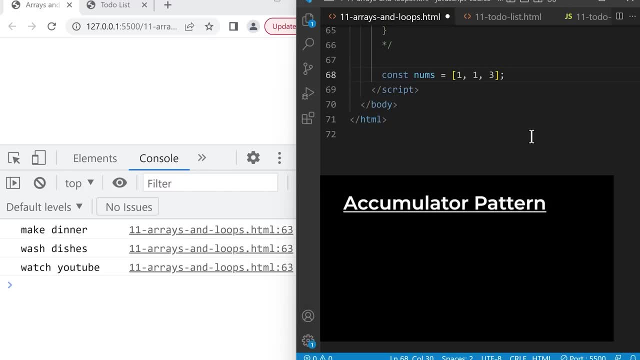 The Total Of All The Numbers In This Array To Calculate The Numbers. So Below This Let's Create A Variable Const Total And We'll Make 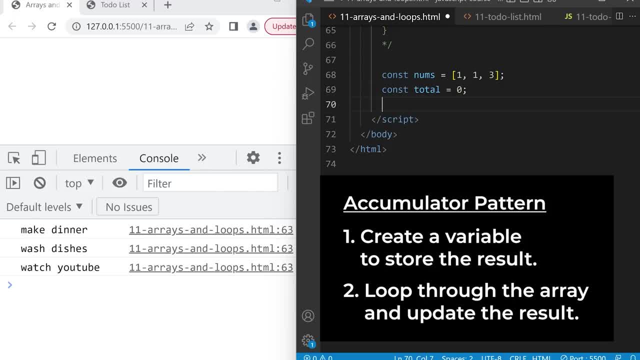 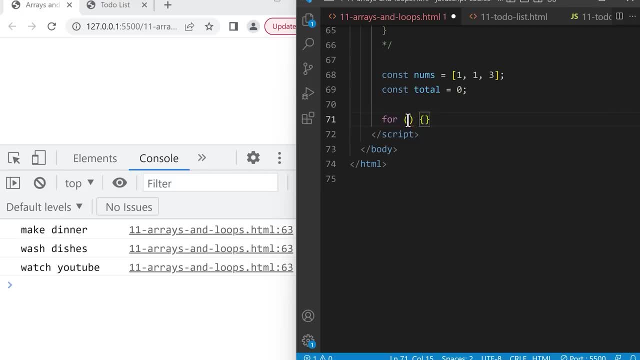 It Equal To Zero And The Next Step Is To Loop Through This Array And Update Or Index Equals Zero, Semicolon Space, And We'll. 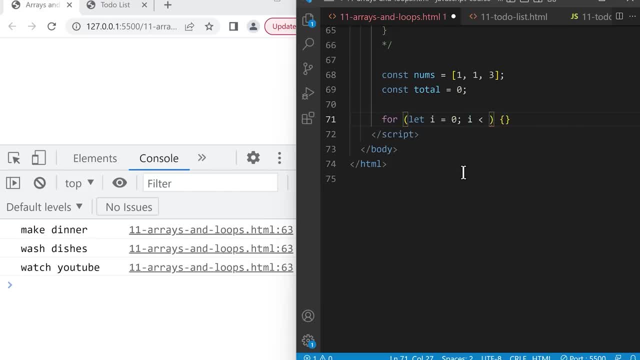 Create The Loop Condition I Less Than Nums Dot Length, And Then Semicolon And The Increment Step I Plus, Plus. So As Between These, 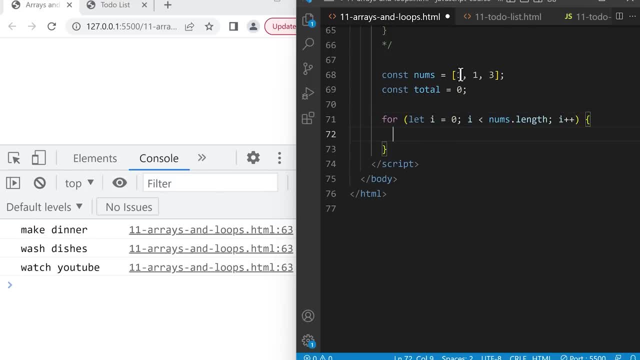 Curly Brackets. First Let's Use The Index To Get Each Value. So We'll Type Nums And Then Square Brackets And Access The Index. 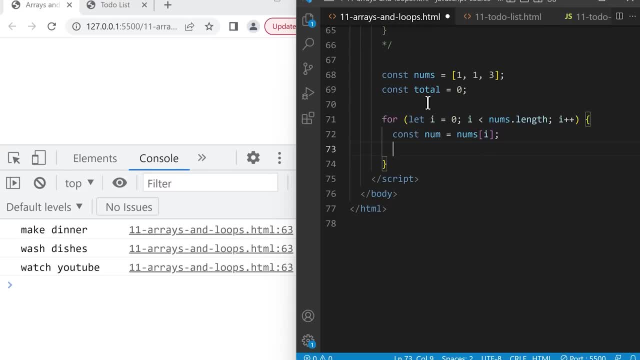 I, And Let's Save This. We Can Type Total And Make It Equal To Itself Plus Each Number. And Remember We Have A Shortcut For. 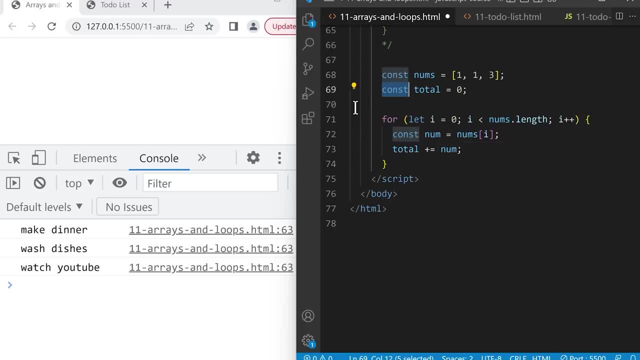 This Which Is Plus Equals. And Finally, Since We're In A Group, We Should Have Added Each Number In The Array To The Total. So 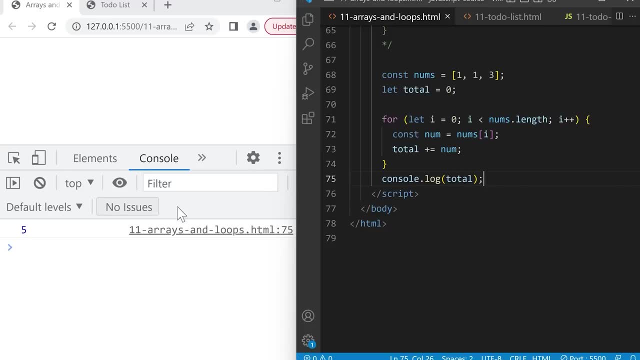 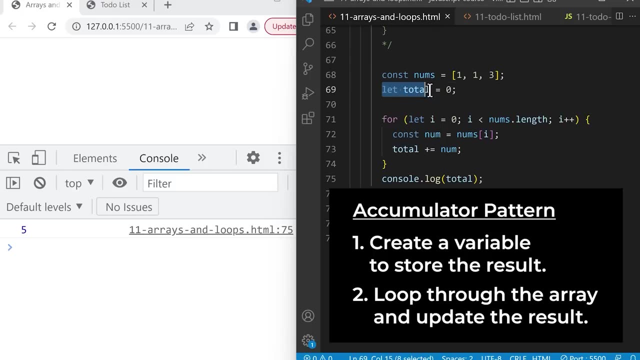 At The Bottom, Let's Console Dot Log The Total And Save And It Stored The Result And Then We Loop Through The Array And Update. 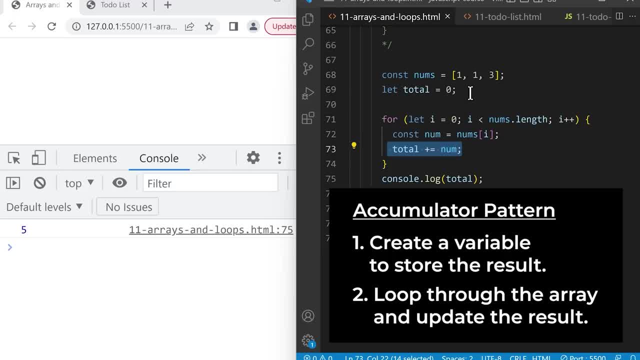 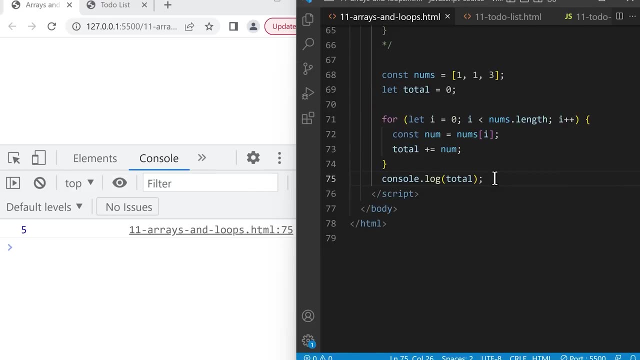 The Result. So Notice That As We Loop Through The Array, We're Adding Or Accumulating The Results Using The Accumulator Pattern. Let's Say We're. 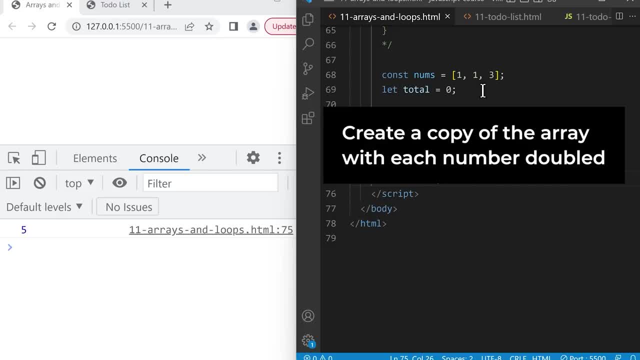 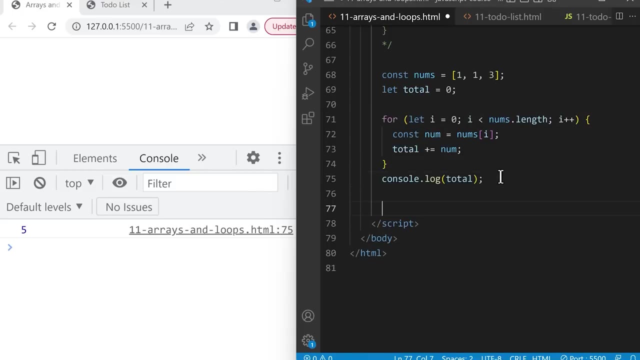 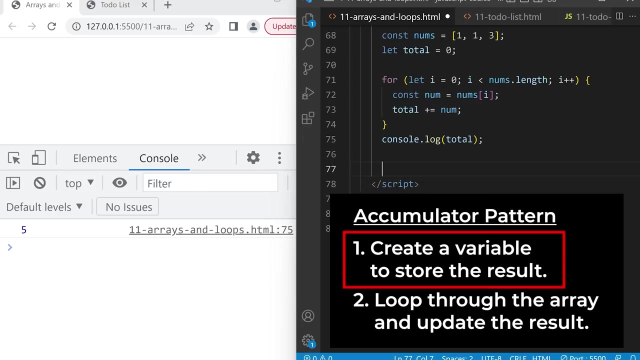 Given This Array Of Numbers Again And We Want To Create A Copy Of The Array Where Each Number Is Doubled. So The First Step. 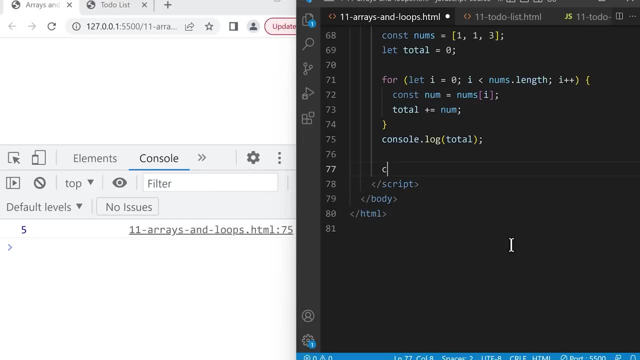 Is To Create A Variable To Store The Result. Let's Type Const And Let's Name This Nums Doubled And We'll Make It Equal. 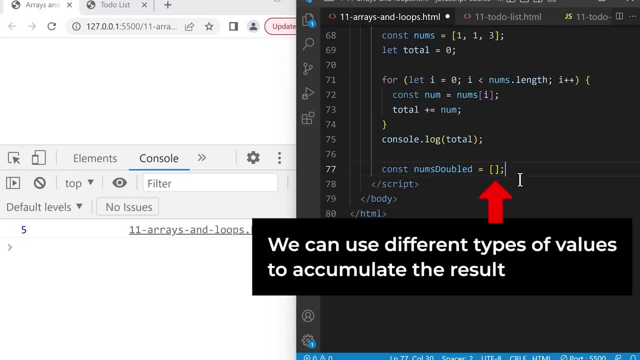 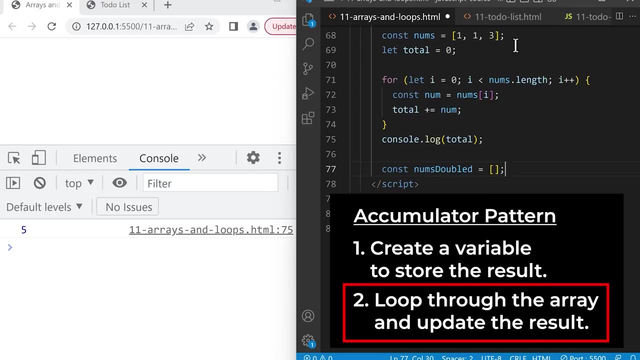 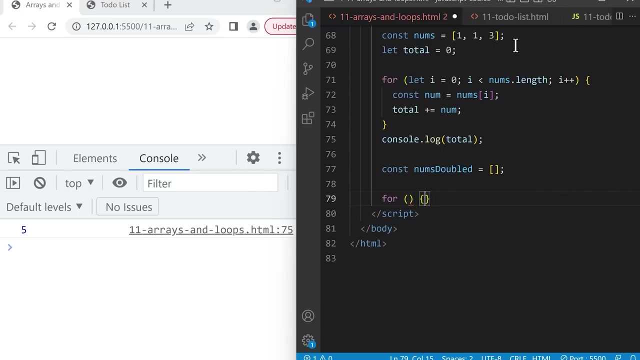 To An Array, So We Can Use Different Types Of Values To Accumulate The Result. It All Depends On The Problem We're Trying To Solve. 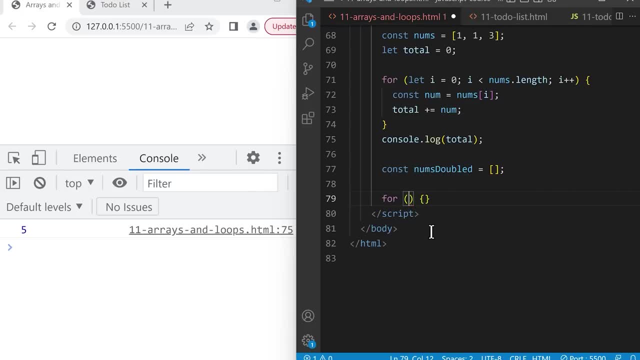 So Now The Next Step Is To I Equals Zero And We'll Create The Loop Condition I Less Than Nums Dot Length, And Then The 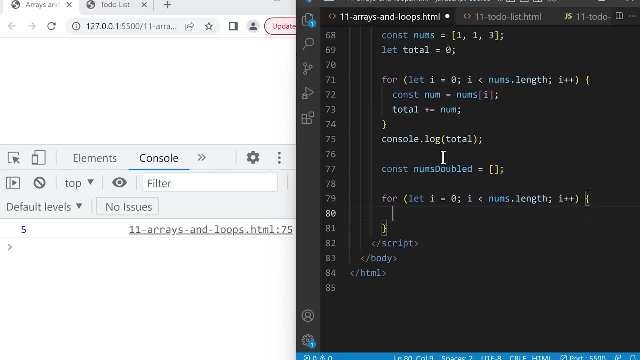 Increment: Step I: Plus, Plus. And Now, Between The Curly Brackets, We're Going To Add The Result. So Down Here We're Going To Add: 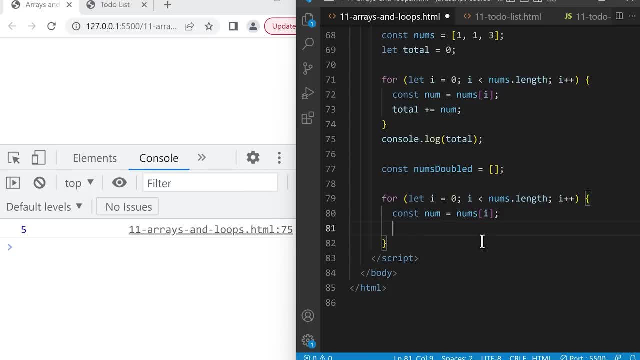 This Number Doubled To This Array. So Remember To Add A Value To An Array. We Can Add To This Array The Number Num Multiplied. 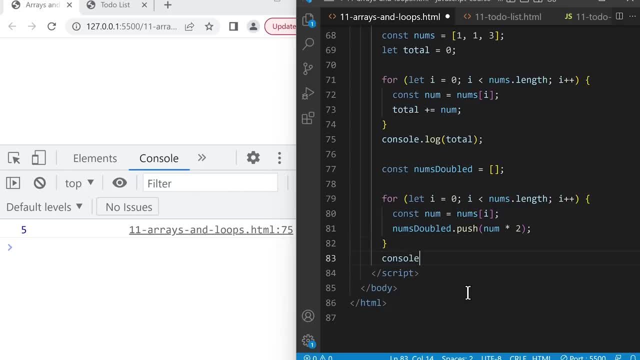 By Two. And Now At The Bottom, Let's Console Dot Log: The Result Nums Doubled And Save. So This Second Example. Alright, Now That. 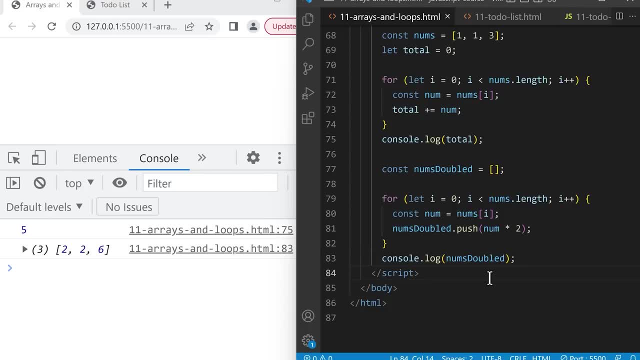 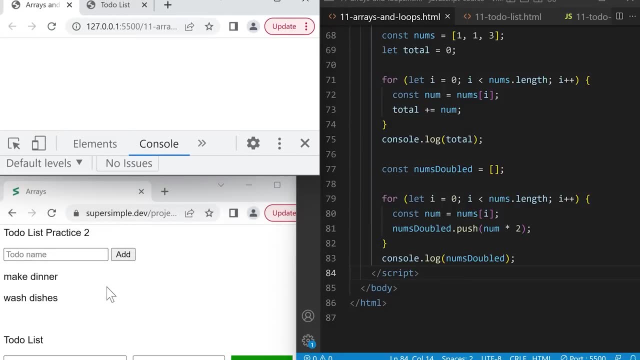 We Understand How To Loop Through An Array And The Accumulator Pattern. Let's Go Back And We'll Create The Second Version Of Our To. 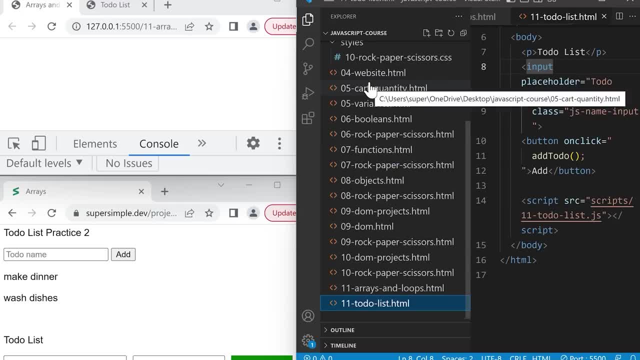 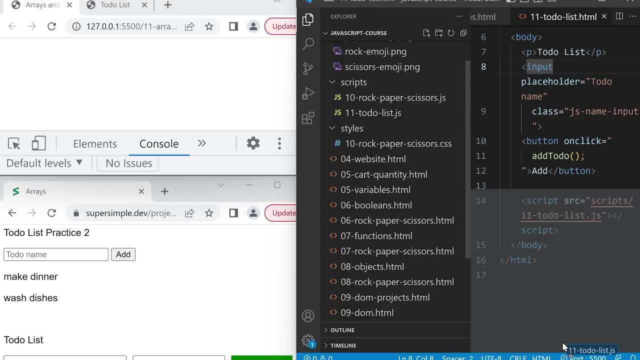 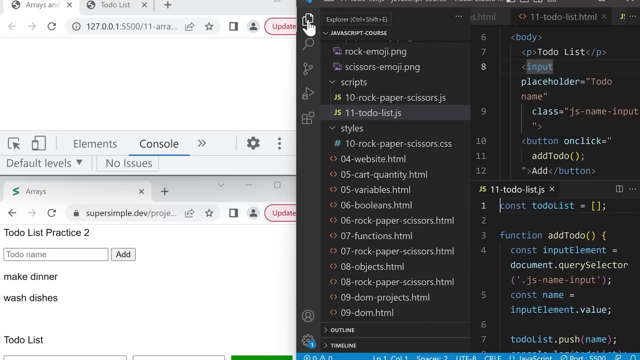 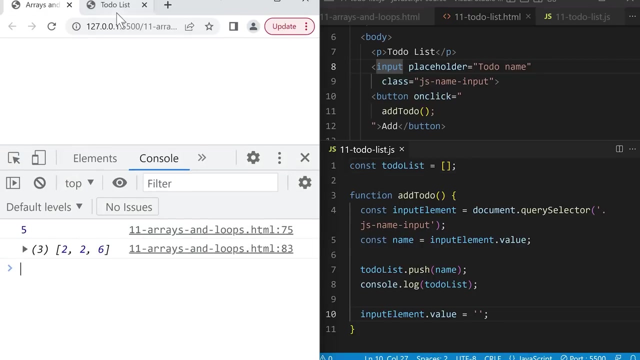 Do List And Open The JavaScript File. So It's This One, And For The Video, I'm Going To Drag It To The Bottom Of My 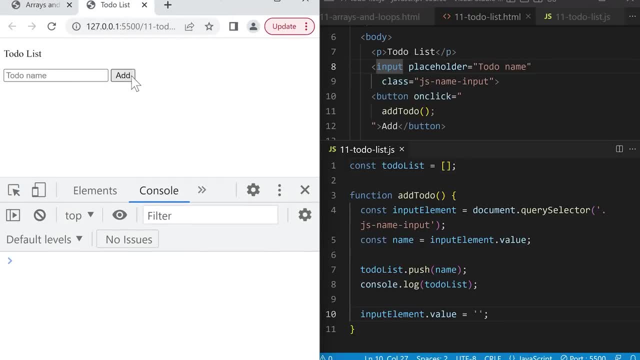 Code Editor So That I Can Click In This Text Box And Type A To Do Like Make Dinner And Click Add And It Will Add. 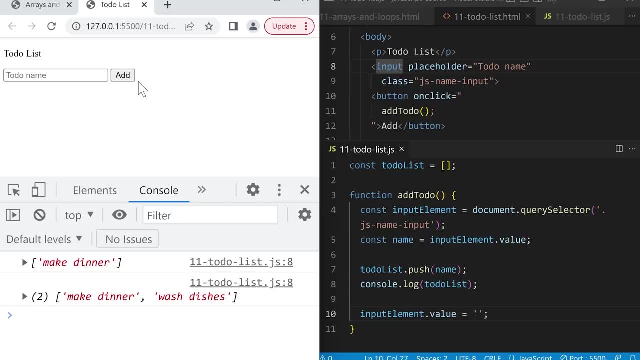 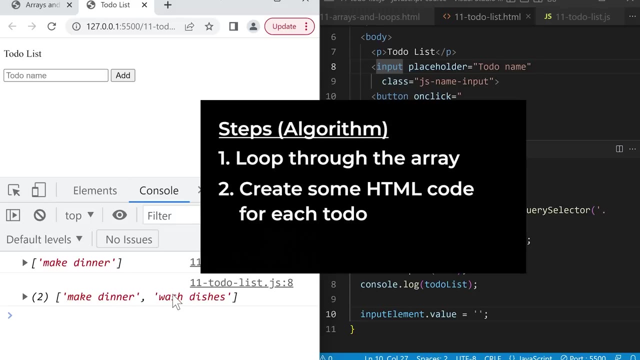 This To Do To This Array, Which Is This Array Of To Do's. We Want To Display It On The Page. To Do That, We're. 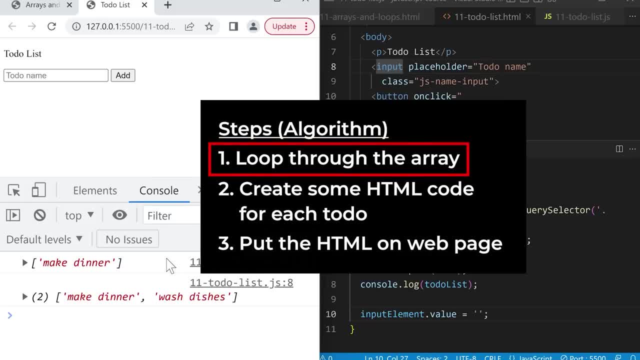 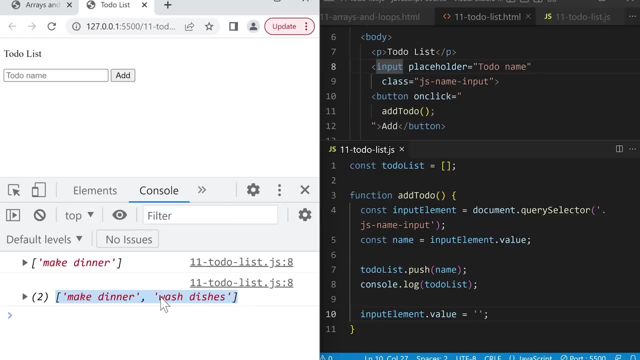 Going To Loop Through This Array And We're Going To Create Some HTML And Then Here We'll Remove This And Right Click And Paste. So 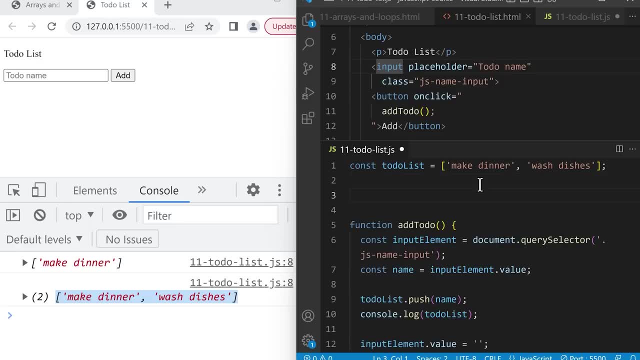 This Will Give Us Some Default Values To Work With. So At The Top, Let's Loop Through This. We're Going To Create The Loop Variable. 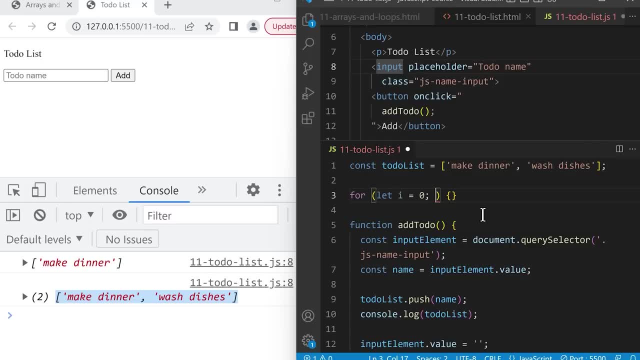 Let I Or Index Equal Zero Semicolon And The Loop Condition I, Less Than To Do List, Dot Length Semicolon And Then The Curly. 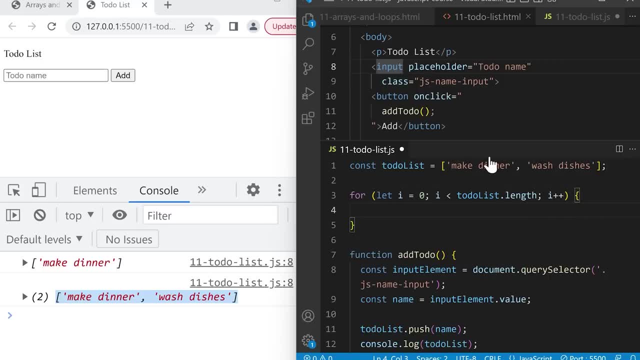 Brackets. Let's Get The String For Each Index, So We'll Create A Variable To Save It Const To Do And We'll Make It Equal. 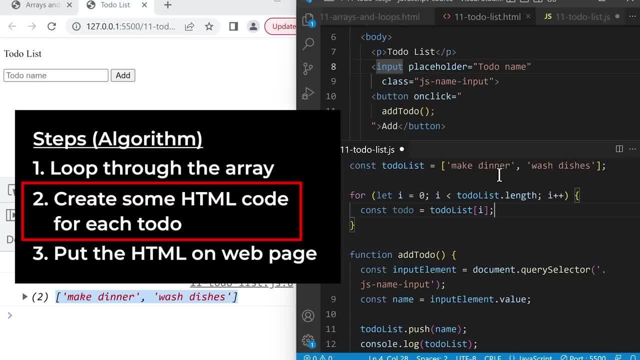 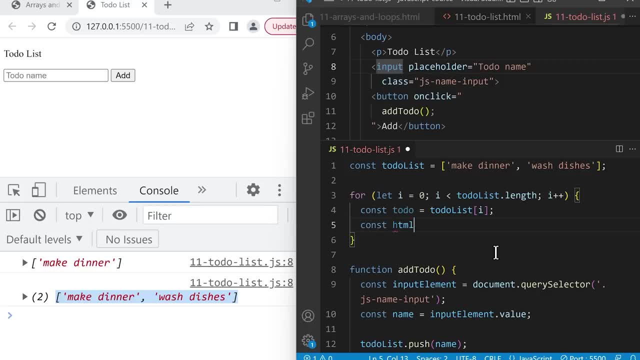 To To Do List. So We'll Create A New Line And Create A Variable Const HTML And Make It Equal And We'll Create Some HTML. 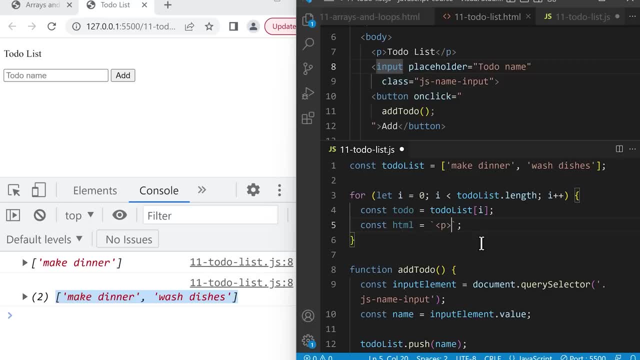 Code. Using This To Do Using A Template String Inside This Paragraph. We're Gonna Insert This To Do So, We'll Type Dollar And Curly. 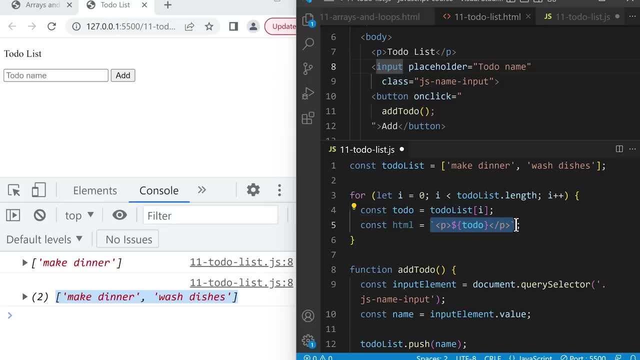 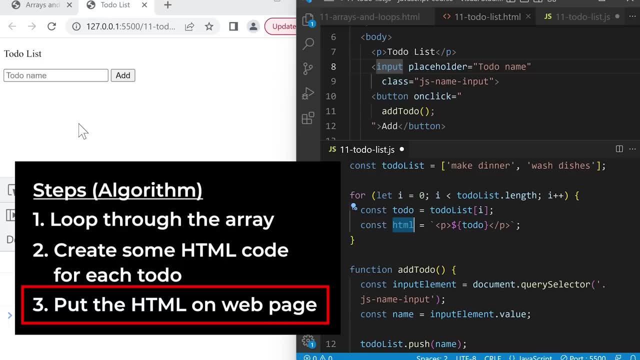 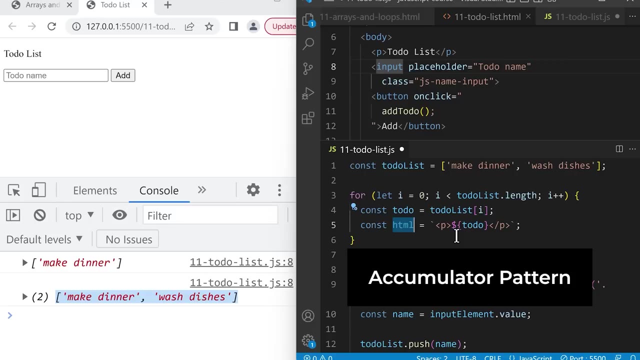 Brackets And To Do All Right. So Now We're Looping Through This Array And All Together We're Gonna Use The Accumulator Pattern. So 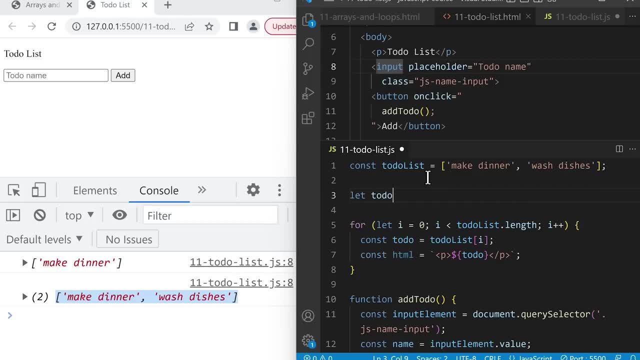 At The Top Of The Loop We'll Create A Variable To Store The Result. Let To Do List Capital HTML And Up Here. So Let's. 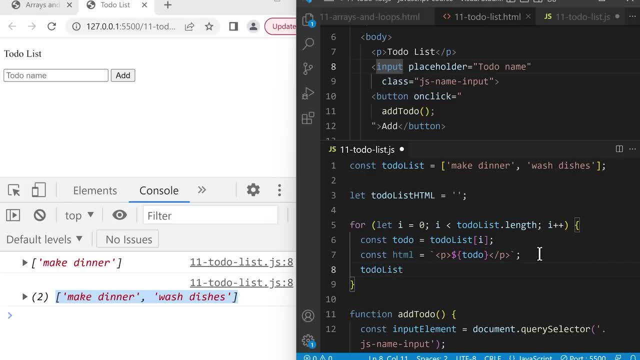 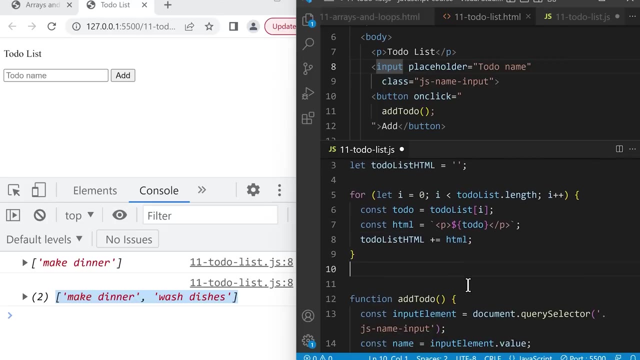 Create A New Line- And We'll Do- To Do List Capital HTML Plus Equals HTML, To Combine All Of This HTML Code Together. So Now, 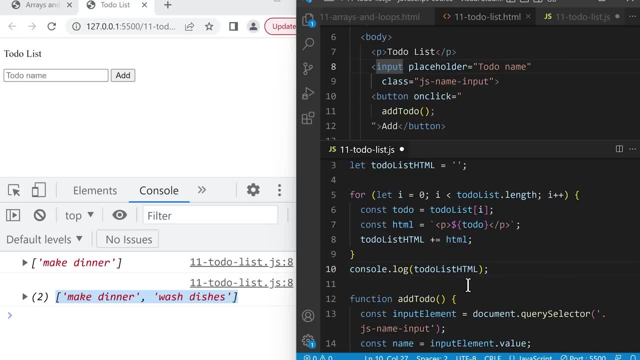 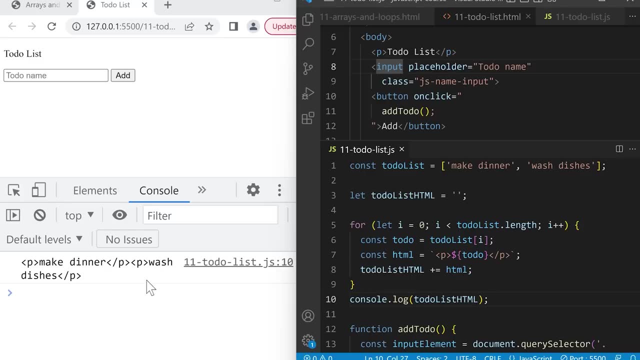 After We Create This HTML, To See What We Get If We Save, We Took This Array Of Strings, Generated Paragraph Elements For Each String And. 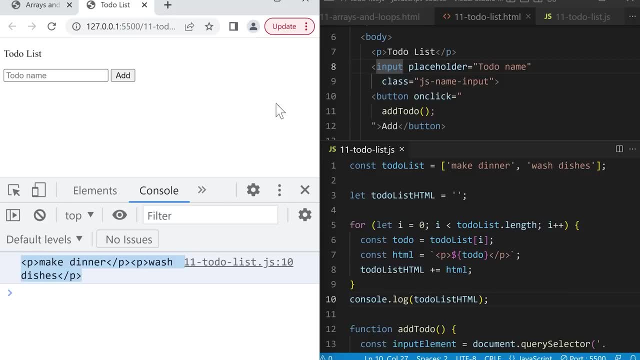 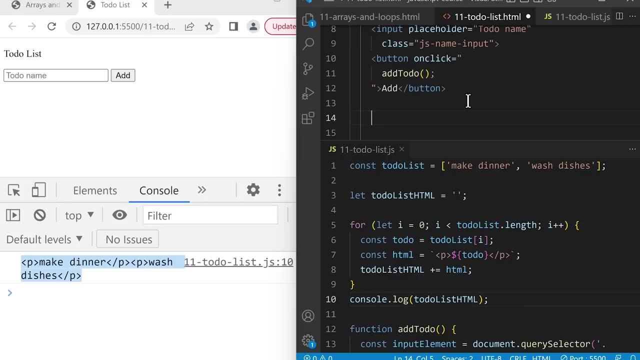 Then Combine Them All In The HTML File. After The Button. We're Going To Create A Different Type Of Element, Called A Div Element. So 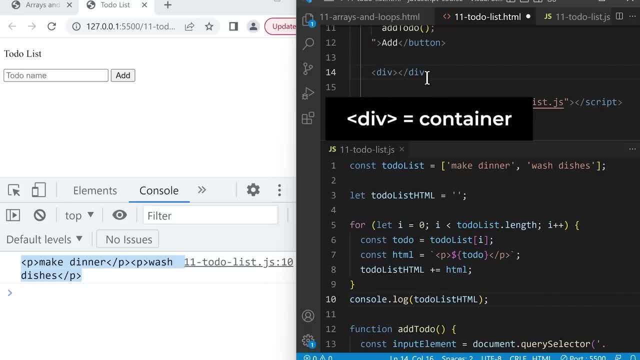 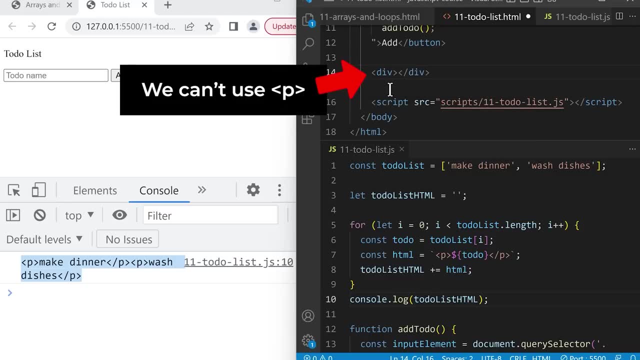 We'll Type Less Than Div, Greater Than So. In This Situation We Can't Actually Use A Paragraph Element, Because In HTML We Cannot Have A. 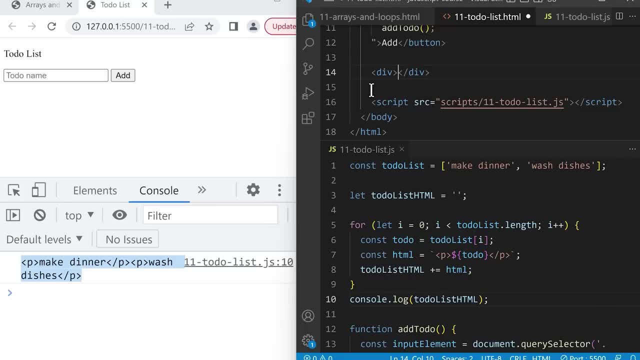 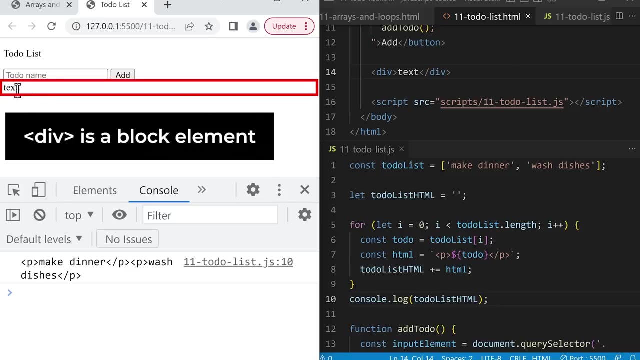 Paragraph Inside Another Paragraph. So That's Why We Have To Use A Paragraph Element. The Div Element Is A Block Element. That Means It Will. 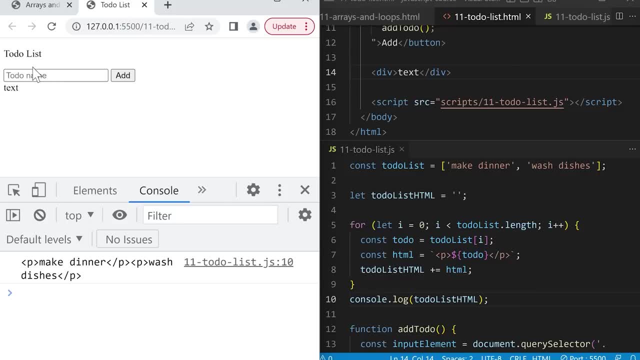 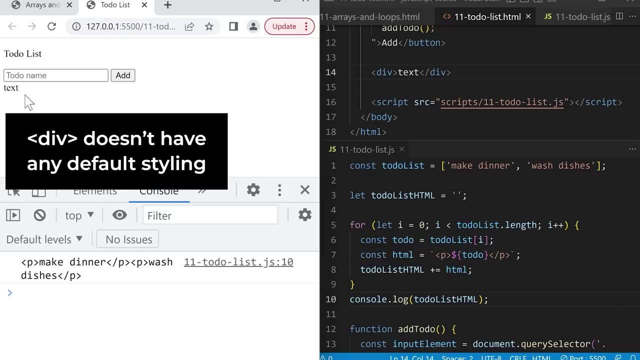 Take Up An Entire Line By Itself And That's Why It Appears Below The Text Box, So It Doesn't Have Any Default Styling, Alright. 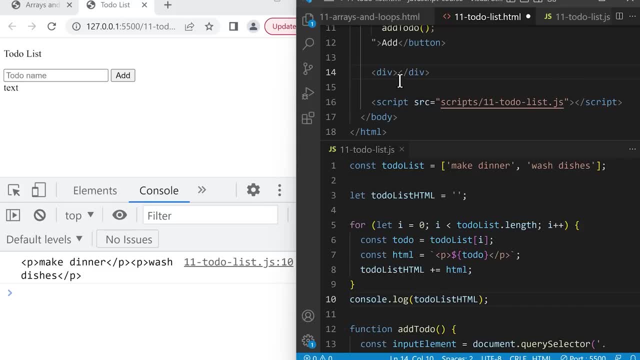 So Now That We Learned The Div, Let's Put This HTML Code Inside This Div. First We Need To Get This Dash List, And Then 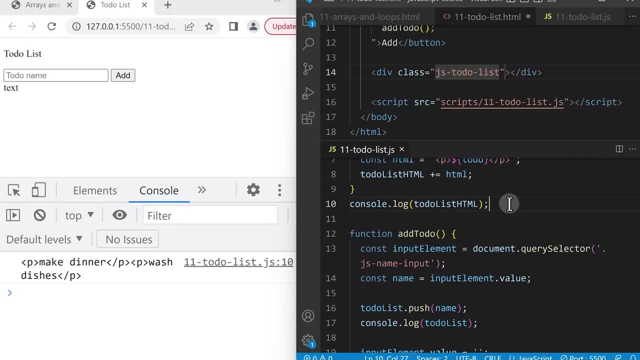 Down Here. Let's Scroll Down And We'll Put This Div Element Inside Our JavaScript. We Can Do That Using Document Dot Query Selector Brackets. 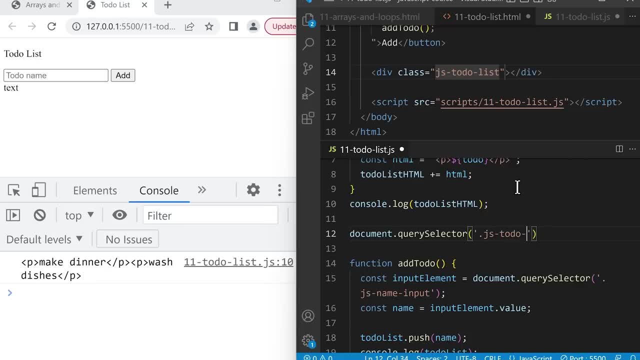 And A To Do Dash List. So This Will Get This Div Element And Put It Inside Our JavaScript And Then Every HTML Element Has A. 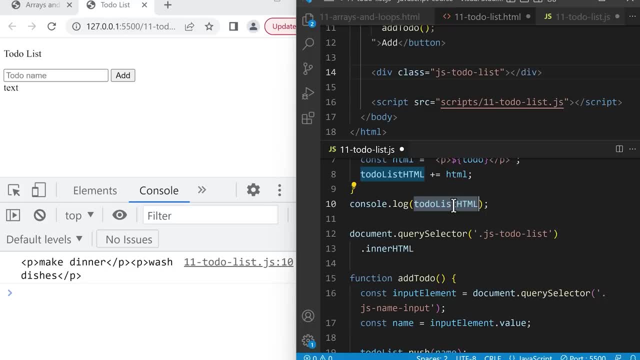 Property Called Dot, Inner Capital HTML. We're Going To Make The Inner HTML Equal To The To Do List HTML. And Now Let's Save This. 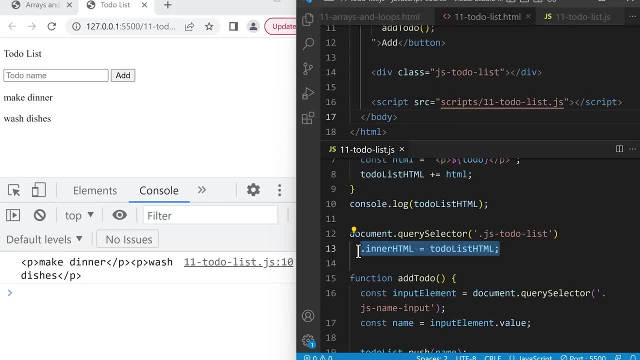 File And Also Save The HTML File, So This Code, And That's How We Make Them Show Up On The Page. So Now Let's Try. 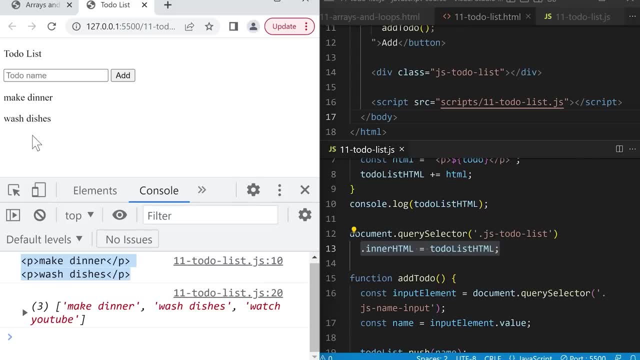 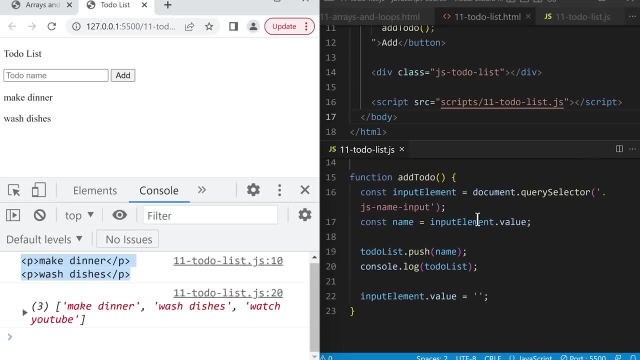 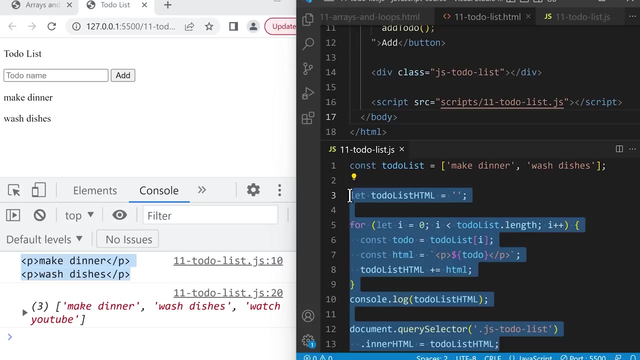 Adding Another To Do. We'll Type Watch YouTube And Click Add, And Unfortunately This Doesn't Actually Update The HTML On The Page. So To Update: 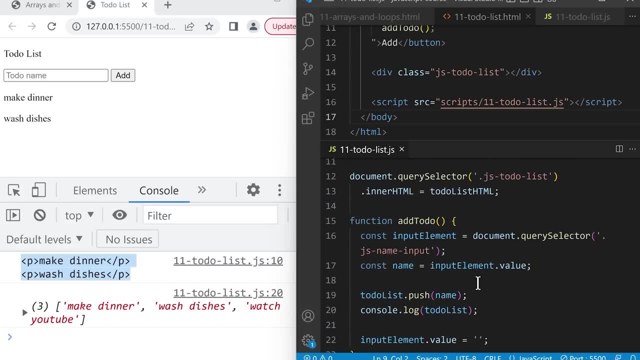 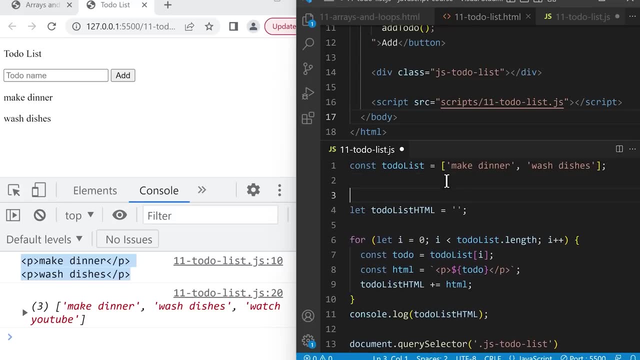 The HTML. We Need To Run All This Code Again Every Time We Add A To Do So. To Do List Brackets And Curly Brackets. 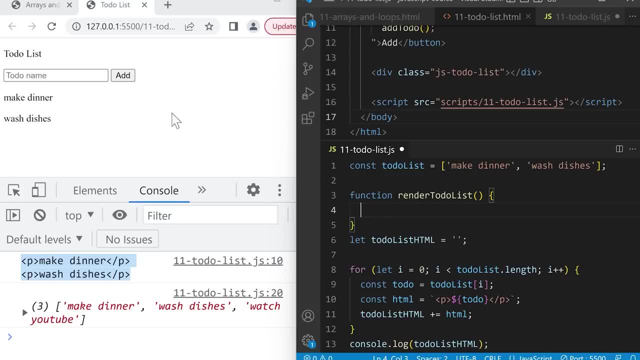 So The Word Render Means To Display Something On The Page. So We'll Put All Of This Code Into This Function. So We're Selecting. 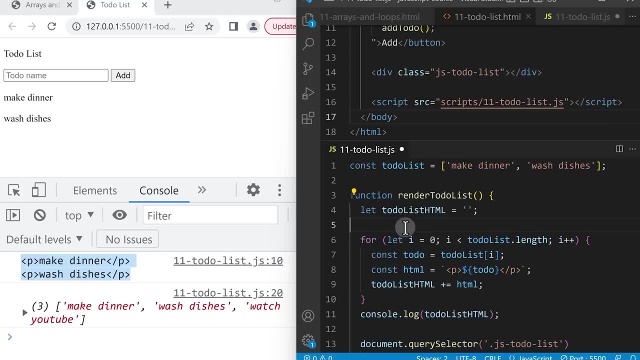 These Lines And Then Press Tab To Add An Indent. So Now Let's Use This Function. At The Start, We'll Display This To Do. 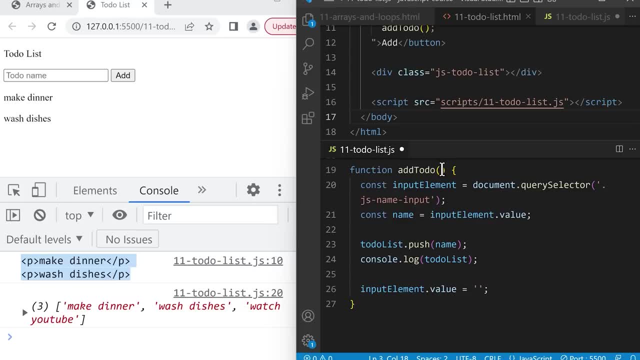 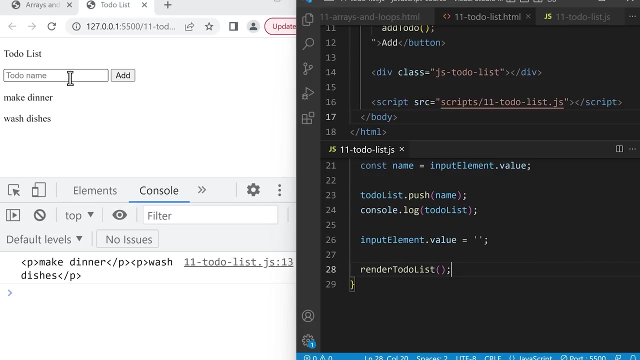 List On The Page. So If We Add A To Do To The List, We're Also Going To Display The List Again. So At The 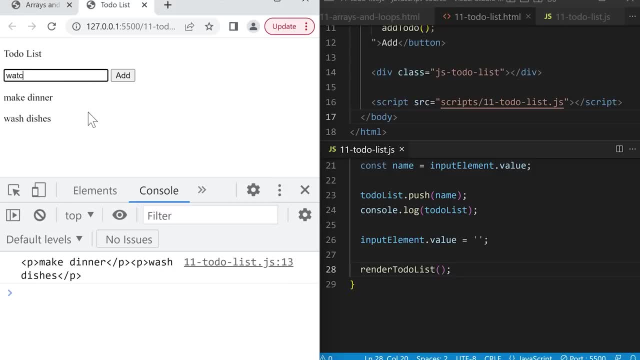 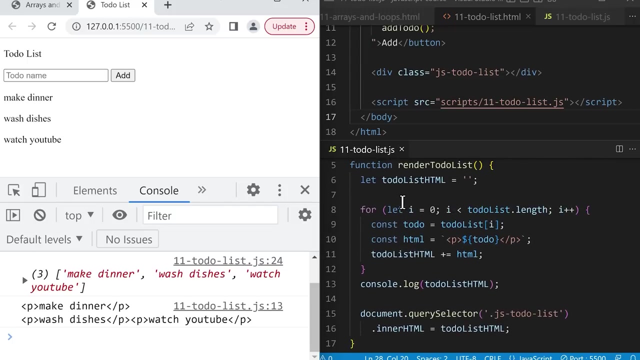 Bottom Render To Do List And Brackets Add. It Will Add It To The List And Also Display It On The Page. So That's How. 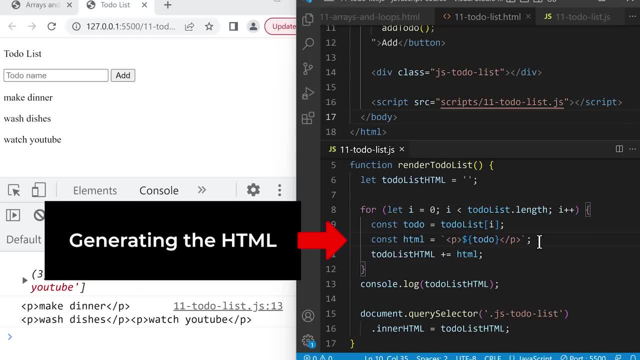 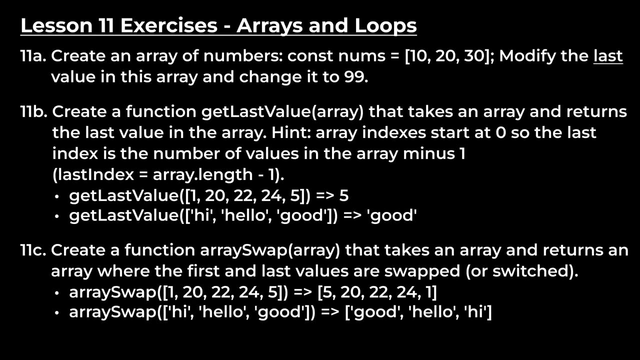 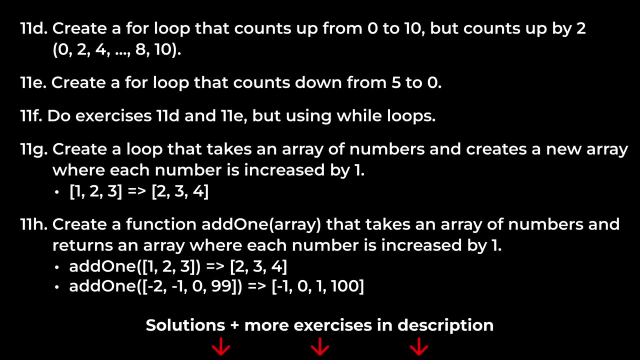 We Create The Second Version Of The To Do List Project And We Generated The HTML Using JavaScript. Let's Take A Break Before Continuing With. 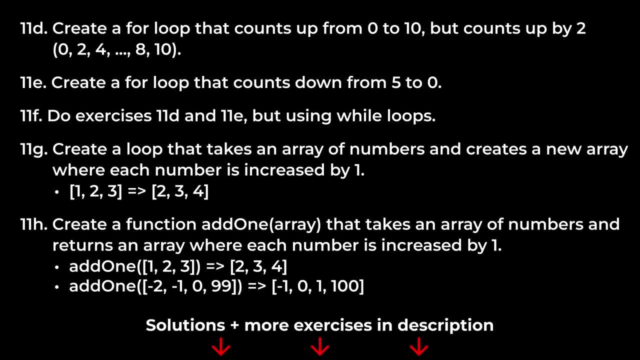 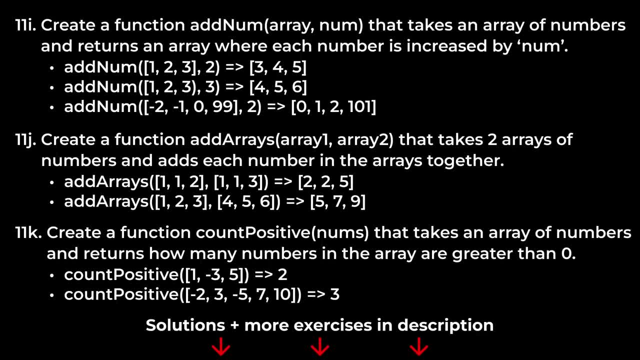 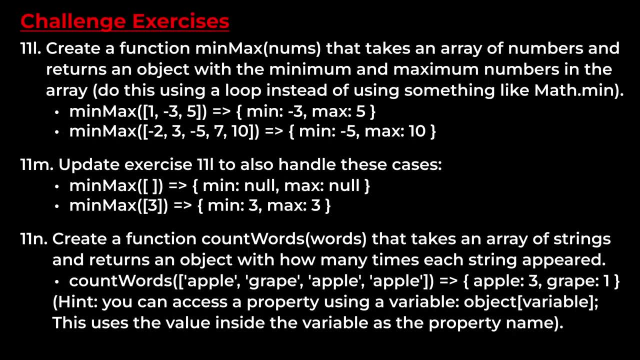 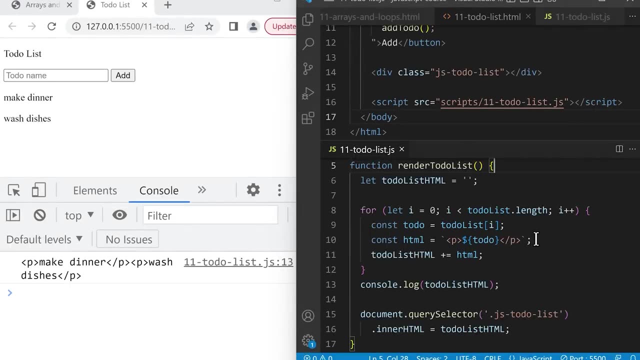 The Rest Of This Lesson. Here Are Some Exercises You Can Do On Your Own List. Now Let's Create The Final Version Of The To. 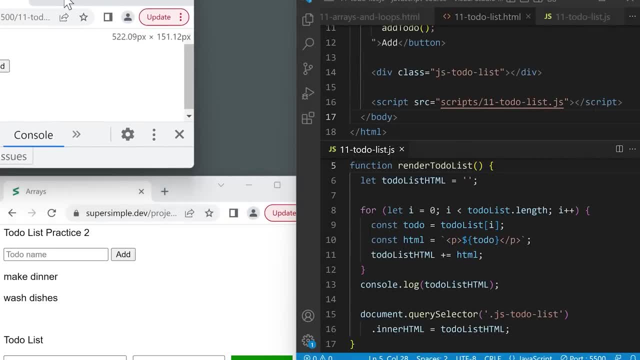 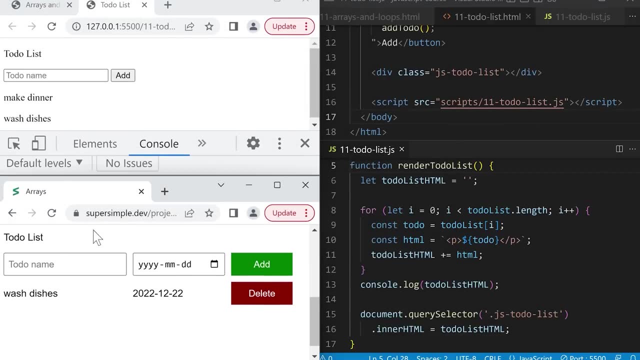 Do List. We'll Go Back To Super Simple Dev And Then Here We'll Scroll Down And We'll Create This Final. We Can Also Add: 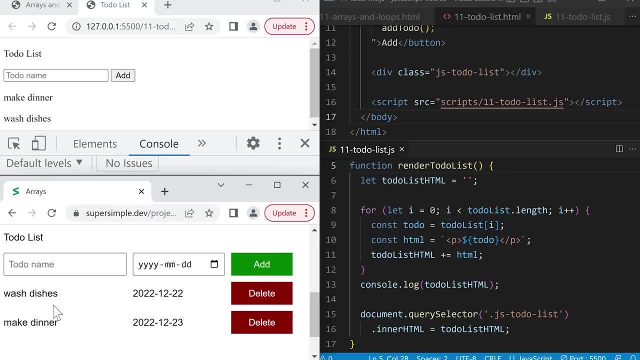 A Due Date And When We Click Add, Each To Do Will Now Have A Name And A Due Date And They Will Also Have Generating. 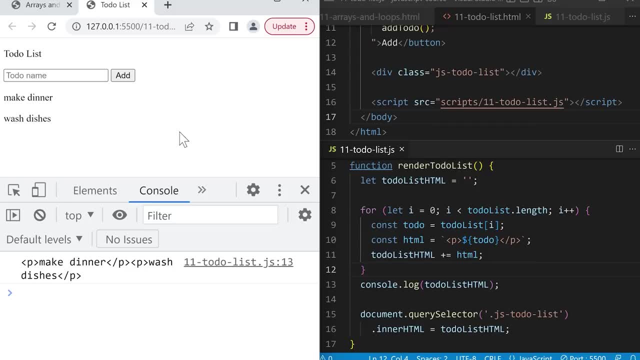 The HTML For The To Do List. So For Each Value In The Array We Create A Paragraph Element. So To Add A Delete Button. We. 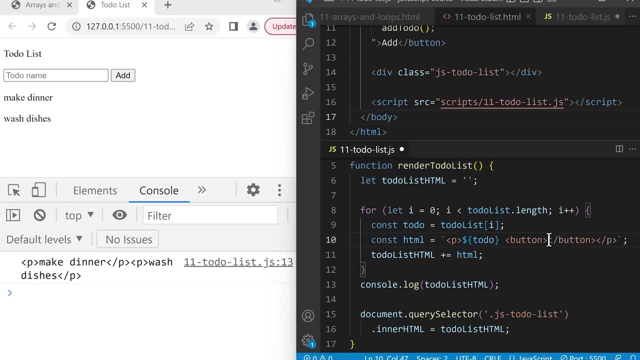 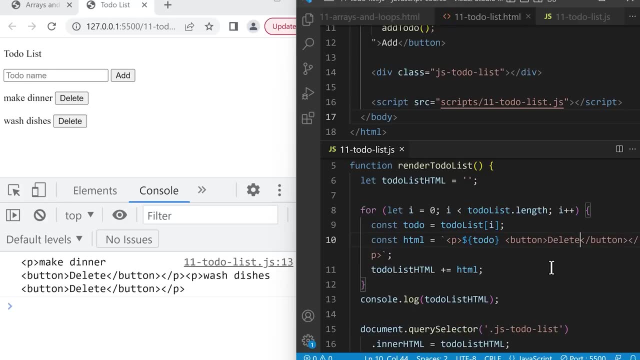 Just Have To Delete And Then Inside This Button We'll Put The Text Delete, Let's Save, And In The Console You'll See That The 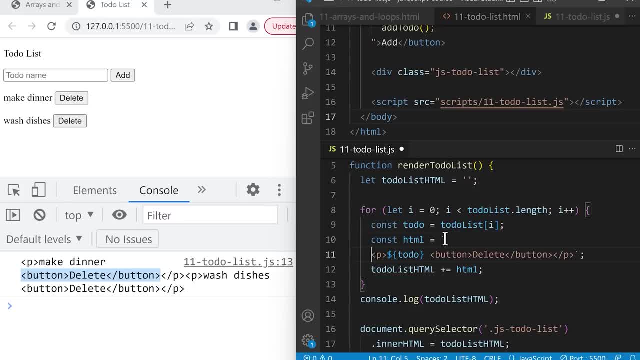 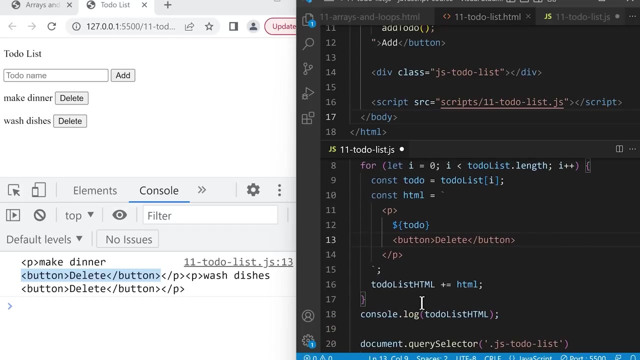 HTML We Generated Now Has A Delete, And At The End, And Let's Put The Content Of The Paragraph On Its Own Line, Like This: 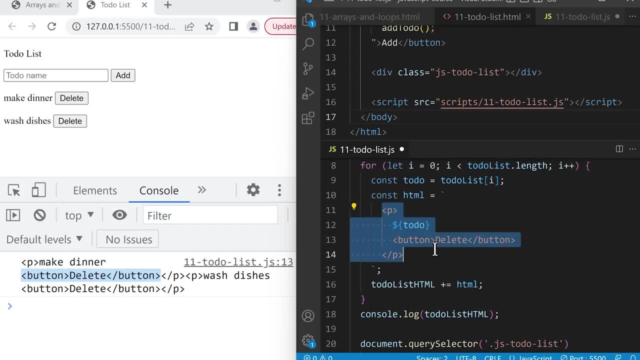 And Also Put The Delete Button On Its Own Line. So We Use The On Click Attribute As Usual. So Inside This Button We're Going. 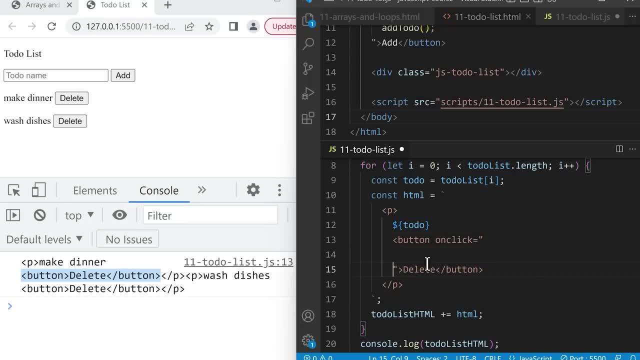 To Add An On Click Attribute Equals Double Quotes And Then Inside These Double Quotes. The Only Difference Now Is That Here We're Generating This. 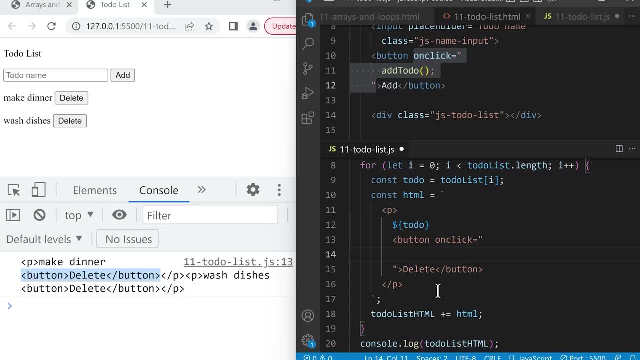 HTML Using JavaScript: Okay, So When We Click One Of These Delete Buttons, We Want To Remove This To-Do List Dot, Splice And Brackets. 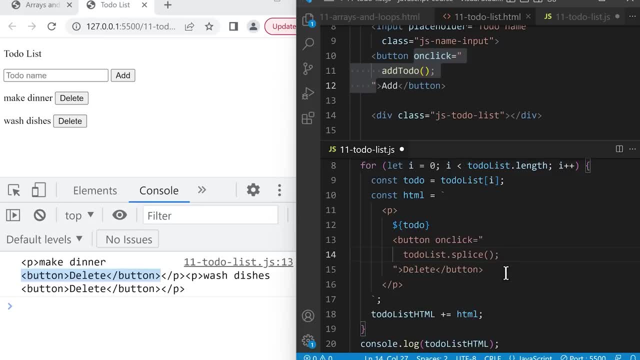 So Splice Takes Two Numbers. The First Number Is The Index That We Want To Remove. So If We Click This Delete Button, So We're. 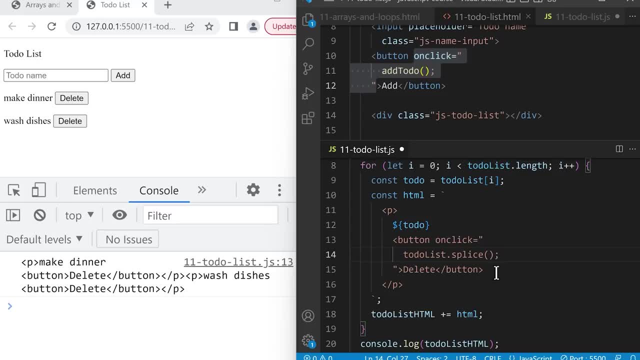 Going To Insert I Into This String And We Can Do That By Typing Dollar, Curly Brackets And I. Now Splice Also Takes Another. 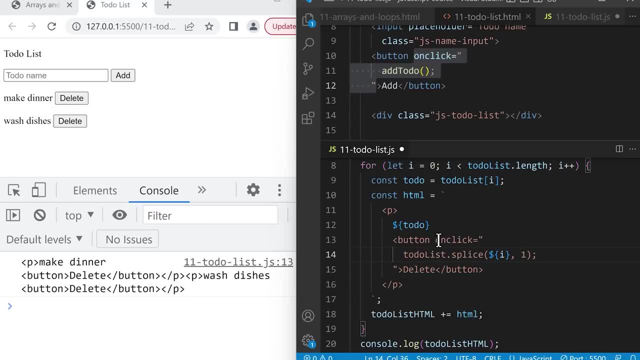 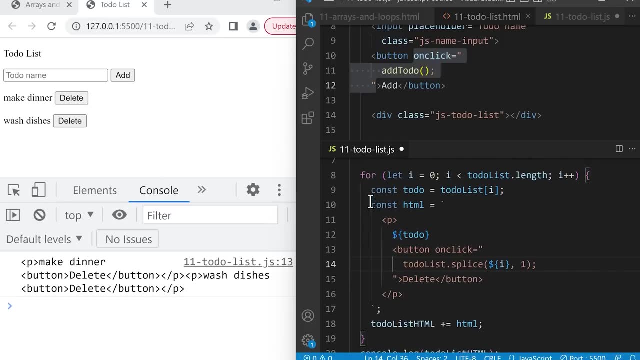 Number. So We'll Update The To Do List. We Need To Display The List Again On The Page. To Display The List We Can Use: 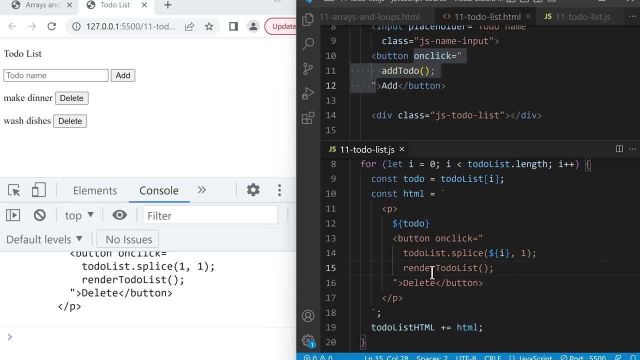 This Function Render To Do List. So When We Click The First Delete Button It Will Remove The Value At Index Zero, Which Is The First. 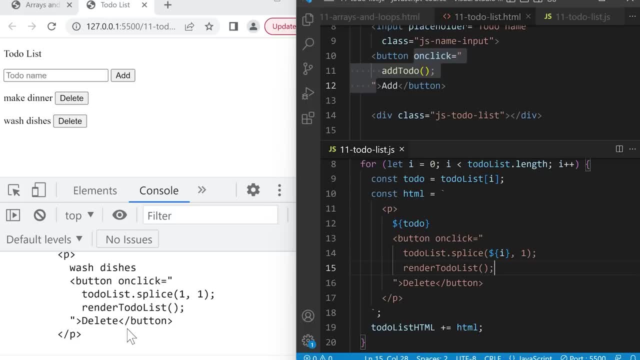 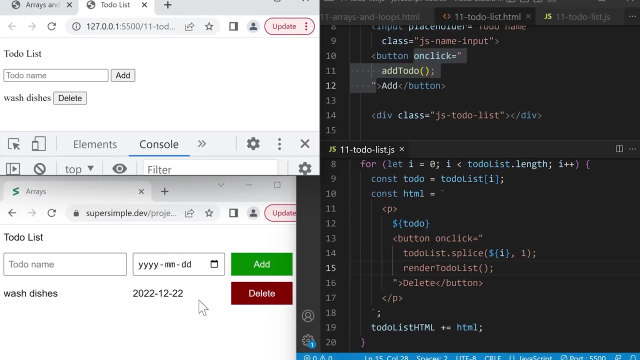 Value. If We Click The Second Button, It Will Remove And Then Display The Updated List On The Page. So That's How We Create The 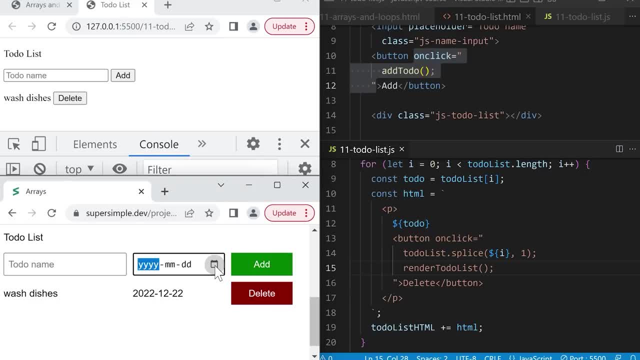 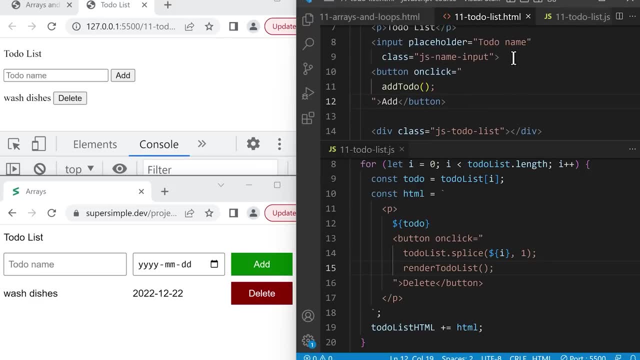 Delete Button. Next, Let's Go Back To Super Simple Dot Dev And We're Going To Our Input Element. So Less Than Input, Greater Than And. 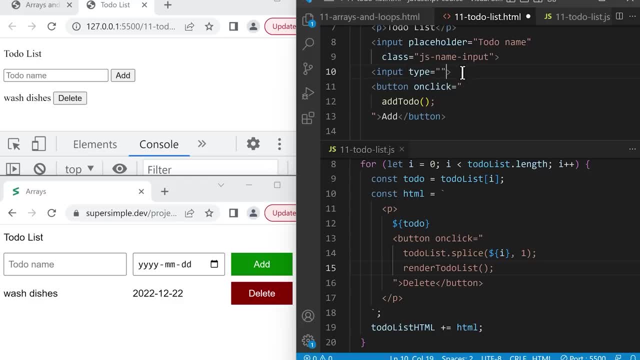 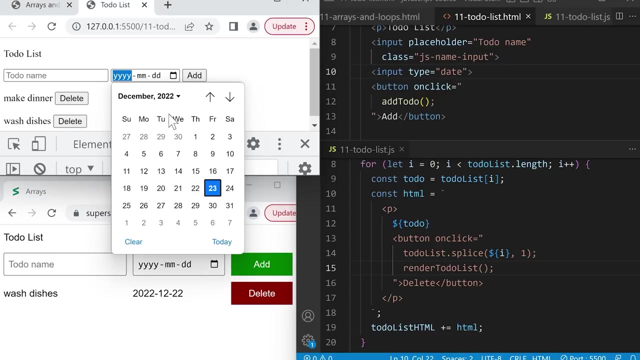 To Make It A Date Selector. Input Elements Have An Attribute Called Type, So This Attribute Determines What Kind And Save It's Going To Create. 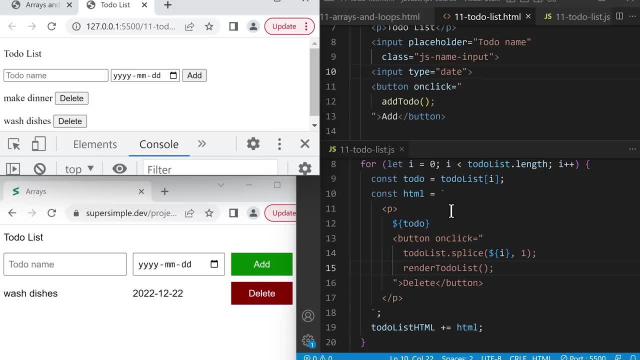 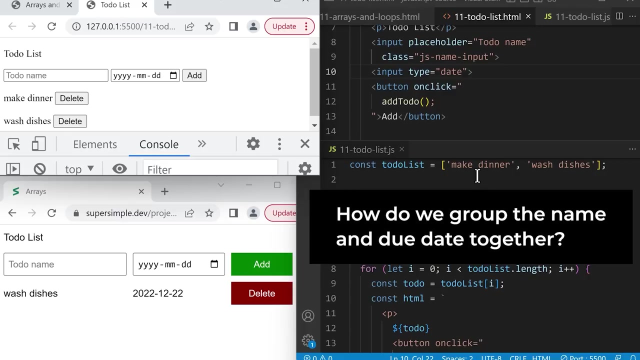 A Date Selector. Now Let's Go Back Into Our JavaScript Code, And First We're Going To Scroll Up And Remember That Right Now We Can. 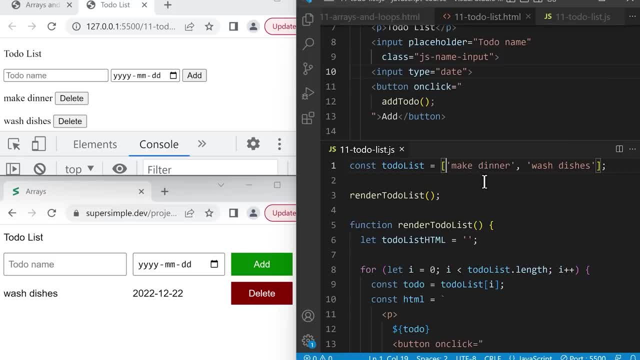 Do That Using An Object. So Here, Instead Of Just A String, We're Going To Create An Object And We'll Give It A Name: Property. 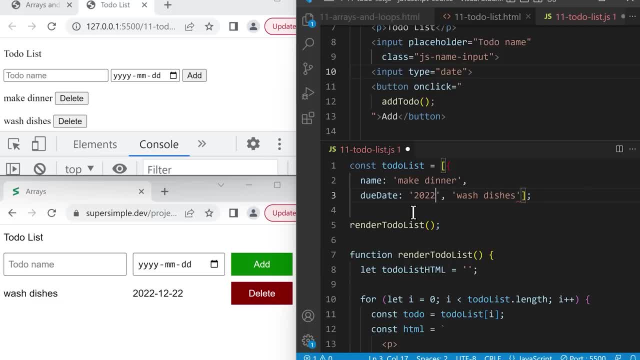 Which Is 2022.. Dash 12.. Dash 22. And I'll End This Object With A Curly Bracket And I'll Turn This Second To. 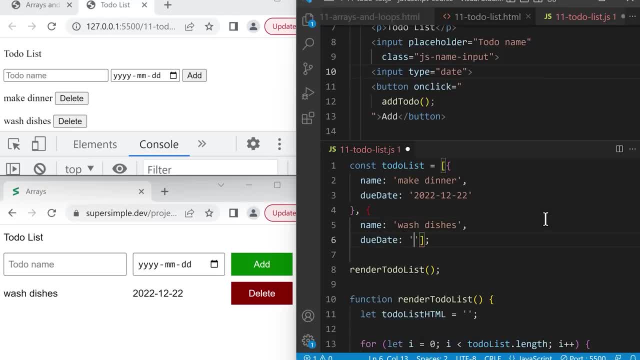 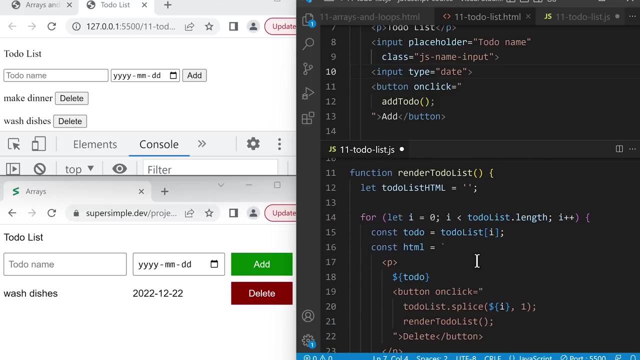 Do Into An Object As Well. So Open Curly To And Closed Curly Bracket, Now That Each To Do Is An Object We Need To. 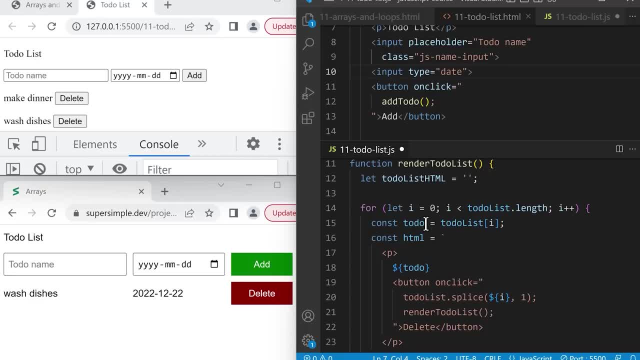 Update The Rest Of Our Code. Let's Scroll Down And We'll Start With It More Clear. And Now We Need To Get The Name And 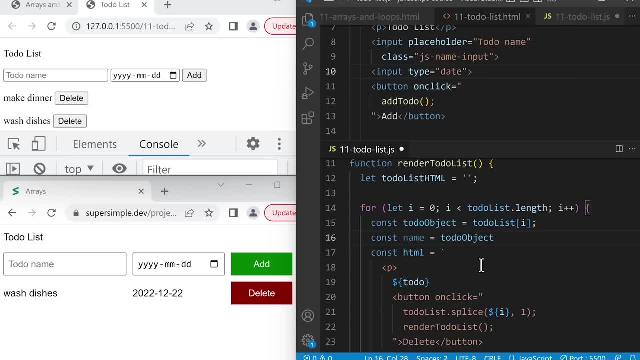 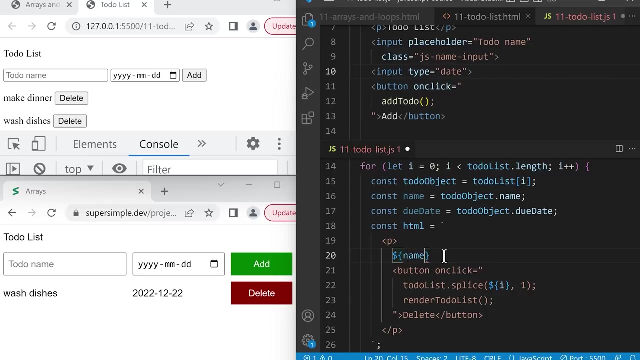 Due Date Out Of This Object. So We'll Type: Const Name Equals To Do Object Dot Name, And So Instead Of Inserting, To Do Which. 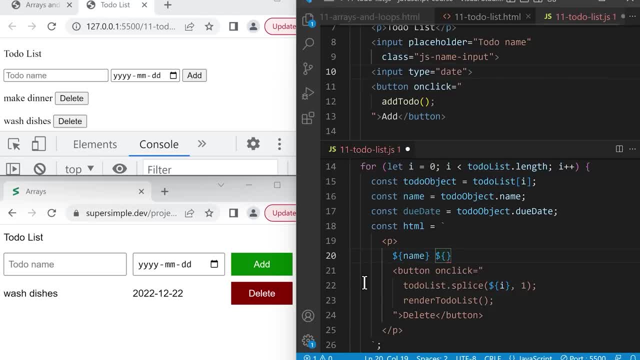 No Longer Exists. We're Going To Insert The Name And We're Also Going To Insert The Due Date. If We Save Now, Each You'll. 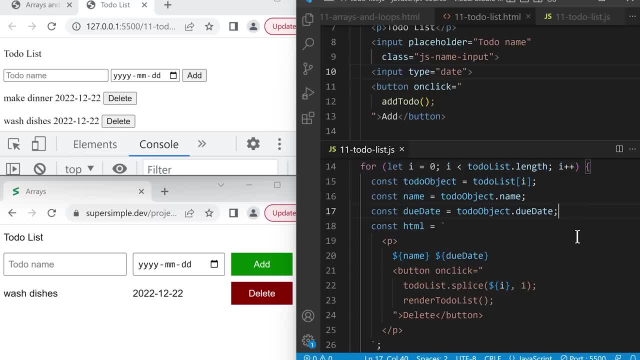 Notice: The Variable Name Is The Same As The Property Name. We Actually Have A Shortcut For This. Using Const Curly Brackets Name Equals To: 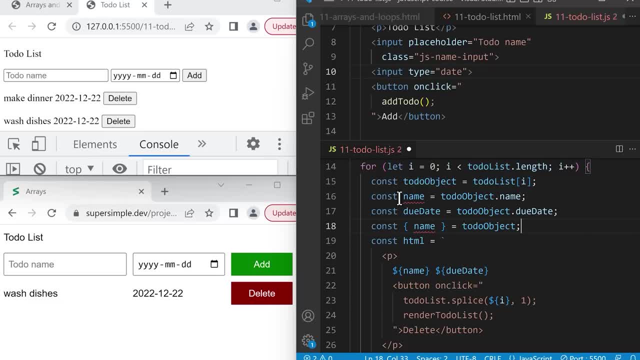 Do Object. So A Shortcut For This Line Up Here So We Can Comment Out This Line. We Can Also Use Multiple Properties In This Shortcut. 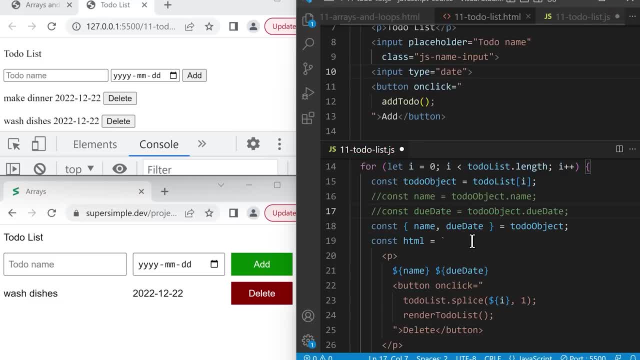 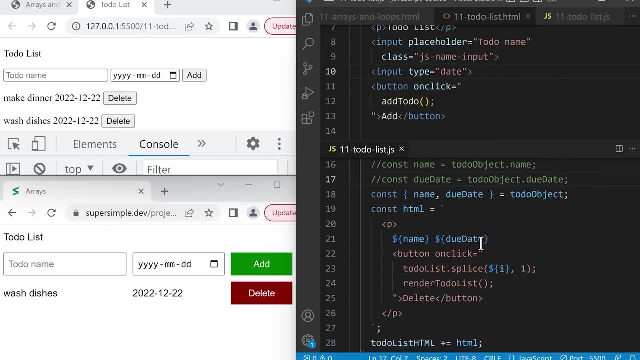 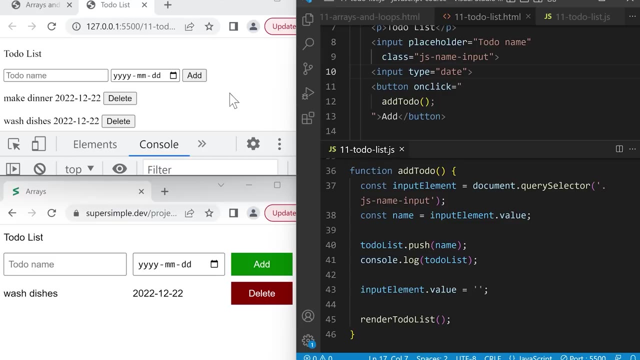 To Also Take The Due Date. Everything Still Works. Next Let's Scroll Down And We're Going To Update Our Add To Do Function. So This: 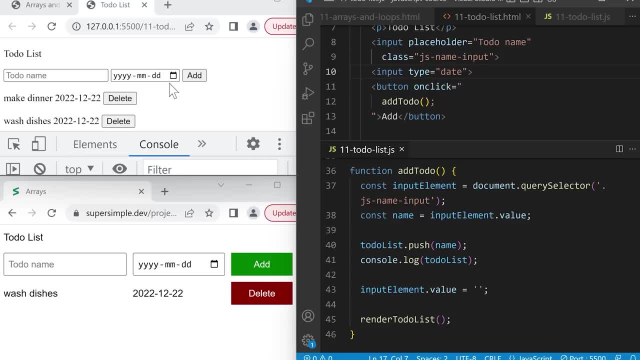 Time When We Click The Add Button, We're Going To A Class Attribute So We Can Get It Using Query Selector J S Dash Do. 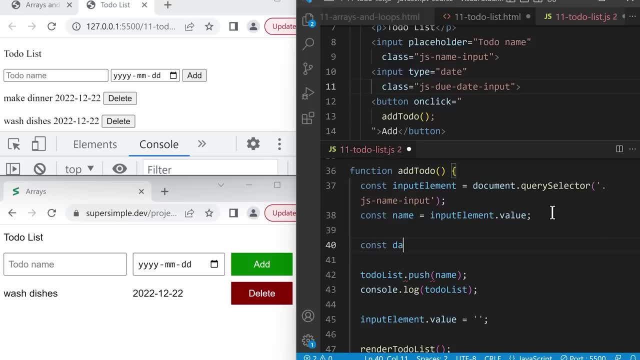 Dash Date Dash Input And Then Down Here Let's Create A Variable Const Date Input And A String Dot And Then The Class We Want. 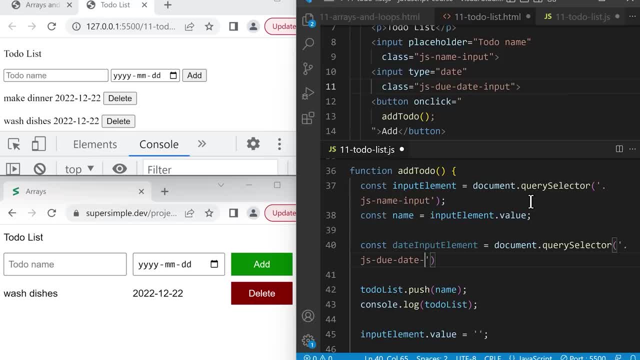 To Select Which Is This: Class J S Dash Do Dash Date, Dash Input. So This Will Get The Value. We Can Do That Using The: 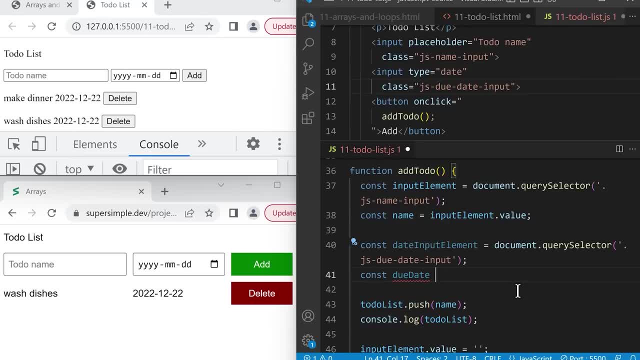 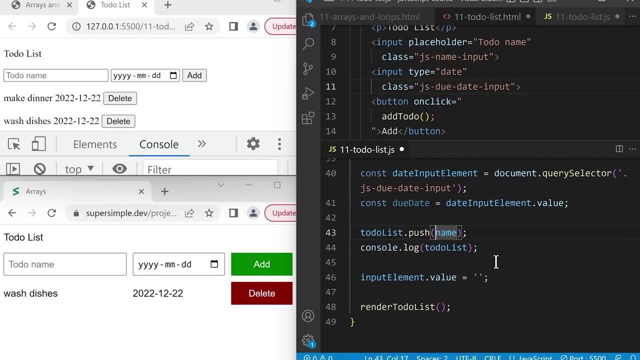 Value Property Again. So Let's Create A Variable First Const Do Date And We'll Make It Equal To The Date Input Element To Our List. 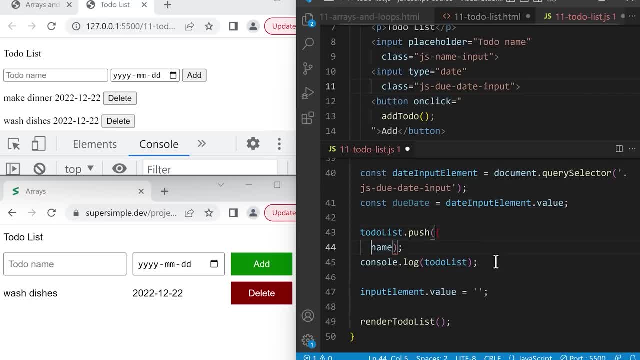 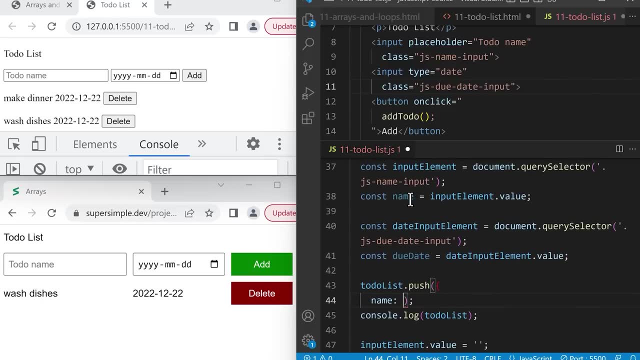 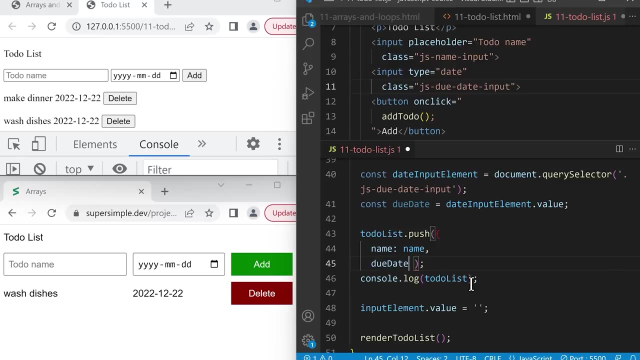 Instead Of Just A Name, We're Gonna Add An Object, So Open Curly Bracket. We'll Add A Name- Property- And The Value Will Be. 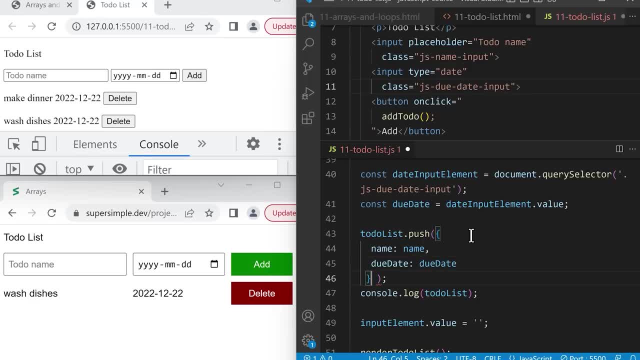 The Name Variable, A Closed Curly Bracket, And Remember That Objects Also Have A Shortcut For This If The Property And The Variable Name Are. 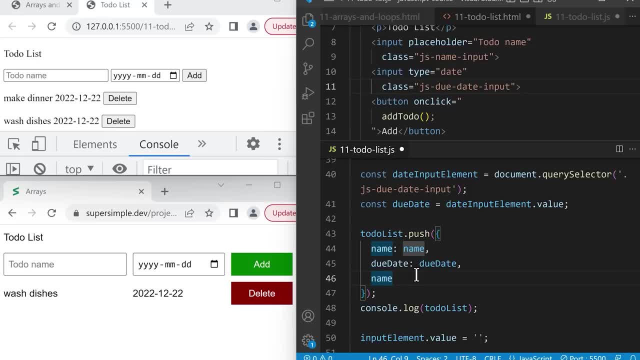 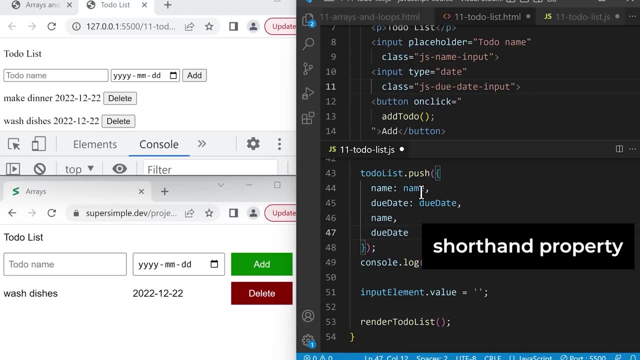 The Same. We Can Just Type A And Type It Out Once. This Is Called The Shorthand Property Syntax. So These Two Lines Do The 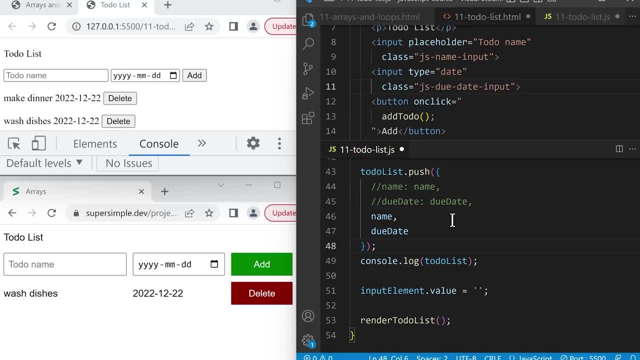 Same Thing As These Lines Above. So We Can Comment This Tml File And Let's Go To Our Project. We'll Add A New To. 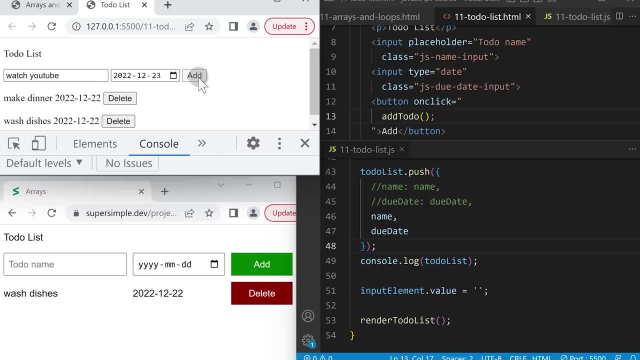 Do Like Watch YouTube And Select A Date And Click Add And Scroll Down. You Can See That To Do If We Click This One. It 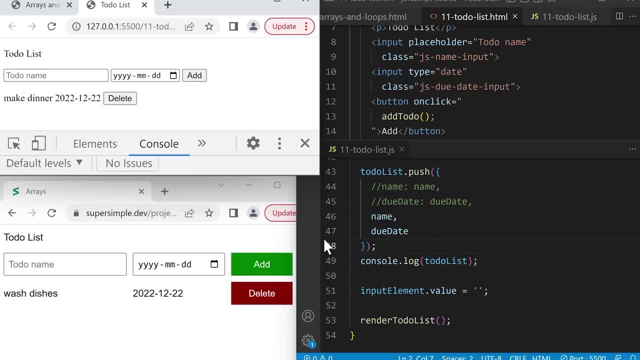 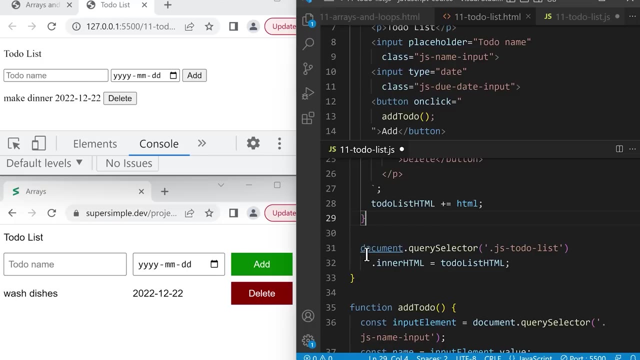 Will Also Remove The Correct To Do, And That's Actually All The Functionality That We Need For This Project. So Finally, Let's Add CSS. 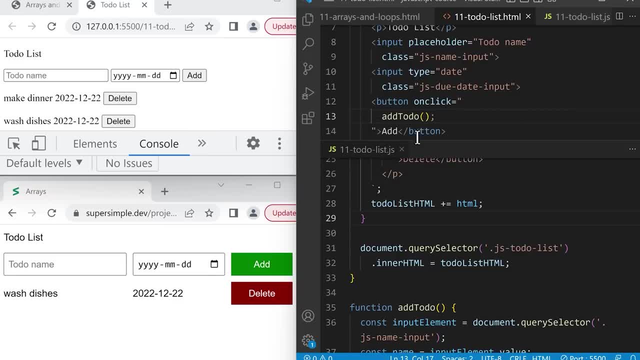 To Our Project To Make It Look Like The Final Design. We'll Go Into Our Code Editor And Scroll To The Top And Instead Of 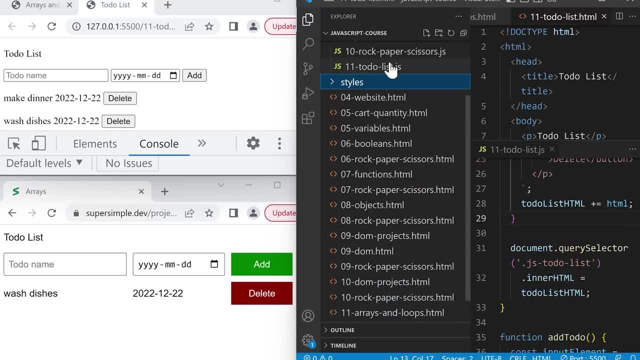 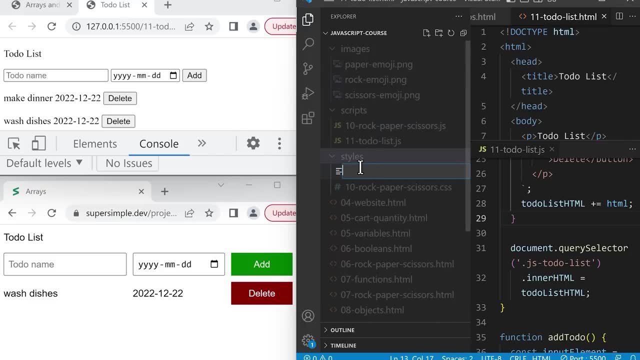 Writing And We'll Click The Styles Folder And Click This Icon To Create A New File Inside And We'll Name This File 11. Dash. 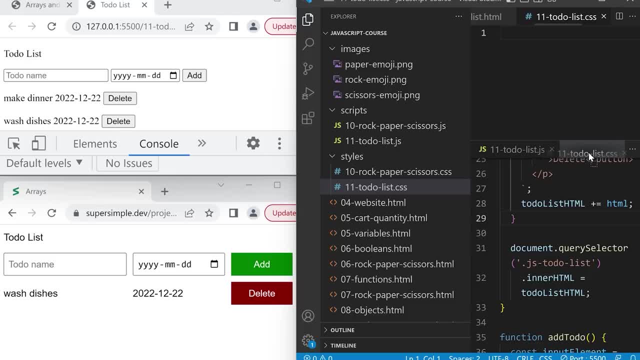 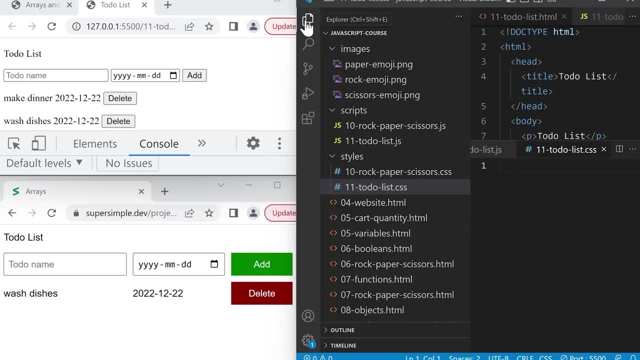 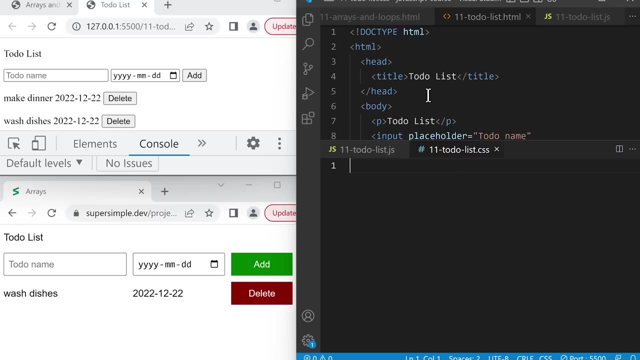 To Do Dash List, Dot CSS And Side By Side. And Now I'll Click Here To Close It And We'll Load This CSS Into Our 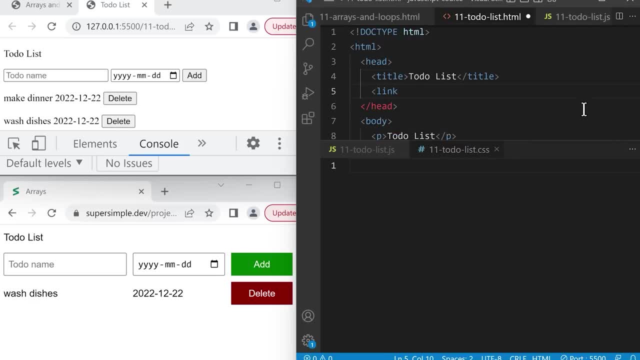 HTML. To Do That We Can Use A Link Element. So Inside This Sheet, And H Ref Equals The File That We Want To Load. So 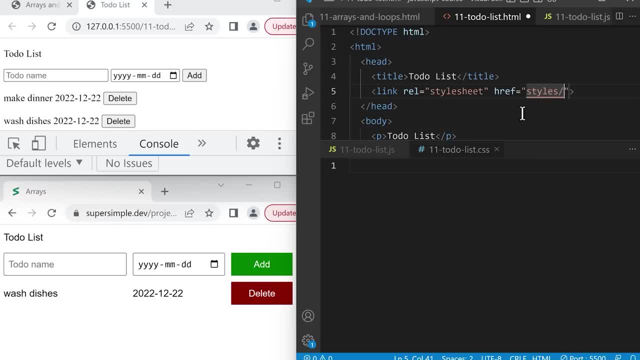 We Created This In The Styles Folder, So We'll Type Styles And Then A Slash Save. Now Let's Style Our Project One By One Until. 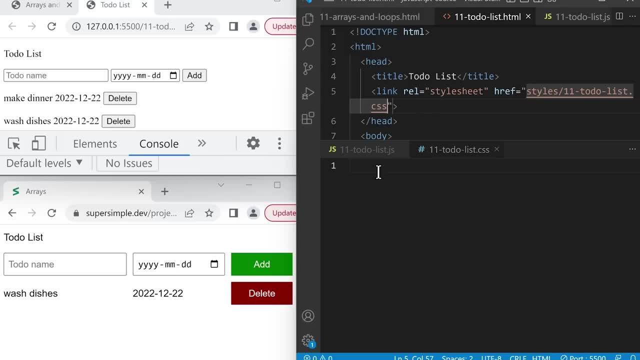 It Matches The Final Design. We'll Start With The Text On The Page. We're Going To Change The List, So That Looks Pretty Good Now. 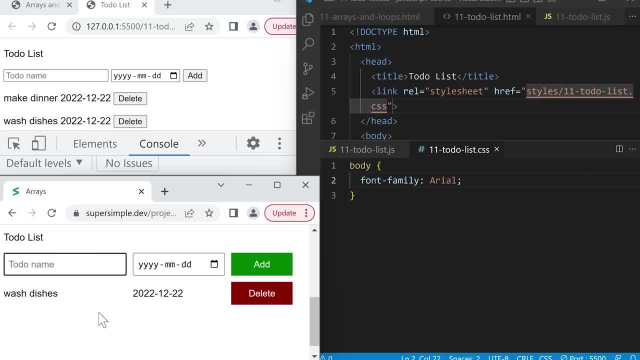 Let's Work On Styling The To Do List. First Let's Add Some More To Do's To The List, So We'll Type: Watch, Sort. 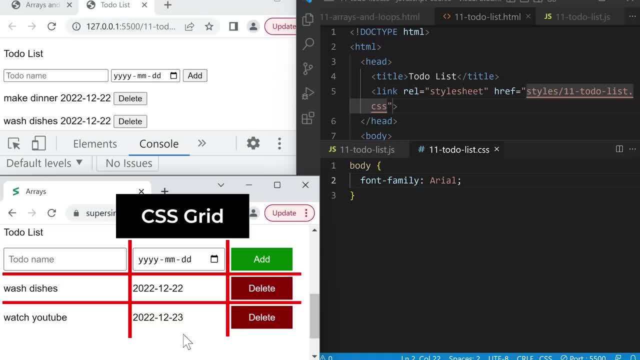 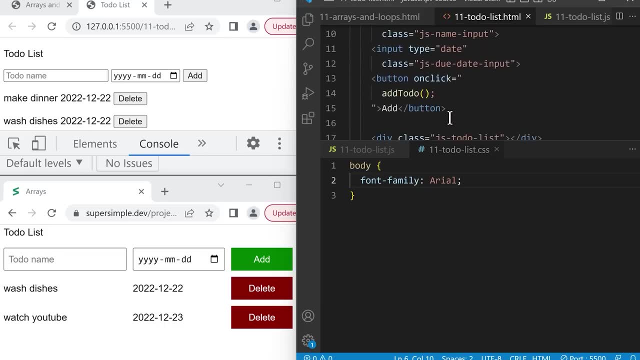 Of Grid. We're Going To Create This Grid Using A Feature Called CSS Grid, So Let's Go Into Our HTML First. We're Going To 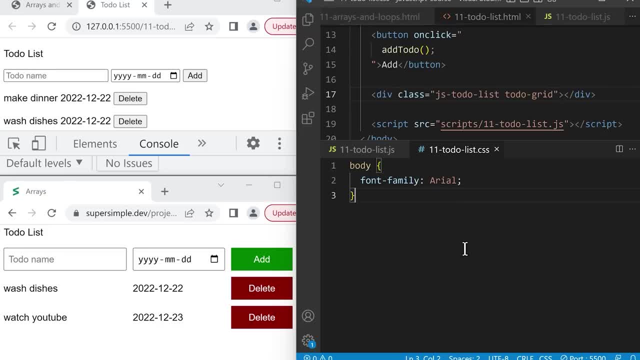 Add A Class To This Class, Using Dot To Do Dash Grid And Curly Brackets And To Turn This Into A Grid. We're Going. 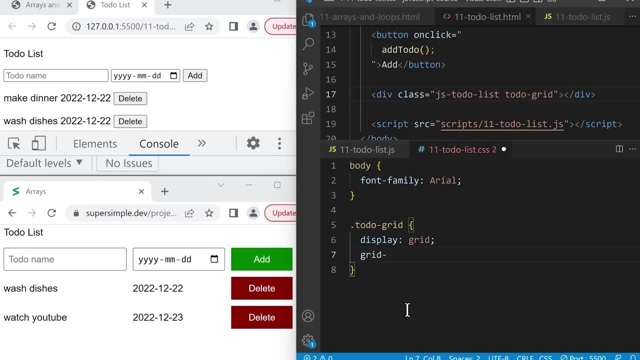 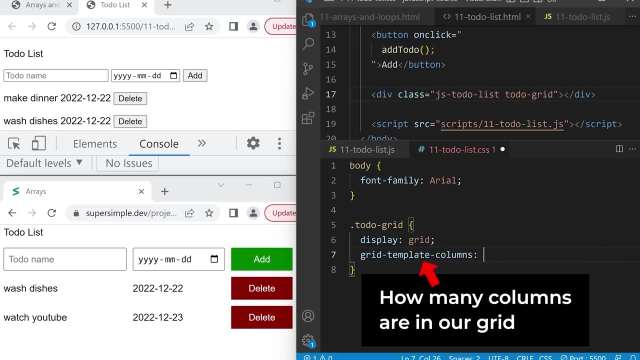 To Use The Property Display And Grid And We're Going To Add Columns To Our Grid. The Number Of Values That We Give It Is: 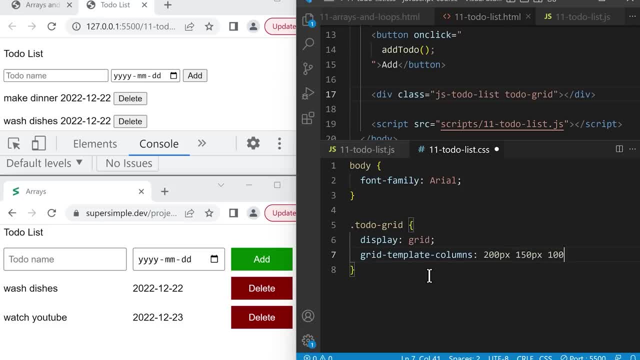 The Number Of Columns. For Example, If We Give It 200. Pixels, 150. Pixels, And The Third Column Will Be 100. Pixels. And Now, 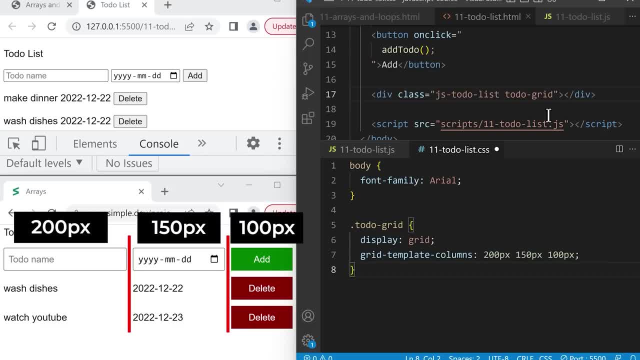 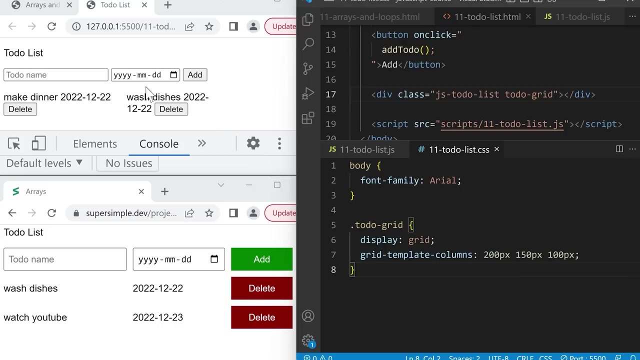 Each Element Inside This Div Will Go Into The Columns, So The First Element Will Go In The First Column We Save And Unfortunately That Didn't. 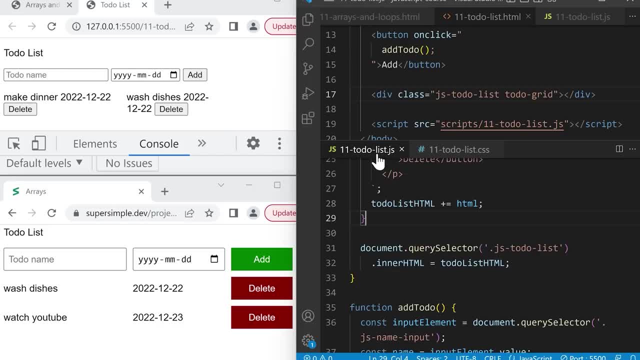 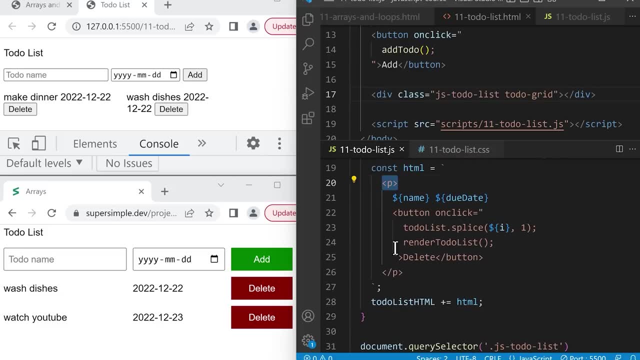 Quite Work, And That's Because, If We Go Back To Our JavaScript, Remember That Each To Do Is One Paragraph Element, So This Is A 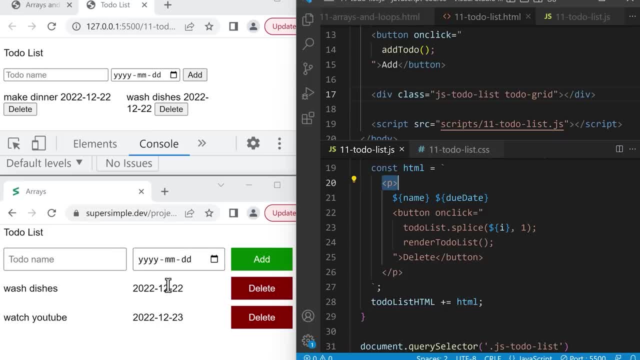 Paragraph. But What We Actually Want Is For The Name To Go In Column One, Due Date, Column Two, And Delete Button, Column Three. To Do: 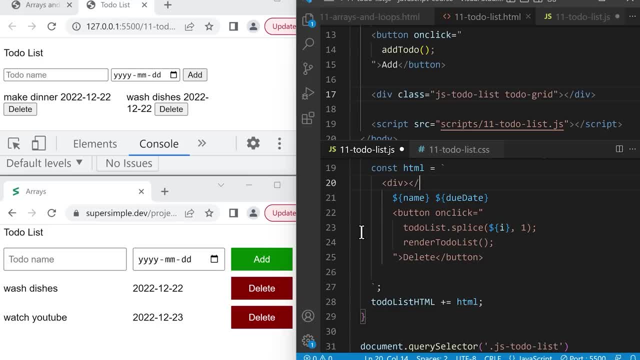 This Is Less Than Slash. Div, Greater Than And In Between Will Insert The Name. So The Reason We Use A Div Element Is Because Div 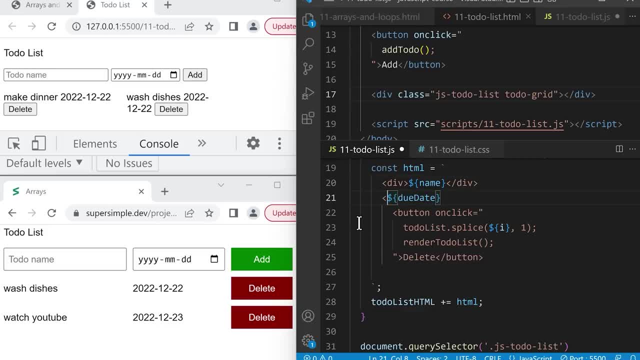 Elements Don't Have Any Default. And Then, At The End, Less Than Slash Div Greater Than. And Finally, For The Delete Button We Already Have. 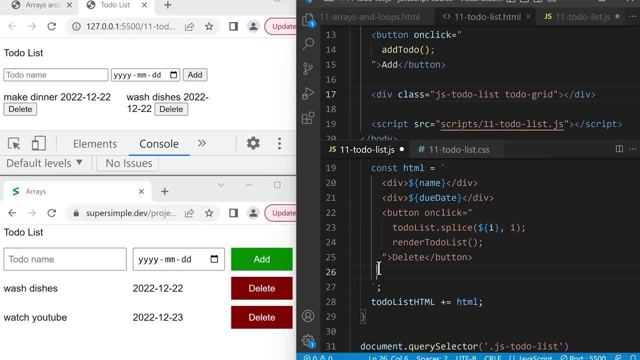 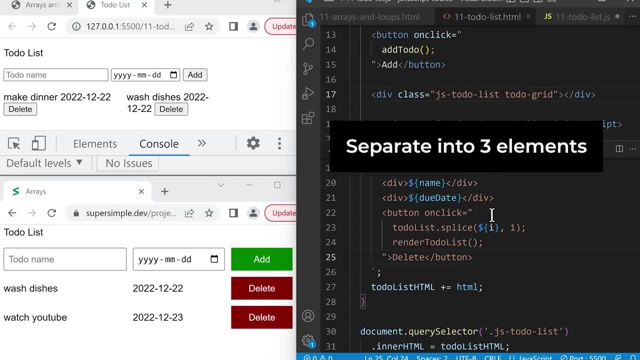 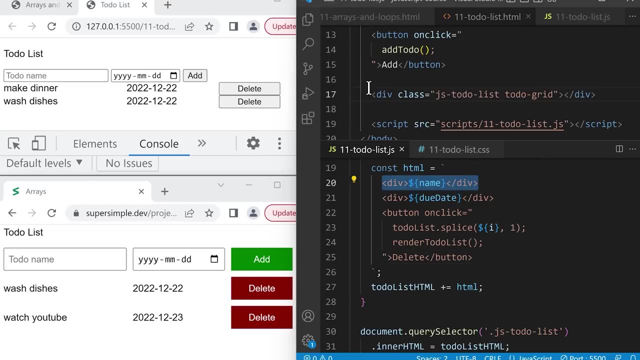 An Element. So Let's Just Reformat These Lines. We'll Select If We Save. Now The Grid Is Working Because This Element Goes Into The 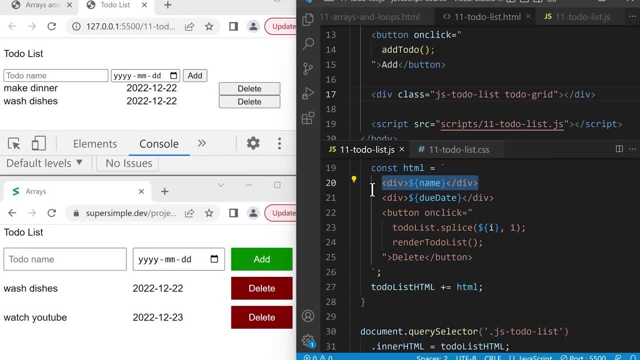 First Column. This Element Goes Into The Second Column And The Button Goes Into The Third. We'll Go To Our HTML And Let's Put These. 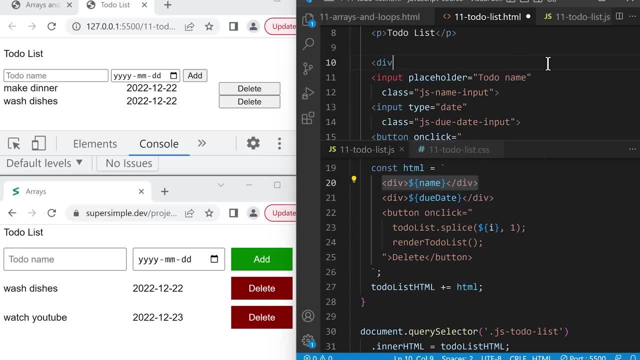 Three Elements In A Div. So We Can Use Grid. So We'll Create A Less Than Div, Greater Than, And Then Press Tab To Add. 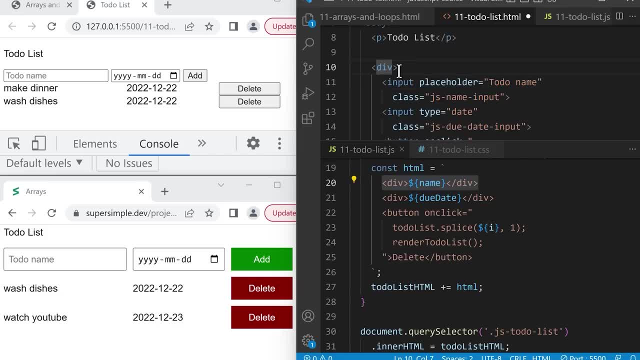 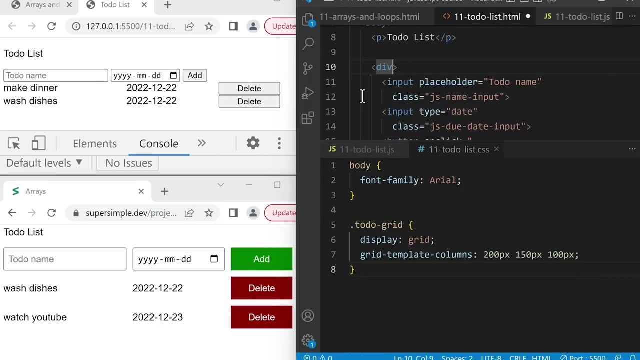 An Indent, And Now Let's Make This Div A Grid As Well. Let's Go Back To Our CSS And We'll Add A Class To. 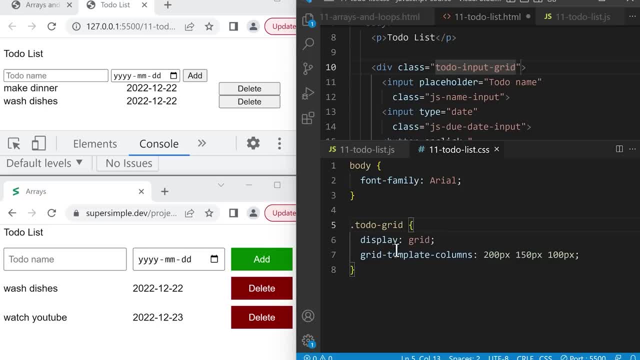 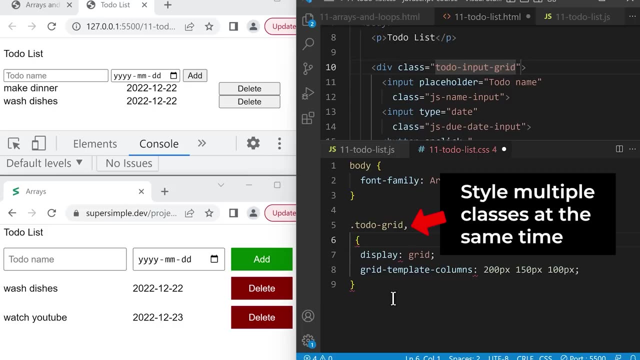 This And Use A Feature Of CSS. So Here We're Going To Type A Comma And Enter. So When We Type A Comma, We 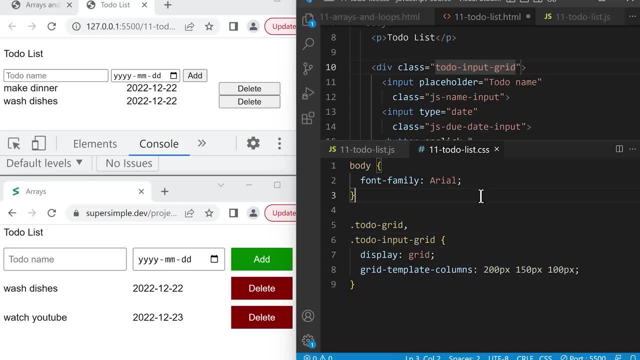 Can Style Multiple Classes At The H, T, M L File. Now The Input And The Add Button Are Also Laid Out In The Same 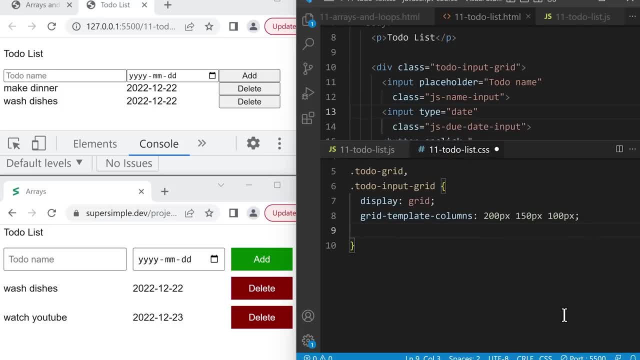 Grid. Next, Let's Adjust The Spacing Inside Our Grid, So The Spacing Between The Columns Of The Grid. So Let's Make This Colon 10.. 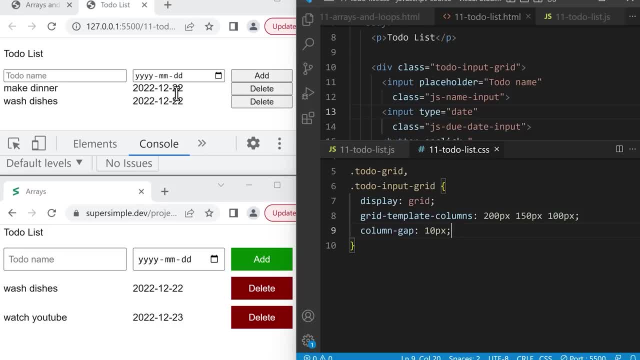 Pixels And Save, So Now It Will Add 10. Pixels. Between Each Column Let's Add Some Space, So That Will Add 10. Pixels Of. 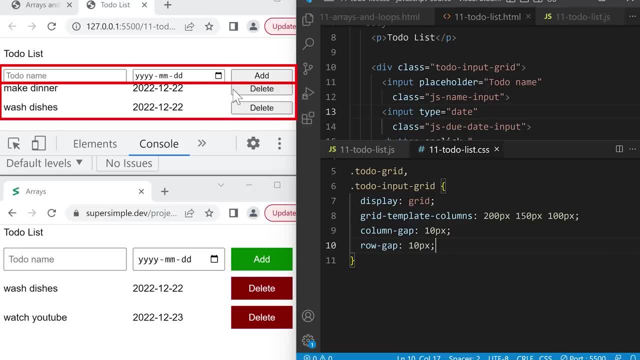 Space Between The Rows. Now Notice, It Didn't Add Space Between These Two Rows And That's Because These Two Are Separate, So Let's Add. 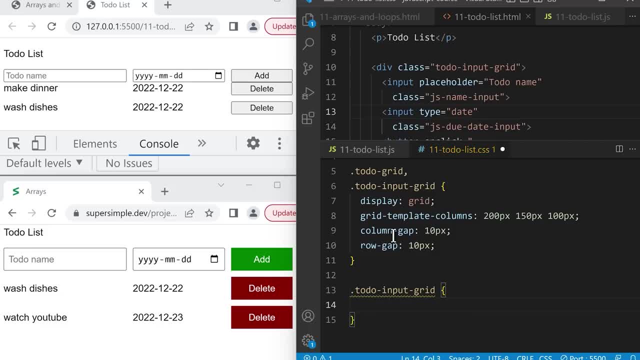 Some Input Dash Grid And We'll Just Add Some Margin Under This Grid. So Margin Dash Bottom Colon, 10. Pixels And Save. Alright, Now Let's. 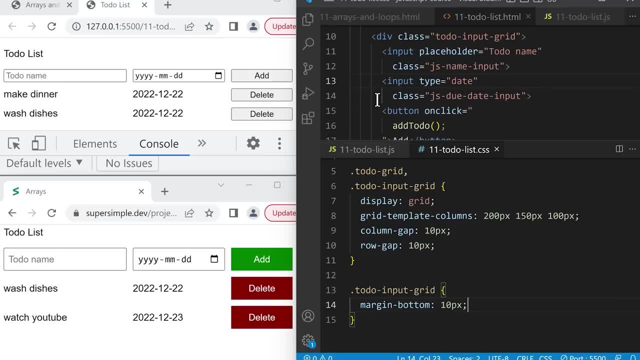 Move On A Class So We Can Style Them. Here Let's Add A Class Name, Dash Input, And Down Here Let's Also Add Another Class. 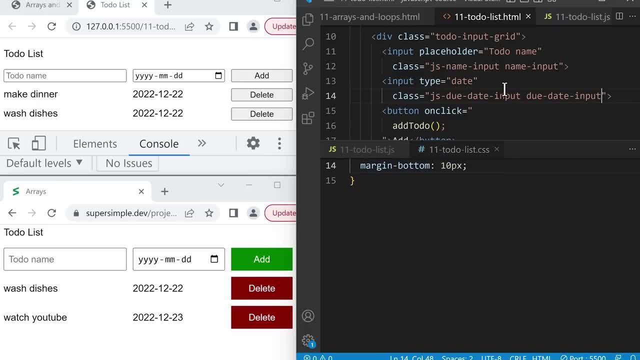 Do Dash Date, Dash Input. Let's Save Dot Name. Dash Input: Curly Brackets. And First Let's Make The Text Bigger, Like The Final. 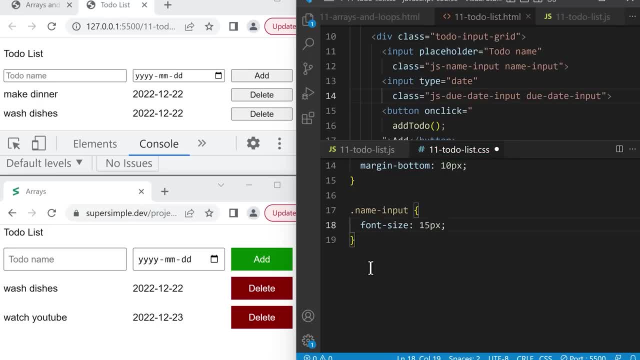 Design. We'll Set The Font Dash Size: Colon 15. Pixels And Save- Okay, Padding. 6. Pixels And Save, And That Looks Pretty Good, Let's. 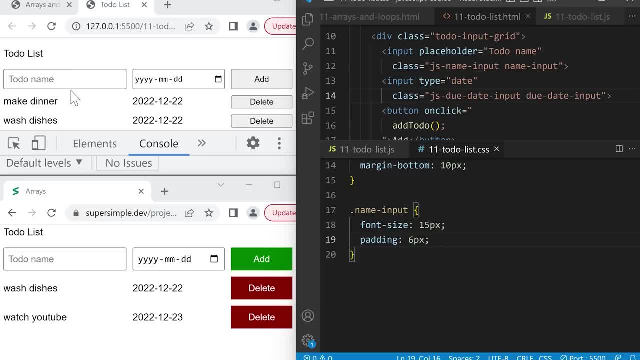 Move On To The Due Date Input. So Again We Can Use That Feature Of CSS. We'll Add A Class, So Now These Styles Will: 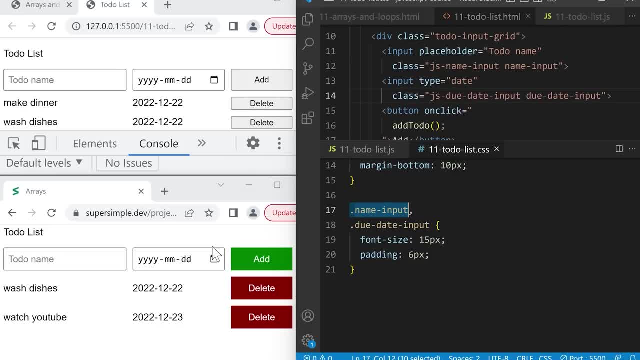 Be Applied To This Class And To This Class. Let's Save, And That Looks Pretty Good To Me. Let's Move On To Do Dash Button. 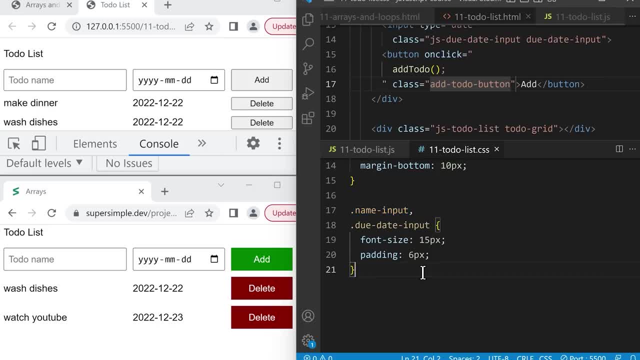 Let's Save, And Then Inside Our CSS We'll Style That Class Using Dot. Add Dash To Do Dash Button, Curly Brackets And Let's. 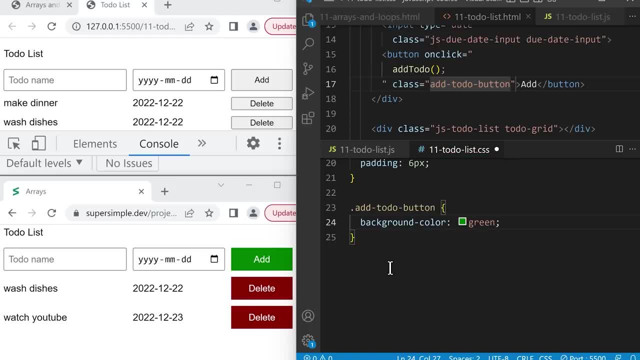 Start With The Text And Save Now. Let's Do The Text Color: Color Colon White And Save Now. Let's Remove The Border Around Our Button. 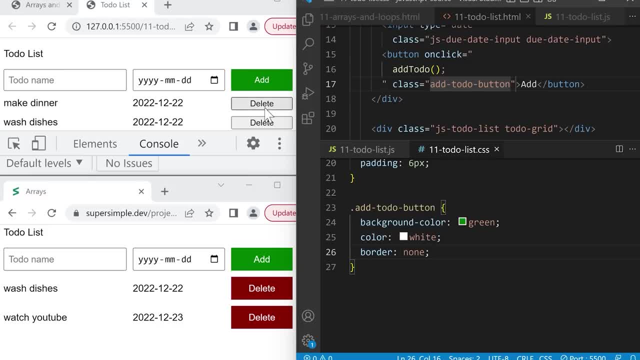 Using Border Colon. None, Save, And Let's Make A Button Dash Size Colon: Fifteen Pixels And Save. And The Last Thing We'll Add Is: 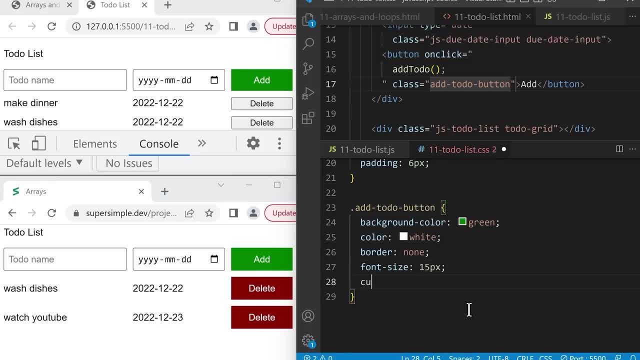 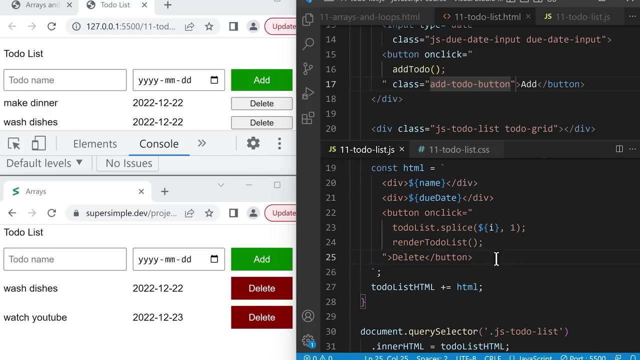 When We Put Our Mouse Over The Button, It Turns Into This Pointer. Let's Style The Delete Buttons So These Delete Buttons Are Created In. 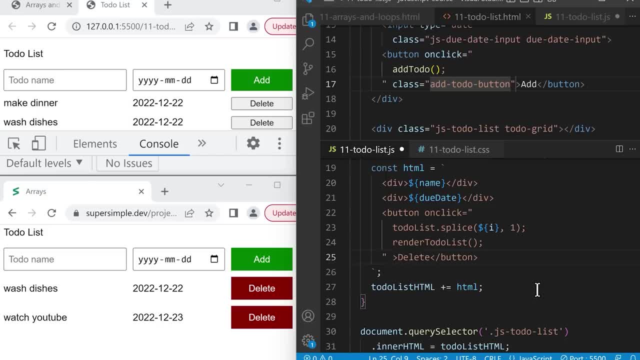 Our JavaScript, We'll Go Into Our JavaScript File And Then Here Let's Add A Class To Each, Let's Save And Then Inside Our CSS. 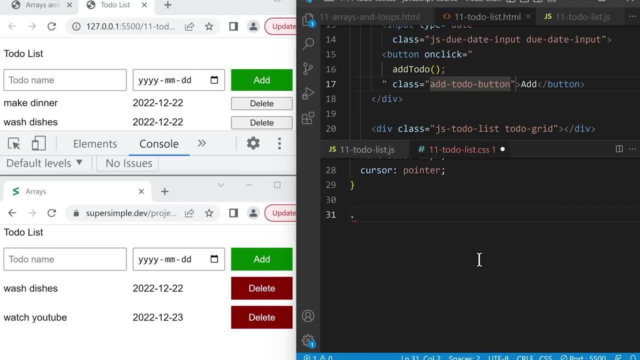 At The Bottom We'll Style Dot, Delete Dash To Do Dash Button, Curly Brackets And Let's Start With The Background Color. So I Use 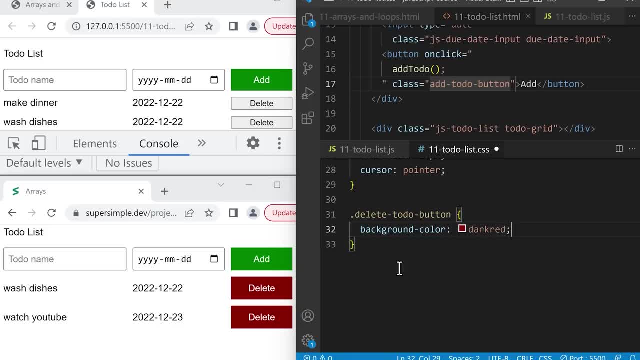 The Color Dark Red And Save, So That Will Style Our Delete Buttons. Now Let's Change The Text Color To White, So We'll Use Color. 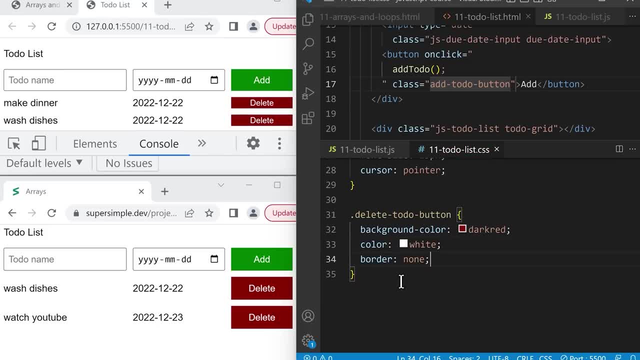 Colon White And Save. And Let's Also Make The Text Bigger Using Font Dash Size: Colon: Fifteen Pixels, Save. Let's Add This Pointer Icon. 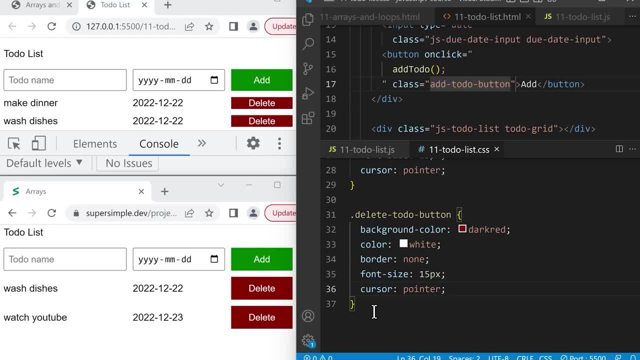 Using Cursor, Colon Pointer, Save And Let's Use The Button, So We'll Add Padding Dash Top Colon Ten Pixels And Padding Dash Bottom, Colon Ten. 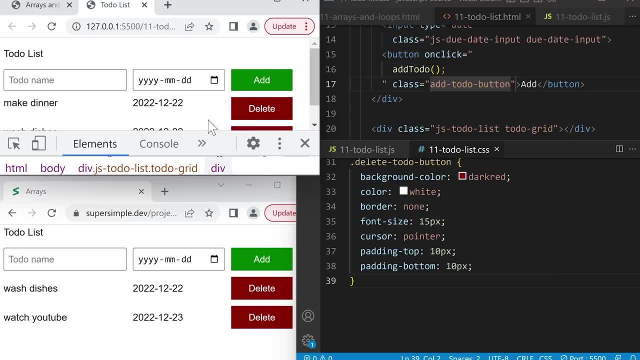 Pixels And Save. So That's All The Styles We Need For Alignment. However, Now We Have Another Problem, Which Is This Text And This Button. 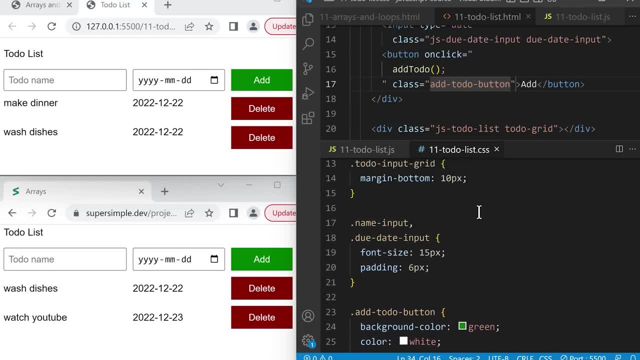 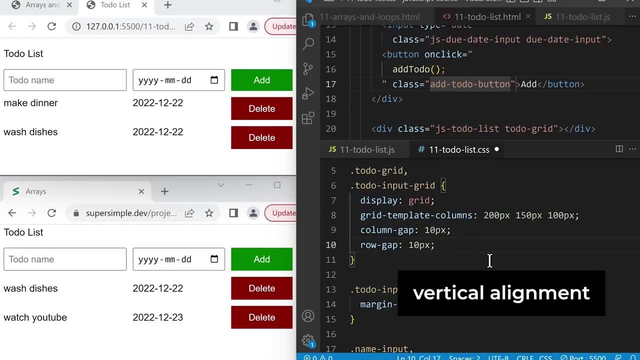 Are Not Vertically Aligned In The Center. To Vertically Align In The Center We're Going To Dash Items Colon Center. To Vertically Align. 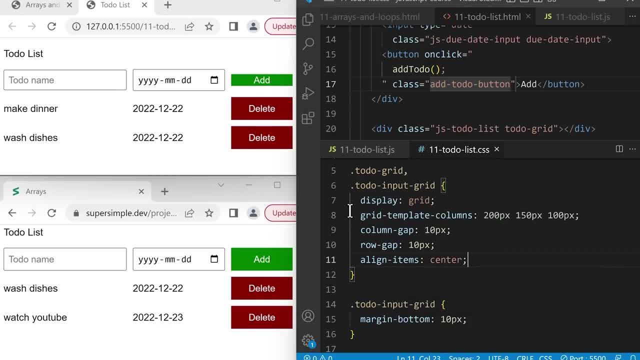 In The Center. If We Save Now, The Text Is Aligned With The Button. But Now We Have A New Problem: Our Grid Stretches. 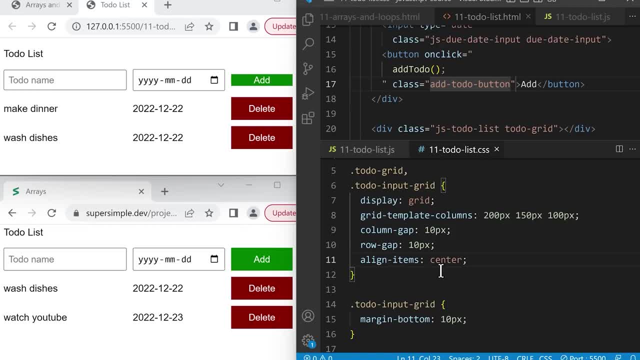 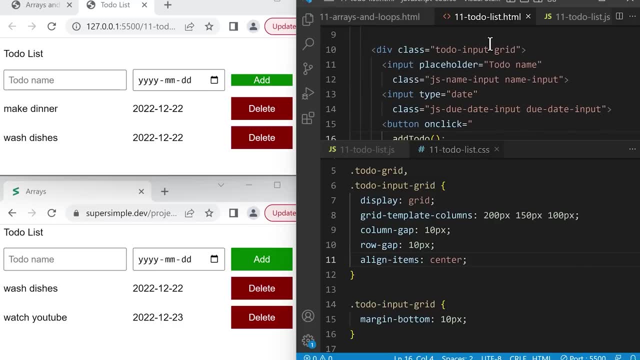 To Match The Inputs And Now That We Changed It To Align Center, It's No Longer Going To Stretch. So To Solve This Problem, We 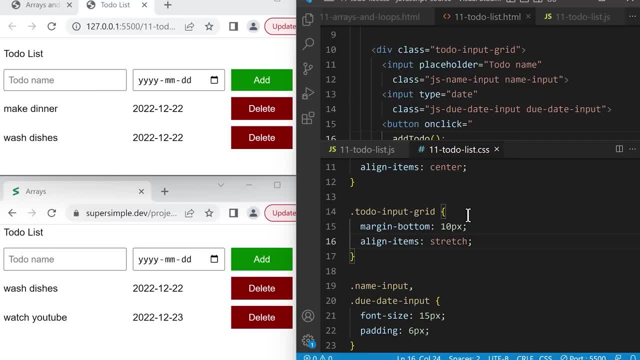 Just Have Save And That Will Cause This Grid At The Top To Stretch Vertically Again, And That's It. That's All The Styling That. 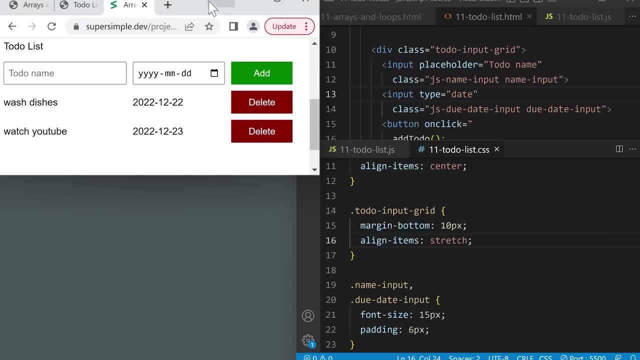 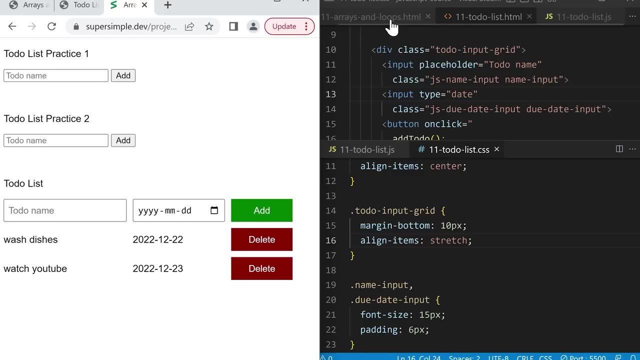 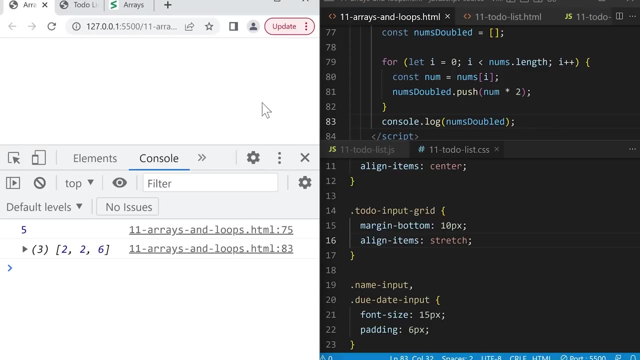 We Need. And Now We Finished. And Now Let's Go Back To Eleven Arrays And Loops, Dot HTML, And We'll Open The Tab For. 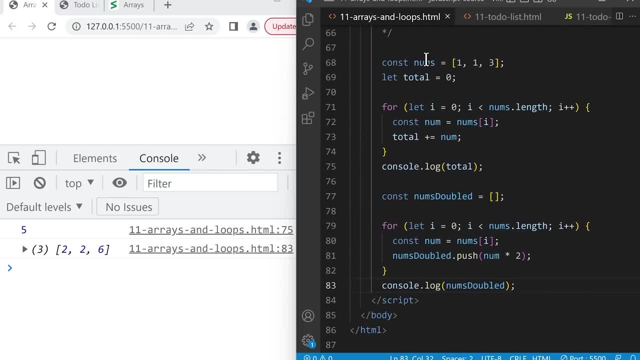 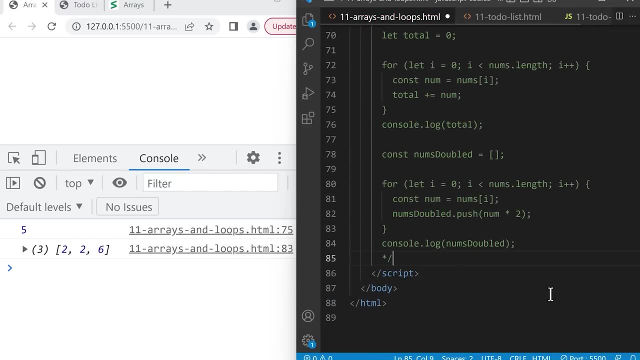 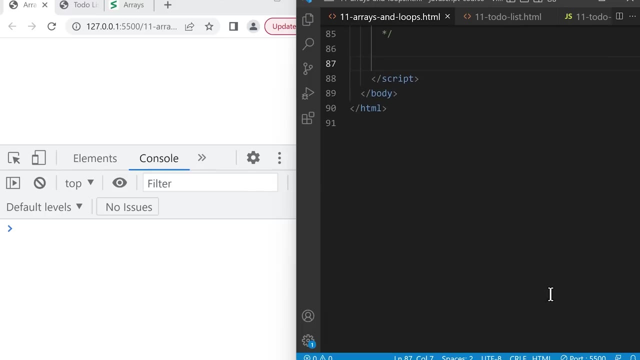 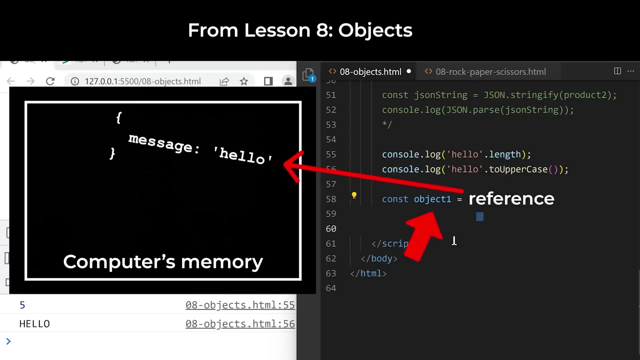 That File And We Can Also Close These Other Files For Arrays And We'll Scroll Down And Save The First Detail We're Going To Learn. 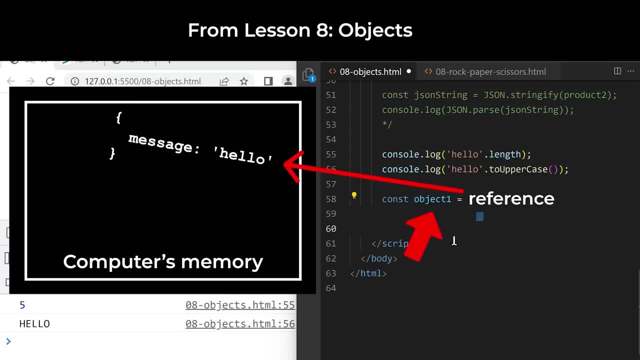 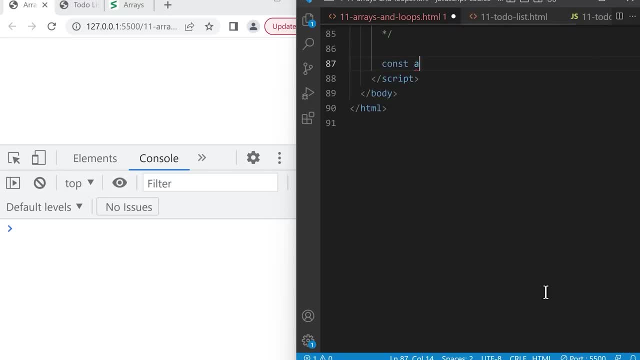 Is That Arrays Are References. So In The Object Lesson We Learn That Objects Are References To Three. This Variable Doesn't Actually Contain The Values. 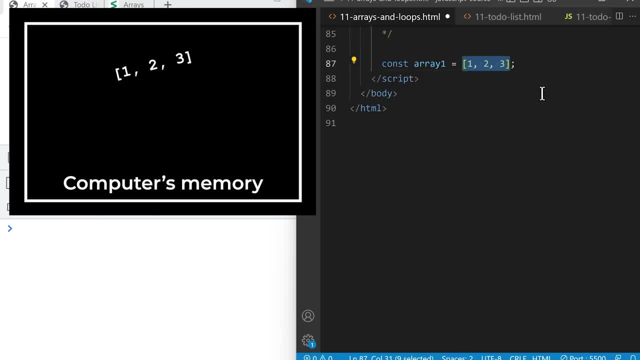 One, Two, Three. This Array Is Saved Somewhere In The Computer's Memory, And This Variable Only Contains A Reference That Points, Equals Array: One Array. 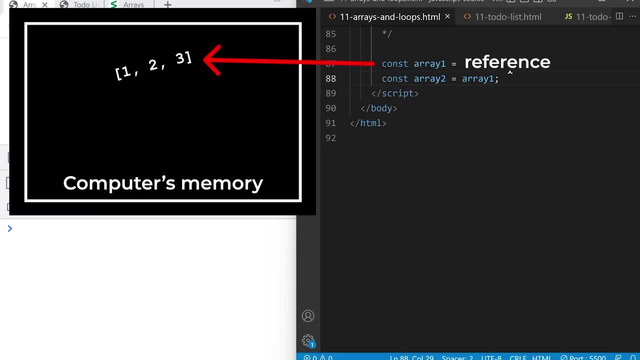 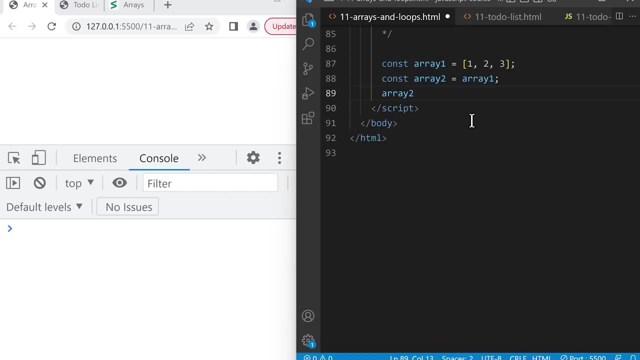 Two Doesn't Contain A Copy Of The Values. It Actually Just Contains A Copy Of The Reference. So Now Both Of These Variables Are Modified. 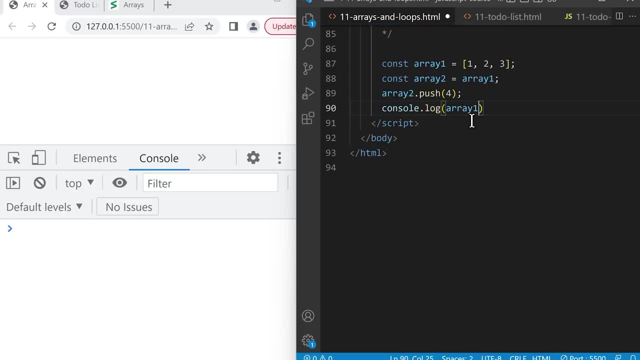 And We Added Four To Array Two, Array One, And We Console Dot Log Array Two And Save. It Will Show Us That, Even Though We 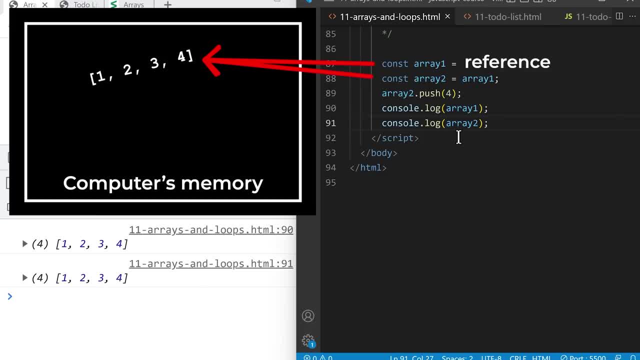 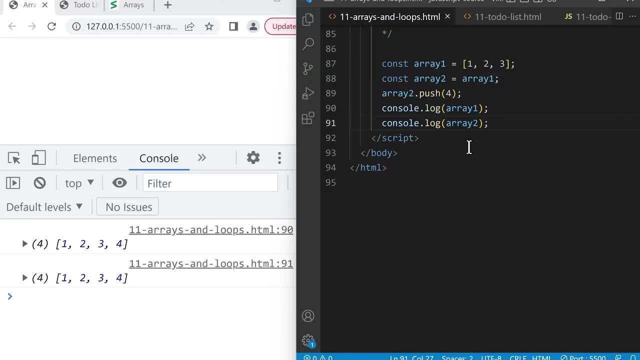 Added Four, So Both Of These Point To The Same Array. In Memory, To Avoid This Behavior, We Can Create A Copy Of The Values In. 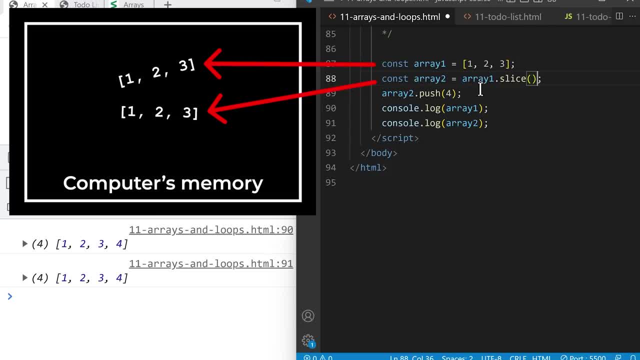 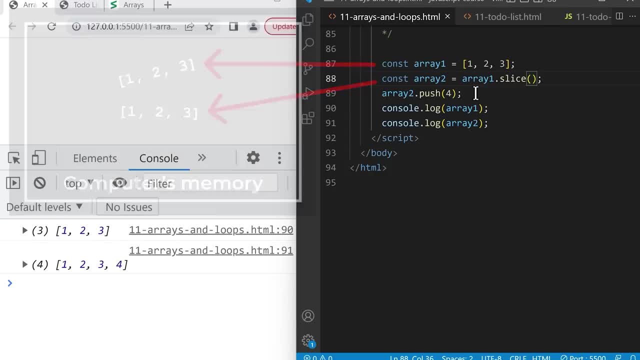 The Array Using A Method Called Two Different Arrays. If We Save Now, You'll See That This Line Only Affected Array Two. The Second Detail. 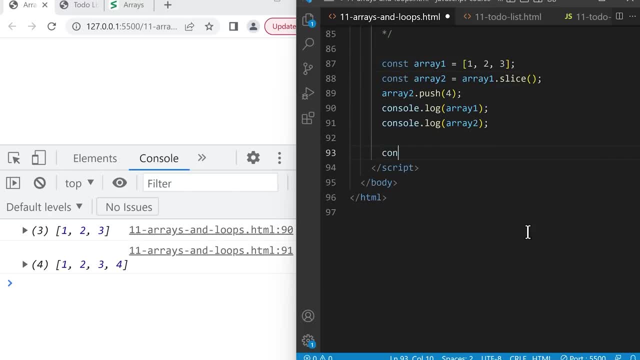 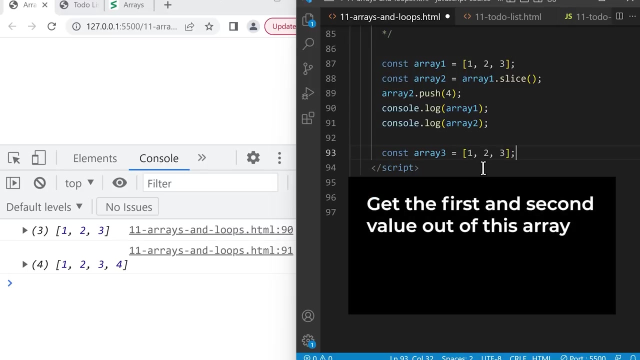 We're Going To Learn Is A Shortcut Called Destructuring. So At One, Two, Three, And Let's Say We Want To Get The First Value. 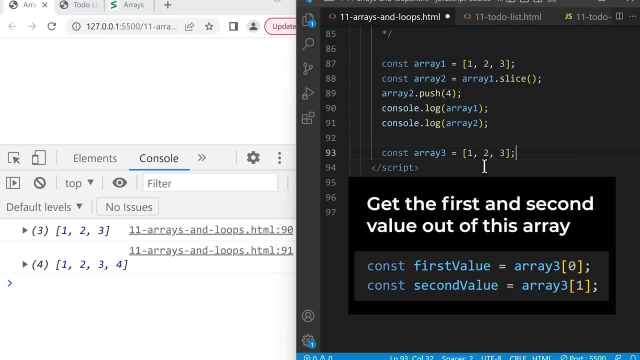 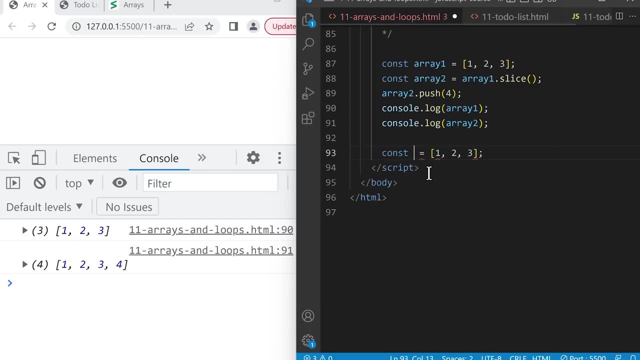 And The Second Value Out Of This Array. One Way To Do This Is To Use. If We Type First Value, It Will Take The First. 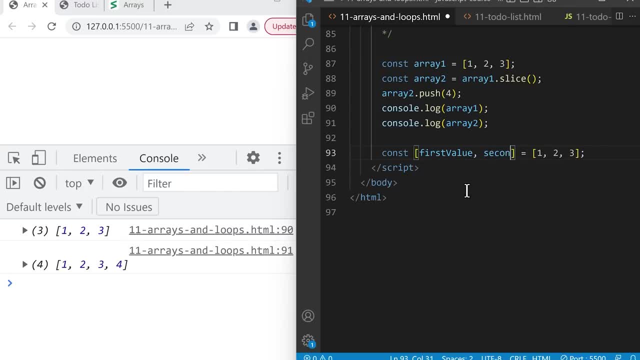 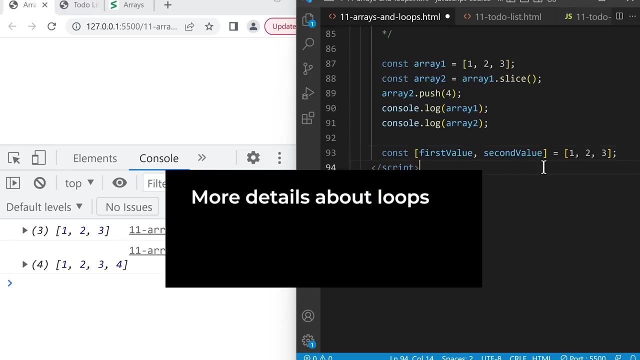 Value And Save It In A Variable Called First Value. If We Type Comma And Second Value, It Will Take Next. We're Going To Learn. 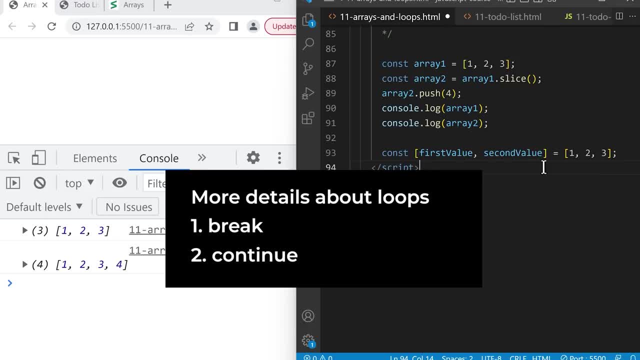 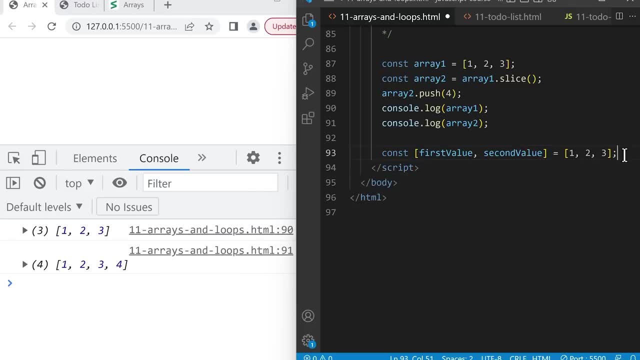 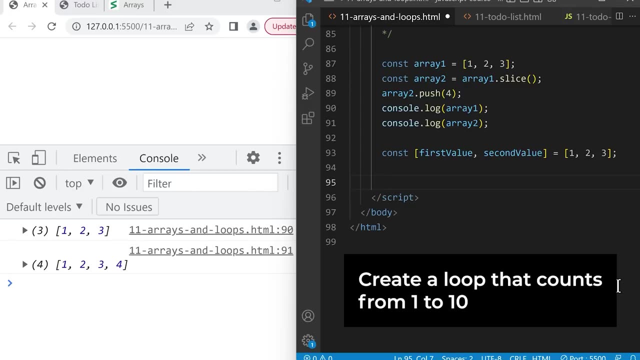 More Details About Loops. So Loops Have Two Features, Called Break And Continue Break. Lets Us Exit A Loop Early. For Example, Let's Create: 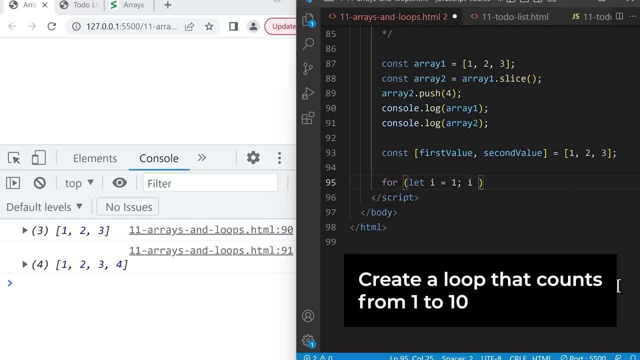 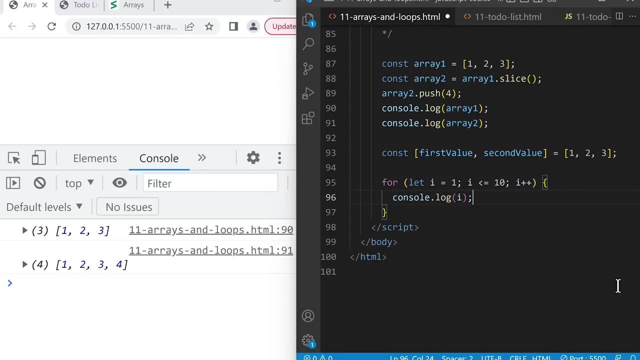 A Loop With 1. Less than Or 10. I Plus Plus And Will Console Log I And Save Count. Count from One To Ten Tell. 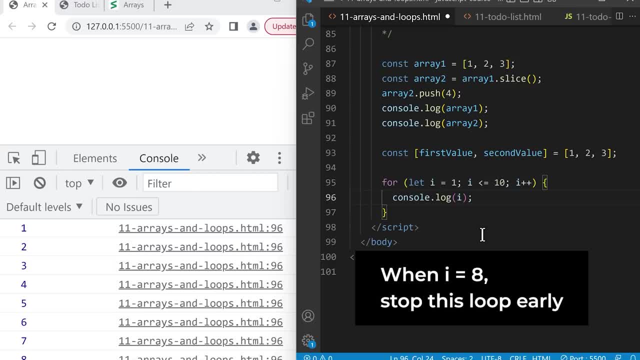 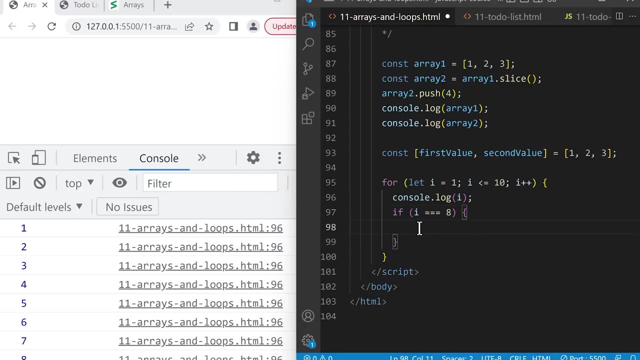 Me That When I Is 8.. So first let's check if i is equal to 8.. If it is equal to 8, we're going to stop this loop by typing break and semicolon. If we save once this reaches 8, break will cause this loop to stop. 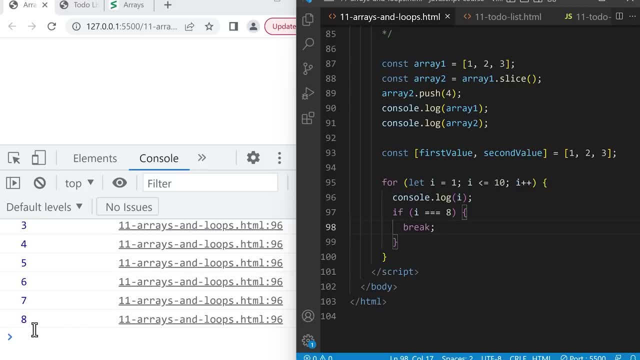 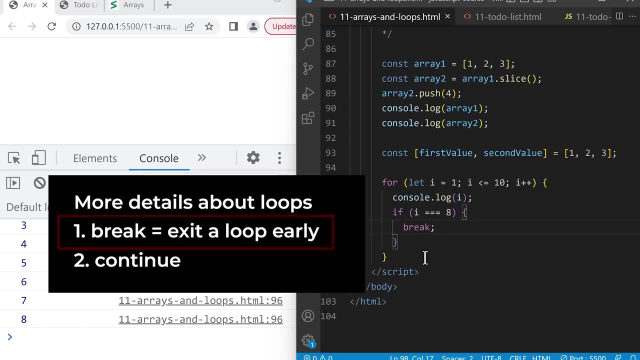 And now it only counts up to 8.. So that's the break feature of a loop. It lets us stop a loop early. The next feature is called continue. Continue lets us skip one iteration of the loop or one run of the loop. 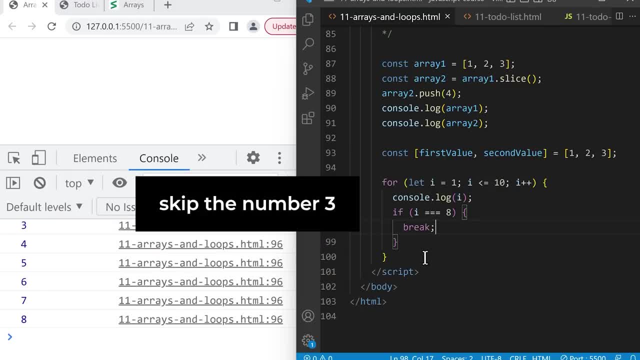 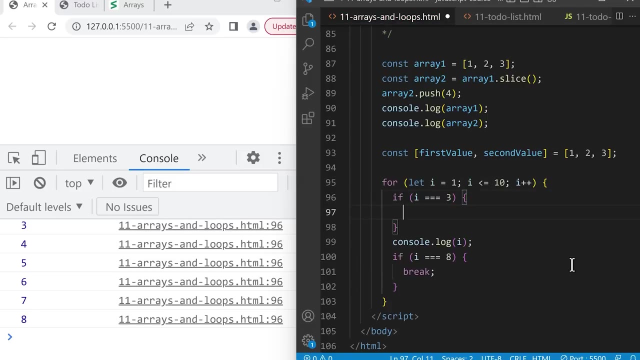 For example, let's say we want to skip the number 3. So at the top we can check if i is equal to 3. And if it is, we can use the code continue. This will skip the rest of this code and go back up to the top of the loop and do i equals. 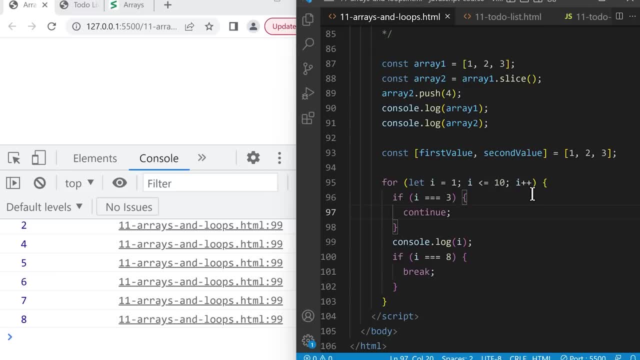 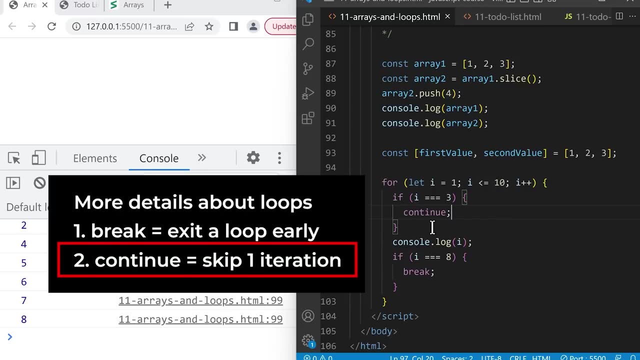 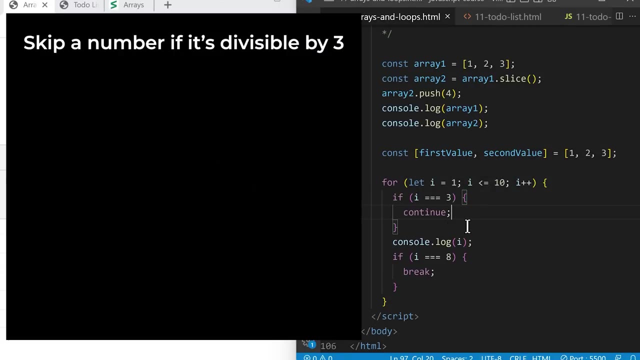 4. If we save this will skip 3 in the loop. So continue, lets us skip one iteration. So now let's say that we want to skip a number if it's divisible by 3. Divisible by 3 means the number can be divided evenly into 3.. 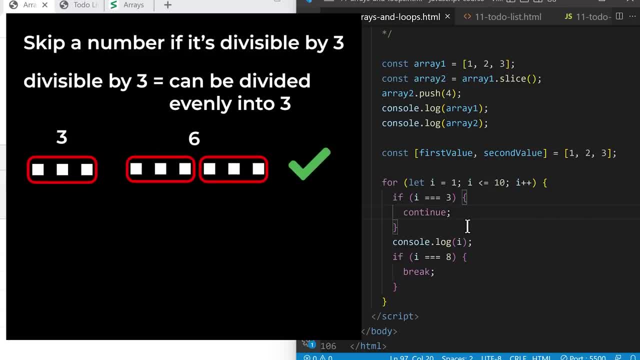 For example, 3 and 6 are both divisible by 3.. But 7 is not divisible by 3 because there's one remaining. This is called the remainder And we can calculate the remainder. We can calculate the remainder using the remainder operator, which looks like this: 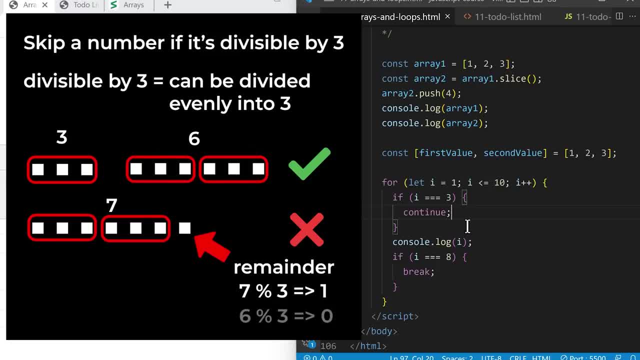 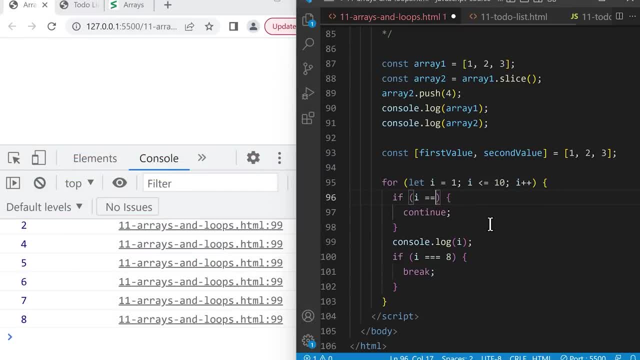 So to check if a number is divisible by 3, we can check if the remainder is 0. So here we're going to replace this with i remainder 3, and we'll check if the remainder is equal to 0.. If we save, this will skip. 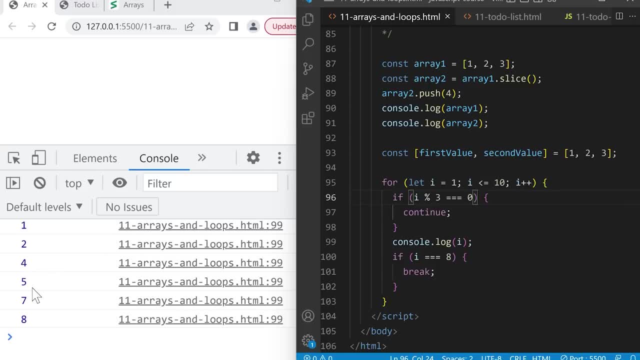 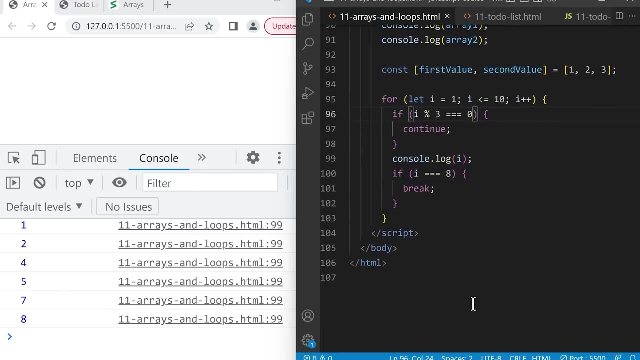 And if we save this will skip This. will skip 3 and 6, because they're both divisible by 3.. Next let's use continue in a while loop. So at the end here we'll create some new lines And let's say we want to count from 1 to 10 using a while loop. 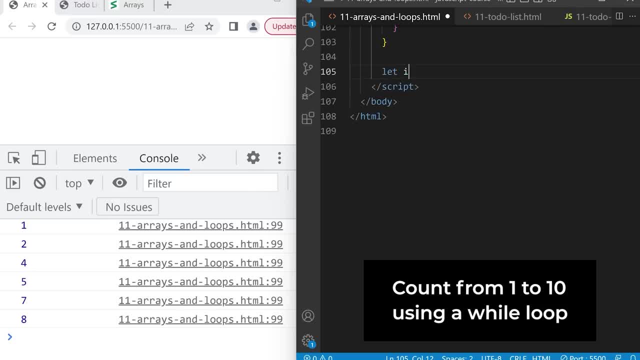 So we'll create a loop variable: Let i equals 1.. And we'll create a loop variable Let i equals 1. And we'll create a while loop. And we'll create a while loop: i less than or equal to 10, curly brackets and the increment step: i plus, plus. 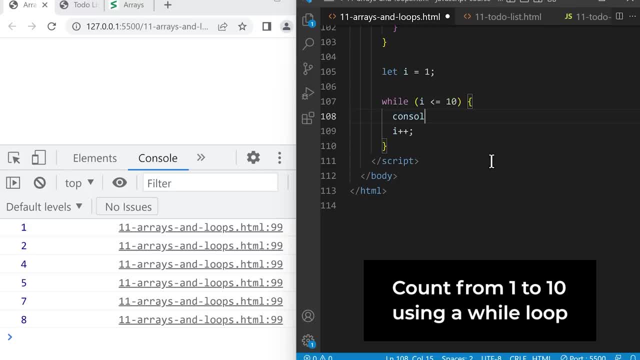 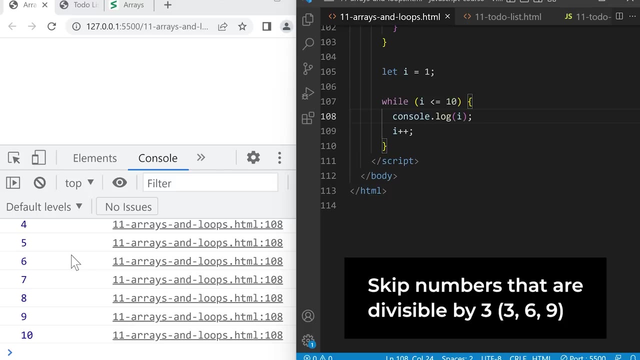 And inside the loop we'll just console, dot, log i and save. So this will count from 1 to 10 again, And let's say we want to do this And let's say we want to not count numbers that are divisible by 3.. 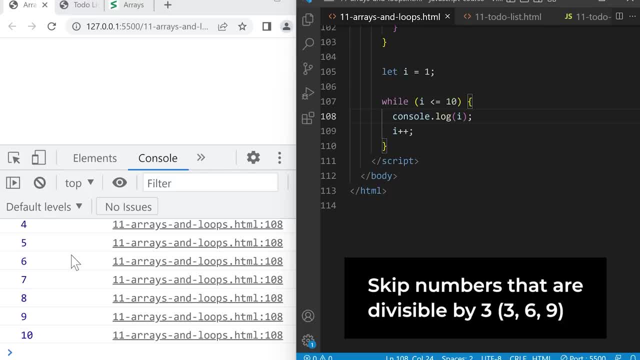 So 3,, 6, and 9.. So at the top here we can check if i remainder. 3 is equal to 0 and curly brackets And we might just try to do continue. However, in a while loop, continue will actually skip the increment step. 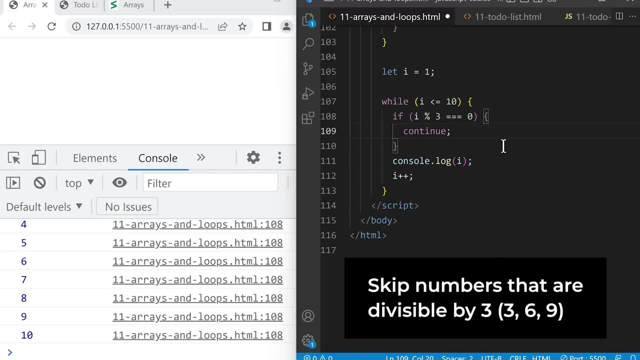 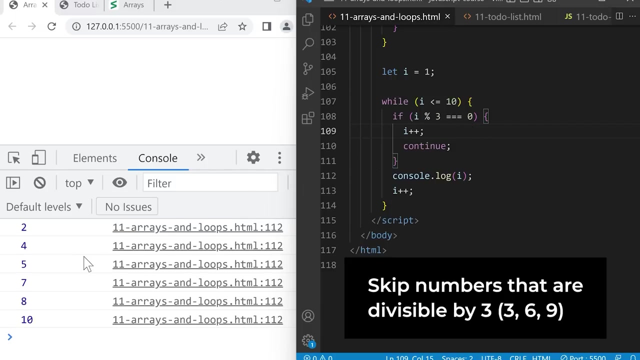 And this will cause an infinite loop. So when using continue in a while loop we have to do this increment step manually. So before continue we have to do i++ to avoid an infinite loop. If we save, It will skip the numbers that are divisible by 3,, which is 3,, 6, and 9.. 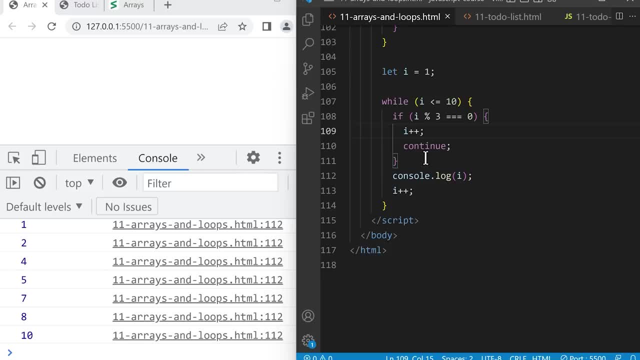 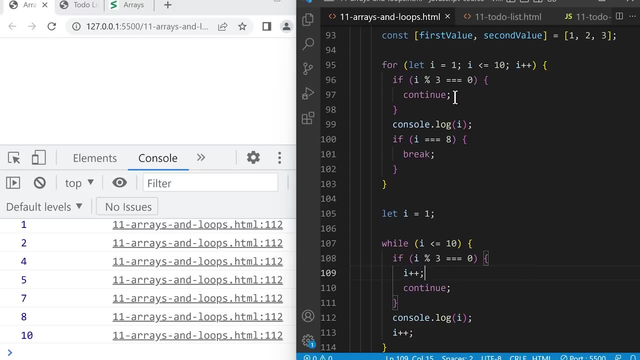 So remember, in a while loop, if we use continue, always do the increment step manually. In a for loop, however, the increment step is done automatically after every iteration. All right, The last detail we're going to learn is how to use loops with for loops. 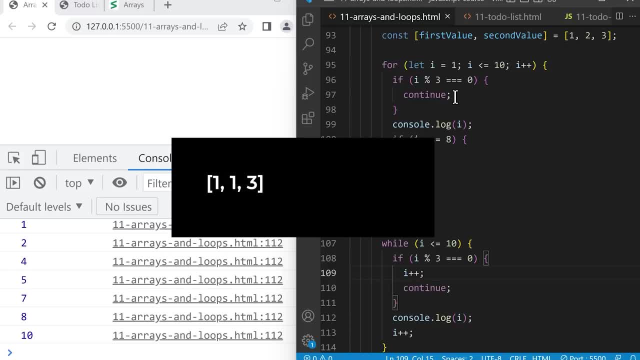 So we're going to use loops with for loops. So we're going to use loops with for loops. So let's say we have an array of numbers and we want to create a copy of this array where each number is doubled. So we already have the code for this. 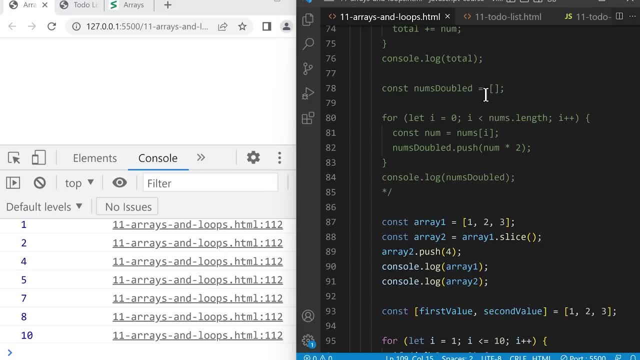 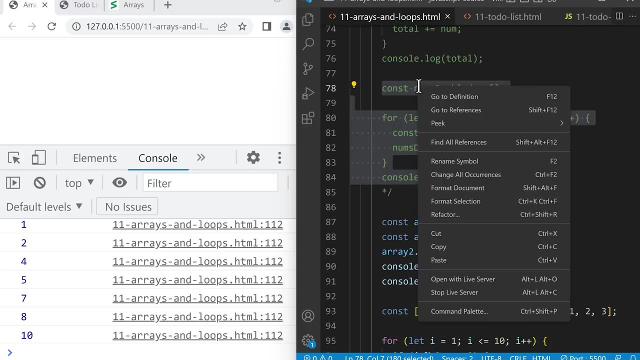 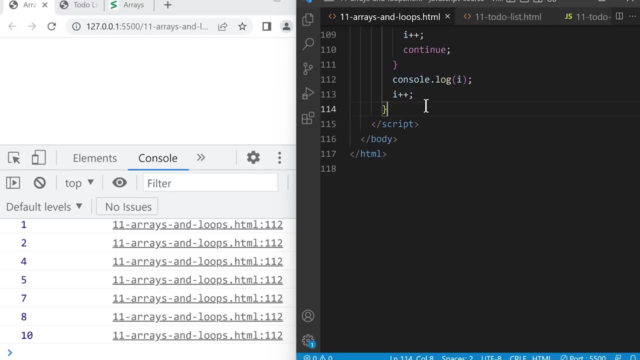 We can scroll up and the code for this is here, So let's actually make a copy of this code from before. We'll right click, copy and scroll down here And at the bottom, right click and paste. At the top, let's create an array called nums. 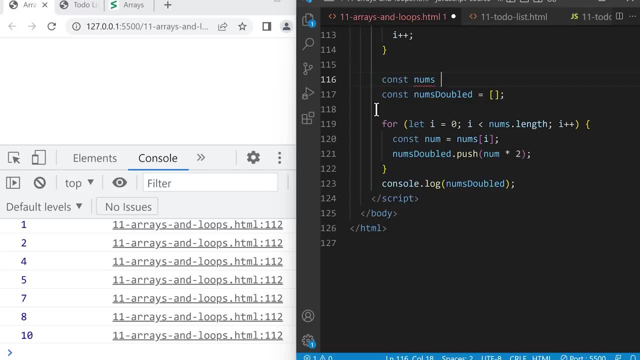 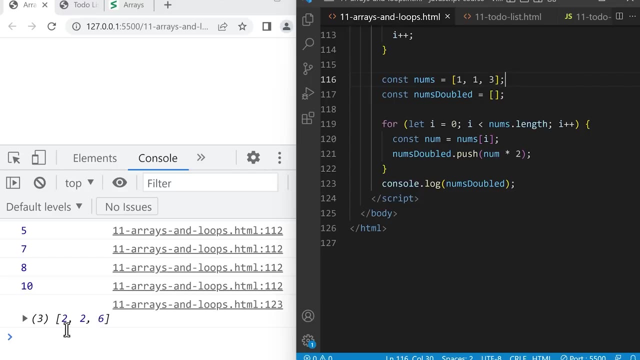 So const nums equals array and 1,, 1, and 3.. Let's see: If we save, This will create an array. This will create an array where each number is doubled. Now what if we wanted to use this loop on a different array other than 1,, 1, and 3?? 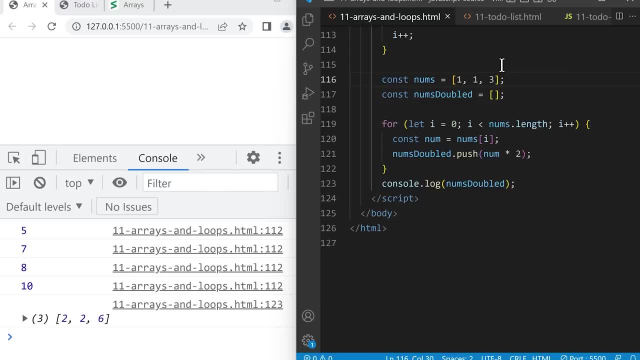 We can do that using a function. So let's create a function around this loop. We'll create function, Let's name it: double array brackets and curly brackets. We'll remove the closed curly bracket and at the bottom we'll add it back and we'll select these lines and press tab. 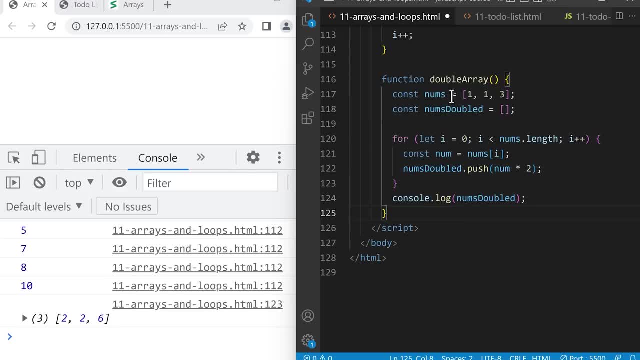 So now, instead of doing this loop on the same array every time, we can turn this into a parameter. So at the top here, we'll create a parameter called nums And we're going to delete this line And we're going to loop over this parameter instead. 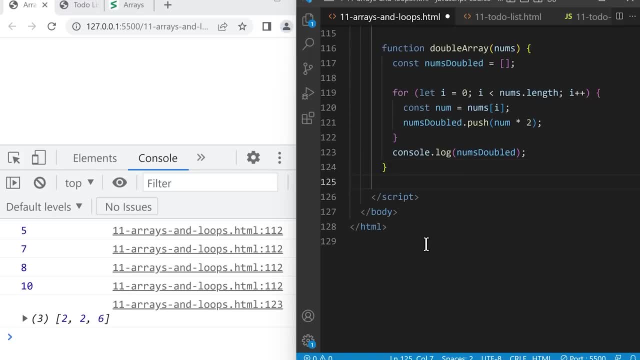 So at the bottom we can call our function using double array and brackets, And between the brackets we're going to save an array into nums, So square bracket 1,, 1, and 3.. If we save, this will do the same thing as before. 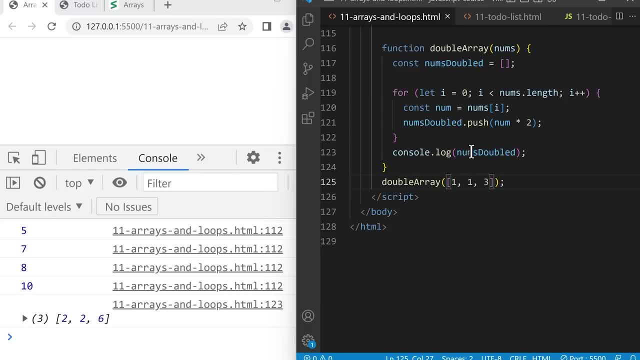 But now, because it's in a function, we can use this loop with any array, not just 1,, 1, and 3.. So at the end we can do double array- brackets and an array- 2,, 2,, 5- this time. 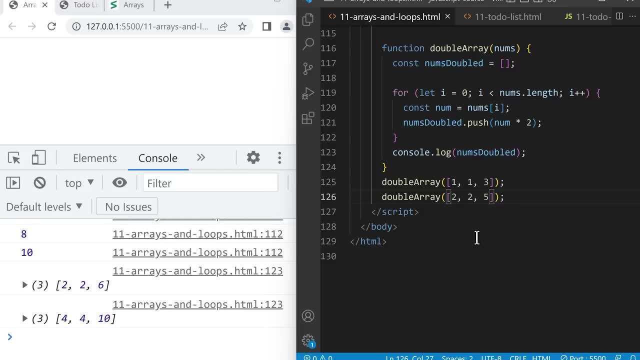 And save, And it will create an array where these numbers are doubled. So, using a function, we can reuse this loop for any value. Another feature of using a function with a loop is that we can break out of this loop using a return instead. 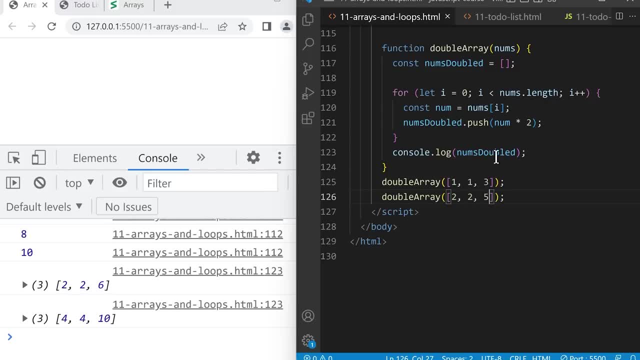 So first let's actually use a return in this function Instead of consolelog. we're going to use a return in this function, So we're going to return nums doubled And here we're going to consolelog. the result: consolelog. 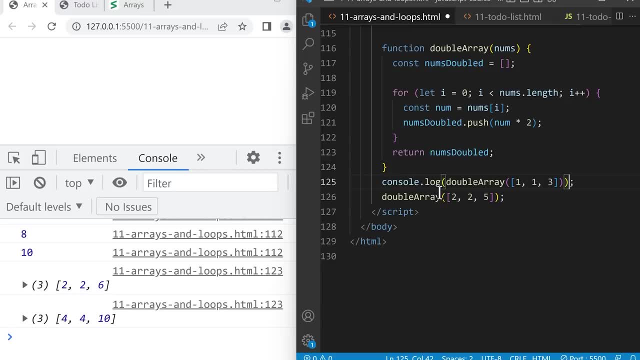 and consolelog and save. So this does the same Same thing as before, except we're returning the result and consolelogging outside of the function. Now let's say that if we see the number 0, we want to stop this loop early. 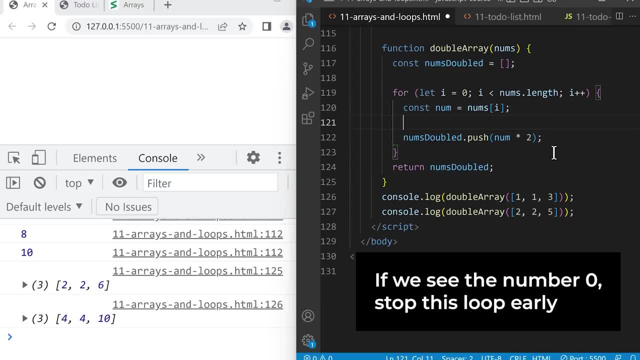 To do that, we can click here and check if num is equal to 0. And if it is, we can break out of this loop. Now, when we're inside a function, we can also use a return statement to break out of this loop. 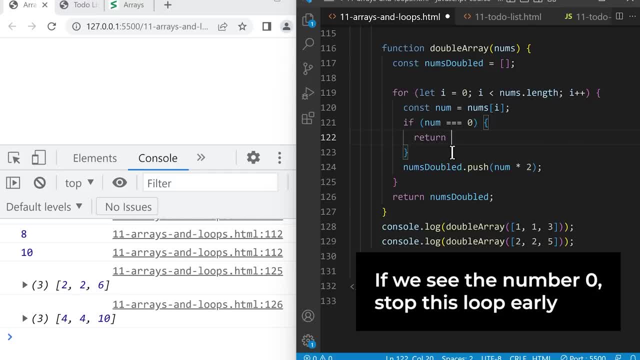 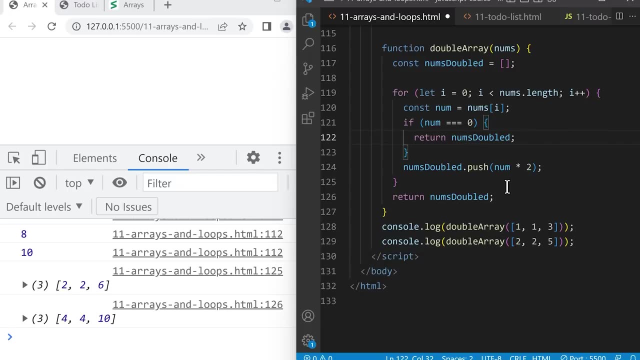 So we can also do return nums doubled, So a return statement will end this function immediately. So this is another way of ending the loop. So down here, if we add the number 0, and then 5, and save, you'll notice that the loop stops when we see the number 0.. 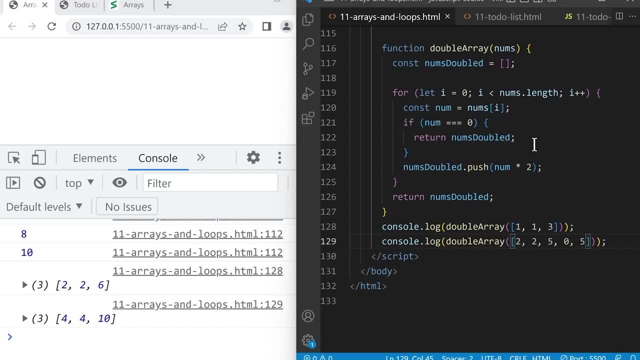 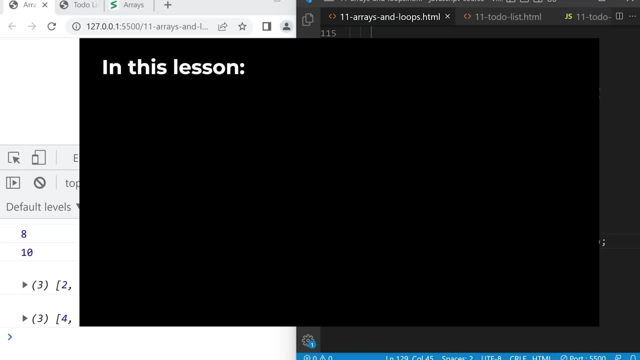 So return is another way of breaking out of a loop when it's inside a function. And that's the end of this lesson. In this lesson, we learned about arrays, which represent a list of values. We learned about loops, which let us run some code over and over again. 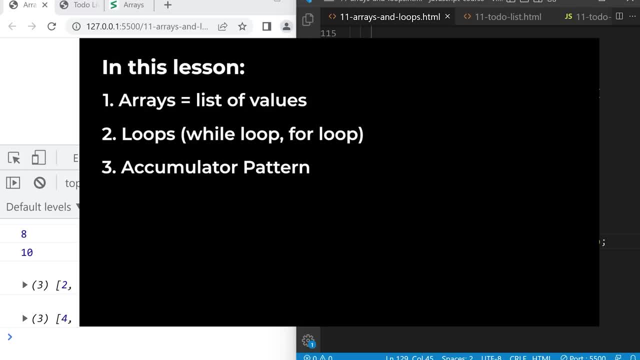 Just like a loop. We learned a technique we can use with loops called the accumulator pattern, And we used it to create a to-do list project. We learned that arrays are references and the destructuring shortcut, And we learned more features of loops, like break, continue and using loops inside a function. 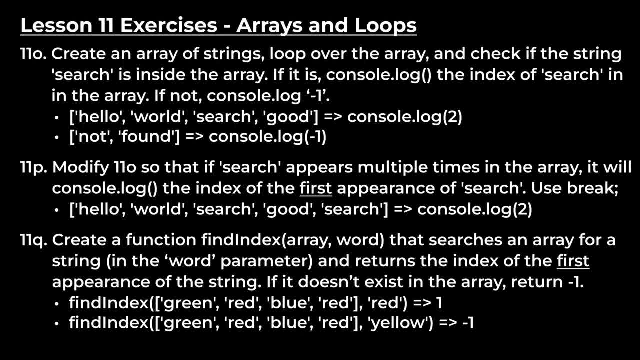 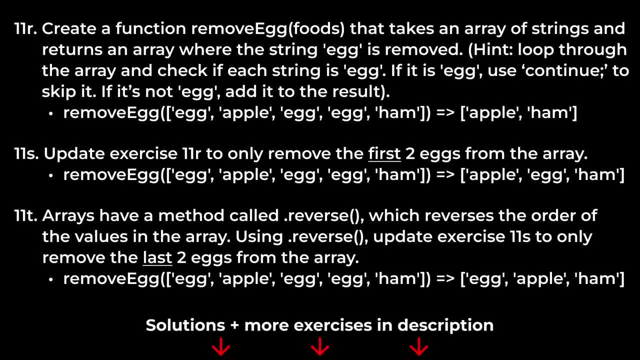 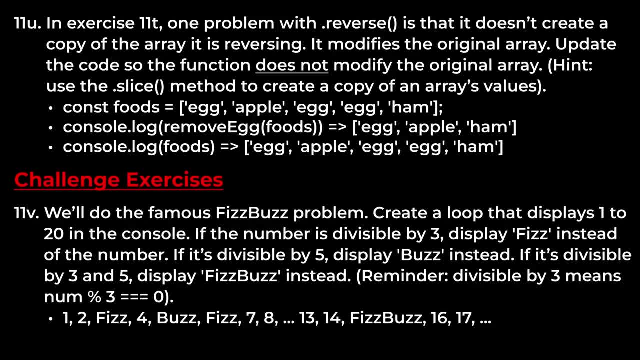 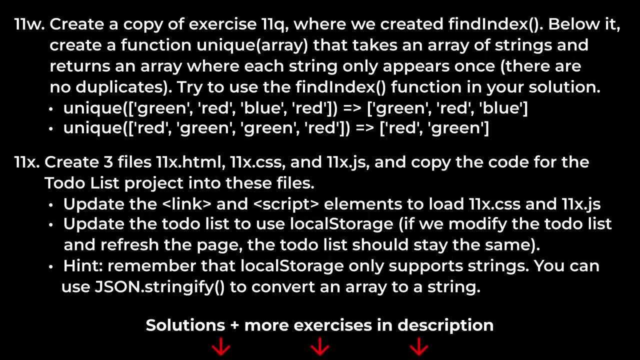 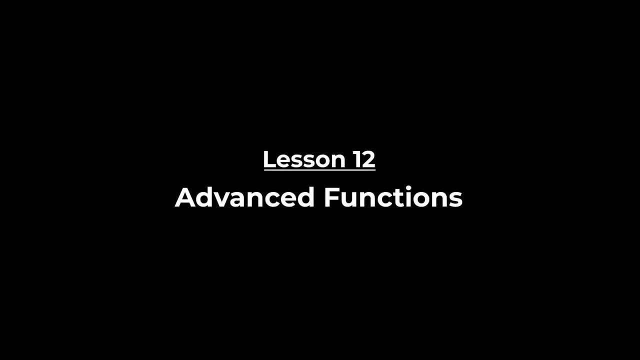 Here are some exercises to help you practice arrays and loops. Here are some exercises to help you practice arrays and loops. Here are some exercises to help you practice arrays and loops. In this lesson, we're going to learn some advanced. In this lesson, we're going to learn some advanced. 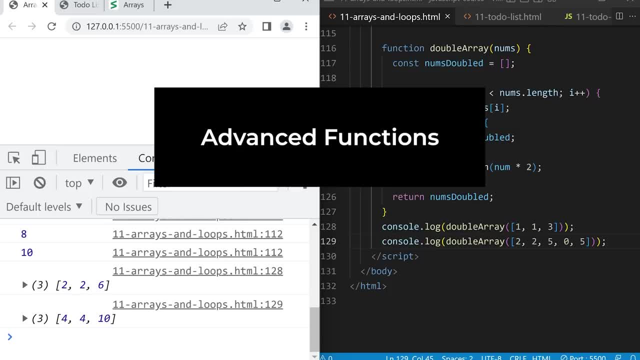 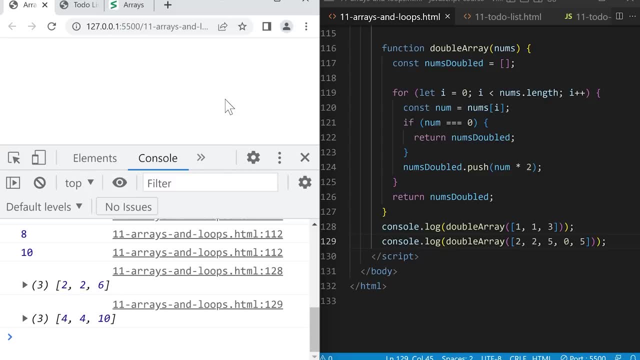 In this lesson we're going to learn some advanced features of functions and we're going to use them to improve our previous projects. First, let's create a new file for this lesson. We'll go to our code editor and click here to show our files. 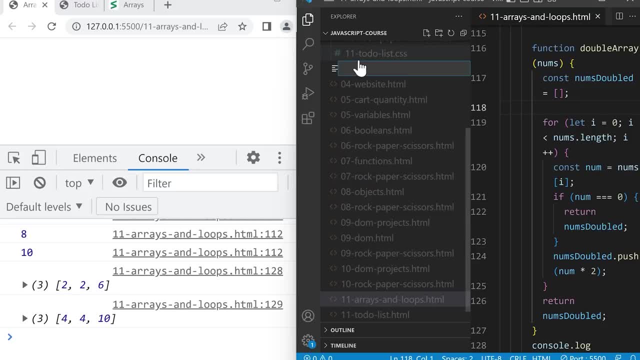 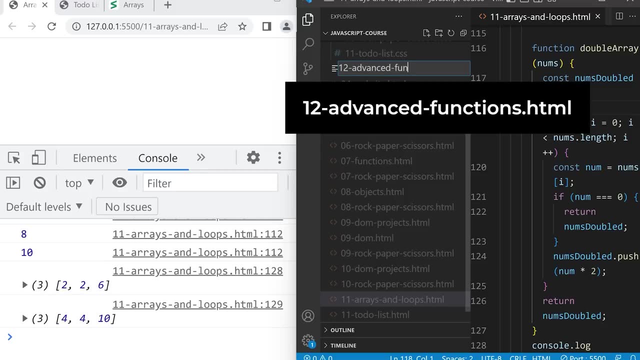 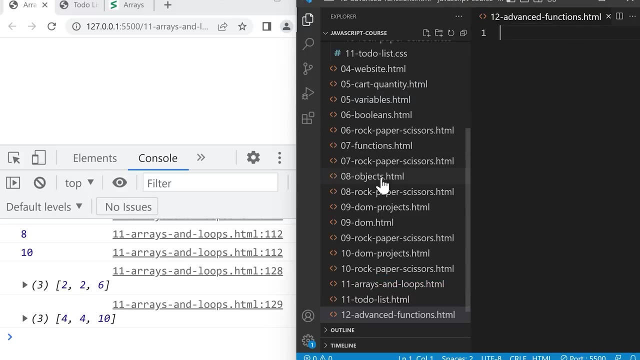 and click here to create a new file, And we'll name this 12-advanced-functionshs, And we'll name this 12-advanced-functionshs. And we'll name this 12-advanced-functionshs. Now, just remember, we just copied 11ravs: 빨리 dieserフай Playing. 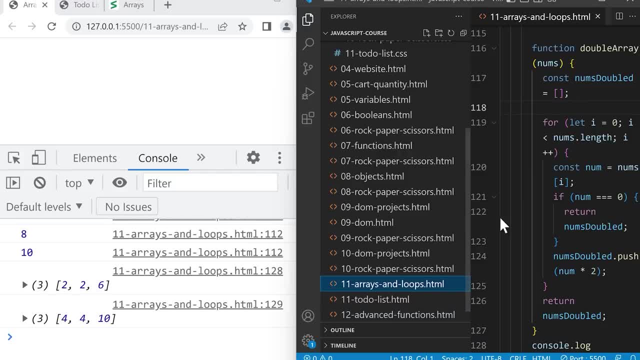 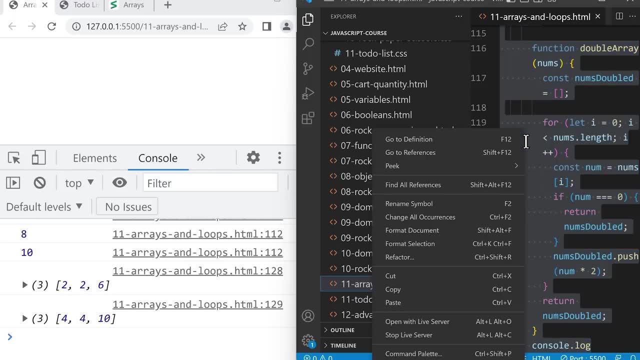 and pressing Enter, And we'll do the same for enter. Now let's copy 11 arrays and loops into this file. Now let's copy 11 arrays and loops into this file. So we'll click here: control a or command a. 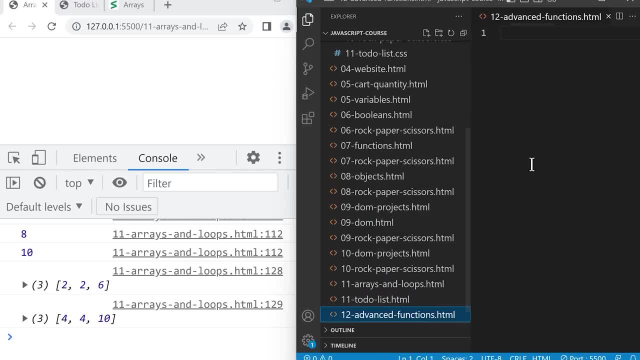 and then right click, copy and in here. and then right click copy and in here. and then right click, copy and in here. base page 1, right click and paste. right click and paste. Right click and paste. 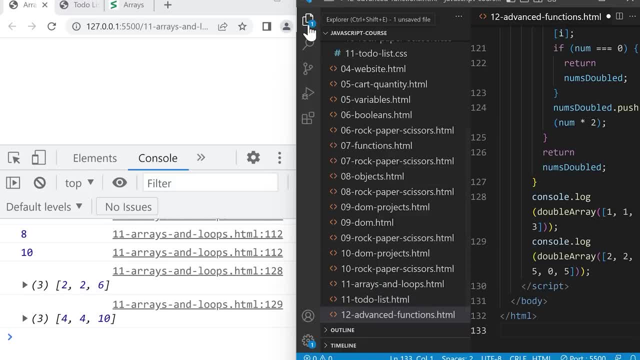 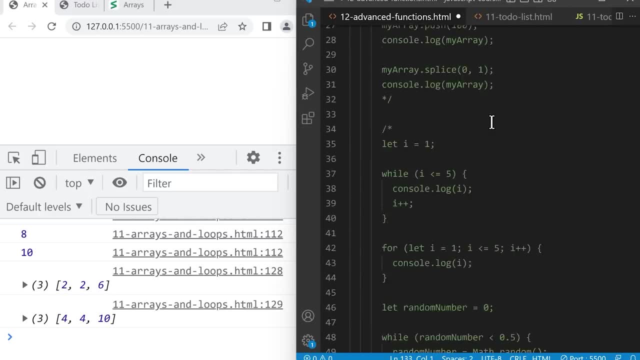 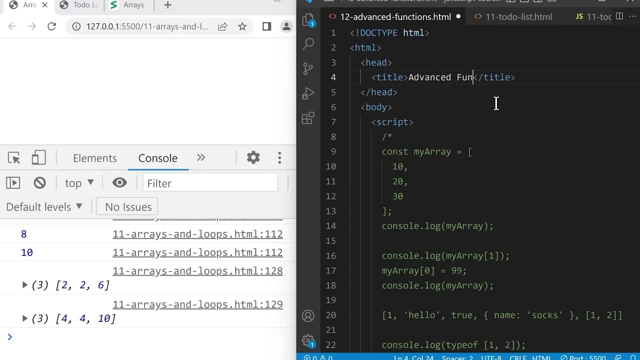 And we can close this for now, But first we're going to translate this over aneds And let's prepare this file for this lesson. So we'll scroll up and change the title to Advanced Functions And let's remove all the JavaScript code from before. 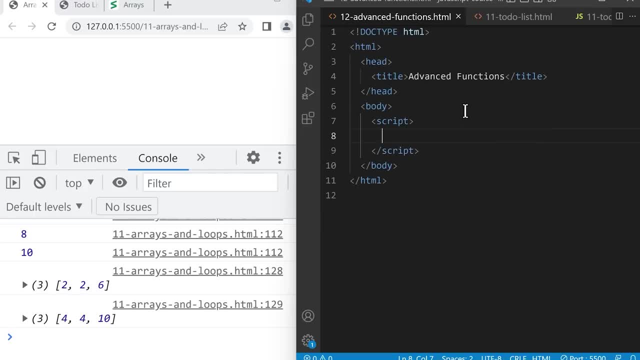 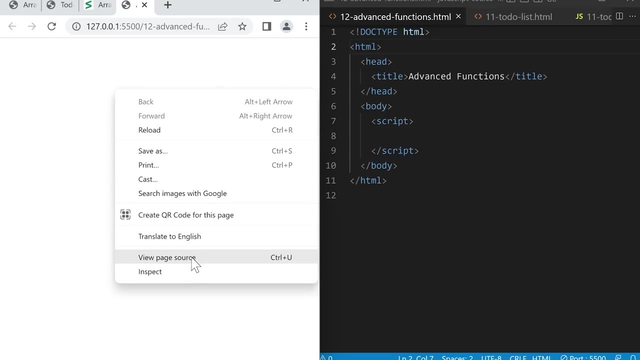 And now let's save and open this file in the browser by right-clicking Open with Live Server. Now let's also open the console on this page, So we'll right-click Inspect and open the console. And now we can close the previous tabs. 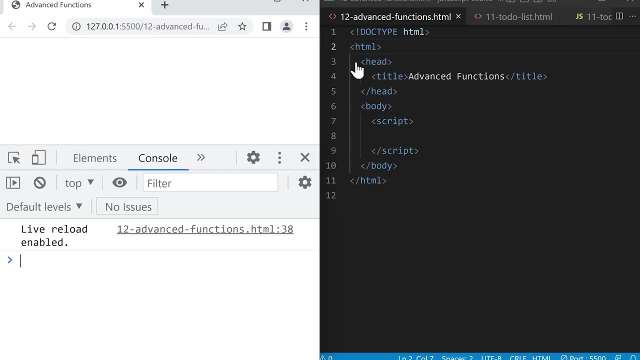 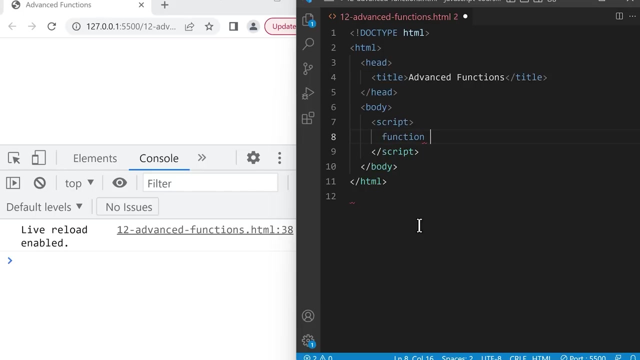 as well as the previous files. And now we're ready, Let's start to begin. So first we're going to review how to use functions Inside the script element. let's create a function using the word function. We'll give it a name. greeting brackets and curly brackets. 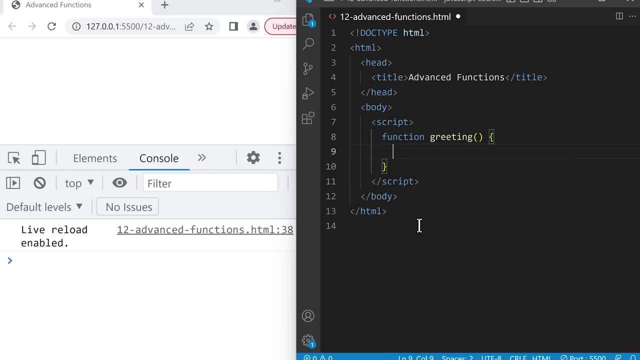 And inside the function we'll type the code consolelog, the string hello. So this is a function and it lets us reuse code. To run the code inside this function we can type the function name, which is greeting, and then brackets. 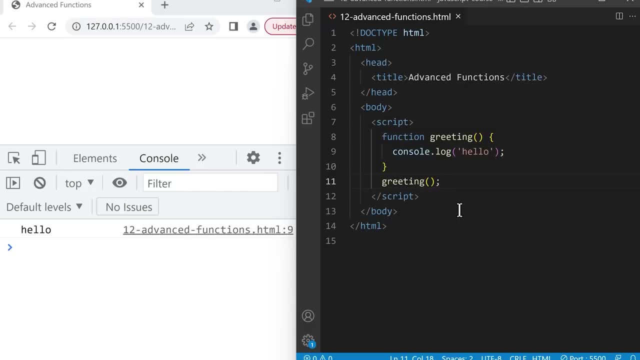 If we save, this line of code will run the code inside the function and display hello. This is known as calling. We can also call it running the function or running the function. So now that we understand functions, we're going to learn an advanced feature of functions. 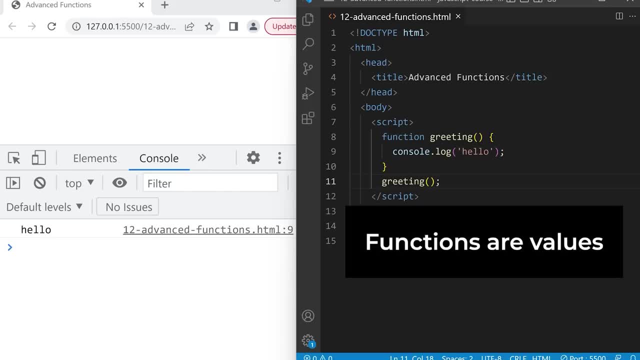 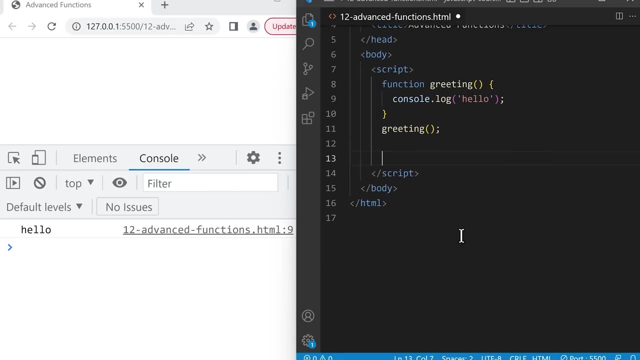 which is functions are values. So we learned many types of values in this course, like numbers, strings and booleans, And we can save a value in a variable. For example, let's create some new lines and we'll create a new line. 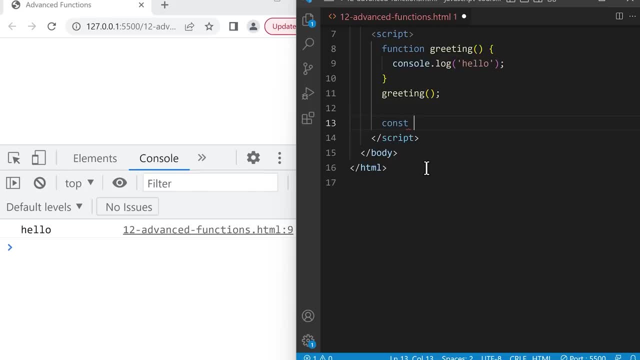 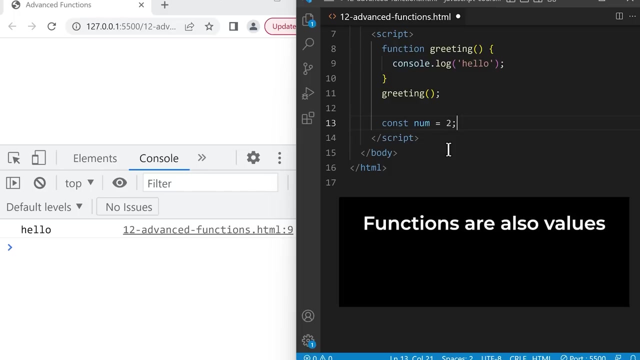 We'll create a variable const num equal two, So this will save the value two inside the variable num. Now, functions are also values, And this means, just like a number, we can save a function inside a variable. So let's give it a try. 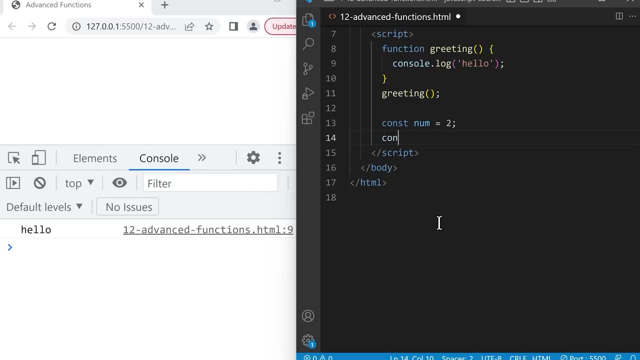 We'll create a new line and type: const. num equal two, Function one, and we'll make this equal to a function this time. So we'll just type function and a name, greeting brackets and curly brackets, And inside the function we'll type consolelog, the string hello two. 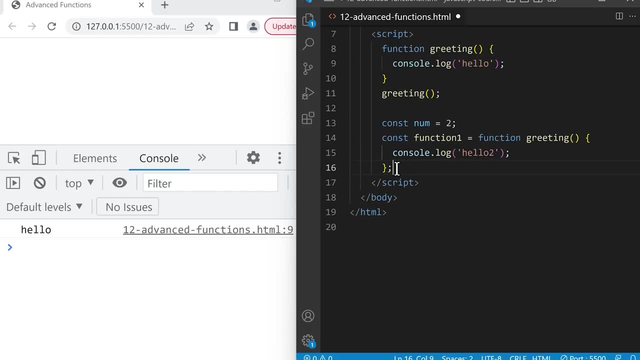 And we'll put a set function And we'll put a semicolon at the end, since we're saving in a variable. So this variable now contains a function. We're using the exact same syntax as before, except we're just taking this function and saving it in a variable. 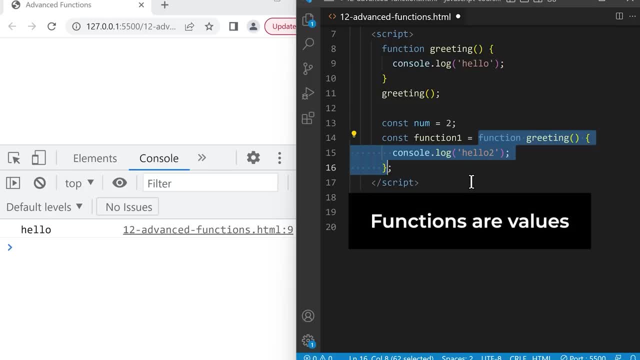 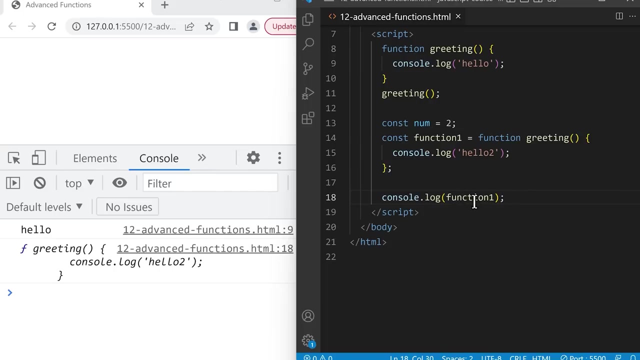 because functions are values. So now that this function is inside this variable, let's actually consolelog it. So we'll console log it, dot log function one and save, and this will show us that the variable function one actually contains this function. now, on a new line, we can also do console dot log and check the. 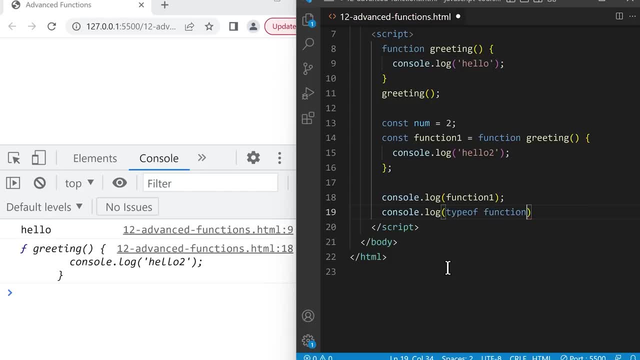 type of function, one and save, and it will tell us that the type of this variable is a function. so, as you can see, a function is just another type of value and we can save it in a variable. we can also run the function inside this variable by typing the variable name. 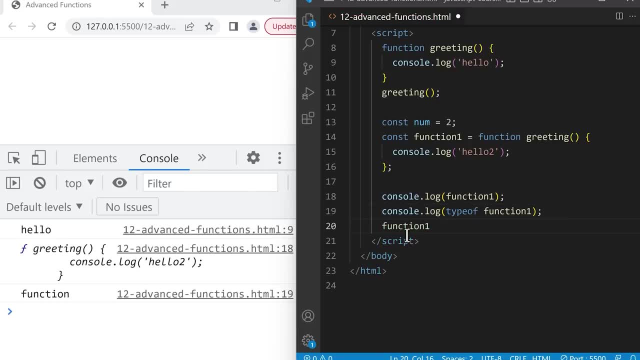 function, function one. and because this contains a function, we can actually just call it using brackets. so this will run the code inside this function. if we save, it displays: hello to. now. let's do some cleanup in this code in javascript. as long as there's a way to access a function, this function. 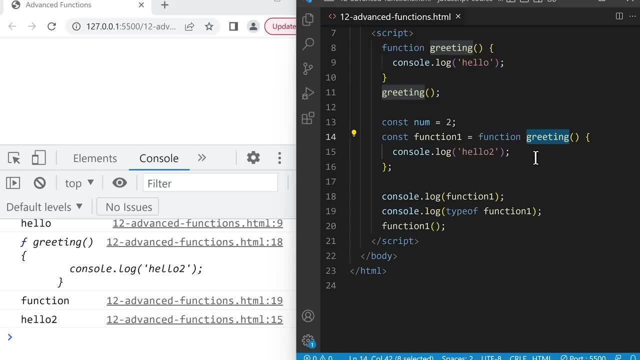 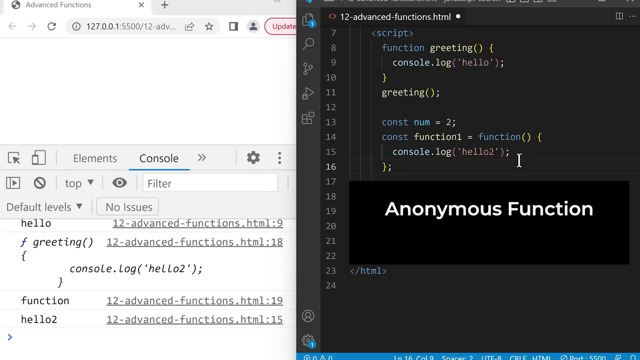 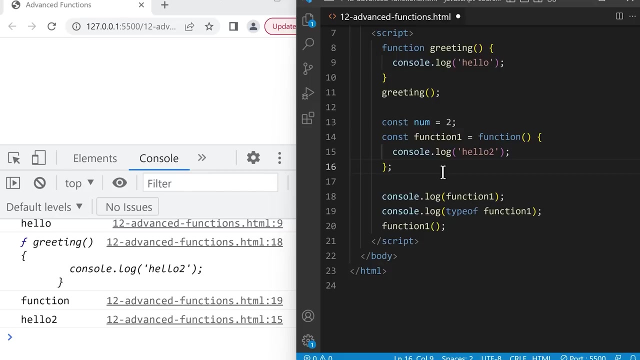 name is not needed. so here we can access this function using this variable, so this function name is not needed and we can actually just delete it like this. and now this is called an anonymous function, which means a function without a name. now, an interesting thing to know is that the 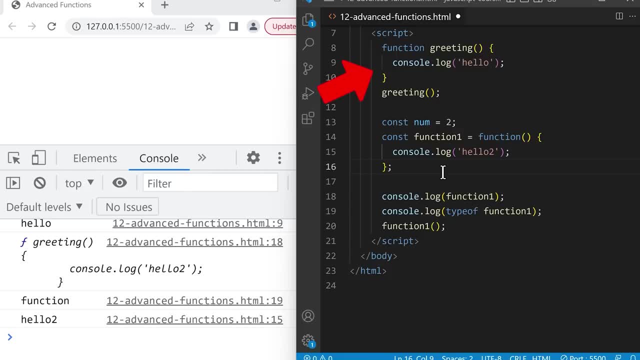 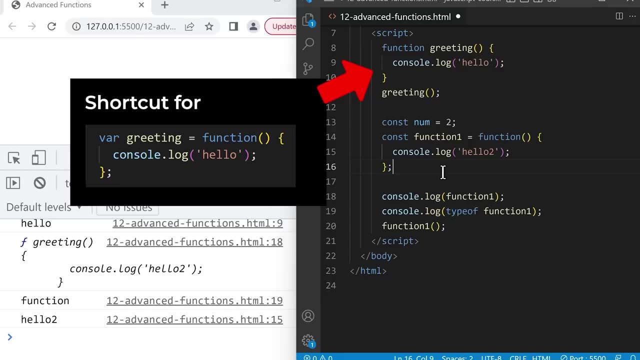 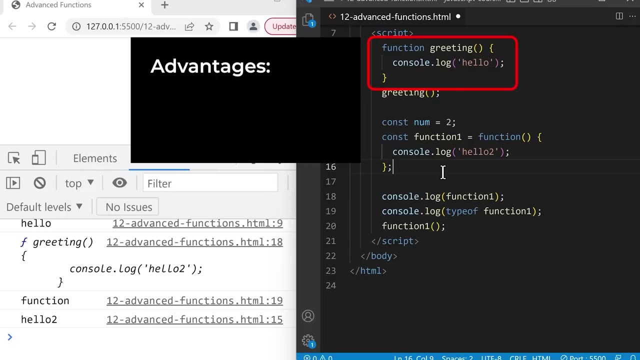 function syntax that we've been using this entire course up here is actually a shortcut for this code. now, even though this syntax uses var- and we usually don't recommend var- this syntax actually has a couple advantages. number one, it's easier to read and number two, it gives us a feature called hoisting, which means we can call this function greeting brackets. 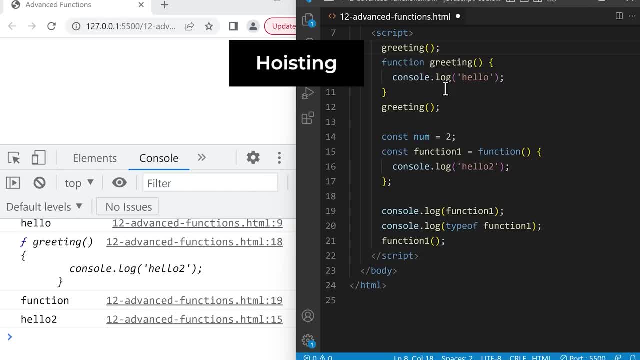 before we create it in the code. so, using hoisting, we don't have to do that hoisting, we don't have to worry about what order we write this code. Hoisting doesn't work when we create our function and save it in a variable like this: 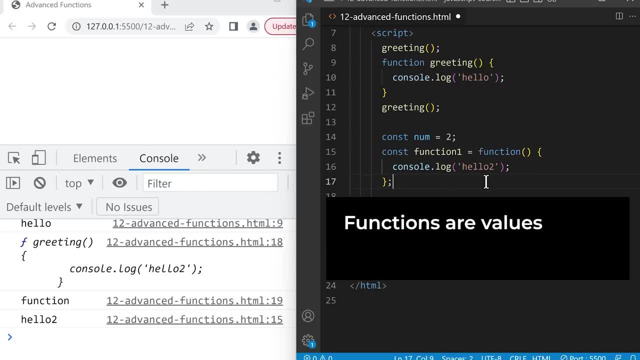 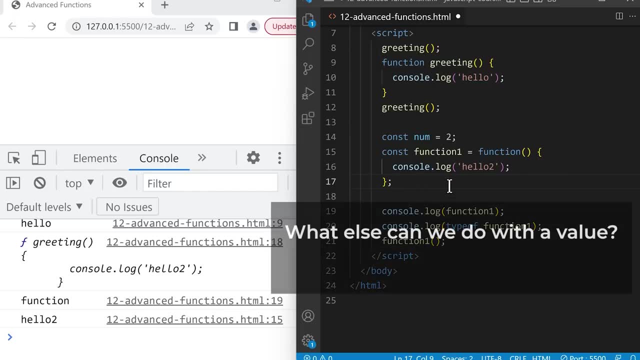 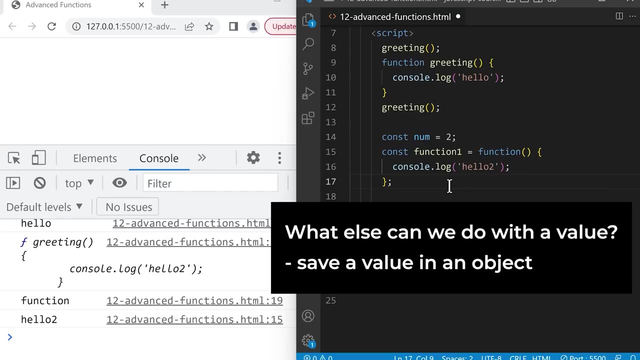 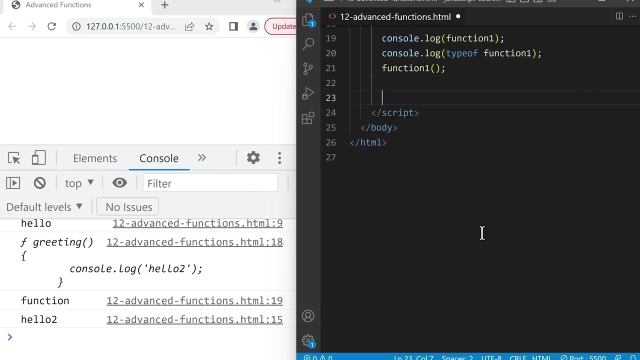 So in JavaScript, functions are values and, just like any other value, we can save it in a variable. Now let's think: what else can we do with a value? Well, we can save a value in an object. For example, let's scroll down and create some new lines and we'll create an object. 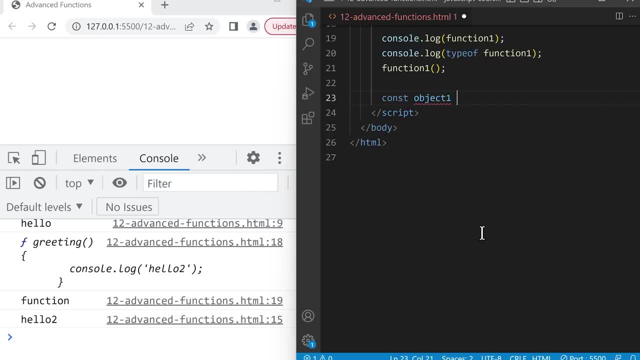 const. object1 equals curly brackets, And inside this object we'll have a property num with the value 2.. So this saves the number 2 inside this object. Now, because functions are values, we can also save a function inside this object. 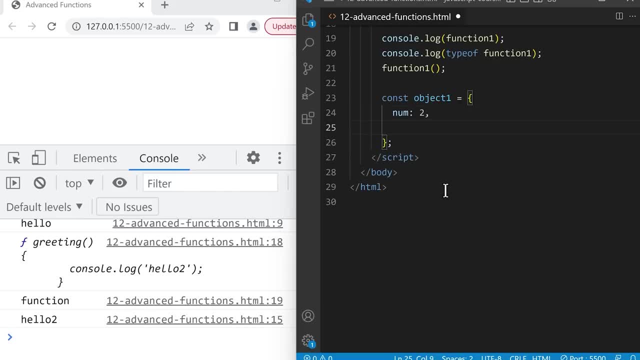 So we'll type comma and then a property fun, colon, and we'll create a function, this time function greeting brackets and curly brackets, And inside And then we'll type console dot, log the string hello 3.. So this saves a function inside this object under the property fun. 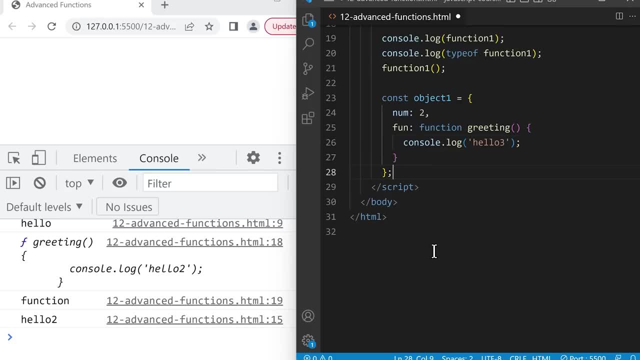 Now to access this function, we just use the dot notation as normal. So object1 dot, fun, And because this value is a function, we can call it using brackets. If we save, this will run the code inside the function and display hello 3.. 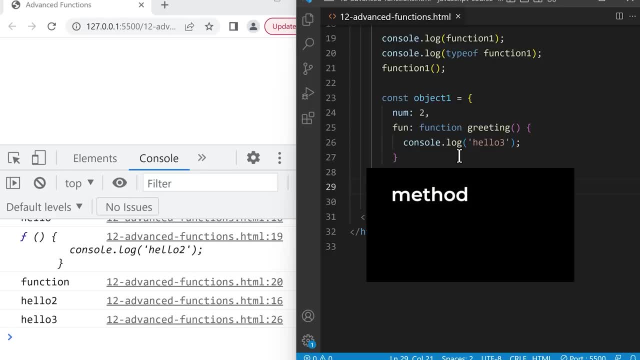 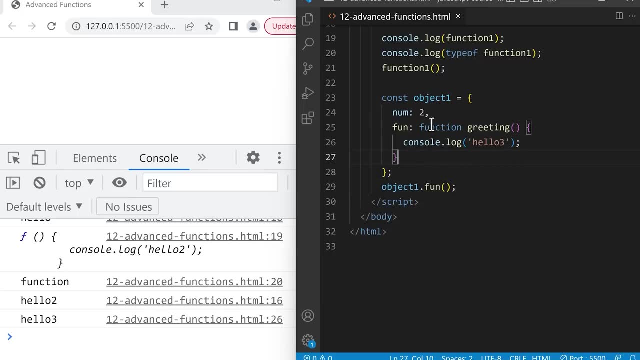 So remember this is called a method when we have a function saved inside an object. Again, as long as there's a way to access this function, For example Using object1 dot fun, then we don't need this function name. 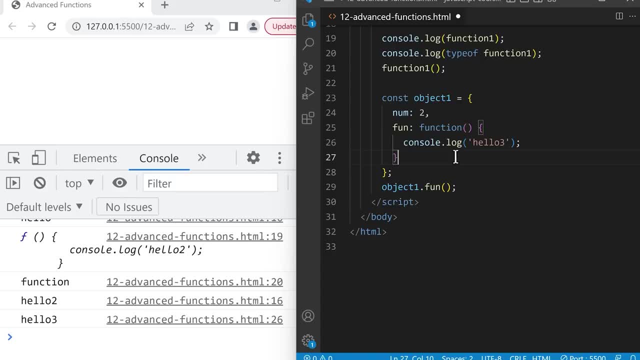 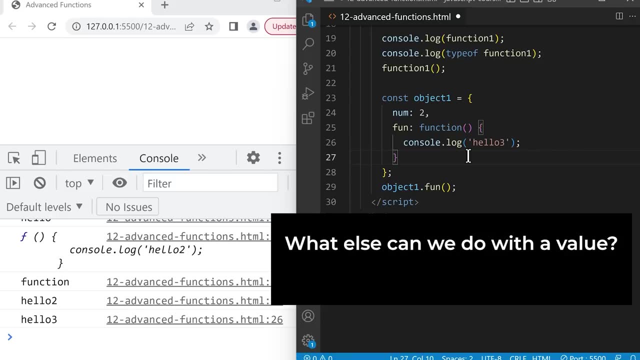 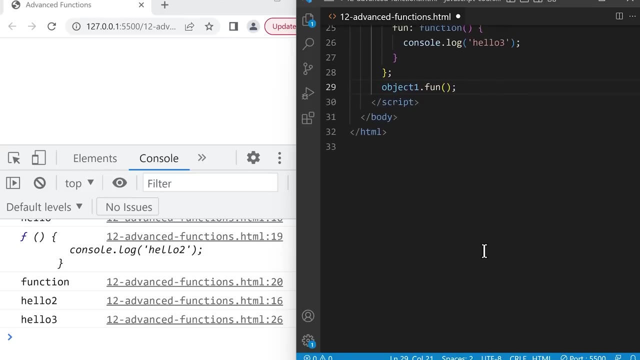 So we'll delete it and use an anonymous function. Now let's think: what else can we do with a value? We can pass a value into a function, For example down here. Let's create a function: Function Display. 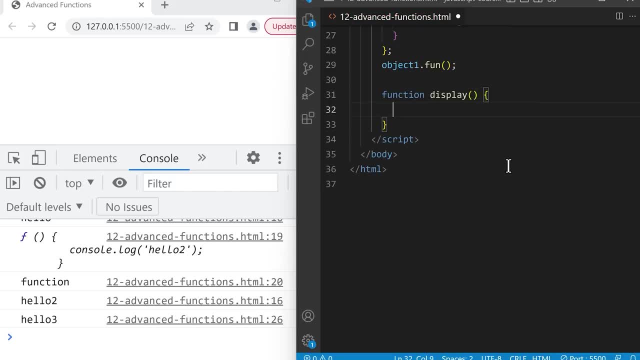 Brackets and curly brackets, And we'll give this function a parameter. So in here we'll create a parameter and name it param, And inside the function we can use a parameter just like a variable. So we'll console, dot, log the param. 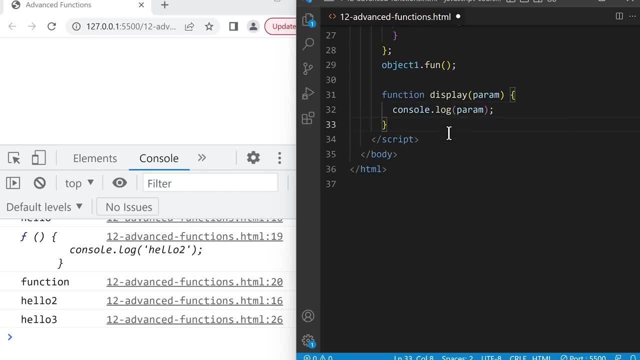 And then down here let's call this function Using display brackets and 2.. This will take the value 2, save it inside param and then we can use it just like a variable. If we save, this will display 2 in the console. 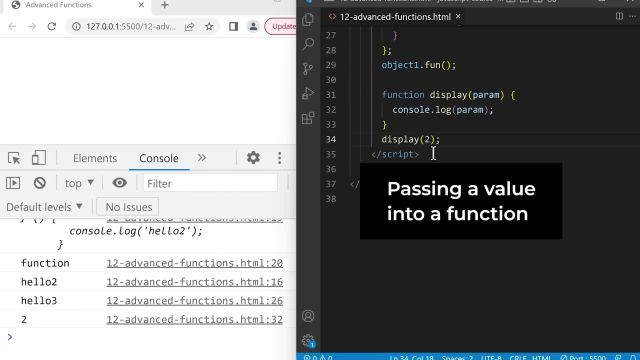 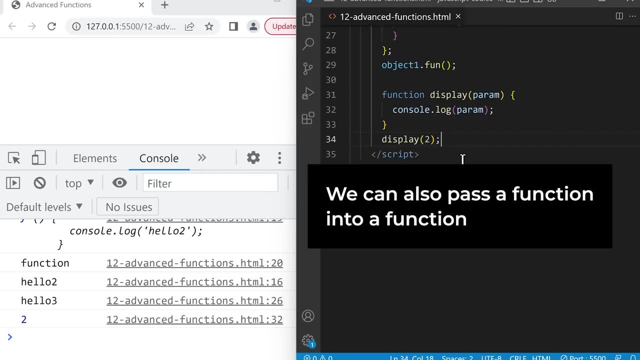 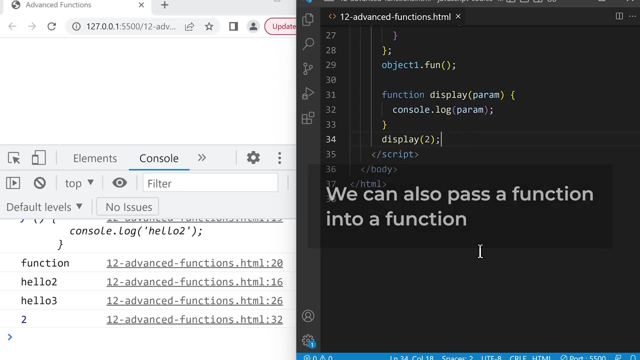 So this is known as passing a value into a function. Now, because functions are values, we can also pass a function into a function, So let's give it a try. Down here we'll create a new function Function: run brackets and curly brackets. 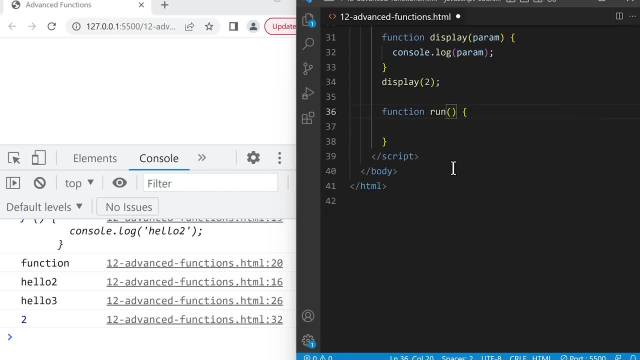 And this function will also have a parameter. Let's call it param And down here we'll call this function run brackets And between the brackets. we're going to give it a function this time, So we'll type function brackets and curly brackets. 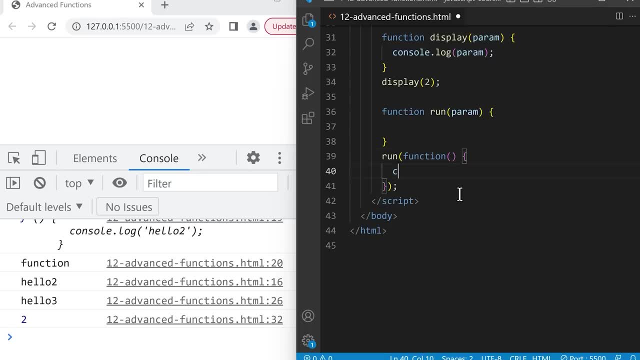 And inside the function we'll type console dot, log, the string hello, 4.. So this will take this function and save it inside param. And now up here we can use param just like a variable. So we can type param And because param contains a function, we can actually just call it using brackets. 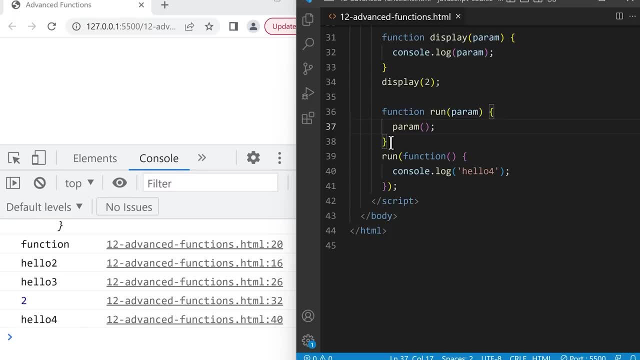 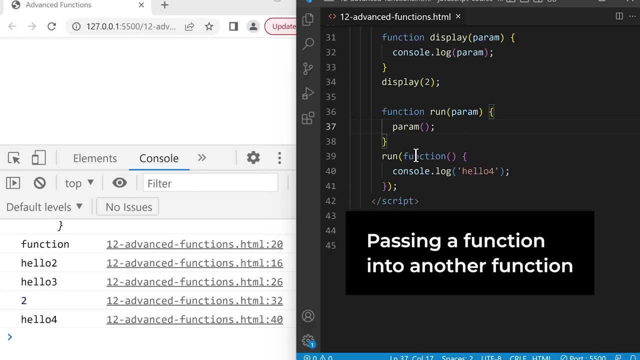 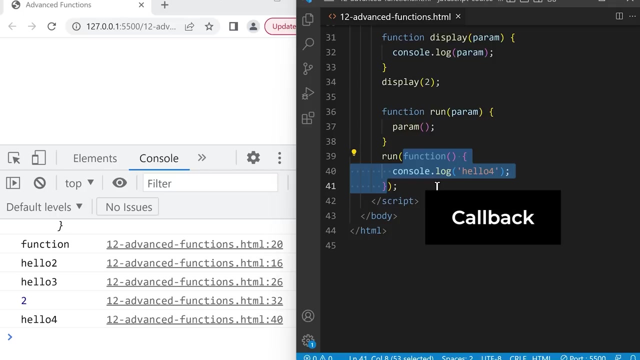 If we save this code will run the function And we can also use a function that we created down here And display hello 4.. So this is called passing a function into another function. The function that we're passing in is called a callback function or a callback. 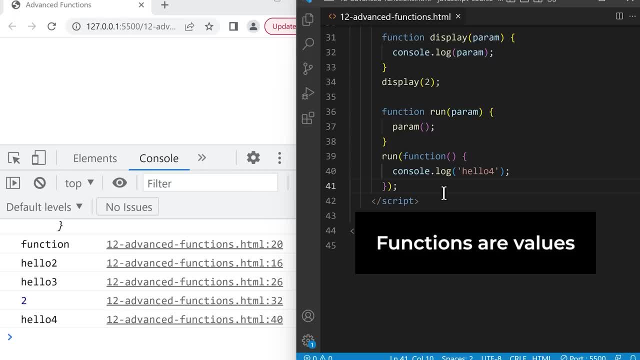 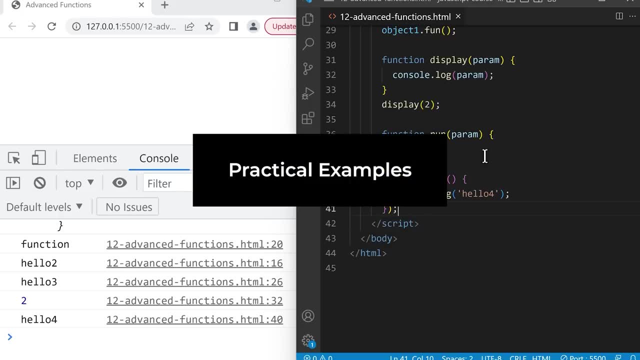 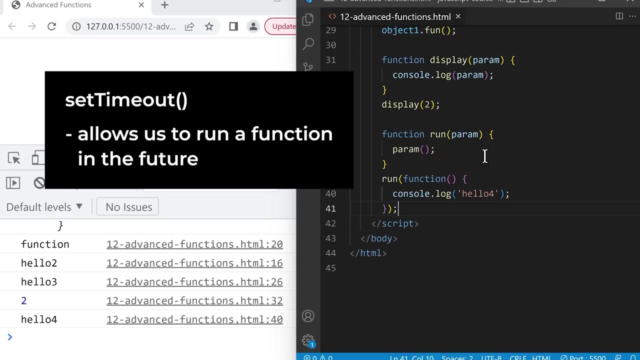 So, to summarize, functions are values. Anything we can do with a value, we can also do with a function. Now let's do some practical examples using functions as values. We're going to learn a feature of JavaScript called setTimeout. setTimeout allows us to run a function in the future. 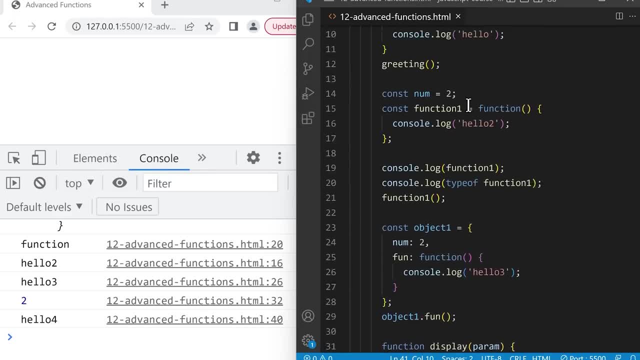 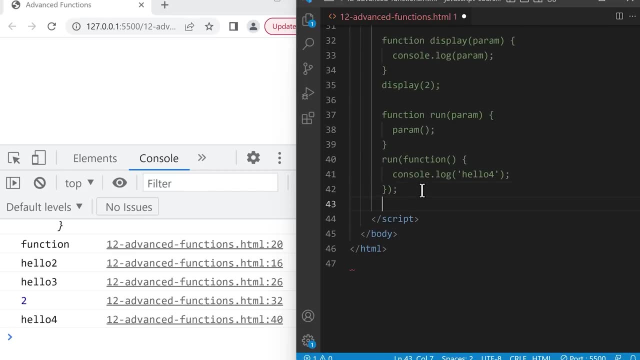 First we'll comment out the previous code Using slash star and at the bottom, star slash. And let's create some new ones And we're going to type the code set capital, T timeout. So setTimeout is a built-in function, So we can type brackets to call this function. 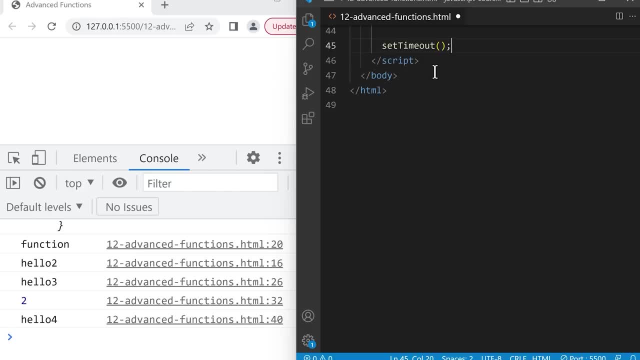 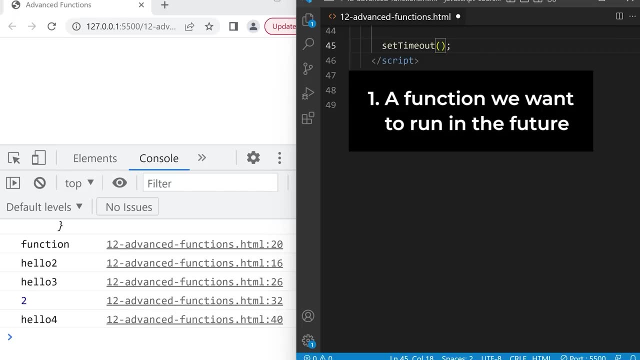 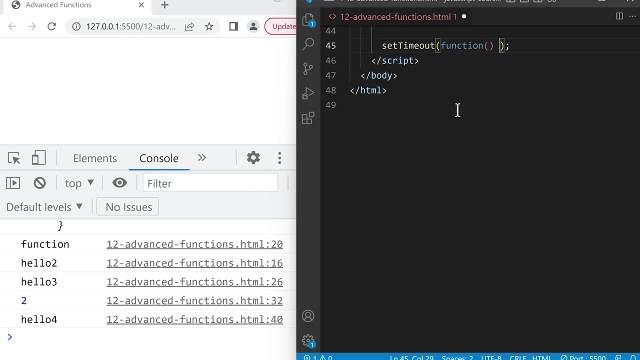 Now setTimeout takes two parameters Inside these brackets. the first parameter is a function that we want to run in the future. Let's create a function, brackets and curly brackets, And inside this function let's type console, dot, log the string timeout. So here we're using a function as a value and we're passing it into another function. 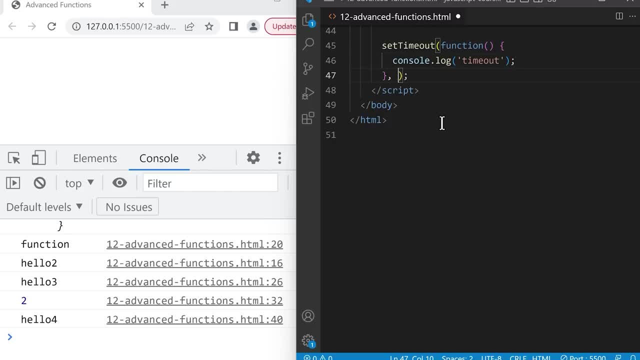 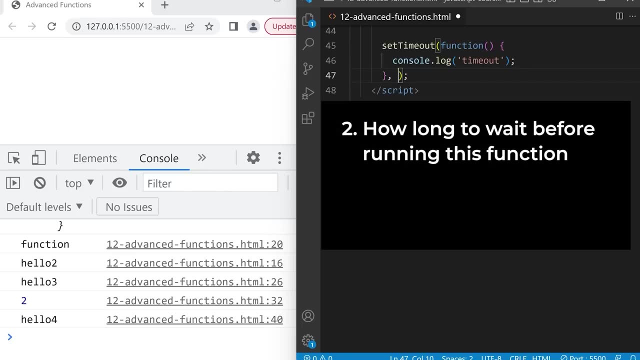 At the end we'll type a comma And we'll give setTimeout a second parameter. The second parameter is how long to wait before running this function. So this is a number in milliseconds. 1000 milliseconds is equal to 1 second. 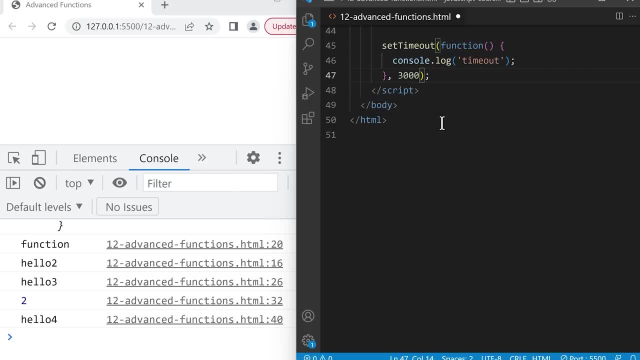 So if we type 3000 milliseconds, this is equal to 3 seconds. So setTimeout will wait for 3 seconds And then call this function. If we save after 3 seconds, it's going to display timeout in the console. 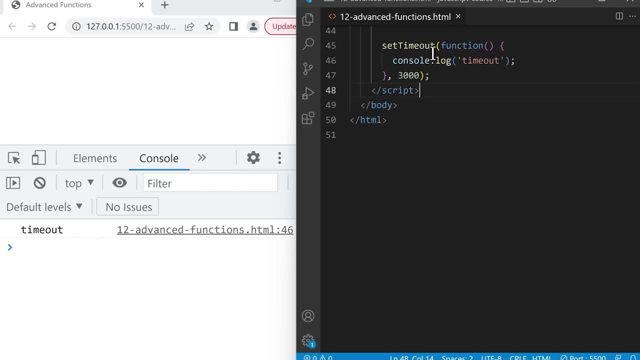 So that's setTimeout: We give it a function and it will call this function after a certain amount of time. So now we're going to learn an important concept called asynchronous code. So after setTimeout, let's type console dot log the string next line. 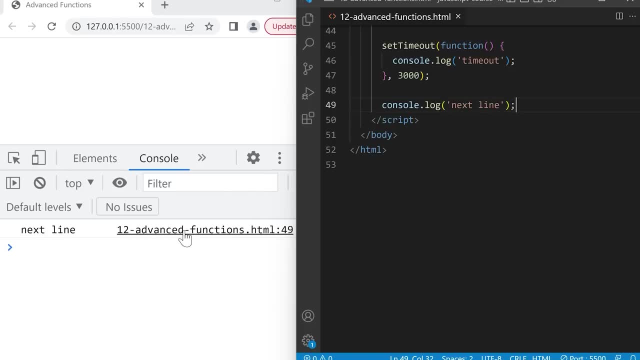 And save. So notice that it displays next line first And then, after 3 seconds, it displays timeout. So what's happening here? Why are they reversed? setTimeout sets up a timer And after 3 seconds it will call this function. 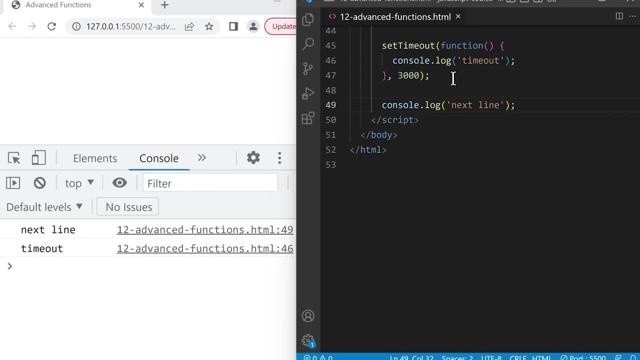 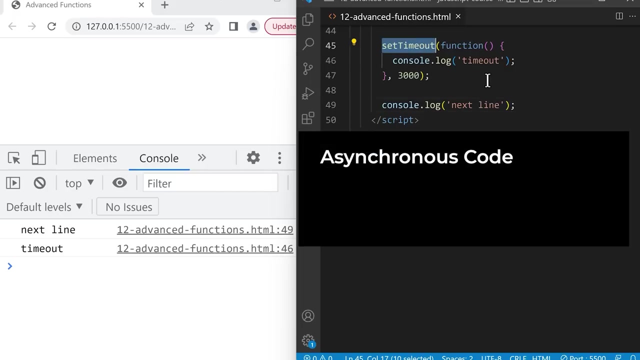 However, it doesn't actually wait for the 3 seconds to finish. It just sets up the timer and immediately goes to the next line. So that's why this line is displayed first. So this is called asynchronous code. Asynchronous code means the computer won't wait for this line to finish. 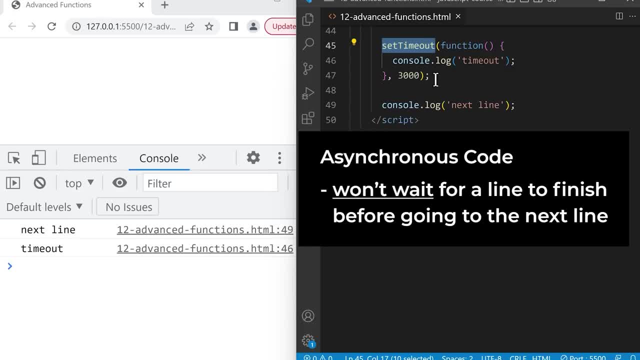 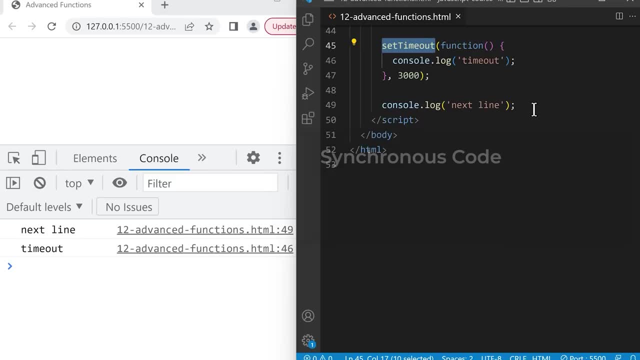 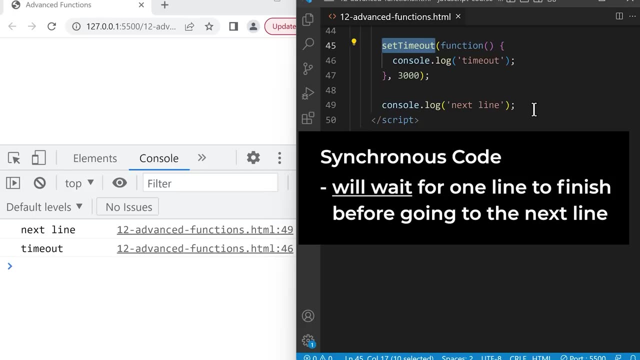 before going on to the next line. So for setTimeout, it'll just set up the timer and then immediately go to the next line. Synchronous code, on the other hand, means the computer will wait for one line to finish before going to the next line. 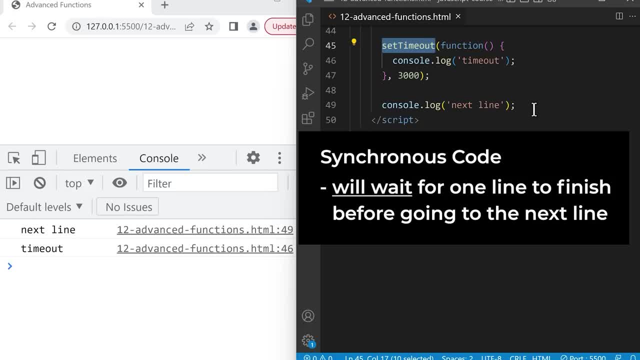 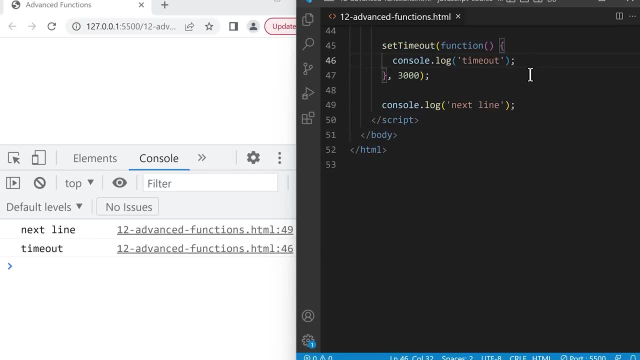 So all the code we've written in this course so far has been synchronous code. In addition, all the code inside this function is also synchronous code. So if we added consolelog the string timeout2 and save the code inside, the function will still run line by line. 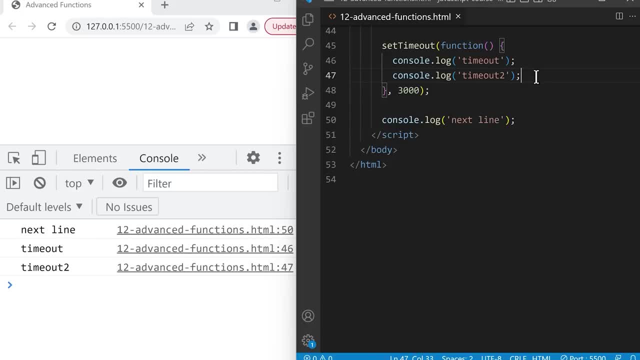 It will wait for each line to finish before going to the next line And after 3 seconds it will display timeout, followed by timeout2.. So, don't worry, all the code that we normally write will be synchronous code. It will run line by line. 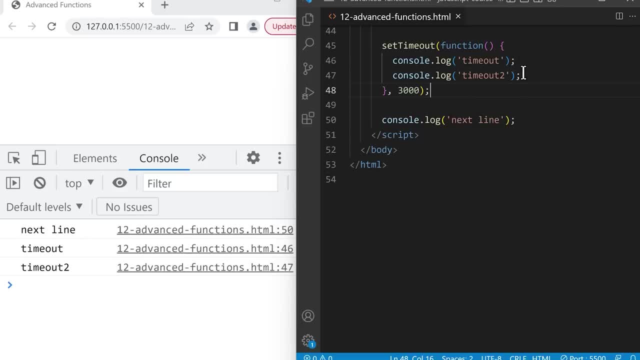 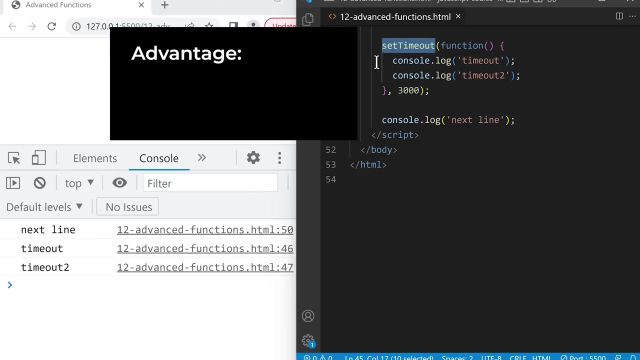 as usual, The only time that code becomes asynchronous is when we use certain features of JavaScript like setTimeout, So setTimeout is the only part that is asynchronous. Now, the advantage of setTimeout being asynchronous is that it doesn't block our code for 3 seconds. 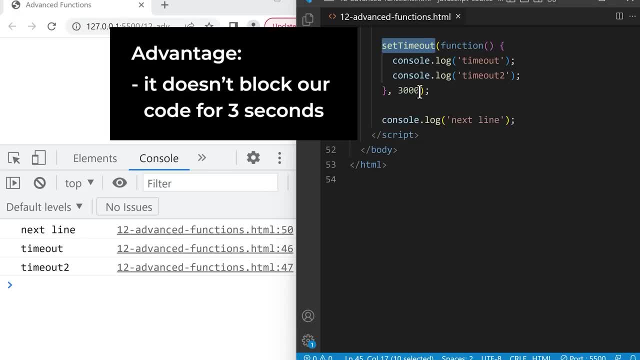 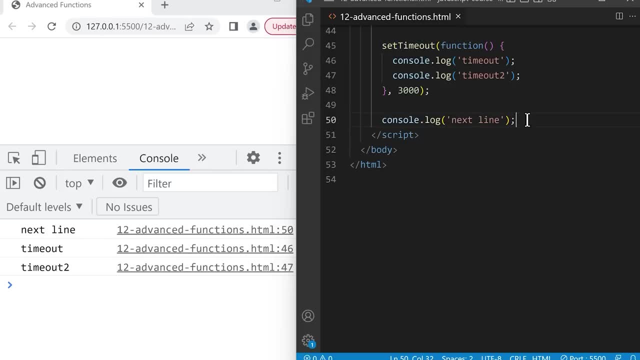 waiting for this timer to finish. It just sets up the timer in the background and then goes to the next line of code, So this allows our code to do other things while this timer is running in the background, And this is similar to real life. 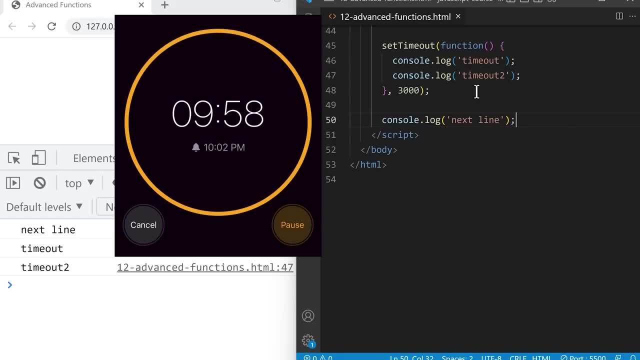 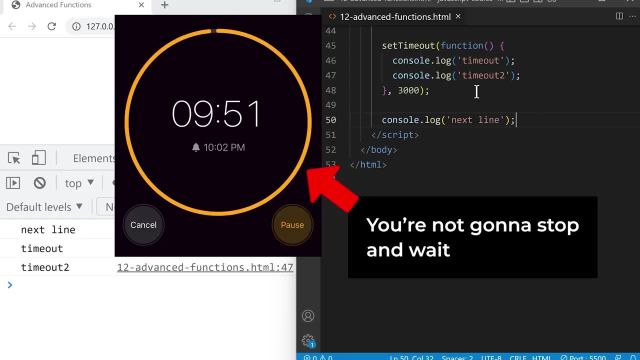 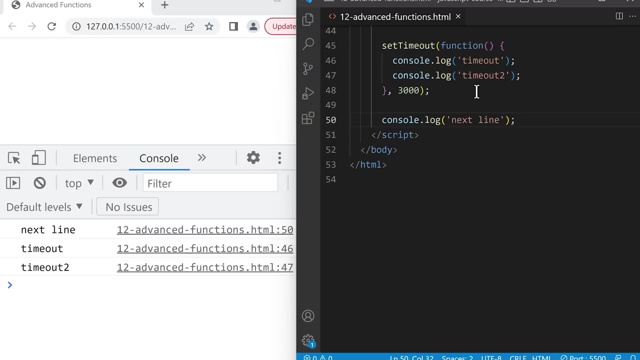 If you set up a timer on your alarm clock, you're not going to stop and wait for the timer to finish. You're going to go and do something else. Asynchronous code is the exact same concept. Next, we're going to learn a similar function. 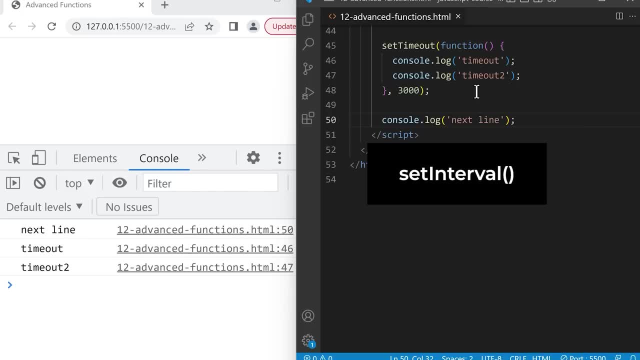 to setTimeout called setInterval. So at the bottom let's type the code setIinterval. and setInterval is another built-in function, So we can call it using brackets, And setInterval takes the same two parameters as setTimeout. The first parameter is a function that we want to run. 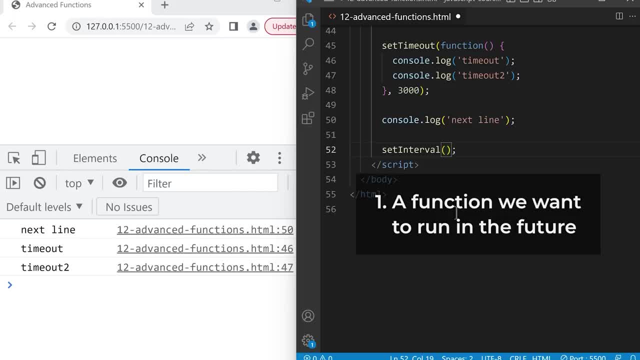 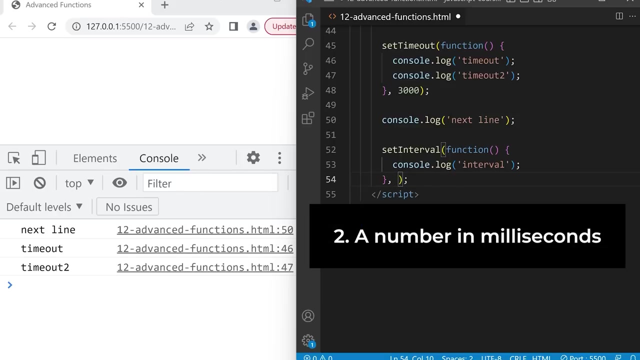 in the future. So let's type function brackets and curly brackets and inside we'll type consolelog, the string interval. Now let's add a comma, and the second parameter is also a number in milliseconds. So we'll type 3000 milliseconds or 3 seconds. 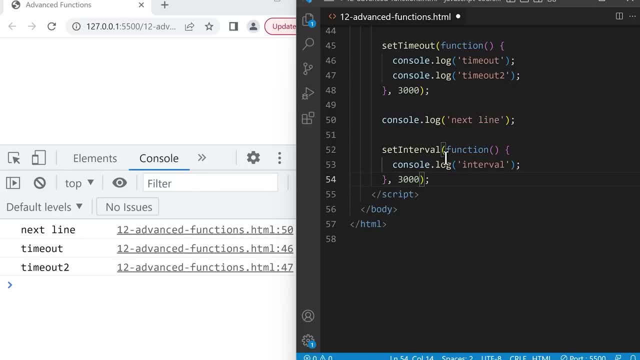 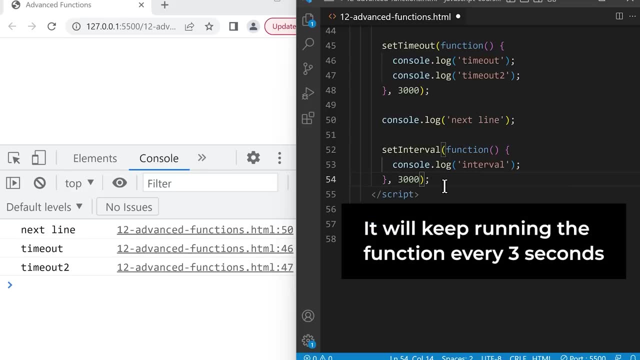 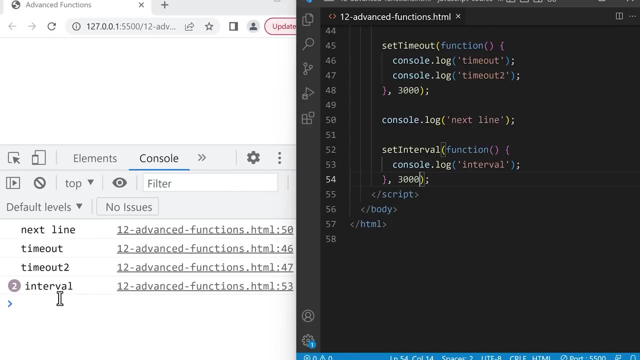 So setInterval will run this function 3 seconds in the future, But this time it will keep running the function every 3 seconds. If we save in the console every 3 seconds, it will run the function and display interval. So setInterval. 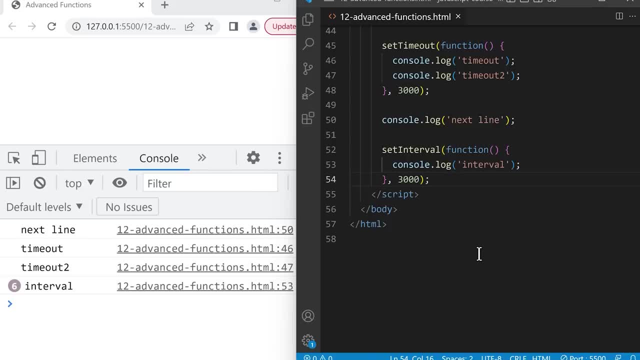 is also asynchronous Below it. if we type consolelog the string nextLine2 and save, it will set up the interval and then immediately go to the next line and display nextLine2.. So that's setInterval. We give it a function and it will keep. 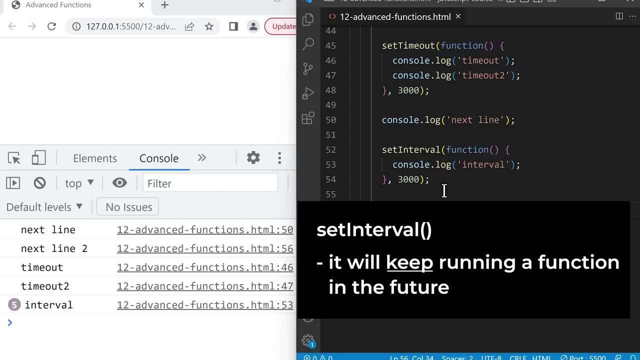 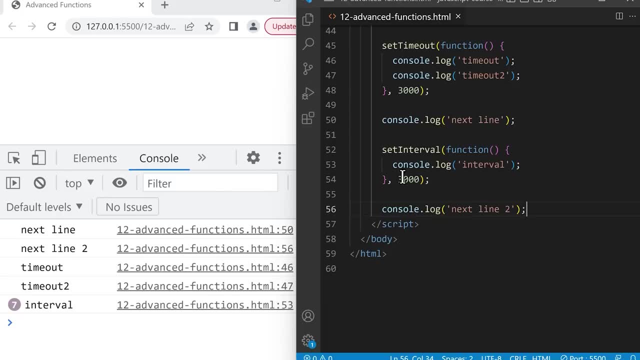 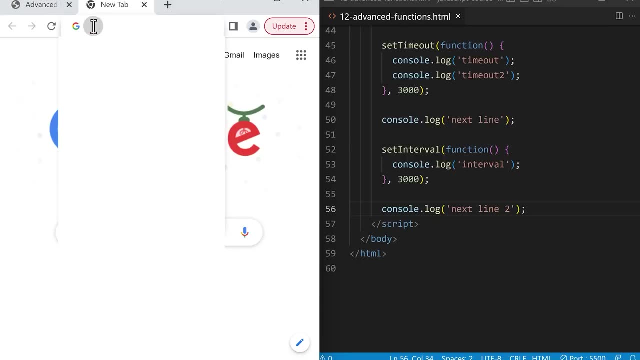 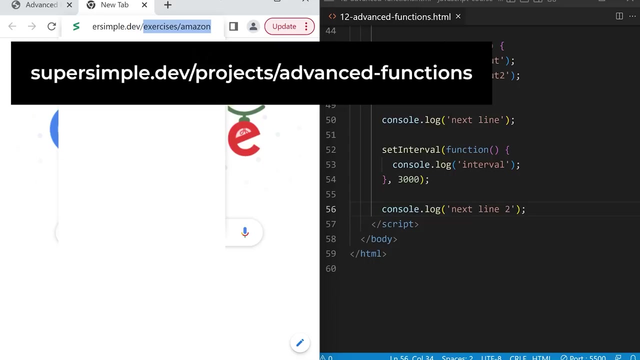 running this function after a certain period of time. So now let's do a project using what we learned so far. Let's go to our browser and we'll create a new tab at the top and here let's type super simple dot dev slash projects. 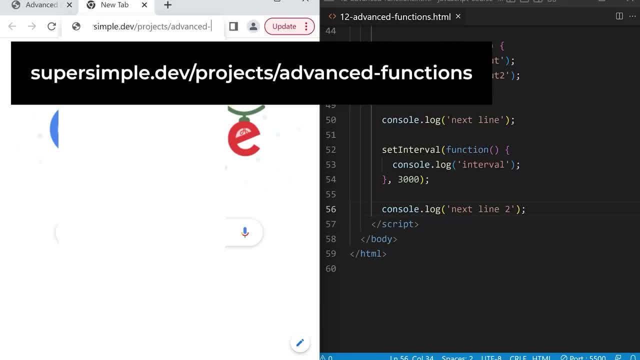 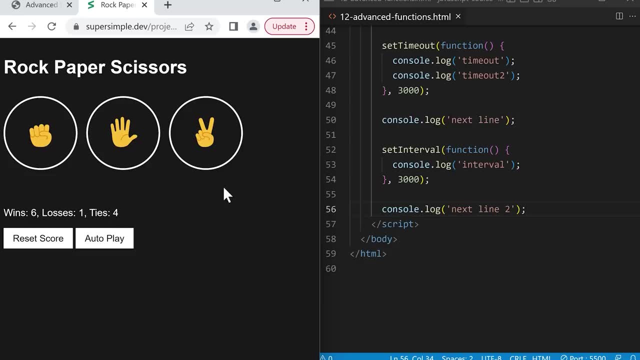 slash advanced dash functions and press enter. So this is basically the rock paper scissors game that we created earlier, Except this time it has an extra button called autoplay. If we click this button every second, the computer will play by itself, So this feature will help us. 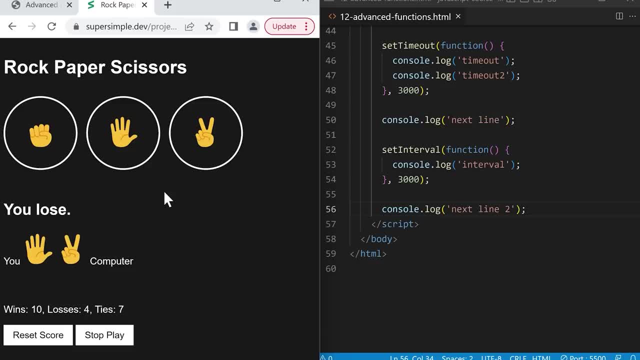 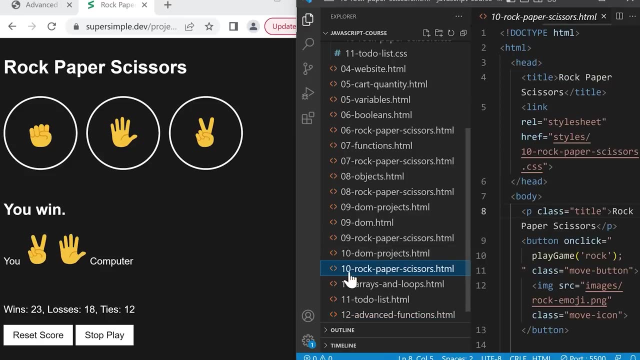 practice using set interval. So first let's make a copy of the project files. We'll go into our code editor and click this icon to show our files. and let's make a copy of 10 rock paper scissors for this lesson. So we'll 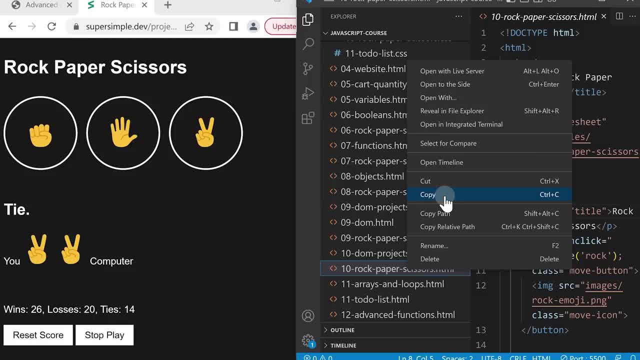 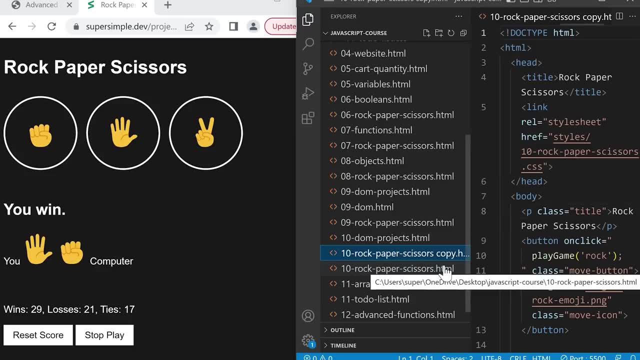 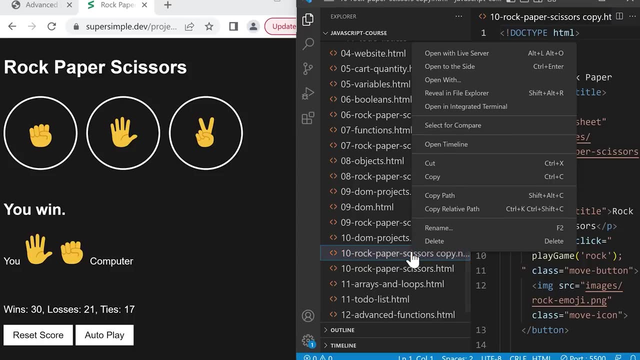 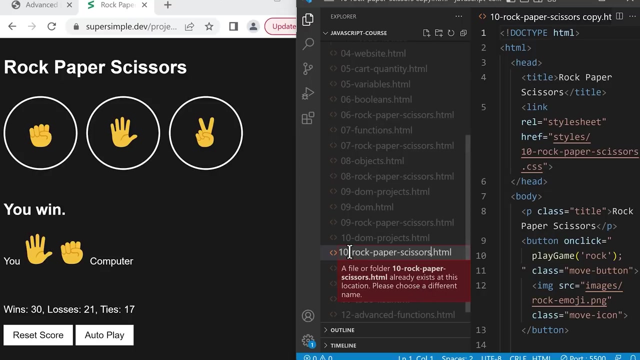 right click copy and down here right click and paste, And I'll stop this for now. So here we're gonna change the name by right clicking rename. We'll remove copy at the end and at the beginning we'll change it to 12 and press. 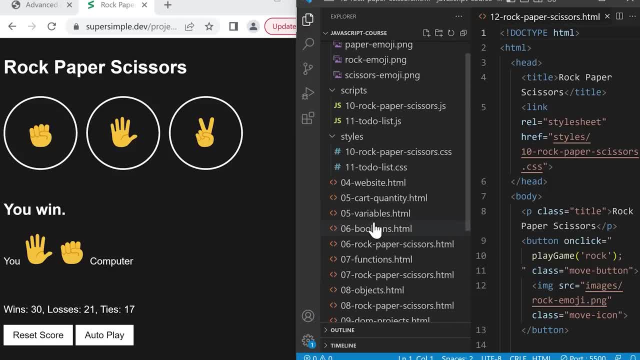 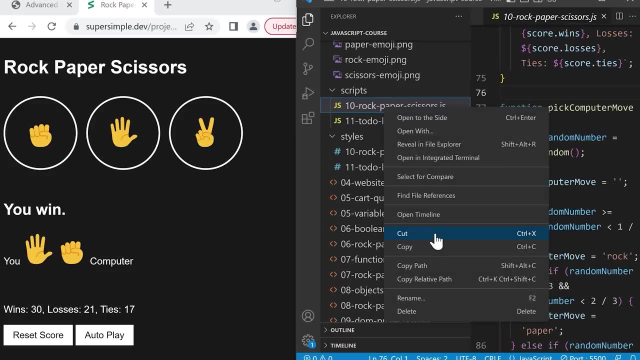 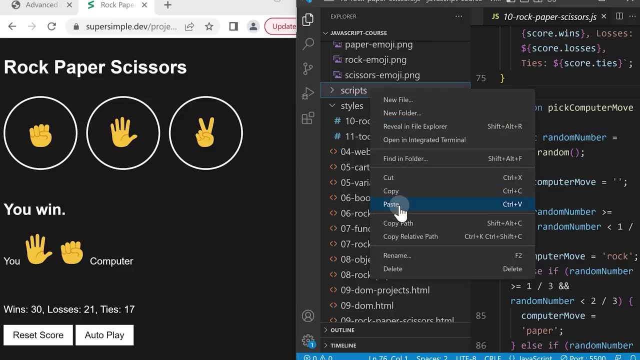 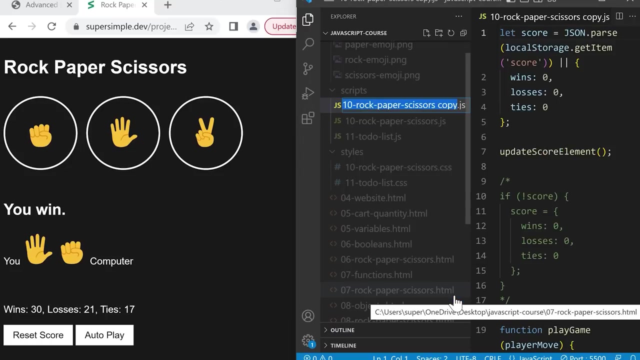 enter And let's also make a copy of the javascript and css files. So we'll click this copy and then click the folder, right click paste and we'll rename this file. Right click rename, remove copy at the end and at the beginning change it. 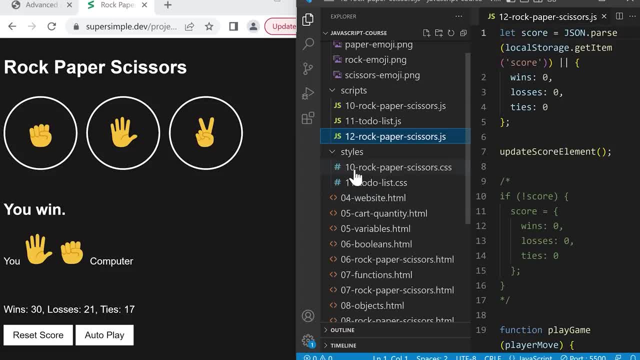 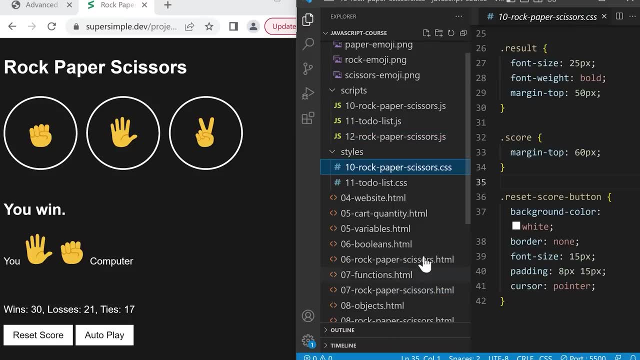 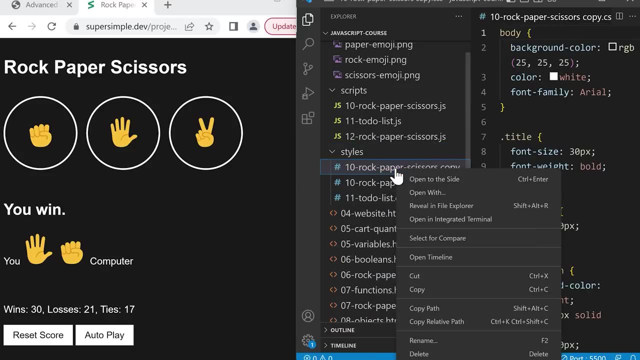 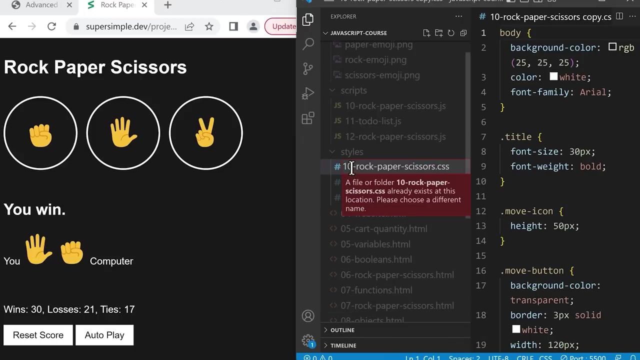 to 12 and press enter. And let's also make a copy of the css file. We'll remove copy and at the front, change it to 12 and press enter. Now let's scroll down to 12 rock paper scissors and I'll close. 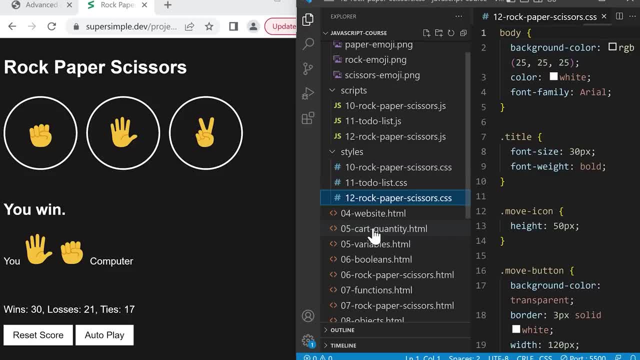 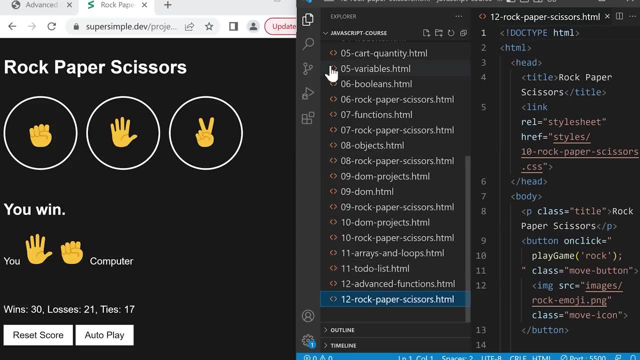 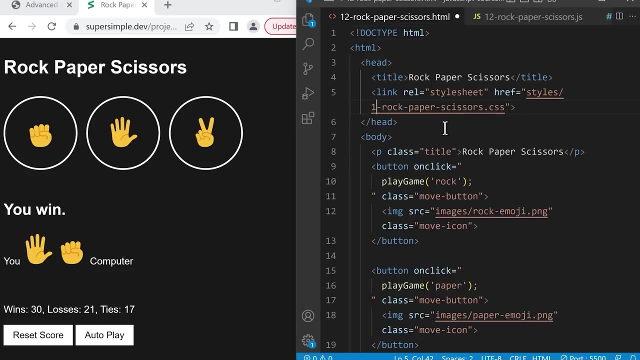 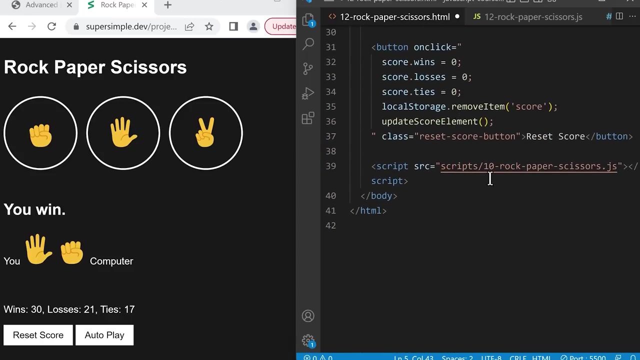 this for now, And now we're gonna change this to 12 rock paper scissors and inside the head let's change this to load 12 rock paper scissors And we'll scroll to the bottom and here, instead of the lesson 10 file, we'll 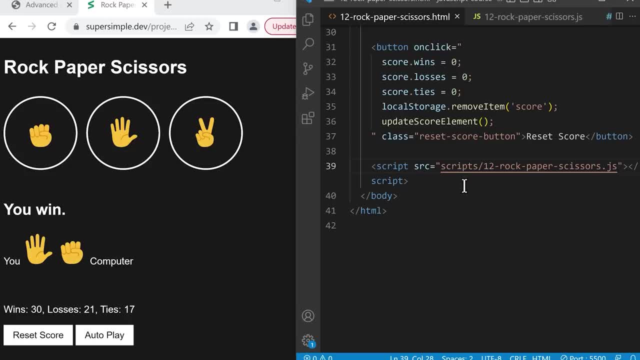 load the lesson 12 javascript file. Let's save and we'll open this file. So now we're ready to begin. Let's go back to supersimpledev, and the first thing we're gonna create is this autoplay button. So, beside the reset, 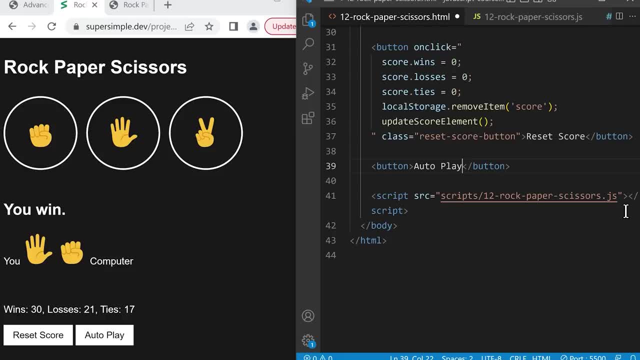 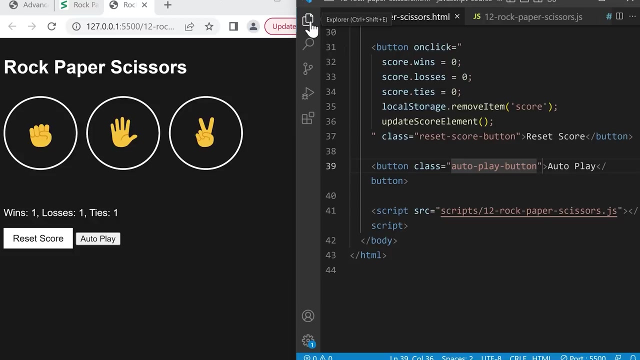 score button, which we've already created. let's save and go back to our tab, and now we have this button. So next let's style this button with CSS So we'll give it a class. class equals auto dash play dash button I'm gonna take. 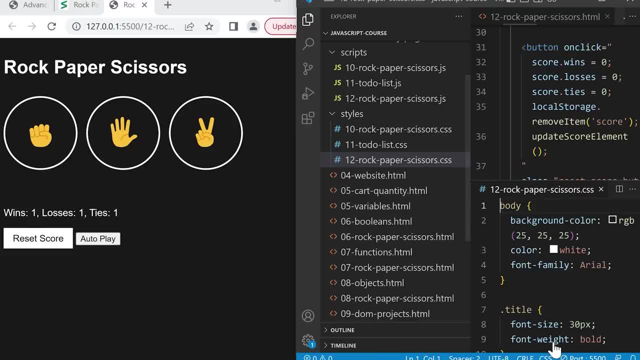 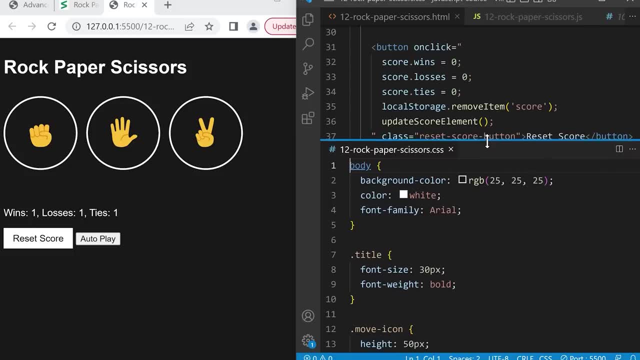 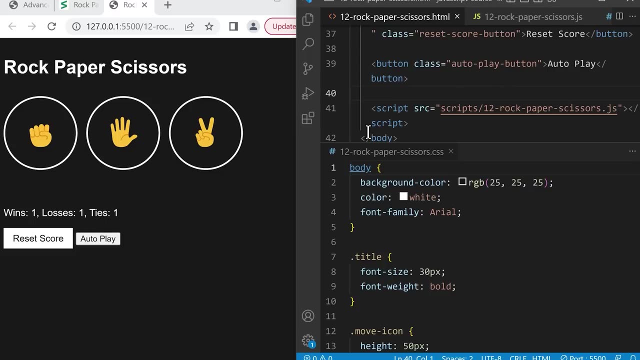 this file and then drag it to the bottom so I can see it side by side. So I'll close this for now and rearrange this a little bit, and then down here and we're gonna style the auto play button. So let's just make. 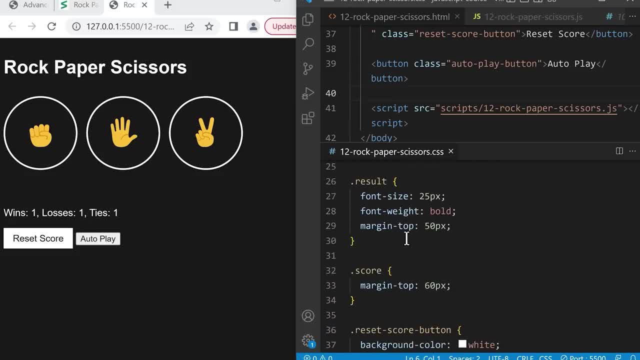 the style the same as the reset score button styles. So we'll add a comma at the end and type dot auto dash, play dash button. So now these styles will apply to the class reset score button and the auto play button If we save this. 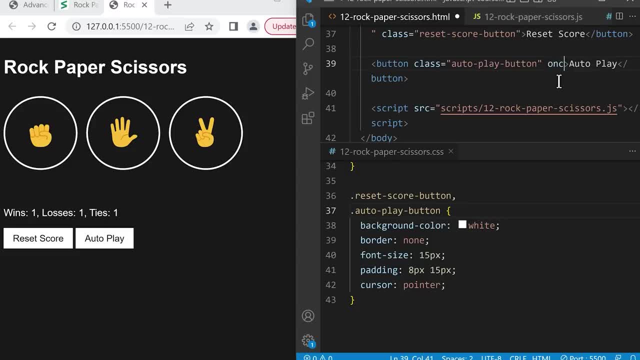 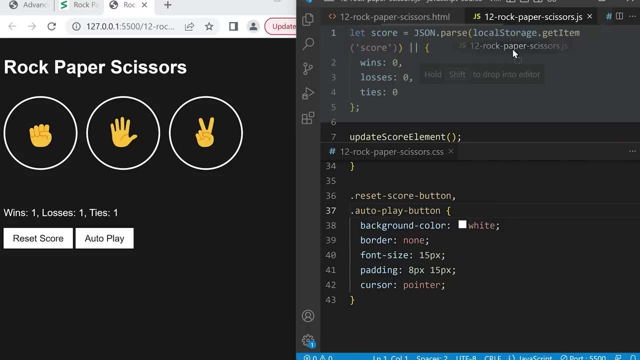 file, we'll see that we have a function called auto play and brackets. So now let's save. and right now this file has a function called auto play, and right now this function doesn't exist. So we have to create this function in the javascript file. 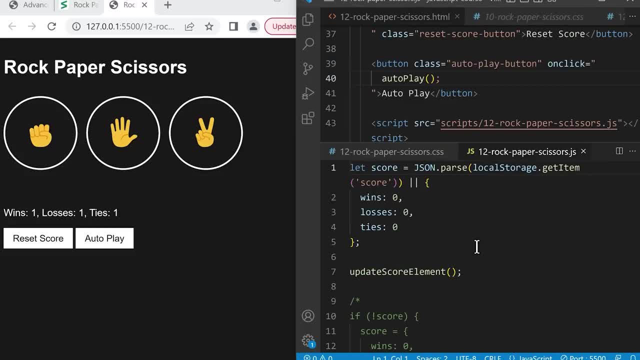 So for me the file is right here. I'll select it and then drag it down here so I can see it side by side. So let's scroll down and we'll see that we have a function called auto play brackets and curly brackets. And now 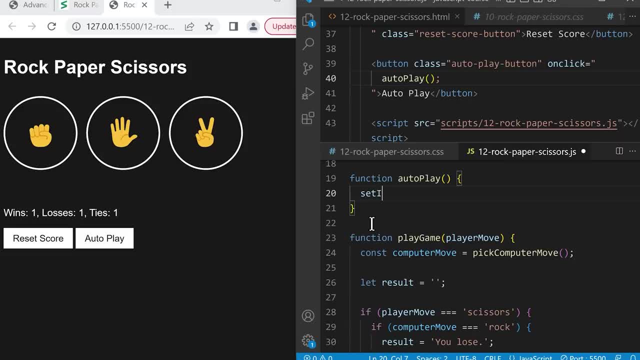 inside this function. we want to play the game every second, So we want to run So brackets and curly brackets, And then at the end let's type a comma and we'll give it 1000.. So this means it will run this function. 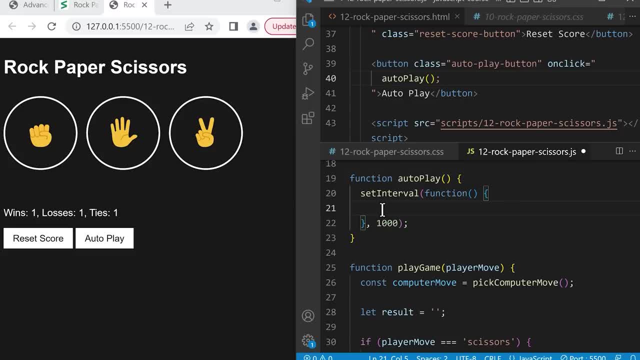 every 1000 milliseconds or one second. And now inside this function we'll type play game. So here we'll type play game brackets. Now we need to provide this function with a player move. And remember we have another function: pick computer move, which? 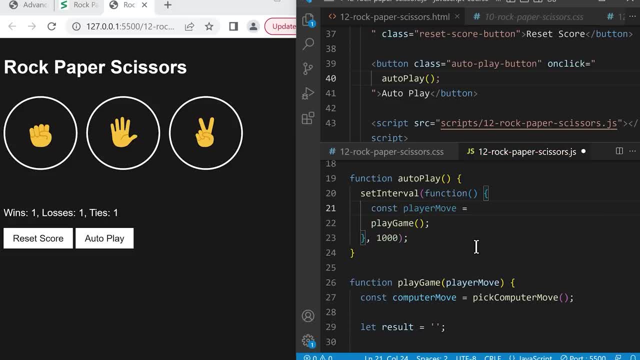 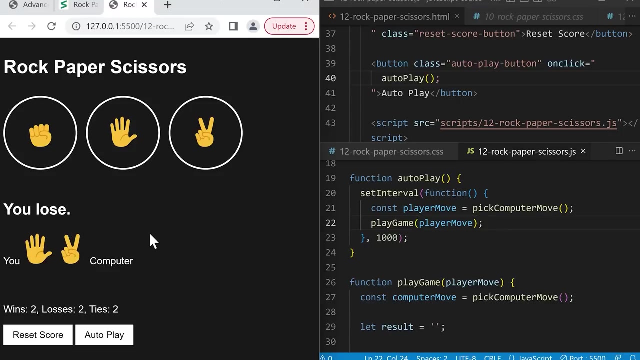 is random move And we'll make it equal and we'll pick a random move using pick, computer move and brackets, And finally we'll take this move that we picked and pass it in every second. Let's save and click autoplay and it works. 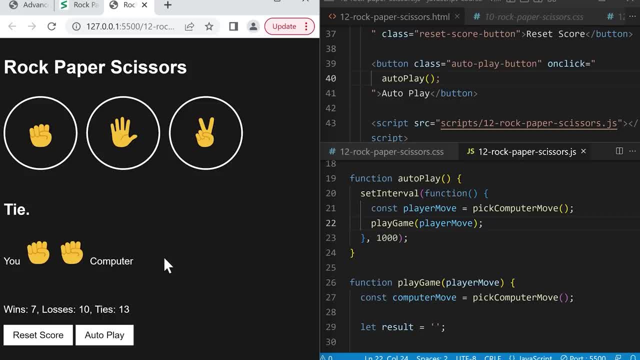 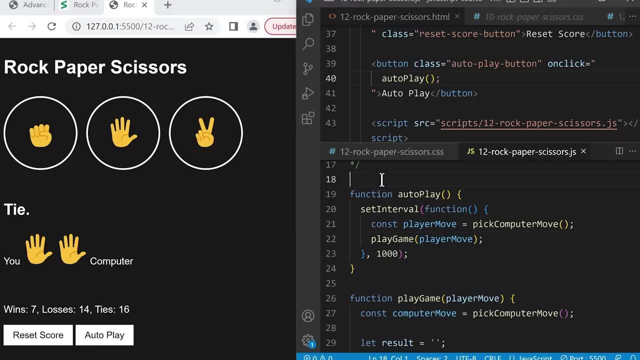 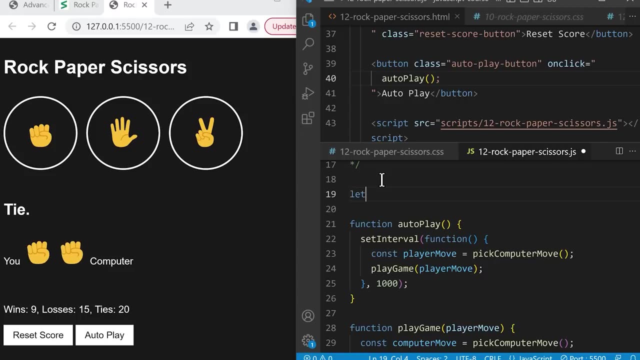 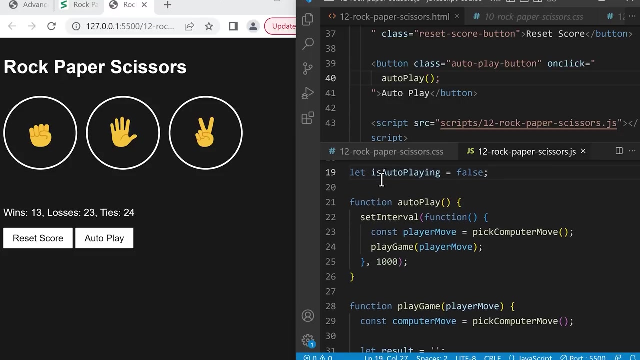 The computer is playing against itself every second. So now let's make this button stop playing when we click it again. So let's check if we're not playing, and at the start we'll make it equal to false and save. And now inside this: 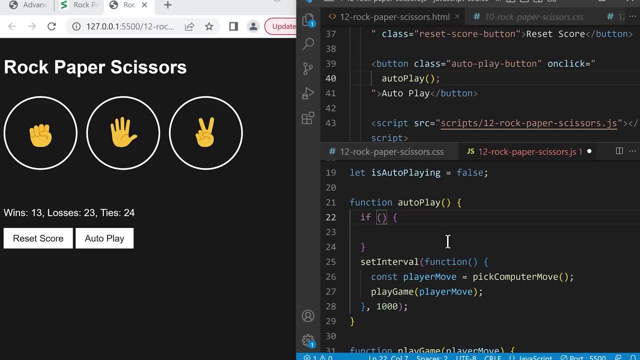 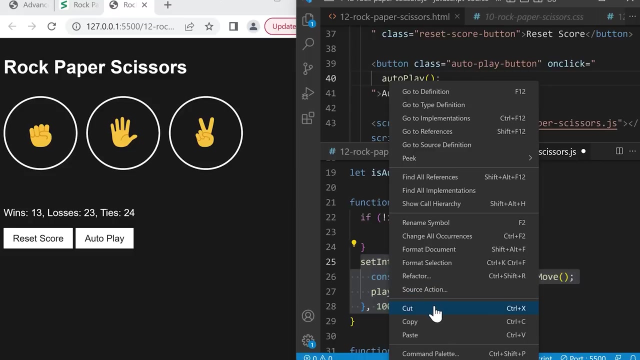 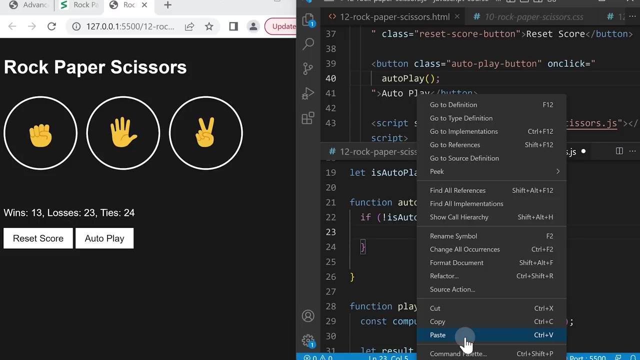 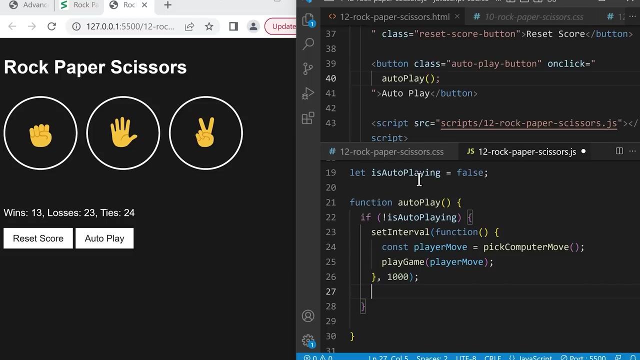 function. we'll check using an if statement, brackets and no playing. So if we're not playing, then we want to start playing the game, which is this code down here. So let's select this code and then right click, cut and in this case we'll. 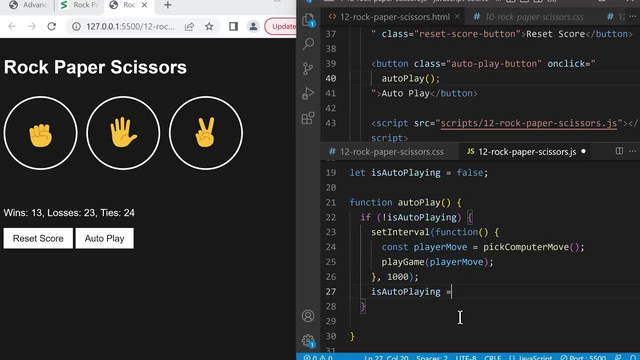 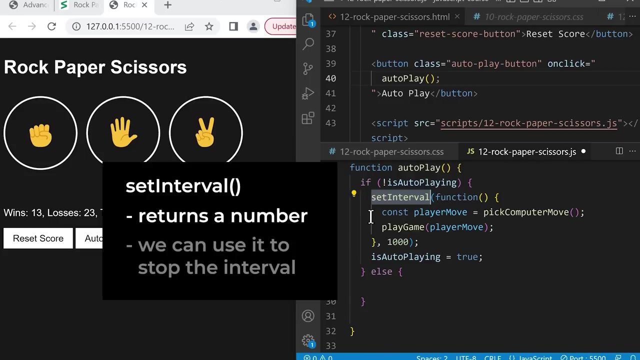 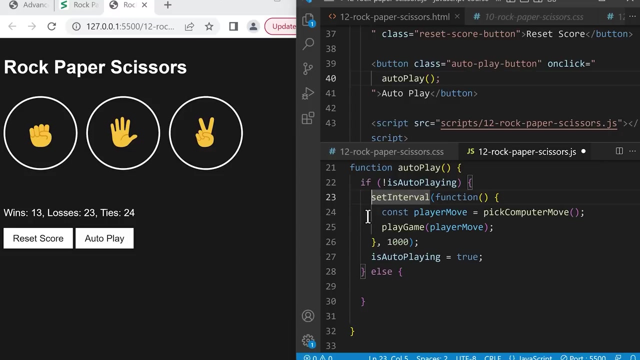 make it equal to true, because now we are auto playing. So now let's add the else branch to this statement: Else curly brackets. so now we need to create a variable that returns a number, and this number is like an id. We can use this. 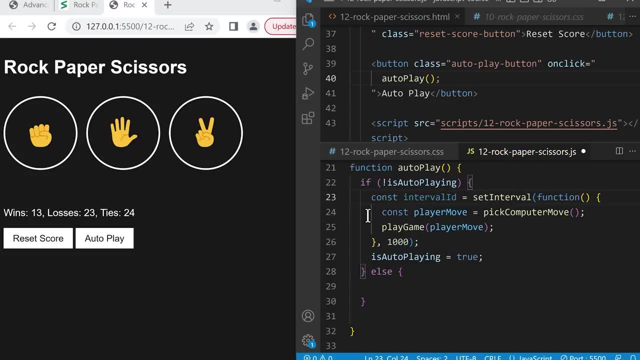 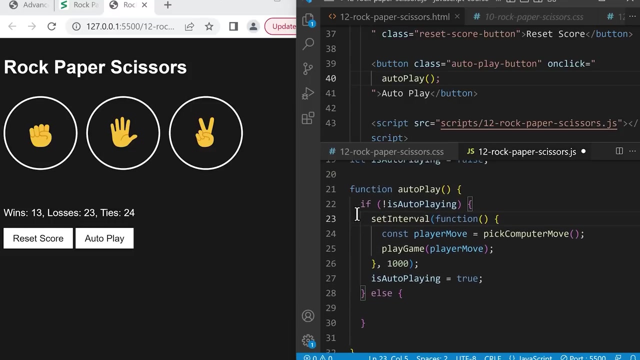 id to stop the interval. So at the front, let's add a different id. So in order to save the id from last time, we need to put this variable outside the function. So let's select this and remove it. and now, down here we're. 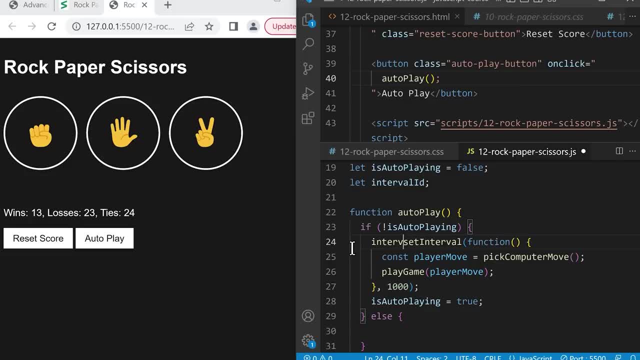 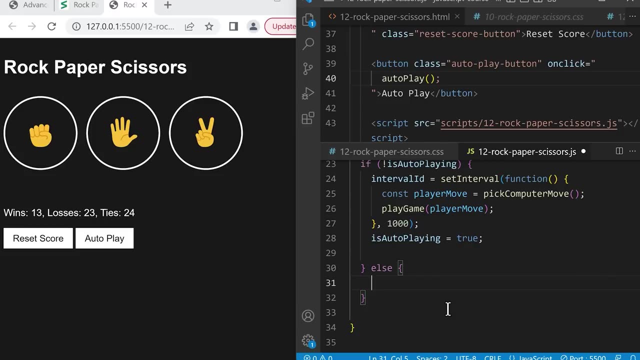 going to save the return value into this variable by typing interval- id equals set interval. and now at the bottom we're going to type clear capital, i, interval and brackets, and between the brackets we're going to give it an id that we want to stop. so we'll 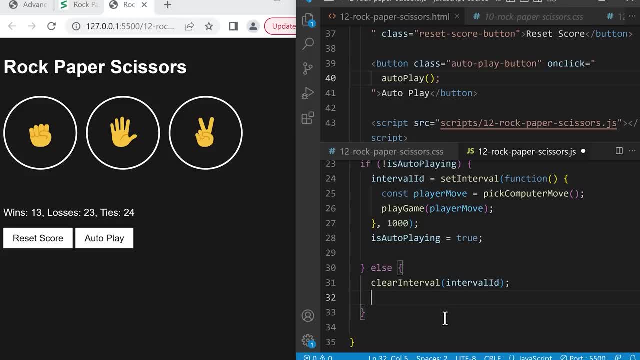 give it this interval id and stop it. so is auto playing equals false and save. so now, if we try out this button, it will start playing the game by itself every second and then call clear interval with this id. so now i'll clean up the code a little. 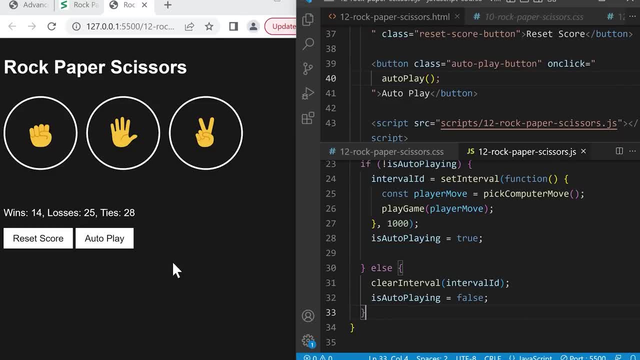 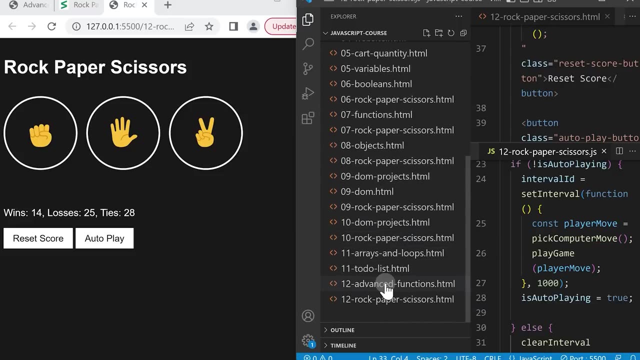 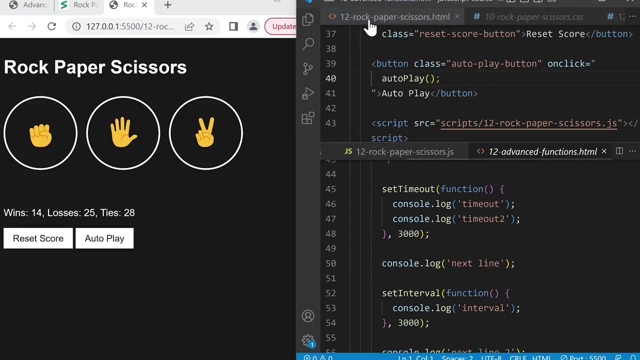 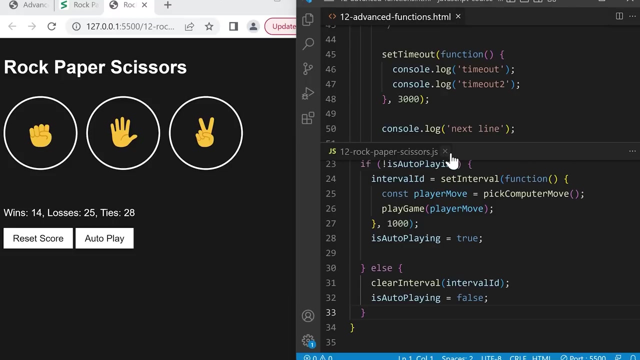 by removing this extra line and save. and now we're finished with this feature. so next let's go back to our advanced functions file and hide the files for now, and we're going to learn some more features of functions as values. so let's actually close the other. 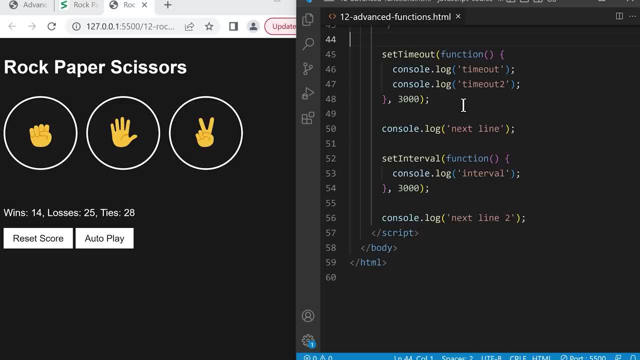 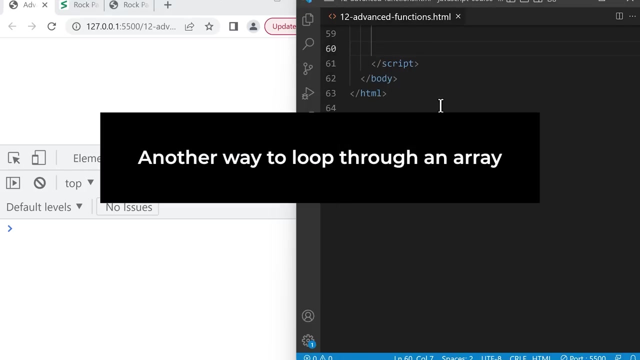 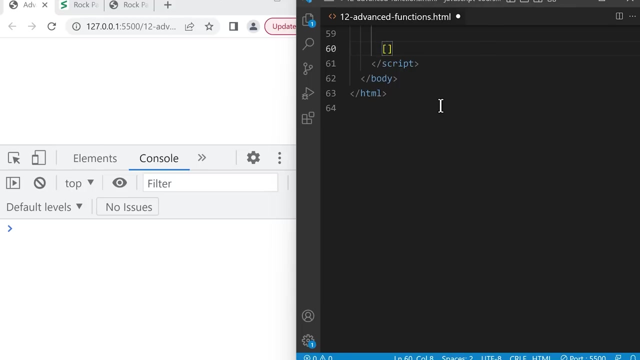 files that we opened. and first let's comment out the previous code with slash and save and let's open the tab for this file. so now we're going to learn another way to loop through an array. first let's create an array. we'll type square brackets. 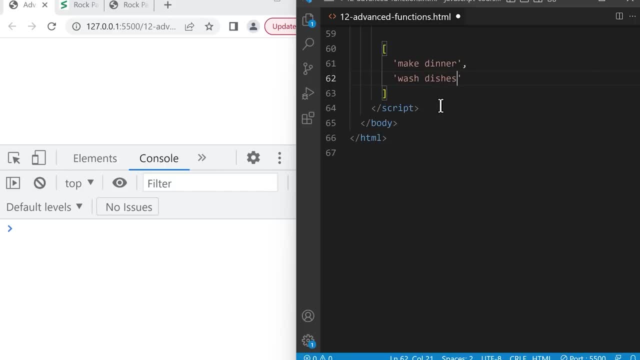 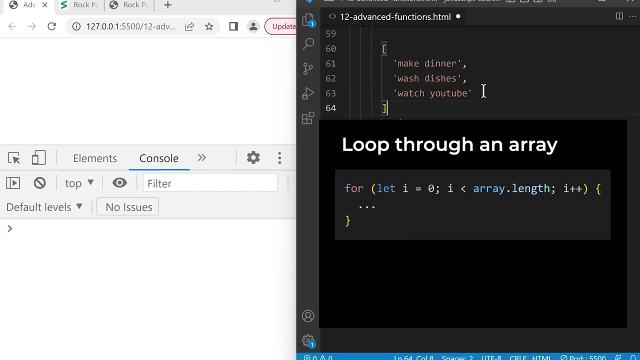 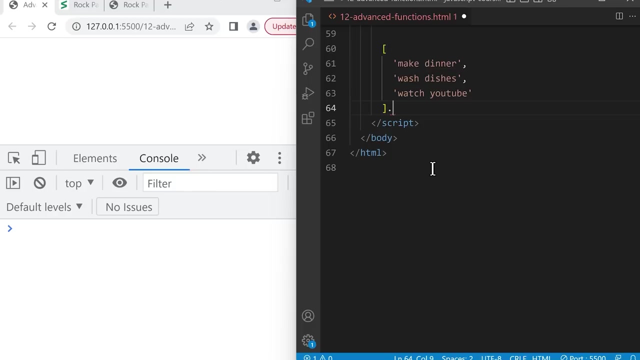 and inside the array we'll type dishes and another string watch youtube. so in the previous lesson we learned how to loop through an array using a for loop or a while loop. another way to loop through an array is to type for each and brackets. so this is the 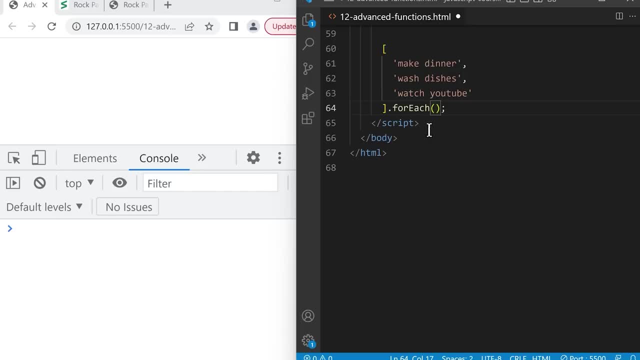 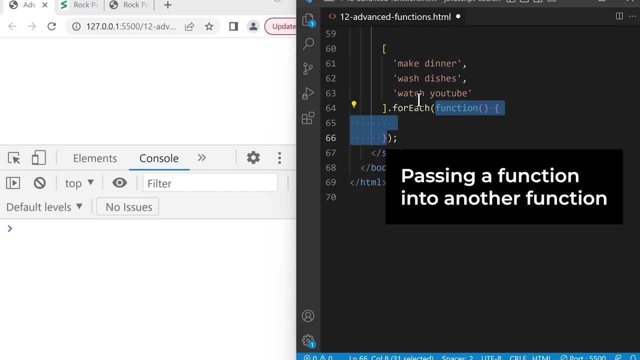 for each method, and it allows us to loop through this array. inside these brackets, we're going to give a function into another function. however, this function will be a little different. we're going to give it a parameter, so up here let's create a parameter called value. 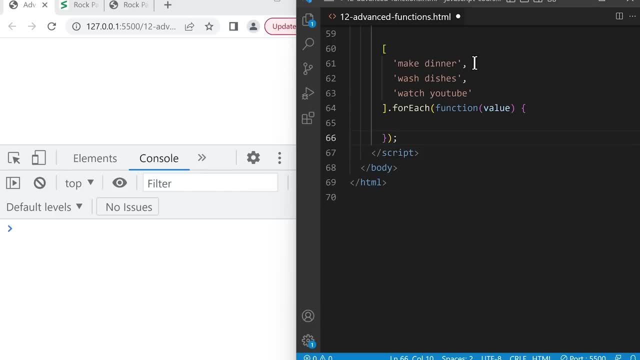 so what for each does is that it loops through the array and displays each value in the console. so let's console dot log value and save. so this will loop through the array and display each value in the console. so let's go into the parameter and run. 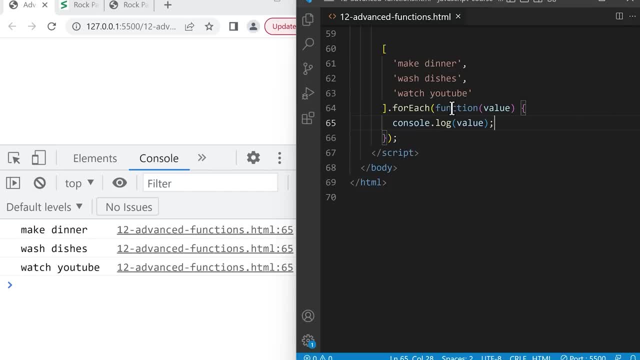 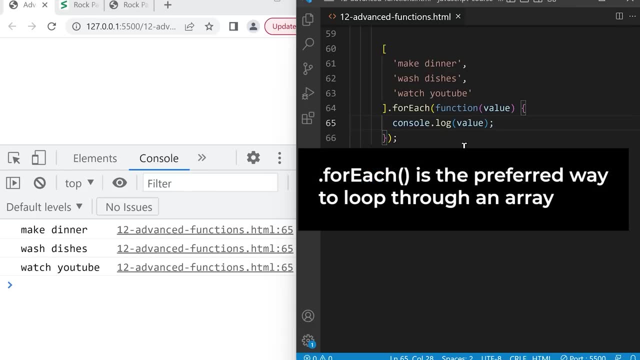 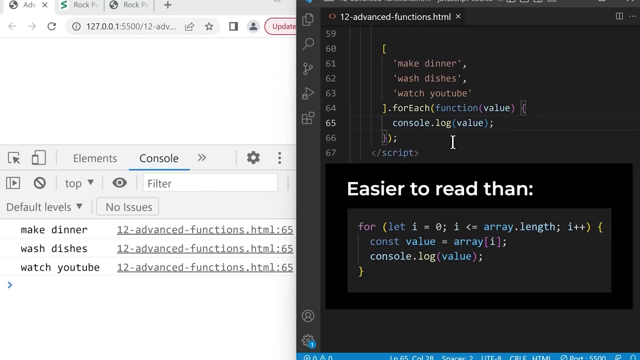 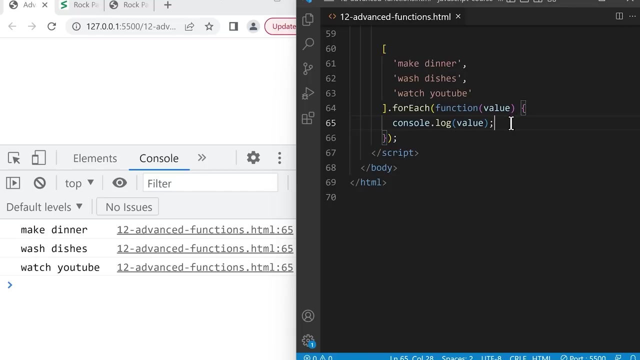 the function. then it will take the third value, save it in the parameter and run the function. so the for each method is actually the preferred way to use the parameter so we can type comma. and the second parameter is the index or the position of the value in the. 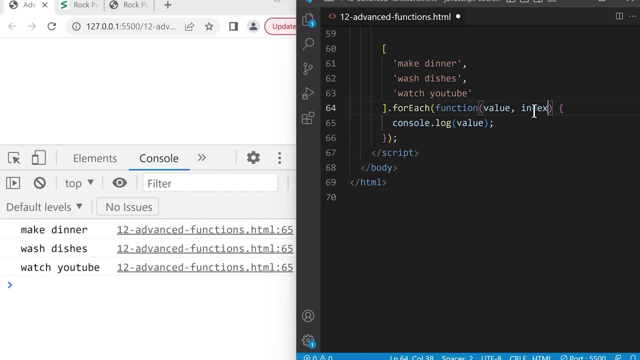 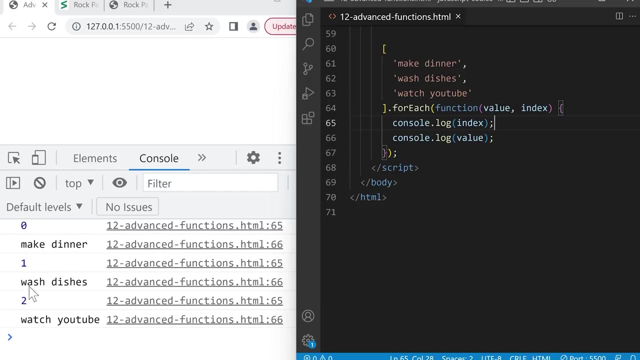 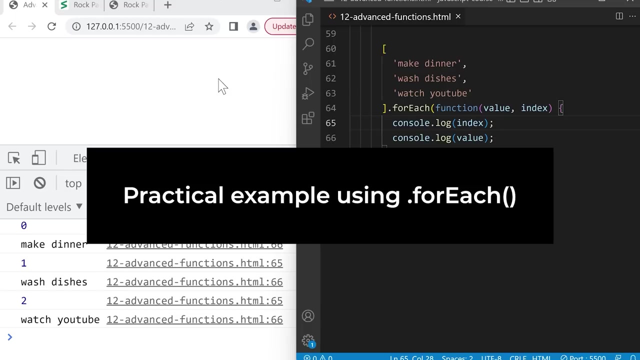 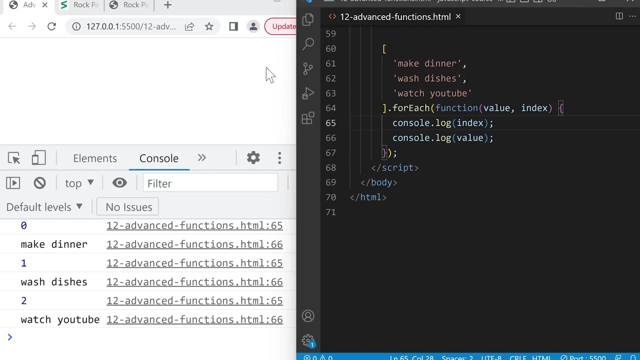 array. so for the first value index will be zero. for the second value index will be one third value. log the index and save, and this will also display the index of each value. all right, now let's do a practical example using the for each method we're. 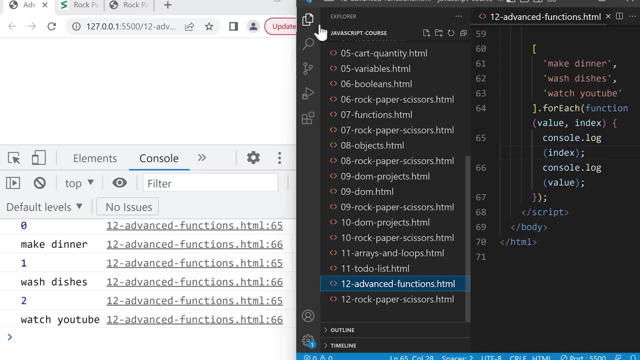 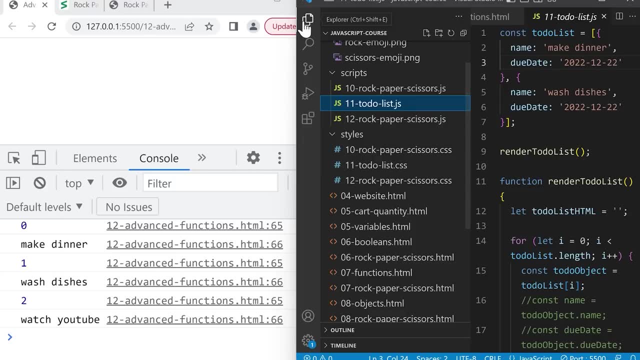 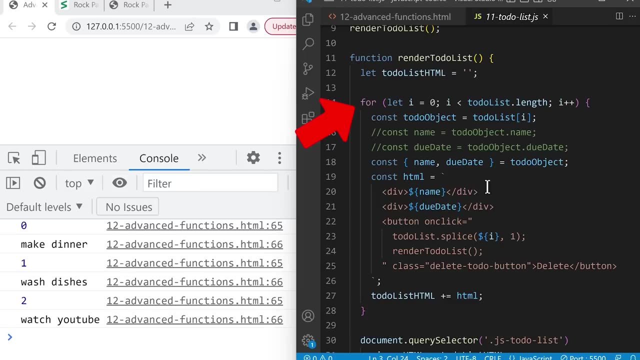 going to go back to the to-do list project and let's open 11 to-do list dot js. so in this code we used a for loop to display the to-do list on the page. we're going to switch this to using a for each method. 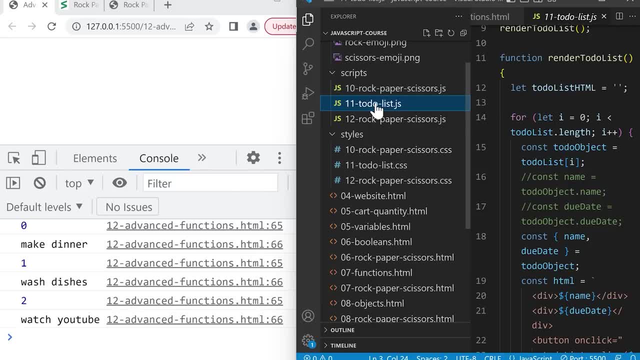 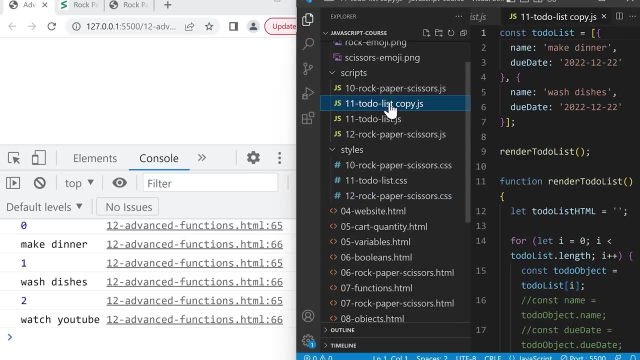 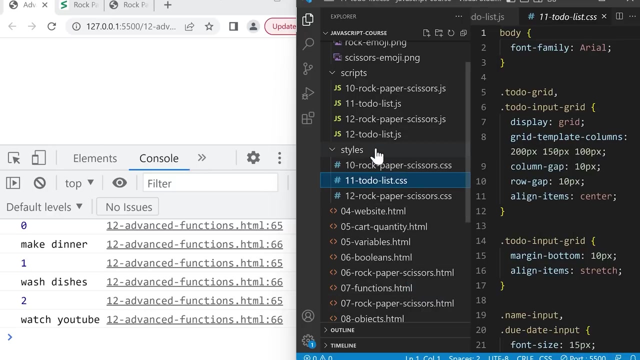 instead. so first let's actually make a copy of the script folder right click and paste, and now we'll rename this by right clicking rename, remove copy from the end and change the beginning to 12. copy of the css and html file for this project. so we'll 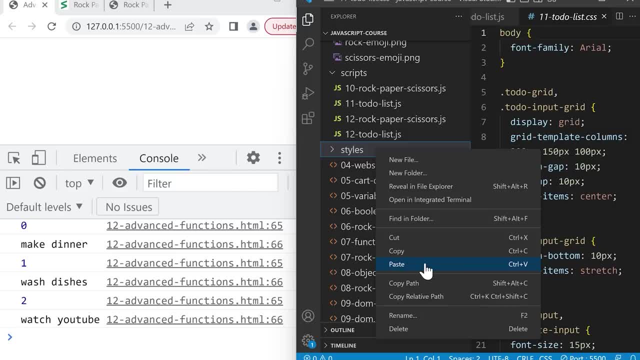 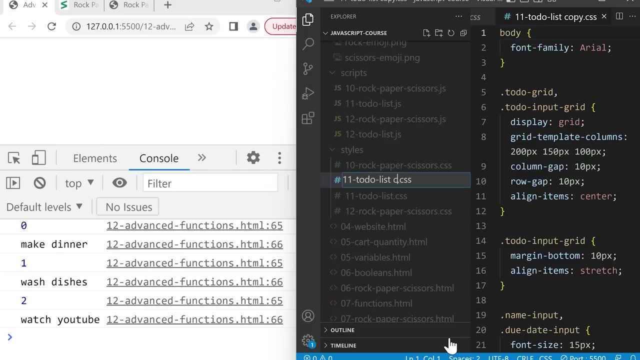 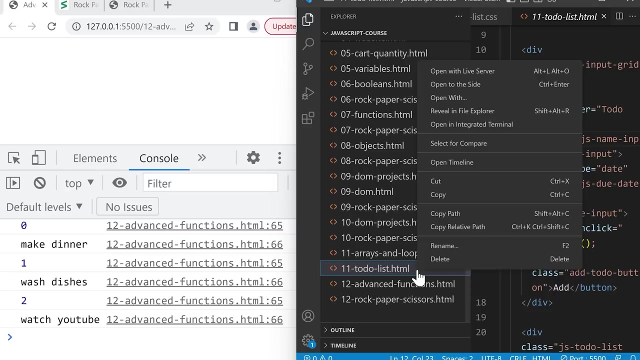 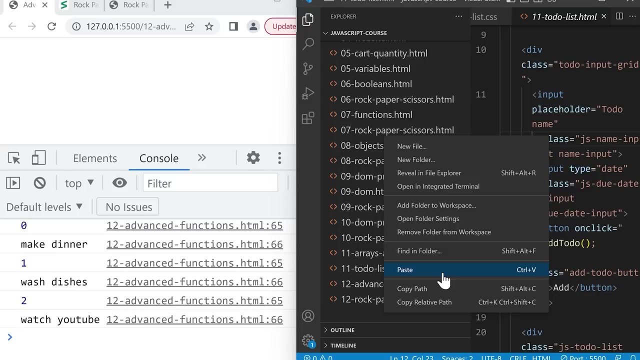 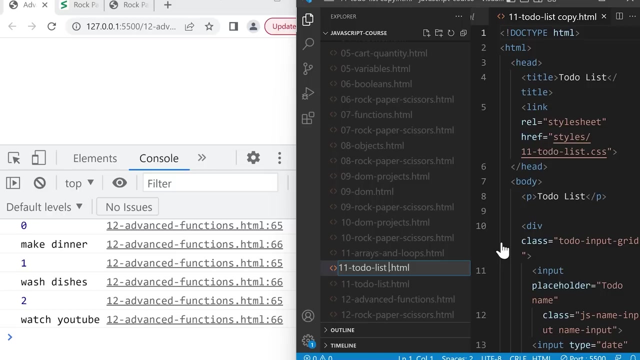 click this css file, right click copy. click the styles folder, right click and paste, right click remove. to list that html, right click copy and then down here, right click and paste, right click rename. remove copy at the end and at the beginning, change it to 12 and. 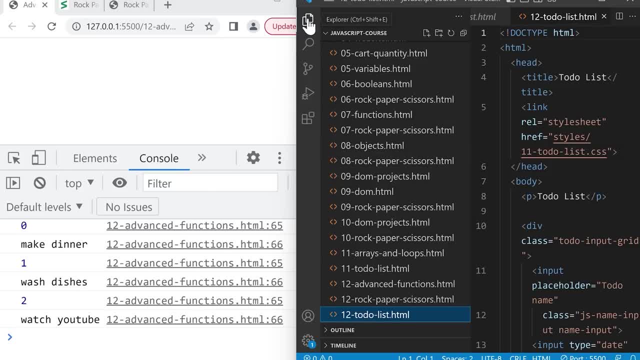 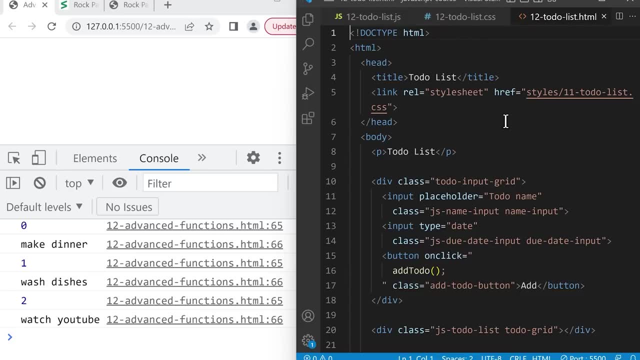 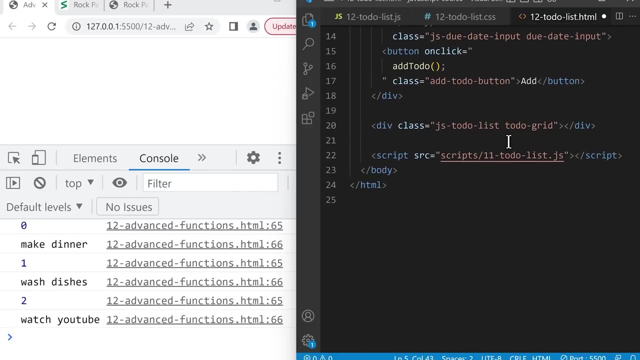 press enter and click. Now we can hide these files and we can close the lesson 11 files. And now here we're going to change the CSS file that we load to 12 to-do list And we'll scroll down and we'll also change the JavaScript file that we load to 12 to-do. 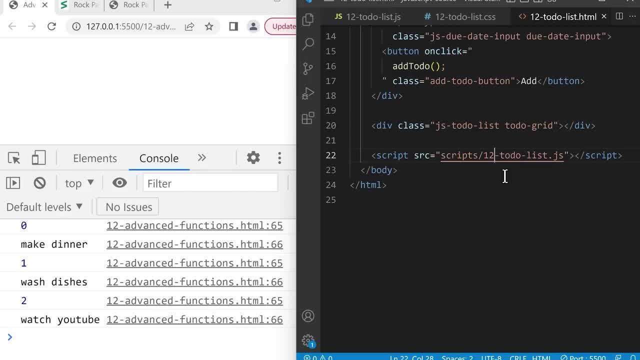 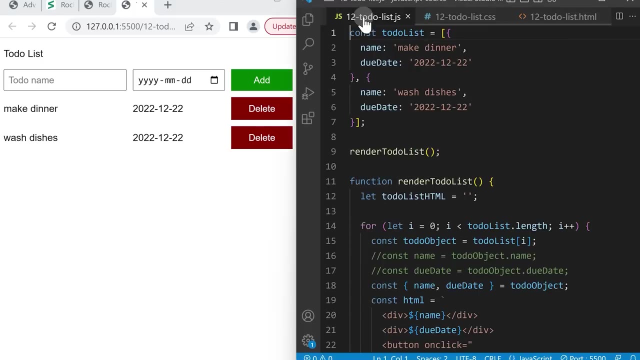 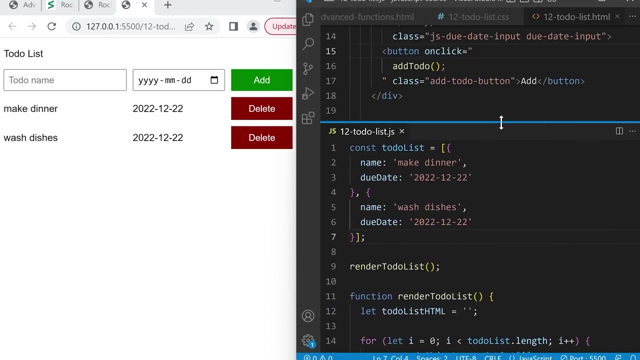 list. Now let's save and we'll open this in the browser by right-clicking: Open with Live Server. Okay, now let's go back to the JS file. So I'll take this file and drag it to the bottom and I'll rearrange the windows here. 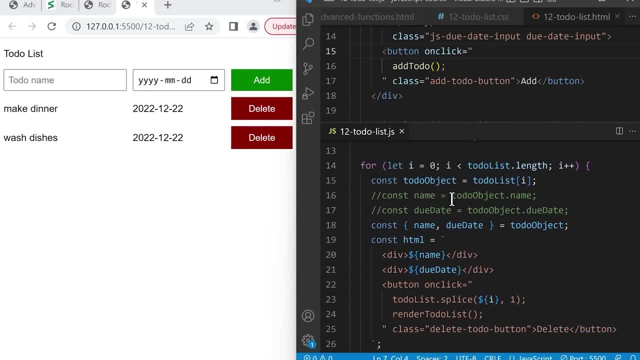 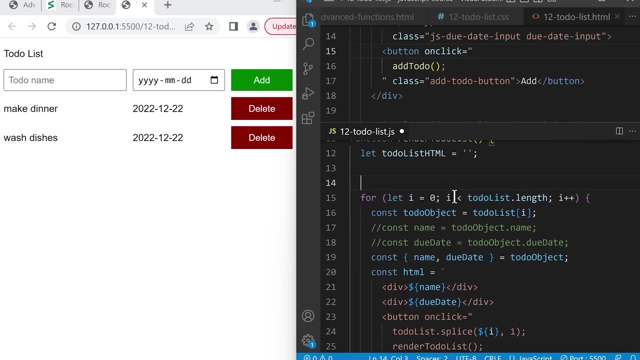 We're going to scroll down and we'll change this for loop to use a forEach method. Okay, So first let's type above this for loop and we'll type the array that we want to loop through, which is to-do list. 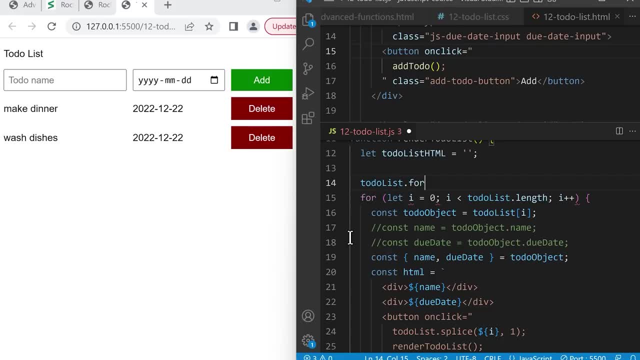 And we'll type, dot and use the forEach method and brackets Inside the brackets. we'll give it a function that we want to run for each to-do. So we'll type function brackets And curly brackets, And this function can have two parameters. 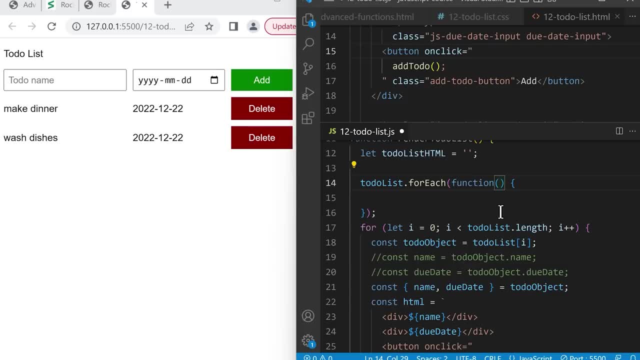 The first parameter will contain each value in the array, So we'll call it to-do object, We'll type a comma. and the second parameter contains each index in the array, So we'll just call it index. And now, inside this loop, 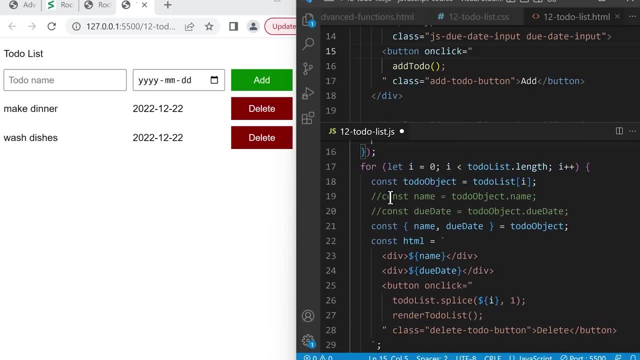 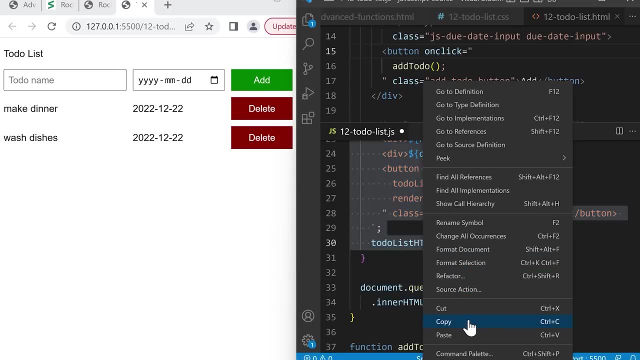 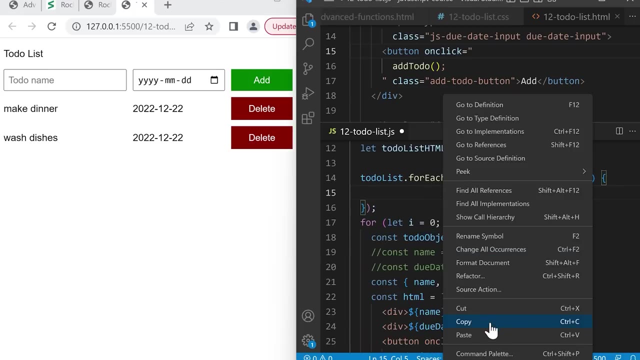 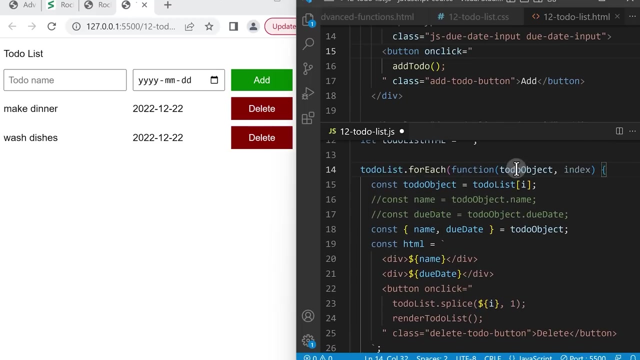 We basically want to do everything that we did here. So let's just make a copy of this code: right click, copy and then up here inside forEach right click and paste. So now, if we scroll up, we already have the to-do object up here. 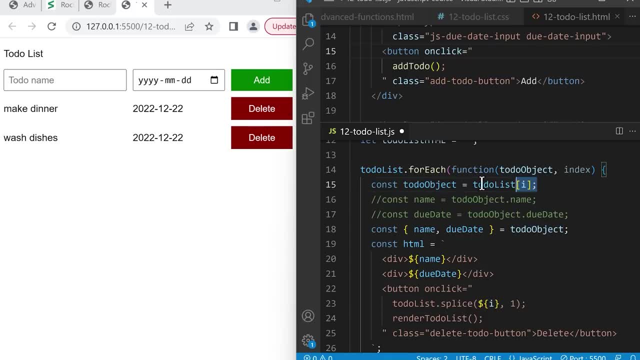 So we don't need to get it from the array like before. Okay, So we can remove this line, And let's also remove these comments. The other thing we have to change is that previously we were using i for the index, But now the index is called index. 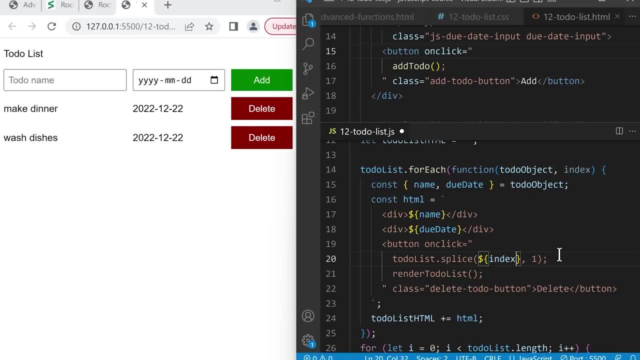 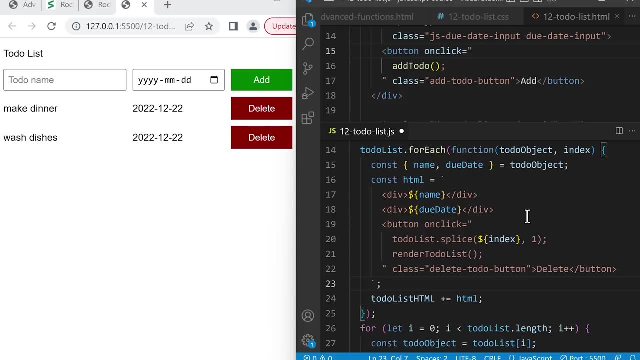 So we just change this to index. So that's how we use a forEach method instead of a for loop. So that's how we use a for each method instead of a for loop. So that's how we use a for each method instead of a for loop. 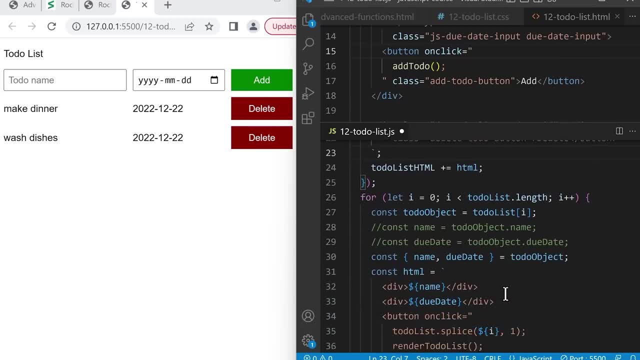 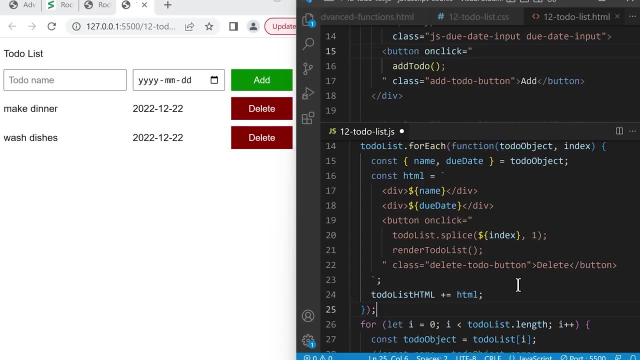 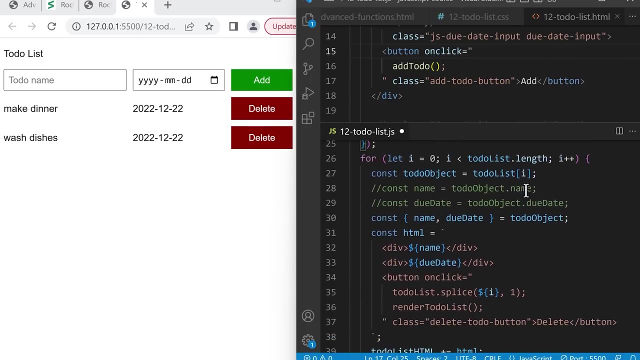 If we compare this code to the for loop that we had before, The for, each method is easier to read. So for the rest of this course, we're gonna prefer to use forEach instead of a for loop, So we're going to remove this for loop. 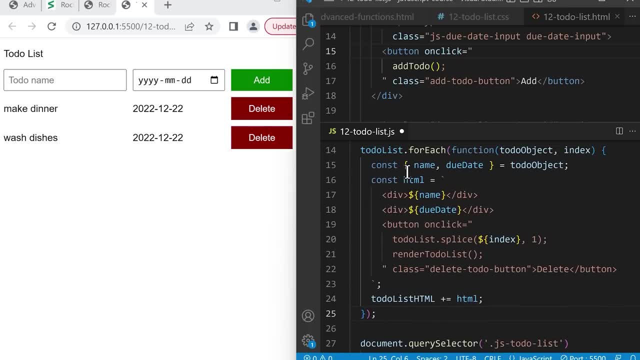 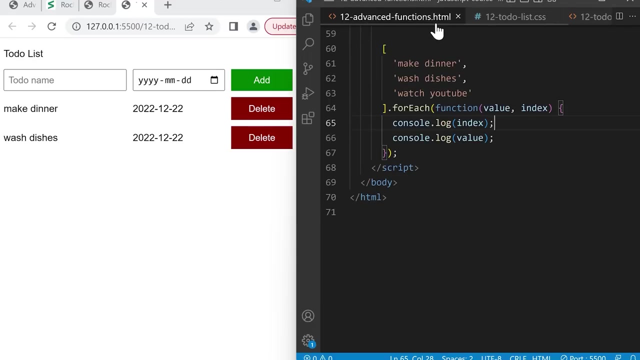 Let's scroll back up and save, And the project's still working. works. So that's a practical example of using the foreach method. Now let's go back and learn some more details about foreach. We'll close the JavaScript file for now and go back to advancedfunctionshtml and. 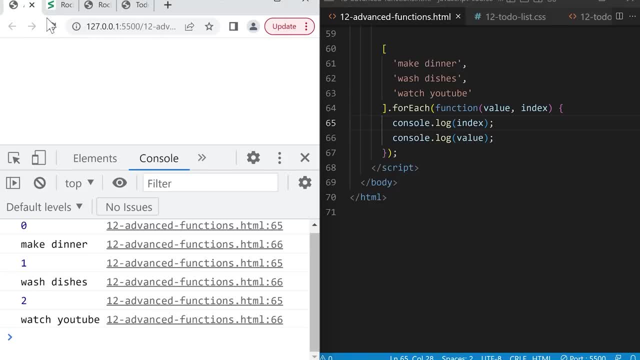 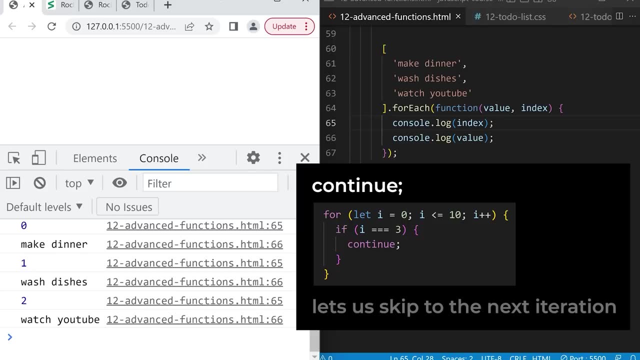 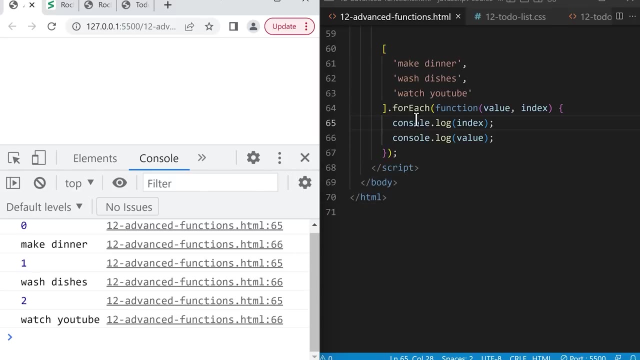 open the tab for this file. So in the previous lesson we learned a feature of loops called continue. Continue. lets us skip to the next iteration or the next run of the loop. Foreach methods don't have continue, but we can do the same thing with a return statement. 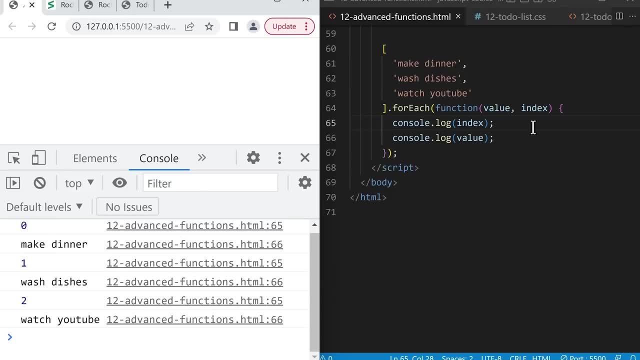 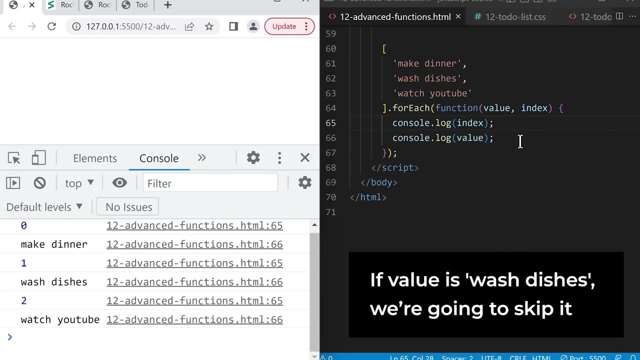 So let's say in this loop: we don't like washing dishes. If the value is wash dishes, we're gonna skip it and not display it in the console. So above we'll create an if statement And then inside the condition we'll check if value is equal to the string wash dishes. 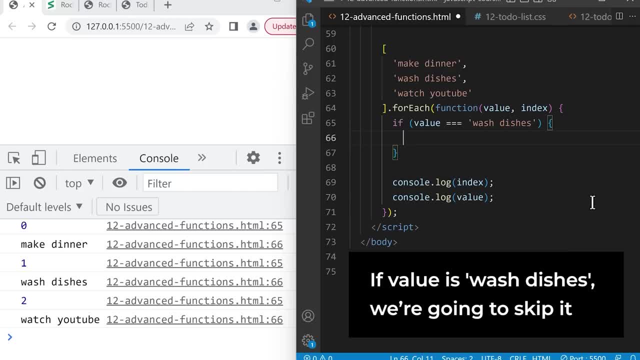 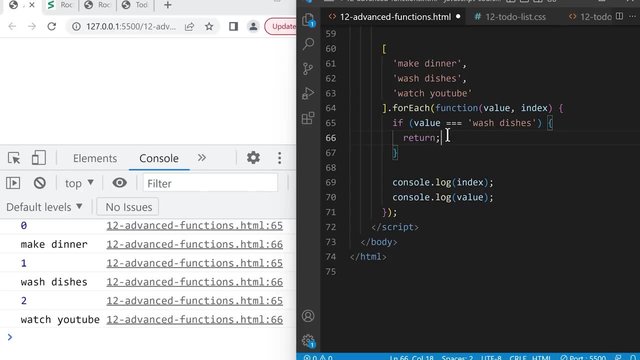 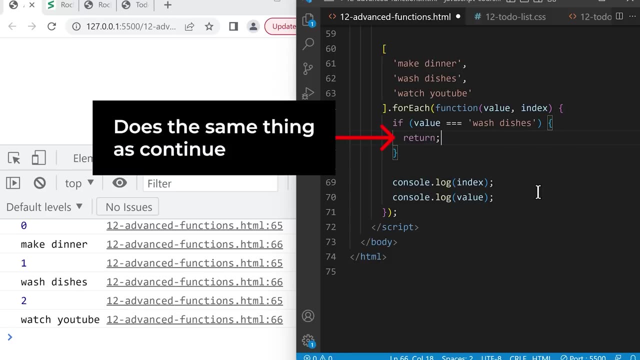 And then in the curly brackets, if it is equal, we'll return and semicolon. So this return statement will end this function early. Let's go back to the first iteration And it will go on to the next function. So it basically does the same thing as continue in a for loop. 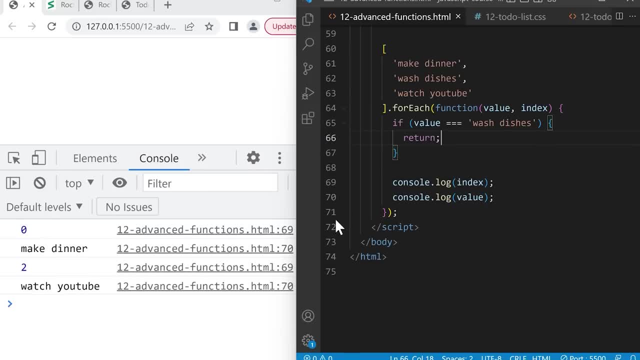 If we save, you'll notice that it skipped wash dishes. In the previous lesson we also learned a feature of loops called break. Break lets us exit a loop early. Unfortunately, there's not an easy way to break in a for each loop. 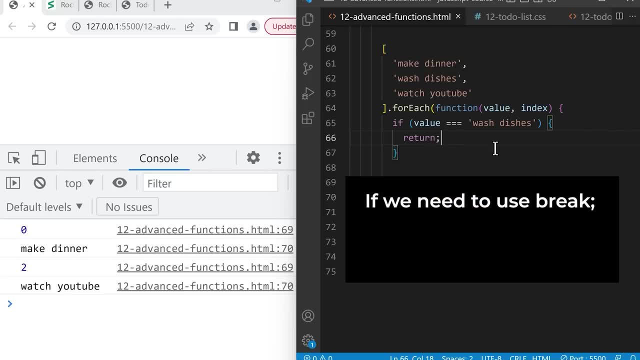 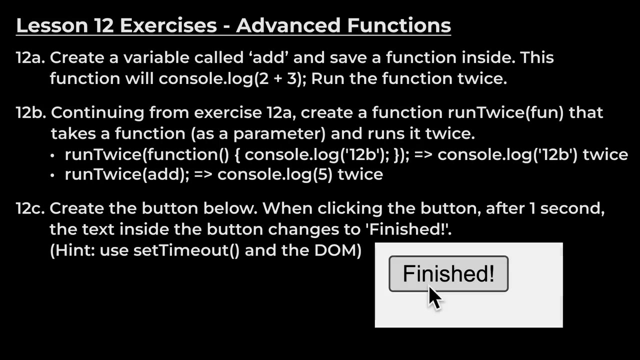 So if we need to use break to exit this loop early, then it's better to use a regular for loop. Let's take a break before continuing with the rest of this lesson. Here are some exercises you can do on your own to practice what we learned so far. 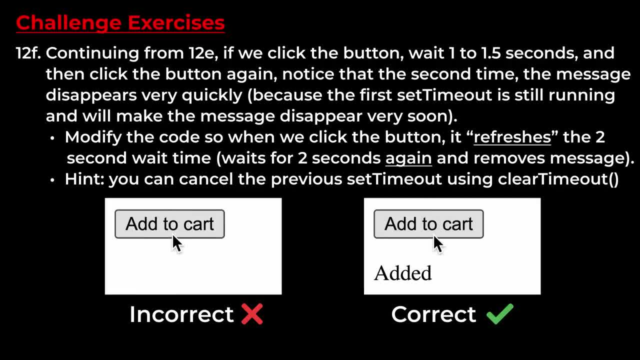 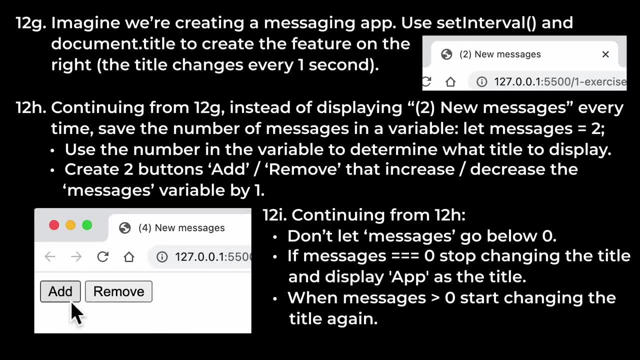 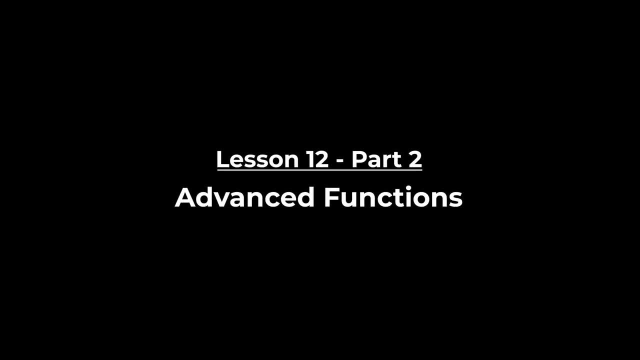 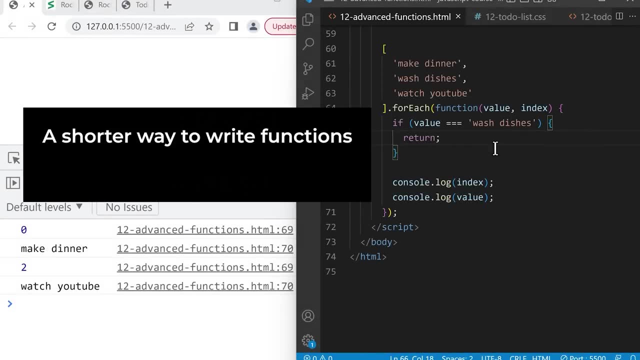 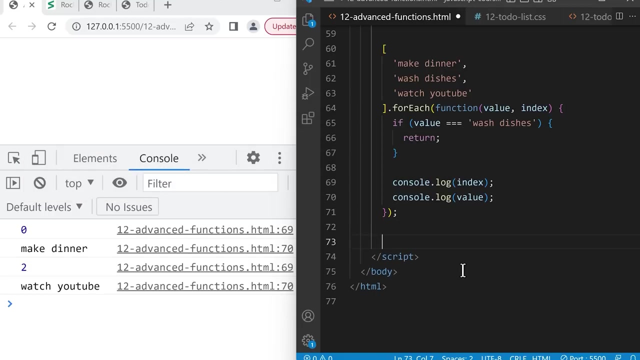 So next we're going to move on and learn a shorter way to write functions called arrow functions. So let's go to the bottom of this code, We'll create some new lines And let's create a variable const And we'll name the variable arrow function. 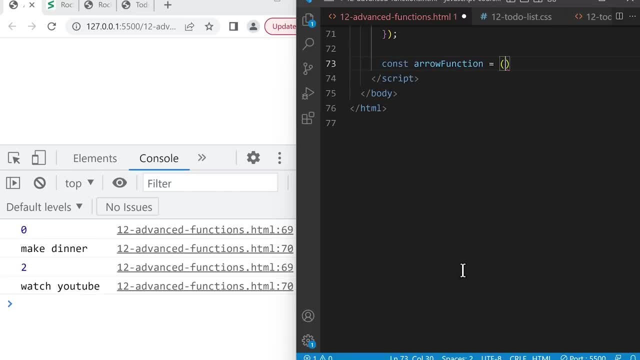 And we'll make it equal to brackets, equal greater than or an arrow, and then curly brackets. Inside the curly brackets we'll type some code, Console log brackets and the string hello, And we'll put a semicolon at the end. 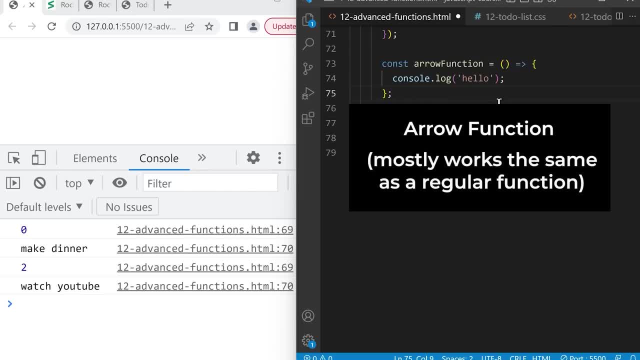 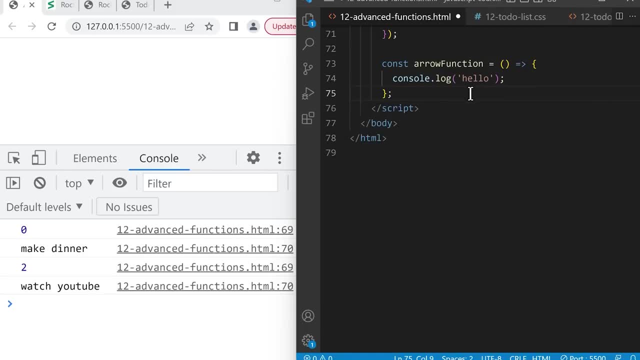 So this is an arrow function. It works the same way as a regular function. For example, we can call this arrow function by typing the variable name: arrow function and brackets. If we save this line of code, we'll run the code inside this arrow function and display hello. 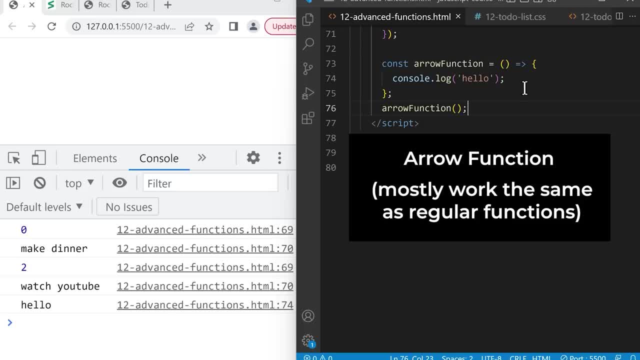 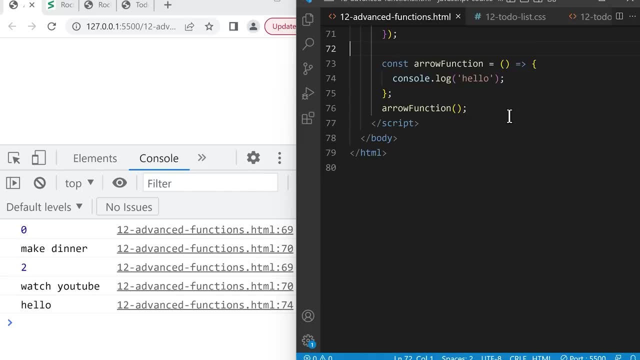 So arrow functions mostly work the same way as regular functions. So to compare them, let's actually type above this code: We'll create some new lines and type: const: regular function Equals the word function brackets and curly brackets. Console log string: hello. 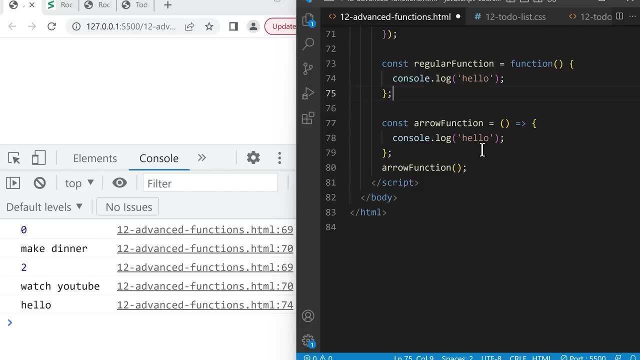 So these two syntaxes do the same thing. The difference is that, instead of using the word function, an arrow function just uses an arrow. Now, parameters work. They work the same way. in an arrow function, We just type the parameter between these round brackets. 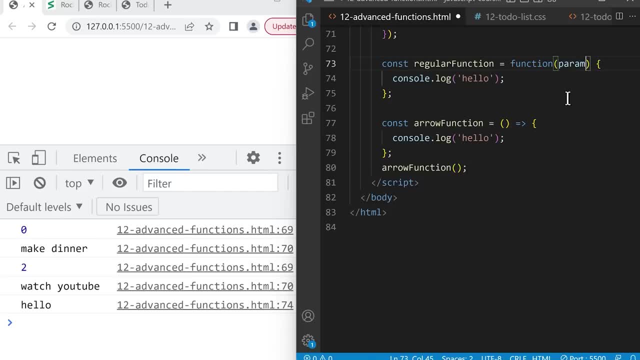 So here let's type param, and here as well, If we want multiple parameters. it also works the same way. Up here we can type comma param2.. And down here comma param2.. And finally, return statements also work the same way. 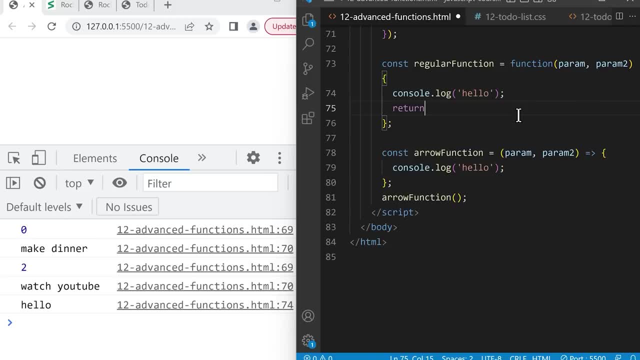 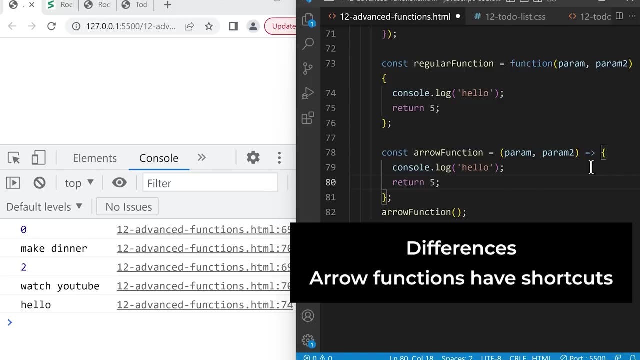 So in this function we can return 5.. And in the arrow function we can also return 5.. So now let's learn some differences between these two. Arrow functions have a few shortcuts that regular functions don't have, For example, at the bottom. 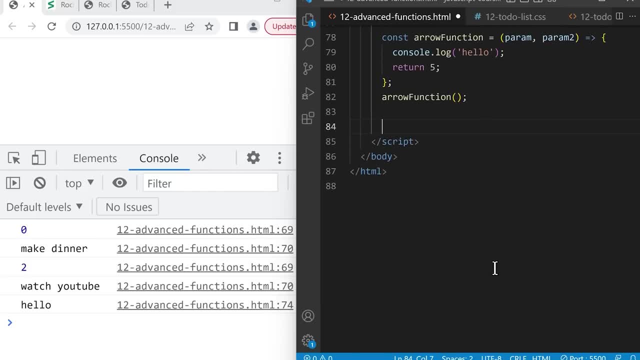 let's create an arrow function using const, and we'll name it 1param And make it equal to an arrow function. Brackets, arrow and curly brackets. Now, in this arrow function, we're going to give it one parameter: param. 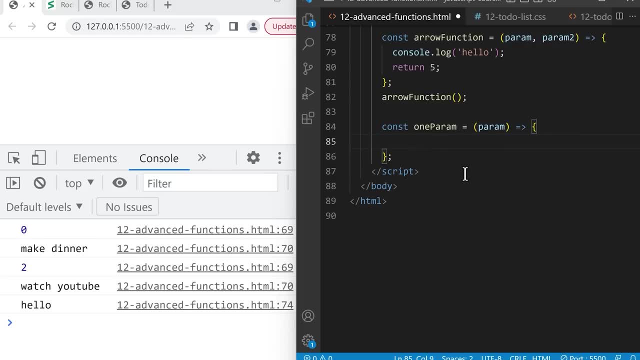 And inside the function we'll console dot log, param plus 1.. So when an arrow function only has one parameter, these round brackets are optional. So we can actually remove them If we do 1param brackets 2.. 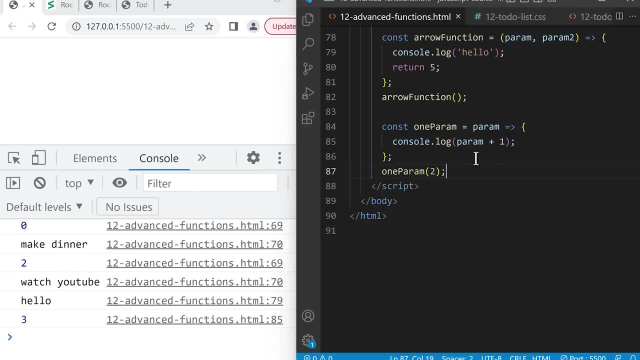 If we save, it will display 2 plus 1, which is 3.. So now let's learn another shortcut. We'll create some new lines And type: const one line And make it equal to an arrow, function brackets, arrow and curly brackets. 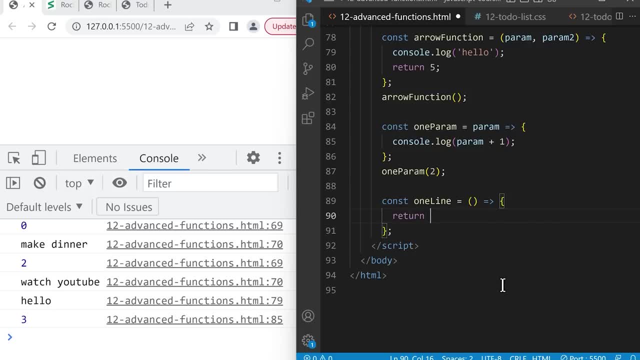 And inside we'll return 2, plus 3.. So in an arrow function only layouts are optional, and we can also have few brackets. let me name them, And here we'll. healthy little things like this only has one line. like this, we can actually put it on the same line as the arrow. And now that 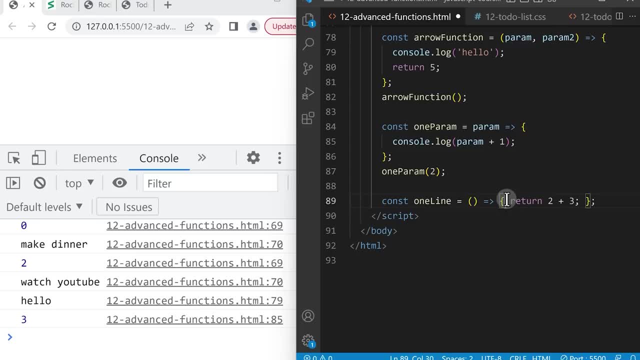 everything's on the same line. the curly brackets are actually optional So we can remove them, and we can also remove the return statement. So this is a one line arrow function. If we just have an arrow, it will automatically return the result on the right. So at the bottom we can console dot. 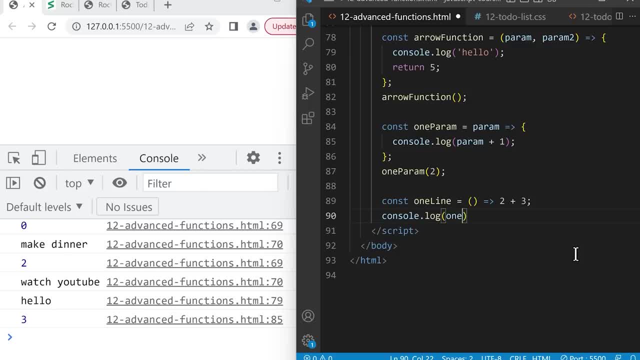 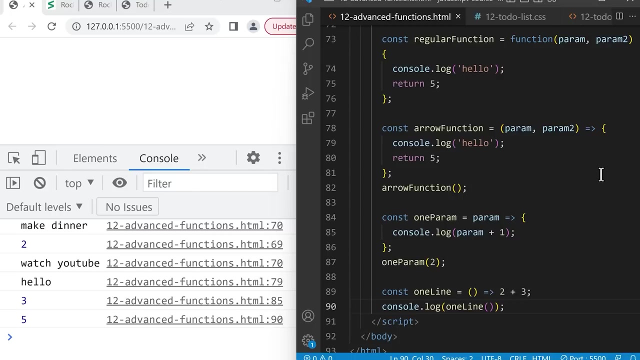 log and call the one line function with brackets. If we save, this function will return two plus three and it will display five in the console. So that's arrow functions. It's a shorter way of writing a regular function And it has a few shortcuts. For now, let's get some. 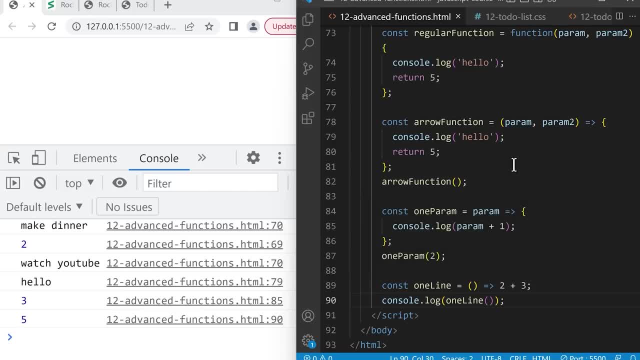 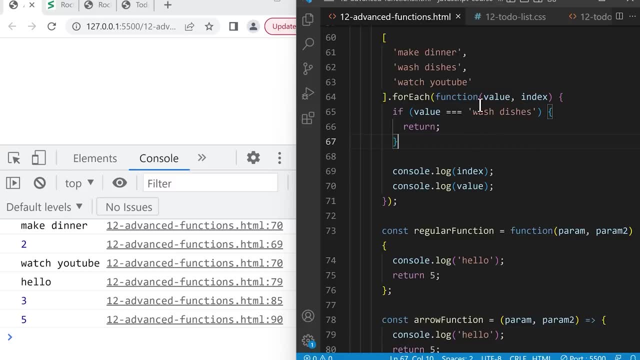 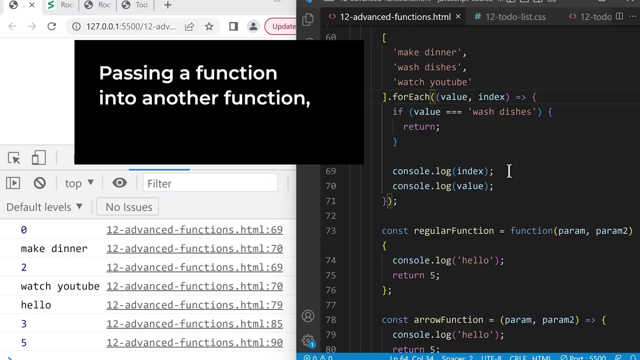 practice using arrow functions. So let's scroll up in this code to the for each method. So let's use an arrow function here instead. we just have to remove the word function And after the round equals greater than. If we save, the loop still works. So when we're passing a function into, 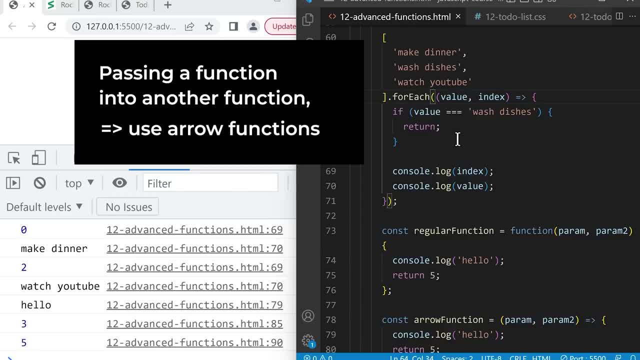 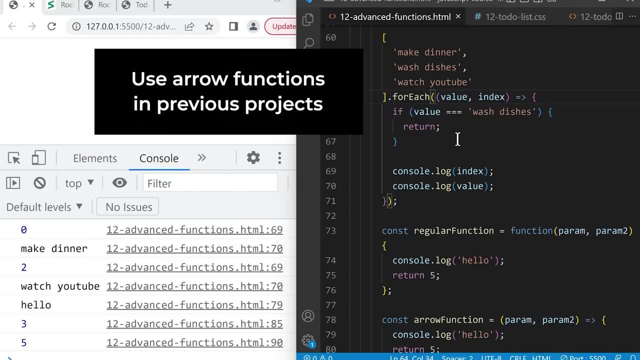 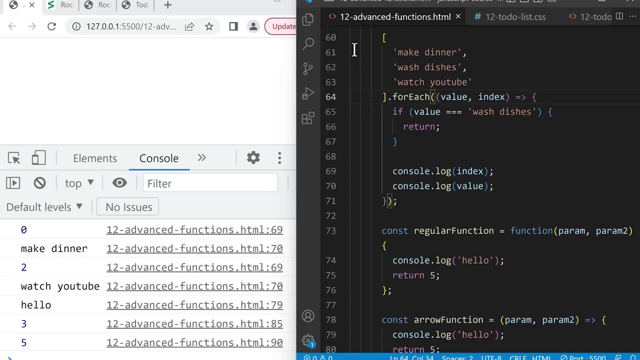 another function. like for each, it's recommended to use arrow functions because it makes our code easier to read. So now let's use arrow functions in some of our previous projects. We'll start with the rock paper scissors game. Let's open our files by clicking here. 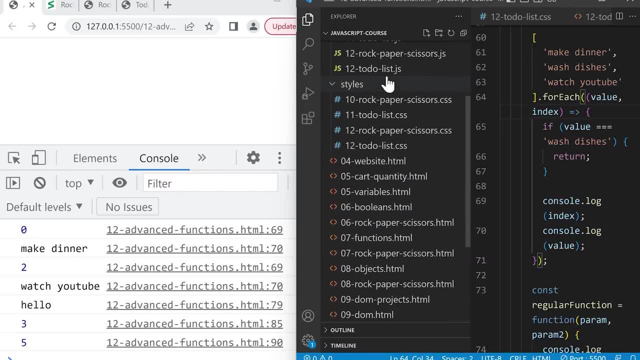 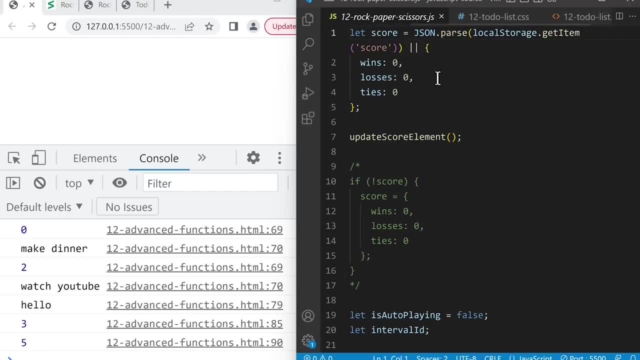 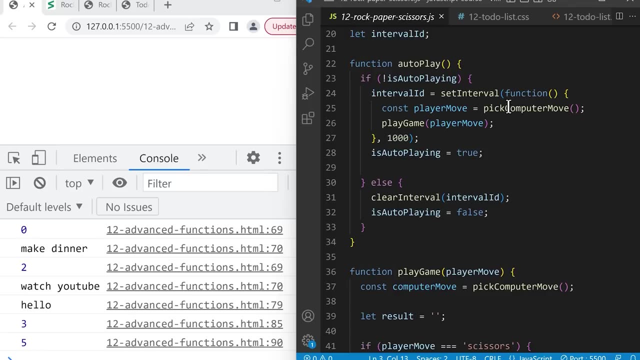 And we'll find the 12 rock paper scissors, dot j s file, And then inside this file we're going to scroll down to the autoplay function. So here we're passing a function into another function, So it's recommended to use an arrow function. Let's remove the word function. 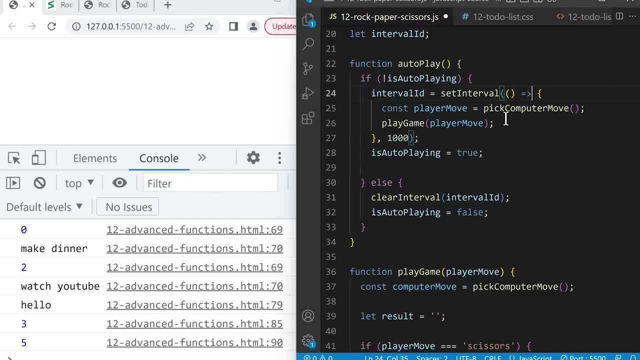 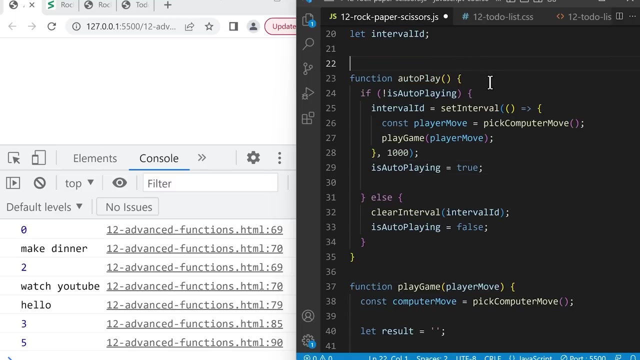 And add an arrow. So now this code is a little easier to read. Now what about this function up here, function autoplay. Should we also switch this to an arrow function? So this situation is more personal preference. So, above this, let's actually create an arrow function version of this const auto play. 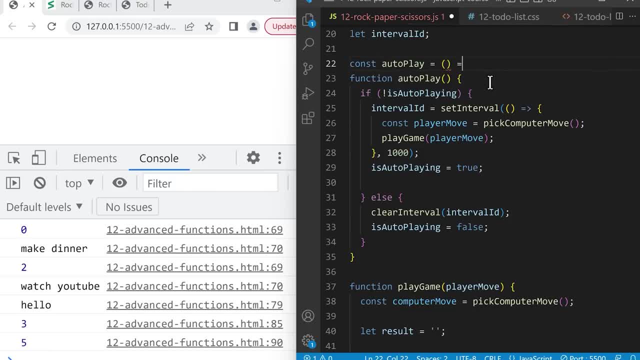 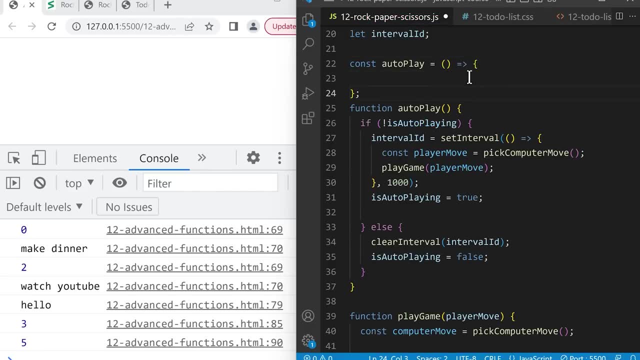 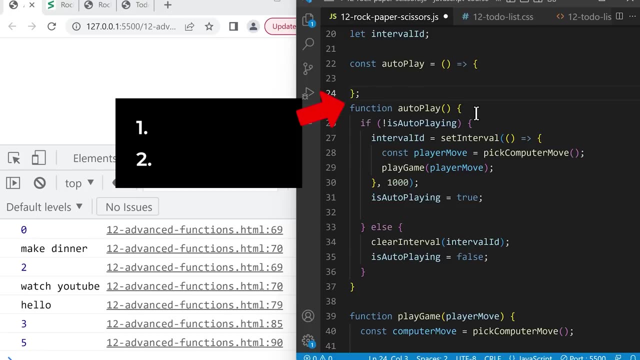 equals brackets and arrow and curly brackets. So even though we could create an arrow function version of this, I actually prefer the regular function syntax here for two reasons. Number one, I think this is easier to read than this. And number two, this function syntax enables hoisting, which means we 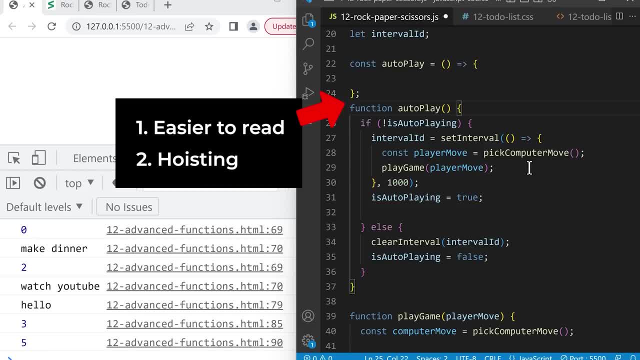 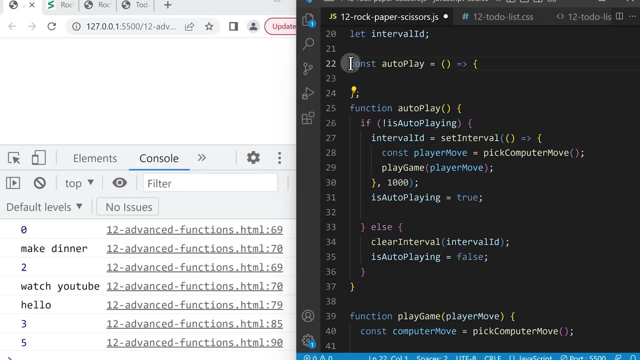 call this function before we create it and we don't have to worry about which order we write the code. so for these reasons, i actually prefer this situation: to use a regular function syntax and not an arrow function. so we'll comment out the arrow function using double slash. 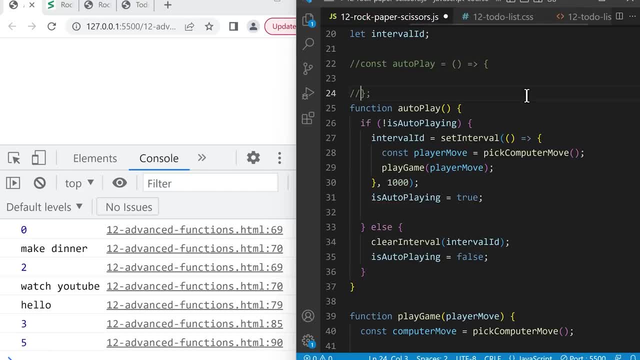 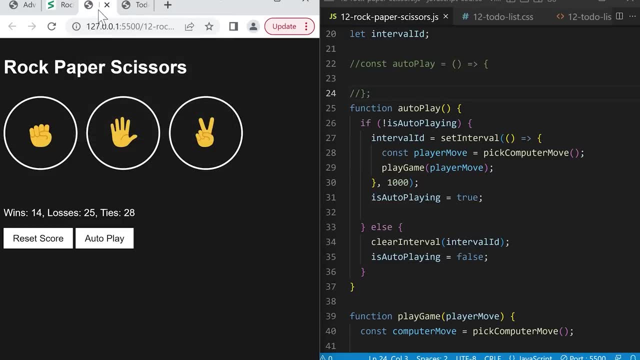 and double slash. now let's save and let's open the tab for this project and we'll give it a try. so click autoplay, and this still works after replacing with an arrow function. next let's go to the to-do list project and switch to arrow functions. so we'll go to our code editor. 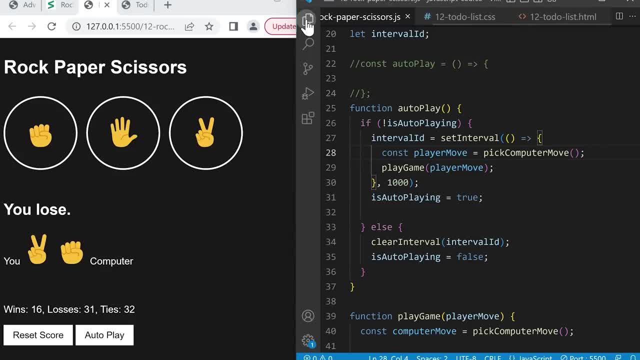 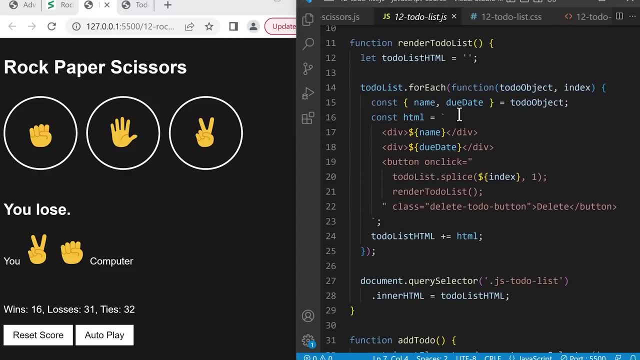 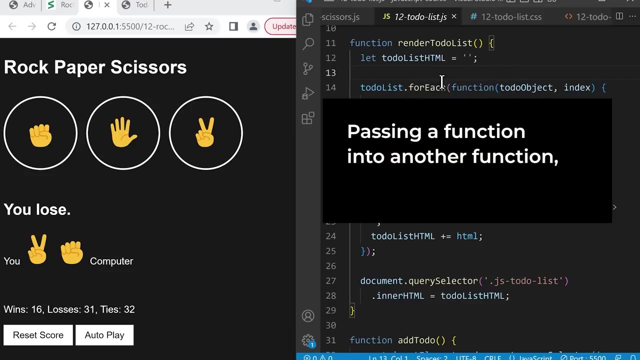 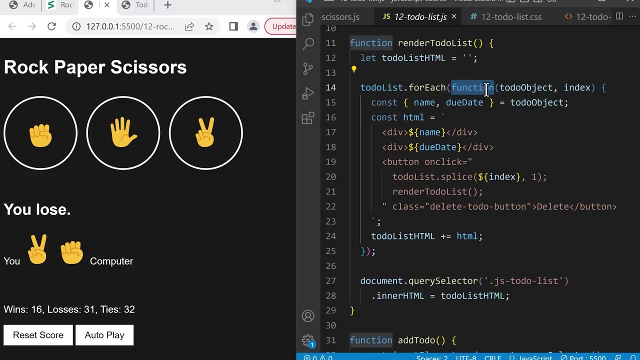 and find the to-do list project which is here, and let's scroll down. so inside render to-do list we're using for each and we're passing this function into another function, so it's recommended to use an arrow function here. so we'll remove the word function and after the brackets: 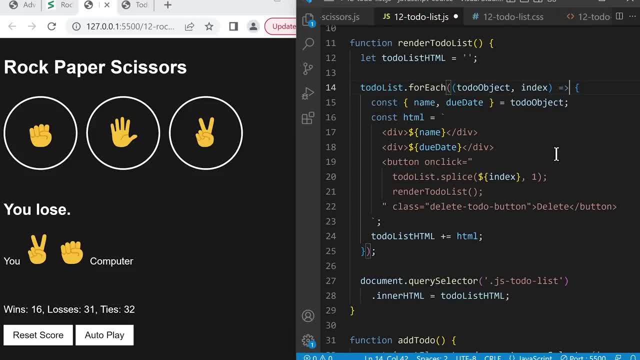 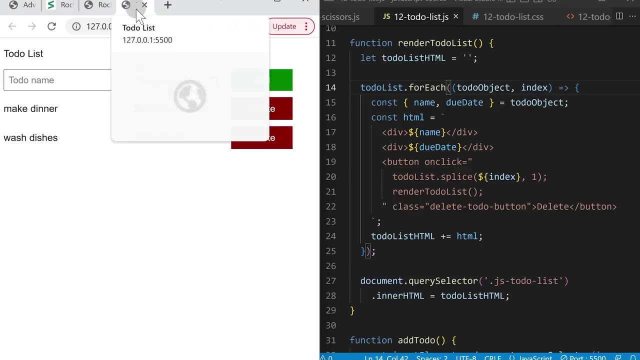 we'll add an arrow and again i'll leave this function- syntax- as a regular function, because it's easier to read and enables hoisting. so let's save and go back to our to-do list, and everything still works. next let's go back to 12 advanced functions: dot html. 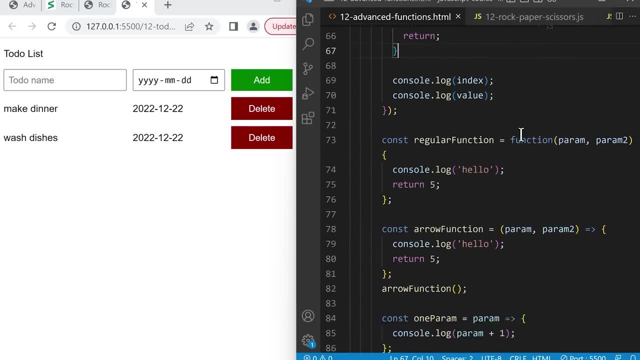 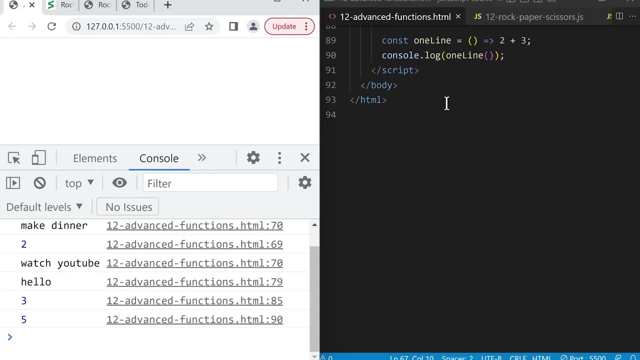 and we'll scroll to the bottom and we'll open the tab for this file and we'll review another place we could use arrow functions, which is inside an object. so at the bottom here let's create a new object. const object2 equals object, and then inside the object, let's create a new object. 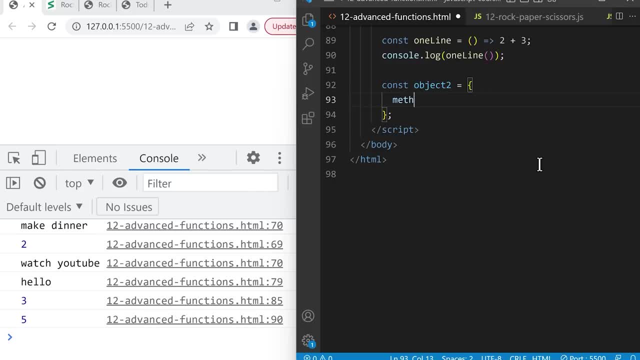 Inside let's type the property method, colon and an arrow function: brackets, arrow and curly brackets. So even though we could save an arrow function inside an object like this, objects already have a shortcut for functions, So at the bottom we could just type method, brackets and curly brackets. 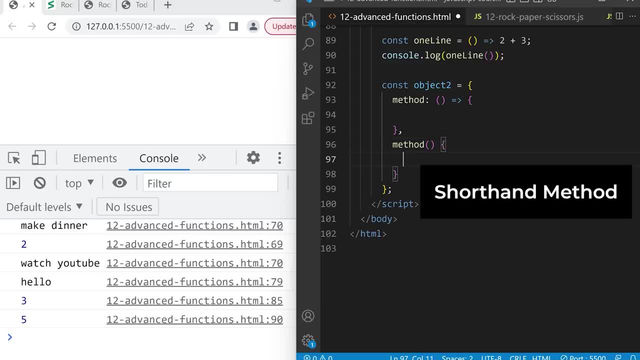 So this syntax is called the shorthand method syntax. So this shorthand method syntax is actually easier to read than an arrow function. So when saving a function in an object, it's actually recommended to use this syntax instead. There's also another difference Between regular functions and arrow functions, but we'll learn about it later in this course. 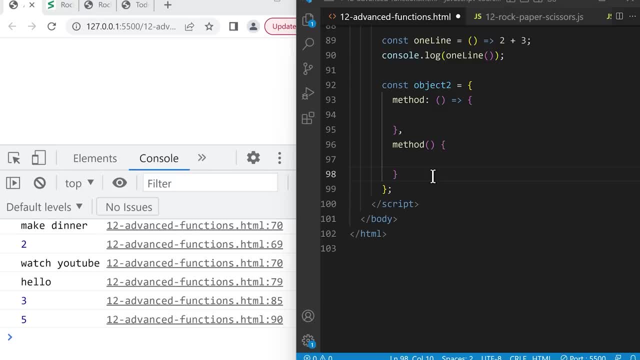 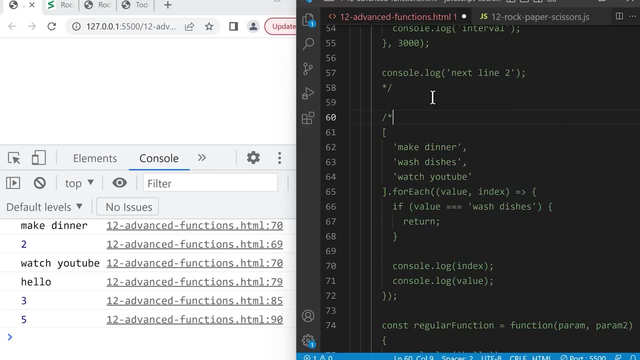 because it's a more advanced feature. Now let's move on and we're going to learn another improvement we can make to our projects. So let's comment out this code. We'll scroll up and type slash, star and at the bottom, star, slash. 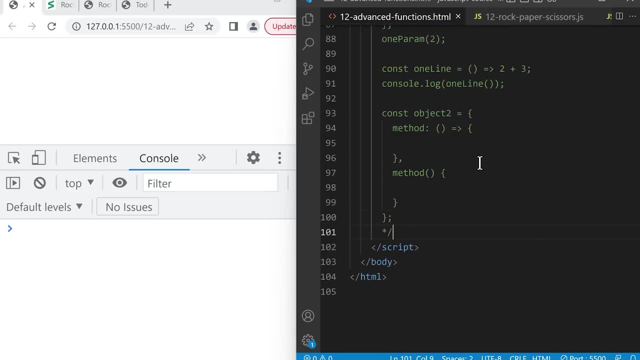 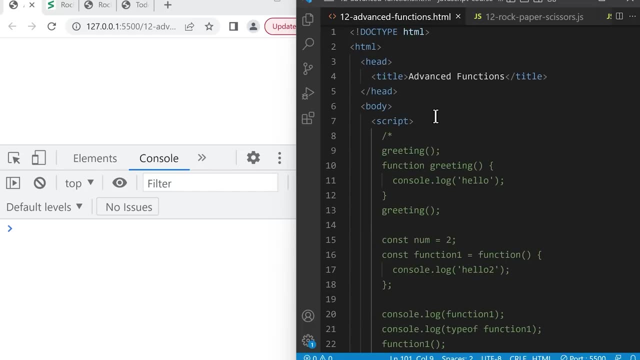 And save. And next we're actually going to scroll up to the very top of this file And we're going to create a button on the page. So inside the body we'll type less than, button, greater than, And inside the button we'll have the text click. 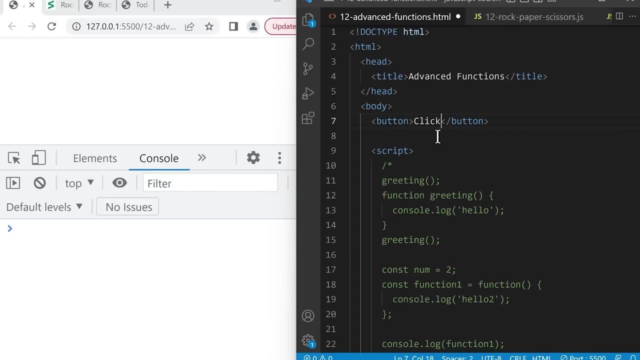 Now let's say that we want to run some JavaScript code Click When we click this button. So here we can type on click equals double quotes and write some JavaScript inside this double quotes. Now we're going to learn a better way of doing this, called add event listener. 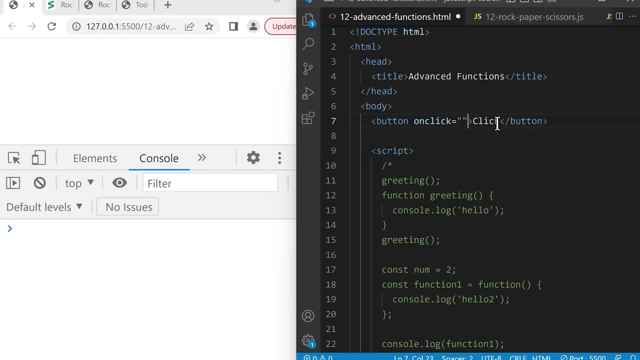 To use: add event listener. first, we're going to get this button and put it into our JavaScript using document dot query selector Click. Let's add a class to this button so we can select it and we'll set it to js dash button. 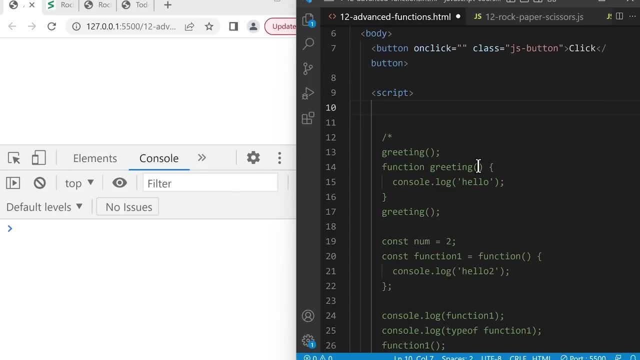 And now, inside the script element, we're going to use document dot query selector brackets and the string dot js dash button And we're going to give it an element. And we're going to use a class element And we're going to add this class up to our document. 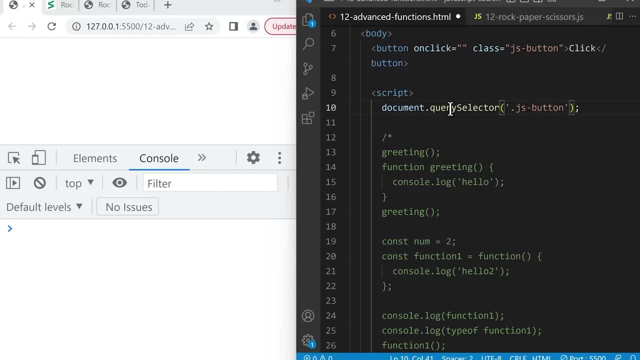 And we're going to give it a name And we're going to set it to j s dash button. So now let's save this button in a variable so we can use it later. At the front we'll type const button. element equals this result. 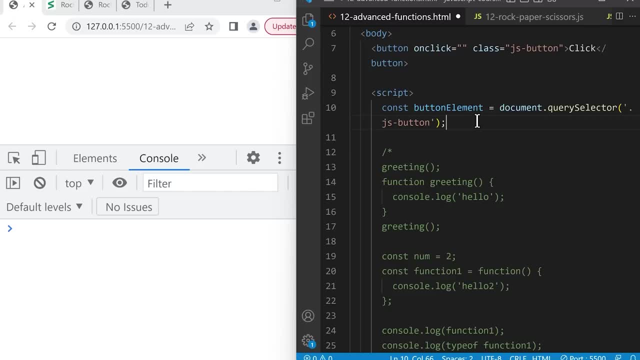 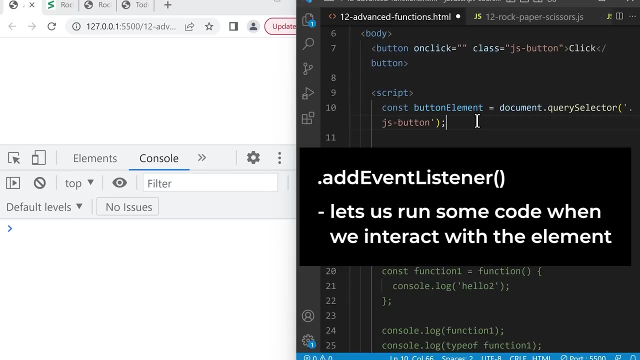 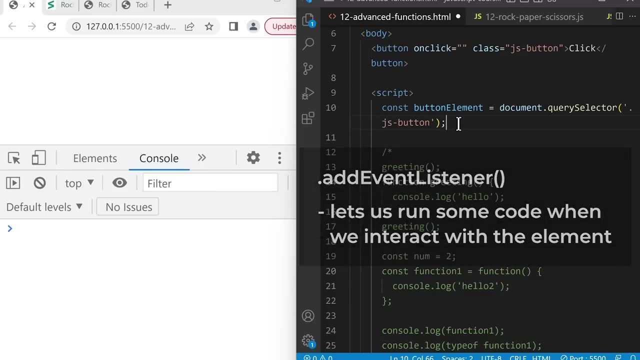 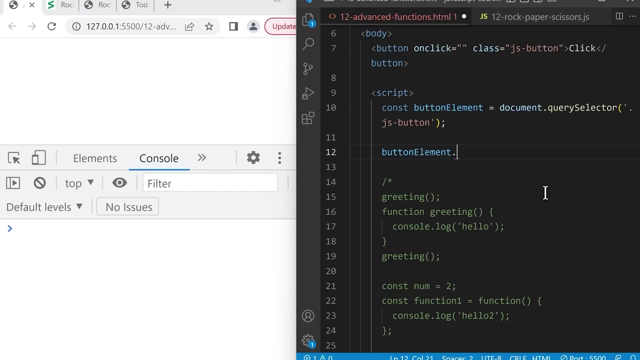 Now every HTML element has a method called addEventListener. addEventListener lets us run some code when we interact with the element, So it sort of does the same thing as onClick. So at the bottom let's type button element dot. add capital E, event capital, L, listener and brackets. 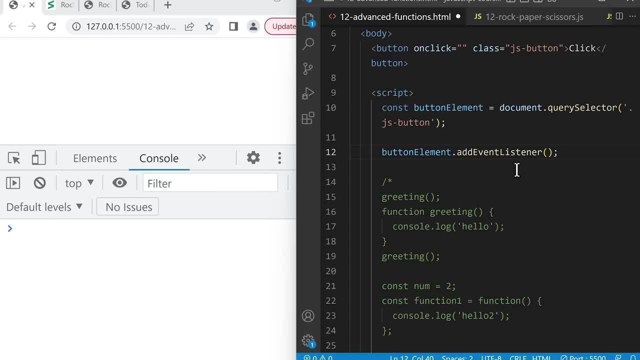 So addEventListener has two parameters. The first parameter is the event Or what type of interaction we want to listen for. So between these brackets let's type the string click. So this will run some code when we click the button. The way to find these event names is to look at this attribute. 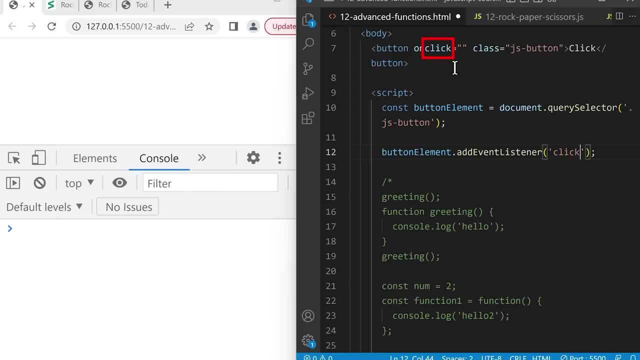 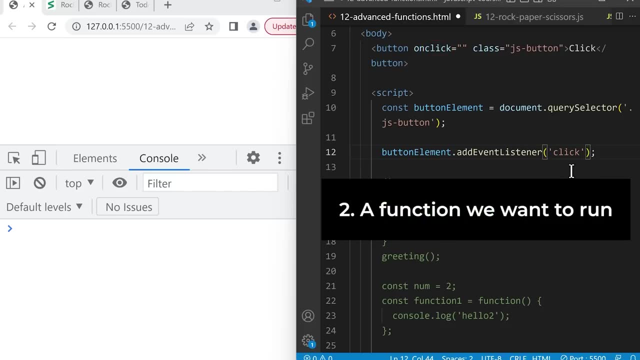 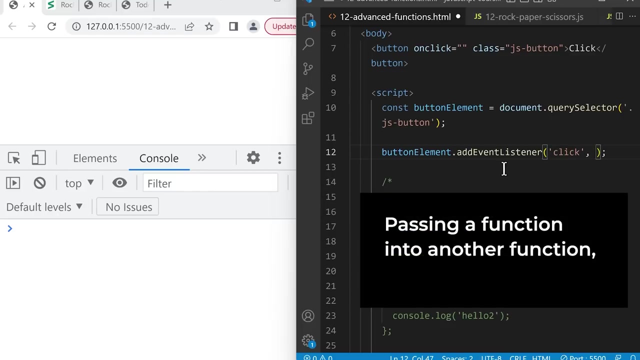 The word after on is the event. Next, the second parameter is a function that we want to run When we click this element. So we'll type a comma And because we're passing a function into another function, we're going to use an arrow function. 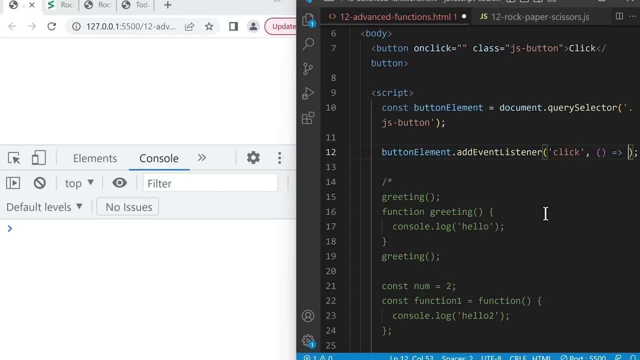 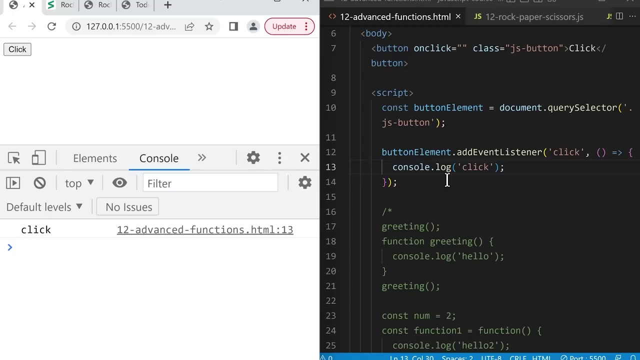 So we'll type brackets, arrow and curly brackets. So inside here let's just do console dot log string click And save, save. and now when we click this button it will run this function and display click. so this code does the same thing as the on click attribute. however, add event listener. 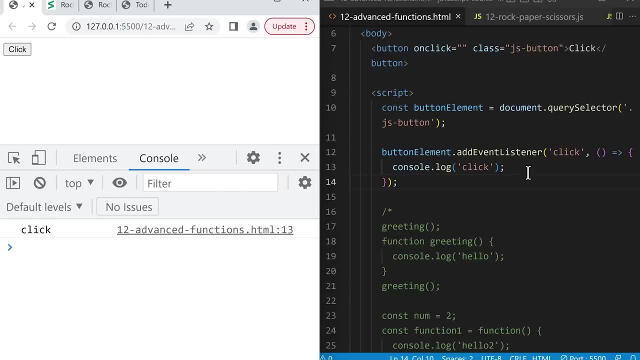 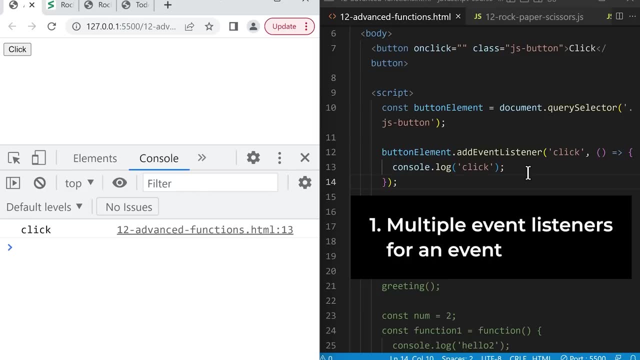 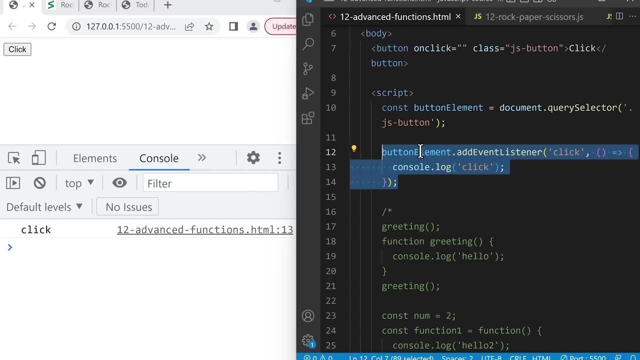 has some advantages over using an attribute. first, it lets us add multiple event listeners for an event, for example. let's add another click event listener. we can select this code and right click copy and then down here right click and paste and let's change this to log click to if we save. 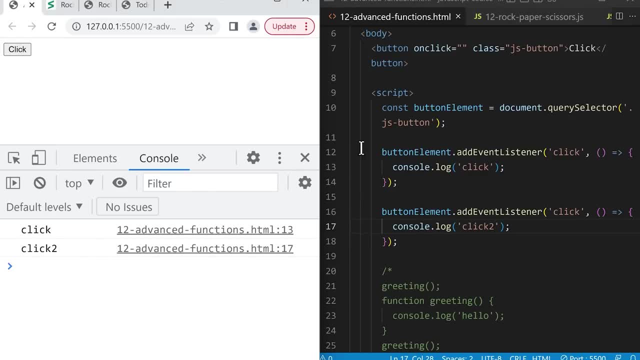 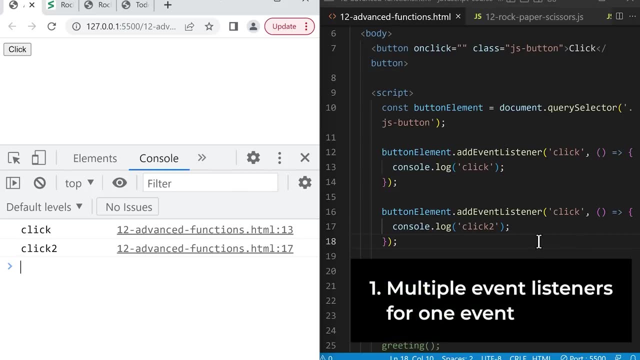 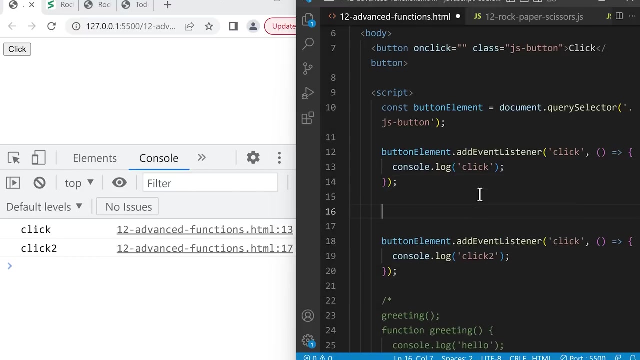 and click the button, it will run both these functions. so add event listener. lets us add multiple listeners to one event. another advantage of doing this is that we can remove an event listener using a method called remove event listener. so under this code we can type button element dot. 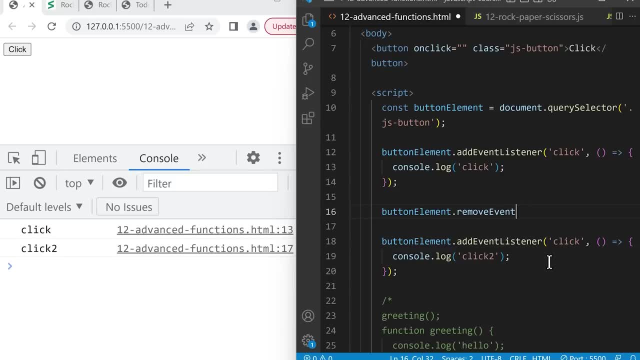 remove capital e, event, capital l, listener and brackets. and remove event. listener also has two parameters. the first parameter is the event, so in this case it is the string: click and we'll type a comma. and the second parameter is the function that we want to remove, so that when we click this button it will no longer run that function. now we can't just type. 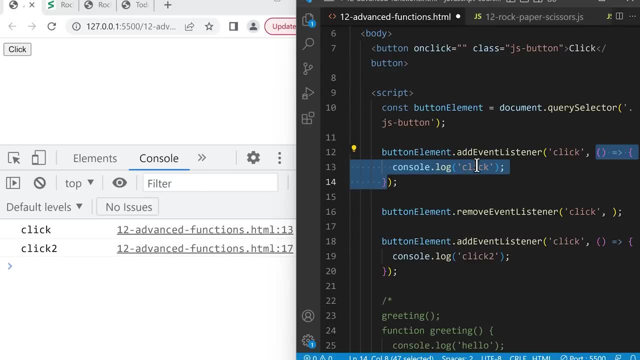 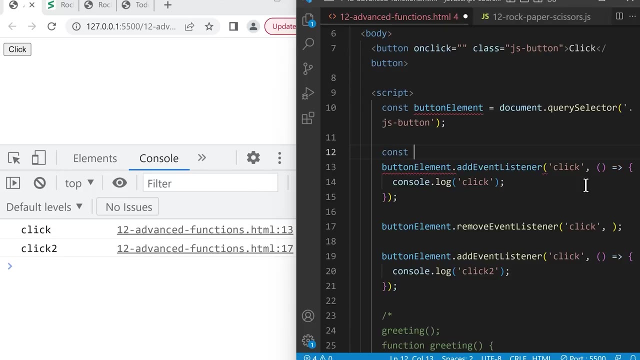 a copy of this function. we need to use this exact function inside remove event listener. to do that, we'll save this in a variable first. so above this, let's create a variable: const event listener equals and we'll select this code right click, copy and in here, right click and paste. 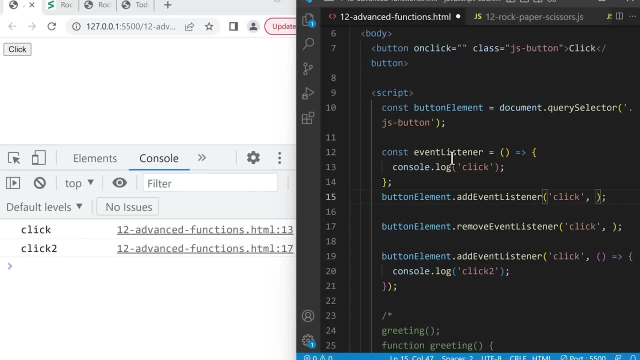 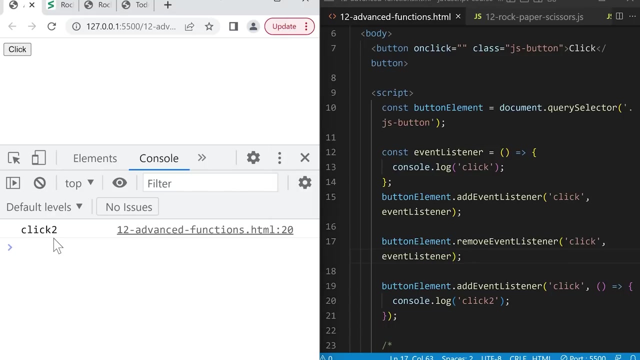 and now we'll replace this with the variable event listener and down here we'll remove this same variable event listener. if we save and click the button again, it will only display click to, because we added this event listener and then we removed it, so it will no longer run this function when we click the button. 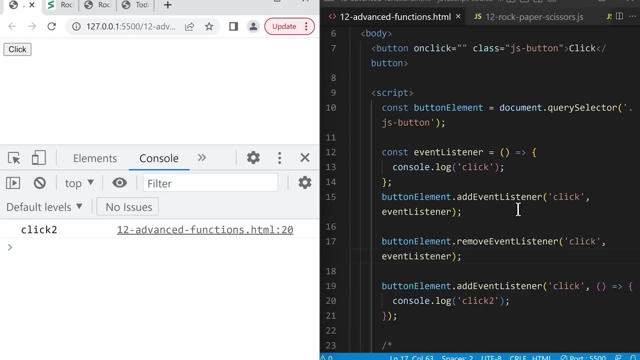 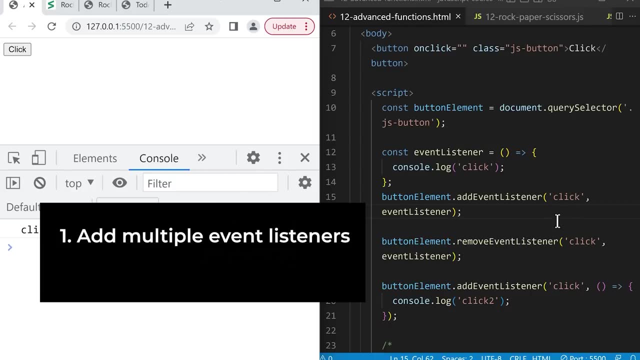 so, as you can see, add event listener gives us more control over event listeners. we can add multiple listeners to an event and we can also add event listeners. so let's say that we want to add several event listeners over event listeners. we can add multiple listeners to an event and we can also. 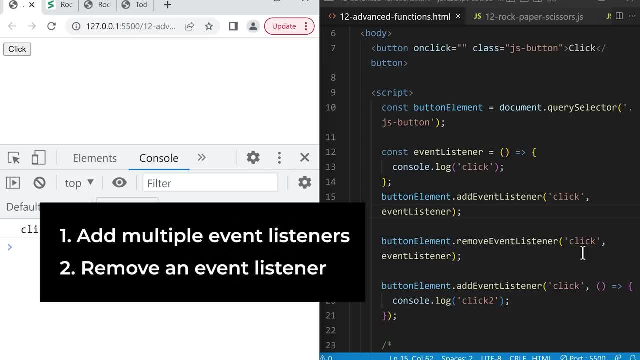 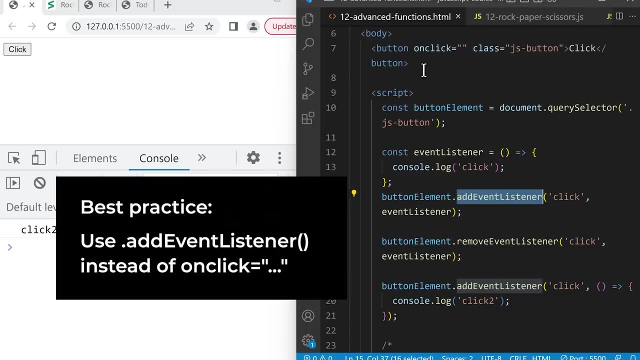 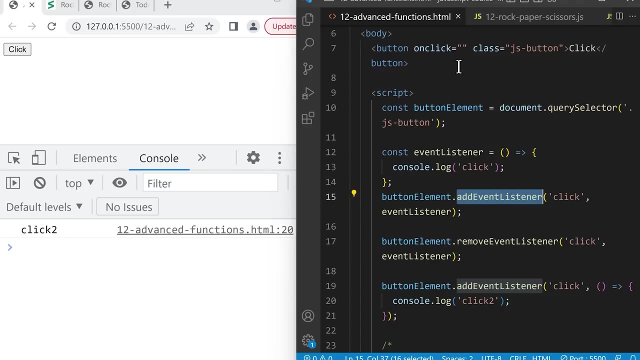 we can also remove a listener from an event. so because of these advantages, the best practice is to use add event listener instead of an on click attribute. so let's go back into our projects and switch to using add event listener. we'll start with the rock paper scissors project. 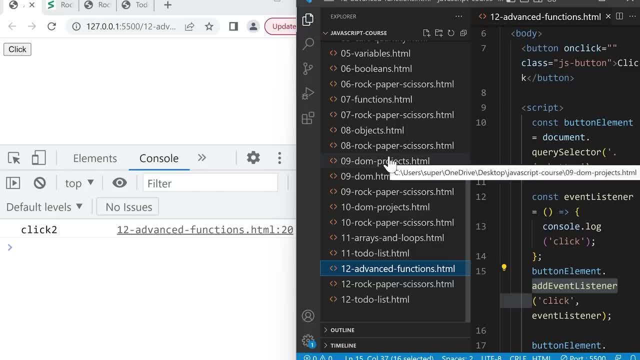 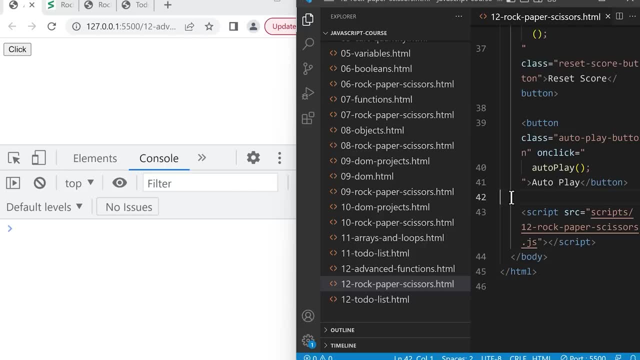 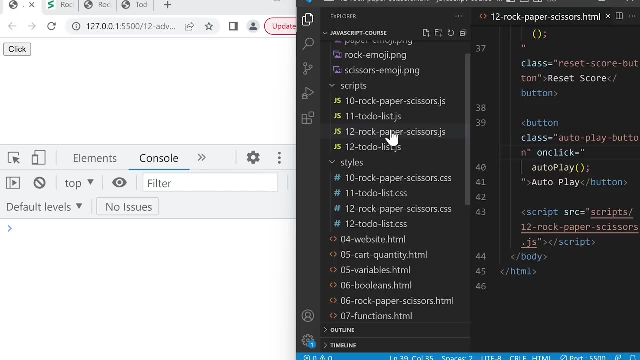 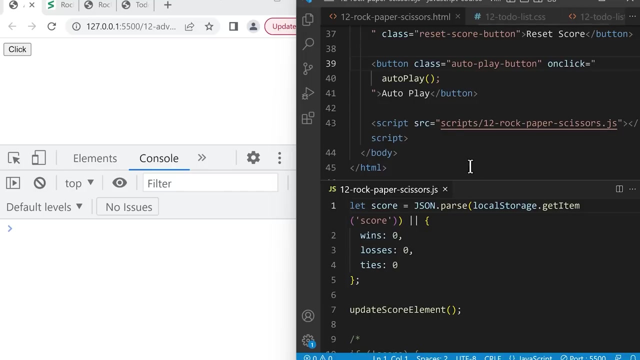 so we'll open our files and we'll open 12 rock paper scissors and click here and save and we'll scroll up to 12 rock paper scissorsjs and for the video i'll drag this down to the bottom and i'll hide the files for now and then rearrange the windows. 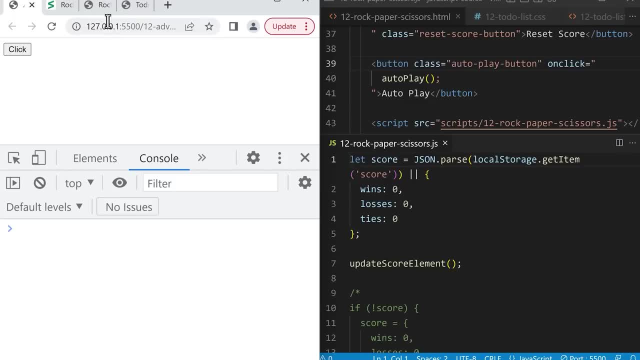 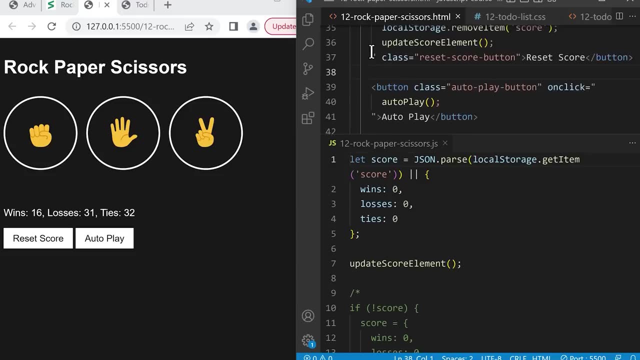 and and finally open the tab for this file. now let's go to the html. we'll scroll up to these move buttons which is up here. so here we're using the on click attribute and we're going to switch it to add event listener. so first let's get this button into our javascript. we'll add a class so we can. 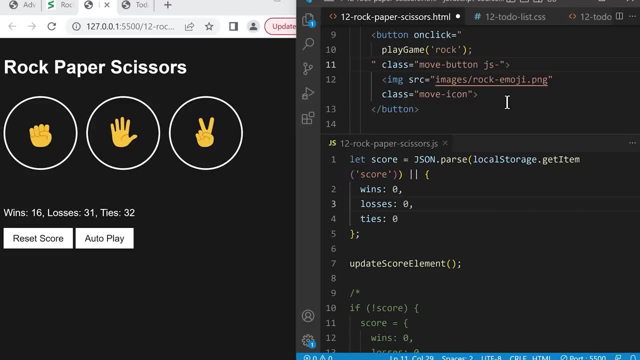 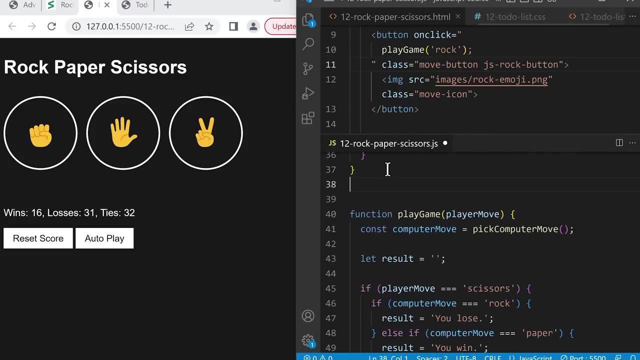 select it: js dash rock, dash button and save and then down here let's go below the autoplay function right here and we'll use add event listener. so we'll get this button into our javascript using document dot, query selector brackets and a string: dot. js dash rock, dash button. 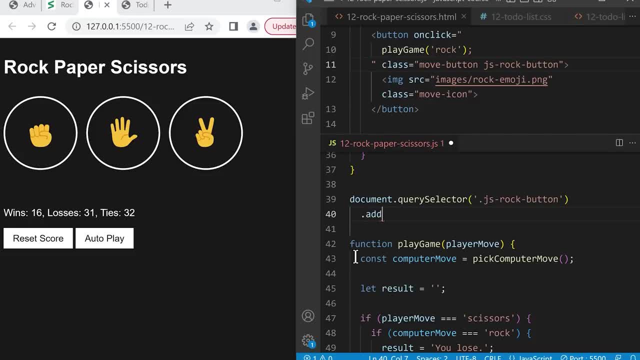 and we're going to use dot add event listener brackets. so we're going to listen for a click and a comma and we'll give it a function that we want to run. so a common mistake here is to actually run the function. for example, play game brackets and the string rock. so we're supposed to give a function to add event. 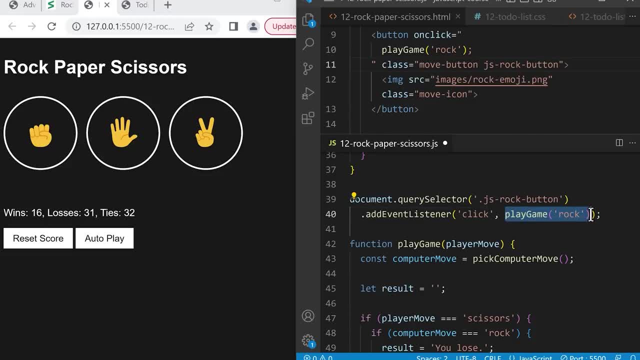 listener. however, this doesn't result in a function. this will actually run play game and give us the return value, which is undefined. so this code will actually result in undefined and then we're giving undefined to add event listener, so it won't work. so, in order to give add event listener a function, we need to. 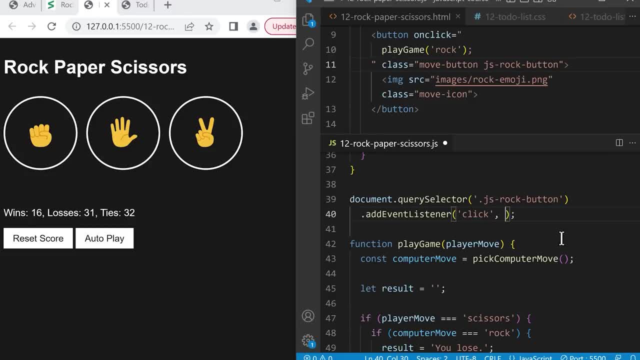 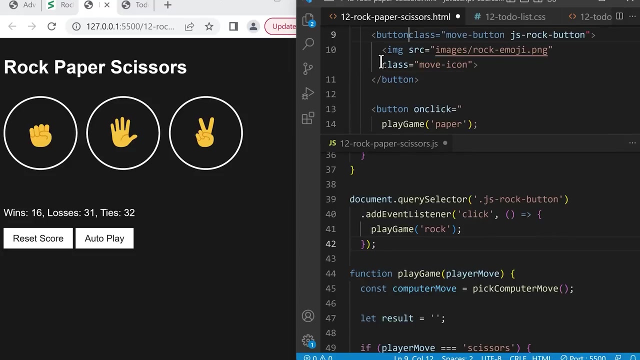 create a function here. so let's remove this code and we'll create a function using brackets, arrow and curly brackets, and then inside this function we're gonna call play game, so a type play game- brackets and rock. so now when we click the rock button it will run this function and play the game. so let's remove the on click attribute. 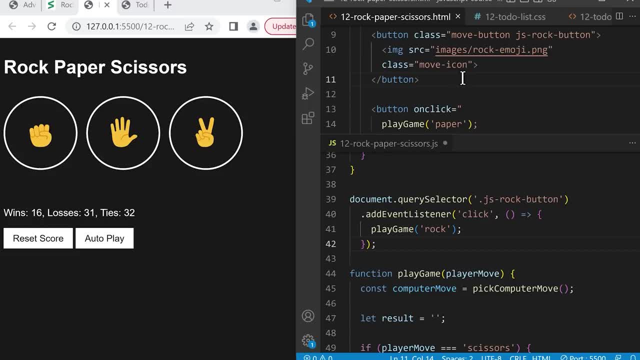 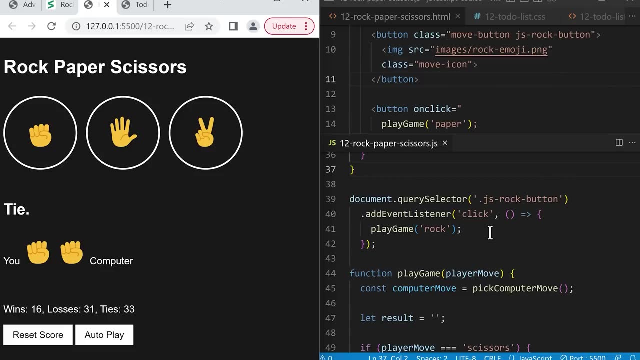 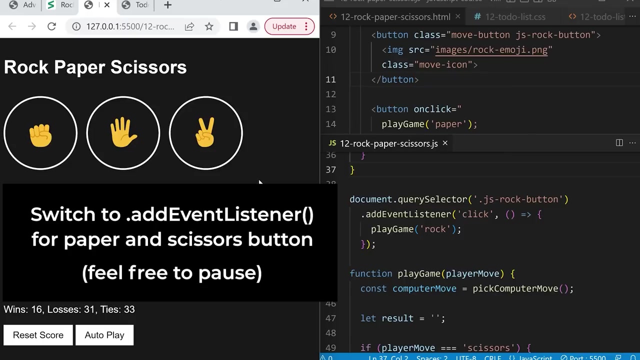 and and save the html and also save the javascript, and then go to our project and click the rock button. you can see that it works, except this time we're using add event listener, so let's do the same thing for the paper and the scissors button. feel free to pause the video if you. 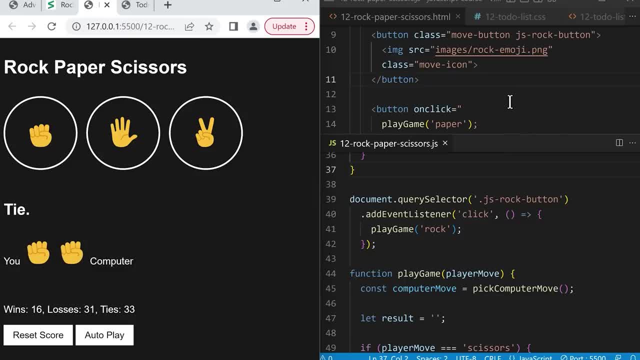 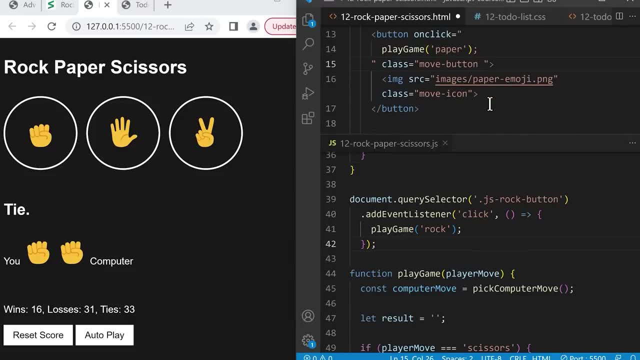 want to try it yourself. so we'll scroll down here and let's add a class to the paper button so we can select it: js dash, paper dash button. and then in our javascript we'll make a copy of this code. so right click, copy and then down here. 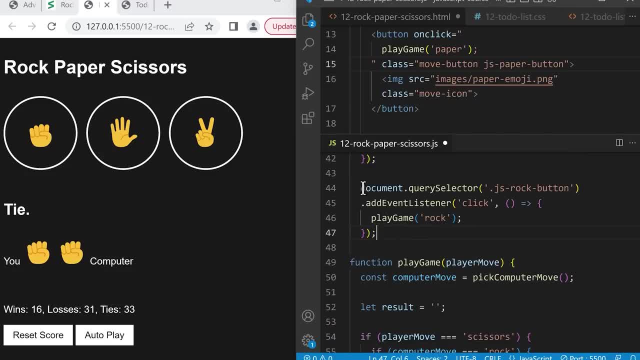 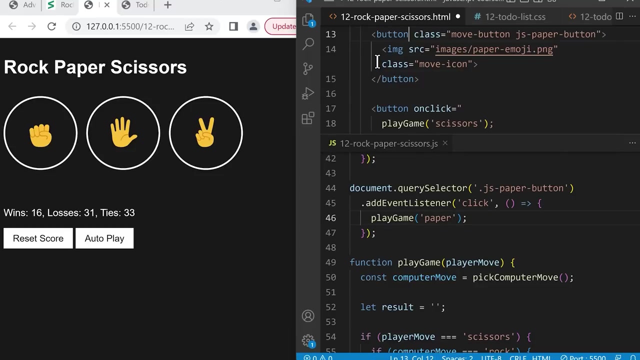 right click and paste, and now we're going to replace the rock button with paper. and when we click this button, we're going to play the game with paper. now let's save and we'll remove the on click attribute and save the html. if we click the paper button, it works as before. 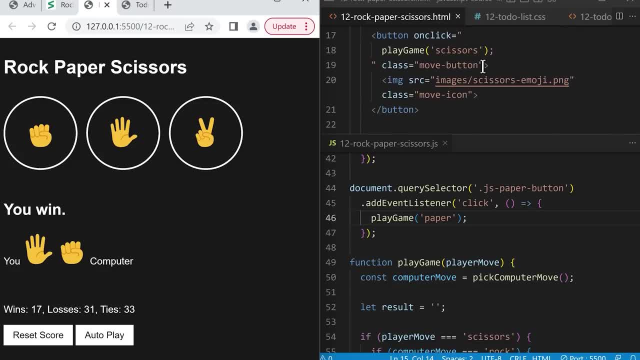 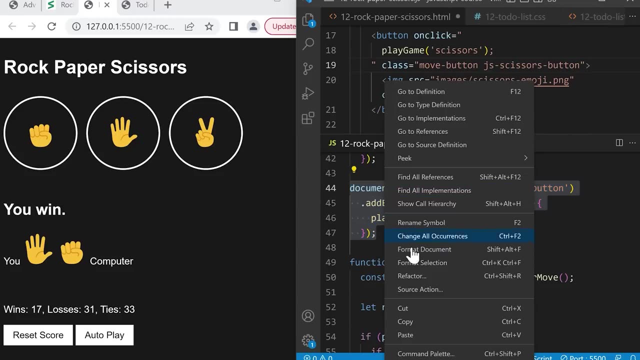 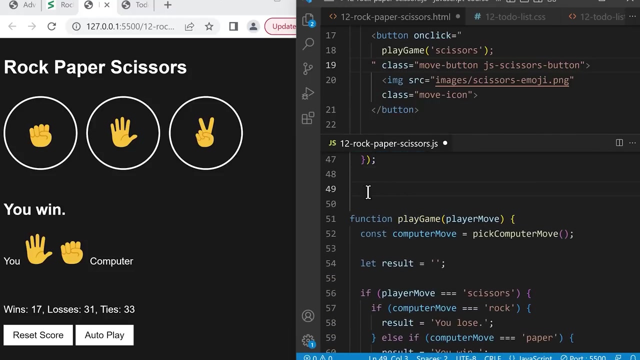 finally, let's do the scissors button. so we'll add a class js dash, scissors dash button and then inside our javascript we'll make a copy of this right click, copy and then down here create some new lines, right click and paste and now switch to the scissors button and play game with scissors. let's save and remove the on click attribute. 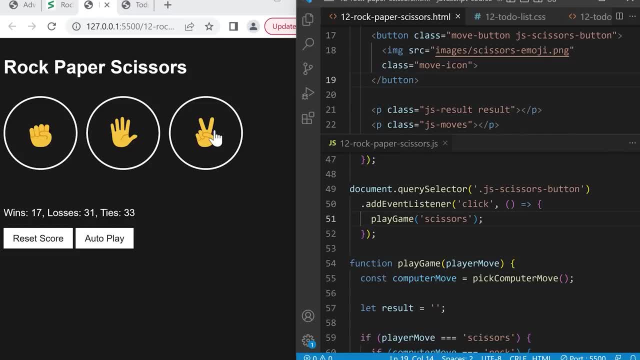 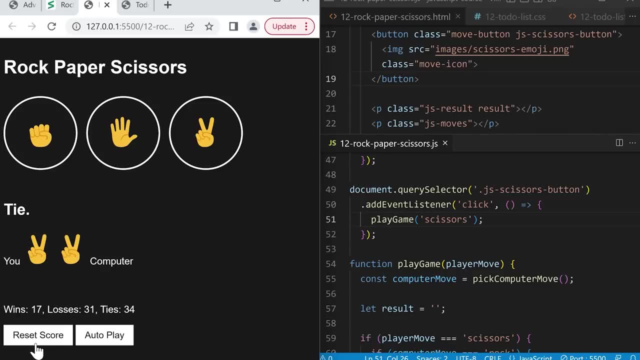 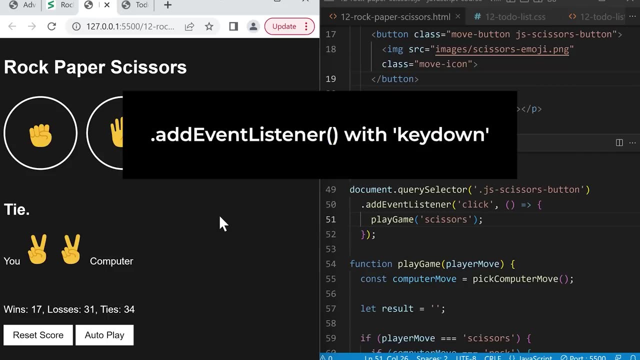 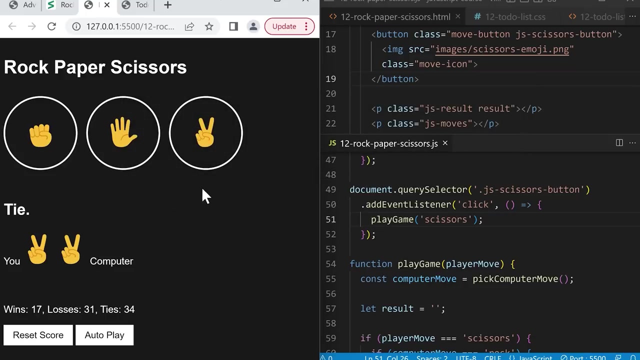 save the html and try the scissors button. so everything still works, and i'll leave switching the reset score button and the auto play button as exercises. so now let's try add event listener with a different event. we'll use it with key down. so let's say that in our project we want to make it so we can play the game with our keyboard. 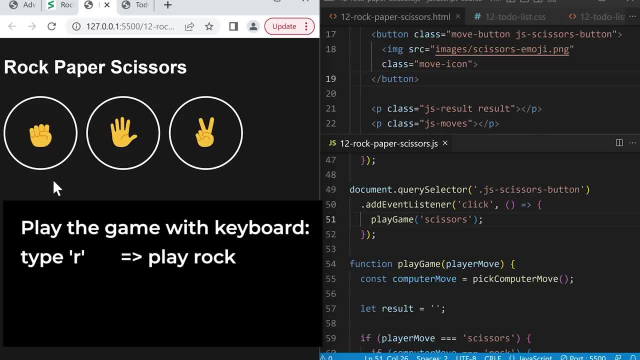 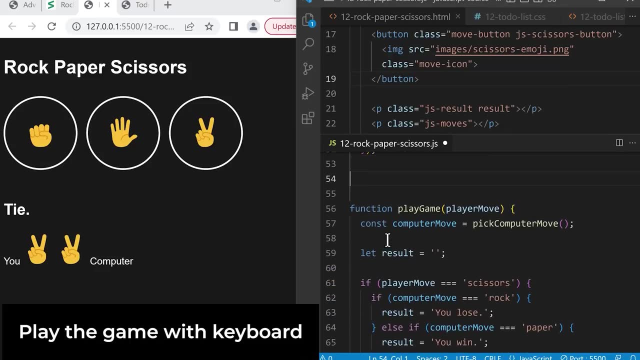 if we type r, it will play rock, if we type p, it will play paper and if we type s, it will play scissors. let's go into our javascript and we'll scroll down and we're going to add an event listener to the body this time, so that if we type anywhere on the page we can run some code. 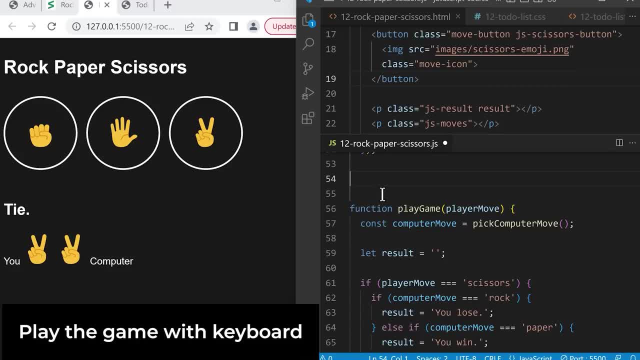 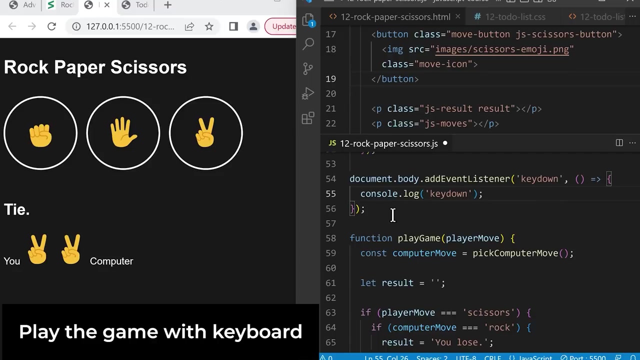 so we're going to get the body element using document, dot, body and then dot, add event, listener and brackets. this time the first parameter or the event will be the string key down and let's type comma and give it a function that we want to run brackets arrow and curly brackets inside. here let's just type console dot, log key down for now and save. 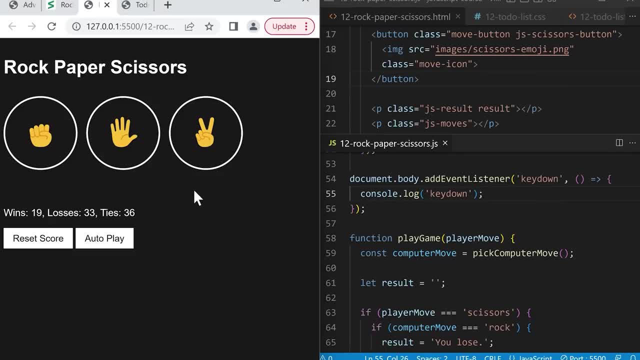 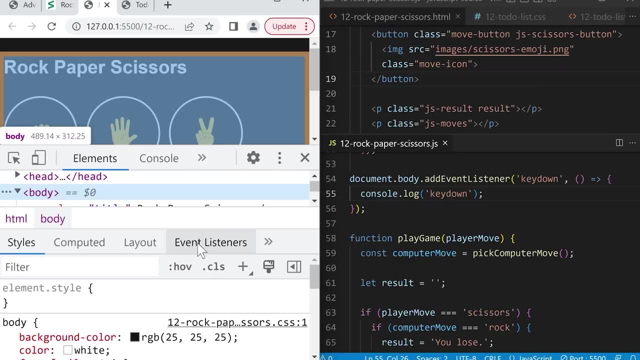 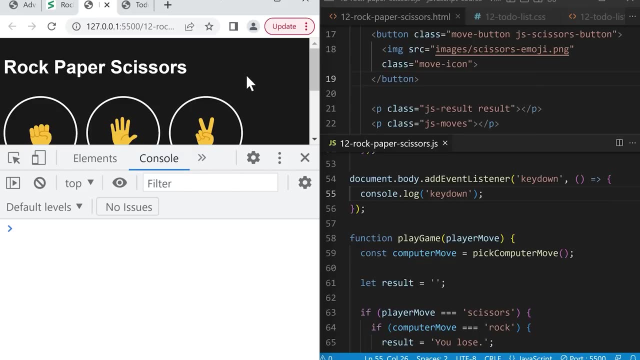 So now, if we go to the project and we open the console, right click and click Inspect, click the console and then click on the page. if we type a key on our keyboard, it will run this function and display keyDown. 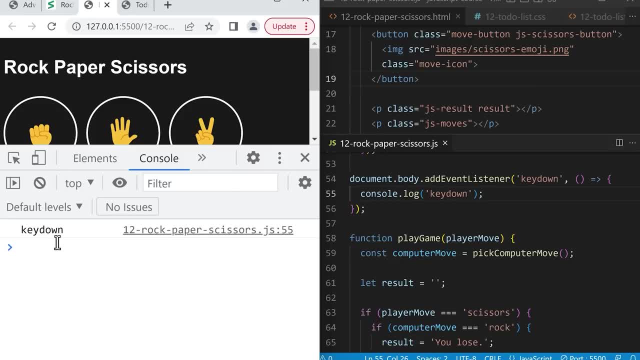 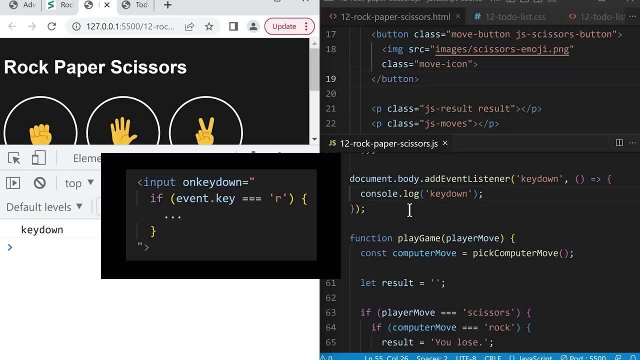 So now we have to check what key was pressed and play the game. So how do we know which key that we pressed? Earlier in this course we used the attribute onKeyDown and we learned that it gets a special object called event and the event object contains which key was pressed. 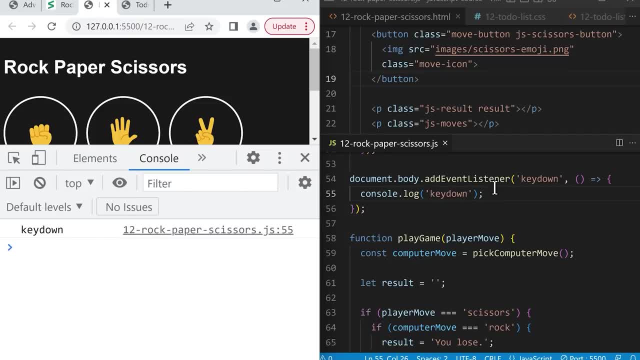 AddEventListener also provides this event object, but it provides it as a parameter to this function. So inside the round brackets let's add a parameter event. Now, every time we type on our keyboard, addEventListener will save the event object in here and run. 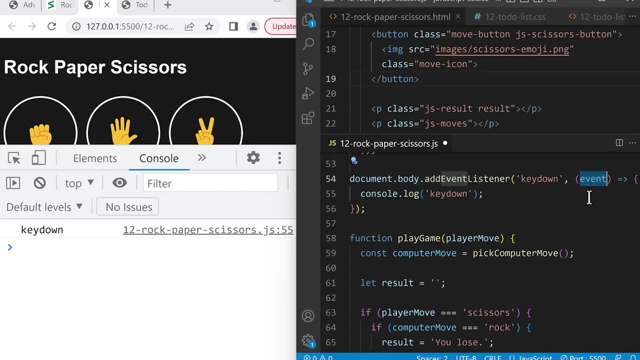 the function And this event object contains the key that we pressed. So in the consolelog, let's display eventkey this time and save. Now. if we click on the page And type r, eventkey will contain r. If we press p, eventkey will contain p. 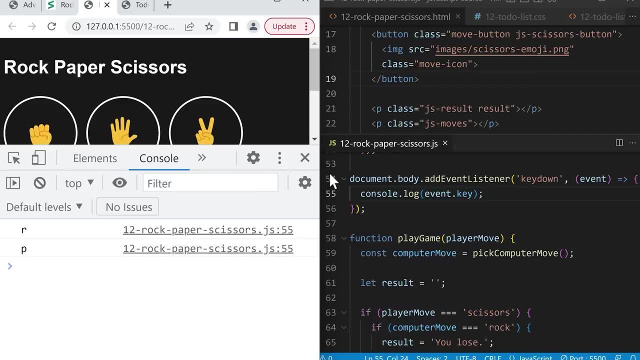 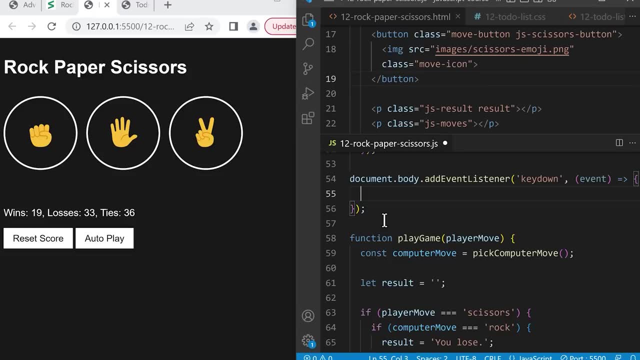 So that's how we know which key we pressed. So now let's close this and instead of consolelog we'll create an if statement to check which key we pressed. So if brackets And curly brackets, And here we'll check if eventkey is equal to the string r. 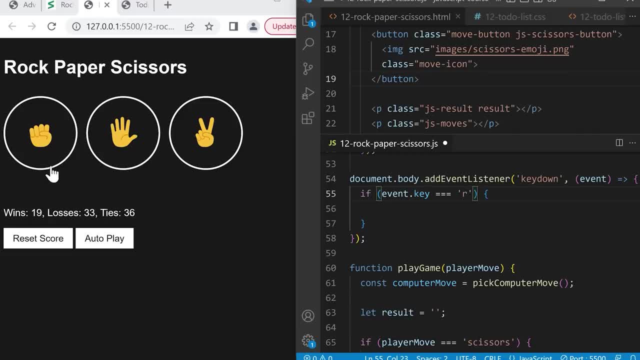 If it is, we're going to play the game with rock. So inside here we can just run this, play game, function, Play game and brackets, And inside we'll type the string rock. Now let's check if we pressed p. 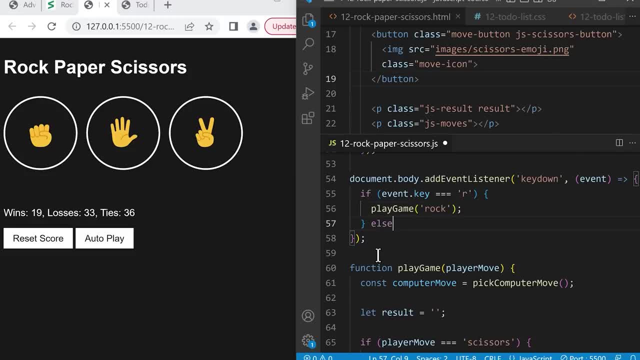 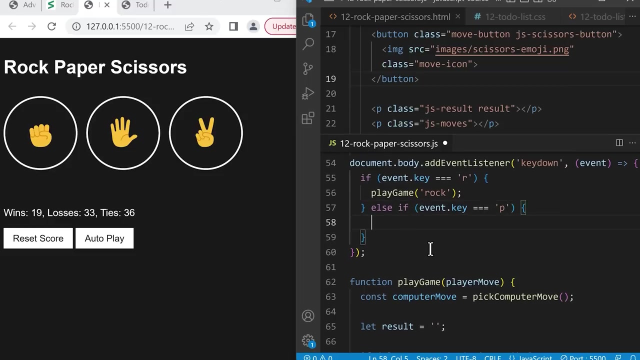 So we'll add another branch, else if brackets and curly brackets, And in this second condition we'll check if eventkey is equal to the string p. If it is, we'll play the game with paper. So inside here we'll run play. 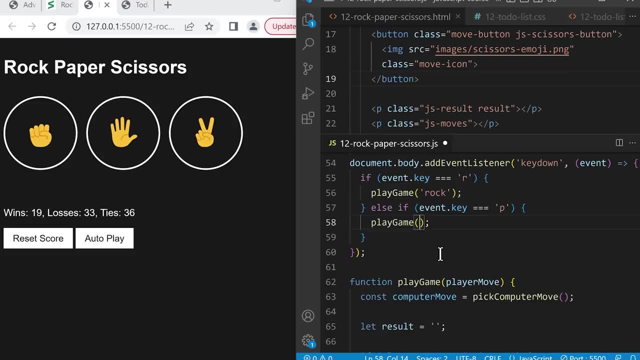 Play game brackets and the string paper. And finally we'll check if we pressed s. So at the end we'll add another else, if brackets curly brackets, And inside here we'll check if eventkey is equal to the string s. 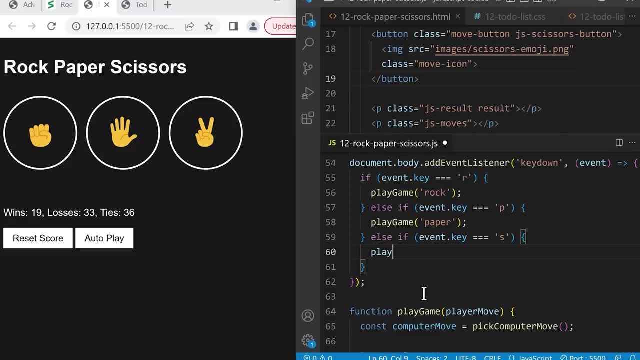 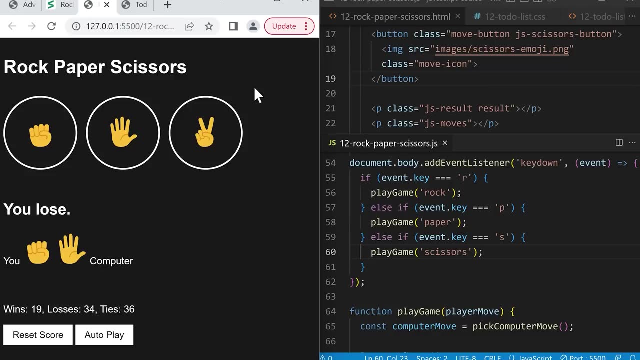 If it is, we'll, We'll play the game with the string scissors. Now let's save, click our page and type r, And it plays a game with rock. If we type p, it will play the game with paper. 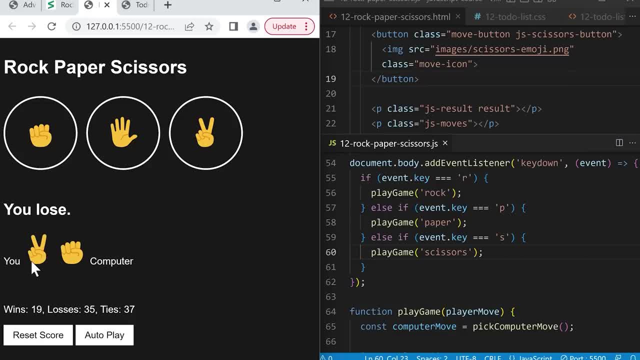 And if we type s, it will play the game with scissors. So that's an example Of using add event listener with a different type of event with a key down. If we need the event object, we can get it using a parameter up here. 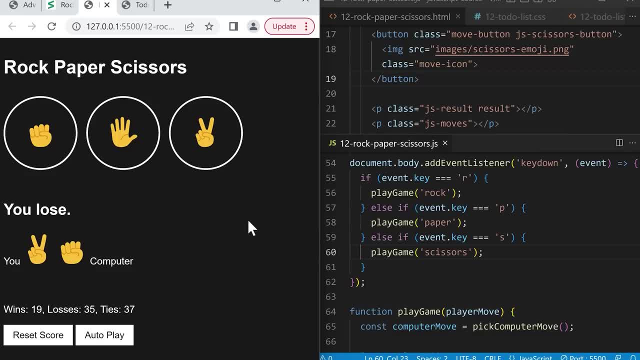 So those are all the features we're going to create for our rock-paper-scissors project. Now let's move on to the to-do list project and switch to add event listener. We'll go into our code editor, click up here And click on add event listener. 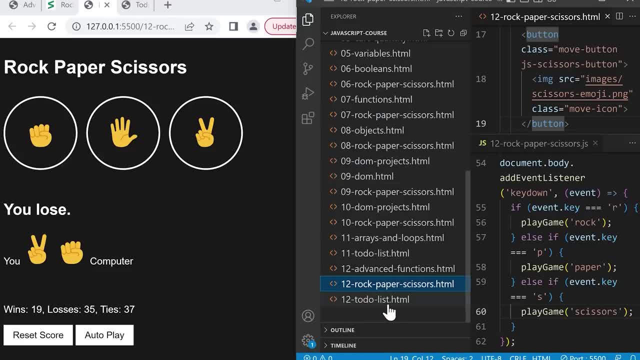 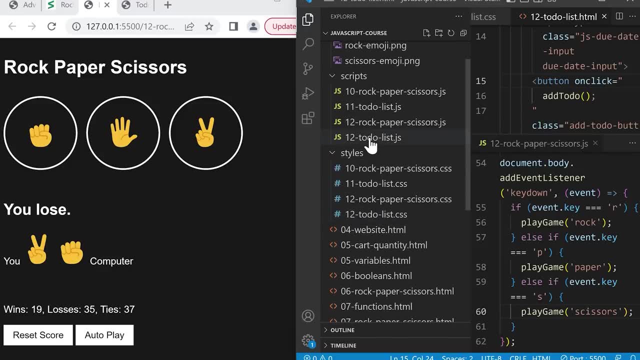 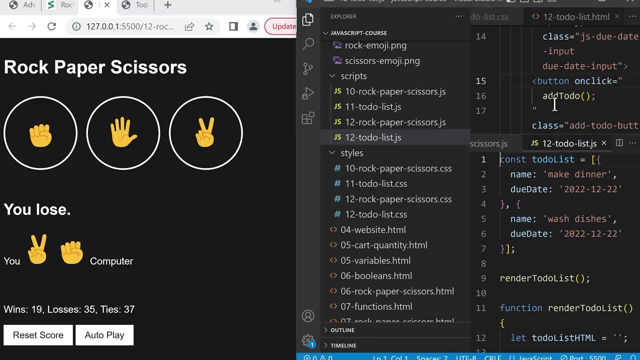 And click if parameters And find 12.. We'll also scroll up to the scripts folder, find 12todolistjs and open this file And I'm going to put it at the bottom here so I can see it side by side. 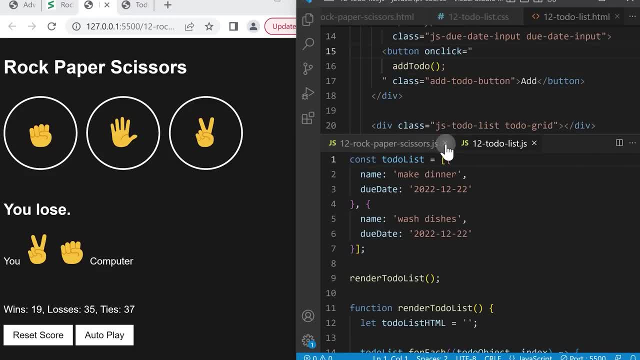 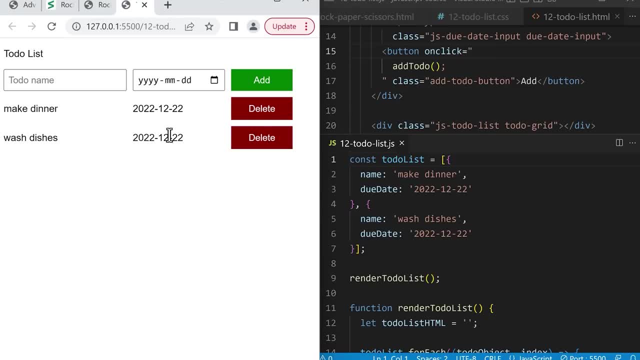 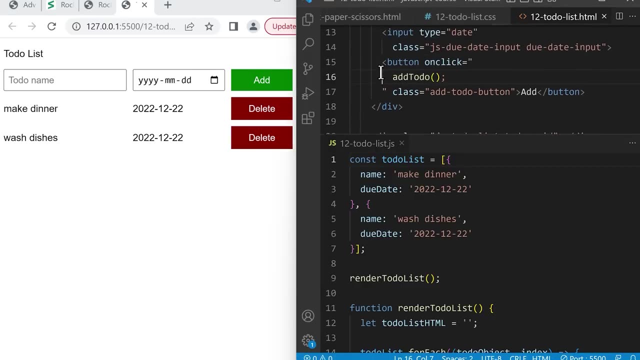 I'll close this for now and close Rock Paper Scissors and then open the tab for this project. Okay, so let's start by switching the add button to use addEventListener. We'll go into our HTML and find the add button, which is here, and we're going to add a class. 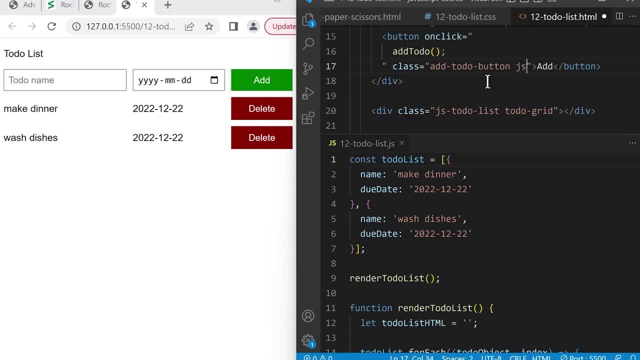 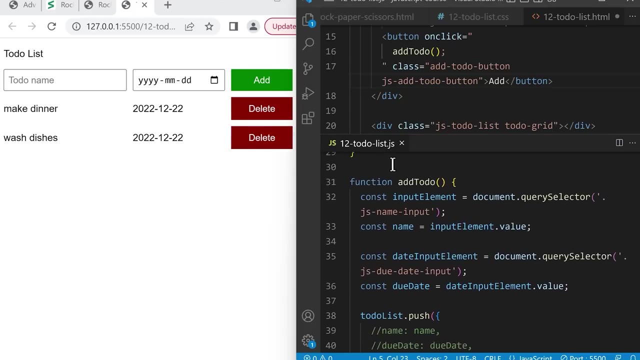 so we can select it in JavaScript: js-add-todo-button. Now let's go to our JavaScript And scroll down above the addTodo function. we'll get this button into our JavaScript using documentquery selector brackets and then a string dot and the class we want. 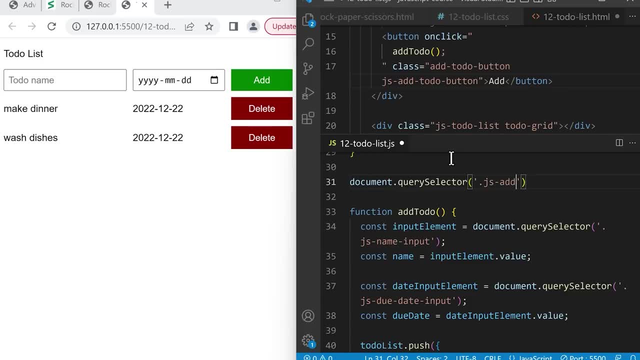 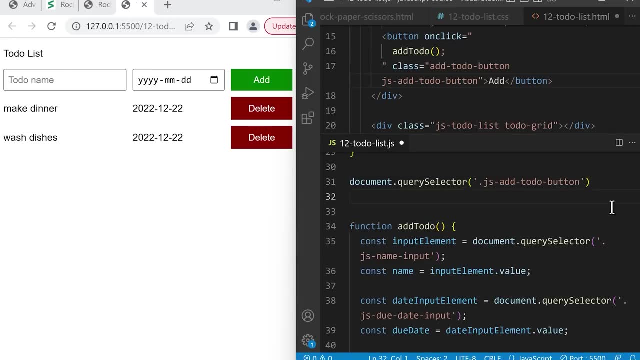 to get js-add-todo-button And then after this we'll use dot addEventListener brackets. Inside these brackets we'll give it the event, the string, click comma and then a function to run when this event happens. 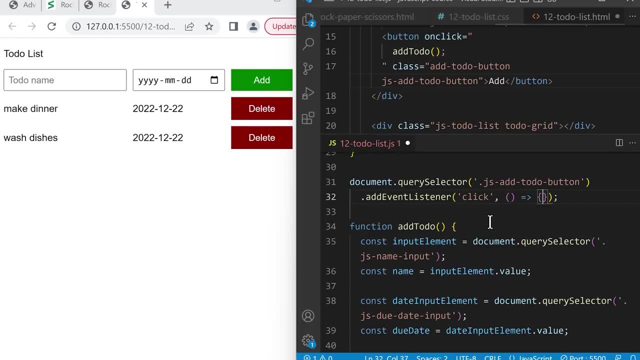 So brackets, arrow and curly brackets. And in here We just want to do the same thing as the onClick attribute, which is addTodo, and call this function, Let's save. and then in the HTML, let's remove the onClick attribute and save, and let's. 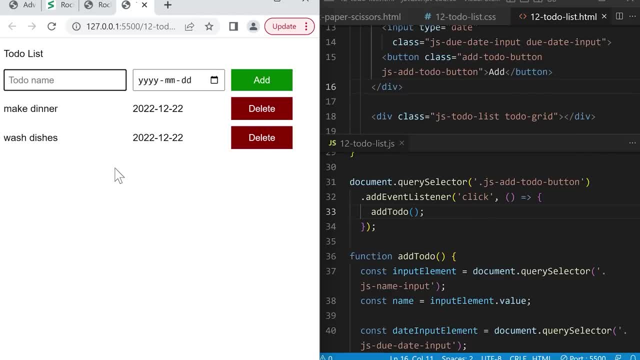 try it out. So we'll type aTodowatchyoutubeaddEventListener. Okay, Select a due date and then click add, And the add button still works as before, but we're just using addEventListener. Next, let's switch all the delete buttons. 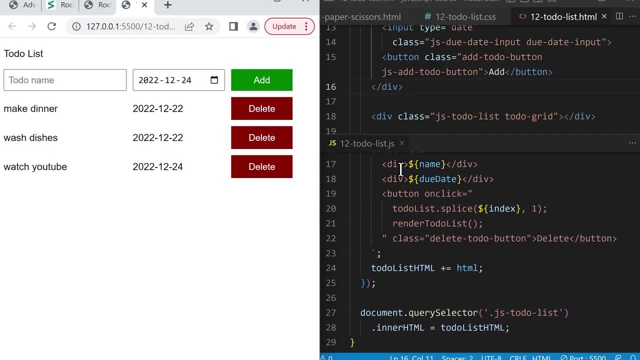 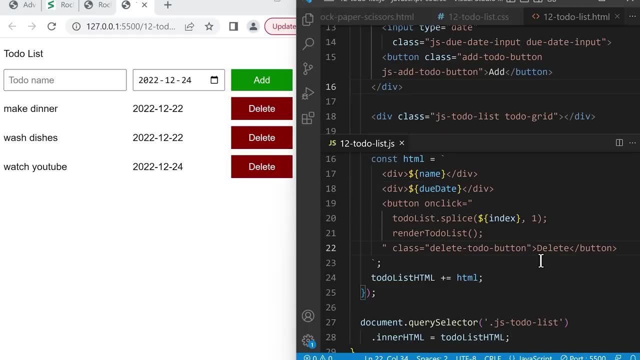 Let's scroll up to where we create these delete buttons, which is here, And first we'll add a class to all the delete buttons so we can select them in JavaScript js-delete-todo-button. And now we're going to use documentquerySelector and add an event listener to all of these. 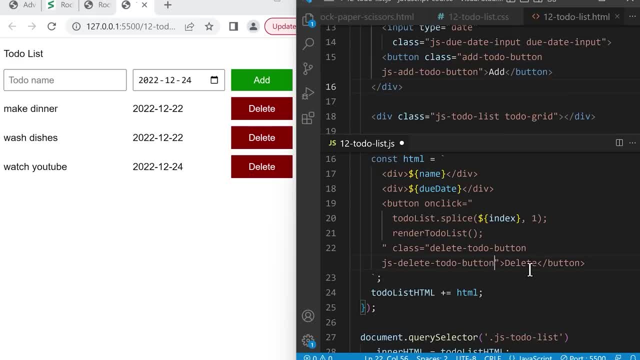 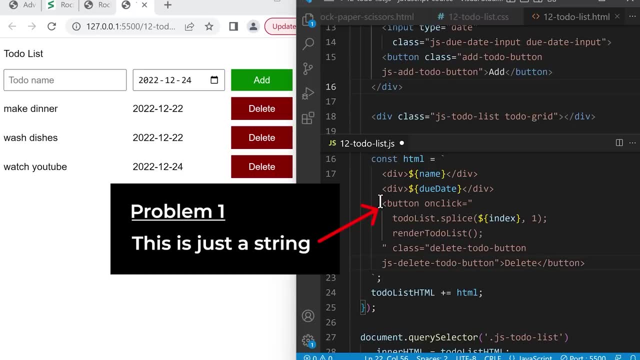 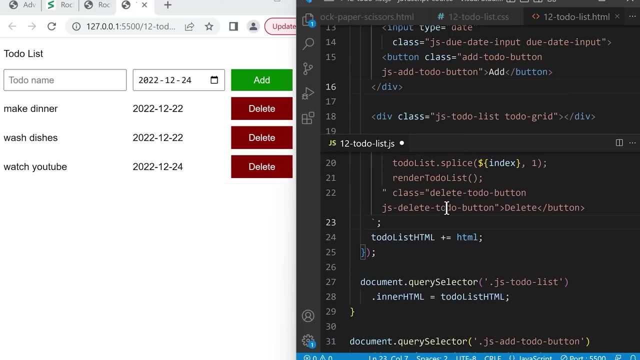 buttons. However, there's two problems here. First is that at this point in the code this is just a string. We haven't actually put this button on the page yet. We do that down here In this line of code. We put the HTML that we generated onto the page. 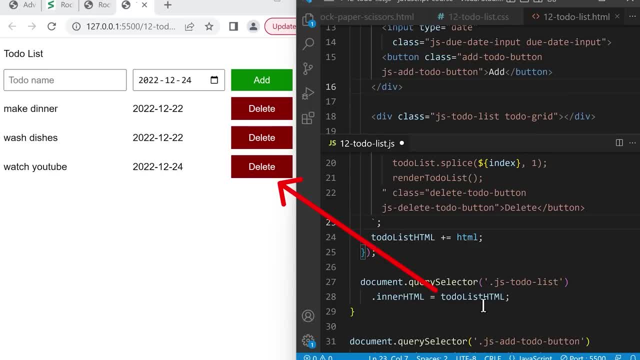 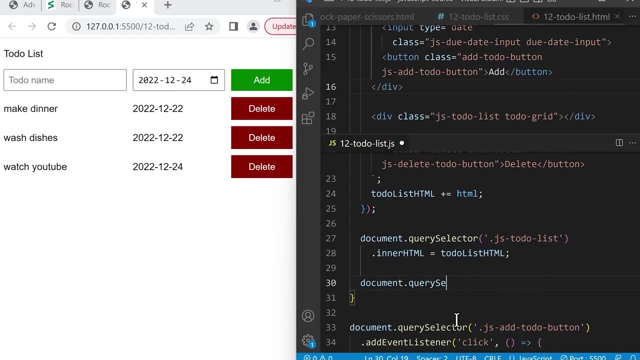 So in order to add an event listener, we need to put the HTML on the page first, so we have to do it after this code. So down here we're going. type: DocumentquerySelector: Okay, Boolean. Run the string dot and we'll select this class j s dash. delete dash to do dash. 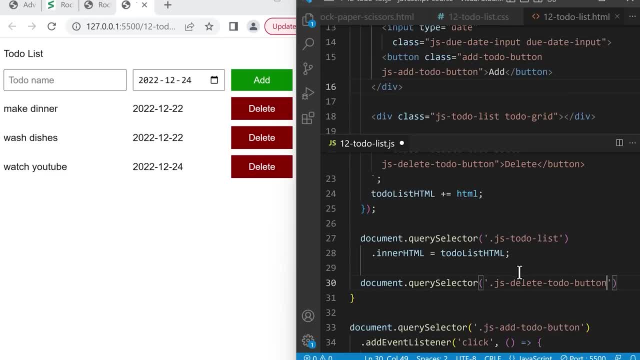 button. however, there's also a second problem here, which is we're gonna have multiple delete buttons and a query selector only gives us the first one. so how do we select all the buttons on the page that match this criteria instead of just the first one? to do that, the document object has another method. 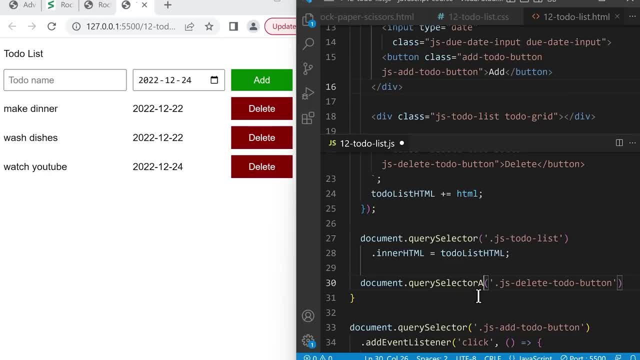 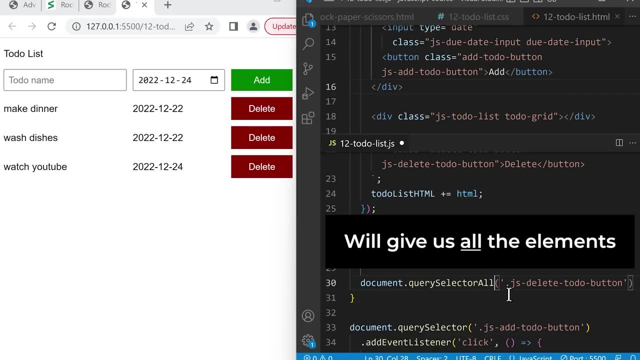 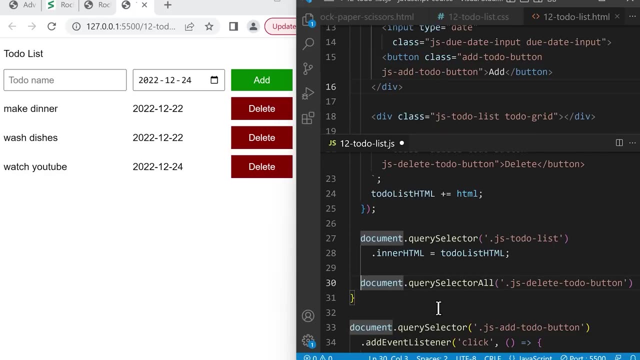 called query selector all. so query selector all will give us all the elements on the page that have the class j s delete to do button. so down here let's console dot log this result to see what it looks like. console dot log brackets and close bracket and save. 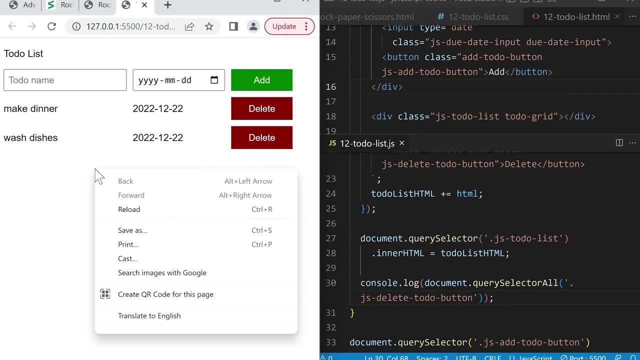 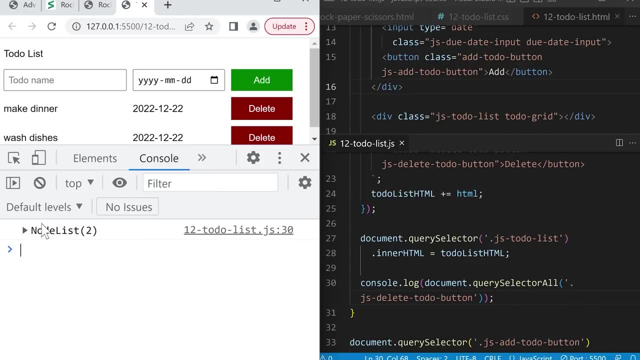 and then here right click inspect and the console and expand this. you'll see that document dot query selector all gives us a list of elements. you'll see that document dot query selector all gives us a list of elements and this list works just like an array. this is index zero or the first button. 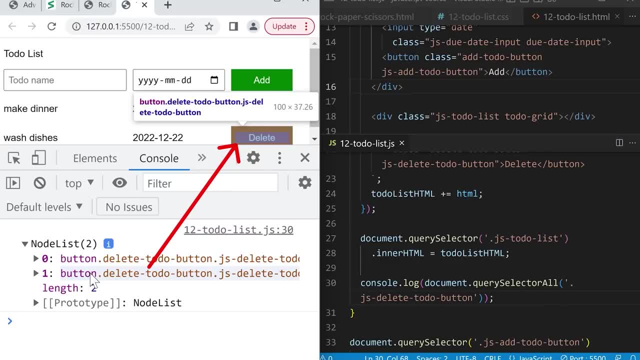 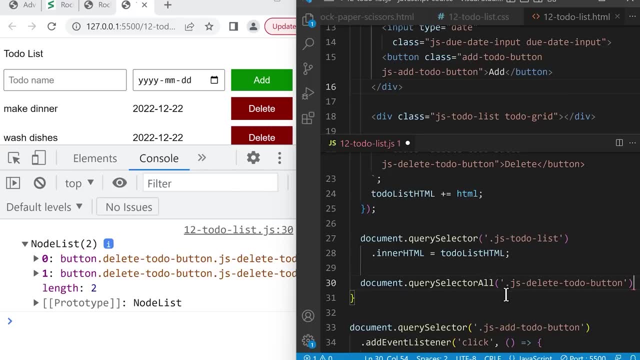 and this is index one, which is the second button. so now let's remove console dot log and add event listeners to all of these buttons. to do that we're going to loop through this list of delete buttons. so again, this list has works like an array so we can use a foreach method to loop through it. 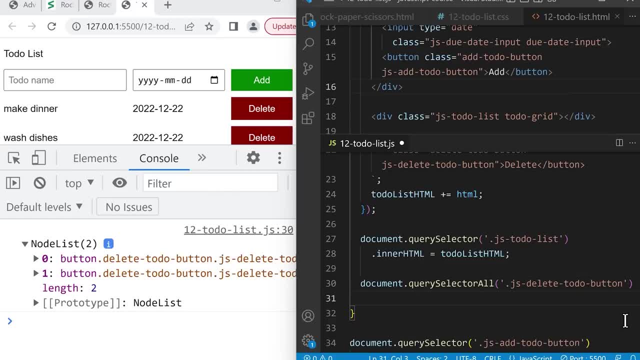 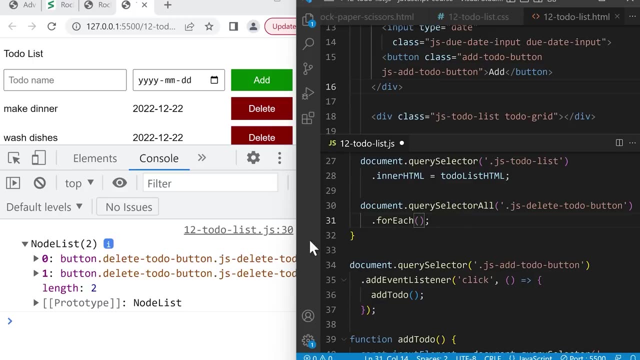 So at the end let's type enter and tab and then dot foreach and brackets. As usual, we'll give foreach a function that we want to run for each of these values. So we'll type brackets, arrow and curly brackets, And now every time we loop through the list, foreach will give us two parameters. 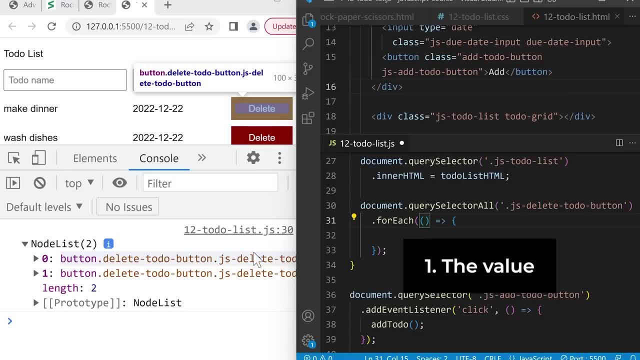 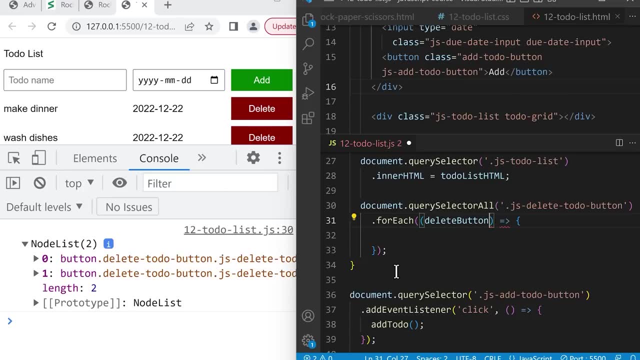 The first one is the value in the list, which is a deleteButton element. So let's name it deleteButton And we'll type comma. And the second parameter is the index, So index And index. So now we want to add an event listener to each deleteButton. 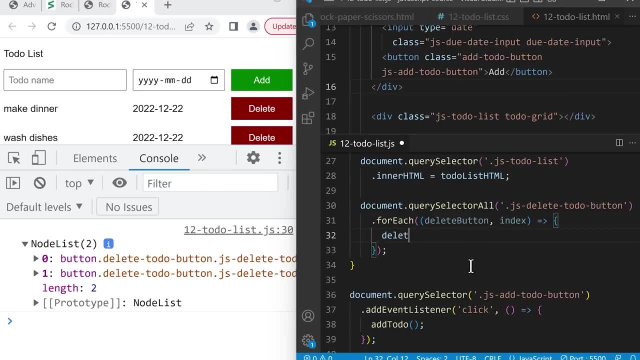 So inside here we'll type deleteButtonaddEventListener and brackets. Inside these brackets we'll tell it what event we want to listen to, which is the string, click And comma And then a function that we want to run when this event happens. 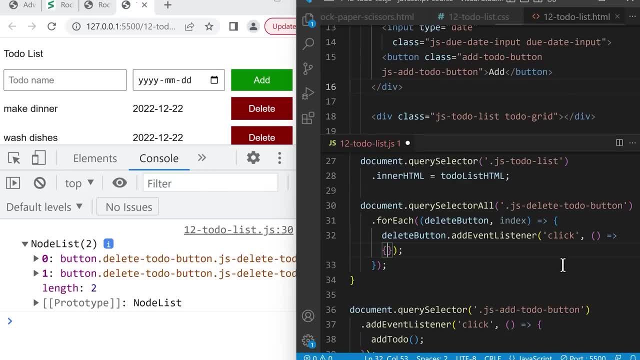 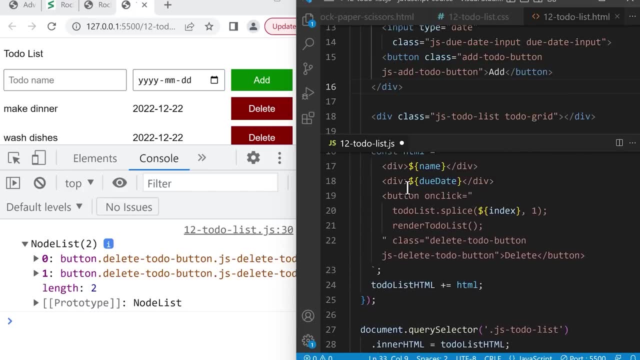 So brackets, arrow and curly brackets. So now, when we click a deleteButton, we want to do the same thing as this onClick attribute above. So let's select this code, We'll right-click, copy And then down here we'll add a deleteButtonaddEventListener. 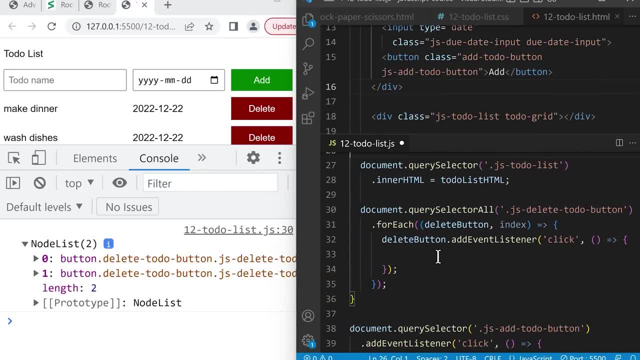 And then a function that we want to run when this event happens, And then down here, right-click and paste, And now we can remove these characters because we're not in a string anymore, And that's all we need to do. So, to summarize: we used querySelectorAll to get a list of all the delete buttons on the page. 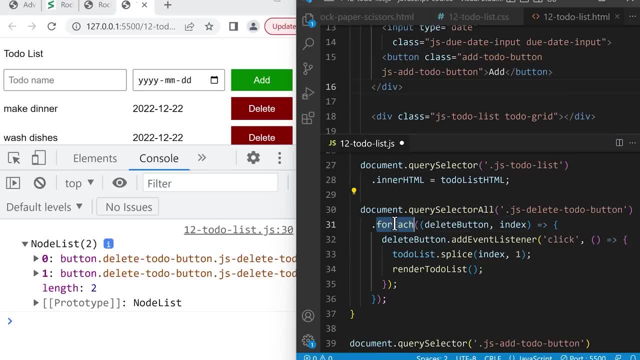 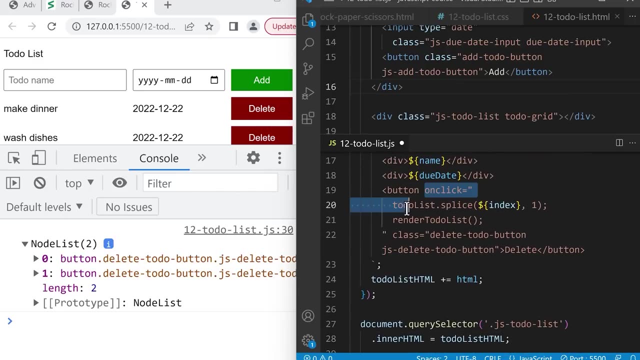 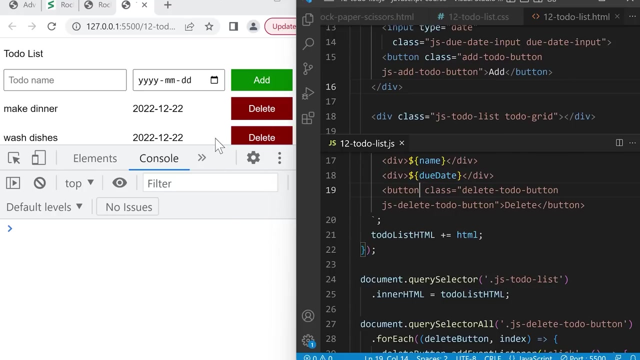 and then we looped through the list using forEach, And for each delete button we added a clickEventListener and ran the same code that we did before. So now we can scroll up and remove this onClick attribute and save, go back to the page, close the console and try out the delete button. 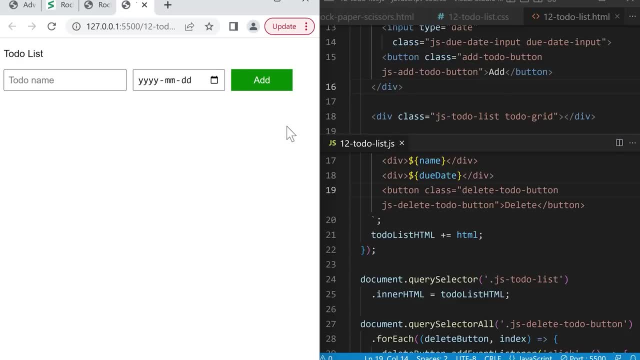 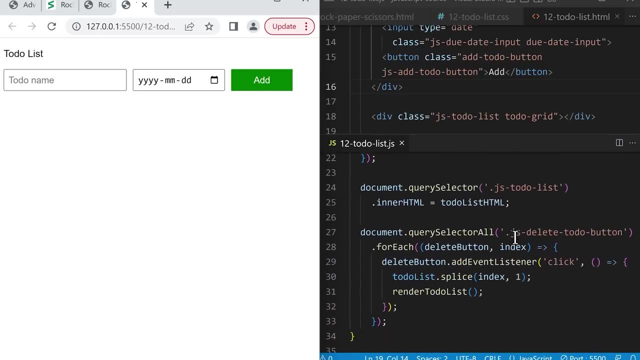 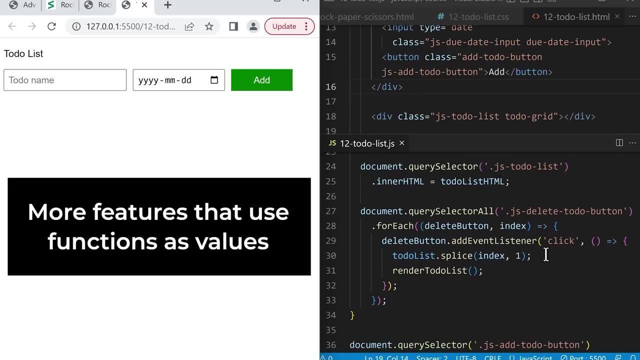 And you can see that it still works. So that's how we switch the toDoList project to use addEventListener. So now we're finished improving all of our projects. In the rest of this lesson we're going to learn more features that use functions as values. 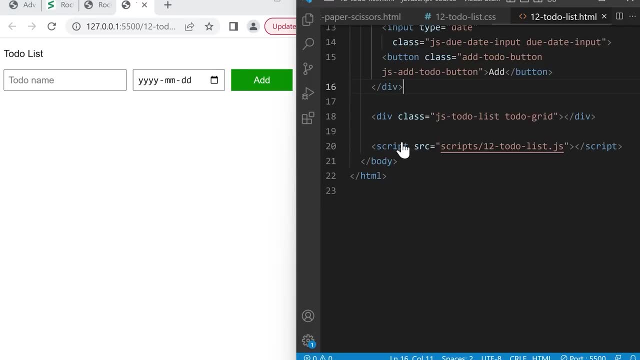 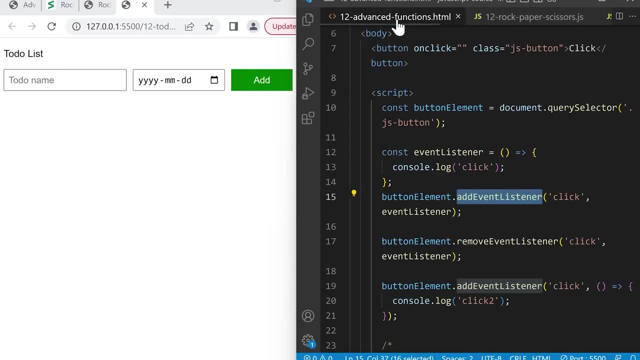 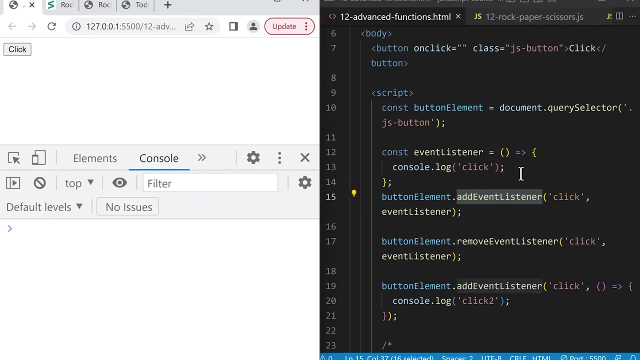 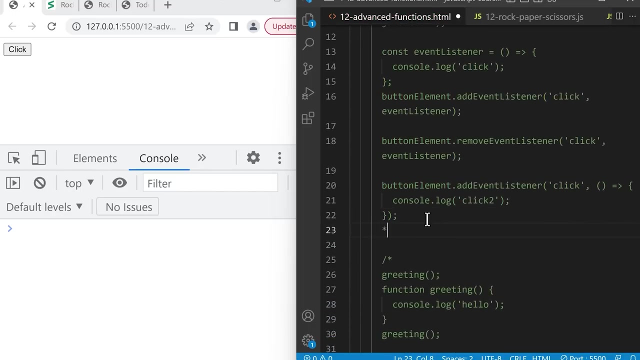 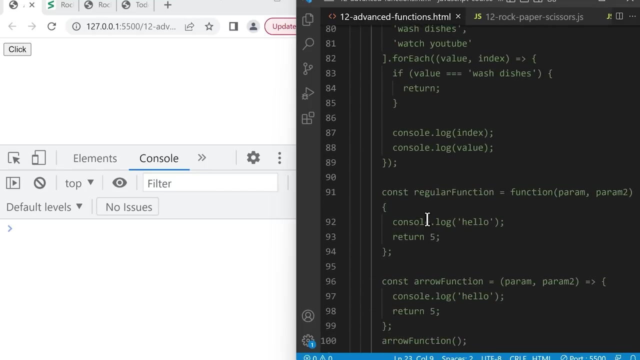 So let's close this for now and we'll go back to 12AdvancedFunctionshtml And we'll open the tab And let's comment out this JavaScript code using slash, star and star slash. Let's save And now let's scroll to the bottom of this code. 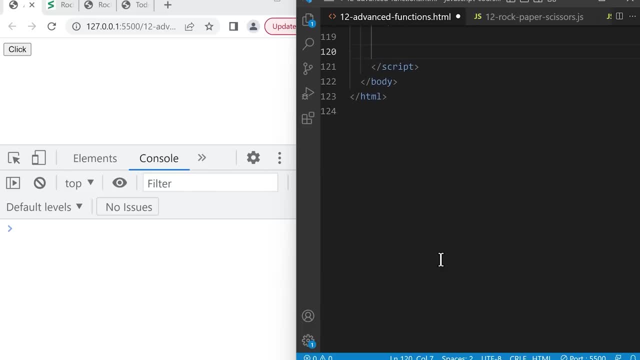 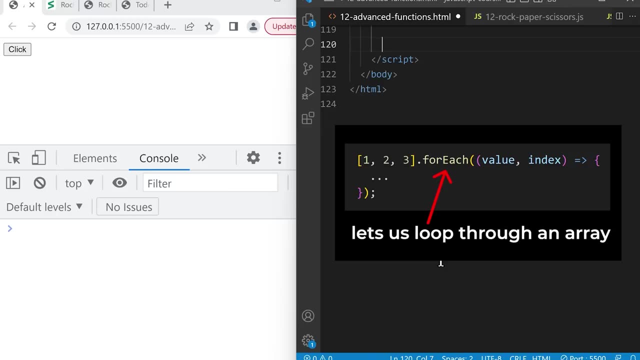 And create some new lines. So in this lesson we learned the array method forEach, which lets us create a list of all the delete buttons on the page, lets us loop through an array. Now we're going to learn two more array methods, called filter and 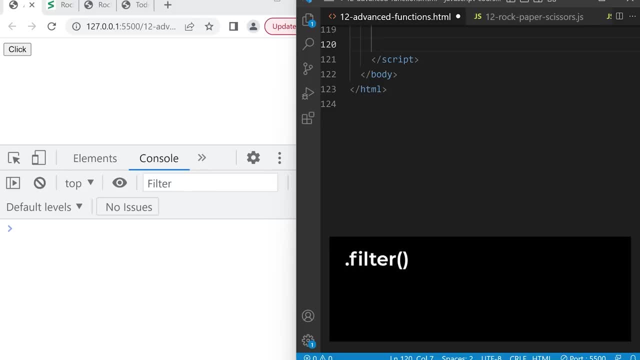 map. So let's start with filter. Let's say we have an array of numbers and we want to create a copy of this array with all the negative numbers removed. So let's go up here and create an array of the number 1 comma negative, 3 comma 5- and type the method dot filter. 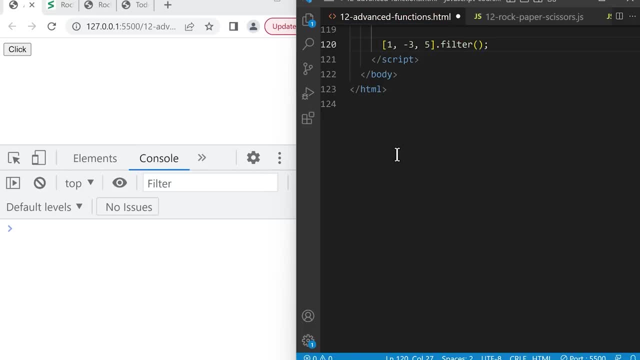 and brackets. So filter works the same way as for each. We give it a function, so bracket, arrow and curly, bracket. And this function has two parameters: The value and the index. So filter will take the first value, save it in here and run. 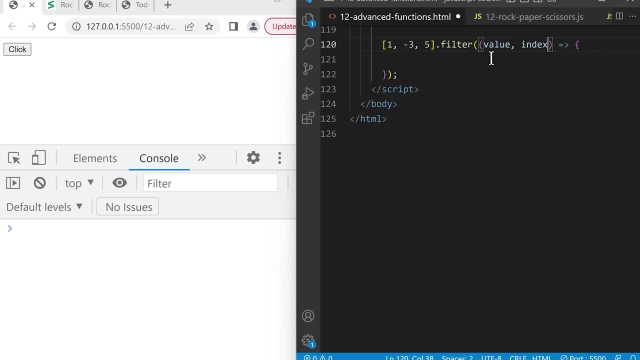 the function. Then it will take the second value- save it in here, run the function- and the third value: save it and run the function Now. the only difference is that this time this inner function will return a value, So we'll type return. 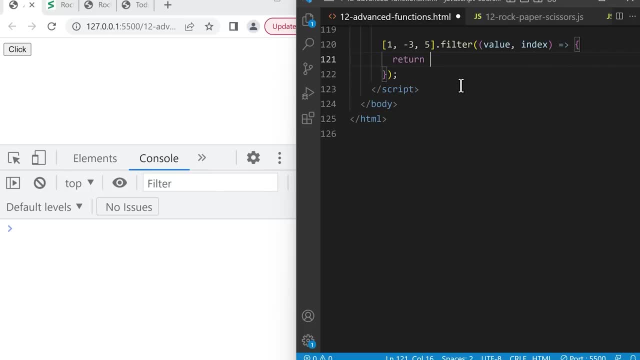 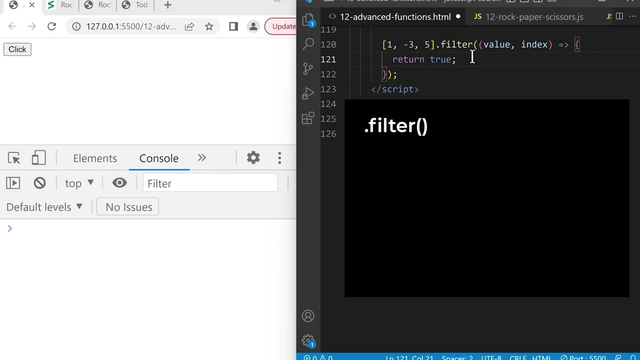 And we're going to return a boolean like true. So now the return value matters. So what filter does is it creates a new array. If the inner function returns true, it will put this value in the new array. If the inner function returns false, it will not put this value in the new array. 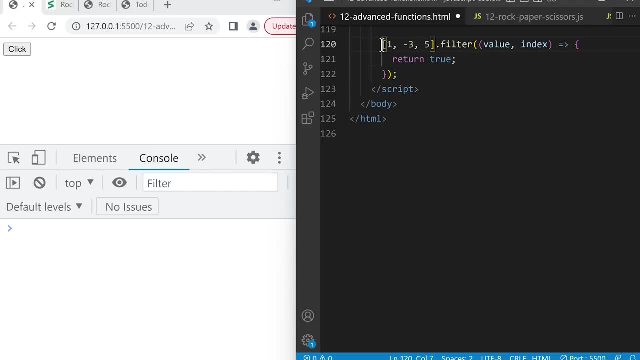 For example at the front consolelog the result of this. So we'll type consolelog, open bracket and down here, close bracket and save. So in this example the inner function always returns true. So all three values will be in the new array If we change the return value to false every time and save. 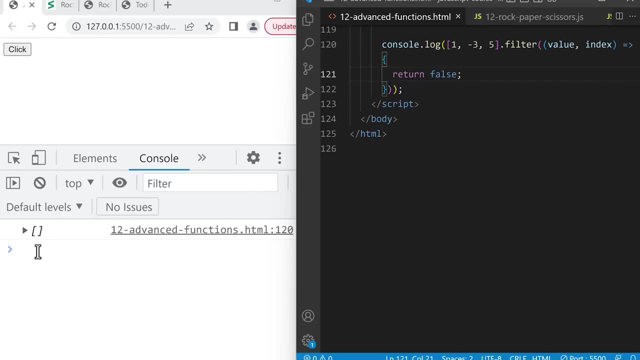 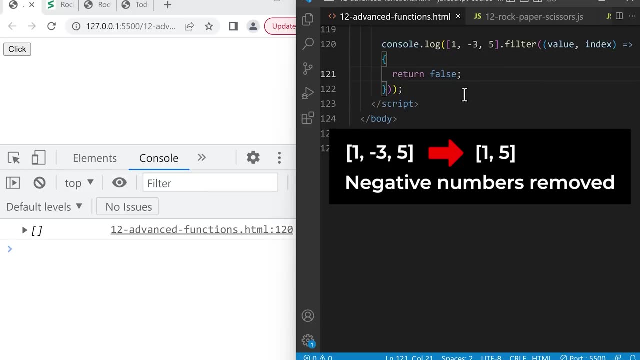 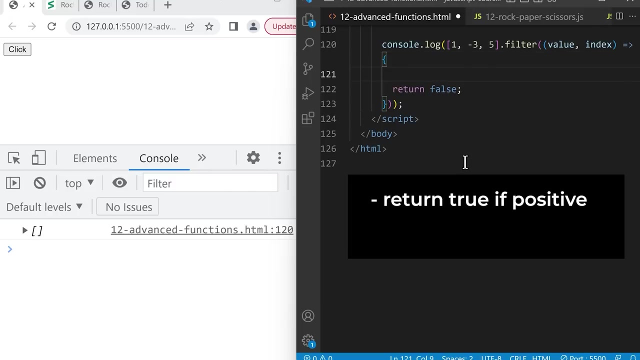 all three values will not be added to the new array. So now let's use this to solve our problem. We want to remove the negative numbers from this array. So inside this inner function, we're going to return true if the number is positive and return false if the number is. 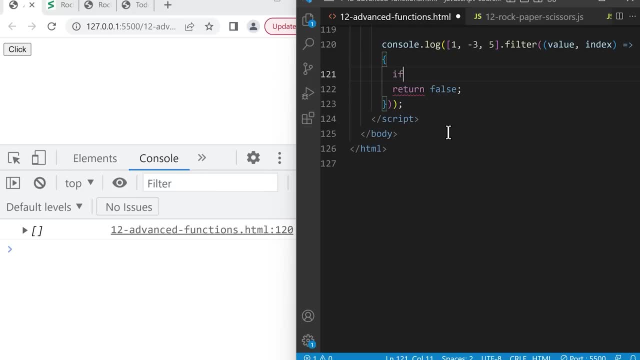 negative. So we'll check if value is greater than or equal to zero. curly brackets will return true and include it in the new array. Else will return false and not include it in the new array. So let's remove this and save. So now only values. 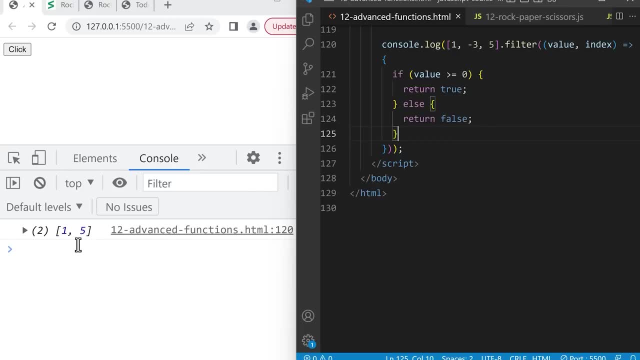 that are greater than zero will be in the new copy. So using this we can sort of filter out values based on a criteria. That's why this method is called filter. Now we can shorten this logic by using this code: return value greater than. 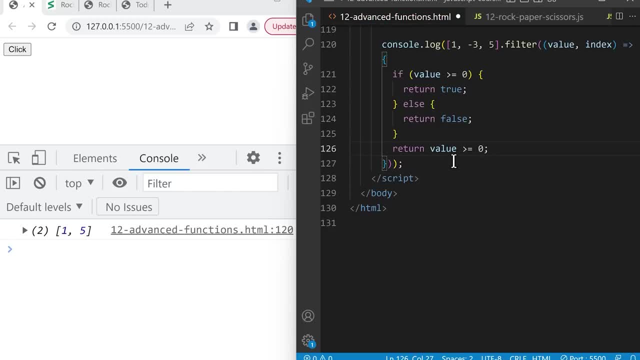 or equal to zero. So this comparison will return true if it's greater than or equal to zero, and it will return false otherwise. So this line does the same thing as this code up here. So we can comment this out with slash, star and star, slash and save And, as always, we can return a truthy or falsy value instead of just. 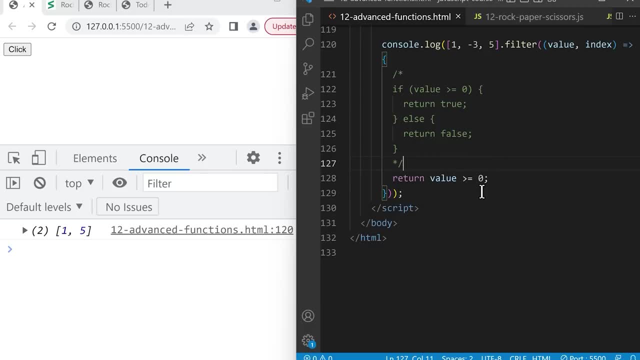 true or false. The last array method we're going to learn is called map. So let's create some new lines And scroll down And let's say we have an array of numbers again, like the array 1,, 1,, 3.. And we 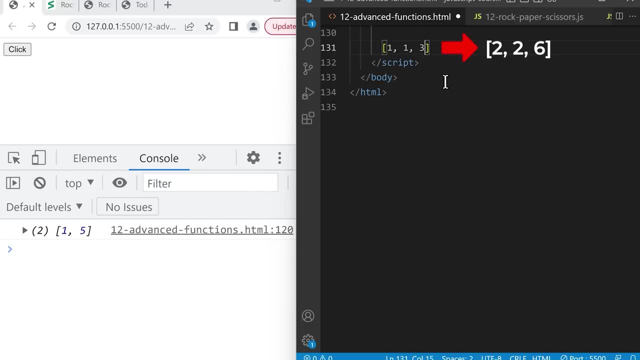 want to make a copy of this array with each number doubled. So at the end we'll type dot, map, brackets And map works just like for each, and filter Between the brackets. we'll give it a function: bracket arrow and curly brackets And this: 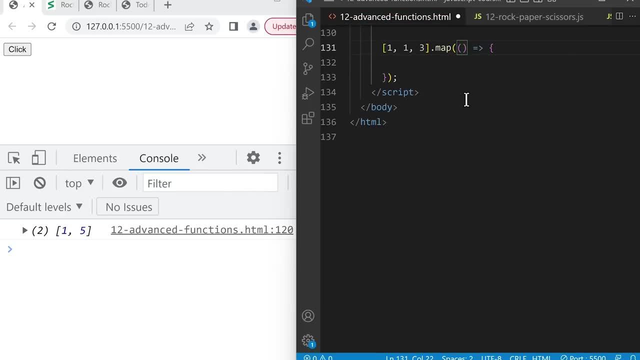 function will get two parameters. The first parameter is each value in the array And the second parameter, comma, is the index. So map will take the first value, save it in this parameter and run the function. Take the second value, save it in this parameter, run the function. Third value: save it and run the. 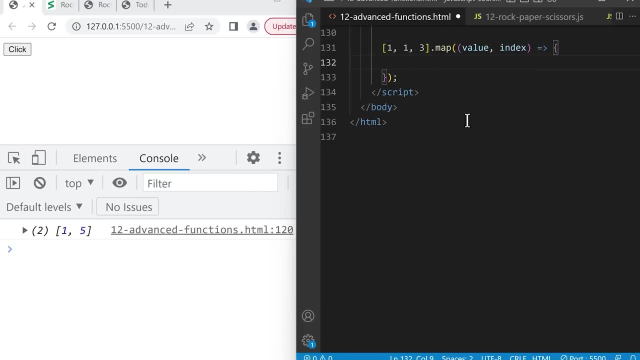 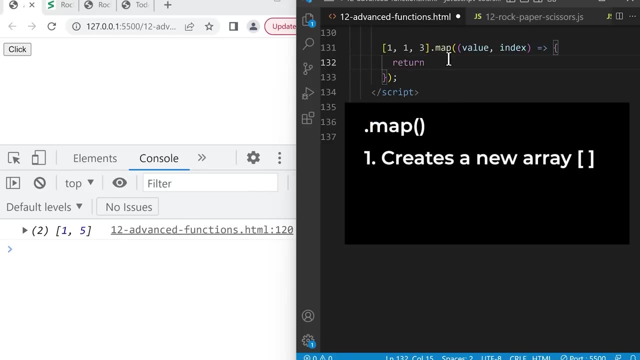 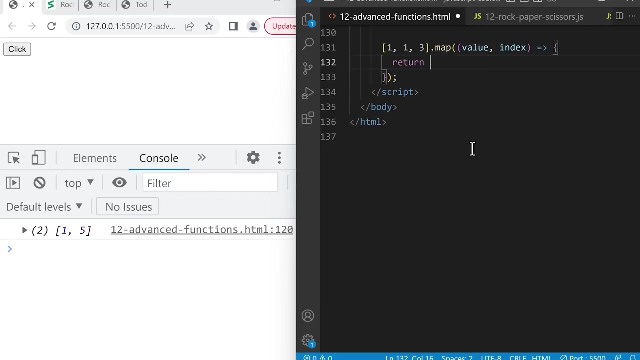 function And inside this function we're going to return a value. So what map does is it creates a new array And then whatever we return will be added to the new array. So if we return 10, and then we console dot, log this result. 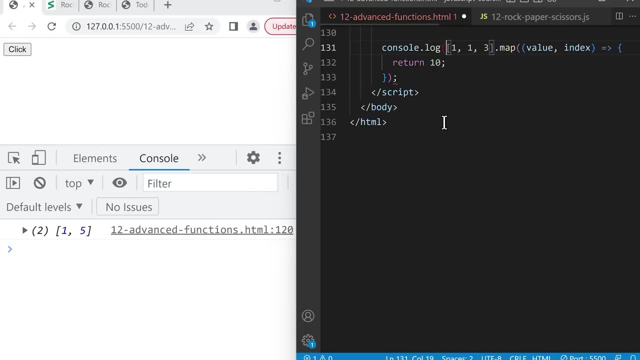 console, dot, log and close, bracket and save. it will create an array where each value becomes 10.. Now the interesting thing is that we can actually use the value itself in the return. So here, if we did value plus 10, and save, it will take each value from the new value to this new value and run. 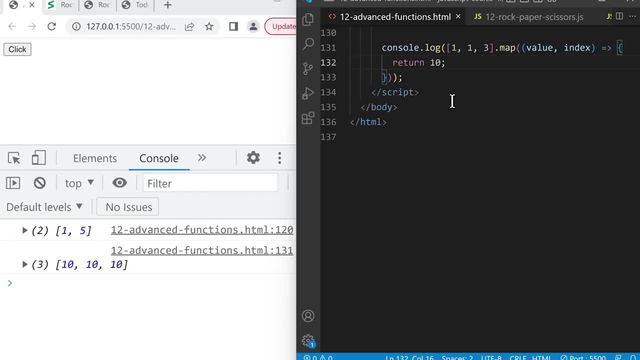 this function And choose the series we have here And create another set space And paint in this today. match it with could use do better e-e-0.. And save each value in the original array, add 10, and put it in the new array. 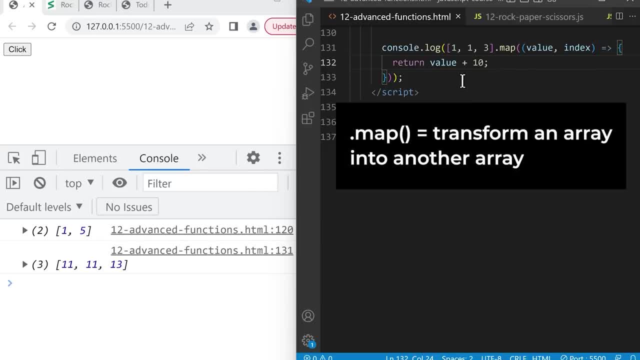 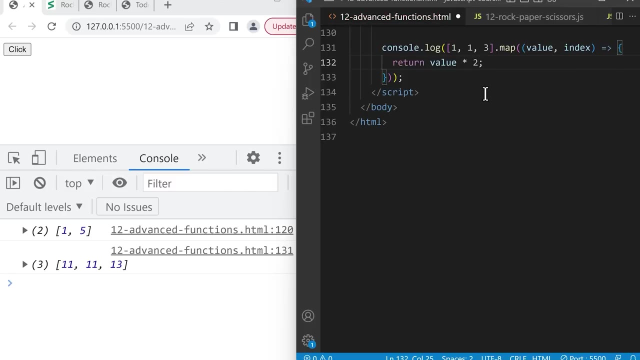 So map will transform an array into another array based on the return value. So if we want to return an array where each number is doubled, we just have to multiply each value by 2, and save, And this will give us 2,, 2,, 6.. 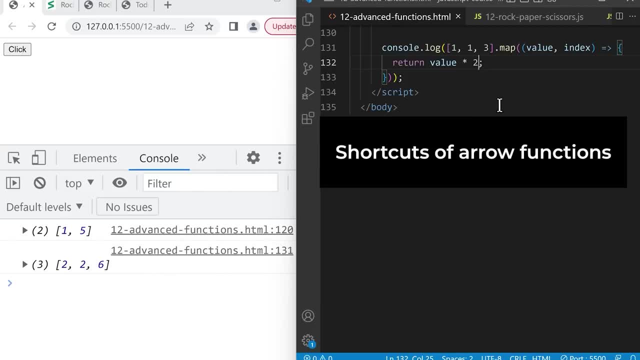 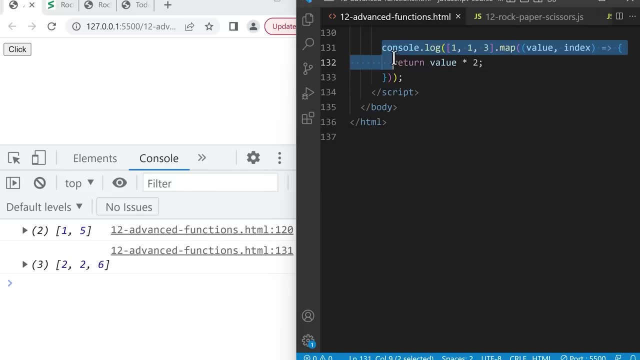 Next we're going to review some shortcuts of arrow functions to make this code more compact. First let's make a copy of this code: Right click, copy And down here. right click and paste. So notice in the inner function we're not using index. 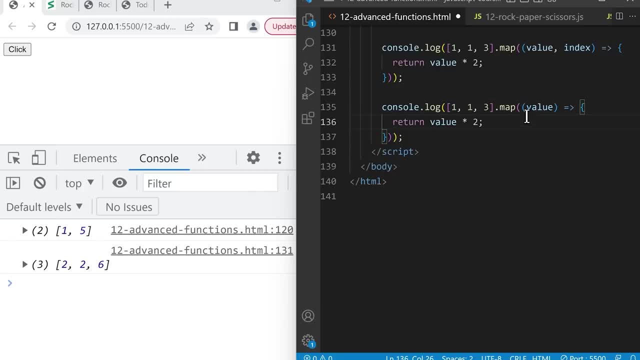 So let's just remove it for now And now that this arrow function only has one parameter, these round brackets are optional, So we can also remove these to make the code more compact. Another shortcut is, if we only have one line of code in an arrow function, we can put the 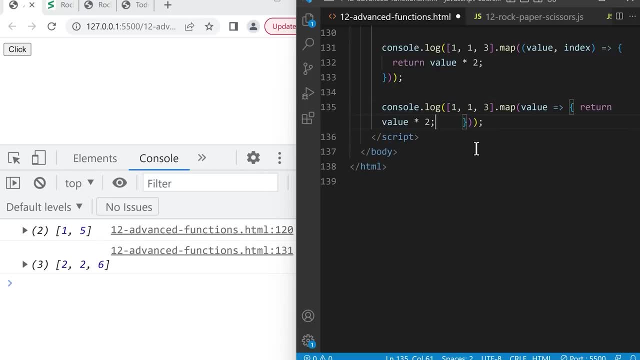 code on one line Like this, And now the curly brackets and the return are optional, So we can actually just remove all of this code. So if we have just an arrow, it will automatically return this result on the right And we don't have to type return ourselves. 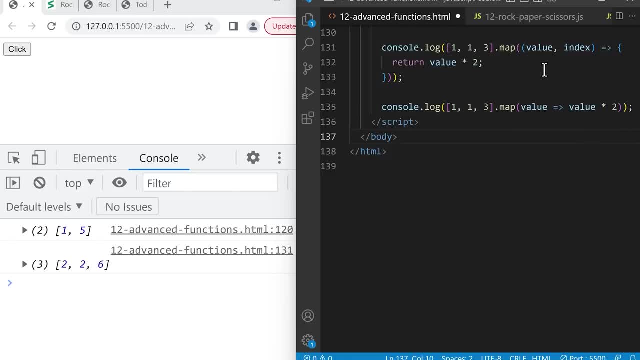 So this code does the same thing as the code above. This is the same thing as the code above, But, as you can see, these shortcuts make our code very compact and clean. So let's save, And this will give us the same result. 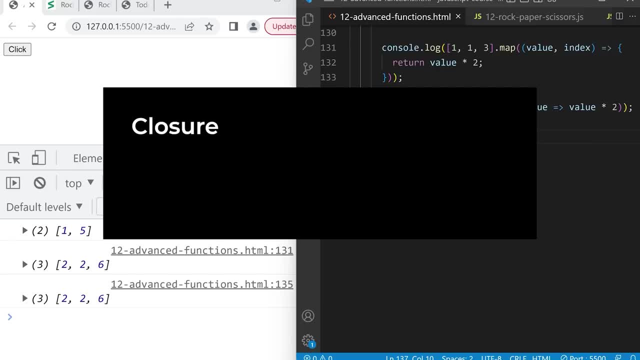 The last thing we're gonna learn in this lesson is a feature of functions called a closure. A closure means if a function has access to a value, it will always have access to that value. So let's take a look at an example. 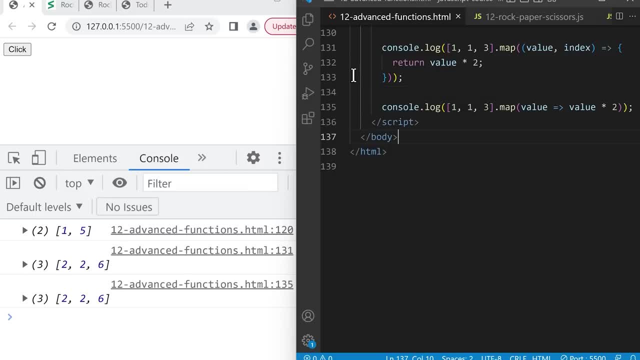 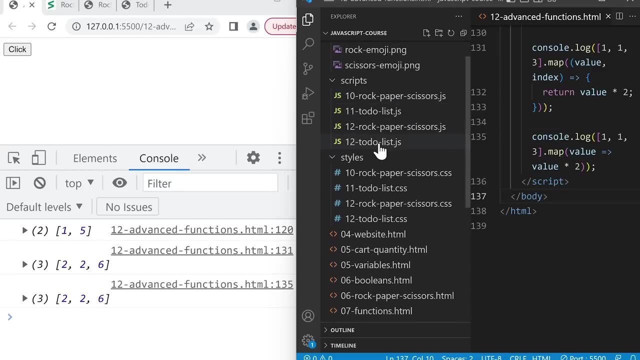 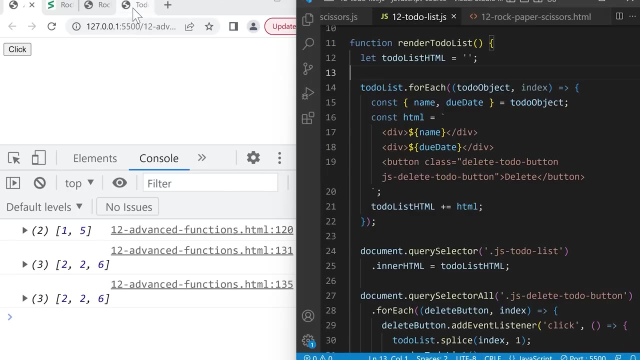 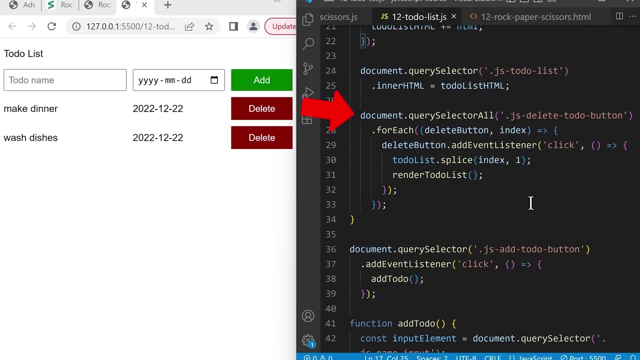 We're gonna go back to the to-do list project, So we'll click up here And then scroll up to 12todolistjs And close this And then open the tab for the to-do list, which is here, And let's scroll down to the query selector. all. 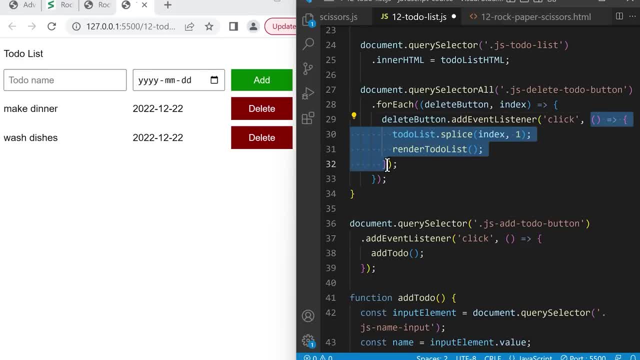 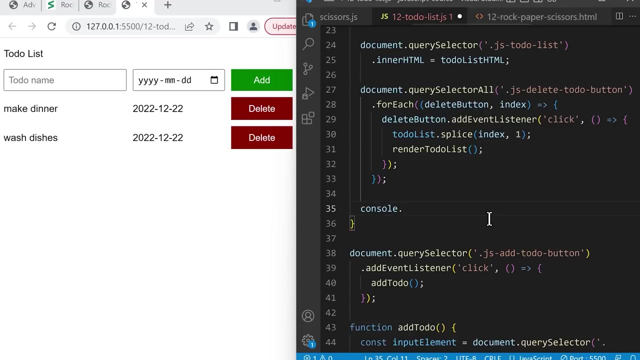 So we're gonna focus on this inner function here. So notice that this function uses index from above. Now the interesting thing about index is that as soon as this for each ends, index gets deleted. For example, if we add some new lines and we try to consolelog index and save and 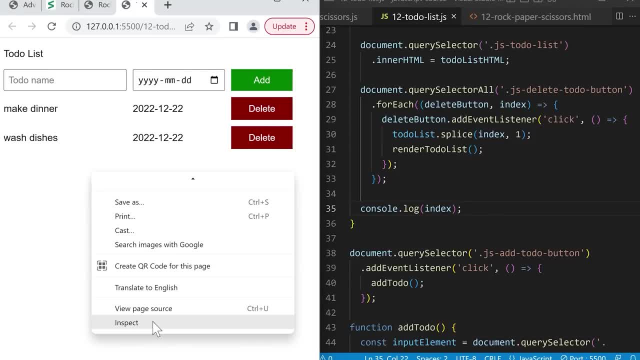 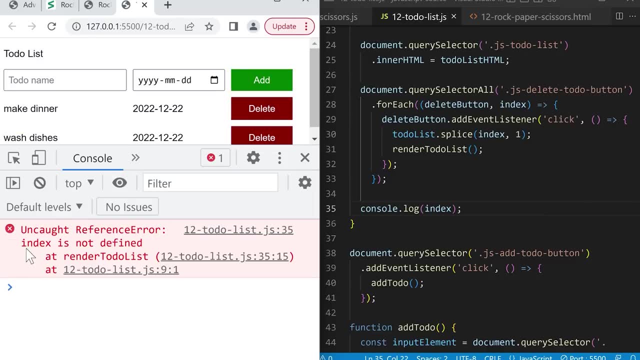 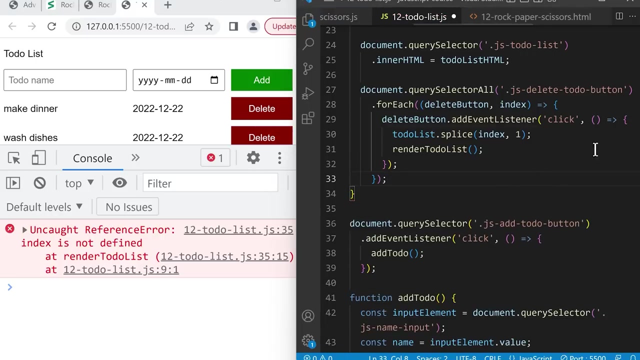 then go into our project, Right-click Inspect And the console It'll tell us that the index is not defined. So as soon as we end the for each loop index doesn't exist anymore. However, if we move this into the inner function, so inside here, and we consolelog index. 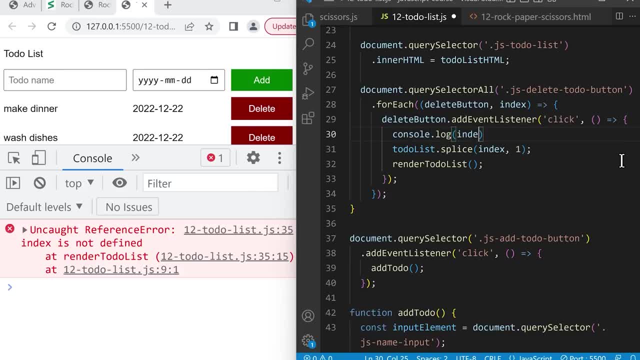 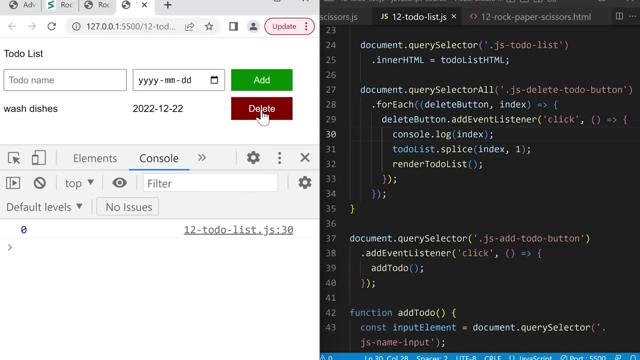 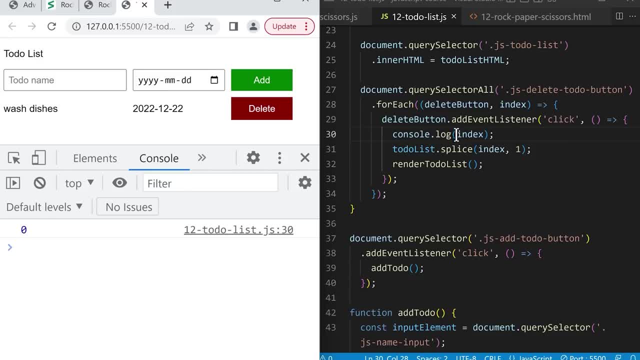 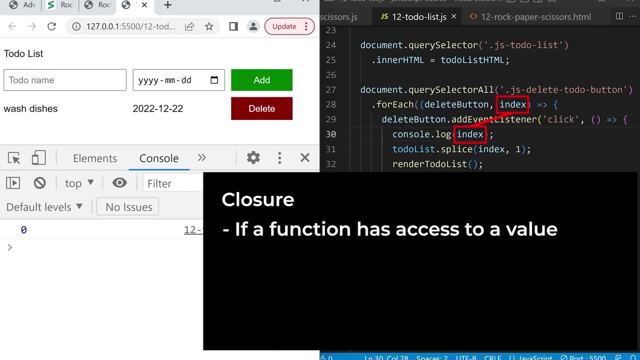 If we click one of these buttons later on, It still has access to index. This feature is called a closure. If a function has access to a value, That the index or event- We would specify an index- now have access to that value. 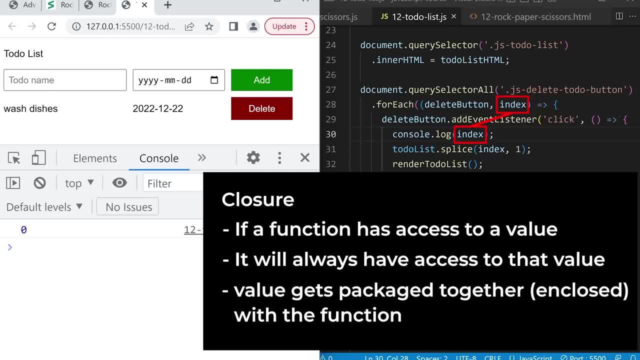 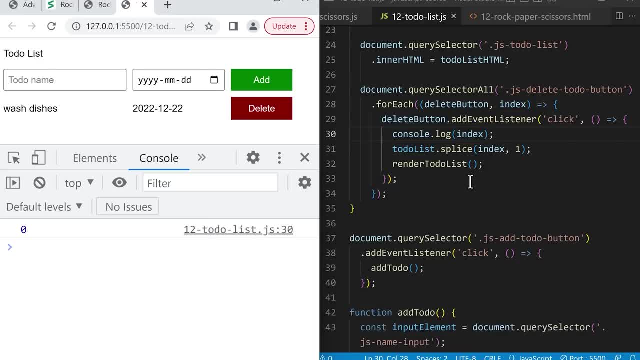 The value, like index, gets packaged together or enclosed with the function. That's why we call it a closure. So even if the value index gets deleted after the loop, we can click the delete button 5 seconds later or even 5 minutes later, and this function will always have access to index. 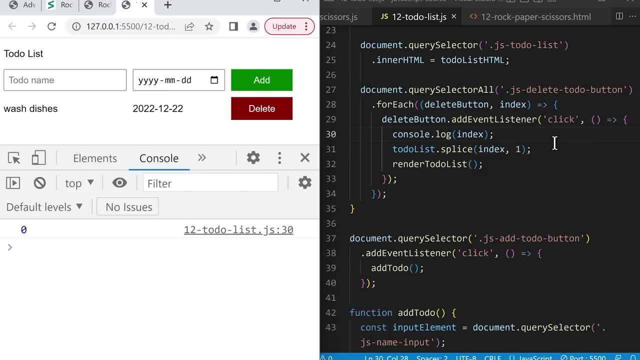 That naturally happens as we write JavaScript code, and it's nice to know how this feature works. There are some advanced techniques that we can do with closures, but they're not used that often, so I won't be covering them in this course, but maybe in a different video. 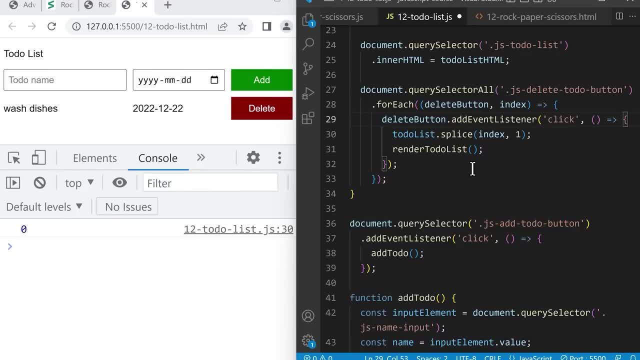 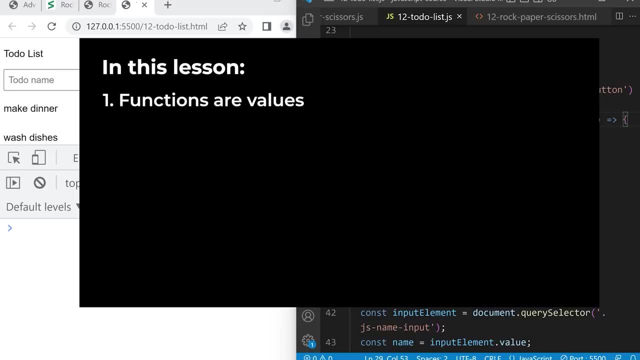 Now let's remove consolelog and save, And that's the end of this lesson. In this lesson, we learned that functions are values. We learned setTimeout and setInterval, which lets us run a function in the future. We learned an array method called foreach, which is a cleaner way of looping through. 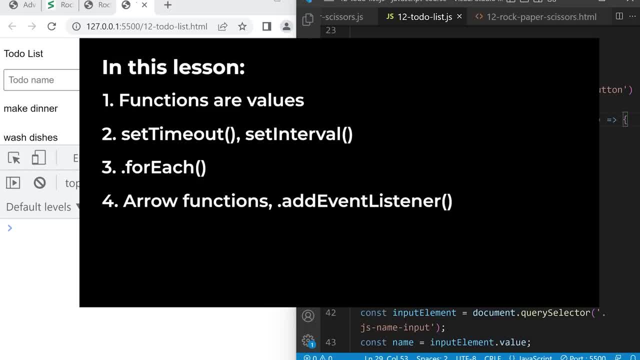 an array. We used foreach arrow functions and addEventListener to improve our projects. We learned two more array methods- filter and map, And we learned a feature of functions called loop, called closures. Here are some exercises to help you practice what we learned in this lesson.